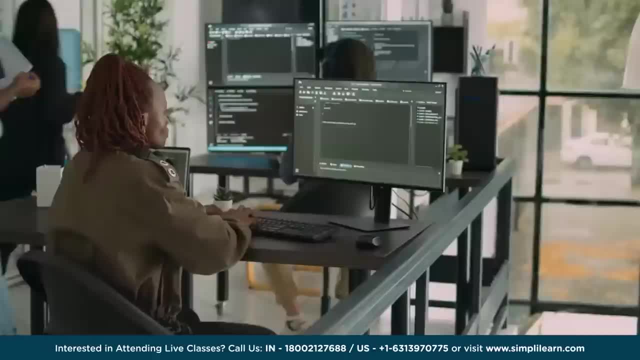 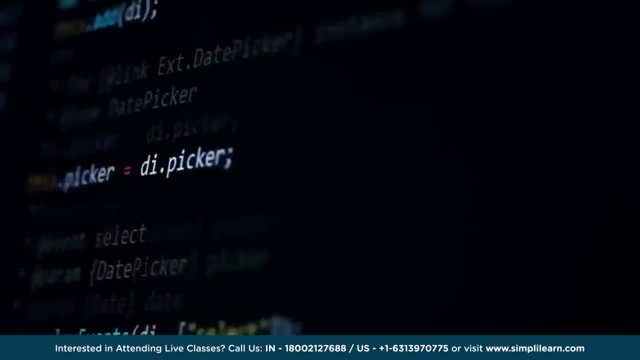 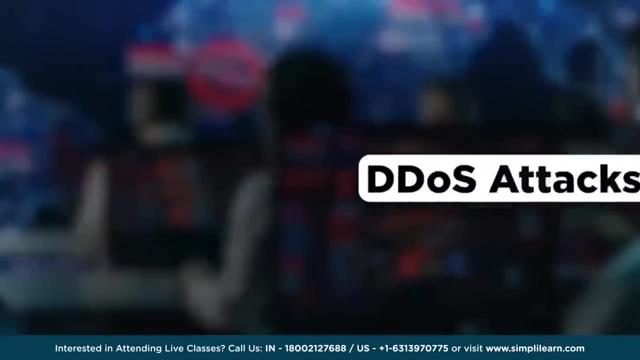 advanced topics. We provide a small introduction to cybersecurity, followed by explainers regarding the career scope in this domain and the job roles offered. After covering a few cybersecurity skills, we will learn about ethical hacking and network masking techniques like VPNs and proxies. Further, we delve into various attacks, like DDoS attacks. 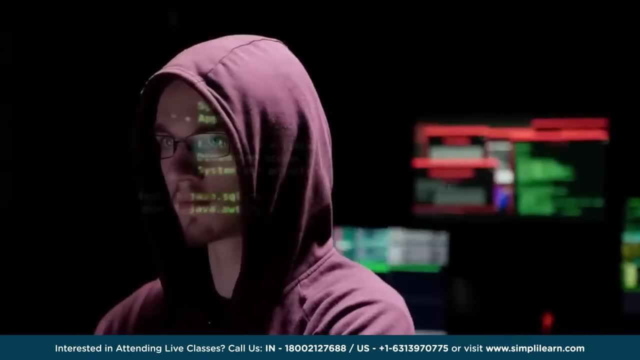 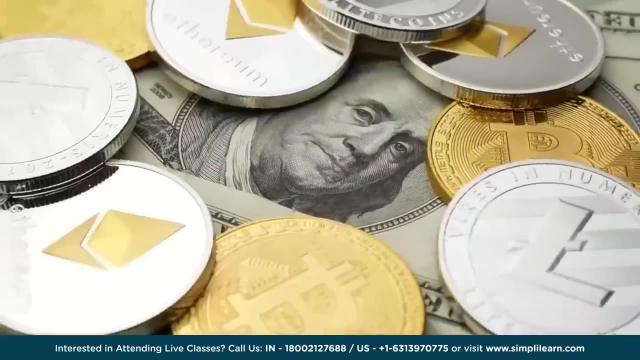 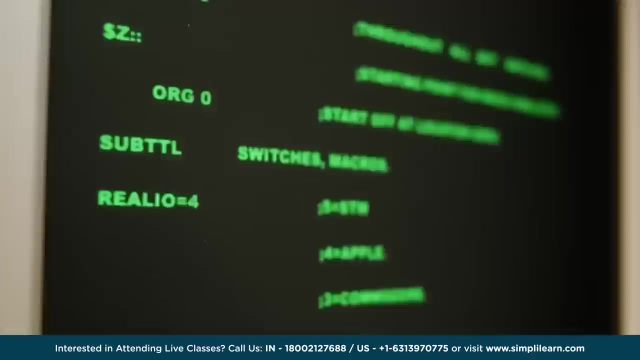 SQL injection and cross-site scripting, with live demonstrations that you can carry out on your own system for practice. After learning a bit more about different cyberattacks, we will learn about cryptography, covering topics like encryption, encryption, encryption famous algorithms like RSA and AES, and hashing algorithms like SHA-256 algorithms. 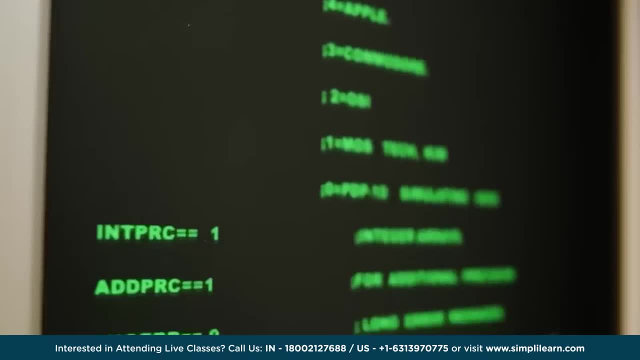 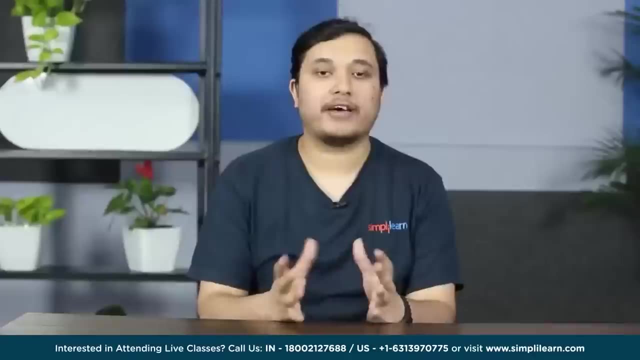 Next, we look at the Linux-based operating systems that you can use for ethical hacking, like Kali Linux and Parrot Security. We then further dive into some of the tools that cybersecurity analysts use to secure their systems. Finally, we cover the industry's most well-known 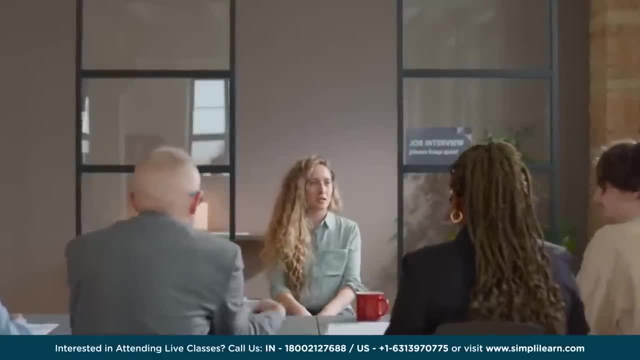 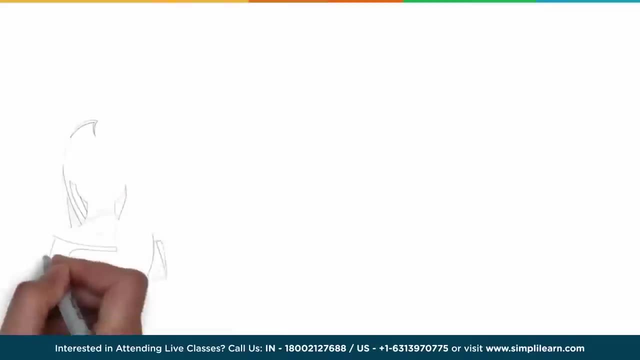 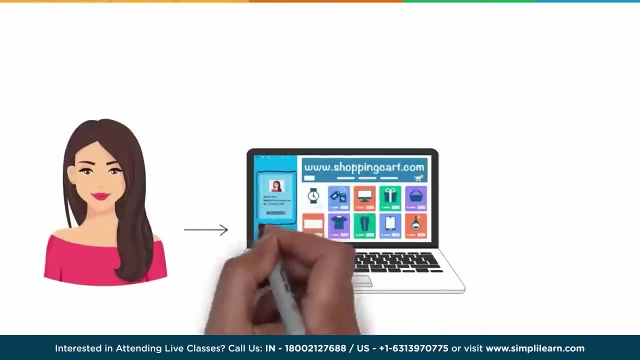 certifications, followed by a series of interview questions to prepare you for your first job in cybersecurity. So let's get started. Meet Anne. She often shops from wwwshoppingcartcom. She has her information, like email ID, address and credit card details, saved on the website to enable a faster and hassle-free shopping. 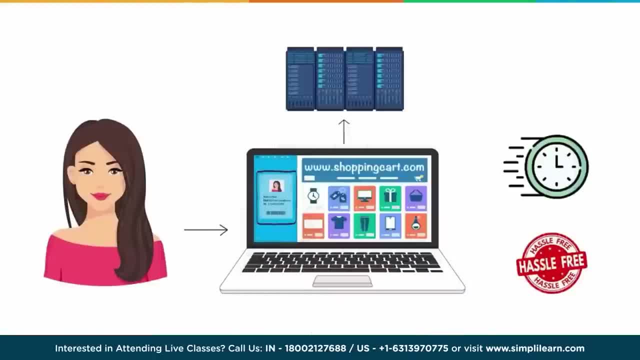 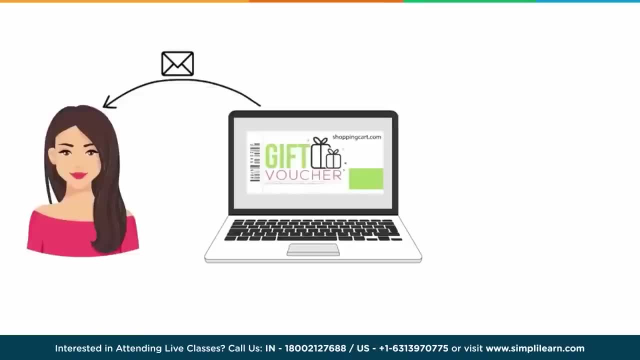 experience. The required information is stored in a server. One day, Anne received an email which stated her eligibility for a special discount voucher from shoppingcartcom. In order to receive the coupon code, she was asked to fill in her shoppingcartcom account credentials. This didn't seem fishy to her at the time. 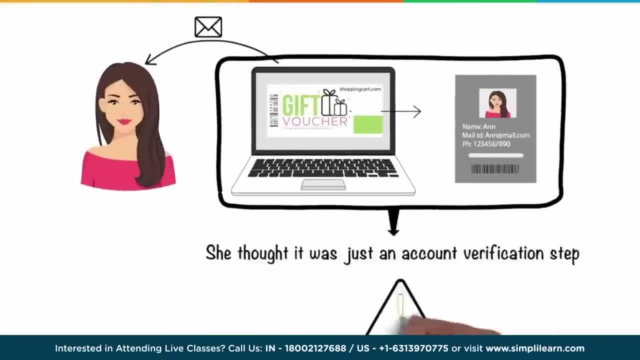 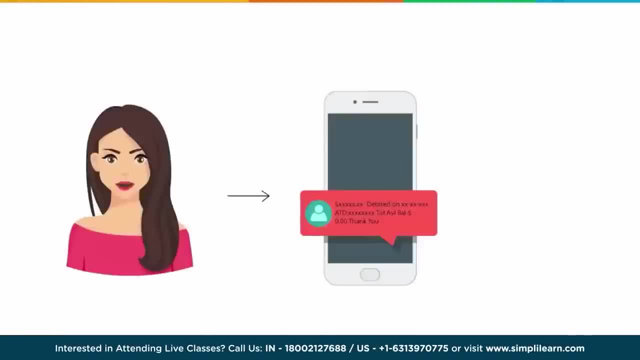 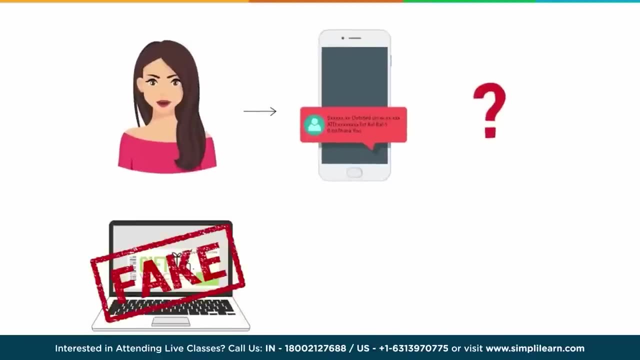 as she thought it was just an account verification step. Little did she realize the danger she would be facing. She was knocked off her feet when a substantial amount of money was wiped off her account. How do you think this happened? Well, yes, the email she received was fake Anne's. 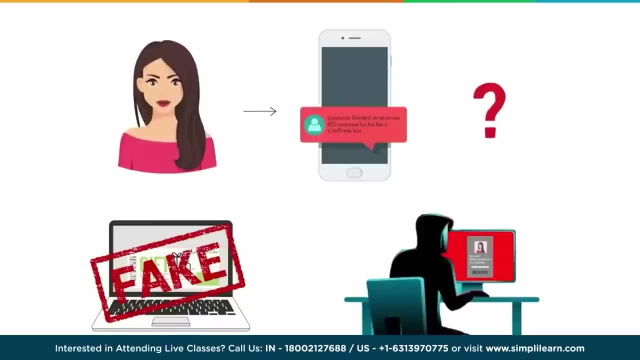 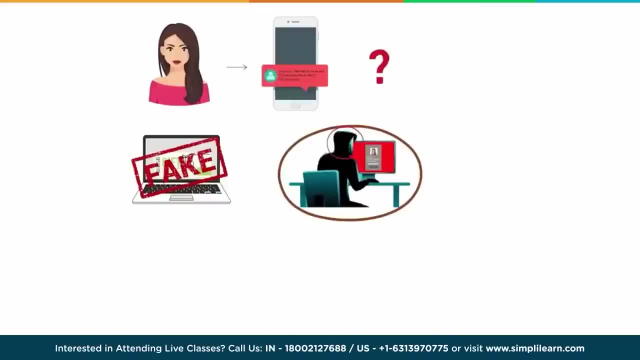 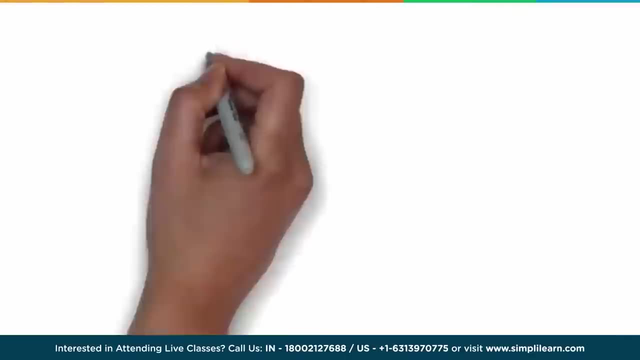 shoppingcartcom account witnessed unauthorized access from a third party. This type of attack is known as a cyberattack, and the person who carries it out is called a hacker. Could Anne have prevented this attack? Indeed, she could have- with the help of cybersecurity. 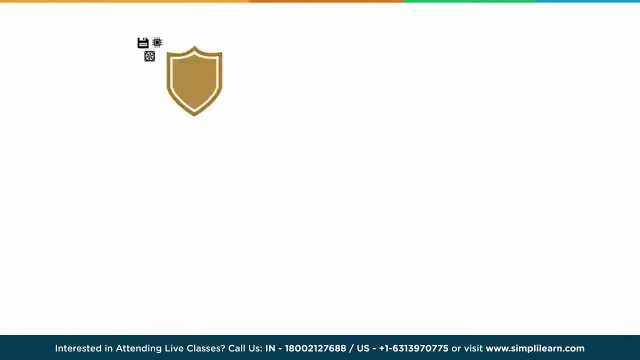 Cybersecurity involves techniques that help in securing various digital components, networks, data and computer systems from unauthorized digital access. There are multiple ways to implement cybersecurity, depending on the kind of network you are connected to and the type of cyberattacks you are prone to. 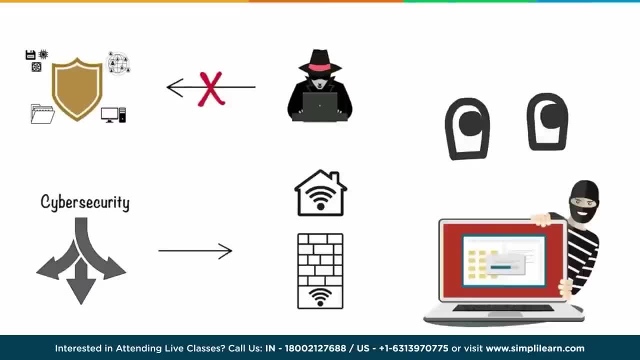 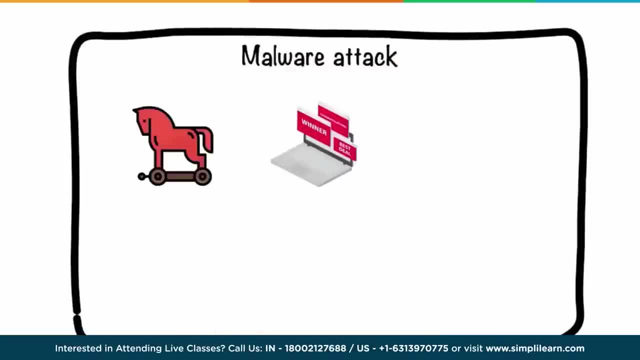 So let's take a look at the various cyberattacks that Anne could have been exposed to. One of the most common types of cyberattacks is a malware attack like Trojan, Adware and Spyware, to name a few. Had Anne downloaded any suspicious attachments online, her system could have gotten corrupted. 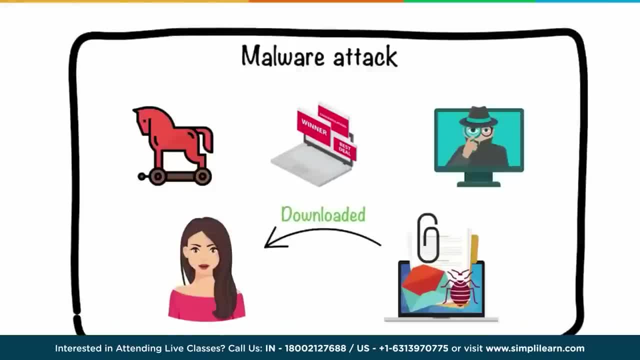 by certain malicious viruses embedded within the attachments. Next is a phishing attack: The type of cyberattack which can be used to spy on other people. The type of cyberattack which can be used to spy on other people. The type of cyberattack which can be used to spy on other people. 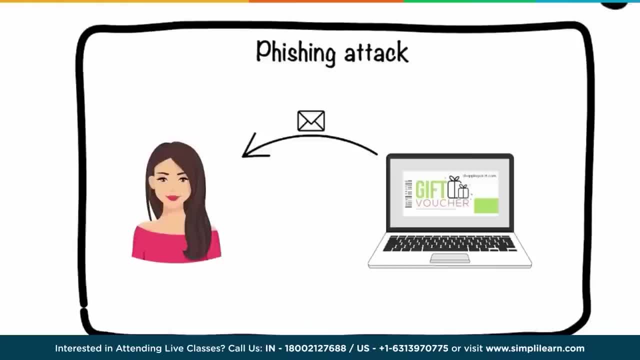 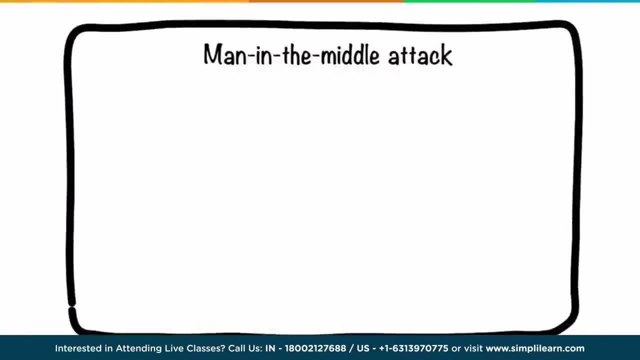 Here, though, the hacker usually sends fraudulent emails which appear to be coming from a legitimate source. This is done to install malware or to steal sensitive data like credit card information and login credentials. Another type of attack is the man-in-the-middle attack. 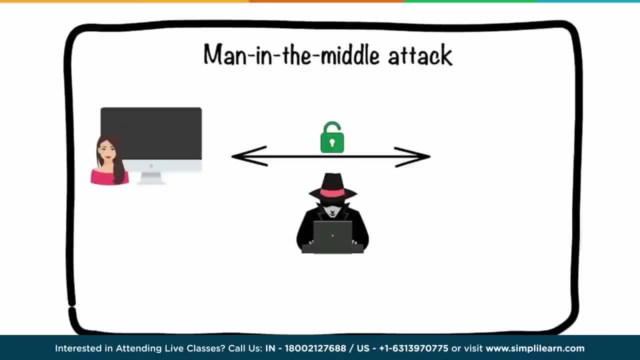 Here the hacker gains access to the information path between Anne's device and the website's server. The hacker's computer takes over Anne's IP address. By doing so, the communication between Anne's computer and the website is shifted. line between Anne and the website is secretly intercepted. This commonly happens with unsecured 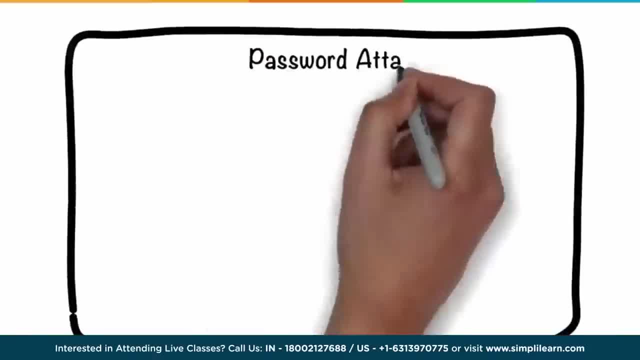 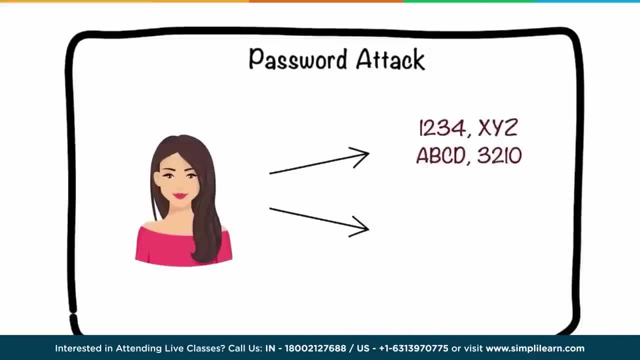 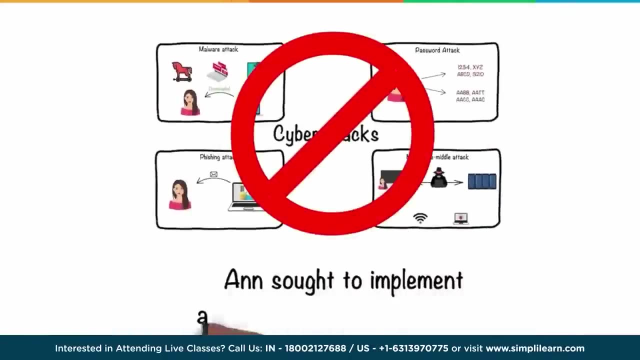 Wi-Fi networks and also through malware. Password attack is one of the easiest ways to hack a system. Here, Anne's password could have been cracked by using either common passwords or trying all possible alphabetical combinations. To prevent future cyber attacks, Anne sought to implement. 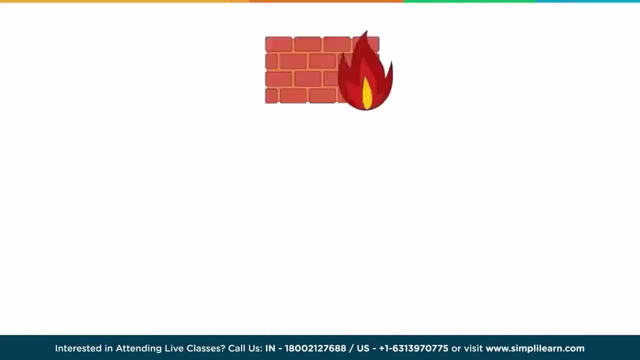 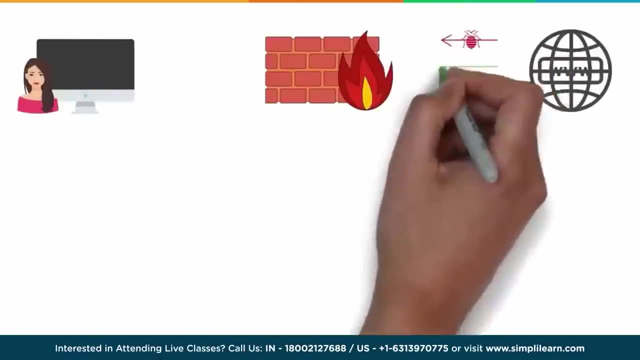 a few cybersecurity practices. First, she installed a firewall. As the name suggests, it is a virtual wall between Anne's computer and the internet. Firewalls filter the incoming and outgoing traffic from your device to safeguard your network, and they can either be software. 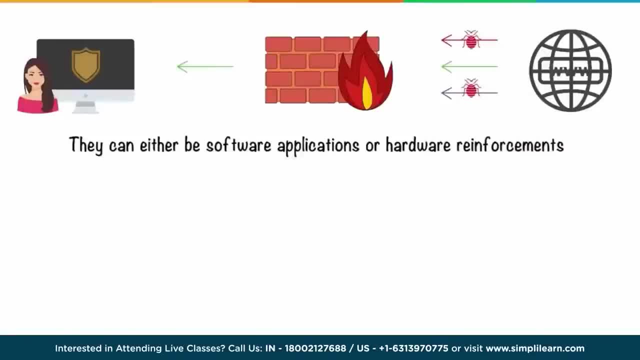 applications or hardware reinforcements. Secondly, Anne implemented honeypots. Just like how flowers attract bees, dummy computer systems called honeypots are used to attract attackers. These systems can be used to attack the internet and can also be used to attack the internet. 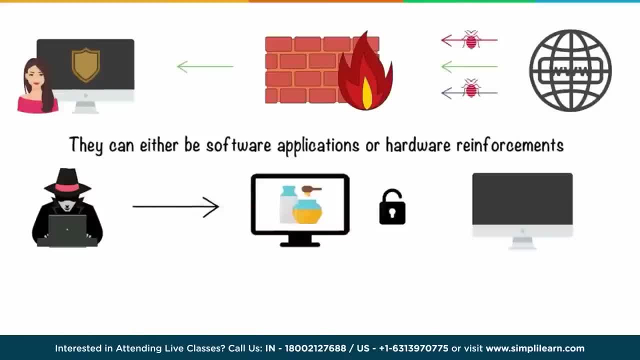 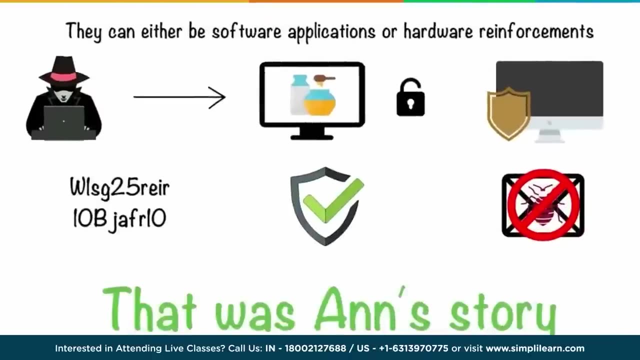 These systems are made to look vulnerable in order to deceive attackers, and this, in turn, defends the real system. In addition to these, she also decided to use unique alphanumeric passwords, antivirus software and started avoiding mails from unknown senders. That was Anne's story. 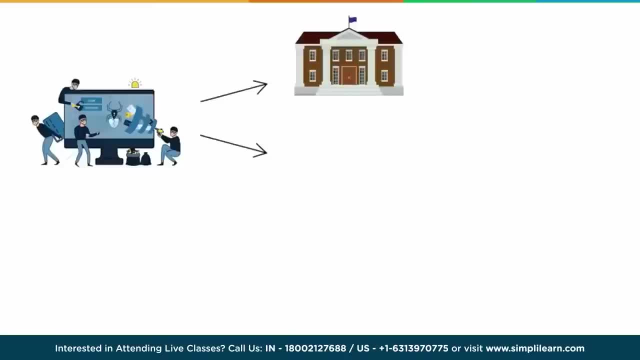 Cyber attacks are not just confined to individuals, but also to public and private organizations. The cyber attacks carried out in such places are more deadly and they result in colossal losses. Motives of such attacks are many, starting from tampering with crucial data. 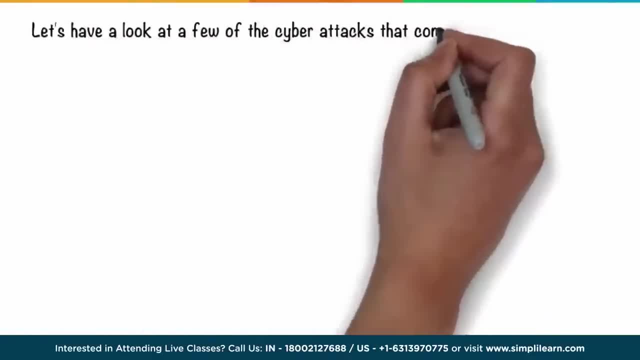 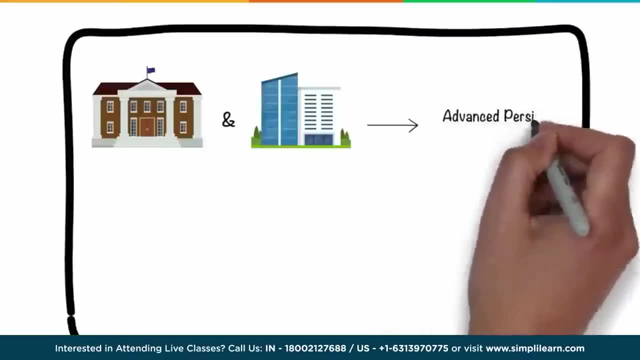 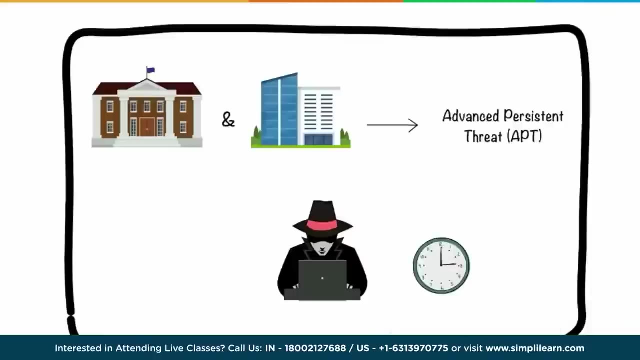 to monetary gains. Let's have a look at a few of the cyber attacks that companies are subjected to. Various public sector organizations and large corporations face the Advanced Persistent Threat APT. In this form of attack, hackers gain access to networks for a prolonged period. 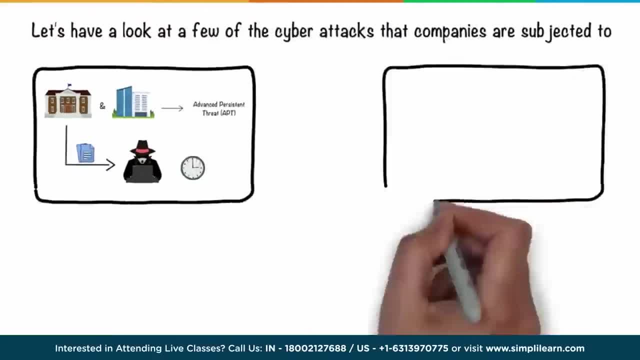 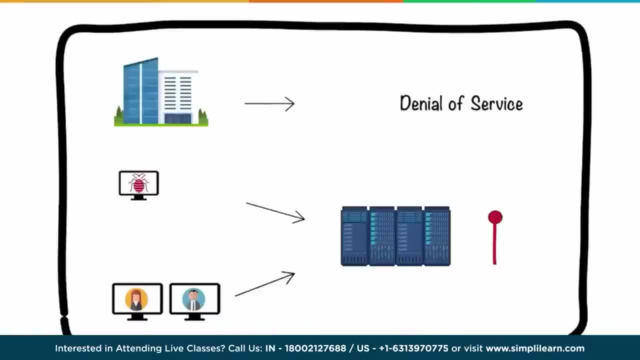 in order to continuously gain confidential information. Companies also witness the denial of service attack, where networks are flooded with traffic, which in turn, leaves legitimate service requests unattended. A variant of this is the Distributed Denial of Service- DDoS- attack, when multiple systems are used to launch the attack. When a hacker manipulates a. 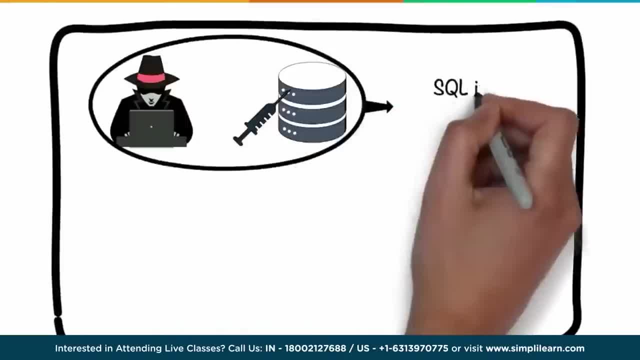 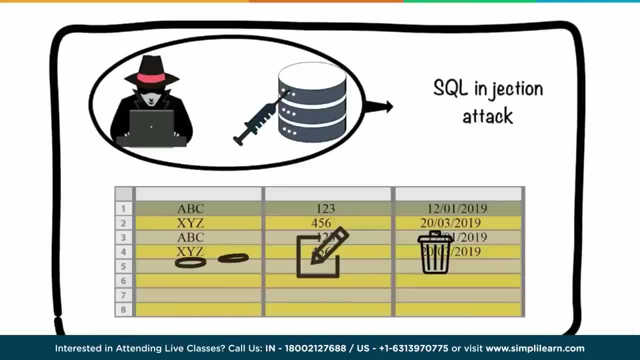 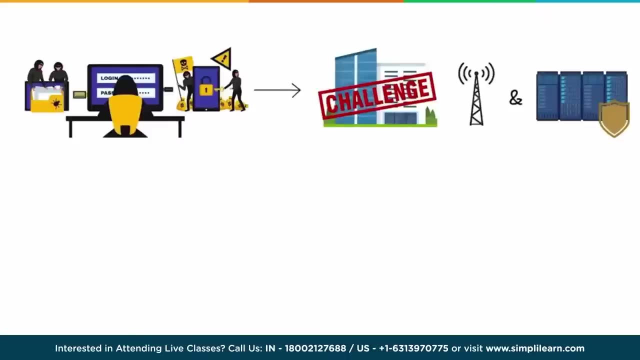 standard SQL query in a database-driven website. it is known as a SQL injection attack. By doing so, hackers can view, edit and delete tables from databases. Amidst a plethora of cyber attacks, it is indeed a challenge for organizations with several networks and servers to ensure 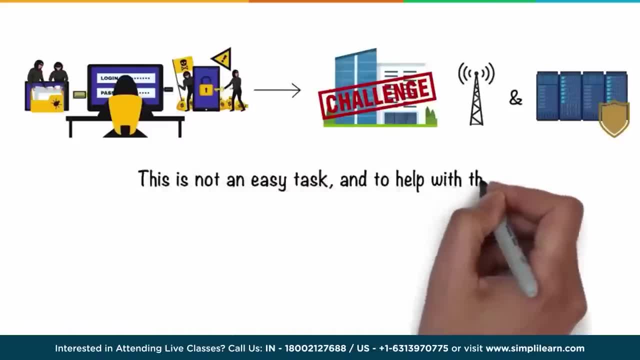 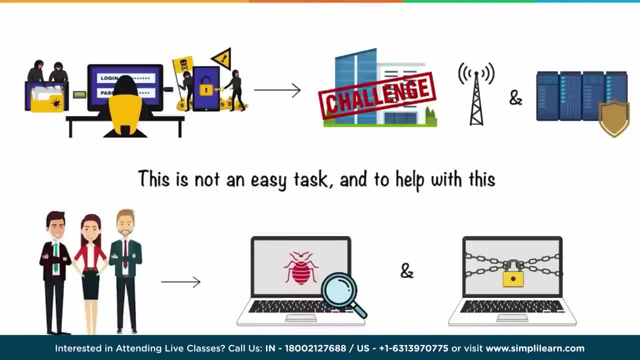 complete security. This is not an easy task and to help with this, cybersecurity professionals are hired to work on identifying cyber threats and securing a company's network. There are multiple job roles in the field of cybersecurity If hacking fascinates you. 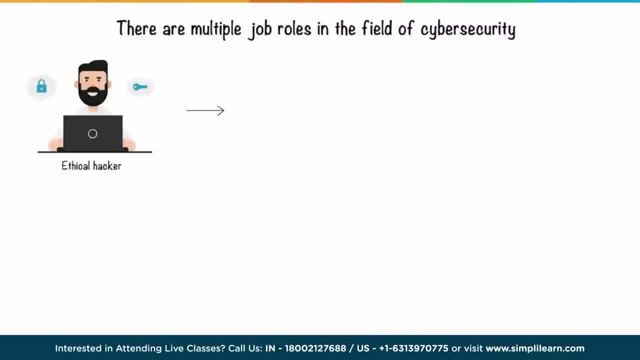 then the role of an ethical hacker is something to be explored. Such professionals try to explain a network's vulnerabilities just like how a hacker would do, But only to identify those vulnerabilities and resolve them for protection against an actual cyber attack. But if you are looking to design robust security structures, then the role of a 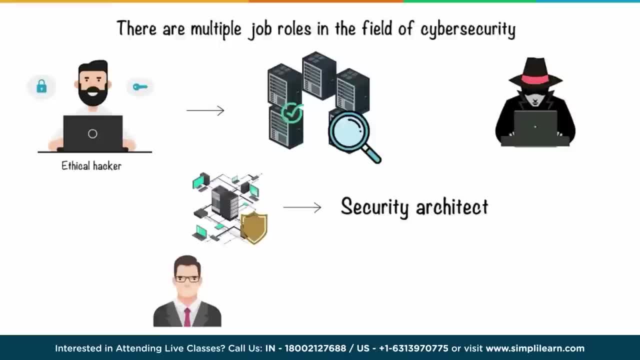 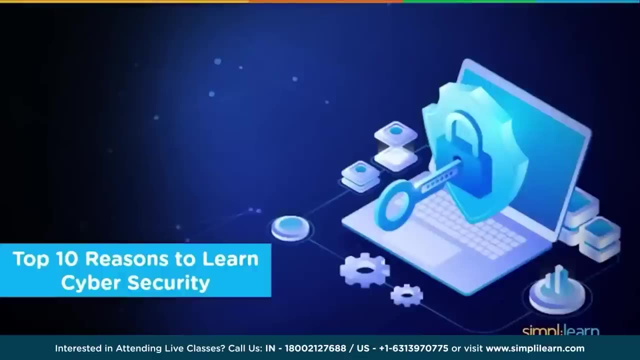 security architect is more apt A chief information security officer. CISO plays a crucial role in enterprise security and is entrusted with the overall safety of the information in an organization. Now there are several reasons as to why you should learn cybersecurity. Here we have the top three. 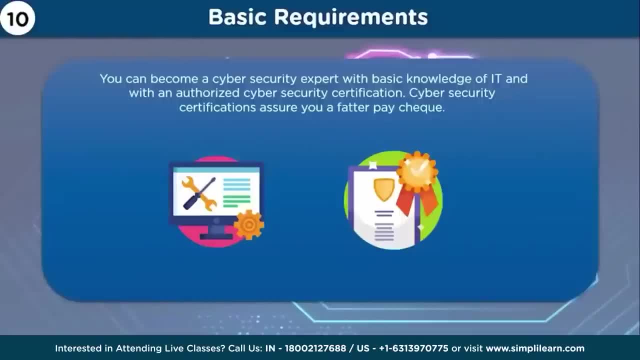 At number 10, the reason we have is basic requirements. There is a wrong notion that building a career in cybersecurity is daunting. Well, it is not A fancy college degree is not at all that it takes to become a successful cybersecurity professional. You can venture. 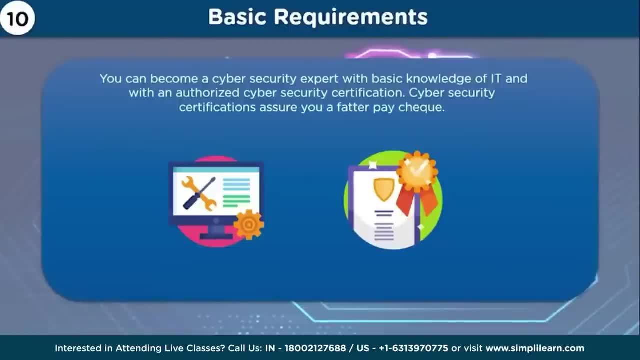 into the domain of cybersecurity with some basic knowledge of IT and with an authorized cybersecurity certification. The overall eligibility criterion for the cybersecurity domain is relaxing across the world. IT professionals with cybersecurity certifications are known to receive higher salary packages. Certifications are always given extra weightage in the infosec field and it. 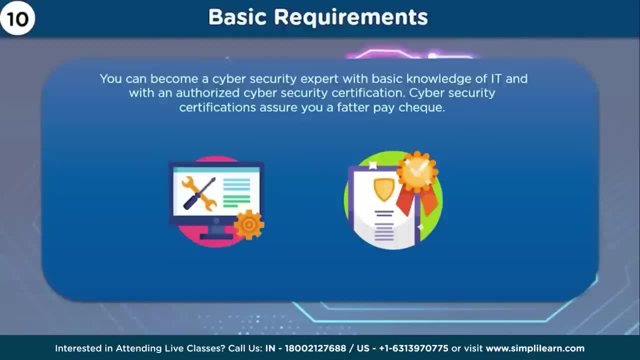 opens doors to bigger opportunities. These cybersecurity certifications can be opted by anyone, as the eligibility for these are very basic. Cybersecurity certifications train professionals and thus helps in bridging the gap between the supply and demand of skilled cybersecurity professionals. So don't take a step back from learning cybersecurity thinking. it is a tedious process. 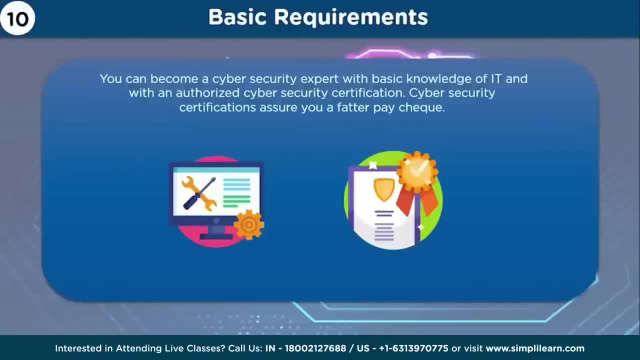 If you are a fresher or a professional, you can go ahead with just these basic requirements. Before moving on to our next reason, here is a question for you all. How many of you like mathematics? Please let us know in the comment section below. I am sure not everyone. 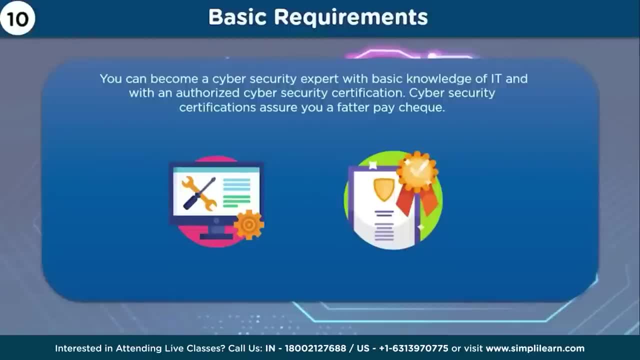 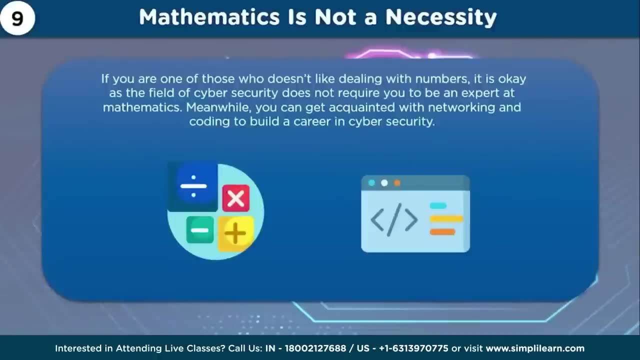 loves mathematics, and that is completely okay when it comes to learning cybersecurity. And our 9th reason is: Mathematics is not a concern for learning cybersecurity. Many of us find mathematics challenging. Some have the aptitude for dealing with numbers and some don't, And for those, 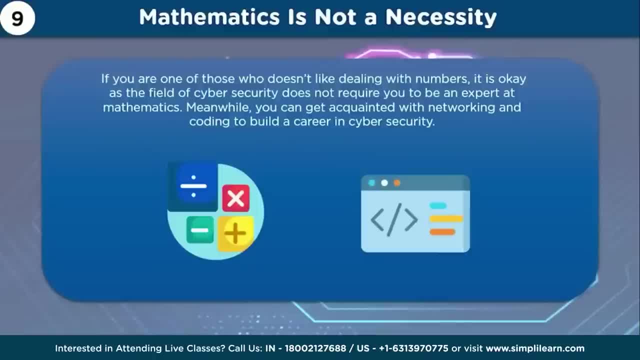 who don't. they find it difficult to proceed with a career that has maths involved. However, you can take your decision without any worries when it comes to cybersecurity, as the domain of cybersecurity does not involve mathematics. So if maths is not your strong point, then 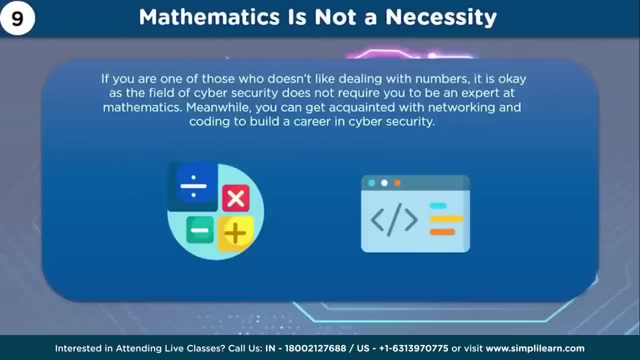 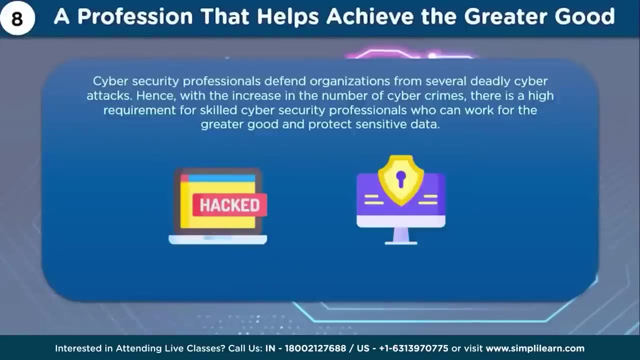 choosing to learn cybersecurity is the right decision. Cybersecurity is a great choice. This can definitely be a relief to many. Instead, you can get acquainted with networking, network security, control and coding to build a career in cybersecurity. Our 8th reason is that cybersecurity is a profession that helps achieve the greater 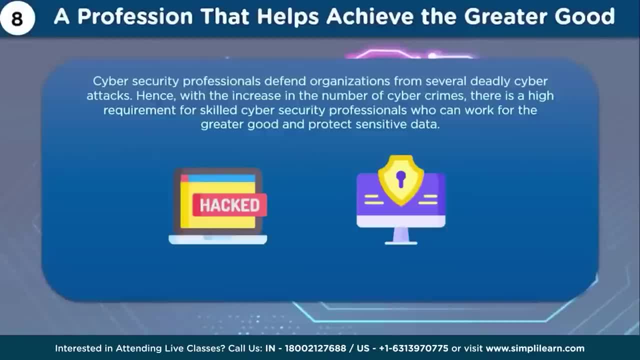 good Cybersecurity consists of a set of measures and approaches that help companies and individuals data from being compromised and stolen. Cybersecurity professionals have defended organizations from several times. They have been able to do this for decades. They have been able to tackle many more cybercrimes and cybercrime-zoned cybercrime attacks. 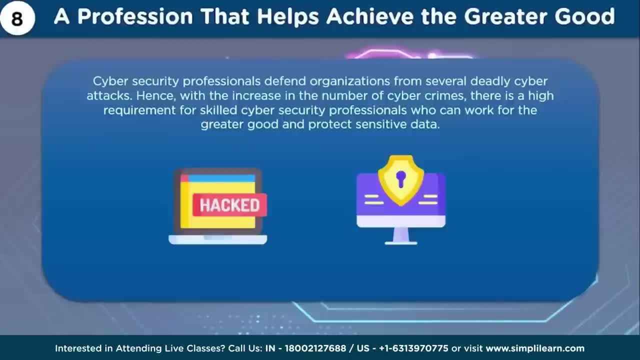 So what is a cybercrime-zoned cybercrime? Cybercrime is a type of cyber anticorruption that isannielled at governments. It is a type of cybercrime system that is essential to save lives and protect people's lived and %. 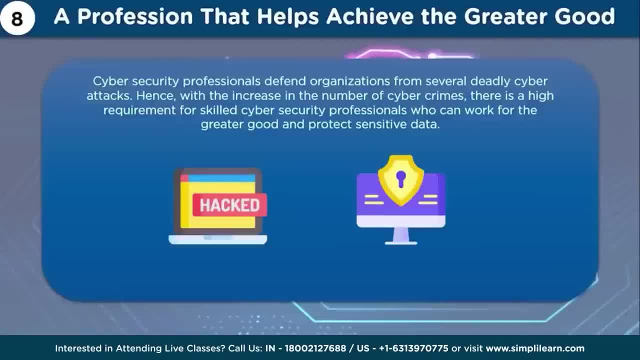 Cybercrime's role in cybercrime is to eliminate the threat of cybercrime in organizations and individuals alike. Cybercrime is used as a tool for면ing cybercrime's delivery. When cybercrime is used, it is also used to protect organizations and individuals alike. 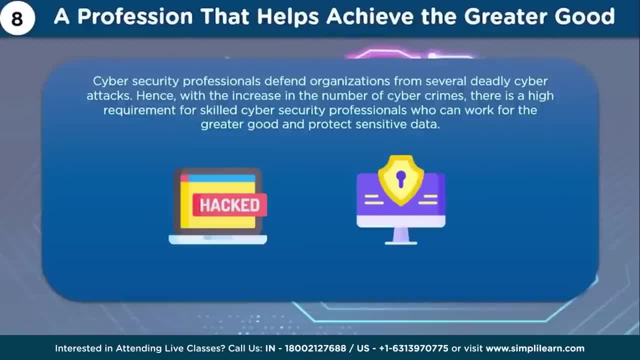 There is a deep connection to cybercrime. in the cybercrime industry, Cybercrime is the most common weapon of cybercrime development. It is used to track cybersecurity implementation in the real world. Cybercrime is the most common way cybercrime is used. Therefore, if you want to bring about a positive impact and a meaningful difference to the society we live in, then learning cybersecurity is a great choice. 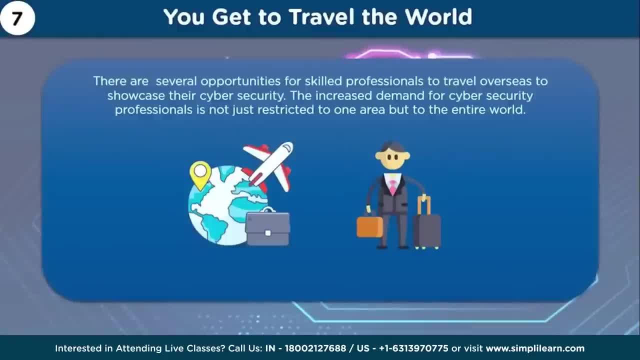 Our seventh reason is that you get to travel the world. Who doesn't love to travel the globe? Learning cybersecurity is a great reason, especially for those of you who aspire to travel the world. With the lack of cybersecurity professionals in the world, there are plenty of opportunities for skilled experts to travel overseas to showcase their cybersecurity skills, which are in high demand. 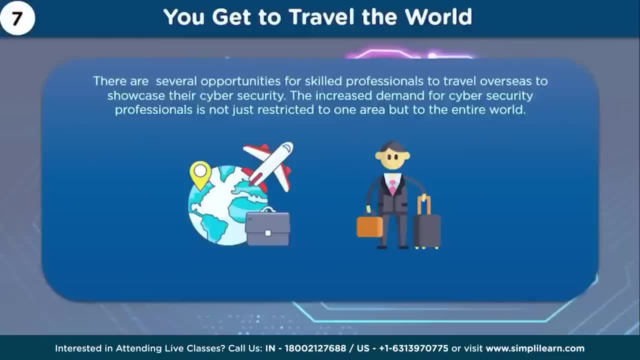 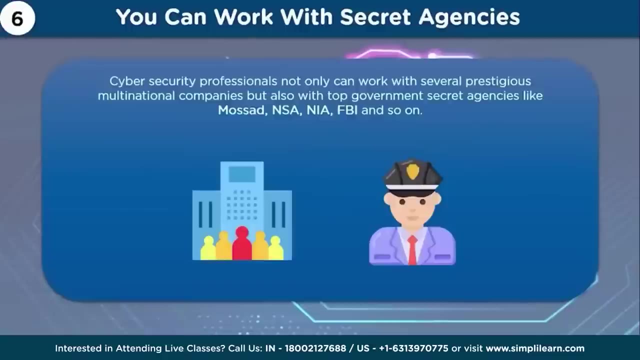 The increased demand for cybersecurity professionals is not just restricted to one area, but to the entire world. There are several employment opportunities for cybersecurity professionals across the globe, so learning cybersecurity can open new doors for you overseas as well. Our sixth reason is very interesting. 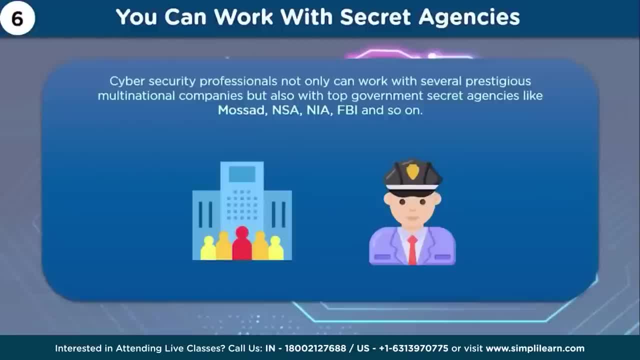 And that is the fact that you get to work with secret agencies, and high-profile ones. Like other professionals, cybersecurity professionals also have the opportunity to work with several prestigious multinational companies and big giants like Google, Dell, Accenture and others. However, a cybersecurity professional's career opportunities can go beyond MNCs and they might get the opportunity to work with top government secret agencies like Mossad. 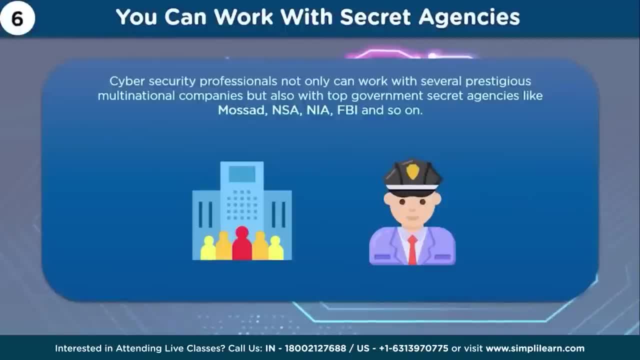 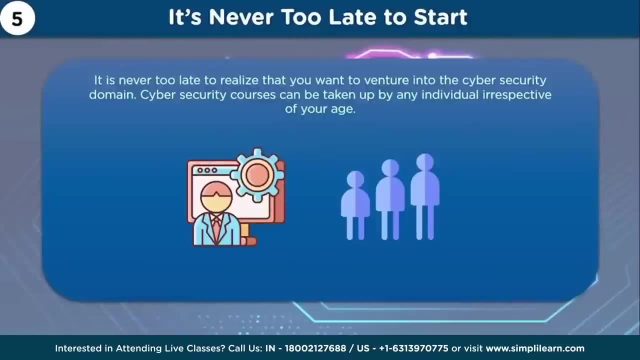 NIC and others. So what are you waiting for? Become a cybersecurity expert and showcase your skills to grab the chance to work with these top agencies. Our fifth reason is it is never too late to begin with. There are very few professions that give you the liberty to begin late. 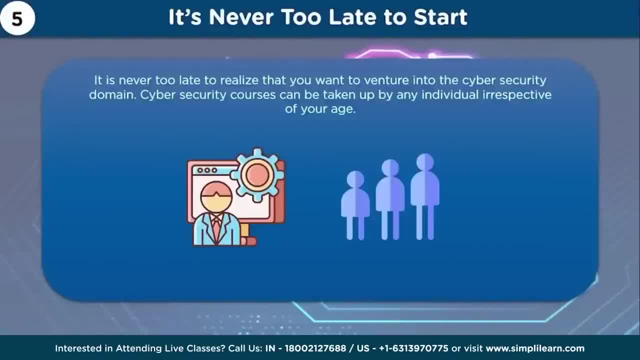 And one such profession is cybersecurity. It is never too late to realize that you want to become a cybersecurity expert. Many people work as cybersecurity professionals in the field of cybersecurity Even after their retirement. if they have a good knowledge about IT, You could also join cybersecurity courses that train you irrespective of your age. 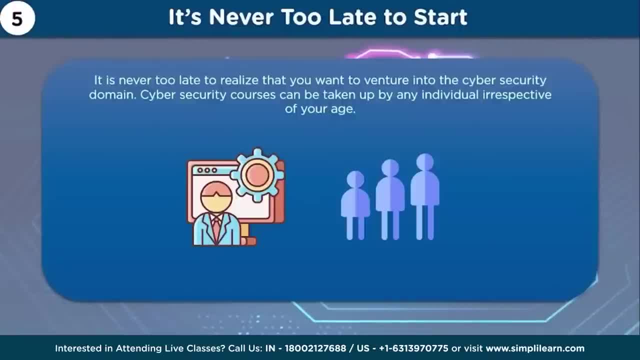 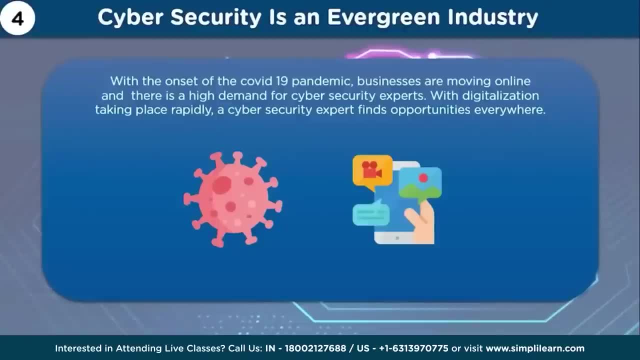 As long as you have good cybersecurity skills, there is no need to worry about job security, however late it is. Our fourth reason is cybersecurity is an evergreen industry. Cybersecurity has gradually become an evergreen industry In the current times with the onset of the COVID-19 pandemic. 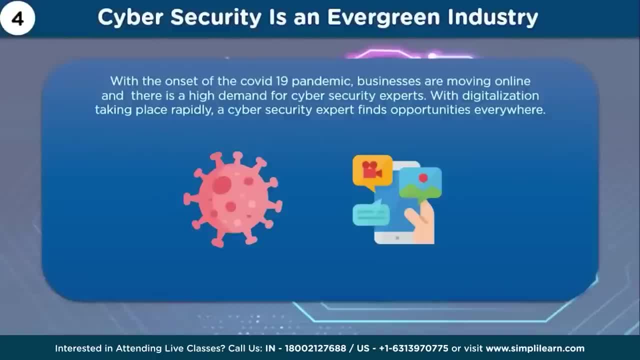 businesses are moving online and shifting to cloud storage, The demand for cybersecurity is at its peak. There is a high demand for cybersecurity experts who can safeguard digital data. Hence, we can be rest assured that cybersecurity is here to stay, And this domain is only going to grow in the coming years. 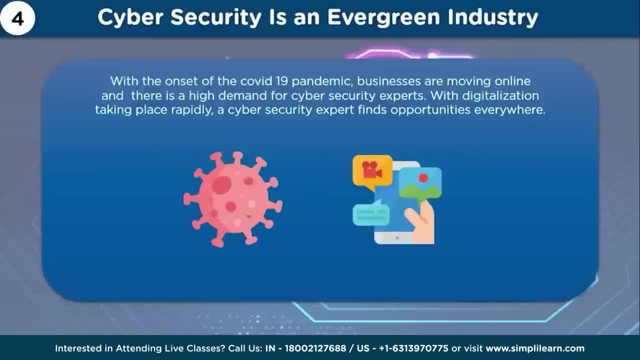 According to cybersecurity ventures, the number of internet users will hit a whopping 6 billion by 2022.. These numbers speak volumes, And this reveals the growing demand for cybersecurity professionals across the globe. Digitalization is taking place across several industries. A cybersecurity expert finds opportunities in every field, as every organization wants to be secure on the digital front. 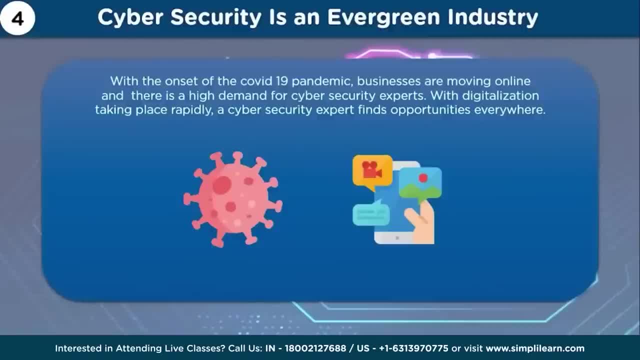 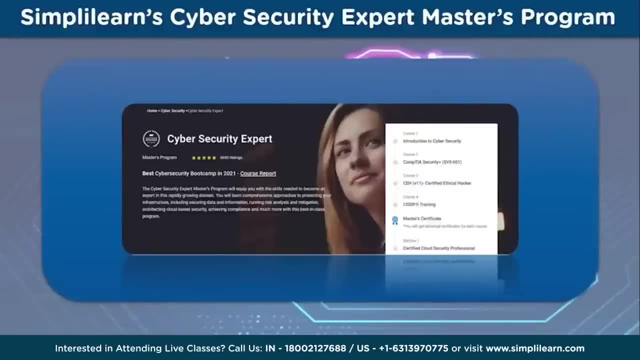 So now is the right time if you are looking to learn and start a career in cybersecurity. Before moving to our top three reasons to learn cybersecurity, Here are some crucial information for you. As you know, with relevant certifications, you can grow your cybersecurity career. 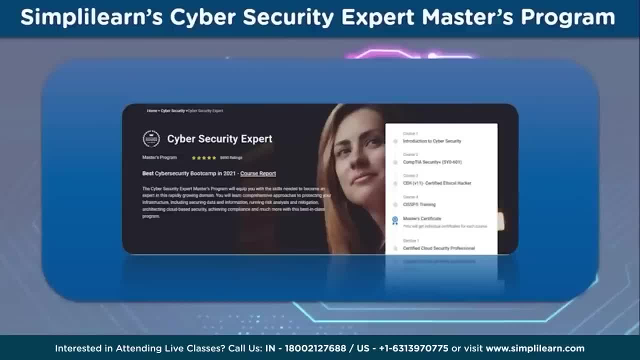 And here we are to help you with that. You can check out SimplyLearn's cybersecurity expert master's program to equip you with the necessary skills to become an expert in this rapidly growing domain. Training for highly sought-after certifications like CompTIA, Security+, CEH, CISM and CISSP is at the forefront of this course. 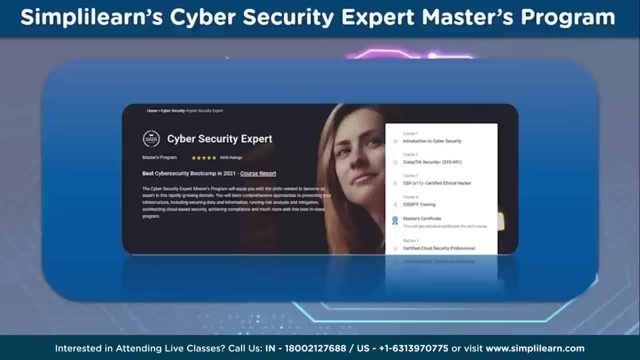 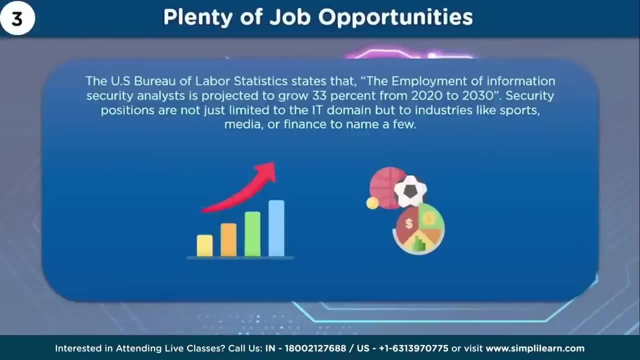 Preparing you for the industry's best jobs. So what are you waiting for? Get certified with SimplyLearn and grow your career in cybersecurity today. So our third reason to learn cybersecurity is because of the plenty of job opportunities it offers. According to the US Bureau of Labor Statistics, the employment of information security analysts is projected to grow 33% from 2020 to 2030.. 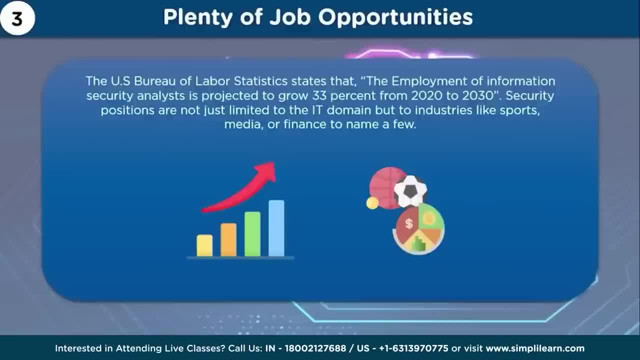 Much faster than ever And the average for all occupations. With the world turning digital, there is a dire need for companies to hire cybersecurity experts who can protect and safeguard sensitive data. As firms work to improve their cybersecurity structure, they are also hiring several cybersecurity experts to design, implement and maintain their cybersecurity solutions. 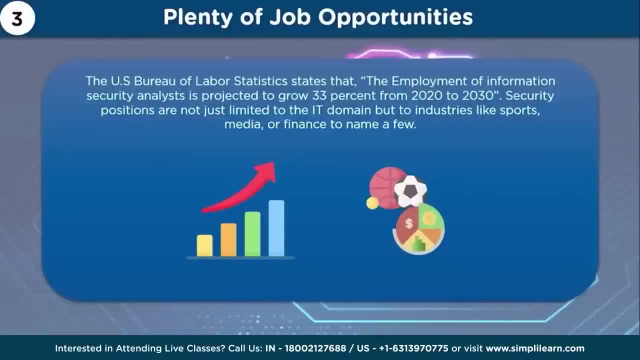 Cybersecurity jobs are not limited to the IT domain. Many security positions are found at companies outside of IT, Including industries like media, sports or finance, to name a few. This emphasizes on the fact that a cybersecurity expert is exposed to several job opportunities from different types of companies across the globe. 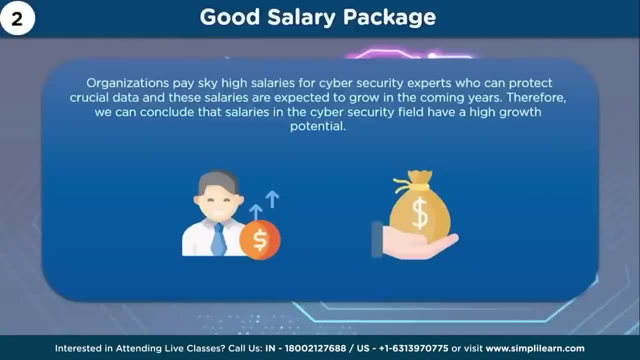 Our second reason for you to learn cybersecurity is the good salary package it offers. Salaries play a crucial part in any job that you undertake, isn't it? Every individual likes to get duly rewarded for their work, and cybersecurity is one such domain that provides fat paychecks. 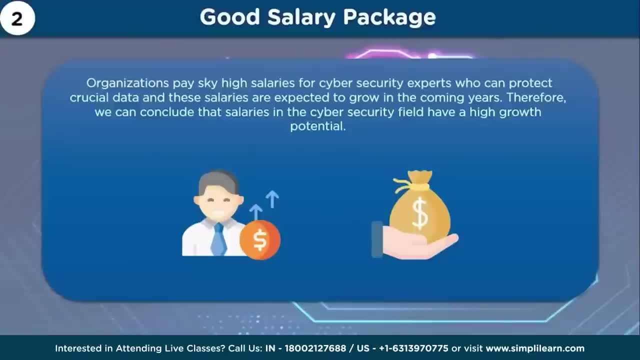 Cybersecurity experts are the individuals who have come to the rescue with the unprecedented rise in cybercrimes across the world. Organizations are willing to pay sky-high salaries for these cybersecurity experts. There is a lack of skilled cybersecurity professionals, and this is another reason cybersecurity experts are paid well. 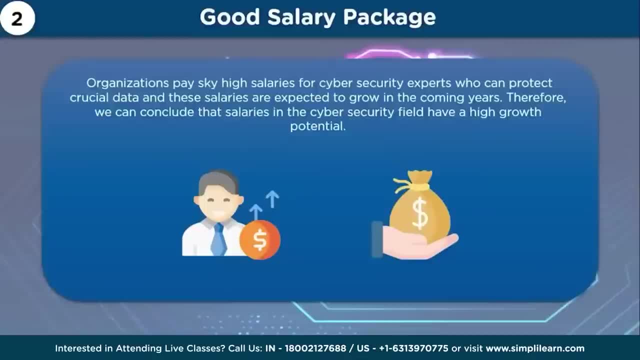 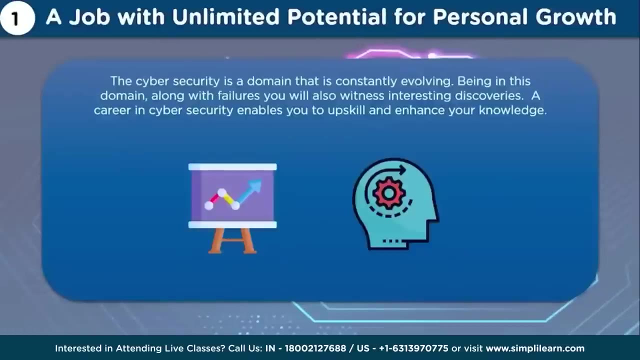 The salaries of cybersecurity professionals are still expected to grow in the coming times owing to the high demand. Salaries in cybersecurity have a high growth potential and if you are a skilled cybersecurity professional, you can always negotiate your salary. Finally, a top reason to learn cybersecurity is that you will have a job that never gets boring and a domain that offers unlimited potential for personal growth. 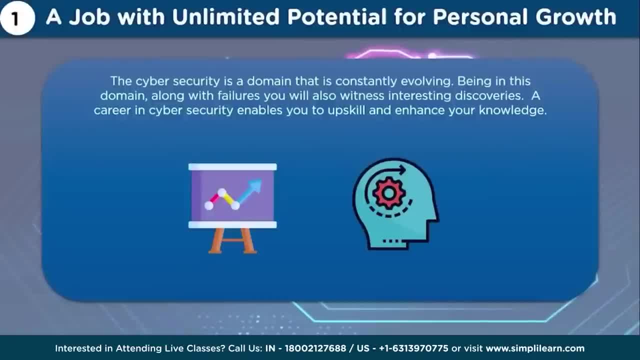 Several times, individuals find themselves lost in their career due to lack of challenges, due to their mundane work and also due to stagnation at work. These reasons play a major role when it comes to a professional quitting their job. However, a job role in cybersecurity tackles these reasons to an extent. 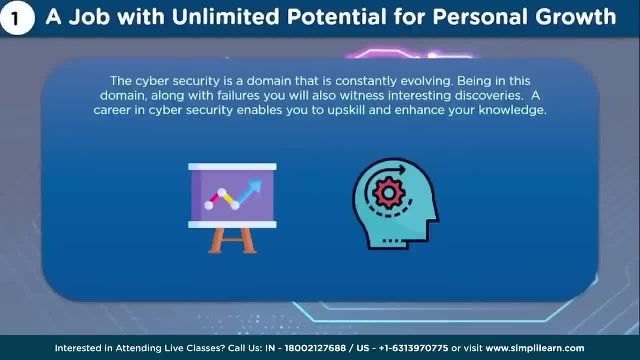 And that is why we have this reason at number one. Cybersecurity is a domain that is constantly evolving, and so are the nature of cyberattacks. Hackers are always trying to develop new methods to get to your data. They develop new exploits regularly. 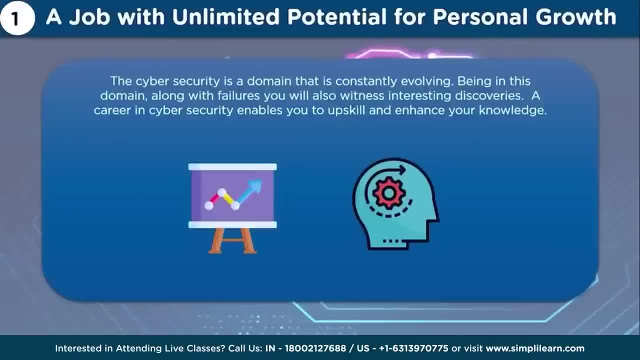 And hence, as a cybersecurity professional, you will face interesting challenges to find optimal solutions for new exploits. You will have new puzzles to solve. A cybersecurity career is not going to be stale. Along with failures, you will also be exposed to new and interesting discoveries. 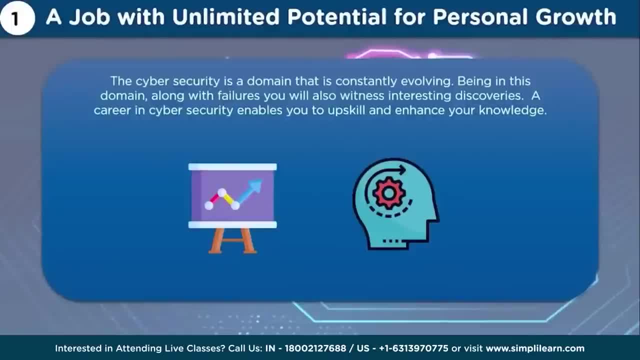 To keep yourself updated in this field and in the future, and to tackle cyberattacks. you should be in a position to outsmart the hackers. Being in the field of cybersecurity allows you to constantly upskill and enhance your knowledge and experience. It also ensures that your learning journey will never stop. 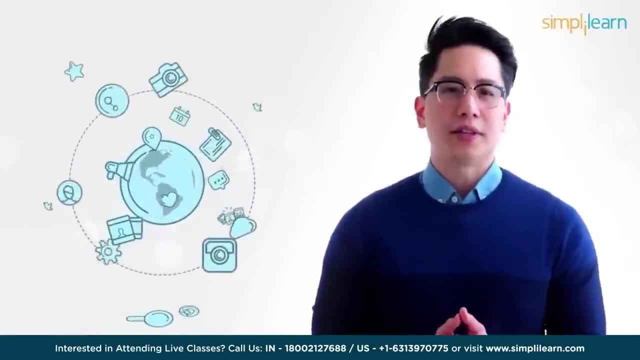 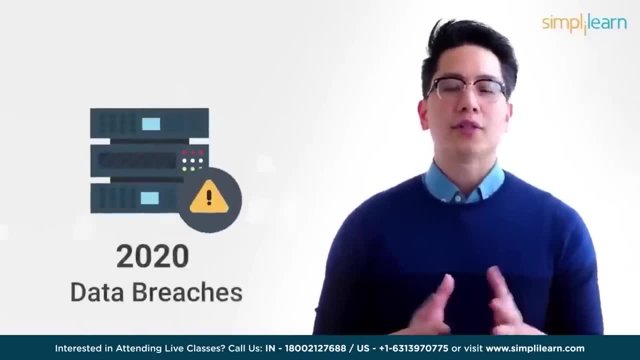 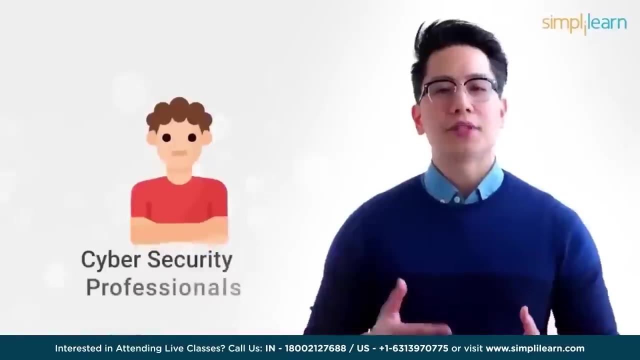 With the world turning, virtual cyberattacks are constantly flooding new headlines. COVID-19 accelerated the current digital transformation and the year 2020 witnessed several data breaches. Since technology has become more intertwined with our data, it is no surprise that the need for skilled cybersecurity professionals is increasing. 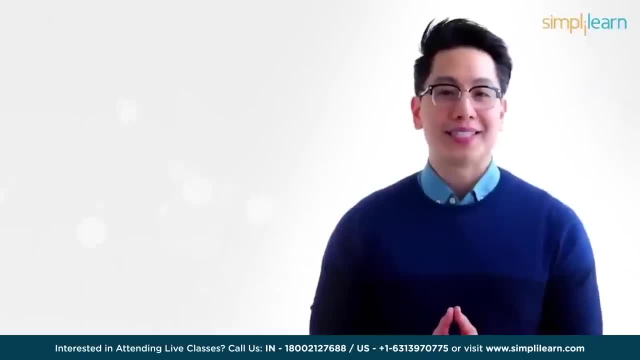 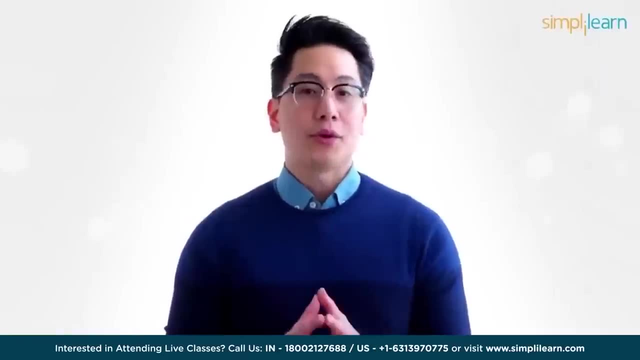 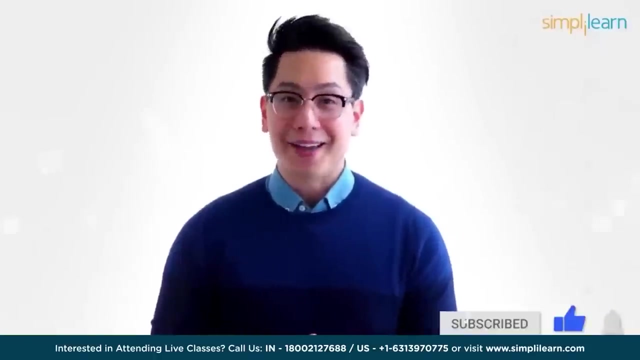 On that note, hey, everyone, welcome yet to another exciting video by Simply Learn, which will take you through the top cybersecurity career options available today. But before we begin, if you're new here and haven't subscribed already, make sure to hit the subscribe button and that bell icon for interesting tech videos every day. 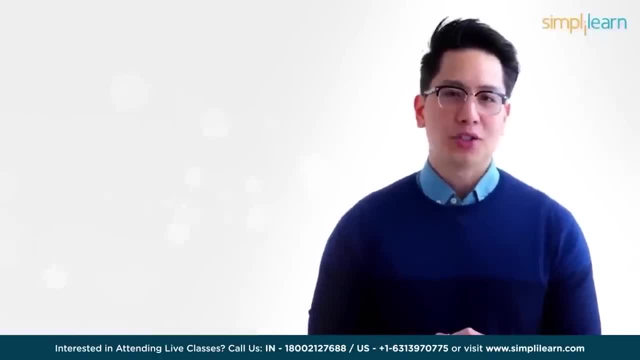 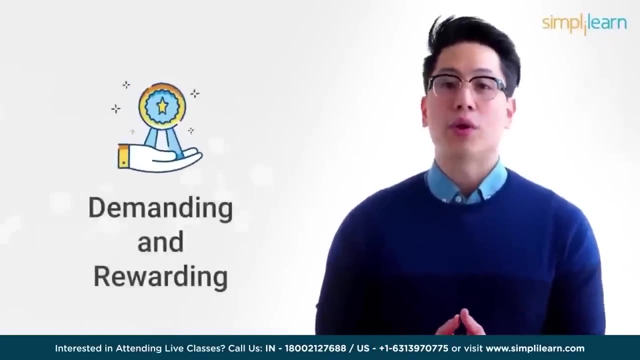 There is a significant lack of skilled cybersecurity professionals who can tackle the cybersecurity challenges facing them. There is a significant lack of skilled cybersecurity professionals who can tackle the cybersecurity challenges facing them. Hence, a career in cybersecurity is demanding and equally rewarding. Finding the right career path in the cybersecurity industry isn't always easy. 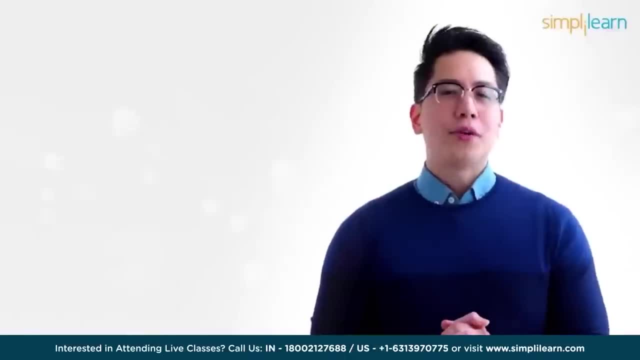 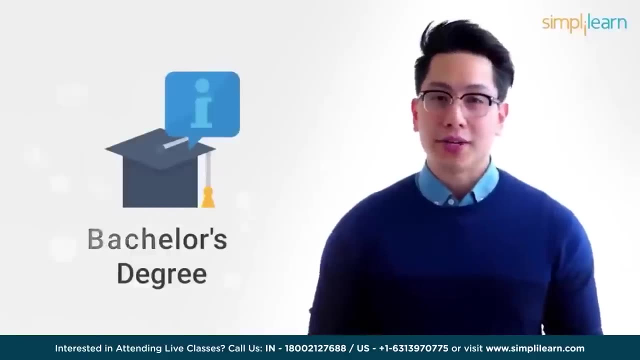 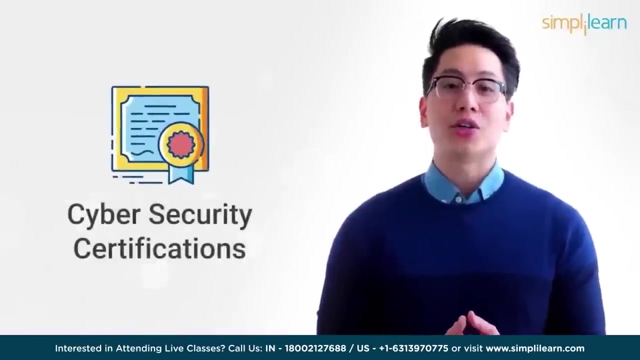 Here. we are here to help you with that. There are a few prerequisites for a career in cybersecurity, the basic one being a bachelor's degree in a subject relating to cybersecurity. However, if you don't have a relevant degree, you can always take up relevant cybersecurity certifications and kickstart your cybersecurity journey. 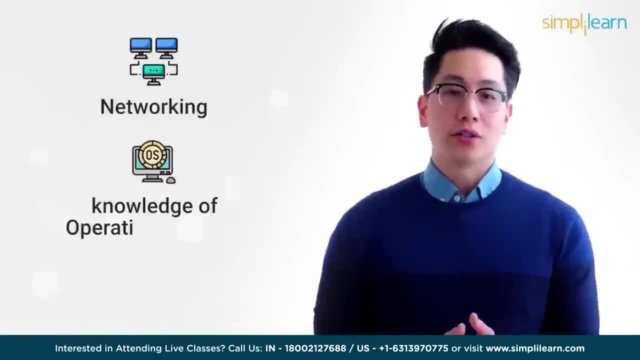 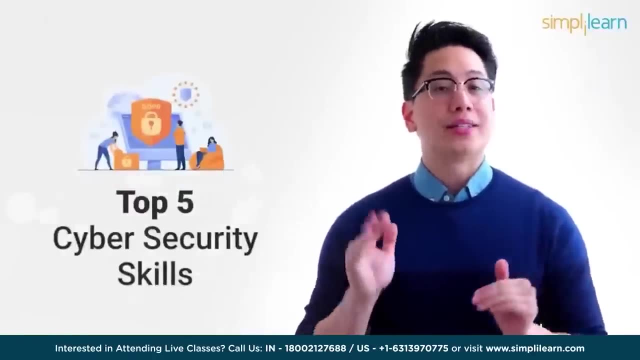 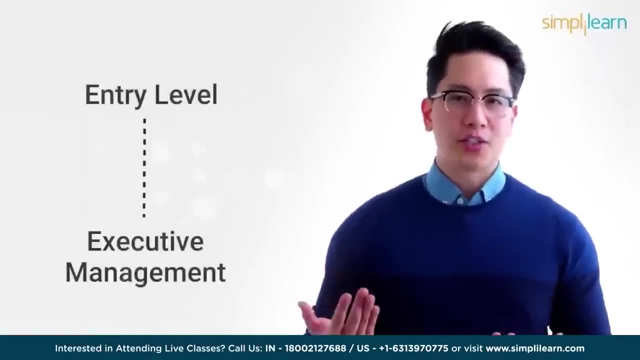 A few other skills like networking, knowledge of operating systems and cloud security are required to start and grow your cybersecurity career. You can check out our video on the top five cybersecurity skills to know more. Cybersecurity jobs vary from entry level to executive management and everything in between. 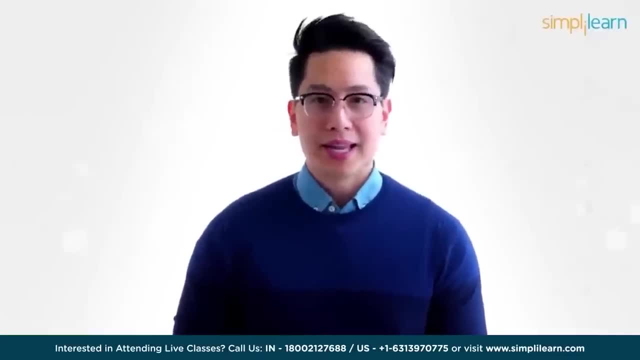 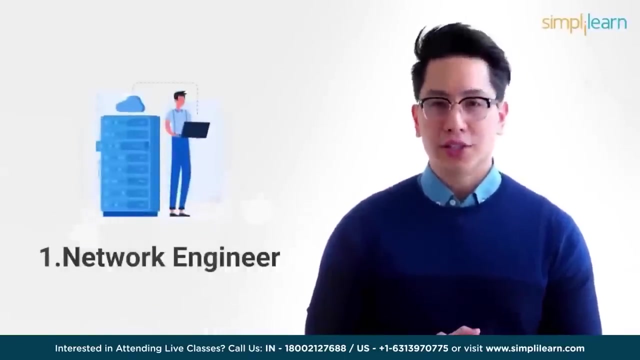 There are several cybersecurity paths available today. It is best if you start with entry level and then move on to the next level with the help of certifications and relevant experience. Here let us have a look at the top five cybersecurity job roles today. The first job role is that of a network engineer. 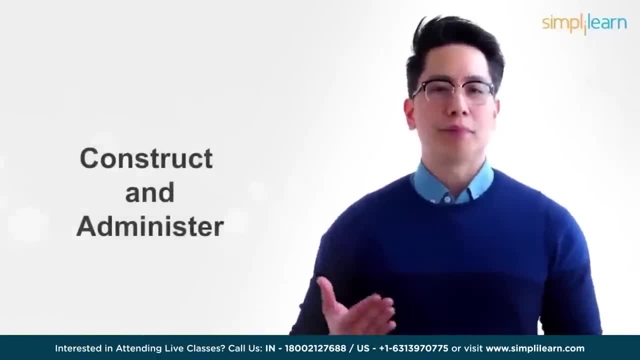 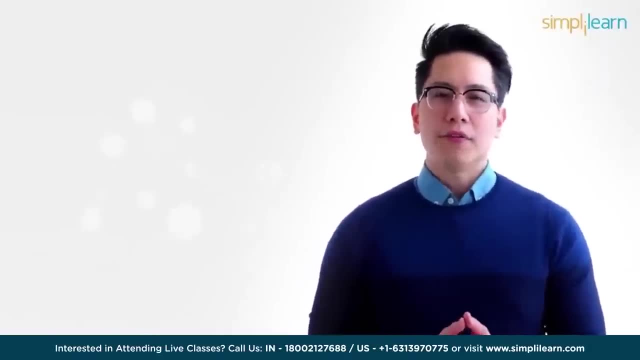 Network engineers construct and administer a company's computer networks. They are responsible for installing, configuring and supporting network equipment. They also configure and maintain firewalls, switches and routers. This entry level cybersecurity job can help you start your journey to become an ethical hacker. 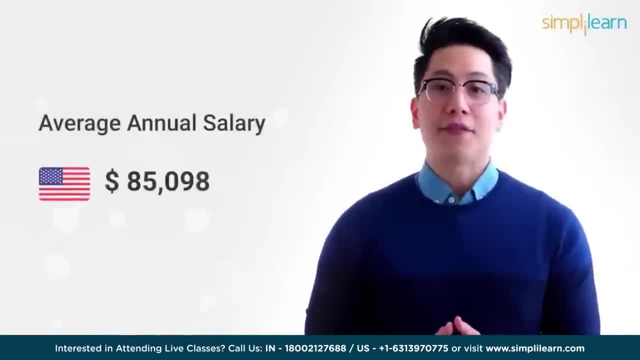 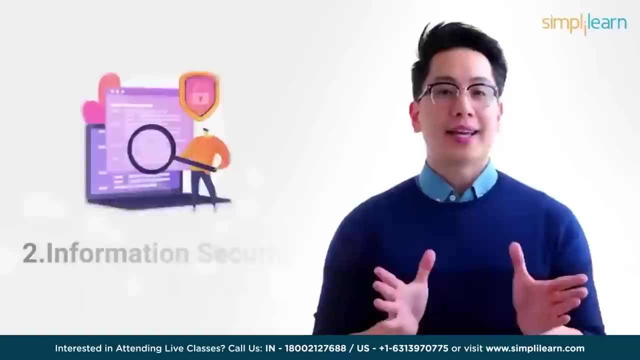 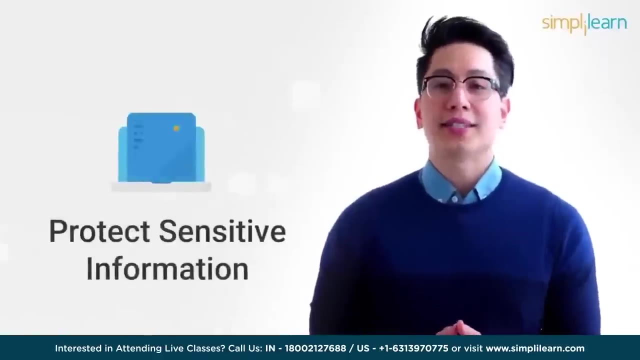 The annual average salary of a network engineer in the US is $85,098. And in India it is around 510,000 rupees. Second on our list is information security analyst. As an information security analyst, your primary duty is to protect sensitive information. Information security analysts create and implement plans for preventing cyber attacks. They monitor data access and ensure compliance with policies. Depending on the cyber threat, they decide if it has to be resolved or escalated further. In the US, an information security analyst earns $89,140 annually. 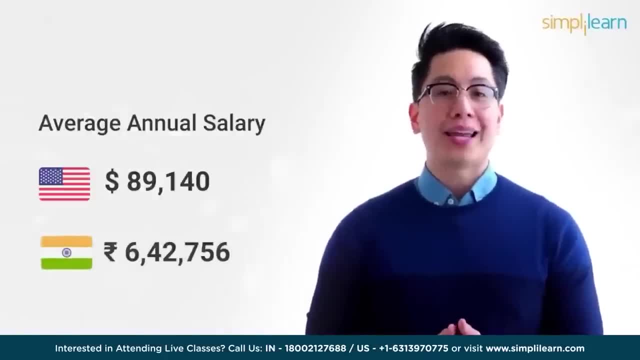 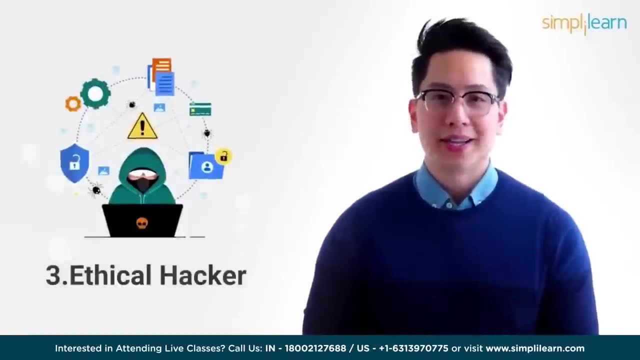 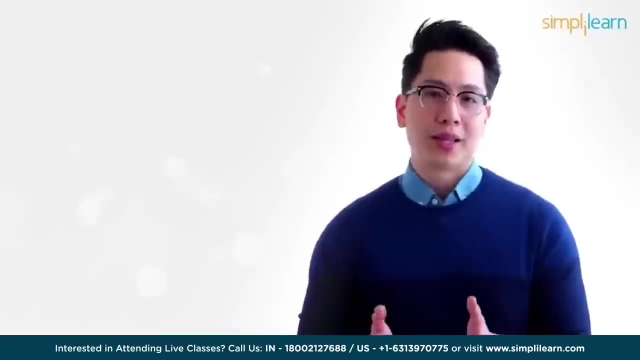 And in India they earn 6,42,756 rupees. Third on our list is ethical hacker. They are also known as penetration testers. They are network security consultants who identify and exploit system vulnerabilities just like how a hacker would do. They probe and test the network using various penetration tools and software. 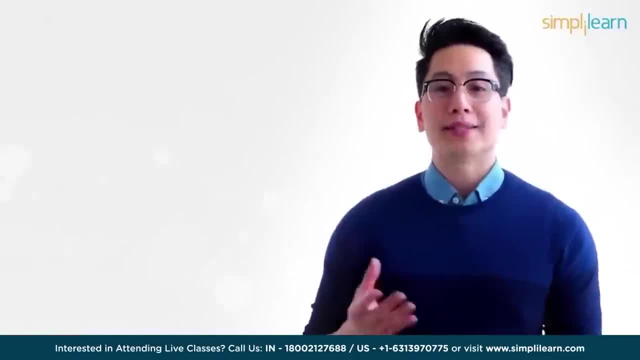 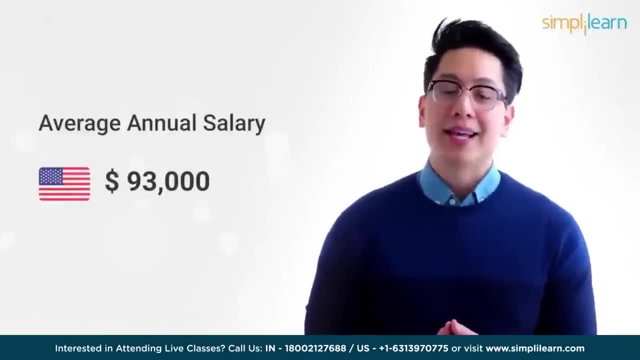 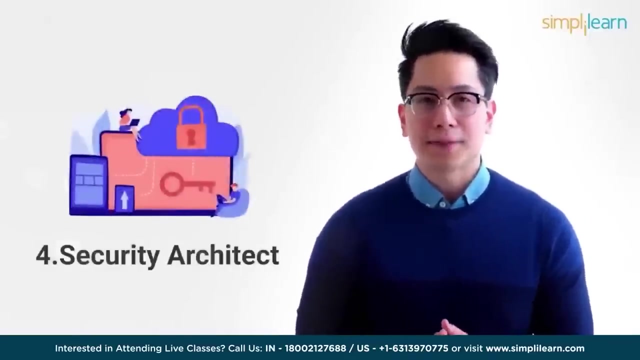 They also design new penetration tools And document the test results. In the US, a certified ethical hacker earns around $93,000 on an annual average basis, And in India they make around 5 lakh rupees. The fourth job role that we are going to talk about is security architect. 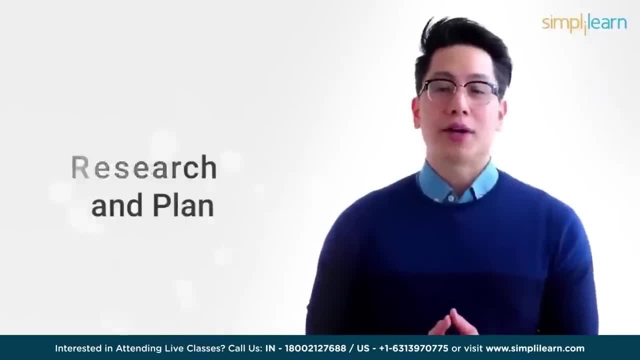 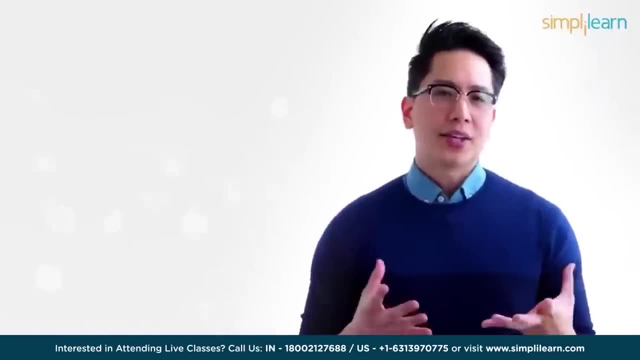 Security architects research and plan the security elements for their organizations. They design robust security structures that are capable of preventing malware attacks. A security architect approves the installation of routers, VPNs and firewalls. Their duties go beyond just architecture building and including formulating company procedures. 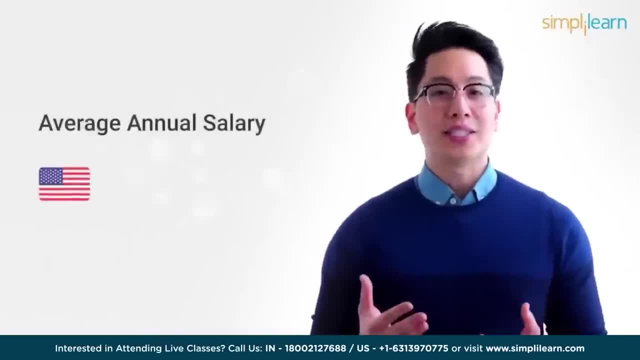 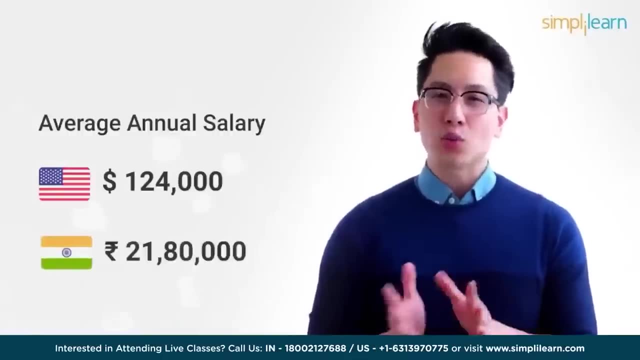 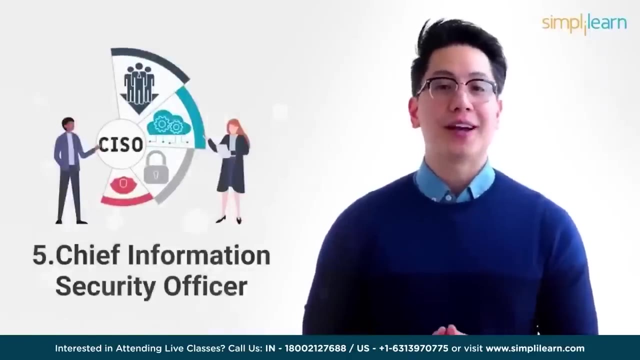 guidelines and user guides. Security architects in the US make a handsome sum of $124,000 a year on an average, And in India they make nearly 21,80,000 rupees. And finally, fifth on our list is chief information security officer CISO. 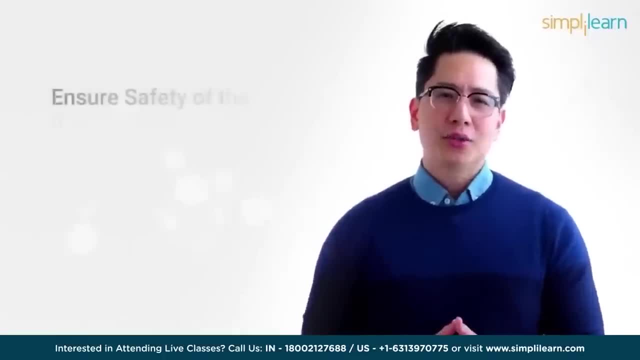 They are senior level officers in an organization. They ensure the safety of the information. they develop, implement and maintain information security and risk management programs. They also interact with stakeholders and regularly brief them with information security concerns. The average annual salary of a chief information security officer in the States is a whopping $165,000 annually. 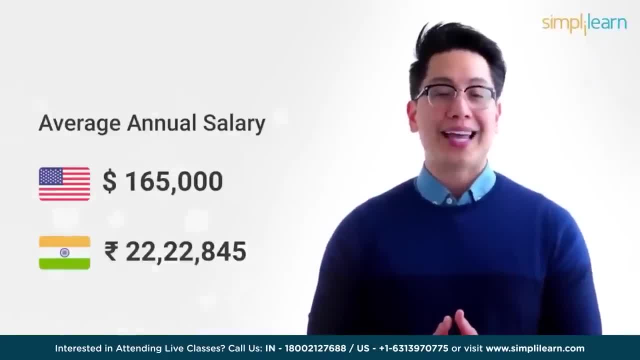 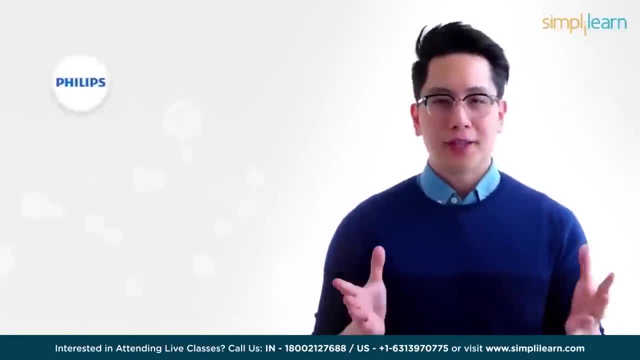 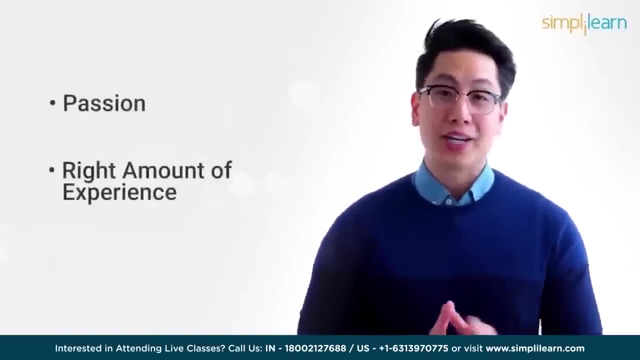 And in India it is 22,22,845 rupees. Several companies are looking for skilled cybersecurity experts. Some of them are cybersecurity professionals: Philips, Siemens, Google, Microsoft and GE, to name a few. With passion, the right amount of experience and relevant certifications, you can grow your cybersecurity career. 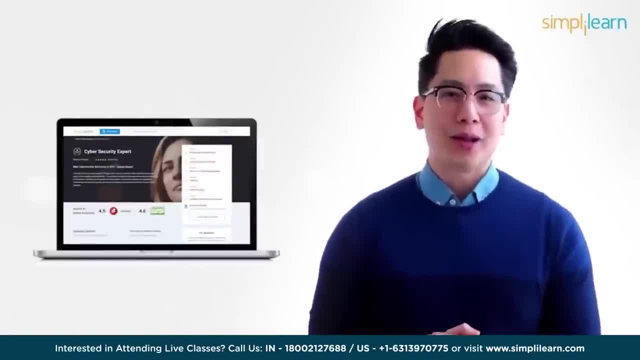 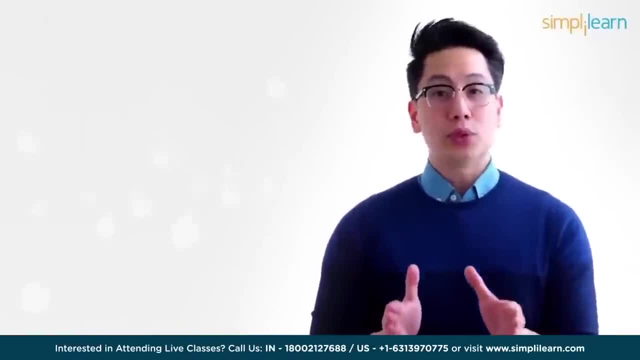 You can check out Simply Learn Cybersecurity Expert Master's Program to equip you with the necessary skills needed to become an expert in this rapidly growing domain. This course will help you learn various methods as to how you can protect your infrastructure, secure your data. 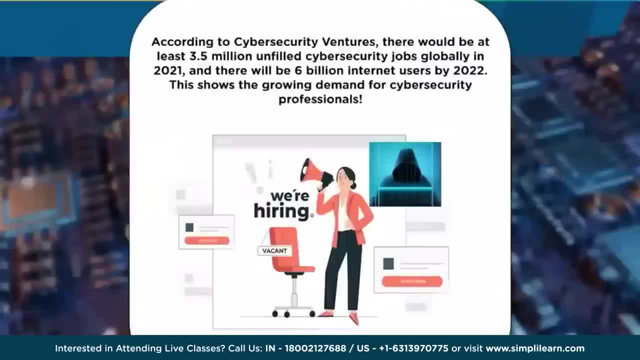 run risk analysis, achieve compliance and much more. According to Cybercrime Magazine, by Cybersecurity Ventures, globally there would be nearly 3.5 million unfilled cybersecurity jobs by 2021, and the number of internet users will hit a whopping 6 billion by 2022. 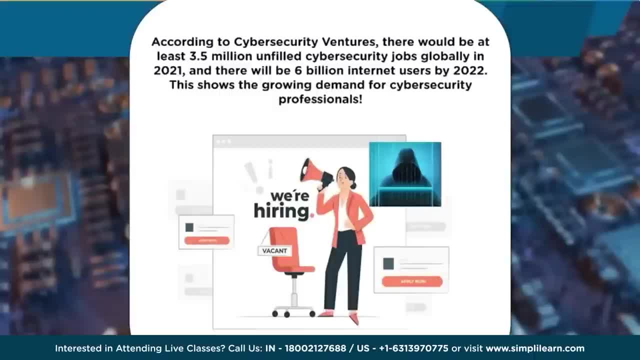 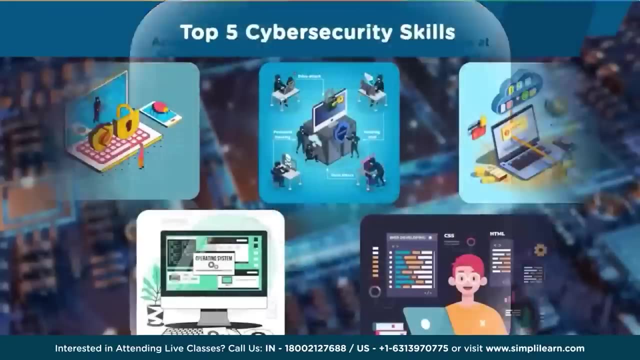 These numbers speak volumes and this shows the growing demand for cybersecurity professionals across the globe. Now that you know the high demand for cybersecurity professionals, let us help you start your cybersecurity career by bagging the right skill set. Many of you out there might be waiting to become a cybersecurity professional. 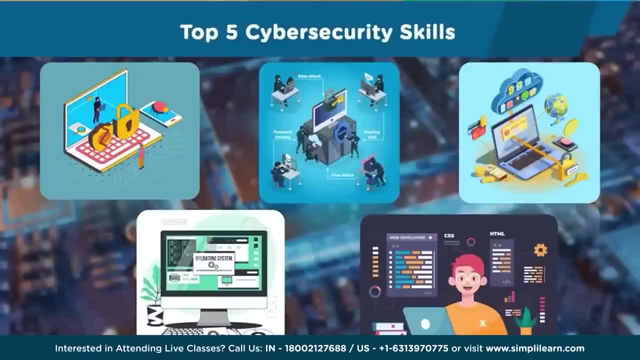 but are unsure of how to go about it and what skills you would need to get a cybersecurity job. Not to worry, we are here to help you with that. After extensive research, we have come up with the top 5 skills that will help you get into the field of cybersecurity. 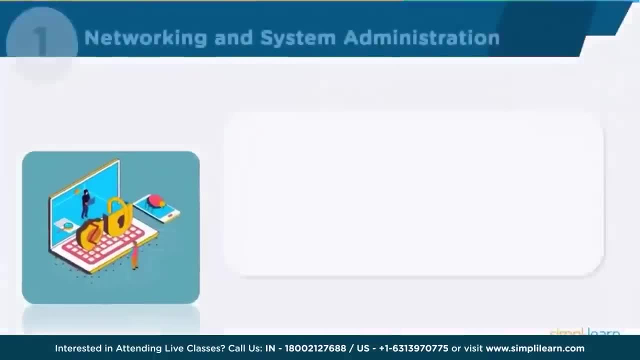 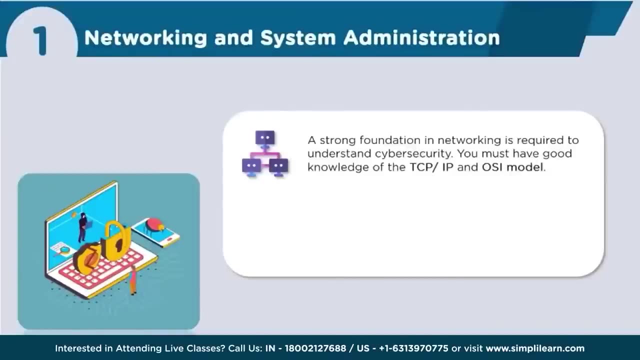 Let's have a look at these skills individually. First we have networking and system administration. The number one skill you need to have to enter the field of cybersecurity is computer networking. Networking is the backbone of the internet. It is imperative that you have an in-depth understanding of networking to start a career in cybersecurity. 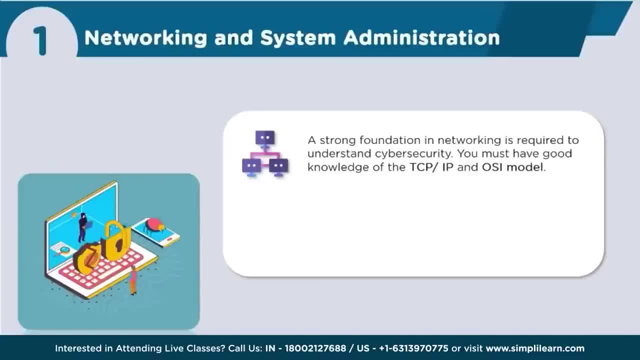 A network is a group of interconnected devices and networking is the art of understanding how data is sent, transmitted and received amongst these devices. You need to know various routing protocols. The TCP, IP and OSI models govern networking. The OSI model is comparatively newer. 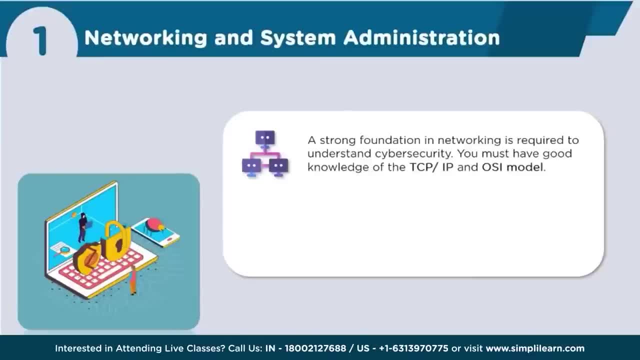 Basically, in these models, all the protocols are grouped into layers and work together to help you receive data on your device sent from a server. Learning networking will help you understand the technical aspects of data transmission, which will help you secure your data. You can take up networking certifications like SecurityPlus and Cisco CCNA. 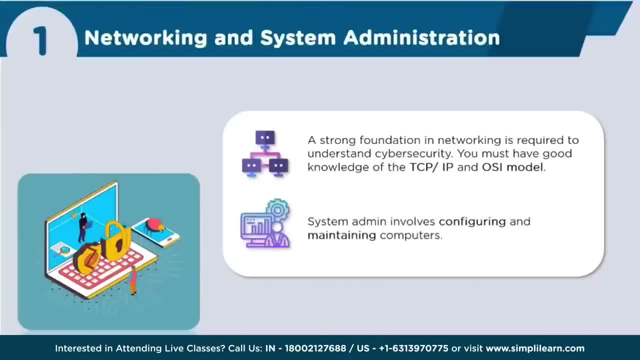 to gain a strong networking foundation. Another skill that'll be beneficial for you is to master system administration. If you think about it, all of us are sysadmins at some level. System administration is all about configuring and maintaining computers. You must be curious to know every aspect of your computer features and settings and play around a bit. 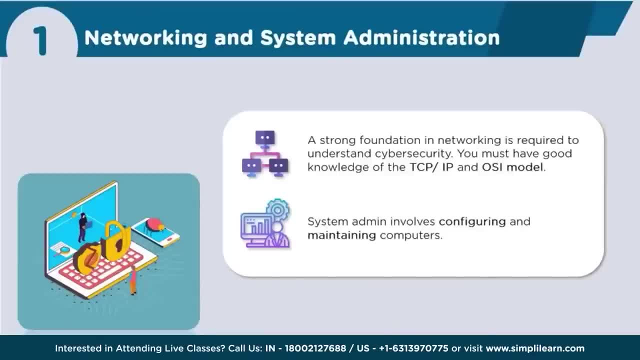 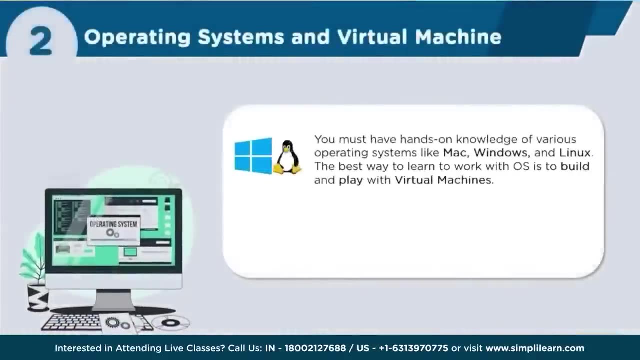 Carry out a trial and error method and give yourself small tasks like recovering deleted files or monitoring old viruses on a VM. Explore new techniques, put them into use and expand your knowledge. Let us now move on to our second skill: Knowledge of Operating Systems and Virtual Machines. 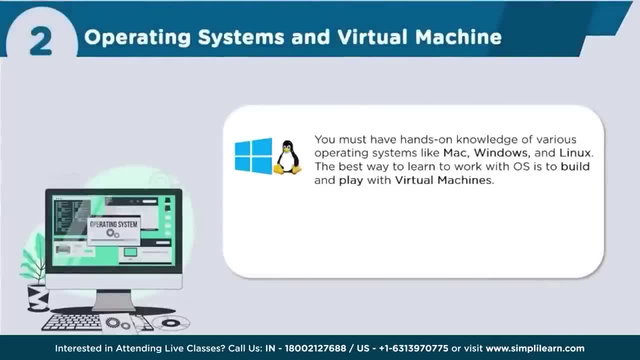 To become a cybersecurity professional, you need to have a strong knowledge of operating environments such as Windows, Linux and Mac OS. Cybersecurity professionals largely use Linux and it comes with several tools To learn operating systems, go ahead and set up and use virtual machines and play around with them. 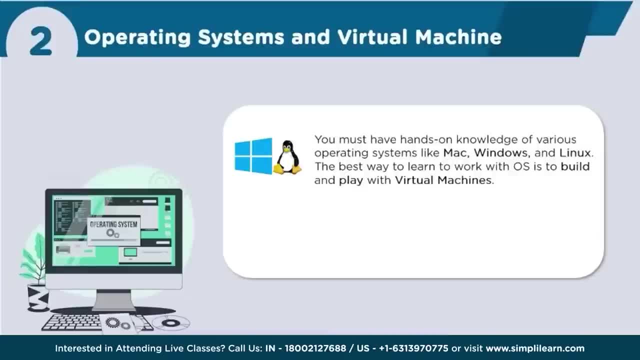 This will help you gain hands-on experience As a cybersecurity expert. you should be comfortable working on any OS. VMs allow you to train and research in an isolated environment and help you maximize your skills. The next point to remember is to know Kali Linux. 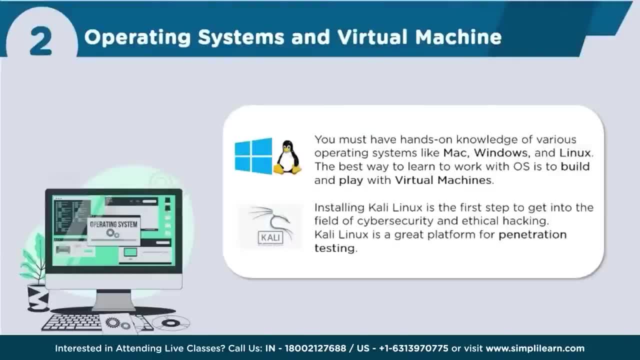 It is the most widely known Linux distribution for ethical hacking and penetration testing. It comes with several hundred tools related to penetration testing, malware analysis, security research, computer forensics and so on. Kali contains several projects and you can learn a lot. 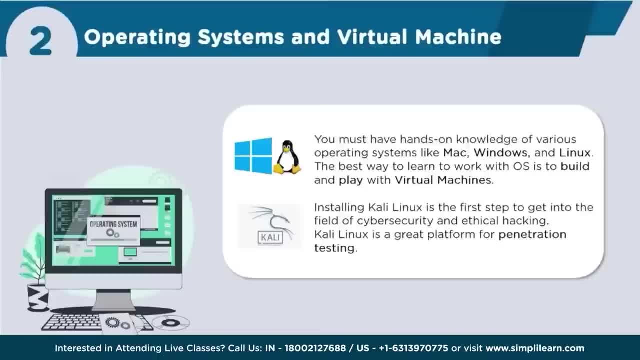 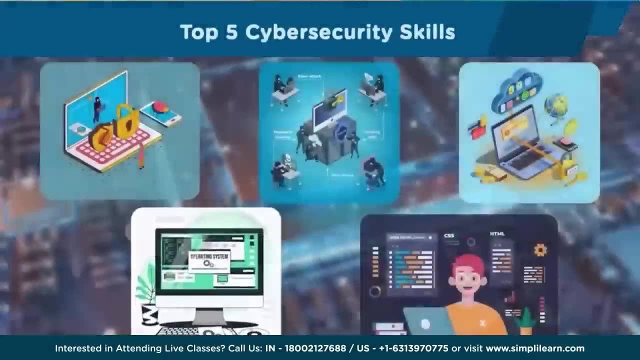 Another good thing about Kali is that it is free to use. So what are you waiting for? Download and start right away. Remember that Linux is the backbone of cybersecurity and a commonly asked topic for cybersecurity interviews, especially for pentesting roles. Moving on to our third skill, 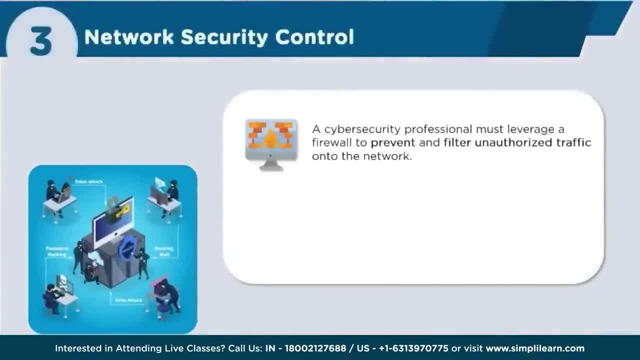 Our third skill is Network Security Control. It is another big one. It is another basic skill that every cybersecurity professional should have. Network Security Control refers to the different measures which are employed to enhance the security of a network. It is simple: You can only safeguard your network if you know how it works. 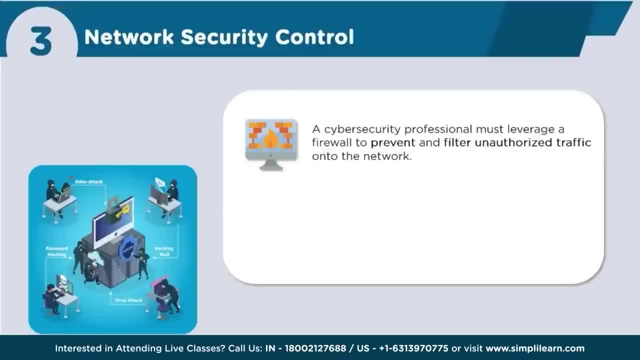 how routers, firewalls and other devices work. A firewall is a hardware or software that blocks incoming or outgoing traffic from the internet to your computer. Firewalls are required to secure a network. As a cybersecurity expert, you must be able to leverage a firewall to filter and prevent unauthorized traffic onto the network. 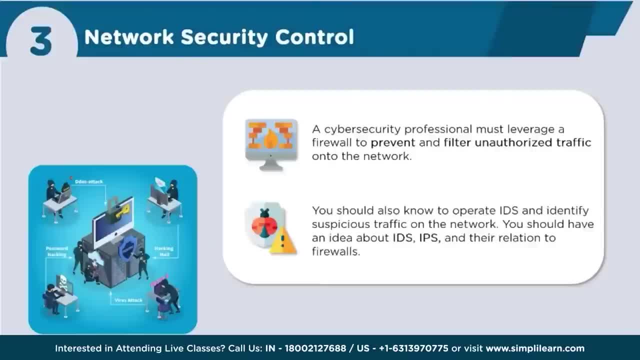 In addition to that, as a cybersecurity expert, you must know about intrusion detection systems, intrusion prevention systems, virtual private networks and remote access. An intrusion detection system is designed to detect unauthorized access to a system. It is used together with a firewall and a router. 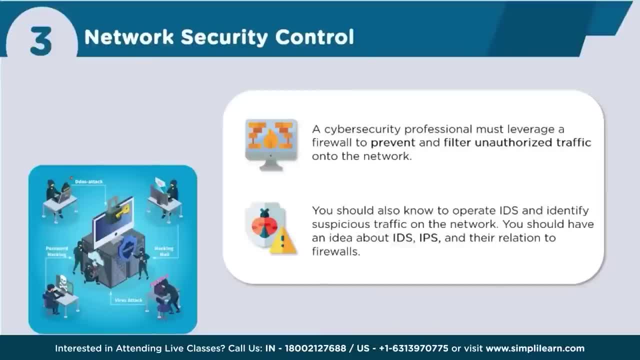 You should be able to operate the IDS and recognize any security policy violations and malicious traffic on the network. As many of you may have used, a VPN is a connection between a VPN server and a VPN client. It is a secure tunnel across the internet. 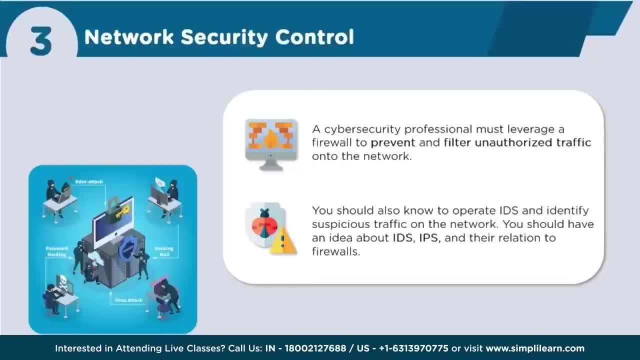 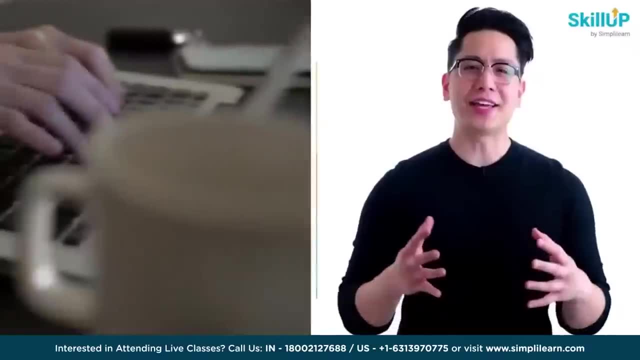 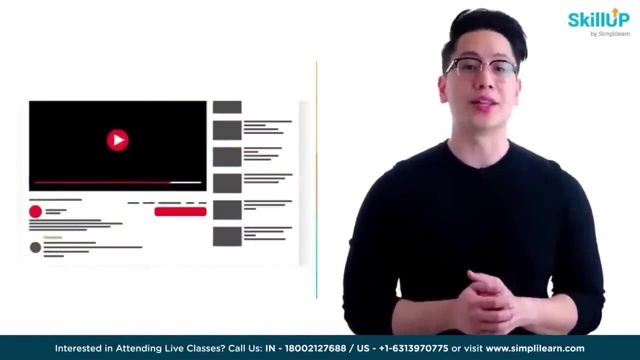 Moving on next up, we have an interesting skill. Any idea what that is? If yes, pause and leave a comment as to what you think the next skill will be. Visit SkillUp by SimplyLearn. Click on the link in the description to know more. 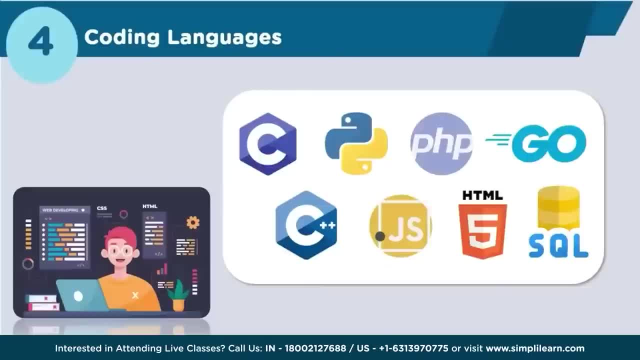 We have a lot of opportunities in the future. Knowing a couple of programming languages will help you identify the plan behind an attack and defend against deadly hacking techniques. So, as seen on your screens, these are the best programming languages to learn to make your cybersecurity career worthwhile. 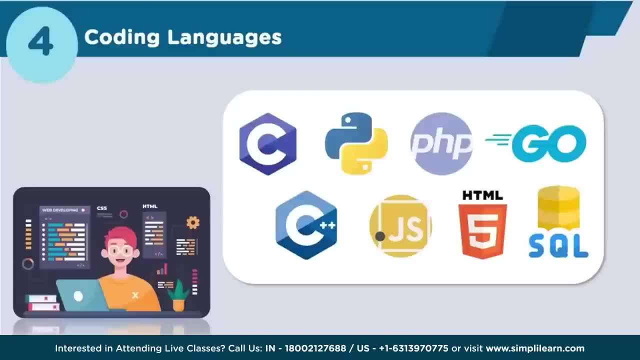 We have C and C++. The C programming language is the backbone of most operating systems. C and C++ are low-level programming languages that you need to know as a cybersecurity professional. On the other hand, Python is a high-level programming language that is becoming popular among cybersecurity experts today. 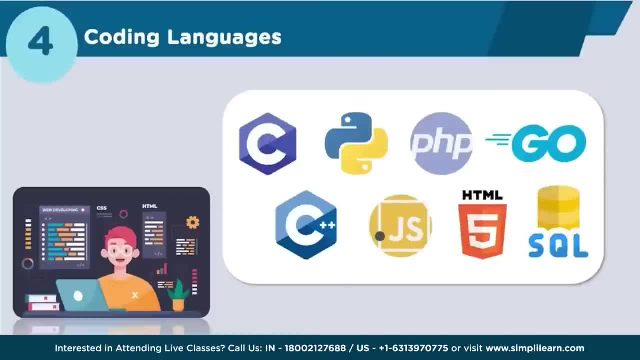 Knowing Python will give you an upper hand in your career. It will help you identify and fix vulnerabilities. JavaScript is another high-level programming language that adds interactivity to web pages. A good advantage of knowing JavaScript is that you can prevent cross-site scripting attacks from occurring. 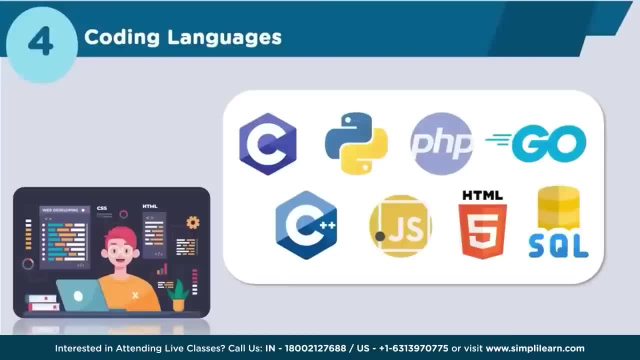 As in these attacks, the attacker implants malicious code in a web application Speaking of PHP, because most of the websites are created using PHP learning it will help you defend against intruders. Similarly, HTML is another language cybersecurity professionals should understand, as most websites use it. 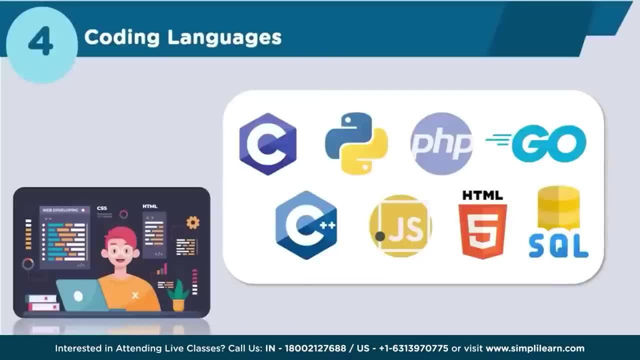 And it is one of the easiest languages to learn. Another programming language that you can use is Golang. It is great for cryptography. You can solve various cybersecurity problems with it. Then we have SQL. That is Structured Query Language. Attackers use this language to damage the stored data. 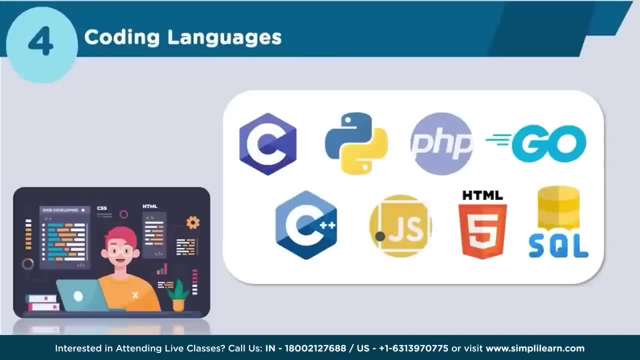 One such example is the SQL injection attack. Hence, having a good understanding of SQL will be highly beneficial. Another point we'd like to highlight is to have knowledge of assembly language. This will help you become a cybersecurity engineer. Assembly will help you understand how malware functions. 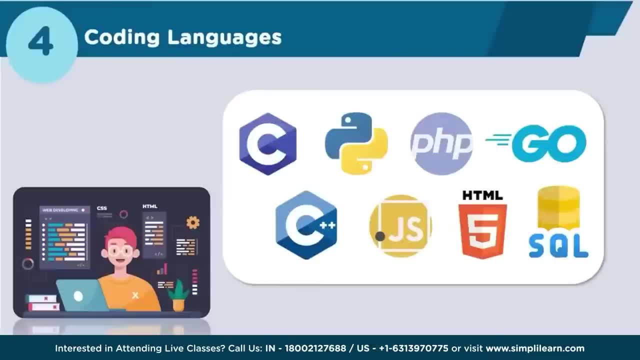 and thereby help you defend against it. In the cybersecurity domain, you can't just lock into a single language, and hence it is advised that you're acquainted with a couple of them. You can also do a crash course with these languages and learn them. 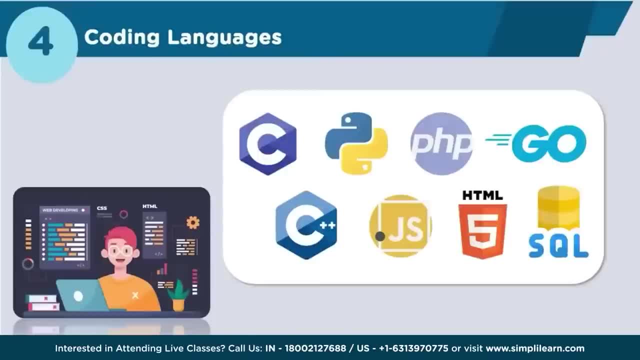 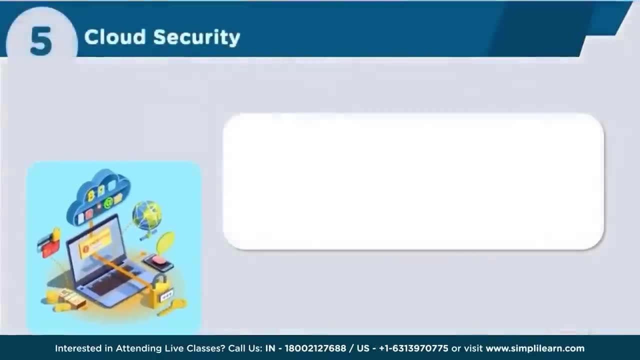 Hence determine the best programming language for your cybersecurity role and get familiar with the basics. Moving on, our fifth skill on the list is cloud security. There is a growing demand for cybersecurity professionals with cloud security skills in the coming years. Companies are on the lookout for professionals with security skills. 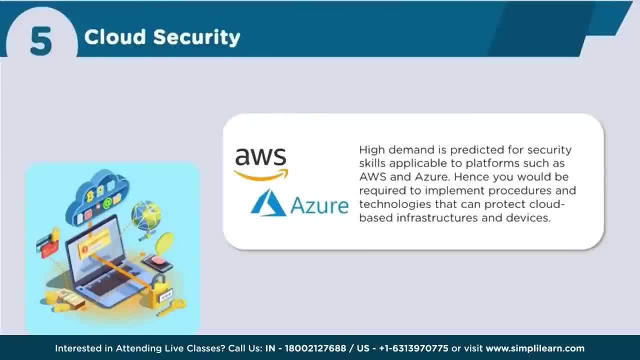 applicable to public and hybrid cloud platforms such as Amazon Web Services and Azure. More organizations look to cloud infrastructure to store data and run applications. This includes the implementation of policies and technologies that protect cloud-based systems and devices, Just like application development security. 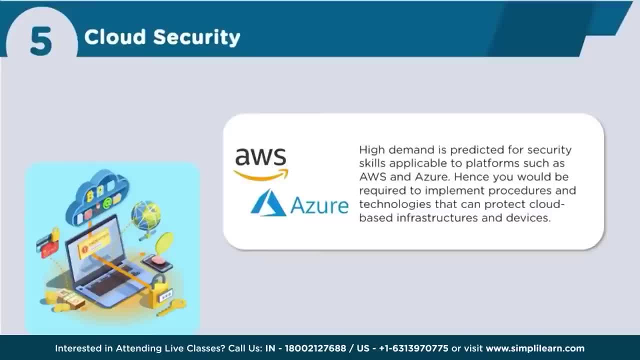 cloud security also involves building secure systems from the start. Companies want professionals who can manage the cloud security tools to identify and prevent any cloud breaches. People with experience and knowledge in managing big platforms such as Microsoft Azure, AWS and the GCP are in high demand. 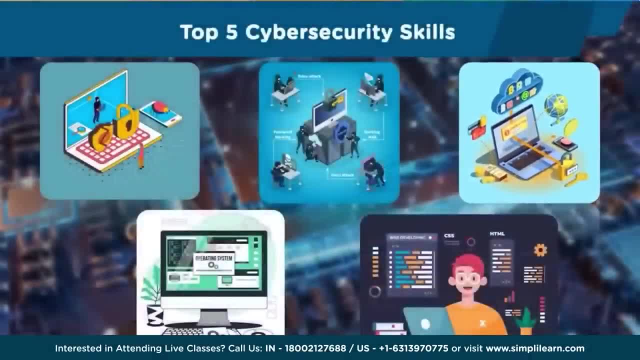 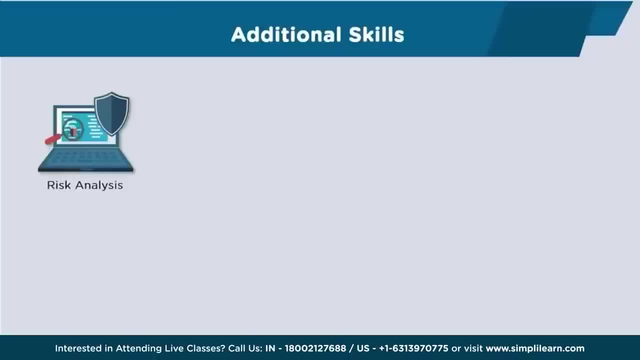 Now that we have seen the top five cybersecurity skills, let us go through a set of additional skills that can help you get into the cybersecurity field. Remember that to become a successful cybersecurity expert, you must possess a rich and diverse skill set. So in our list of additional skills, 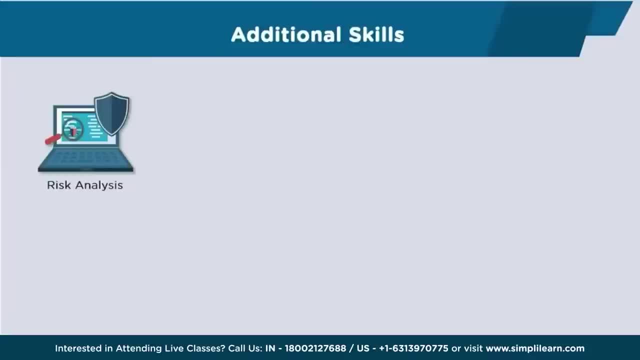 first we have risk analysis. Identifying risks even before their arrival is a great skill. Cybersecurity professionals are required to identify, manage and mitigate risks. Risk management and mitigation is a skill set that is going to be highly in demand in the coming years. 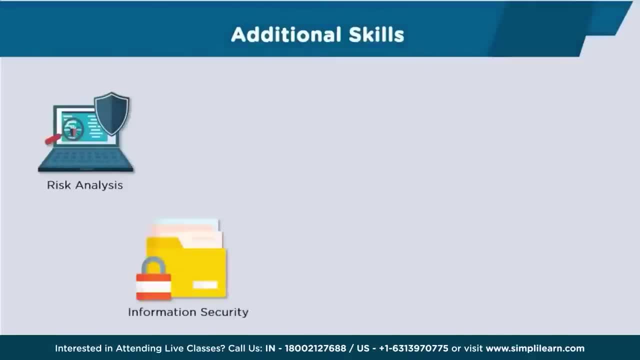 Next we have information security. Companies require skilled professionals who can protect their electronic data from unauthorized access. Here, in-demand skills are authentication, authorization, malware analysis and data recovery. Next on our list is security: incident handling and response As a cybersecurity expert. 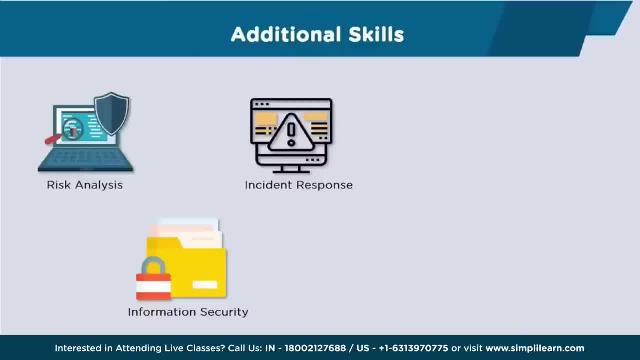 you must be prepared to handle any forthcoming threat of violating an organization's security policy. By following an updated incident response plan, your team can proactively protect your data and minimize the damages In security. incident management, you are required to identify, manage, record. 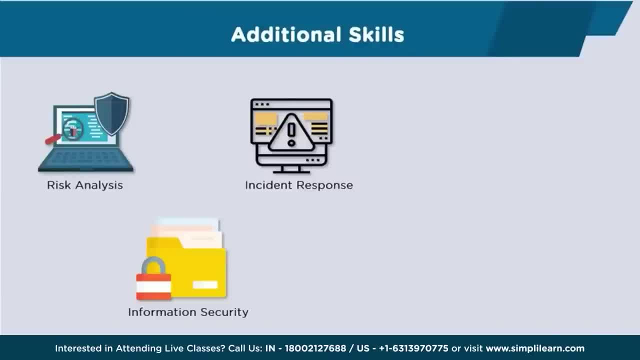 and analyze security threats in real time. A security incident can be an active threat or a successful compromise of data or an attempted intrusion. It can also be incidents like DDoS attacks, phishing, APTs, ransomware and many more. 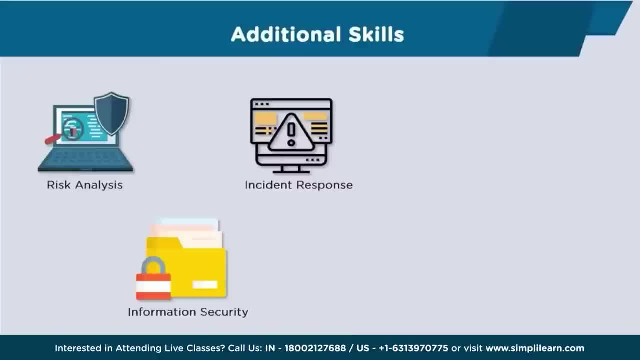 Another important pointer is that, as a security practitioner, you must also manage and analyze the security information and event management tools and services. Moving on, we have security audit. Security auditing is an internal check that is carried out to find flaws in the organization's information system. 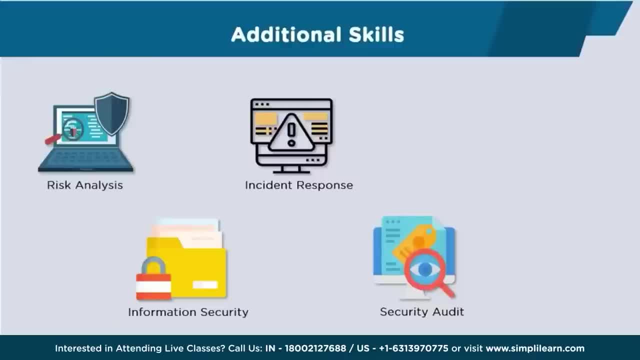 You must be able to conduct a review of the organization's adherence to regulatory guidelines. Security, audit and compliance knowledge are very crucial, as any misdeed of regulatory compliance could lead to hefty penalties. Soon organizations will need people who are more familiar with the various 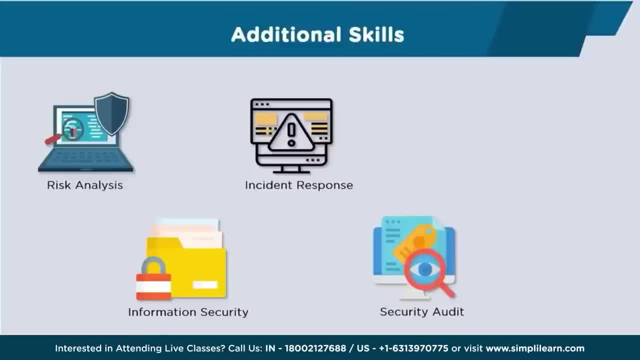 data privacy regulations. If you are good at paperwork, you can capitalize on this skill. Companies will need people who can understand what paperwork to file and which security protocols to use to comply with the regulations. Finally, we have laws and regulations and- often overlooked- cybersecurity aspect. 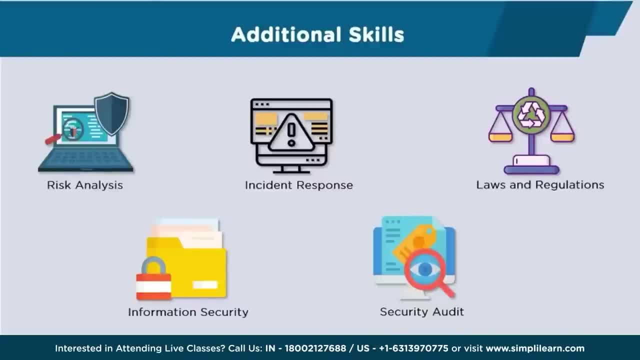 There are several cybersecurity laws and regulations, and if you break these laws, intentionally or not, it doesn't matter, as you will still be charged. These laws define how you can use the internet, and it also defines how people can be protected from becoming the victims of cybercrimes. 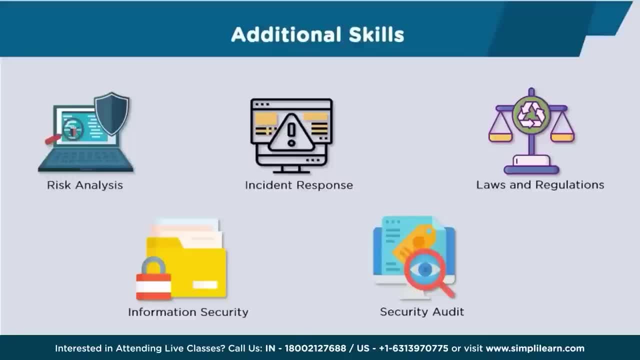 Knowing these laws and regulations and following the best practice will make you ethical at your job, and this will, in turn, be good for your organization. So those were our list of additional skills. Apart from these, make sure you stay updated with new hacks and learn new tools. 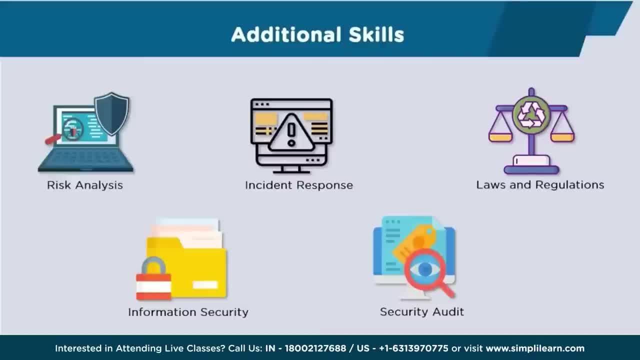 as cybersecurity is ever evolving. Another important skill apart from these technical skills is your soft skills. Having a set of good soft skills will help you bag your dream job. We have a video on the top 5 soft skills that will help you grow in your career. 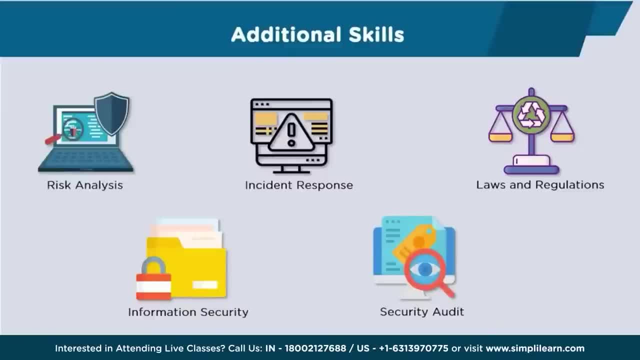 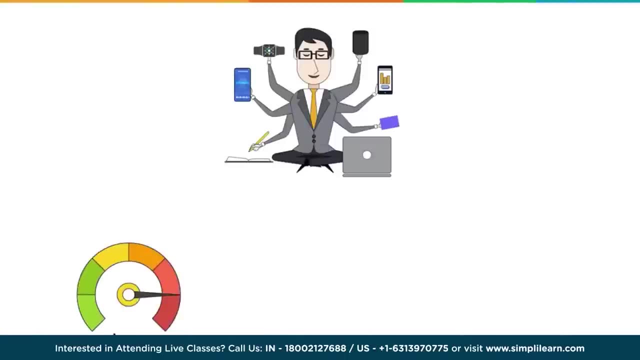 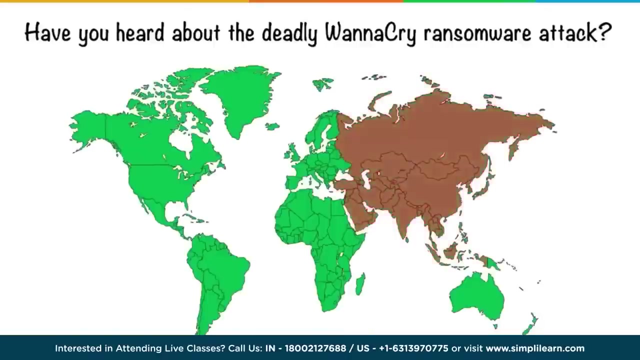 Do watch that and incorporate those skills as well. 8. Protecting all of our digital data, such as our net banking information, account credentials and medical reports. Have you heard about the deadly WannaCry ransomware attack? The attack happened in May 2017 in Asia. 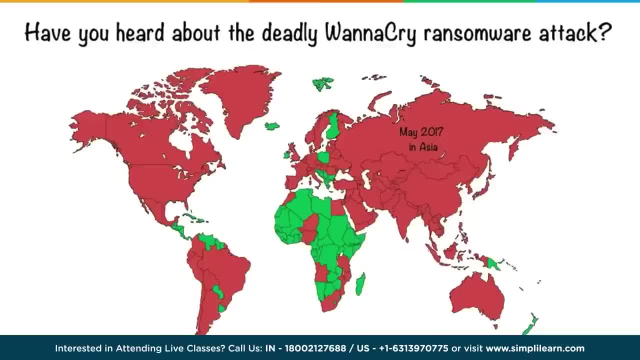 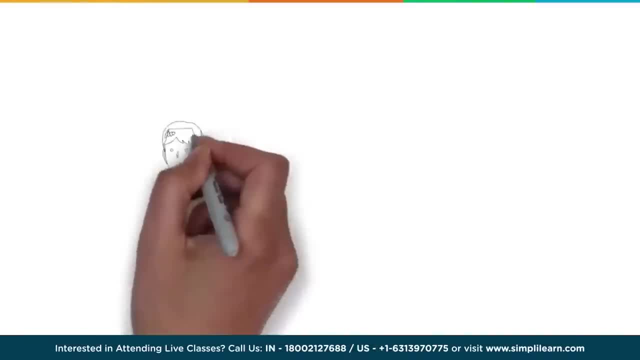 and then it spread across the world. Within a day, more than 230,000 computers were infected across 150 countries. The WannaCry cryptoworm encrypted the data and locked the users out of their systems For decryption of the data. 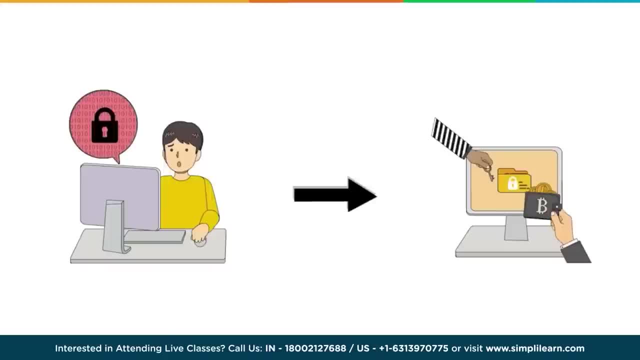 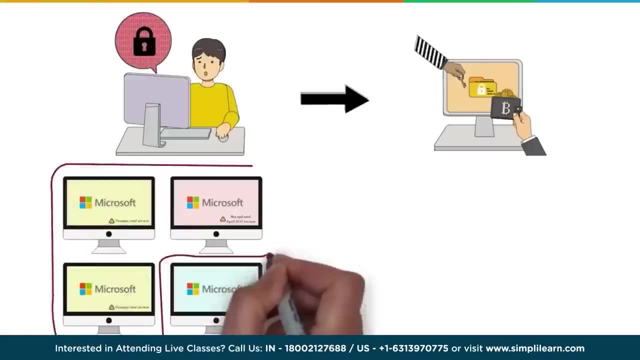 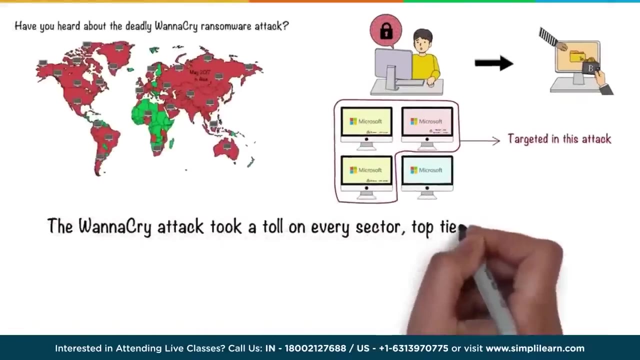 the users were asked for a ransom of $300 to $600 in Bitcoin. The users who used the unsupported version of Microsoft Windows and those who hadn't installed the security update of April 2017 were targeted in this attack. The WannaCry attack took a toll on every sector. 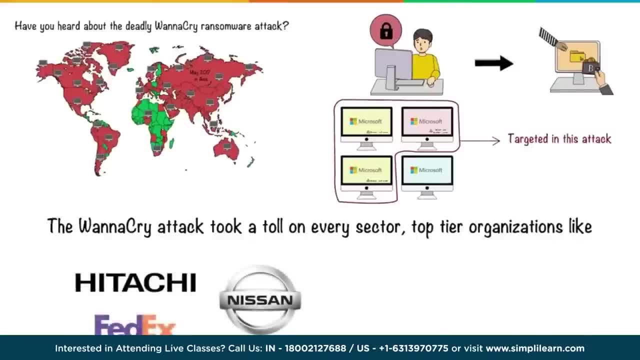 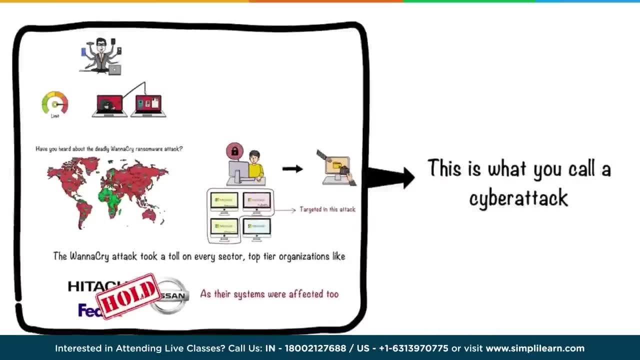 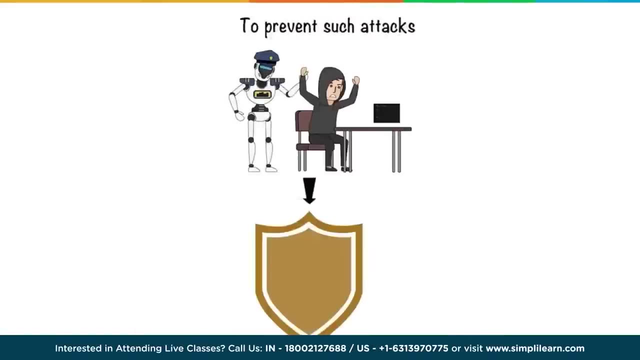 Top-tier organizations like Hitachi, Nissan and FedEx had to put their businesses on hold, as their systems were affected too. Now this is what you call a cyber attack. To prevent such attacks, cybersecurity is implemented. We can define cybersecurity as the practice of protecting networks, programs, computer systems. 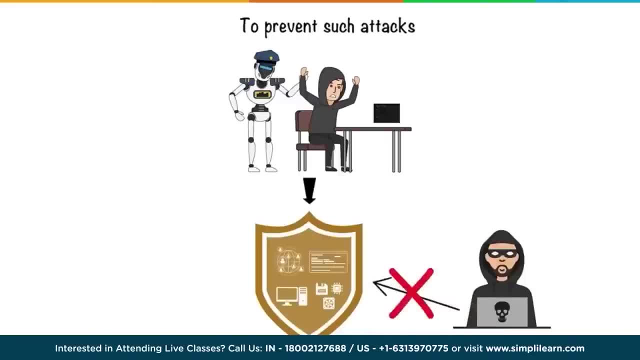 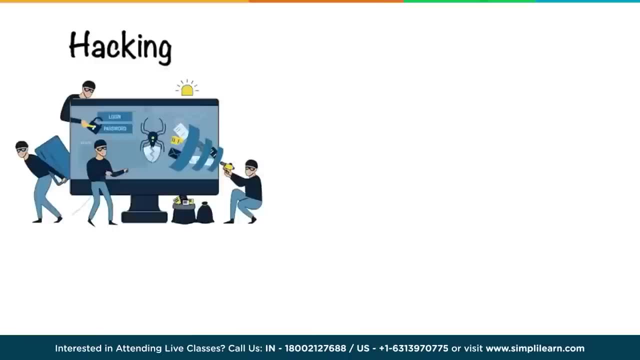 and their components from unauthorized digital attacks. These illegal attacks are often referred to as hacking. Hacking refers to exploiting weaknesses in a computer network to obtain unauthorized access to information. A hacker is a person who tries to hack into computer systems. This is a misconception that hacking is always wrong. 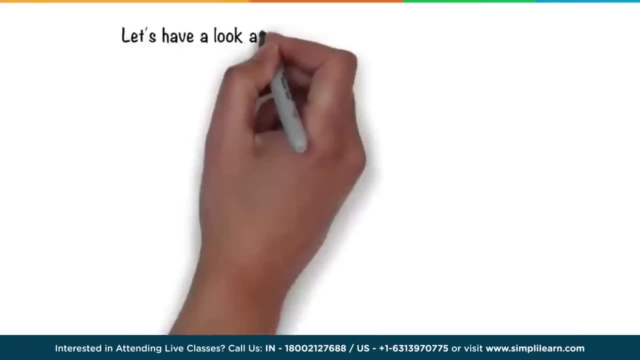 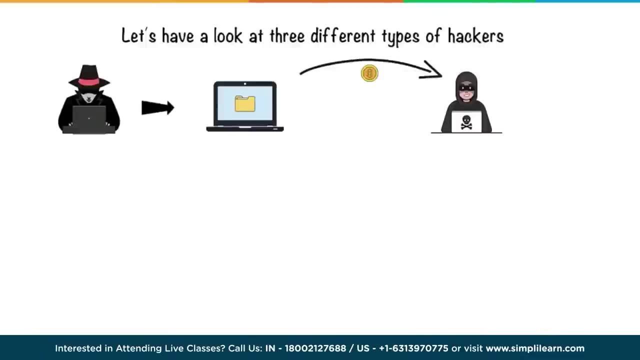 There are hackers who work with different motives. Let's have a look at three different types of hackers. Black hat hackers are individuals who illegally hack into a system for monetary gain. On the contrary, we have white hat hackers who exploit the vulnerabilities in a system. 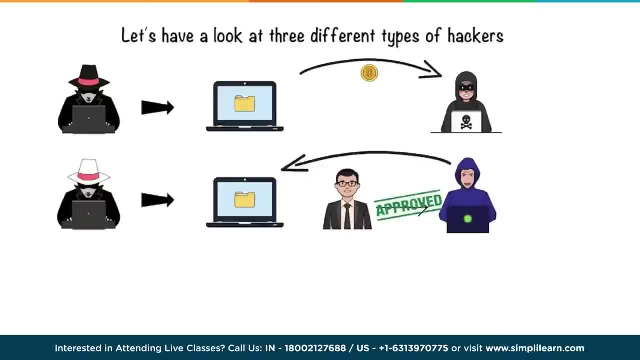 by hacking into it with permission in order to defend the organization. This form of hacking is absolutely legal and ethical. Hence they are also often referred to as ethical hackers. In addition to these hackers, we also have the gray hat hackers. As the name suggests, the color gray is a blend of both white and black. 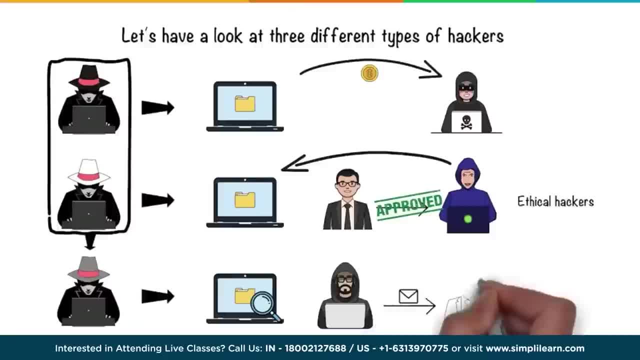 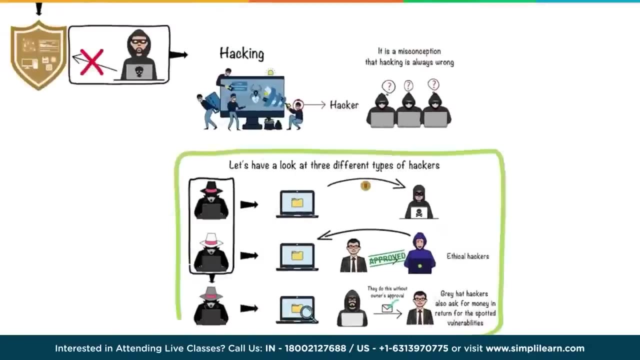 These hackers discover vulnerabilities in a system and report it to the system's owner, which is a good act, But they do this without seeking the owner's approval. Sometimes, gray hat hackers also ask for money in return for the spotted vulnerabilities. Now that you have seen the different types of hackers, 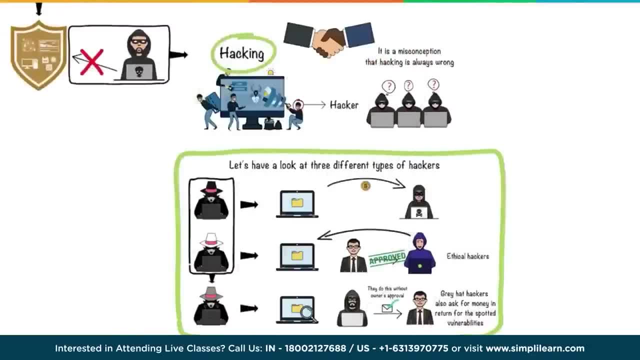 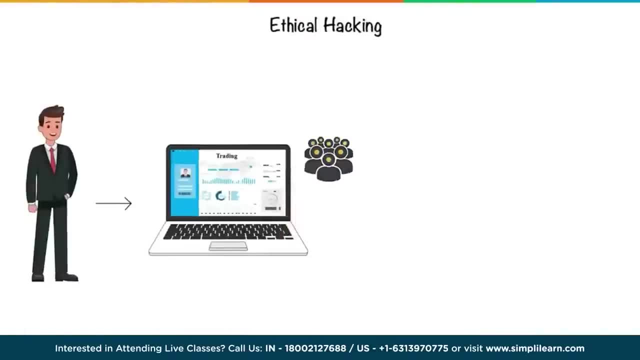 let's understand more about the hacking- that is, legal and valid, Ethical Hacking- Through an interesting story. Dan runs a trading company. He does online trading with the money his customers invest. Everything was going well and Dan's business was booming. 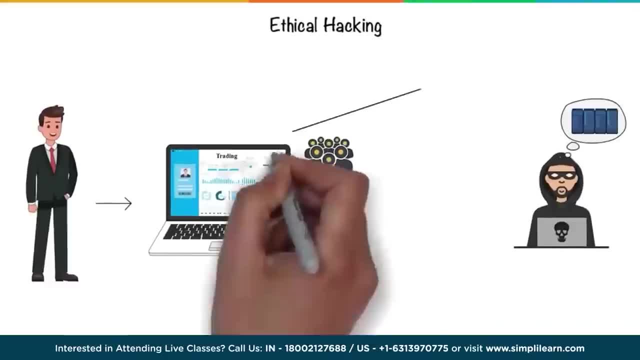 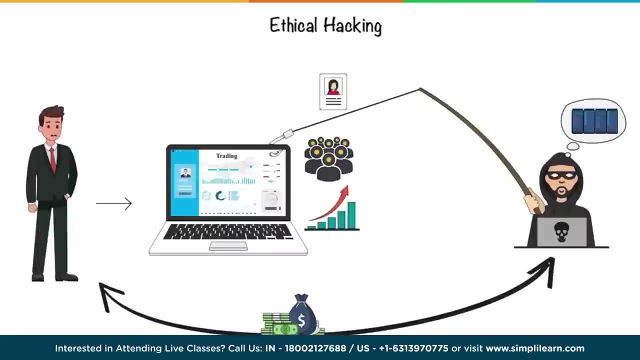 Until a hacker decided to hack the company's servers. The hacker stole the credentials of various trading accounts. He asked for a lump sum ransom in exchange for the stolen credentials. Dan took the hacker's words lightly and didn't pay the hacker. As a result, the hacker withdrew money from various customers' accounts. 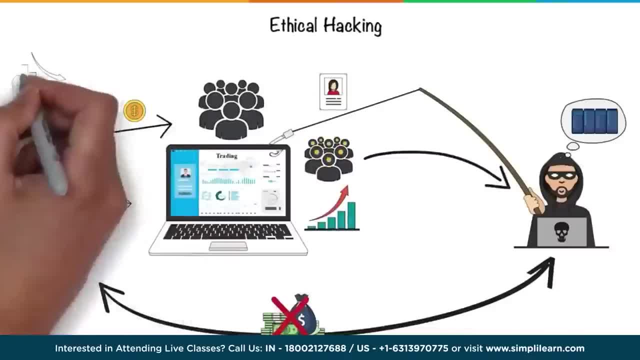 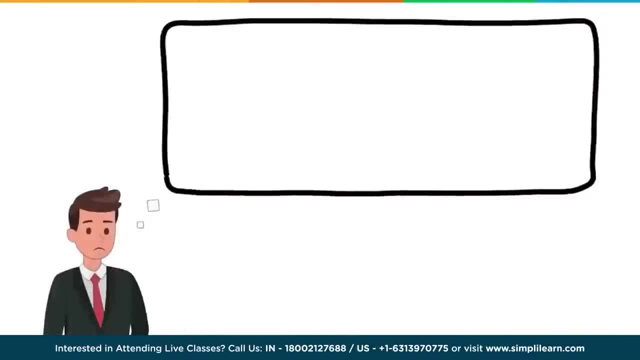 And Dan was liable to pay back the customers. Dan lost a lot of money and also the trust of his customers. After this incident, Dan gave a lot of thought as to what could have gone wrong with the security infrastructure in his company. He wished there was someone from his company who could have run a test attack. 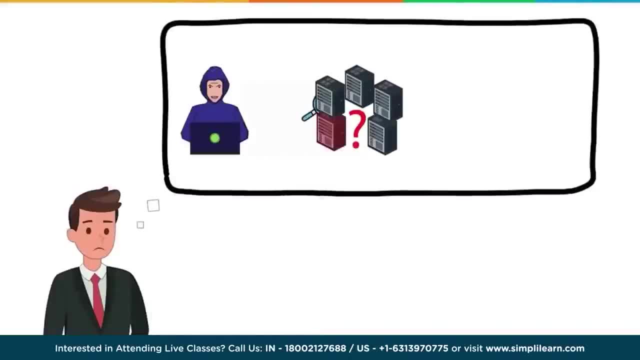 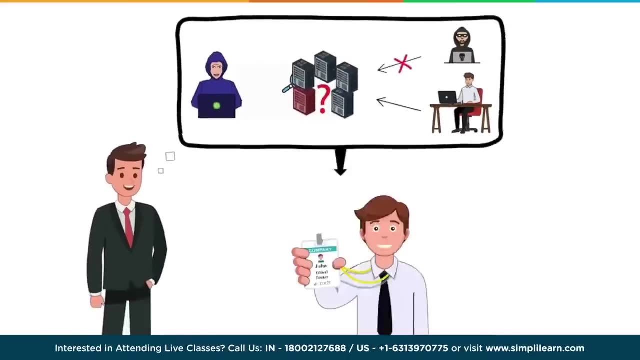 to see how vulnerable his systems were before the hacker penetrated into the network. This was when he realized he needed an employee who thinks like a hacker and identifies the vulnerabilities in his network Before an outsider does. To do this job, he hired an ethical hacker, John. 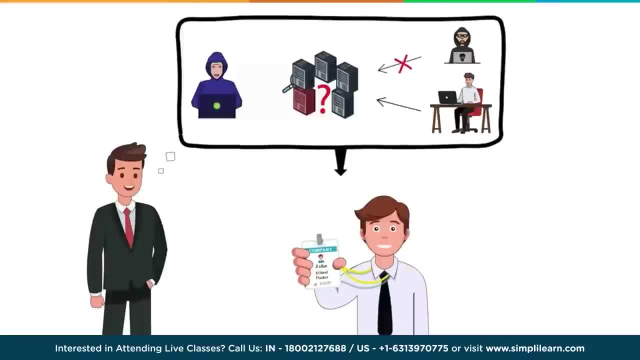 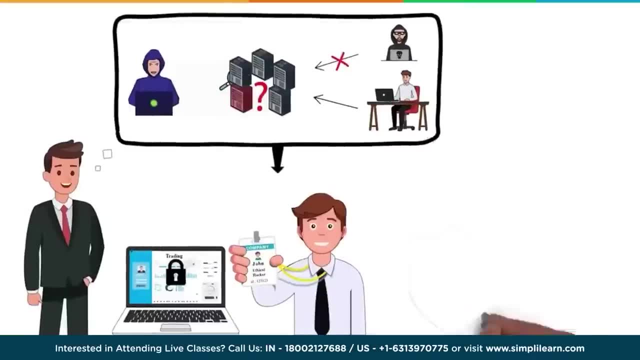 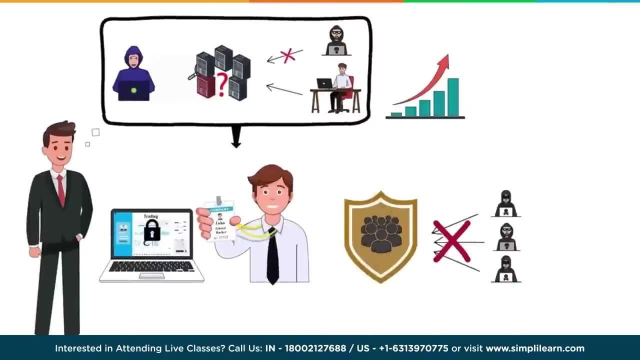 John was a skilled professional who worked precisely like a hacker. In no time he spotted several vulnerabilities in Dan's organization and closed all the loopholes. Hiring an ethical hacker helped Dan protect his customers from further attacks in the future. This, in turn, increased the company's productivity and guarded the company's reputation. 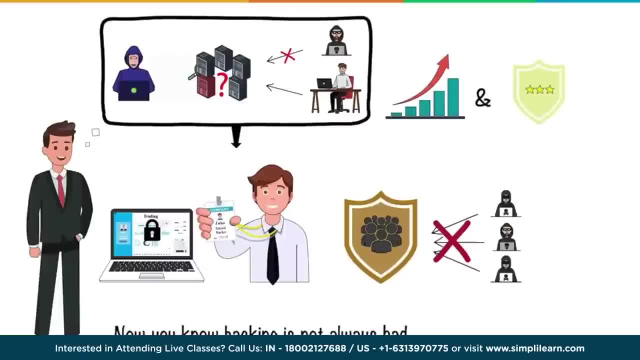 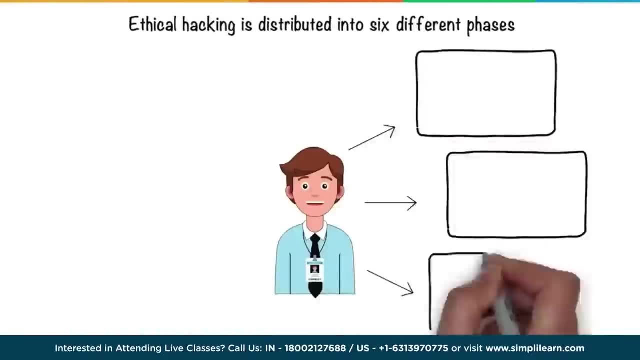 So now you know hackers. Hacking is not always bad. John, in this scenario, exposed the vulnerabilities in the existing network, and such hacking is known as ethical hacking. Ethical hacking is distributed into six different phases. Let us look at these phases step by step with respect to how John, our ethical hacker, will act. 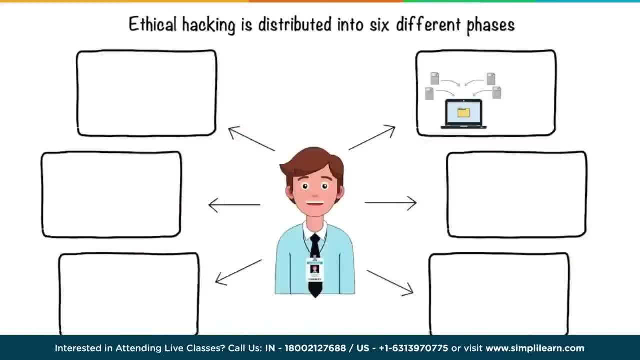 Before launching an attack, the first step John takes is to gather all the necessary information about the organization's system that he intends to attack. This step is called reconnaissance. He uses tools like Nmap and Hping for this purpose. John then tries to spot the vulnerabilities, if any. 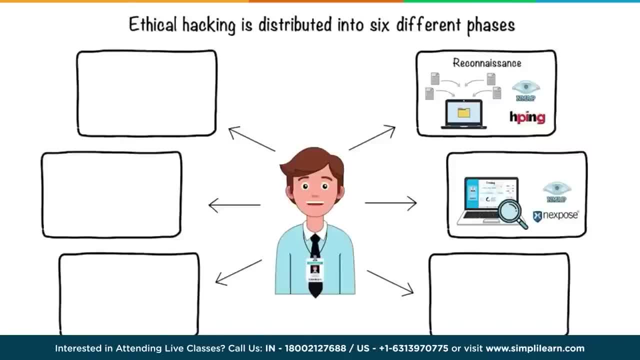 in the target system using tools like Nmap and Expose. This is the scanning phase. Now that he has located the vulnerabilities, he then tries to exploit them. This step is known as gaining access, After John makes his way through the organization's networks. 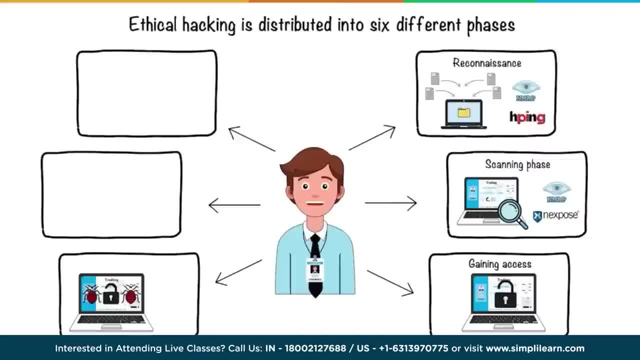 he tries to maintain his access for future attacks by installing back doors in the target system. The Metasploit tool helps him with this. This phase is called maintaining access. John is a brilliant hacker, Hence he tries his best not to leave any evidence of his attack. 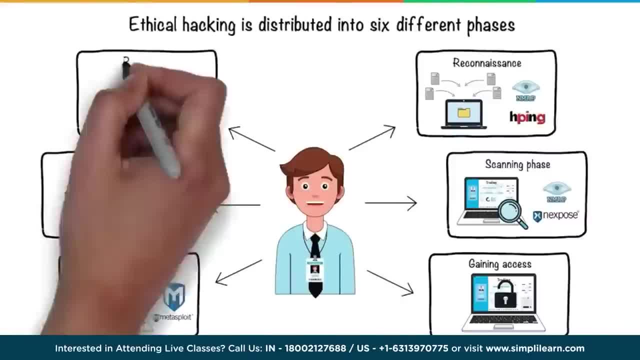 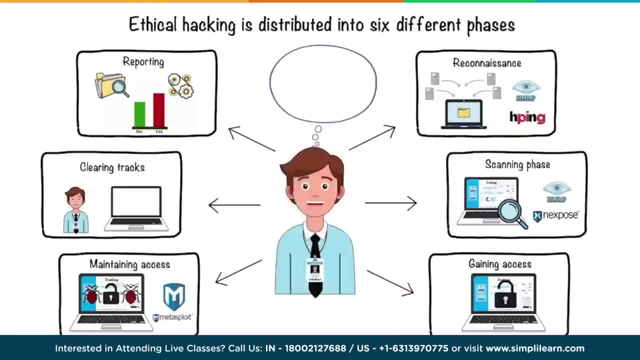 This is the fifth phase, clearing tracks. We now have the last phase that is reported. In this phase, John documents a summary of his entire attack, the vulnerabilities he spotted, the tools he used and the success rate of the attack. Looking into the report: 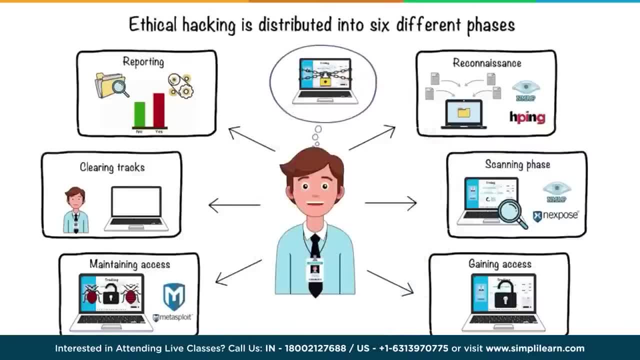 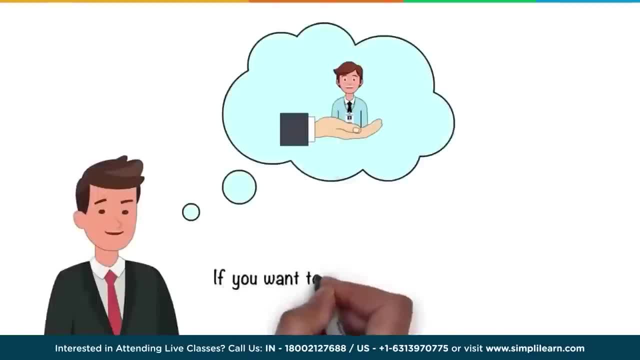 Dan is now able to take a call and see how to protect his organization from any external cyber attacks. Don't you all think John is an asset to any organization? If you want to become an ethical hacker like John, then there are a few skills that you need to acquire. 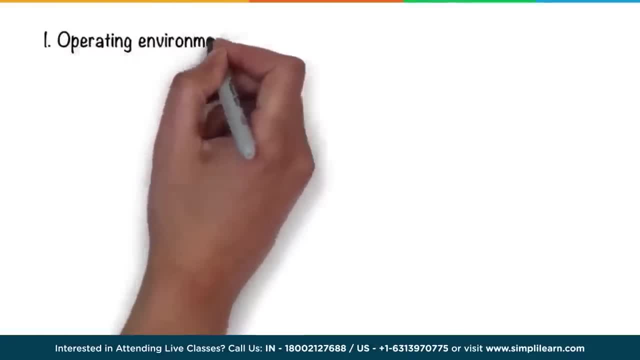 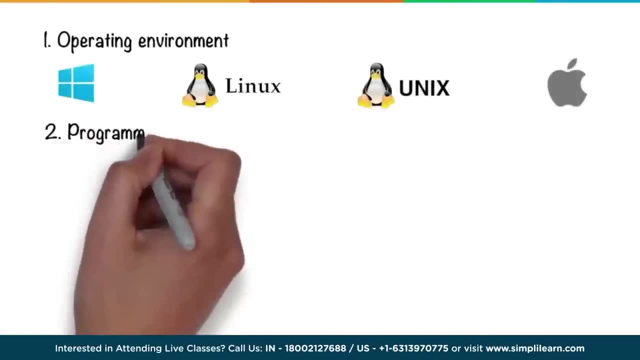 First and foremost, you need to have a good knowledge of operating environments such as Windows, Linux, Unix and Macintosh. You must have reasonably good knowledge of programming language languages such as HTML, PHP, Python, SQL and JavaScript. Networking is the base of ethical hacking. 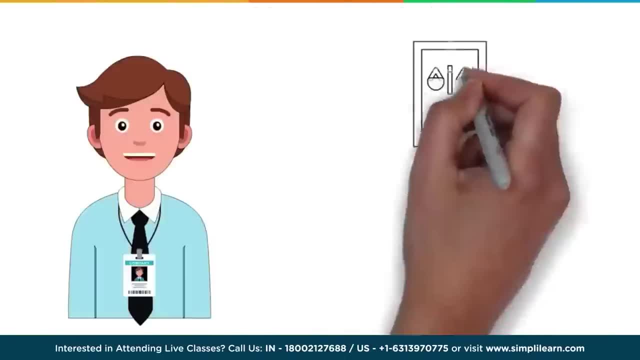 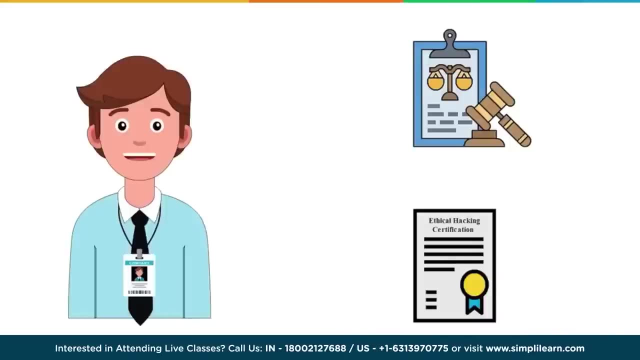 Hence you should be good at it. Ethical hackers should be well aware of security laws so that they don't misuse their skills. Finally, you must have a global certification on ethical hacking to successfully bag a position of an ethical hacker like John. 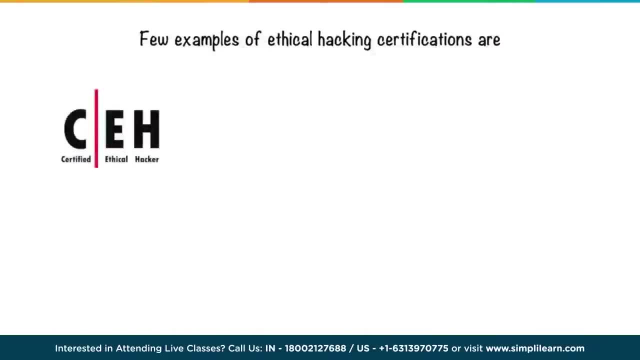 Few examples of ethical hacking certification are Certified Ethical Hacker Certification, CompTIA, PenTest Plus And Licensed Penetration Tester Certification, to name a few. SimplyLearn provides a cybersecurity expert master's program that will equip you with all the skills required by a cybersecurity expert. 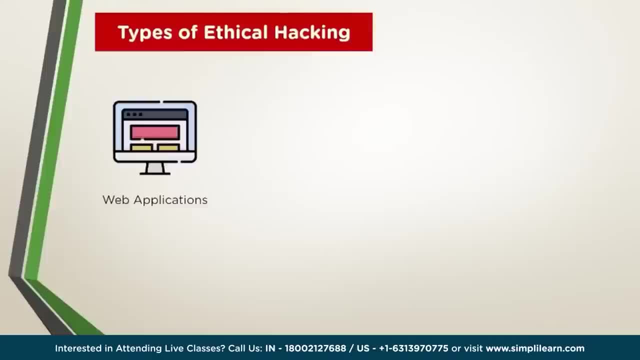 When it comes to web app hacking, it generally refers to the exploitation of applications by HTTP, which can be done by manipulating the applications via its graphical user interface. This is done by tampering with the uniform resource identifier, also known as a URI, or tampering with the HTTP elements. 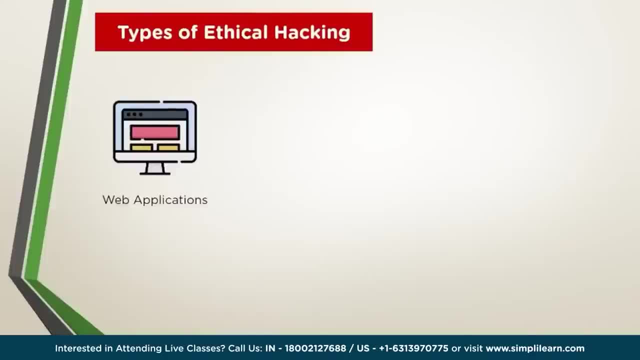 directly which are not a part of the URI. The hacker can send a link via an email or a chat and metric the users of a web application into executing actions. In case the attack is on an administrator account, the entire web application can be compromised. 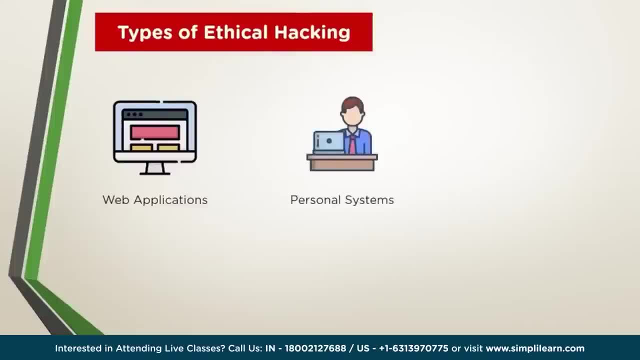 Anyone who uses a computer connected to the Internet is susceptible to the threats that computer hackers and online predators pose. These online villains typically use phishing scams, spam email or instant messages and bogus websites to deliver dangerous malware to your computer and compromise your computer security. Computer hackers can also try to access 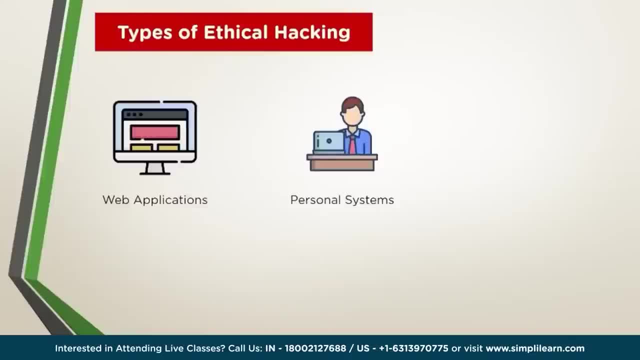 your computer and private information directly. if you're not protected by a firewall, They can monitor your conversations or peruse the back end of your personal website. Usually disguised with a bogus identity, predators can lure you into revealing sensitive personal and financial information. A web server, which can be referred to as the hardware, the computer or the software. 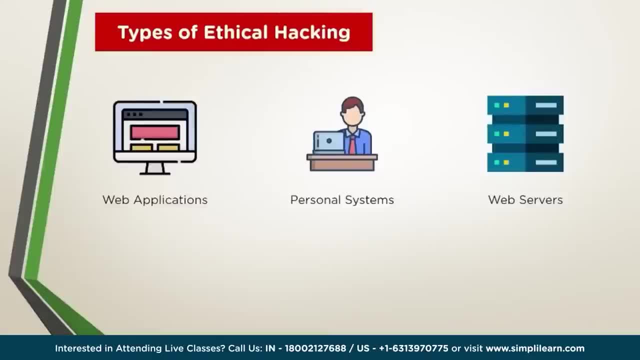 which helps to deliver content that can be accessed through the Internet. The primary function of a web server is to deliver these web pages on the request to clients using the hypertext transfer protocol or HTTP. So hackers attack the web server to steal credential information, passwords and. 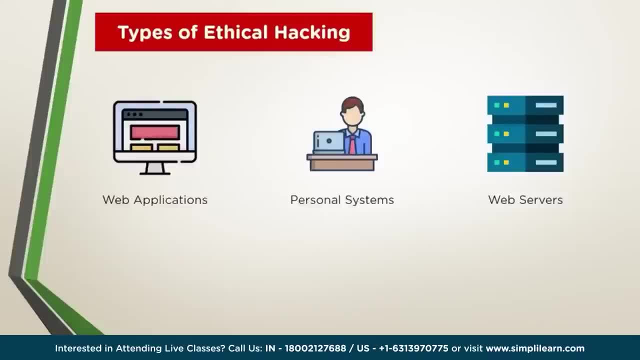 business information by using different types of attacks like DDoS attacks, SYN flooding, ping, flood port scan and social engineering attacks. In the area of web security, despite strong encryption on the browser server channel, web users still have no assurance about what happens at the other end. 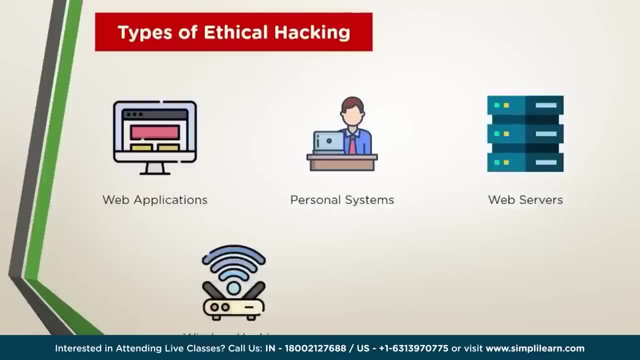 Although wireless networks offer great flexibility, they have their own security problems. A hacker can sniff the network packets without having to be in the same building where the network is located. As wireless networks communicate through radio waves, a hacker can easily sniff the network from a nearby network. 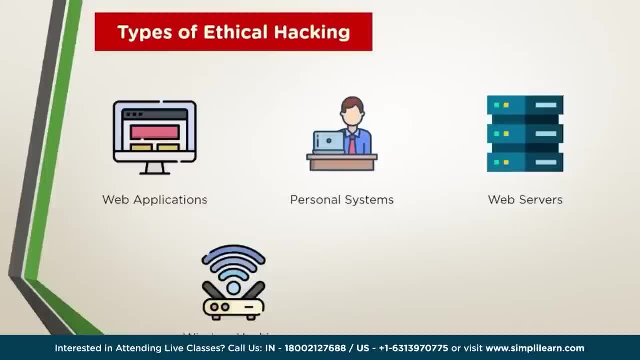 Most attackers use network sniffing to find the SSID and hack a wireless network. An attacker can attack a network from a distance and therefore it is sometimes difficult to collect evidence against the main hacker. Social engineering is the art of manipulating users of a computing system. 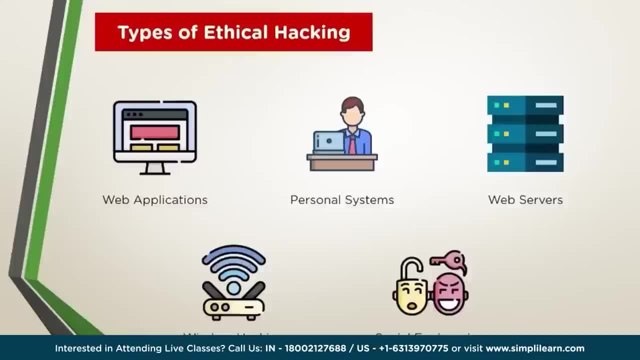 into revealing confidential information which can be later used to gain unauthorized access to a computer system. The term can also include activities such as exploiting human kindness, greed and curiosity to gain access to restricted access buildings or getting the users to installing backdoor software. 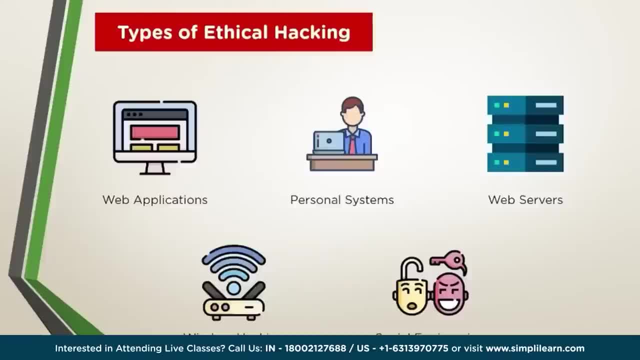 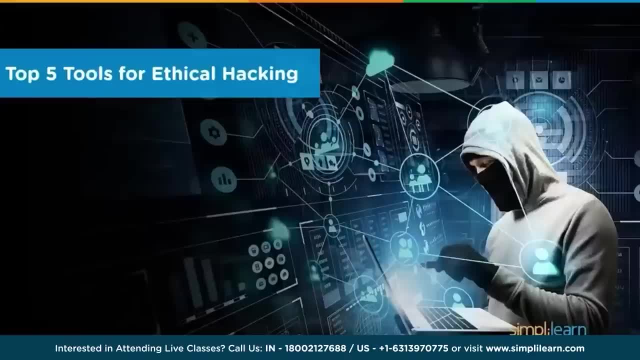 Knowing the tricks used by hackers to trick users into releasing vital login information is fundamental in protecting computer systems. Coming to our main focus for today, let us have a look at the top five most essential ethical hacking tools to be used in 2021. 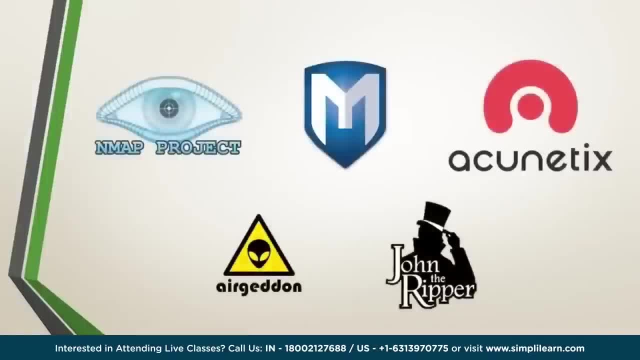 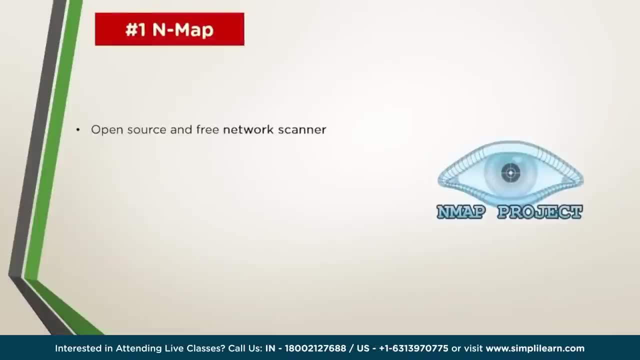 At the top of the chain lies Nmap. Nmap, which stands for network mapper, is a free and open source utility for network discovery and security auditing. Many systems and network administrators also find it useful for tasks such as network inventory, managing service upgrade. 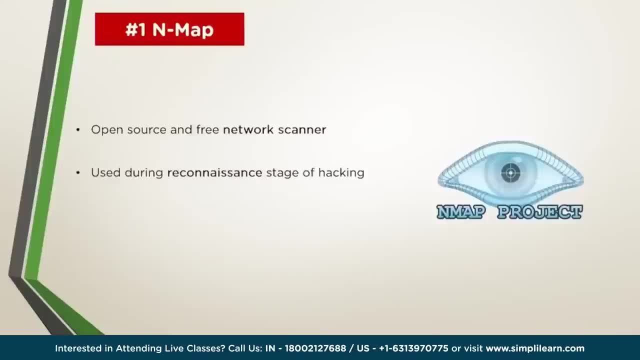 schedules and monitoring host or service uptime. It is most beneficial in the early stages of ethical hacking, where a hacker must figure the possible entry point to a system before running the necessary exploits, thus allowing the hackers to leverage any insecure openings and thus breach the device. 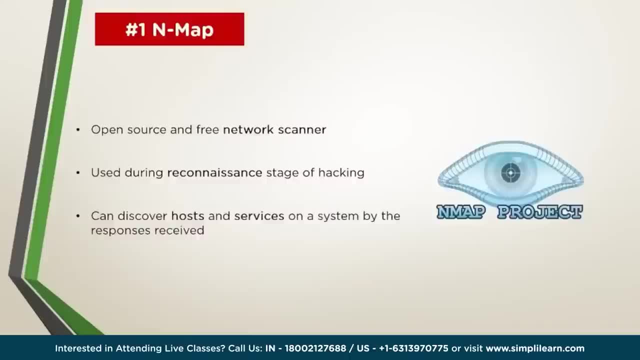 Nmap uses raw IP packets in novel ways to determine what hosts are available on the network, what service they are running, what operating systems are installed, what type of packet filters and firewalls are in use, and dozens of other characteristics. It was designed to rapidly scan large networks, but works fine against single. 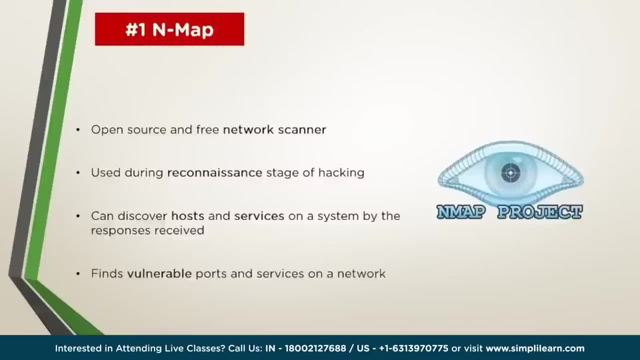 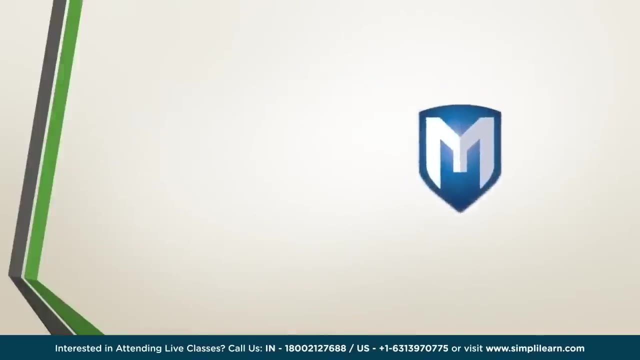 hosts as well, Since every application that connects to a network needs to do so via a port. the wrong port or a server configuration can open a can of worms, which lead to a thorough breach of the system and, ultimately, a fully hacked device. Next on our list, we have Metasploit. 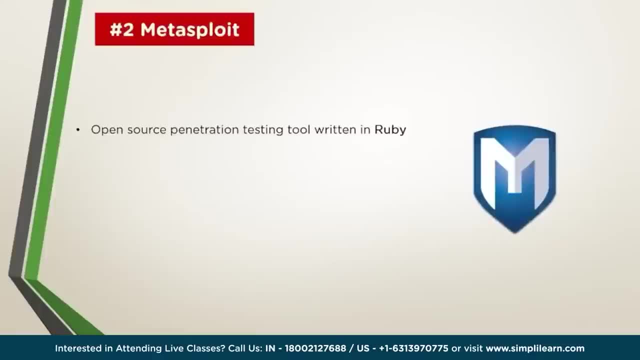 The Metasploit framework is a very powerful tool that can be used by cyber criminals as well as ethical hackers to probe systematic vulnerabilities on both networks and servers. Because it's an open source framework, it can be easily customized and used with most operating systems. 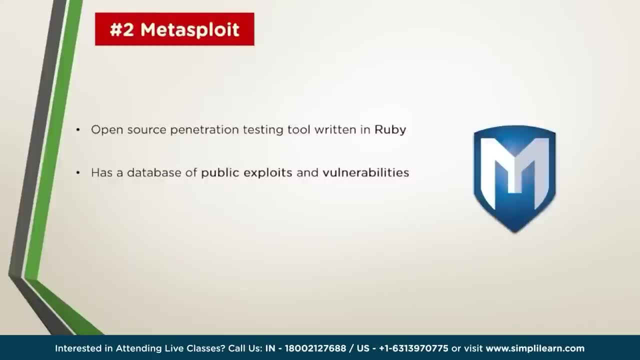 With Metasploit, the ethical hacking team can use readymade or custom code and introduce it into a network to probe for weak spots As another flavor of threat hunting. once the flaws are identified and documented, the information can be used to address systemic weaknesses and prioritize solutions. 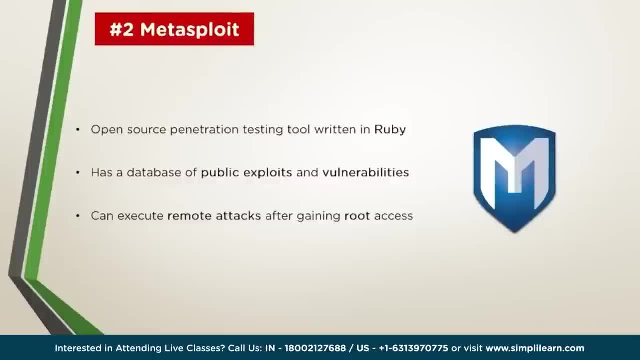 Once a particular vulnerability is identified and the necessary exploit is fed into the system, there are a host of options for the hacker. Depending on the vulnerability, hackers can even run root commands from the terminal, allowing complete control over the activities of the compromised system. 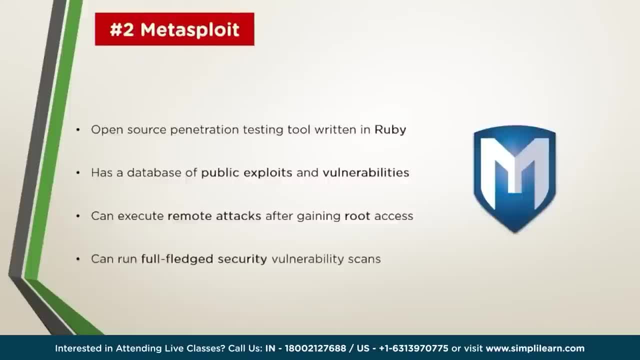 as well as all the personal data stored on the device. A big advantage of Metasploit is the ability to run full fledged scans on the target system, which gives a detailed picture of the security index of the system, along with the necessary exploits that can be used to bypass the antivirus software. 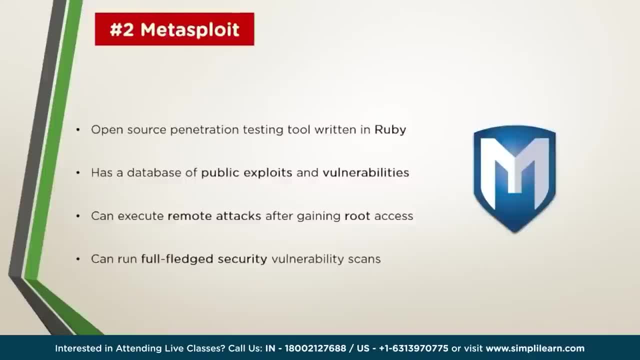 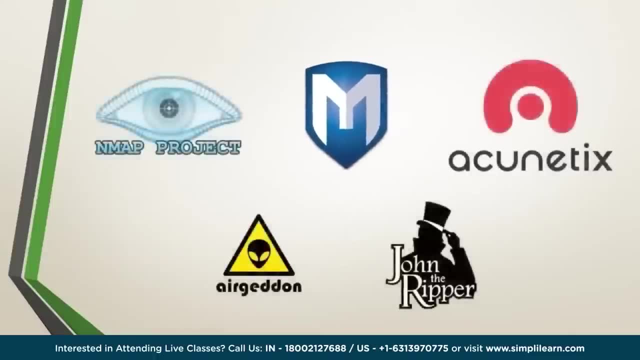 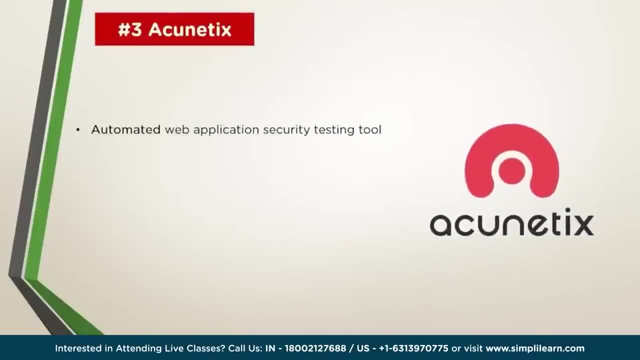 Having a single solution to gather almost all the necessary points of attack is very useful for ethical hackers and penetration testers, as denoted by its high rank in the list. Moving on, we have the Acunetix framework. Acunetix is an end-to-end web security scanner. 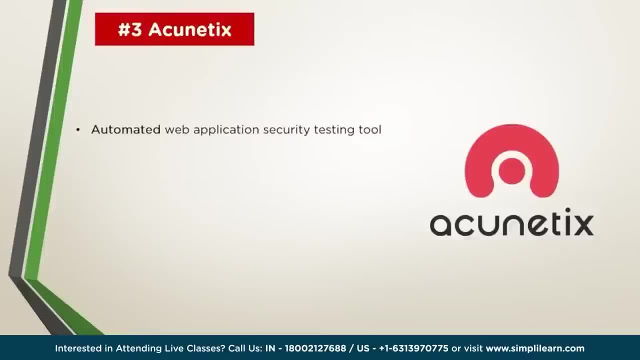 which offers a 360 degree view of an organization's security. It is an application security testing tool that helps the company address vulnerability across all their critical web assets. The need to be able to test applications in depth and further than traditional vulnerability management tools has created a market with several players in the application security space. 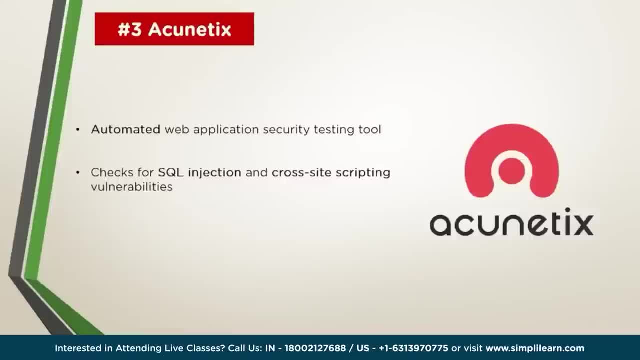 Acunetix can detect over 7000 vulnerabilities, including SQL injections, cross-site scripting, misconfigurations, weak passwords, exposed database and other out-of-band vulnerabilities. It can scan all pages, web apps and complex web applications running HTML5 and JavaScript as well. 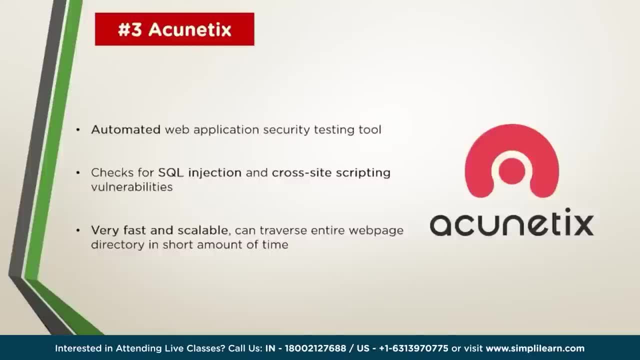 It also lets you scan complex multilevel forms and even password protected areas of the site. Acunetix is a dynamic application security testing package which has definite perks over status application security testing frameworks, which are also known as SAST scanners. 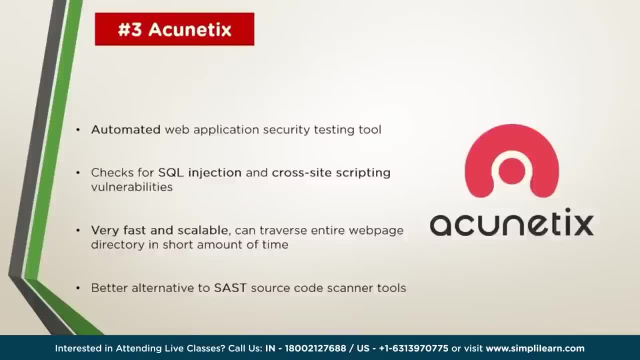 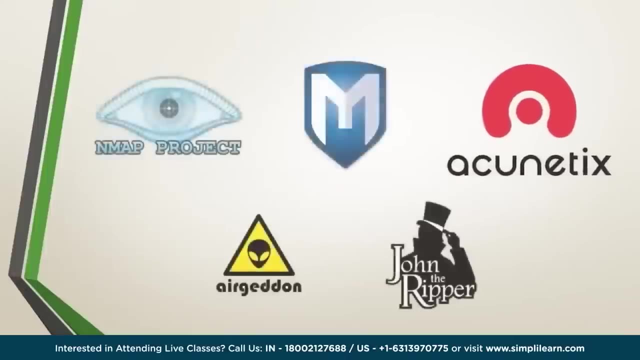 SAST tools only work during development and only for specific languages and have a history of reporting a lot of false positives, whereas dynamic testing tools, also known as DAST, have the ability to streamline testing from development to deployment with minimal issues. Next on our list, we have Ergeddon. 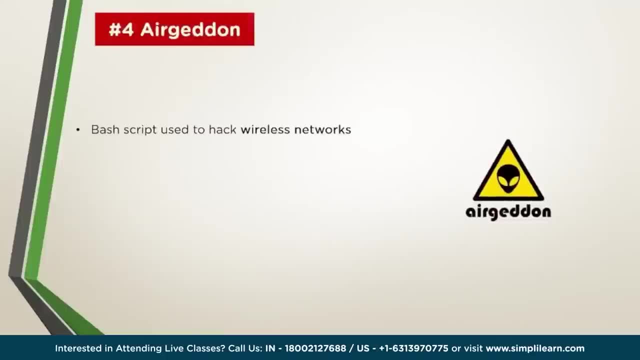 This is a multi-use bash script used for Linux systems to hack and audit wireless networks like our everyday Wi-Fi router and its counterparts. Along with being able to launch denial of service attacks on compromised networks, this multipurpose Wi-Fi hacking tool has very rich features which support multiple methods for Wi-Fi hacking. 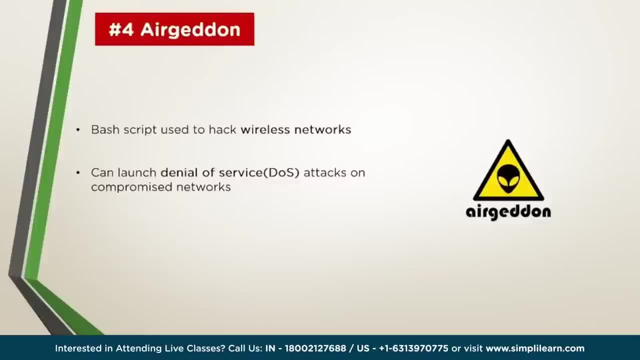 including WPS hacking modes, WP attacks, handshake captures, evil twin and so much more. It usually needs an external network adapter that supports monitor mode, which is necessary to be able to capture wireless traffic that traverse the air channels. Thanks to its open source nature, Ergeddon can be used with multiple community. 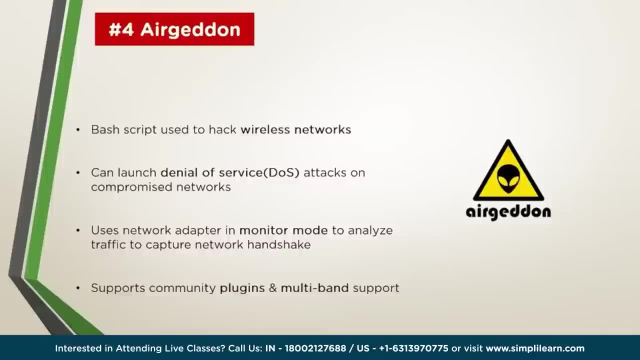 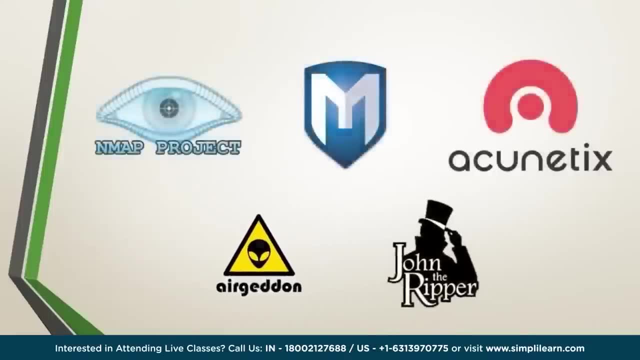 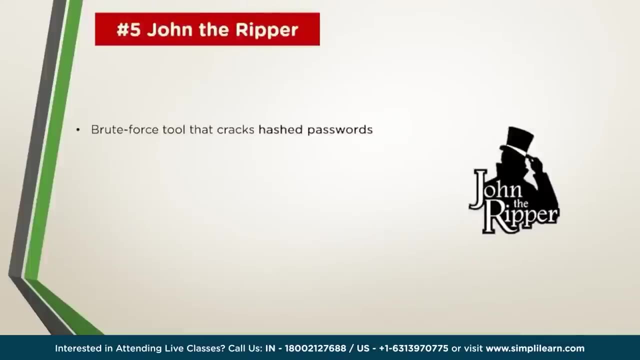 plugins and add-ons, thereby increasing its effectiveness against a wide variety of routers, both in the 2.4 GHz and the 5 GHz. Finally, at number five, we have John the Ripper. John the Ripper is an open source password, security, auditing and the password. 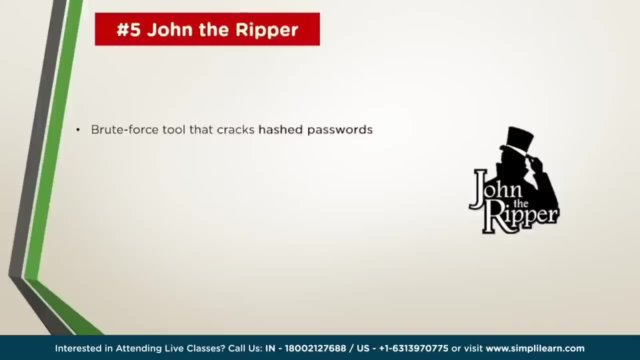 recovery tool which is available for many operating systems. John the Ripper Jumbo supports hundreds of hash and cipher types, including for user passwords of operating systems, web apps, database servers, encrypted keys and document files. Some of the key features of the tool include offering multiple modes to speed. 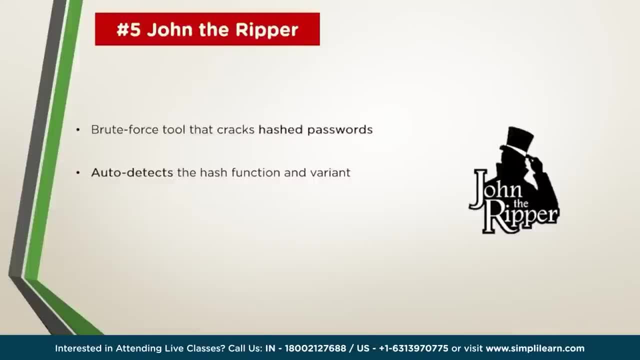 up the password cracking automatically, deselecting the hashing algorithm used by the passwords and the ease of running and configuring the tool to make it password cracking easier. It can use dictionary attacks, along with regular brute forcing, to speed up the process of cracking the correct password without wasting additional resources. 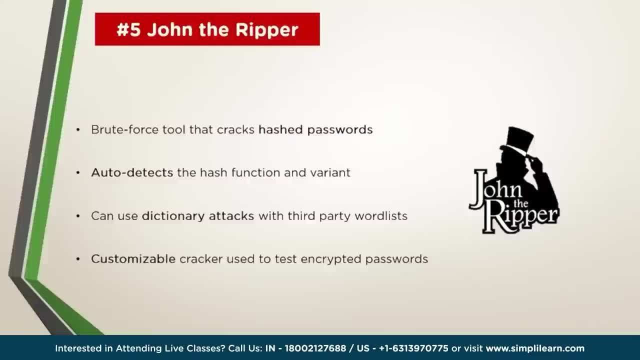 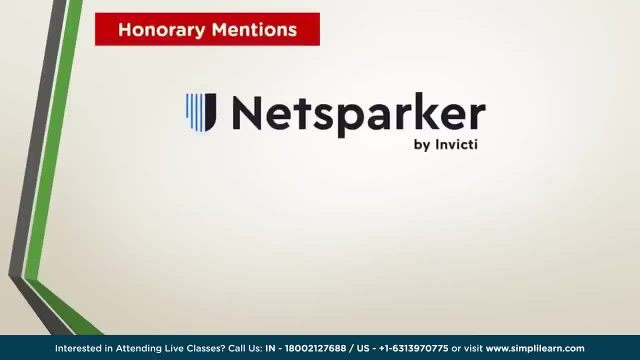 The word list being used in these dictionary attacks can be used by the users and allowing for a completely customizable process. We also have a few honorary mentions in our list that just missed the cut. NetSparker, for instance, is an automated yet fully configurable web. 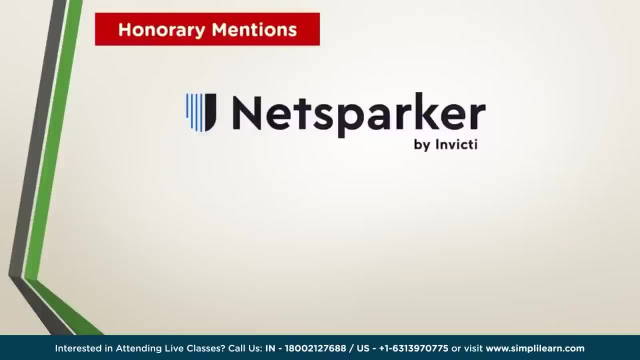 application security scanner that enables you to scan websites, web applications and web services. The scanning technology is designed to help you secure web applications easily, without any fuss, so you can focus on fixing the reported vulnerabilities. The Burp Suite Professional is one of the most popular penetration testing and vulnerability finder tools. 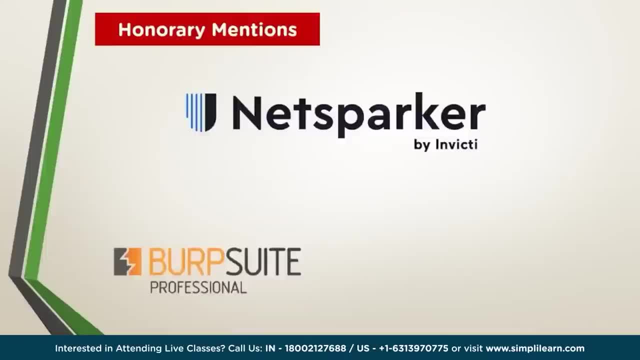 and is used for checking web application security. The term Burp, as it is commonly known, is a proxy based tool which is used to evaluate the security of a web based application and to do hands on testing Moving away from websites and applications. 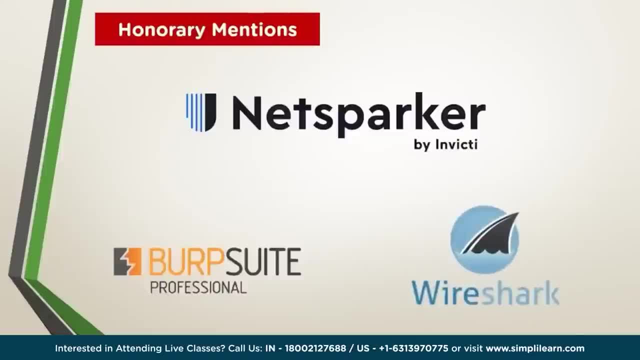 Wireshark is a free and open source packet analyzer which was launched in 2006.. It is used for network troubleshooting, analysis, software and communications protocol development and education. It captures network traffic on the local network and stores data for offline analysis. 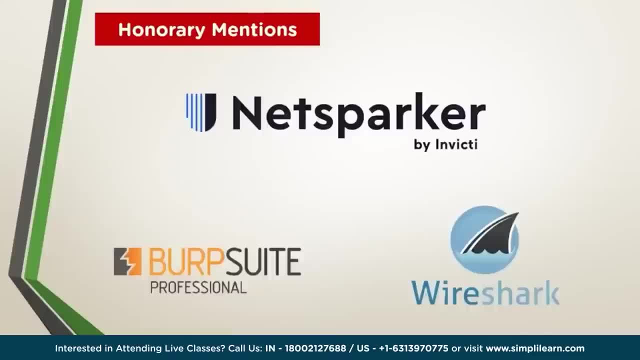 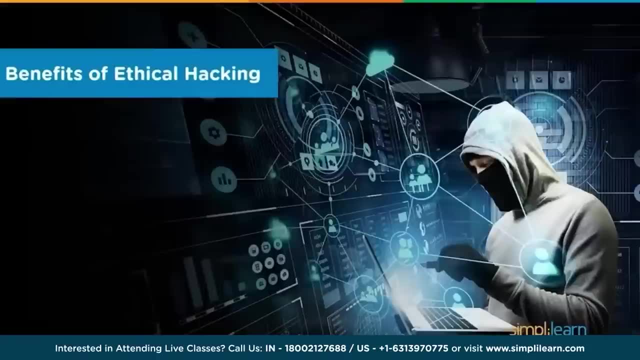 Wireshark captures network traffic from Ethernet, Bluetooth, wireless networks and frame relay connections. Now that we learn about the different types of tools that can be used when conducting an ethical hacking audit, let's learn about some potential benefits of such campaigns and why organizations 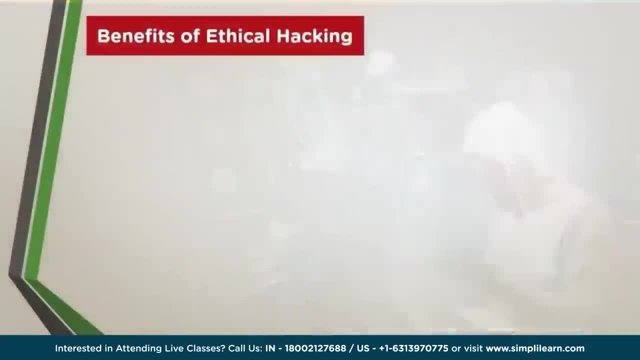 prefer to pay for such audits. Being able to identify defects from an attacker's perspective is game changing, since it displays all the potential avenues of a possible hack. One can only prepare for the known vulnerabilities as a defensive specialist, but proactively trying to breach a network. 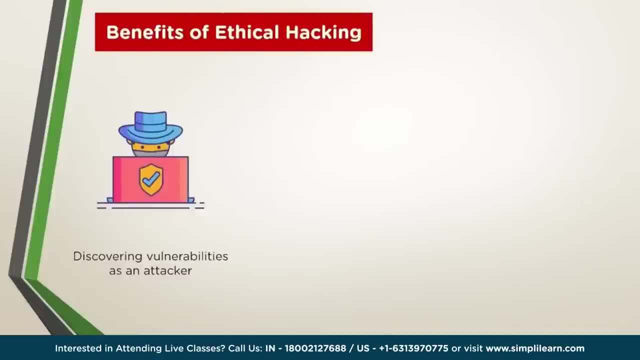 or device can make hackers think of techniques that no defense contractors can account for. This kind of unpredictability goes a long way in securing a network against malicious actors. Another advantage of hiring ethical hackers is the ability to preemptively fix possible weak points in a company's network infrastructure. 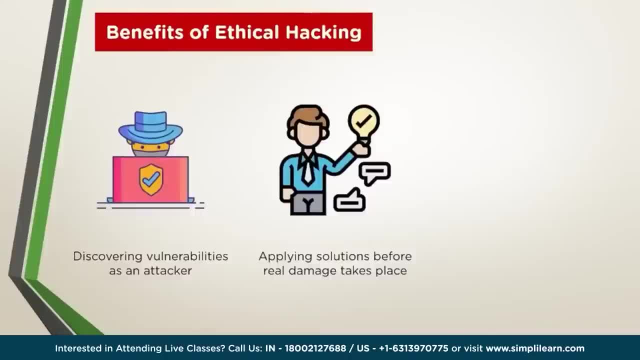 As seen on many occasions, a real breach will cause loss of data and irreparable damage to the foundation of an organization. Being able to gauge such shortcomings before they become public and can be used exploited is a benefit most organizations make use of. This is not to imply that such security 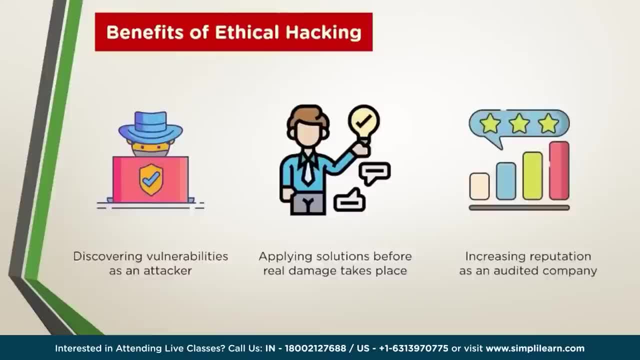 audits are only beneficial to the organization paying for it. When coming across companies that provide certain services, a reliable third party security audit goes a long way in instilling trust and confidence over their craft. If the ethical hackers cannot find any major vulnerabilities that can be leveraged by hackers, it just accentuates the technical 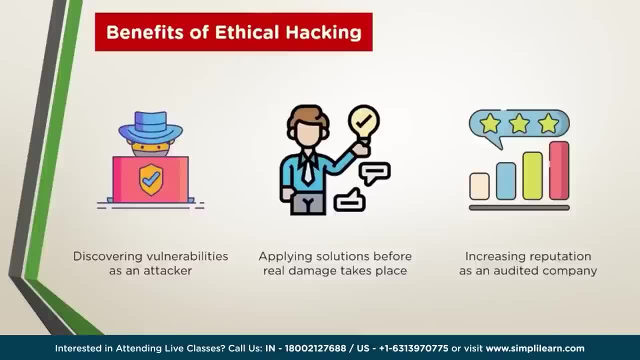 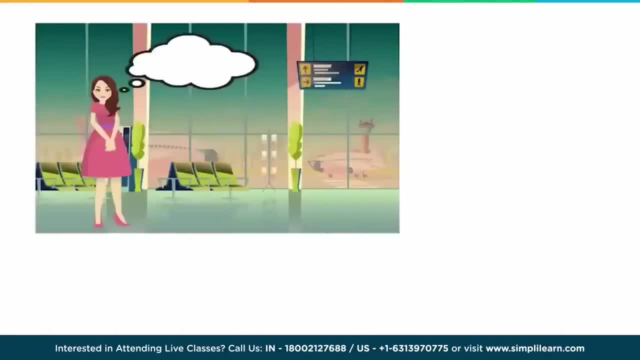 brilliance of the organization and its engineers, thereby increasing the clientele by a substantial amount. Jude is waiting at the airport to hop on her flight back home. when she realizes that she missed making an important bank payment, She connects her laptop to the public Wi-Fi at the airport and goes ahead. 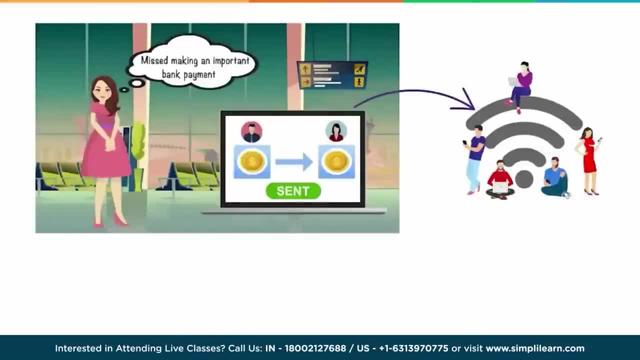 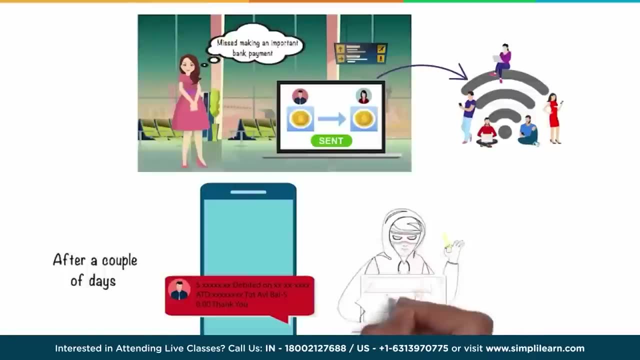 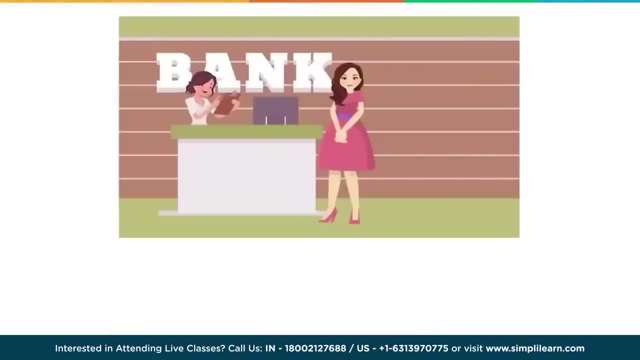 to carry out the bank transaction. Everything goes well and Jude completes her transaction. After a couple of days, she was wiped off her feet when she learned that her bank account was subjected to a cyber attack and a hefty amount was wiped from her account. After getting in touch with the bank authority, 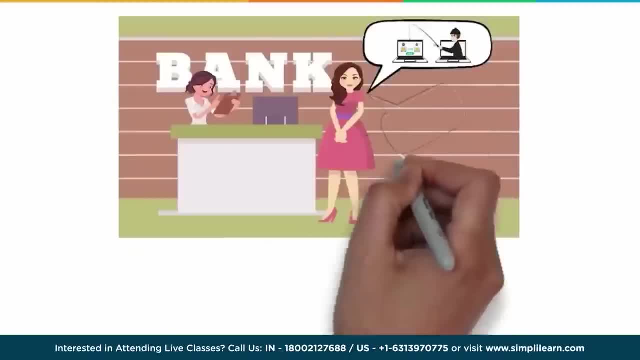 she learned that her account was hacked at the airport. She then realized that the public Wi-Fi she used might have caused her this trouble. Jude wishes that had her bank transfer escaped the hacker's eyes, She would not have been a victim of a cyber attack. 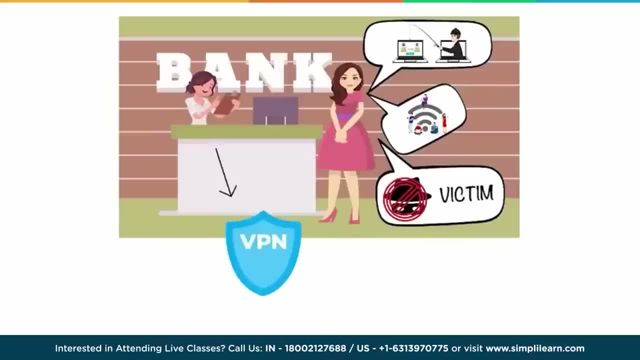 Bank officials advise her to use a VPN for future transactions, especially when connecting to an open or public network. Like most of us, Jude had come across the term VPN several times but didn't know much about it, and little did she think that the repercussions of not using a VPN 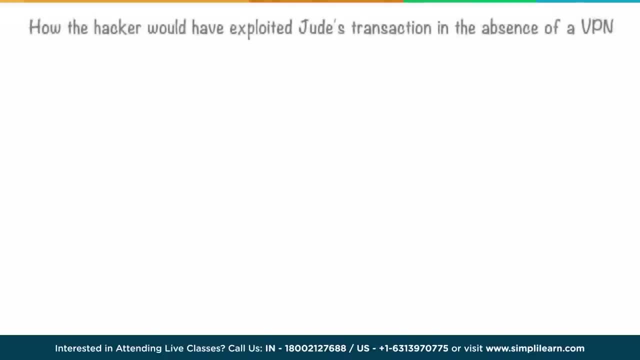 would be this bad. Let's understand how the hacker would have exploited Jude's transaction in the absence of a VPN. In this process, Jude's computer first connects to the Internet Service Provider, ISP, which provides access to the Internet. She sends her details to the bank's server using her IP address. 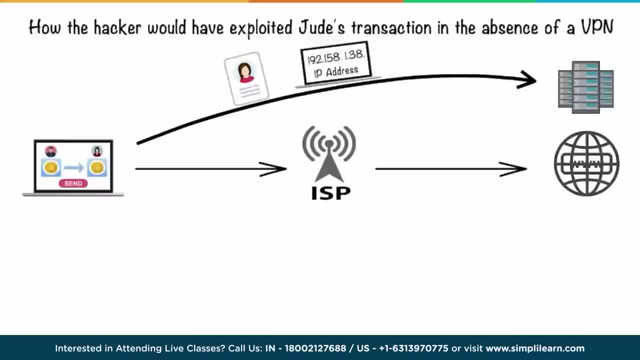 Internet Protocol Address, or IP address, is a unique address that recognizes a particular device, be it a laptop or a smartphone, on the Internet. When these details pass through the public network, the hacker, who passively watches the network traffic, intercepts it. 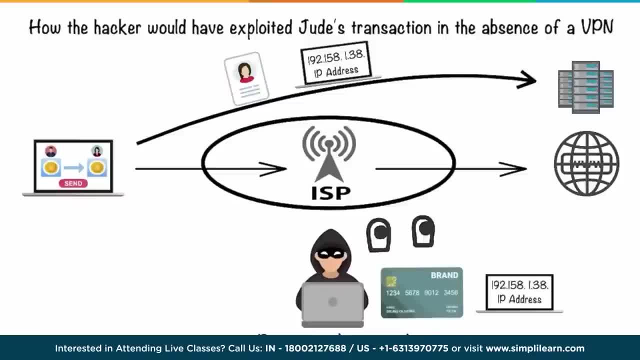 This is a passive cyber attack where the hacker collects Jude's bank details without being detected. More often or not, in such an attack, payment information is likely to be stolen. The targeted data here are the victim's username, passwords and other personal. 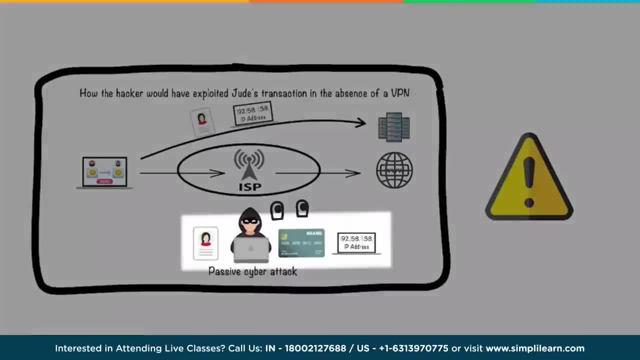 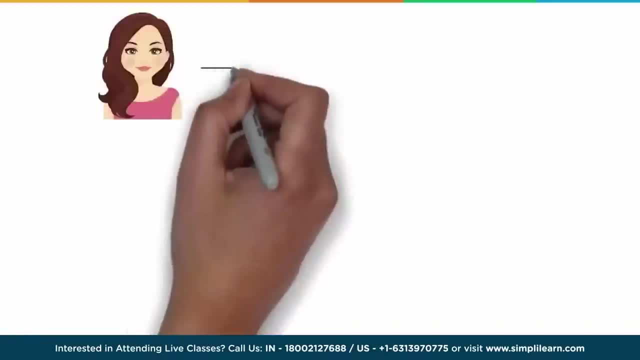 information. Such an unsecured connection exposed Jude's IP address and bank details to the hacker when it passed through the public network. So would Jude have been able to secure her transaction with the help of a VPN? Well, yes, Picture Jude's bank. 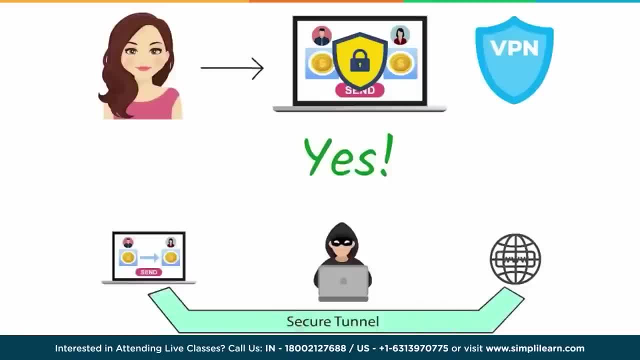 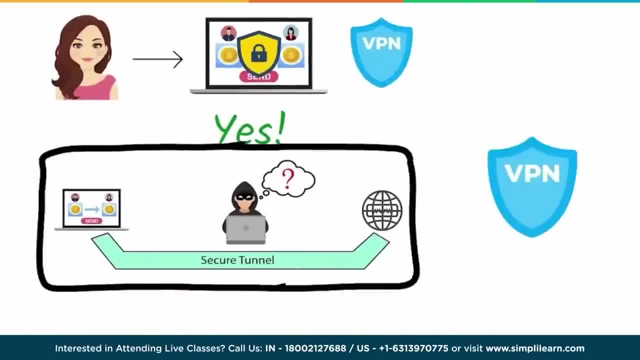 transaction to be happening in a tunnel that is invisible to the hacker. In such a case, the hacker will not be able to spot her transaction, And that is precisely what a VPN does. A virtual private network, more often known as VPN, creates a secure tunnel between your device and the Internet. 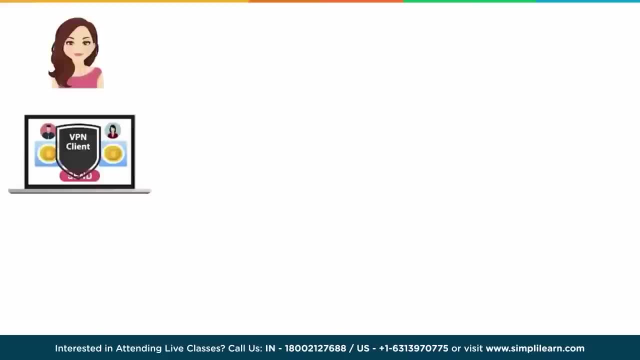 For using a VPN. Jude's first step would be to install software-based technology known as the VPN client on her laptop or smartphone. that would let her establish a secure connection. The VPN client connects to the Wi-Fi and then to the ISP. Here the VPN client encrypts Jude's information using VPN protocols. 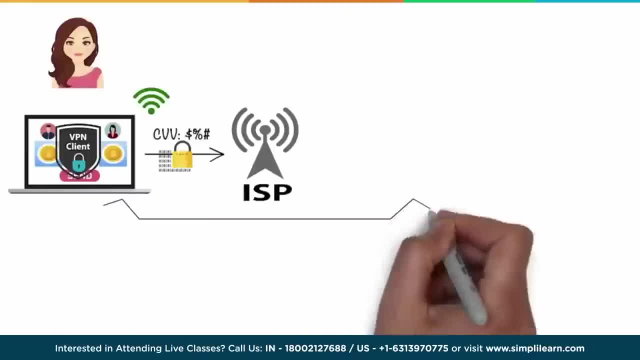 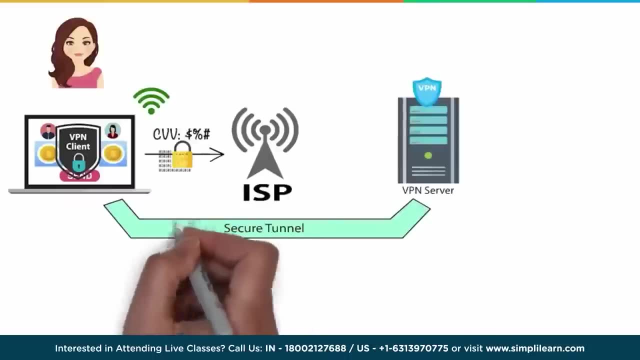 Data is encrypted to make sure it is secure. Next, the VPN client establishes a VPN tunnel within the public network that connects to the VPN server. The VPN tunnel protects Jude's information from being intercepted by the hacker. Jude's IP address and actual location are changed at the VPN server to enable 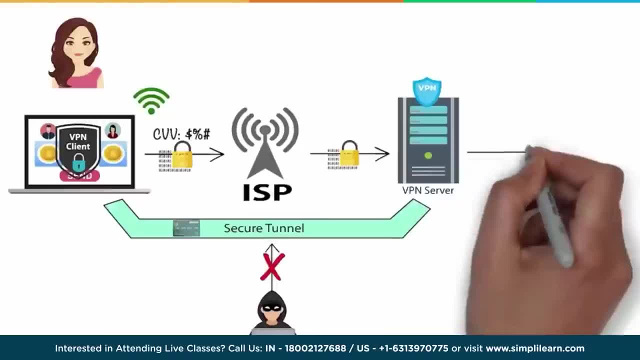 a private and secure connection. Finally, the VPN server connects to Jude's bank server in the last step, where the encrypted message is decrypted. This way, Jude's original IP address is hidden by the VPN and the VPN tunnel protects her data from being hacked. 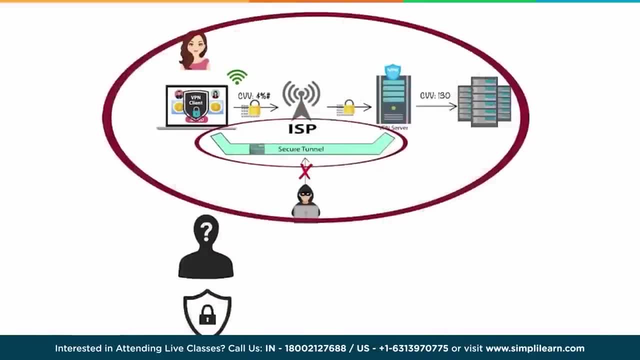 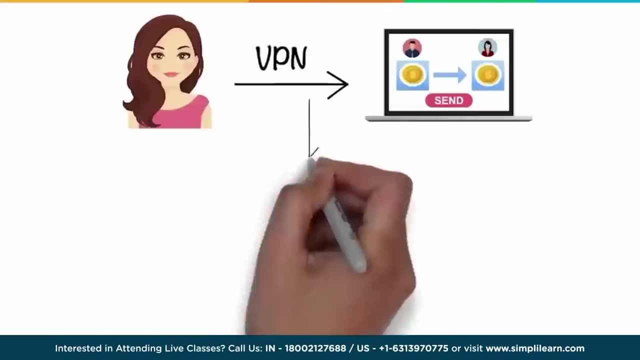 This explains how VPN makes your data anonymous and secure when it passes through the public network and the difference between a normal connection and a VPN connection. After learning about this, Jude was certain that she should start using a VPN to carry out her online transactions in the future. This is also applicable to each one of us. 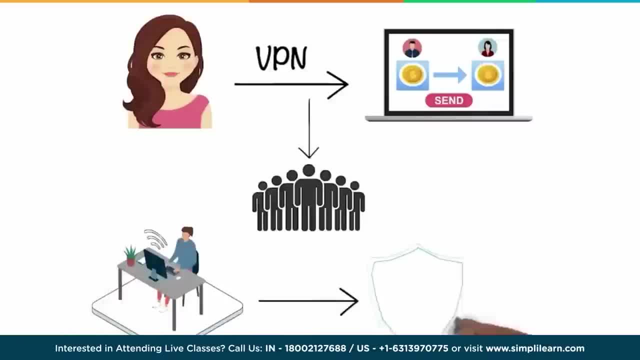 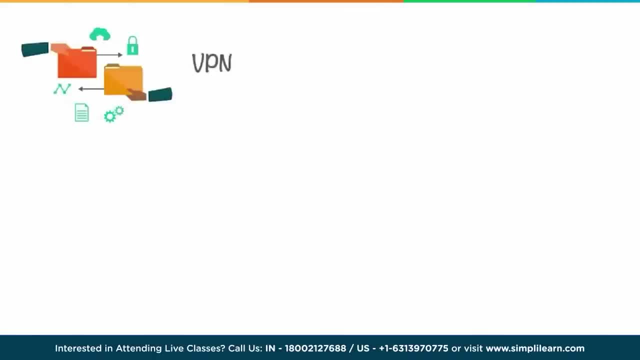 Even if you work remotely or connect to public Wi-Fi, using a VPN is the safest option. In addition to providing a secure, encrypted data transfer, VPNs are also used to disguise your whereabouts and give you access to regional web content. VPN servers act as proxies on the Internet. 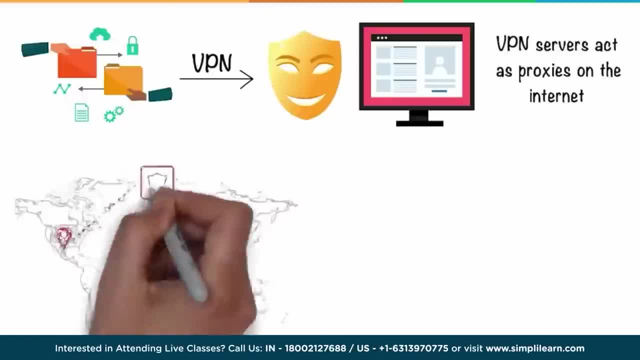 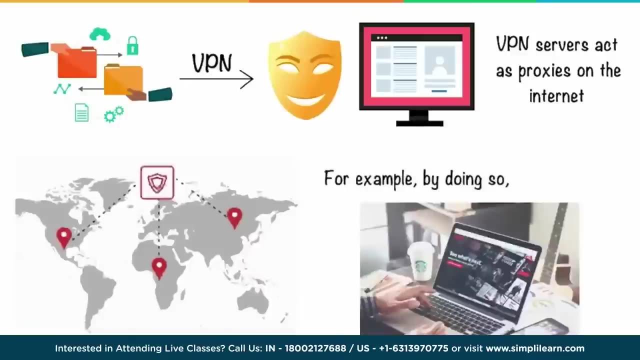 This way, your actual location cannot be established. VPN enables you to spoof your location and switch to a server to another country and thereby change your location. For example, by doing so, you can watch any content on Netflix that might be unavailable for your region. 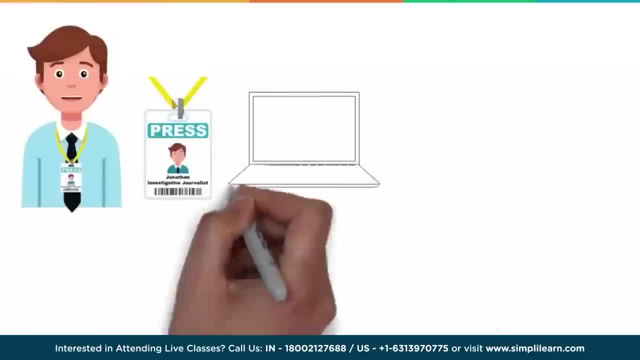 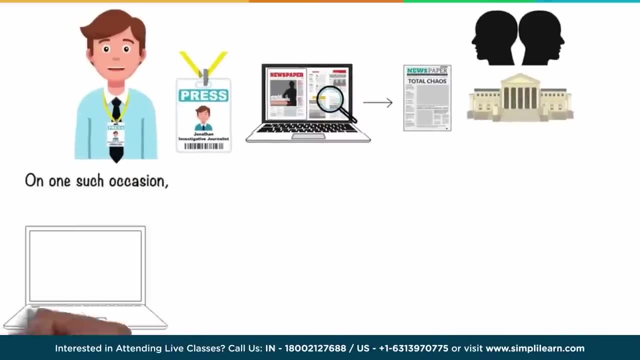 Meet Jonathan. He is an investigative journalist who occasionally researches and publishes news articles contrary to the government's ideologies. On one such occasion, he could not access a global news website dealing with uncensored information. It seemed his IP was blocked from visiting the news website. 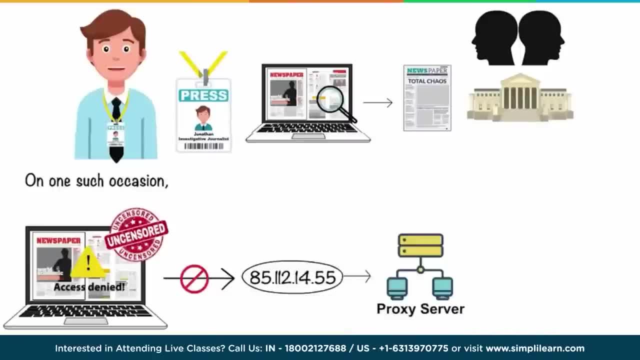 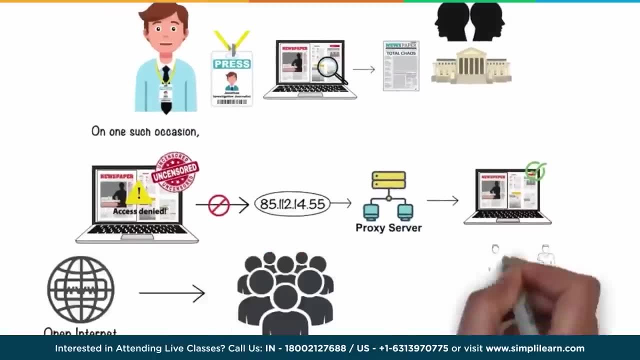 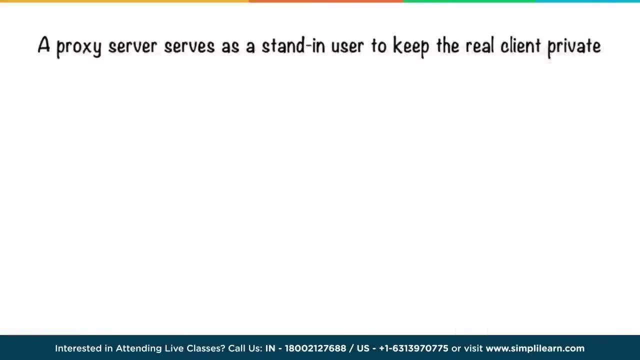 With his IP blocked, Jonathan turned to a popular proxy service that was able to unblock the news website, thereby allowing an open Internet to all users, Just like how your friend gives a proxy attendance for you. a proxy server serves as a stand in user to keep the real client private. 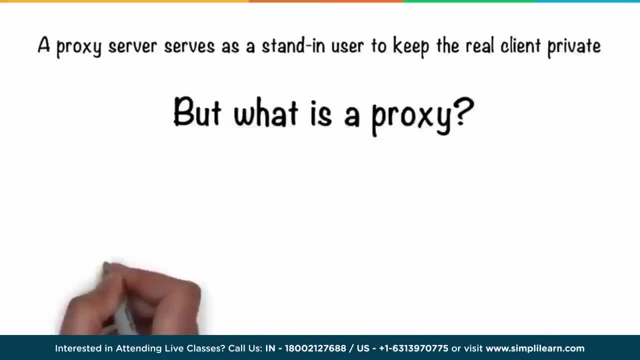 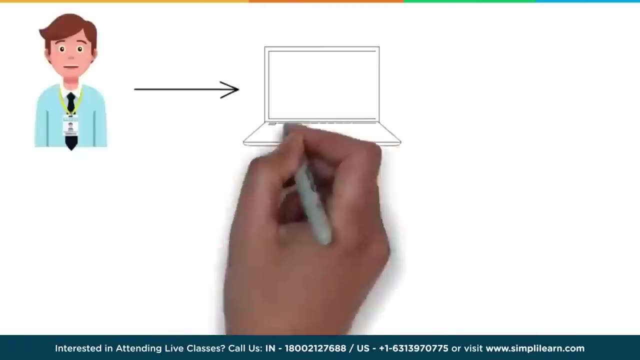 But what is a proxy? Let's understand it's working by taking a look at how Jonathan was able to access geo block content without much hassle. A proxy server acts as a gateway or intermediary server between a user and its destination website, When Jonathan wasn't able to access the news website. 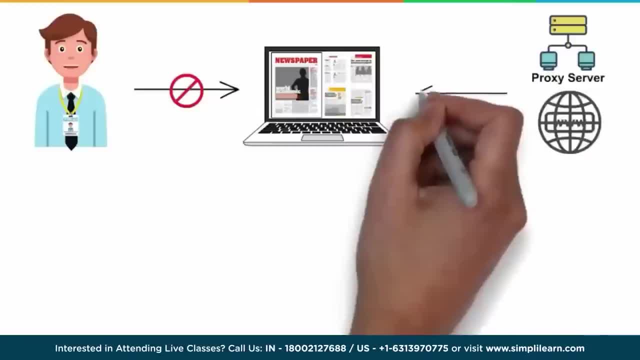 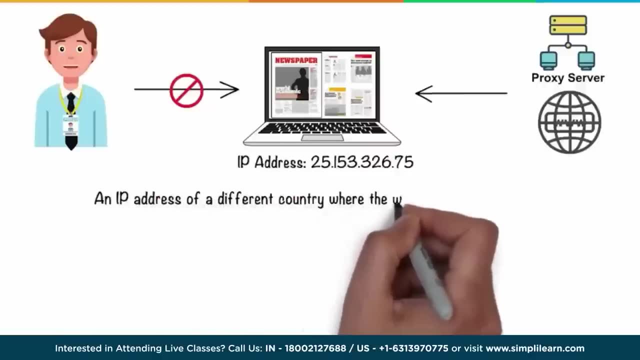 he connected his system to a global proxy server. Once connected, the proxy server assigns a new IP address to Jonathan's system, an IP address of a different country where the website is not censored, Following this process whenever Jonathan visits that website. 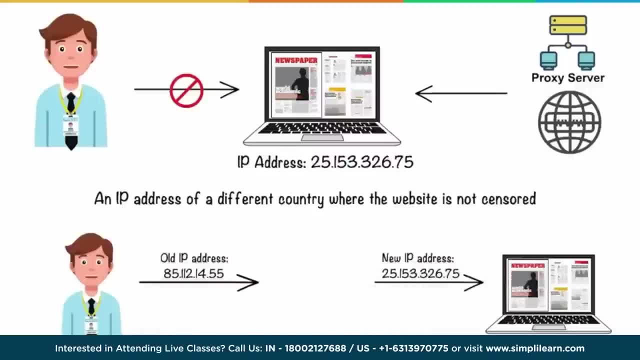 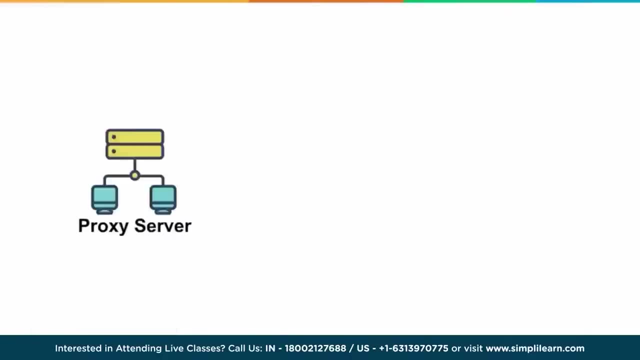 the website administrators see the new IP address assigned via proxy server and sees no reason to deny access to their account. Once the proxy server is able to access the website, it's passed on to Jonathan's system via the same channel. Regarding accessibility to proxy servers, 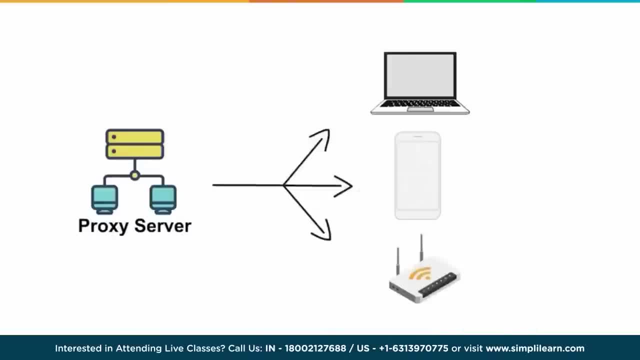 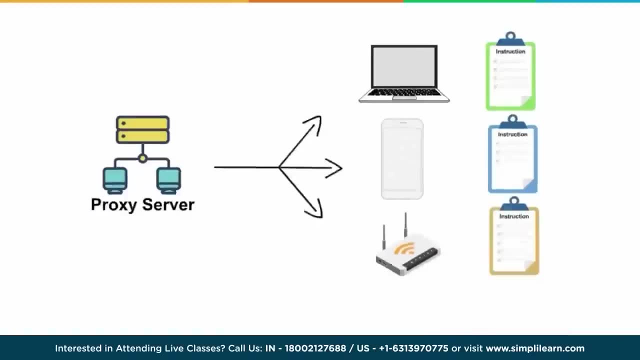 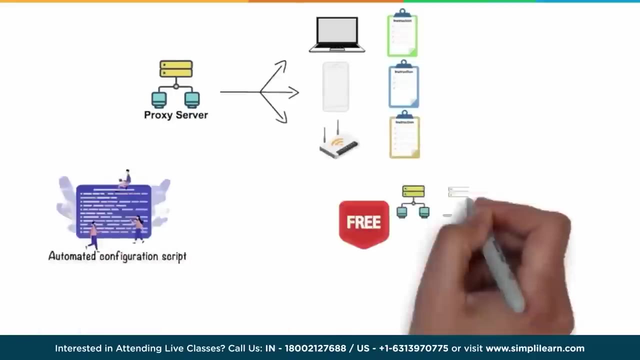 you must first set it up on your computer device or network. Next check the steps required for your computer or network, as each operating system has its setup procedures. In most cases, however, setup entails using an automated configuration script. There are plenty of free proxy services available on the Internet. 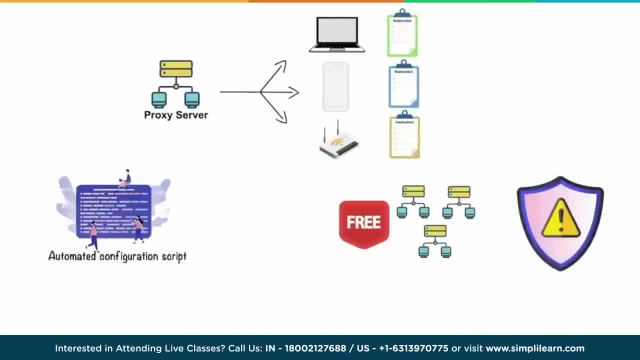 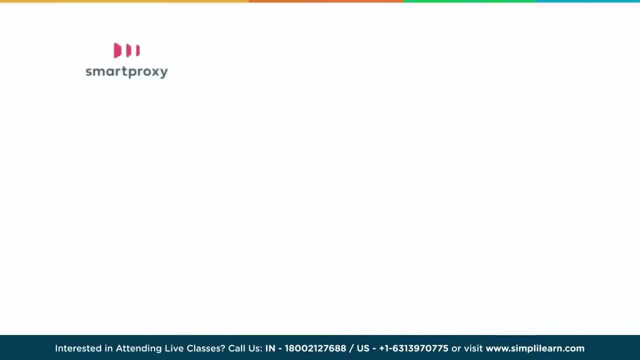 However, the safety of such proxies is rarely verified. Most free proxies will provide an IP address and a relevant port for connection purposes. Reputed proxy providers like Smart Proxy and BrightData that run on subscription models will most likely provide credentials to log into when establishing the connection. 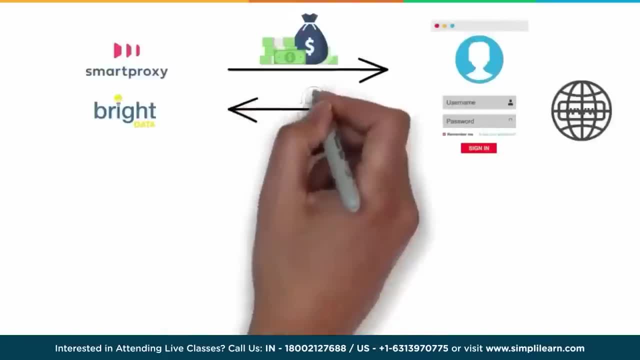 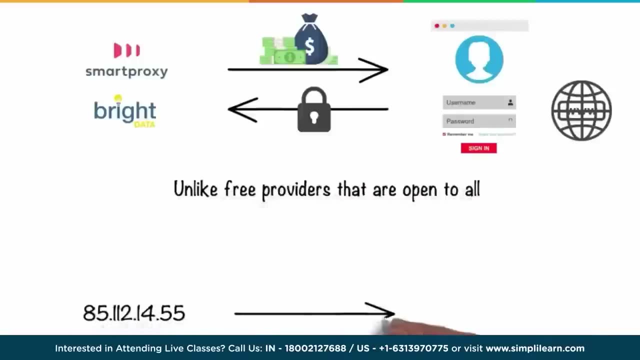 This extra step acts as a way for Jonathan to be able to access the internet. There is authentication that verifies an existing subscription on the proxy provider server, unlike free providers that are open to all. When it comes to hiding IP addresses, many people consider a VPN to be the primary solution. 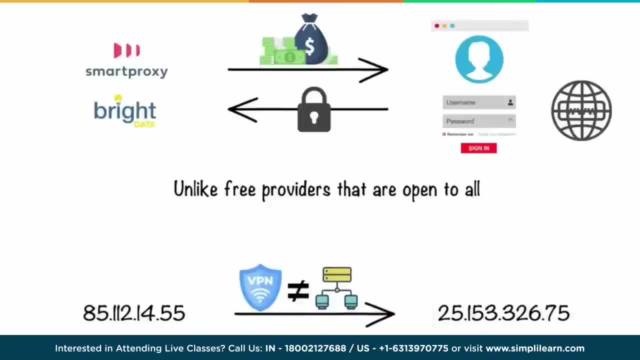 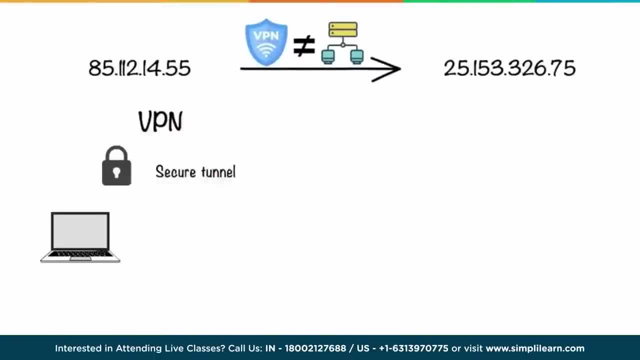 While that's true up to some extent, there are a few things proxies do differently. In the case of VPNs, extra encryption is also carried out to create a secure tunnel between the user's device and a VPN server. A VPN is usually much faster. 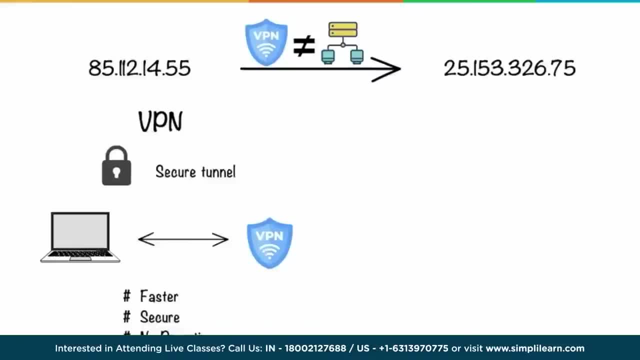 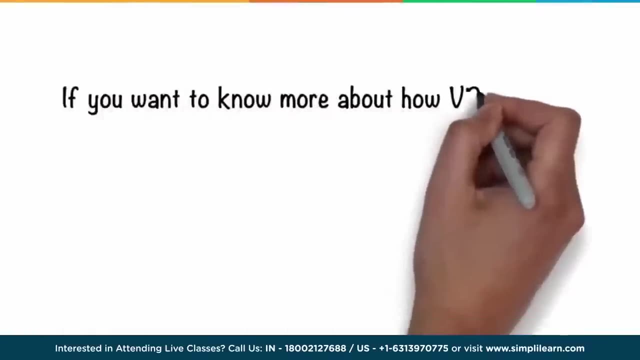 More secure thanks to multiple layers of encryption and has little to no downtime. Proxies tend to be comparatively unsafe, with the service owners having the exact IP address of the end user and having no guarantees regarding downtimes and reliability. If you want to know more about how VPNs work, do watch how Jude could have. 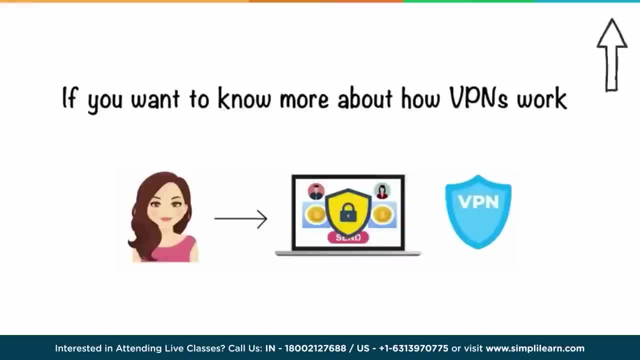 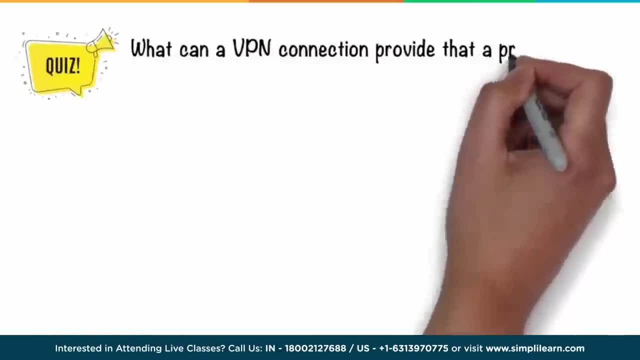 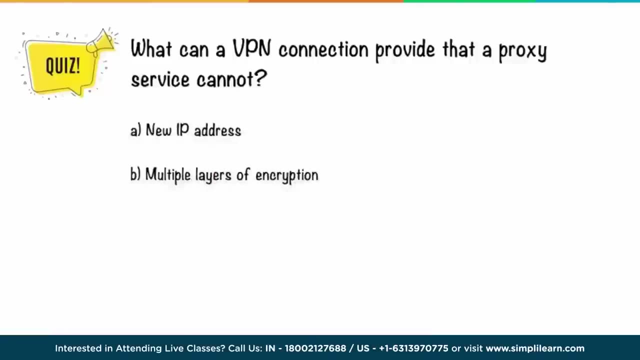 protected her banking credentials using VPNs in our detailed video linked above. Now let's take a small quiz to check how much we have learned. What can a VPN connection provide that a proxy service cannot? A New IP address. B Multiple layers of encryption. 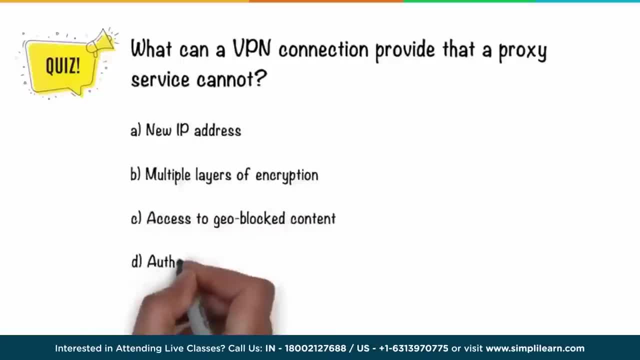 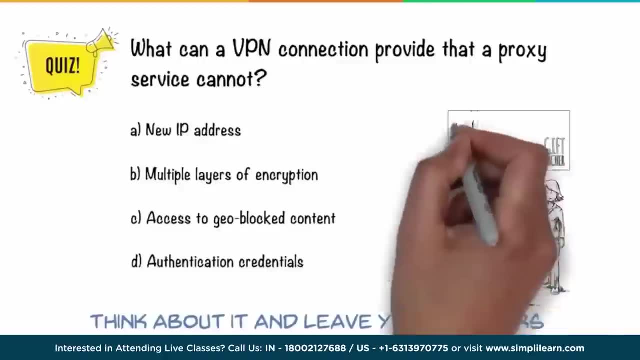 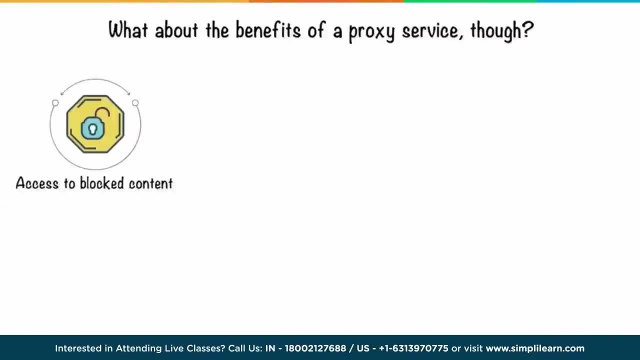 C- Access to geoblocked content. D- Authentication credentials. Think about it and leave your answers below in the comments section, and three lucky winners will receive Amazon gift vouchers. What about the benefits of a proxy service, though? Besides allowing access to blocked content, proxies can serve as an efficient 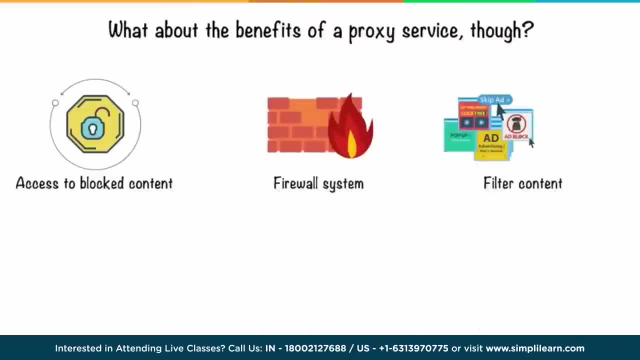 system. They can also filter content from third party websites, allowing control over Internet usage. In many cases, browsing speeds are stabilized compared to vanilla Internet, thanks to proper optimization on the base proxy server. The element of privacy proxies provides is highly lucrative to people looking. 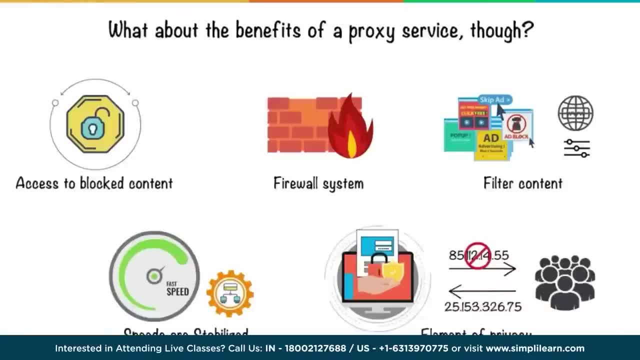 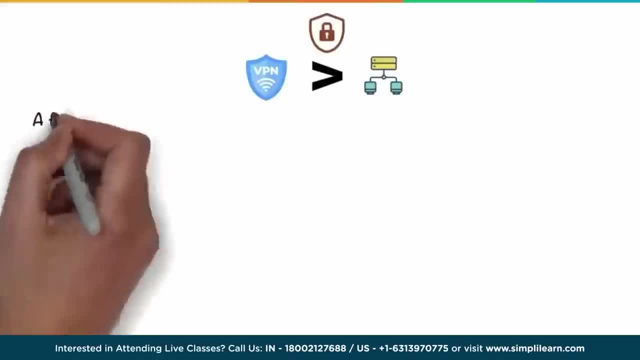 to hide their actual IP address from as many crying eyes as possible. One can easily argue the benefits of using VPNs over proxies for added security measures. However, a few basic tasks don't warrant maximum privacy for the user's side, as in other cases. For example, many consumers worldwide find proxy services. 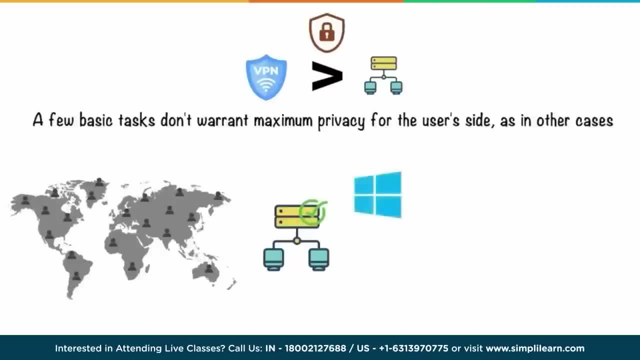 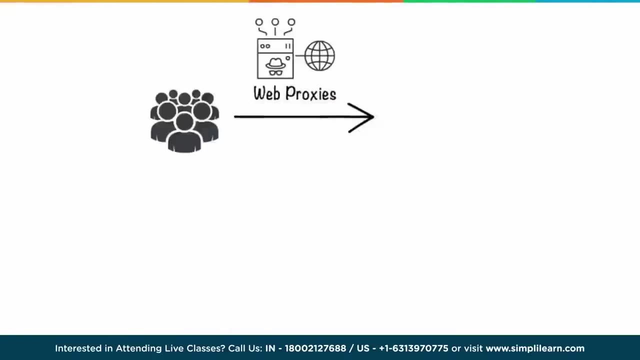 more convenient, since all major operating systems, starting from Windows to Android, allow proxy configuration without the hassle of installing new applications, as is in the case of a VPN. In addition, there are services online that function as web proxies, allowing users to access blocked content without any. 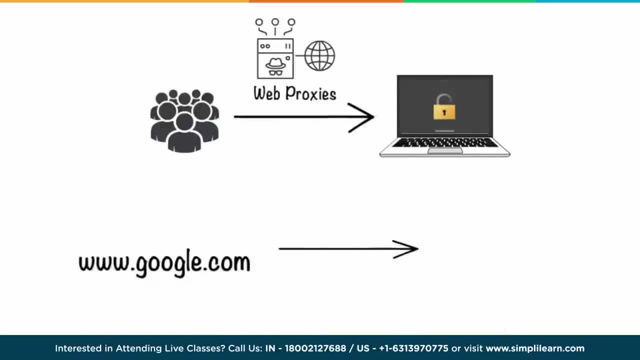 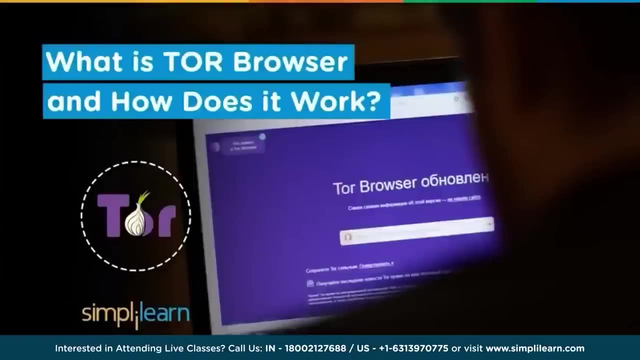 backup from their end. They can enter the target URL and the web proxy will route data from its physical server. This level of freedom is hard to come by in the case of VPNs, making proxies an ideal solution for casual browsing, With the next generation of Internet exchanges focused on maximum privacy. 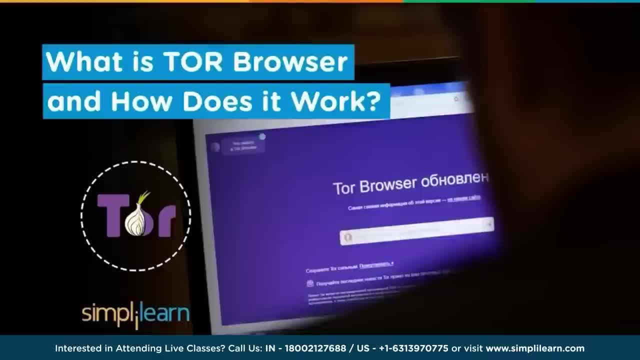 and security, a variety of ways have been enforced to maintain them. as such, Censorship has been shifted from the streets to the digital domain, forces the standard citizen to derive alternative ways to maintain anonymity. A major weapon in this battle for privacy and security is the Tor Browser. 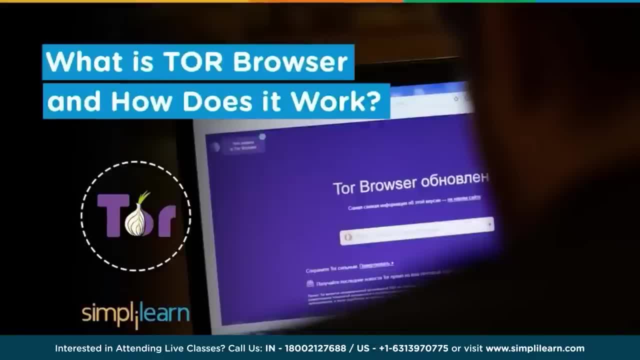 an independent browser meant to browse the Internet while reeling information through the Tor network. It serves as a meaningful alternative to the standard Internet browsing habits. To better understand the purpose of this browser and such, we must learn about the work of the Tor network. 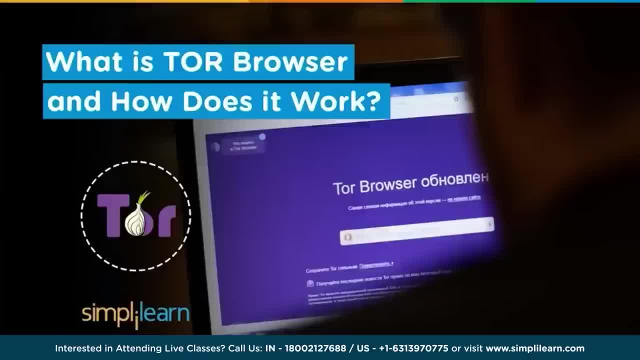 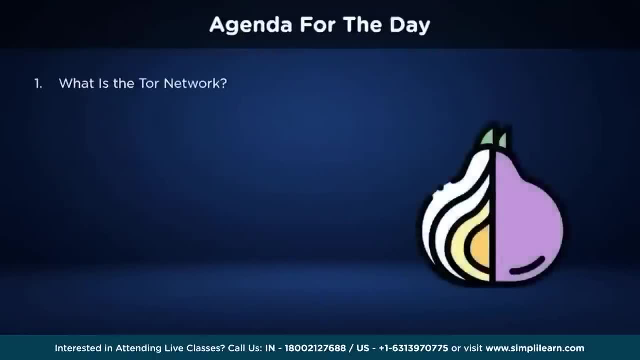 Featuring its own routing protocol, the Tor browser is an easy way to maintain anonymity while browsing without emptying one's wallet. Let's take a look at the topics to be covered today. We start at the explanation of what is the Tor network and its significance. 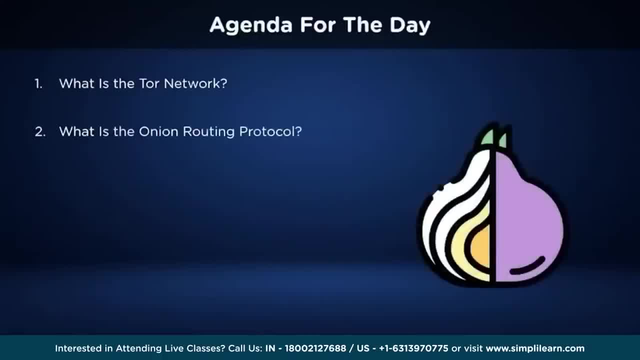 in the working of the Tor browser. We take a look at the onion routing protocol and how it transmits the data from the client devices to the Tor directories in order to circumvent government censorship. Moving on, we learn a few features of the Tor browser. 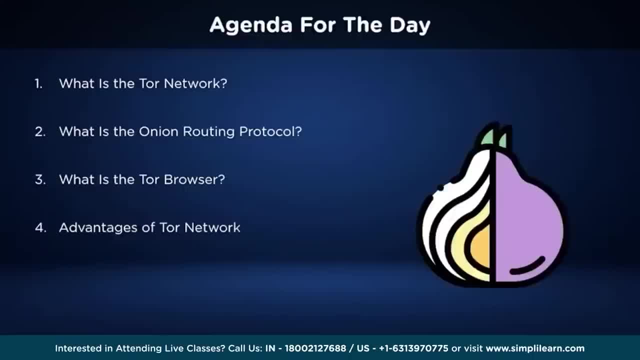 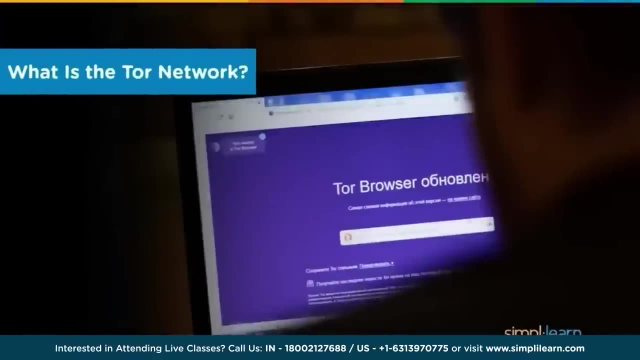 and the distinct advantages the Tor network provides. Next, we learn the difference between using a VPN and a Tor to anonymize Internet usage. And finally, we have a live demonstration of the Tor browser anonymization features in action. Let's move on to learning about the Tor network. 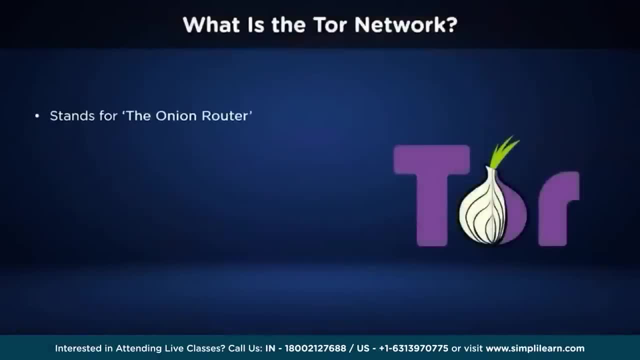 Tor, short for the Onion Router. it's an open source privacy network that permits users to browse the web anonymously. The Tor was initially developed and solely used by the US Navy to protect sensitive government communications, before the network was made publicly available. In the early days of the Tor network. 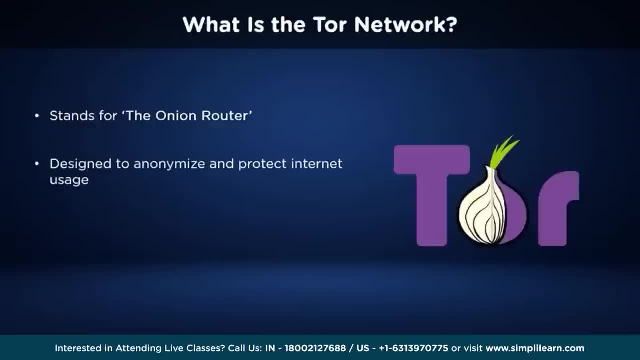 the digital era has disrupted the traditional way of doing things in every sector of the economy. The rapid rise in development and innovation of digital products has given way to frequent data breaches and cyber thefts. In response, consumers are increasingly opting for products that offer data privacy and cybersecurity. 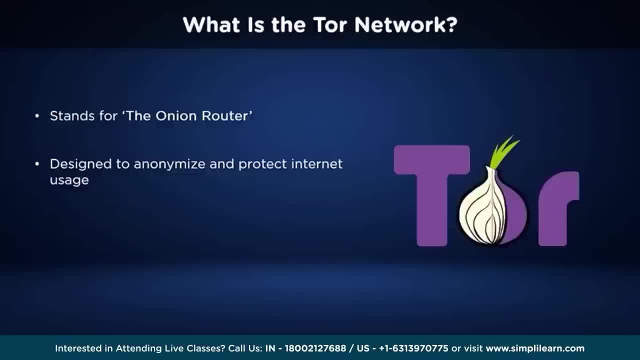 Tor is one such underground network that was implemented for the purpose of protecting users' identities. The Tor network is one example of the many emerging technologies that attempt to fill a data privacy void in a digital space plagued by cybersecurity concerns. The Tor network intercepts the traffic from your browser and bounces a user's 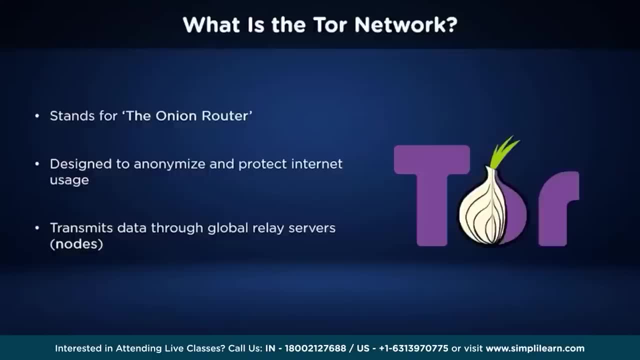 request of a random number of other user IP addresses, Then the data is passed to the user request's final destination. These random users are volunteer devices which are called as nodes or relays. The Tor network disguises your identity by encrypting the traffic and moving it across different Tor relays within the network. 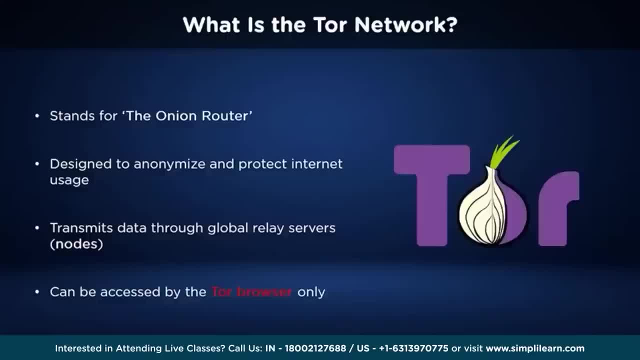 The Tor network uses an onion routing technique for transmitting data, hence the original name of Onion Router. To operate within the Tor network, a user has to install the Tor browser. Any address or information requested using the browser is transmitted through the Tor network. 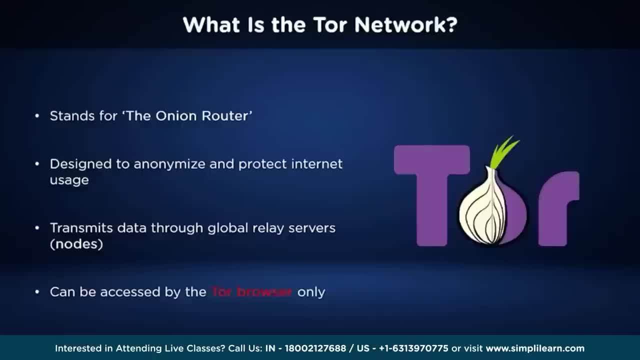 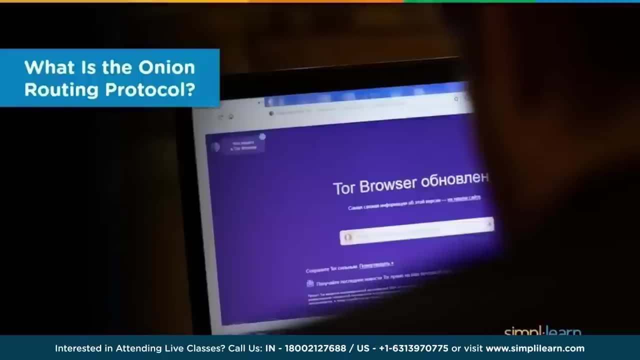 It has its own feature set, which we will be covering over later in this video. As we discussed already, the data passing through the Tor network must follow a unique protocol known as the Onion Routing Protocol. Let us learn more about its unique characteristics. 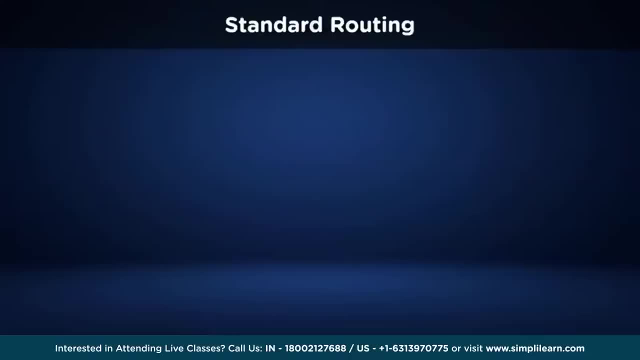 In our normal network usage, the data is transmitted directly. The sender has data packets to transmit, which is done directly over a line of communication with either a receiving party or a server of some kind. However, since the data can easily be captured while being transmitted, 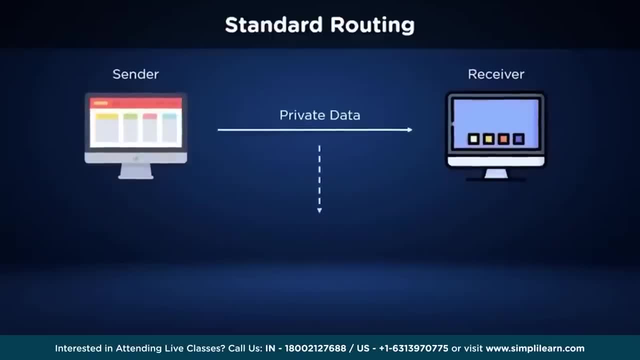 the security of this exchange is not very reliable. Moreover, it becomes very easy to trace the origin of such requests. On many occasions, websites with questions of questionable and controversial content are blocked from the ISP. This is possible since the ISP is able to detect and spy on user information passing through the network. 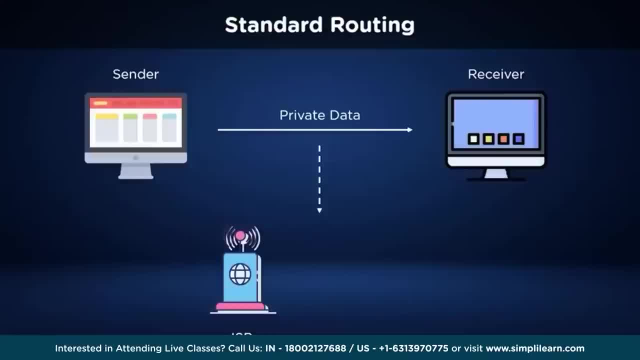 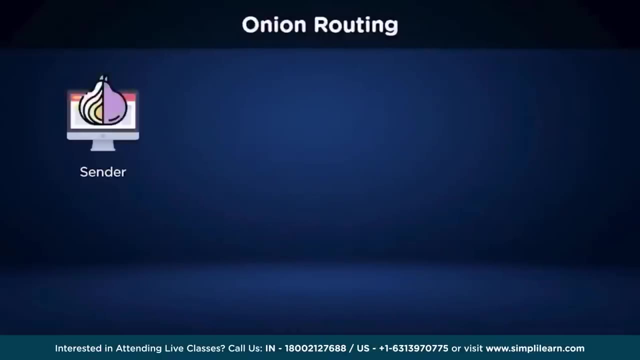 Apart from ISPs, there is a steady chance of your private information being intercepted by hackers. Unfortunately, easy detection of the source and contents of a web request make the entire network extremely vulnerable for people who seek anonymity over the Internet. However, in the Onion Routing Protocol, things take a longer route. 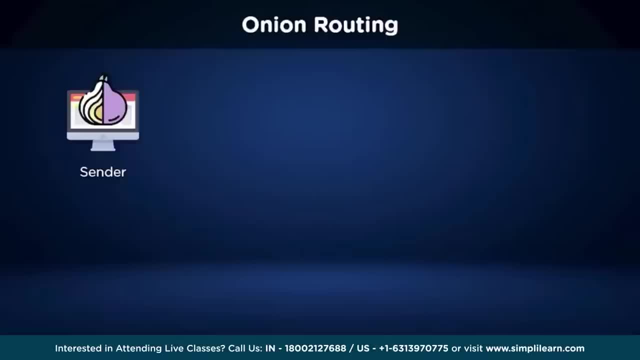 We have a sender with the Tor browser installed on the client system. The network sends the information to Node 1's IP address, which encrypts the information, and passes it on to Node 2's address, which performs another encryption and passes it on to Node 3's address. 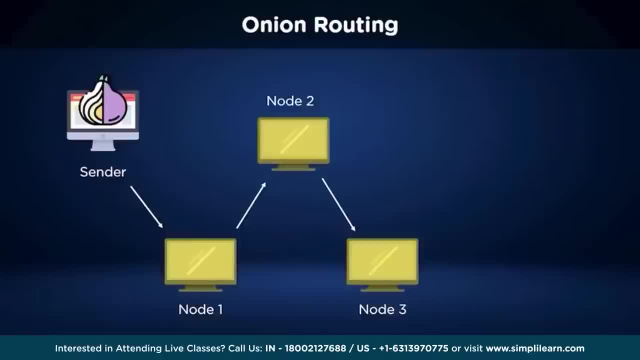 This is the last address, which is also known as the exit node. This last node decrypts the encrypted data and finally relays the request to the final destination, which can be another device or a server end. This final address thinks the request came. 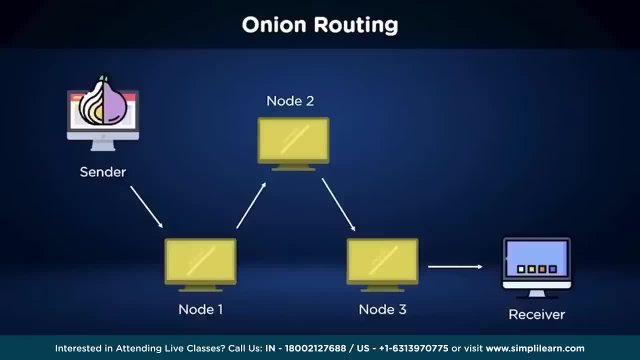 to the exit node and grants access to it. The encryption process across multiple computers repeats itself from the exit node to the original user. The Tor network obfuscates user IP addresses from unwanted surveillance by keeping the user's request untraceable, With multiple servers touching the data. 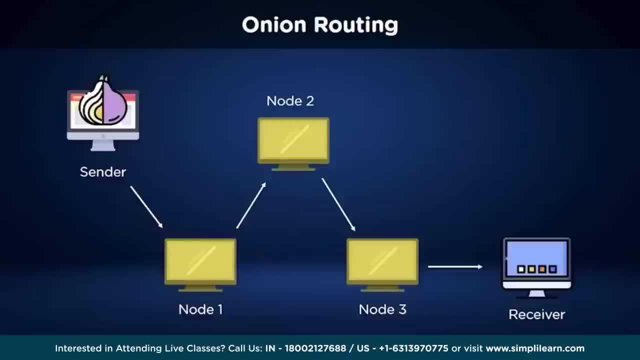 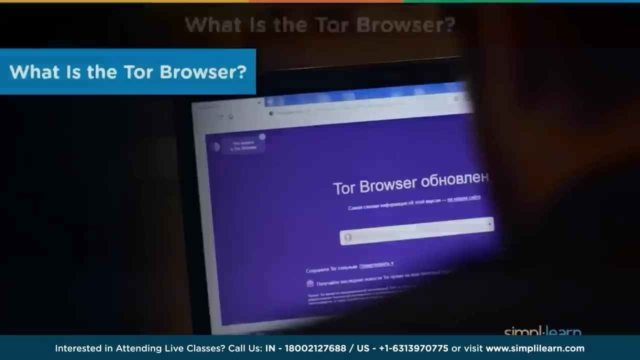 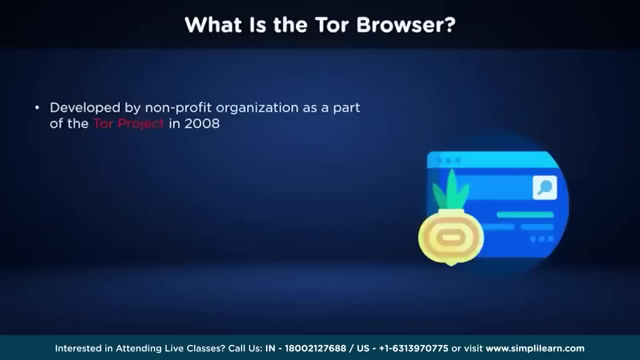 it makes the tracking very difficult for both ISPs and malicious attackers. Now that we understand the way Tor works, let us learn more about the Tor browser. The Tor browser was developed by a nonprofit organization as a part of the Tor project in 2008,. 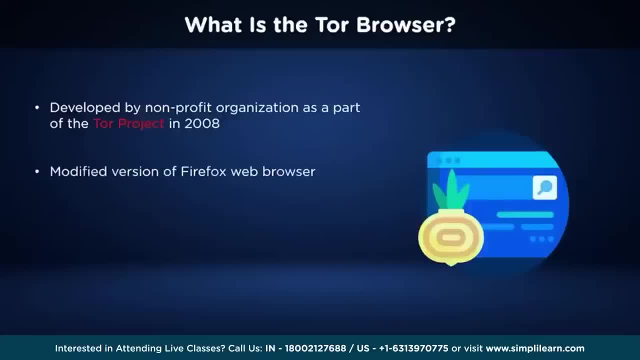 and its first public release was announced. The Tor browser is a browser forked from the popular Firefox that anonymizes your web traffic using the Tor network If you're investigating a competitor, researching an opposing litigant in a legal dispute, or just think it's creepy. 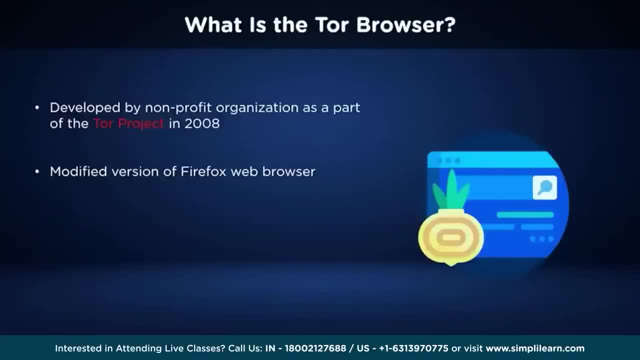 for your ISP or the government to know what websites you visit, the Tor browser might be the right solution. Before the Tor browser was developed, using the Tor network to maintain anonymity was a huge task for everyday consumers, Starting from the setup to the usage. 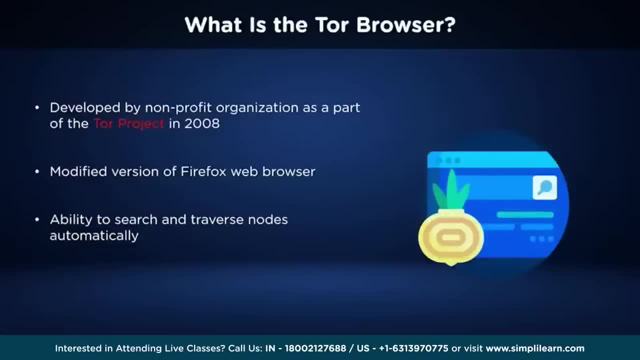 the entire process demanded a lot of knowledge and practice. The Tor browser managed to make it easy for users to traverse the relay servers in Tor and guarantee the privacy of the data exchange. A major feature of the Tor browser is the ability to delete all browser history, cookies and tracking data the moment it is closed. 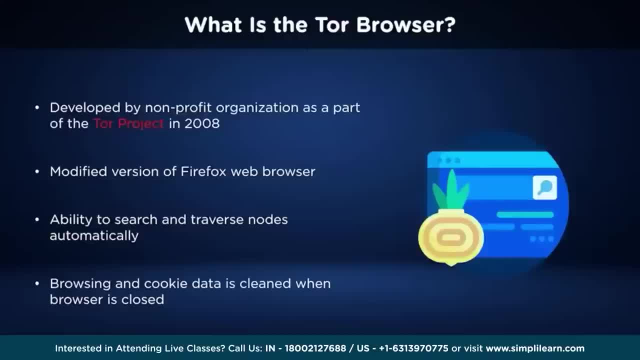 Every new launch of the browser opens an empty slate, having your usage habits from being tracked and singled out. A major feature that is the highlight of the Tor network is the availability of onion links. Only a small portion of the worldwide web is available to the general public. 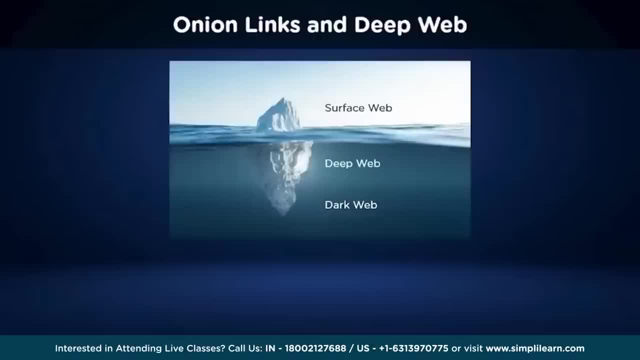 We have the deep web that contains links that are not allowed to be indexed by standard search engines like Google and Bing. The dark web is a further subset of the deep web, which contains onion links. Tor browser gives you access to these dot onion websites. 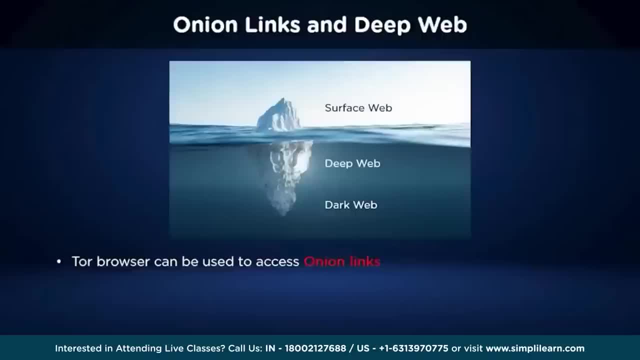 which are only available within the Tor network. Onion is a special use top level domain which designates an anonymous onion service, which is also known as a hidden service. Similar to the links of the deep web, these onion links provide services like online shopping. 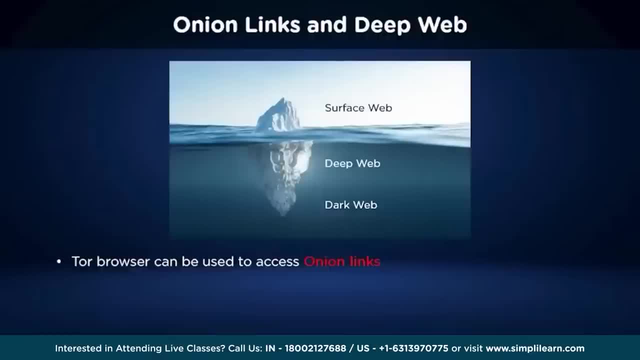 cryptocurrency and many other products not available in the consumer Internet space. Often being considered as a haven for illegal activities and sales, onion links provide both information and assets in a private manner without the risk of spying by authorities. Browsing the web over Tor is slower than the clear net due to the multiple layers of encryption. 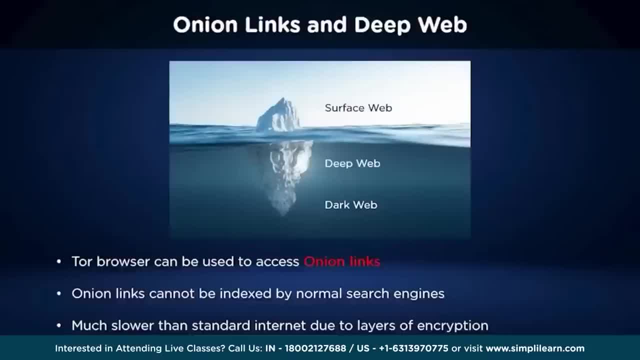 Some web services also block Tor users. Tor browser is also illegal in authoritarian regimes that want to prevent citizens from reading, publishing and communicating anonymously. Journalists and dissidents around the world have embraced Tor as a cornerstone of democracy, and researchers are hard at work at improving Tor's anonymity properties. 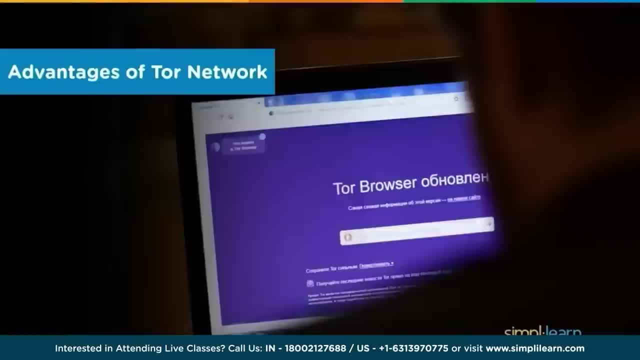 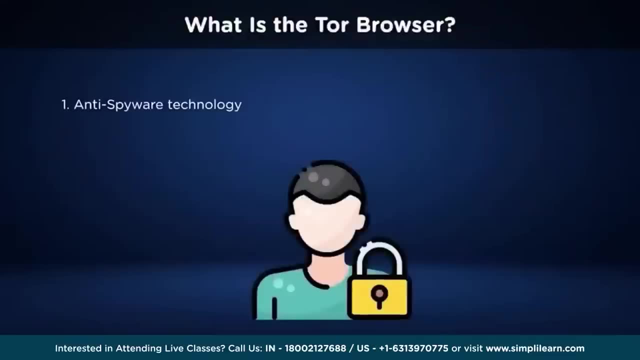 Let us take a look at some of the advantages of using the Tor browser, especially in standard web browsers. The highlight of using the Tor browser is to maintain anonymity over the Internet. The cause for such requests can differ from person to person, but all of these concerns are answered by the Tor network. 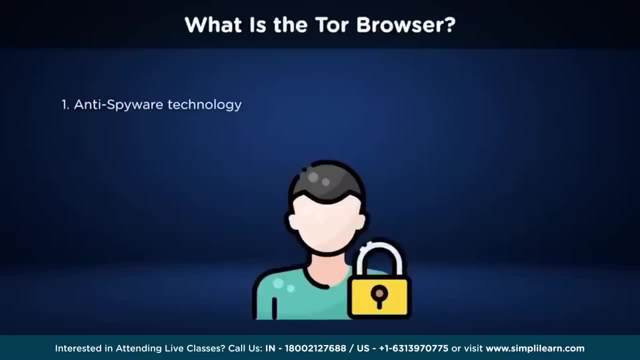 Doubting the information via multiple nodes and relay servers make it entirely difficult for the ISP to keep a track of usage data. The entire Tor project is designed to be completely free and open source. allowing the code for the browser to be protected and audited by third parties helps in the early detection of faulty. 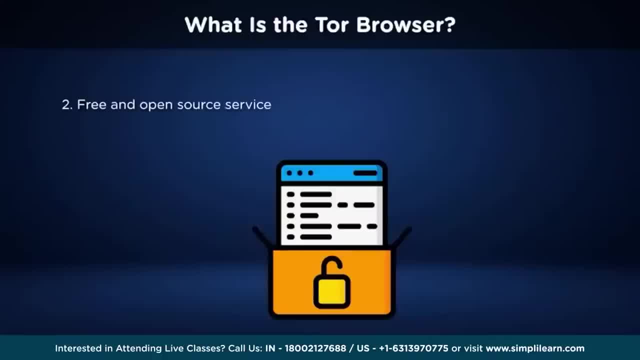 configurations and critical bugs. It is present for multiple operating systems, starting from laptops to mobile devices. A number of websites are blocked by governments for a variety of reasons. Journalists under authoritarian regimes have difficulty in getting the word out regarding the situation Since the onion routing protocol transfers. 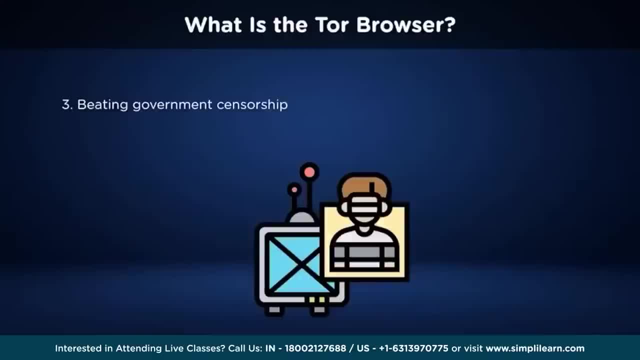 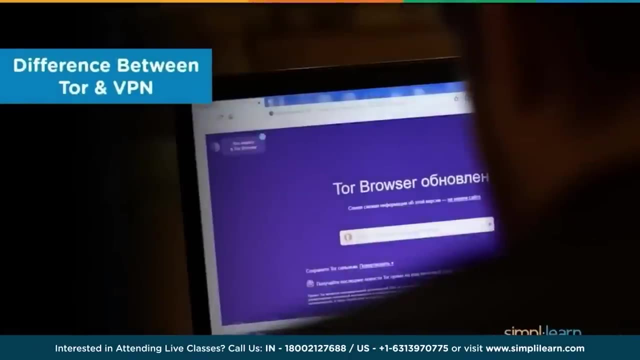 data between multiple servers of random countries. the domains being blocked become available when used via Tor. Usage of these encryption messaging platforms is easily enforced using the Tor browser, which otherwise would have been a difficult task under oppressive circumstances. Many people believe that a VPN offers the same benefits as the Tor browser. 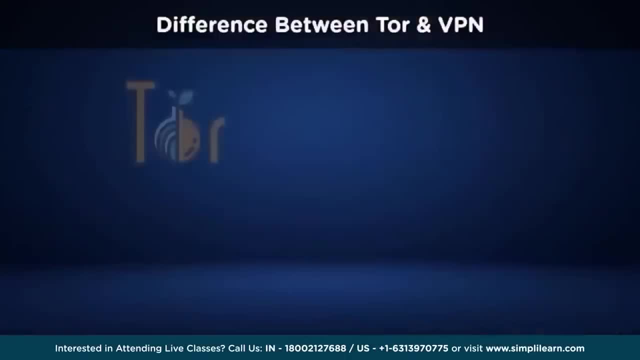 Let's put both of them to the test and see the differences between them. Coming to the first point of difference, Tor is completely free and open source. All of the code for the browser and the network can be audited and has been used for security concerns. 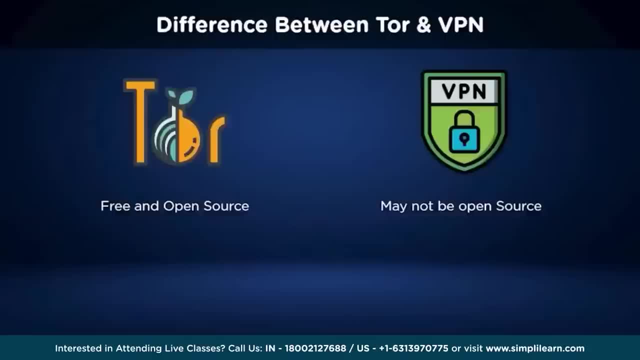 When it comes to VPN, there are many different brands which have open source clients, but the same cannot be said for their counterparts. Some have partly open source, while some have completely locked up their code so that they cannot be stolen further. Moving on, Tor has multiple relay points in its data transfer protocol. 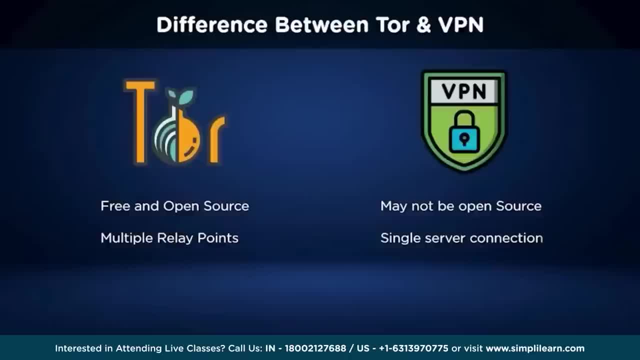 Between the server and the receiver, there are three different IP nodes. That number can increase, but it will always be more than two. Once the data is passed from the sender, it goes through all of those relay points, While in the case of a VPN, the connection is made from the client. 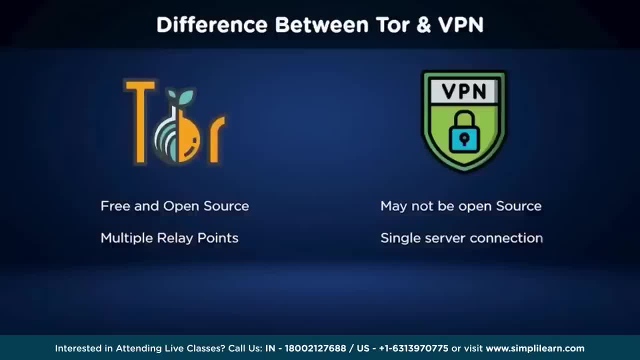 device to the VPN server and then to the requested destination. There is no other IP node that comes into work here, thereby making the connection a one to one between the client and a VPN. As a next point, since Tor handles multiple layers of encryption and the data passes. 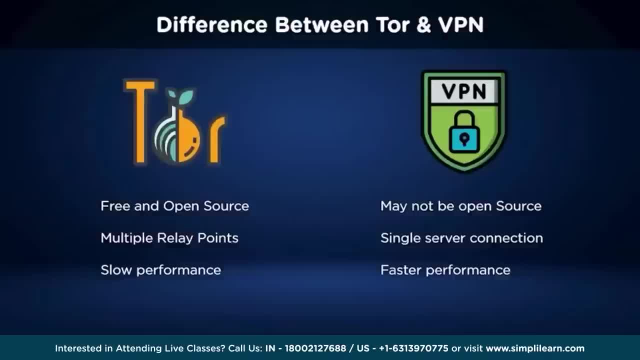 through multiple systems along the way. the performance is slow compared to a VPN, where the performance is relatively fast due to the less number of nodes the data passes through. Similarly, the multi-layer encryption of Tor is consistent. If you use Tor browser, every single request passes. 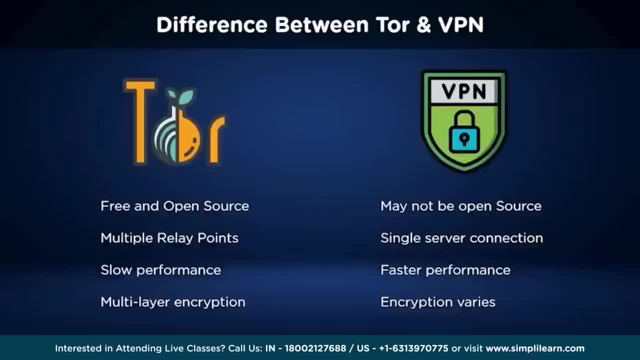 through the same layer of encryption and follows the same routing protocol. In the case of a VPN, different companies offer different levels of encryption. Some have multi-hop, some prefer a single one to one connection, and these kind of differences make the choice much more variable. 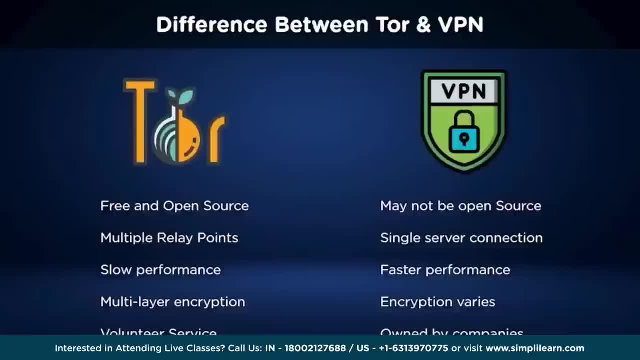 Finally, the nodes and relays being used in the Tor network are volunteer. There is no company holding over them, so jurisdiction becomes relatively straightforward, Whereas in the case of VPNs, many such VPNs are hosted by adware companies or are being monitored by central governments. to note the usage information: 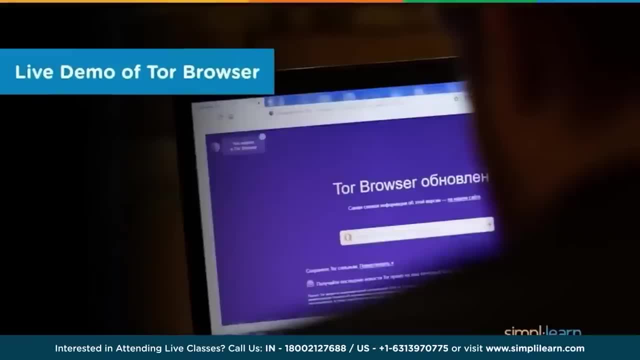 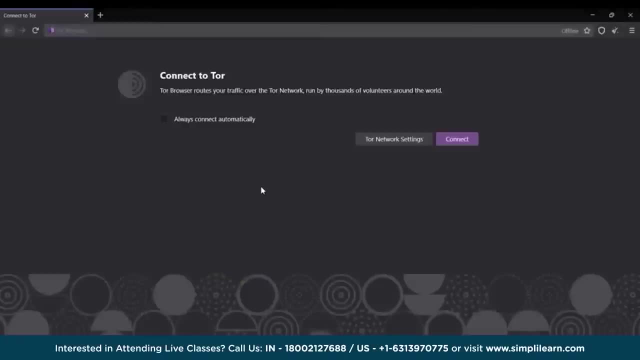 Now that we have a better understanding of the Tor browser and its routing, let us take a look at how the Tor browser can anonymize and protect our Internet usage. On opening up the Tor browser for the first time, this is the page that you are going to be welcomed with. 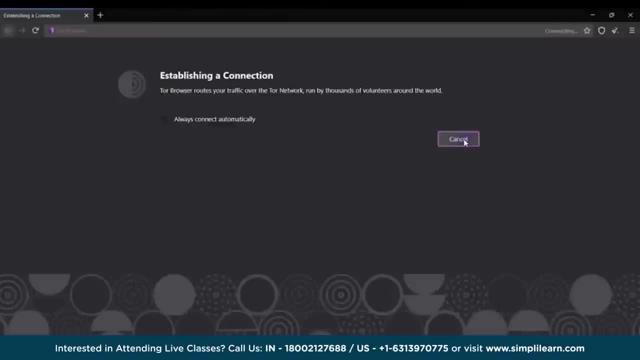 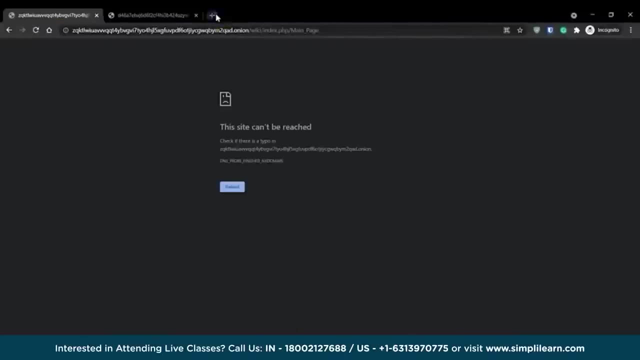 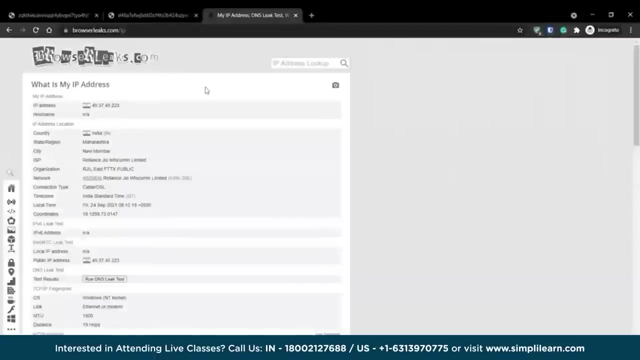 You have the option of connecting to the Tor network before we start our browsing, So let's press connect and we can see that it is connected. Coming to the anonymization, let's check my current location on Google Chrome. Currently is showing as Navi Mumbai, in Maharashtra. 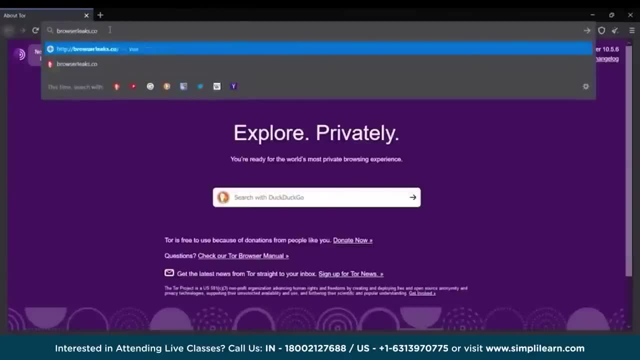 If we check the same link on the Tor browser, we should get a different address. Now, every link that we open in the Tor browser will be a little delayed and the speed will be hampered because of the multiple layers of encryption, like we discussed. 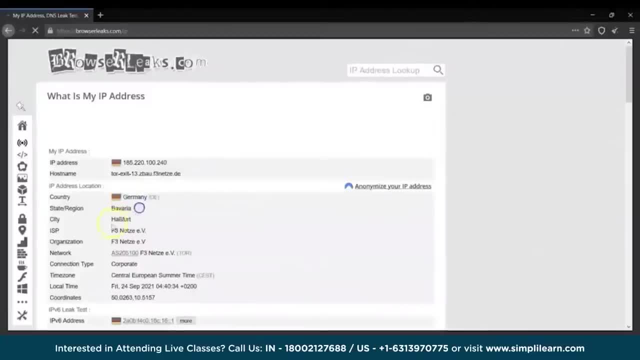 Now, as you can see, it's showing a German IP and the state of Bavaria. This is how the anonymization works. There is no VPN configured. there is no proxy attached. It's straight up out of the box settings that come inbuilt with the Tor browser. 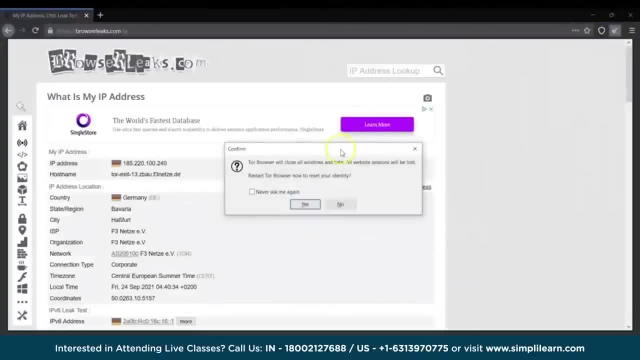 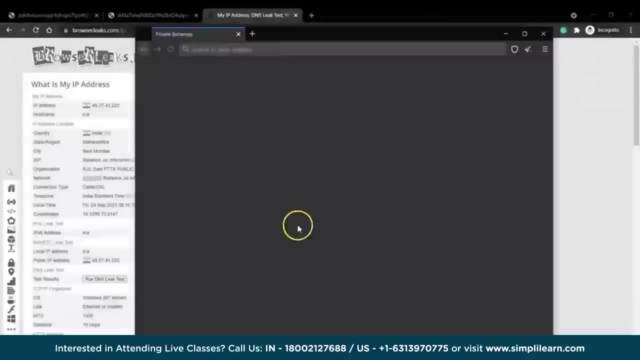 Similarly, we have an option of cleaning up the data. Let's say, if you want to refresh your location and you want to use a different ID for the next browsing session, If you just restart it once and you can have to check it again. 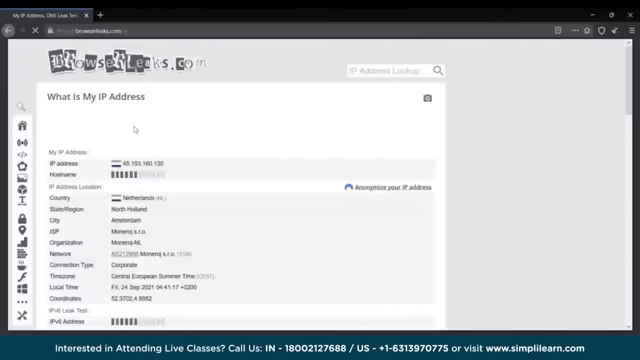 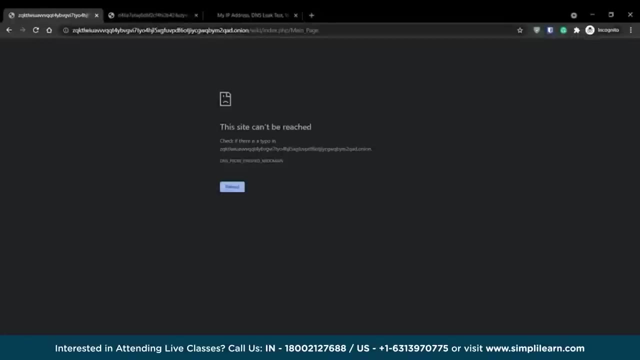 we should be seeing a different country this time. As you can see, we have Netherlands right now, So this is how you can keep refreshing your address. You can keep refreshing your host location so that you cannot be tracked when browsing the Internet. Like we discussed, we have some onion links that can only be used on the Tor network. 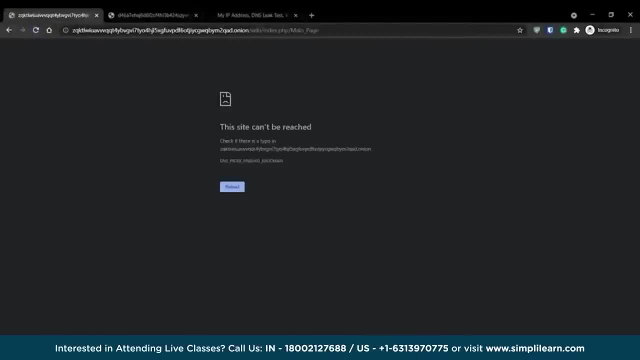 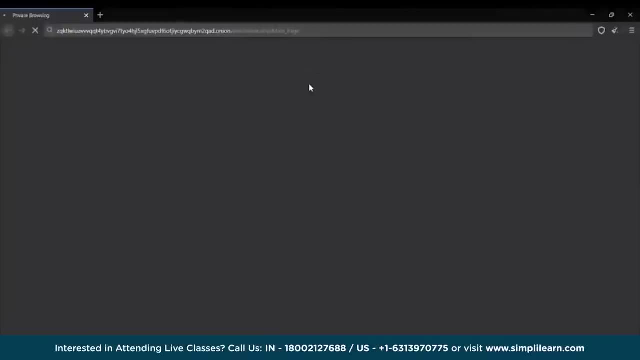 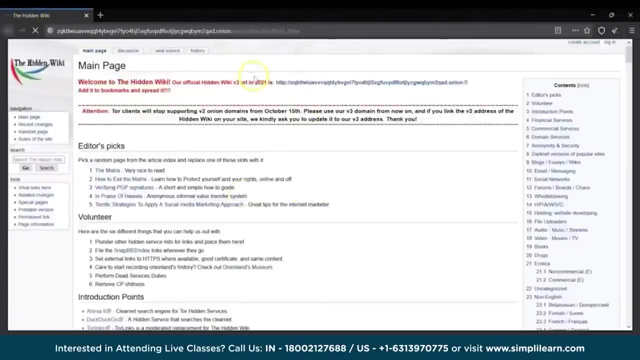 As you can see, these kind of links do not open in the Google Chrome browser, but once we copy these over to the Tor browser. As you can see, we have opened the hidden wiki, which is available only on the Tor network. This is kind. 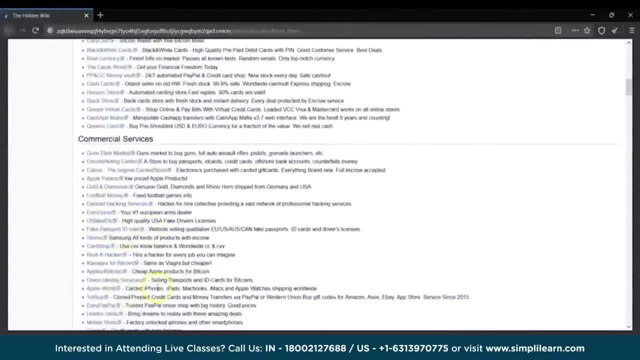 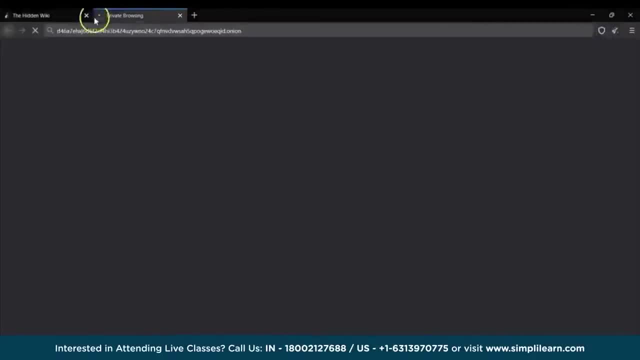 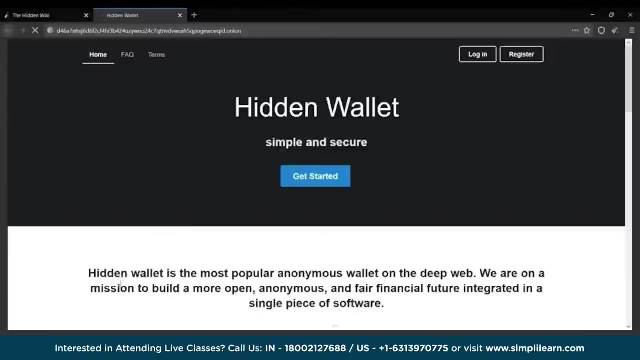 of an alternative Wikipedia website where we can find articles to read and more information to learn. Similarly, we have another onion link over here which is once again available only for the Tor browser. Now, these kind of delays are expected, but they are a valid compromise. 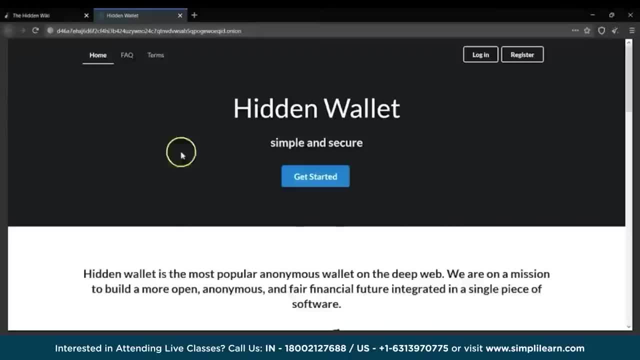 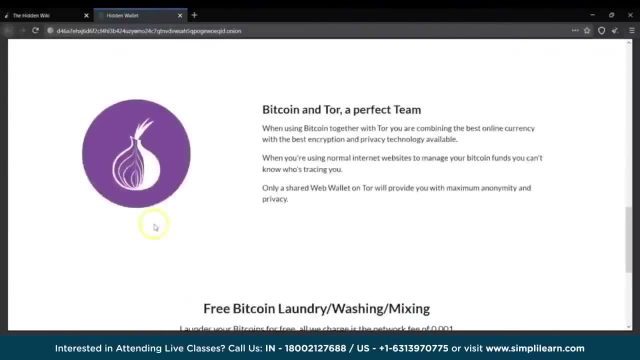 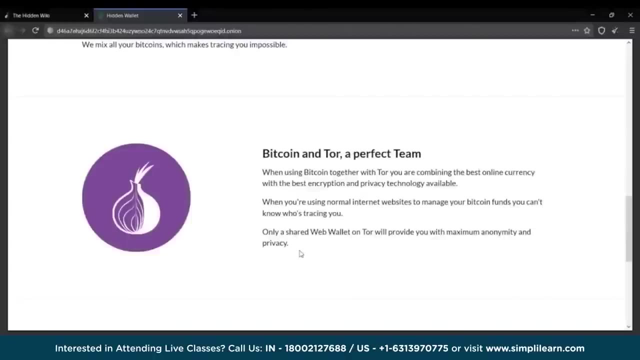 because they maintain the anonymity that many people desire. Similarly, we have found a hidden wallet, which is a cryptocurrency wallet, which is specifically for dark web members. This operates over the Tor network and this is used by mostly journalists and people who want to anonymize their Internet transactions when it comes. 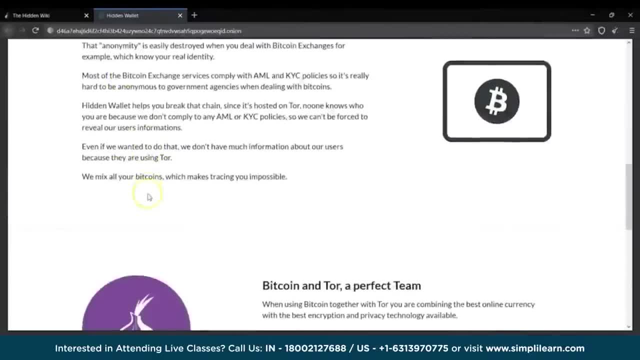 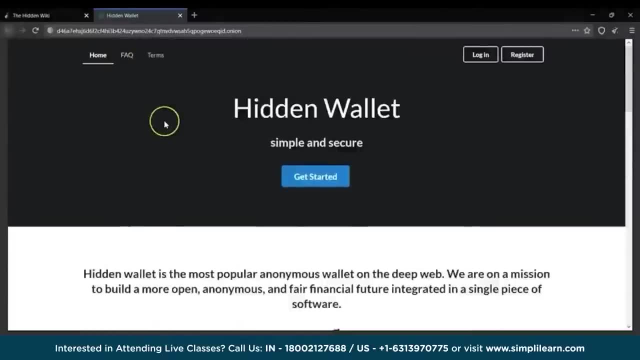 to dealing money. All of the transactions that occur over the Tor network are almost impossible to track. Therefore, these kind of cryptocurrency wallets are very big on the deep web. This is just one example. While having multiple different wallets for every single cryptocurrency available, imagine our houses without 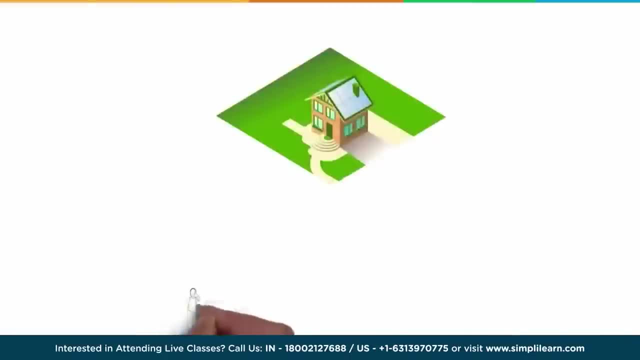 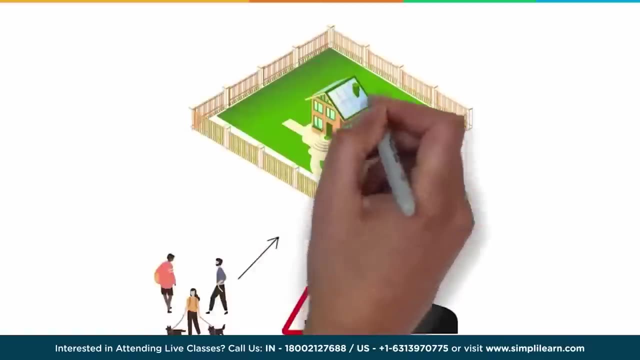 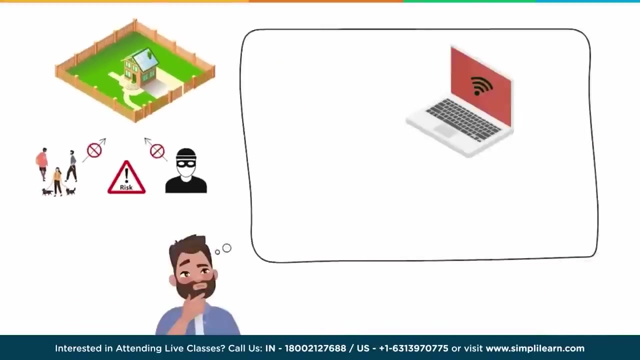 a fence or boundary wall. this would make our properly easy accessible to trespassers and robbers and place our homes at great risk. Right Hence fencing our property helps safeguard it and keeps trespassers at bay. Similarly, imagine our computers and networks without protection. 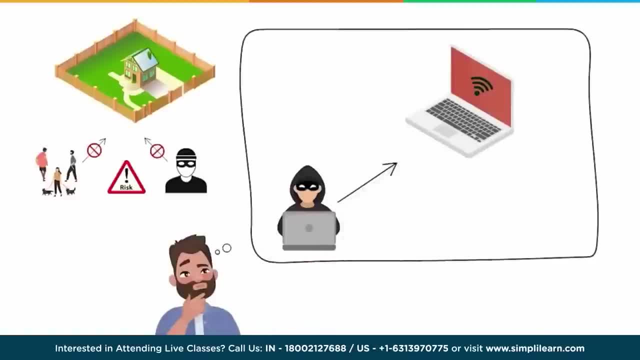 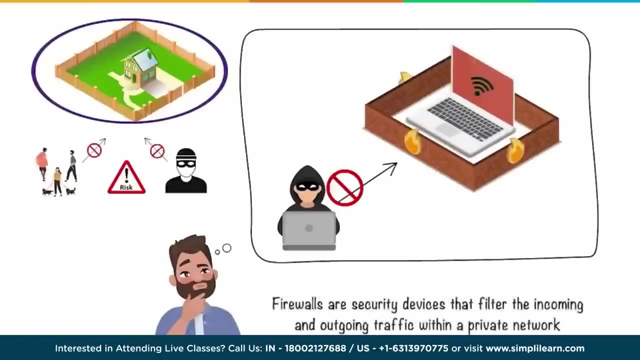 This would increase the probability of hackers infiltrating our networks. To overcome this challenge, just like how boundary walls protect our houses, a virtual wall helps safeguard and secure our devices from intruders, And such a wall is known as a firewall. Firewalls are security devices that filter. 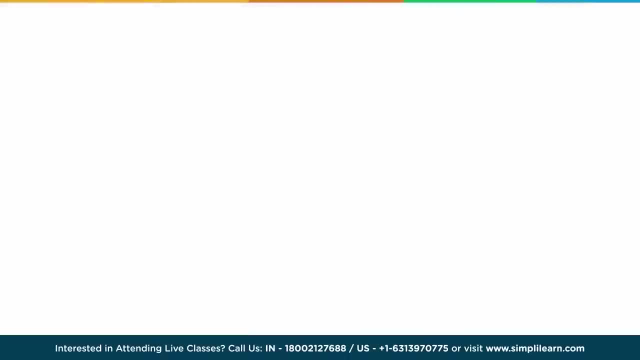 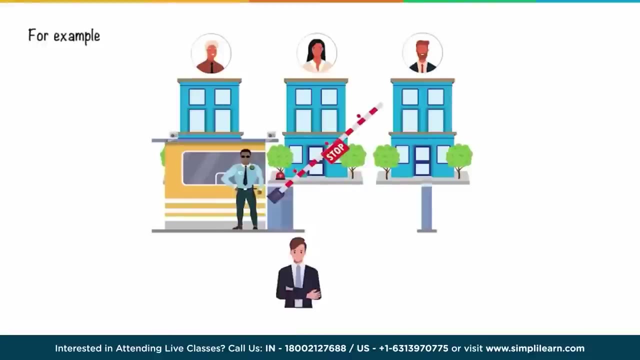 the incoming and outgoing traffic within a private network. For example, if you were to visit your friend who lives in a gated community, you would first take permission from the security guard. The security guard would check with your friend if you should be allowed entry or not. 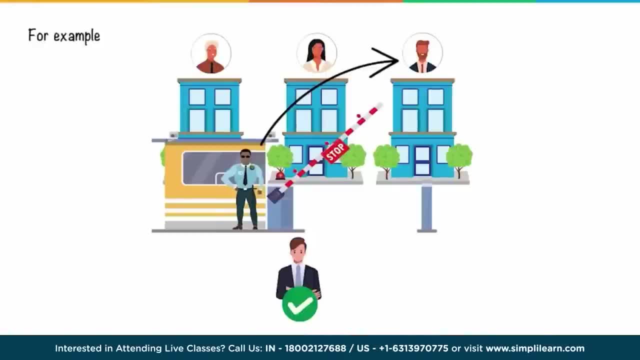 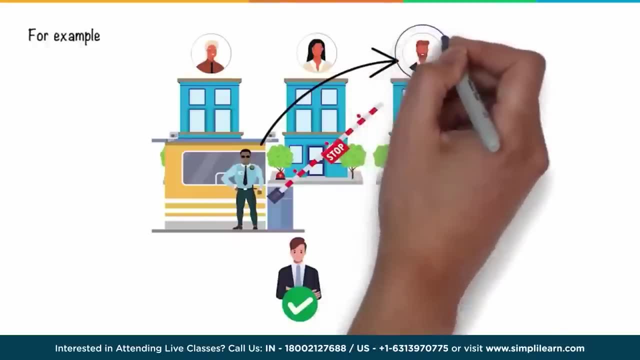 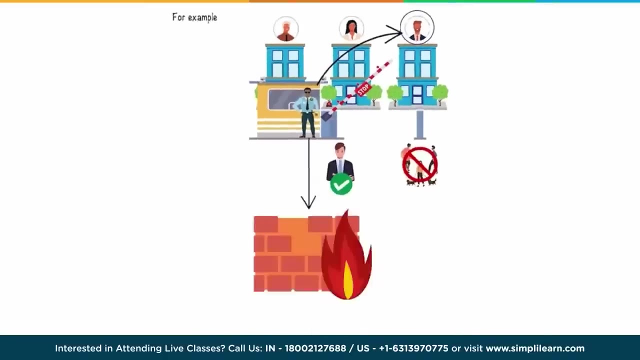 If all goes well, your access is granted. On the other hand, the security guard would not grant permission to a trespasser looking to enter the same premises. Here, the entry access depends solely on your friend, the resident's discretion. The role of the security guard in this case is similar to that of a firewall. 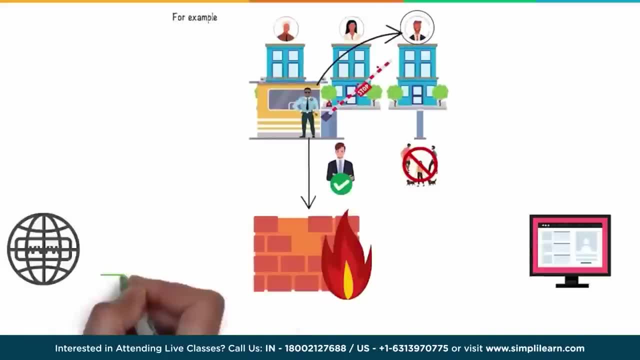 The firewall works like a gatekeeper at your computer's entry point which only welcomes incoming traffic that it has been configured to accept. Firewalls filter the network traffic within your network and assesses which traffic should be allowed or restricted, based on a set of rules in order to spot and prevent cyber attacks. 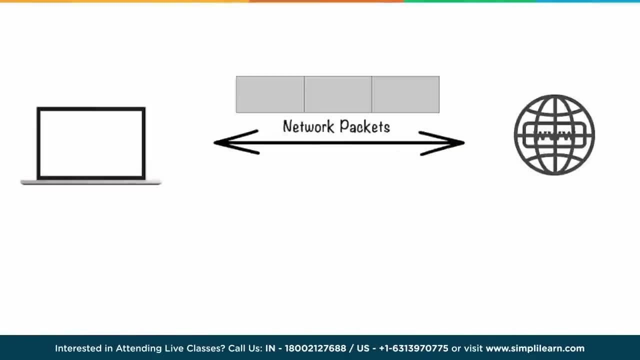 Your computer communicates with the Internet in the form of network packets that hold details like the source address, destination address and information. These network packets enter your computer through ports. The firewall works on a set of rules based on the details of these network packets. 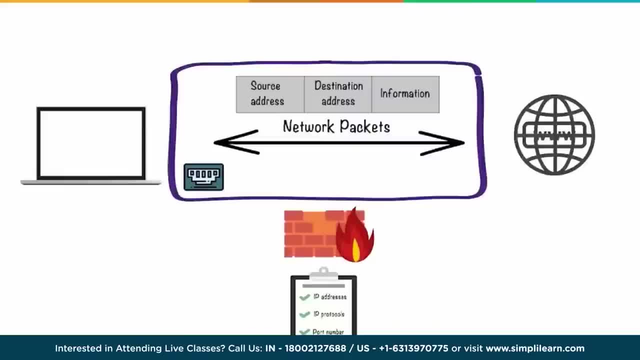 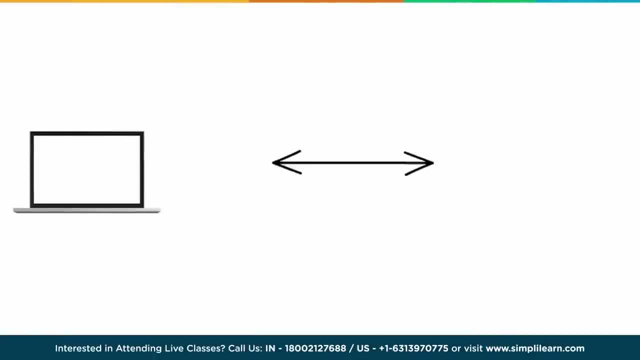 like their source address, a destination address, content and port numbers. Only trusted traffic sources or IP addresses are allowed to enter your network. When you connect your computer to the Internet, there is a high chance of hackers infiltrating your network. This is when a firewall comes to your rescue by acting as a barrier between your 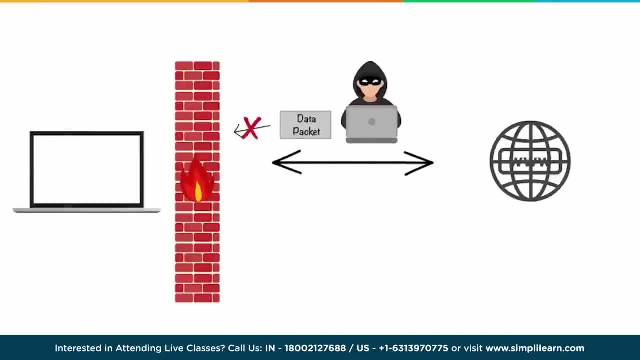 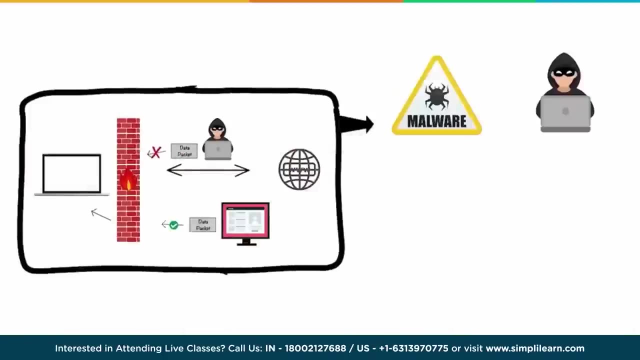 computer and the Internet. The firewall rejects the malicious data packet and thus protects your network from hackers. On the other hand, traffic from trusted websites is allowed access to your network. This way, the firewall carries out quick assessments to detect malware and other suspicious activities, thereby protecting your network from being 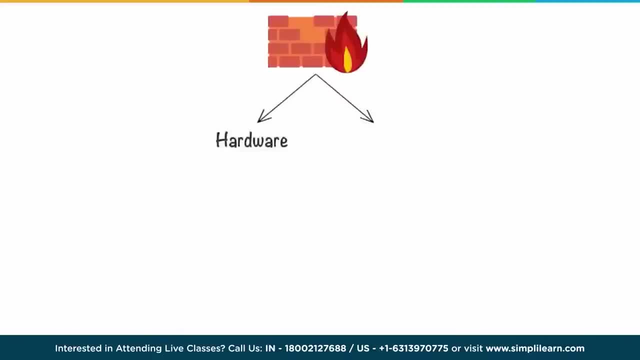 susceptible to a cyber attack. Firewalls can either be hardware or software. Software firewalls are programs installed on each computer. This is also called a host firewall. Meanwhile, hardware firewalls are equipments that are established between the gateway and your network. Linksys routers are a good example of a hardware firewall. 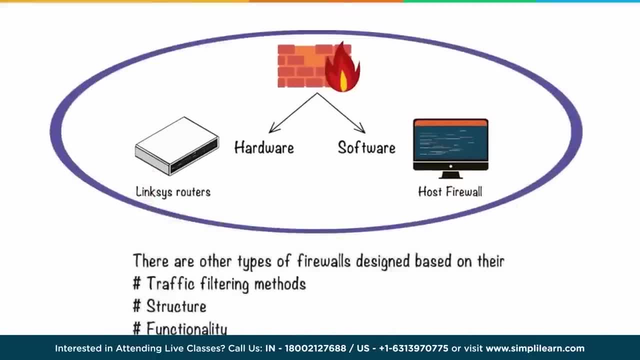 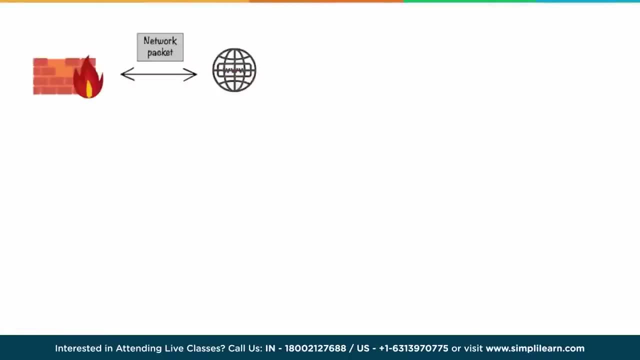 Besides this, there are other types of firewalls designed based on their traffic filtering methods, structure and functionality. The firewall that compares each outgoing and incoming network packet to a set of established rules, such as the allowed IP addresses, IP protocols, port number and other aspects of the packet, is known. 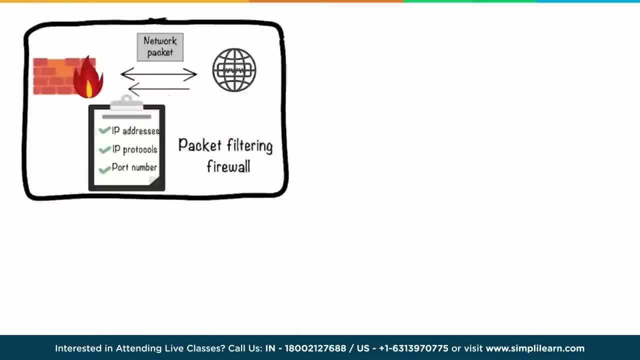 as a packet filtering firewall. If the incoming network traffic is not per the predefined rules, that traffic is blocked. A variant of the packet filtering firewall is the stateful inspection firewall. These types of firewalls not only examine each network packet but also check whether or not that network packet is part of an established network connection. 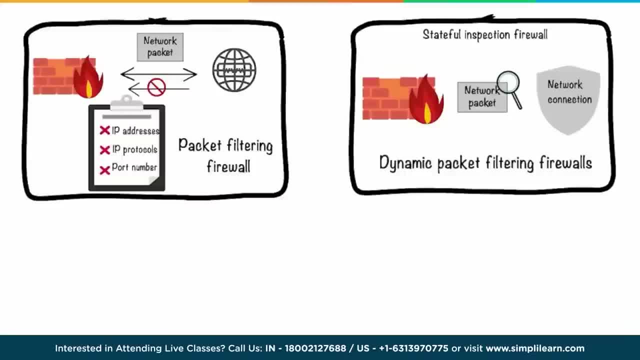 Such firewalls are also referred to as dynamic packet filtering firewalls. Our next type of firewall is called a proxy firewall. This draws close comparison to how you give proxy attendance for a friend, like how you take the authority to represent your friend. The proxy firewall pretends to be you and interacts with the Internet. 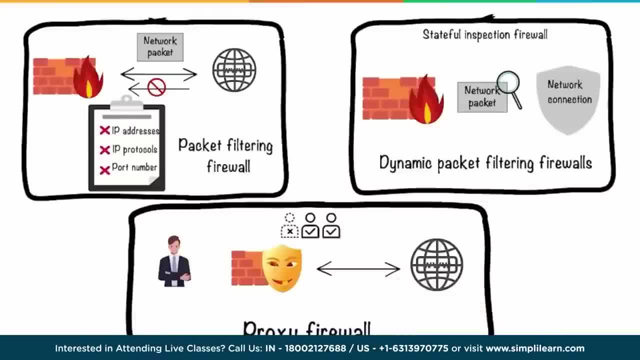 They come between you and the Internet and thereby prevents direct connections. This protects your device's identity and keeps the network safe from potential attacks. Only if the incoming data packet contents are protected, the proxy firewall transfers it to you. They're also known as application level gateway. 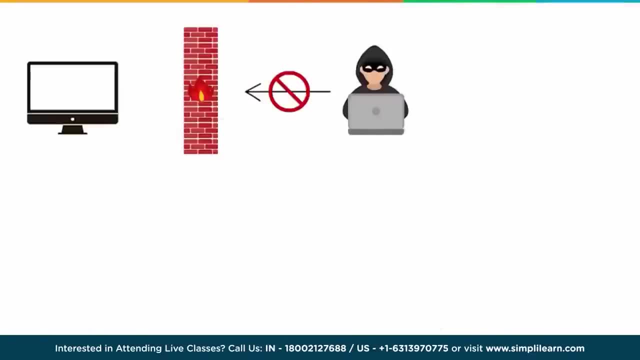 The firewall can spot malicious actions and block your computer from receiving data packets from harmful sources. In addition to preventing cyber attacks, firewalls are also used in educational institutions and offices to restrict users access to certain websites or applications. It is used to avoid access to unauthorized content. 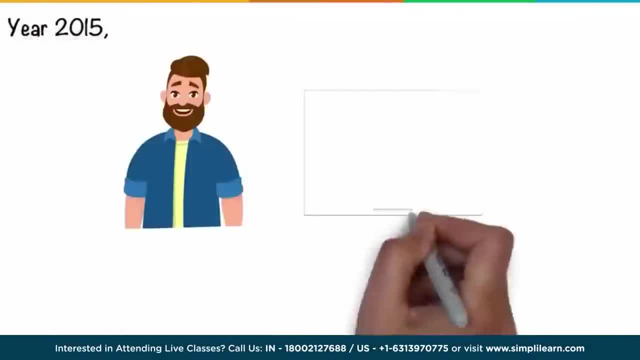 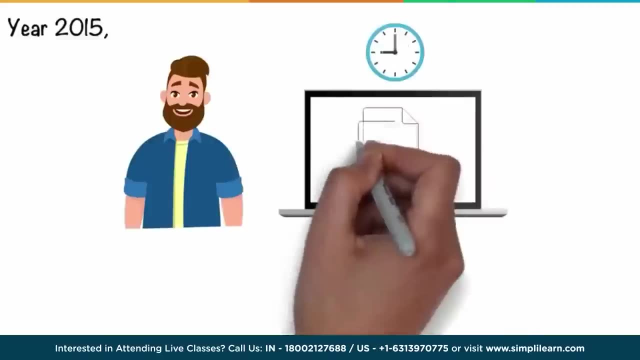 It's the year 2015, and Richard has just finished playing games on his computer. After a long gaming session, Richard tries to shut it down, but finds some random text file on the desktop that says Ransom. Note: The text file mentioned how a hacking 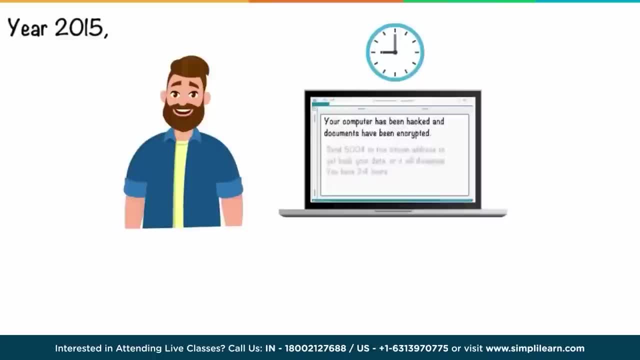 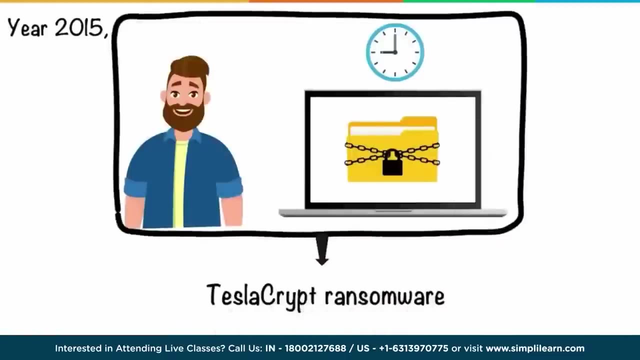 group had encrypted Richard's game files and private documents and he had to pay a ransom of $500 worth of Bitcoin in a specified Bitcoin address. Richard quickly checked his files only to see them being encrypted and unreadable. This is the story of how the Tesla Crypt ransomware spread in 2015,. 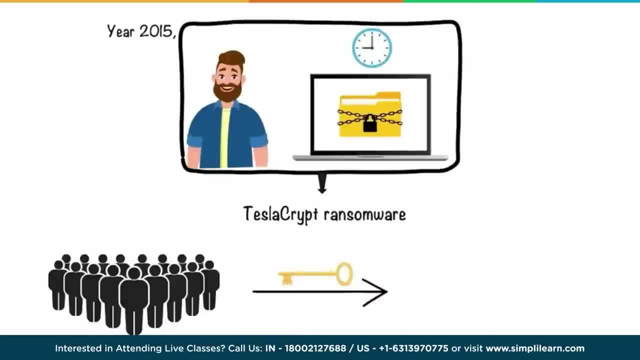 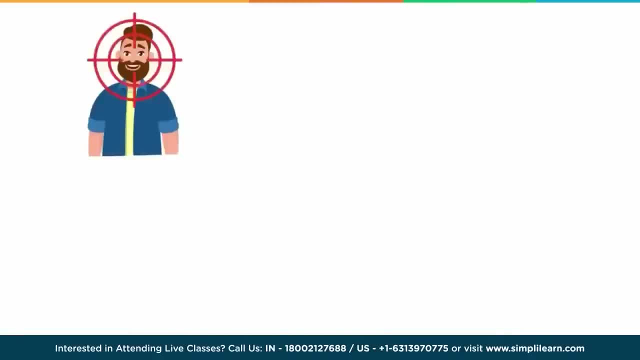 which affected thousands of gamers, before releasing the master key used for encrypting the files. So what is ransomware? For Richard to be targeted by such an attack, he must have installed applications from untrusted sources or clicked an unverified link. Both of them can function as gateways for a ransomware breach. 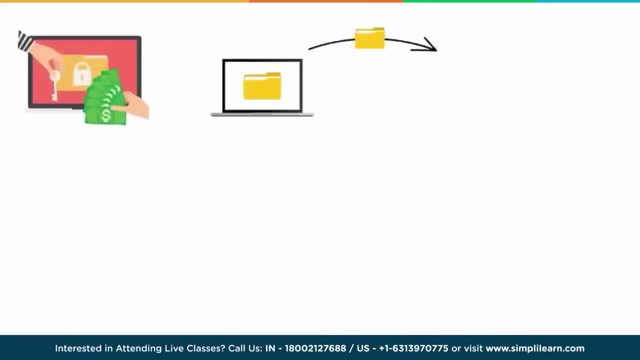 Ransomware is a type of malware that encrypts personal information and documents while demanding a ransom amount to decrypt them. This ransom payment is mainly done using cryptocurrency to ensure anonymity, but can also employ other routes Once the files are encrypted or locked behind a password. 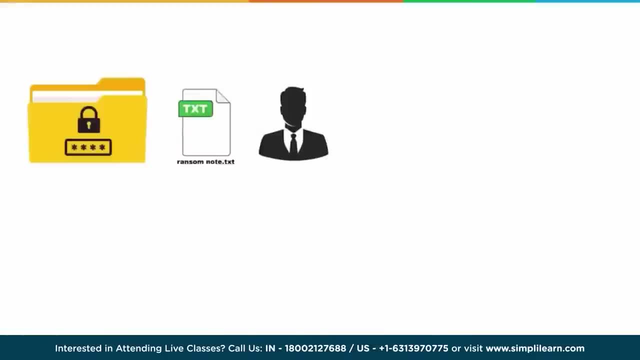 a text file is available to the victim explaining how to make the ransom payment and unlock the files for it, Just like Richard found the Ransom Note text file on his desktop. Even after the money has been paid, there is no guarantee that the hackers will send the decryption key or unlock the files. 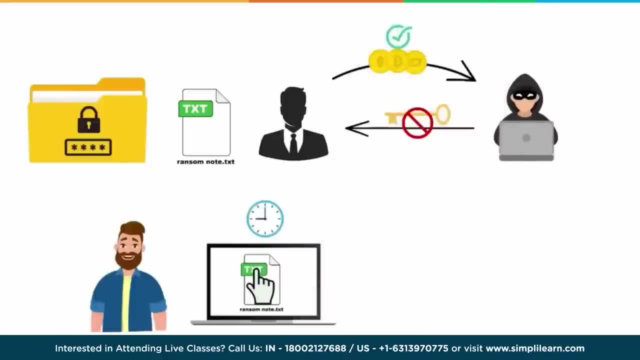 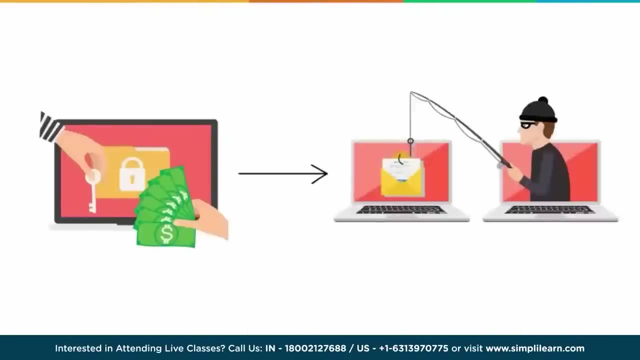 But in certain sensitive situations, victims make the payment, hoping for the best. Having never been introduced to ransomware attacks before, this gave Richard an opportunity to learn more about this and he began his research on the topic. The spread of ransomware mostly starts with phishing attacks. 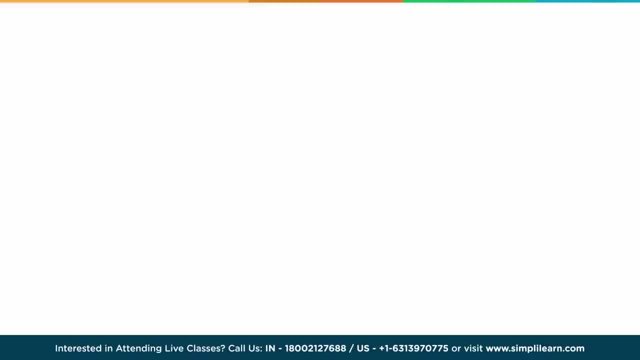 To know more about phishing attacks, click the link in the button above. Users tend to click on unknown links received via emails and chat applications promising rewards of some nature. Once clicked, a ransomware file is installed on the system that encrypts all. 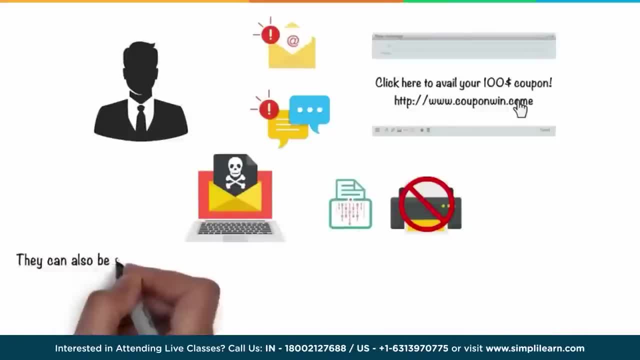 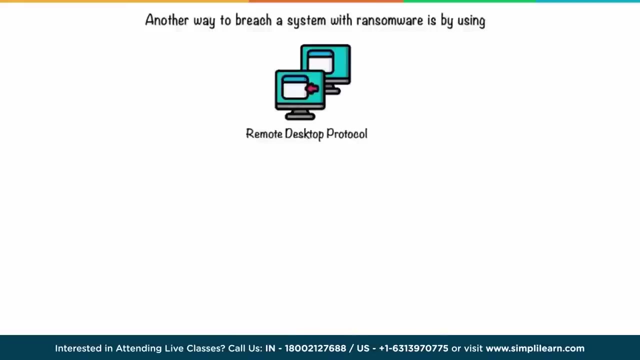 the files or blocks access to computer functions. They can also be spread via malware transmitted via untrusted application installation or even a compromised wireless network. Another way to breach a system with ransomware is by using the Remote Desktop Protocol, or RDP access. 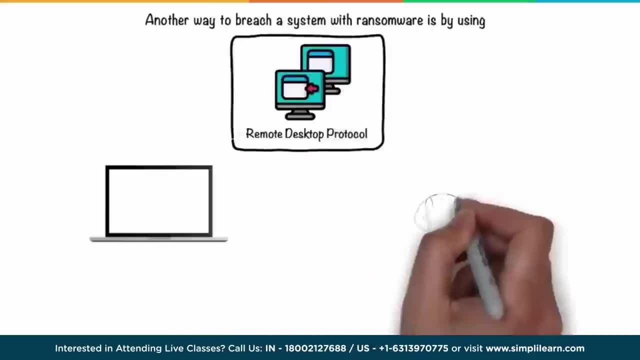 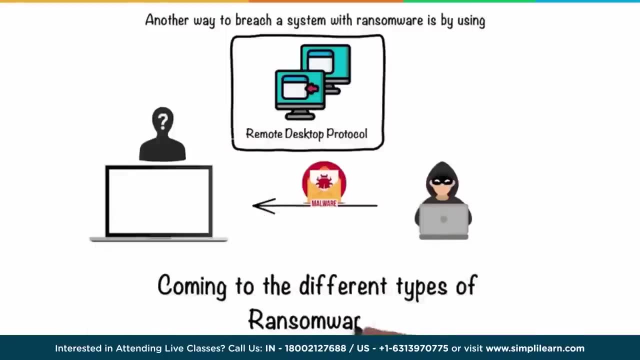 The computer can be accessed remotely using this protocol, Allowing a hacker to install malicious software on the system, with the owner unaware of these developments. Coming to the different types of ransomware, First we have Locker Ransomware, which is a type of malware that blocks standard. 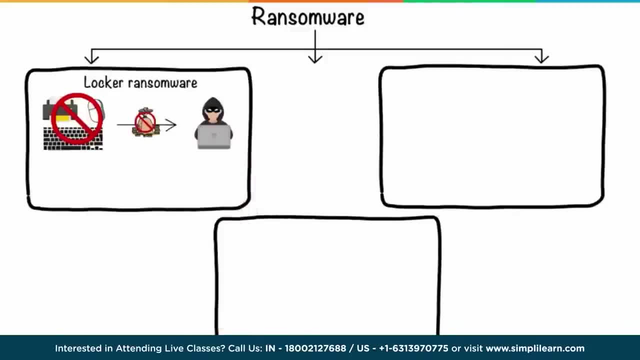 computer functions from being accessed until the payment to the hackers is complete. It shows a lock screen that doesn't allow the victim to use the computer for even basic purposes. Another type is Crypto Ransomware, which encrypts the local files and documents in the computers. 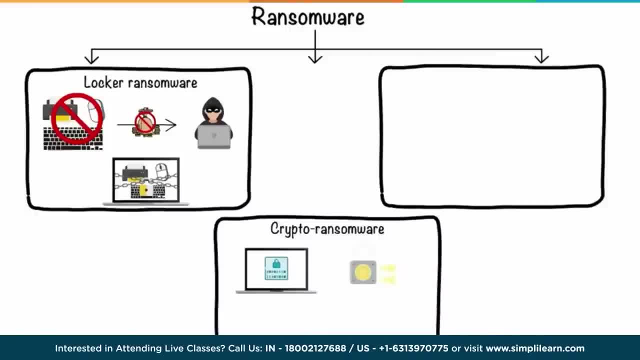 Once the files are encrypted, finding the decryption key is impossible, unless the ransomware variant is old and the keys are already available on the Internet. Scareware is fake software that claims to have detected a virus or other issue on your computer and directs you to pay to resolve the problem. 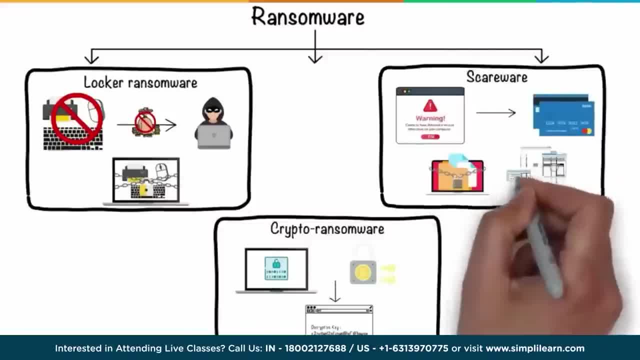 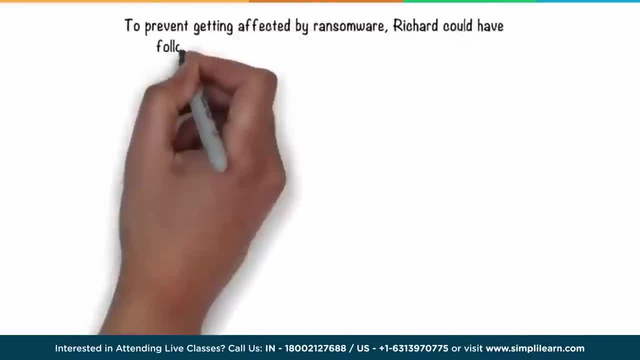 Some types of scareware lock the computer, while others simply flood the screen with pop up alerts without actually damaging files. To prevent getting affected by ransomware, Richard could have followed a few steps to further enhance his security. One must always have backups of their data. 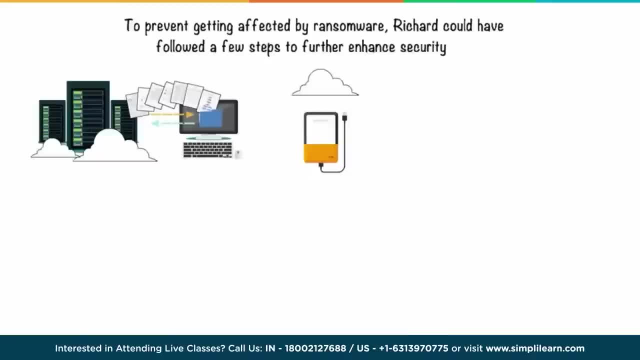 Cloud storage for backup is easy, but a physical backup in a hard drive is always recommended. Keeping the system updated with the latest security patches is always a good idea. Apart from system updates, one must always have reputed antivirus software installed. Many antivirus software like Kaspersky. 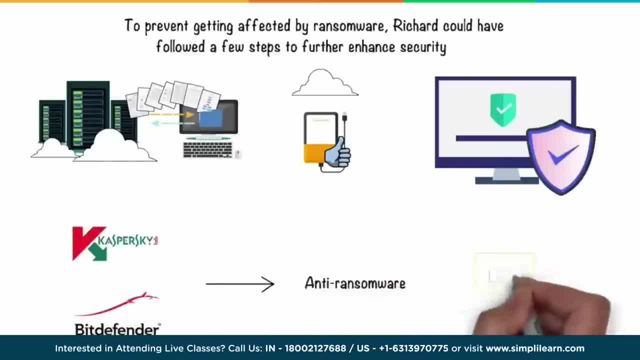 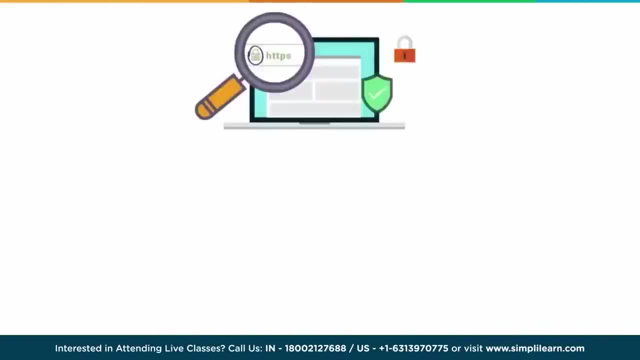 and Bitdefender have anti ransomware features that periodically check for encryption of private documents. when browsing the Internet, A user must always check for the lock symbol on the address bar, which signifies the presence of HTTPS protocol for additional security. If a system is infected with ransomware already, there is a website. 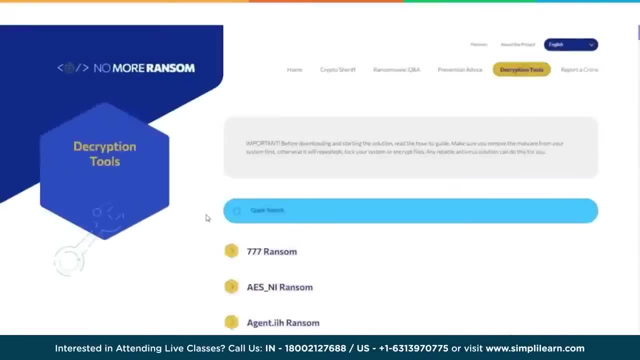 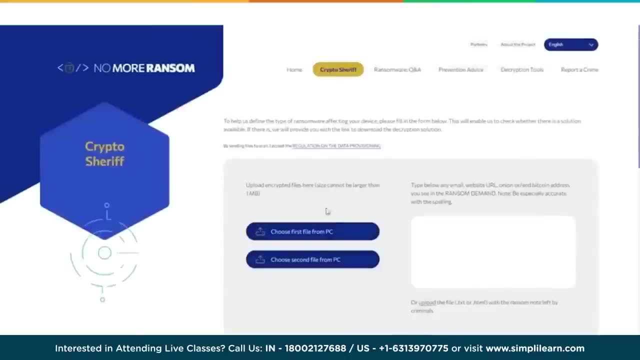 NoMoreRansomorg. It has a collection of decryption tools for most well-known ransomware packages. It can also help decrypt specific encrypted files if the list of anti ransomware tools didn't help the victim. Malware is a malicious software that is. 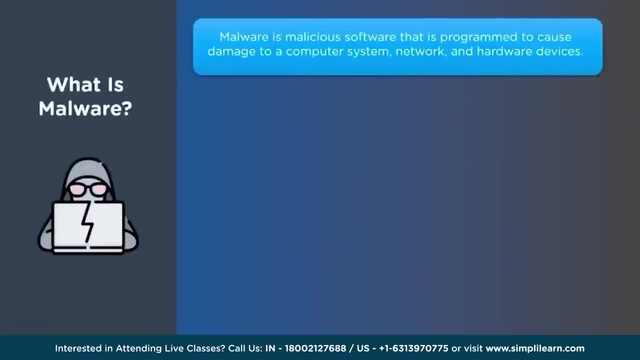 programmed to cause damage to a computer system, network and hardware devices. Many malicious programs, like Trojan viruses, bombs and bots, which cause damage to the system, are known as malware. Most of the malware programs are designed to steal information from the targeted user or to steal money from the target by stealing sensitive data. 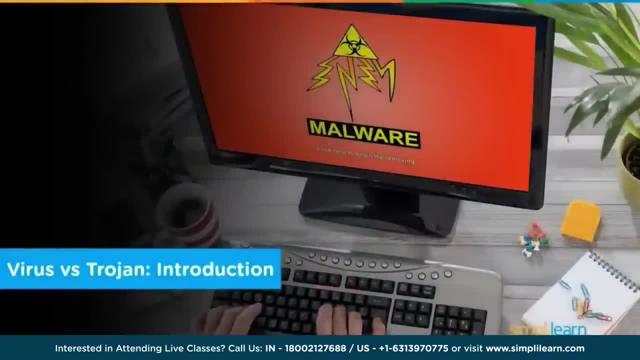 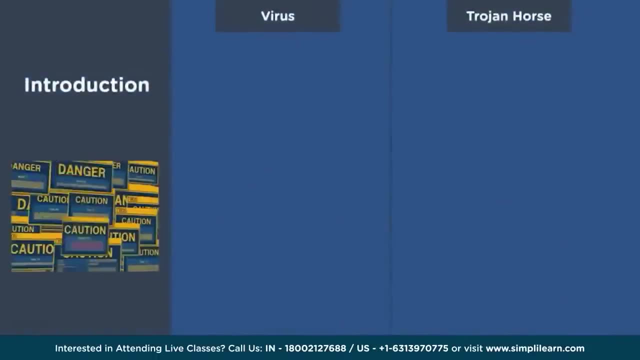 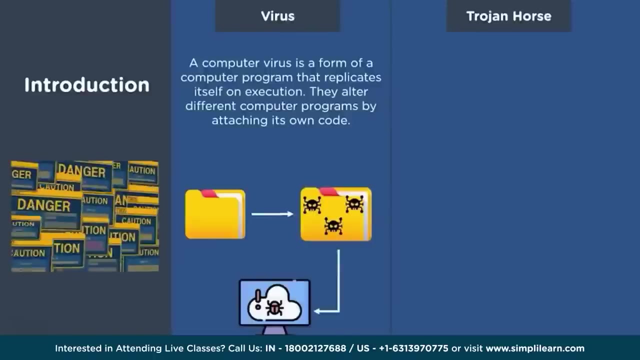 Let's take a look at the introduction for two different types of malware: virus and Trojan. Firstly, let's take a look at what exactly is a virus program. A computer virus is a type of malicious program that, on execution, replicates itself. They get attached to different files. 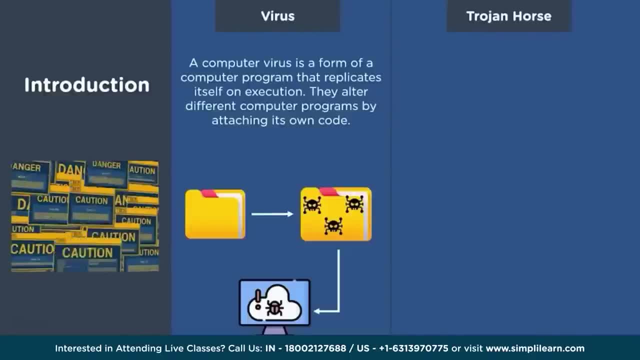 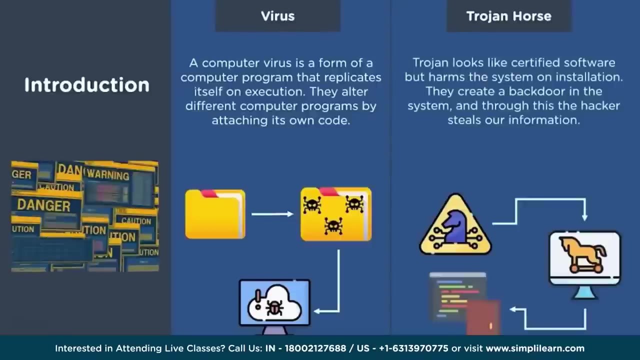 and programs, which are termed as host programs, by inserting their code When the attachment succeeds, the targeted program is termed as infected with a computer virus. Now let's take a look at the Trojan Horse. Trojan Horse program is a program that disguises itself as a legitimate program. 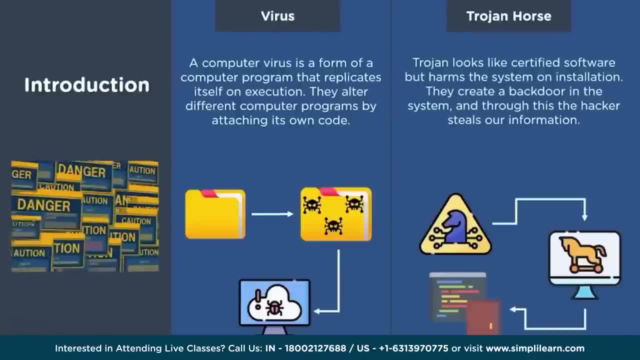 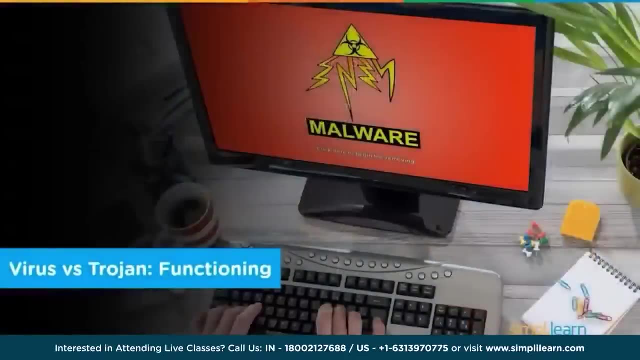 but harms the system on installation. They hide within the attachments and emails, then transfer from one system to another. They create bad doors into a system to allow the cyber criminal to steal our information. Let's take a look how they function after getting installed into a system. 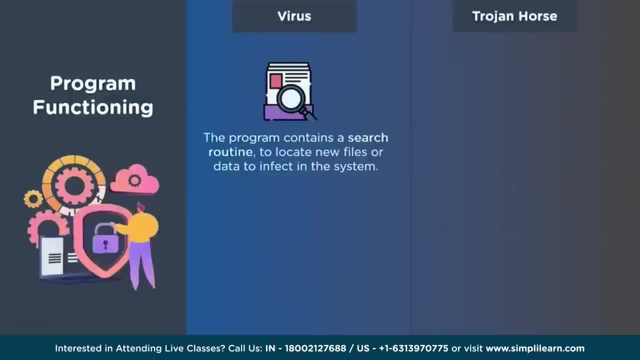 Firstly, we have virus programs. The computer virus must contain two parts to infect the system. First is a search routine which locates new files and data that is to be infected by the virus program, And the second part is known as the copy. 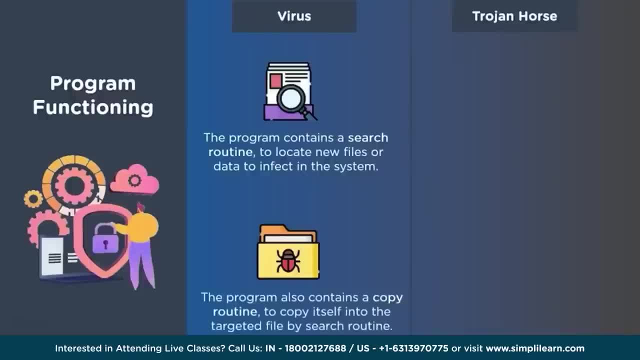 routine, which is necessary for the program to copy itself into the targeted file, which is located by the search routine. Now let's take a look at the Trojan Horse functioning. For Trojan Horses, entryway into our system is through emails that may look: 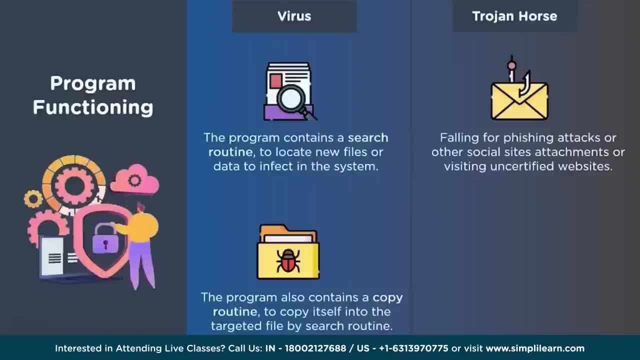 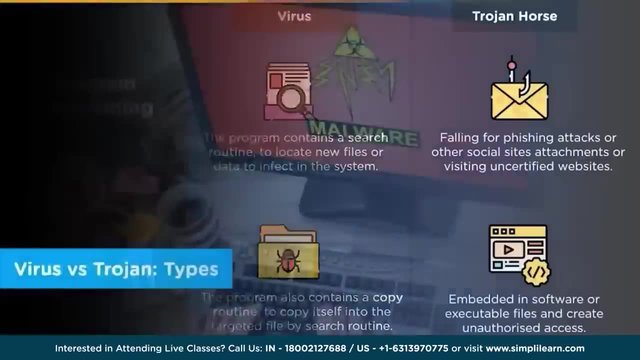 legitimate but may have unknown attachments, And when such files are downloaded into the device, the Trojan program gets installed and infects the system. They also infect the system on the execution of infected application or the executable file and attacks the system. Now that we understand what virus and Trojans are. 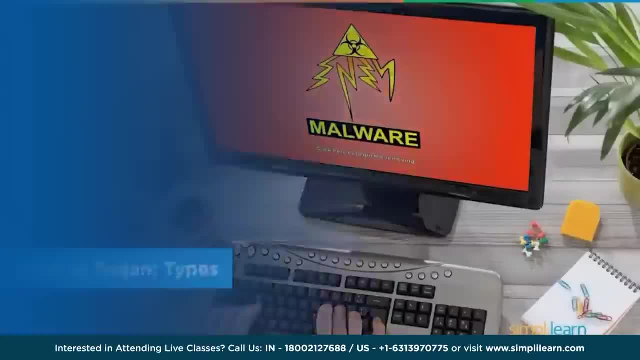 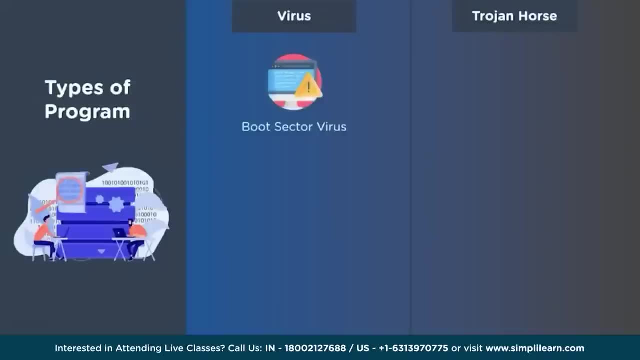 let's understand different types of virus and Trojans. Let's take a look at different types of viruses. The first one is known as the boot sector virus. This type of virus damages the booting section of the system by infecting the master board record, which is also known as MBR. 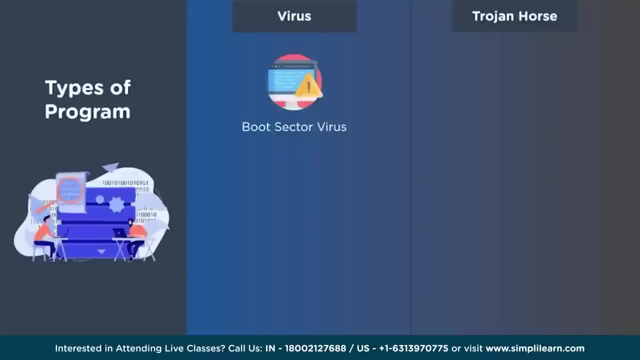 This damages the boot sector section by targeting the hard disk of the system. Then we have the macro virus. Macro virus is a type of virus that gets embedded into the document related data and is executed when the file is open. They also are designed to replicate themselves and infect the system on a larger scale. 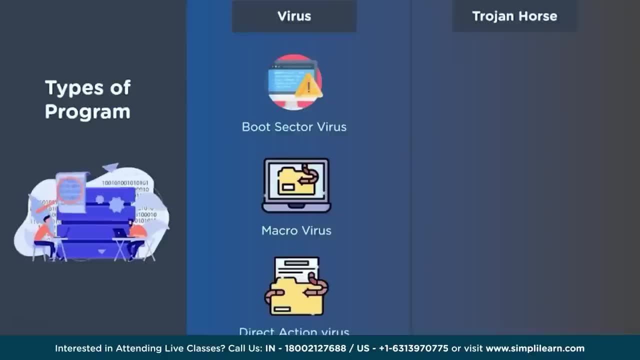 And lastly, we have the direct action virus. This type of virus gets attached to executable files which, on execution, activates the virus program and infects the system. Once the infection of the file is completed, they exit the system, which is also the reason it is known as a non-resident virus. 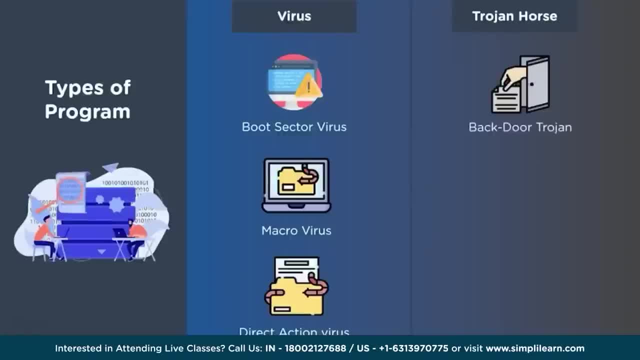 Let's take a look at different types of Trojans. The first type of Trojan is the backdoor Trojan. They are designed to create a backdoor in the system on execution of an infected program. They provide remote access of a system to the hacker. 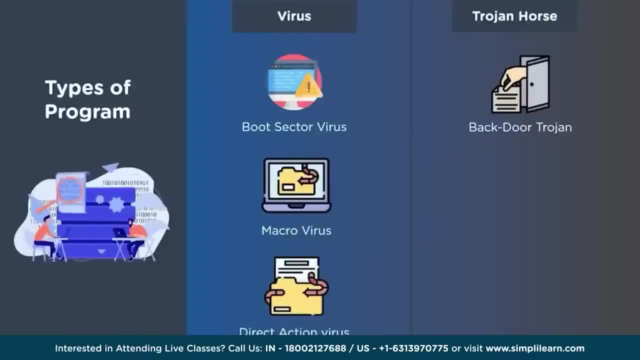 This way, the cybercriminal can steal our system data and may use it for illegal activities. Next we have CrickSource Trojan. They enter the system by clicking the random pop ups which we come across on the Internet. They attempt the user to give their 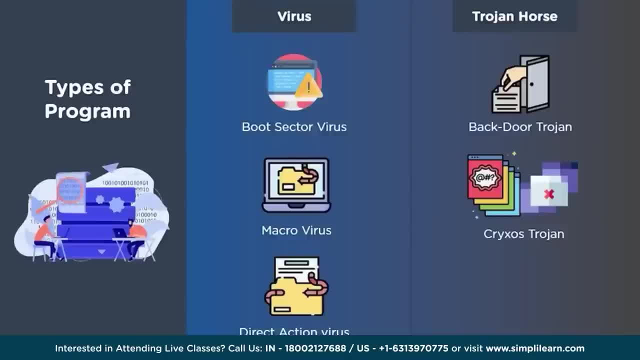 personal details for different transactions or schemes which may provide a remote access of a system to the cybercriminal. And the last Trojan type is Ransom Trojan. This type of Trojan program, after entering the system, blocks the user from accessing its own system and also affects the system function. 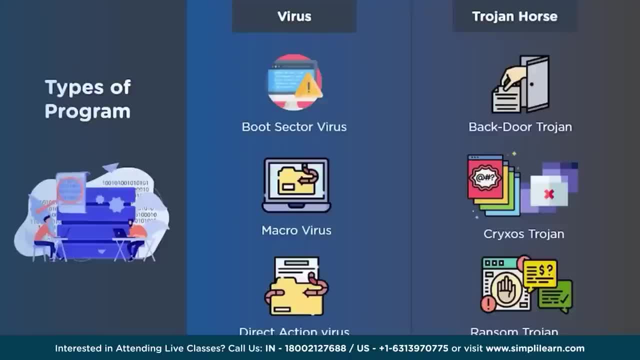 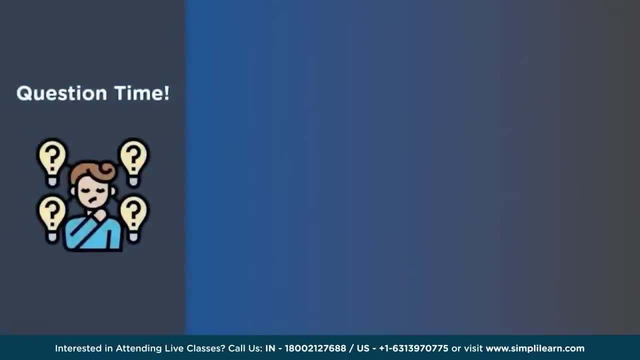 The cybercriminal demands a ransom from the targeted user for the removal of the Trojan program from the device. Now that we understand some details regarding viruses and Trojan, let's solve a question. The question is: Jake was denied access to his system and he 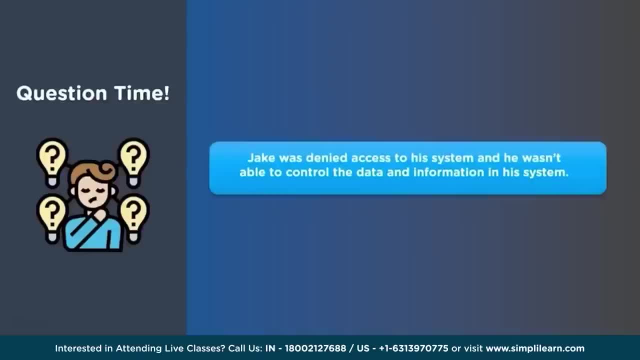 wasn't able to control the data and information in his system. Now the actual question is: what could be the reason behind this system's problem? Option A- Macro virus. Option B- Ransom Trojan. Option C- Backdoor Trojan. 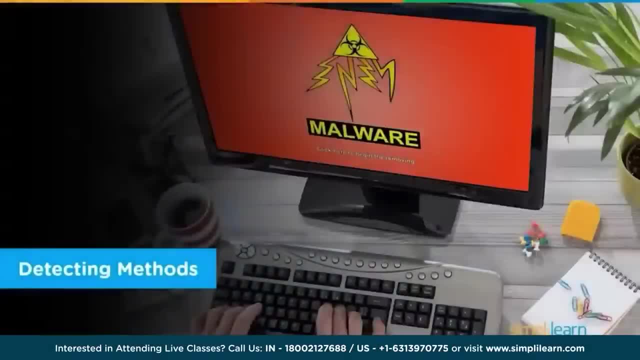 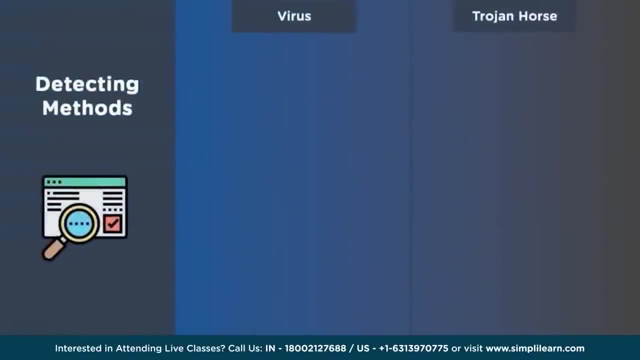 Give your answers in the comments section. Now let's understand how to detect the activity of viruses and Trojan in a system. To detect virus or Trojan activity in a system, we can refer to the following points. For viruses, we have slowing down of the system and frequent application freeze. 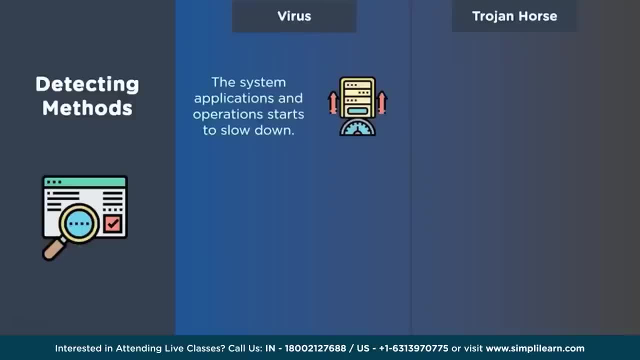 shows that the infection of the virus is present in the system. Then we have: the viruses can also steal sensitive data, including passwords, account details, which may lead to unexpected logout from the accounts or corruption of the sensitive data. And lastly, we have frequent system crashes due to virus infection. 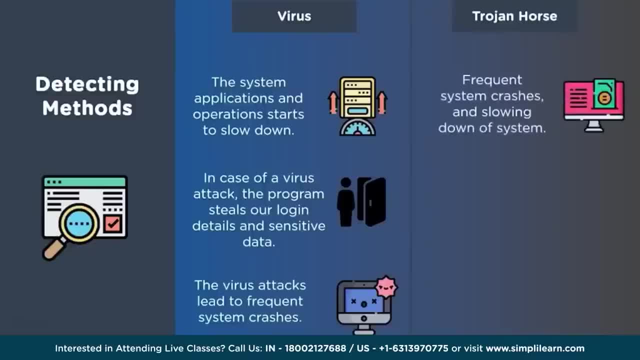 which damages the operating system For Trojan. we have frequent system crashes and system also faces slow reaction time. Then we have there are more random pop ups from the system which may indicate Trojan activity And lastly, we have modification in the system application and change of the desktop. 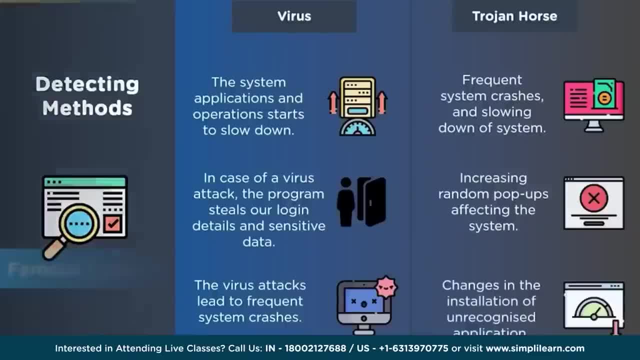 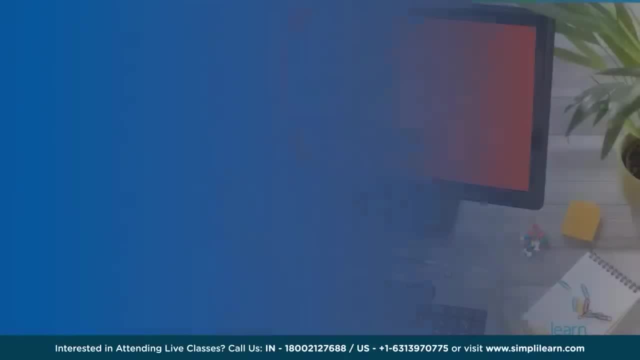 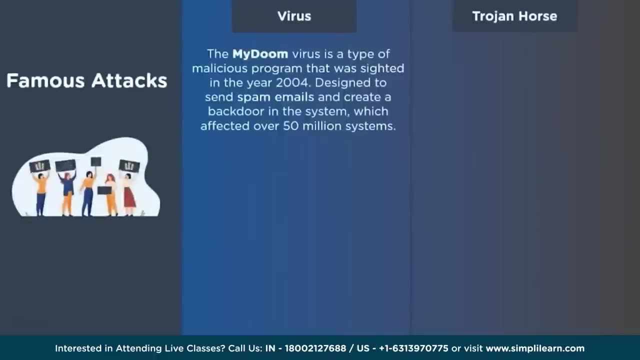 appearance can be also due to the infection of a Trojan program. Next, let's take a look at a famous cyber attack for virus and a Trojan horse For virus. we have the MyDoom virus, which was identified in the year 2004,. 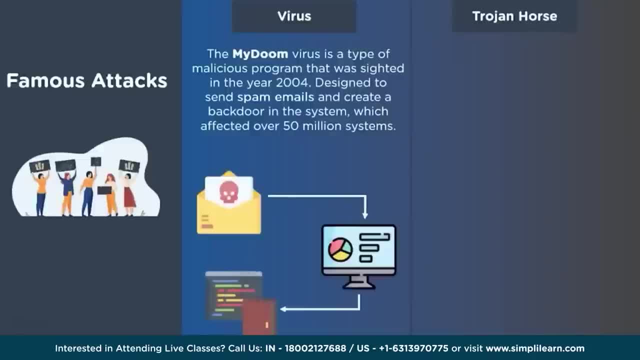 which affected over 50 million systems by creating a network of sending spam emails, which was to gain backdoor access into our systems. Next, for the Trojan horse, we have the Emotat Trojan program, which is a specific designed for financial theft and for stealing bank related information. 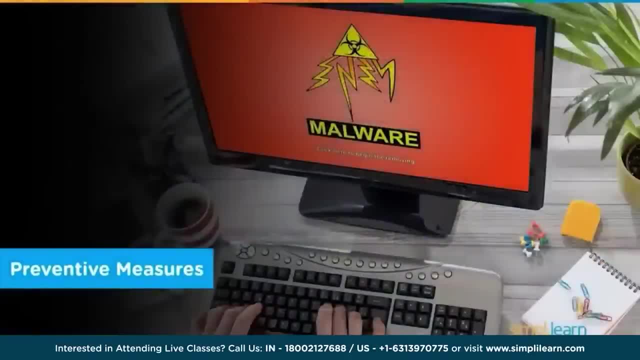 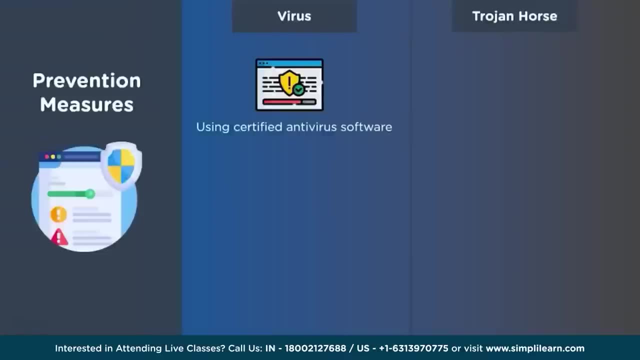 Next we have a few points for how to prevent virus entry or Trojan attack for a system. The most basic way of virus protection is to using antivirus and do regular virus scan. This will prevent virus entry in the system and also having more than one. 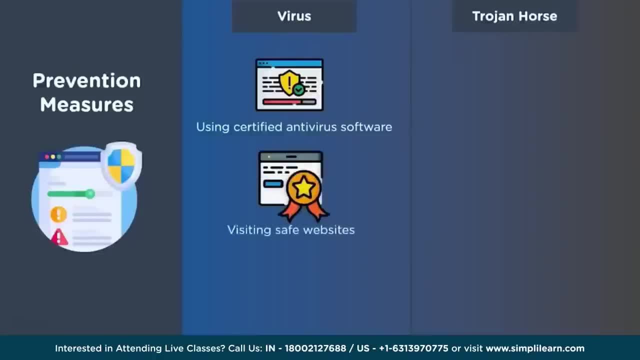 antivirus provides a much better protection. Then avoid visiting uncertified websites can also prevent virus entry into our system. Then we have using regular driver updates and system updates to prevent virus entry For Trojan. we have using certified softwares from legal sites to prevent any Trojan activity in our system. 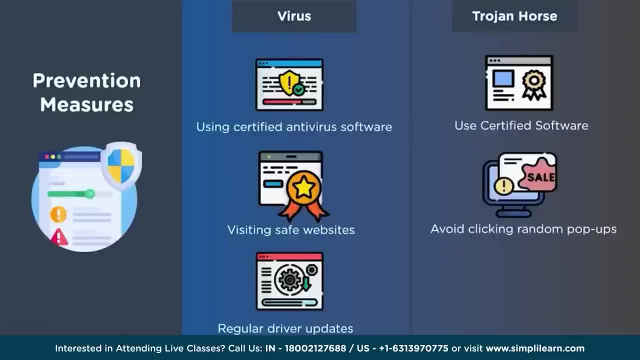 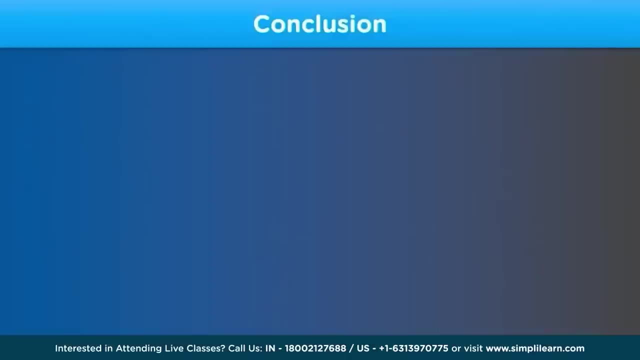 And also avoid clicking random pop ups that we often see on the Internet. And lastly, using antivirus and firewalls for protection against Trojan horses is a good habit. Now that we have reached the end of the video, let's take a look what we learned. 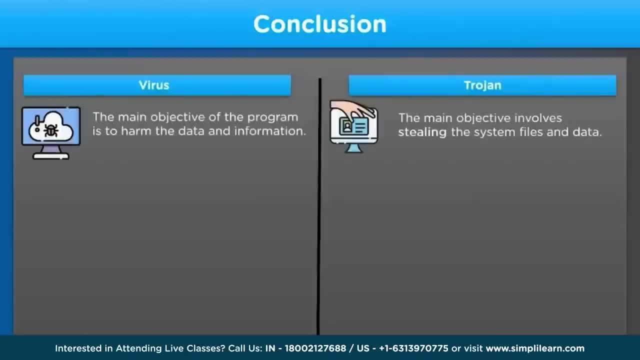 For the first part we saw the main objective of the virus is to harm the data and information in a system, whereas for the Trojan we have stealing of the data files and information. Effect of viruses is more drastic in comparison to the Trojan horses. 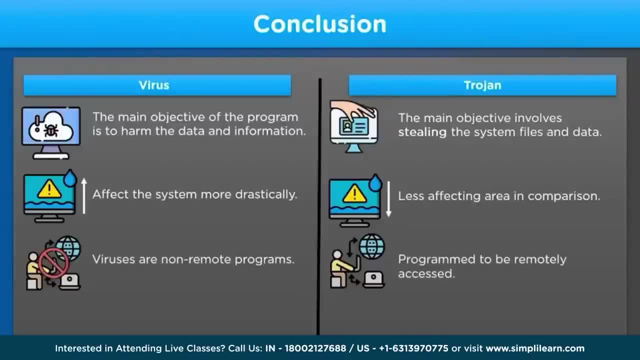 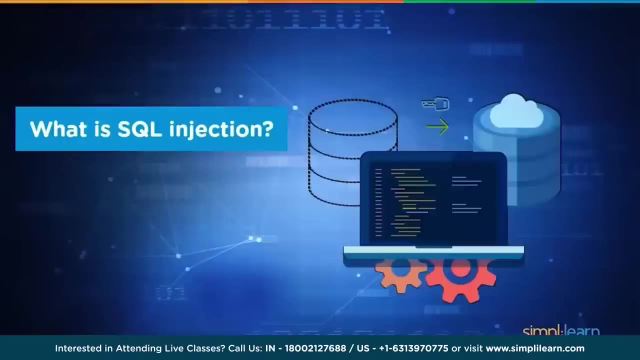 Then we have viruses, which are non-remote programs, whereas Trojan horses are remote accessed. And, lastly, viruses have the ability to replicate itself to harm multiple files, whereas Trojan does not have the replication ability. So let's begin with. what is SQL injection? 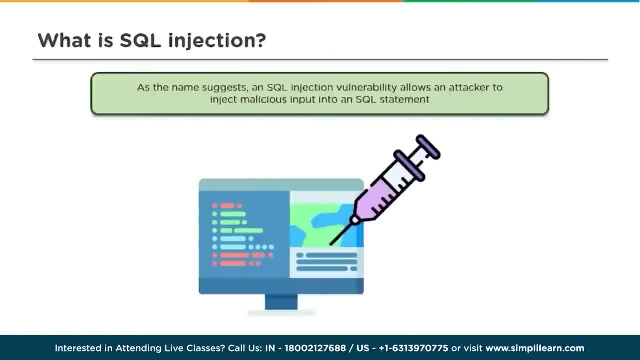 As the name suggests, SQL injection vulnerability allows an attacker to inject malicious input into a SQL statement. So SQL stands for structured query language, which is a language used by an application to interact with a database. Now, normally this attack is targeted towards a database to extract. 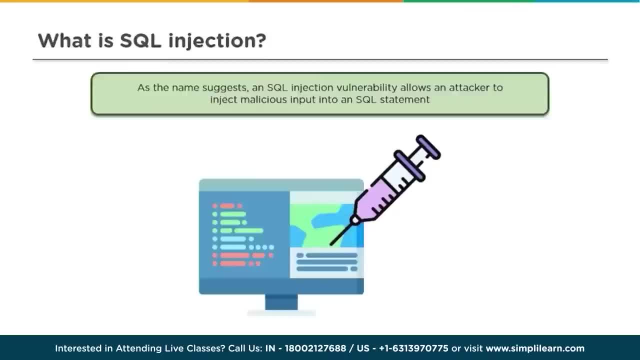 the data that is stored within. However, the vulnerability does not lie in the database itself. The vulnerability will always lie in the application. It is the developer's prerogative of how to develop the application, how to configure it to prevent SQL injection queries from happening. 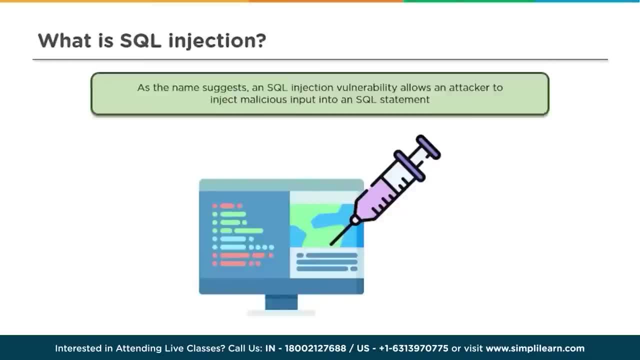 A database is created to answer questions, And if a question is asked it is supposed to answer it. The database needs to be configured for some amount of security, but the vulnerability, the flaw here for SQL injection will always lie in the application itself. It does how the application interacts. 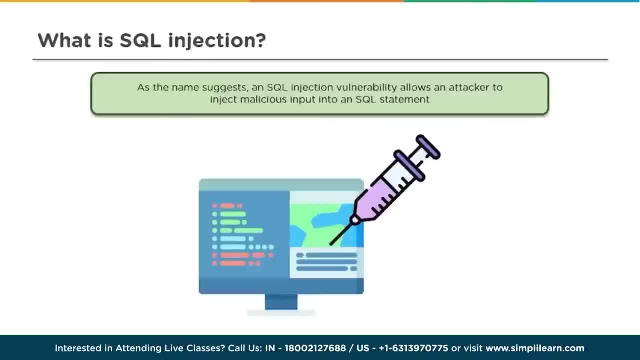 with the database. that needs to be modified, that needs to be maintained by the developer, rather than just configuring the database itself. So the attacker, at this point in time when they send a query to the application, will form a malformed query by injecting a particular command or an operator that 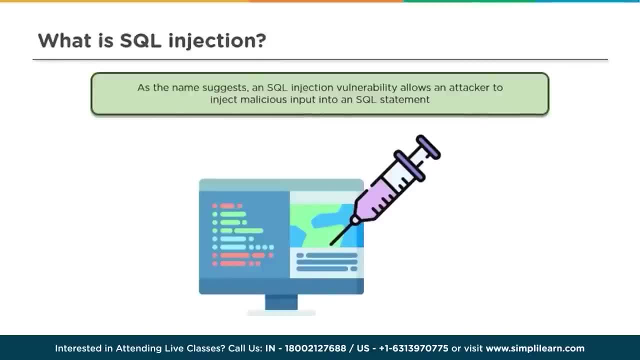 is recognized by the SQL language And if that operator is passed through the application to the database, then the database basically gets cracked or does a data dump because of that unwanted character coming in. So this character needs to be filtered at the application level itself. 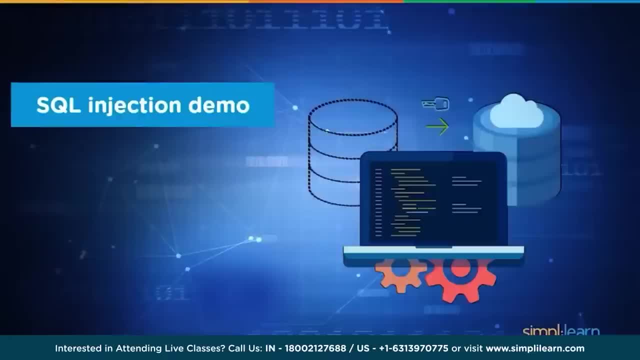 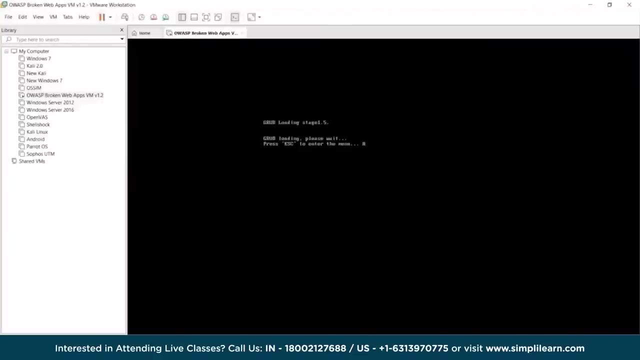 Now let's look at a quick demo. So what we have done here is I have this virtual machine called OWASP, Broken Web Applications Virtual Machine, version 1.2.. I'm going to power this on. Till this power is on, I'm going to show you where we can. 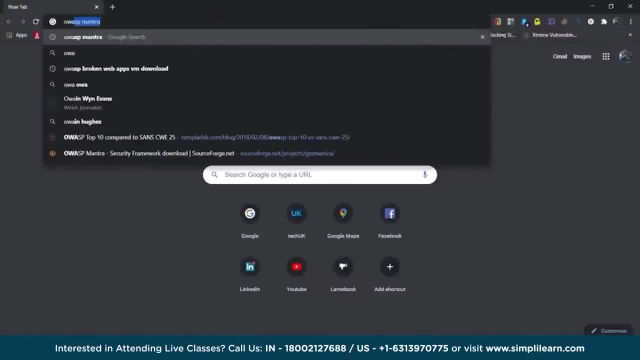 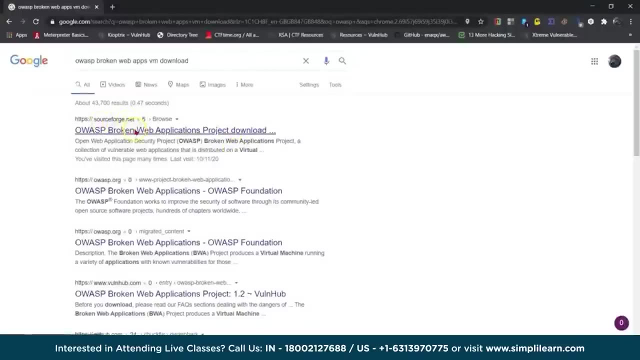 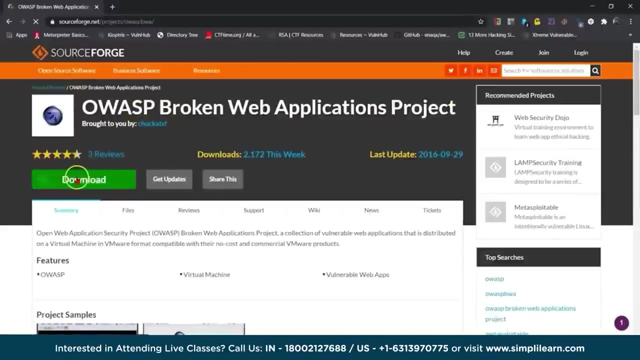 download this utility from. so you can just look for OWASP Broken Web Application Project download. You'll find it on sourceforcenet. Click on the link. You can download the Broken Web Application Project from here. This is a 1.9 GB download and you can have. 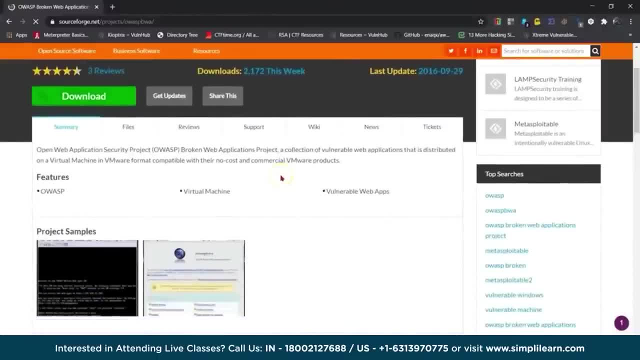 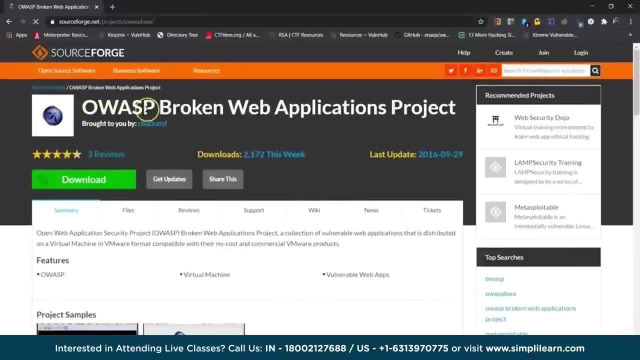 a zip machine directly for VMware or Oracle VirtualBox. Now, this is an application that has been developed by OWASP, which stands for Open Web Application Security Project, which is a not-for-profit organization and periodically releases the most top 10 risks that an application will face for that particular year. 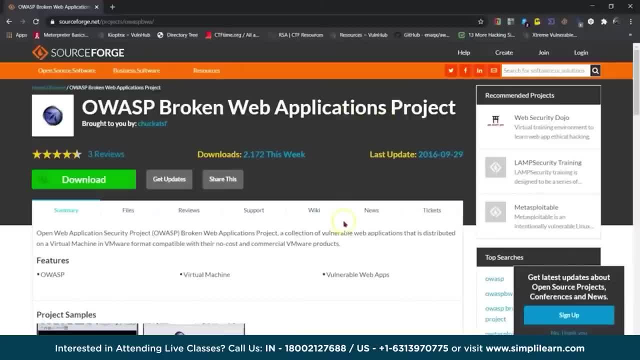 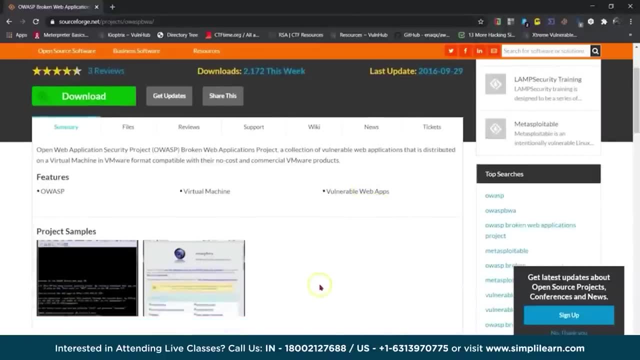 So they have given a web application with inbuilt vulnerabilities, So this is a very good opportunity for professionals like us to practice upon, to develop our skills upon, because doing this in the real world is illegal. I cannot go onto a website to demonstrate how a SQL injection attack works. 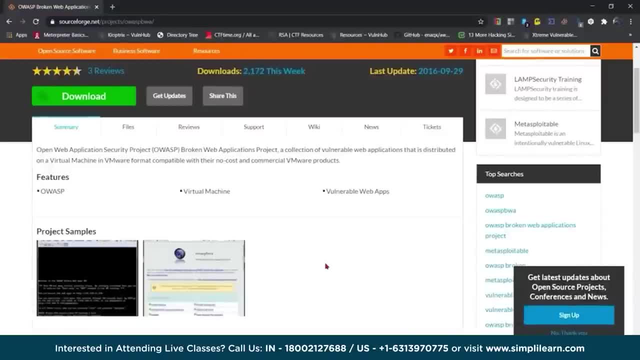 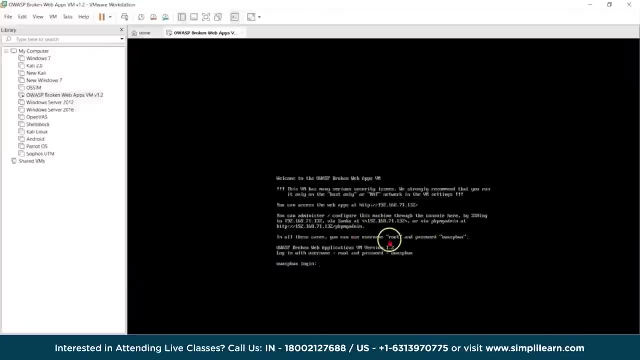 Neither should you try your hands on it till you become very well rehearsed with it. So to upgrade your skills, to upskill yourself, please download this machine hosted in a VMware workstation or Oracle VirtualBox, And then try your skills on it. 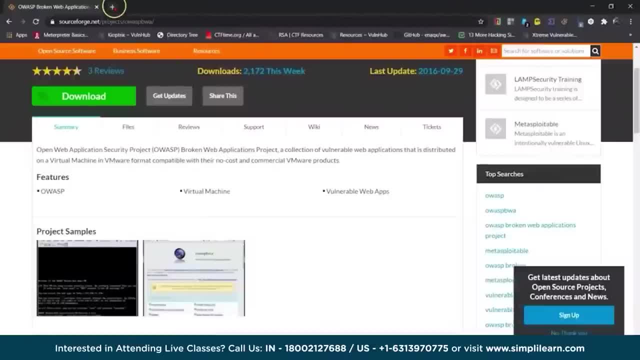 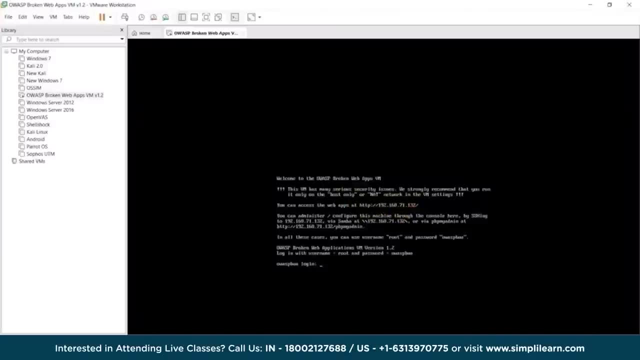 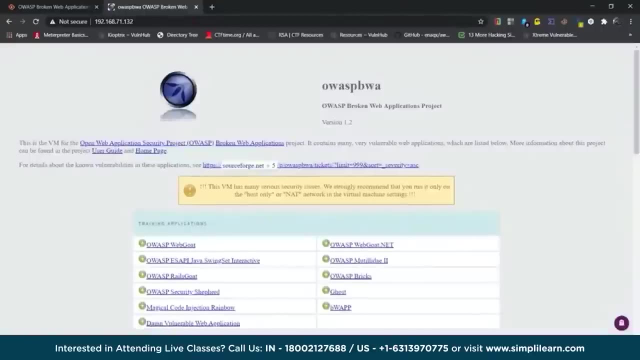 Right. So just going back to the browser here, if I open up a new tab, you will see that this machine has booted up and has an IP address called 71.132.. So if I just go onto that IP address and I type in 192.168.71.132, 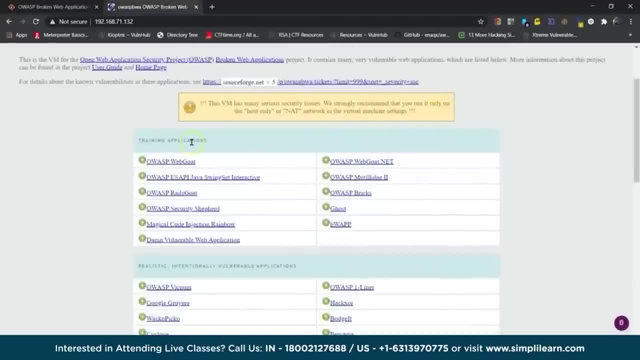 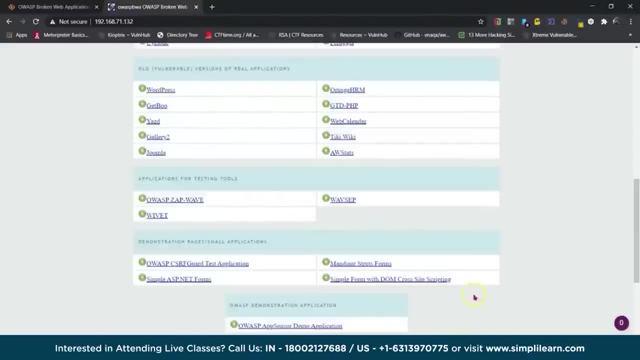 and you'll see the OWASP Broken Web Application Project and there are a lot of training applications, realistic, intentionally vulnerable applications, old versions of real applications and so on so forth. So there is a lot of applications inbuilt over here that you can try your skills upon. 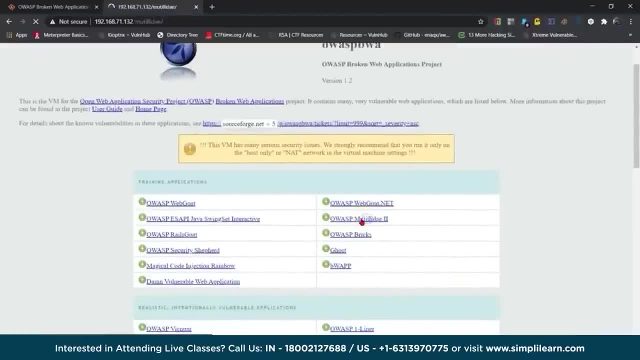 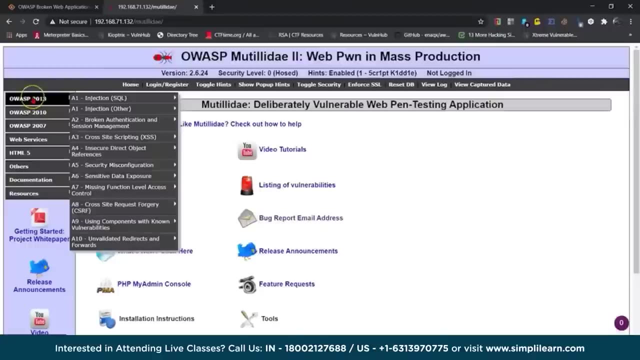 We are going to try to use the OWASP Mutility over here. This gives you the OWASP top 10 risks for 2010,. 2013,. 2017 is the latest one so far, But the difference between 2013 and 2017 is that some of these have changed. 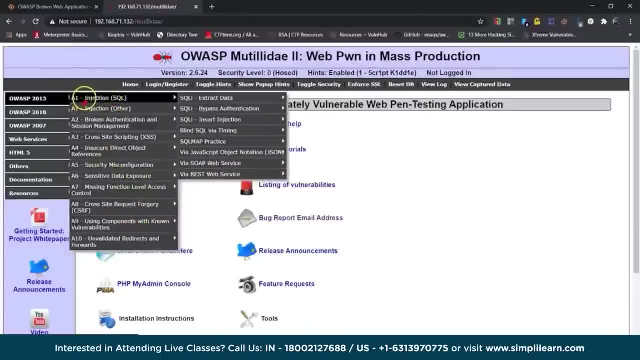 but not all of them. The order has changed a little bit, but you can see that SQL injection is on the top A1 amongst the injection attacks Right, And you can see there are multiple types that have been given here: The SQL injection for extracting data or SQL injection for bypass authentication. 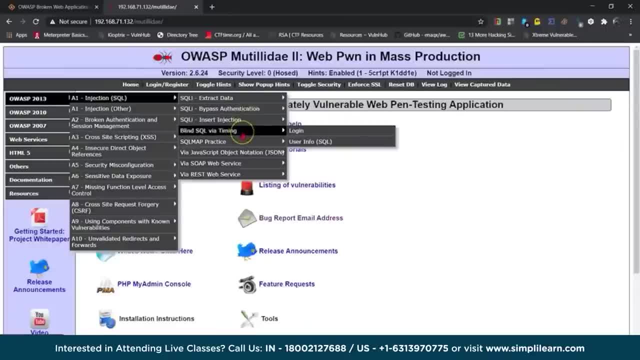 or insert your injection attacks, blind SQL injection. And then there is a tool called SQL Map which is available freely on your Linux machines- Kali Linux or Parrot Linux, whichever you want to use for your practice targets, And so on, so forth. 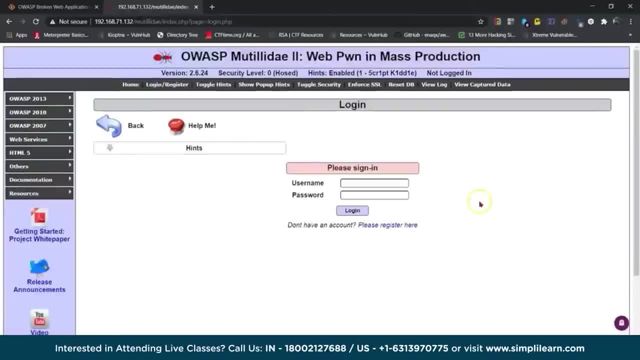 So if I just take you here for bypass authentication- and this is a regular login page that an application may have, Right, You look at a username, you look at a password, You type that in and you log in. So let's say, I don't know a password here. 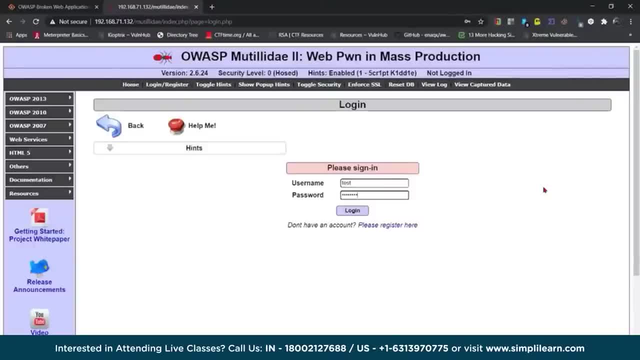 I'm just going to type in a username. test Password is P-A-S-S-W-O-R-D. I try to log in and it shows me that the account does not exist. So the authentication mechanism does work. I did try typing a username and password. 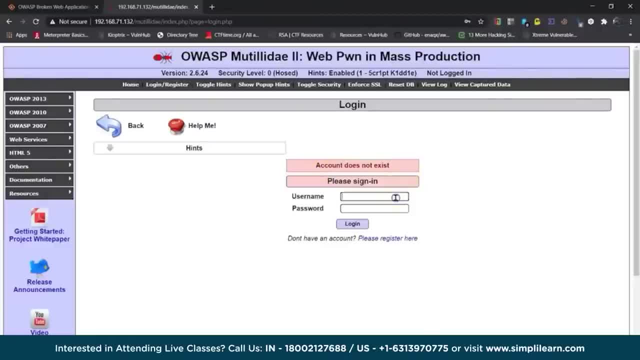 It doesn't recognize that the account does not exist. Now let's try to type in a SQL query here. I'm going to just give it a single quote- which is an operator that is recognized by the SQL language which, when the database tries to execute, will cause the database to 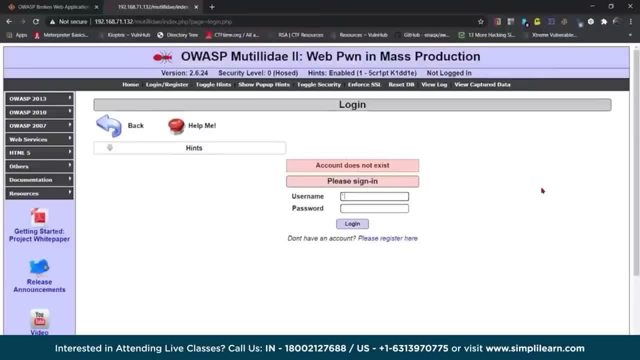 dump some data or to bypass authentication, in this case. And I'm going to give it a condition: single quote Or one equals one. So I'm going to type in, I'm going to say I am logged in using your URL space, hyphen, hyphen space, and I'm going to click on login. 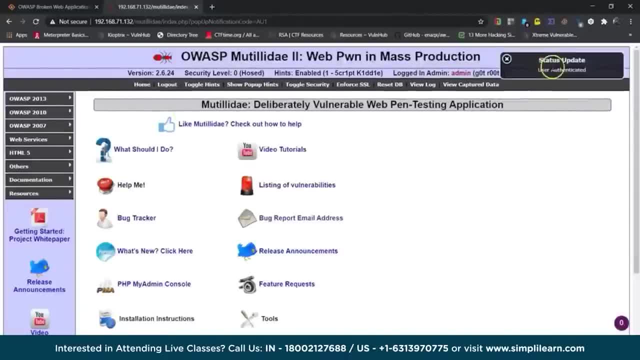 Now, right now I'm not logged in at all And we tried our username and password and we weren't able to log in. So now, if I log in, you will see that it give me a state, a status update, saying the user has been authenticated and I'm. 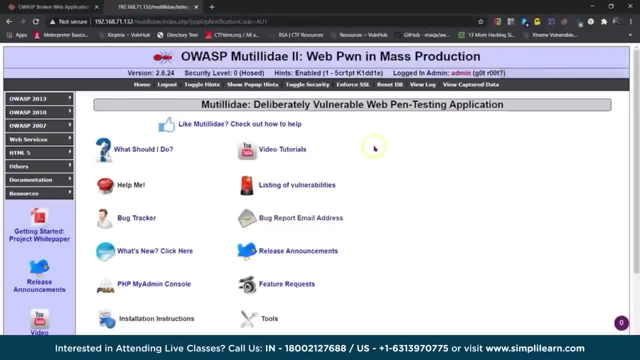 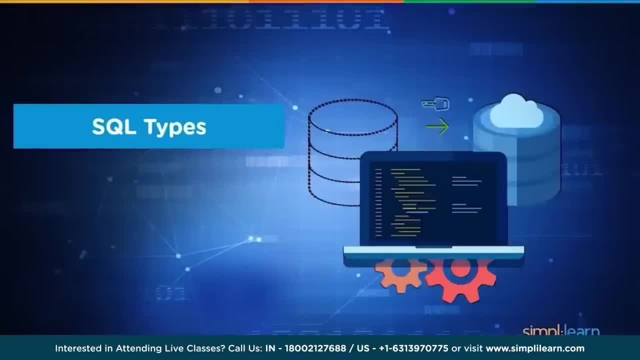 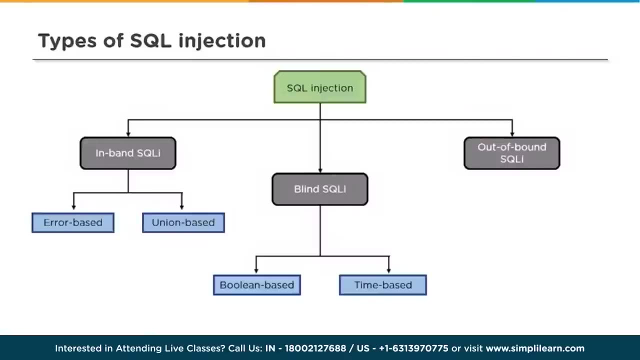 logged in as admin got root. so that is what these SQL queries can achieve. I'm going to log out right now. injection. So looking at that small demo, now let's look at what types of SQL injections are available. So the first is in-band SQL injection. There are two subtypes within in-band error-based. 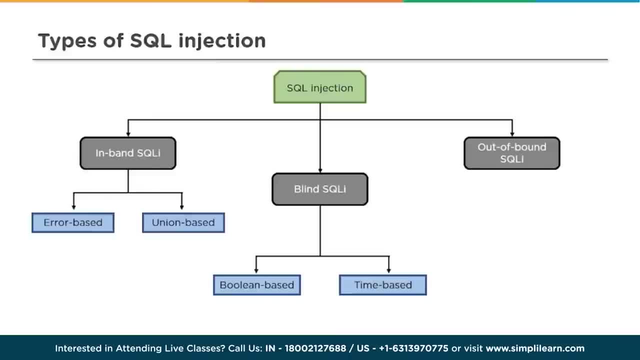 injection attack and a union-based injection attack. The second type is blind SQL injection attack, where there's a Boolean-based and a time-based attack, And the third one is out-of-bound SQL injection attack. Now, what is in-band SQL injection attack? In-band is where we are either. 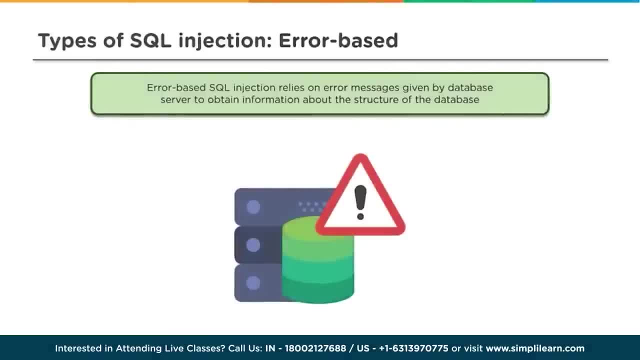 attempting the error-based or the union-based. What is error-based? We send a query to the database, we craft a query to the database and it generates an error message. and it dumps the error message right in front of us on the screen. That makes us realize that there is a flaw and 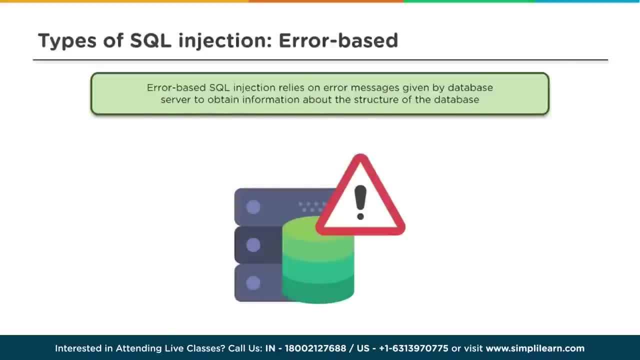 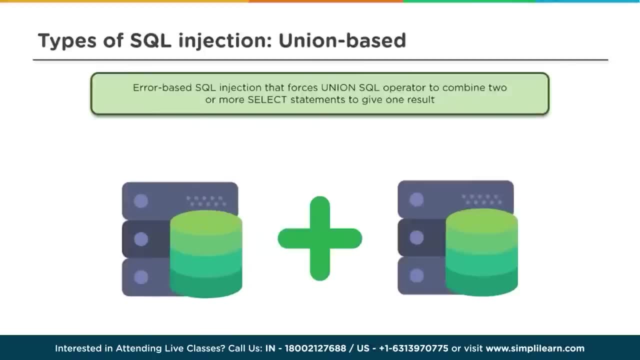 there is some information that is dumped on the screen which we can then further utilize to craft our further queries as we go ahead. Whereas union-based is, it is where we combine multiple statements at the same time. So if you look at the URL earlier in the URL you would see a large structure. in that URL We can try to add more. 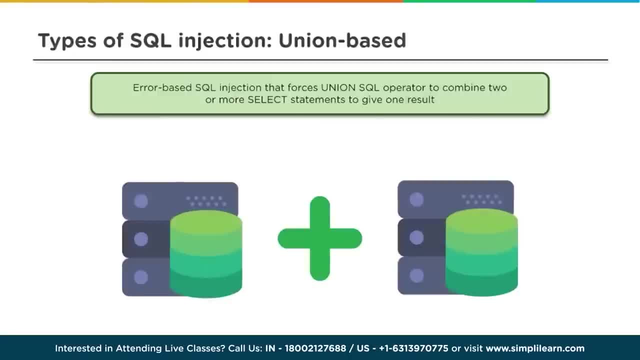 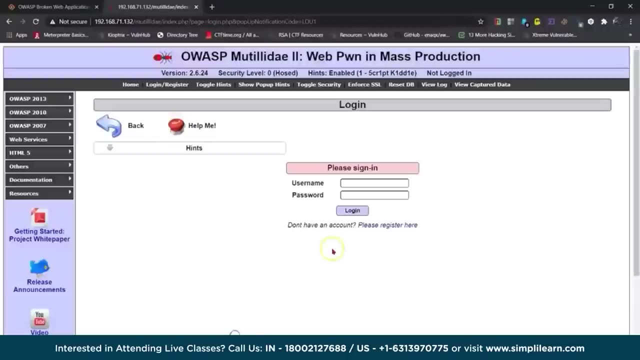 two or more statements within the URL itself, to combine them and then confuse the database into executing both the statements together and giving a data dump at the same time, right? So what would an error-based SQL injection look like? If I go back to the same database, which is here, right, And if you remember the username, 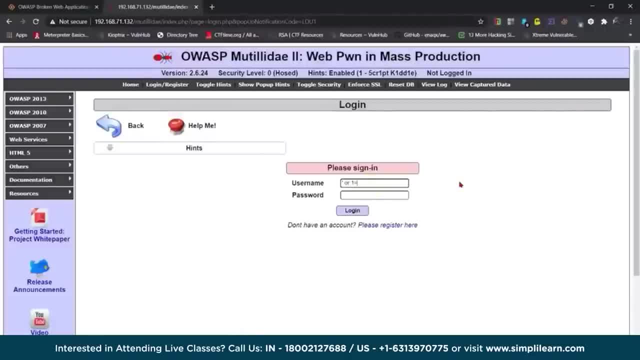 we gave it a single quote, or one equals one space, hyphen, hyphen, space. We gave it the condition right. So basically what it did was a single quote is an operator that goes to the database, selects the default table in the user tables in this database column and then compares it. 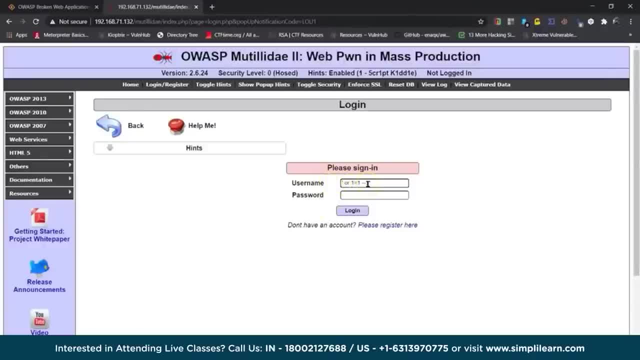 to the condition that is given. So the condition that we gave was one equals one, which is always true. So what it did was it selected the default user table that was available in the database And, instead of comparing it to a password, it compared it to. 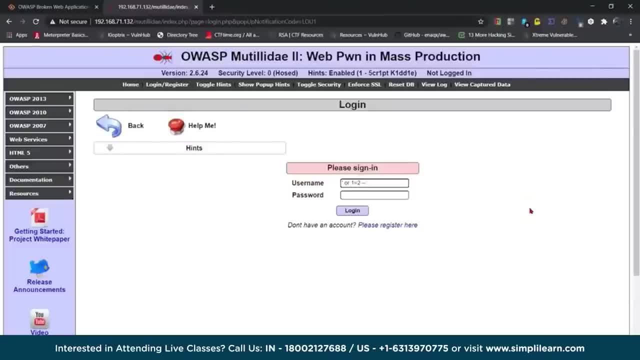 the condition. So if I give it one equals two. where the condition is false, and if I log in, you will see that the account doesn't exist- comes back again because the condition was false And instead of comparing the user account to the password, it basically compared the user account to. 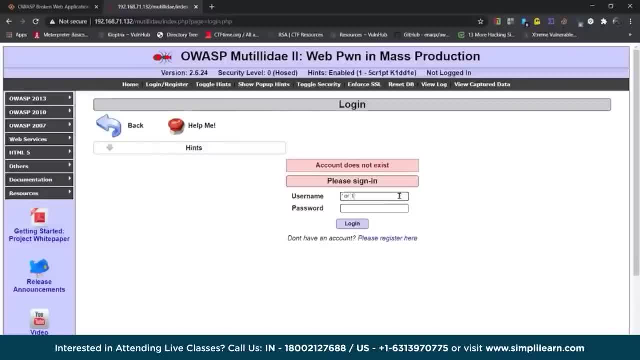 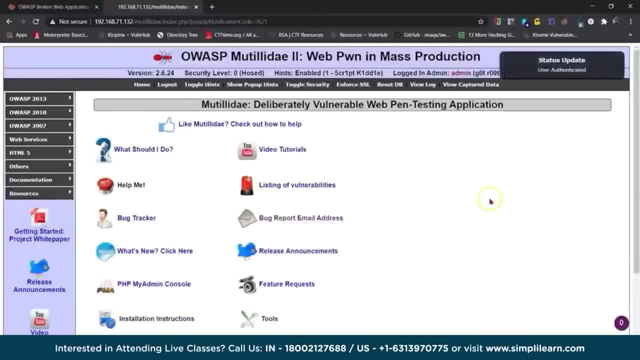 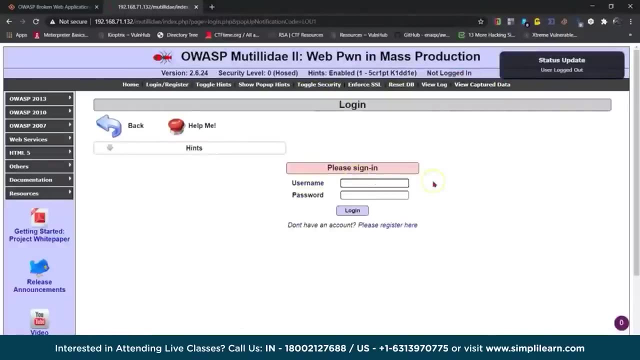 the condition. So if I give it a single quote, or one equals one hyphen, hyphen space, and log in, you can see that this is a correct condition and thus we are able to log in Now, before we even go to that extent, if I just forget the condition over here and I just give it a single quote. 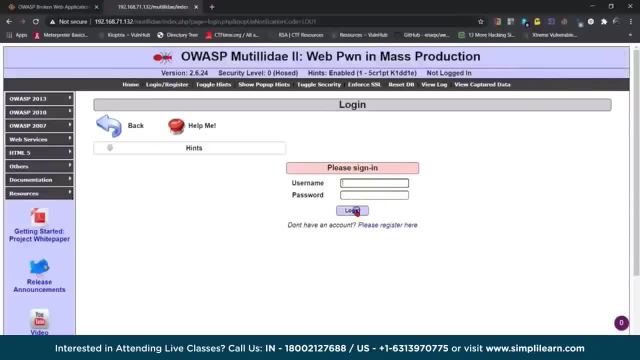 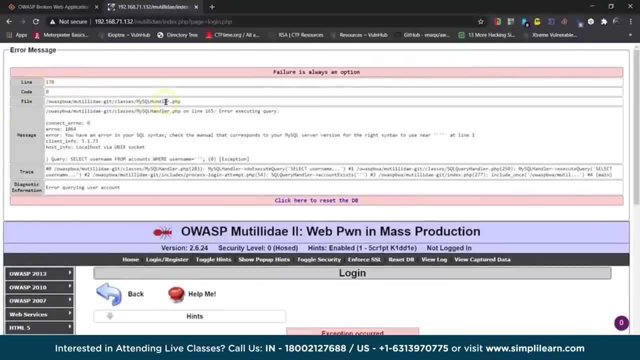 the operator and I send this operator to the database and I click on log in. you will see that it generates an error, which is right on top, And it tells us the line, the file, the error happened And you can see it happened in the MySQL handlerphp file, right, And then it. 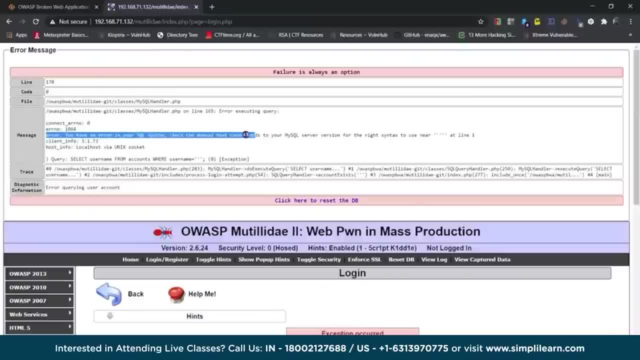 gives us the message you have an error in your SQL syntax. check the manual that corresponds to your MySQL server version for the right syntax to use. Now why would a hacker want to do this in the first place? Because there are different types of databases. So there is a MySQL, MS SQL. 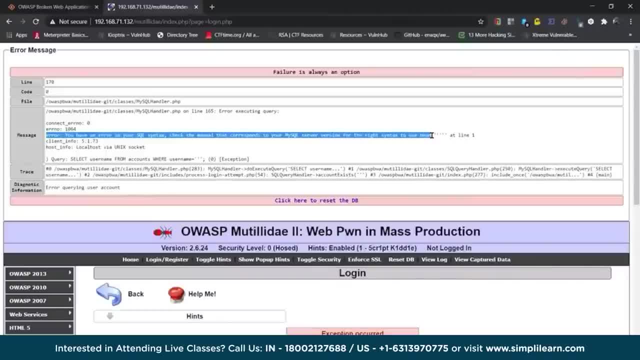 or Microsoft SQL, Oracle SQL, IBM, DB2,. all of these are variations of the SQL database. They use the SQL language. However, every database has its own command right. They have their own syntax. they have their own specific commands that are utilized for the database. 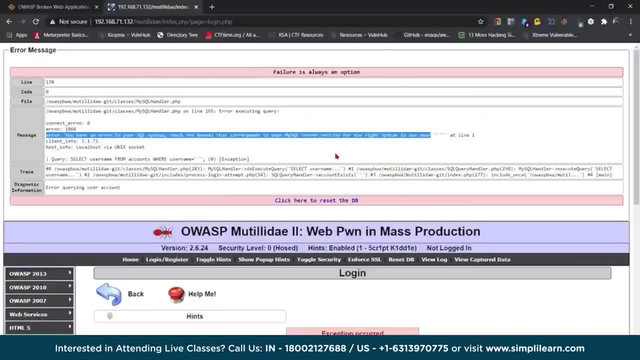 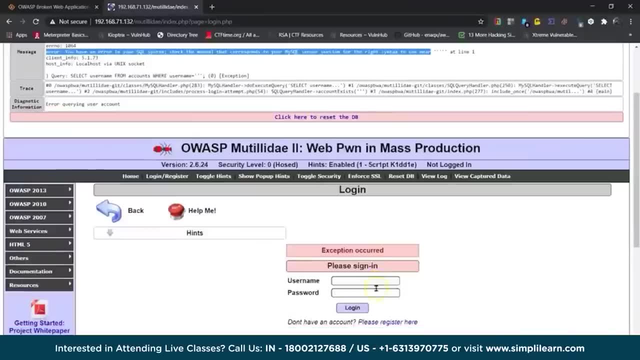 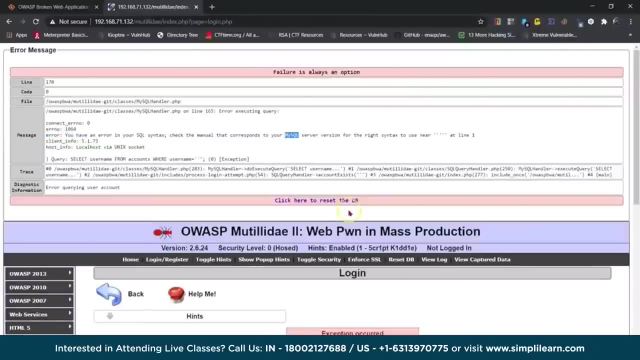 So in this scenario, the hacker wants to identify what database is being currently utilized so they can craft those particular queries. So now, with this injection, with just me sending the quote and the error getting generated, I now come to know that we are using a MySQL server. 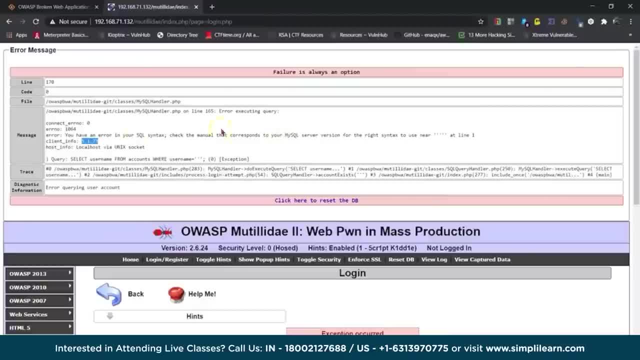 and the version of that server is 5.1.73, and the rest of the information about where the handlers are located and so on, so forth. right, This gives the information to the hacker of how they want to proceed next, what kind of queries they want to create, what kind of syntax they. 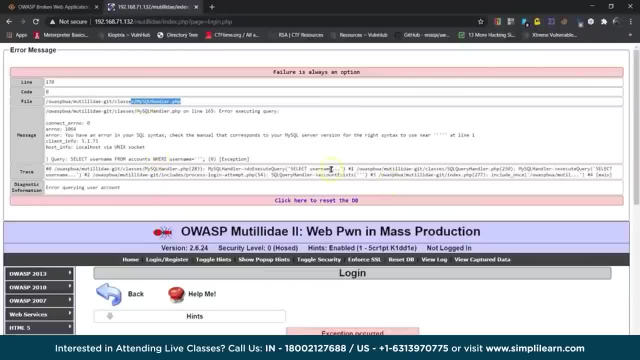 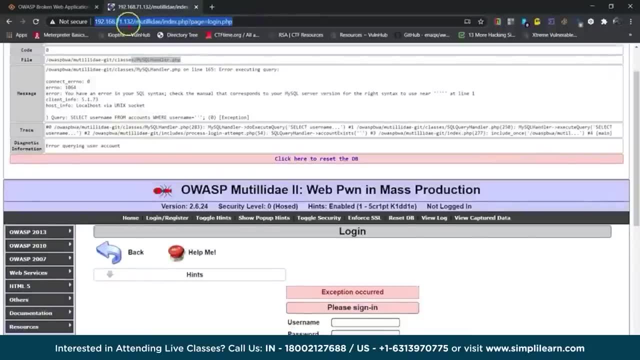 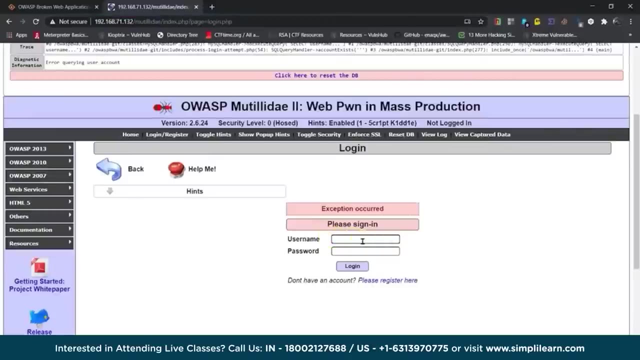 want to utilize. So error-based attack is where you generate these kind of errors and you get this information. The union base is where you craft your queries within the URL and you can try to combine multiple statements within the input fields and try to generate a. 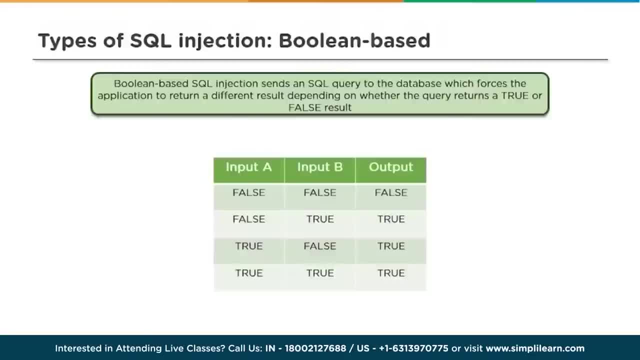 response from that. Then we come to Boolean-based SQL injection. It sends a SQL query to the database which forces the application to return a different result depending on whether the query returns a true or a false result. So basically, if the input is false, 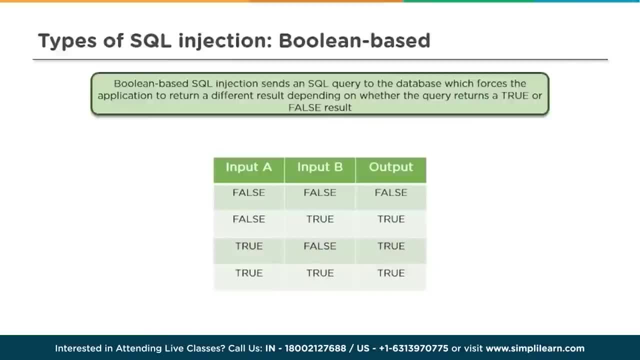 both the inputs are false, the output would be false. There's one input that is false, the other is true- input b- the output would be true, and so on, so forth. right, so depending on the result from the inputs, the attacker will come to know which input is true. with this, he can then access the. 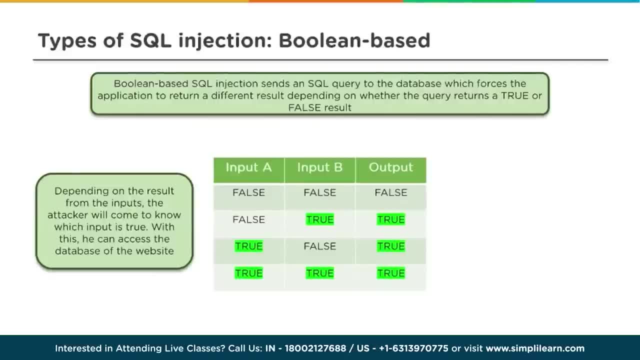 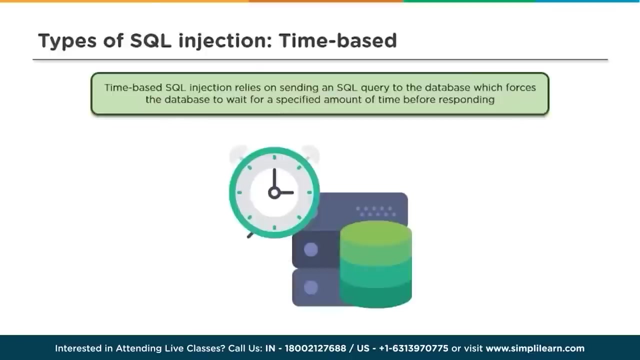 database of the website. so you're trying to figure out by sending out multiple inputs and then analyzing the output to see what exactly which command exactly worked. what was the resultant output of that command? thus, from this kind of an information, the hacker can infer their next step forward. then you have time-based SQL injections. now there are times when a database 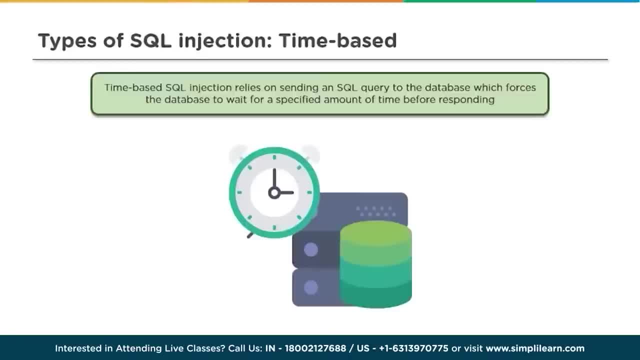 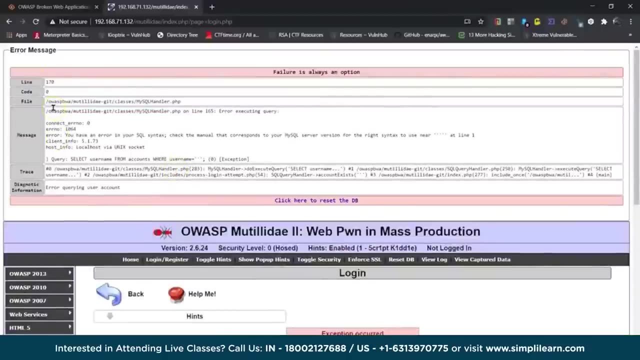 administrator or an application administrator has done some security configuration and does have disabled verbose error messages. now, what is a verbose error message? the error message that we saw right here is a verbose error message. that means that the message gives out details. the message gives out details about what the database is. 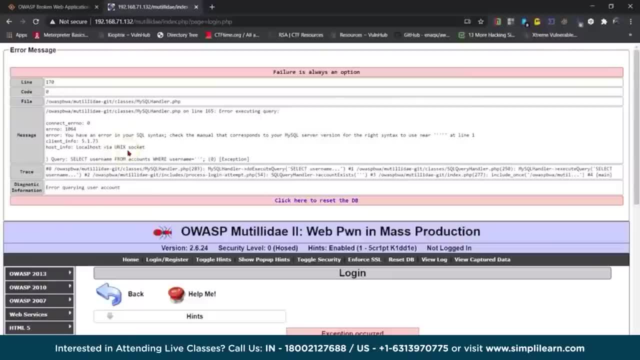 you're not exactly sure of what you're actually doing, and so on and so forth. right? so this the version, and whatnot? so if they have sanitized these errors and you no longer can generate these errors and thus you cannot figure out what database is, then what do you do? right? 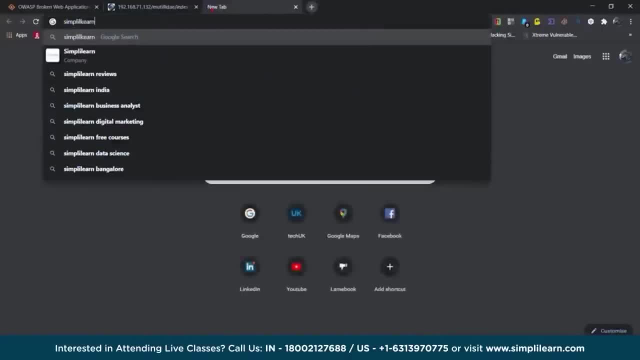 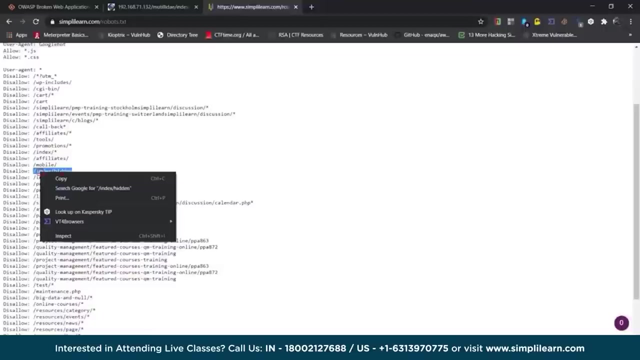 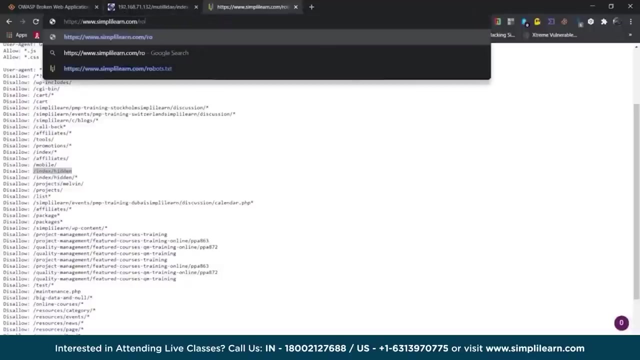 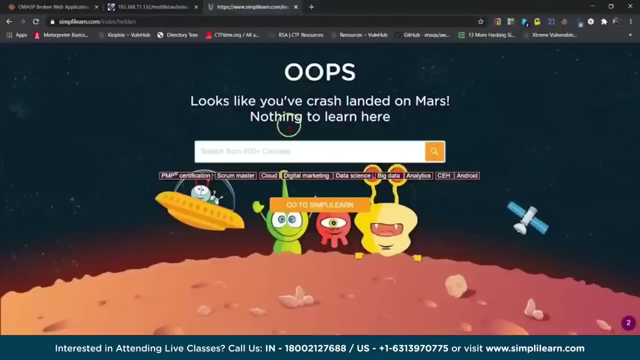 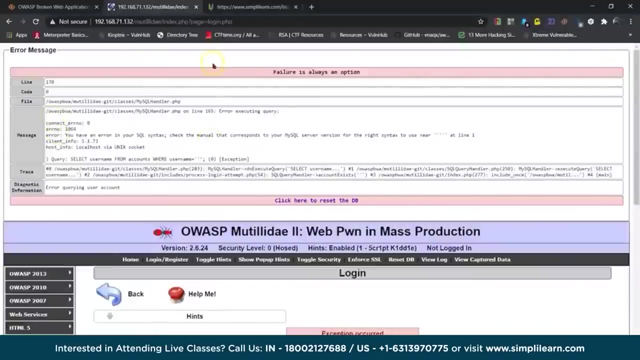 for example, if I just take you to simply learn and take you to a URL that is supposedly not accessible, you can see that that gives a generic error: oops layer, it looks like you have crash landed on March. it doesn't give you a verbose error that we saw here. so this gives us a detail error of what went wrong where it gives us. 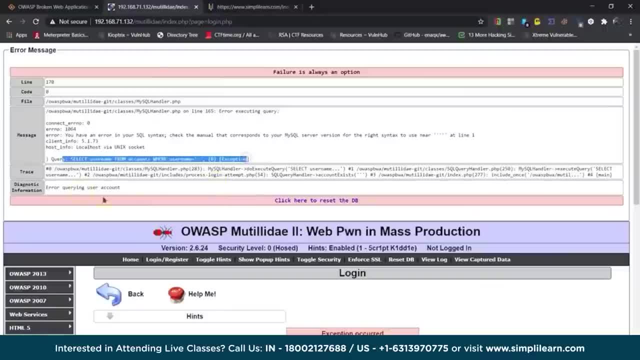 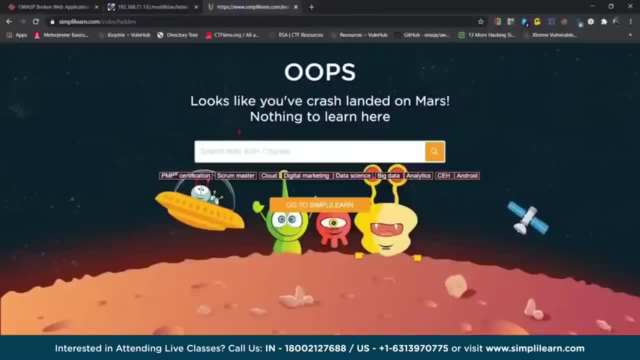 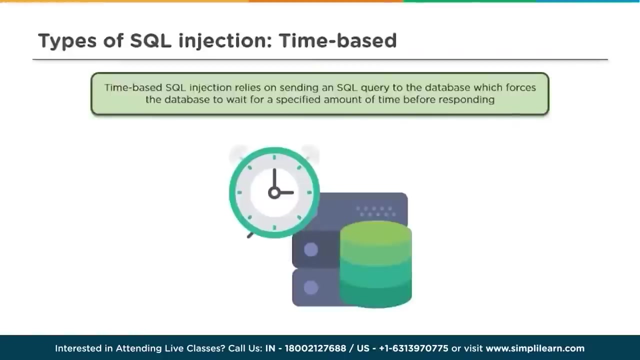 the database, the version of the database and where the query went wrong, and etc. etc. so you can see that it doesn't generate a error. it just get a generic page in front of you. so in that case, what does a hacker do? so the hacker then injects a time-based query in 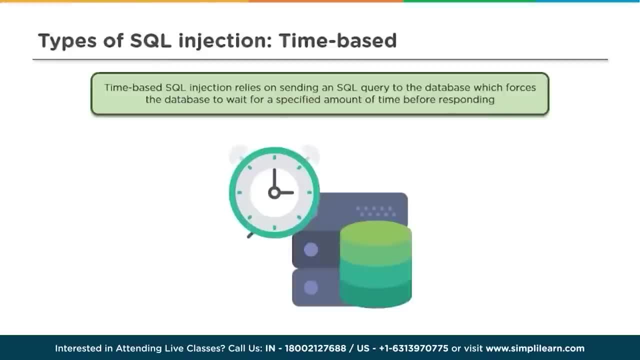 the URL which allows us to verify whether the command is being executed or not. so we put in a time wait, let's say 10 seconds of time wait. so if we, the moment we inject the query, if the query times for 10 seconds and then gets executed, that means that the SQL injection is possible. however, if we inject the query, 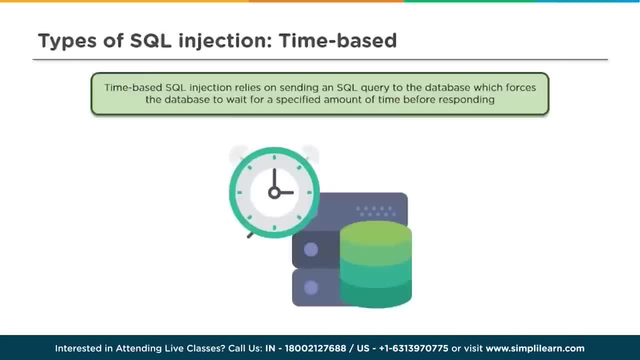 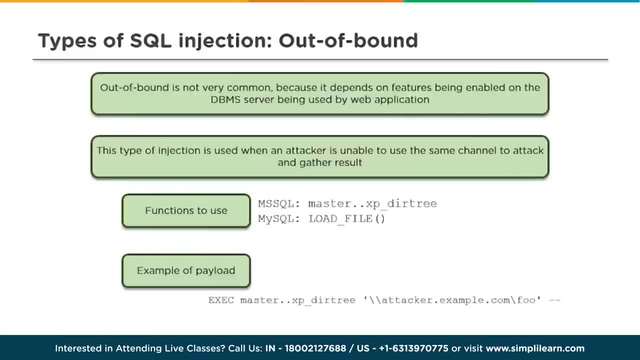 and it just gets executed without the delay. that means that the time injection attack would not be possible on that particular site. out of bound is not a very common attack. it depends on the features being enabled on the database management system that is being used by the web application. 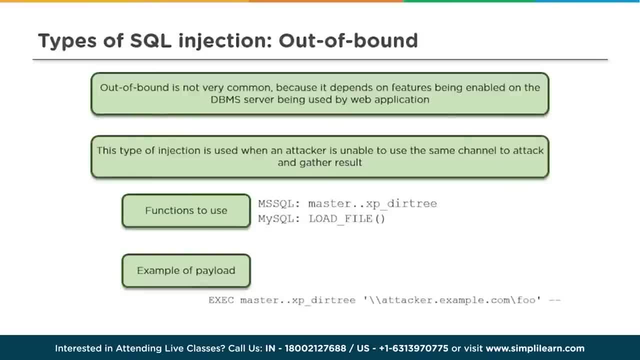 So this can be a somewhat of a misconfiguration error by the database administrator, where you have enabled functions and not sanitized them. so you have not done in access controls properly, you have not given account control. so queries should never be executed at an administrative level. they should always be executed at a user level with minimum privileges. 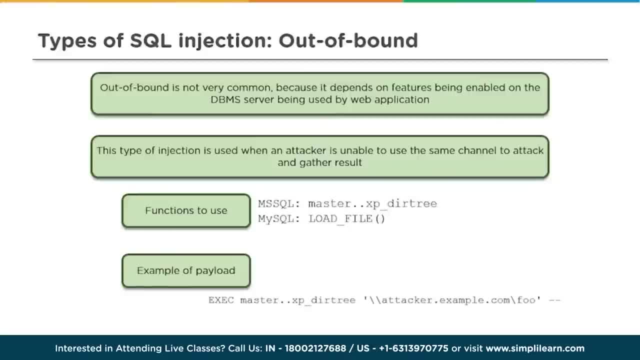 that are required for that query to be executed. now, if you're allowing these kind of functions to be to be enabled at the DBMS and there is an administrative account that can have access to them, at that point in time an out-of-bound injection attack is possible. so let's look at 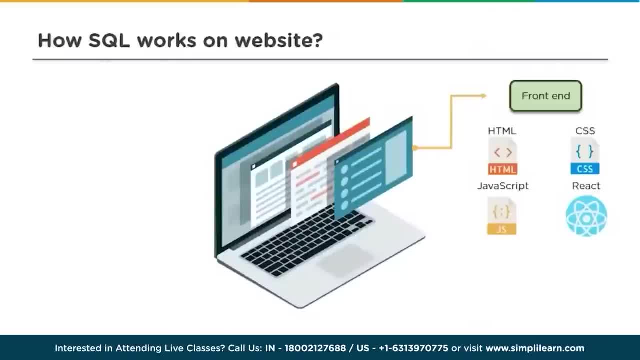 how a website works, right, how SQL works on a website. now the website is constructed of HTML hypertext markup language, which would include javascripting for functionality, cascading style sheets for the mapping of the website, right, and then the reactjs and whatnot, and then the. 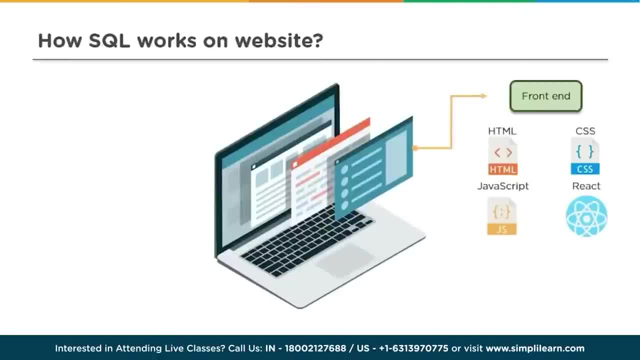 application itself would be automatically generated to the website, which is not for further functionality. now, when we send a query to the website, it is normally using the HTTP protocol or HTTPS protocol. when the query reaches the application, the application would then go ahead and generate the SQL query At the client side. you'll have all these scripting languages coming. 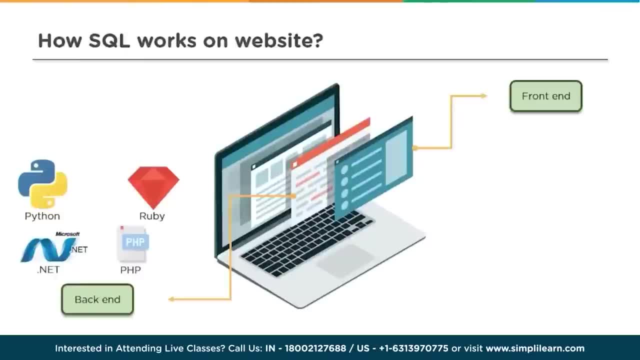 in on the front end that we can utilize to craft queries and then send them across. at the server you'll have databases like Oracle, MySQL and so forth that are used to generate SQL queries. At the server side you'll have databases like Oracle, MySQL and so forth that are used to generate 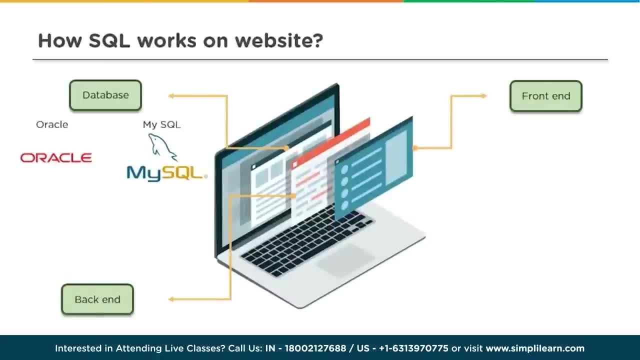 and generate SQL queries. At the server side you'll have databases like Oracle, MySQL and so on- sql, msql and so on, so forth that will then execute those queries right. so just to give you an example, if i use a tool called postman, what we generally do when we craft a query is we send out a. 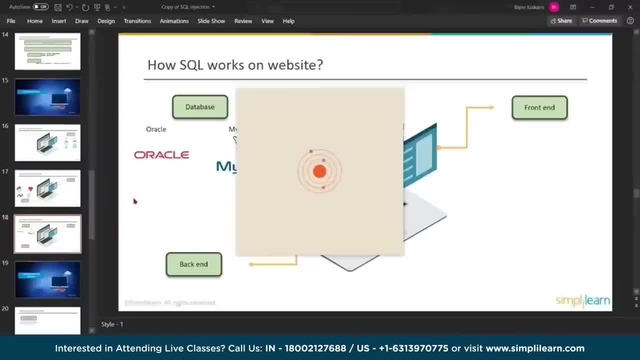 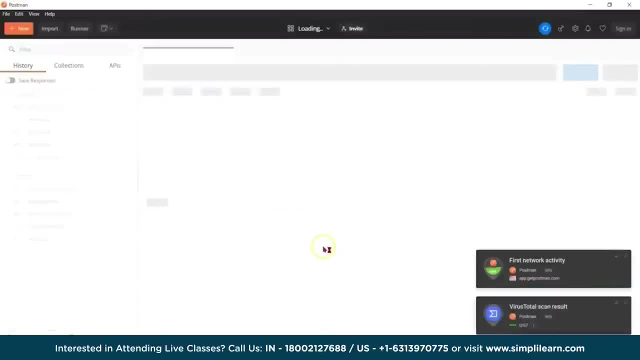 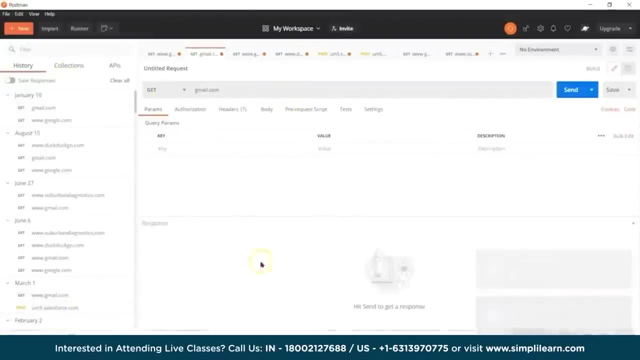 get request to the website and then we receive a response from the site with the html code and everything. so this is a tool that is utilized by software testers to test the responses that you're going to get from various websites. so on the left hand side you can see i've used it on quite a bit. 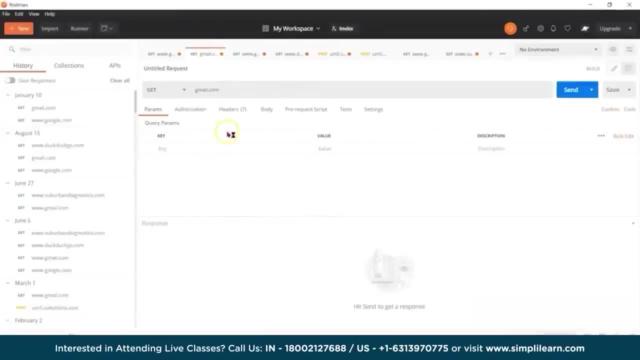 uh, here we have an example for gmailcom, so let's continue with that. so this is a get request being sent to gmail. the moment i send it, it's going to create an http request and send it across. the response that i get is this: this is the html code for gmailcom. right, these are the cookies. 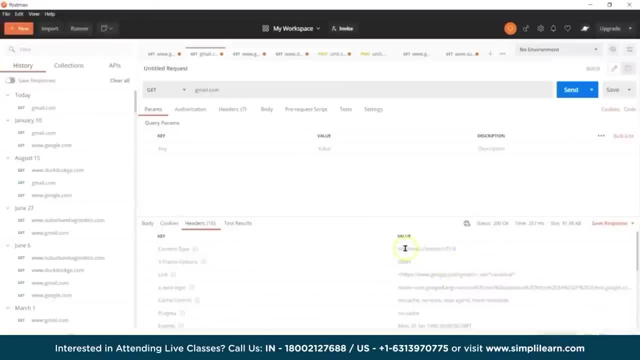 these are the headings that i've added and those are the status of the html data set that i've used. and then let's take a look at the other embeddors that include information. so you can see this is a text html, character set utilized is utf-8 and the configuration that has been done with the application right. so this is. 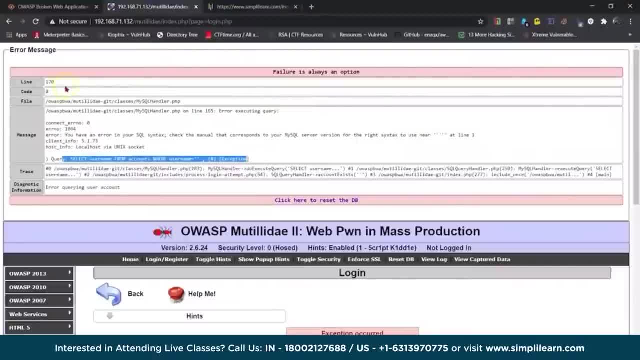 where everything comes in. this is the cookie that has been sent with that particular request that i had sent out now, if you analyze this query right. so when we went on to this application and i typed in that single quote and we generated this error, application converted this into a SQL query, so the query was select username. 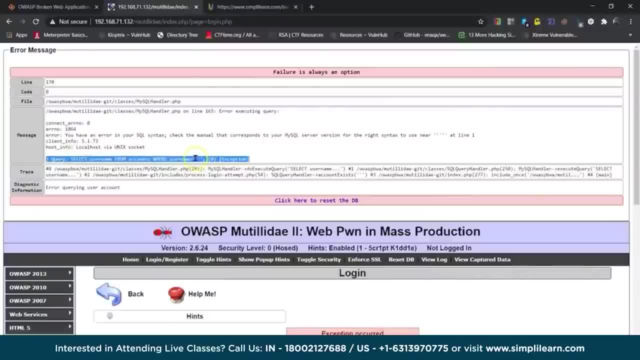 from accounts where the username in quotes single quotes and we use this quote right, the single quote, right there. so that's where we use that operator and that's where the exception error occurred. so these are the kind of queries that are structured by the application and then taken on to the 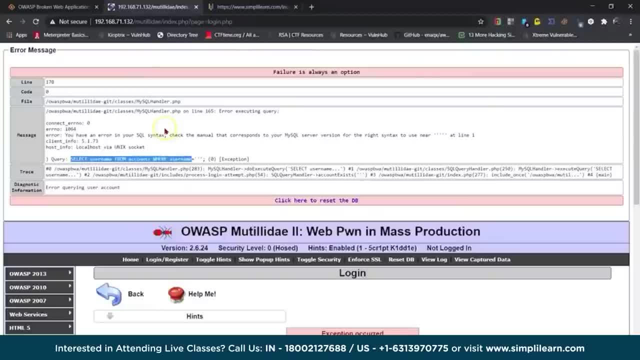 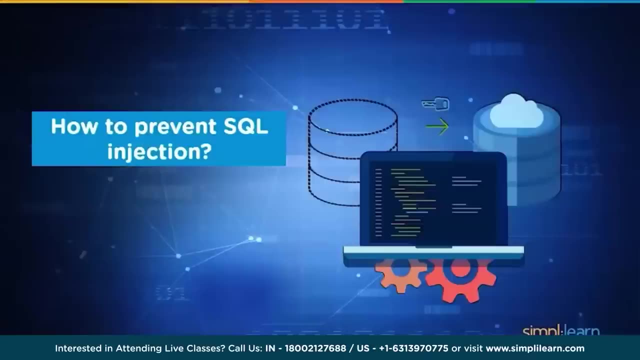 database for execution. when we type in it is a HTTP get request with the username and password within that query that is sent to the application. the application converts it into a sequel query, sends it to the database and the database responds with the appropriate response. so how do we prevent sequel? 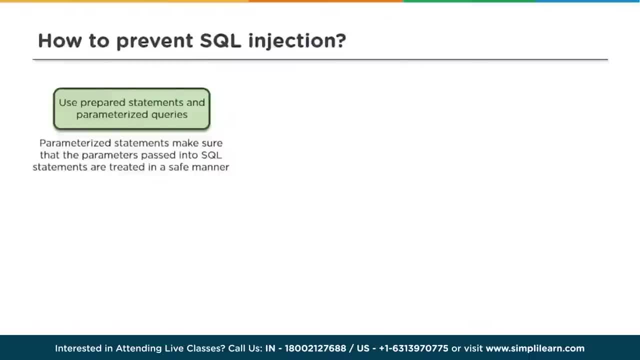 injection in the first place. use prepared statement and parameterized queries. these statements make sure that the parameters pass into SQL. statements are treated in a safe manner. so, for example, we saw that the single quote was an operator. this shouldn't be allowed to be utilized in the first place. 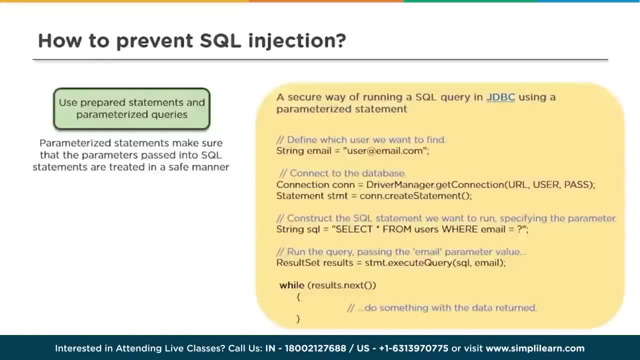 right. so here, what we are doing here is a secure way of running a sequel query in the JDBC using a parameterized statement: define which user we want to find. so there's a string. the email comes in connection to the database. we are going to figure out how the connection is going to be passed, how it is going to. 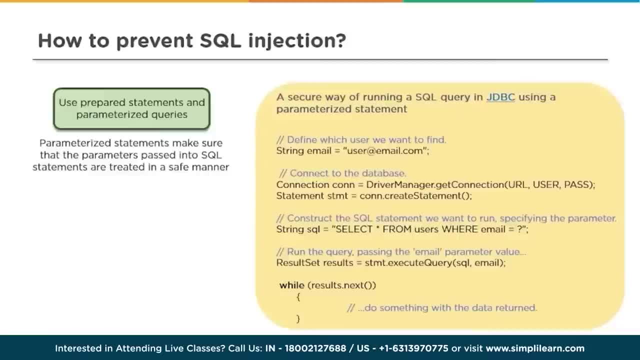 be created. construct the sequel statement we want to run specifying the parameter, right, so we define how is it going to be created, what is going to be created, what can be passed to the database and what should not be passed. so that is one way of utilizing prepared statements and parameterized queries. 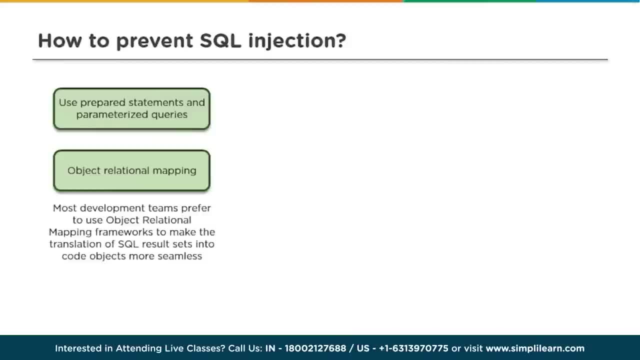 then we have object relational mapping. most development teams prefer to use object relational mapping frameworks to evade the translation of sequel results set into core objects more seamless. so there's an example of object relational mapping where we map certain objects and allow that to be executed and then escaping inputs in a simple way. 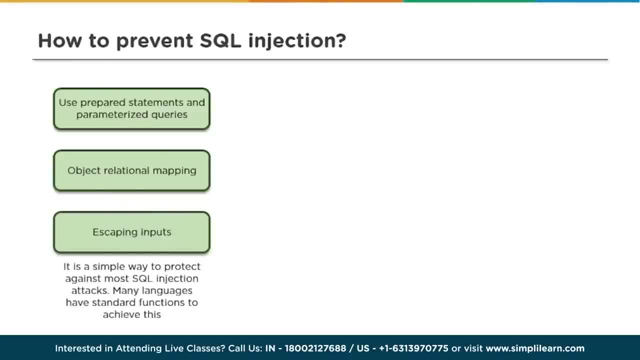 way to protect against most SQL injection attacks. many languages have standard functions to achieve this right, so you need to be very careful while using escape characters in your code base when a sequel statement is constructed. not all injection attacks rely on abuse of code characters, so you need to know what characters are being utilized in the configuration that you. 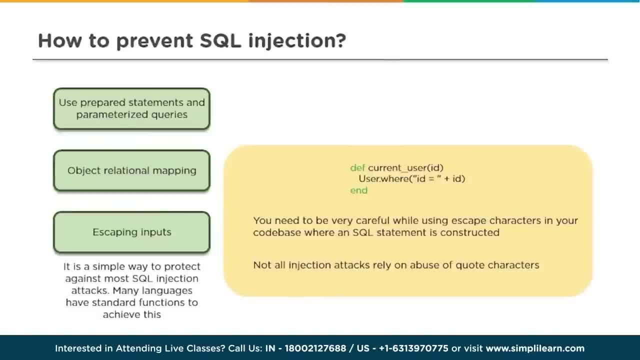 have created, in the structure that you have created, in the code that you have created, which characters are being recognized as operators. you need to sanitize those operators and you need to basically ensure that these operators cannot be accepted as user input. if they are, they're veered out by the 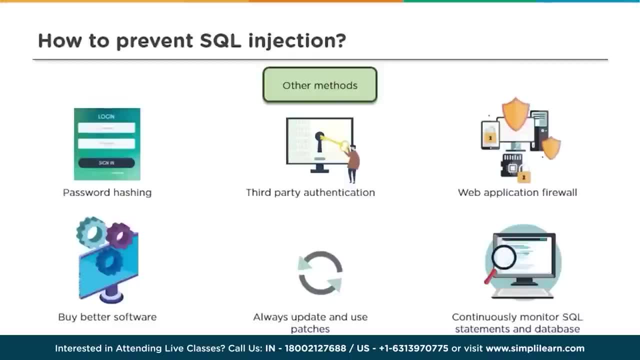 application and they never reach the database. other methods of preventing sequel injection are password hashing, so that passwords cannot be bypassed, the passwords cannot be recovered, passwords cannot be cracked. third-party authentication: you use what or some other service for a single sign-on mechanism. does you rely? 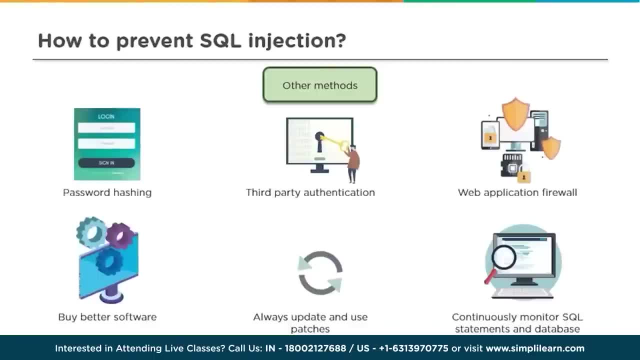 on a third party to maintain the security of authentication, and what kind of parameters are passed? for example, using LinkedIn logins or Facebook logins? right, for the layman: you normally go on to Facebook and you allow if you're using a game. right, if you start playing a game, you're allowed to log in. 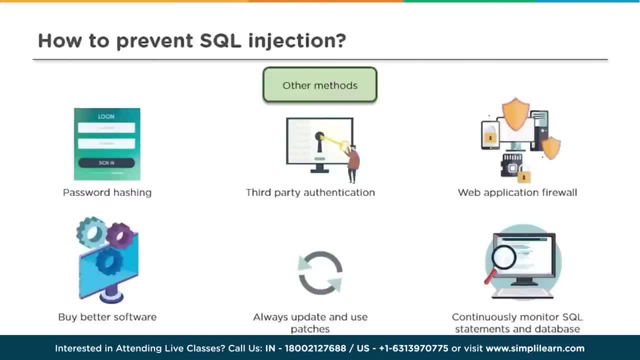 to the game using your Facebook credentials or your Google credentials. now, that is not just for ease of use, but the game user, the developer, has outsourced the authentication mechanisms to third parties such as Facebook or Google, because they understand that that authentication mechanism is as safe as 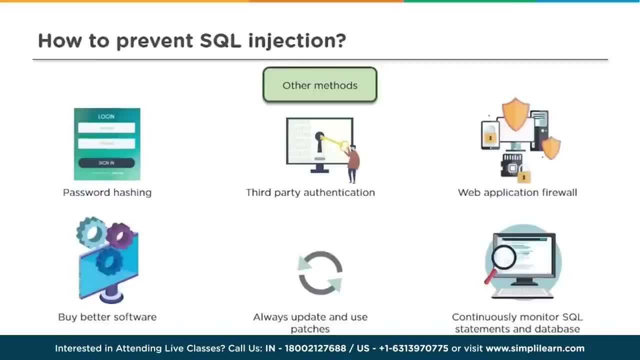 can be. Facebook and Google are wealthy organizations, hire a lot of security experts, and the development for their authentication mechanisms is top-notch. the small organization cannot spend that kind of money on security itself, right? so you use a third-party authentication mechanism to ensure that these kind of attacks may not happen. then web. 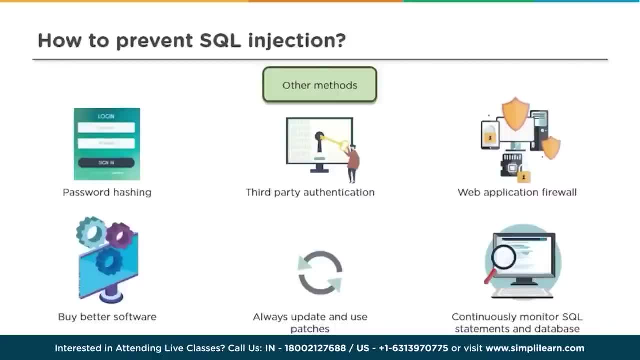 application firewalls. having a web application firewall and configuring it properly for sequel injection attacks is one of the sure-shot method of mitigating or minimizing the threat in the first place. so at this point in time, you have realized that the application has some vulnerabilities for sequel injection and 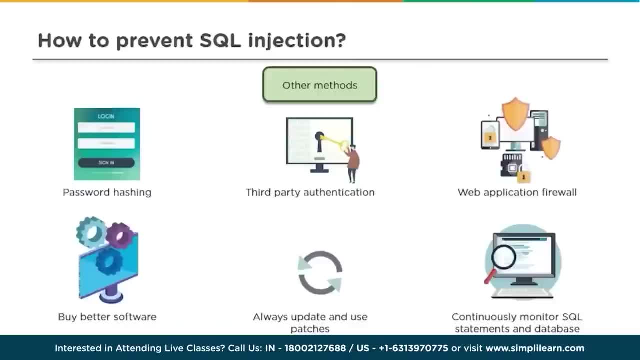 instead of recording or restructuring the application, you want to take the easier way out or the cheaper way out. so what you do is you: you install a web application firewall and you configure the web application firewall to identify malicious queries and stop them at the firewall level itself. so then, never. 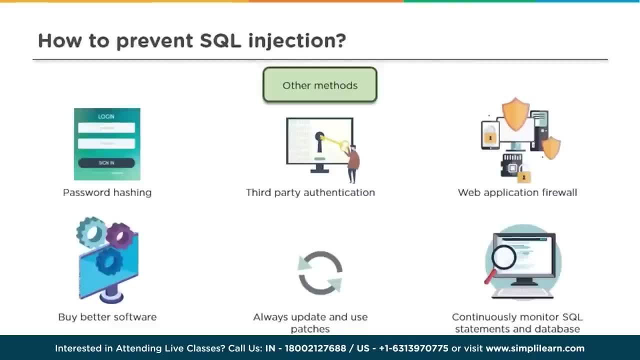 reach the application and does the vulnerabilities in the application don't get executed. buy better software and keep on updating the software. so it's not necessarily that oneこう you have a software, you install it. it's going to be safe for life. new vulnerabilities are discovered. 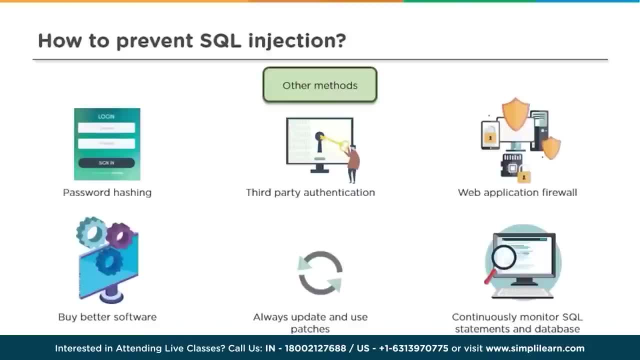 every day, every hour, and it may so happen. what is secure today may be completely insecure tomorrow or the day after right, so you need to keep on upgrading the software. if there are no upgrades available and the vulnerabilities still exist, you might want to migrate to a better software. 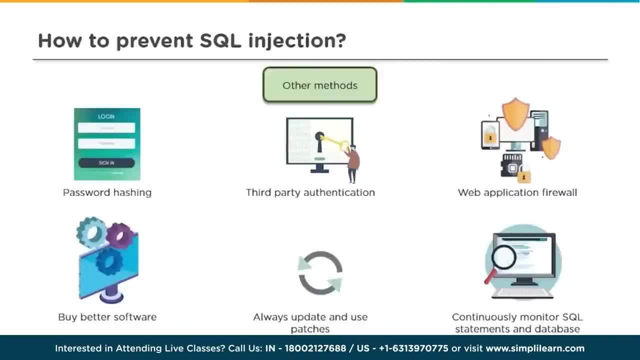 and thus ensure that you don't get hacked right. always update and use patches. organizations keep on sending out updates and patches as and when they are released. you need to install them to enhance your security portions and then continuously monitor sql statements and databases. use protocol monitors. use different softwares. use the firewalls to keep on monitoring. 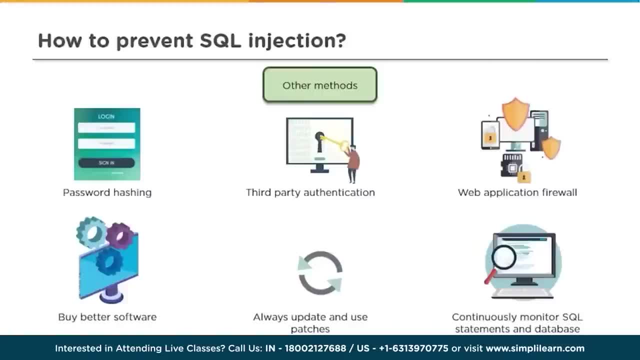 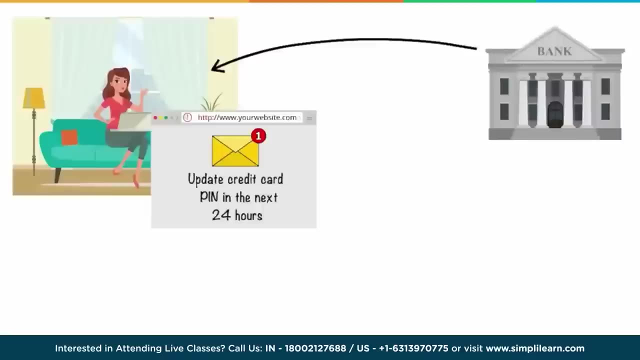 what kind of queries you're getting and, based on those queries, you want to ensure the inputs and the queries that are creating are not detrimental to the health of the software that you have. gmail: jane is relaxing at home when she receives an email from a bank that asks her to update her. 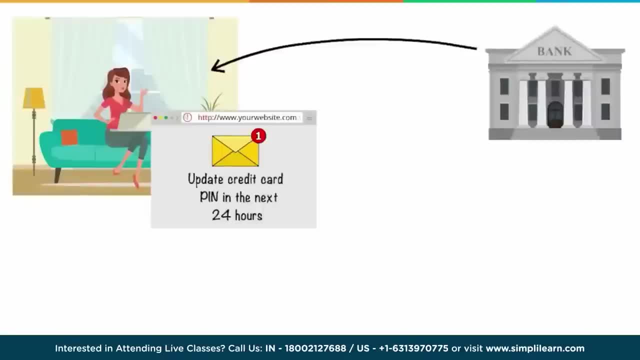 credit card pin in the next 24 hours as a security measure. judging the severity of the message, jane follows the link provided in the email on delivering her current credit card pin and the supposedly updated one. the website became unresponsive, which prompted her to try sometime later. however, after a couple of hours she noticed a significant purchase from a random website on 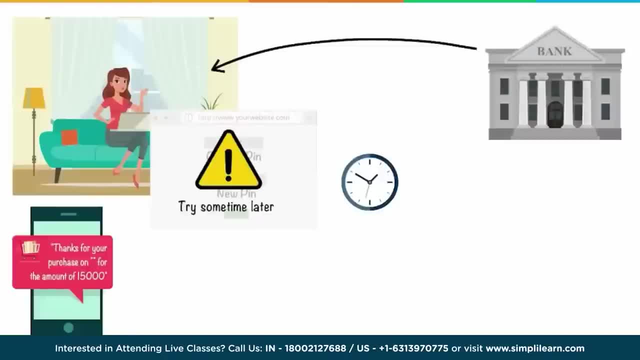 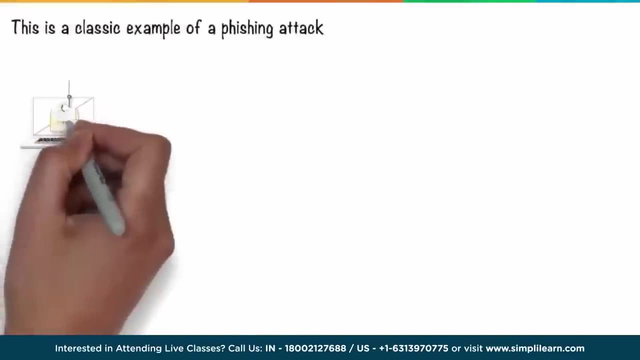 that same credit card which she cooling, she the most frantically contacting the bank. jane realized the original email was a counterfeit or reflecting message with the malicious link of credit card fraud. this is a classic example of the phishing attack. phishing attacks R type of social engineering where fraudulent messages sent. 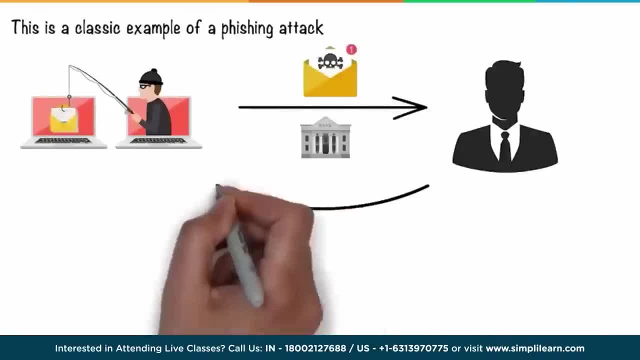 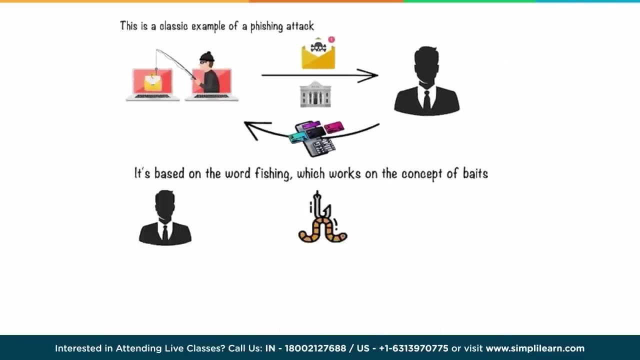 to a target on the premise of arriving for the trusted source. it's basic purpose is to trick the victim into revealing sensitive information like pass, such an payment, information, cash- based on the word phishing, which works on the concept of baits. If a supposed victim catches the bait, the attack can go ahead, which, in our case, makes 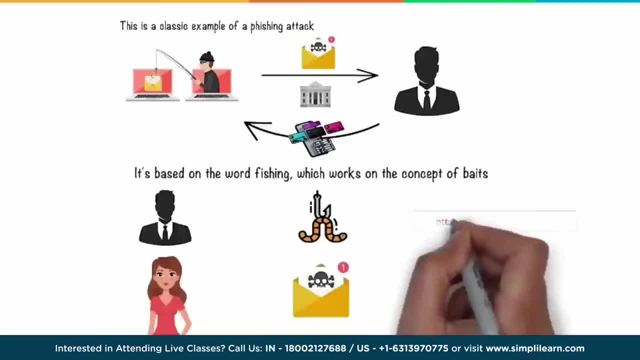 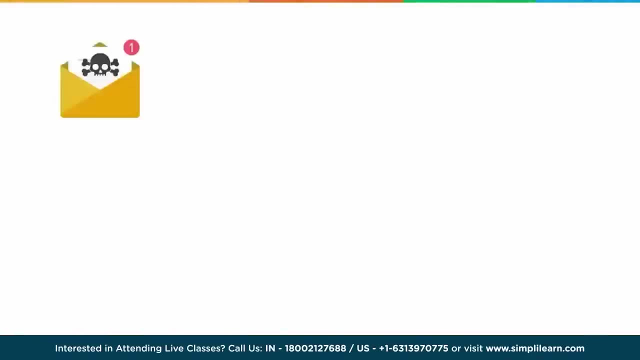 Jane the phish and the phishing emails the bait. If Jane never opened the malicious link or was cautious about the email authenticity, an attack of this nature would have been relatively ineffective. But how does the hacker gain access to these credentials? A phishing attack starts with a fraudulent message which can be transmitted via email. 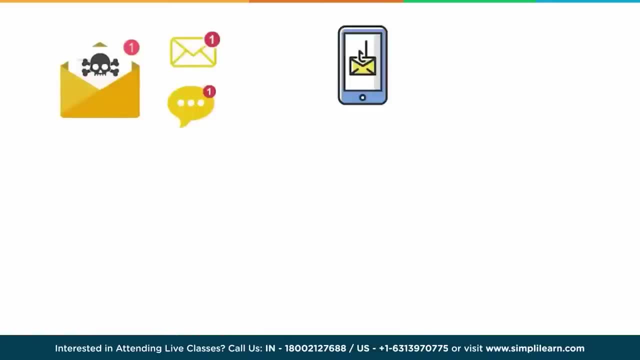 or chat applications, Even using SMS conversations, to impersonate legitimate sources is known as smishing, which is a specific category of phishing attacks. Irrespective of the manner of transmission, the message targets the victim in a way that coaxes them to open a malicious link and provide critical information on the requisite website. 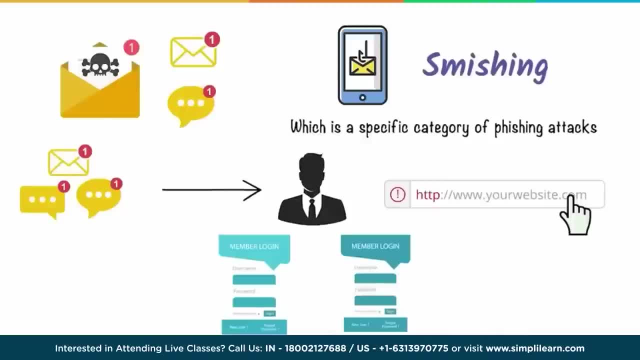 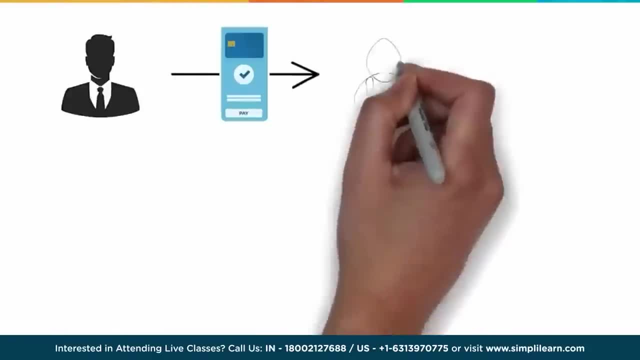 More often than not, the websites are designed to look as authentic as possible. Once the victim submits information using the link, be it a password or credit card details, the data is sent to the hacker who designed the email and the fake website giving. 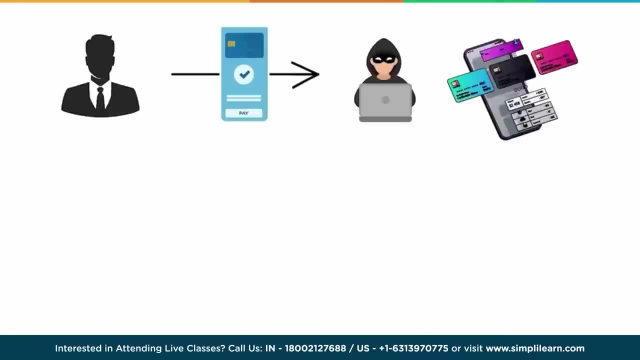 him complete control over the account whose password was just provided. Often carried out in campaigns where an identical phishing mail is sent to thousands of users, the rate of success is relatively low, but never zero. Between 2013 and 2015, corporate giants like Facebook and Google were able to use phishing. 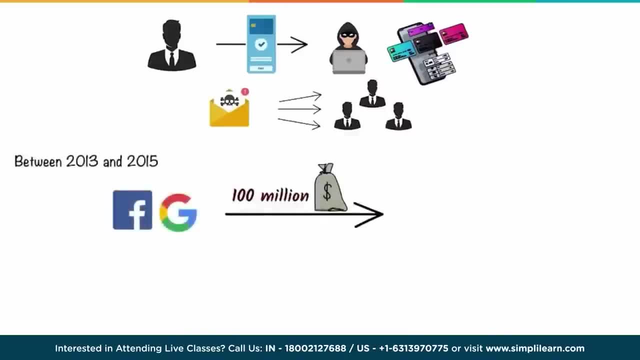 as a tool to counter phishing attacks. For example, Facebook and Google were tricked off of $100 million due to an extensive phishing campaign where a known common associate was impersonated by the hackers. Apart from credit access, some of these campaigns target the victim device and install malware. 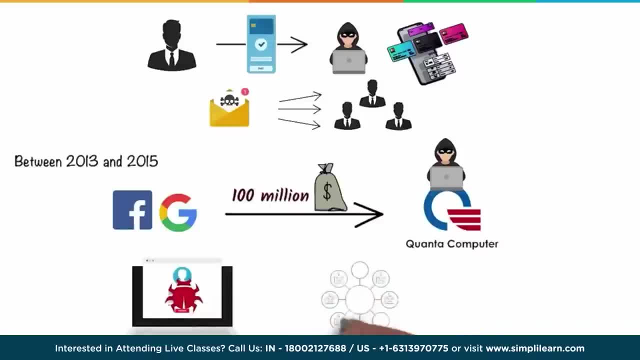 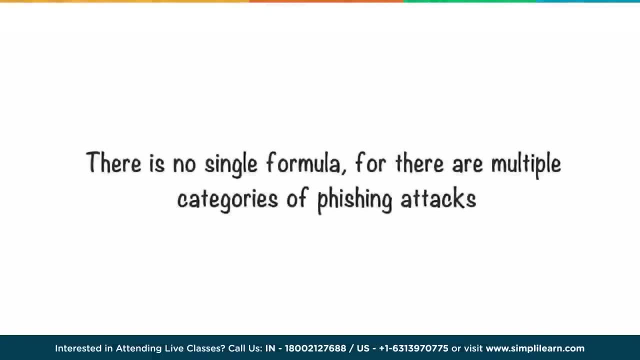 when clicked on the malicious links, which can later function as a botnet or a target for ransomware attacks. There is no single formula, for there are multiple categories of phishing attacks. The issue with Jane, where the hacker stole her bank credentials, falls under the category. 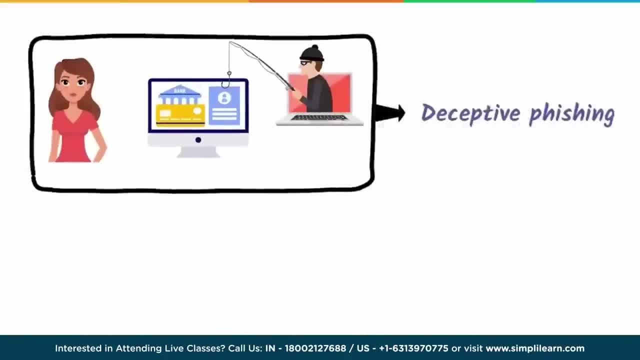 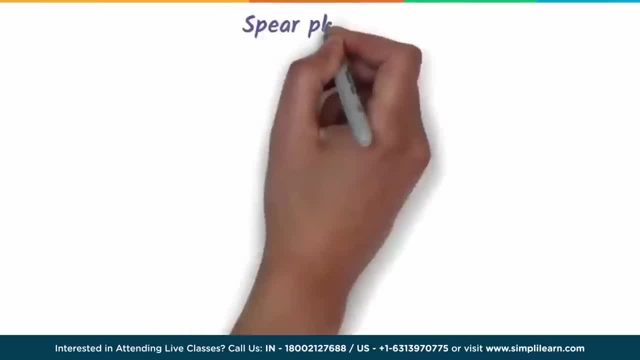 of phishing attacks. A general email is sent out to thousands of users in this category, hoping some of them fall prey to this scam. In the case of Facebook, the type of phishing attacks is a very common one. Spearfishing, on the other hand, is a bit of a customized version. 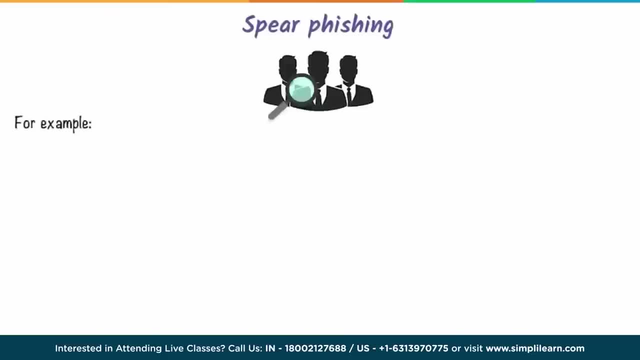 The targets are researched before being sent an email. For example, if you never had a Netflix subscription, sending you an email that seems like the Netflix team sends it becomes pointless. This is a potential drawback of deceptive phishing techniques. On the other hand, a simple screenshot of a specific product is always the best way. 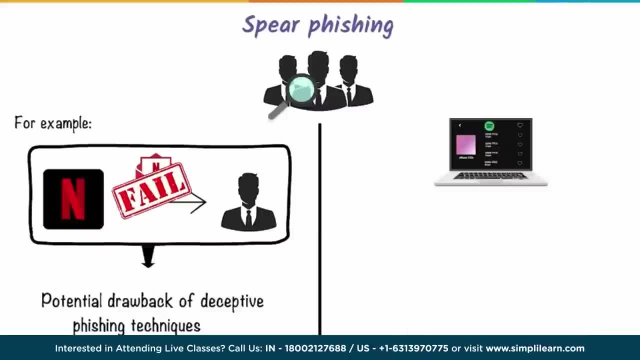 to use it. Spotify playlist being shared on social media indicates a probable point of entry. The hacker can send counterfeit messages to the target user while implying the source of such messages being Spotify, tricking them into sharing private information. Since the hacker already knows the target uses Spotify, the chances of victims taking 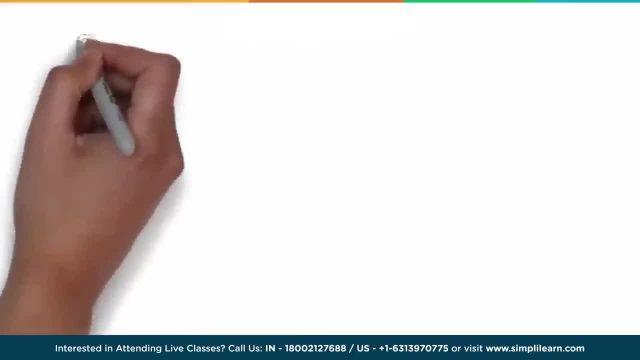 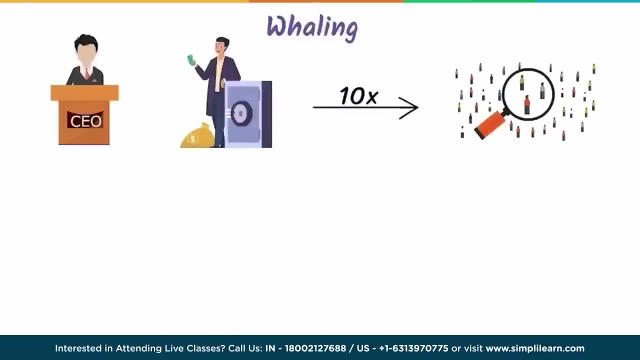 the bait increase substantially. For more important targets, like CEOs and people with a fortune on their back, the research done is tenfold, which can be called a case of whaling. The hackers prepare and wait for the right moment to launch their phishing attack. often, 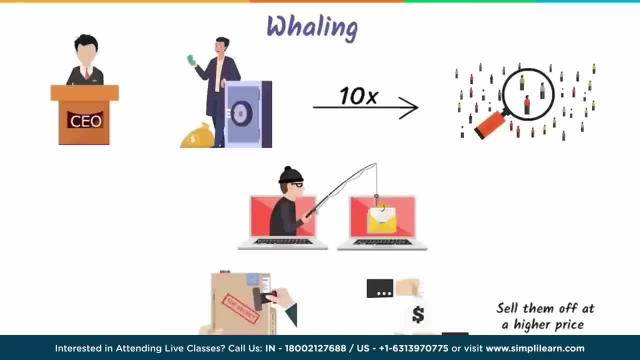 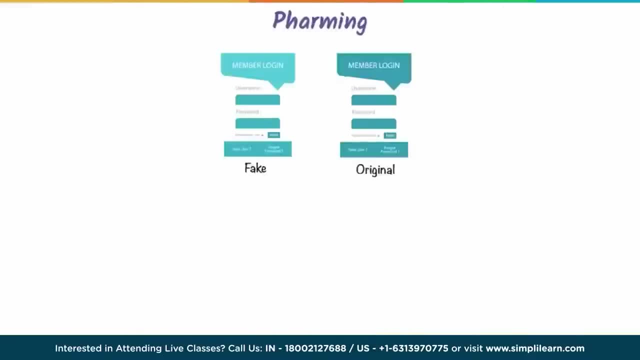 to steal industry secrets for rival companies or sell them off at a higher price. Apart from just emails, farming focuses on fake websites that resemble their original counterparts as much as possible. A prevalent method is to use domain names like Facebook with a single O or YouTube with 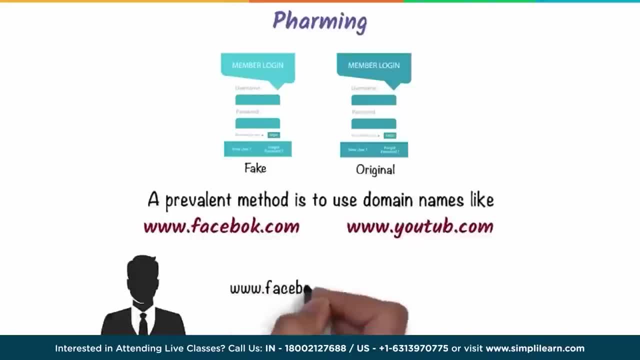 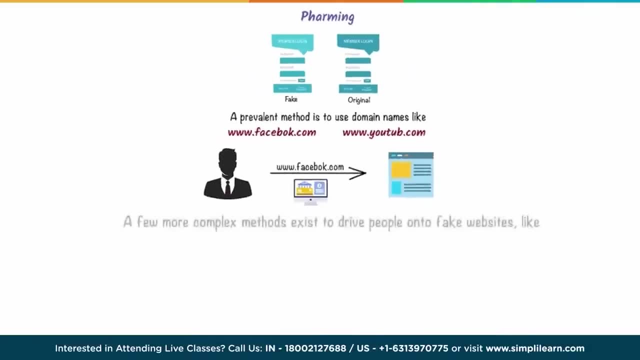 no E. These are mistakes that people make when typing the full URL. This leads them straight to a counterfeit web page, which can fool them into submitting private data. A few more complex methods exist to drive people onto fake websites like ARP spoofing. 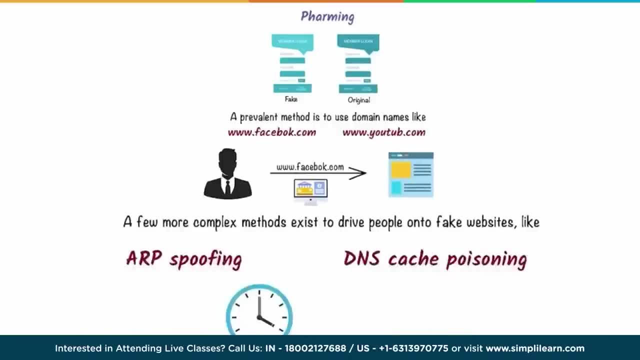 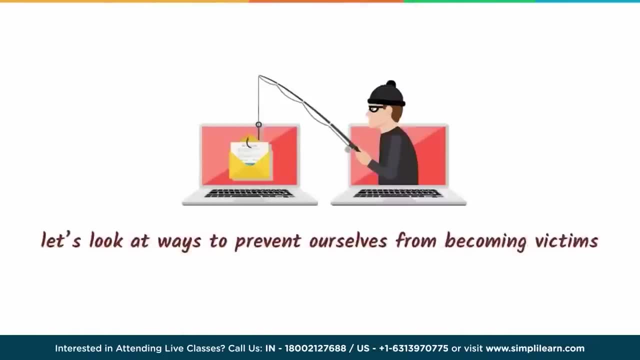 and DNS cache poisoning, but they are rarely carried out due to time and resource constraints. Now that we know how phishing attacks work, let's look at ways to prevent ourselves from becoming victims. While the implications of a phishing attack can be extreme, protecting yourself against. 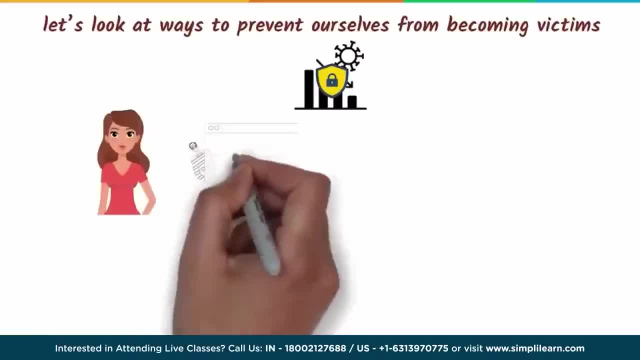 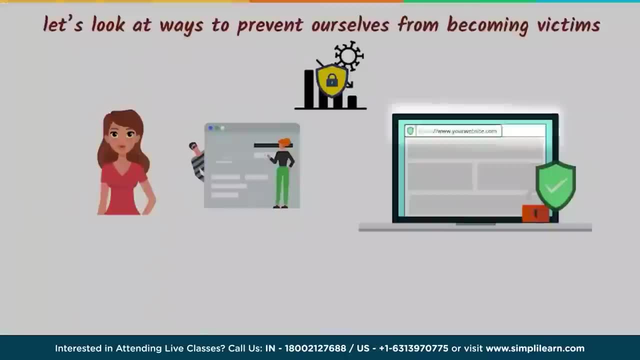 these is relatively straightforward. Jane could have saved herself from credit card fraud had she checked the link in the email for authenticity and that it redirected to a secure website that runs on the HTTPS protocol. Even suspicious messages shouldn't be entertained. One must also refrain from entering private information on random websites or pop-up windows. 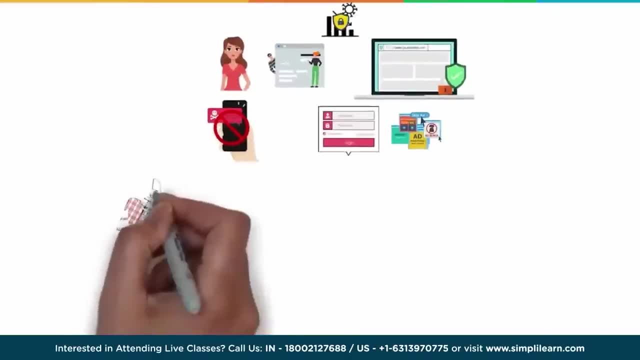 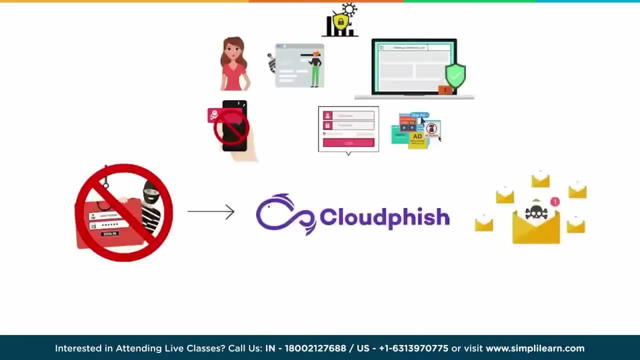 irrespective of how legitimate they seem. It is also recommended to use secure anti-phishing browser extensions like Cloudfish to snip out malicious emails from legitimate ones. The best way to prevent phishing is browsing the internet with care and being on alert for malicious attempts at all times. 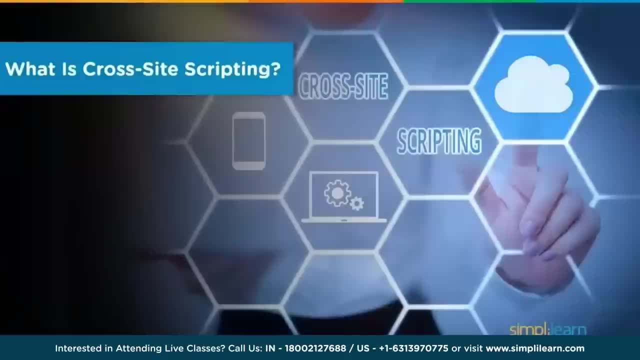 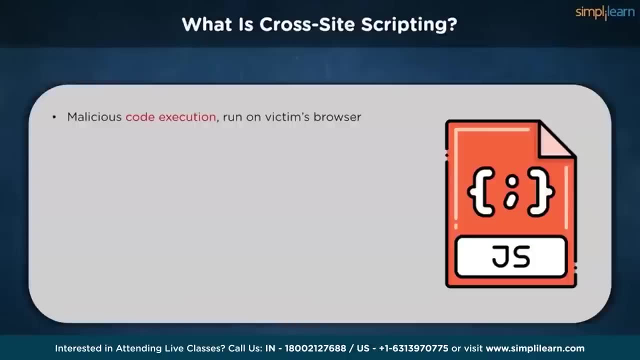 Let's start by learning about cross-site scripting from a layman's perspective. Cross-site scripting, also known as XSS, is a type of code injection attack that occurs on the client's site. The attacker intends to run harmful scripts in the victim's web browser by embedding. 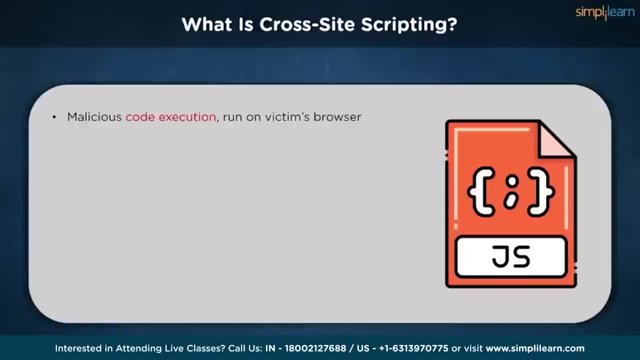 malicious code in a genuine web page or online application. The real attack takes place when the victim hits the malicious code-infected web page or online application. The web page or application serves as a vehicle for the malicious script to be sent to the user's browser. 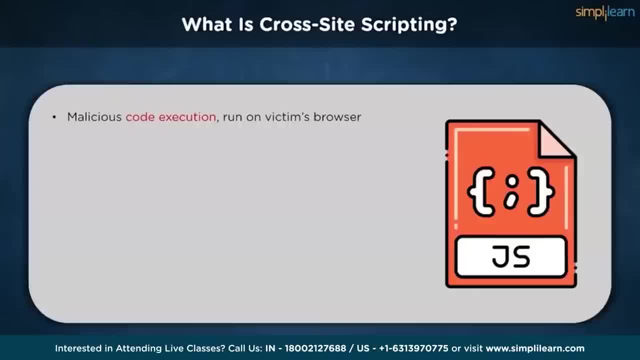 Forums, message boards and online pages that enable comments are vulnerable vehicles that are frequently utilized for cross-scripting assaults. A web page or web application is vulnerable to XSS if the output it creates contains unsanitized user information. The victim's browser must then parse this user input. 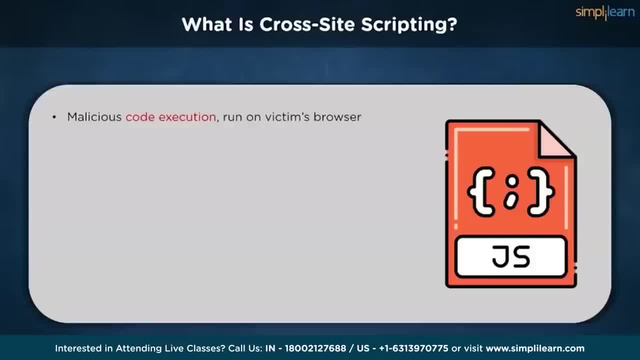 In VBScript, ActiveX, Flash and even CSS. cross-site scripting attacks are conceivable. They are nevertheless most ubiquitous in JavaScript, owing to the fact that JavaScript is most important to most browser experiences nowadays. The main purpose of this attack is to steal the other user's identity, be it via cookies. 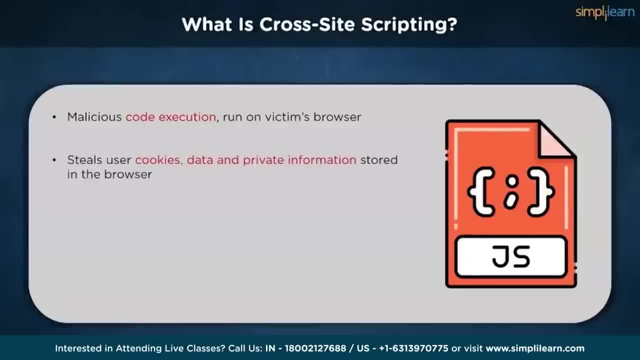 session tokens and other information. If the user's profile is not visible in the web, then the user can't access the web. The user can't access the web. this attack is being used to steal the other person's cookies, As we know. 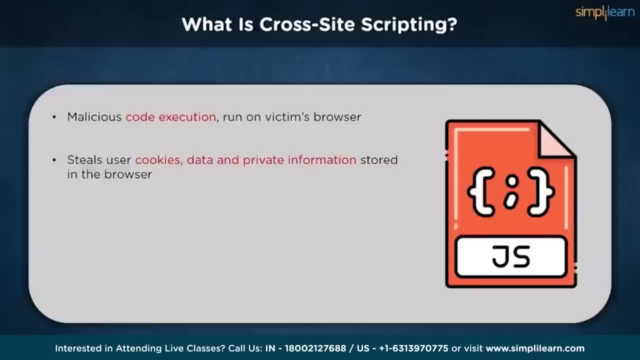 cookies help us to log in automatically. Therefore, with the stolen cookies, we can log in with other identities, and this is one of the reasons why this attack is considered as one of the riskiest attacks. It can be performed with different client-side programming languages as well. Cross-site scripting. 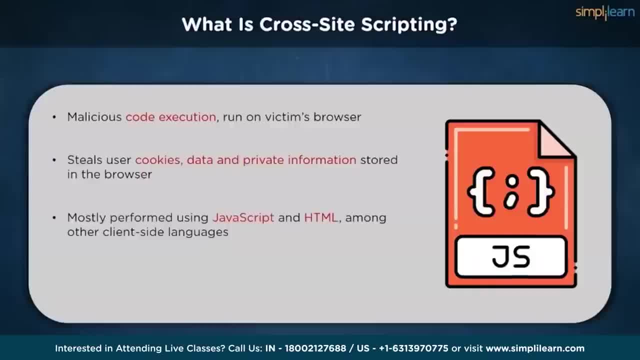 is often compared with similar client-side attacks, as client-side languages are mostly being used during this. However, an XSS attack is considered riskier because of its ability to damage even less vulnerable technologies. Most often, this attack is performed with JavaScript and HTML. JavaScript is a programming. 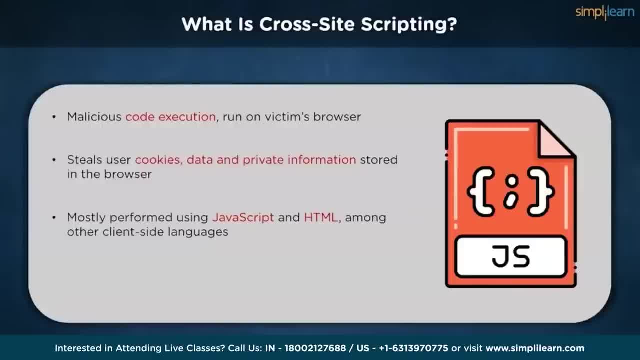 language that runs on web pages inside your browser. The client-side code adds functionality and interactivity to the web page and is used extensively on all major applications and CMS platforms, Unlike server-side languages such as PHP, PHP or Linux. JavaScript is a programming language that runs on web pages. The client-side code adds functionality and interactivity to the web page and is used extensively on all major applications and CMS platforms, Unlike server-side languages such as PHP. 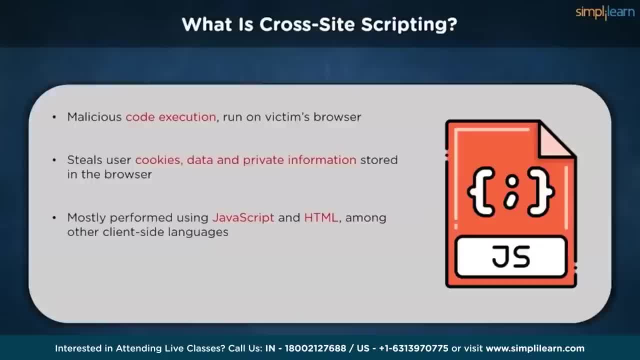 JavaScript is a programming language that runs on web pages inside your browser and is used extensively on all major applications and CMS platforms. Unlike server-side languages such as PHP, JavaScript code runs inside your browser and cannot impact the website for other visitors. It is sandboxed to your own navigator and can only perform actions within your own. 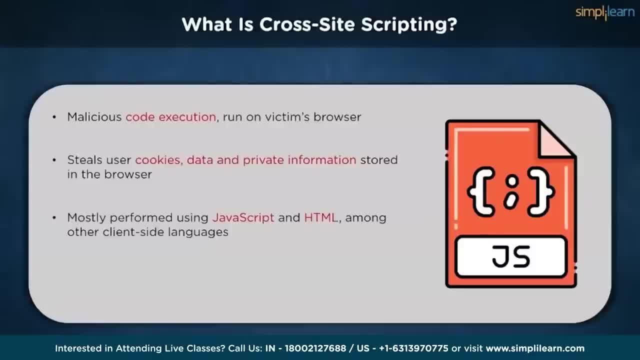 browser window. While JavaScript is client-side and does not run on the server, it can be used to interact with the server by performing background requests. Attackers can then use these background requests to add unwanted spam content to a web page without refreshing it. They can then gather. 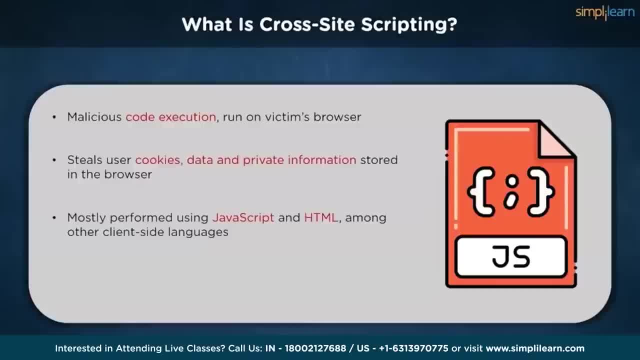 analytics about the client's browser or perform actions asynchronously. The manner of attack can range in a variety of phases. It can be a single link which the user must click on to initiate a JavaScript piece of code. It can be used to show any piece of images that can be. 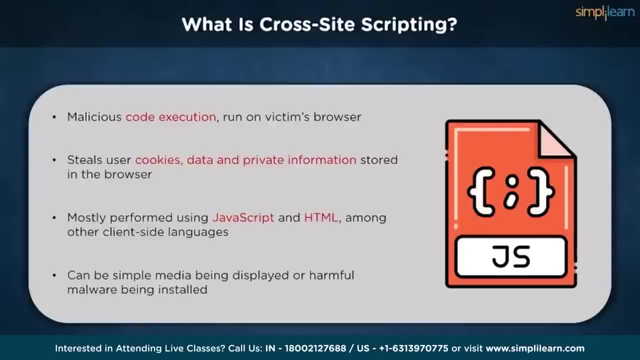 later used as a front-end for malicious code being installed as malware. With the majority of internet users unaware of how metadata works or the ways in which web requests are called, the chances of victims clicking on and redirecting links is far too high. Cross-site scripting can. 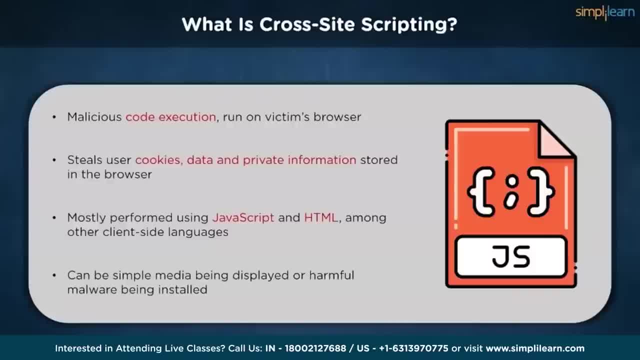 occur on the malicious script executed at the client's side using a fake page or even a form that is displayed to the user. On websites with displayed advertisements, malicious emails can also be sent to the victim. These attacks occur when the malicious user finds the vulnerable parts of the website and 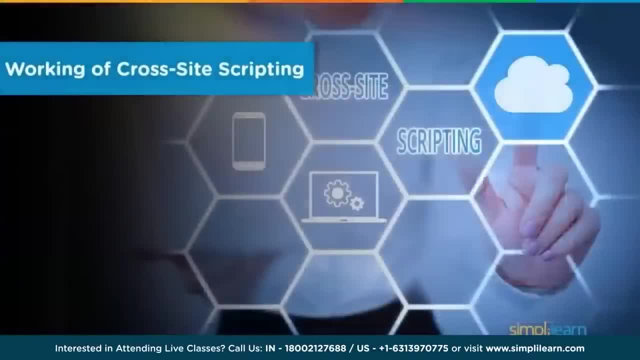 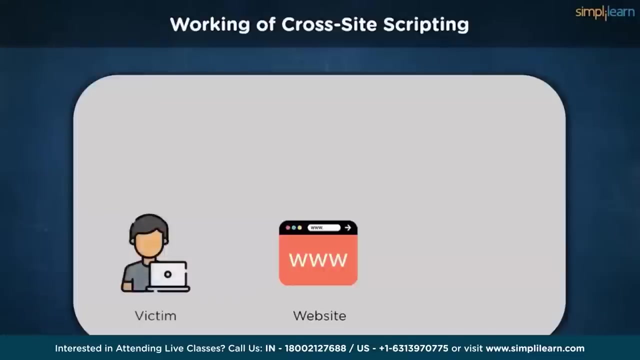 sends it as appropriate malicious input. Now that we understand the basics of cross-site scripting, let us learn more about how this kind of attack works Now. first, we have the website or the web browser which is used to show content to the victim, or which is the user in our case, Whenever the user wants to grab some. 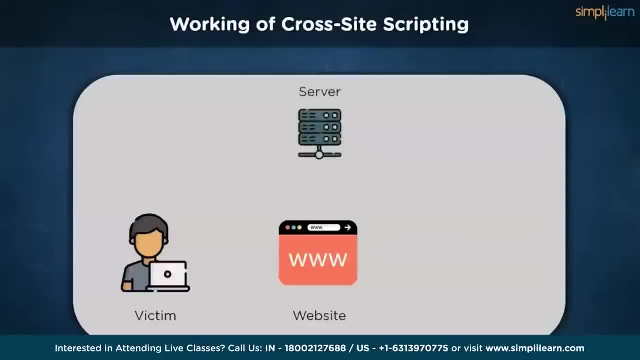 content from the website. the website asks the data from the server. The server provides this information to the website and the web browser, which ultimately resists the victim. How the hacker comes into play here. it passes on certain arguments to the web browser, which can be then forwarded back to the server or 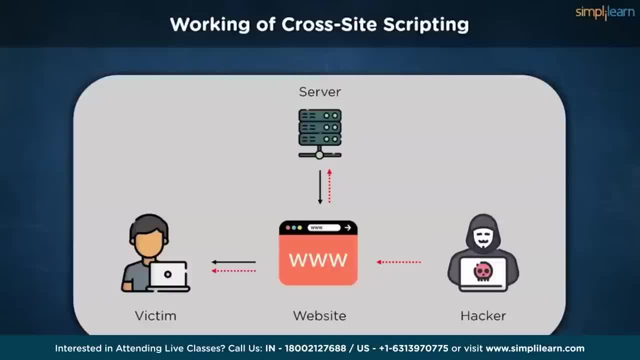 to the user at hand. The entire cross-site scripting attack vector means sending and injecting malicious code or script. Tthis attack can be performed in different ways Depending on the type of attack. the malicious script may be reflected on the victim's browser or stored in the database and executed every time when. 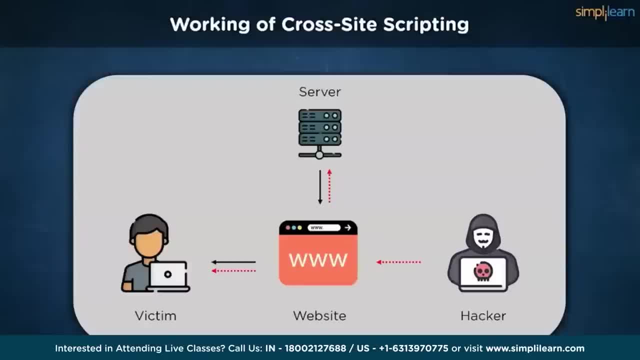 the user calls the appropriate function. The main reason for this attack is inappropriate users input validation, where the malicious input can get into the output. A malicious user can enter a script, get the malicious input and then send the malicious script to the specific user. 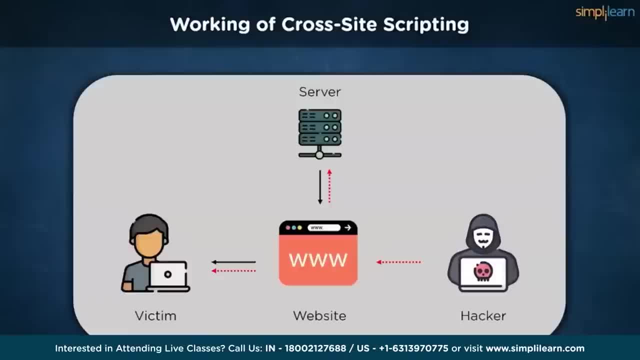 enter a script which will be injected onto the website's code. Then the browser is not able to know if the executed code is malicious or not. Therefore, this malicious script is being executed on the victim's browser or any faked form, if that is being displayed for the users. 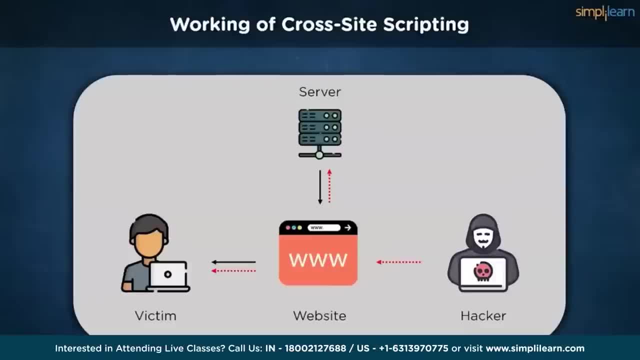 There are many ways to trigger an XSS attack. For example, the execution could be triggered automatically when the page loads or when a user hovers over specific elements of the page, like hyperlinks. Potential consequences of XSS attacks include capturing keystrokes of a user. 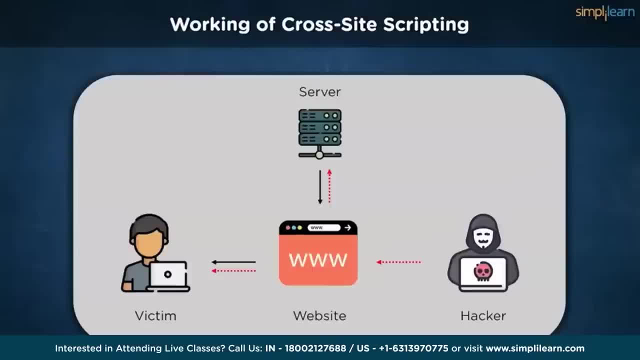 redirecting a user to malicious websites, running web browser-based exploits, obtaining cookie information of a user who is logged into a website, and many more. In some cases, XSS attack leads to complete compromise of the victim's account. Attackers can trick users into entering credentials on a fake form. 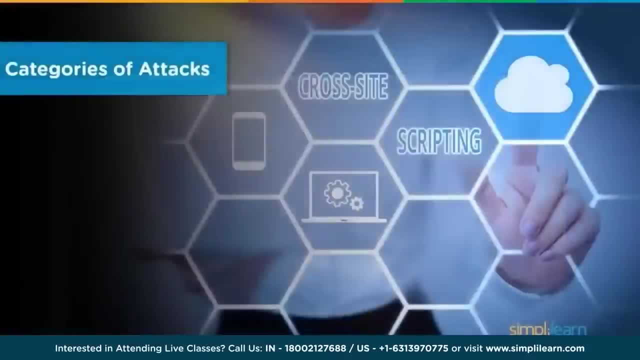 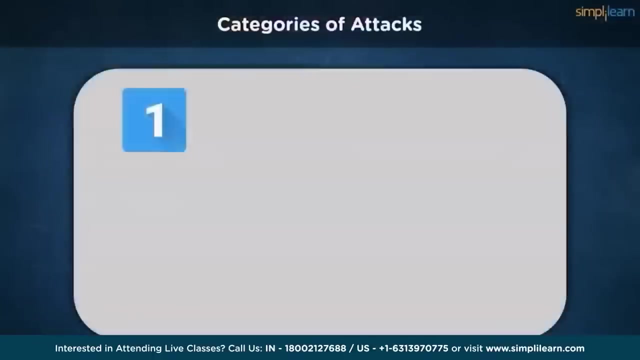 which can then provide all information to the attacker. With the basic working of a XSS, let us go over the different ways hackers can leverage vulnerable web applications to gather information and eventually breach those systems. The prime purpose of performing XSS attack is to steal the other person's identity. 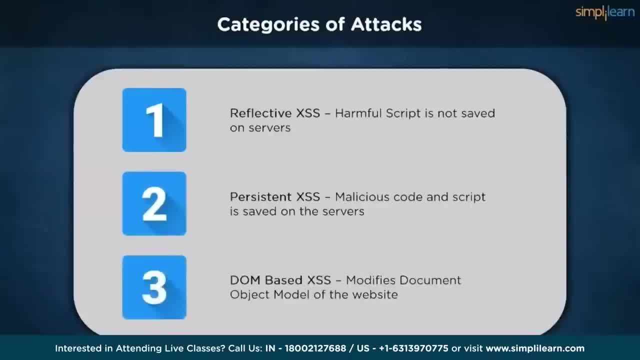 As mentioned, it may be cookies, session tokens, etc. XSS may also be used to display faked pages or forms for the victim. However, this can be performed in several ways. We have a few examples. We have a reflected attack. 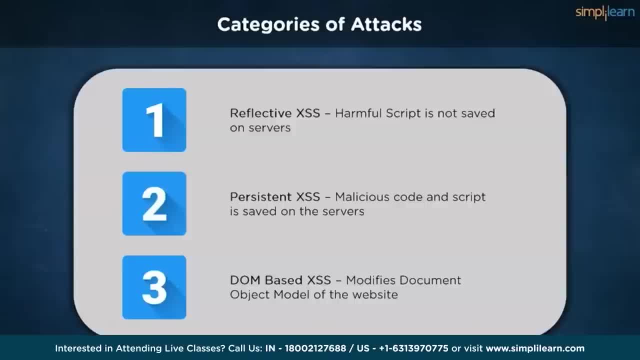 This attack occurs when a malicious script is not being saved on the web server but is reflected in the website results. Reflected XSS code is not being saved permanently. In this case, the malicious code is being reflected in any website result. The attack code can be included in the faked URL or in the HTTP parameters. 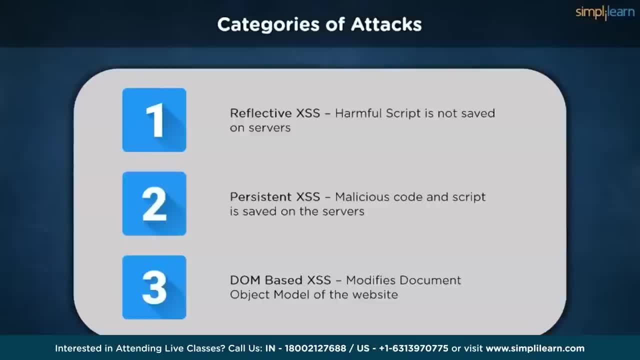 It can affect the victim in different ways, by displaying fake malicious page or by sending a malicious email. In a reflected cross-site scripting, the input of a search form is reflected on the page to show what the search key was. An attacker may craft a URL that contains malicious code. 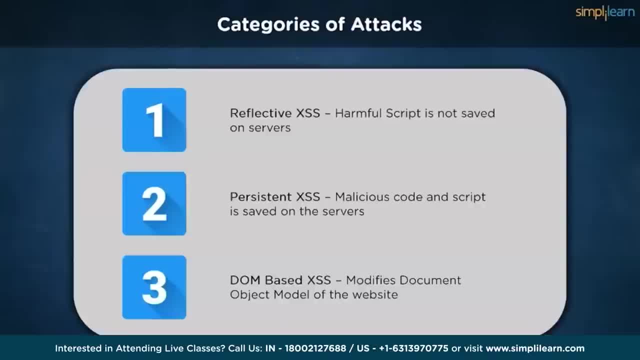 and then spread the same URL via email or social media. A user who clicks on this link opens the valid web application, which then runs the malicious code in the browser. This script is not stored in the web application and malicious code is shown only to one user. 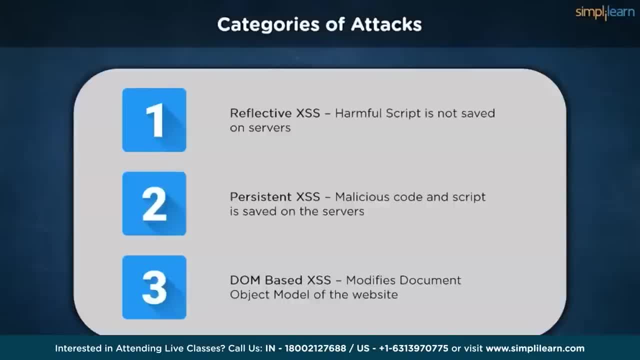 The user that opens the link executes the script and the attack is not necessarily valid. The user that opens the link executes the script and the attack is not necessarily valid. The user that opens the link executes the script and the attack is not necessarily valid. 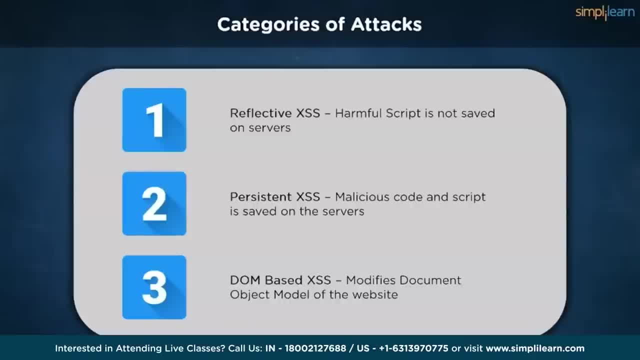 The next variant is a stored cross-site scripting attack. This occurs when a malicious script is being saved on the web server permanently. This can be considered a riskier attack, since it has leverage for more damage. In this type of attack, the malicious code or script is being saved on the server. 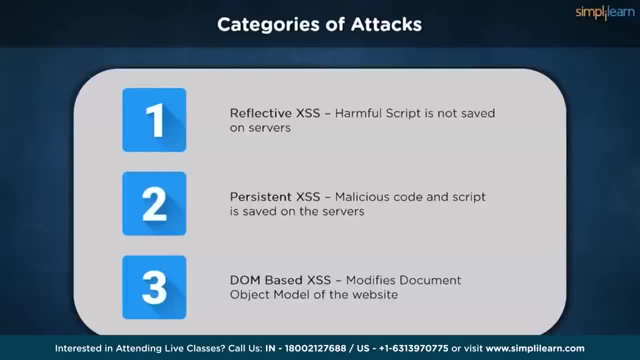 for example, in the database of the website. It is executed every time the user has called the appropriate functionality. This way stored XSS attack can affect many users Also. as the script is being stored on the web server, it will affect the website for a longer time. 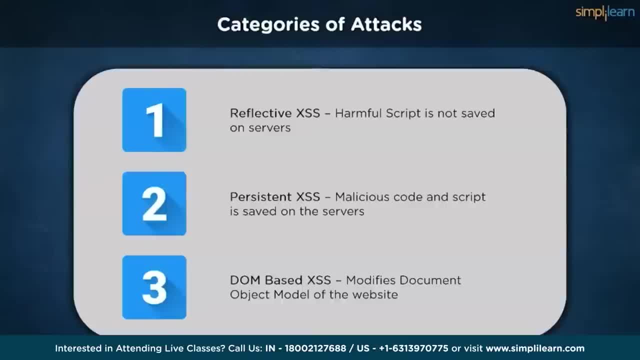 In order to perform stored XSS attack, the malicious scripts should be sent through the vulnerable input form. For example can be a comment field or a review field. This way, the appropriate script will be saved in the database and evaluated on the page load or appropriate function calling. 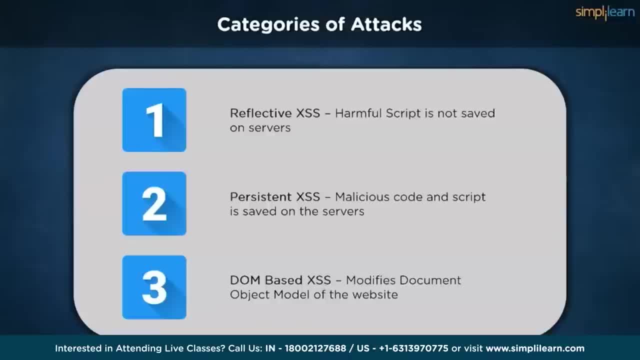 In a stored XSS example, the script might have been submitted via an input field to the web server, which did not perform a sufficient validation and stores the script permanently in the database. The consequence of this might be that this script is now being delivered to all users visiting the web application. 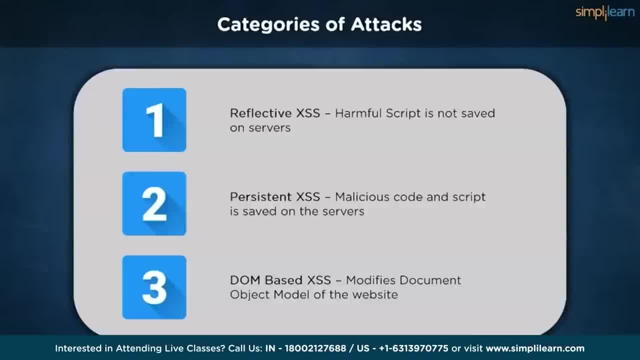 and they, for example, able to gain access to the user session cookies. In this attack, the script is permanently stored in the web app. The users visiting the app after the information retrieve this. The malicious code then exploits the flaws in the web application and the script and the attack is visible on the server side or to the app owner as well. 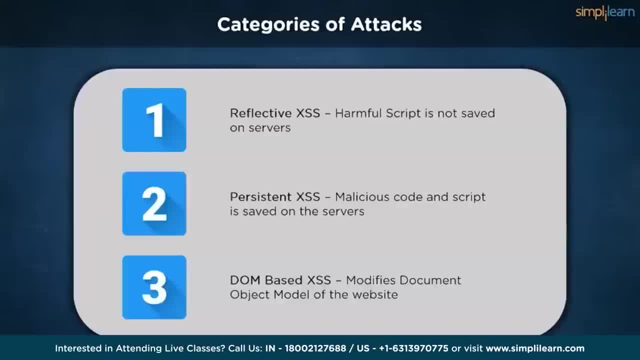 The third variant is DOM-based cross-site scripting attacks. This type of attack occurs when the DOM environment is being changed, but the client-side code does not change. When the DOM environment is being modified in the victim's browser, the client-side code executes differently. 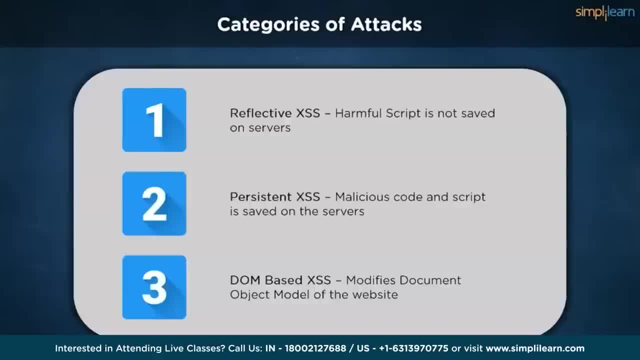 In order to get a better understanding of the client-side code. the client-side code executes differently. In order to get a better understanding of how XSS DOM attack is being performed, let us analyze the following example. If there is a website called textincom, we know default is a parameter. 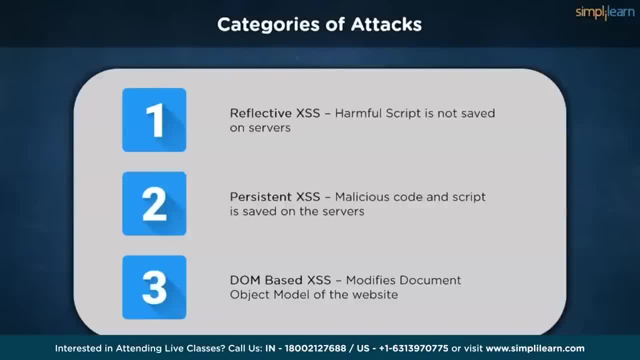 Therefore, in order to perform XSS DOM attack, we should send a script as parameters. A DOM-based XSS attack may be successfully executed even when the server does not embed any malicious code into the web page by using a flaw in the JavaScript executed in the browser. 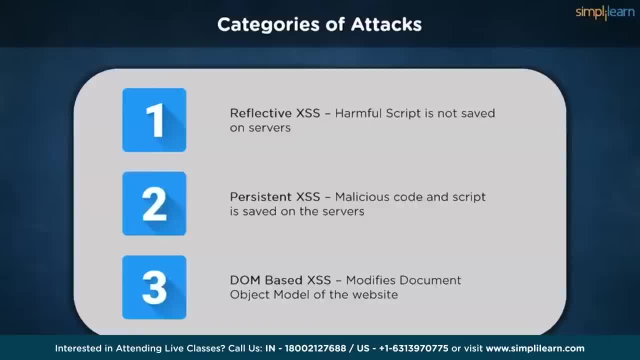 For example, if the client-side JavaScript modifies the DOM tree of the web page, it can be based on an input field or the GET parameter, without validating the input. This allows the malicious code to be executed- The malicious code that exploits flaws in the browser on the user side and the script. 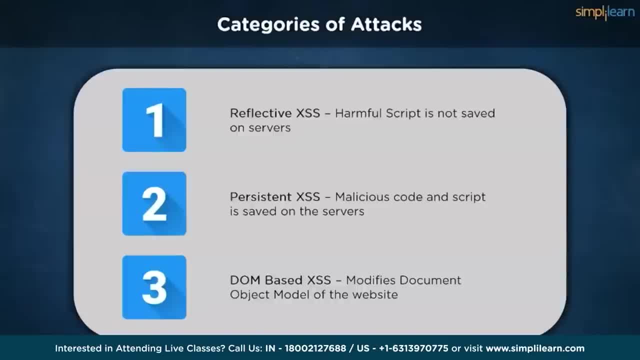 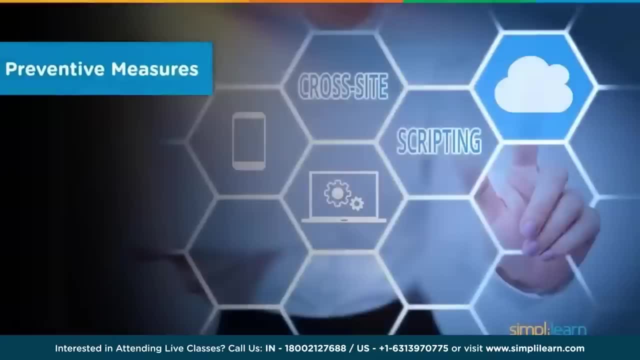 and the attack is not necessarily visible on the server side or to the app owner. By now it is clear that cross-site scripting attacks are difficult to detect and even tougher to fight against. However, plenty of ways one can safeguard against such attacks. 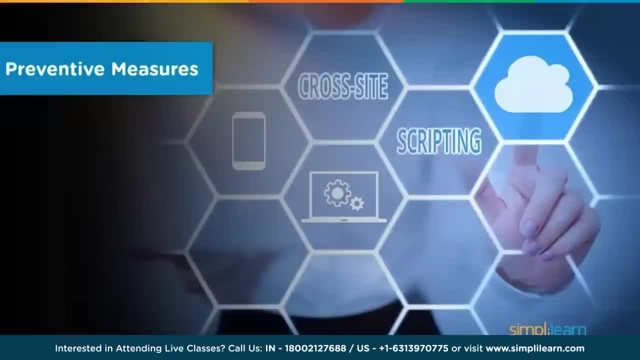 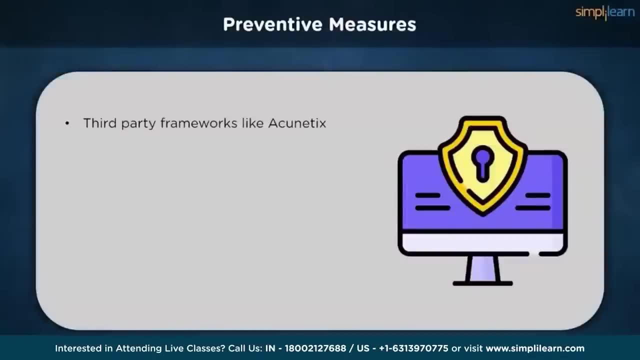 Let's go through some of these preventive measures. Like mentioned earlier, XSS attacks are sometimes difficult to detect. However, this can be changed if you get some external help. A way to prevent XSS attacks is using automated testing tools like Crashtest Security Suite. 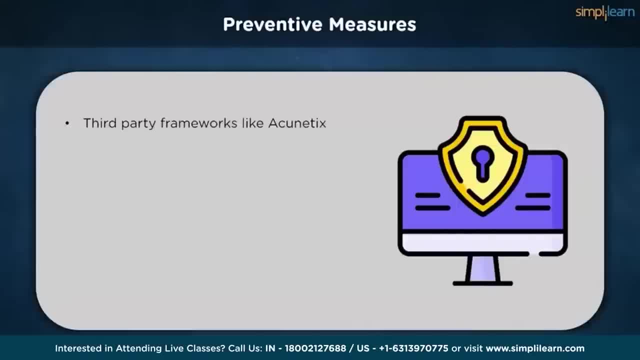 or Acunetix Security Suite. Still, manual testing is highly time-consuming and costly, and therefore not possible to be done for every iteration of your web application. Consequently, your code shouldn't be untested before any release. Using automated security, you can scan your web application for cross-site scripting and. 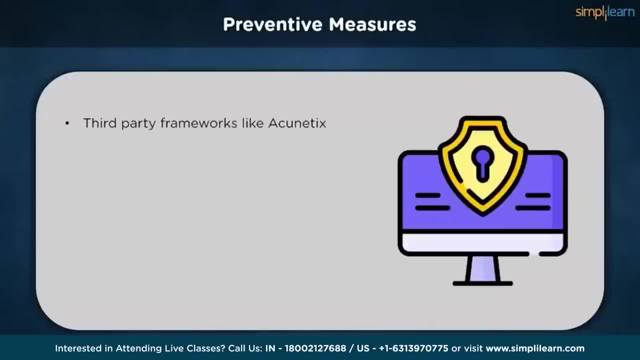 other critical vulnerabilities before every release. This way, you can ensure that your web application's live version is still secured whenever you alter or add a feature. Input fields are the most important. This is the most common point of entry for XSS attack scripts. 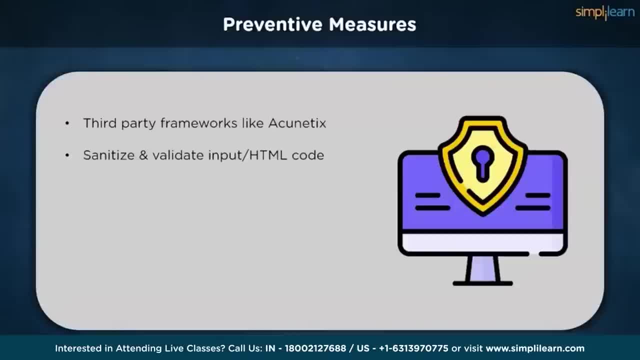 Therefore, you should always screen and validate any information input into data fields. This is particularly important if the data will be included as HTML output. This can be used to protect against reflected XSS attacks. Validation should occur on both the client side and server side as an added precaution. 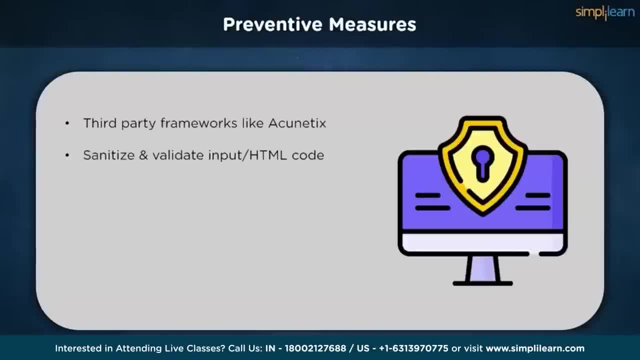 This helps validating the data before it's being sent to the servers and can also protect against persistent XSS scripts. Thanks for watching. This can be accomplished using JavaScript. XSS attacks only appear if any user input is being displayed on the web page. Therefore, try to avoid displaying any untrusted user input if possible. 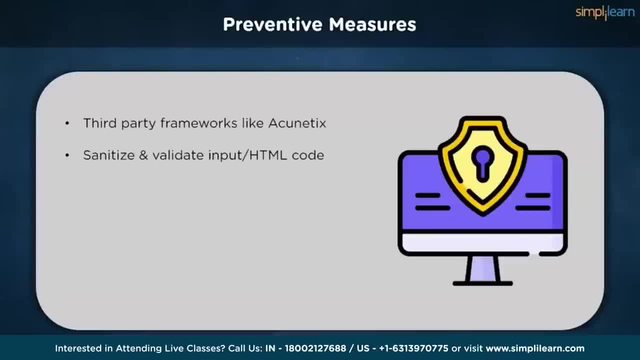 If you need to display user data, restrict the places where the user input might appear. Any input displayed inside a JavaScript tag or a URL shown on the site is much more likely to be exploited than the input that appears inside a division or a span element inside. 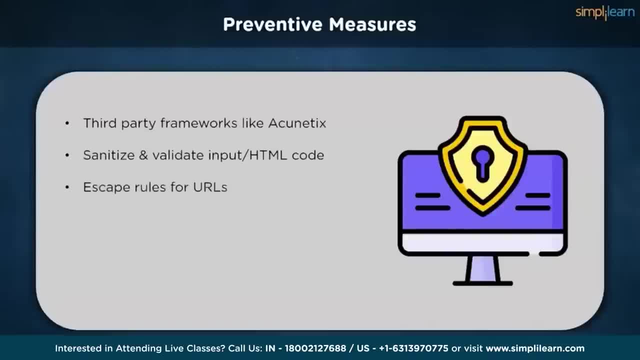 the HTML body. Protecting against XSS vulnerabilities typically requires properly escaping user provided data that is placed on the page. Rather than trying to determine if the data is user provided and could be compromised, we should always play it safe and escape data, whether it is user provided or not. 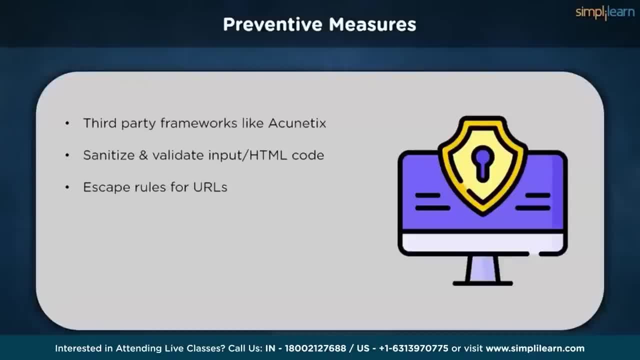 Unfortunately, because there are many different rules for escaping, you still must choose the proper type of escaping before settling on a final code. 7. Encoding should be applied directly before user controllable data is written to a page, because the context you're writing into determines what kind of encoding you need to use. 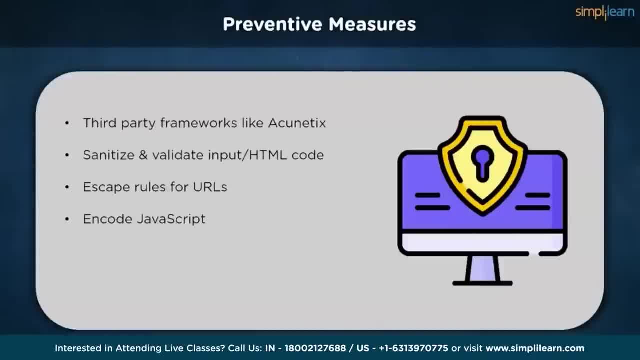 For example, values inside a JavaScript string require a different type of escaping to those in an HTML context. Sometimes you'll need to apply multiple layers of encoding in the correct order, For example, to safely embed user input inside an event handler. you need to deal with both. 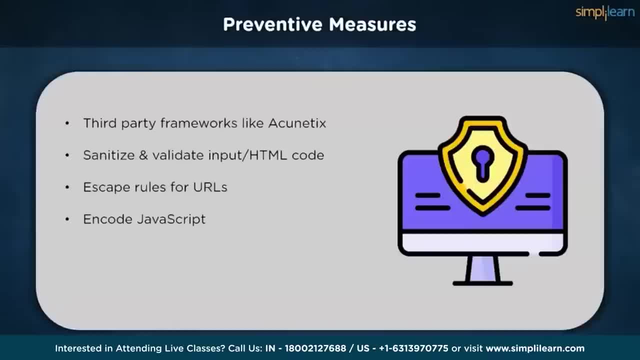 JavaScript context and the HTML context, So you need to first Unicode escape the input and then HTML encode it. Content Security Policy, or CSP, is a computer security standard introduced to prevent cross-site scripting, click-jacking and other code injection attacks resulting from the execution of malicious. 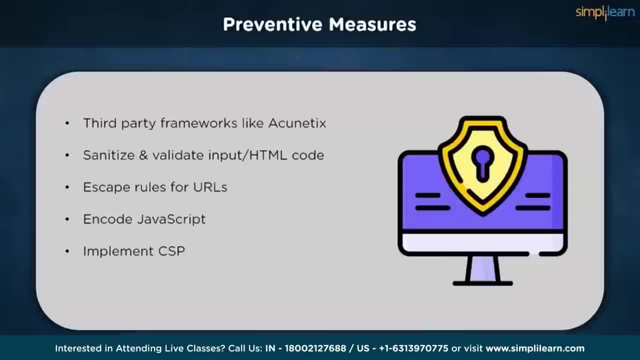 content in the trusted web page context. It is a candidate recommendation of the W3C working group on web application security. It's widely supported by modern web browsers And provides a standard method for website owners to declare approved origins of content that browsers should be allowed to load on that website. 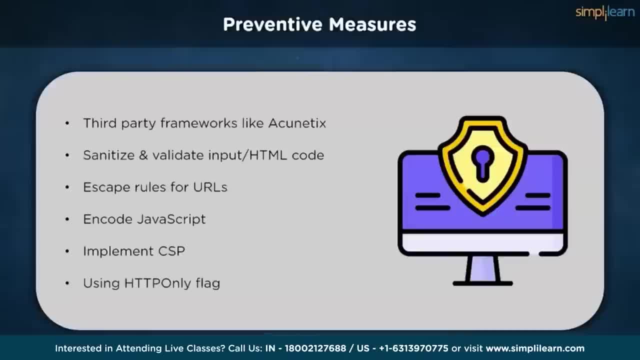 HTTP-only is an additional flag included in a set-cookie HTTP response header. Using the HTTP-only flag when generating a cookie helps mitigate the risk of client-side script accessing the protected cookie, that is, if the browser supports it. If the HTTP-only flag is included in the HTTP response header, the cookie cannot be accessed. 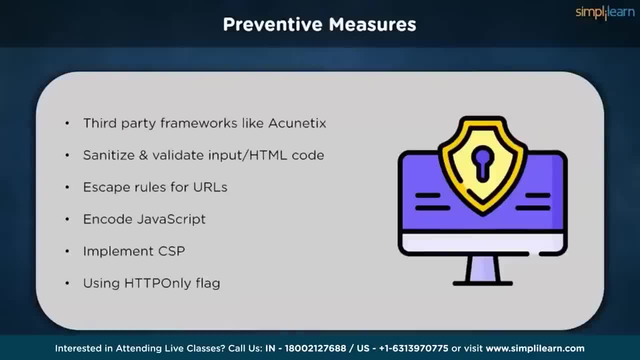 through a client-side script. again, this is if the browser supports this flag. As a result, even if a cross-site scripting flaw exists and a user accidentally accesses a link that exploits this flaw, the browser will not reveal the cookie to a third party. 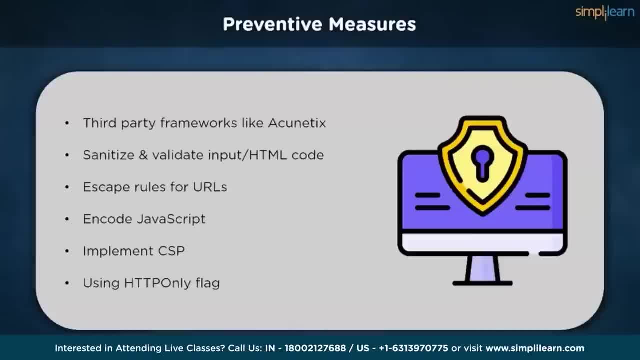 If a browser does not support HTTP-only and a website attempts to set an HTTP-only cookie, the HTTP-only flag will be ignored by the browser, thus creating a traditional script-accessible cookie. As a result, the cookie becomes vulnerable to theft of modification by any malicious. 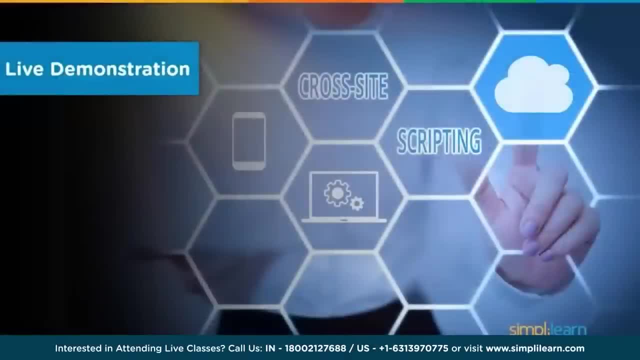 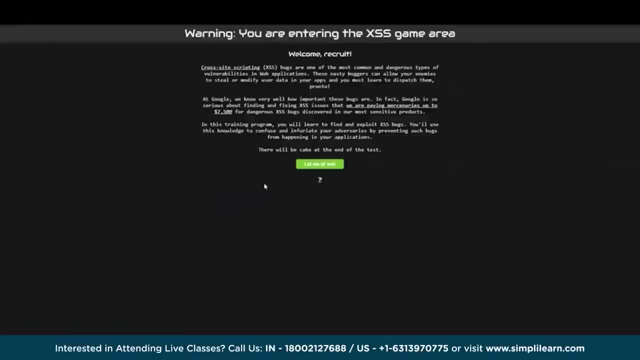 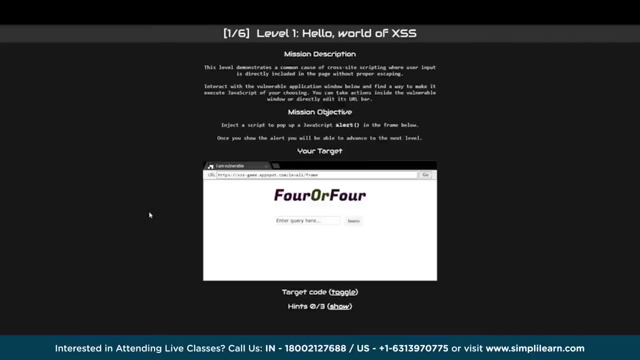 script. Next on our docket is a live demonstration where we solve a set of cross-site scripting problems, starting from the basic level to the topmost level 6. We are going to start at level 1.. In this verb application, it demonstrates a common cause of cross-site scripting, where 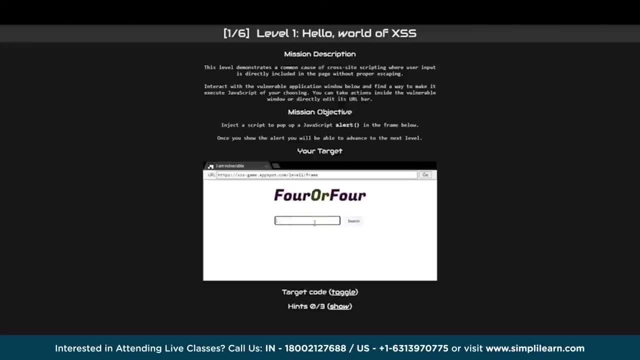 user input is directly included in the page without proper escaping. If we interact with the Vulnerable Application window here and find a way to make it execute JavaScript of our choosing, we can take actions inside the Vulnerable window or directly edit its URL bar. 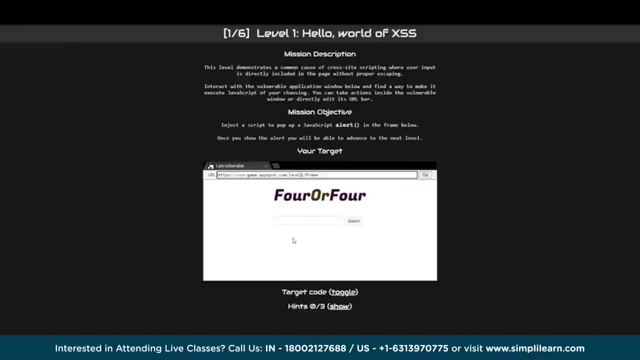 This task needs only basic knowledge. Let's see why the most primitive injections work here right away. Let's do a simple query and inspect the resulting HTML page. I'm going to use this phrase. Let's do. it is with a single quote as a special character. 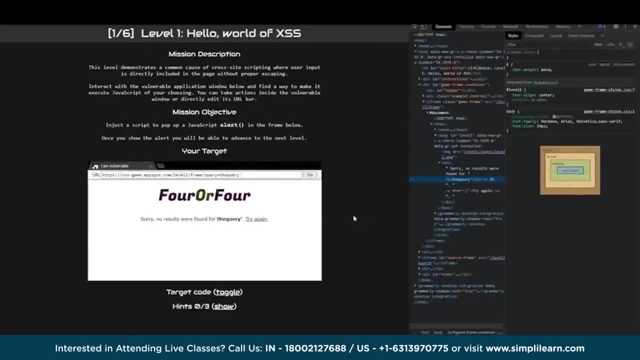 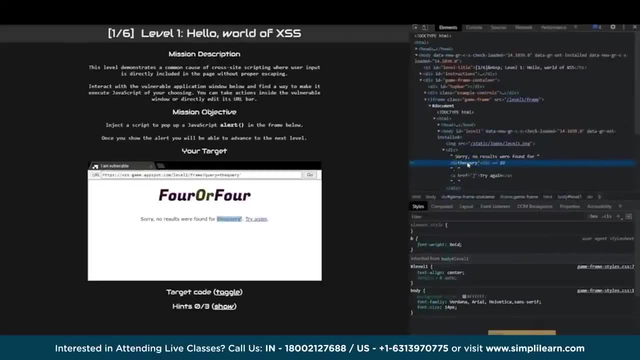 We can now inspect the HTML page. We can see here in this line, the special character single quote appears in the result over here. The provided query text is placed directly in a tag as in a body element. We need to perform a reflected XSS into the web application because they are non-persistent. 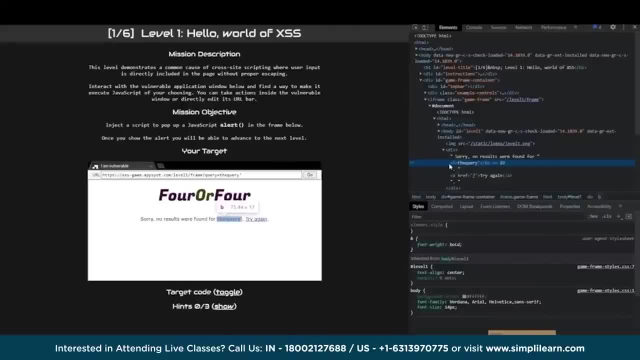 XSS attacks and the payload should be included in the URL to perform successful exploitation. We can use any payload, but we're going to use the simple one to perform an alert in this web application. It's simple and can be shown easily. We're just going to write the script. 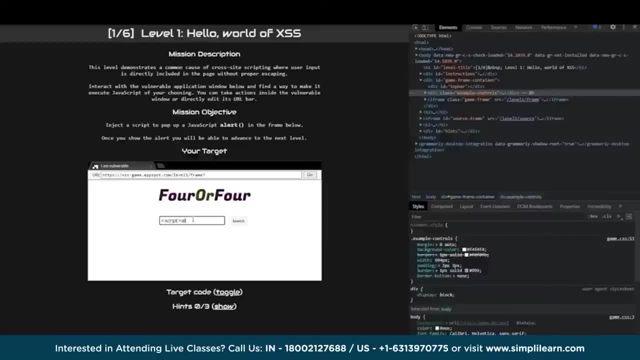 Select over here and we're going to press search. As you can see, we have successfully launched our first cross-site scripting attack. We can see an alert box pop up with the necessary message, And a similar process can be used to steal browser cookies and passwords, albeit with. 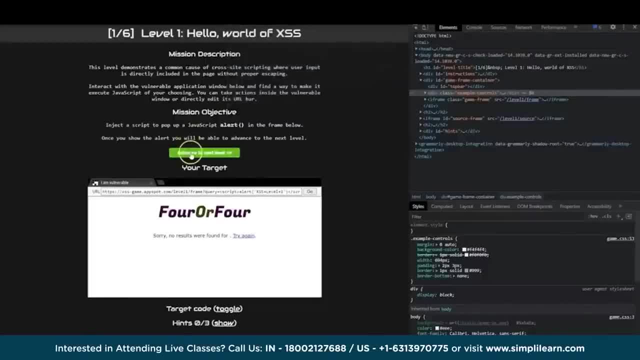 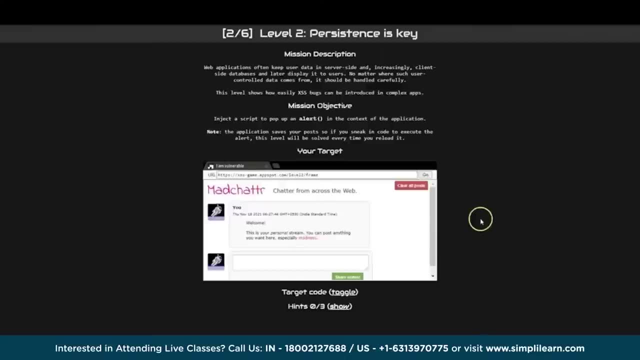 different commands. Now we have the option to move to level two In this web application. it shows that how easily XSS bugs can be introduced in complex chat applications. Chat app conversations are stored in a database and retrieved when a user wants to see the. 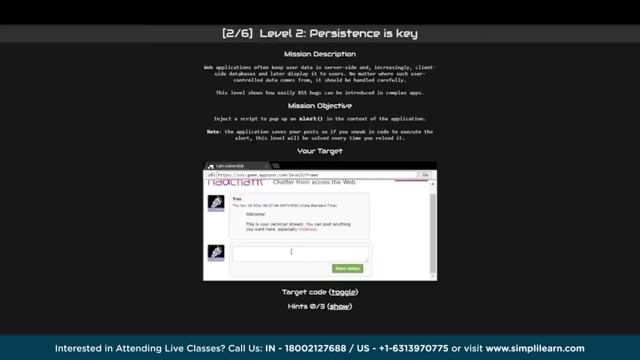 conversation. Therefore, if a malicious user injects some JavaScript code, All visitors will be infected. This kind of cross-site scripting attack is more powerful and it is more riskier than reflected cross-site scripting attacks, and that's why it's known as stored XSS. 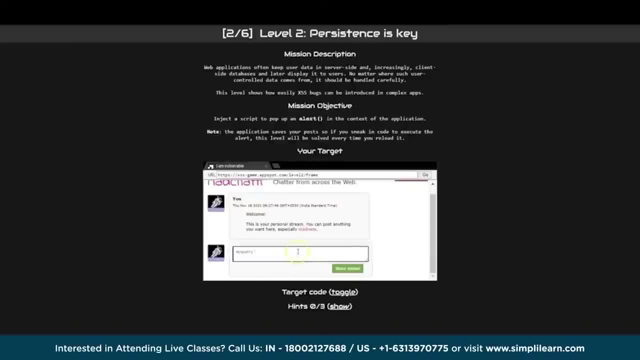 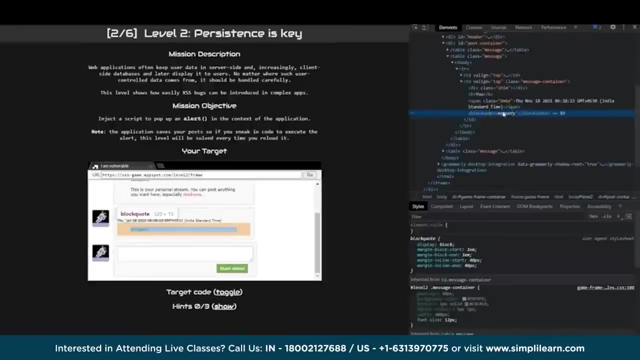 I posted my query with a special character of a single quote and this is what I get. Whatever I typed in simply appeared on the page right after I click on share status. Let's see the source You can see here. the text I posted seems directly put inside a block code tag. 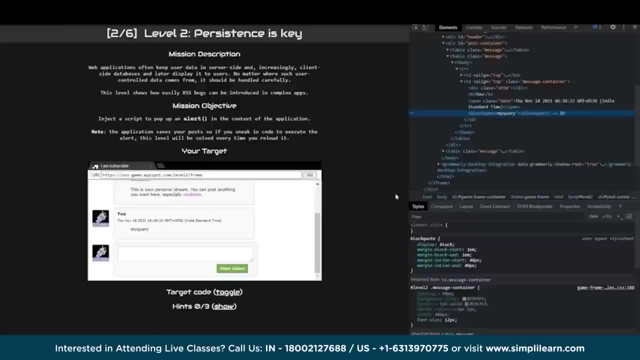 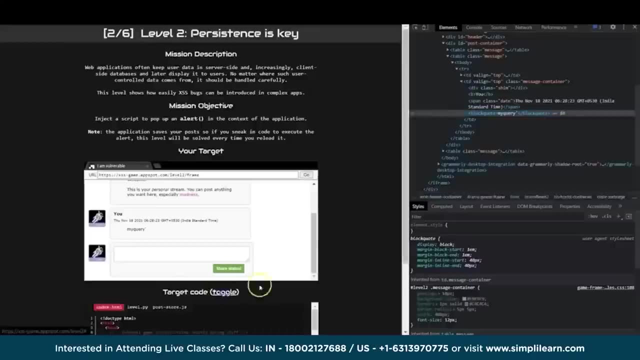 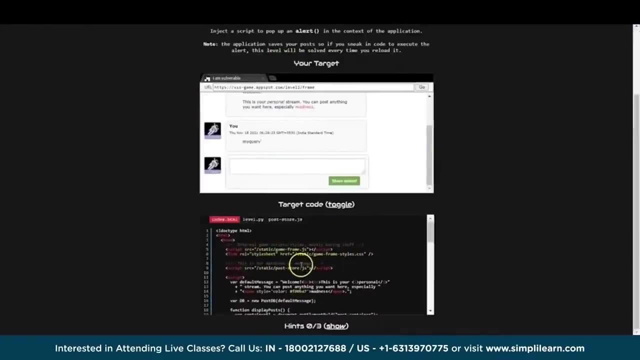 So even a simple script tag we used in level one should work here, but it will not. Let us examine the code to understand why. We're going to toggle the code over here and check the indexhtml file. Important part is line 32.. 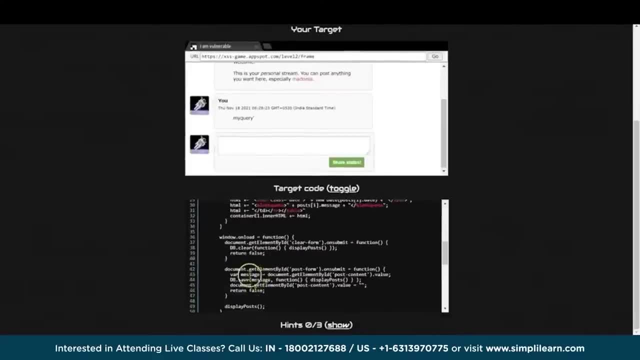 The generated HTML fragment, which is the HTML variable in the code, is added to the male HTML using the inner HTML method. So when the browser parsing this HTML fragment, it will not execute any script tag defined within that HTML fragment. HTML parser will not execute a script tag when it parses HTMLs via this method. So what happens is the header is treated in yell, but the HTML tag is not here in the HTML tag. So the HTML tag is here in the HTML tag. So when the browser parses this HTML method, it is also considered a script tag, and this has beenoperation for the HTML tag's. 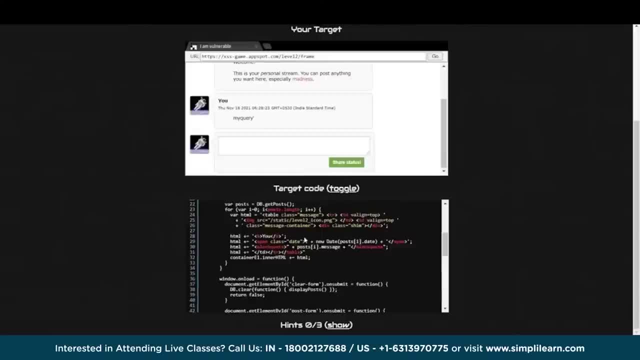 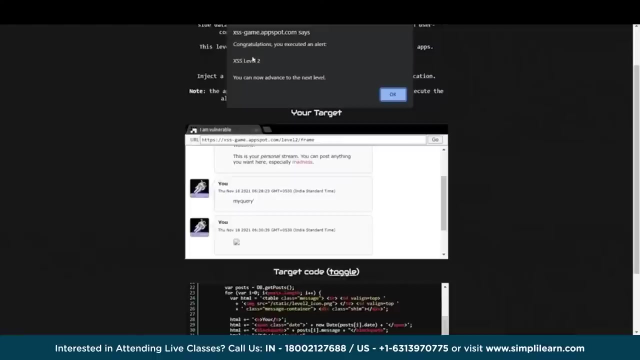 This is why the script tag, like we used in level 1, is not going to work here. Our solution is to use events. Events will execute the defined JavaScript. We're going to use an image over here. When we press on share status in the above injection, we are loading an image that doesn't. 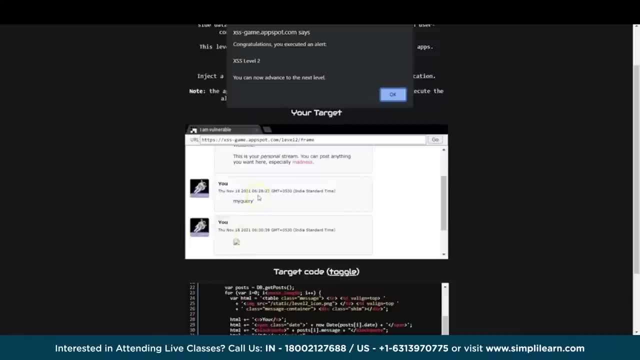 exist which causes to trigger an onError event. In onError event, it will execute our alert method. With that, we are able to beat level 2.. We can now move up to the next step. We can now move up to the next level in our challenge. 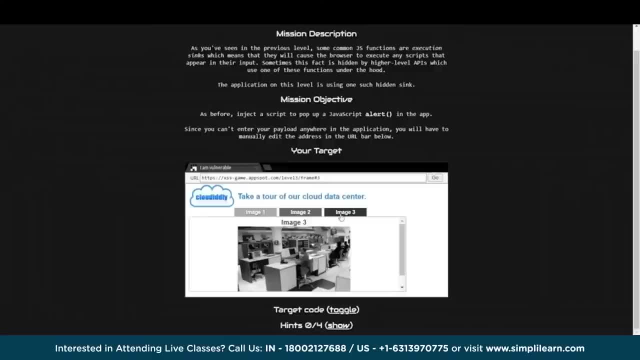 As you can see, clicking on any tab causes the tab number to be displayed in the URL fragment. This hints that the value after the hashtag controls the behavior of the page. That is, it is an input variable. To confirm, let's analyze the code. 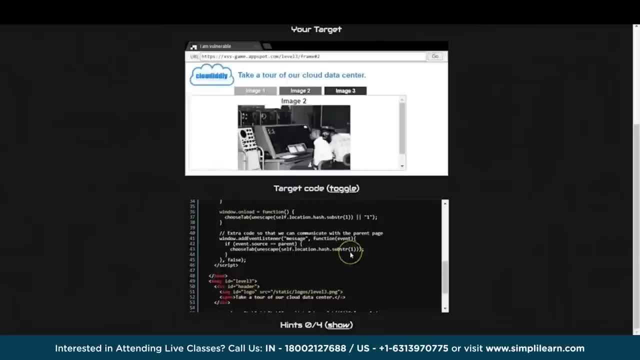 As you can see in line 43, inside the event handling, the value provided after the hash in the URL is directly passed onto the true tab method. No input validation is being performed. The value passed to the choose tab method is directly injected into the img tag in line. 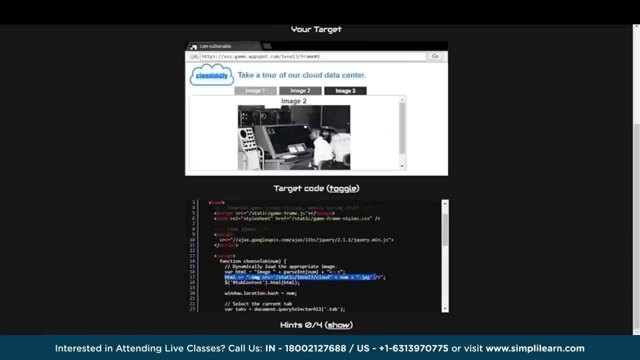 17.. This is an unsafe assignment and it is the vulnerable part of the code. So let's see how it works Now. all we have to do now is to craft a payload that would adjust the img tag to execute our JavaScript. 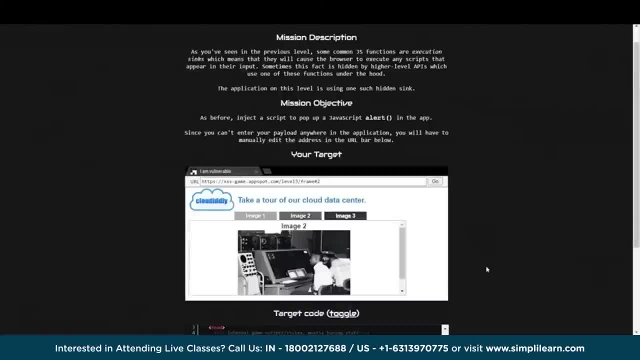 Remember, the script tag from level 1 would not work here, since the variable HTML is used to add the DOM dynamically. hence the events are our aces here. once again, I will choose to use the existing img tag and change the source to something that doesn't. 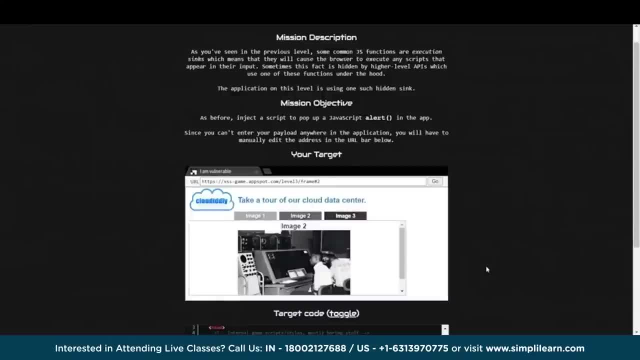 exist, hence forcing it to fall in to execute an onError event which I will pass the img tag to. In this case, I will pass the url. Once we visit that url, we can see that our java popup has opened up here with the same. 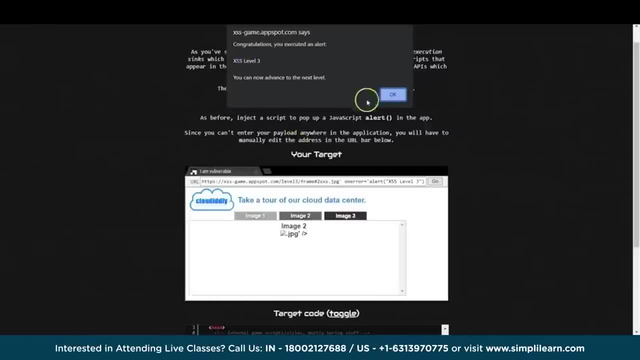 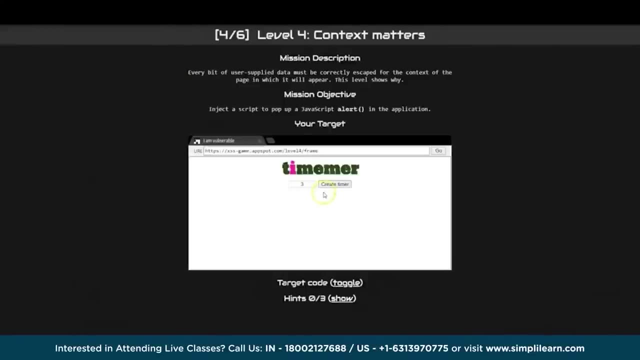 message of XSS. level 3 has been completed. With this, we can now move on to level 4, which is going to present a different kind of attack. In this server application, there is a timer on the page. that means whatever numbers we. 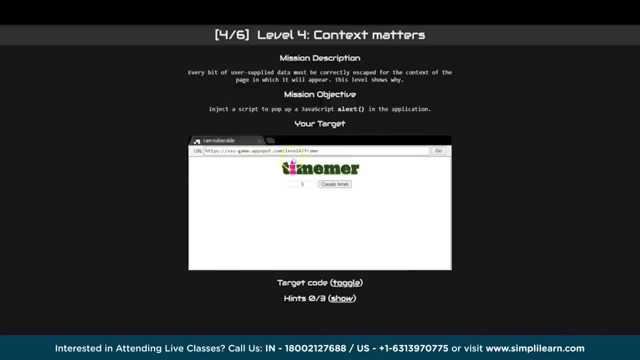 put in the box, a countdown will take place. The countdown starts and then, when it finishes, the application alerts that the countdown is finished And we can see the timer popup appearing over here and this resets the timer again. Now it is obvious that the value entered in the text box is transferred to the server. 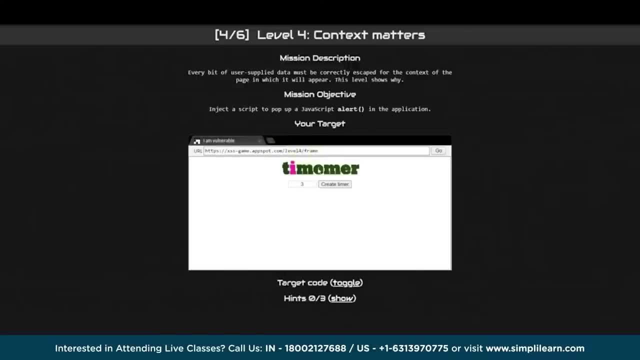 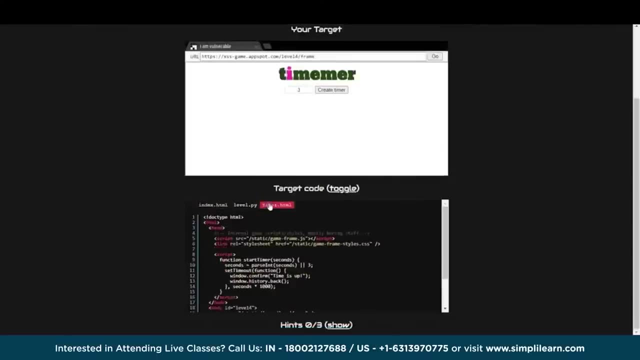 over the timer parameter in the url. Let us examine the code to see how the timer parameter is being handled. We're going to visit timerhtml Over here and we're going to check over here in line 21,. the start timer method is: 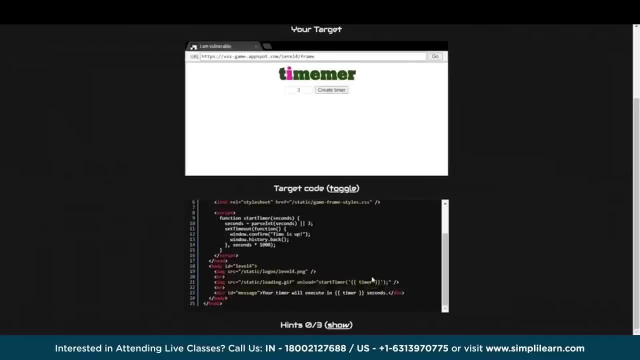 being called in the on load event. However, the timer parameter is being directly passed to the start timer method. We need to perform a popup alert in the web application which escapes the content of the function start timer without baking the java script code. the parameter value is directly. 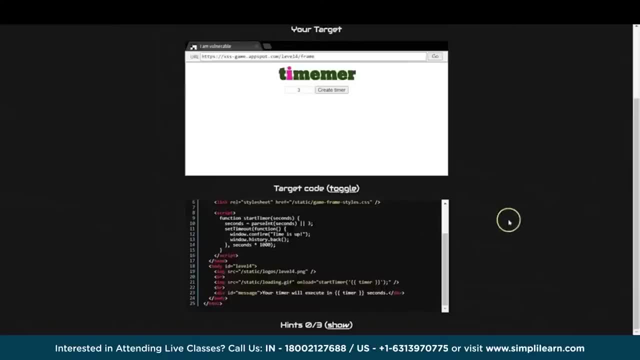 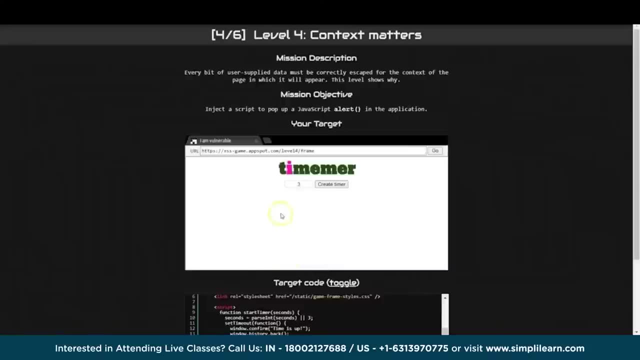 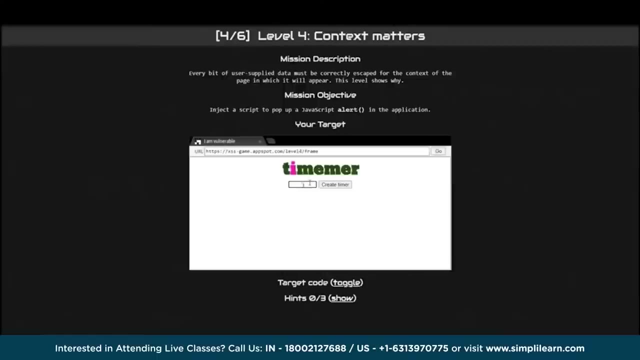 added timer method without any filtering. What we can try to do here is to inject an alert function to be executed inside the onLoan event along with the start timer method. We're going to remove this argument and put our script over here. Now let me press on create timer and we have a pop-up with the XSS level 4. 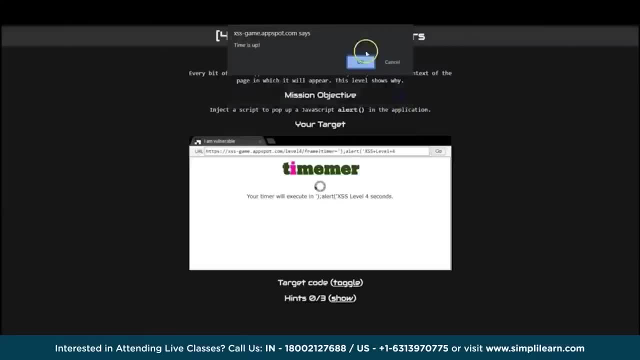 completed, We can now move on to level 5.. In this web application, this application, XSS, is different because this challenge description says cross-site scripting isn't just about correctly escaping data. Sometimes attackers can do bad things even without injecting new elements into the DOM. It's kind of open redirect, because the attack payload is 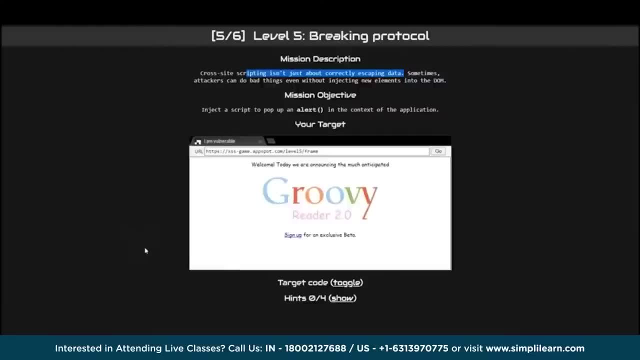 executed as a result of modifying the DOM environment in the victim's browser. This environment is used by the original client-side script so that the client-side code runs in an unexpected manner. The vulnerability can be easily detected if the next link in the signup page is inspected. 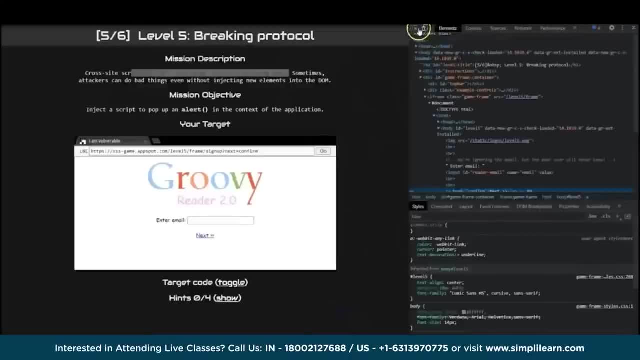 Now let's see how this works. The HREF attribute value of next link is confirm, which is exactly the value of the next URL query parameter. as you can see over here, This means using the next query parameter can be used to inject a JavaScript code to the HREF attribute. 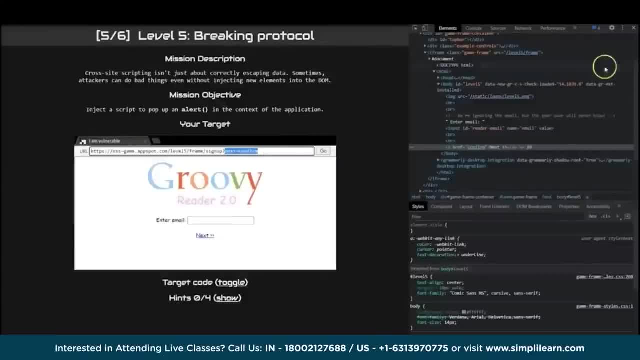 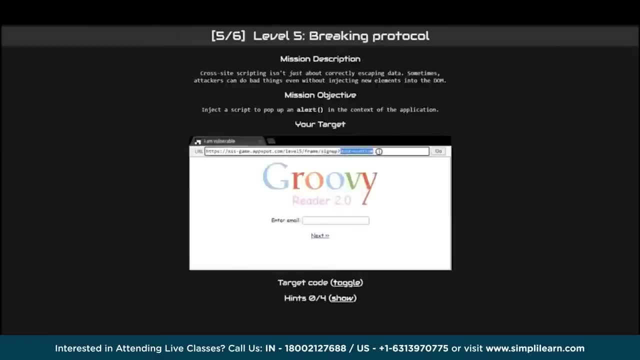 of the next link. The following is the best way to do it: As soon as the user clicks on the link, the script will be triggered. The command that i used is item cleanser, and the user will get a webinar called in� the chapter intrinsic to it. 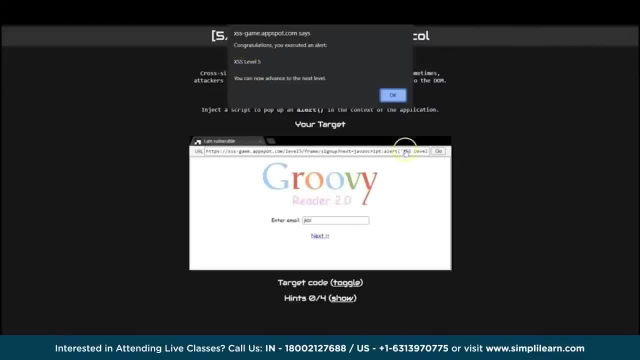 We are going to press anything random and now that we click next, we can see the XSS Level-5 that we had provided in the URL as a parameter to the next variable. Since the value of next provided appears in a pop up, we can consider the attack. 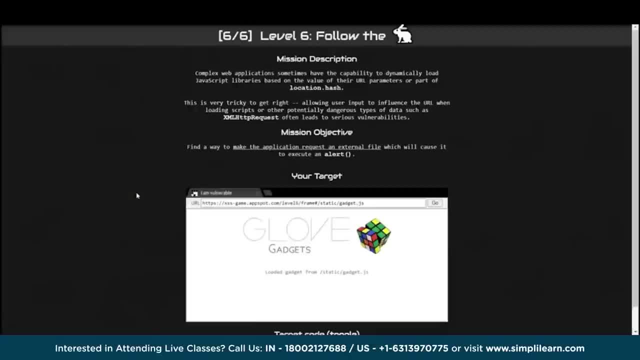 a success and move on to the final level, 6.. In this server application it shows some of the excuse if your external JavaScript is streeted. Plans issued these days support custom organizers for some of your existing URL. you can see that the script is loaded already. 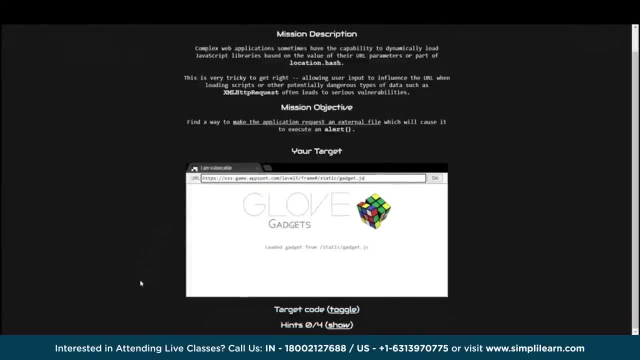 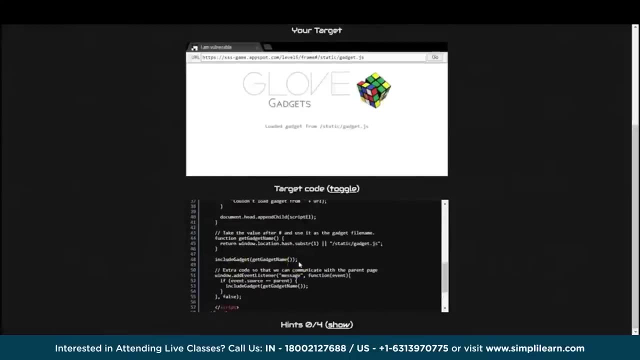 The vulnerability lies within how the code handles the value after the hashtag. If you check on line 45, the value right after the hashtag is taken as the gadget name And then in line 48, the value is directly passed on to the includeGadget method and 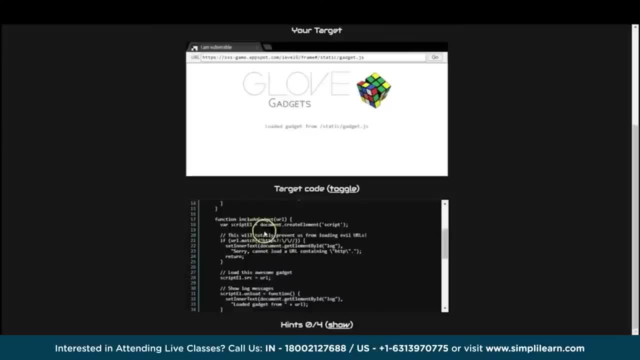 the includeGadget method that we can see over here. You can see in line 18, a script tag is created and the URL gadget name parameter value is directly used as the source attribute of the script tag in line 28.. This means we can completely control the source attribute of the script tag that is being 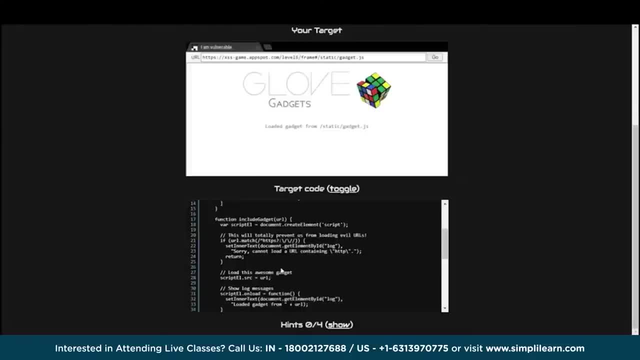 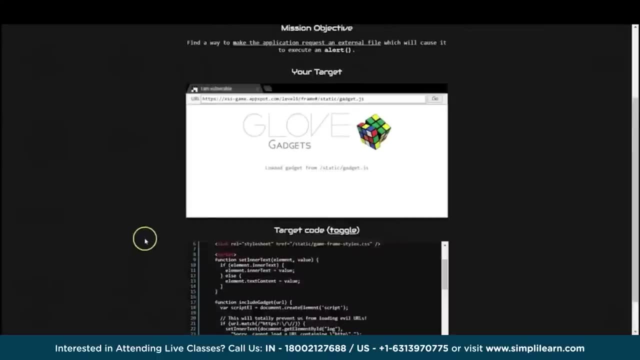 created, That is, with this vulnerability. we can inject our own JavaScript file into the code. We can inject a URL of our own. We can inject a URL of our own. We can inject a URL of our own hosted JavaScript into the web applications URL after the hashtag. 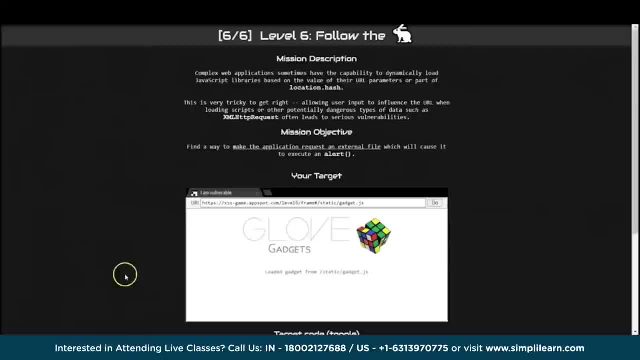 and the URL should not be using HTTPS but anything like that to bypass the regular expression for security checking. Going to remove the pre-stored URL and we're going to load our own JavaScript file. Finally, we have reached the end of our challenge. 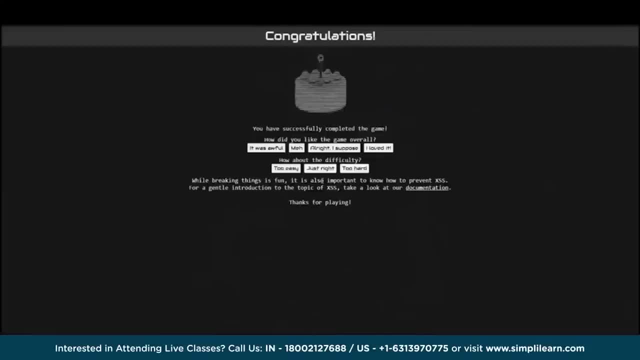 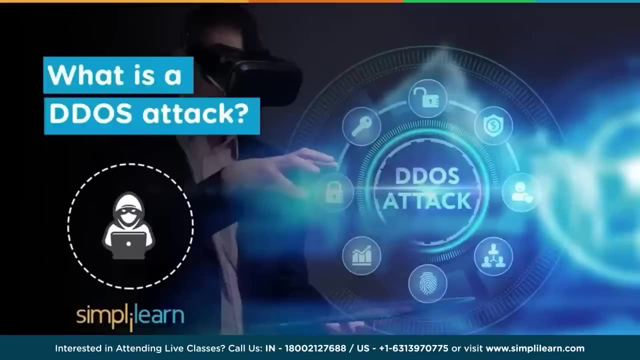 Completed six different varieties of cross-scripting attacks and used different solutions for all of the six questions. With work from home being the norm in today's era, people spend considerable amount of time on the internet, often without specific measures to ensure a secure session. 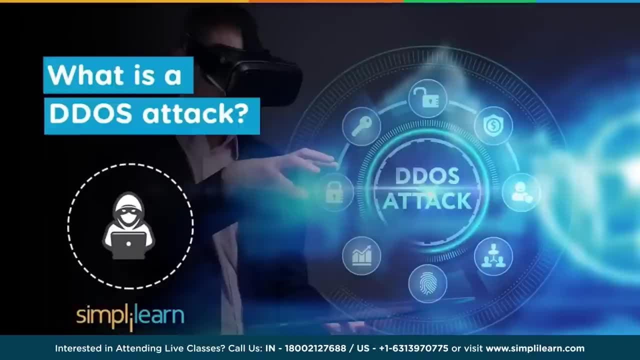 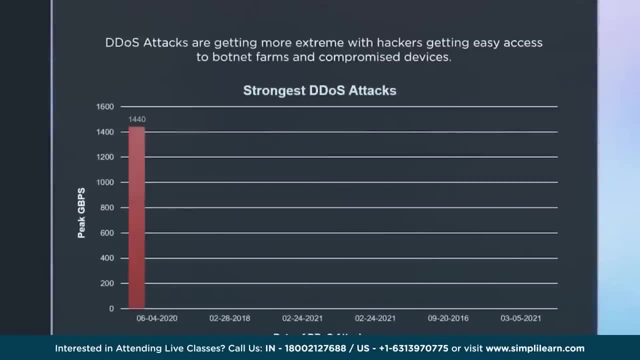 Apart from individuals, organizations worldwide that host data and conduct business over the internet are always at the risk of a DDoS attack. These DDoS attacks are getting more extreme, with hackers getting easy access to botnet farms and compromised devices. As can be seen in the graph, three of the six strongest DDoS attacks are being used to. 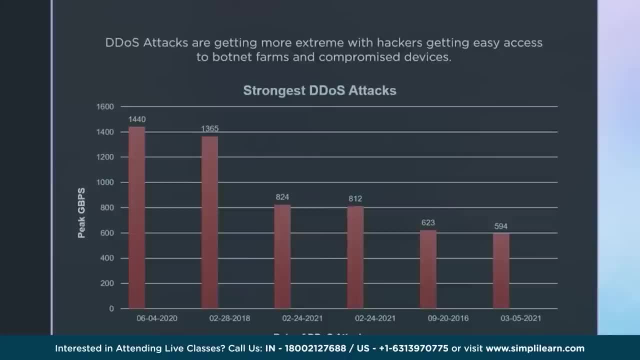 counter DDoS attacks. These DDoS attacks were launched in 2021, with the most extreme attack occurring just last year in 2020.. Lately, cybercriminals have been actively seeking out new services and protocols for amplifying these DDoS attacks. 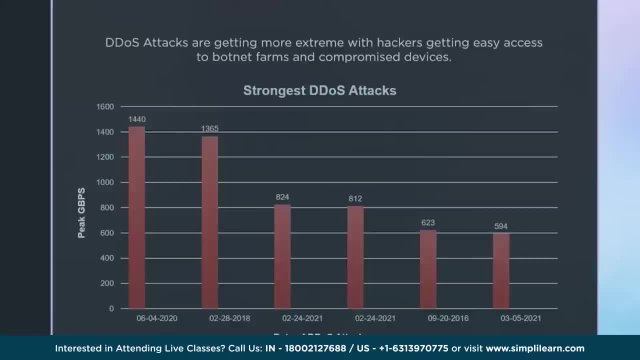 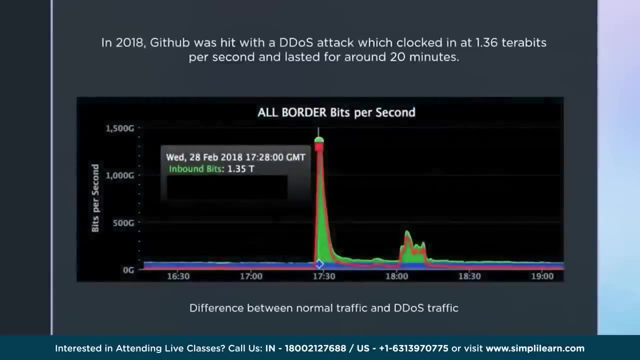 Active involvement with hacked machines and botnets allow further penetration into the consumer space, allowing much more elaborate attack campaigns. Apart from general users, multinational corporations have also had their fair share of problems, GitHub, for example. GitHub, a platform for software developers, was the target of a DDoS attack in 2018.. 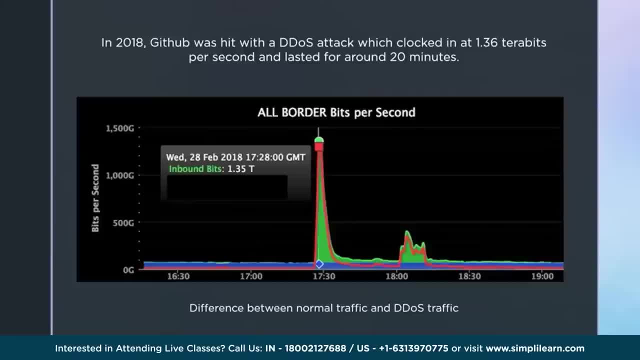 Widely suspected to be conducted by Chinese authorities. this attack went on for about 20 minutes, after which the systems were brought into a stable condition. It was the strongest DDoS attack to date at the time, and made a lot of companies reconsider. 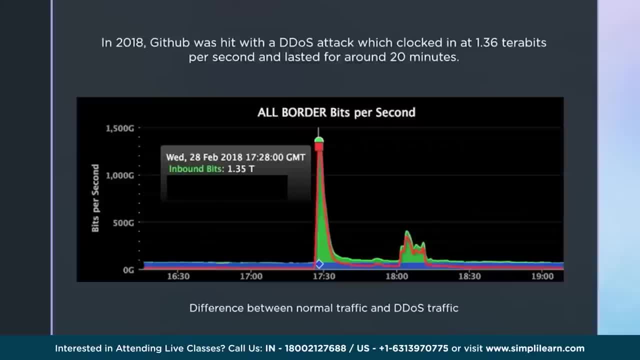 their security practices to combat such attacks. Even after years of experimentation, DDoS attacks are still at large and can affect anyone in the consumer and corporate world. Hey everyone, this is Baibab from Simply Learn, and welcome to this video on what is. 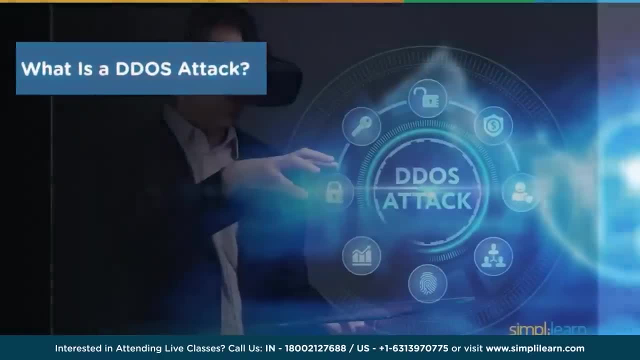 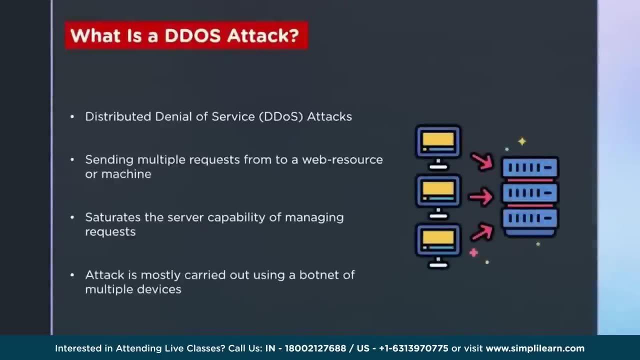 a DDoS attack. Let's learn more about what is a DDoS attack. A Distributed Denial of Service attack, or DDoS, is when an attacker or attackers attempt to make it impossible for a service to be delivered. This can be achieved by thwarting access to virtually anything – servers, devices, services. 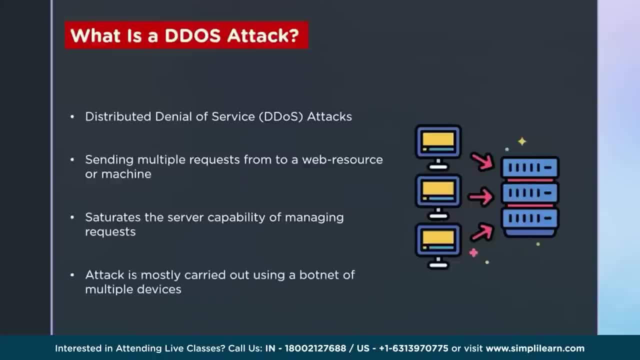 networks, applications and even specific transactions. DDoS attacks can be achieved by thwarting access to virtually anything – servers, devices, services, networks, applications and even specific transactions. In a DDoS attack, it's one system that is sending the malicious data or requests. 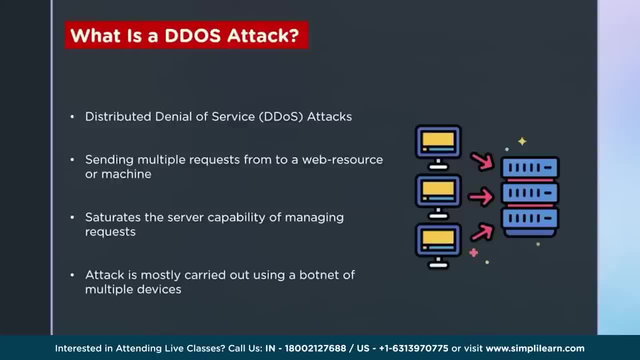 A DDoS attack comes from multiple systems. Generally, these attacks work by drowning a system with requests for data. This could be sending a web server so many requests to serve a page that it crashes under the demand, or it could be a database being hit with a high volume of queries. 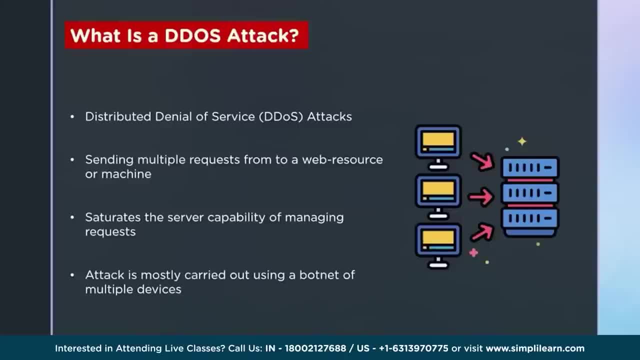 The result is available: internet bandwidth, CPU and RAM capacity become overwhelmed. The impact could range from a minor annoyance from disrupted services to experiencing entire websites, applications or even entire businesses taking offline. More often than not, these attacks are launched using machines in a botnet. 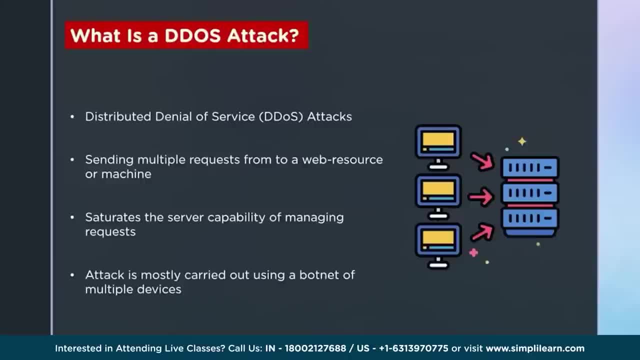 A botnet is a network of devices that can be triggered to send requests from a remote source, often known as the command and control center. The bots in the network attack a particular target, thereby hiding the original perpetrator of the DDoS campaign. 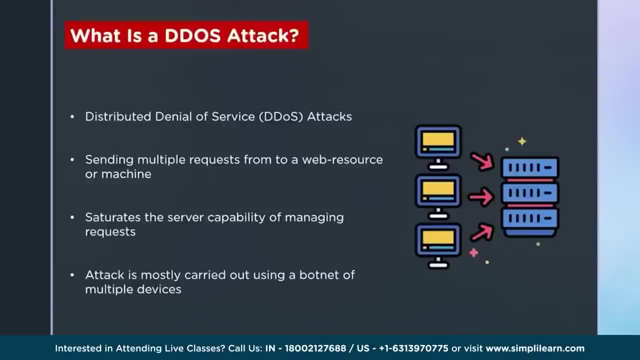 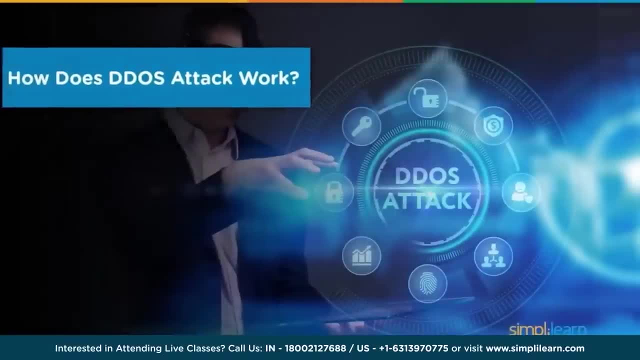 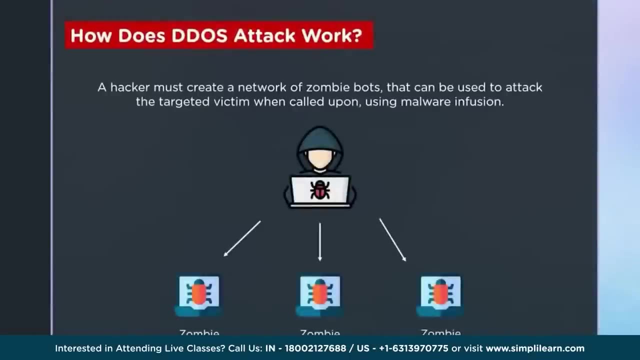 But how do these devices come under a botnet And what are the requests being made to the web servers? Let's learn more about these and how DDoS attack work. A DDoS attack is a two-phase process. In the first phase, a hacker creates a botnet of devices. 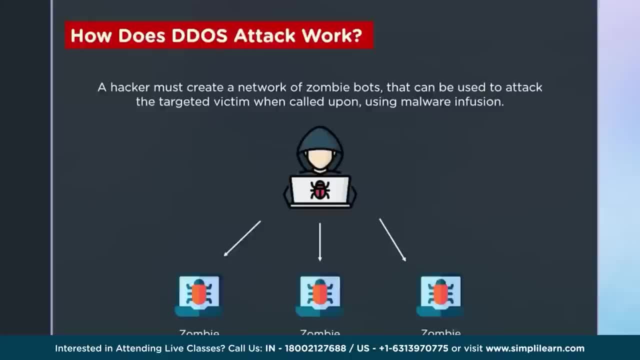 Simply put, a vast network of computers are hacked via malware, ransomware or just simple social engineering. These devices become a part of the botnet, which can be triggered anytime. The botnet is a system that is created by a hacker to start bombarding a system or a. 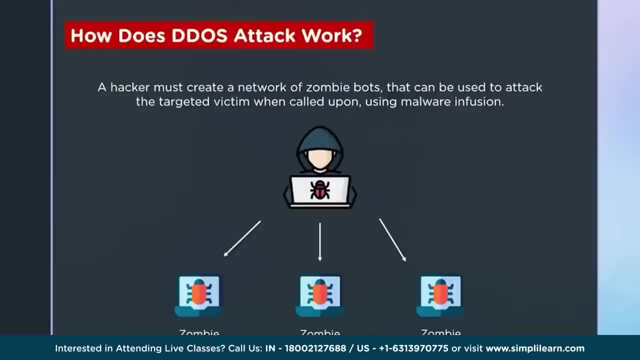 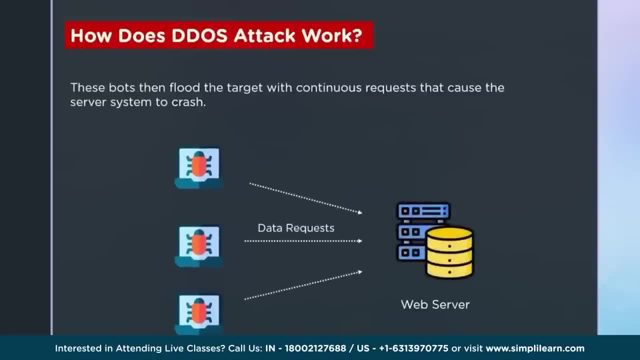 server on the instruction of the hacker that created the botnet. The devices in these networks are called bots or zombies. In the second phase, a particular target is selected for the attack. When the hacker finds the right time to attack, all the zombies in the botnet network, send. 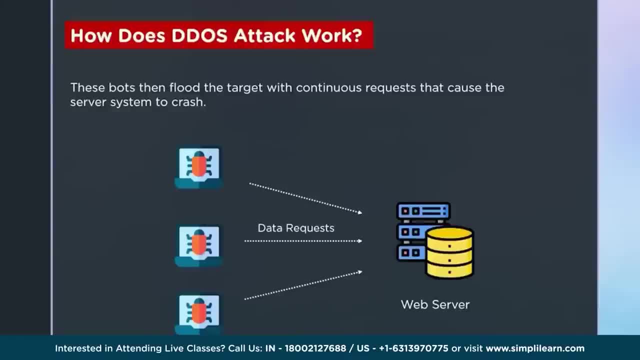 these requests to the target, thereby taking up all the server's available bandwidth. These can be simple ping requests or complex attacks like SYN flooding and UDP flooding. The aim is to overwhelm them with more traffic than the server or the network can accommodate. 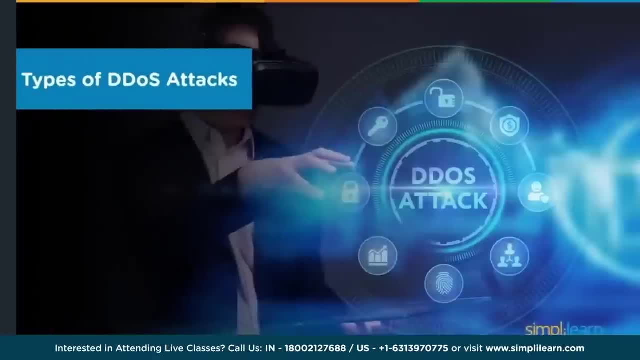 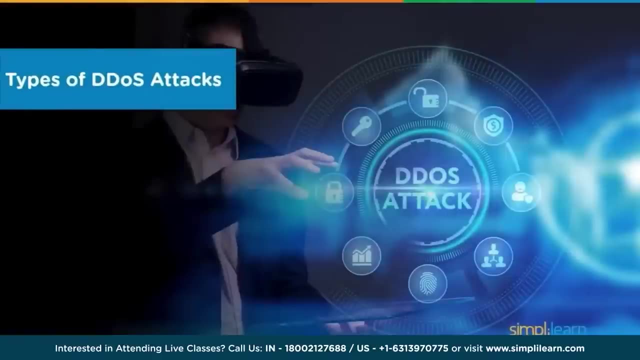 The goal is to render the website or service inoperable. There is a lot of wiggle room when it comes to the type of DDoS attack a hacker can go with, Depending on the target's vulnerability. we can choose one of the three broad categories. 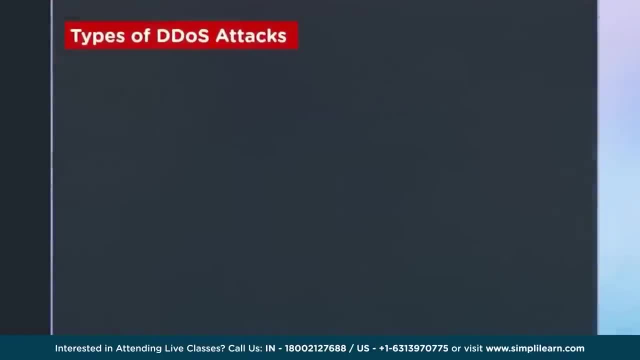 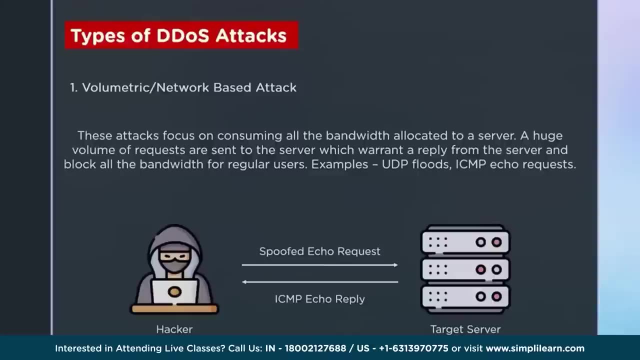 of DDoS attacks. Volume-based attacks use massive amounts of bogus traffic to overwhelm a resource. It can be a website or a server. They increase the number of attacks. They include ICMP, UDAP and spoofed packet flood attacks. The size of volume-based attack is measured in bits per second. 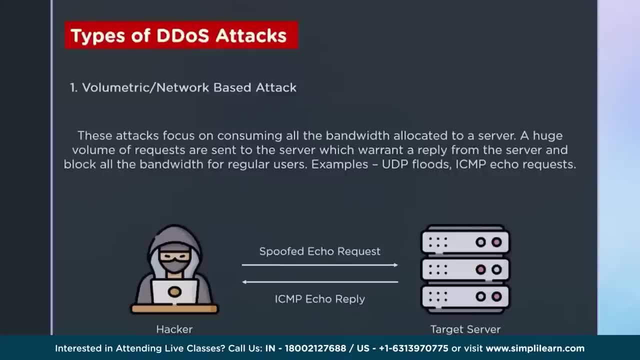 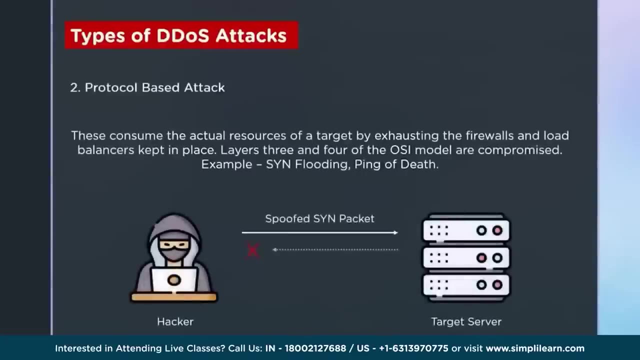 These attacks focus on clogging all the available bandwidth for the server, thereby cutting the supply short. Several requests are sent to the server, all of which warrant a reply, thereby not allowing the target to cater to the general legitimate users. Next we have the protocol-level attacks. 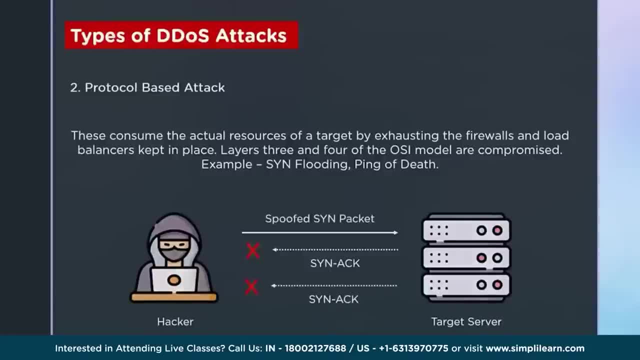 These attacks are meant to consume essential resources of the target. They exhaust the load balancers and firewalls which are meant to protect the system against the DDoS attacks. These protocol attacks include SYN floods and smurf DDoS, among others, and the size. 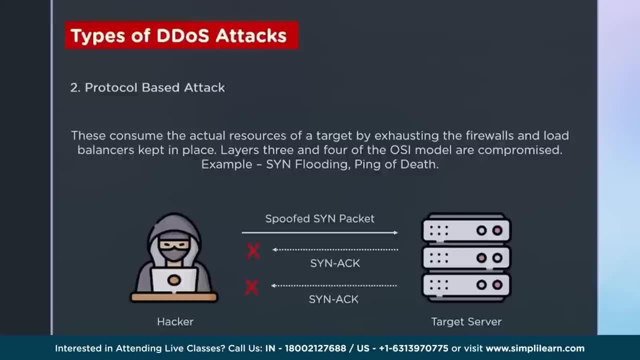 is measured in packets per second. For example, in an SSL handshake server replies to the hello message sent by the hacker, which will be the client in this case. but since the IP is spoofed and leads nowhere, the server gets stuck in an endless loop of sending messages. 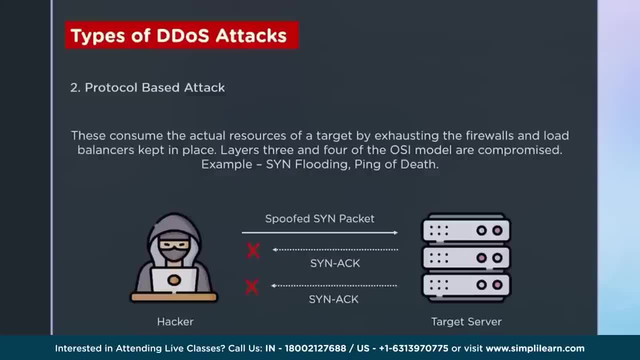 The server then gets stuck in an endless loop of sending messages. This means that the end in site of the application cannot be used. The server will not be able to understand the acknowledgement without any end in site. Next we have the application-level attacks. 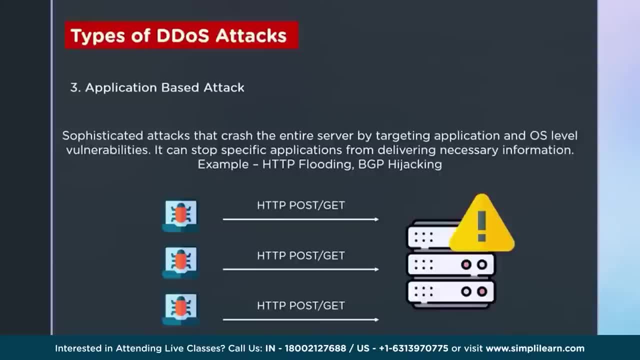 Application-layer attacks are conducted by flooding applications with maliciously crafted requests. The size of application-layer attacks is measured in requests per second. These are relatively sophisticated attacks that target the application and operating system-level vulnerabilities. They prevent the specific applications from delivering necessary information to users. 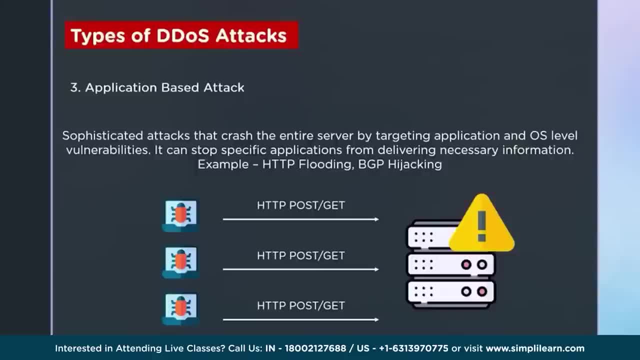 and hog the network bandwidth up to the point of a system crash. Examples of such an attack are HTTP flooding and BGP hijacking. A single device can request data from a server using HTTP POST or GET without any issues. However, when the requisite botnet is instructed to bombard the server with thousands of requests, 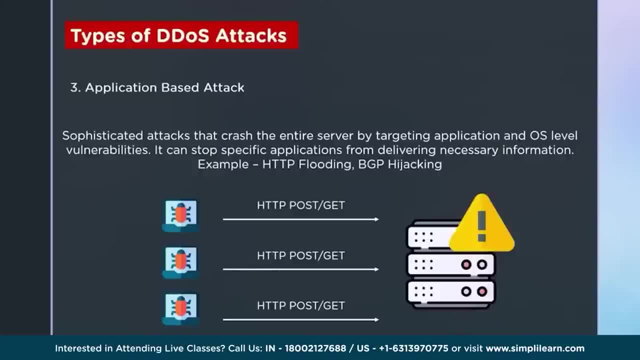 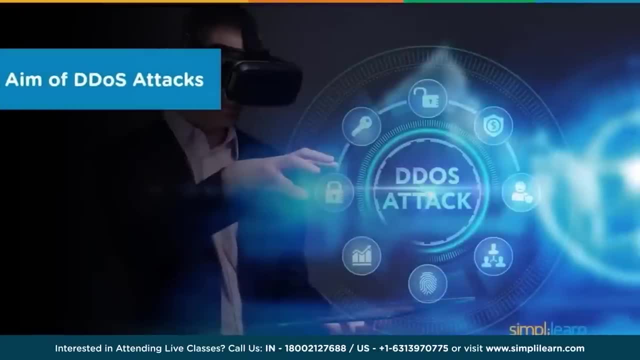 the database, bandwidth gets jammed and it eventually becomes unresponsive and unusable. But what about the reasons for such an attack? There are multiple lines of thought as to why a hacker decides to launch a DDoS attack on unsuspecting targets. Let's take a look at a few of them. 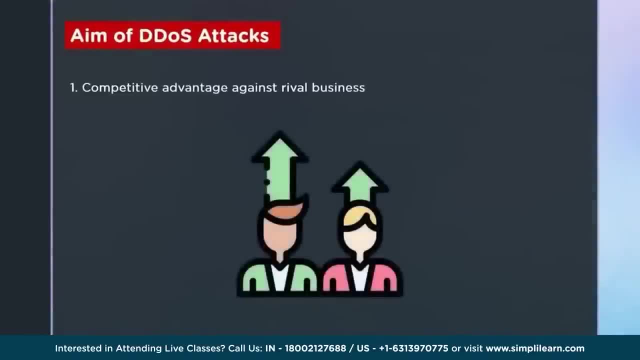 The first option is to gain a competitive advantage. Many DDoS attacks are conducted by hacking communities against rival groups. Some organizations hire such communities to stagger their rival's resources at a network level to gain an advantage in the playing field, Since being a victim of a DDoS attack indicates a lack of security. 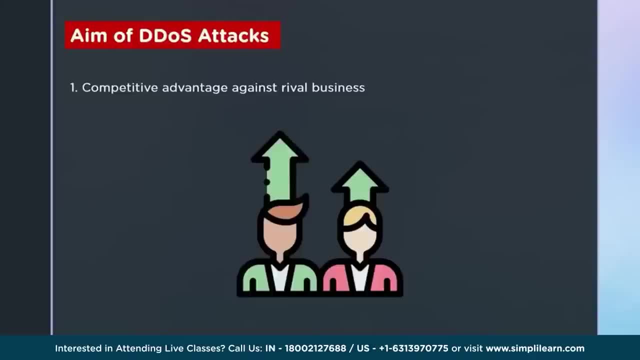 the reputation of a DDoS attacker is reduced. The reputation of such a company takes a significant hit, allowing the rivals to cover up some ground. Secondly, some hackers launch these DDoS attacks to hold multinational corporations at ransom. The resources are jammed and the only way to clear the way is if the target company agrees to pay. 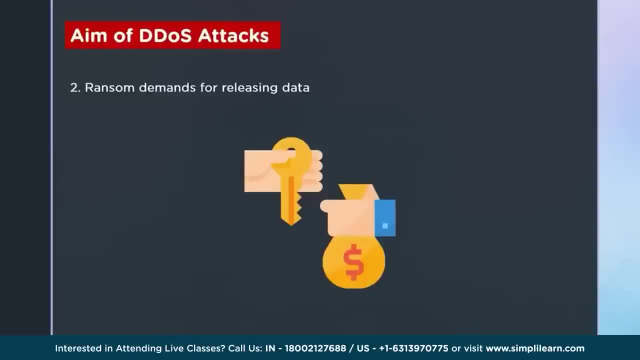 a designated amount of money to the hackers. Even a few minutes of inactivity is detrimental to a company's reputation in the global market and it can cause a spiral effect, both in terms of market value and the impact it has on the company. DDoS attacks are also used in product security index. 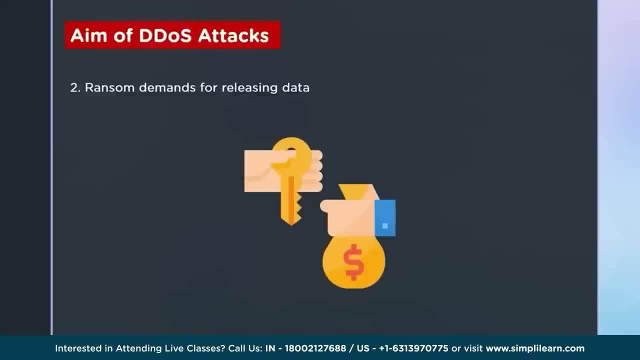 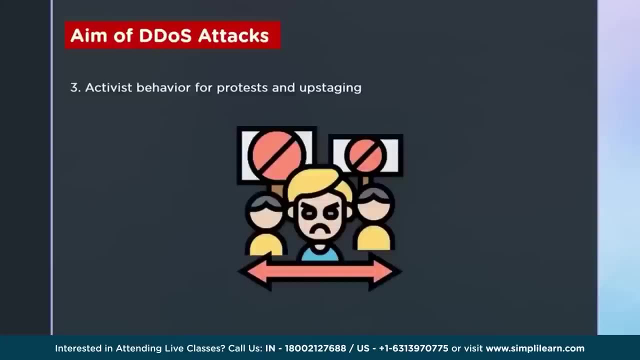 Most of the time, a compromise is reached and the resources are freed after a while. DDoS attacks have also found use in the political segment. Certain activists tend to use DDoS attacks to voice their opinion. Spreading the word online is much faster than any local rally or forum. 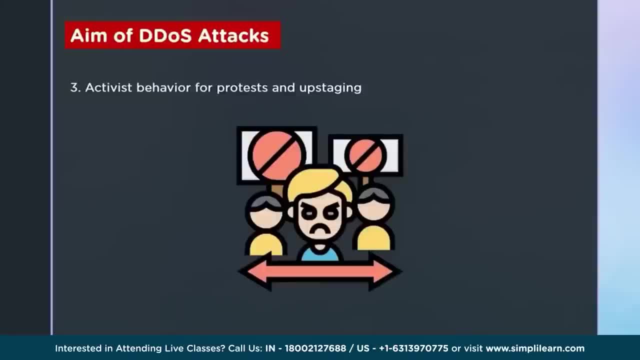 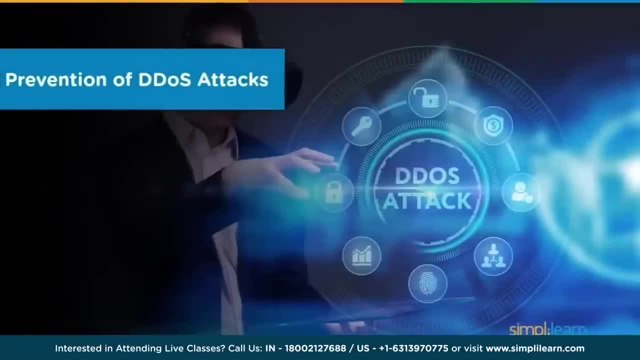 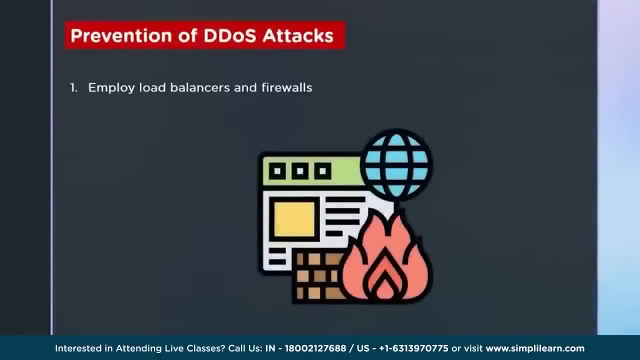 Primarily political, these attacks also focus on online communities, ethical dilemmas or even protests against corporations. Let's take a look at a few of them, a few ways that companies and individuals can protect themselves against DDoS attacks. The company can employ load balancers and firewalls to help protect the data from such 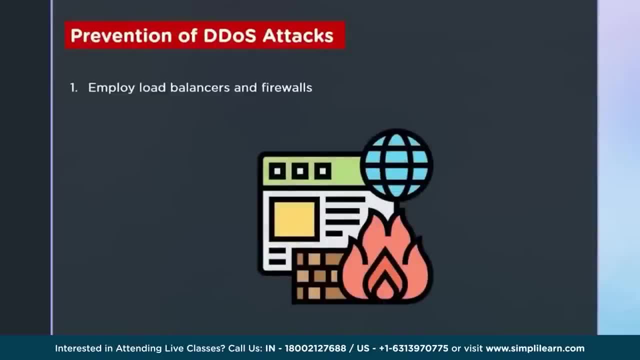 attacks. Load balancers reroute the traffic from one server to another in a DDoS attack. This reduces the single pointer failure and adds resiliency to the server data. A firewall blocks unwanted traffic into a system and manages the number of requests. 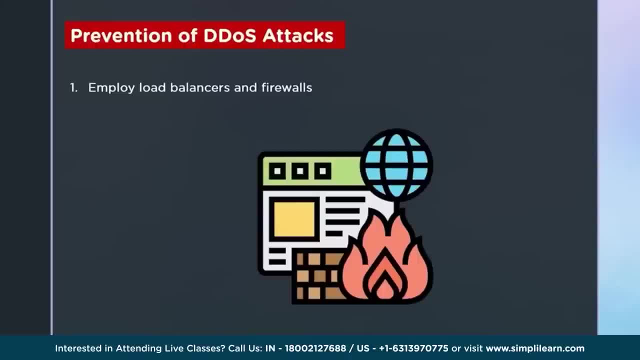 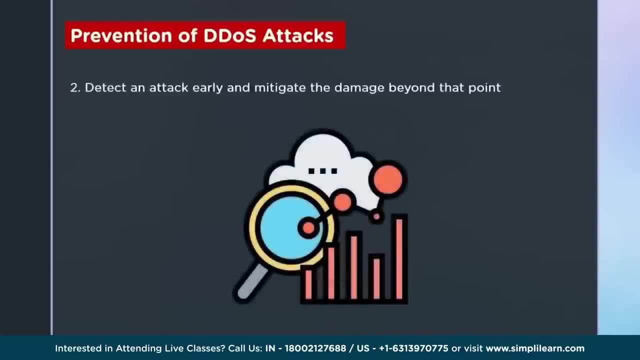 made at a definite rate. It checks for multiple attacks from a single IP and occasional slowdowns to detect a DDoS attack in action. Early detection of a DDoS attack goes a long way in recovering the data lost in such an event. 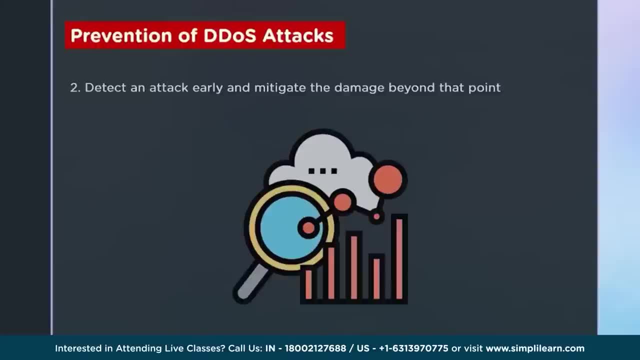 Once you've detected the attack, you will have to find a way to respond. For example, you will have to work on dropping the malicious DDoS traffic before it reaches your server, so that it doesn't throttle and exhaust your bandwidth. Here's where you will filter the. data from the DDoS server to the DDoS server. Here's where you will filter the data from the DDoS server to the DDoS server. Here's where you will filter the data from the DDoS server to the. 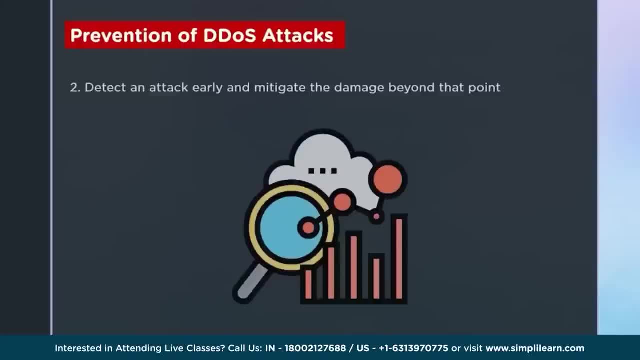 DDoS server to the DDoS server so that only legitimate traffic reaches the server. By intelligent routing you can break the remaining traffic into manageable chunks that can be handled by your cluster resources. The most important stage in DDoS mitigation is 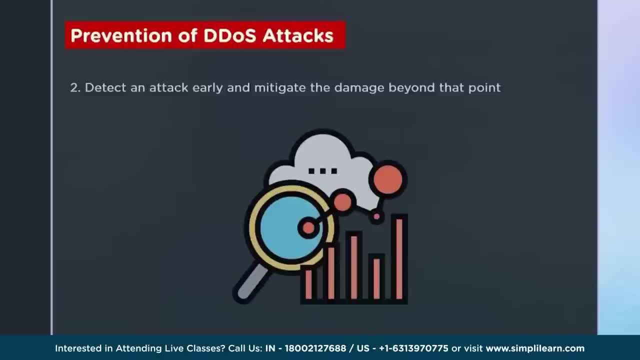 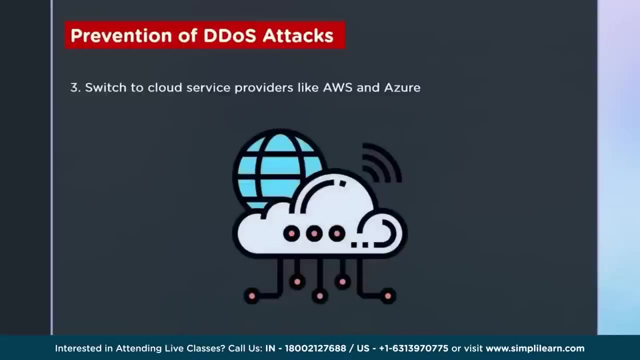 where you will look for patterns of DDoS attacks and use those to analyze and strengthen your mitigation techniques. For example, blocking an IP that's repeatedly found to be offending is a first step. Cloud providers like Amazon Web Services and Microsoft Azure, who offer high levels of cybersecurity, including firewalls and threat monitoring. 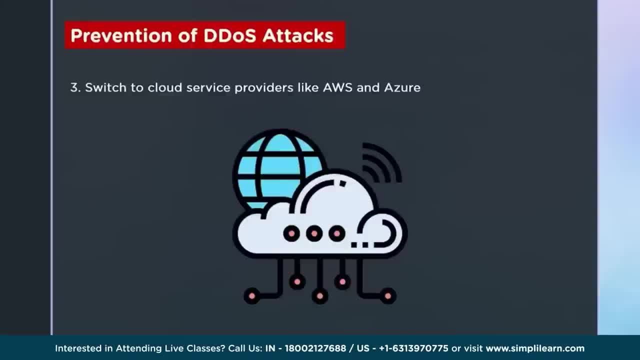 software can help protect your assets and network from DDoS criminals. The cloud also has greater bandwidth than most private networks, so it is likely to fail if under the pressure of increased DDoS attacks. Additionally, reputable cloud providers offer network redundancy duplicating. 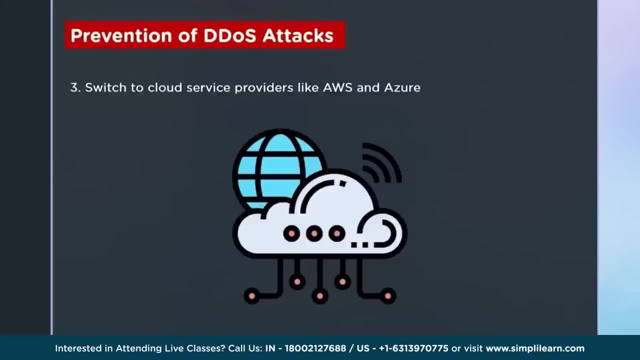 copies of your data systems and equipment so that, if your service becomes corrupted or unavailable due to a DDoS attack, you will not be able to access your data and systems. You can switch to a secure access on backed-up versions without missing a beat. 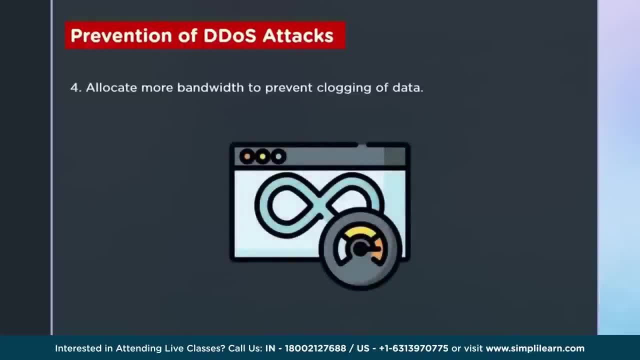 One can also increase the amount of bandwidth available to a host server being targeted. Since DDoS attacks fundamentally operate on the principle of overwhelming systems with heavy traffic, simply provisioning extra bandwidth to handle unexpected traffic spikes can provide a measure of protection. This solution can prove expensive. 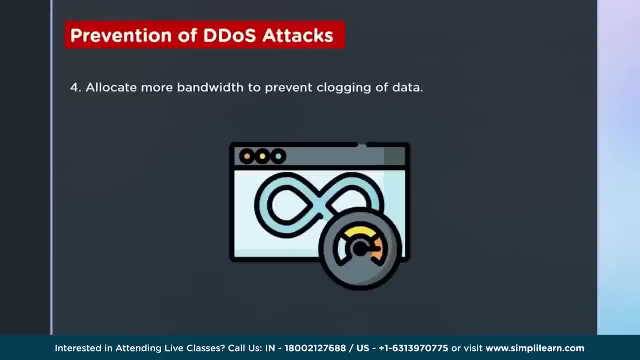 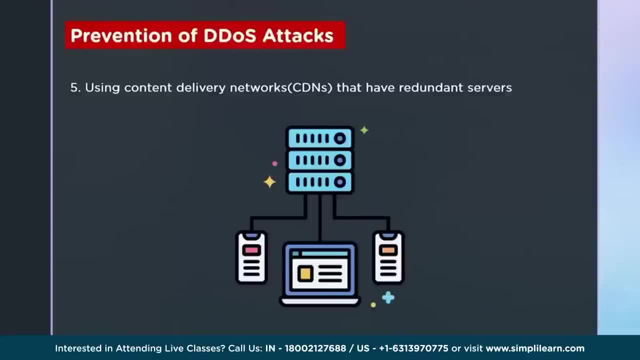 as a lot of that bandwidth is going to go unused most of the time. The next thing I want to share on the top is that a content delivery network distributes your content and boosts performance by minimizing the distance between your resources and end users. It stores the 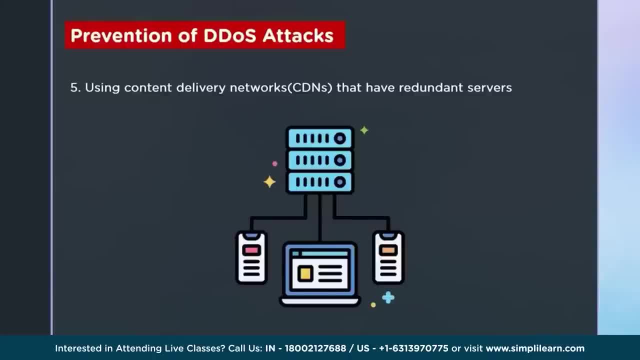 cached version of your content in multiple locations, and this eventually mitigates DDoS attacks by avoiding a single point of failure when the attacker is trying to focus on a single target. Popular CDNs include Akamai CDN, Cloudflare, AWS, CloudFront, etc. Let's start with a few examples of the most popular CDNs in the market. The most popular CDNs include Akamai, CDN, Cloudflare, AWS, CloudFront, etc. The most popular CDNs include Akamai, CDN, Cloudflare, AWS, CloudFront, etc. 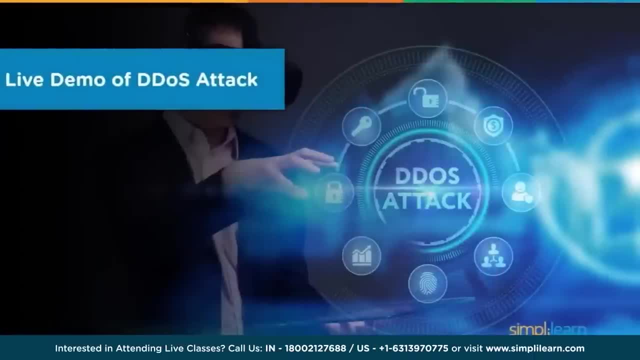 The most popular CDNs include Akamai, CDN, Cloudflare, AWS, CloudFront, etc. Let's start with our demo regarding the effects of DDoS attacks on a system. For our demo, we have a single device that will attack a target, making it a DDoS attack. 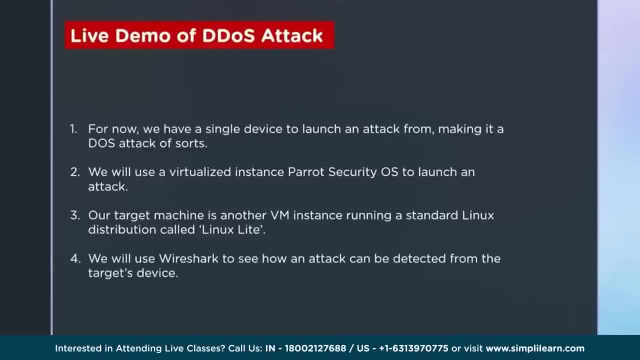 of sorts. Once a botnet is ready, multiple devices can do the same and eventually emulate a DDoS attack. To do so we will use the virtualization software called VMware. with an instance of Parag Security operating system running For a target machine, we will be running another VMware instance of a standard Linux. 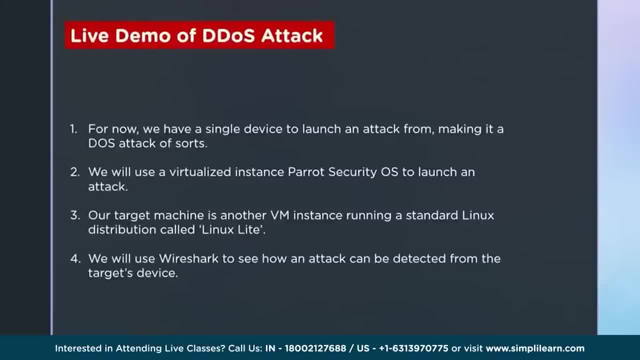 distribution known as Linux Lite. In a target device, we can use Wireshark to determine when the attack begins and see the effects of the attack accordingly. This is Linux Lite which is our target machine, and this is Parag Security which is used. 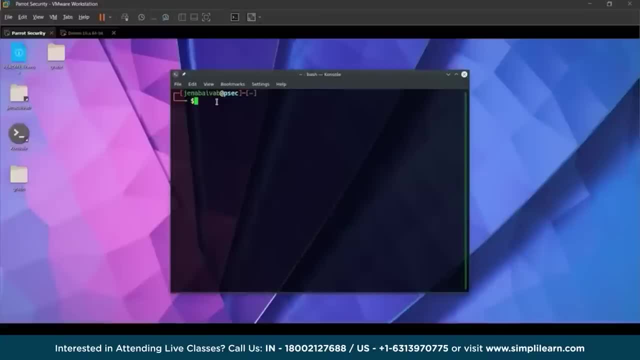 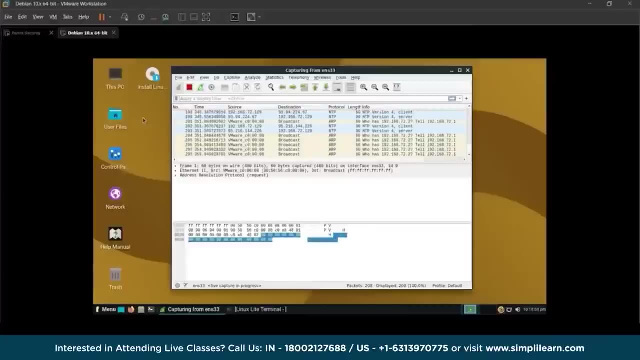 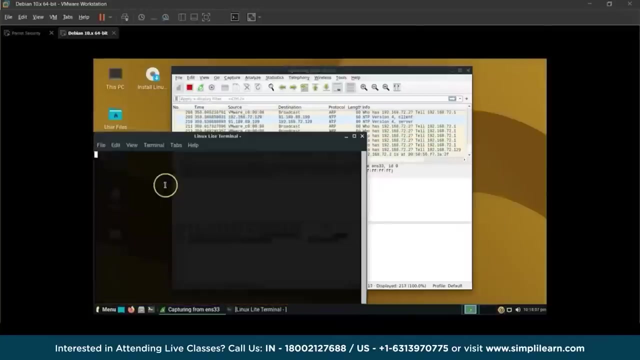 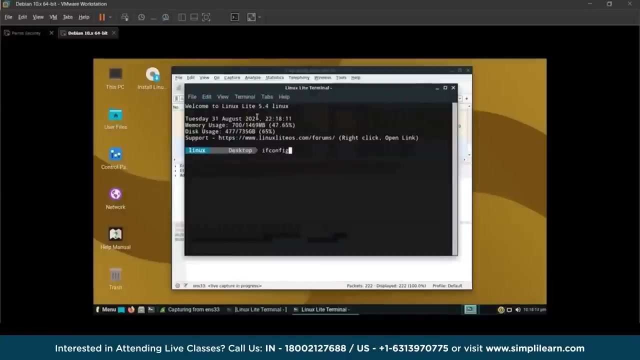 by the hacker when trying to launch a DDoS attack. This is just one of the distros that can be used To launch the attack. we must first find the IP address of our target. And to find the IP address we open the terminal, we use the command ifconfig, and here we can. 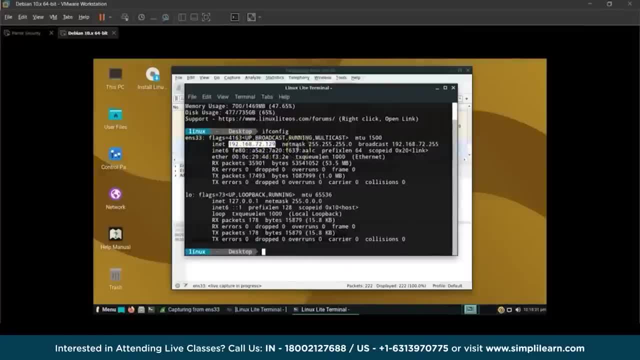 find the IP address Now. remember we're launching this attack in VMware. Now, both the instances of Parag Security and Linux Lite are being run on my local network, So the address that you can see here is 192.168.72.129,, which is a private address. 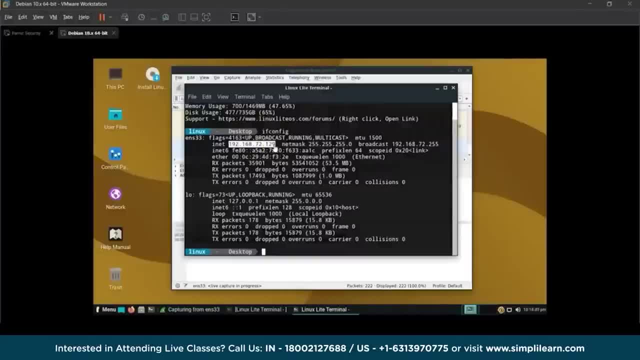 This IP cannot be accessed from outside the network- basically anyone who is not connected to my Wi-Fi. When launching attacks with public servers or public addresses, it will have a public IP address that does not belong to the 192.168 subnet. Once we have the IP address, we can use a tool called Parag Security. 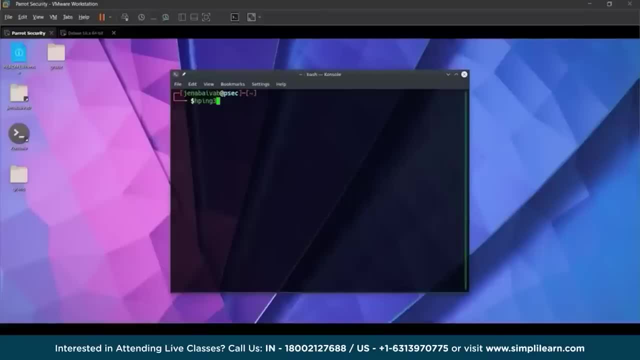 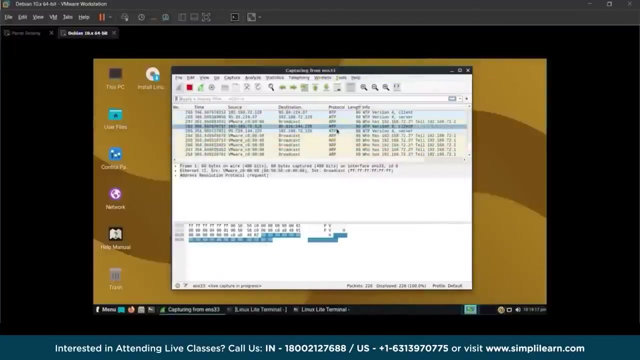 Hping3.. Hping3 is an open source packet generator and analyzer for the TCP IP protocol. To check what are the effects of an attack, we will be using Wireshark. Wireshark is a network traffic analyzer. We can see whatever traffic that is passing through. the Linux Lite distro is being displayed. 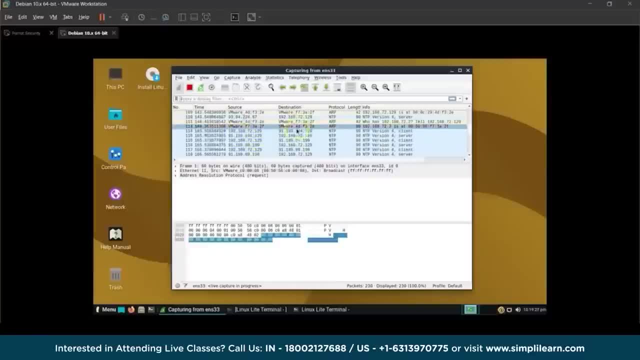 over here with the IP address, the source IP and the destination IP, So where the request is being transferred to. Once we have the DOS attack launched, you can see the results coming over here from the source IP, which will be Parag Security. 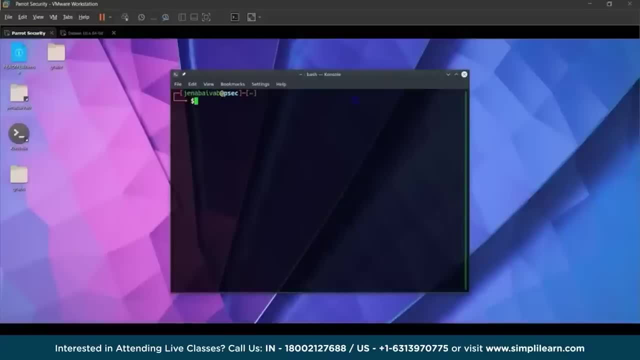 Now, to launch the Hping3 command, we need to give sudo access to the console, which is the root access. Now we have the root access for the console, The Hping3 command will have a few arguments to go with it, Which are, as you can see on the screen, minus s and a flood, a hyphen v, hyphen p80, and. 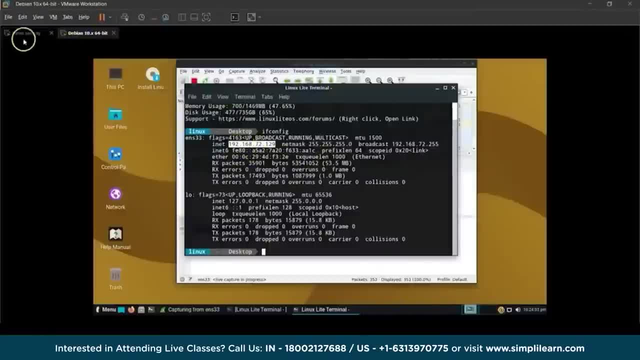 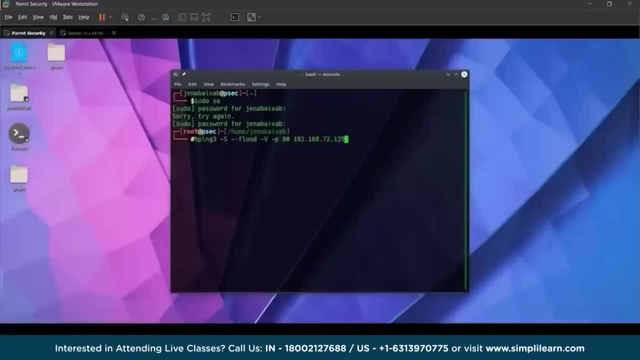 the IP address of the target, which is 192.168.72.129.. In this command we have a few arguments, such as the minus s, Which specifies: sya. Like in an SSL handshake, we have the syn request that the client sends to the server. 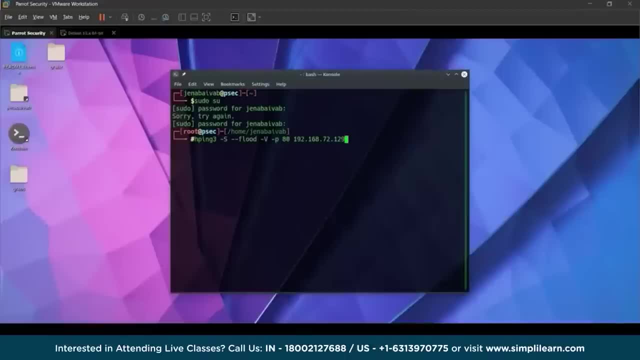 to initiate a connection. The hyphen flood aims to ignore the replies that the server will send back to the client in response to the syn packets. Here the Parag Security OS is the client and Linux Lite being the server. Minus v stands for verbosity, as in where we will see some output when the requests. 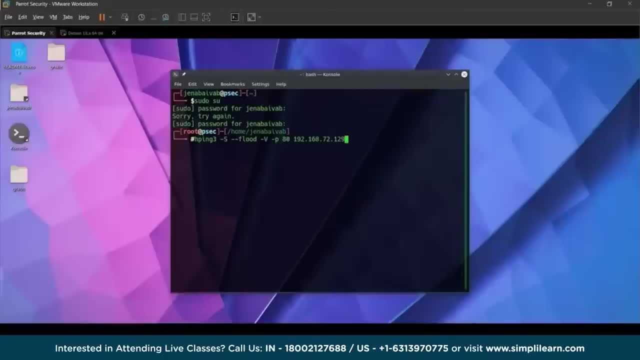 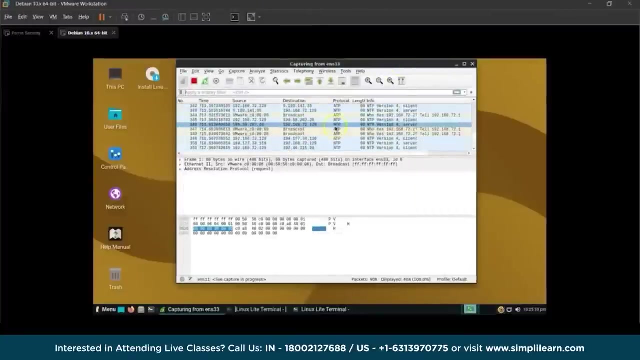 are being sent. The hyphen p80 stands for port 80, which we can replace the port number if we want to attack a different port. And finally, we have the IP address of our target As of right now. if we check wireshark, it is relatively clear and there is no indication. 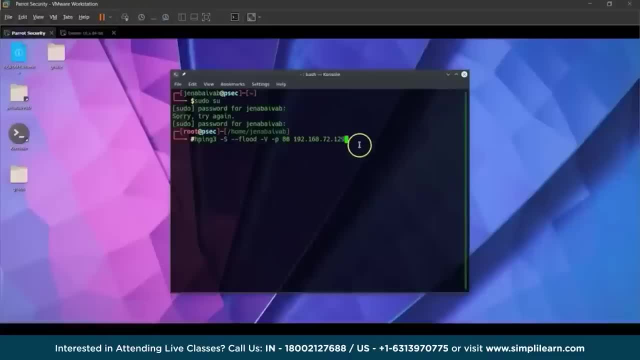 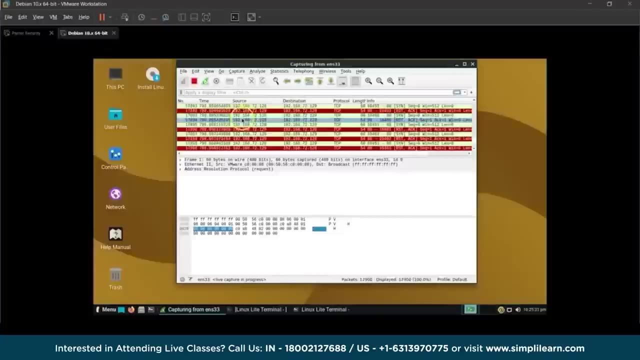 of a DDoS attack incoming Now. once we launch the attack over here, we can see the requests coming in from this IP, which is 192.168.72.128.. Till now, even if the network is responsive, and so is Linux Lite. 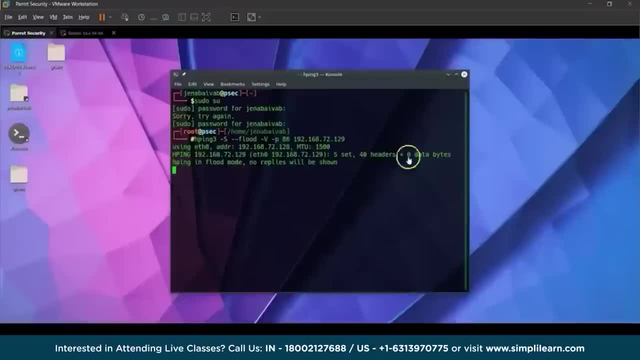 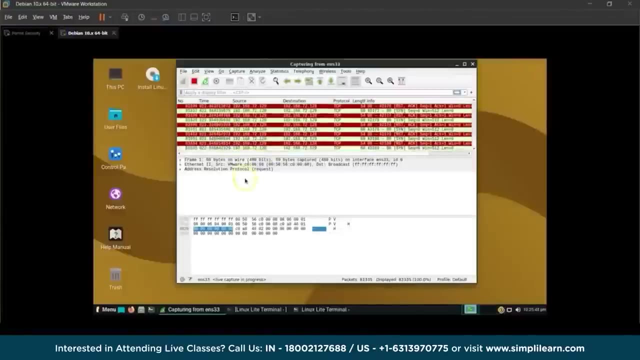 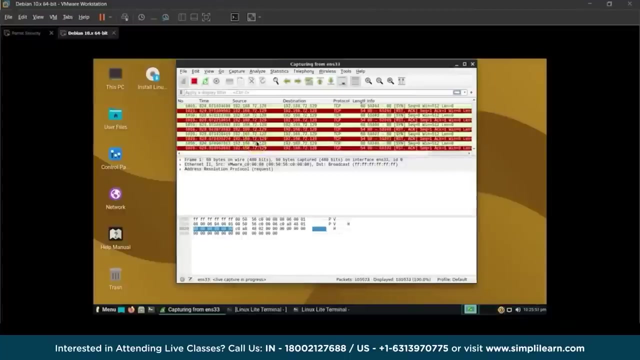 The requests keep on coming and we can see the HTTP flooding has started in flood mode. After a few seconds of this attack continuing, the server will start shutting down. Now remember: Linux Lite is a server. It's not a server. Linux Lite is a distro that can focus on. that serves as a backend. 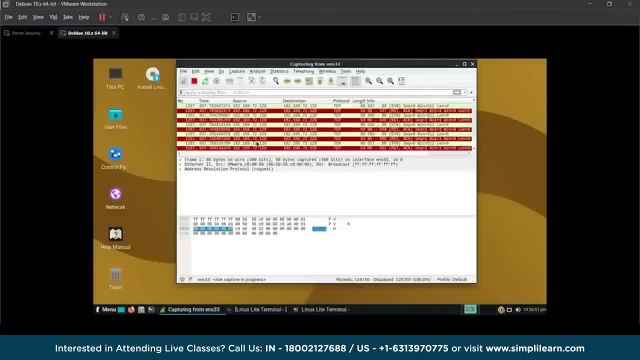 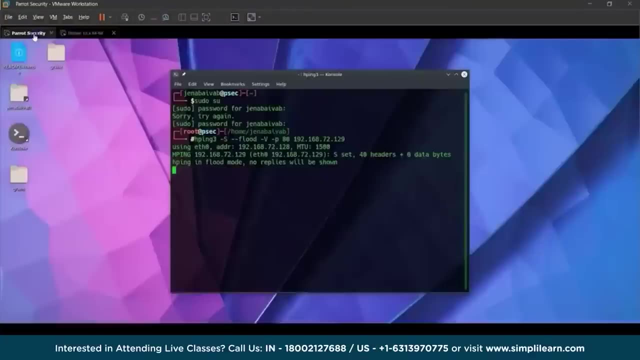 Remember, Linux Lite is a distro and such Linux distros are served as backend to many servers across the world. For example, a few seconds have passed from the attack. Now the system has become completely responsive. This has happened due to the huge number of requests that came from Parallel Security. 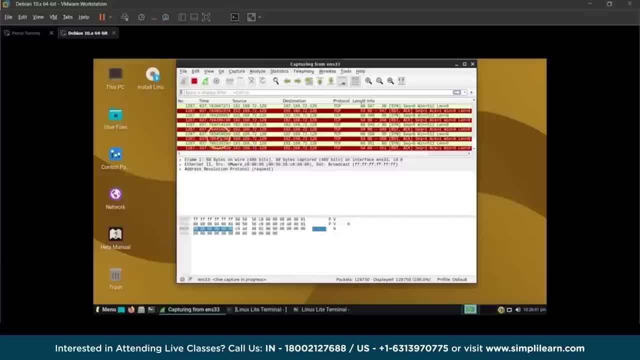 You can see, whatever I press, nothing is responded. Even the wireshark has stopped. The network has stopped capturing new requests because the CPU usage right now is completely 100% and at this point of time anyone who is trying to request some information from 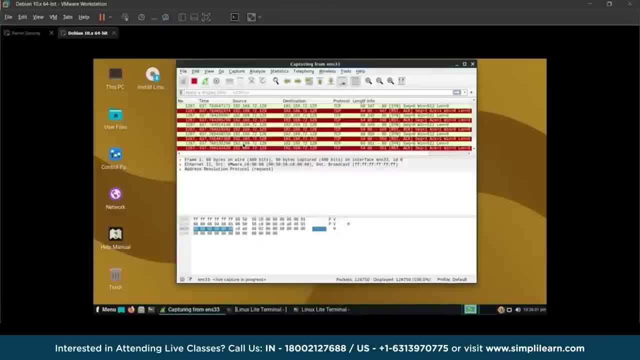 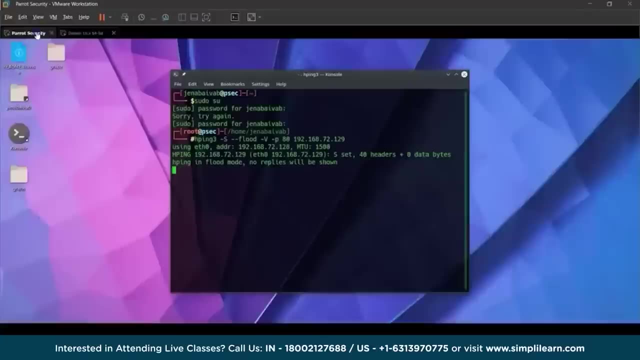 this Linux distro, or where this Linux distro is being used as a backend for a server or a database, cannot access anything else. The system has completely stopped responding and any requests, any legitimate requests from legitimate users, will be dropped Once we stop the attack over here. 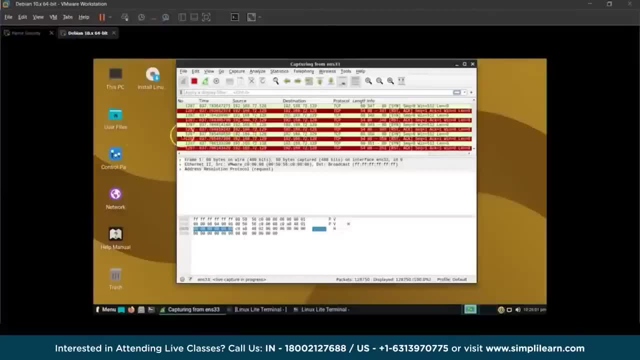 It takes a bit of time to settle down. Now, remember it's still out of control, but eventually the traffic dies down and the system regains its strength. It is relatively easy to gauge right now the effect of a DOS attack. 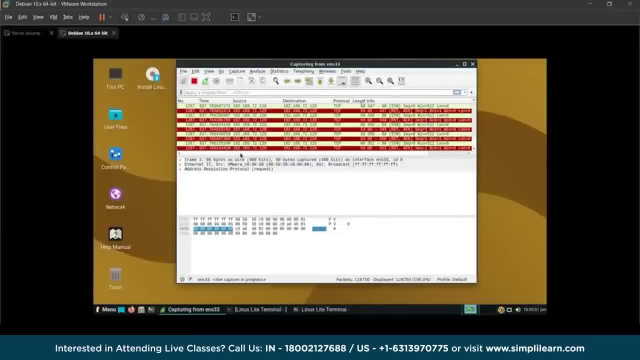 Now remember this: Linux Lite is just a VM instance- Actual website servers and web databases. they have much more bandwidth and are very secure and it is tough to break into. That is why we cannot use a single machine to break into. 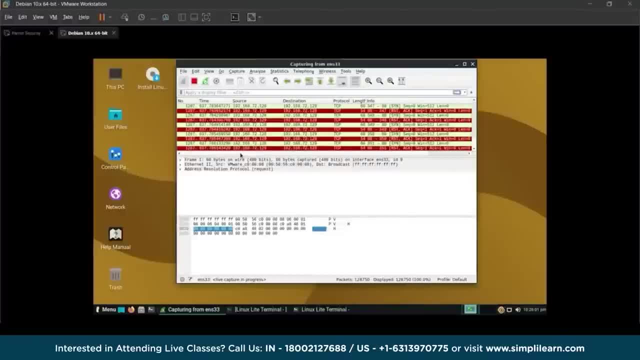 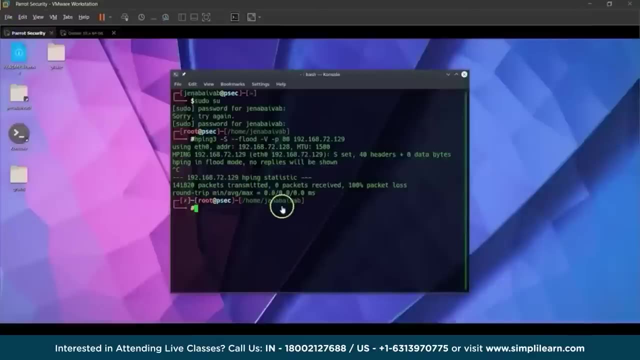 That is where a DDoS attack comes into play. What we did right now is a DOS attack, As in a single system is being used to penetrate a target server using a single request. Now, in a DDoS attack, multiple systems, such as multiple pilot security instances or multiple 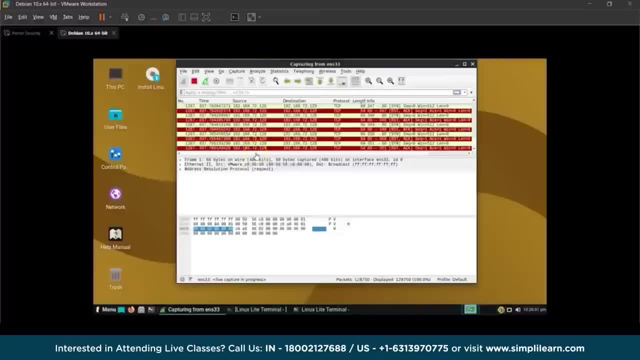 zombies or bots in a botnet network can attack a target server to completely shut down the machine and drop any legitimate requests, thereby rendering the service and the target completely unusable and inoperable. As a final note, we would like to remind that this is for educational purposes only and 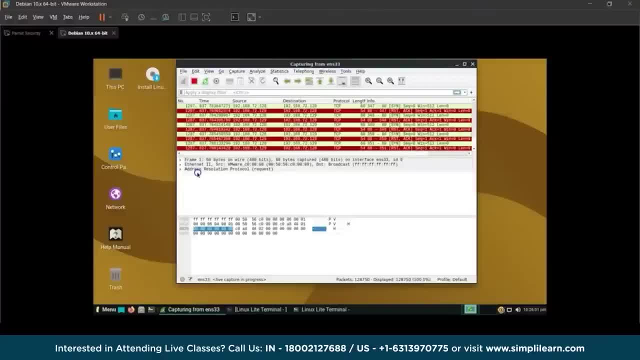 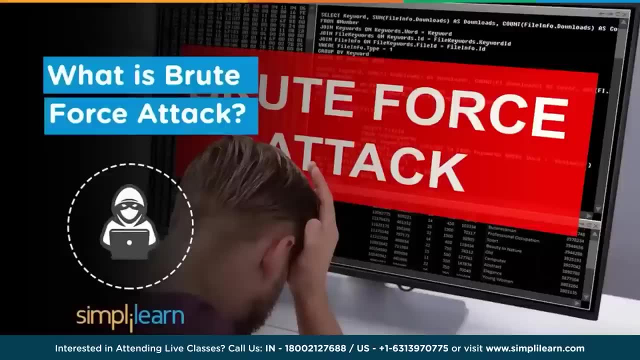 we do not endorse any attacks on any proven domains. Only test this on servers and networks that you have permission to test on. Cybersecurity has become one of the most rigid industries in the last decade, while simultaneously being the most challenged With every aspect of corporate culture going online and embracing cloud computing there. 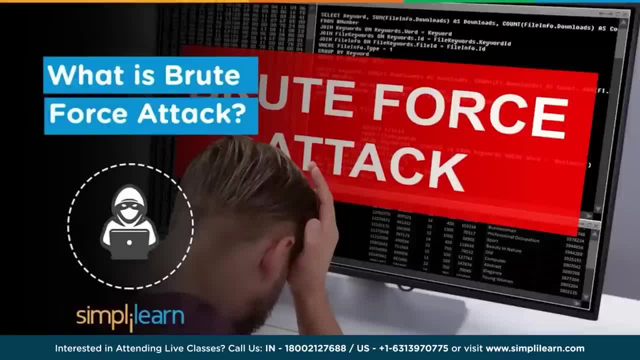 is a plethora of critical data circulating through the internet, all worth billions of dollars to the right person. Increasing benefits require more complex attacks, and one of these attacks is a brute force attack. A brute force, or known as brute force cracking, is the cyber attack equivalent of trying every 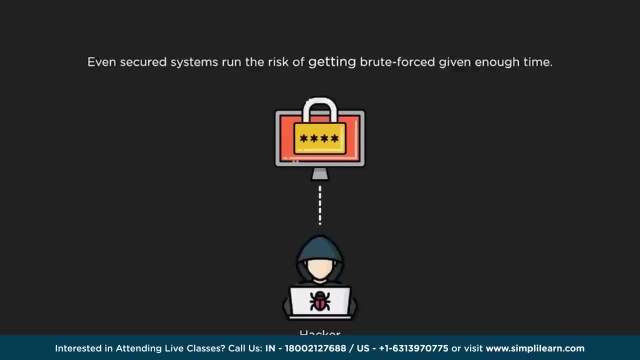 key on your keyring and eventually finding the right one. Brute force attacks are simple and reliable. There is no prior knowledge needed about the victim to start an attack. Most of the systems falling prey to brute force attacks are actually based on the fact. 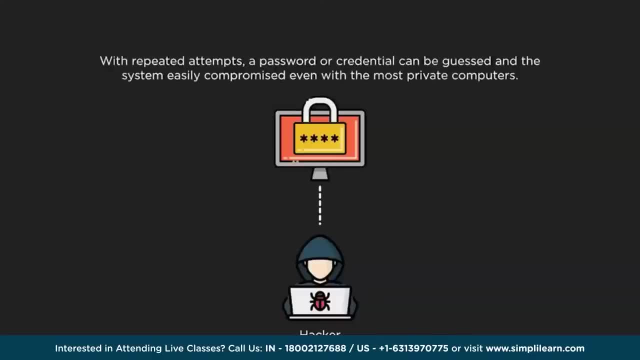 that the system is not designed to attack the victim. Although many of the cyber attacks are well-secured attackers, let a computer do the work, ie trying different combinations of usernames and passwords until they find one that works. Due to this repeated trial and error format, the strength of passwords matters a great. 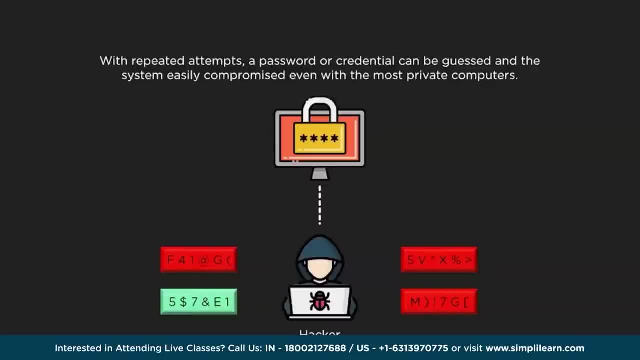 deal, Although, with enough time and resources, brute force will break a system, since they run multiple combinations until they find the right passcode. Hey everyone, this is Bhavab from Simply Learn, and welcome to this video on what is a brute force attack. 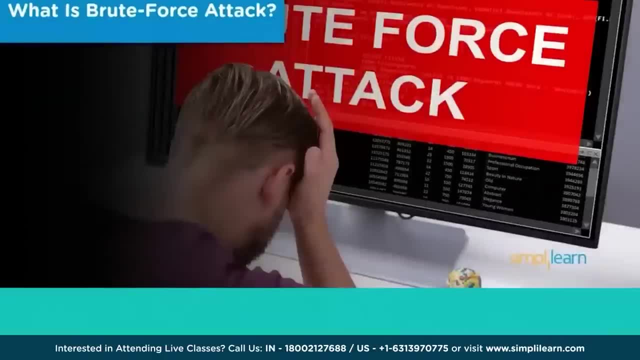 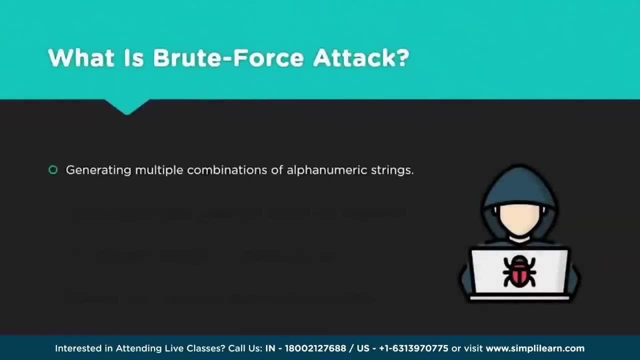 Let's begin with learning about brute force attacks in detail. A brute force attack, also known as an exhaustive search, is a cryptographic hack that relies on guessing passable combinations of targeted passwords until the current password is discovered, It can be used to break into online accounts, encrypted documents or even network peripheral. 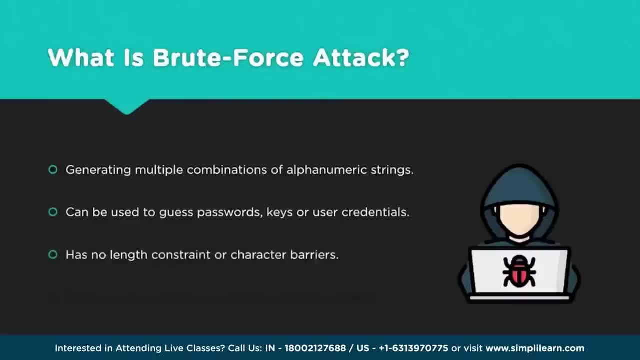 devices. The longer the password, the more combinations that will need to be tested. A brute force attack can be time consuming and difficult to perform if methods such as data obfuscation are used, and, at times, downright impossible. However, if the password is weak, it could merely take seconds with hardly any effort. 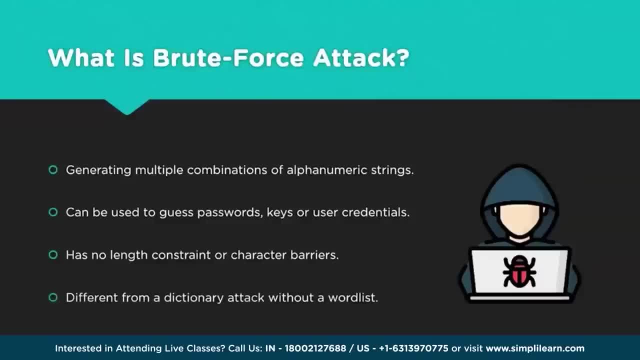 Dictionary attacks are an alternative to brute force attacks, where the attacker already has a list of usernames and passwords that need to be tested against the target. It doesn't need to create any other combinations on its own. Dictionary attacks are much more reliable than brute force attacks. 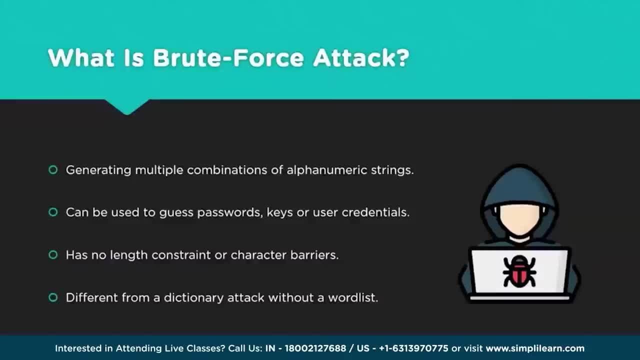 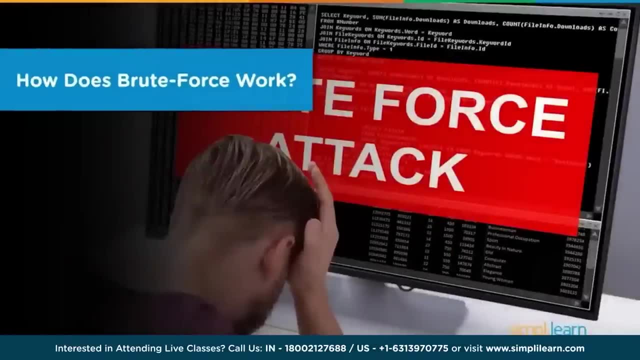 They can be used in a real-world context, but the usefulness depends entirely on the strength of passwords being used by the general population. There is a three-step process when it comes to brute forcing a system. Let's learn about each of them in detail. 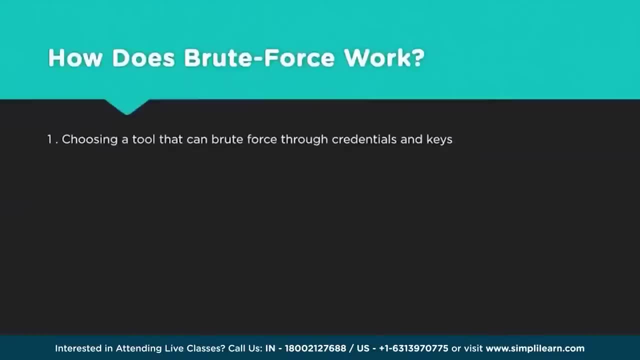 In step one, we have to settle on a tool that we are going to use for brute forcing. There are some popular names on the market, like Hashcat, Hydra and John the Ripper. While each of them has its own name, they are called brute force attacks. 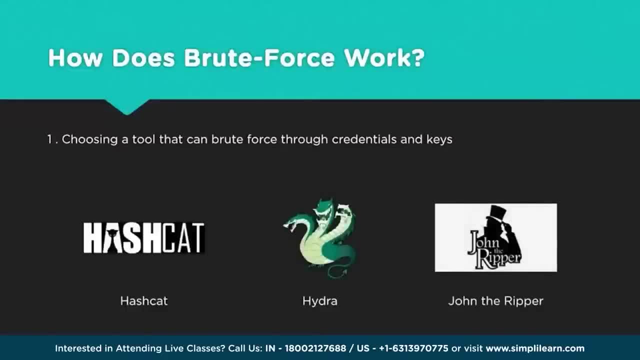 Each of them has its own strengths and weaknesses. Each of them perform well with the right configuration. All of these tools come pre-installed with certain Linux distributions that cater to penetration testers and cybersecurity analysts, like Kali Linux and Parrot Security. After deciding what tool to use, we can start generating combinations of alphanumeric variables. 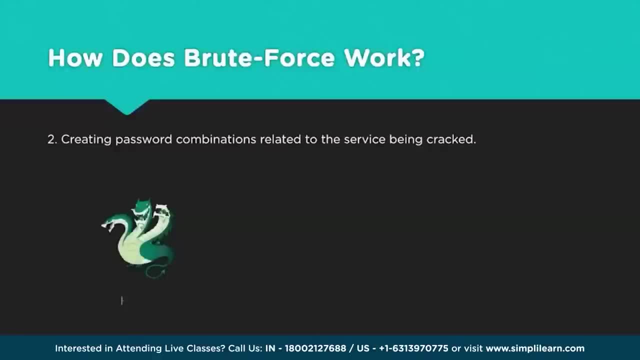 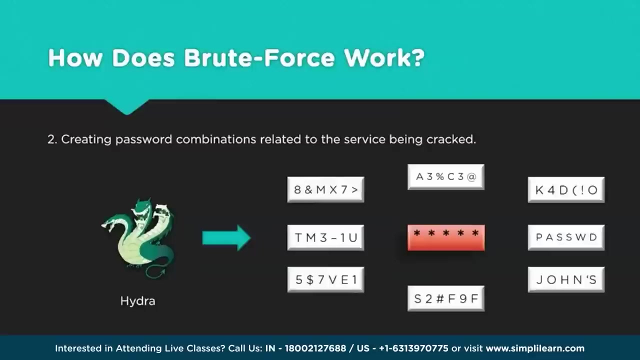 whose only limitation is the number of characters. For example, while using Hydra, a single six-digit password will create nine different alphanumeric variables. We can create nine hundred thousand passwords with only digits involved. Add alphabets and symbols to that sample space and that number grows exponentially. 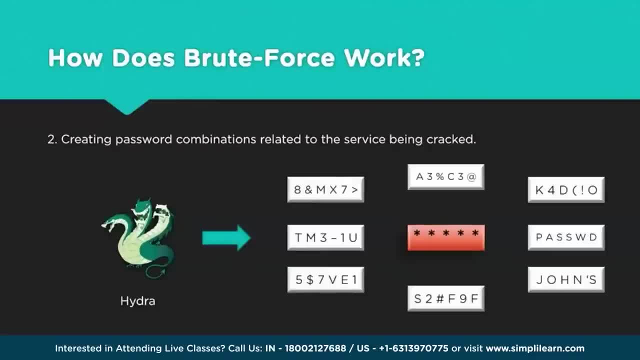 The popular tools allow customizing this process. Let's say the hacker is aware of the password being a specific eight-digit word containing only letters and symbols. This will substantially increase the chances of being able to guess the right password, since we remove the time taken to generate the longer ones. 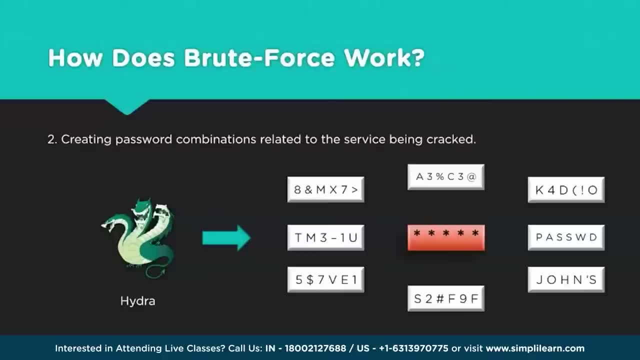 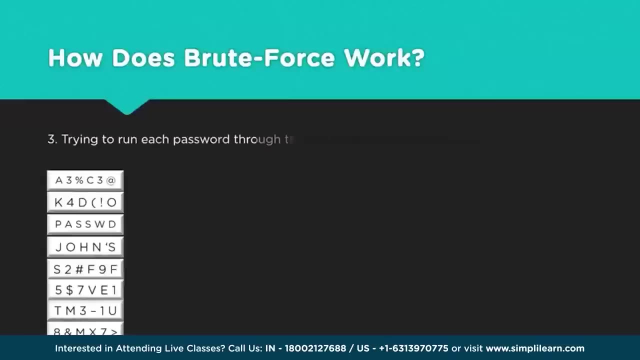 We omit the need for including digits in such combinations. These small tweaks go a long way in organizing an efficient brute force attack, since running all the combinations with no filters will dramatically reduce the odds of finding the right credentials in time. In the final step, we run these combinations against the file or service that is being 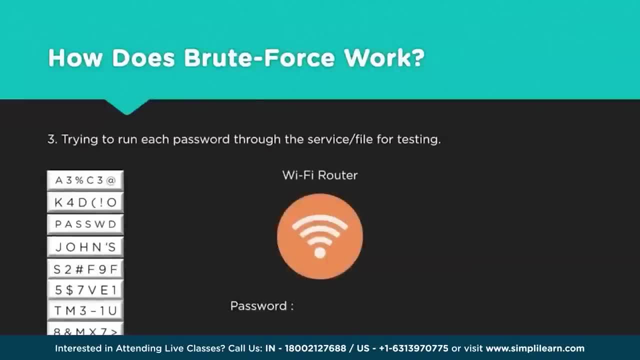 broken. We can try and break into a specific encrypted document, a social media account or even devices at home that connect to the internet. The generated passwords are then fed into the connection, one after the other. It is a long and arduous process, but the work is left to the computer other than someone. 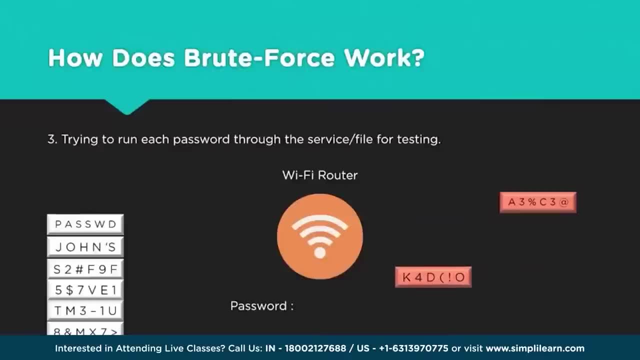 manually clicking and checking each of these passcodes. Any password that doesn't unlock the router is discarded and the brute force tool simply moves on to the next one. This keeps going on until we find the right combination which unlocks the router. Sometimes, reaching the success stage takes days and weeks, which makes it complicated. 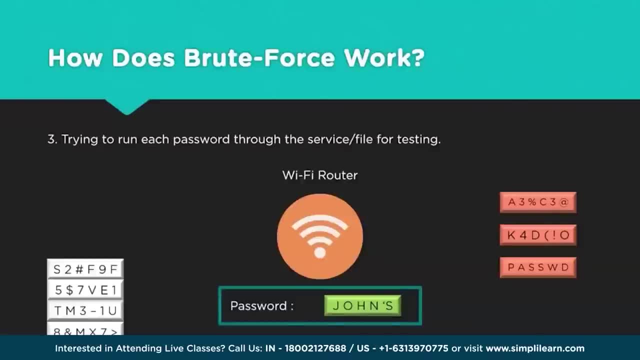 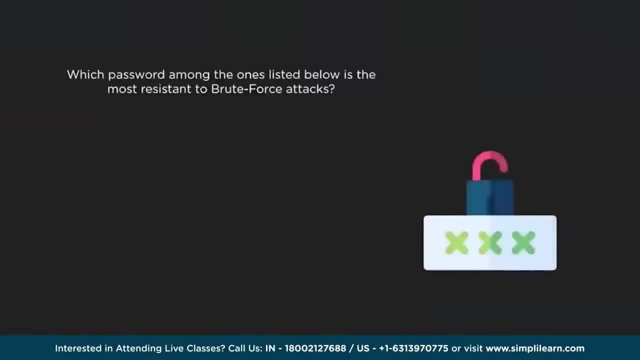 and cumbersome for people with low computing power at their disposal. However, the ability to crack any system in the world purely due to bad password habits is very appealing, and the general public tends to stick with simple and easy to use passwords. Now that we have a fair idea about how brute force works, let's see if we can answer. 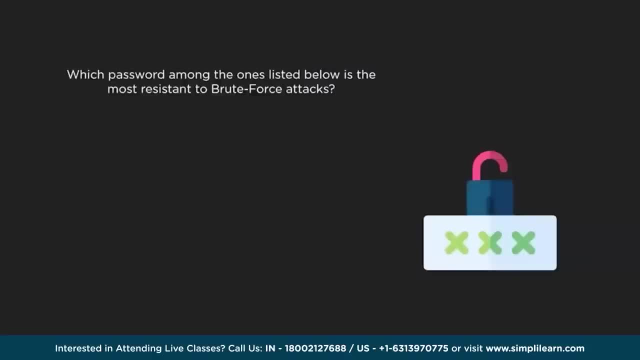 this question, We learnt about how complex passwords are tougher to crack by brute force. Among the ones listed on the screens, which one do you believe will take the longest to be broken when using brute force tools? Leave your answers in the comment section and we will get back to you with the correct. 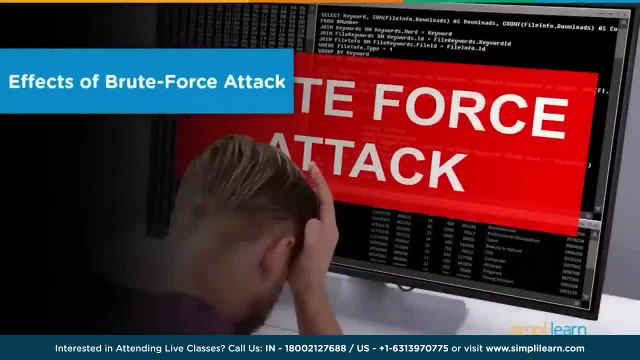 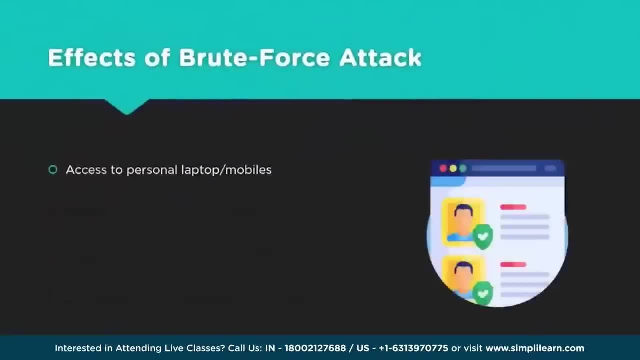 option next week. Let's move on to the harmful effects of getting a system compromised due to brute force attacks. A hacked laptop or mobile can have social media accounts logged in, giving the hackers free access to the victim's connections. It has been reported on multiple occasions where compromised Facebook accounts are sent. 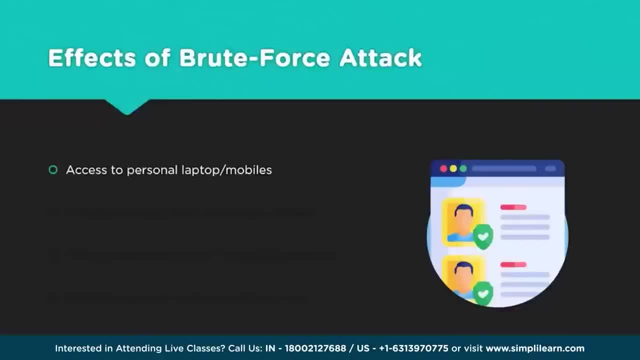 with malicious links and attachments to people on their friends list. One of the significant reasons for hacking: malware infusion is best done when spread from multiple devices similar to distributing spam. This reduces the chance of circling back the source to a single device which belongs to. 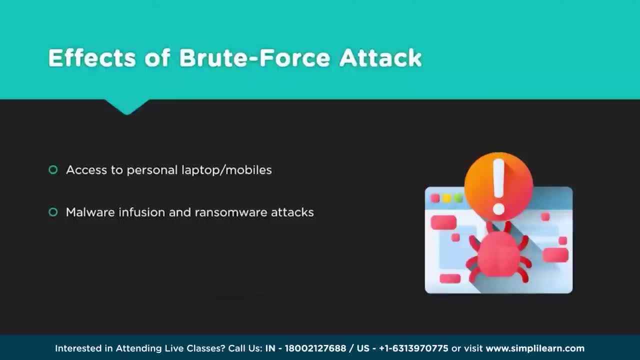 the hacker, Once brute forced a system, can spread malware via email attachments, sharing links, file upload via FTP, etc. Personal information such as credit cards, e-mails etc. can be shared with the hacker. This can also be done by using malicious links and attachments to people on their friends list. 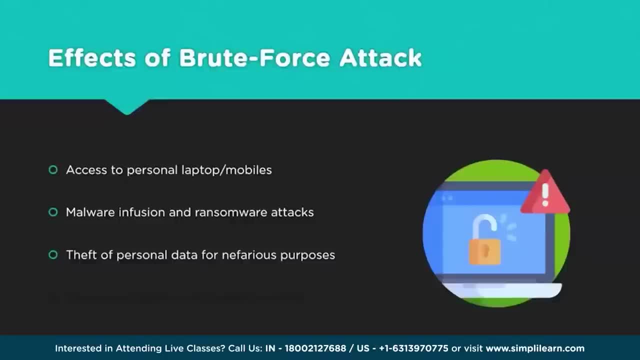 Data usage habits, private images and videos are stored in our systems, be it in plain format or root folders. A compromised laptop means easy access to this information that can be further used to impersonate the victim regarding bank verification, among other things. 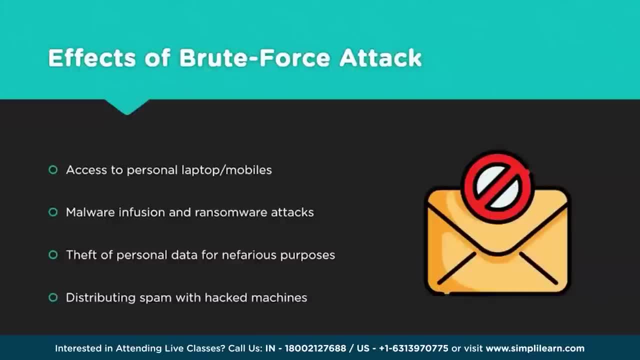 Once a system is hacked, it can also be used as a mail server that distributes spam across lists of victims. Since the hacked machines all have different IP addresses and MAC addresses, it becomes challenging for the hacker to access these lists to trace the spam back to the original hacker. 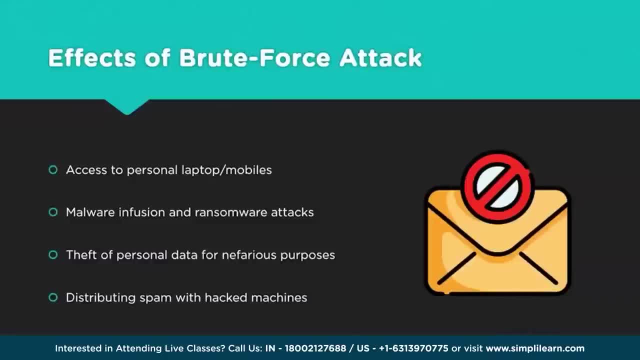 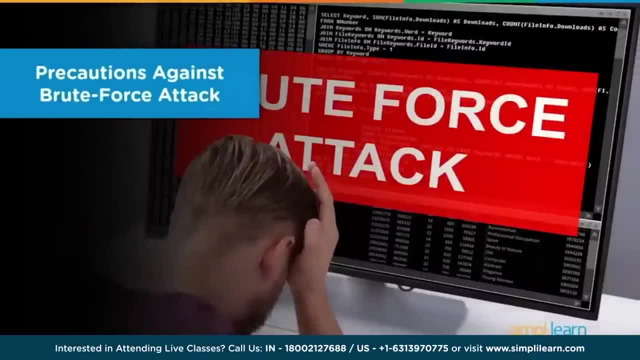 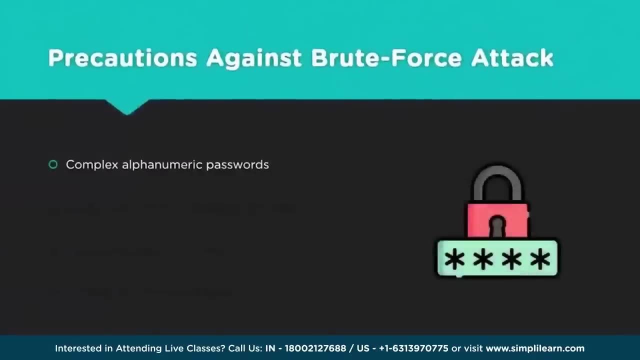 With so many harmful implications arising from a brute force attack, it's imperative that the general public must be protected against such. Let's learn about some of the ways we can prevent ourselves from becoming a victim of brute force attacks. Using passwords consisting of alphabets, letters and numbers. 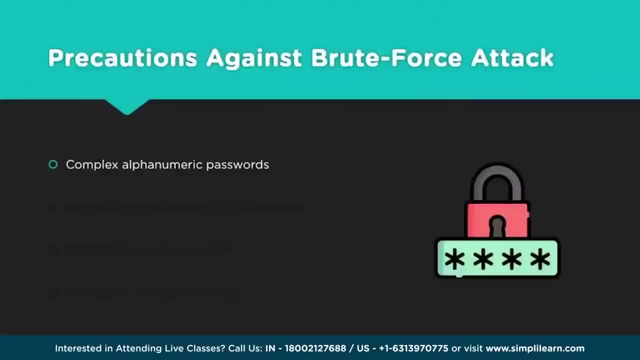 have a much higher chance of extending brute force attacks thanks to the sheer number of combinations they can produce. The longer the password, the less likely it is that a hacker will devote the time and resources to brute force them. Having alphanumeric passwords also allows the user. 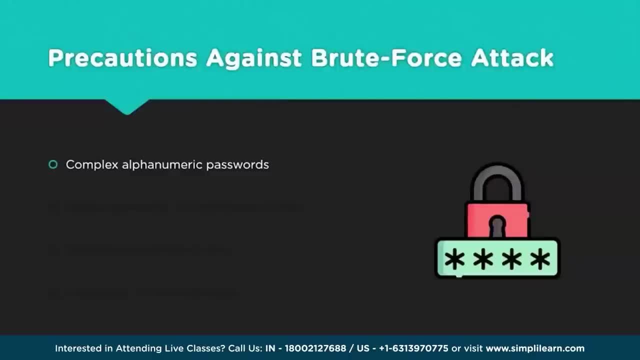 to keep different passwords for different websites. This is to ensure that if a single account or a password is compromised due to a breach or a hack, the rest of the accounts are isolated from the incident. Two-factor authentication involves receiving a one-time password on a trusted device before a new login is allowed. 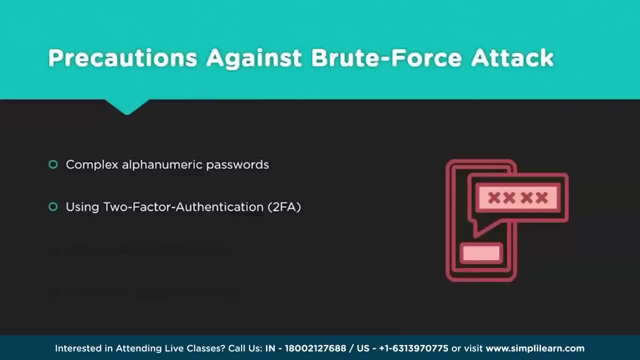 This OTP can be obtained either via email, SMS or specific 2FA applications like Authy and Aegis. Email and SMS-based OTPs are considered relatively less secure nowadays due to the ease with which SIM cards can be duplicated and mailboxes can be hacked. 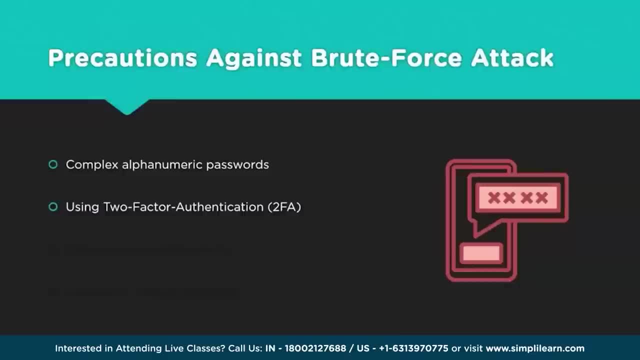 Applications that are specifically made for 2FA codes are much more reliable and secure. CAPTCHAs are used to stop bots from running through webpages precisely to prevent brute forcing through the internet, Since brute force tools are automated, forcing the hacker to solve CAPTCHA for every iteration. 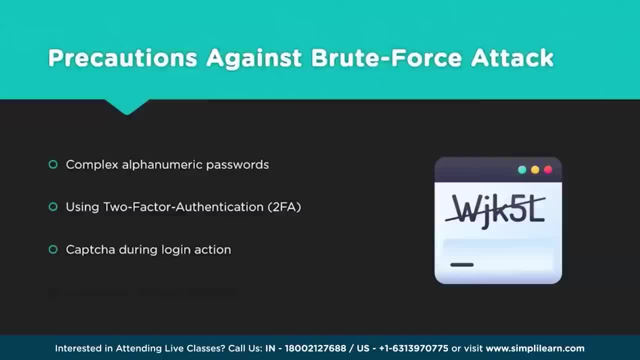 of a password manually is very challenging. The CAPTCHA system can filter out these automated bots that keep refreshing the page with different credentials, thereby reducing the chances of brute force considerably. A definite rule that locks the account being hacked for 30 minutes after a specified number of attempts. 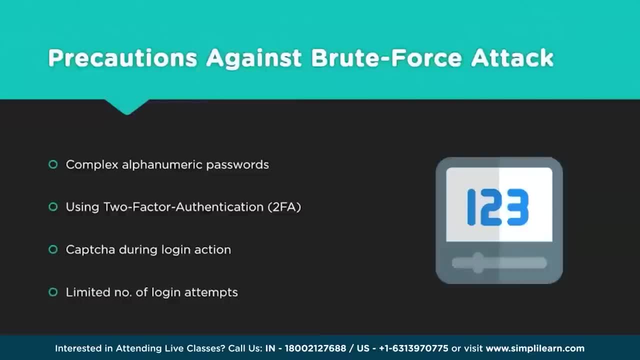 is a good way to prevent brute force attempts. Many websites lock account for 30 minutes after 3 failed password attempts to secure the account against any such attack. On an additional note, some websites also send an email instructing the user that there have been 3 insecure attempts to log in to the website. 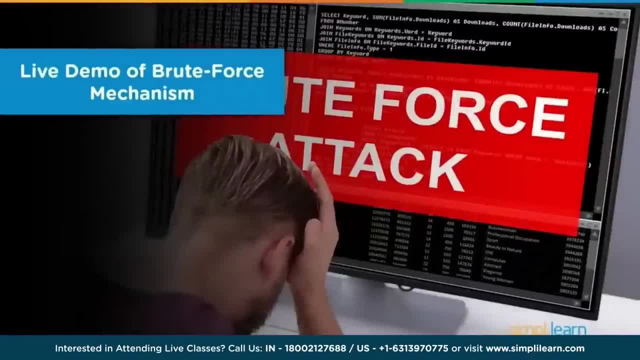 Let's look at a demonstration of how brute force attacks work in a real-world situation. The world has gone wireless, With Wi-Fi taking the reins in every household. it's natural that their security will always be up for debate. To further test their security index. 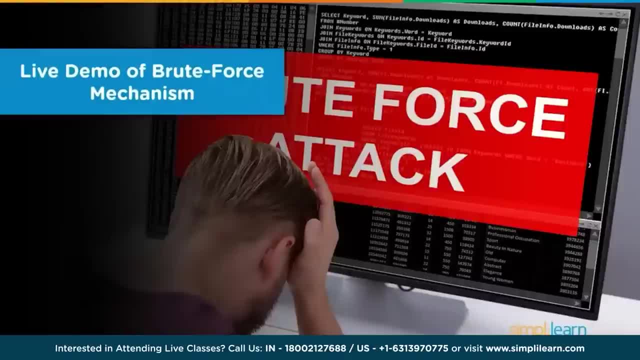 and understand brute force attacks, we will attempt to break into the password of a Wi-Fi router. For that to happen, we first need to capture a handshake file, which is a connection file from the Wi-Fi router to a connecting device like a mobile or a laptop. 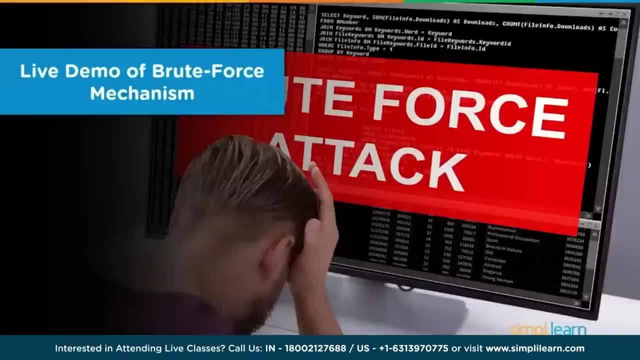 The operating system used for this process is Parrot Security, a Linux distribution that is catered to penetration testers. All the tools being used in this demo can easily be found pre-installed in this operating system. If getting your learning started is half the battle, 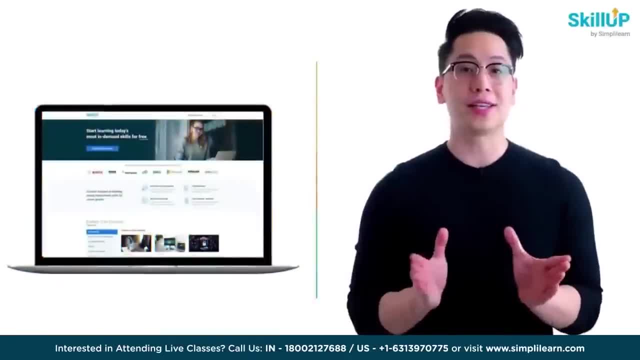 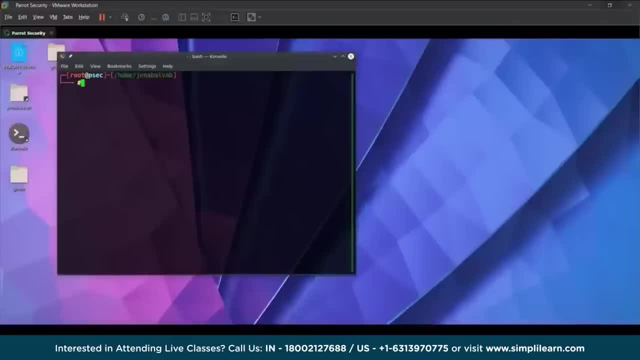 what if you could do that for free? Visit SkillUp by SimplyLearn. Click on the link in the description to know more. To start our demo, we're going to use a tool called Airgeddon, which is made to hack into wireless networks specifically. 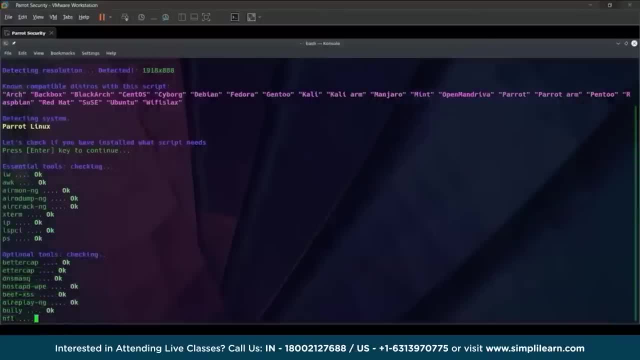 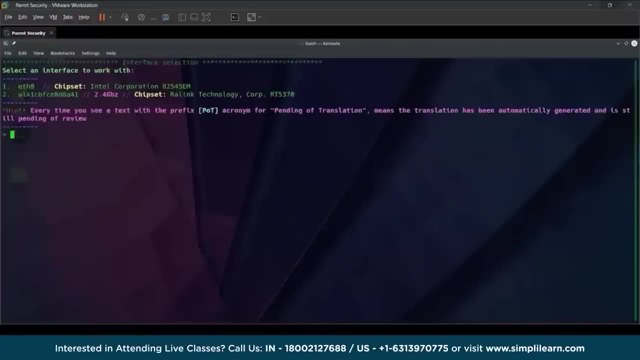 At this point it's going to check for all the necessary scripts that are installed in the system. To crack into a Wi-Fi and to capture the handshake file, we're going to need an external network card. The significance of the external network card. 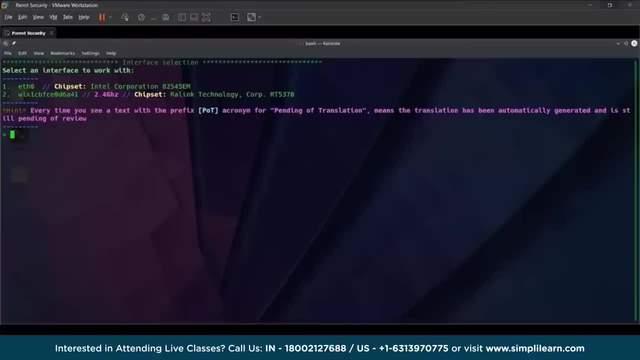 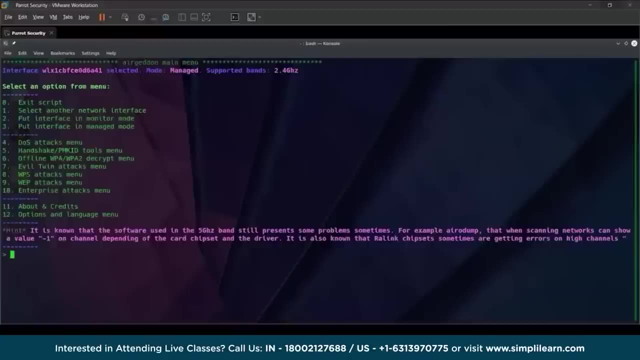 is a managed mode and a monitor mode. For now. the WLX1 named card is my external network adapter, which I'm going to select To be able to capture data over the air. we're going to need to put it in monitor mode. 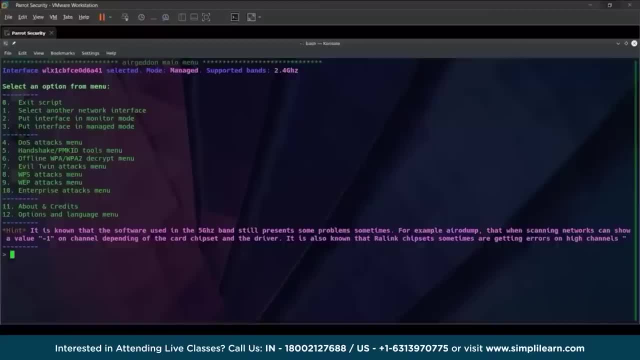 As you can see above, it's written: it is in managed mode right now, So we're going to select option 2, which is to put the interface in monitor mode, And its name is now WLAN0 monitor. The monitor mode is necessary to capture data over the air. 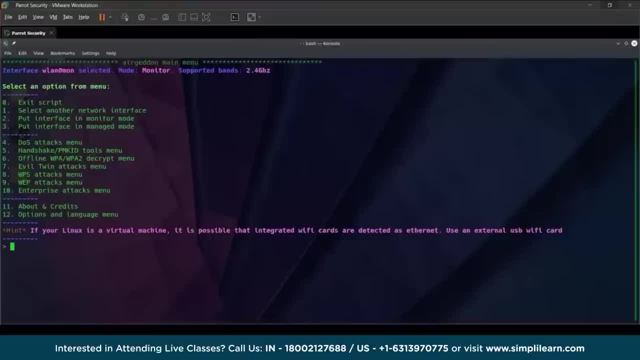 That is the necessary reason why we need an external card, since a lot of inbuilt cards that come with the laptops and the systems they cannot have a monitor mode installed. Once we select the mode, we can go into the fifth, which is the handshake tools menu. 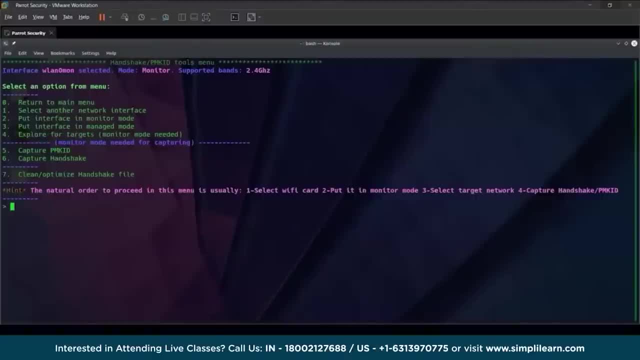 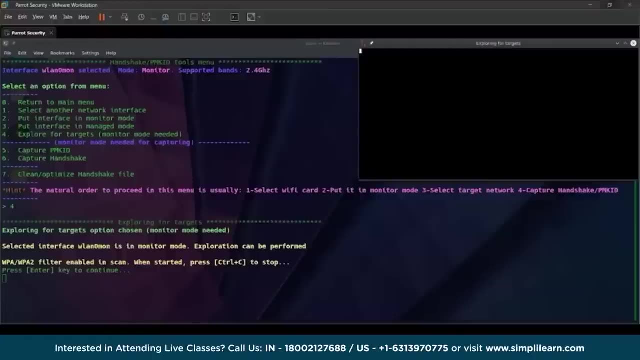 In the first step we have to explore for targets and it is written that monitor mode is necessary to select a target. So let's explore for targets and press enter. We have to let this run for about 60 seconds to get a fair idea about the networks. 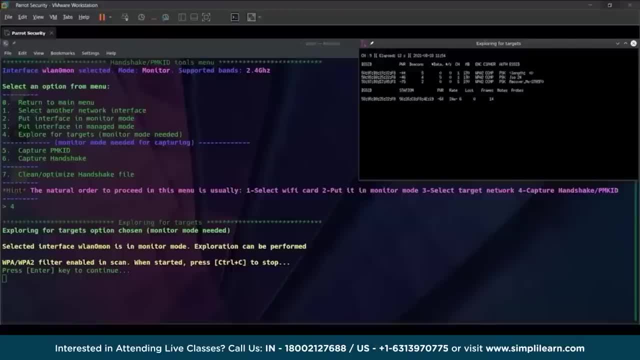 that are currently working in this system. For example, this ESS ID is supposed to be the Wi-Fi name that we see when connecting to a network. Geo24, RecoverMe- these are all the names that we see on our mobile when trying to search for the Wi-Fi. 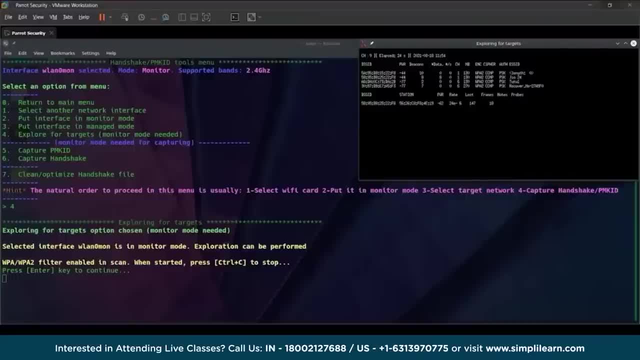 This BSS ID is supposed to be an identifier, somewhat like a MAC address, that identifies this network from other devices. The channels features on one or two. there are some many channels that the networks can focus on. This here is supposed to be a client. 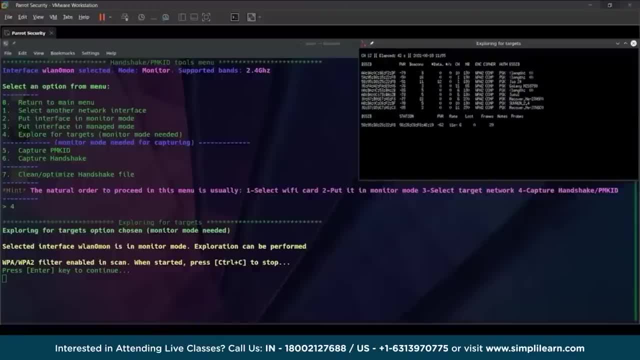 that is connected to one such network, For example, the station that you can see, 5626,. this is supposed to be the MAC address of the device that is connected to a router. This BSS ID is supposed to be which Wi-Fi it is connected to. 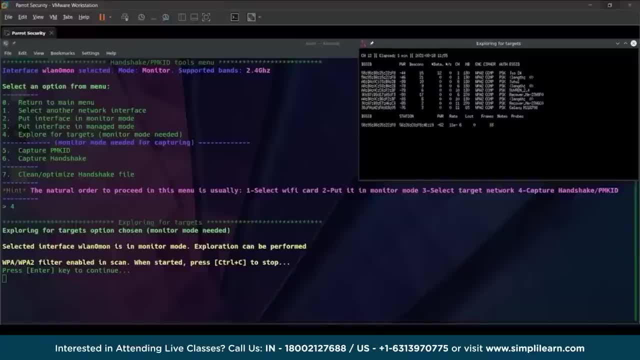 For example, 5895D8 is this one, which is the Geo24 router. So we already know which router has a device connected to it and we can use our attack to capture this handshake Now that we it has already run for one minute. 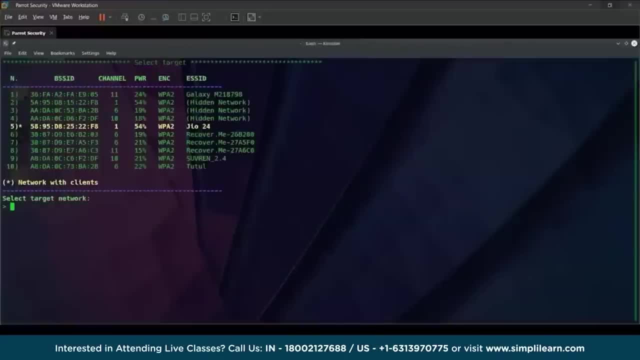 now that we press CTRL C, it will be asked to select a target. See, it has already selected the number 5,, which is the Geo24 router, as the one with clients. So it is easy to run an attack on and it is easy to capture a handshake for. 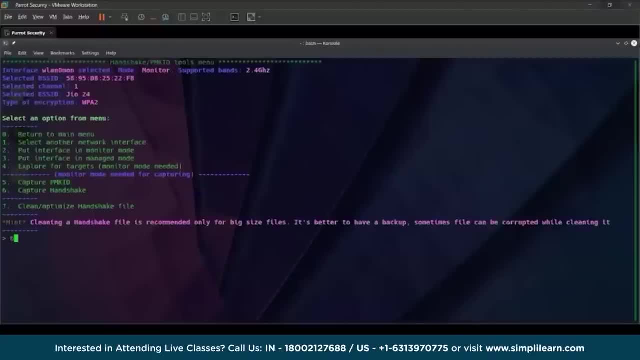 Select network 5, and we run a capture handshake. It says we have a valid WPA WPA2 network target selected and that the script can continue Now to capture the handshake. we have a couple of attacks: a deauth or a deauth air replay attack. 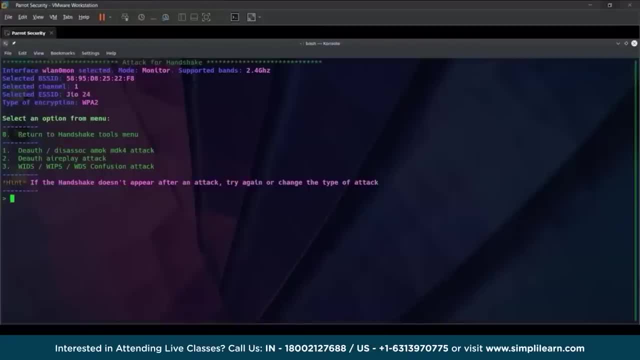 What this attack does is kick the clients out of the network In return when they try to reconnect to the Wi-Fi, as they are configured that way that when a client is disconnected, it tries to reconnect it immediately. it tries to capture a handshake file. 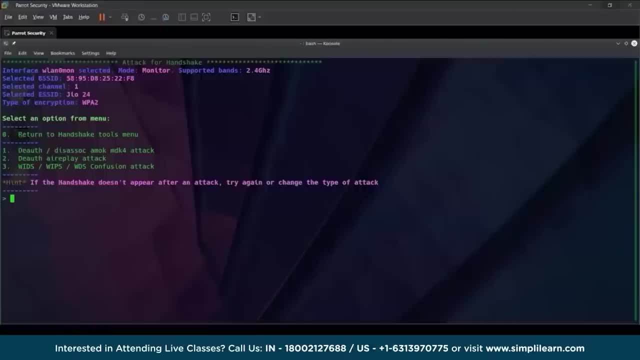 which in turn contains the security key which is necessary to initiate the handshake For our demo. let's go with the second option, that is, the deauth air replay attack. Select a timeout value. let's say we give it 60 seconds. 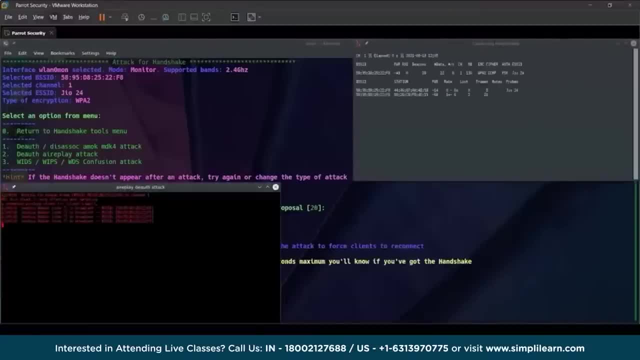 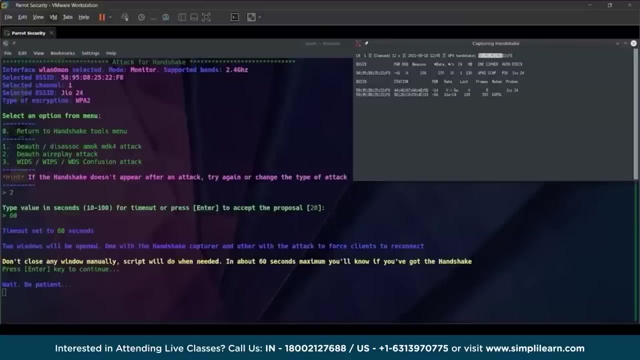 and we start the script, We can see it capturing data from the Geo24 network. and here we go. We have the WPA handshake file. Once the handshake file is captured, we can actually close this. and here we go, congratulations. 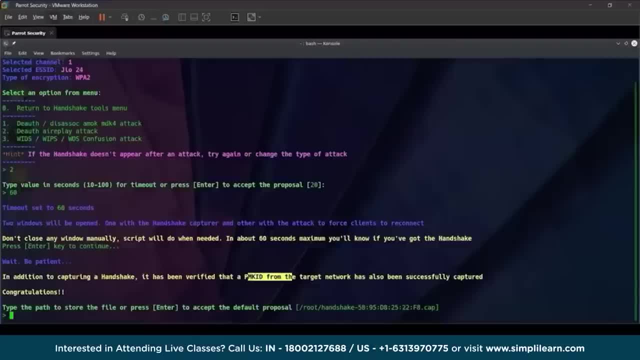 In order to capture a handshake. it has verified that a PMKID from the target network has successfully been captured. This is the file that is already stored. It's a cap file For the path. let's say we can keep it in a desktop. 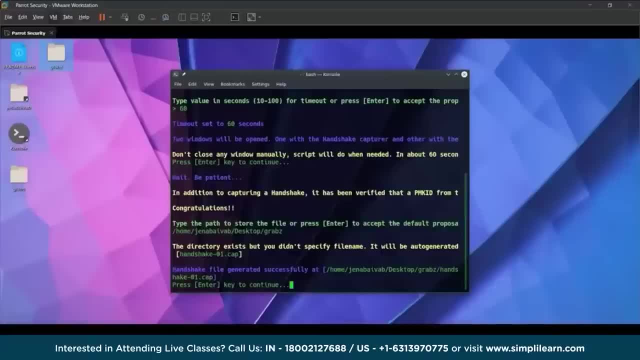 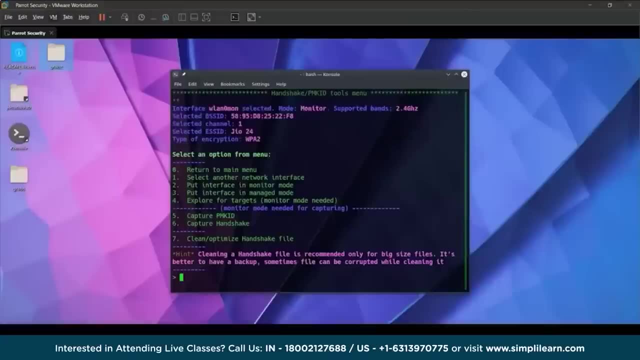 Okay, we give the path and the handshake file is generated. We can already see a target over here: Same Geo24 router with the BSSID. Now, if we return to its main menu, we already have the handshake file captured with us. 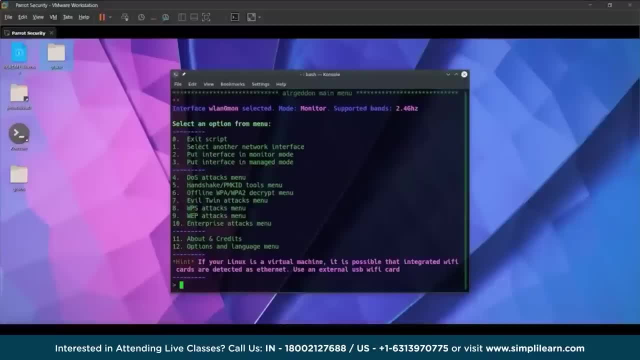 Now our job is to brute force into that handshake capture file. The capture file is often encrypted with the security key of the Wi-Fi network. If we know how to decrypt it, we will automatically get the security key. So let's go to the offline WPA WPA2 decrypt menu. 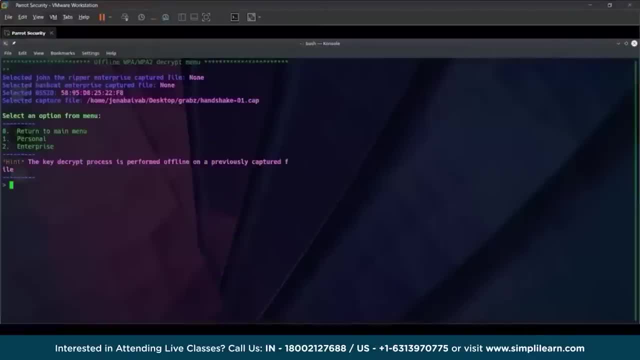 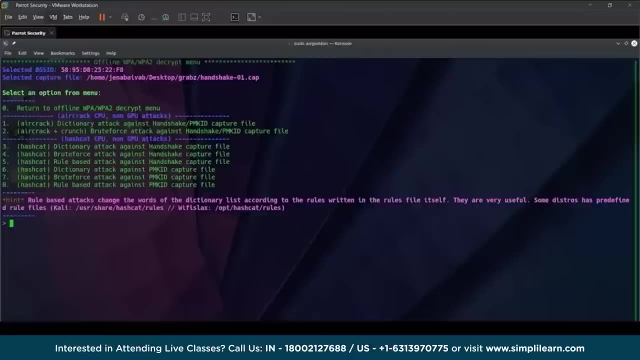 Since we'll be cracking personal networks, we can go with option 1.. Now to run the brute force tool, we have two options: Either we can go with the aircrack or we can go with the hashcat. Let's go with aircrack plus crunch. 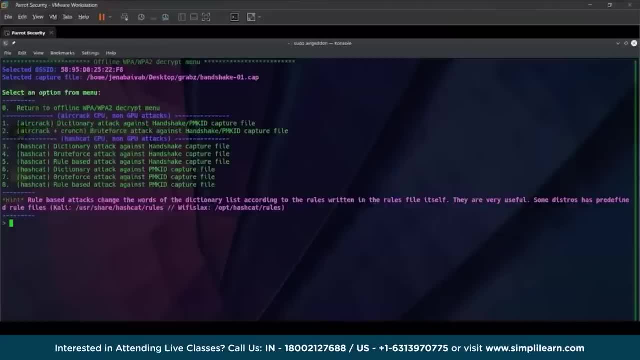 which is a brute force attack against a handshake file. We can go with option 2.. It can already detect the capture file that we have generated, So we select yes. The BSSID is the one which denotes the Jio24 router, So we're going to select yes as well. 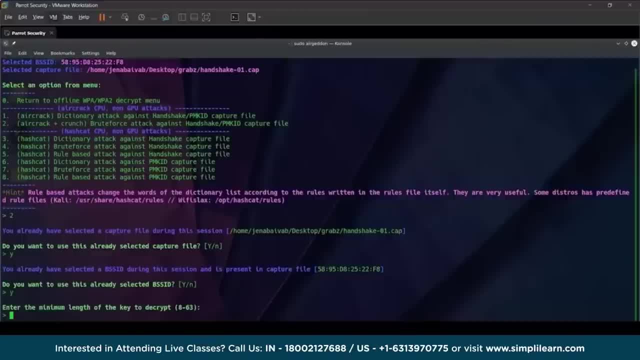 The minimum length of the key. for example, it has already checked that the minimum length of a Wi-Fi security key, which is a WPA2 PSK key, will always be more than 8 digits and below 64 digits. So we have to select something in between this range. 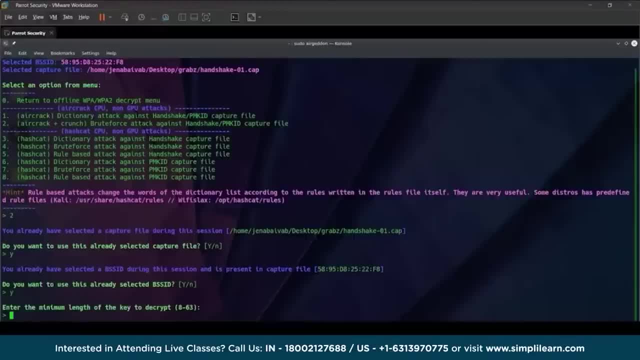 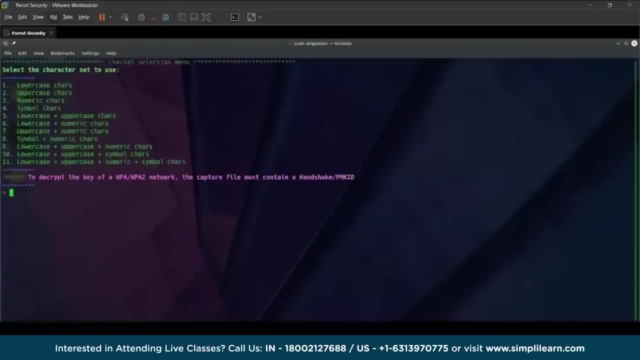 So if we already know, let's say, that the password is at least 10 digits, we can go with the minimum length as 10.. And as a reference, if we have guessed, let's say we put the maximum length as 20.. 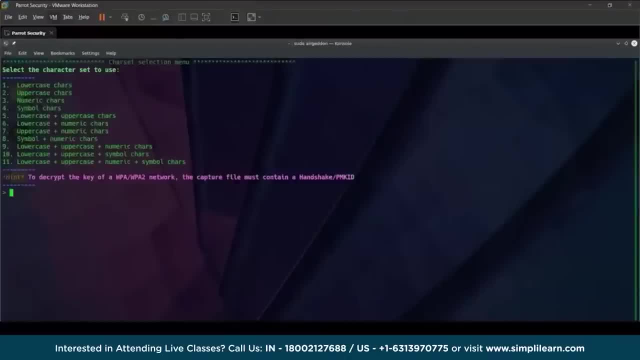 The character set that we're going to use for checking the password will affect the time taken to brute force, For example, if we already know that we have seen a user use a password while connecting to the router as something that has only numbers and symbols. 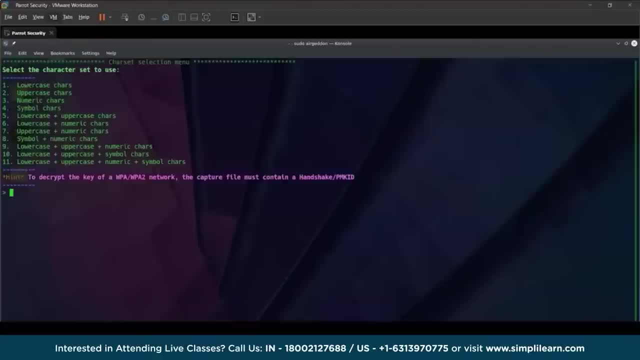 then we can choose accordingly. Let's say, if we go with only uppercase characters and numeric characters, Go with option 7. And it's going to start decrypting. So how Aircrack is working right here. you can see this passphrase over here. 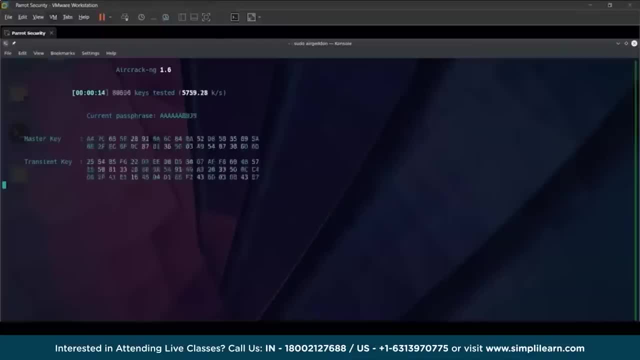 The first 5 or 6 digits are A. It starts working its way from the end, from the last character. It keeps trying every single combination. You can see the last, the fourth character from the right side, the D. It will eventually turn to E. 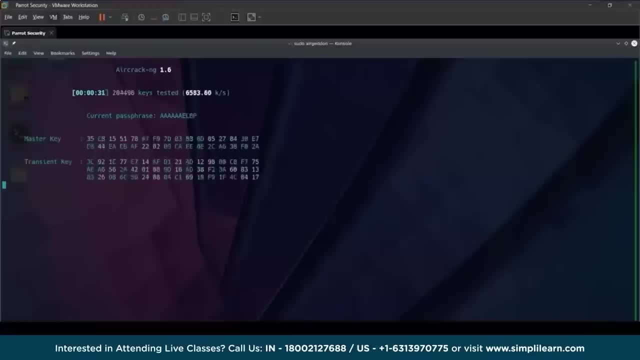 because it keeps checking up every single character from the end. This will keep going on until all the single characters are tested and every single combination is tried out, Since the handshake file is encrypted using the security key, that is, the WPA2 key of the router. 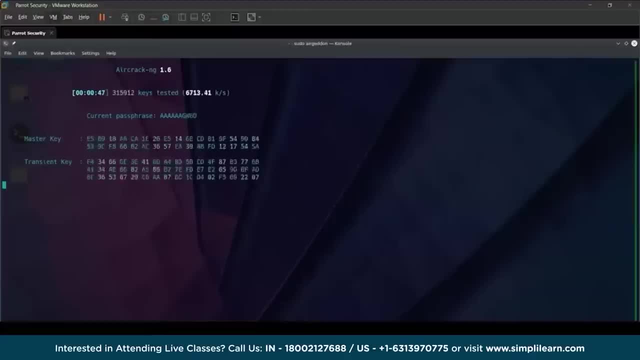 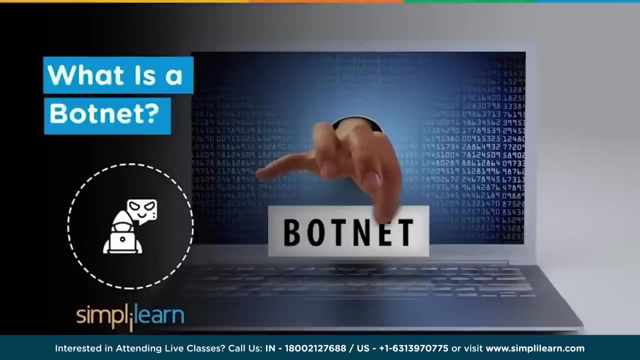 whichever passphrase is able to decrypt the handshake key completely will be the key of the Wi-Fi router. This is the way we can brute force into Wi-Fi routers anywhere in the world. Cyberattacks are frequently making headlines in today's digital environment. At any time, everyone who uses a computer. 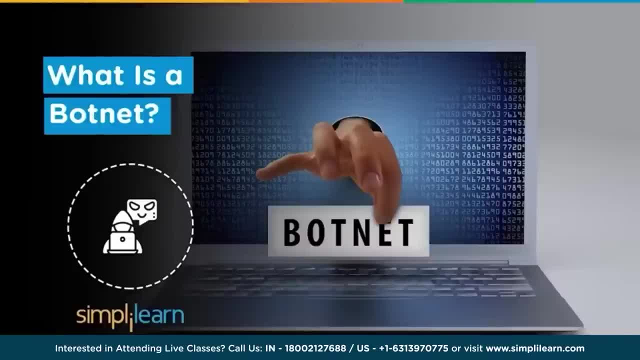 could become a victim of a cyberattack. There are various sorts of cyberattacks, ranging from phishing to password attacks. In this video we'll look into one such attack, that is known as botnet. But before we begin, if you love watching tech videos, 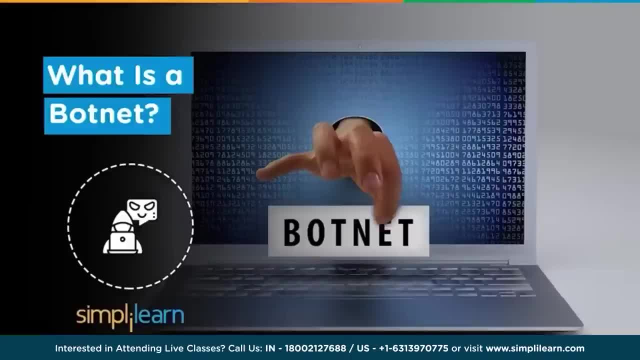 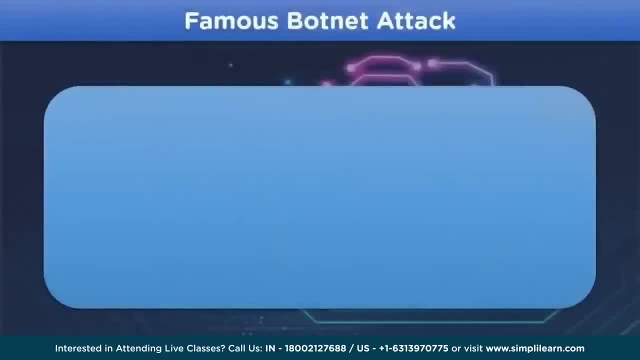 subscribe to our channel and hit the bell icon never to miss an update. To begin with, let's take a look at some of the famous botnet attacks. The first one is Mirai Botnet, which is a malicious program designed to attack vulnerable IoT devices. 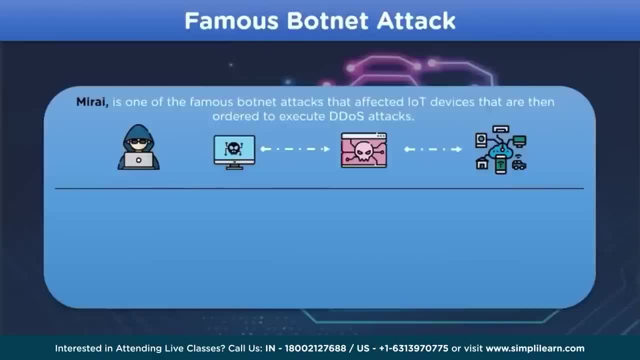 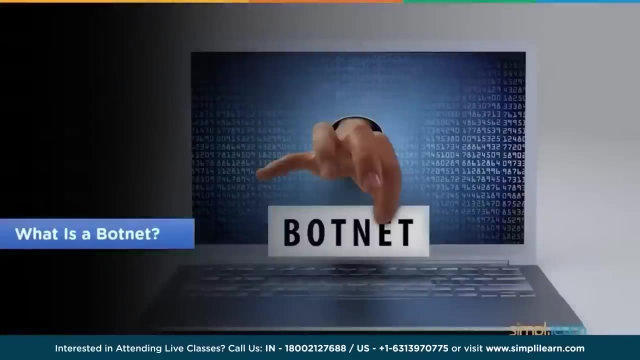 and infect them to form a network of bots that, on command, perform basic and medium-level denial-of-service attacks. Then we have the Zeus Bot, specifically designed for attacking the system for bank-related information and data. Now let's see what exactly a botnet is. 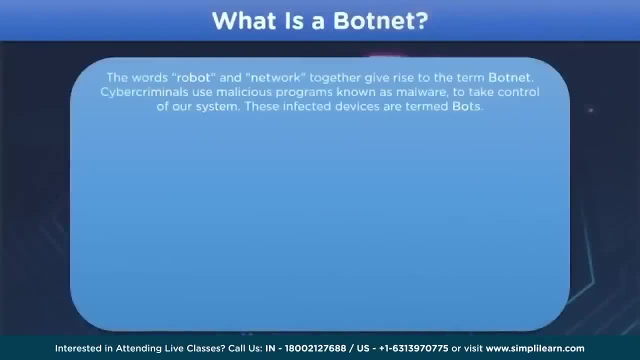 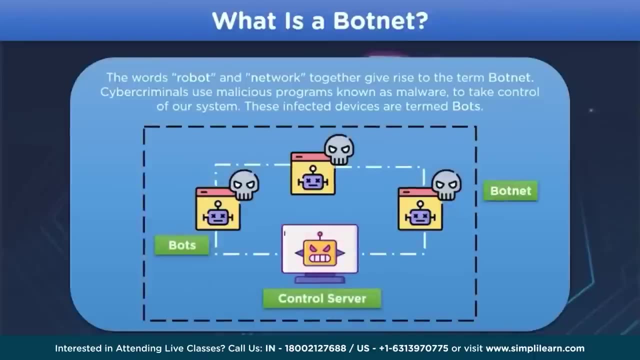 Botnet refers to a network of hijacked interconnected devices that are installed with malicious codes known as malware. Each of these infected devices are known as bots and a hijacked criminal, known as Bot Herder, remotely controls them. The bots are used to automate large-scale attacks. 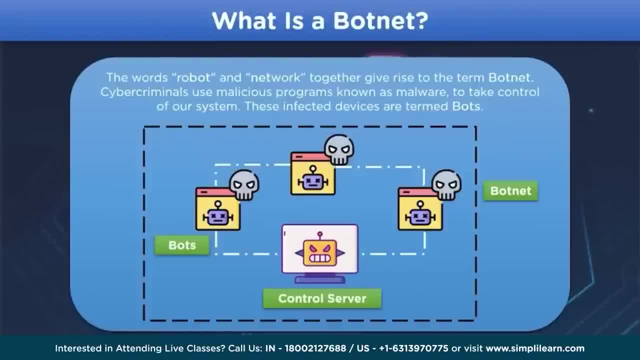 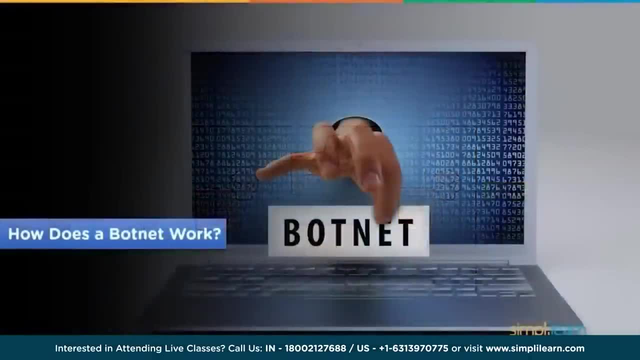 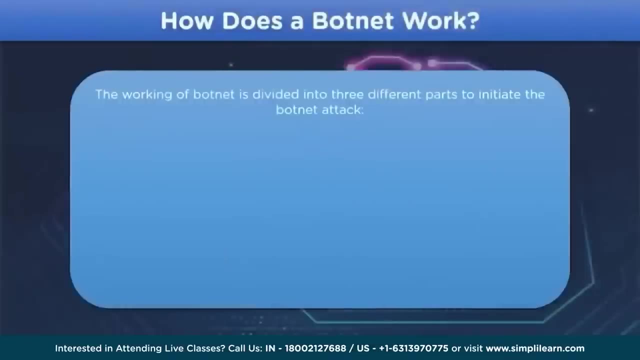 including data theft, server failure, malware propagation and denial-of-service attacks. Now that we know what exactly a botnet is, let's dive deeper into learning how a botnet works. During the preparation of a botnet network, the first step involves preparing the botnet army. 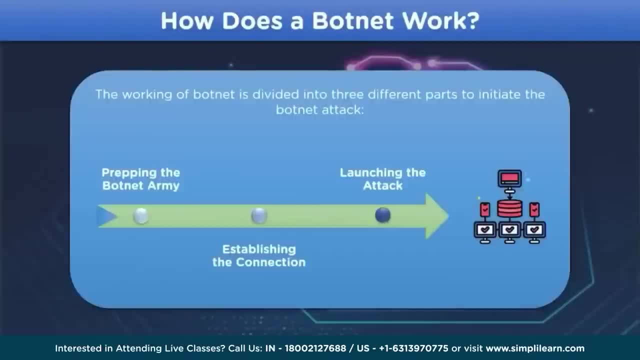 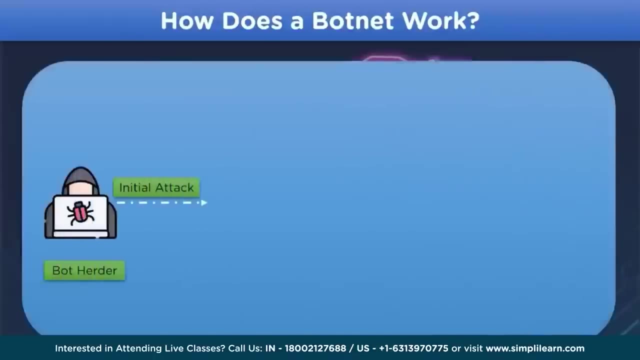 After that, the connection between the botnet army and the control server is established. At the end, the launching of the attack is done by the Bot Herder. Let's understand through an illustration. Firstly, we have a Bot Herder that initiates the attack. 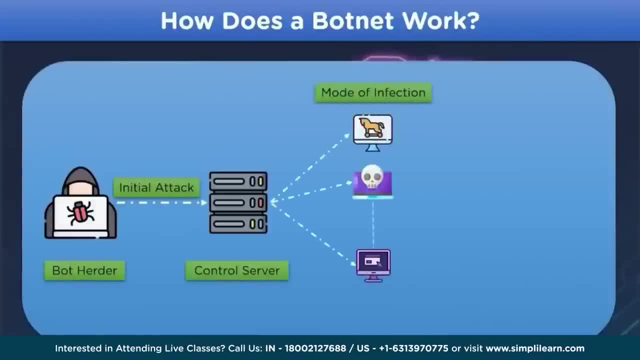 According to, the control server commands the devices that are infected with the malware programs and begins to attack the infected system. Let's see some details regarding the preparation of the botnet army. The first step is known as the prepping the botnet army. 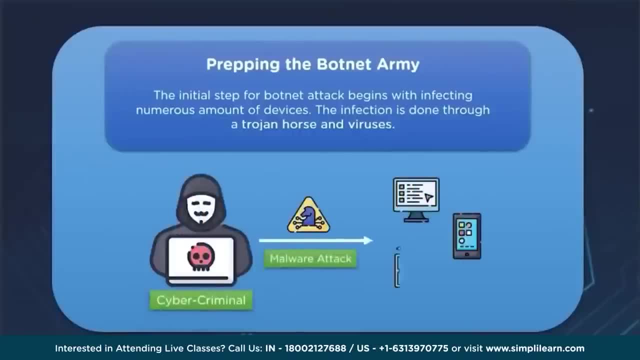 The first step in creating a botnet is to infect as many as connected devices as possible. This ensures that there are enough bots to carry out the attack. This way, it creates bots either by exploiting the security gaps in the software or websites or using phishing attacks. 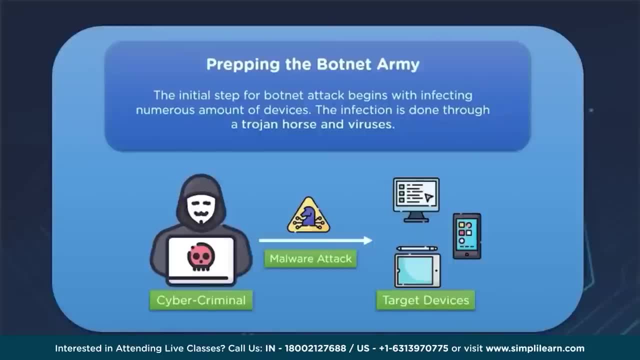 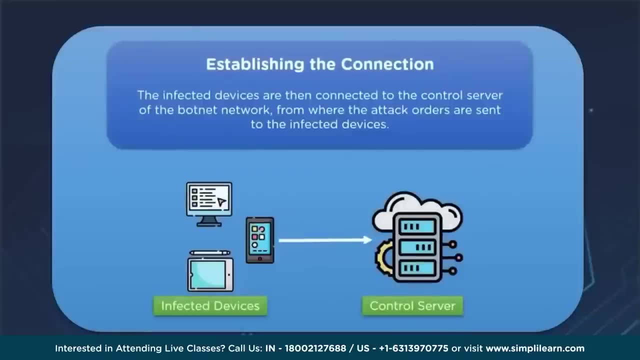 They are often deployed through Trojan horses. For the next step we have establishing the connection. Once it hacks the device, as per previous step, it infects it with the specific malware that connects the device back to the control bot server. A Bot Herder uses command programming. 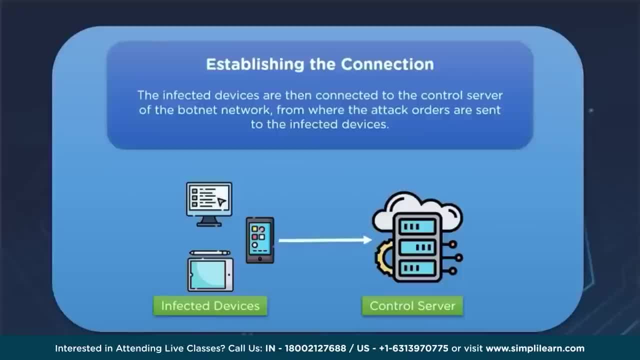 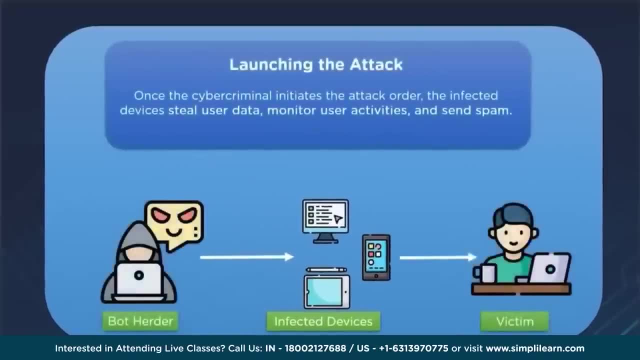 to drive the bot's actions, And the last step is known as launching the attack. Once infected, a bot allows access to admin-level operation like gathering and stealing of data, reading and rewriting the system, data monitoring user activities, performing denial-of-service attacks. 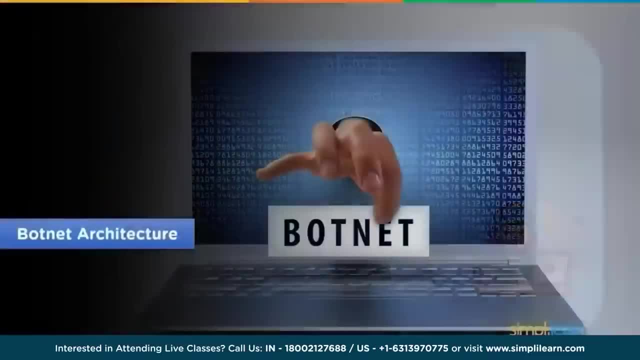 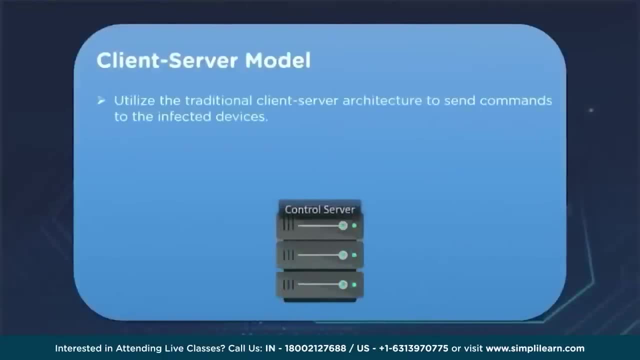 including other cybercrimes. Now let's take a look at the botnet architecture. The first type is known as client-server model. The client-server model is a traditional model that operates with the help of a command and control center server and communication protocols like IRC. 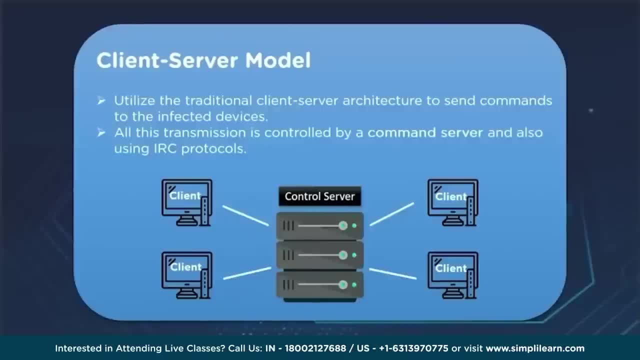 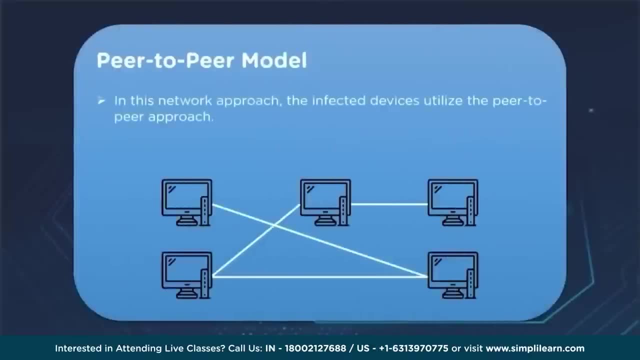 When the Bot Herder issues a command to the server, it is then relayed to the client to perform malicious actions. Then we have peer-to-peer model Here. controlling the infected bots involves a peer-to-peer network that relies on a decentralized approach. 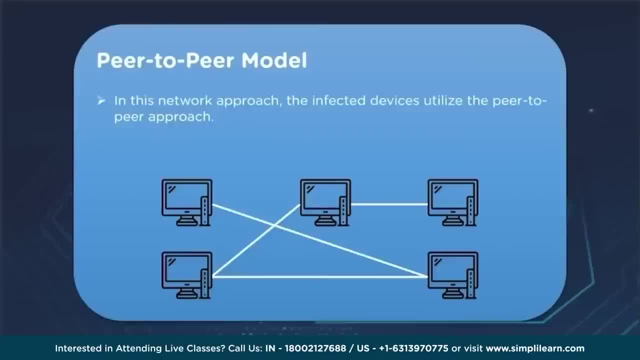 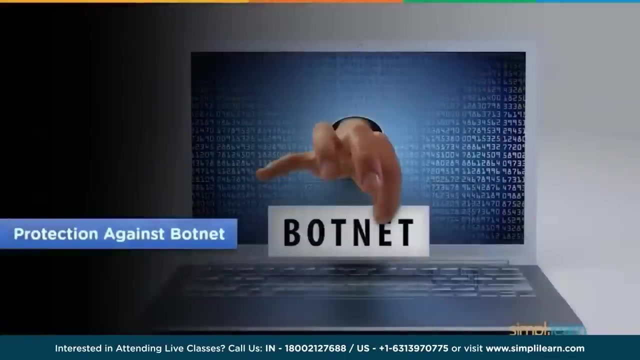 That is, the bots are topologically interconnected and acts as both CNC servers, that is, the server and the client. Today, hackers adopt this approach to avoid detection and single-point failure. In the end we will see some points on some countermeasures against botnet attacks. 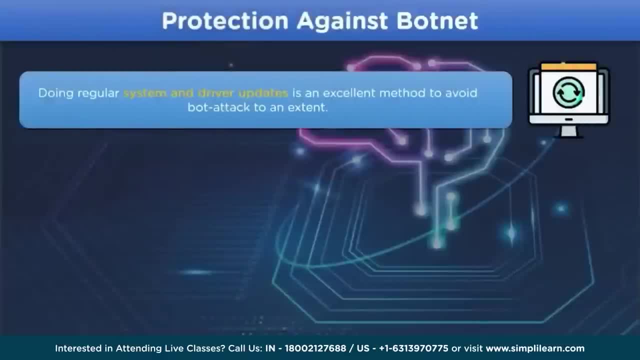 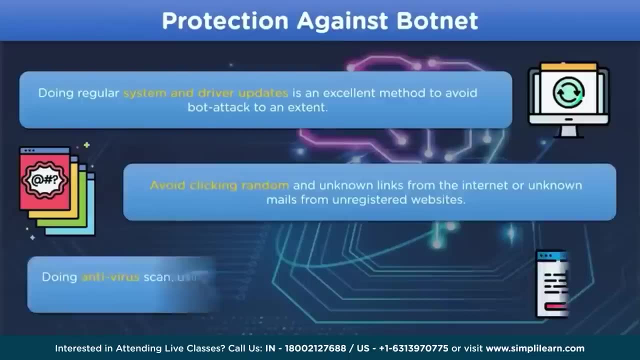 The first step is to have updated drivers and system updates. After that, we should avoid clicking random pop-ups or links that we often see on the Internet. And, lastly, having certified antivirus, anti-spyware software and firewall installed into a system. 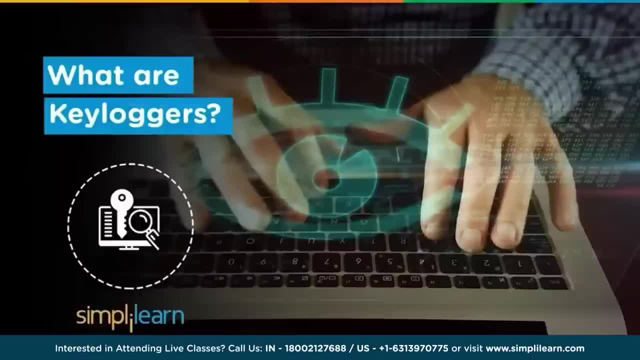 will protect against malware attacks. The Internet is an endless source of information and data. Still, in some cases, we come across some occurrences like cyberattacks, hacking, force entry, which may affect our time on the web. Hi everyone and welcome to the SimplyLaunch channel. 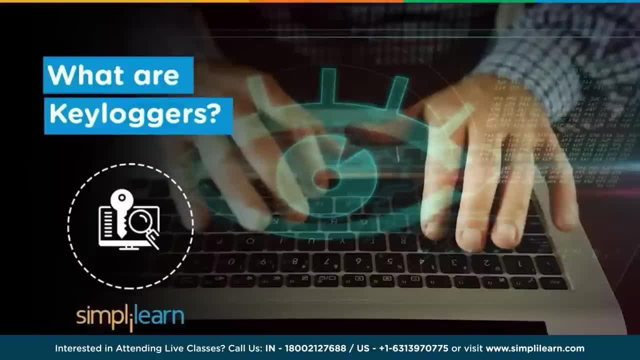 Today we will discuss a topic that secretly records our input data, that is known as e-loggers. But before we begin, if you like watching tech videos, subscribe to our channel and hit the bell icon to never miss an update. To understand the e-logging problem better, 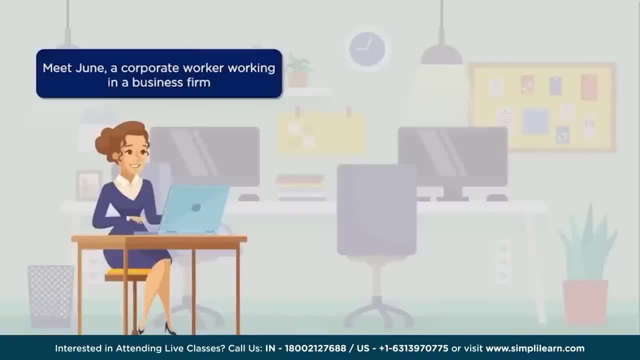 let's take a look at an example. This is June. She works in a business firm where she manages the company's data regularly. This is Jacob from the information department, who is here to inform her about some of the security protocols During the briefing. 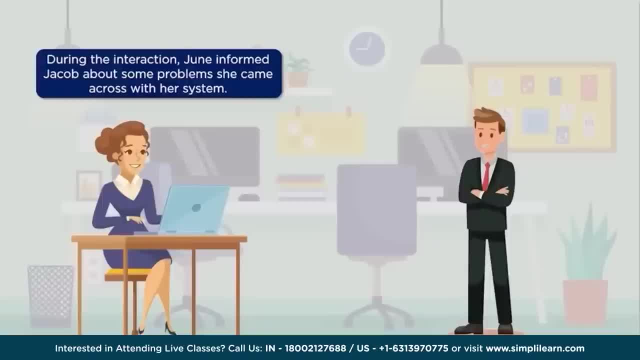 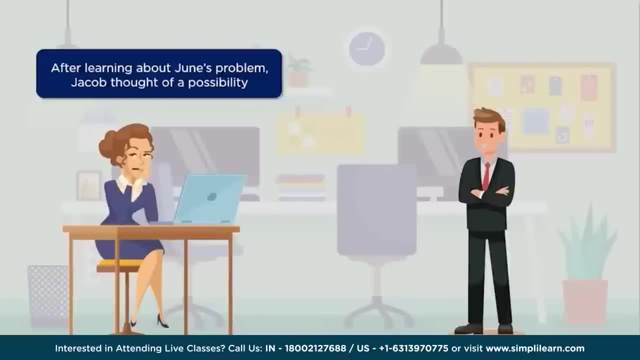 she informed him about some of the problems her system was facing with, which included slow reaction speed and unusual internet activity. As Jacob heard about the problems with the system, he thinks of the possibility what could be the reason behind these problems her system was facing with? 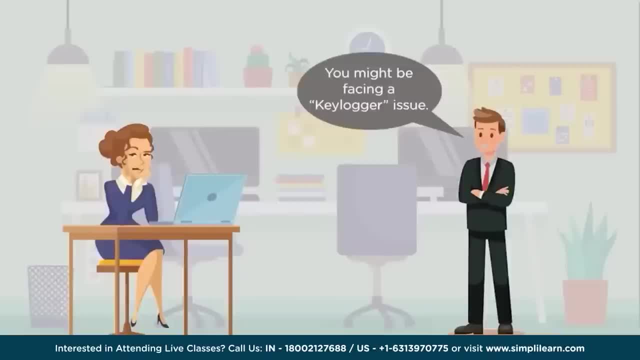 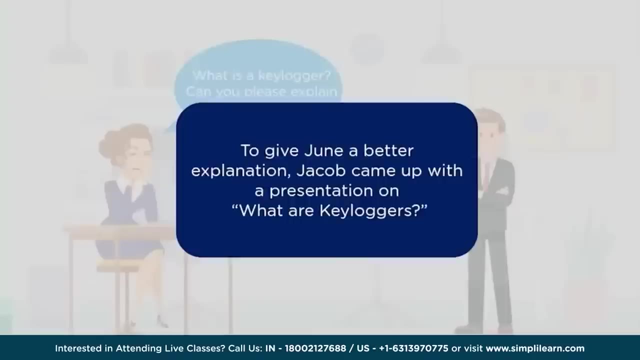 The conclusion that he came across was the keylogging issue, Unknown to the problem her system was facing with. she asked him about some of the details regarding it. For today's topic, we'll learn what exactly keyloggers are and how they affect our system. 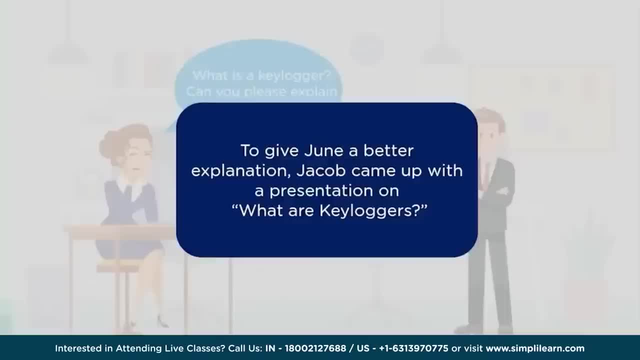 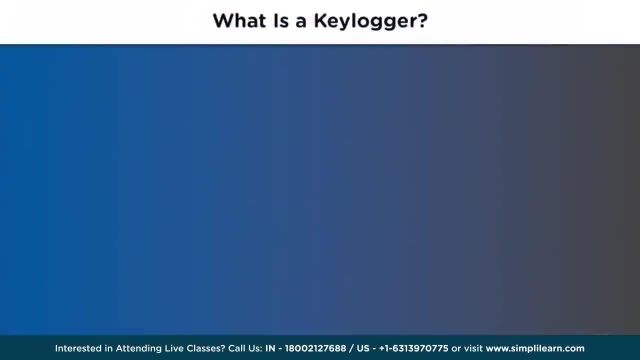 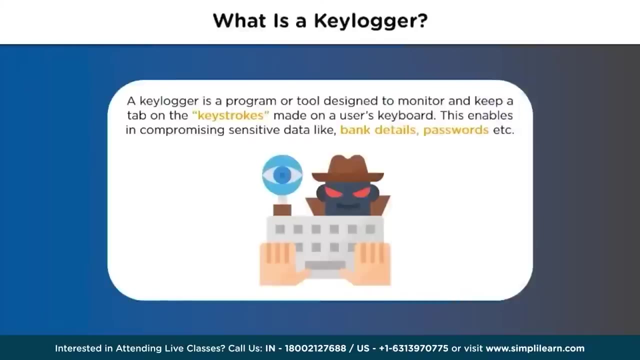 what are the harmful effects that keylogging can bring into the system? To begin with, we'll learn what exactly the keylogging program is. As the name suggests, keylogger is a malicious program or a tool that is designed to record keystrokes that are typed during data input. 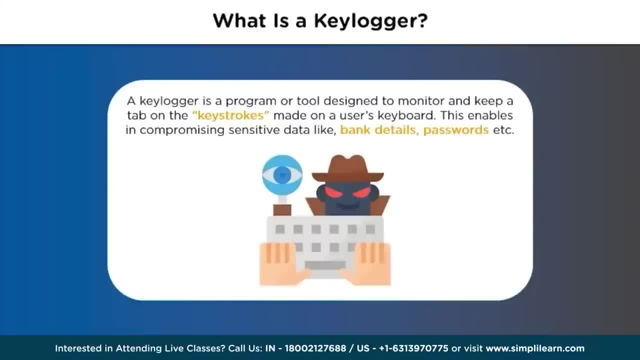 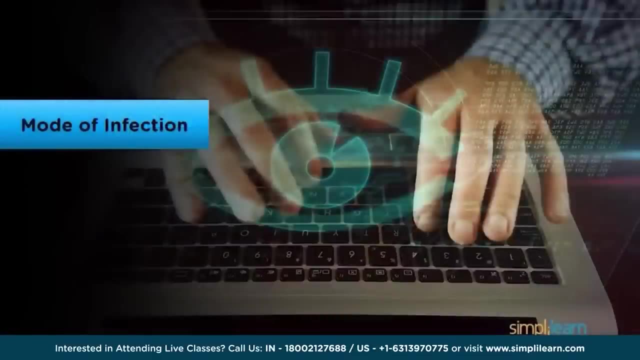 and record them into a log file. Then the same program secretly sends these log files to its origin, Where they can be used for malicious acts by the hacker. Now that we know what the keylogging program is, let's take a look how they enter into the system. 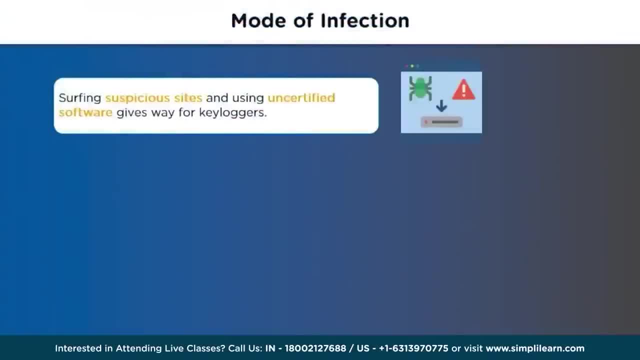 Searching for a suitable driver for a system can often lead to the installation of the keylogging program into the system. If we often visit suspicious sites and uncertified software are installed into a system, Then if we use unknown links or visiting unknown websites, 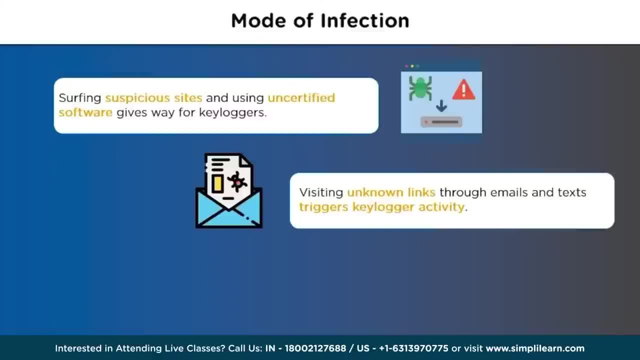 which come through unknown addresses can also be a reason behind the keylogging issue entering into the system. And lastly, there are often cases where different pop-ups that we often see on social sites or different media sites can lead to the installation of keylogging program into a system. 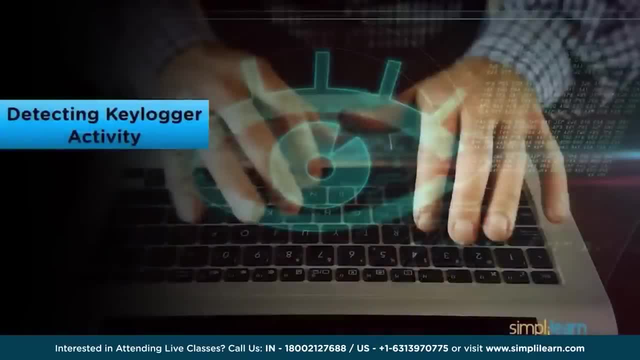 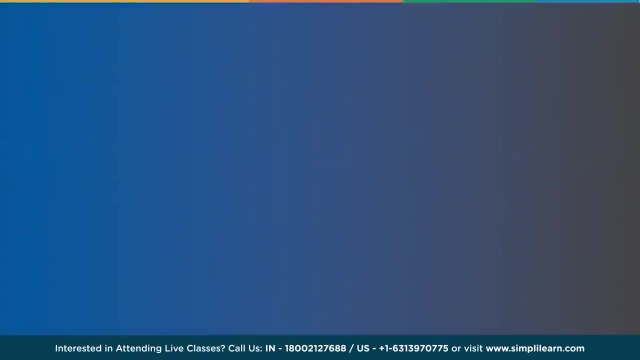 Now that we know how the problem gets into the system, let's take a look how to identify whether the system is infected by the keylogging issue. The keylogging issue can be identified if there are often cases when a keyboard lags behind the system. 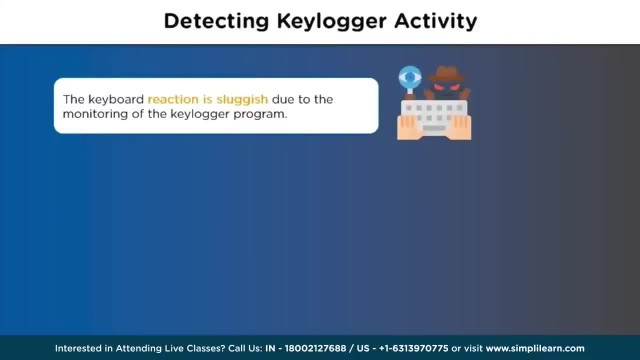 The data that we enter sometimes is stuck in between when we type through the input. Then there are cases when the system freeze occurs unknowingly to what exactly could be the reason behind them, And also there are delayed reaction time for different applications that run on the system. 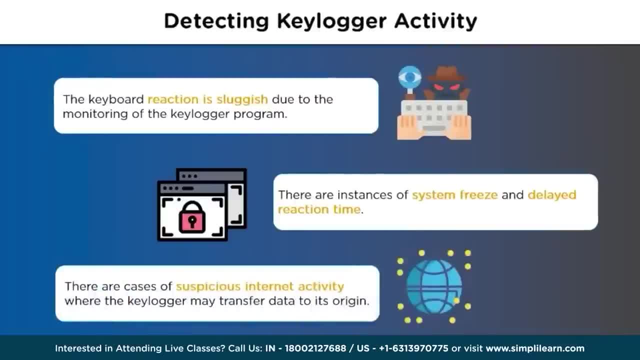 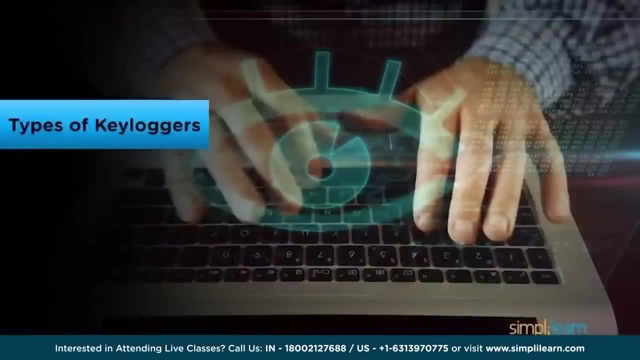 And lastly, there are different cases when we often see suspicious internet activity on the system that we don't know about, This could lead to the identification of a problem into the system. Now we'll take a look at different types of keyloggers. 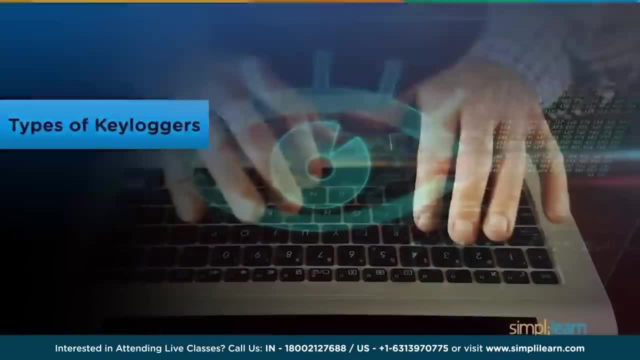 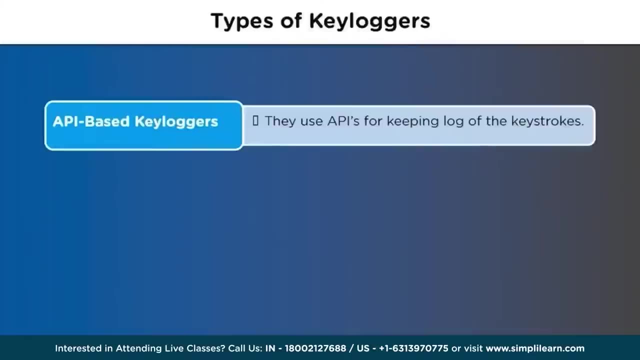 that are present on the net which can harm our system differently. The first problem that keyloggers arouse is API-based- The most common keylogging case, which uses APIs to keep a log of the typed data and share it to its origin for malicious purposes. 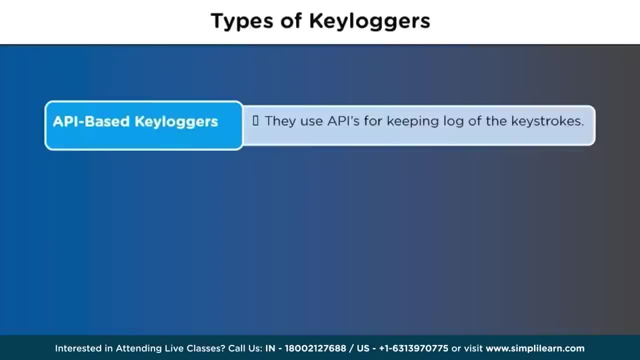 Each time we press a key, the keylogger intercepts the signal and logs it. Then we have form-grabbing-based keyloggers. as the name suggests, They are based keyloggers that store the form data, That is, if we often use web forms. 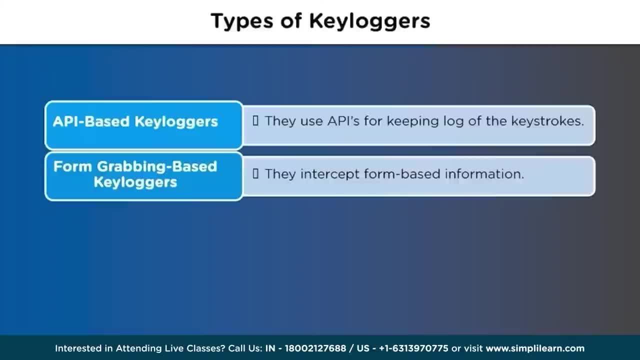 or different kinds of forms to enter different data. they can be recorded into the system by the program and send it to its origin. Then we have kernel-based keyloggers. These keyloggers are installed deeply into the operating system where they can hide. 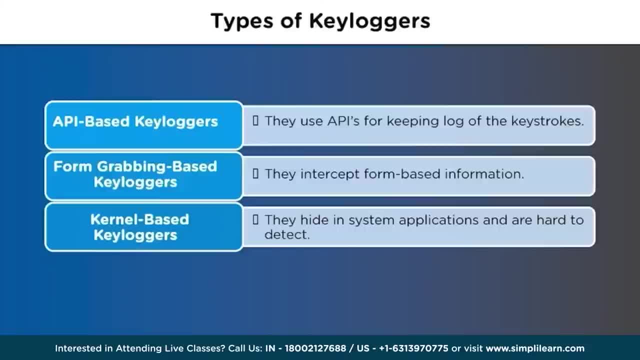 from different antivirus, if not checked properly, And they record the data that we type on the keyboard and send it to its origin. And lastly, we have hardware keyloggers. These keyloggers are present directly into the hardware, that is, they are embedded into the system. 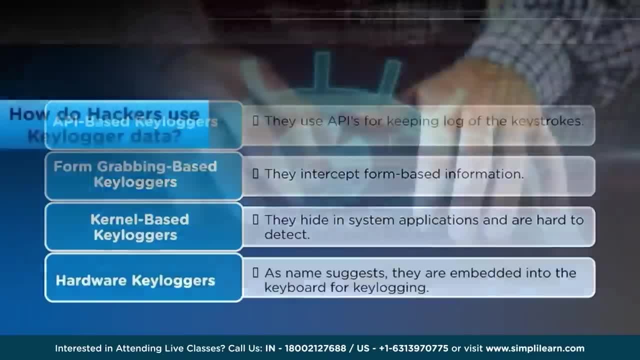 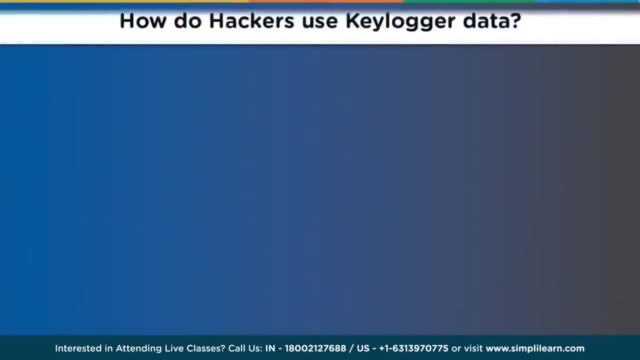 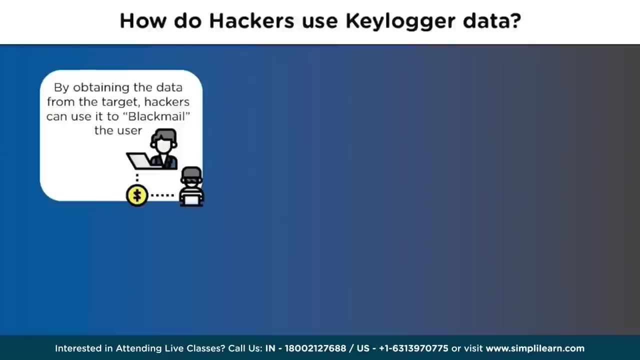 where they record the data that we type on the keyboard. Now let's take a look how hackers differentiate different types of recorded data and exploit them. When hackers receive information about the target, they might use it to blackmail the target, which may affect. 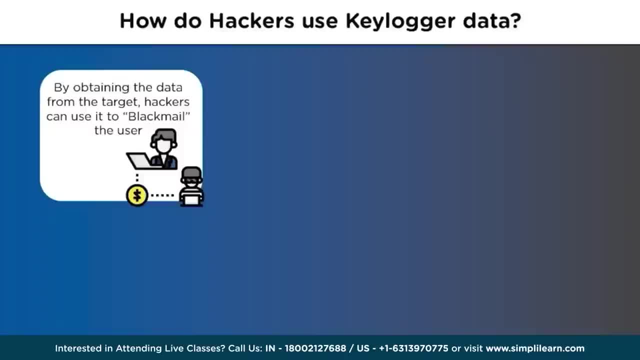 the personal life of the target and also blackmail them for different money-related issues. Then, in case of company, data that is recorded by the keylogging program can also affect the economic value of the company in the market, which may lead to the downfall of the company. 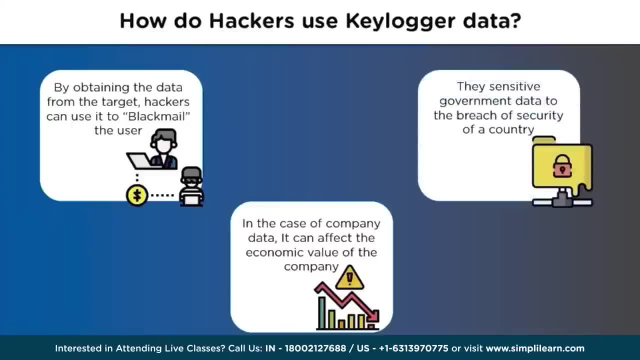 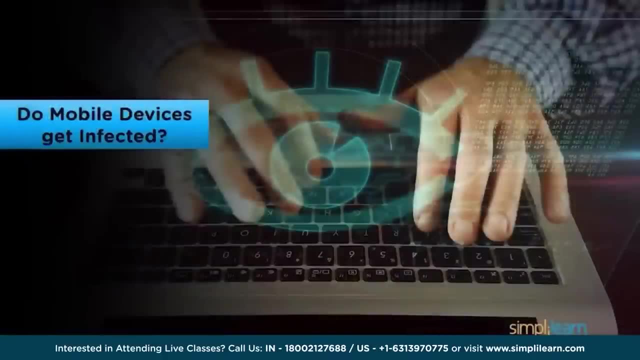 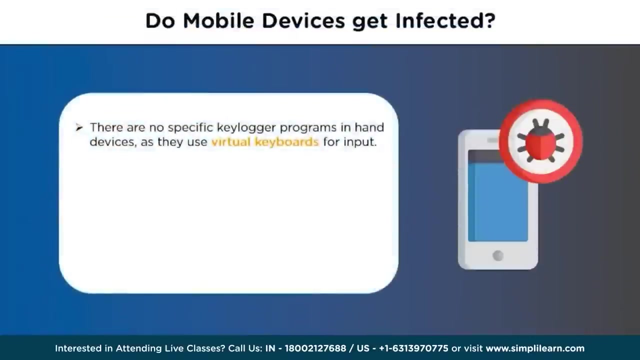 Also, in some cases, the keylogging program can also log data about military secrets, which may include nuclear codes or security protocols, which are necessary to maintain the security of a country. Now let's take a look whether mobile devices get infected with the keylogging issue or not. 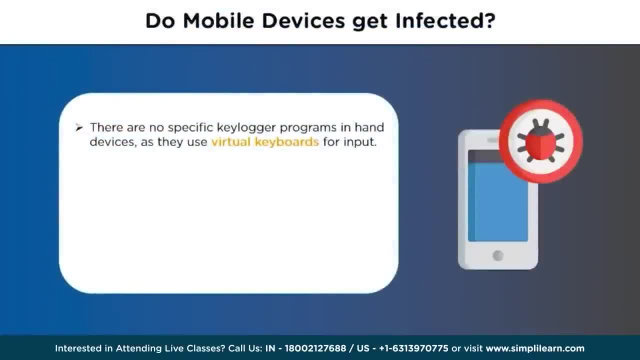 In the case of hand devices, infection of keyloggers are low in comparison to the computer systems as they use on-screen keyboard or virtual keyboard, But in some cases we often see different kinds of malicious programs getting installed into the hand device. if we often visit. 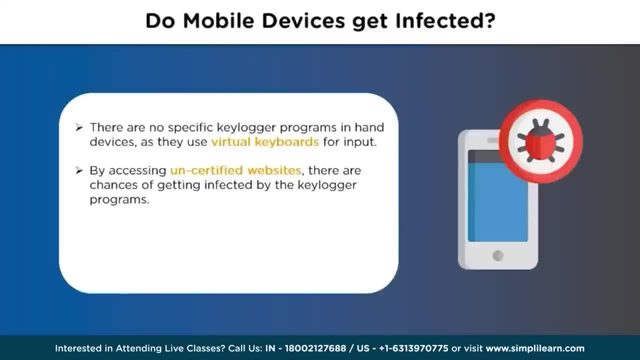 different uncertified websites or illegal websites. So let's take a look at different kinds of malicious programs that get infected by the hacker or the cyber criminal that installs the particular malicious program into the system. Now, to prevent a system from getting infected by the keylogging program: 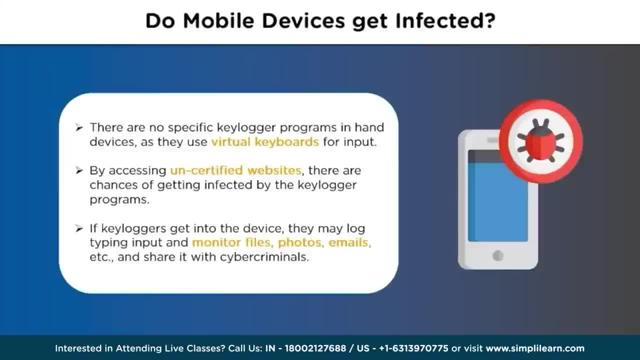 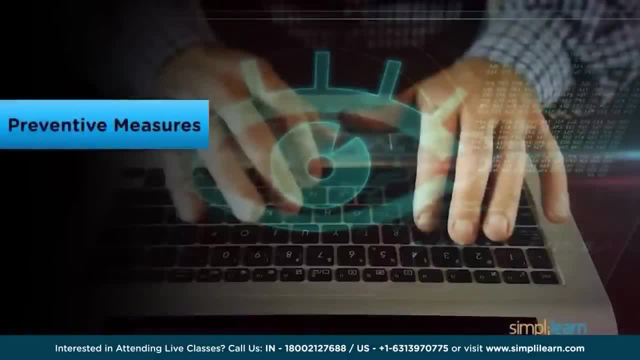 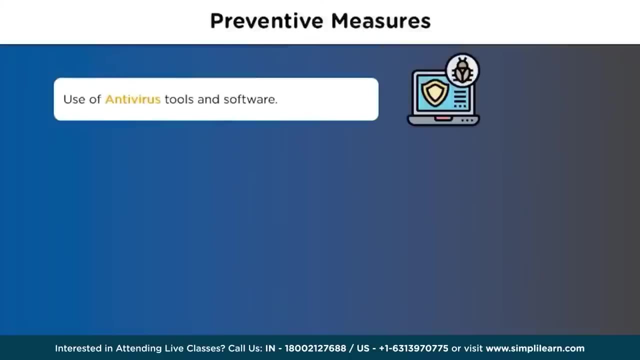 let's take a look at different points. For example, if the hacker or the cyber criminal installs the particular malicious program into the system, the hacker or the cyber criminal can also get infected with the keylogging program. The first point includes using of different 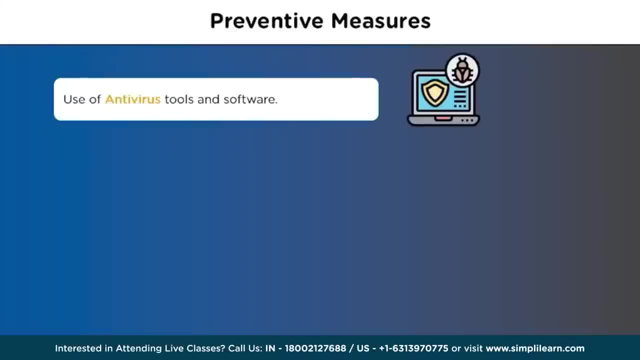 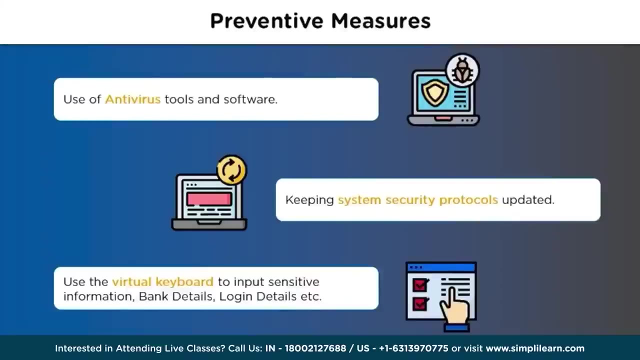 antivirus softwares or tools which can prevent the entering of malicious program into the system. Then, keeping system security protocols regularly updated is also a good habit. And, lastly, using virtual keyboard to input our sensitive data, which may include bank details, login details. 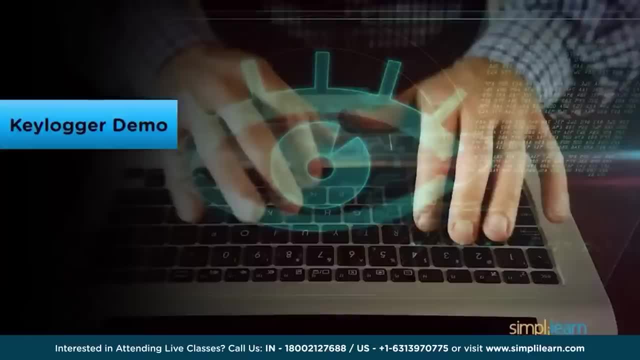 or different passwords related to different websites. Now that we have some understanding of the topic of keyloggers, let's take a look at the demo to further increase the knowledge about the topic. For the first step, we have to download some of the 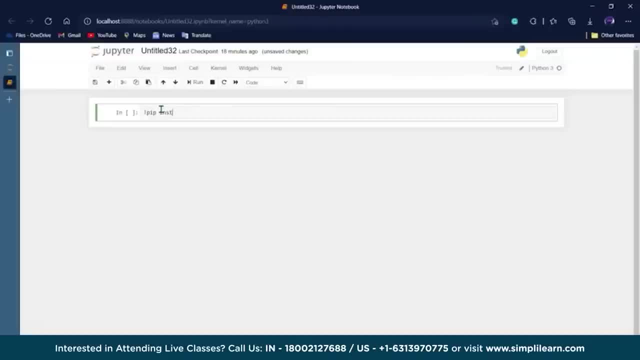 important libraries that are required into the system, which is this library. Now we will run it. The system says the library is already installed into the system. Now let's take a look at the system and see what exactly modules are required from the. 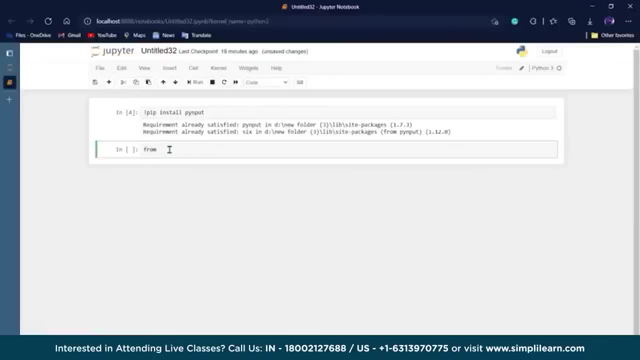 particular library. From this library, we will import the keyboard module, which will help us to record the data that we type on the keyboard. Now, from the same, we will also import key module and the login module, which will help us to record. 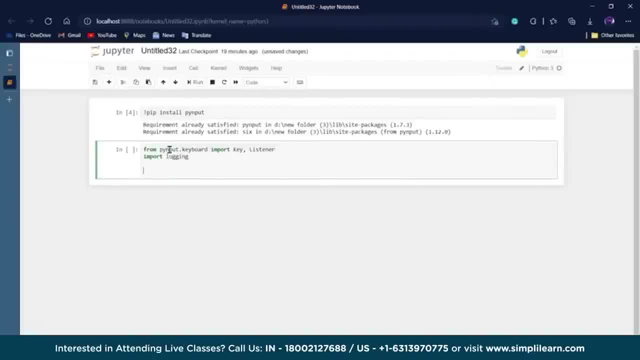 the data into a log file. For the next part, we will write a piece of code that will allow us to save the data that is recorded by the program into a text file that will be named as key underscore file. Now we will provide. 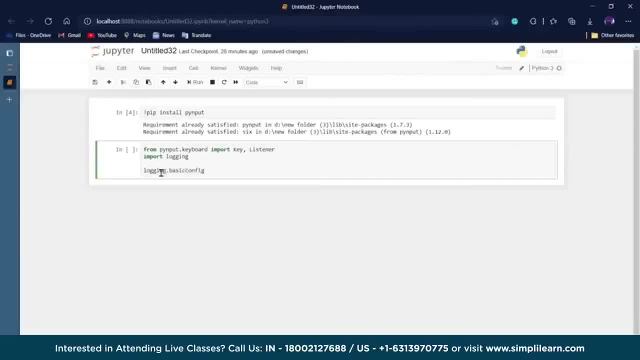 it with the file name that will be given as klog dot txt file, and also through the part where the format of the data is recorded in the log file. Now we will write the format in which the data will be recorded into the log file. 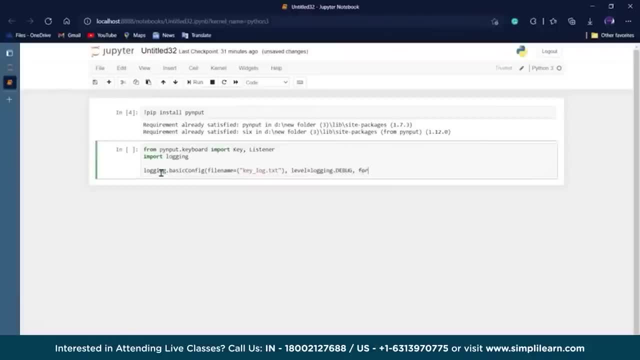 which will be given, as the format would be the message and the time, along with the time stamp given as percentage and ending it with the bracket. Now for the next step. we will design two of the functions that will be used as while press function. 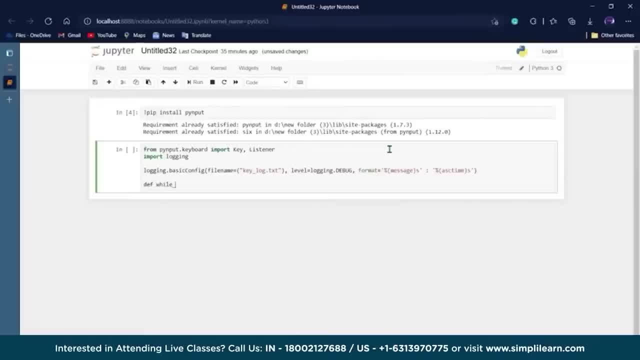 and while release function. Let's take a look. While press function would be a function that will come into play when the keyboard key has been pressed- And this would go for the format that we designed in the above line- And logging the pressed key, 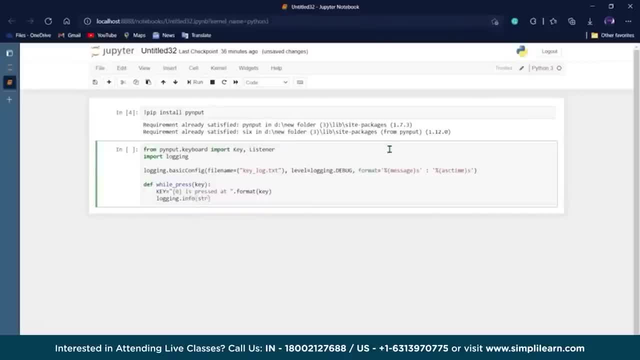 info, a string file to be recorded into the log file. Now we'll design a function that is while release. That will come into play. The escape key has been pressed, That is, the program will dominate itself and the program will stop from. 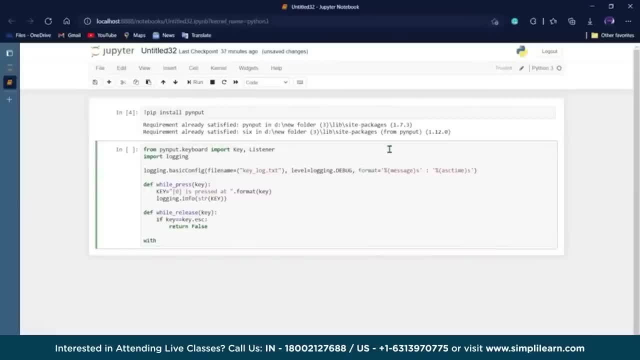 running And in the end that will be going for while press and on release will contain while release function as listener. So this is the function that will be going for while press, and now this part would join the different threads and store them. 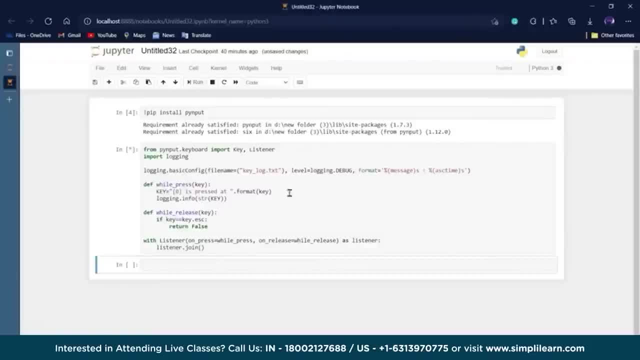 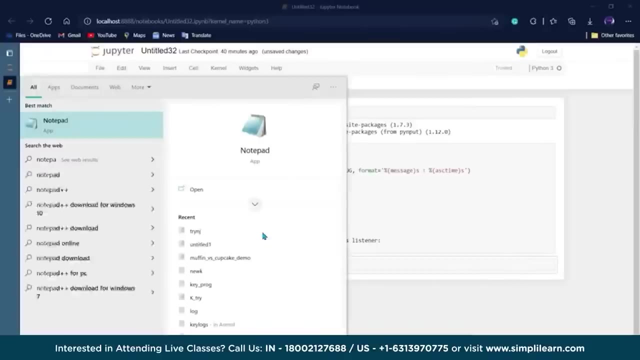 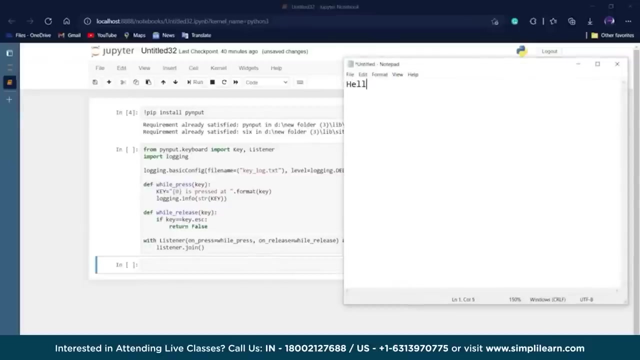 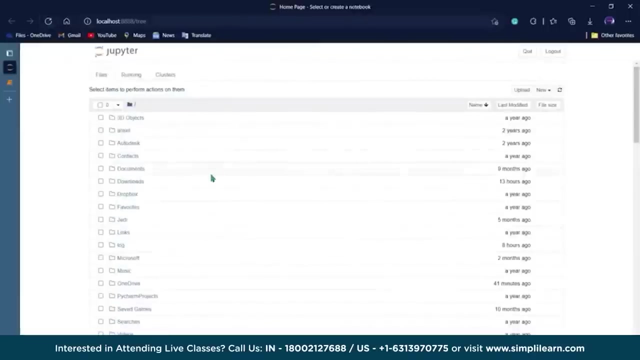 into the log file. Now that we have completed the code for the program, let's run it And on the notepad we'll write hello world, which will be the basic whether the program is working or not. Let's take a. 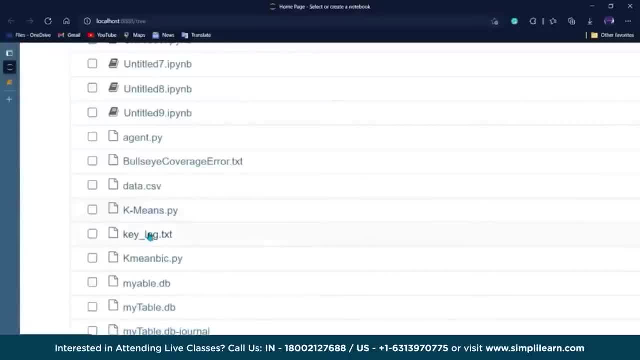 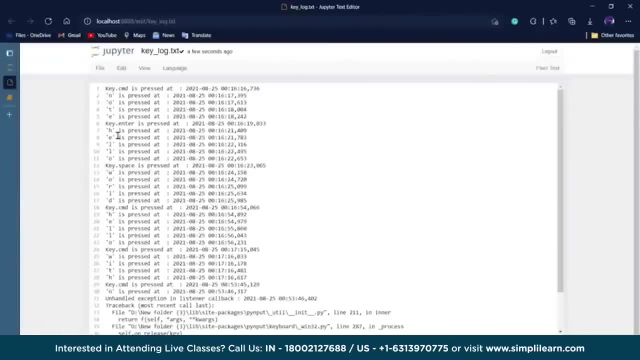 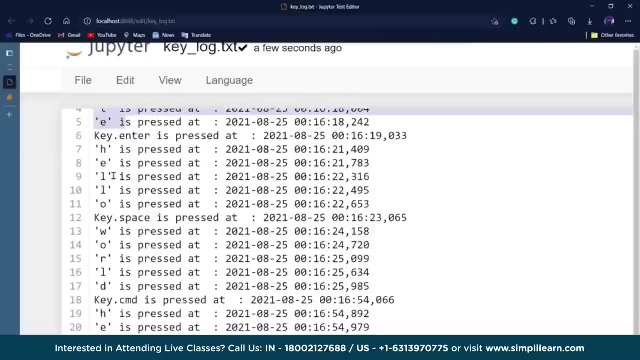 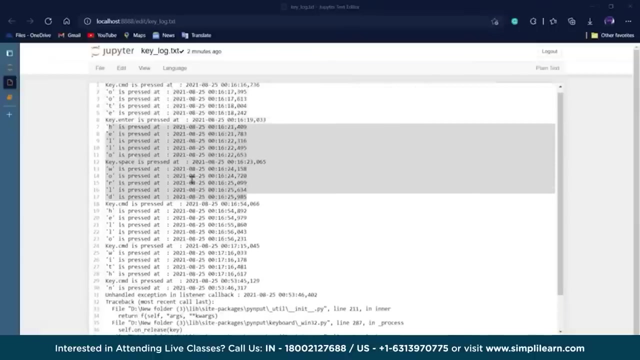 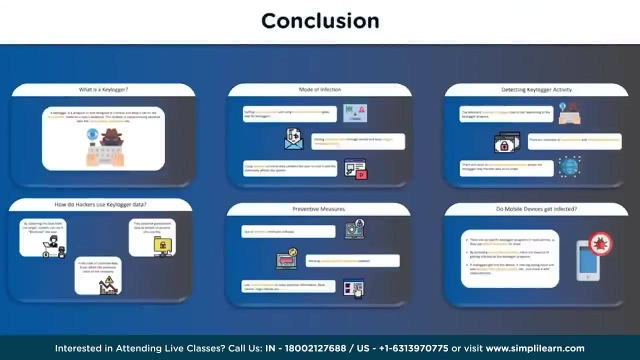 look And we'll go for the main part that we created. Let's open it And over here we have the data that is created. As we started with note, then this is the hello world part that we created. Then we learned. 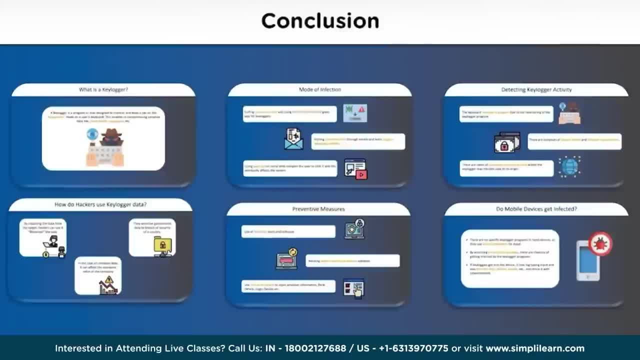 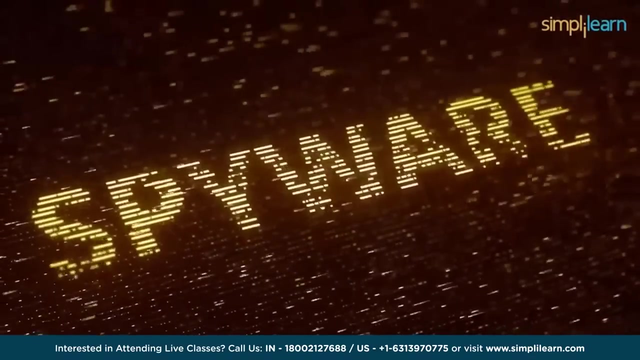 what different modes are present, how the system get infected with the key logging problem. Then we learned what different types of key loggers are present in the system. Before we learn about the Pegasus platform, let us understand what spyware is and it's. 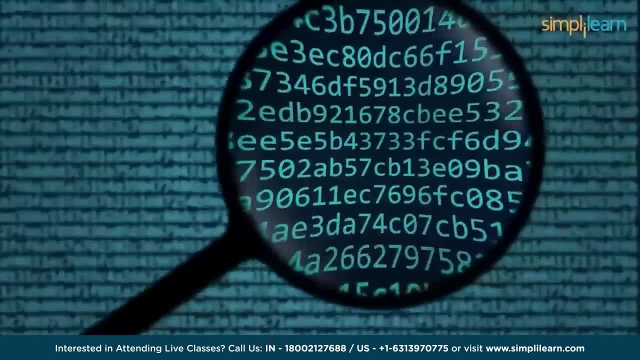 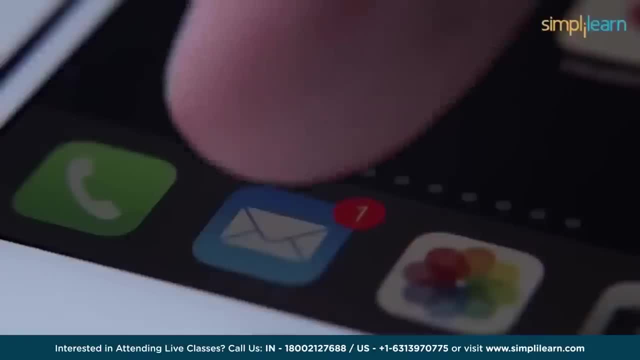 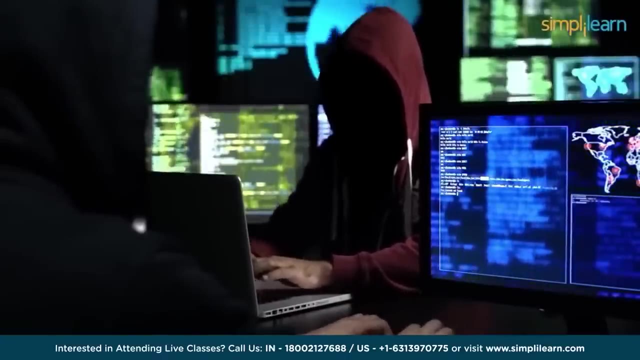 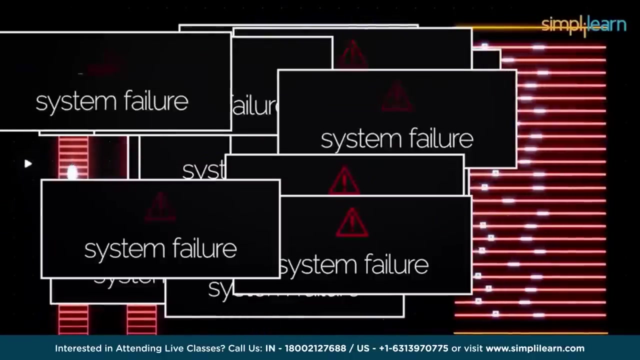 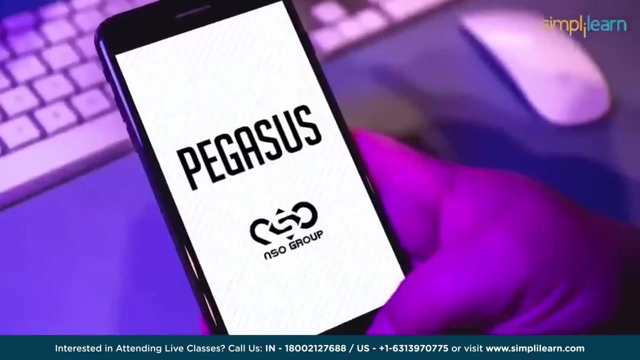 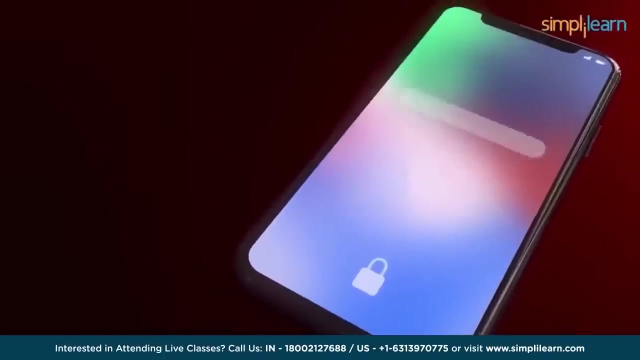 working. Spyware is a category of malware that can gather information regarding a user or a device straight from the system. Some spyware systems, even clicking on the link isn't necessary to trigger the malicious payload. This can ultimately cause security complications and further loss. 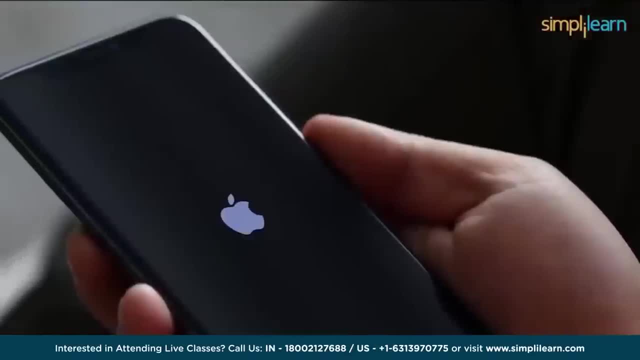 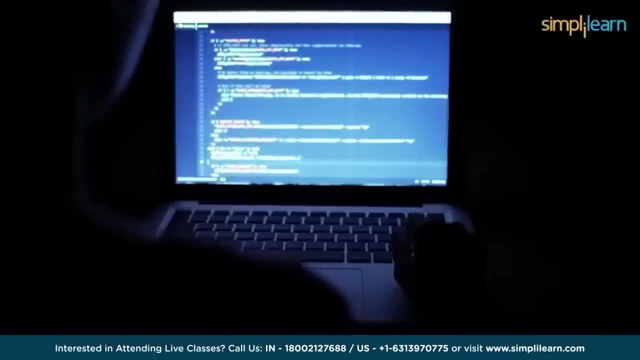 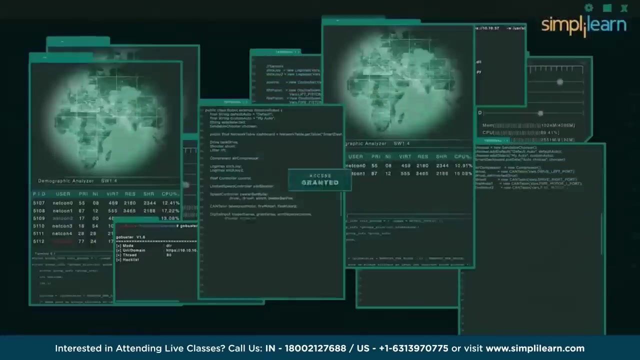 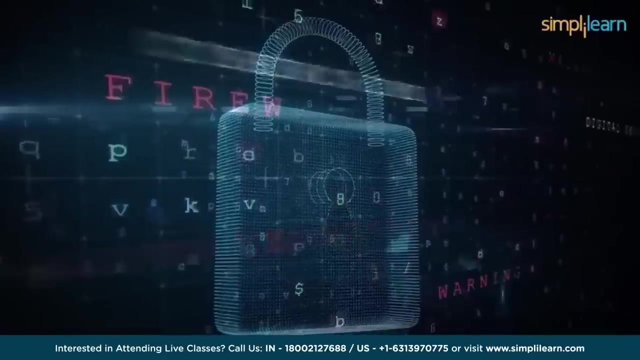 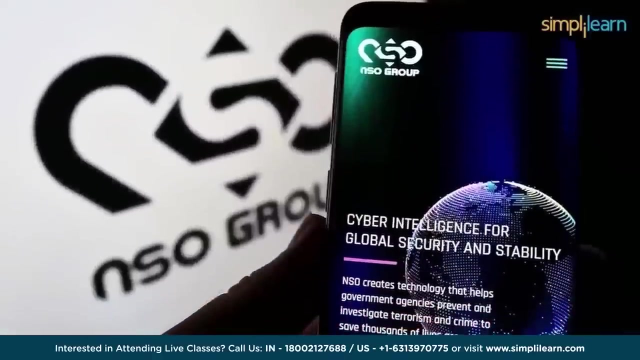 of privacy. One such spyware system is Pegasus. This is not a newly developed platform, since Pegasus has existed since as early as 2016.. A highly intricate spyware program that can track user location, read text messages, scan through mobile. 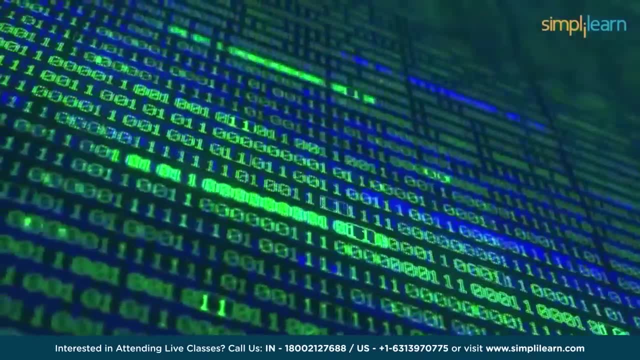 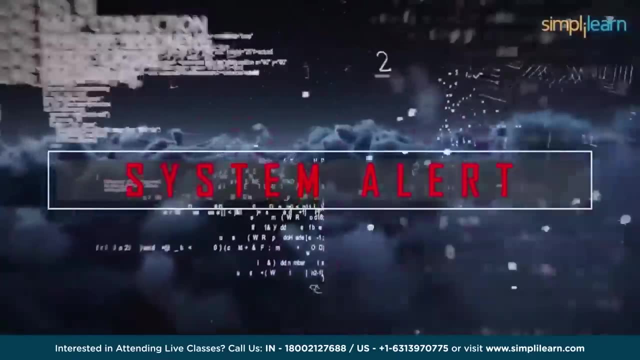 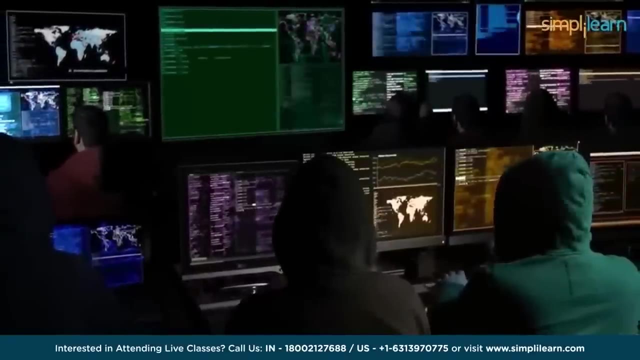 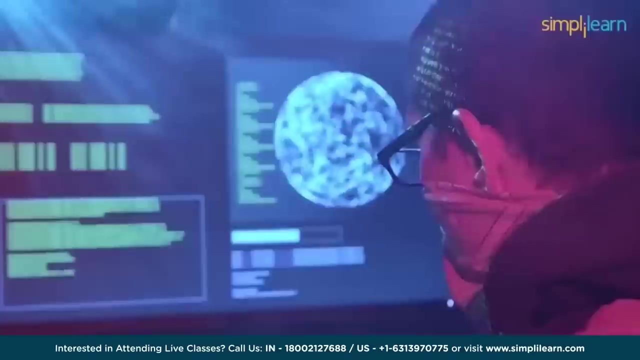 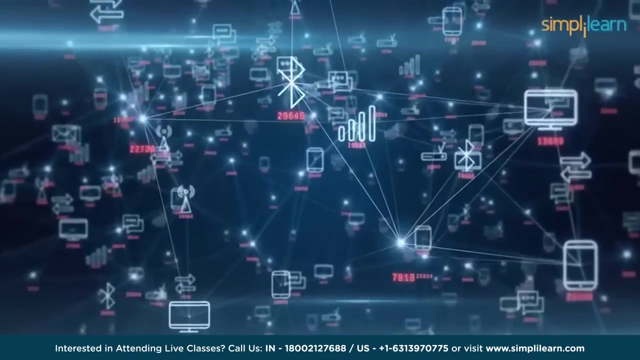 files, access and other information. With more and more encrypted communication channels coming to the forefront, Pegasus was designed to maintain control over the data transmission that can be a threat to national security. Unfortunately, the people who bought the software had no idea that Pegasus 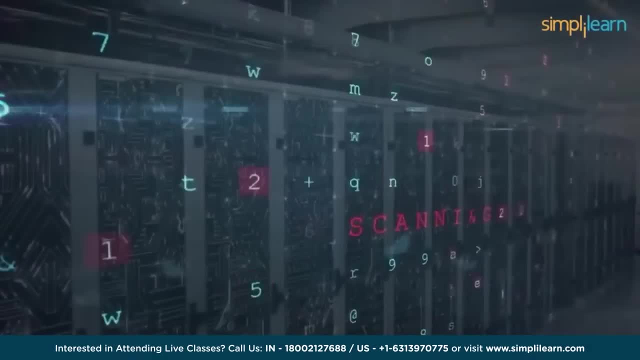 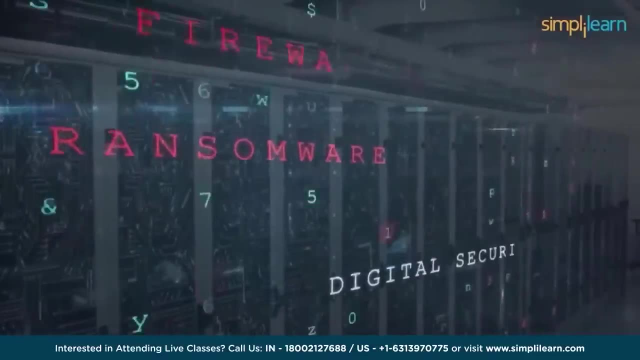 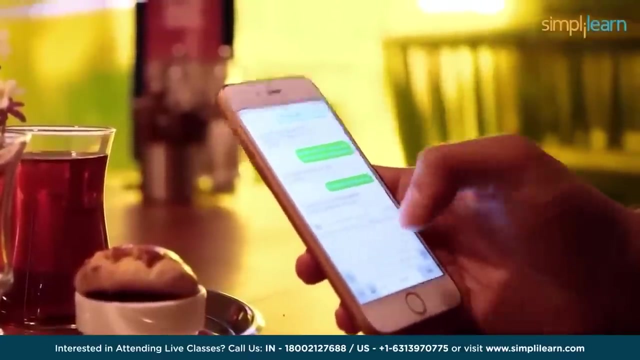 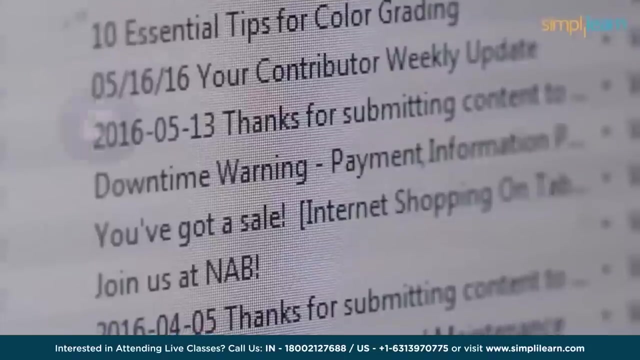 can be affected with the same spyware system to create our network information. This network keeps feeding data to the host To understand how a network can be created. let's know how a mobile device can be affected by Pegasus, The Pegasus spyware. 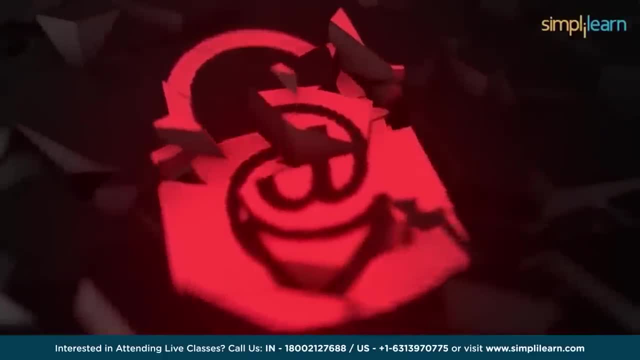 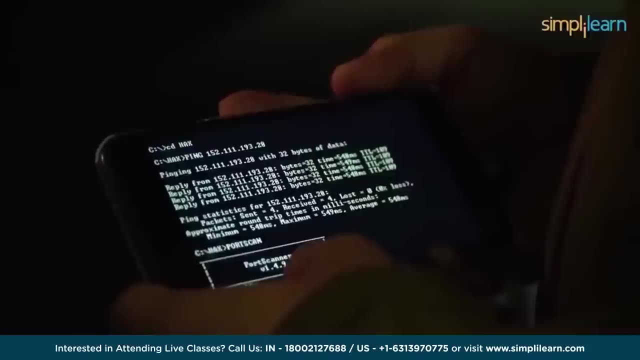 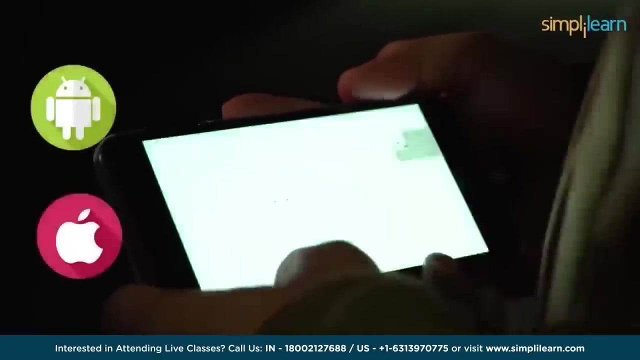 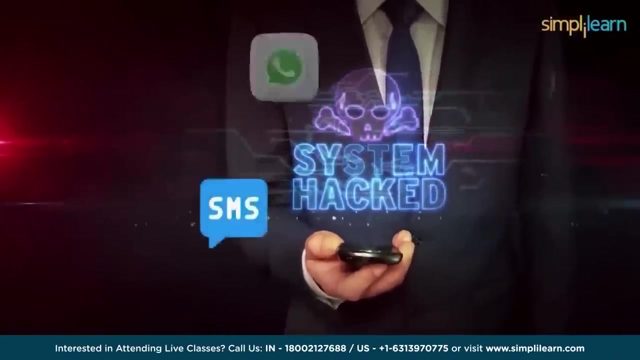 is a spam folder. Some of these messages bypass this filter and make their way into a person's inbox. They look like generic emails which are supposed to be safe. The Pegasus spyware targets such occurrences, bypassing malicious messages and links to secure. 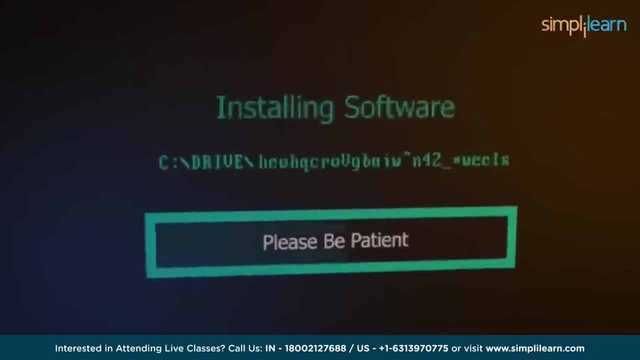 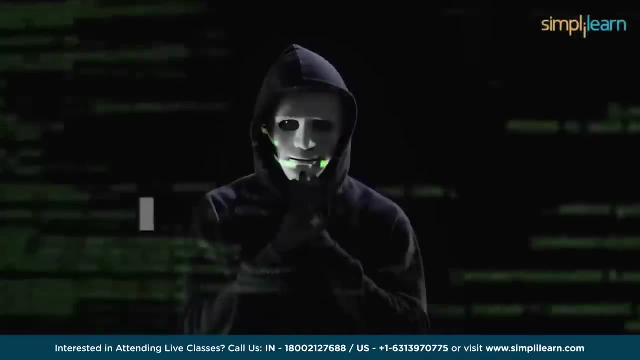 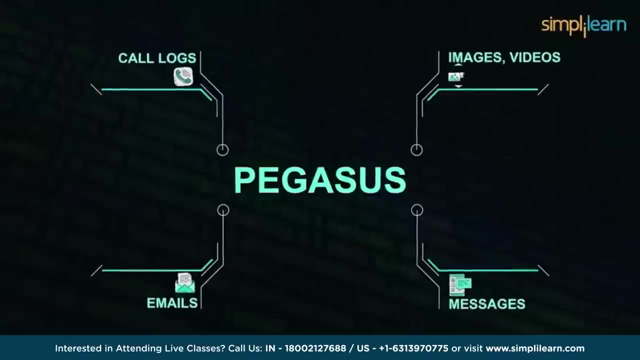 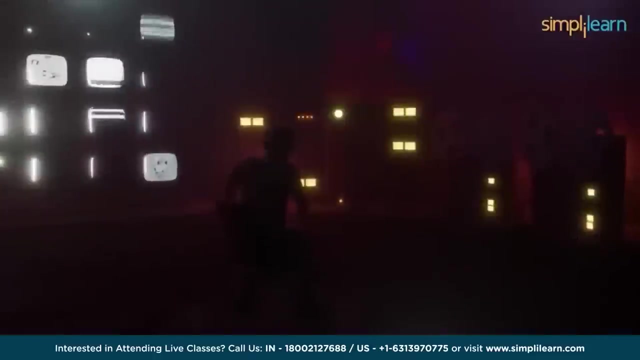 messaging apps like Signal and Threema. Once the malicious links are clicked, a spyware package is downloaded and installed on the device. After the spyware is successfully installed, the perpetrator who sent the payload to the victim can monitor everything the user does. 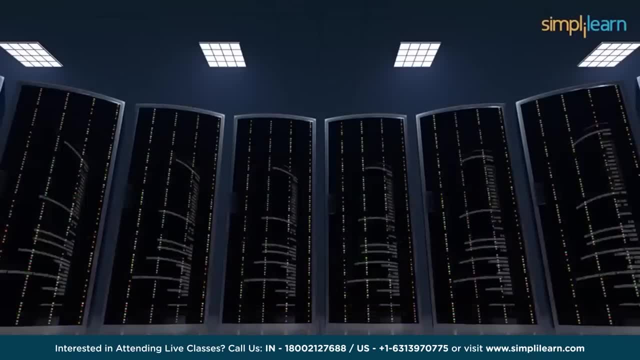 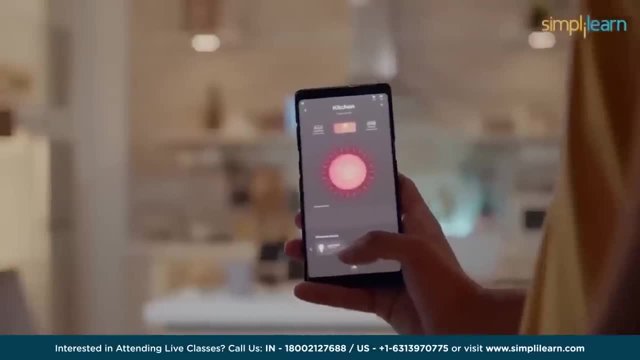 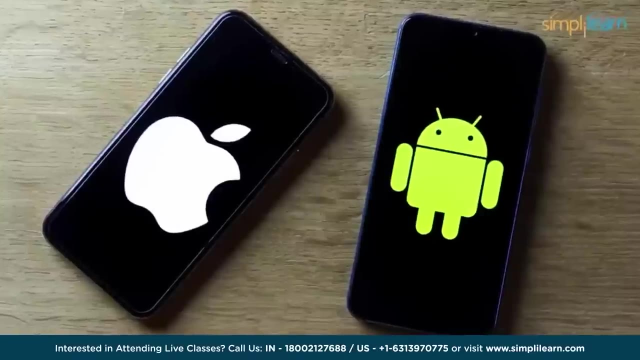 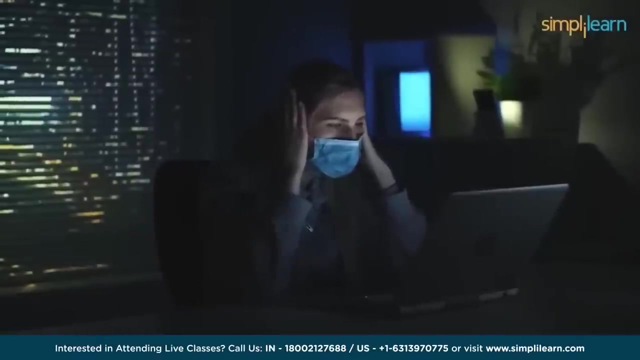 Pegasus can collect all the information that is needed to spy on the victim. Many spying organizations can monitor their activities at a granular level. This is not even surface level, since complex spyware software like Pegasus can access the root files on our mobiles. 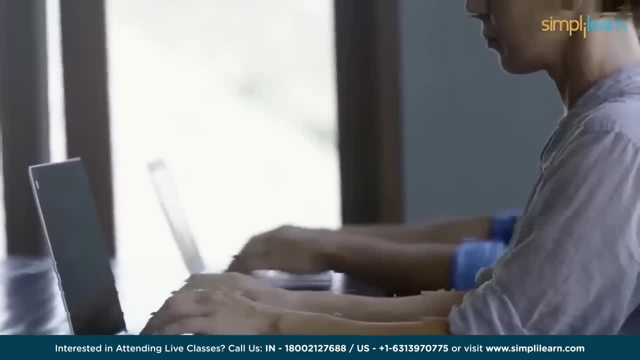 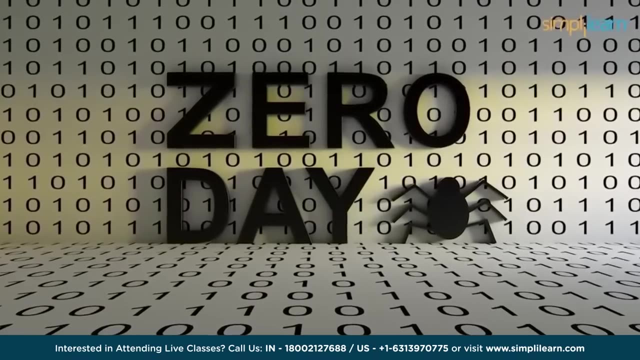 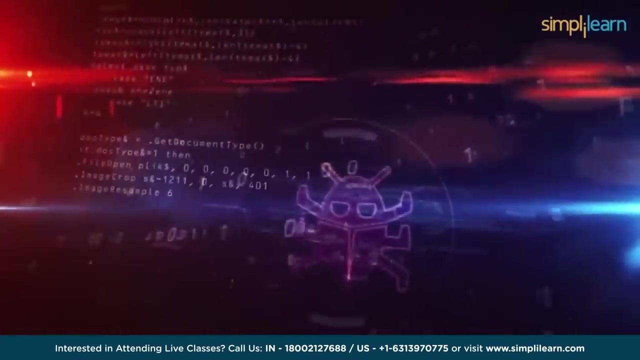 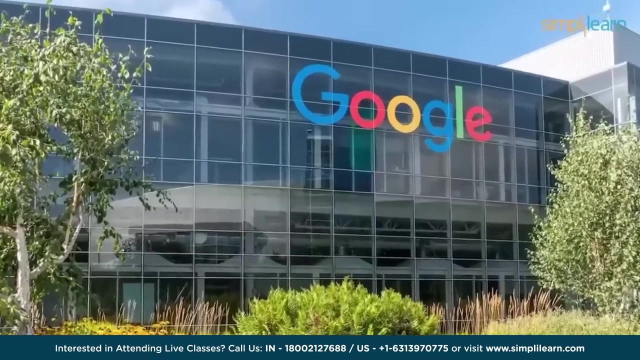 These are all valuable information. This exploitation is primarily possible due to the zero-day vulnerabilities, known as bugs, in the software development process. The zero-day bugs are the ones that have just been discovered by some independent security company or a researcher. Once they are found, 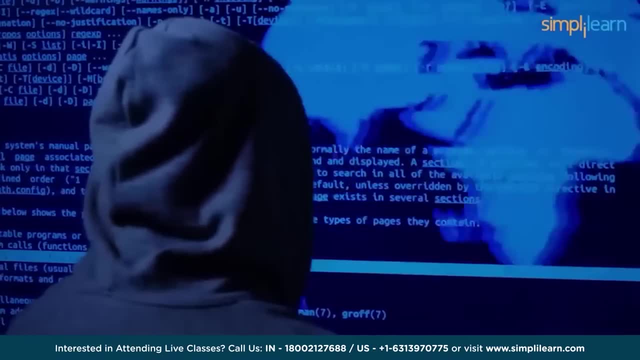 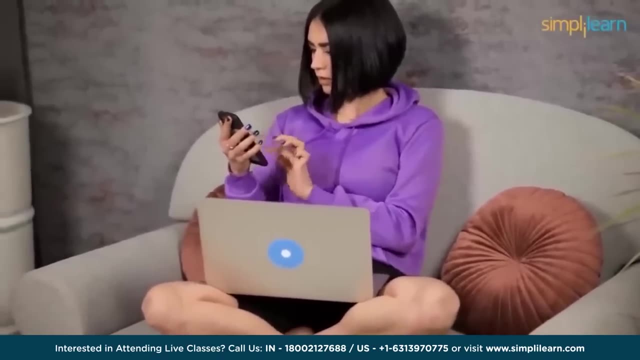 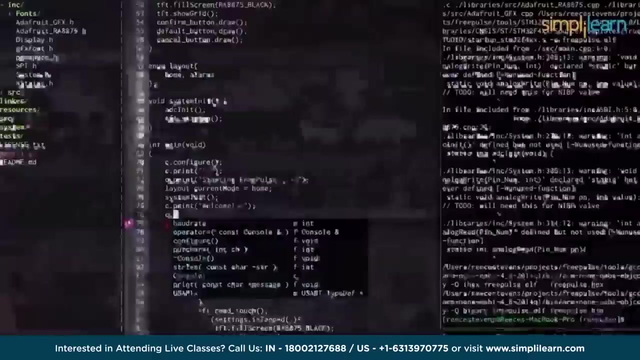 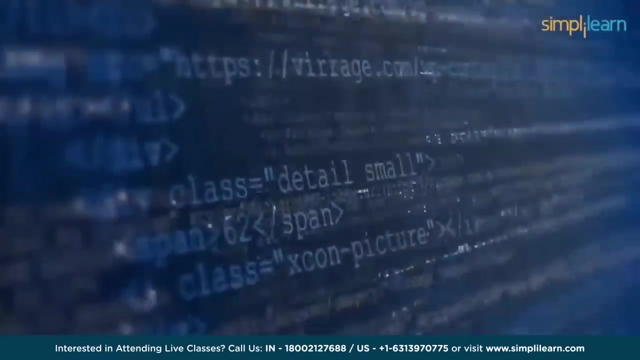 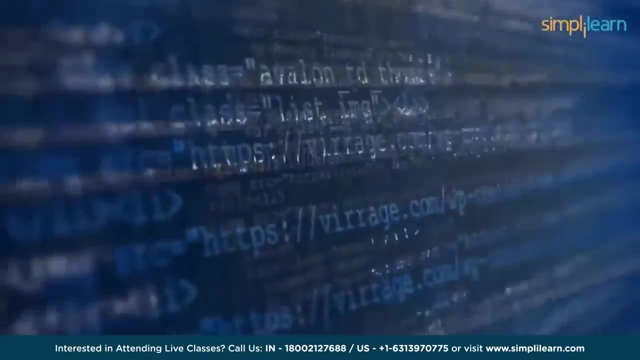 reporting to the developers is done, These bugs make their way onto the dark web, where hackers can use them to create exploits. These exploits are then sent to innocent users with a link or a message, like we sent to the central server, Once the message arrives. 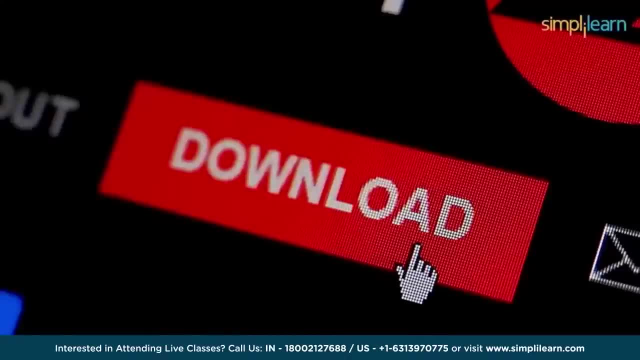 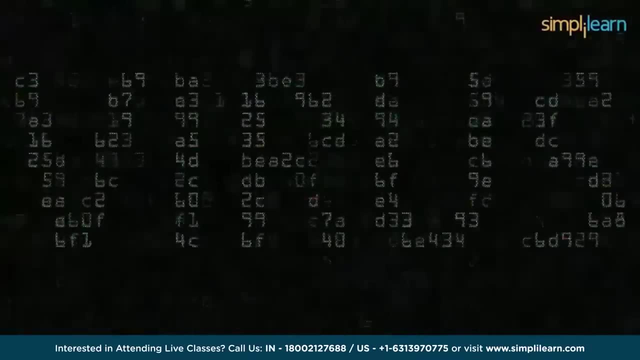 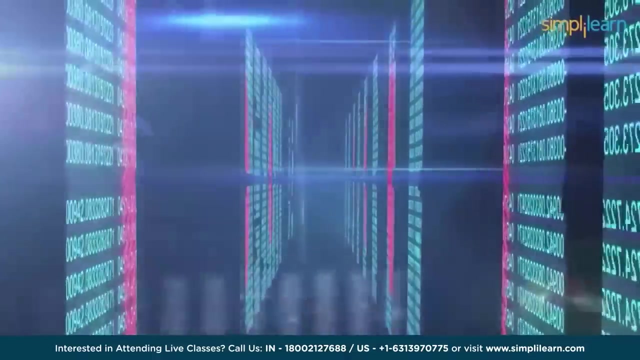 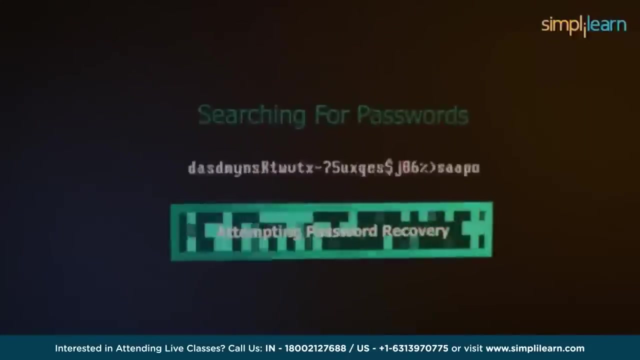 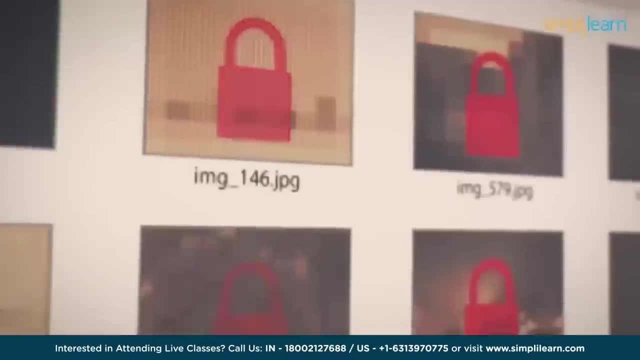 in the inbox of WhatsApp, Gmail or any other chat application, the spyware gets activated and everything can be recorded and sent back to the user. The primary issue with being affected by spyware as a victim is detection, Unlike crypto miners and trojans. 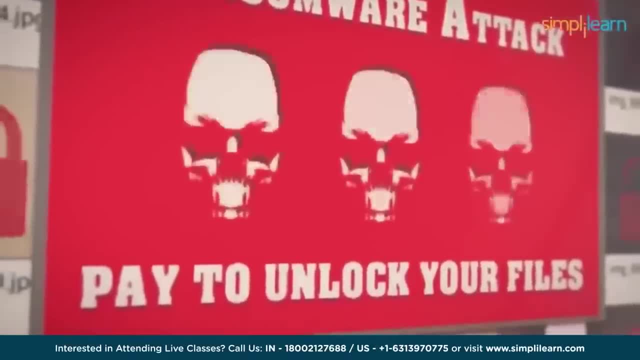 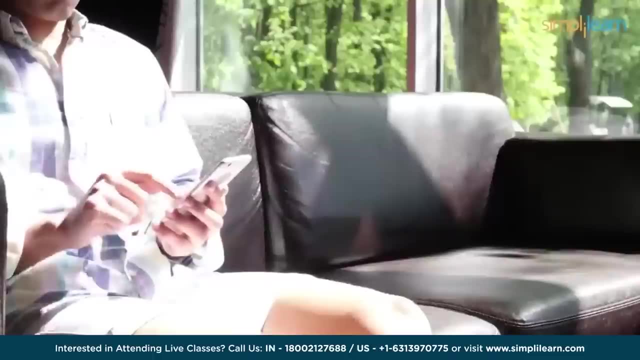 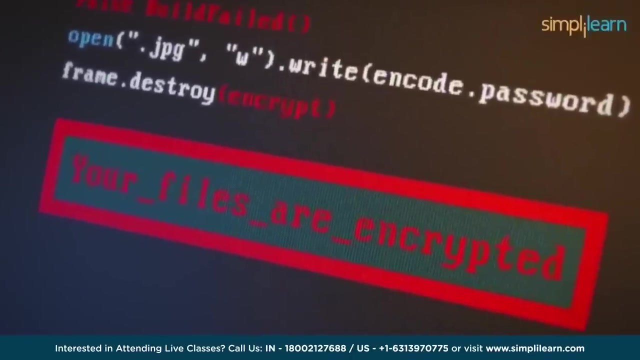 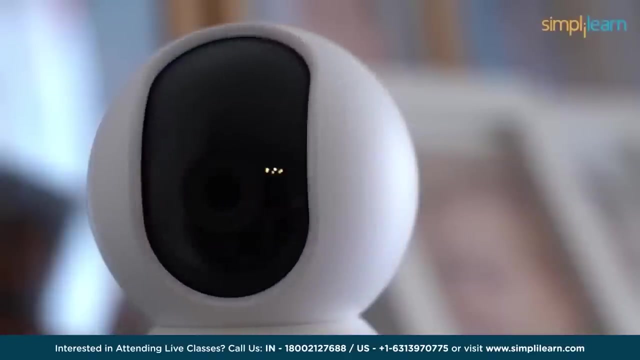 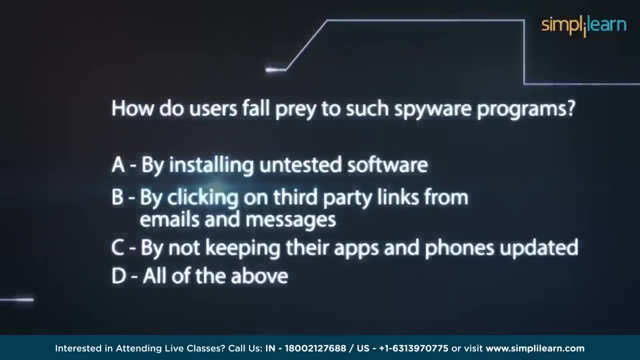 spying services usually do not demand many system resources, which makes them tough to detect after they have been detected. When left unchecked, these devices can capture voice and video from the mobile sensors while keeping the owner in the dark. Let's take a moment to check if. 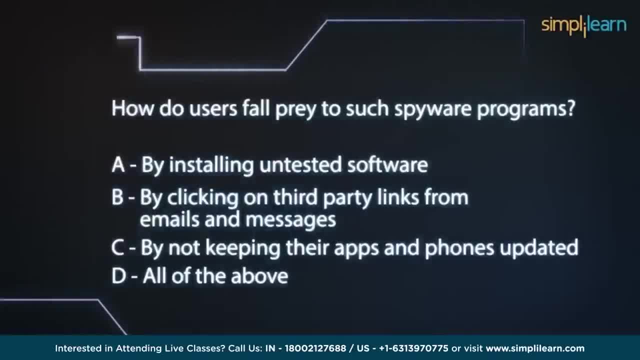 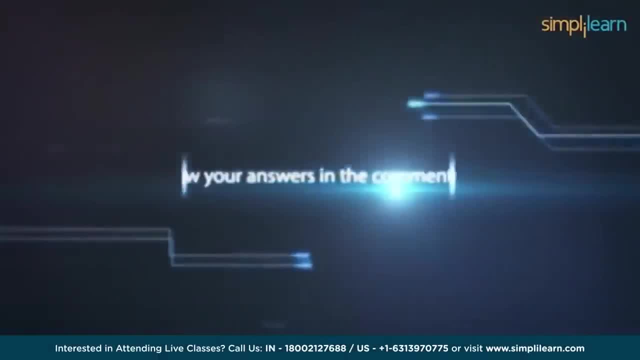 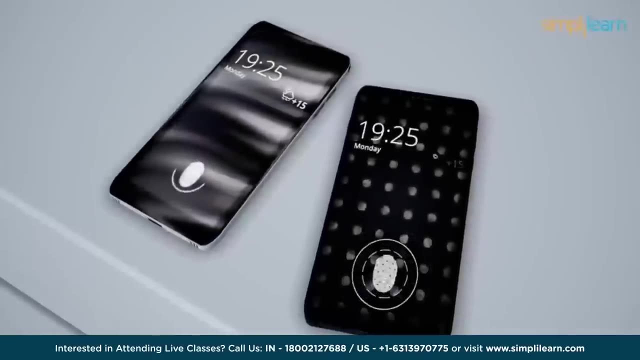 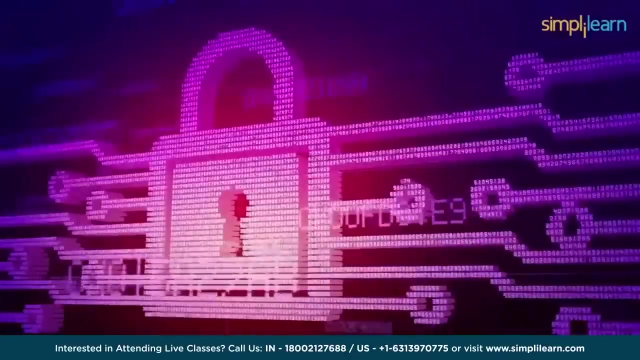 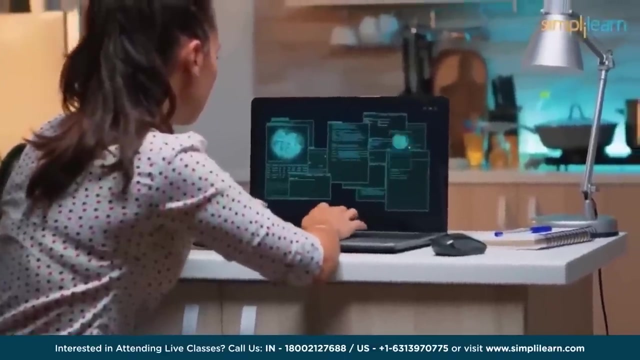 you are well aware of the causes of such attacks. How do users fall prey to such spyware programs? Please comment below and we will revise the correct answer next week. But what about the unaffected devices, the vulnerable ones? While we cannot be certain, 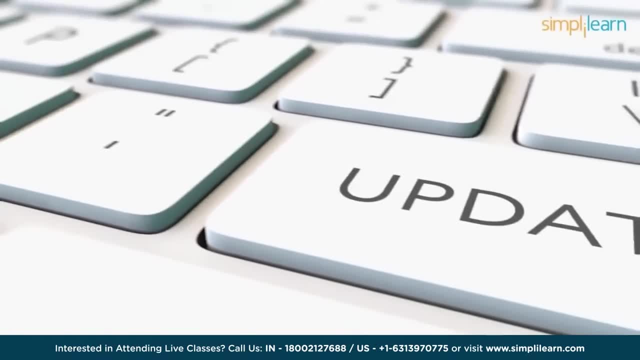 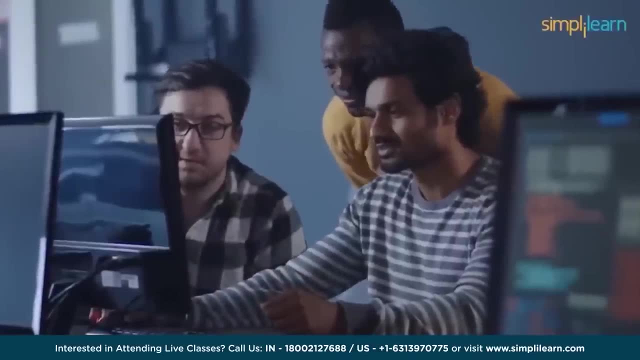 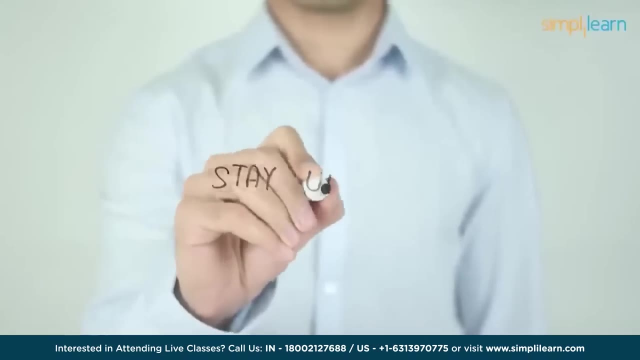 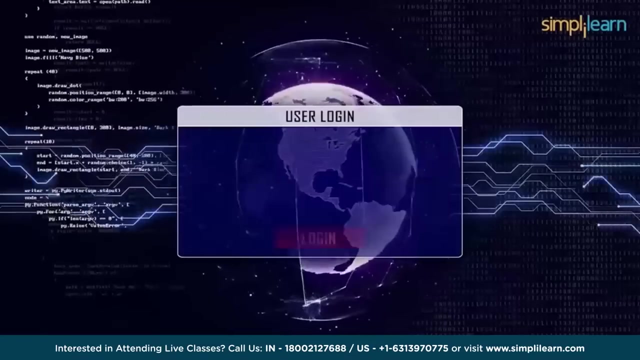 of our security. there are several security patches. The vulnerabilities that the exploit target are often discovered by developers from Google and Apple, which send the security patches quickly. This can be done for individual apps as well, so keeping them updated is of utmost importance. 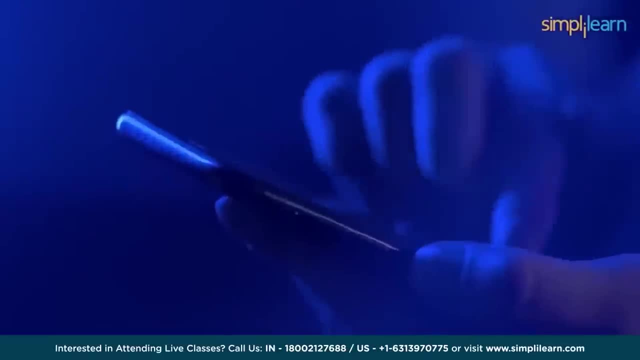 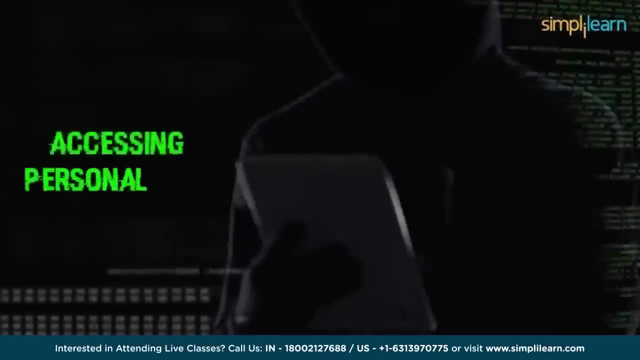 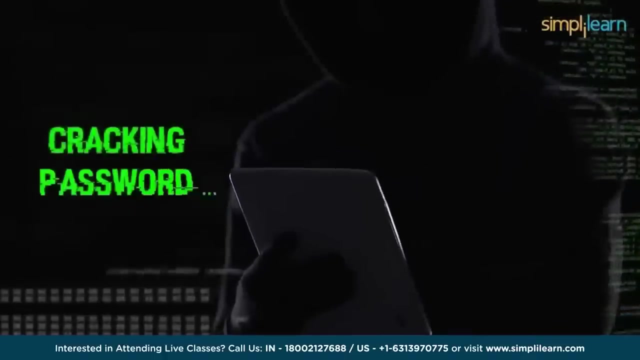 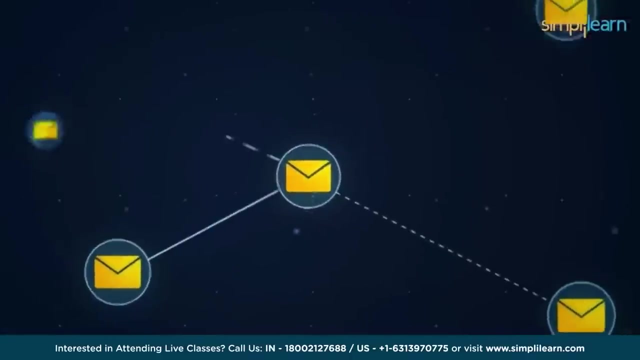 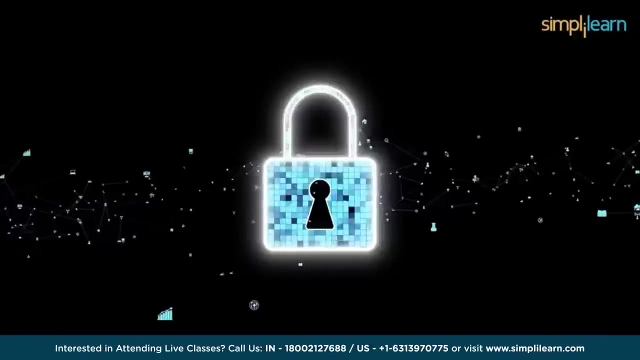 While the most secure devices are of malware, it's the trend of sideloading android applications using apk files. Downloading such apps from a third-party website have no security checks involved and are mostly responsible for adware and spyware fraud. It's: 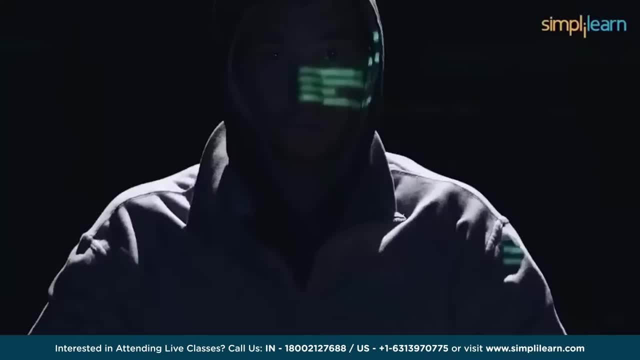 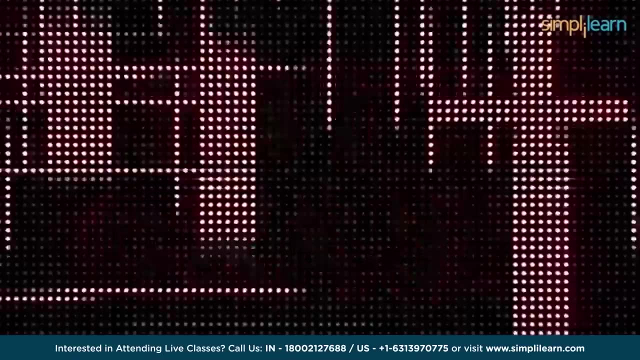 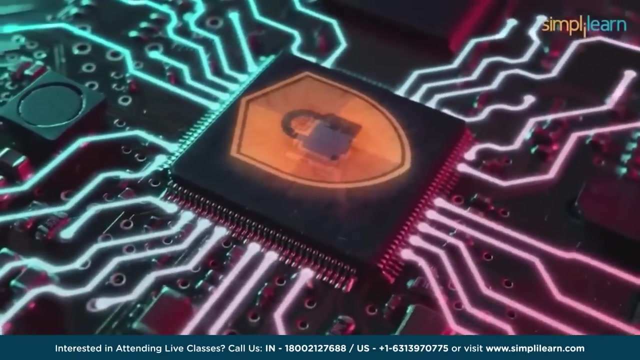 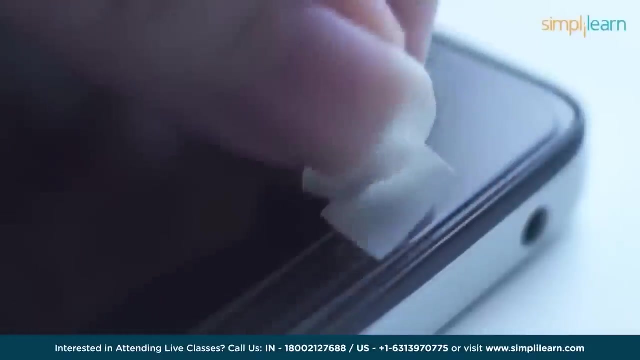 not easy to follow the trusted websites and not click on any links that redirect us to unknown domains. Spyware is a controversial segment in governance. While the ramifications are pretty extreme in theory, it severely impacts user privacy against authoritarian regimes. It's not easy to 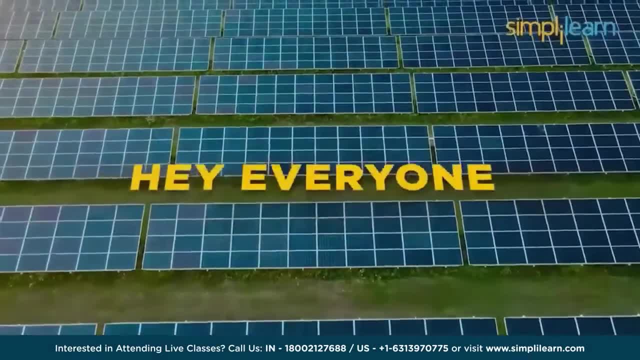 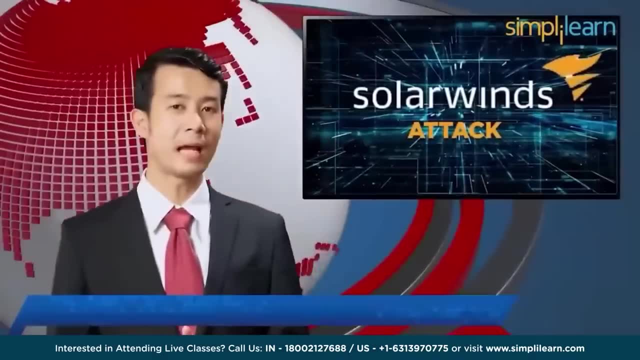 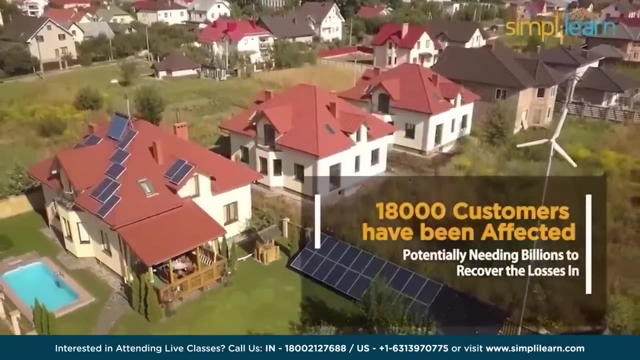 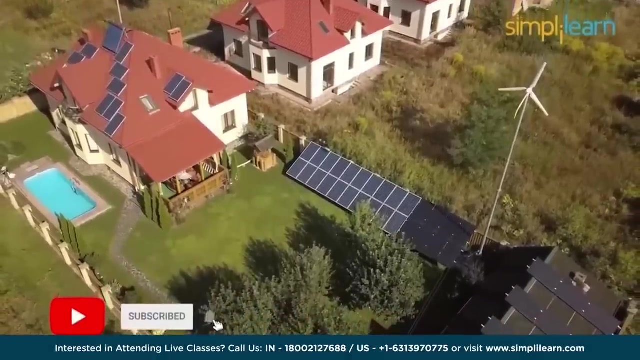 protect. It stands for everything we have to share with the outside world, both rhetorically and literally. Hey everyone. Today we look at the hack which took the world by storm and affected the entire IT community. The date is December 8,. 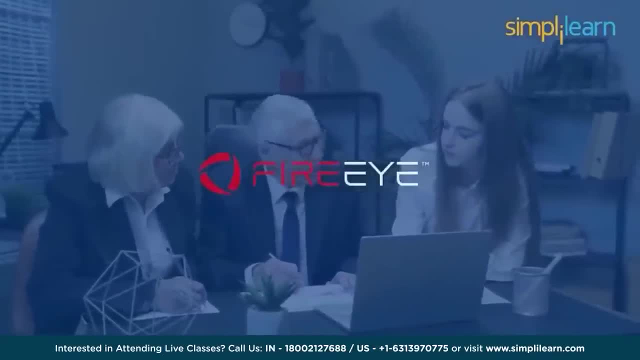 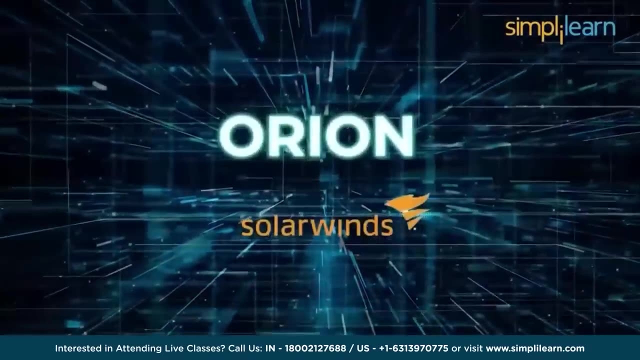 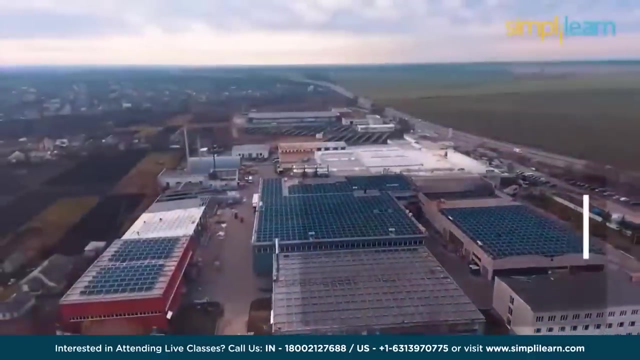 2020.. FireEye, a global leader in companies specialising in cybersecurity, released a blog post that caught the attention of the entire IT community. A software known as Orion, which was developed by SolarWinds Incorporated, had become a victim of a 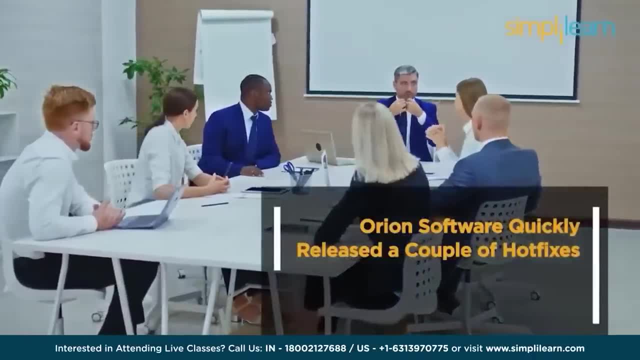 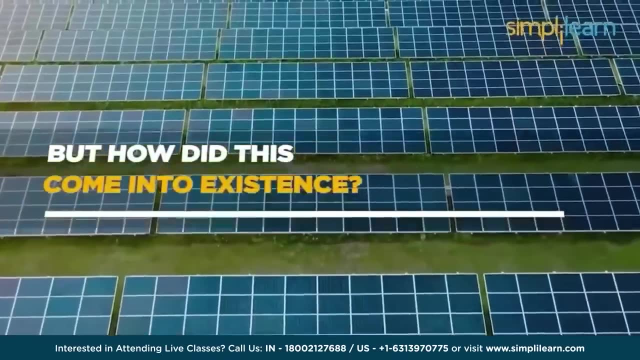 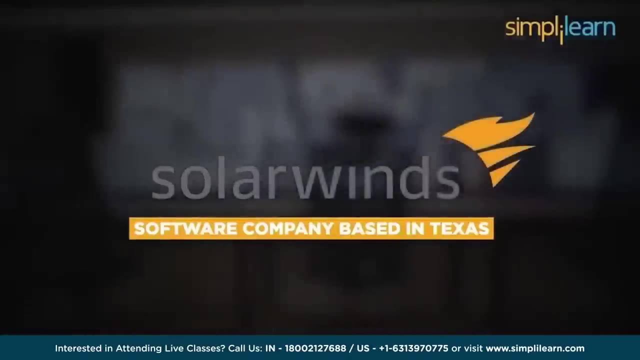 remote-access feature into a frenzy, as they quickly released a couple of hotfixes for their platform in order to mitigate this threat and prevent further damage. But how did this come into existence? We first need to understand the platform which was responsible for this. 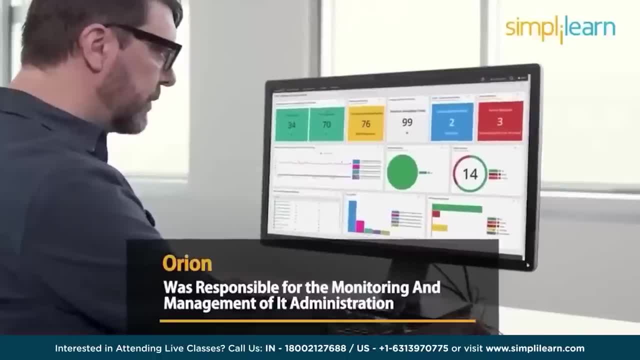 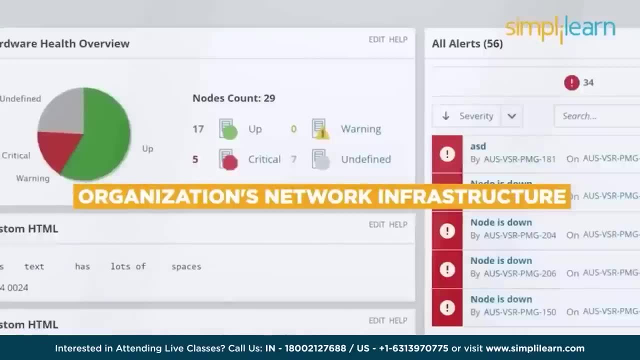 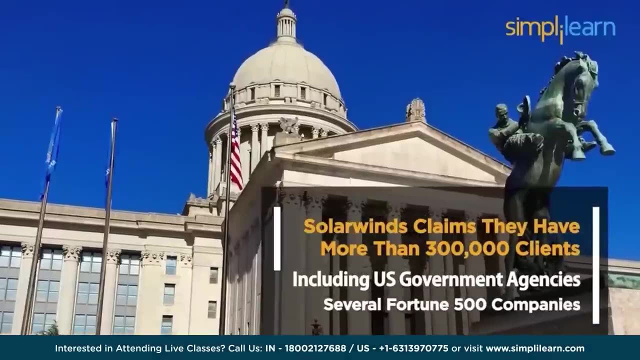 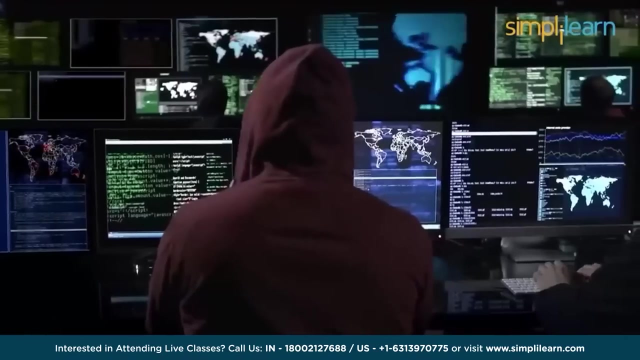 breach. SolarWinds, a software company based in Texas, was the first company in the United States to launch a software called SolarWinds. SolarWinds claims they have more than 300,000 clients, including US government agencies and several. 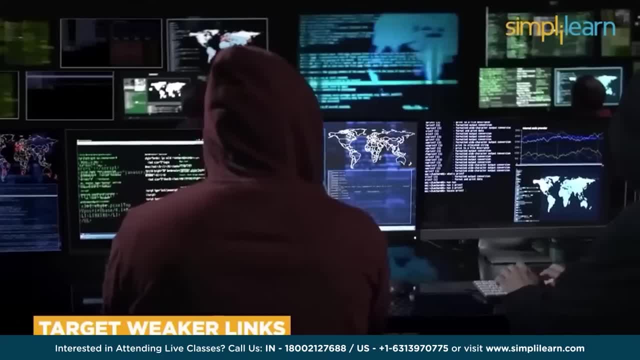 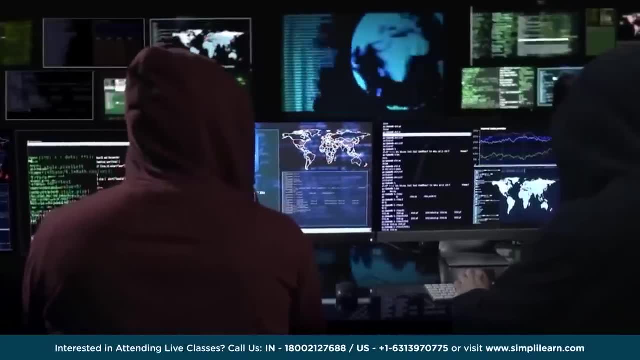 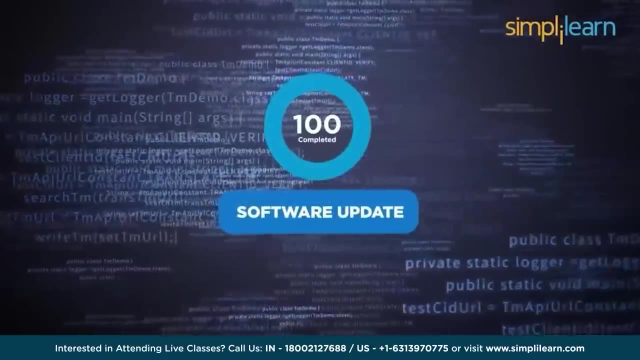 Fortune 500 companies. This entire chain can be classified as a supply chain attack. In this variant of cybercrime, there was no protection over it. In this case, the Orion platform was the primary target. The culprit, however, was software updates. 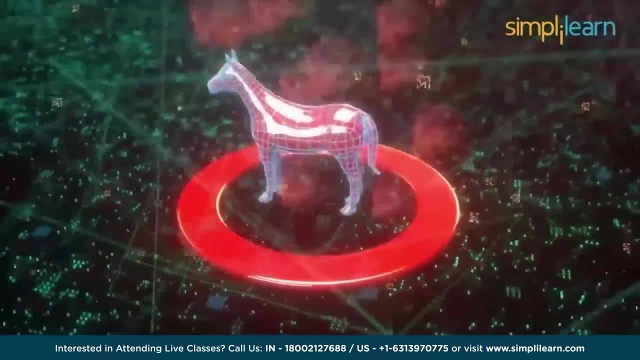 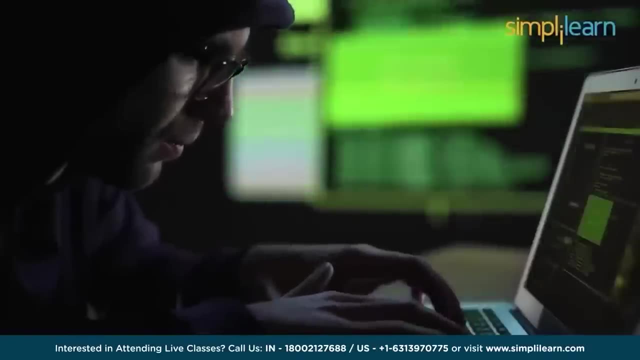 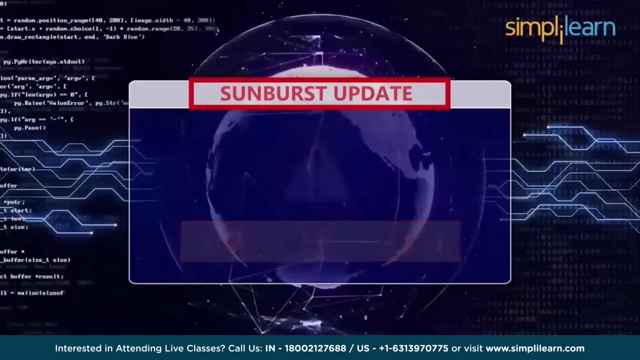 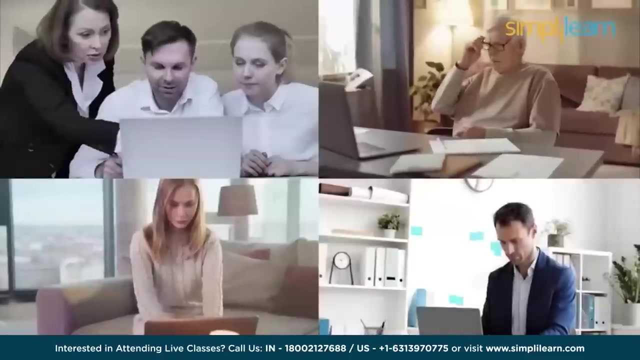 The update server for SolarWinds Orion had a malicious version attached, with malware, or a trojan to be precise. This was made possible since the code attached to a potential update nicknamed the Sunburst update. This update gave hackers backdoor access to any client. 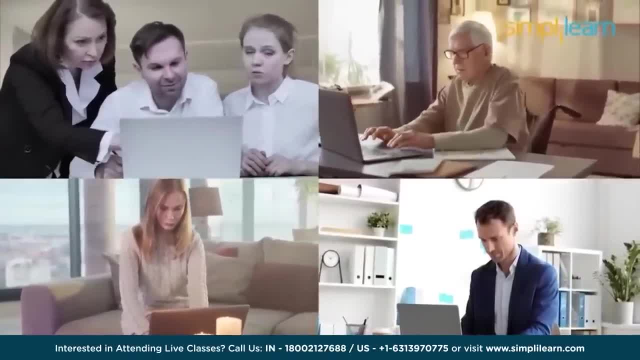 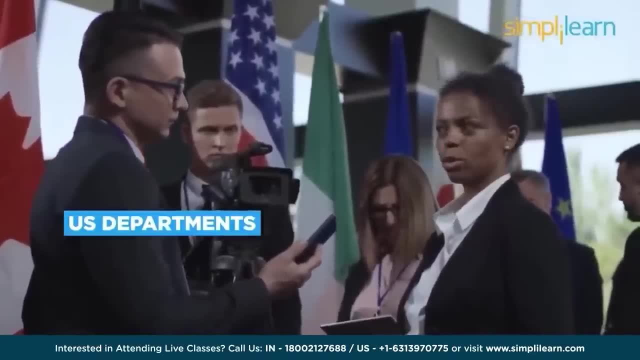 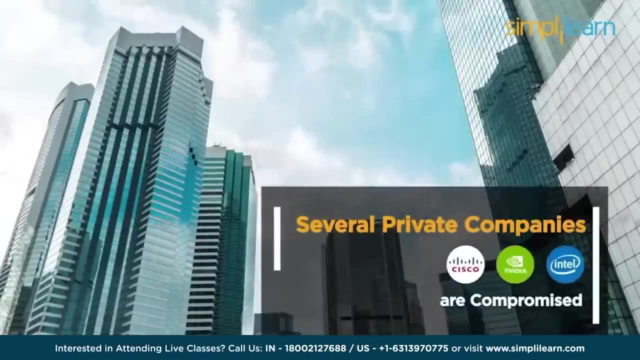 that uses the correct version. On its release, many clients believed the update to be legitimate, since it came from the right source, and they had no reason to believe otherwise. According to a list published by the cyber security firm TruSec, most of the 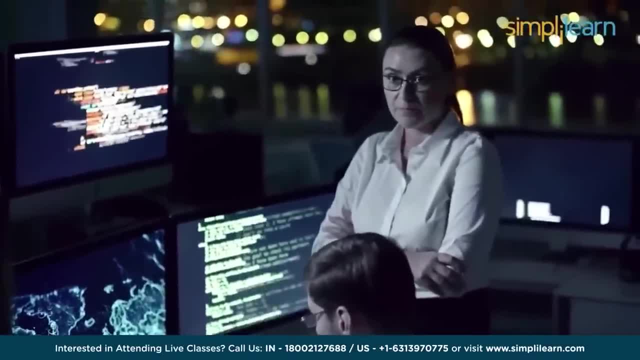 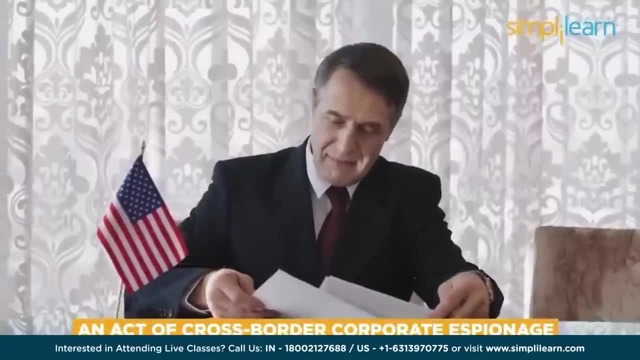 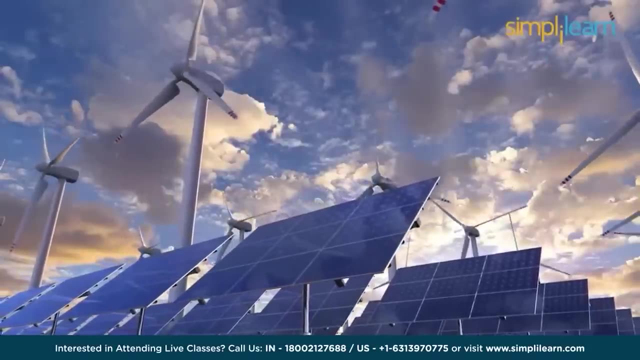 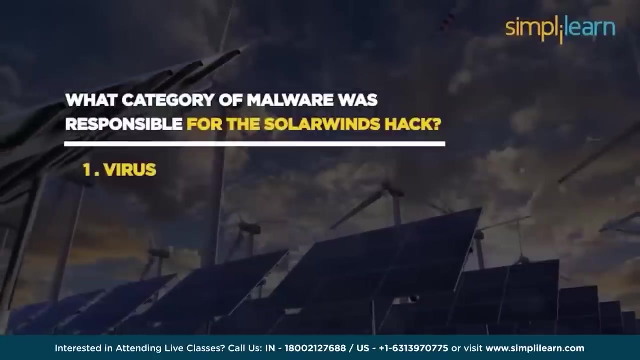 companies had issued quick updates to fix the vulnerabilities introduced by the software. While the actual perpetrators have never been found, it is believed that this was an act of cross-border corporate espionage conducted by state-sponsored hackers either from Russia or China. Is it a virus? 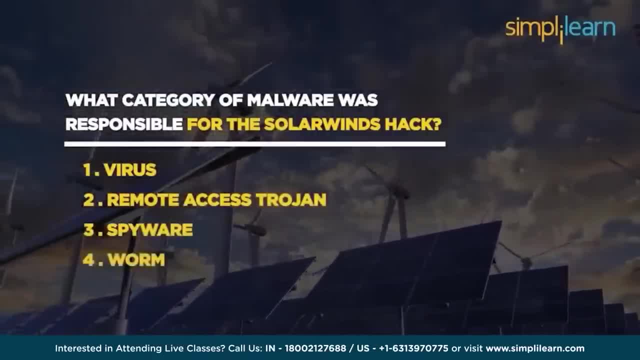 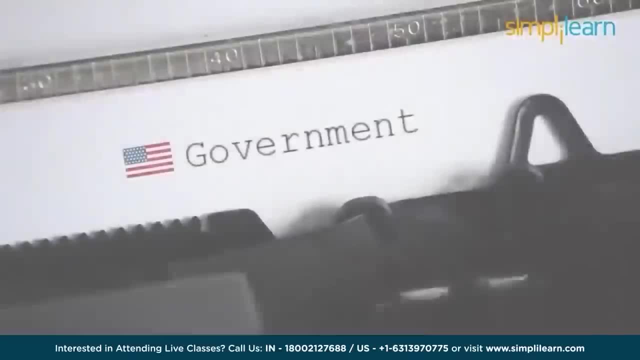 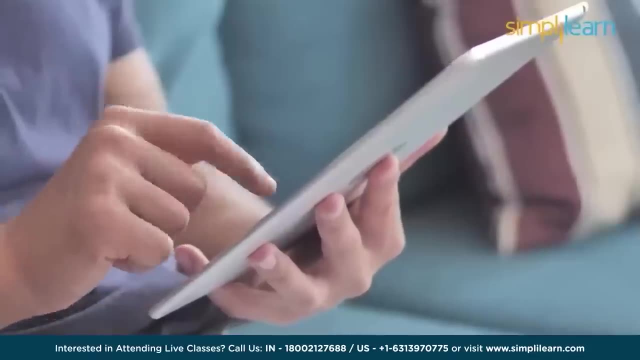 a remote-access trojan, a spyware or a worm? Let us know your answers in the comments section right away and we will reveal the correct answer in a week, Coming to possible reparations. the Biden government has launched a full investigation on the. 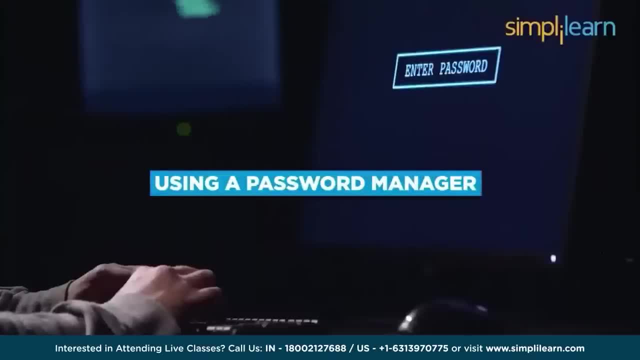 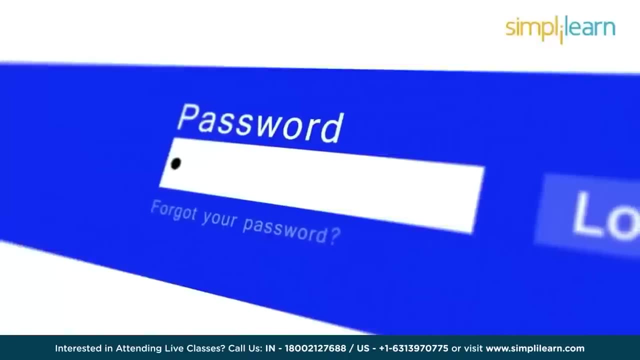 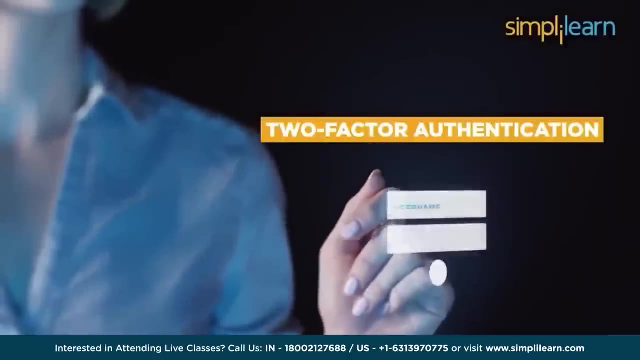 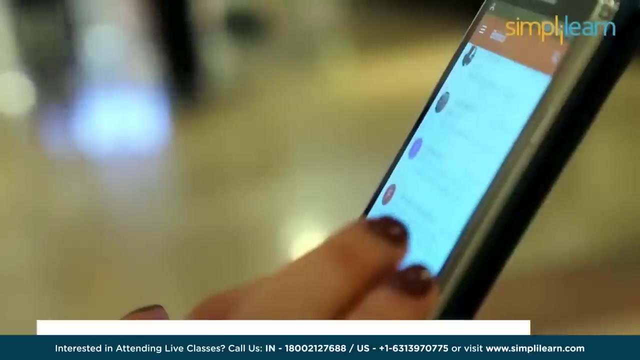 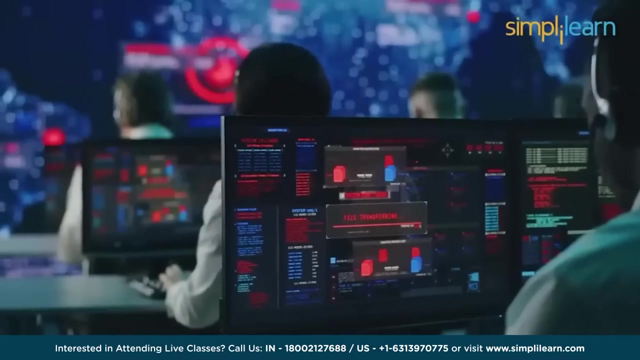 effects and repercussions of this breach. There are a couple of reasons for this breach. The first reason is that the government does not want to use passwords for different accounts. They must also use different passwords for different accounts, thereby reducing the chances of a single. 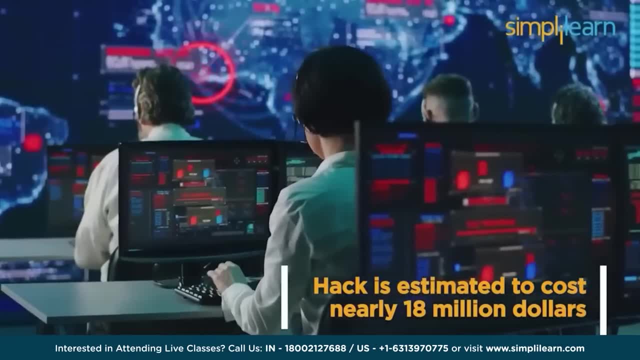 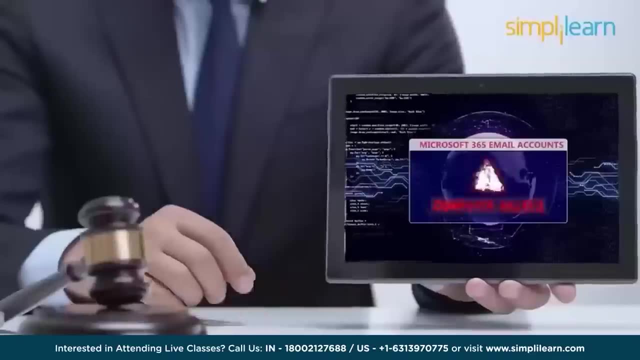 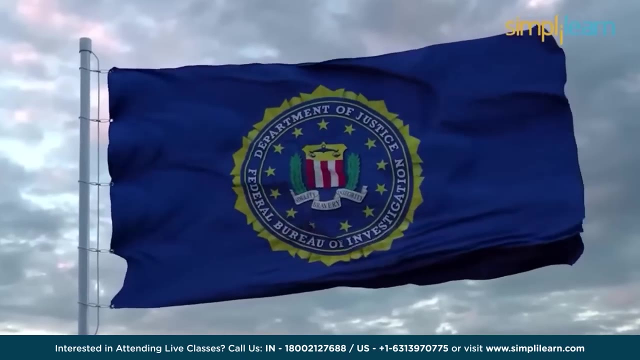 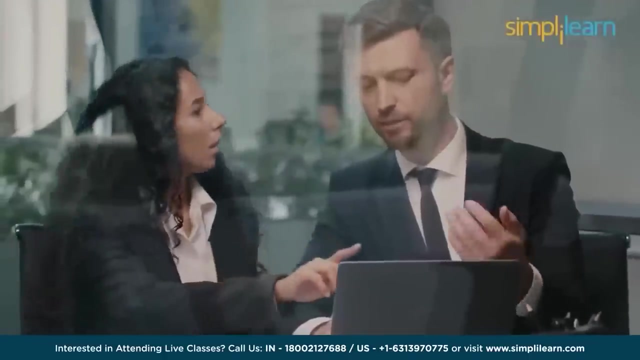 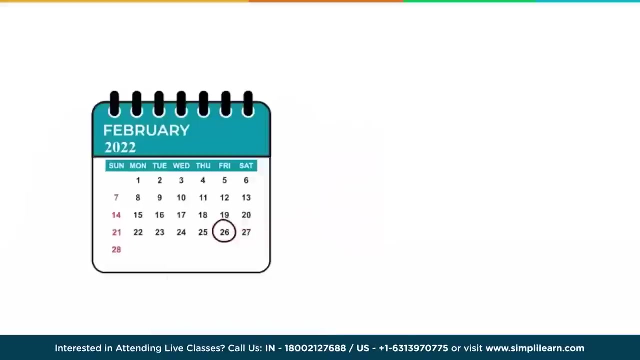 point of breach happening. The second reason is that the government does not want to use passwords for different accounts. The second reason is that the government does not want to use passwords for different accounts. The third reason is that the government does not want to use 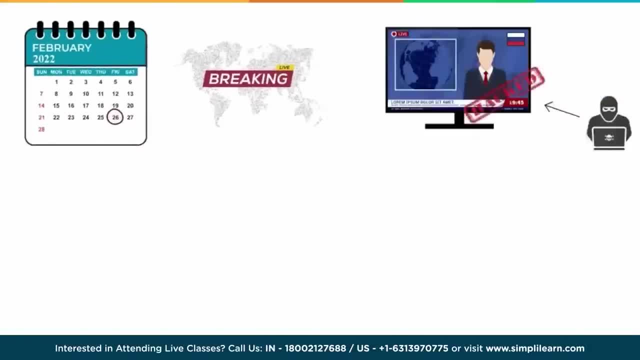 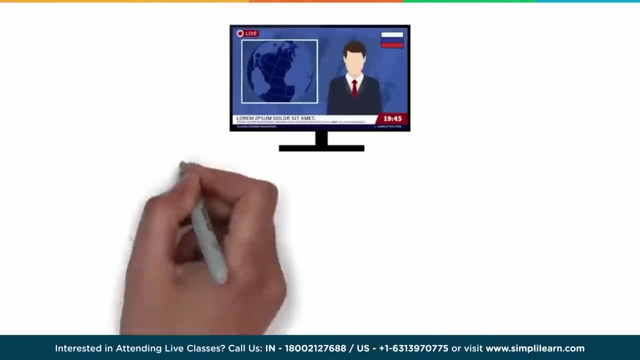 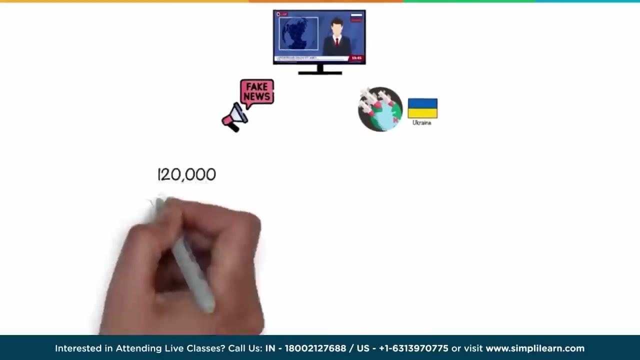 passwords for different accounts. The fourth reason is that the government does not want to use passwords for different accounts. The third reason is that the government does not troops' personal information and the Russian Central Bank stealing 35,000 files. This served as a clear indicator of how cyber war can change the momentum in battle, something which people 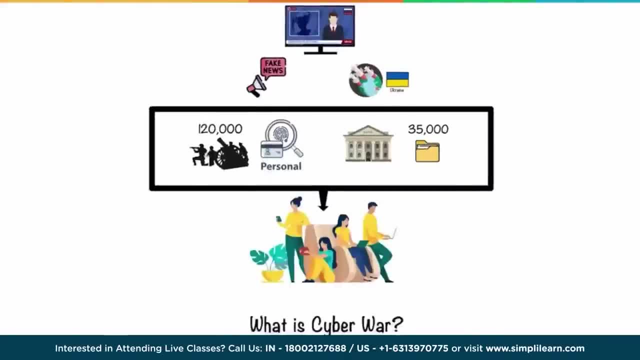 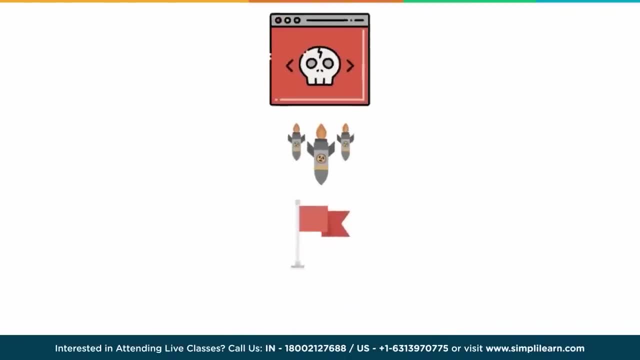 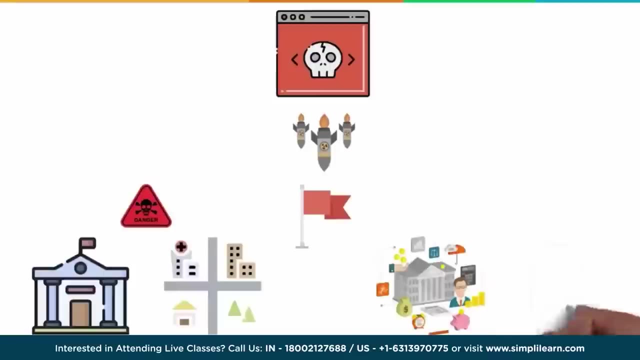 had never seen so closely. So what is cyber war? A digital assault or series of strikes or hacks against a country is sometimes referred to as a cyber war. It has the ability to cause havoc on government and civilian infrastructure, as well as disrupt essential systems, causing state harm. 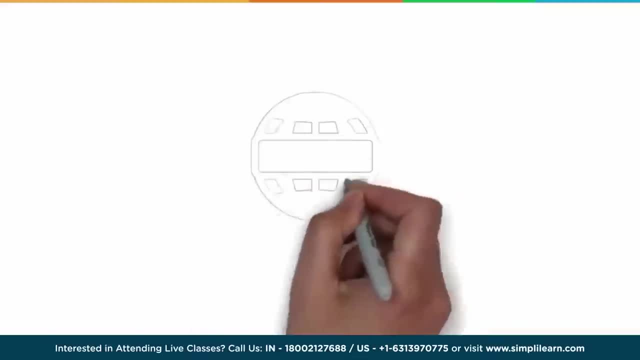 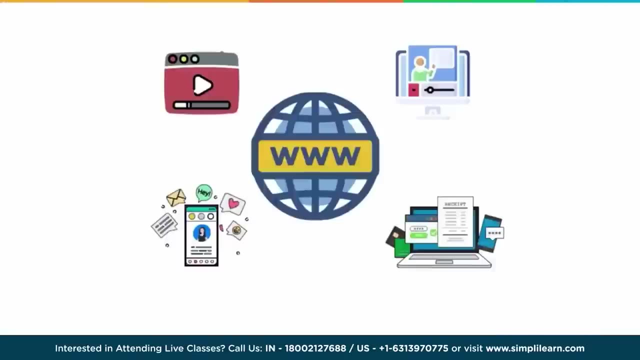 and even death. In this day and age, the internet plays a bigger role than just watching videos and learning content. It's where you have your personal data and carry financial transactions. So, rather than resorting to physical violence, cyber wars become the new means to cause havoc. 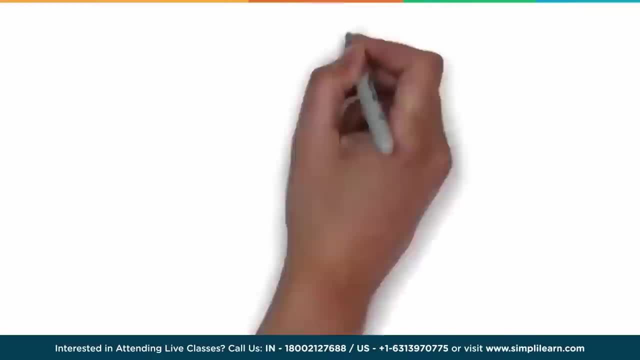 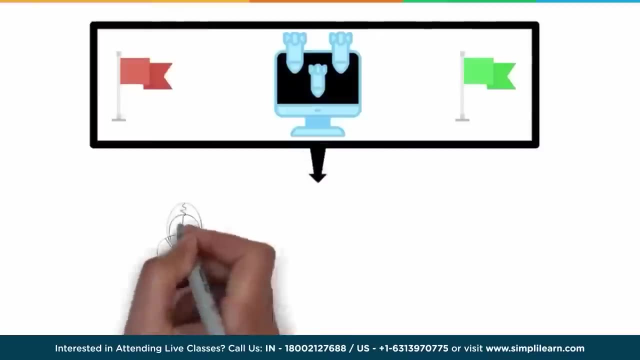 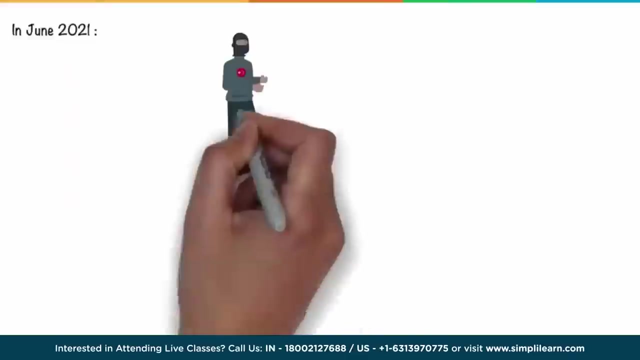 considering the vulnerability of the data passing through the internet. In most circumstances, cyber warfare involves a nation-state attacking another. In certain cases, the assaults are carried out by terrorist organizations or non-state actors pursuing a hostile nation's aim. In June 2021, Chinese hackers targeted organizations like 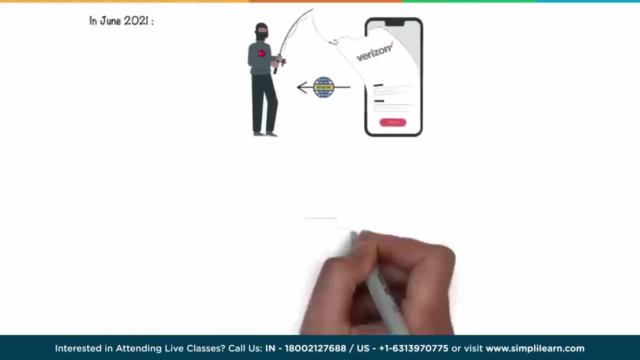 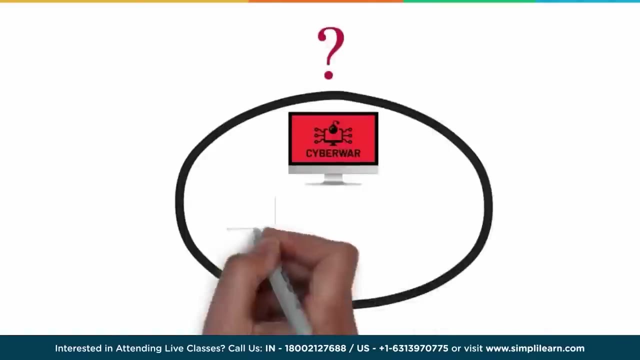 Verizon to secure remote access to their networks. Stuxnet was a computer worm designed to attack Iran's nuclear facilities, but evolved and expanded to many other industrial and energy-producing sites in 2010.. Since the definition of cyber war is so vague, applying rules and sanctions based 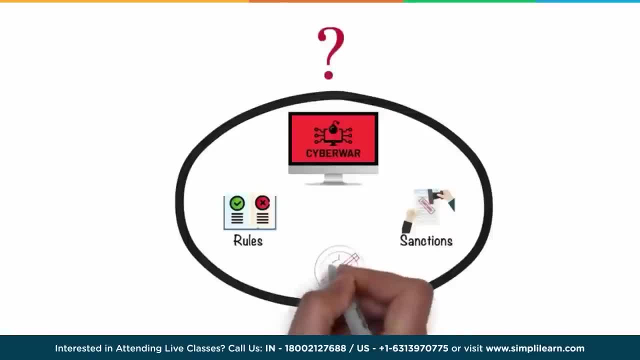 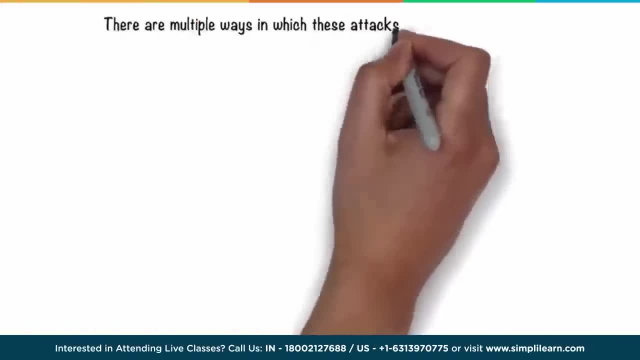 on cyber warfare is not a good idea. So why is cyber warfare so vague? It's even tougher Making the field of cyber warfare a lawless land not bound by any rules or policies. There are multiple ways in which these attacks can be carried out. A major category. 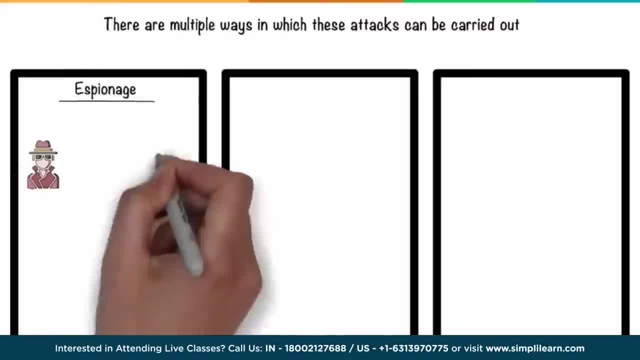 of cyber attack is espionage. Espionage entails monitoring other countries to steal critical secrets. This might include compromising vulnerable computer systems with botnets or spear phishing attempts before extracting sensitive data in cyber warfare. The next weapon in cyber war is cyber attack. The next weapon in cyber warfare is cyber attack. The next weapon in cyber 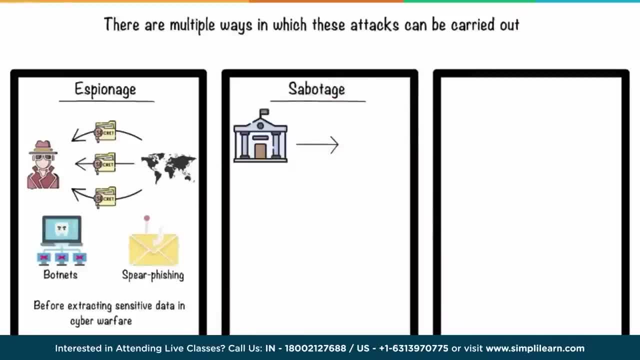 war is sabotage. Government agencies must identify sensitive data and its dangers if it is exploited. Insider threats, such as disgruntled or irresponsible personnel or government staff with ties to the attacking country, can be used by hostile countries or terrorists to steal or destroy information By overwhelming a website with bogus requests and forcing it to handle them. 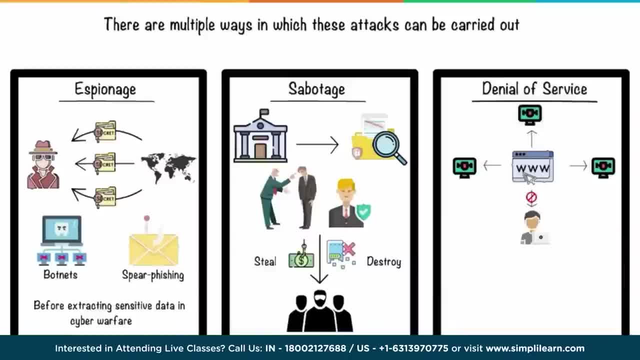 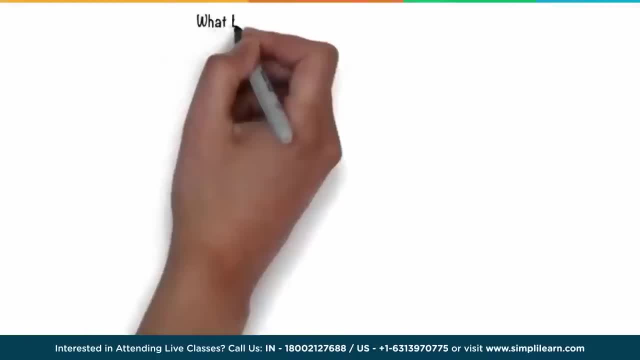 denial-of-service attacks prohibit real users from accessing it. Attacking parties may use this form of assault to prevent the attack from happening. The government agencies must identify sensitive data to disrupt key operations and systems and prevent citizens, military and security officials and research organizations from accessing sensitive websites. But what benefits does cyber war offer in? 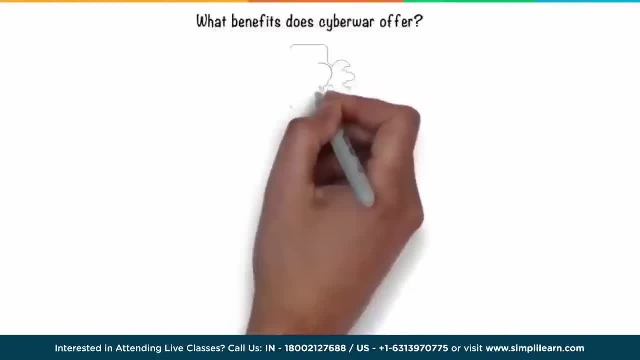 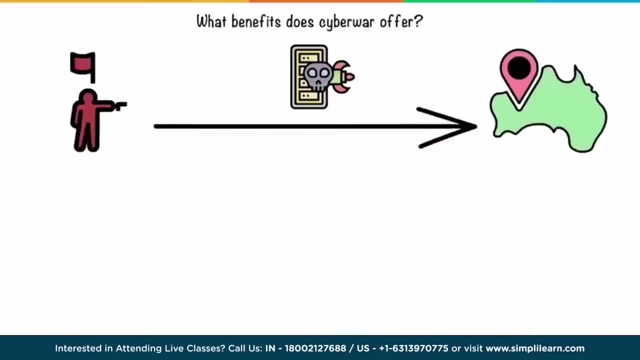 contrast to traditional physical warfare, The most important advantage is the ability to conduct attacks from anywhere global without having to travel thousands of miles. As long as the attacker and target are connected to the internet, organizing and launching cyber wars is relatively less tedious than addressing cyber warfare. 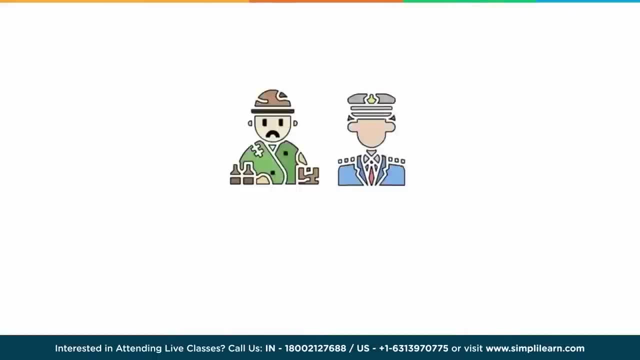 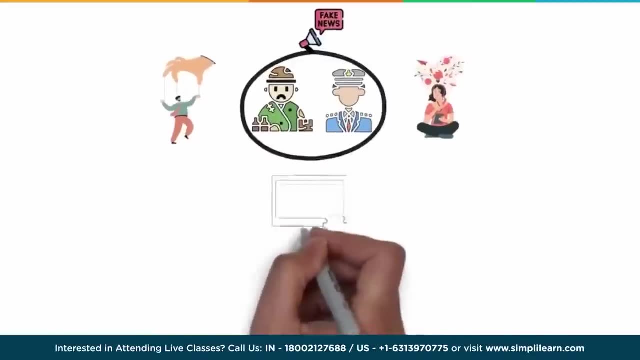 than physical warfare. People living in or battling for a country are subjected to propaganda attacks in an attempt to manipulate their emotions and thoughts. Digital infrastructure is highly crucial in today's modern world, Starting from communication channels to secure storage servers. crippling a country's footprint and control on the internet. 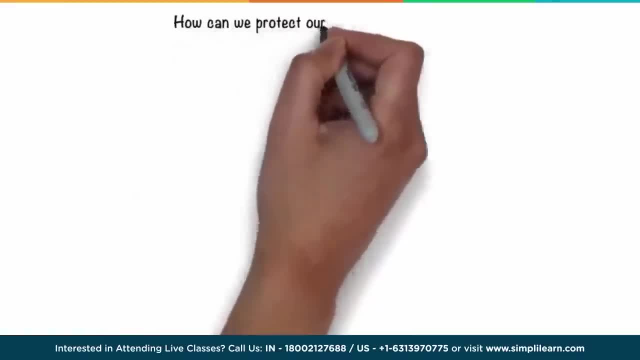 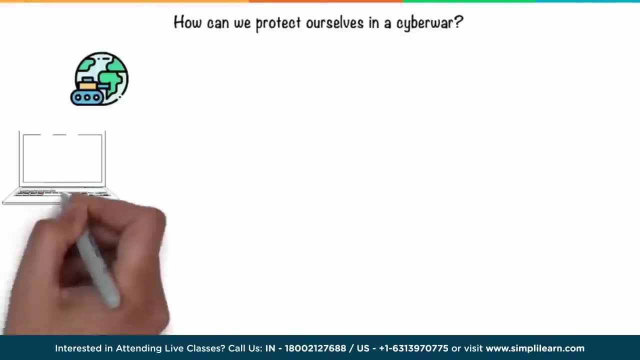 is very damaging, But what are some of the ways we, as citizens, protect ourselves in the case of a cyber war? In the unfortunate event that your country is involved in warfare, be sure to fact-check every piece of information and follow only trusted sources in that frame of time. 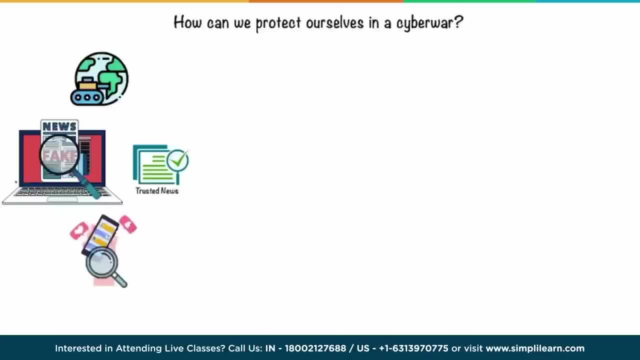 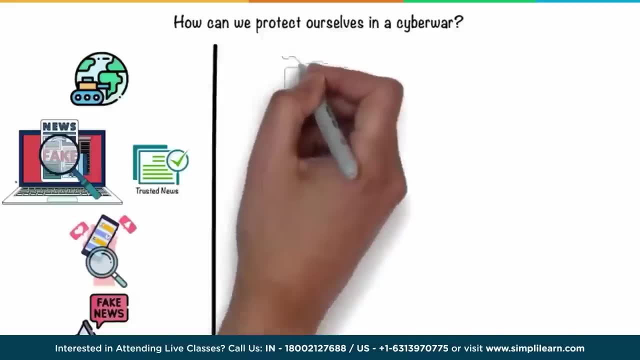 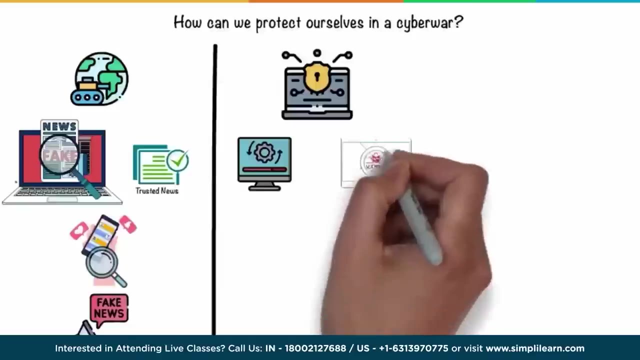 Even conversations online should be limited to a need-to-know basis, considering propaganda campaigns have the power to influence the tide of war drastically. It is highly crucial to follow basic security guidelines to secure our devices, like regularly updating our operating systems, occasionally running full system antivirus scans, et cetera. 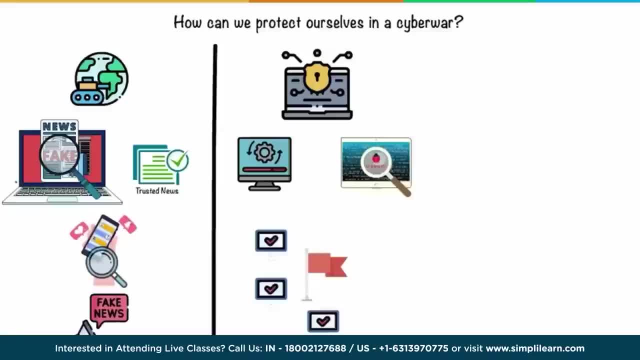 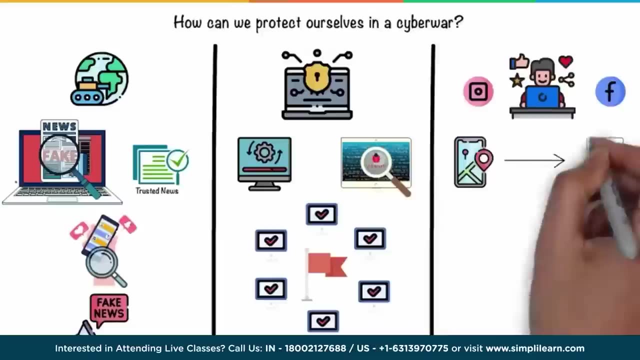 If your country or organization is being attacked. having devices segregated in a network goes a long way in bolstering security. Try to avoid sharing a lot of personal data online In this era of Instagram and Facebook. divulging private information can be detrimental to keeping a secure firewall for your data. 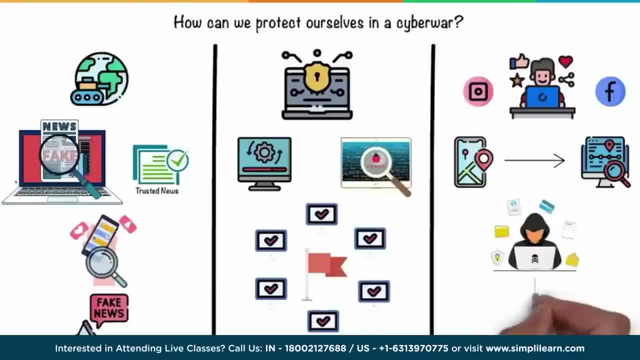 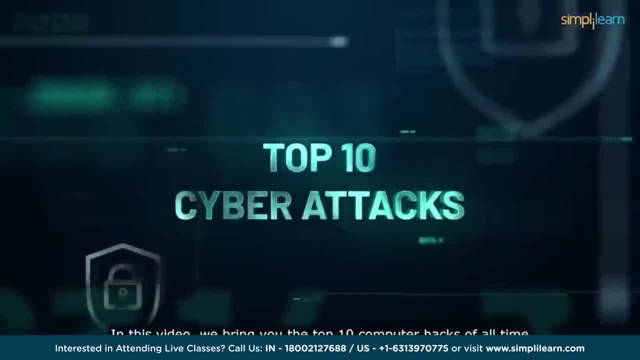 The more information an attacker has access to, the higher his chances of being able to devise a plan to infiltrate defenses. In this video we bring you the top 10 computer hacks you can do to keep your data safe. But before we begin, 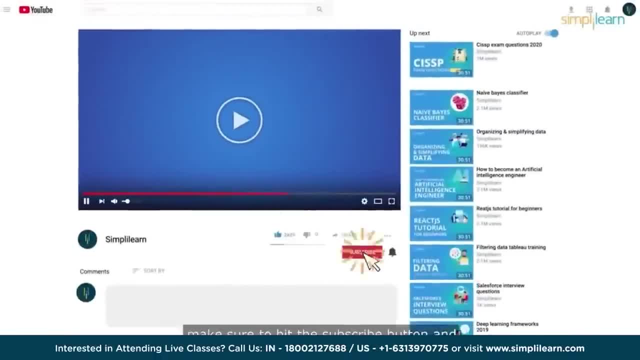 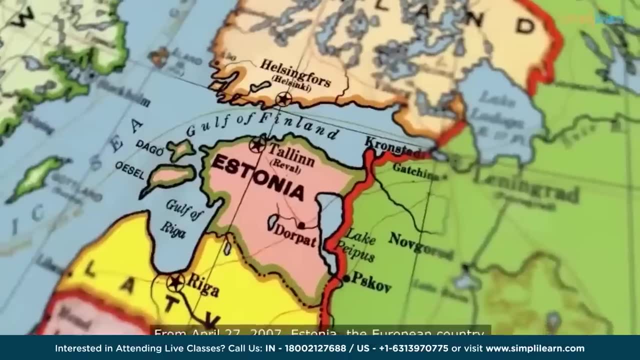 if you're new here and haven't subscribed already, make sure to hit the subscribe button and the bell icon for interesting tech videos. every day, Let's see what we have at number 10.. From April 27, 2007,. Estonia, the European country. 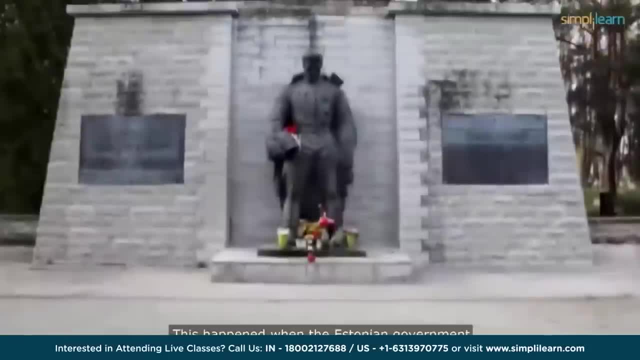 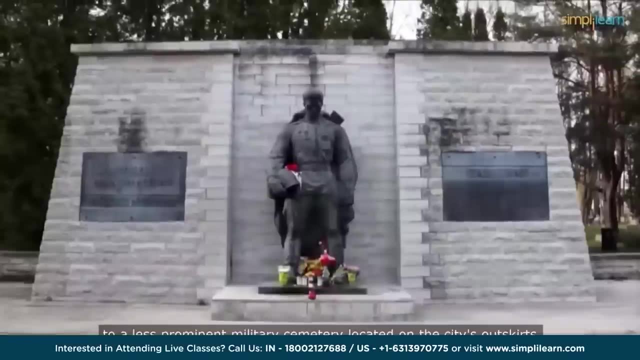 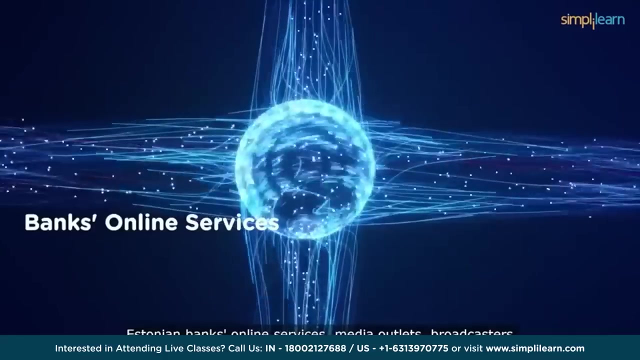 faced a series of cyberattacks that lasted for weeks. This happened when the Estonian government decided to move the bronze soldier from Tallinn Center to a less-prominent military cemetery located on the city's outskirts. Unprecedented levels of internet traffic took down Estonian banks' online services. 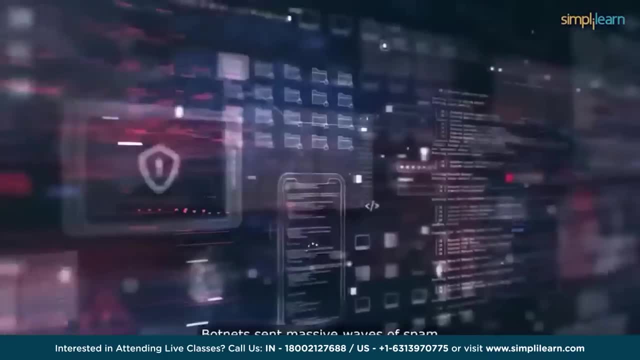 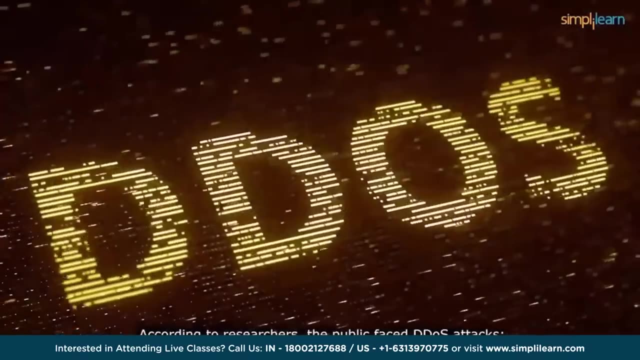 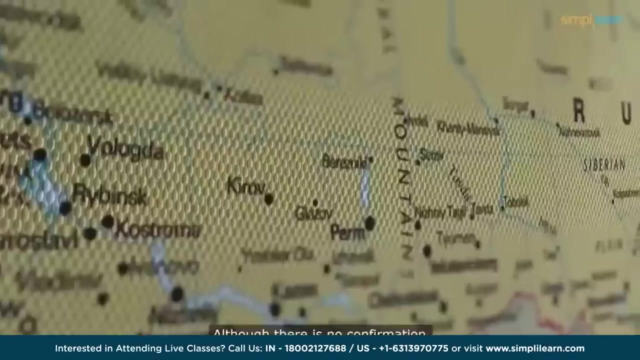 media outlets, broadcasters and government bodies. Botnet sent massive waves of spam and vast amounts of automated online requests. According to researchers, the public faced DDoS attacks. There were conflicts to edit the English-language version of the bronze soldier's Wikipedia page as well. 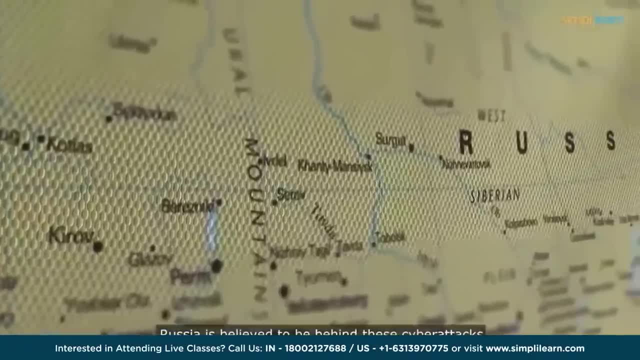 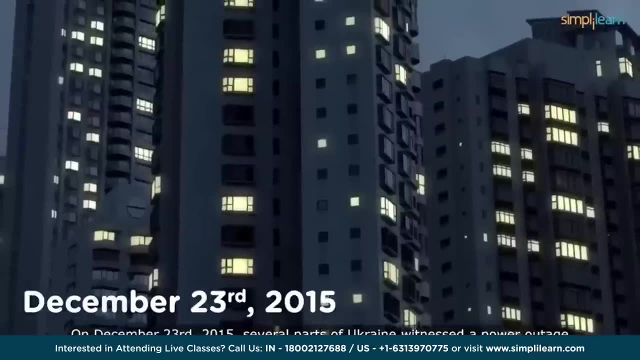 Although there is no confirmation, Russia is believed to be behind these cyberattacks that largely crippled the Estonian society. Let's now move on to the next attack. On December 23, 2015,, several parts of Ukraine witnessed a power outage. 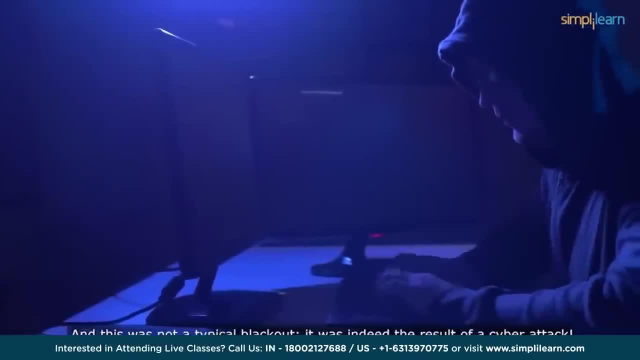 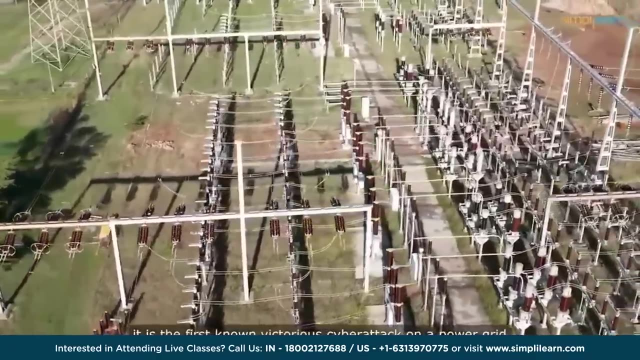 And this was not a typical blackout. It was indeed the result of a cyberattack. Information systems of three energy distribution companies in Ukraine were compromised. It is the first known victorious cyberattack on a power grid. It is said that here, hackers sent out phishing emails to the power companies. 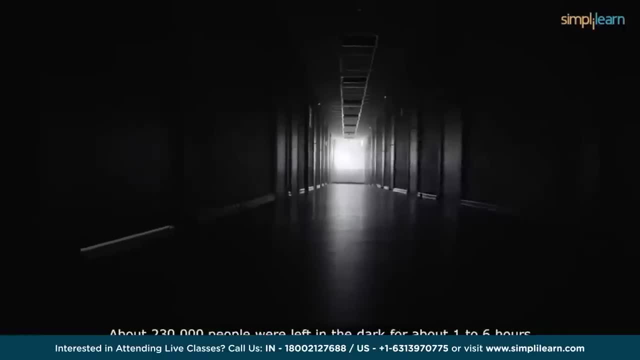 30 substations were switched off and about 230,000 people were left in the dark. It is said that here, hackers sent out phishing emails to the power companies. 30 substations were switched off and about 230,000 people were left in the dark. 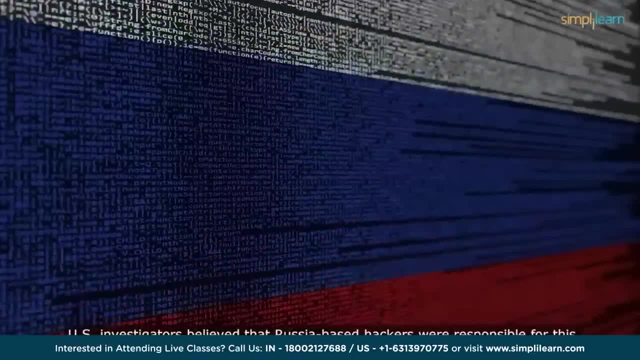 It is said that here, hackers sent out phishing emails to the power companies. It is said that here, hackers sent out phishing emails to the power companies. This was in the dark for about 1 to 6 hours. US investigators believed that Russia-based hackers were responsible for this. 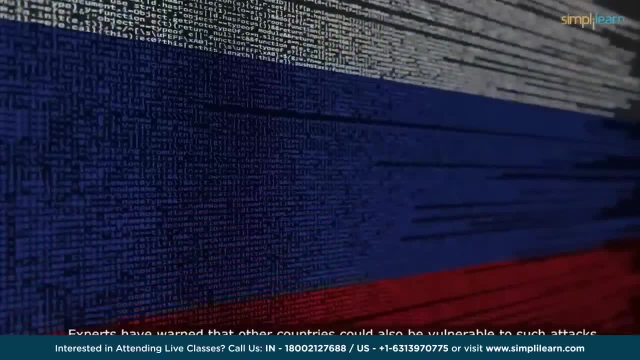 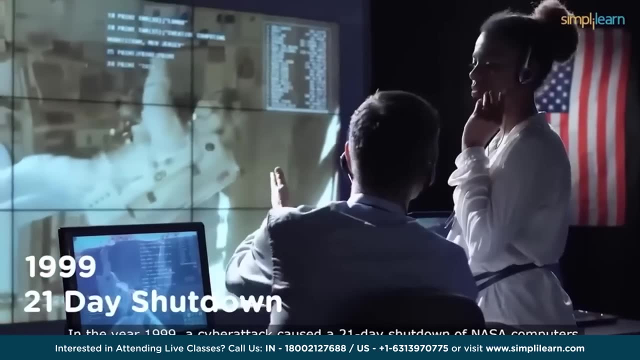 Experts have warned that other countries could also be vulnerable to such attacks. Let's see what we have at number 8.. In the year 1999, a cyberattack caused a 21-day shutdown of NASA computers. Unbelievable, isn't it? 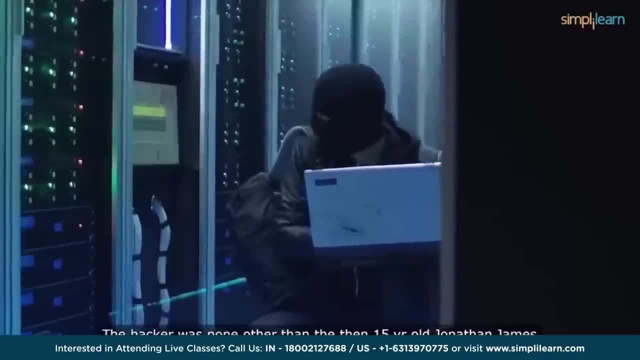 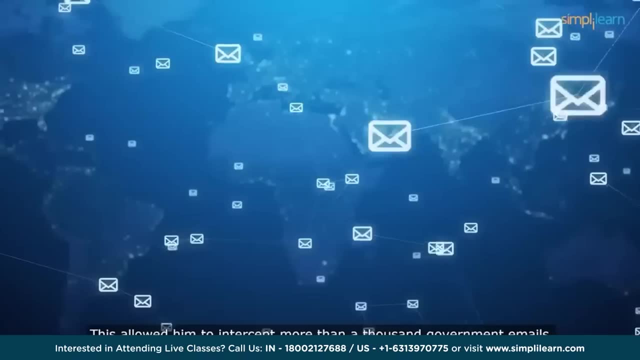 The hacker was none other than the then-15-year-old Jonathan James. He first penetrated US Department of Defense Division's computers and installed a security, installed a backdoor on its servers. This allowed him to intercept more than a thousand government emails, including the. 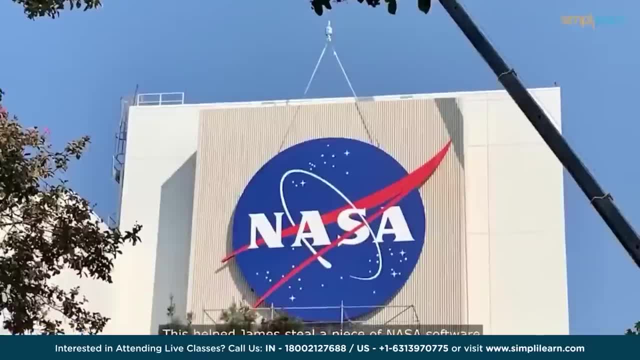 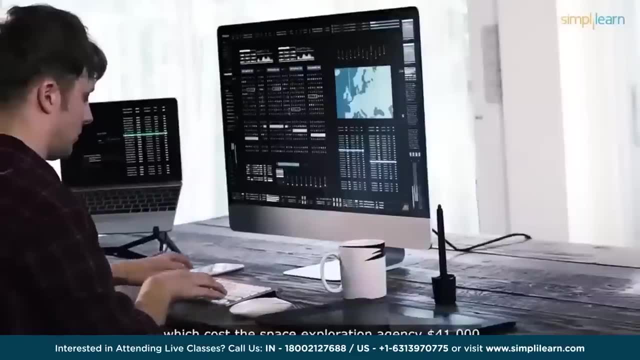 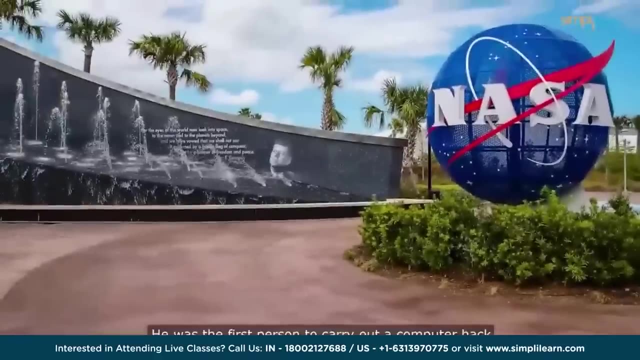 ones containing usernames and passwords. This helped James steal a piece of NASA software and crack the NASA computers that support the International Space Station, which cost the space exploration agencies $41,000. as systems were shut down for three weeks, He was the first person to carry out a computer hack against the American Space Agency. 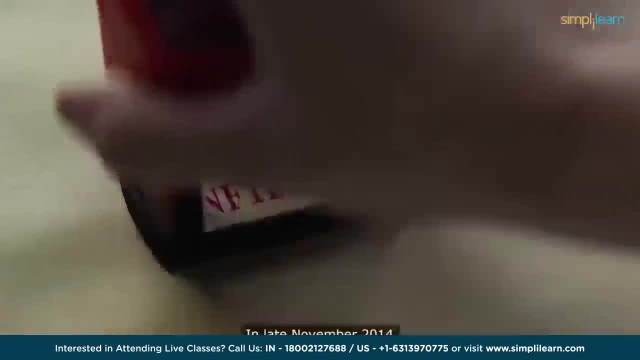 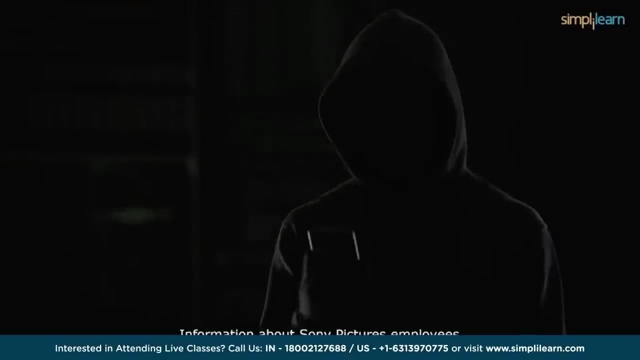 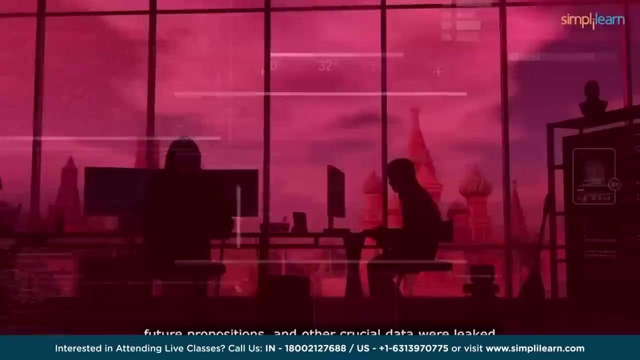 Let's now move on to the next attack. In late November 2014,, there was a leak of confidential data from the film studio of Sony Pictures. Information about Sony Pictures' employees, their emails, copies of the then-unreleased Sony films, future propositions and other crucial data were leaked. 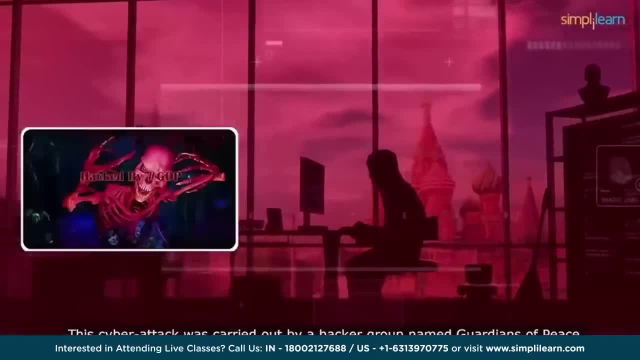 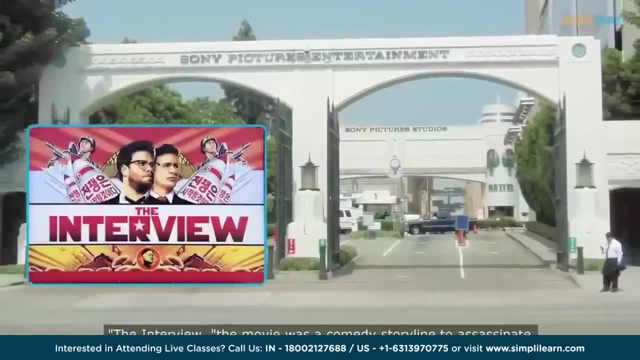 This cyber attack was carried out by a hacker group named Guardians of Peace. So what did the hackers want? Well, they demanded that Sony withdraw its then-upcoming movie, The Interview. This movie was a comedy storyline To assassinate the North Korean leader, Kim Jong-un. Sony then decided to cancel the film's. 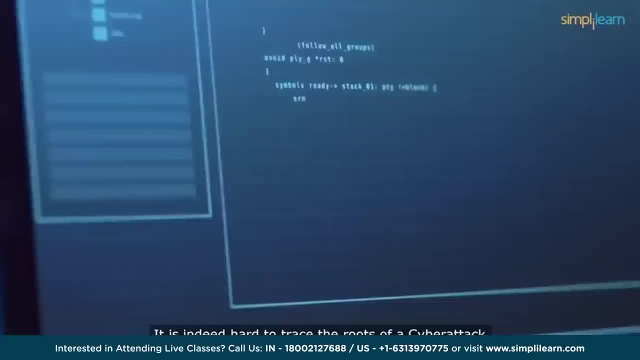 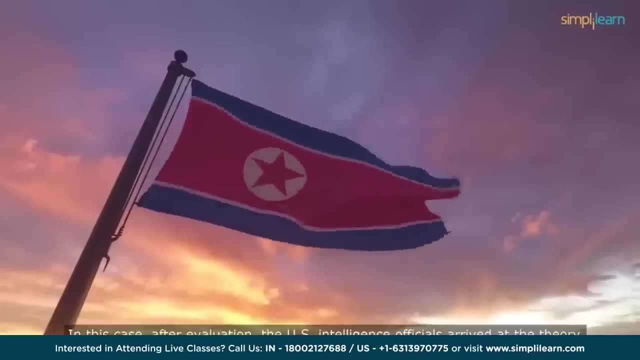 theatrical release due to the threats at cinema screening the movie. It is indeed hard to trace the roots of a cyber attack In this case. after evaluation, the US intelligence officials arrived at the theory that the attack was in a way related to the government of North Korea. 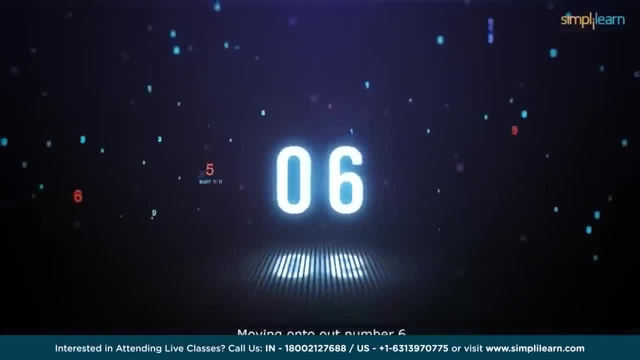 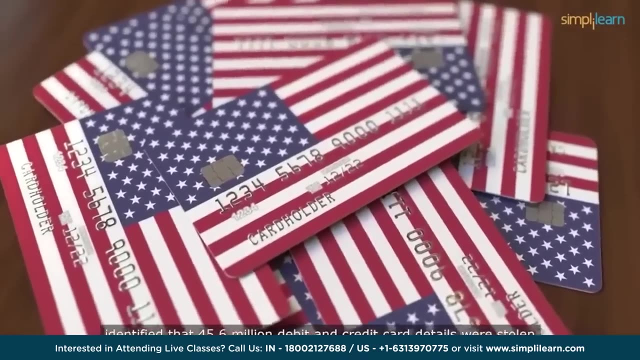 However, North Korea had denied the same. Moving on to our number 6.. In December 2006, TJX, the US retailer company, identified that 45.5% of the film's content was fake. When its beers covered 18.4 percent of all the data involved, there was about 15 million. 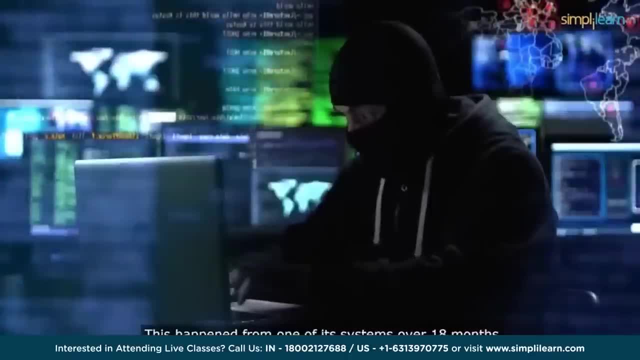 medical medicalzona, Six million debit and credit card details were stolen. This happened from one of its systems over 18 months by an unknown number of intrusions After giving birth to Naremberg's dealing with obtainally dangerous phobic disease. 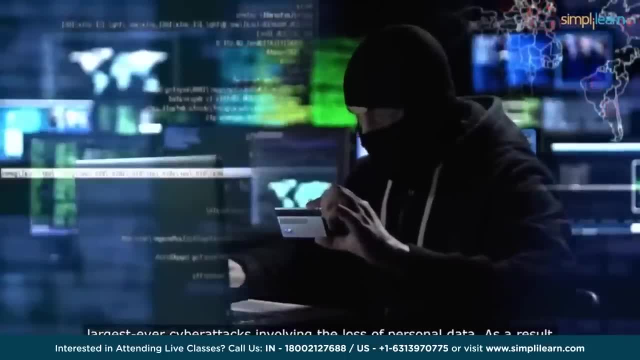 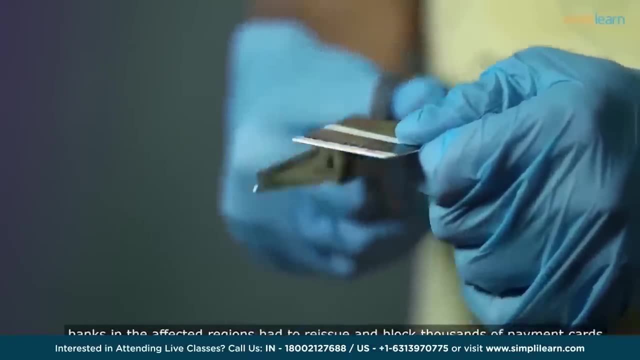 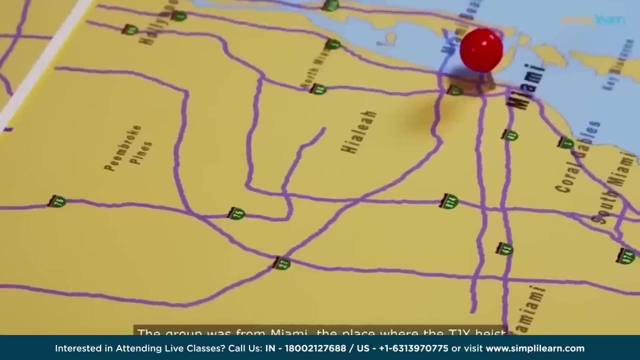 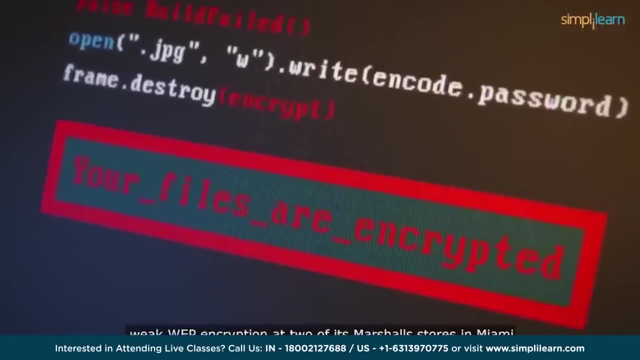 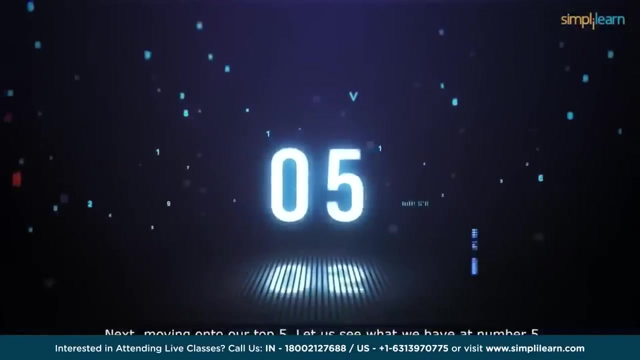 what was declared to be a false word, the virus spread by Naremberg's Mind間blocker. Reports said that the TJX data breach occurred because of weak web encryption at two of its Marshall stores in Miami. Next, moving on to our top 5, let us see what we have at number 5.. 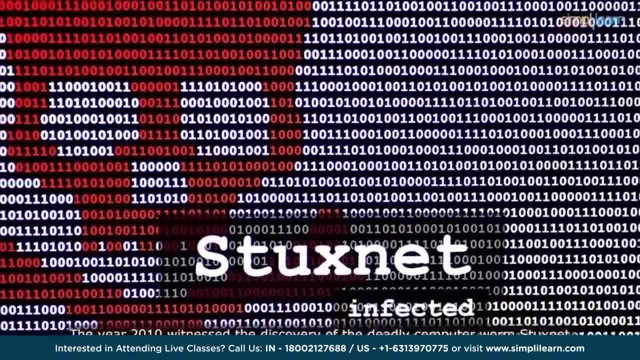 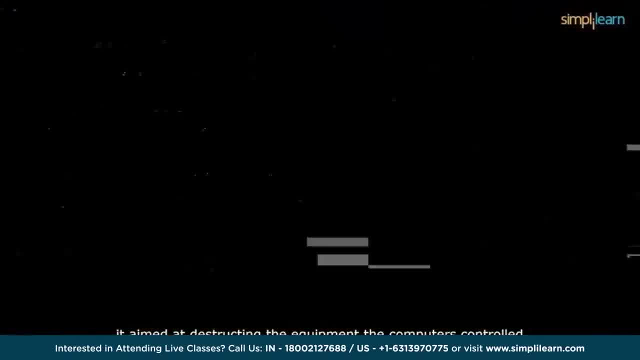 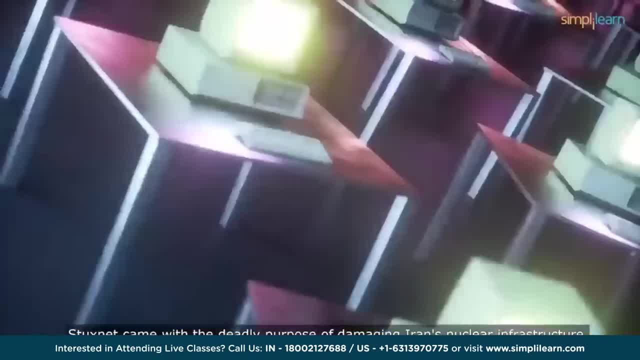 The year 2010 witnessed the discovery of the deadly computer worm Stuxnet. This malware's motive was unlike any other usual cyberattacks: It aimed at destructing the equipment the computers controlled. Stuxnet came with the deadly purpose of damaging Iran's nuclear infrastructure. 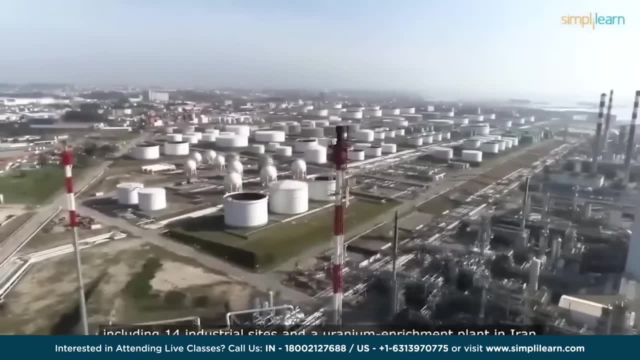 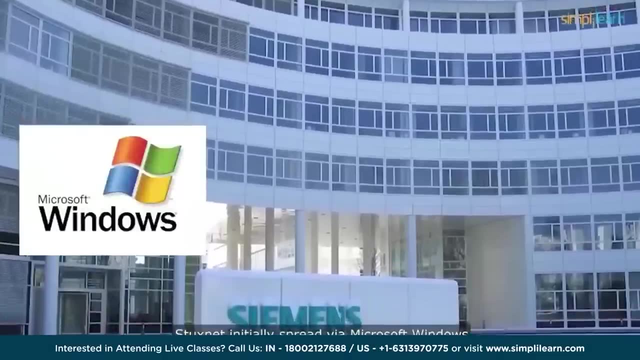 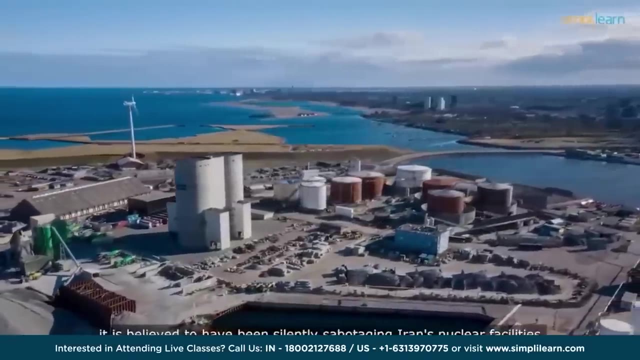 It infected more than 200,000 computers, including 14 industrial sites and a uranium enrichment plant in Iran. Stuxnet initially spread via Microsoft Windows and targeted Siemens Industrial Control Systems. Although it was discovered only in 2010,, it is believed to have been silently sabotaging. 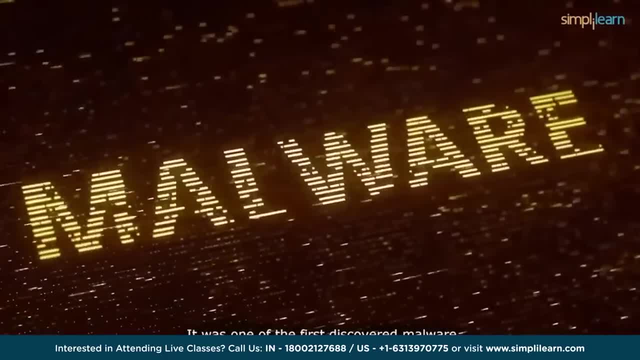 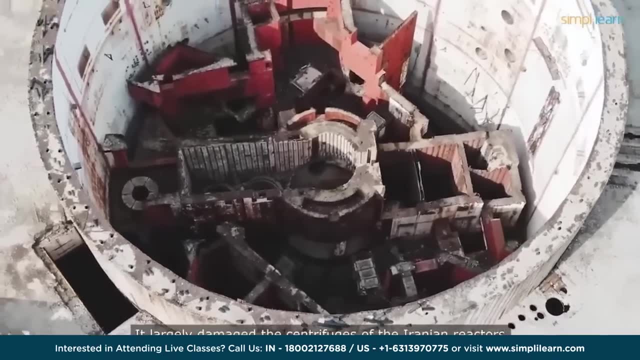 Iran's nuclear facilities. It was one of the first discovered malware that was capable of hampering hardware systems. It largely damaged the centrifuges of the Iranian reactors. This is believed to be a cyberweapon created by the US and the Israeli intelligence, although 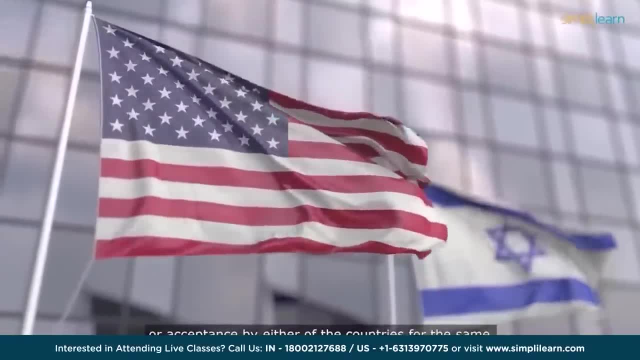 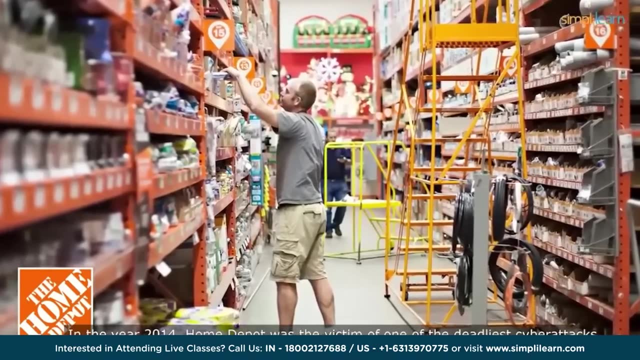 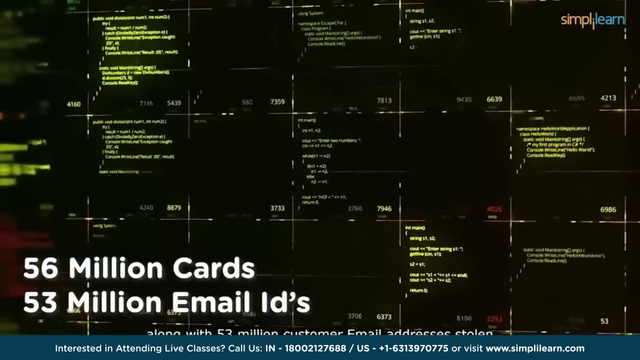 there is no documented evidence or acceptance by either of the countries for the same. Moving on to number 4,, in the year 2014,, Home Depot was the victim of one of the deadliest cyberattacks: 56 million payment cards were compromised, along with 53 million customer email addresses. 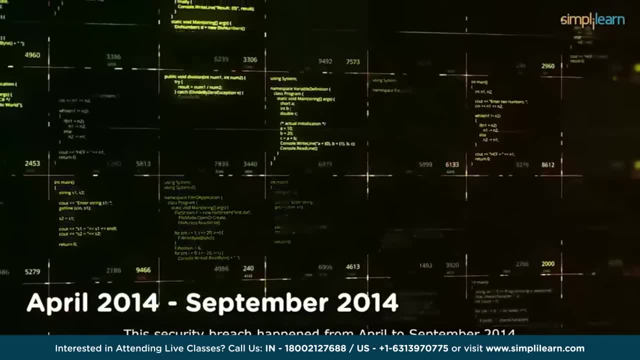 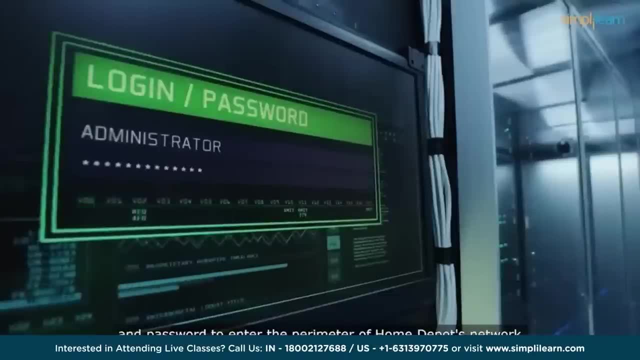 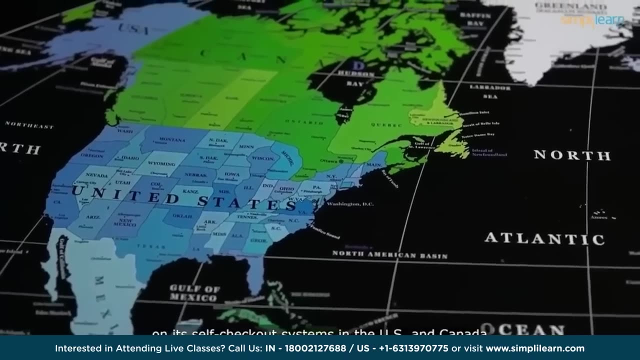 stolen. This security breach happened from April to September 2014.. Criminals were believed to have used a third-party vendor's username and password to enter the perimeter of Home Depot's network. The attackers were then able to deploy custom-built malware on its self-checkout systems in the 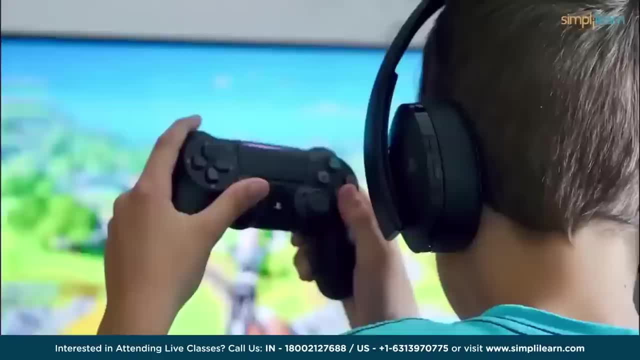 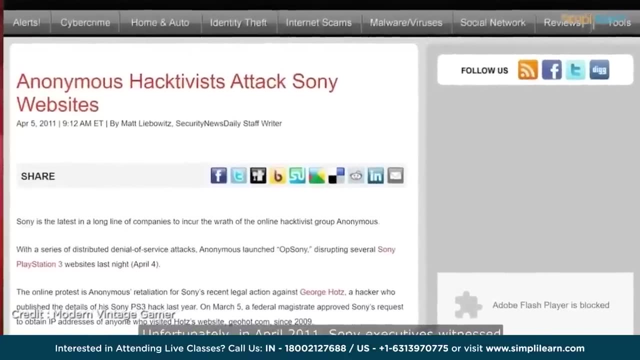 US and Canada, Moving on to our top 3.. As you might be aware, the PlayStation gaming system is one of Sony's most popular products. Unfortunately, in April 2011,, Sony executives witnessed a cyberattack. The system was used by the US and Canada. 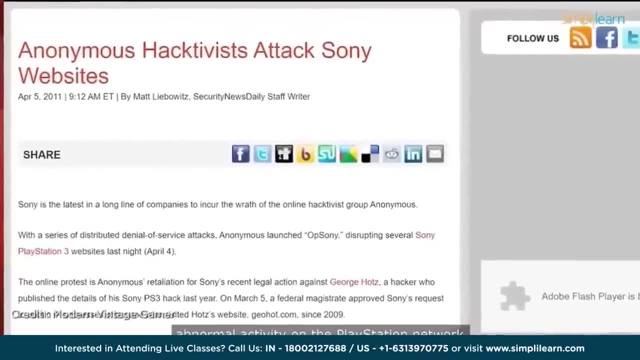 The system was used by the US and Canada. The system was used by the US and Canada. All of these companies were involved with the PlayStation gaming system, as well as the PlayStation Network. In 2018, the new version of the PlayStation came out. 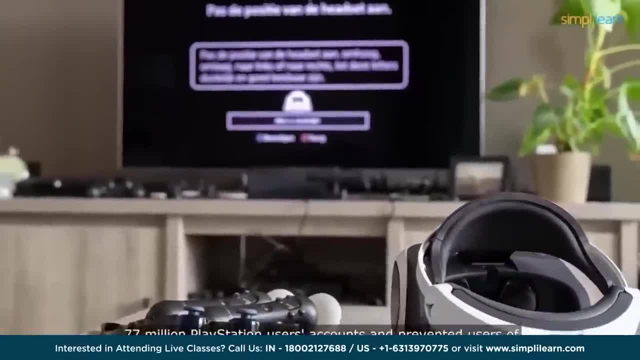 It became a popular topic for the US network and the world, with some uptick in its allowing users to install and use PlayStation PlayStore and other PlayStation games, It turned into a B extremes event. If you haven't played the PlayStation game yet, you should definitely go for it. 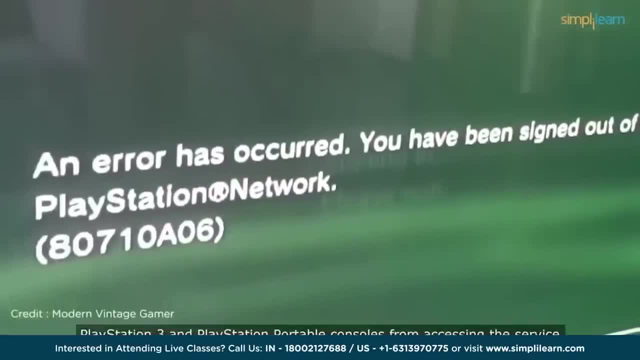 The PlayStation Network was the first sports game developed by Sony in 2018.. The PlayStation 3, the PlayStation 3, and the PlayStation Portable had been released on April 20, 2014.. The PlayStation system was used by Sony for more than 47 years and was again replaced. by Sony for the first time during the year 2014.. The PlayStation was released recently, in October 2014.. The PlayStation 3 was released in August 2014.. This forced Sony to turn off the PlayStation Network on April 20.. 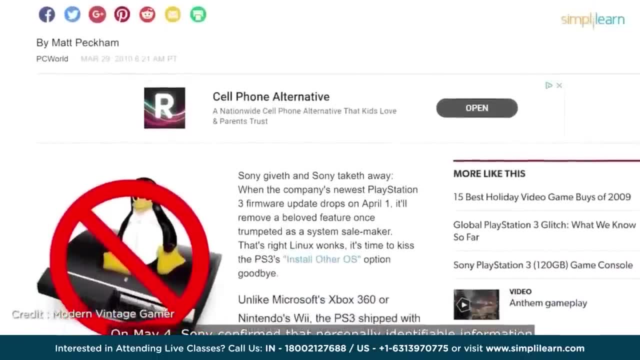 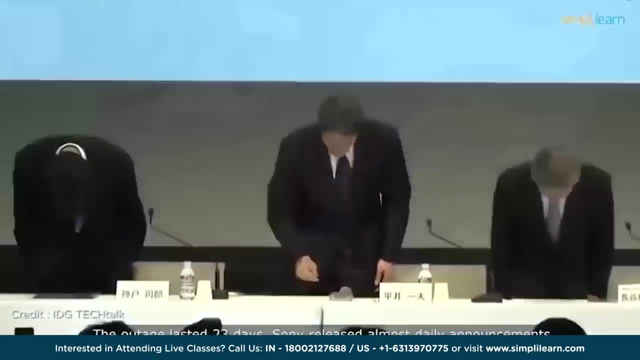 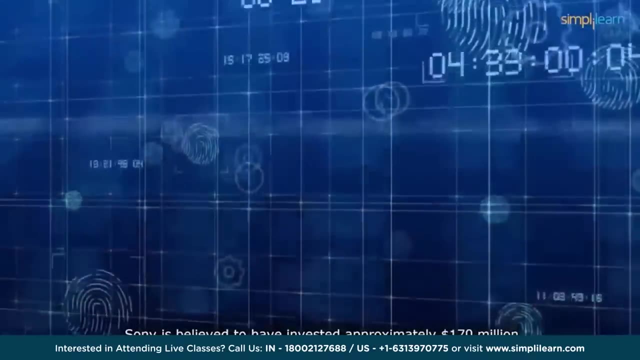 On May 4,, Sony confirmed that personally identifiable information from each of the 77 million accounts had been exposed. The outage lasted for 23 days. Sony released almost daily announcements concerning the system outage. In the end, Sony is believed to have invested approximately $170 million to improve the 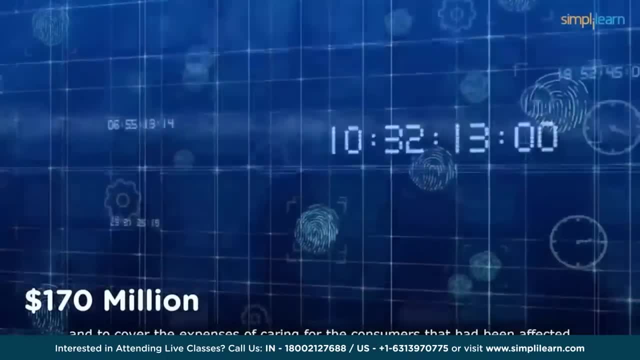 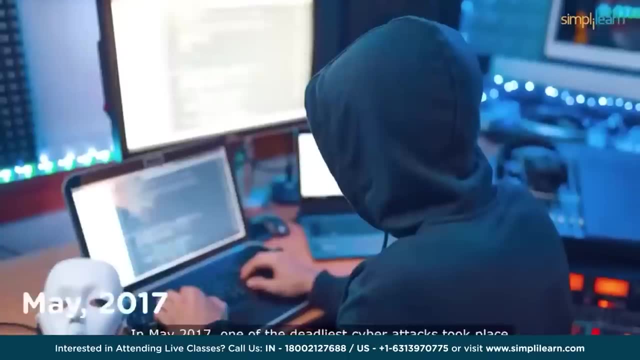 network's security, to investigate the attack and to cover the expenses of caring for the consumers that had been affected. Let's now move on to the next attack, at number 2.. In May 2017, one of the most dangerous cyberattacks took place. 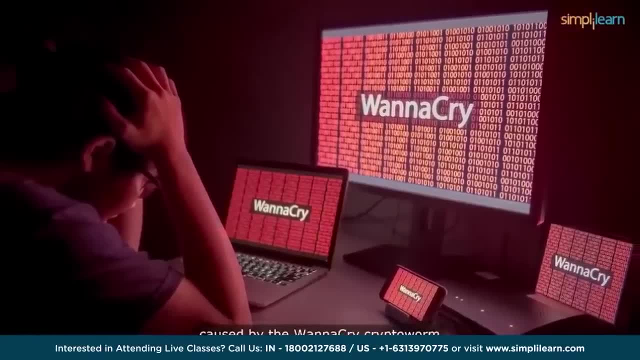 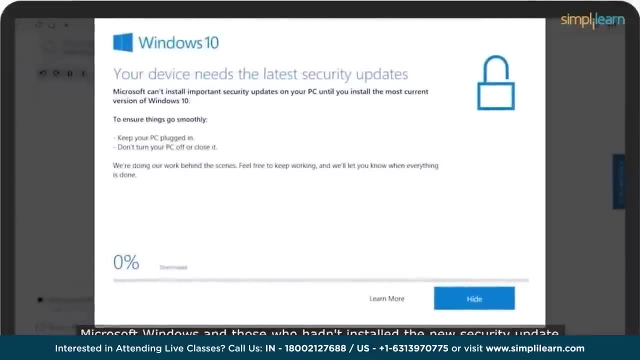 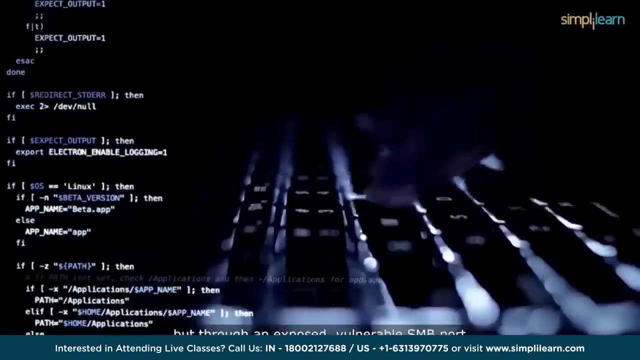 It was known as the WannaCry ransomware attack, caused by the WannaCry crypto worm. The victims were the users that used the unsupported version of Microsoft Windows and those who hadn't installed the new security update. This did not take place through phishing, like other attacks, but through an exposed vulnerable. 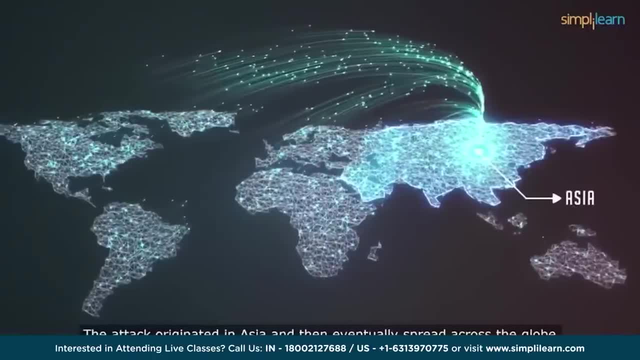 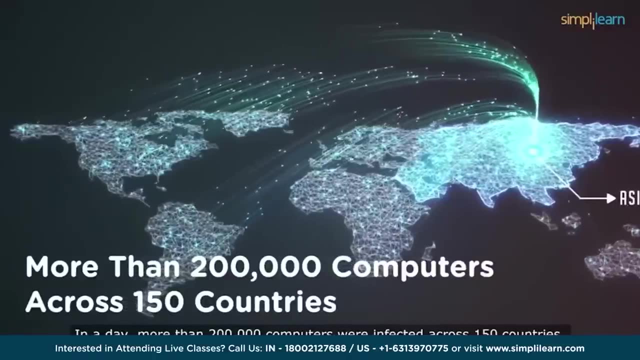 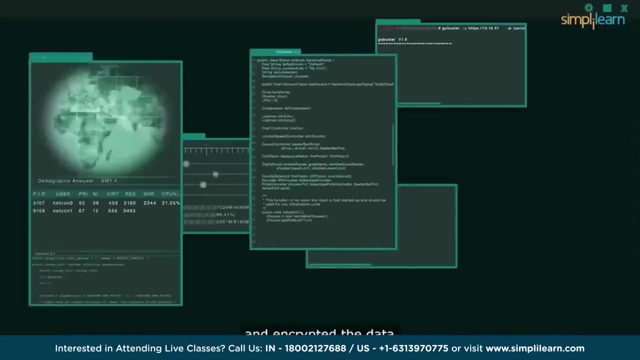 SMB port. The attack originated in Asia and then eventually spread across the globe. In a day, more than 200,000 computers were infected across 150 countries. The WannaCry crypto worm locked the users out of the targeted systems and encrypted their data. The users were asked for a ransom of $300 to $600,, which had to be paid via Bitcoin, in exchange for their data. This attack took a toll on both private and government organizations. It resulted in damages from hundreds of thousands of people. The attack took a toll on both private and government organizations. 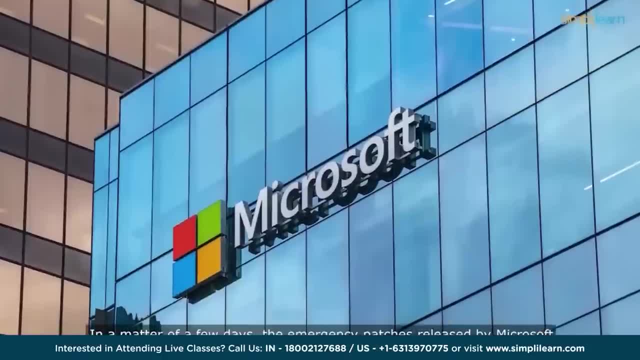 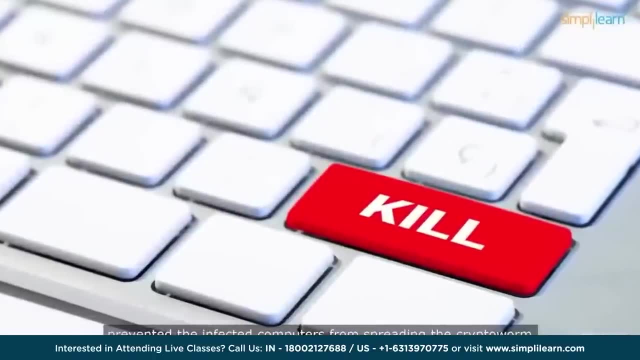 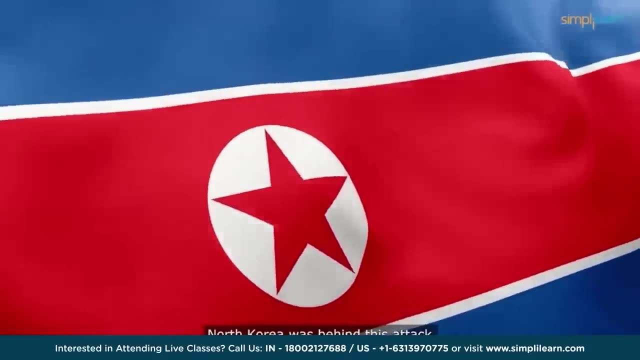 It resulted in damages from hundreds of thousands of people In a matter of few days. the emergency patches released by Microsoft halted the attack. Also, the discovery of a kill switch prevented the infected computers from spreading the crypto worm. Security experts in a few countries believed that North Korea was behind this attack. 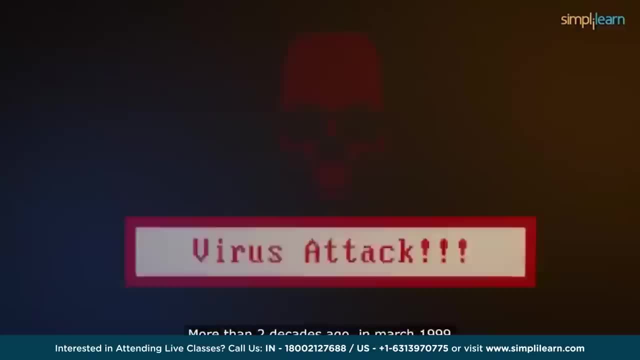 And finally, let's see what we have at number one. More than two decades ago, in March 1999, the Melisa virus, a mass-mailing macrovirus, was released. More than two decades ago, in March 1999, the Melisa virus, a mass-mailing macrovirus, was released. 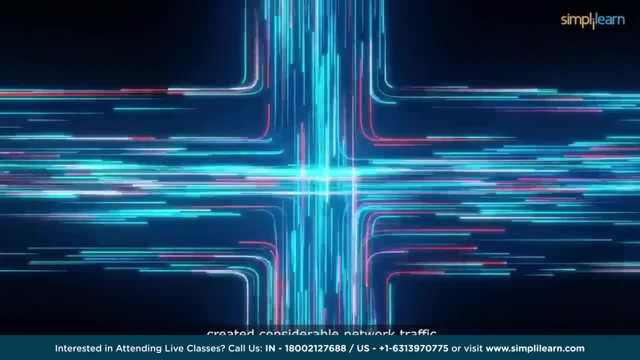 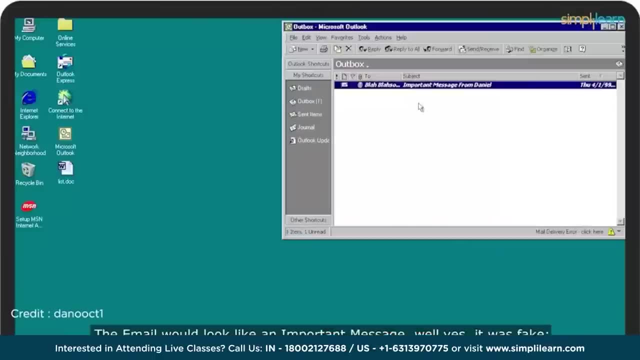 Microsoft Word and Outlook-based systems and created considerable network traffic. Melissa virus infected computers via emails. The email would look like an important message. Well, yes, it was fake If the recipient opens the attachments in the mail and downloads the document and then 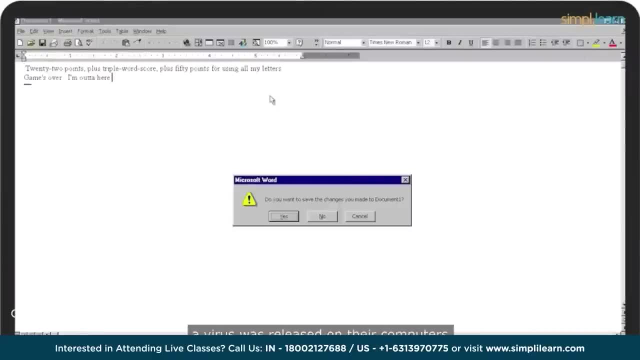 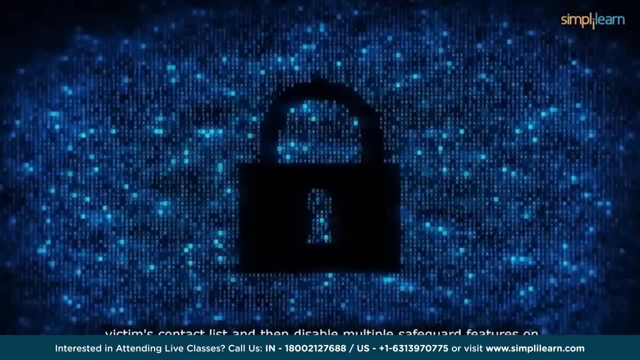 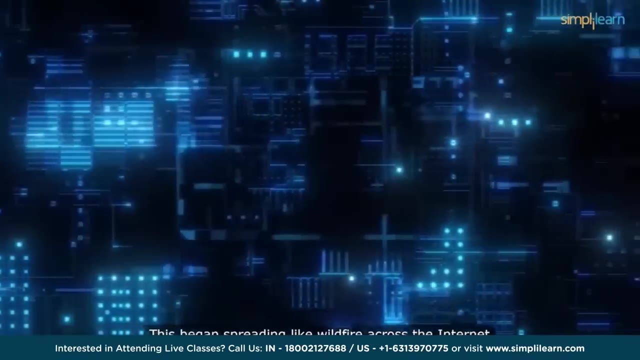 opens it with Microsoft Word, a virus was released on their computers. This would then mass mail itself to the first 50 people in the victim's contact list and then disable multiple safeguard features on Microsoft Word and Microsoft Outlook. This began spreading like a wildfire across the Internet. 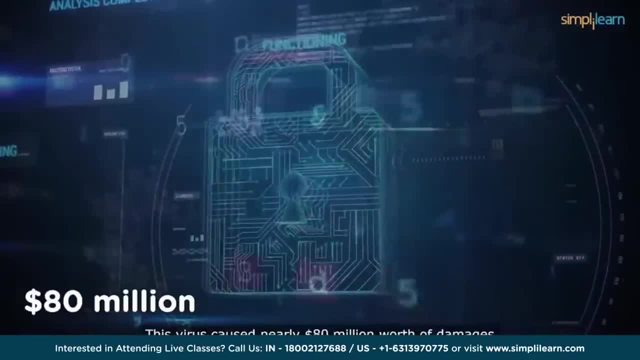 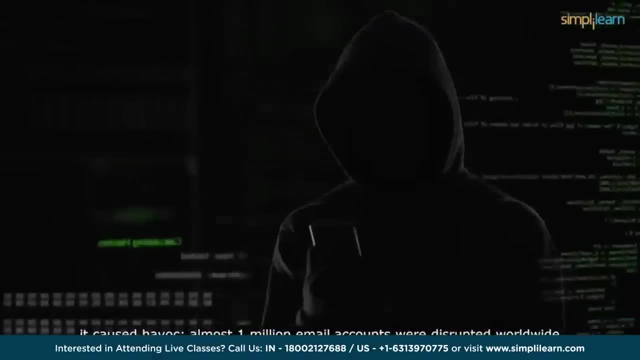 David L Smith released the virus. The virus caused nearly 80 million worth of damages. It did not steal data or money. However, it caused a havoc. Almost one million email accounts were disrupted. worldwide Agencies were overloaded and some had to be shut down entirely. 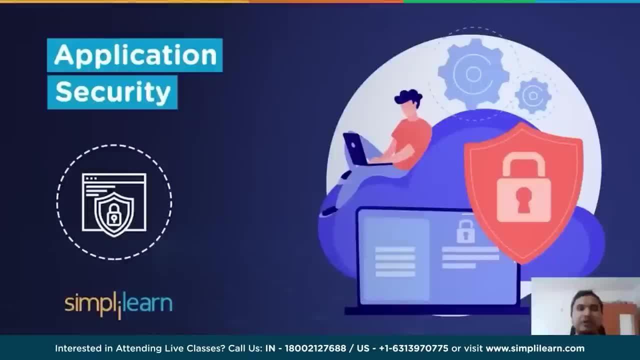 And Internet traffic in some locations was slowed down. Security was considered an afterthought in software development. It is becoming an increasingly important concern for all aspects of app development, from design to deployment and beyond. The number of programs produced, distributed, deployed and patched across networks continually. 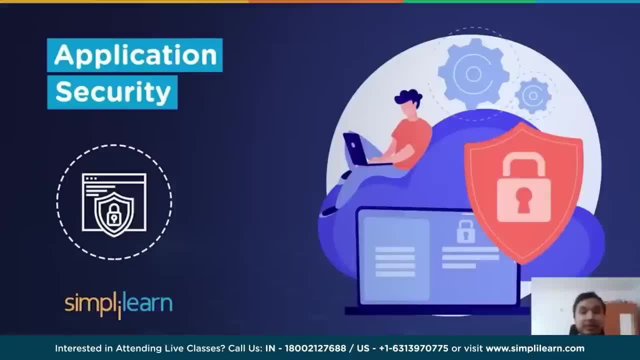 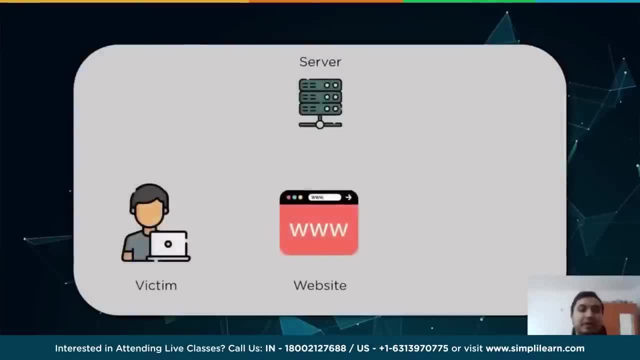 increases As a result. application security features must deal with a wide range of risks. Let's take an example. A malicious script may be mirrored on the victim's web browser or kept in a database and run whenever the user contacts. This allows malicious code to be entered in the case of an output. 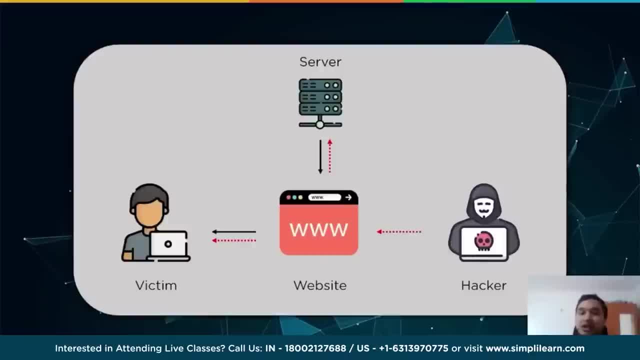 The major cause of this attack is faulty user input validation, which allows malicious input to enter the final output. An evil user can enter a script that will be injected into the website's code. The browser will then be unable to determine whether the processed code is helpful. 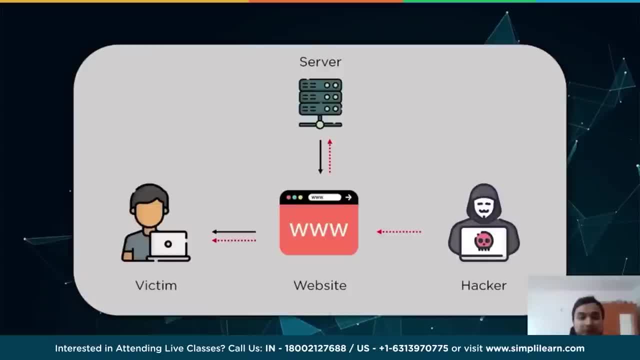 As a result, a malicious script is performed on the victim's browser or a bogus form of code is performed is shown to the users. Are you aware of which attack this is? If not, do stay till the end to find the correct answer. Are you aware of which attack this is? If not, please stay till the end. 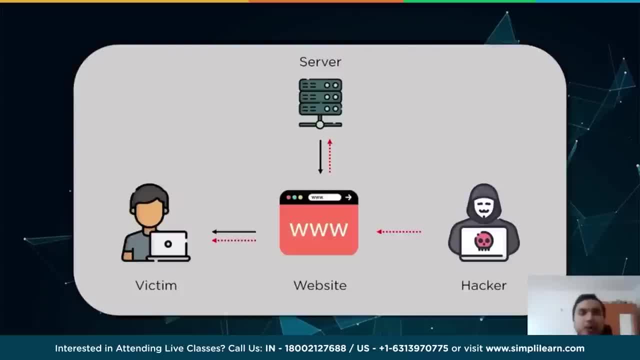 of the video to know the correct answer. Hey everyone, welcome to today's video on application security. Before we move forward, subscribe to our channel and hit the bell icon to never miss an update from us. Let's take a look at the topics to be covered today. We start by learning about 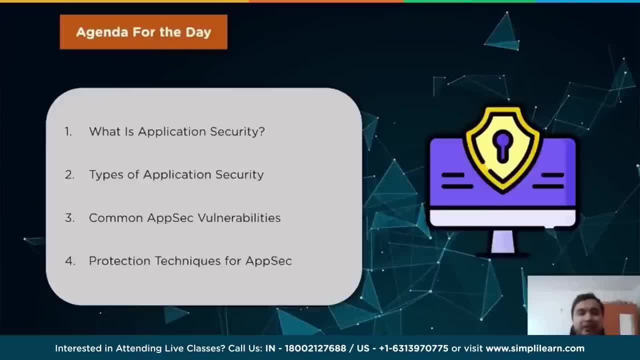 application security and its different types. We learn about the most common vulnerabilities in AppSec, followed by the importance of application security in today's cybersecurity space. Next, we cover some attacks against application layer security and end the video with some protection techniques to enforce application security parameters. Let's start by learning. 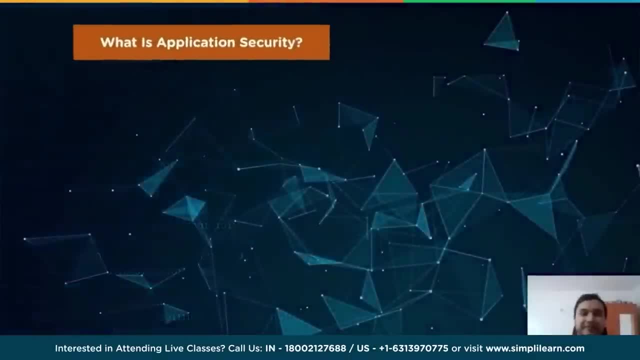 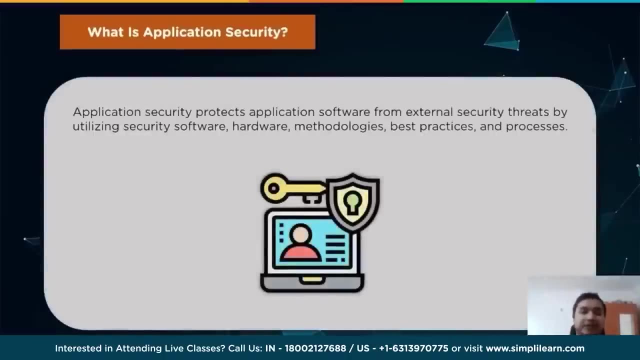 about application security from a grassroots perspective. Application security, which is often known as AppSec, protects application software against risk issues, such as attack on from external security threats, by utilizing security software, hardware, methodologies, best practices and different processes. Organizations require application security. 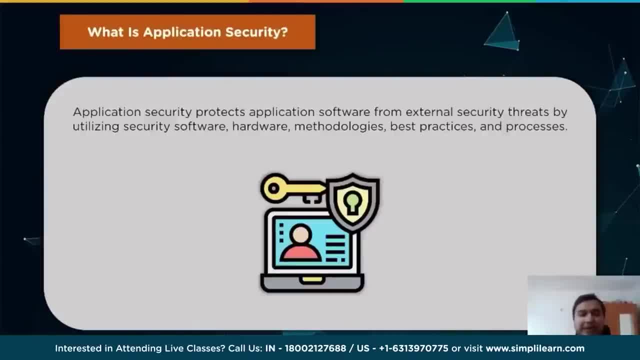 technologies that safeguard all of their programs, from internal to popular external apps on consumer mobile phones. These solutions must address the whole development cycle and provide testing after an application has been deployed to detect possible issues. Application security mechanisms must be capable of testing web pages for possible and exploitable vulnerabilities. analyzing code. 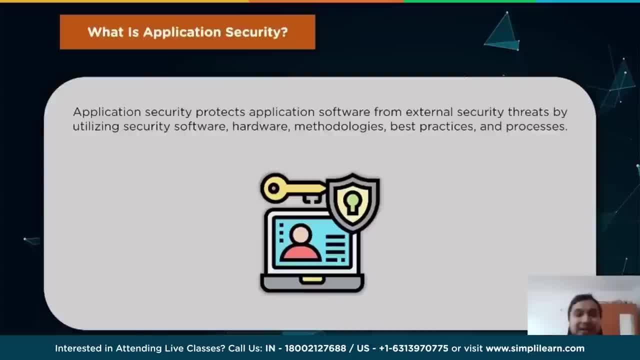 and assisting in the administration of development and safety management processes. The testing solutions must also be simple and easy to install for system administrators. worldwide, Consumers utilize hundreds of applications daily to access theoretically important and favored services such as e-commerce, banking, music, etc. To be productive, 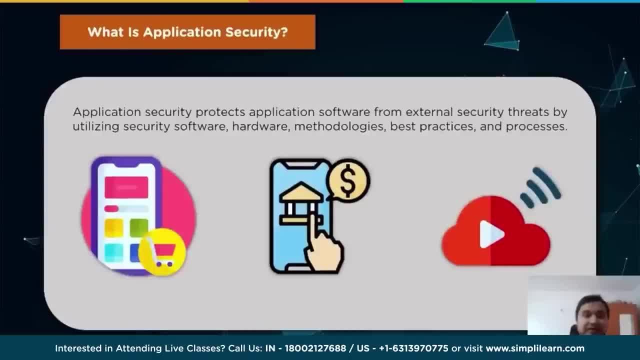 these professionals use a wide range of technologies and technologies, A variety of software solutions as well, ranging from online word checkers to tablet-based creative tools, among other things. Backend software, of course, exists to automate essential operations and processes and decreases human labor. But to make matters worse, the quantity and complexity 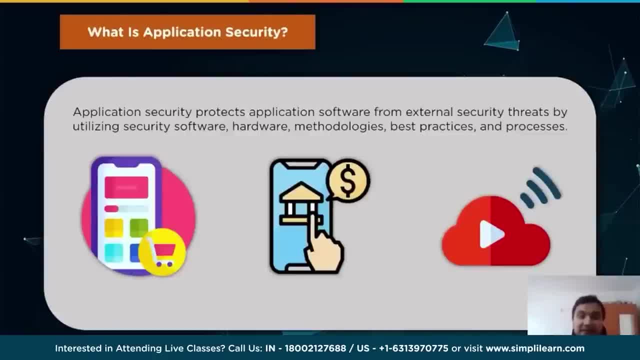 of these apps and their backend code is increasing. The software security problem 10 years ago was about securing desktop apps and static web pages that were natively harmless and easy to scale through and defend. The software security problem 10 years ago was about securing desktop apps and static web pages that were natively harmless and easy to scale through and defend. 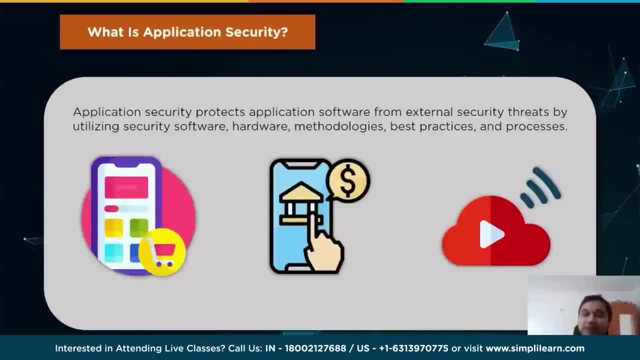 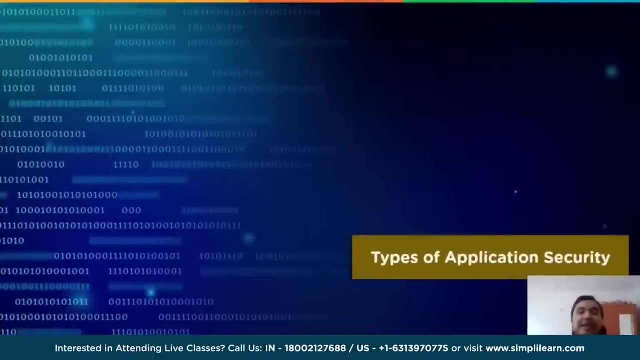 Because of outsourced development, the number of legacy programs and in-house development that uses third-party open-source and commercialized off-the-shelf software modules. the software supply chain has become considerably more convoluted Now that we understand application security on a general level. 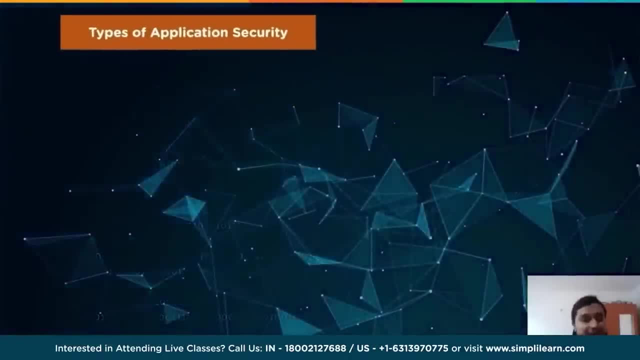 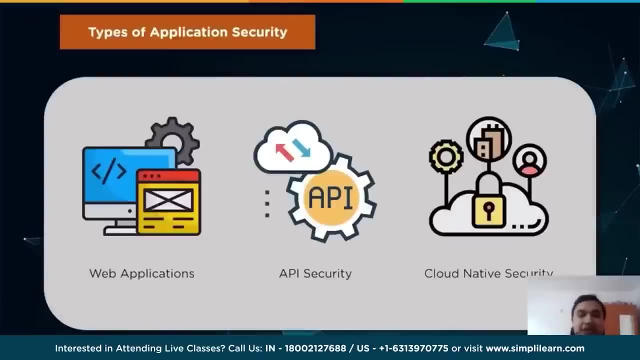 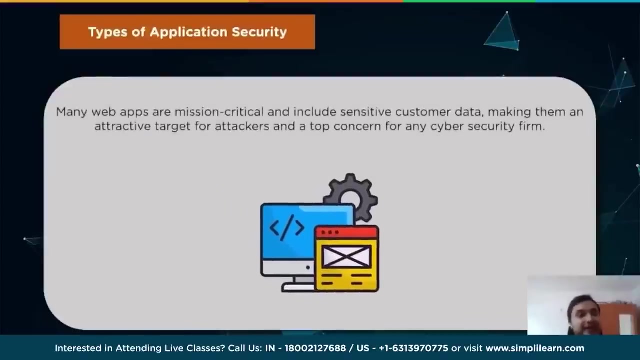 let us go through some of the different categories or the types of application security. There are three major types to be covered in this section: Web application security, API security and cloud-native application security. A web application is a program available through the internet and it operates on a web server. 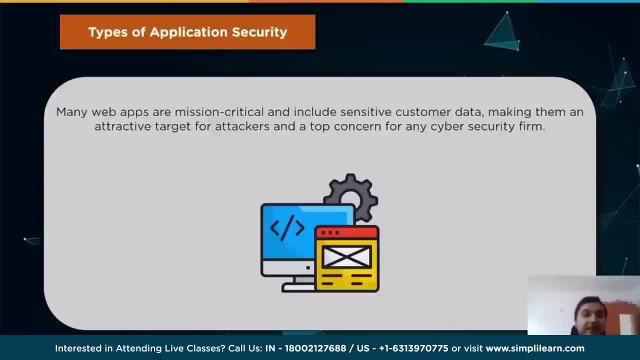 The client is accessed using a web browser. The applications, by definition, must allow connections from clients across unsecured networks. This exposes them to a variety of risks. Many online apps are mission-critical and include sensitive customer data, making them an attractive target for attackers and a top concern for any cybersecurity project. 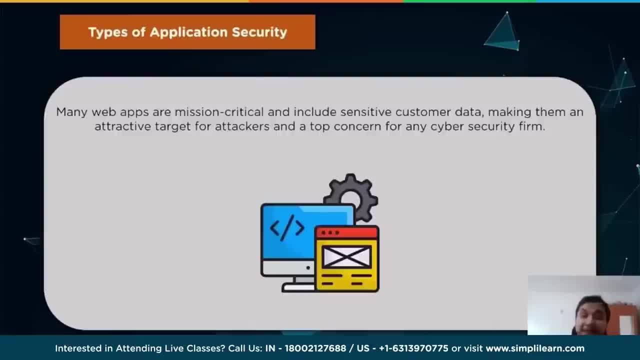 A web application security program or framework. The advert of HTTPS, which offers an encrypted channel of communication guards versus man-in-the-middle attacks or MITM attacks, has addressed several online application weaknesses. Many weaknesses, though, still persist. Many security providers have created solutions specifically geared to safeguard online. 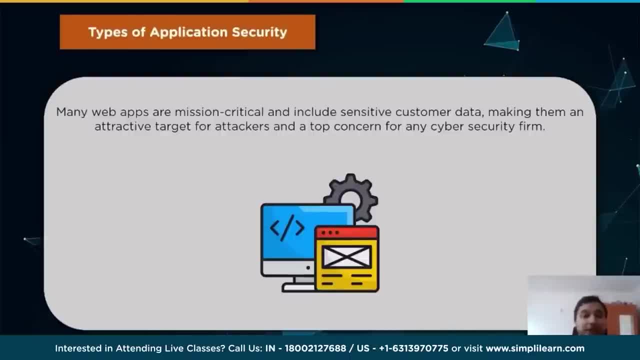 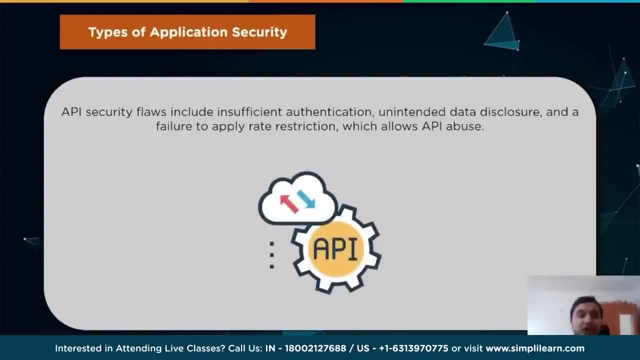 applications in response to the rising challenge of web application security. A web application firewall is an example of a security technology meant to identify and prevent application-layer assaults in the case of web applications. When it comes to APIs, APIs that have security flaws are the root of. 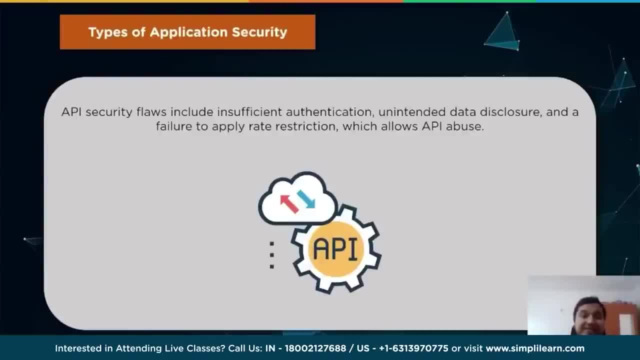 many major data breaches. They have the potential to reveal sensitive data and disrupt vital corporate processes. API security flaws include insufficient authentication, unintended data disclosure and a failure to apply rate restriction, which allows API abuse. The requirements for API security, like the necessity for web applications, 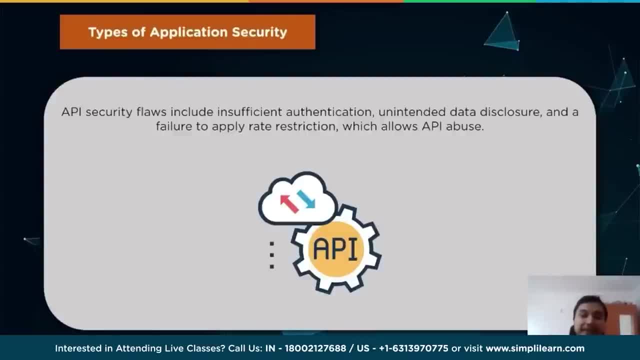 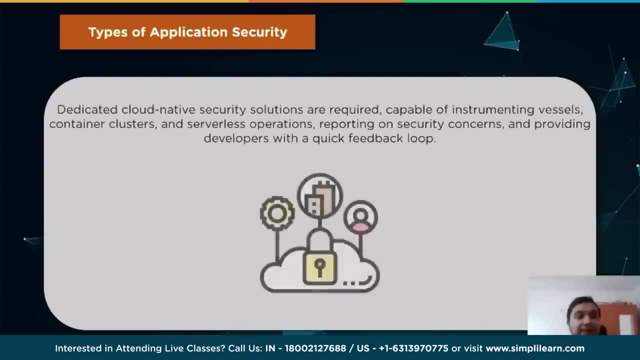 security led to the creation of sophisticated equipment that can discover API vulnerabilities and protect APIs in production level. The third type is cloud-native application security Infrastructure and environments are often built up automatically in cloud-native apps, depending on declarative configuration, which is known as Infrastructure, as Code or IAC. 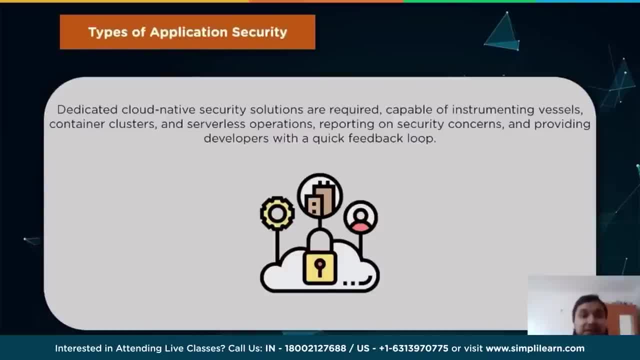 Developers are tasked with developing declarative settings and application code, both of which should be secure. Because practically everything is secure, the application should be secure. The application should be secure because practically everything should be secure. The application should be secure because practically everything is secure. 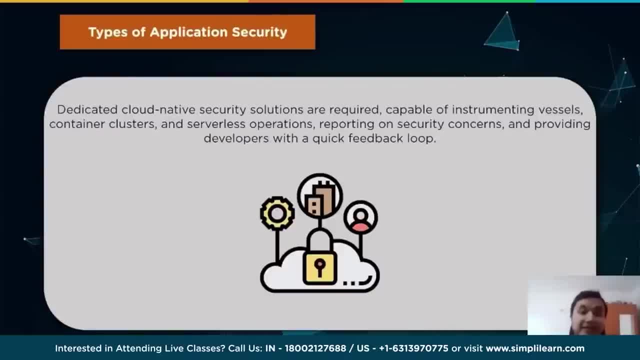 Everything is defined during the development stage. Shifting left is even more crucial in cloud-native setups. Traditional testing techniques can help cloud-native apps, but they are insufficient. Dedicated cloud-native security solutions are mandatory at this point of time, which are capable of instrumenting vessels, container clusters and serverless. 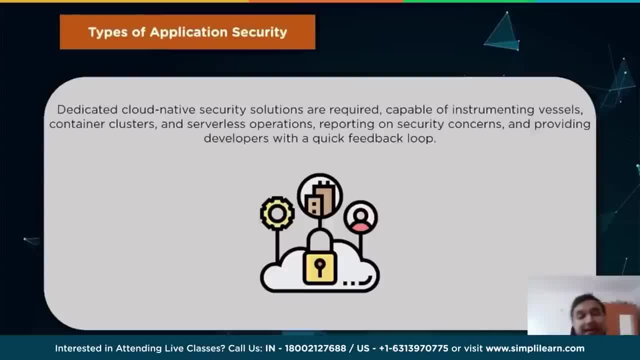 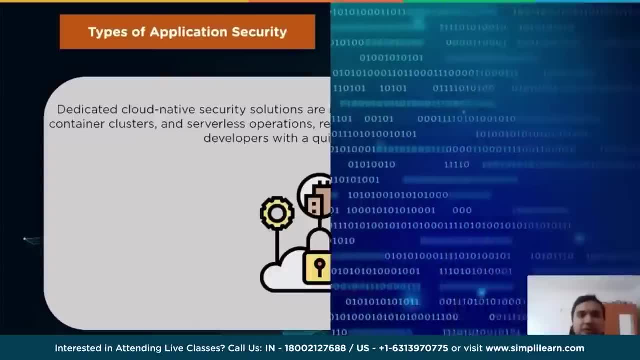 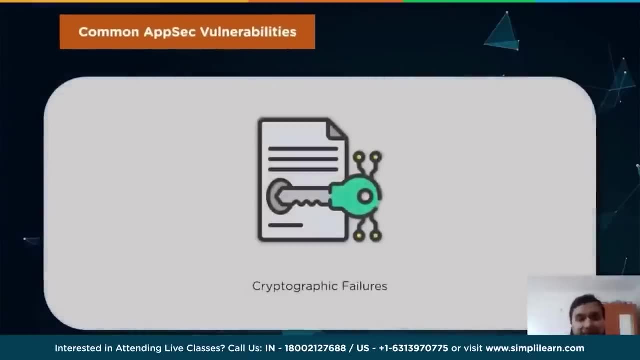 operations, reporting on security concerns and providing developers with a quick feedback loop. Now that you have covered the different types of application security, let us go through some of the most common vulnerabilities that these frameworks face on a daily basis. First is cryptographic failure, When data is not adequately safeguarded in transit and at rest. 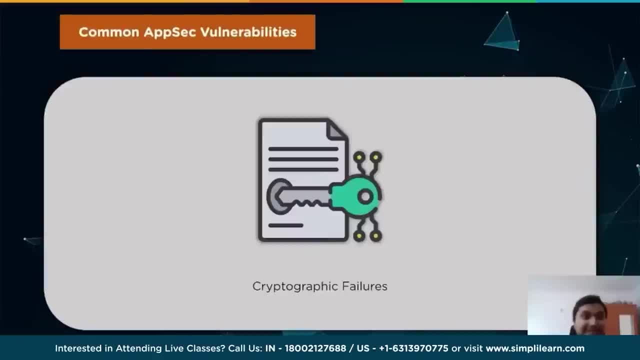 cryptographic failures, which are formerly known as sensitive data exposures, occur. It has the potential to reveal credentials, health information, credit card details and personal information as well, depending on the type of data being protected. in that particular case- Injection attacks- Threat actors can use injection vulnerabilities to protect against. 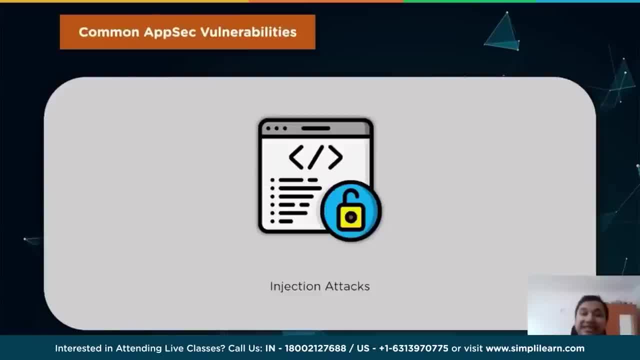 vulnerabilities. to convey malicious information to a web application interpreter, It has the potential to assemble and execute this data on the server. SQL injection is a popular type of injection which I have already covered in an introduction for this video. Another major vulnerability are outdated components: Vulnerable and outdated. 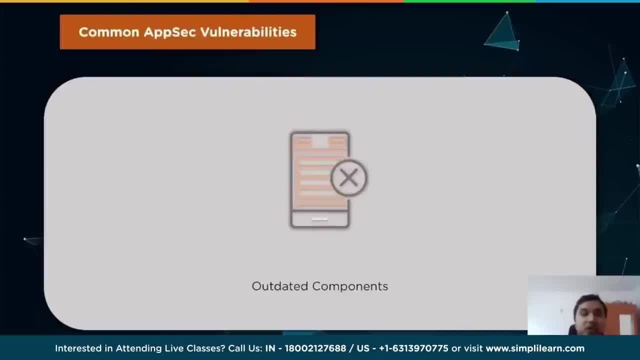 components encompass any vulnerability caused by obsolete or unmaintained software. It can happen if you construct or even use an application without first learning about its core components and versions. Authentication failures, Identification and authentication failure, which are previously known as broken authentication- encompass any security issue involving user identities. 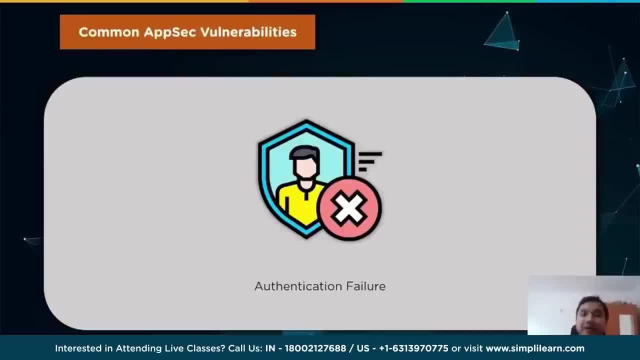 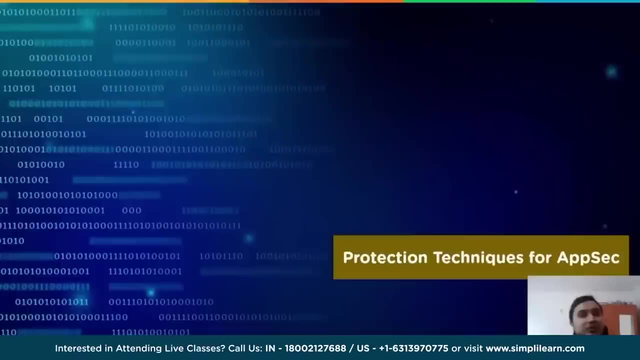 Identity attacks and exploitation may be avoided by implementing secure session administration, authentication and validation for all identities in the organization. In the next section, let us cover some of the protection mechanisms employed by cybersecurity firms and third-party automated software to prevent the application layer from being 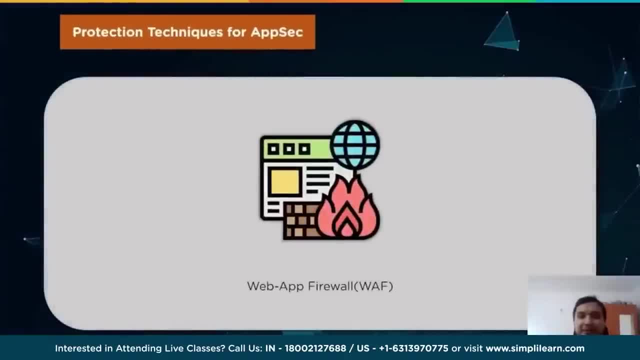 bombarded with SQL injections and other attacks. The first is a web application firewall, or WAF. A web application firewall monitors and filters HTTP traffic between a web application and the World Wide Web. Web application firewall architecture does not address all risks, but it may be used in conjunction with other defense mechanisms. It can be used with a portfolio. 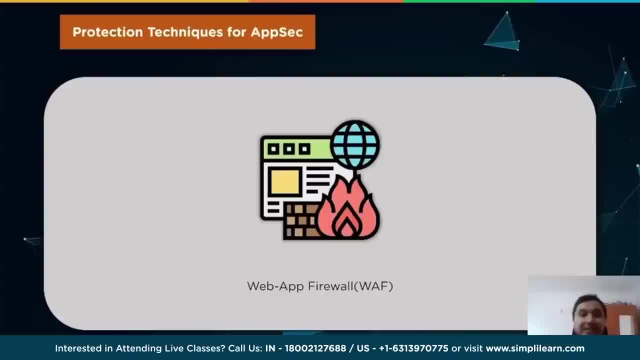 of security solutions to provide a comprehensive defense against diverse attack roles. It is a protocol layer 7 protection in the open systems interconnection or the OSI model paradigm that helps defend online applications against attacks such as cross-site scripting, cross-site fraud, escape injection and file intrusion. 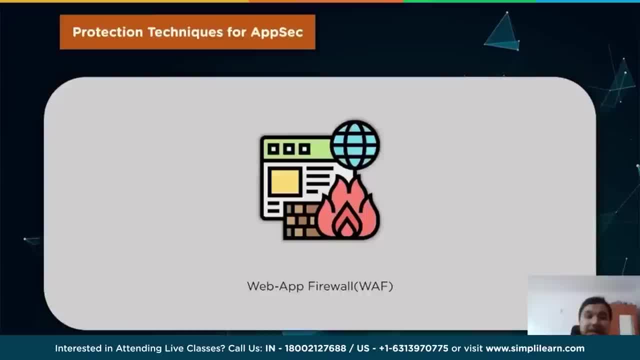 Unlike a proxy server, which conceals the identity of client computers by an intermediary, a WAF functions as a reverse proxy, shielding the server from exposure. It acts as a barrier in front of a web application, protecting it from the internet. The clients must pass through the web application firewall before they can access the application. 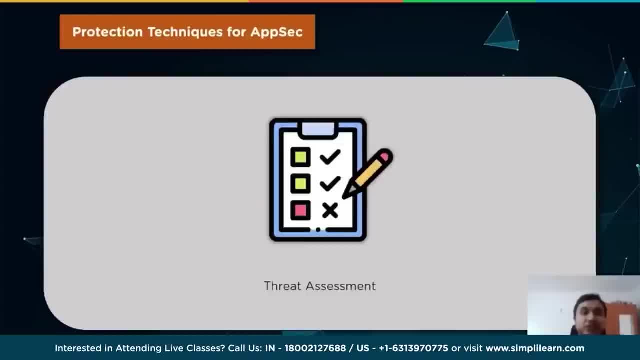 The second is threat assessment. A list of sensitive assets to safeguard will assist you in understanding the threat to your firm and how to minimize them. Considering how a hacker can infiltrate an application if existing security protections are in place and whether additional tools or defense capabilities are required, it is also 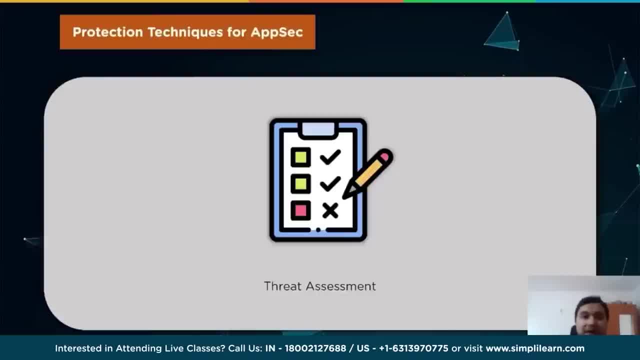 crucial to keep your security expectations in check. Nothing is impenetrable, even with the most stringent security measures. It would be best if you were realistic about what you believe your team can handle in the long term When pushed too aggressively. safety regulations and procedures. 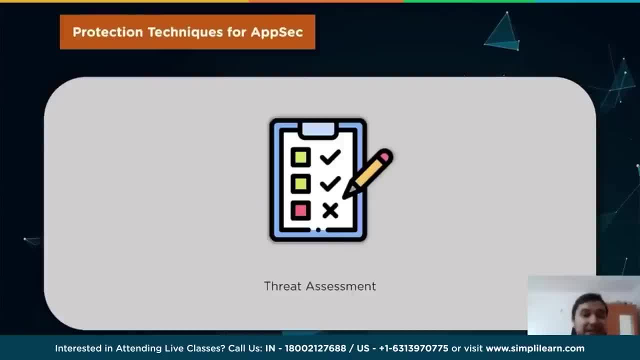 might be disregarded. Remember that safety is a lengthy and time-taking project that requires the collaboration of other employees and sometimes even your customers. The next topic is privilege management. Limiting privileges may be a challenge. However, it is an important aspect in the human 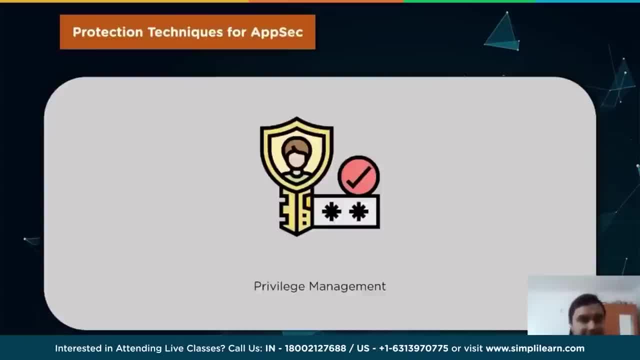 is vital, especially for mission critical and sensitive systems. The least privileged principle states that access to programs and data should be limited to those who require them when they require them. For two reasons, the least privileged principle is absolutely critical. The first is that hackers may 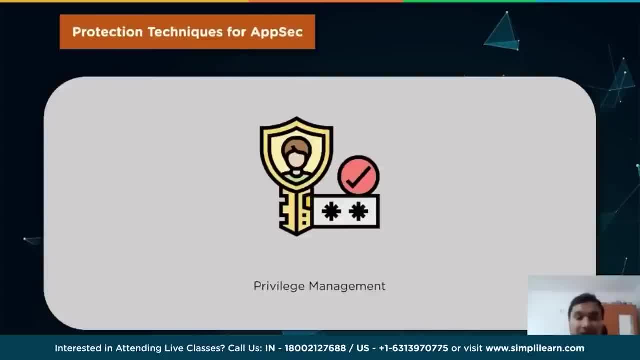 compromise less privileged accounts and ensuring they do not acquire access to highly sensitive systems is critical. The second is that internal dangers are equally harmful as external adversaries. If insiders go bad, it's critical to ensure they never have more power than they need, minimizing the harm that they 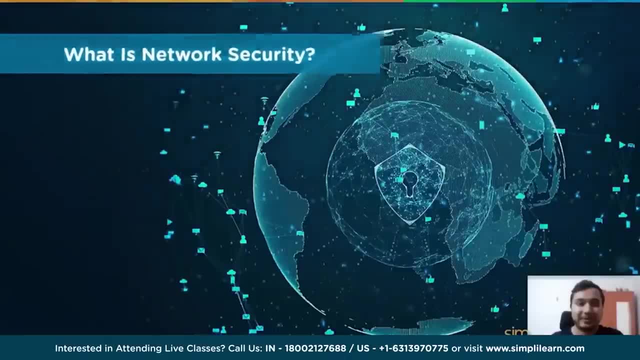 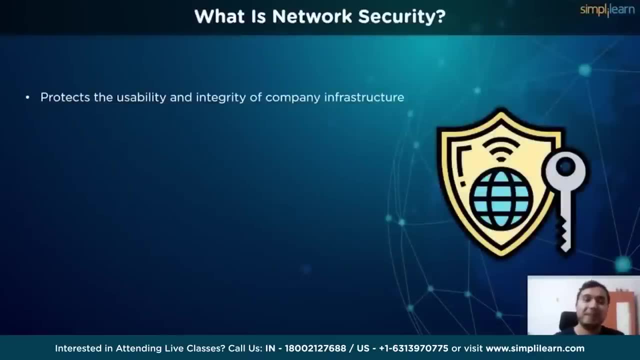 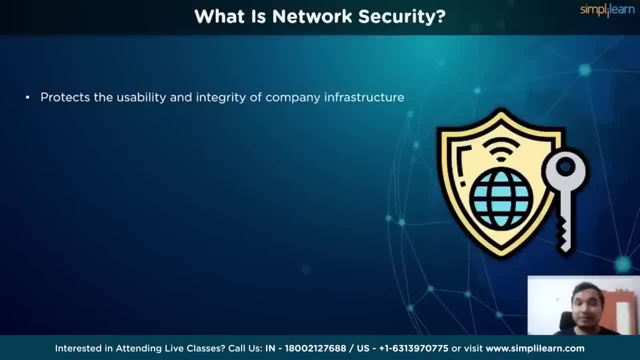 Effective network security is a tool that can be used to protect the network itself and the applications that run over it. Each defensive layer here enforces a set of security policies, which are determined by the administrator beforehand. This aims at securing the confidentiality and accessibility of the data and the 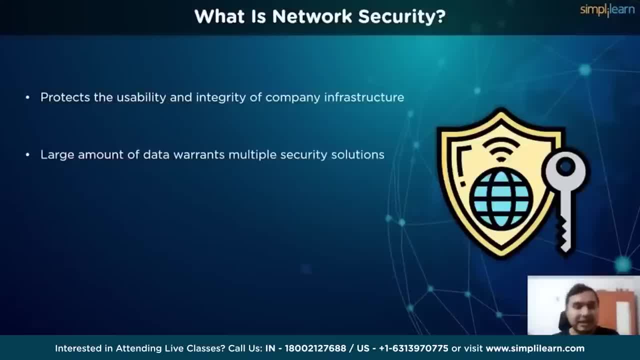 network T? he every company or organization that handles a large amount of data has a degree of solutions against many cyber threats. The most basic example of network security is password protection. It has a network the user chooses. Central network security is the investigator of's network security. If 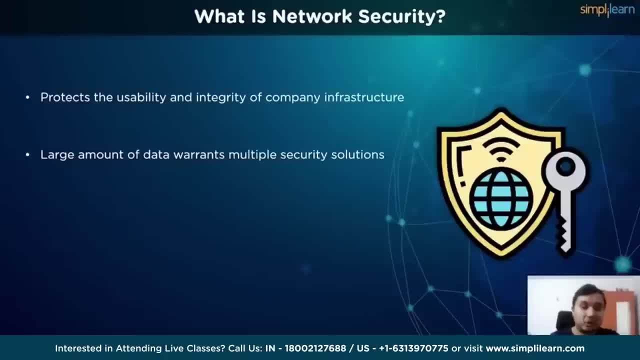 Recently, network security has become the central topic of cybersecurity, with many organizations involving applications from people with skills in this area. It is crucial for both personal and professional networks. Most houses with high-speed internet have one or more wireless routers, which can be. 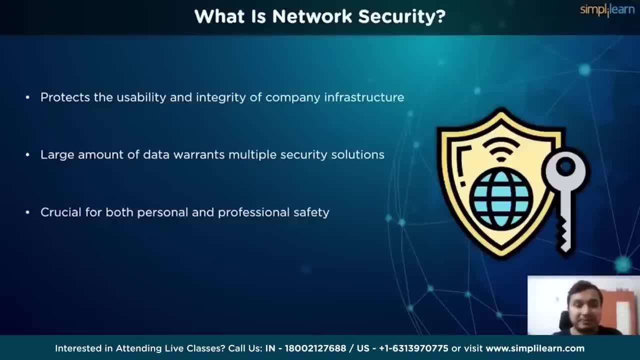 vulnerable to attacks if they are not adequately secured. Data loss, theft and sabotage risk may be decreased with the usage of a strong network security system. The workstations are protected from hazardous firewall thanks to network security. Additionally, it guarantees the security of the data which is being shared over a network. 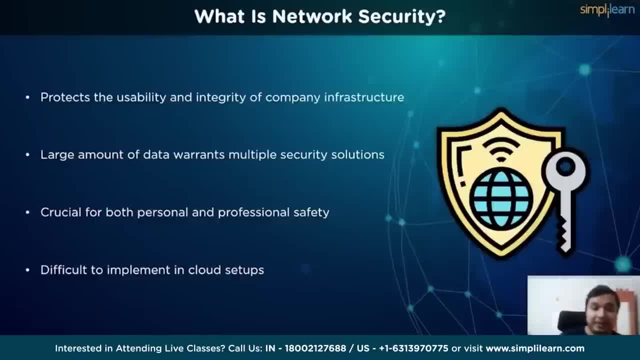 By dividing information into various sections, encrypting these portions and transferring them over separate pathways. network security infrastructure offers multiple levels of protection to thwart man-in-the-middle attacks, preventing situations like eavesdropping, among other harmful attacks. It is becoming increasingly difficult in today's hyper-connected environment, as 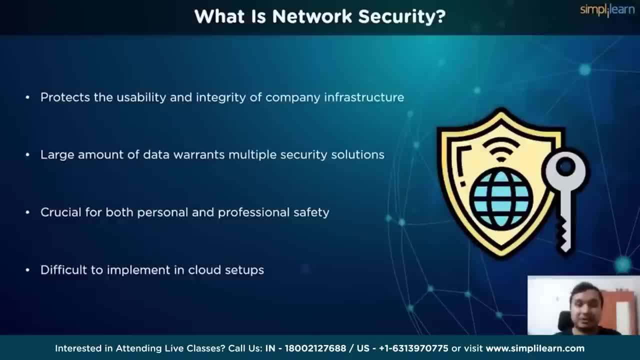 more corporate applications migrate to both public and private networks. Additionally, modern applications are also frequently virtualized and dispersed across several locations, some outside the physical control of the IT team. Network traffic and infrastructure must be protected in these cases, since assaults on businesses are increasing every single day. 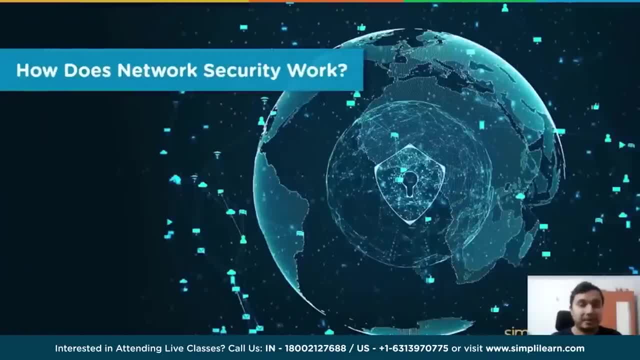 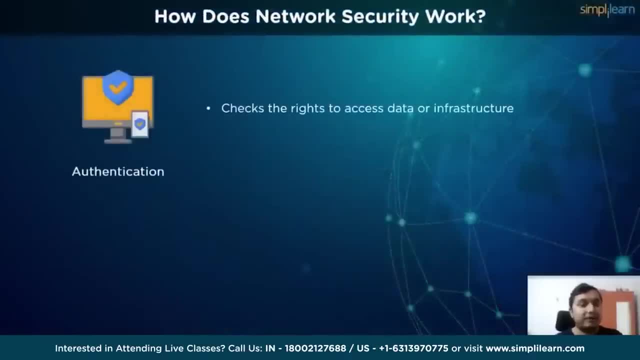 We've now understood the basics of network security, But we need to understand how network security works. in the next section in slightly more detail, Network security revolves around two processes: authentication and authorization. The first process, which is authentication, is similar to access paths which ensure that. 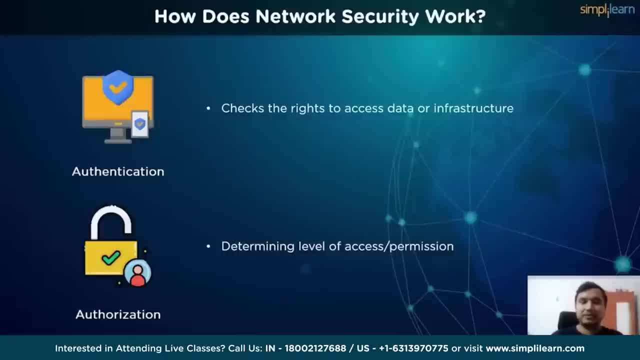 only those who have the right to enter a building. In other words, authentication checks and verifies that it is indeed the user belonging to the network who is trying to access or enter it, thereby preventing unauthorized intruders. Next comes authorization. This process decides the level of access provided to the recently authenticated users. 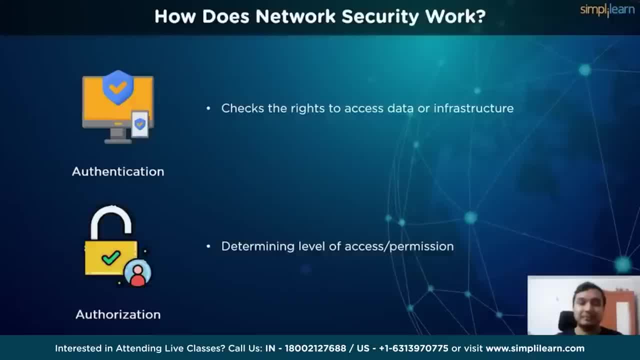 This process is called authentication. This process is called authentication. For example, network admin needs access to the entire network, whereas those working within it probably need access to only certain areas within the network, Based on the network user's role. the process of determining the level of access or permission. 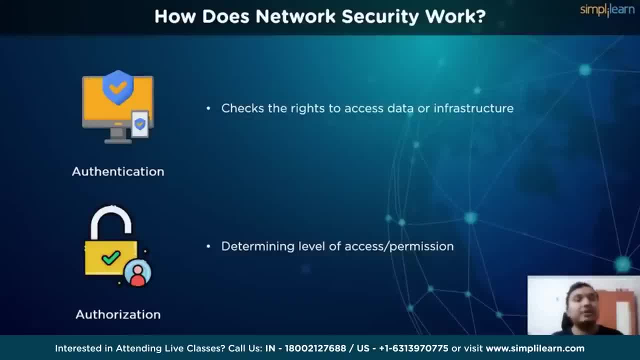 level is known as authorization. Today's network architecture is complex and faces a threat environment that is always changing and attackers that are always trying to find and exploit vulnerabilities. These vulnerabilities can exist in various ways. For example, network security can be used in many areas, including devices, data applications. 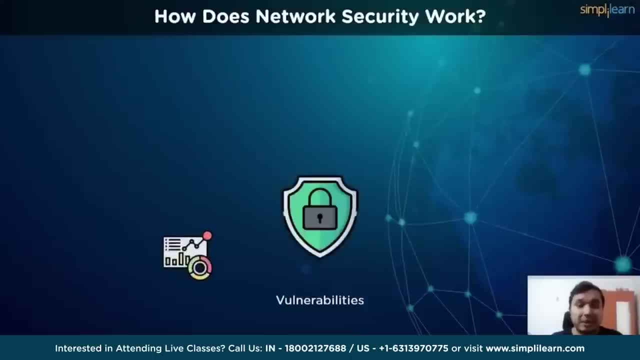 users and applications. For this reason, many network security management tools and applications are in use today that address individual threats. When just a few minutes of downtime can cause widespread disruption and massive damage to an organization's bottom line and reputation, it is essential that these protection measures 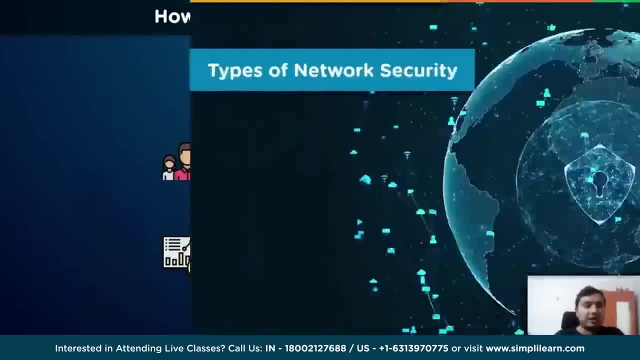 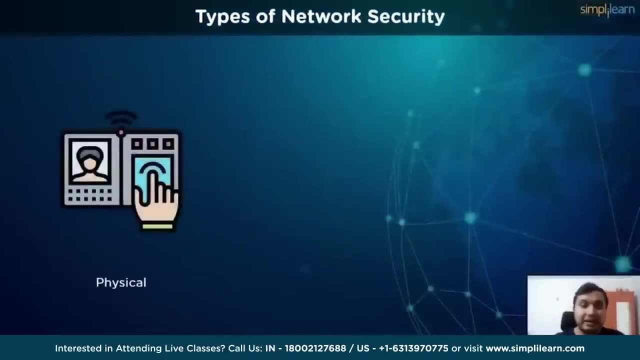 are in place beforehand. Now that we know a little about network security and its working, let's take a look at the next step. Let's cover the different types of network security. The fundamental tenet of network security is the layering of protection for massive 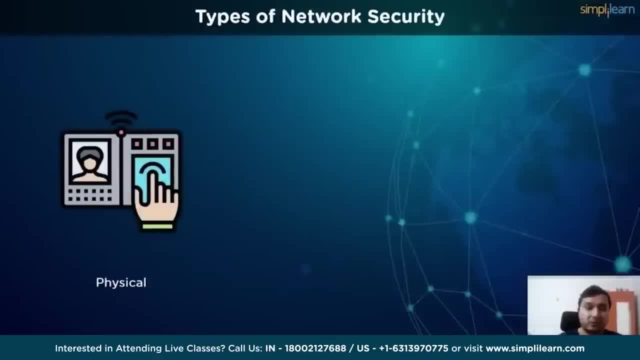 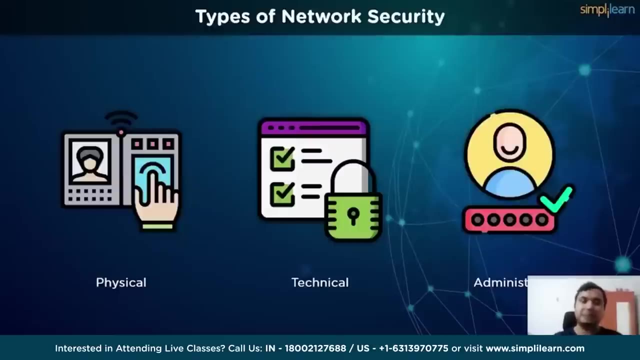 networks and stored data that ensure the acceptance of rules and regulations As a whole. there are three types, the first of which is physical security, the next being technical and the third being administrative. Let's look into physical security first. This is the most basic level. that includes protecting data and network to unauthorized 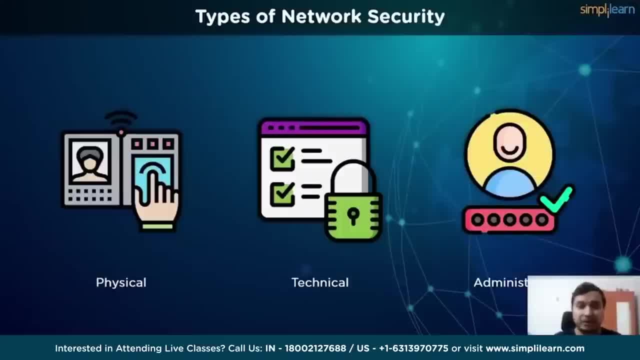 personnel from acquiring and looting. This includes external peripherals and routers that might be used for cable connections. The same can be achieved by using devices like biometric systems. Physical security is critical, especially for small businesses that do not have many resources to devote to security personnel and tools, as opposed to large firms. 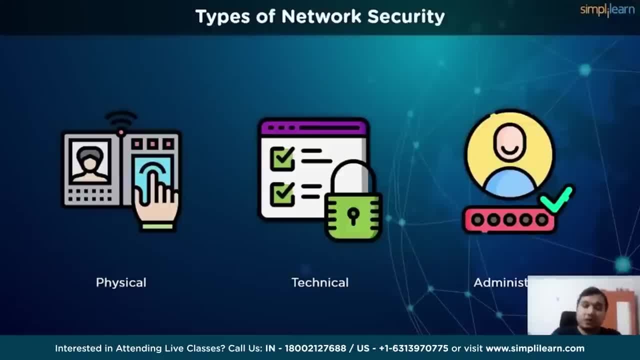 When it comes to technical network security, it focuses mostly on safeguarding data either kept in the network or engaged in network transition. This kind fulfils two functions: One is defense against unauthorized users, The other is a defense against malevolent actions. The last category is administrative. This level of 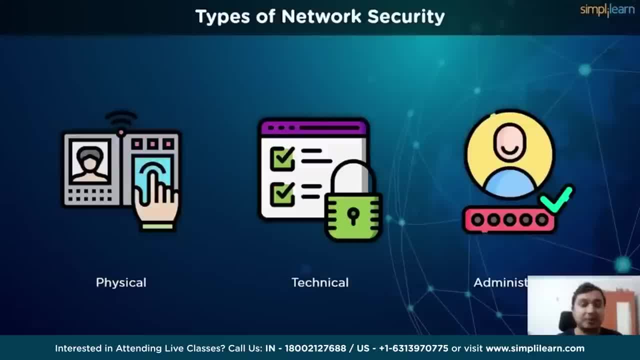 network security protects user behavior, like how the permission has been granted and how the authorization process takes place. This also ensures the level of sophistication the network might need to protect it through all the attacks. This level also suggests necessary amendments that have to be done to the infrastructure. I think that's all the basics that we need to cover on. 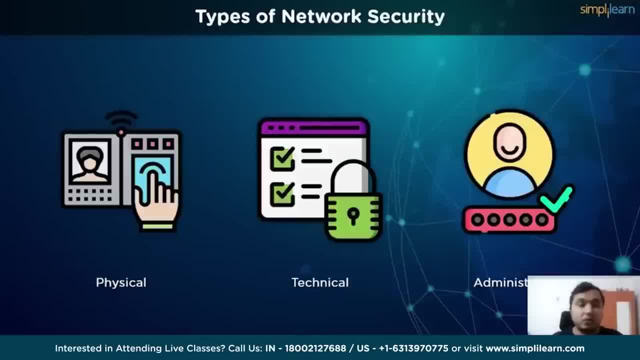 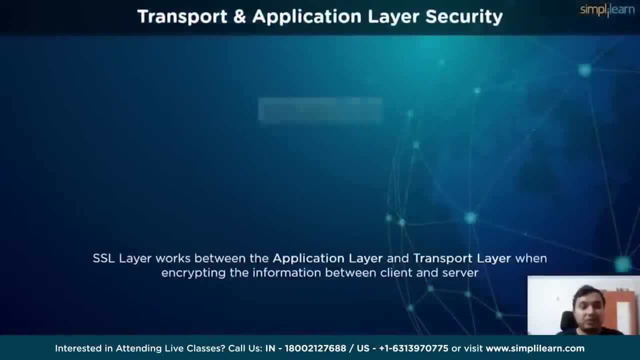 network security, in which our next topic. we're going to go through two mediums of network security, which are the transport layer and the application layer. The transport layer is a way to secure information as it is carried over the internet, with users browsing websites, emails. 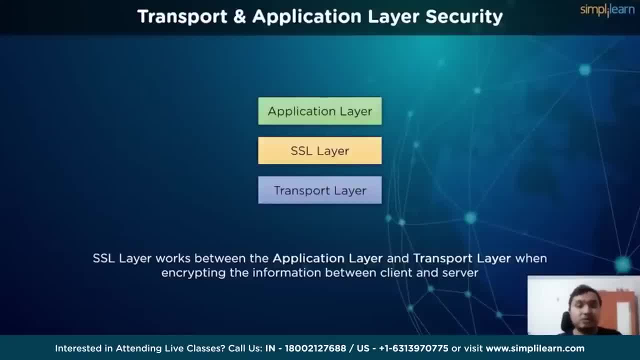 instant messaging, etc. TLS aims to provide a private and secure connection between a web browser and a website server. It does this with the cryptographic handshake between two systems using public key cryptography. The two parties to the connection exchange a secret token and, once each machine validates, 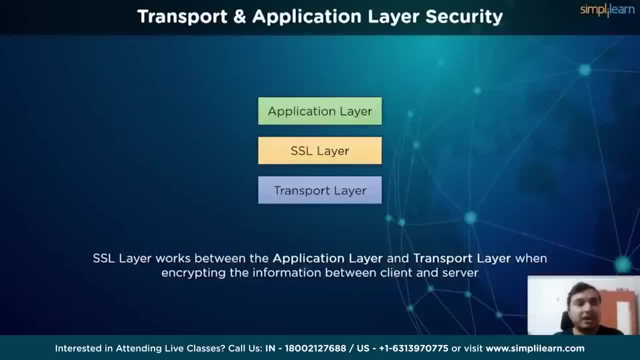 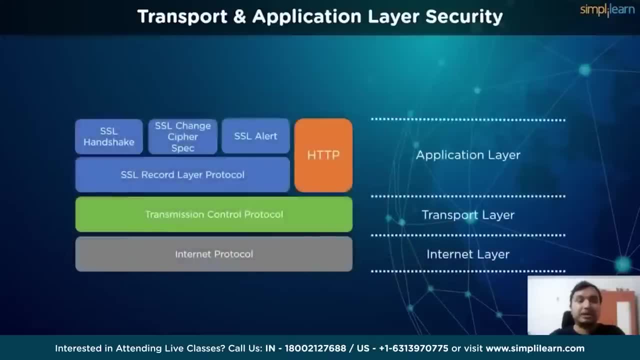 this token, it is used for all communications. The connection employs lighter symmetric cryptography to save bandwidth and processing power. Since the application layer is the closest layer to the end user, it provides hackers with the largest threat surface. Poor app layer security can lead to performance and stability issues. data theft. 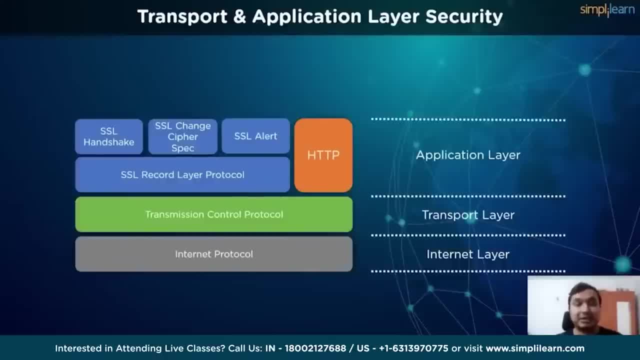 and, in some cases, the network being taken down. Examples of application layer attacks include distributed denial of service attacks or DDoS attacks, HTTP floods, SQL injections, cross-site scripting, etc. Most organizations have an arsenal of application layer security protections to combat these and more, such as web application firewalls, secure web gateway services. 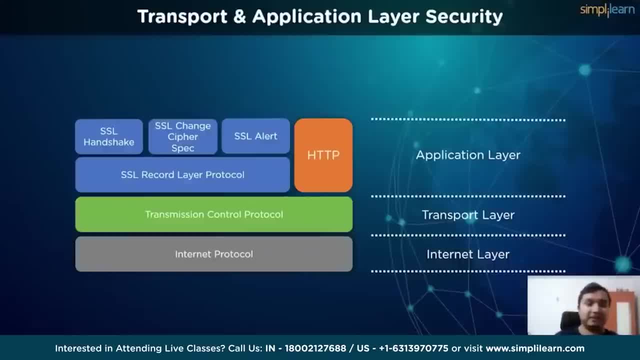 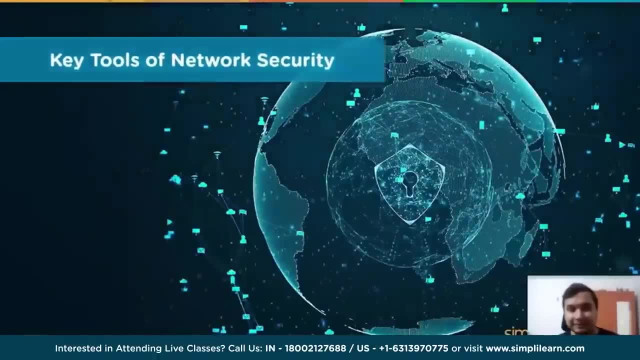 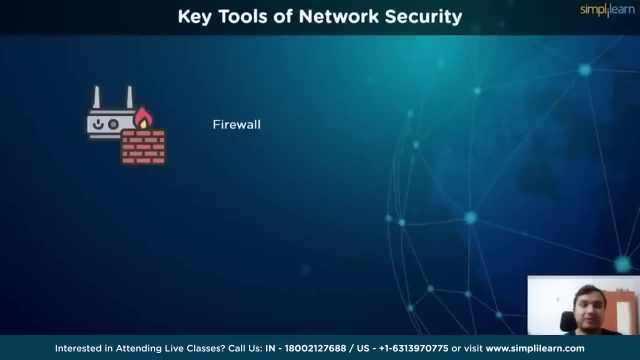 etc. Now that we have the theory behind network security has been covered in detail, let us go through some of the tools that can be used to enforce these network security policies. The first tool to be covered in this section is a firewall. A firewall is a type of network security device that keeps track of incoming and 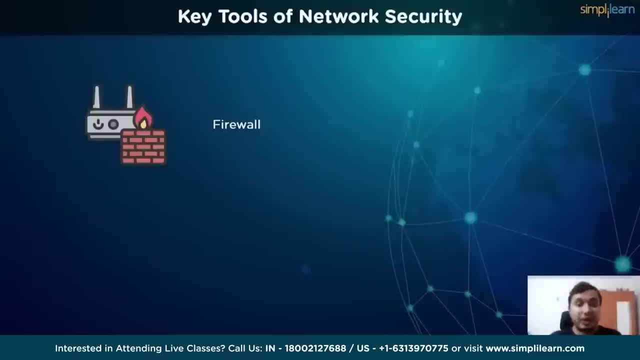 outgoing network traffic and it decides which traffic to allow or deny, in accordance to a set of security rules. For more than 25 years, firewalls have served as network security's first line of defense. They provide a barrier between trustworthy internal, protected and regulated networks from shady external networks like the internet. at some point, 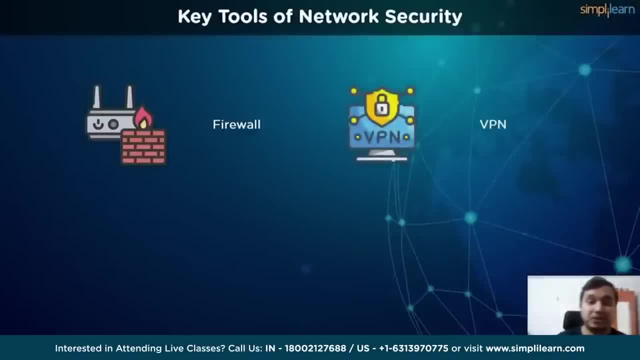 The next tool which can be used to bolster network security is a virtual private network, or VPN for short. It's an encrypted connection between a device and a network via the internet. The encrypted connection aids the secure transmission of sensitive data. It makes it impossible for unauthorized parties to eavesdrop on the traffic. 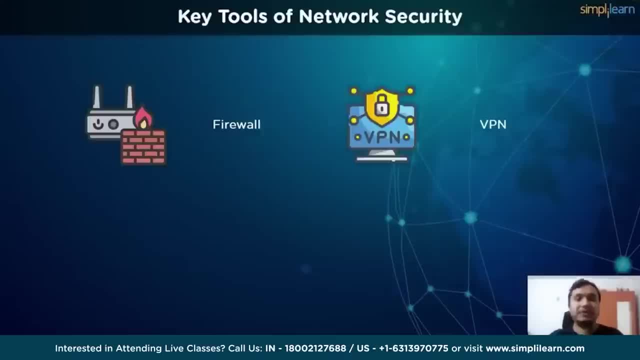 and enables remote work for the user. The usage of VPN technology is common in both corporate and personal networks. Next, we cover the importance of intrusion prevention systems in network security, or IPS frameworks. An intrusion prevention system is a network security tool that continually scans the network for harmful activity. 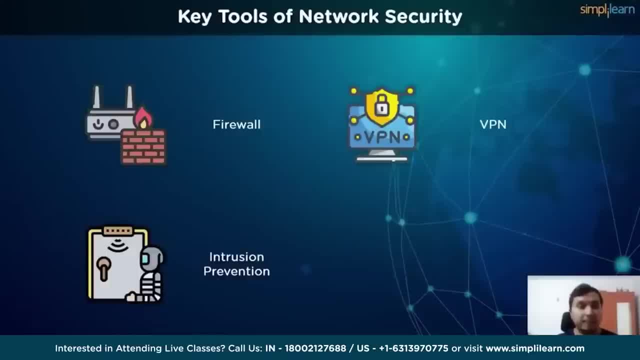 and responds to it when it does occur, by reporting, blocking or discarding it. It can be either hardware or software. It's more sophisticated than an intrusion detection system or an IDS framework which can just warn an administrator and merely identify harmful activities, while in the case of an IPS it actually takes against. 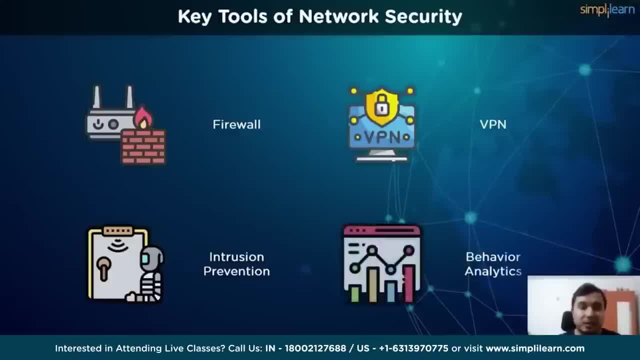 that activity. The next tool in this section, and the final one, are going to be behavioral analytics. Behavioral analytics focus more on the statistics that are being carried over and stored through months and years of usage. Once some kind of similar pattern is noted, where the IT administrator 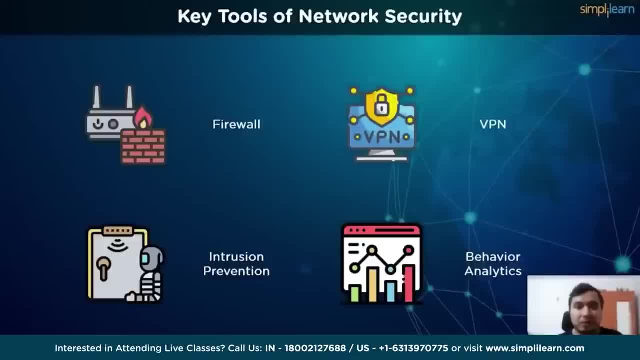 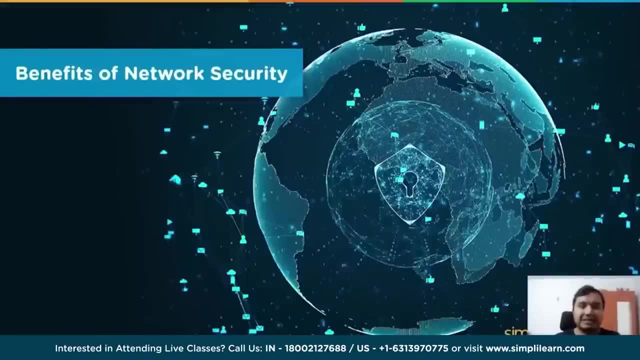 can detect some kind of attack, the similar attacks can be stopped and the security can be further enhanced. Another way: we have covered all that we need to know about network security, the necessary tools, its different types, etc. Let's go to the benefits. 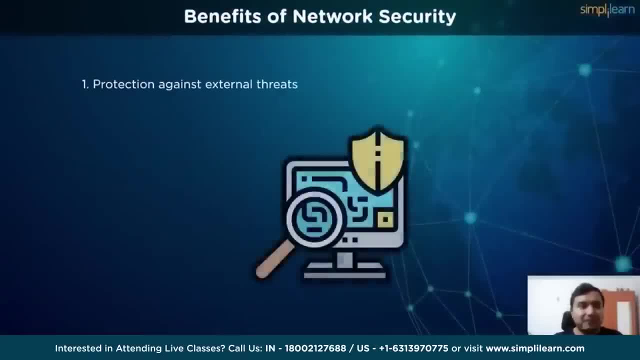 of network security as a whole, The first, which is protection against external threats. The objective for cyber assaults can be as varied as the defenders themselves, Although they are typically initiated for financial gain. whether they are industrial spies, hacktivists or cyber criminals, these bad actors all have one thing in common: 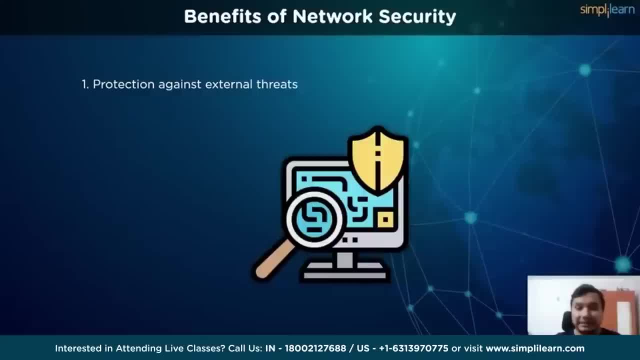 which is how quick, clever and covert the attacks are getting. The most common thing to consider is cyber-attacks, although they are typically initiated for financial gain. Whether they are industrial spies, hacktivists or cyber criminals, these bad actors all have one thing in common, which is how quick, clever and covert their attacks are getting. 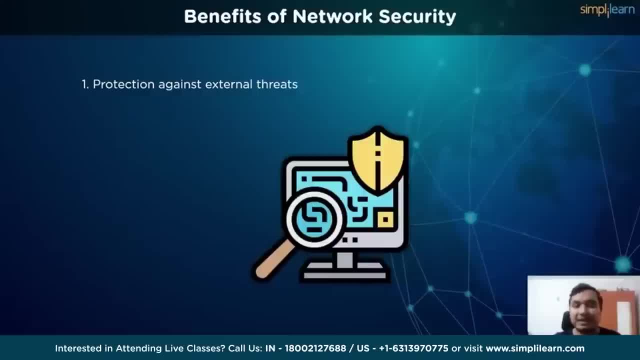 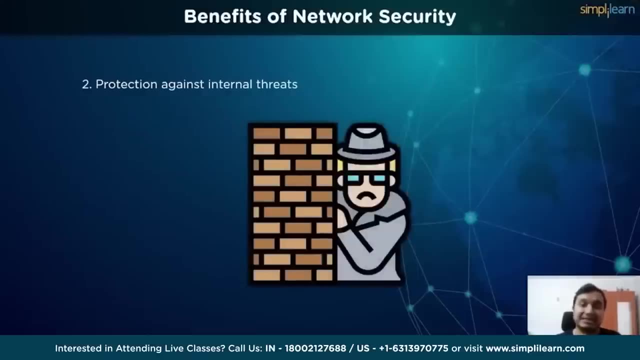 A strong cybersecurity posture that considers routine software updates may assist firms in identifying and responding to the abused techniques, tools and the common entry points. The next benefit is protection against internal threats. The human aspect continues to be the cybersecurity system's weakest link. 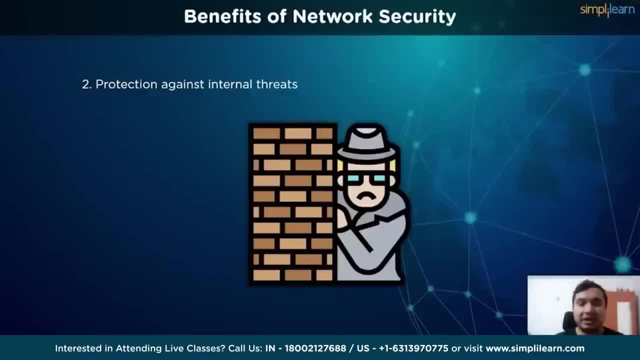 Insider risks can originate from current or former workers, third-party vendors or even trusted partners, and they can be unintentional, careless or downright evil. Aside from that, the rapid expansion of remote work and the personal devices used for business purposes, while even IoT devices in remote locations, can make it easier for these kinds. 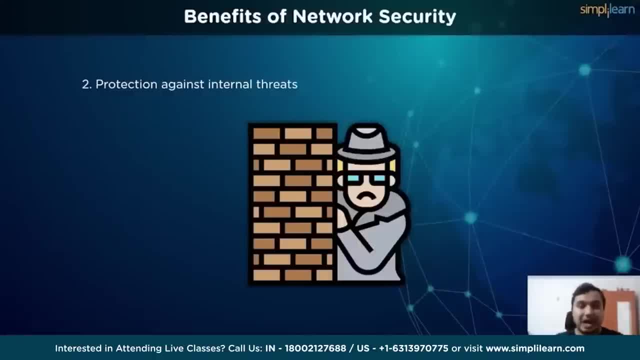 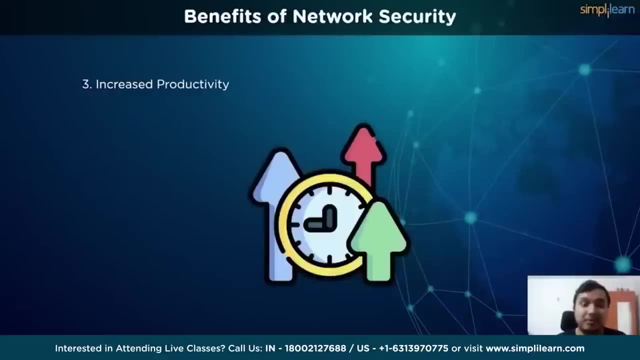 of threats to go undetected until it's too late. However, by proactively monitoring networks and managing access, these dangers may be identified and dealt with before they become expensive disasters. The third benefit is increased productivity. It is nearly impossible for employees to function when networks and personal devices are not 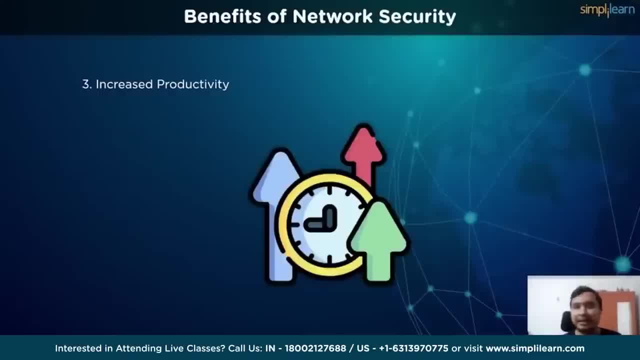 available. It is also impossible for the company to run. You may significantly minimize violations and the amount of downtime required to fix the breach by implementing various cybersecurity measures, such as enhanced firewalls, virus scanning and automatic backups, Employee identification of possible email phishing schemes, suspicious links and other. 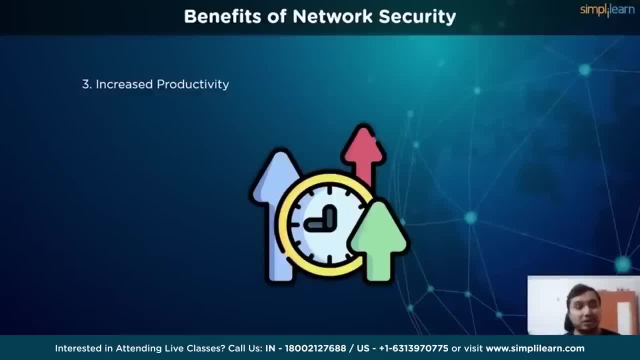 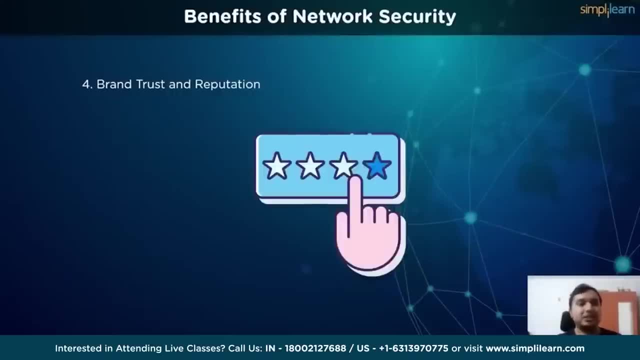 malicious criminal activities can also be aided by education and training. 4. Another benefit is brand trust and reputation. Customer retention is one of the most crucial elements in business development. Customers today pace a premium on maintaining brand loyalty through a strong cybersecurity stance, since this is the fastest way to get other businesses back, get referrals and 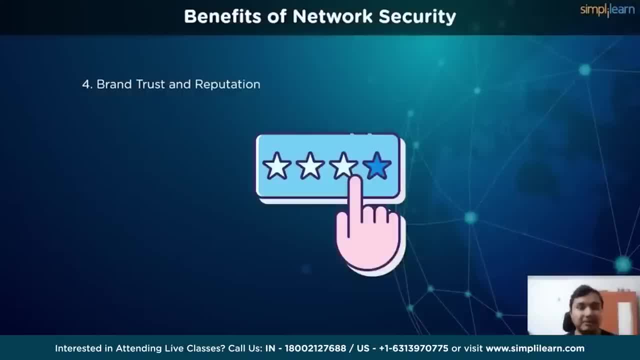 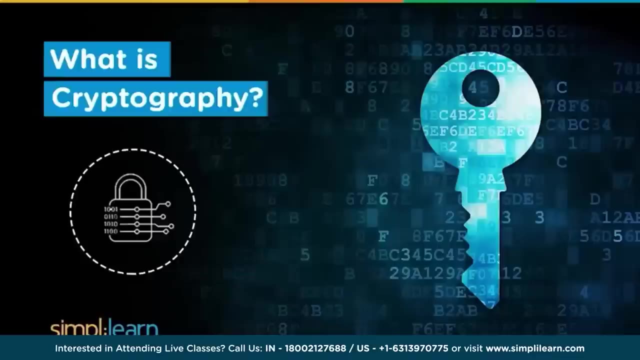 sell more tickets overall. Additionally, it helps manufacturers get on the vendor list with bigger companies as a part of their supply chain, which is only as strong as its weakest link. 5. Possibilities for potential future endeavors and development. With the rise in censorship and general fear over privacy loss, consumer security is at 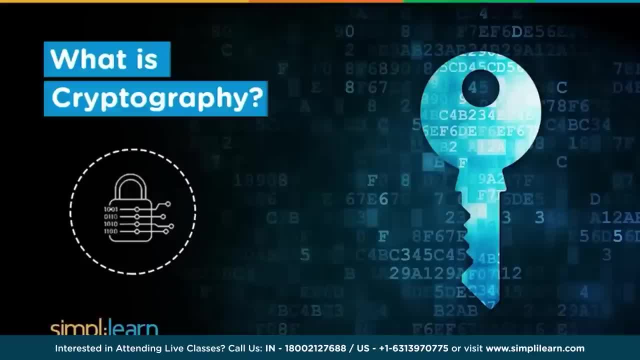 an all-time high risk. Technology has made our lives so much easier. while putting up a decent target on our personal information, It is necessary to understand how to simultaneously safeguard our data and be up to date with the latest technological developments. Maintaining this balance has become easier with cryptography taking its place in today's 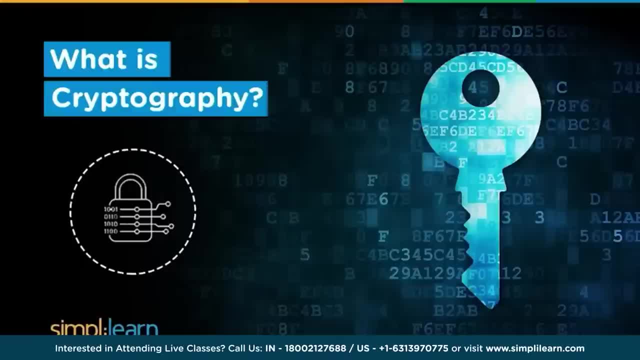 digital world. So hey everyone, this is Bhavab from Simply Learn, and welcome to this video on cryptography. But before we begin, if you love watching tech videos, subscribe to our channel and hit the bell icon to never miss an update from Simply Learn. 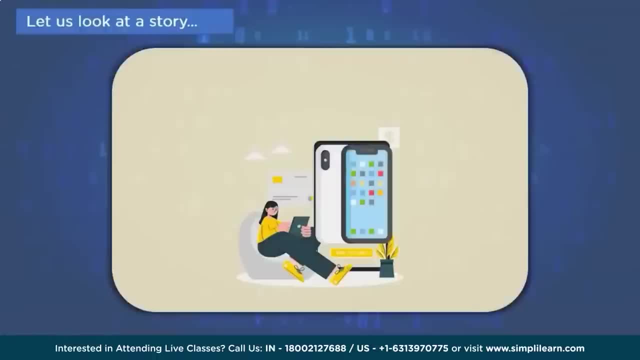 So here's a story to help you understand cryptography. Meet Ann. Ann wanted to look for a decent discount on the latest iPhone. She started searching on the internet and found a rather shady website that offered a 50% discount on the first purchase. 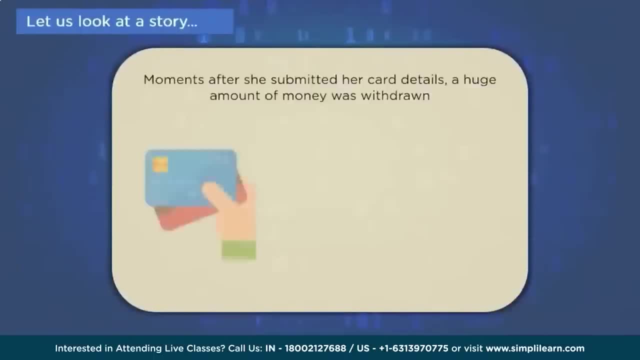 This was the first time she'd seen a 50% discount on the first purchase. Once Ann submitted her payment details, a huge chunk of money was withdrawn from her bank account. just moments after, Devastated, Ann quickly realized she had failed to notice that the website was an HTTP webpage. 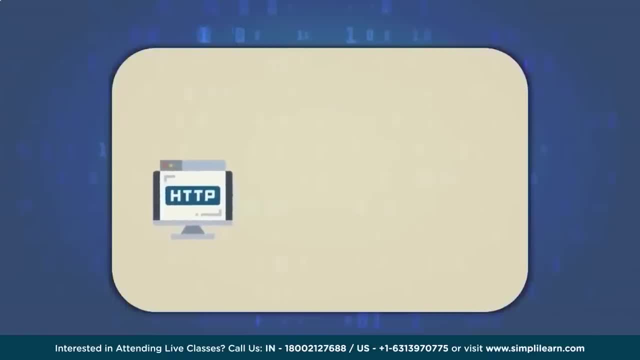 instead of an HTTPS one. The payment information submitted was not encrypted and it was visible to anyone keeping an eye, including the website owner and hackers. Had she used a reputed website which has encrypted transactions and employs cryptography, arrived at the site, the phone enthusiast could have avoided this particular incident. 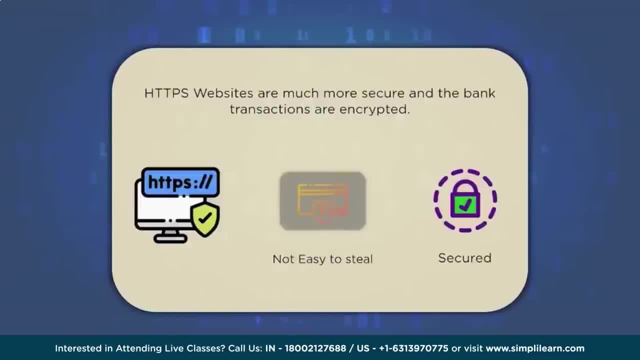 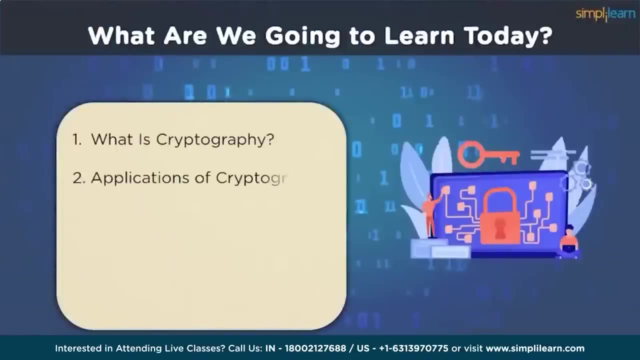 This is why it's never recommended to visit unknown websites or share any personal information on them. Now that we understand why cryptography is so important, let's take a look at the topics to be covered today. We take a look into what cryptography is and how it works. 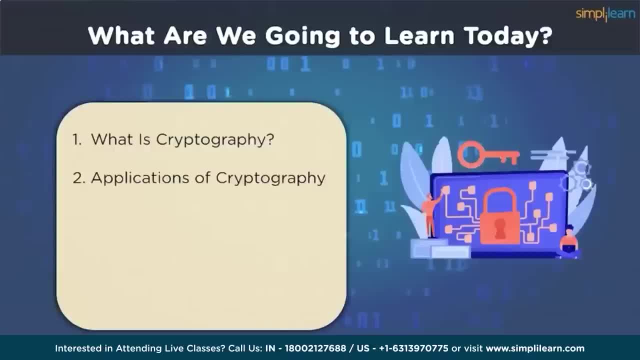 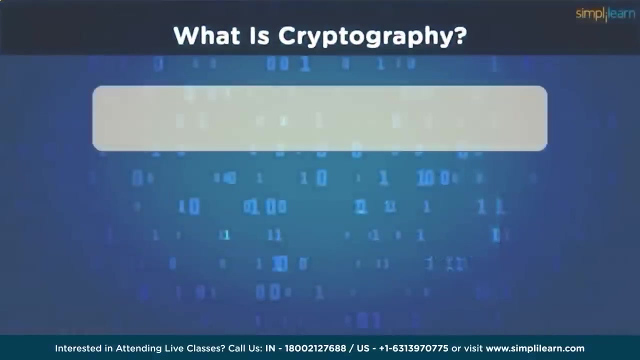 We learn where cryptography is being used in our daily lives and how we are benefiting from it, Then we will understand the different types of cryptography and the benefits of cryptography. Let's get started. 1. Cryptography is the science of encrypting or decrypting information to prevent unauthorized 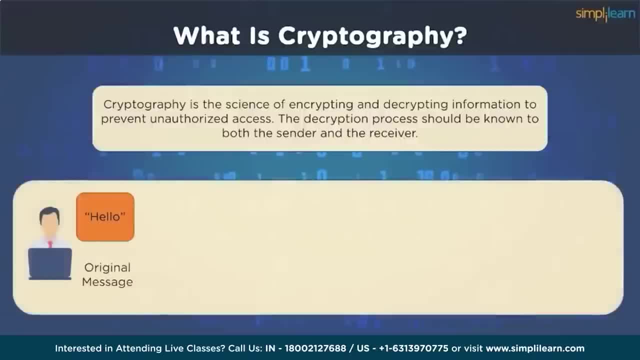 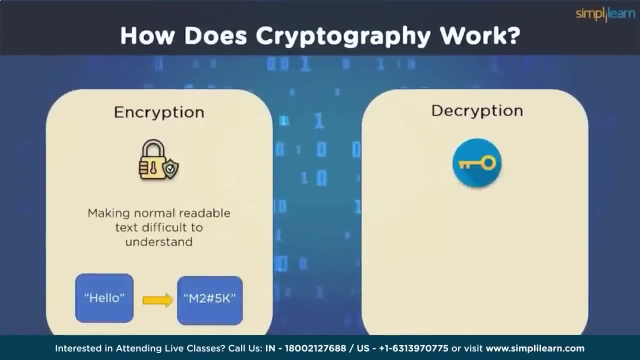 access. We transform our data and personal information so that only the correct recipient can understand the message. 2. Encryption is another aspect of modern data security. Using cryptography allows the secure storage and transmission of data between willing parties. Encryption is the primary route for employing cryptography by adding certain algorithms. 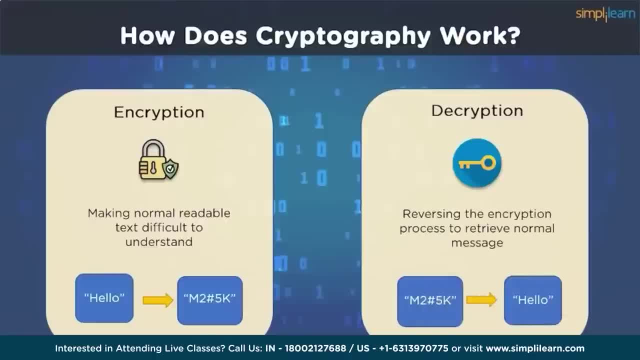 to jumble up the data. Decryption is the process of reversing the work done by encrypting information so that the data becomes readable again. Both of these methods form the basis of cryptography. For example, when Simply Learn is jumbled up or changed in any format, the data becomes. 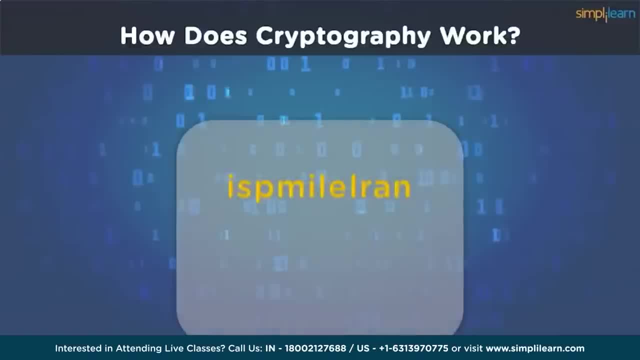 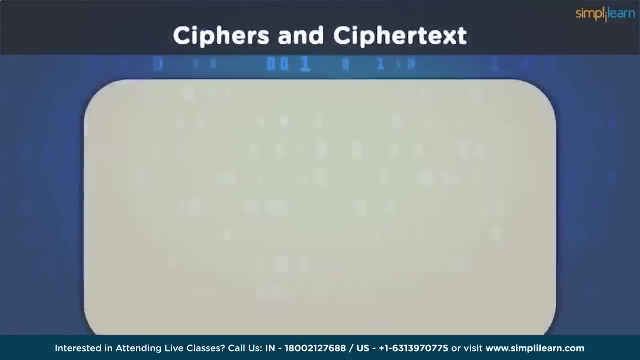 readable again In the same format. not many people can guess the original word by looking at the encrypted text. The only ones who can are the people who know how to decrypt the coded word, thereby reversing the process of encryption. Any data pre-encryption is called plain text or clear text. 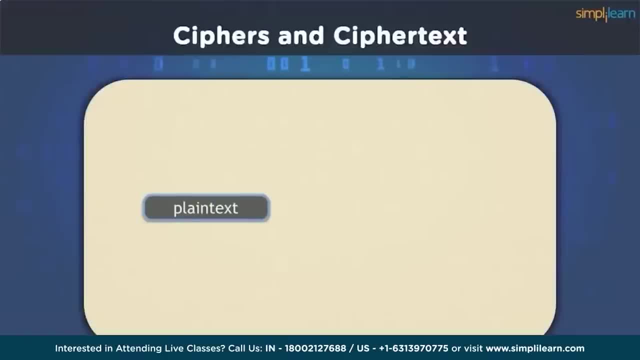 To encrypt the message. we use certain algorithms that serve a single purpose of scrambling the data to make them unreadable without the necessary tools. These algorithms are called ciphers. They are a set of detailed steps to be carried out, one after the other, to make sure the data 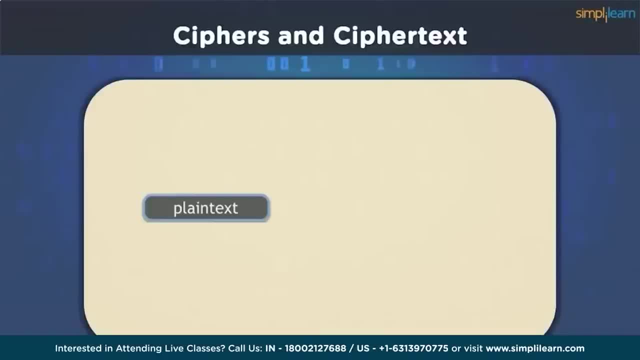 becomes as unreadable as possible until it reaches the receiver. We take the plain text, pass it to the cipher algorithm and get the encrypted data. This encrypted text is called the ciphertext, and this is the message that is transferred between the two parties. 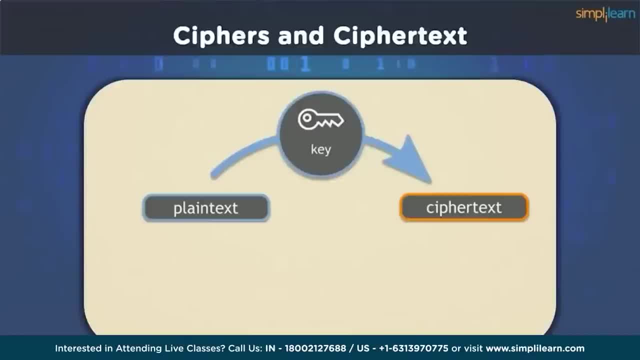 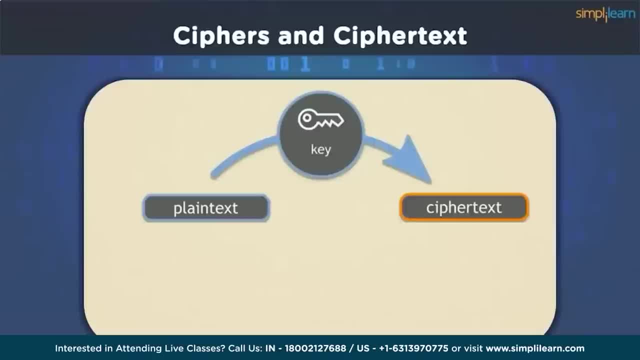 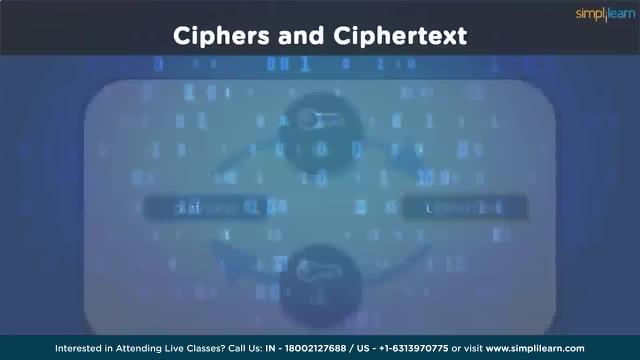 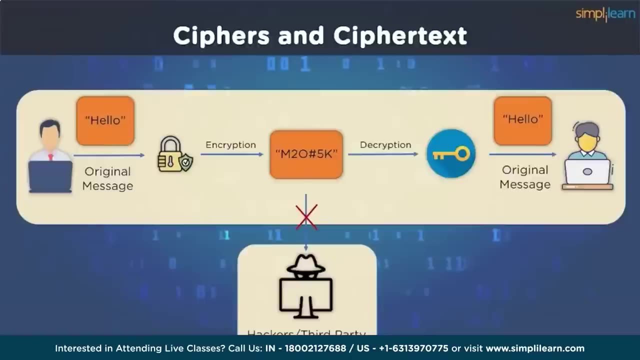 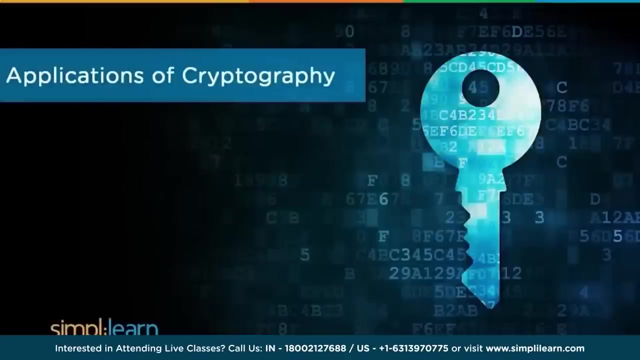 on receiving the message. Unless any third party manages to find out both the algorithm and the secret key that is being used, they cannot decrypt the messages, since both of them are necessary to unlock the hidden content. Wonder what else we would lose if not for cryptography. 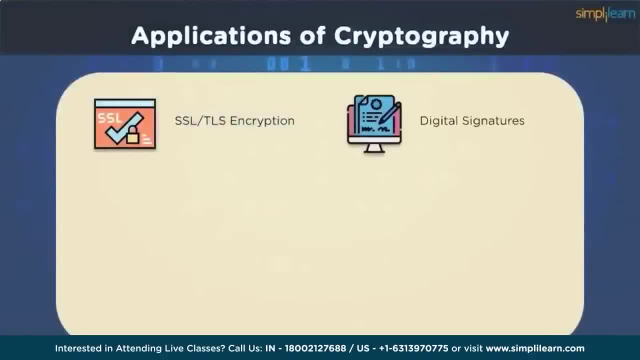 Any website where you have an account can read your passwords, Important emails can be intercepted and their contents can be read without encryption during the transit. more than 65 billion messages are sent on whatsapp every day, all of which are secured thanks to end-to-end encryption. there is a huge market opening up for 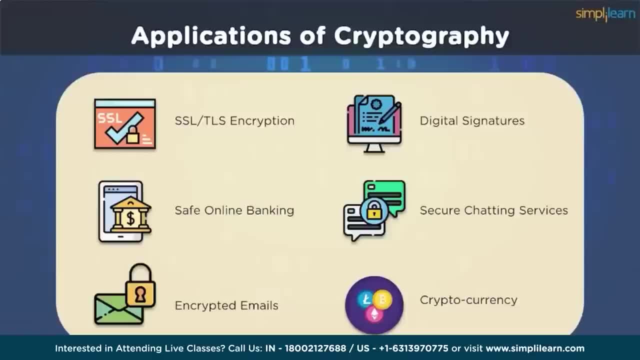 cryptocurrency, which is possible due to blockchain technology that uses encryption algorithms and hashing functions to ensure that the data is secure. if this is of particular interest to you, you can watch our video on blockchain, the link of which will be in the description. of course, there is no. 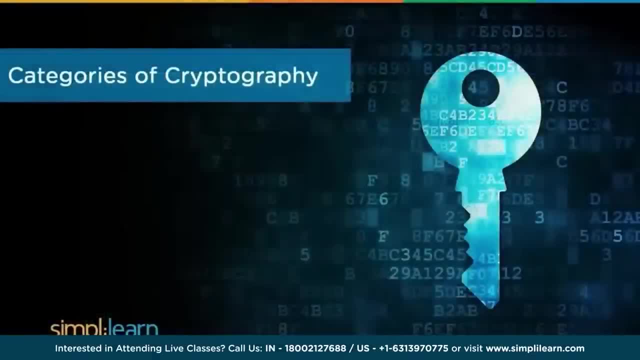 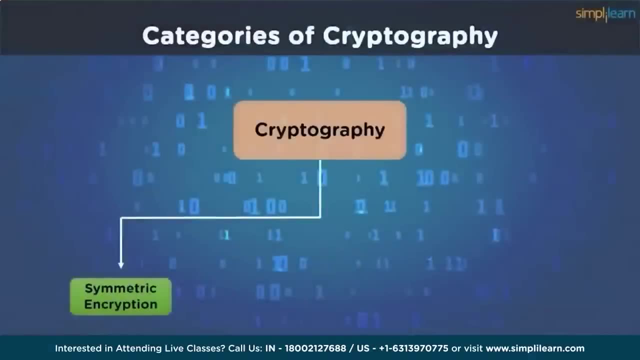 single solution to a problem as diverse. as explained, there are three variants of how cryptography works and is in practice. they are symmetric encryption, asymmetric encryption and hashing. let's find out how much we have understood until now. do you remember the difference between a cipher and ciphertext? leave 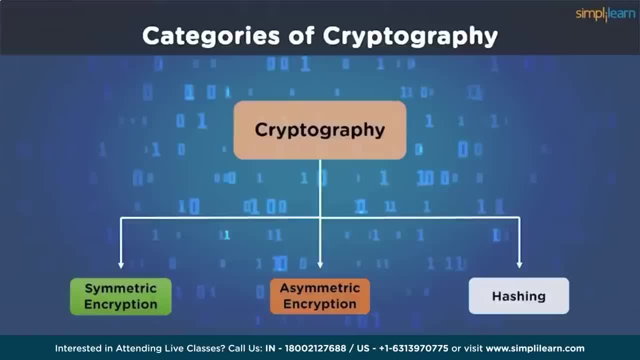 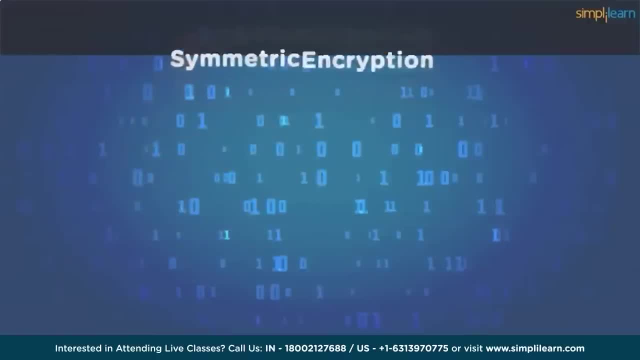 your answers in the comments and before we proceed. if you have found this video helpful, please like, share and subscribe to our channel. if you find this video interesting, make sure to give it a thumbs up before moving ahead. let's look at symmetric encryption first. symmetric encryption uses a single 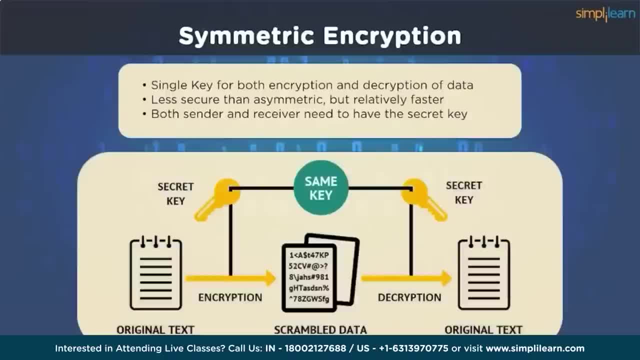 key for both the encryption and decryption of data. it is comparatively less secure than asymmetric encryption, but much faster. it is a compromise that has to be embraced in order to deliver data as fast as possible without leaving information completely vulnerable. this type of encryption is used when data 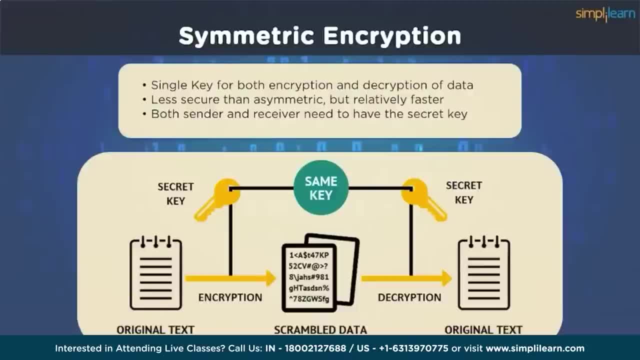 rests on servers and identifies personnel for payment applications and services. the potential drawback with symmetric encryption is that both the sender and receiver need to have the same secret key and it should be kept hidden at all times. Caesar cipher Enigma machine are both symmetric encryption examples that we will look into further. for example, if Alice wants to send a, 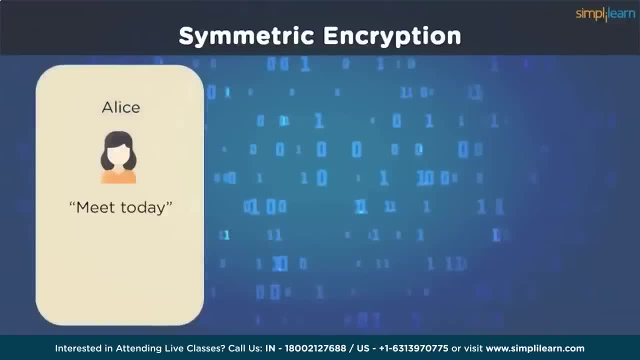 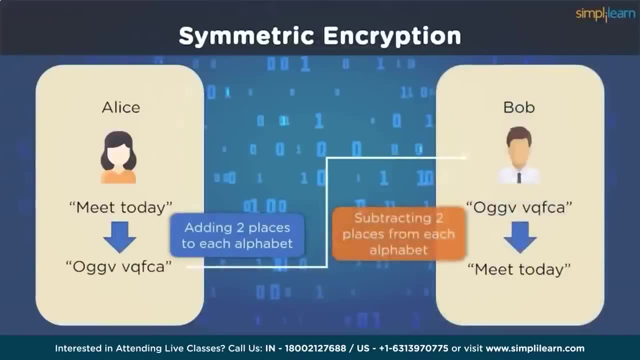 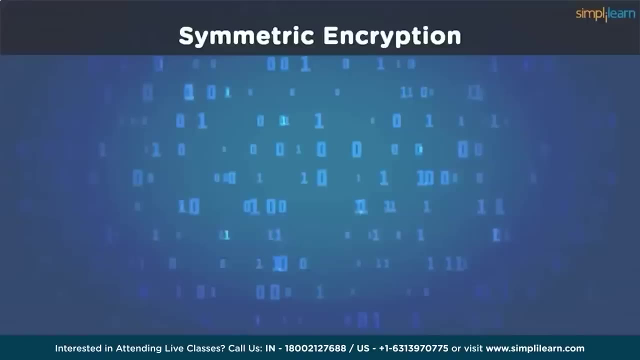 message to Bob. she can apply a substitution cipher or a shift cipher to encrypt the message, But Bob must be aware of the same key itself so he can decrypt it when he finds it necessary to read the entire message. Symmetric encryption uses one of the two types of ciphers: stream ciphers and block ciphers. 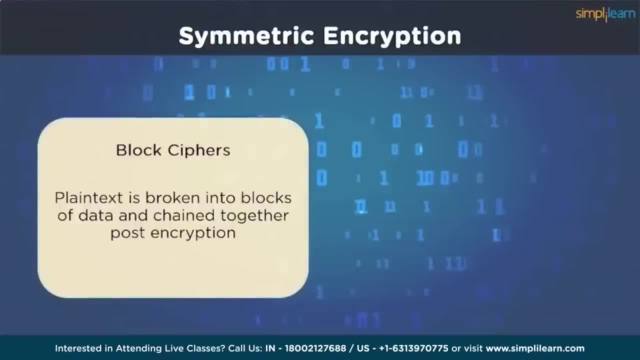 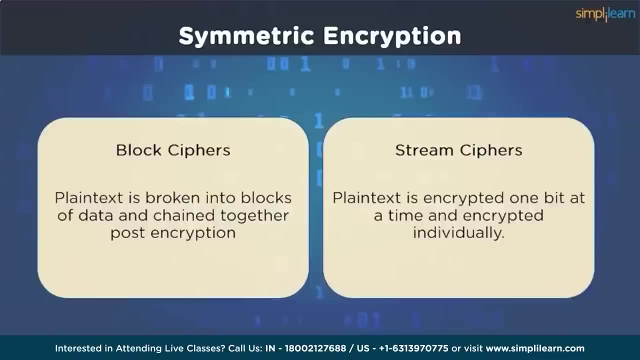 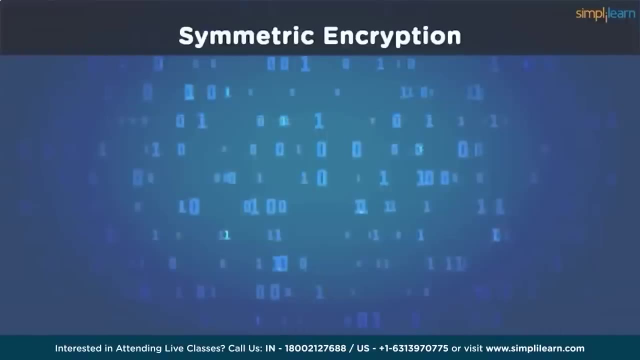 Block ciphers break the plaintext into blocks of fixed size and use the key to convert it into ciphertext. Stream ciphers convert the plaintext into ciphertext one bit at a time, instead of resorting to breaking them up into bigger chunks. In today's world, the most widely used symmetric encryption algorithm is AES-256. that stands: 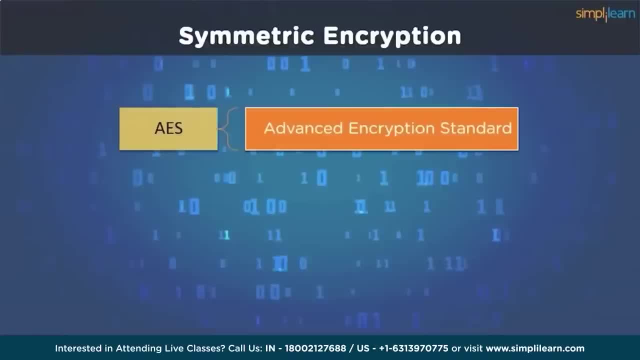 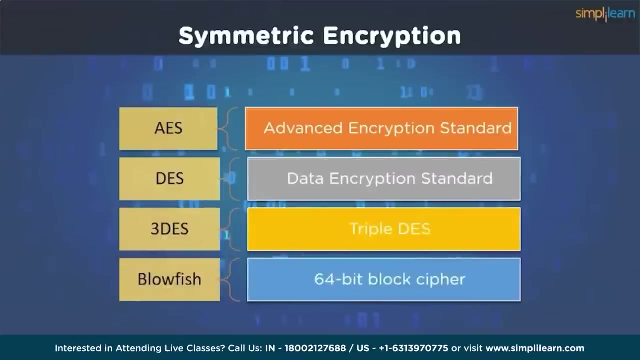 for Advanced Encryption Standard, which has a key size of 256-bit, with 128-bit and 196-bit key sizes also being available. Other primitive algorithms like the Data Encryption Standard that is, the DES, the Triple Data Encryption Standard, 3DES and Blowfish, have all fallen out of favor due to the rise of. 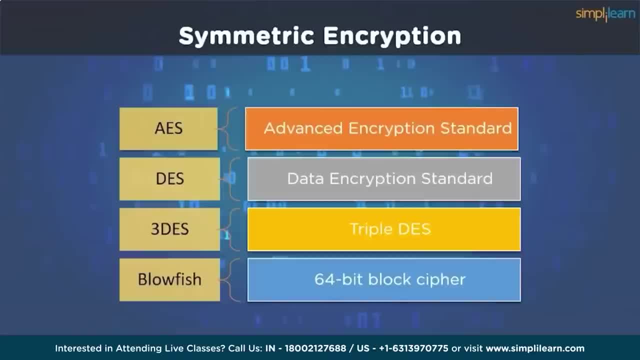 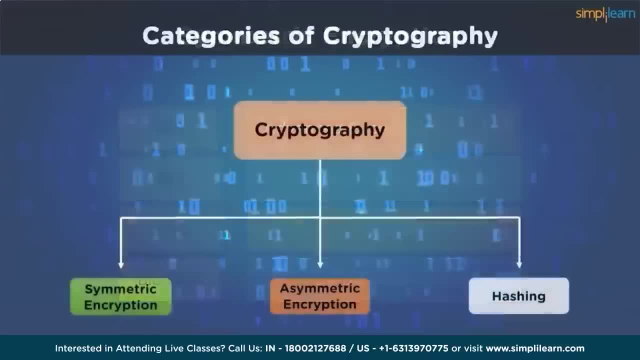 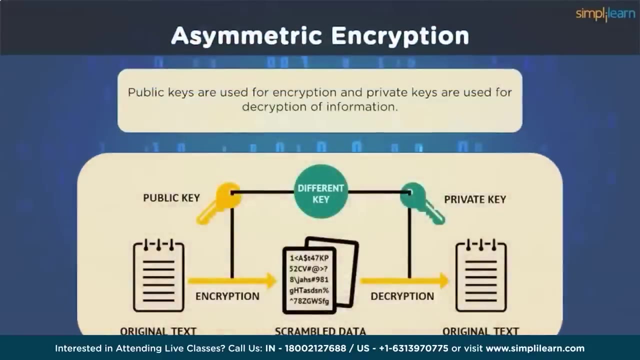 AES. AES chops up the data into blocks. It performs 10-plus rounds of obscuring and substituting the message to make it unreadable. Asymmetric encryption, on the other hand, has a double whammy at its disposal. There are two different keys at play here: a public key and a private key. 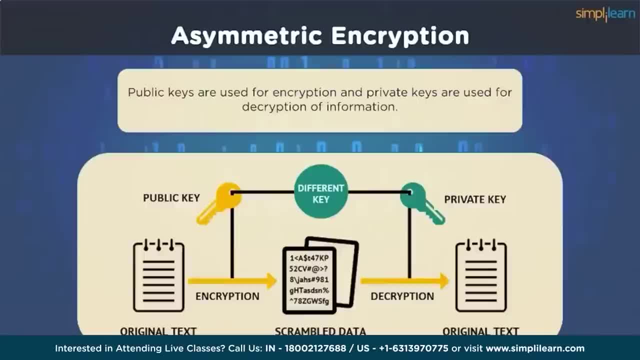 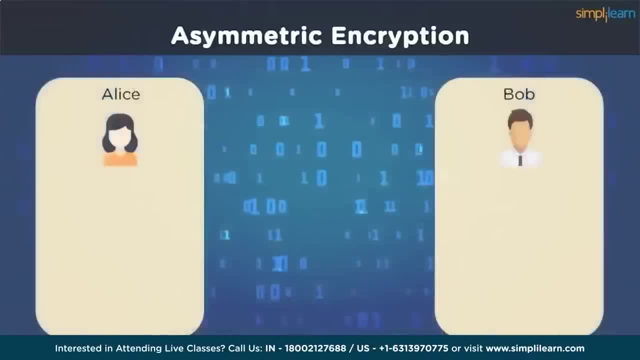 The public key is used to encrypt information pre-transit and a private key is used to decrypt the information post-transit. If Alice wants to communicate with Bob using asymmetric encryption, She encrypts the message using Bob's public key. After receiving the message, Bob uses his own private key to decrypt the data. 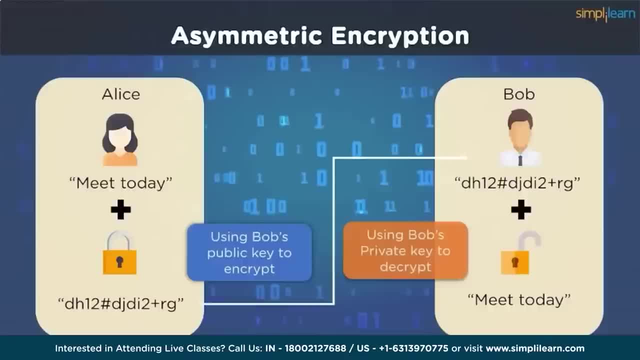 This way, nobody can intercept the message in between transmissions and there is no need for any secure key exchange for this to work, since the encryption is done with the public key and the decryption is done with the private key that no one except Bob has access to. 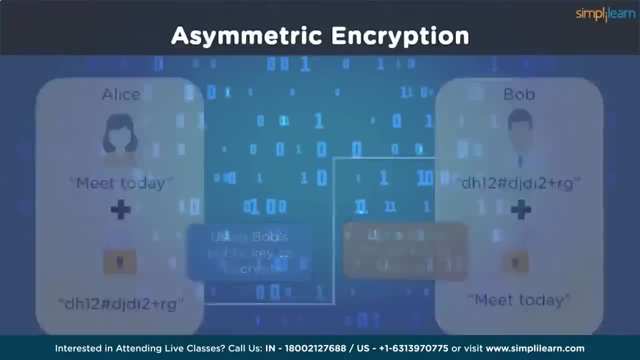 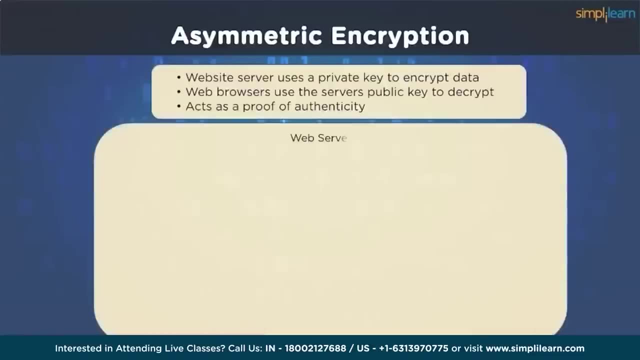 Both the keys are necessary to read the full message. There is also a reverse scenario, where we can use the private key. A server can sign non-confidential information using its private key and anyone who has its public key can decrypt the message. This mechanism also proves that the sender is authenticated and there is no problem with. 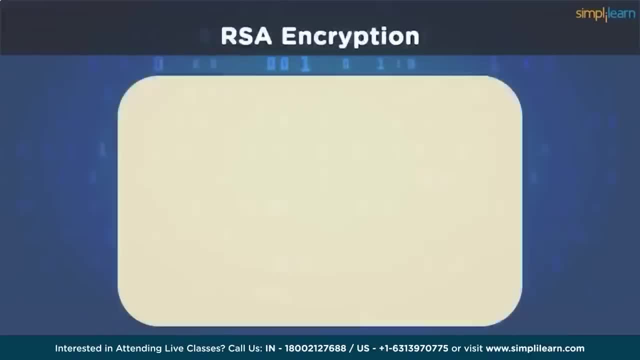 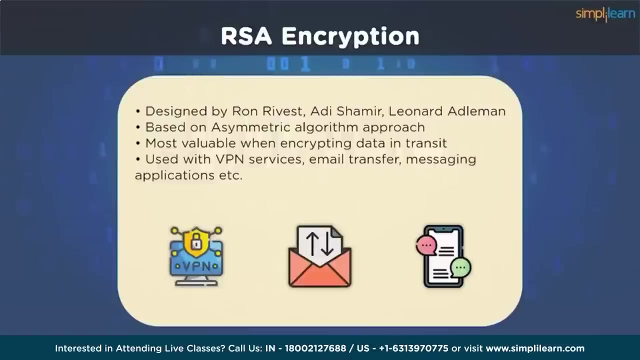 the origin of the information. RSA encryption is the most widely used asymmetric encryption standard. It is named after its founders, Rivest, Shamir and Edelman, And it uses block ciphers. They separate the data into blocks and obscure the information. 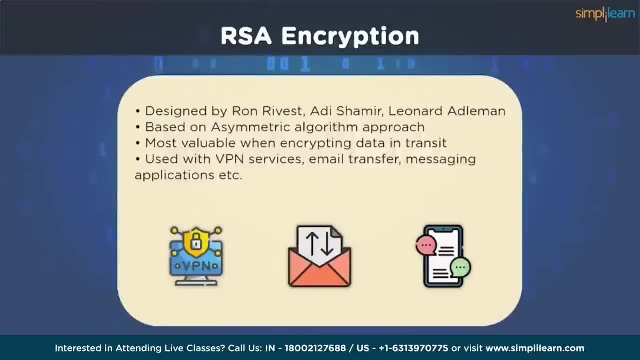 Widely considered the most secure form of encryption, albeit relatively slower than AES. it is widely used in web browsing, secure identification, VPNs, emails and chat applications. With so much hanging on the keys' secrecy, there must be a way to transmit the keys without 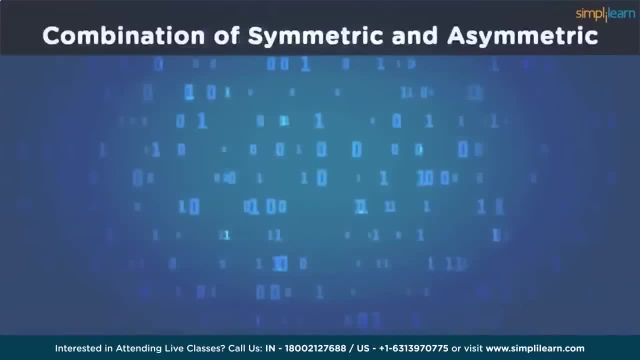 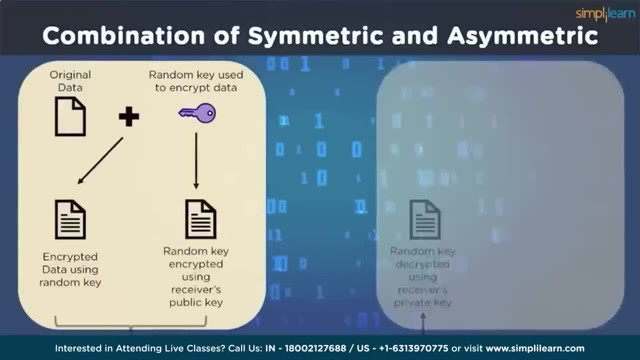 others reading our private data. Many systems use a combination of symmetric encryption and asymmetric encryption to bolster security and match speed. at the same time, Since asymmetric encryption takes longer to decrypt large amounts of data, the full information is encrypted using a single key, ie symmetric encryption. 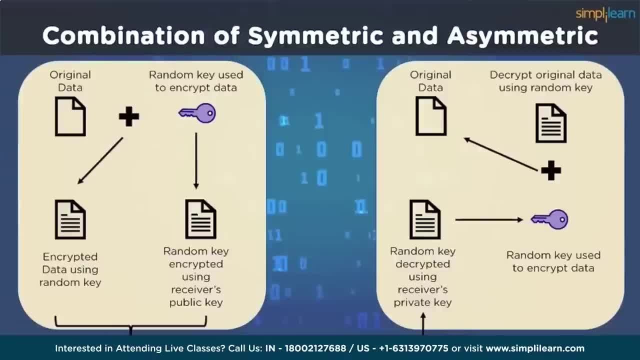 That single key is then transmitted to the receiver using asymmetric encryption, so you don't have to compromise either way. Another route is using the Diffie-Hellman key exchange, which relies on a one-way function and is much tougher to break into. 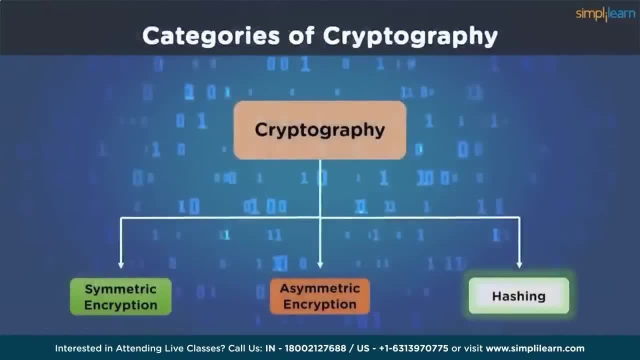 The third variant of cryptography is terminology. The third variant of cryptography is terminology. The third variant of cryptography is terminology. These are the words used for text: Search engine hashing, Diffie-Hellman key exchange: hashing is the process of scrambling a piece of data beyond. 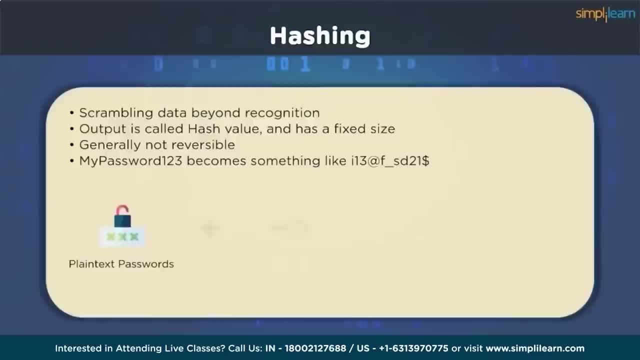 recognition, such as onlynychto- linking words together. Users can display the duration of research services and still create the same information based on types of data used to make the search method. It gives an output of fixed size, which is known as the hash value of the original data. 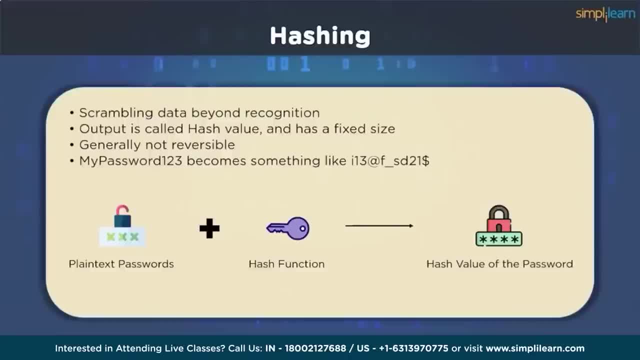 or just hash in general, The calculations that do the job of messing up the data collection form, the hash function. They are generally not reversible without resilient brute force mechanisms and are very helpful when storing data on website servers that need not be stored in plain text. 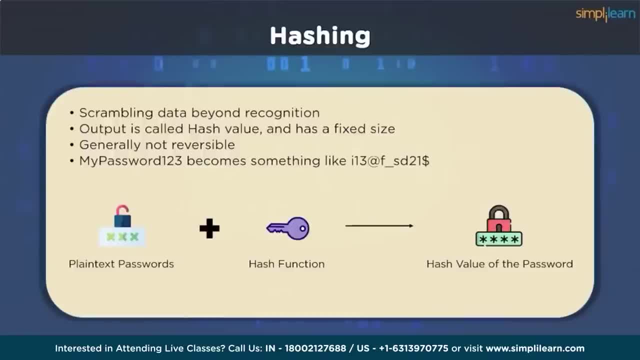 For example, many websites store your account passwords in a hashed format, so that not even the administrator can read your credentials. When a user tries to log in, they can compare the entered password's hash value with the hash value that is already stored on the servers for authentication. since the function will 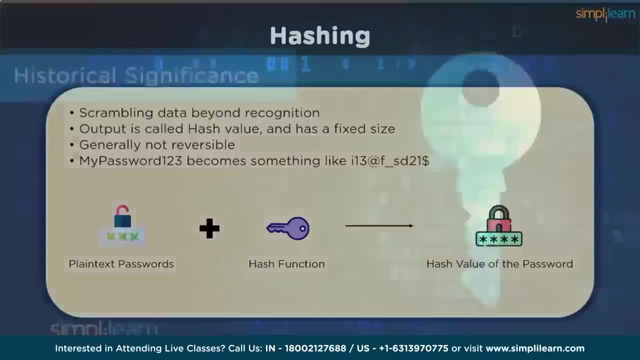 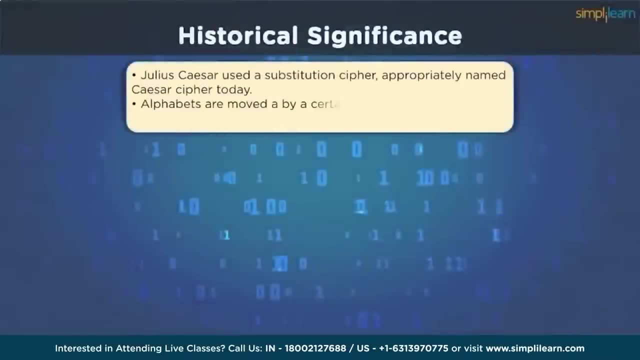 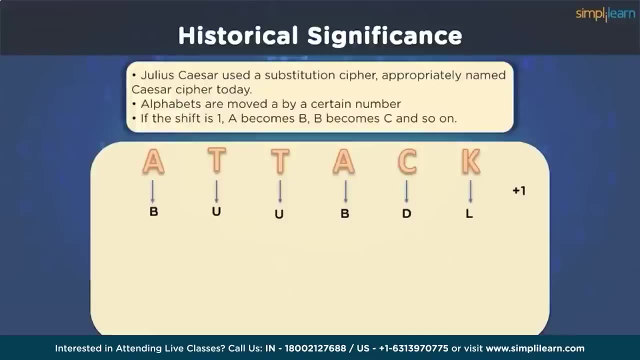 always return the same value for the same input. Cryptography has been in practice for centuries. Julius Caesar used a substitution shift to move alphabets a certain number of spaces beyond their place in the alphabet table. A spy can't decipher the original message at first glance. 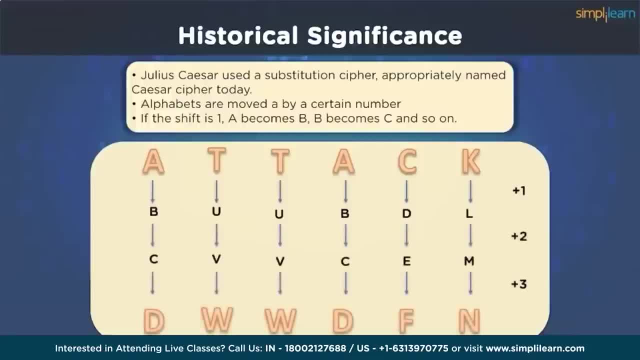 For example, if he wanted to pass confidential information to his armies and decides to use the substitution shift of plus 2, A becomes C, B becomes D, and so on. The word attack, when passed through a substitution shift of plus 3, becomes DWWDEFN. 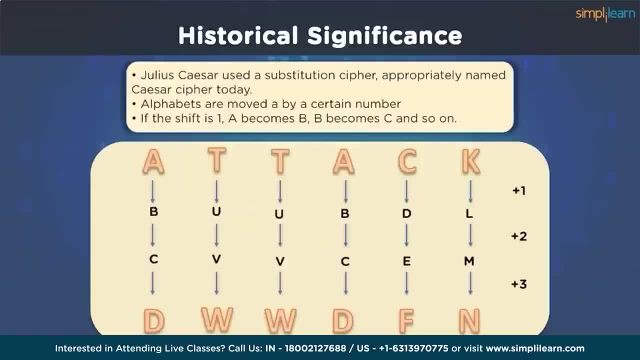 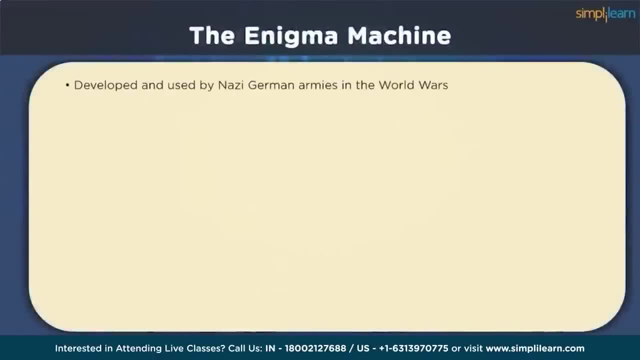 This cipher has been appropriately named the Caesar cipher, which is one of the most widely used algorithms. The Enigma is probably the most famous cryptographic cipher device used in ancient history. It was used by the Nazi German armies in the world wars. They were used to protect confidential political, military and administrative information, and 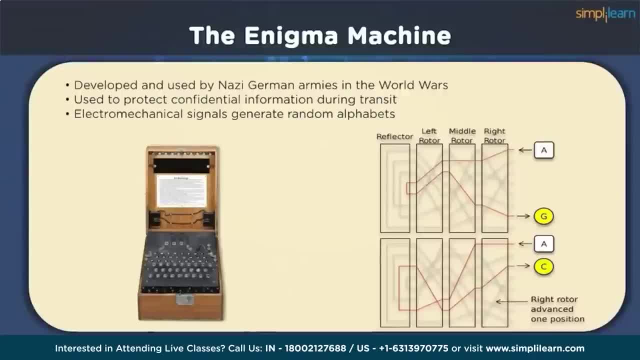 it consisted of 3 or more rotors that scrambled the original message, depending on the machine's state at that time. The decryption is similar, but it needs both machines to stay in the same state before passing the cipher text so that we receive the same plain text message. 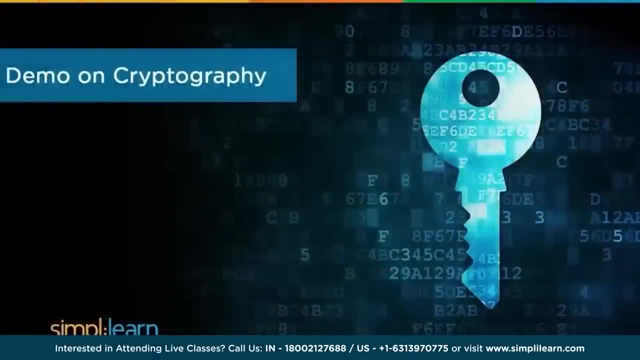 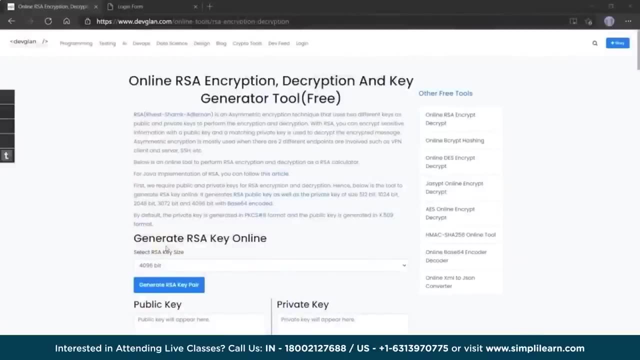 Let's take a look at how our data is protected while we browse the internet thanks to cryptography. Here we have a web-based tool that will help us understand the process of RSA encryption. We see the entire workflow, from selecting the key size to be used until the decryption. 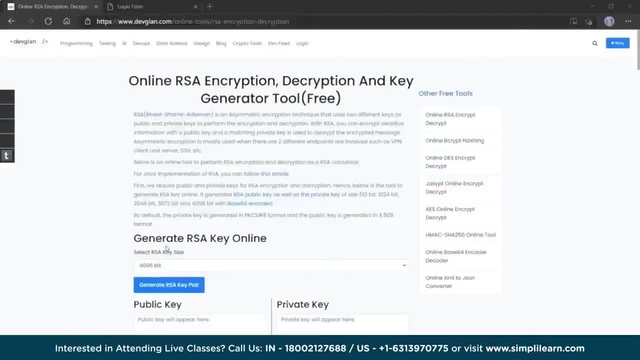 of the cipher text in order to get the plain text back. As we already know, RSA encryption algorithm falls under the umbrella of asymmetric key cryptography. That basically implies that we have two keys at play here, a public key and a private key. Typically, the public key is used by the sender to encrypt the message, and the private key 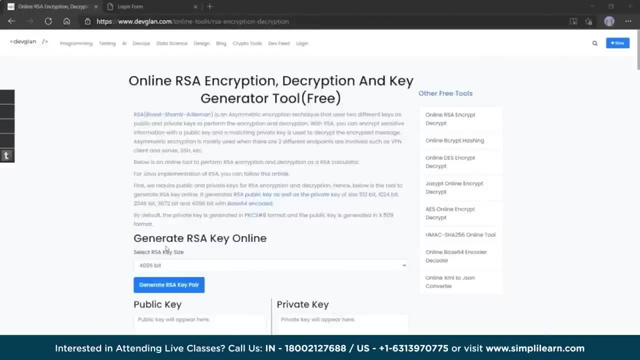 is used by the receiver to decrypt the message. There are some occasions when this allocation is reversed, and we will have a look at them as well. In RSA, we have the choice of key size. We can select any key from a 512-bit to 1024-bit, all the way up to a 4096-bit key. 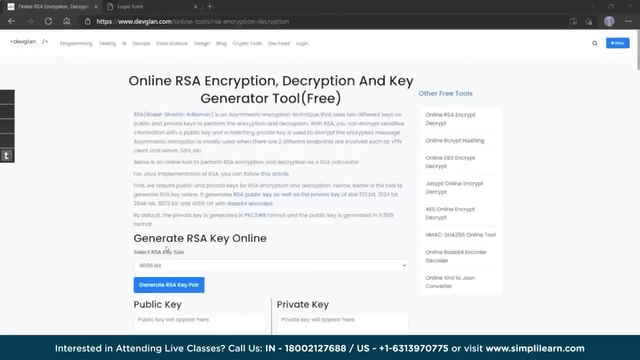 The longer the key length, the more complex the encryption process becomes and thereby strengthening the cipher text. Although, with added security, more complex functions take longer to perform the same operations on similar size of data. We have to keep a balance between both speed and strength, because the strongest encryption 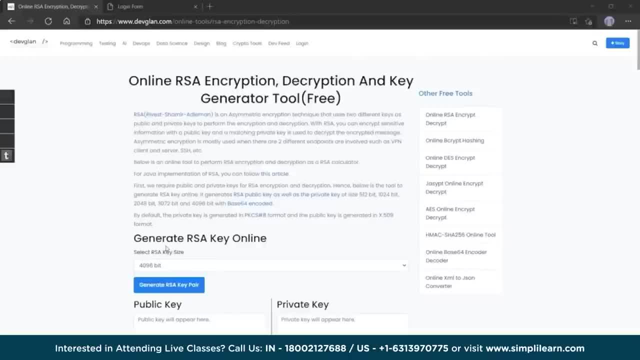 algorithms are of no use if they cannot be practically deployed on systems. We have to keep a balance between both speed and strength, because the strongest encryption algorithms are of no use if they cannot be practically deployed on systems. Let's take a 1024-bit key over here. 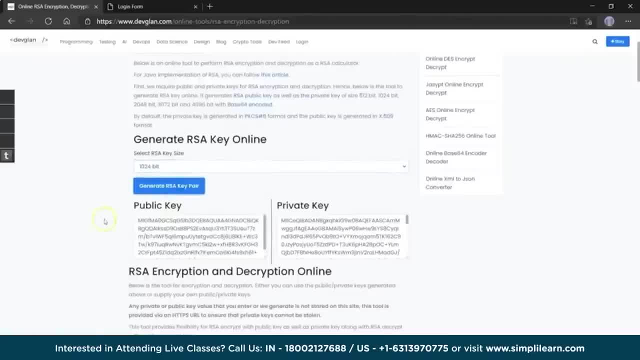 Now we need to generate the keys. This generation is done by functions that operate on passphrases. The tool we are using right now generates the pseudo-random keys to be used in this explanation. Once we generate the keys, you can see the public key is rather smaller than the private. 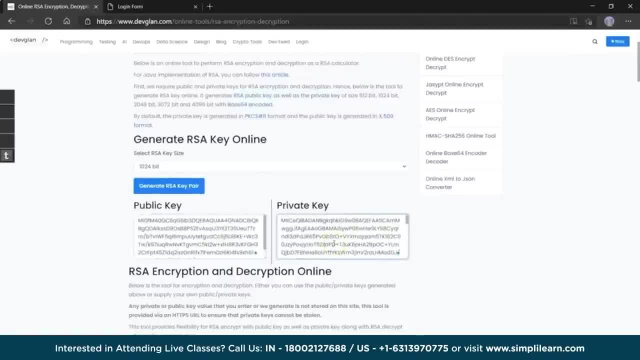 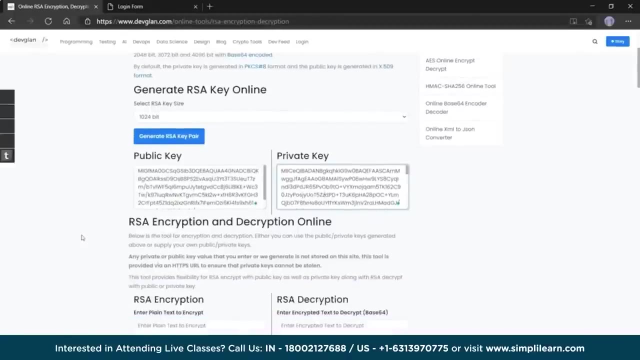 key, which is almost always the case. These two keys are mathematically linked with each other. They cannot be substituted with any other key In order to encrypt the original message or decrypt the cipher text. this pair must be kept together. The public key is then sent to the sender and the receiver keeps the private key with. 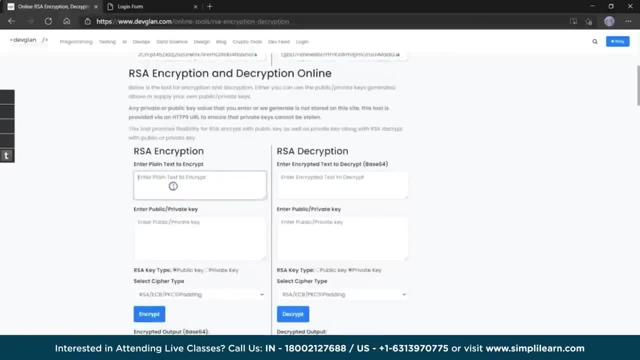 himself. In this scenario, let's try and encrypt a word. simply learn. We have to select if the key being used for encryption is either private or public, since that affects the process of scrambling the information. Since we are using the public key over here, let's select the same and copy it and paste. 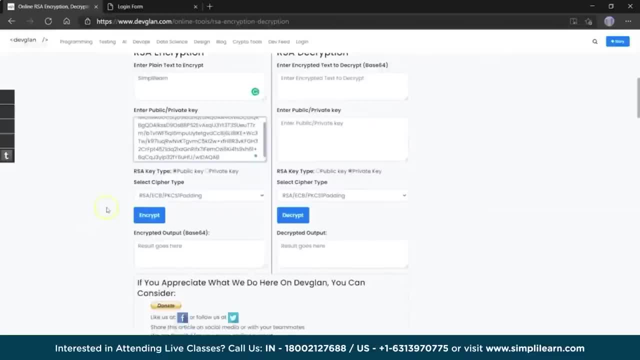 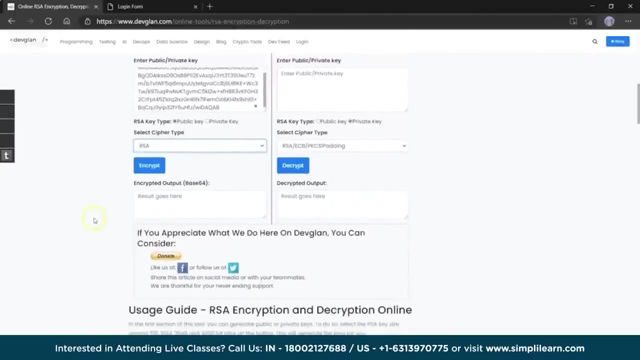 over here. The cipher we are using right now is plain RSA. There are other modified ciphers with their own pros and cons that can also be used, provided we use it on a regular basis and depending on the use case as well. Once you click on encrypt, we can see the ciphers text being generated over here. 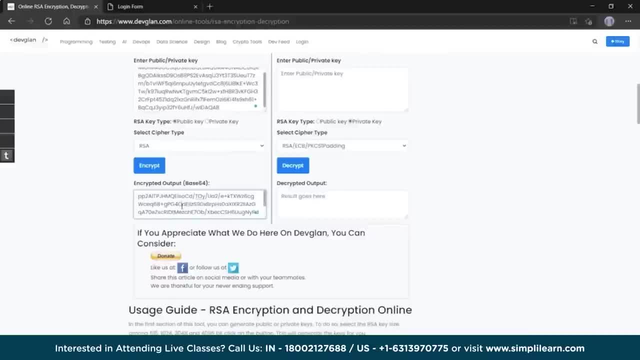 The pseudo-random generating functions are created in such a way that a single character change in the plain text generates an additional component To the 표. we hold Alt17 to help us know if this is stable, which is perfectly fine, will trigger a completely different ciphertext. This is a security feature to strengthen the 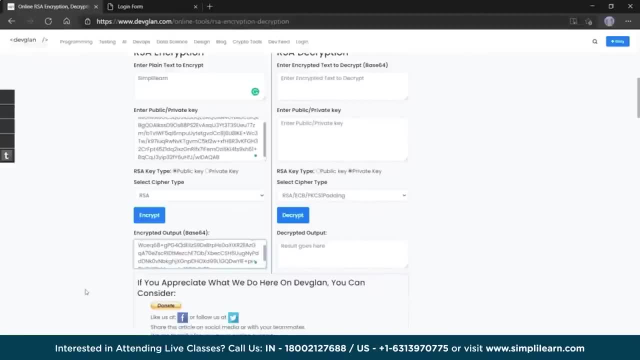 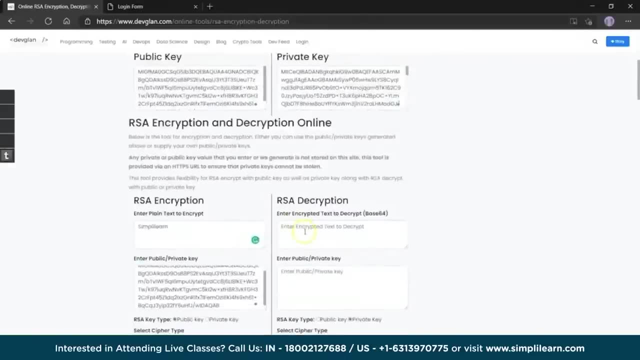 process from brute force methods. Now that we are done with the encryption process, let's take a look at the decryption part. The receiver gets this ciphertext from the sender with no other key or supplement. He or she must already possess the private key generated. 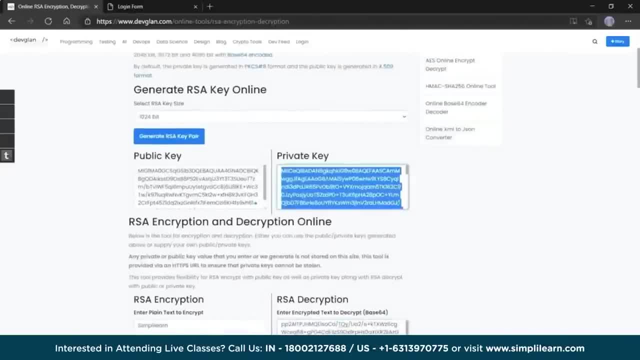 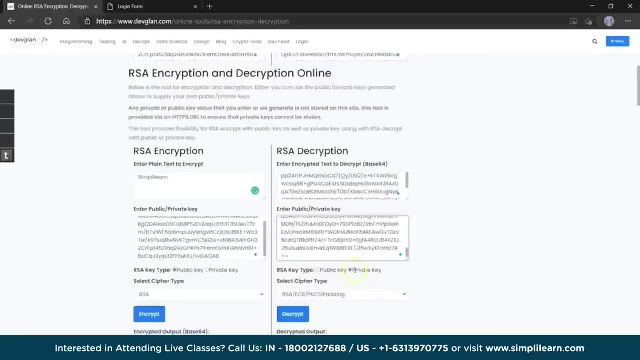 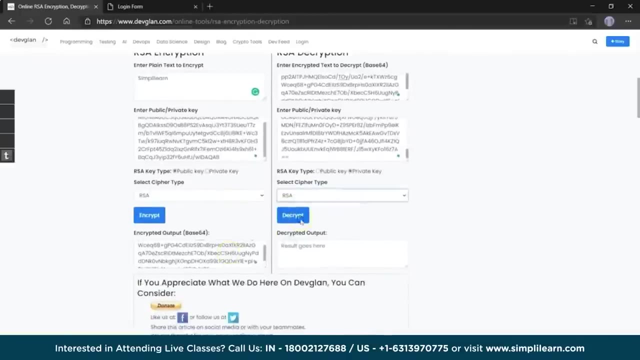 from the same pair. No other private key can be used to decrypt the message. since they are mathematically linked. We paste the private key here and select the same. The cipher must always so be the same used during the encryption process. Once we click decrypt, you can see. 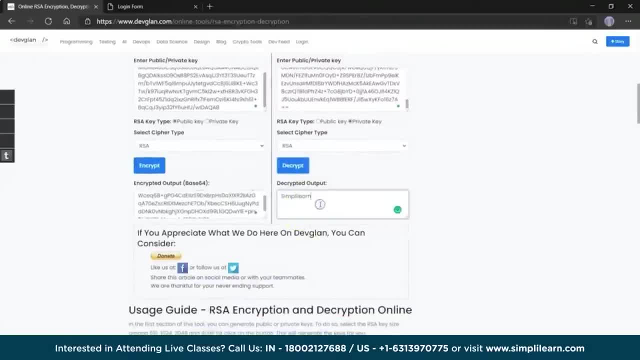 the original plaintext we had decided to encrypt. This sums up the entire process of RSA encryption and decryption. Now some people use it the other way round. We also have the option of using the private key to encrypt information and the public key to decrypt it. This is 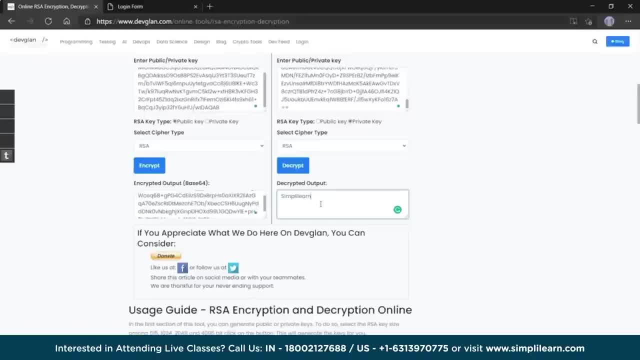 done most frequently to validate the origin of the message, Since the keys only work in pairs. if a different private key is used to encrypt the message, the public key cannot decrypt it. Conversely, if the public key is able to decrypt the message, it must have been encrypted with the right. 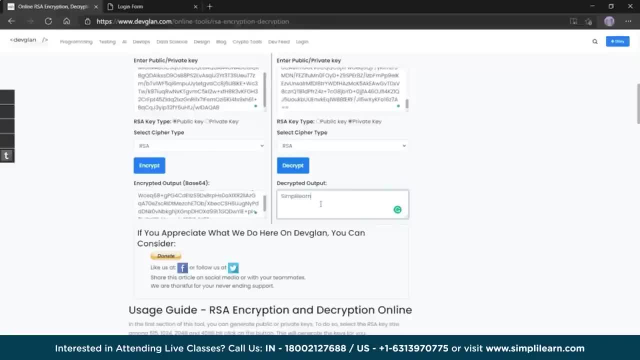 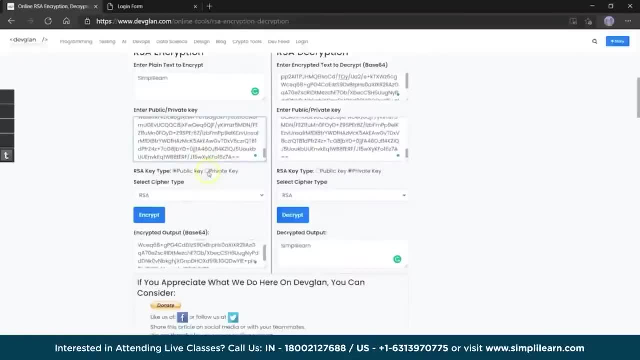 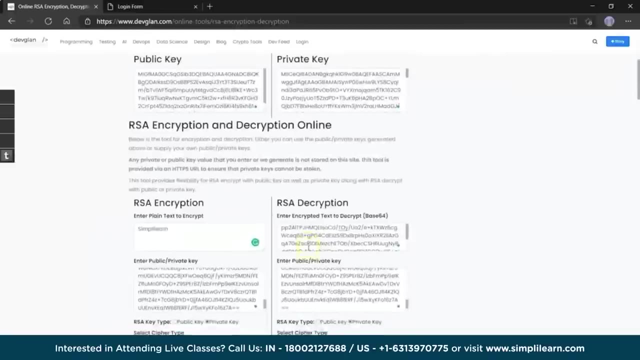 private key and hence the rightful owner. Here we just have to take the private key and use that to encrypt the plaintext and select the same in this checkbox as well. You can see we have generated a completely new ciphertext. This ciphertext will be sent to the receiver, and this time we will use the public key for decryption. Let's select. 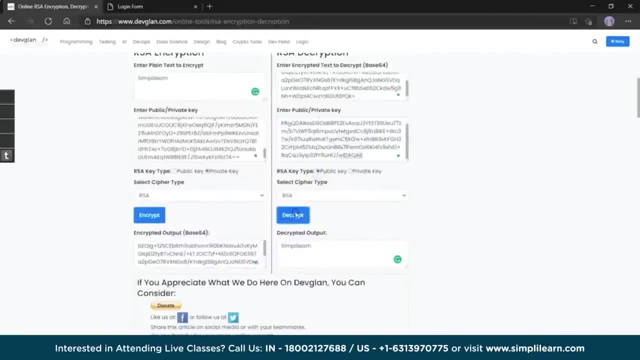 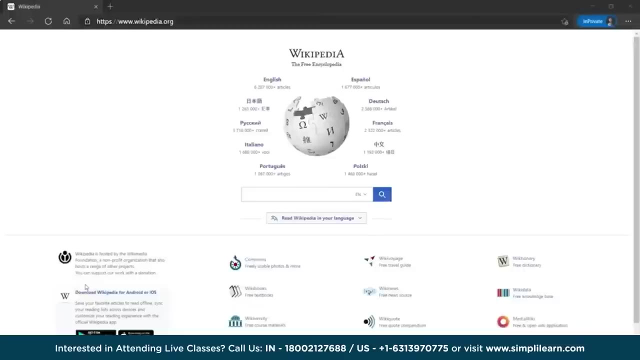 the correct checkbox and decrypt, and we still get the same output. Now let's take a look at practical example of encryption in the real world. We all use the internet on a daily basis and many are aware of the implications of using unsafe web services. 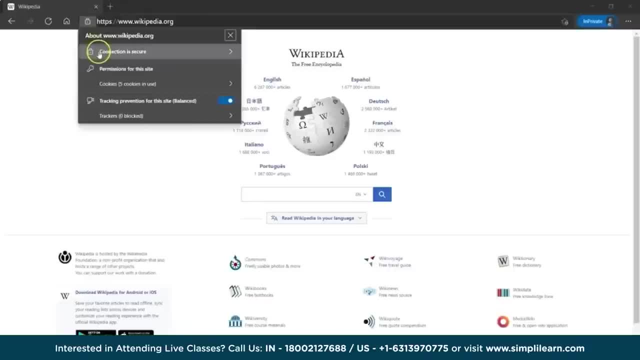 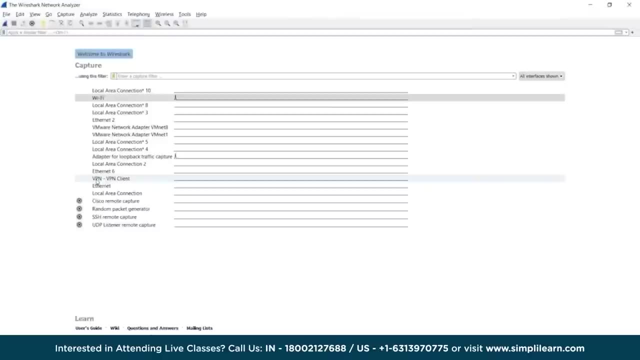 Let's take a look at Wikipedia here. Pretty standard HTTPS website where the H stands for secured. Let's take a look at how it secures the data. Wireshark is the world's foremost and most widely used network protocol analyzer. It lets you see what's happening. 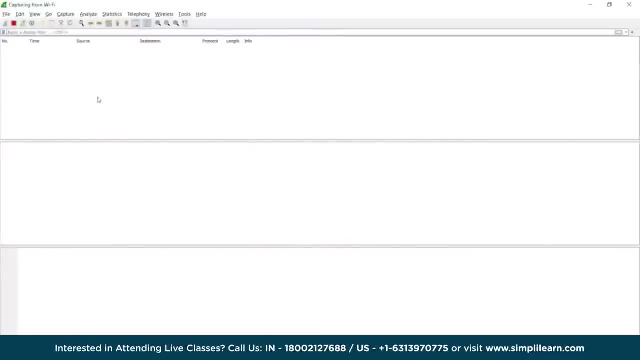 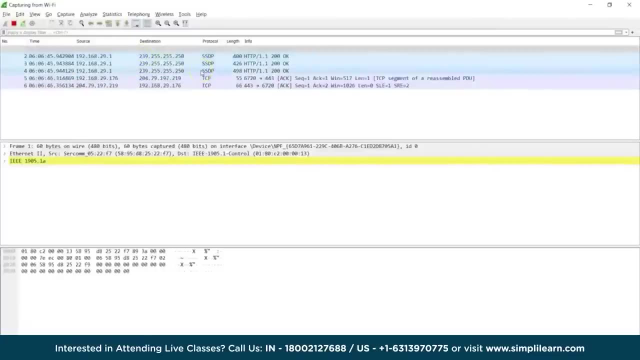 on your network at a microscopic level, and we are going to use this software to see the traffic that is leaving our machine and to understand how vulnerable it is. Since there are many ways to use Wireshark, we are going to use this software to see the traffic that is leaving our machine and to understand how vulnerable it is, Since there are 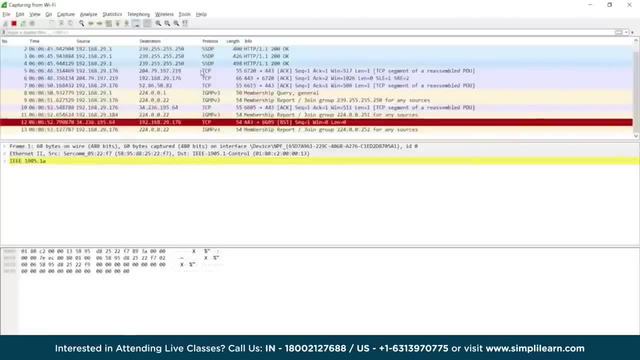 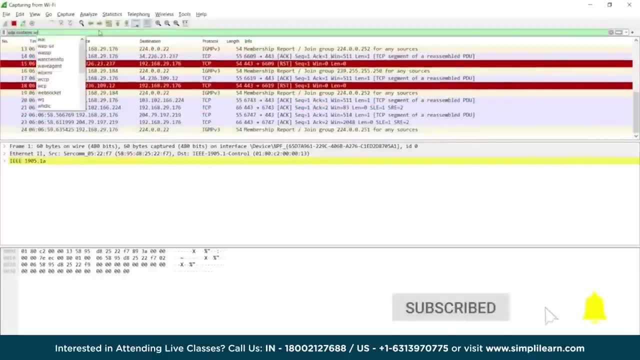 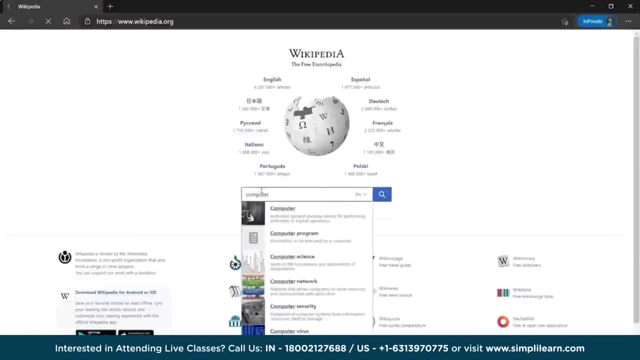 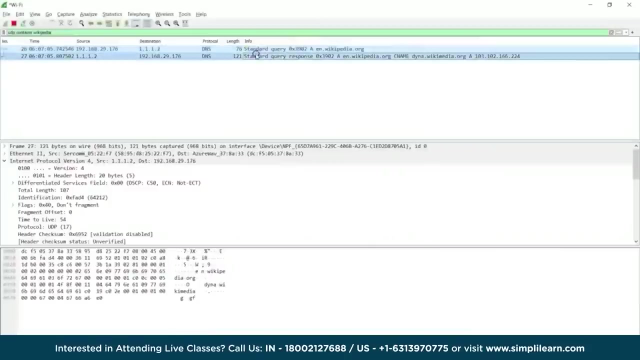 many applications running in this machine. let's apply a filter that will only show us the results related to Wikipedia. Let's search for something that we can navigate the website with. Okay, once we get into it a little, you can see some of the requests. 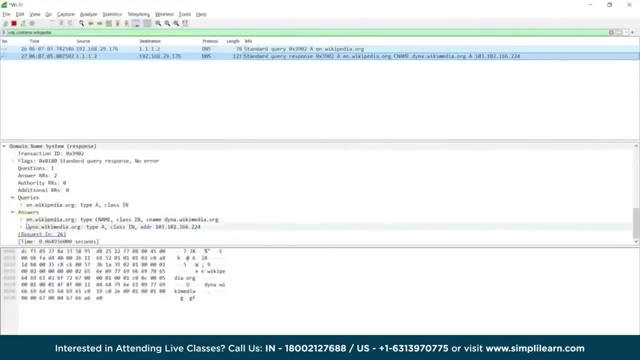 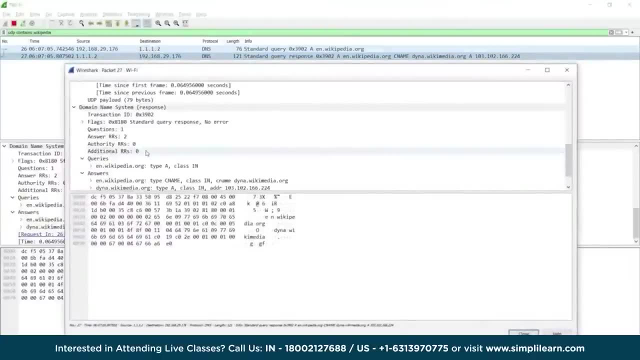 being populated over here. Let's take a look at the specific request. These are the data packets that basically transport the data from our machine to the internet and vice versa. As you can see, there's a bunch of gibberish data here that doesn't really reveal anything that we searched or 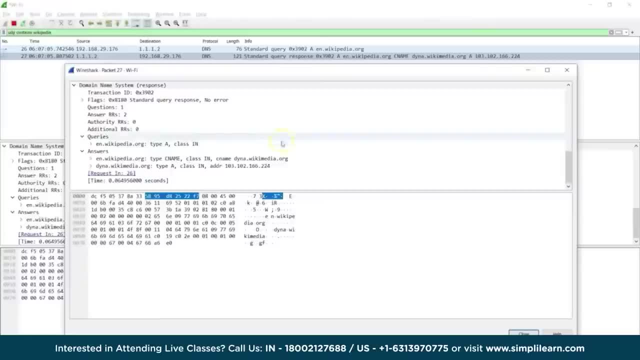 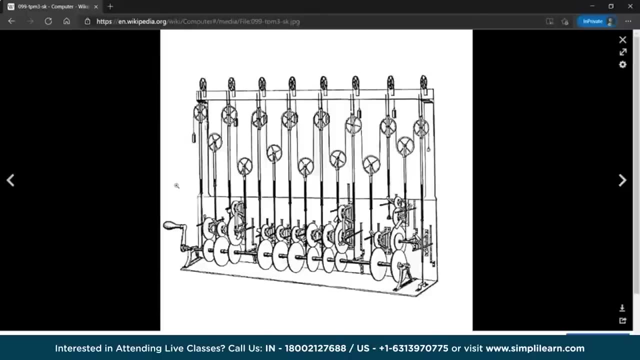 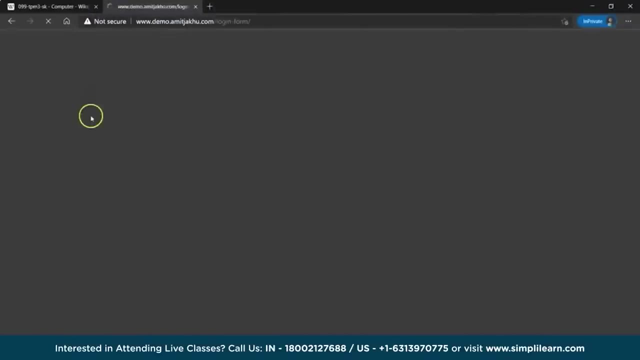 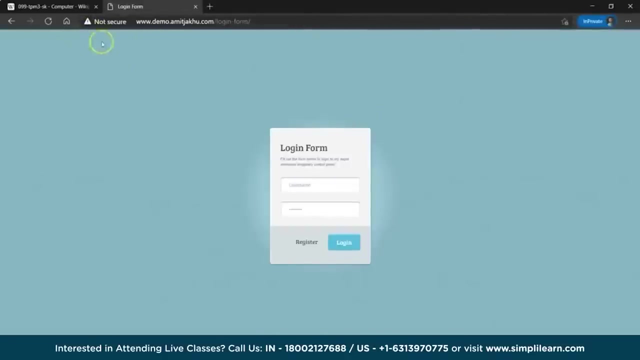 watched. Similarly, other secured websites function the same way, and it is very difficult, if at all possible, to snoop on user data this way. To put this in perspective, let's take a look at another website, which is a HTTP webpage. This has no encryption enabled from. 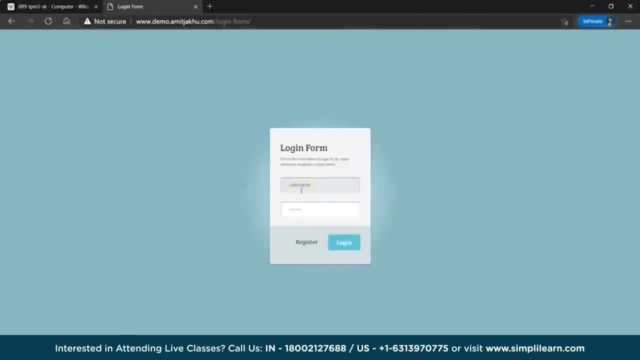 the server end, which makes it vulnerable to attacks. There is a login form here which needs legitimate user credentials in order to grant access. Let's enter a random pair of credentials. These obviously won't work, but we can see the manner of data transfer Unsurprisingly. 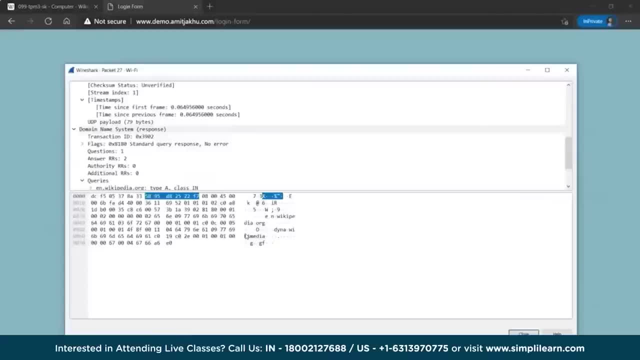 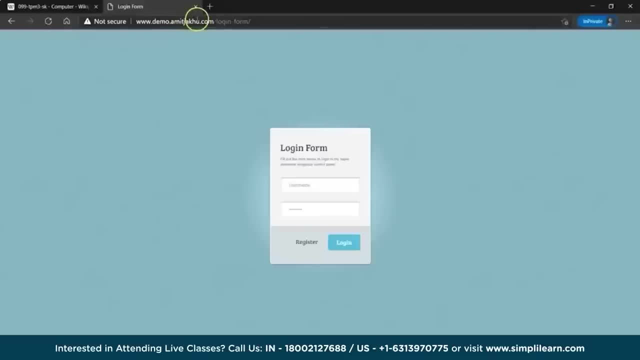 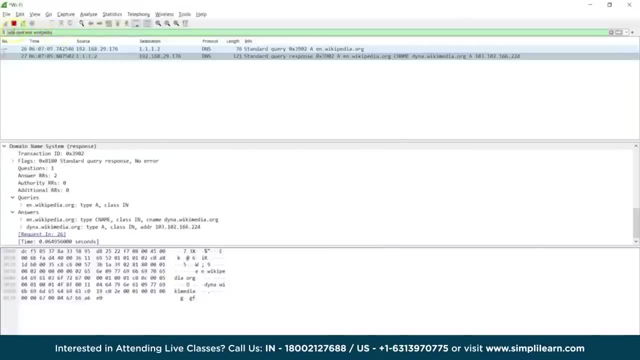 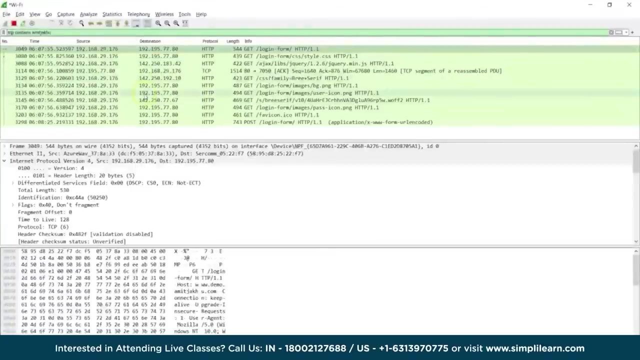 we weren't able to get into the platform. Instead, we can see the data packets. Let's apply a similar filter that will help us understand what request this website is sending. These are the requests being sent by the HTTP login form to the internet, If we check. 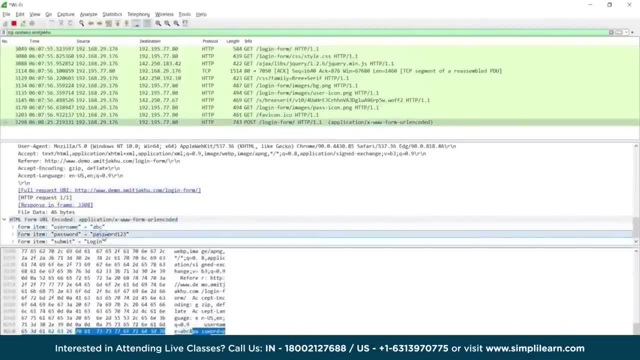 here. whatever username and password that we are entering, we can easily see it with the wireshark. Now, we used a dummy pair of credentials. If we select the right data packet, we can find our correct credentials. If any website had asked for our payment information, 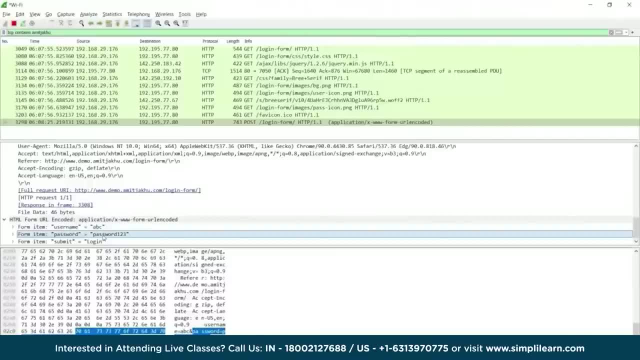 or our legitimate credentials. it would have been really easy to get a hold of them. So let's go ahead and check this out. To reiterate what we have already learned, we must always avoid HTTP websites and just unknown or not trustworthy websites in general, because the problem we saw here is just the 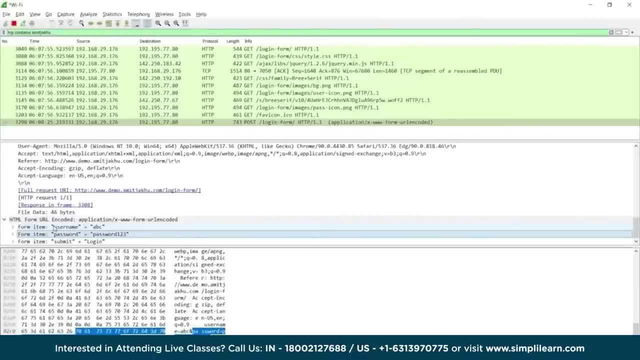 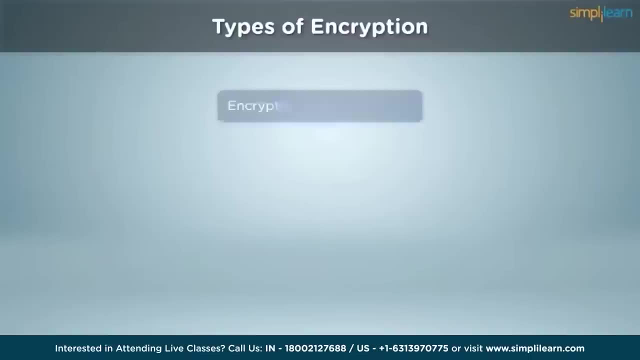 tip of the iceberg. Even though cryptography has managed to lessen the risk of cyber attacks, it is still prevalent and we should always be alert to keep ourselves safe online. There are two types of encryption in cryptography: Symmetric key cryptography and asymmetric key cryptography. 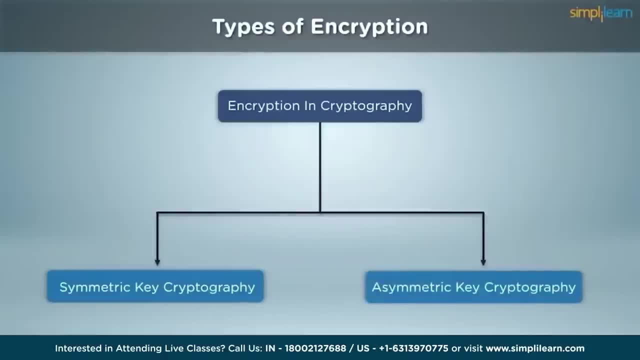 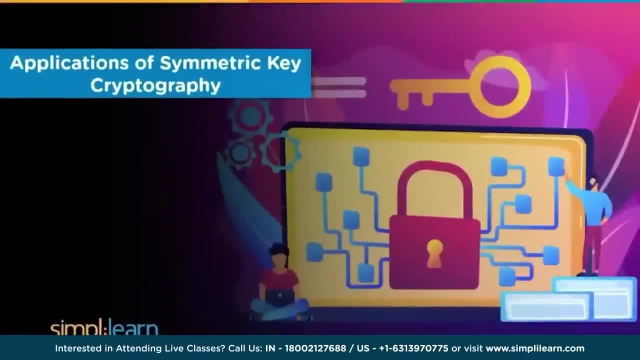 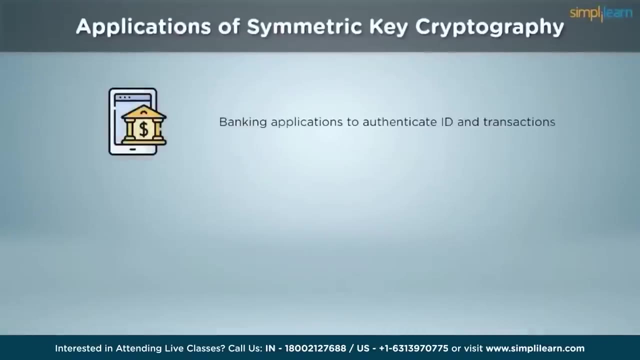 Both of these categories have their pros and cons and differ only by their implementation. Today, we are going to focus exclusively on Symmetric key cryptography. Let us have a look at its applications in order to understand its importance better. This variant of cryptography is primarily used in banking applications, where, personally, 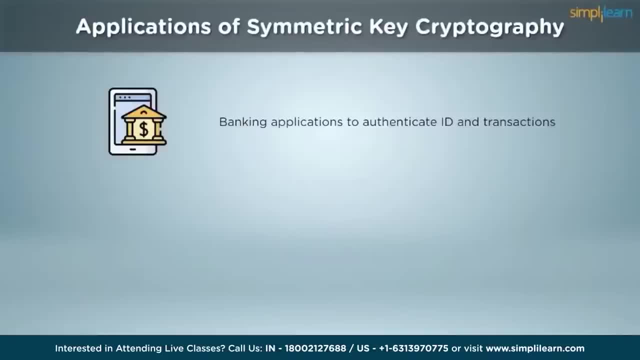 identifiable information needs to be encrypted. With so many aspects of banking moving on to the internet, having a reliable safety net is crucial. Symmetric key cryptography is one of the most popular types of encryption in the world. It is also the most popular type of encryption in the world. It is also the most popular type of encryption in the. 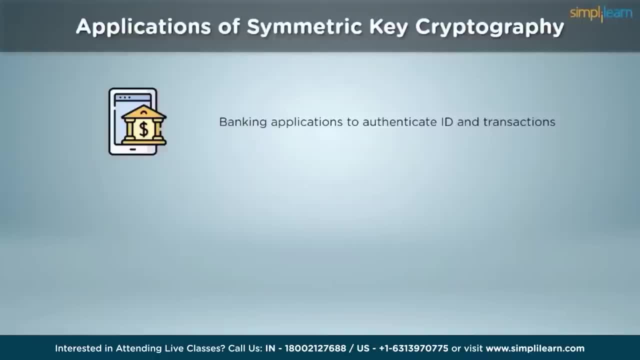 world. Symmetric key cryptography is one of the most popular types of encryption in the world. Symmetric key cryptography helps in detecting bank fraud and boosts the security index of these payment gateways in general. They are also helpful in protecting data that is not in transit and rests on servers, and 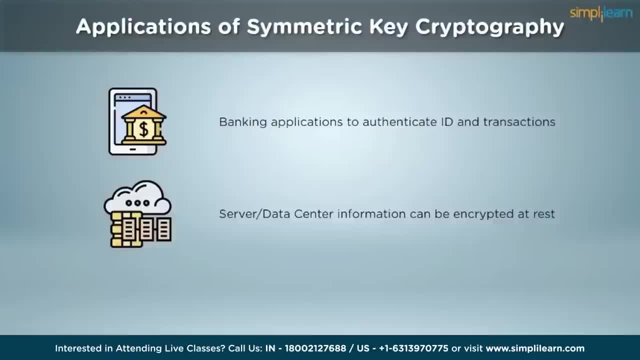 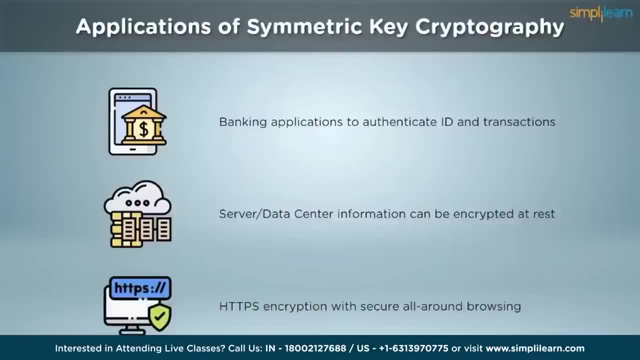 and servers to be able to track the data. We need symmetric encryption to browse secure HTTPS websites so that we can get an all around protection. It plays a significant role in verifying website server authenticity, exchanging the necessary encryption keys required and generating a session using those keys to ensure maximum security. This helps in preventing 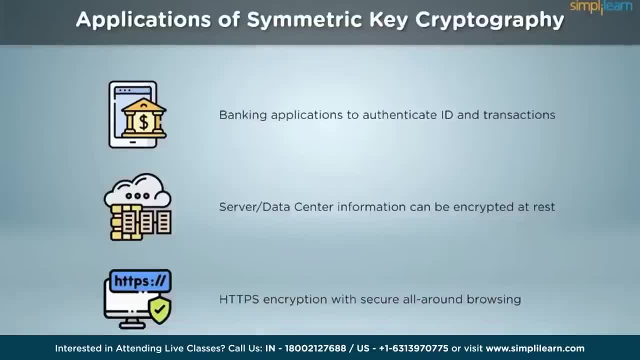 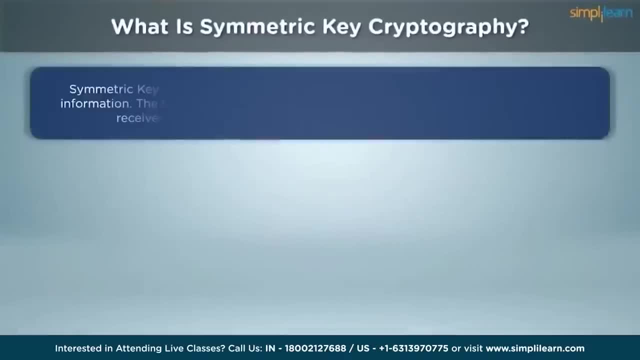 the rather insecure HTTP website format. Symmetric key cryptography works first, before moving on to the specific algorithms. Symmetric key cryptography works as such, before moving on to the specific algorithms. Symmetric key cryptography relies on a single key for the encryption and decryption of information. 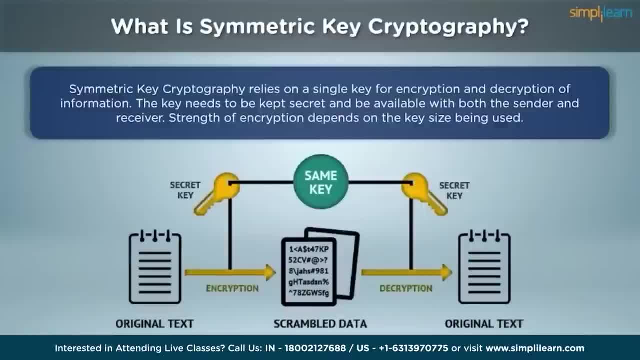 Both the sender and receiver of the message need to have a pre-shared secret key that they will use to convert the plaintext into ciphertext and vice versa. As you can see in the image, the key used for encryption is the same key needed for decrypting the message at the other end. 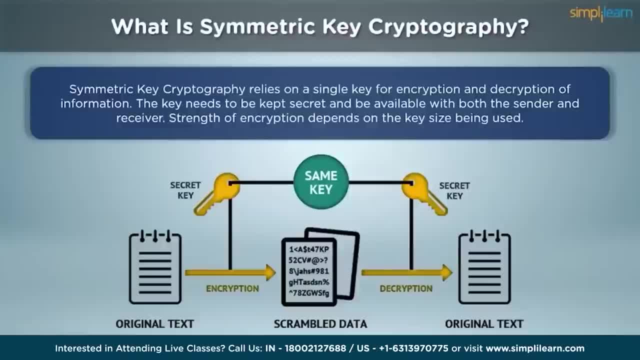 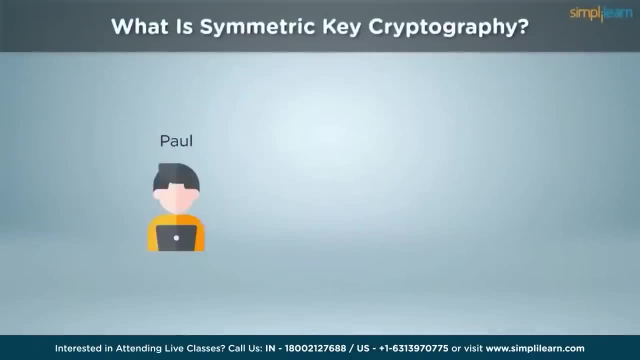 The secret key shouldn't be sent along with the ciphertext to the receiver, because that would defeat the entire purpose of using cryptography. Key exchange can be done beforehand using other algorithms, like the Diffie-Hellman Key Exchange Protocol, for example. For example, if Paul wants to send a simple message to Jane, they need to have a single encryption key that both of them must keep secret to prevent snooping on by malicious actors. 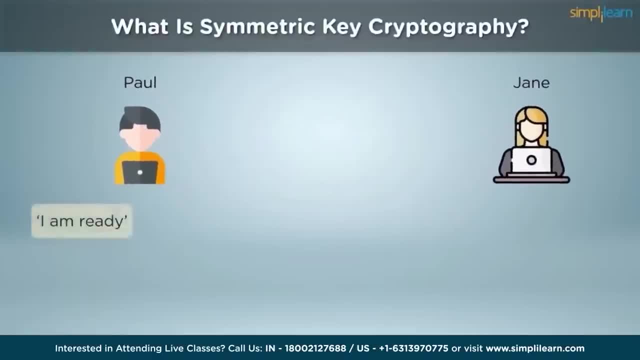 It can be generated by either one of them, but must belong to both of them before the messages start flowing. Suppose the message I am ready is converted into ciphertext using a specific software. In that case, Jane must also be aware of the substitution shift to decrypt this ciphertext once it reaches her. 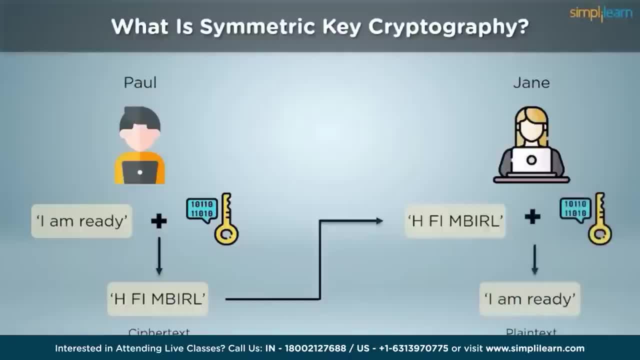 Irrespective of the scenario where someone manages to grab the ciphertext mid-transit to try and read the message, not having the secret key renders everyone helpless looking to snoop in The symmetric key. algorithms like the Data Encryption Standard have been in use since the 1970s, while the popular ones like the AES have become the industry standard today. 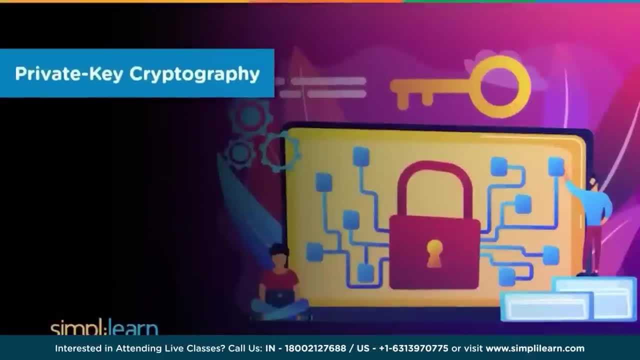 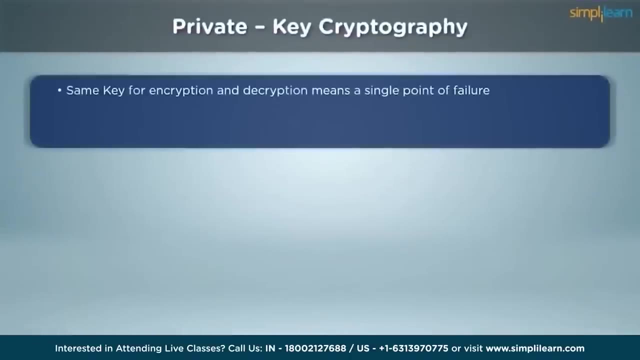 Thank you. With the entire architecture of symmetric cryptography depending on the single key being used, you can understand why it's of paramount importance to keep it secret on all occasions. The side effect of having a single key for the encryption and decryption is it becomes a single point of failure. 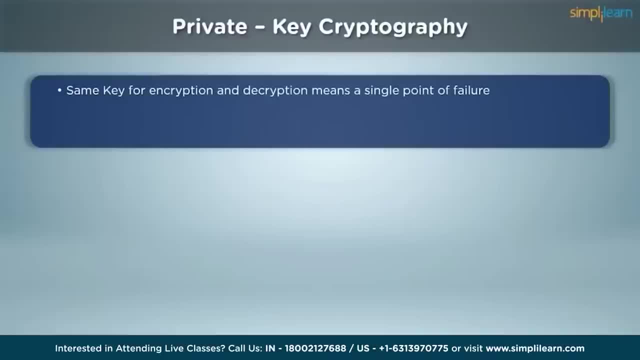 Anyone who gets their hand on it can read all the encrypted messages and do so mainly without the knowledge of the sender and the receiver. So it is the priority to keep the encryption and decryption key private. Should it fall into the wrong hands, the third party can send messages to either the sender or the receiver using the same key to encrypt the message. 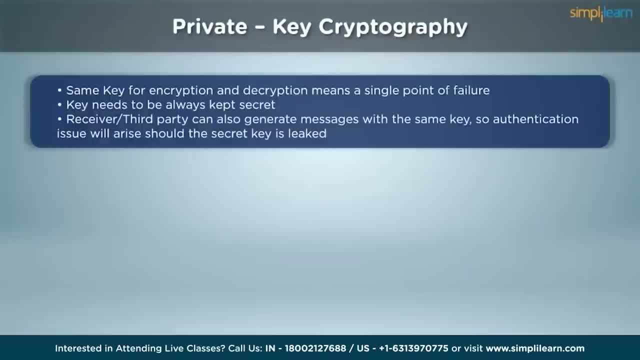 Upon receiving the message and decrypting it with the key, it is impossible to guess its origin. If the sender somehow transmits the secret key along with the ciphertext, anyone can intercept the package and access the information. Consequently, this encryption category is termed private key cryptography, since a big part of the data's integrity is right there. 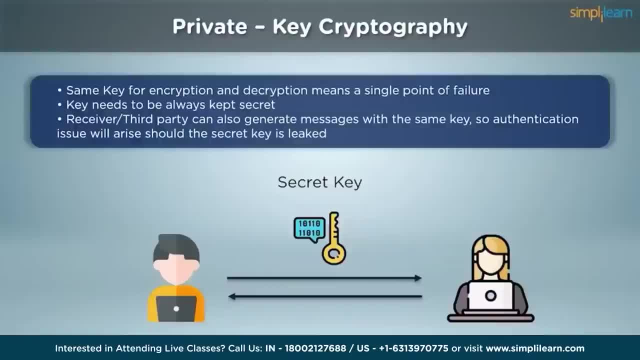 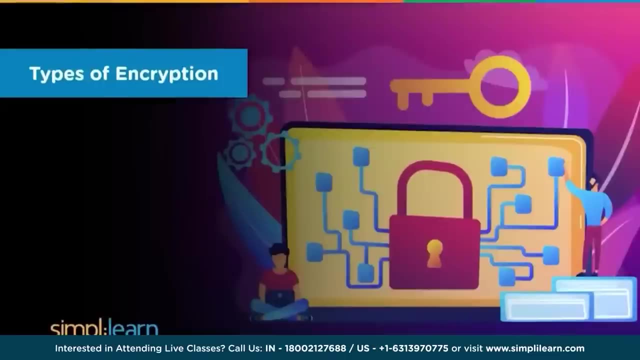 Thank you. Integrity is riding on the promise that the users can keep the key secret. This terminology contrasts with asymmetry key cryptography, which is called public key cryptography because it has two different keys at play, one of which is public. Provided we manage to keep the keys secret, we still have to choose what kind of ciphers we want to use to encrypt this information. 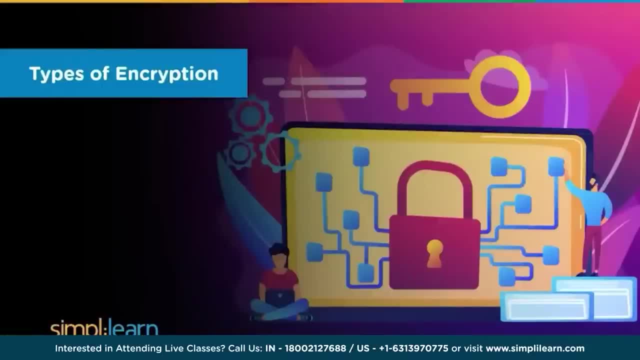 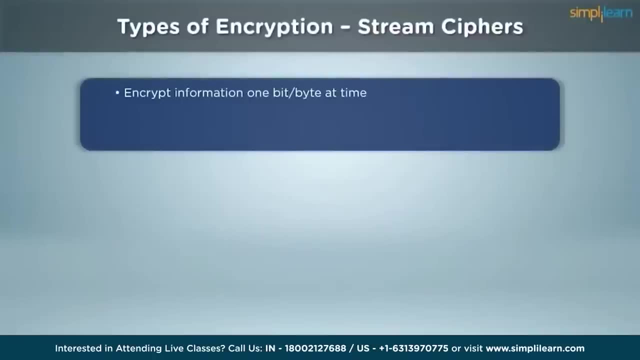 In symmetric key cryptography, there are broadly two categories of ciphers that we can employ. Let us have a look. Stream ciphers are the algorithms that encrypt basic information one bit at a time. It can change depending on the algorithm being used, but usually it relies on a single bit. 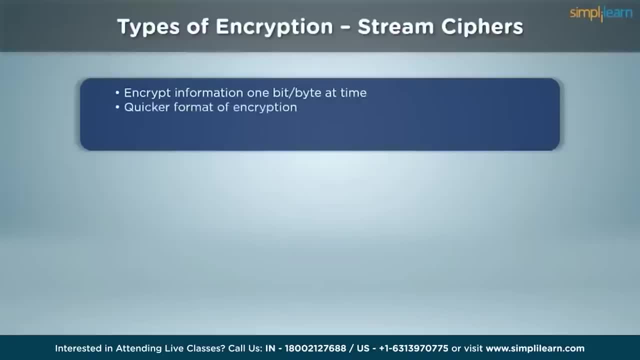 or byte to do the encryption. This is the relatively quicker alternative, considering the algorithm doesn't have to deal with blocks of data at a single time. Every piece of data that goes into the encryption can and needs to be converted into binary format. In stream ciphers, each binary digit is encrypted, one after the other. 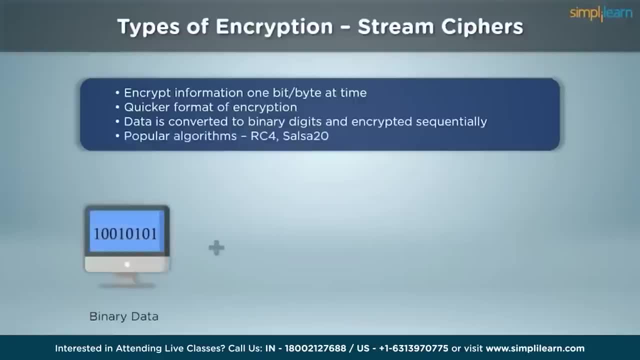 The most popular ones are the RC4, Salsa and Panama. The binary data is passed through an encryption key, which is a randomly generated bitstream. Upon passing it through, we receive the ciphertext that can be transferred to the receiver without fear of man-in-the-middle attacks. 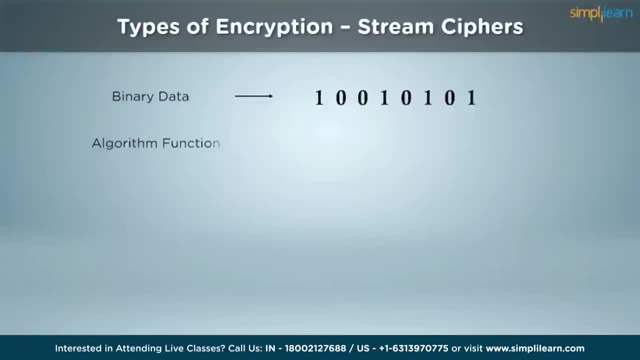 The binary data can be passed through an algorithmic function. It can have either XOR operations, as it is most of the time, or any other mathematical calculations that have the same function. The encryption key is generated using the random bitstream generator and it acts as. 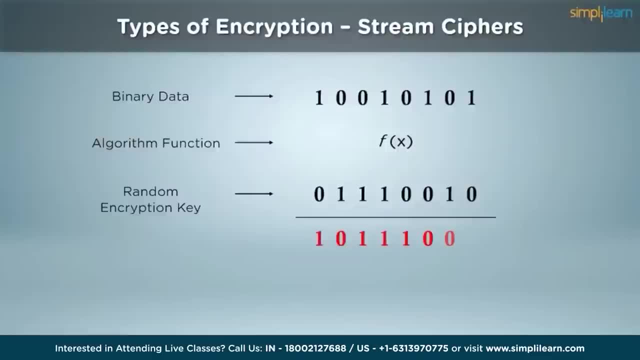 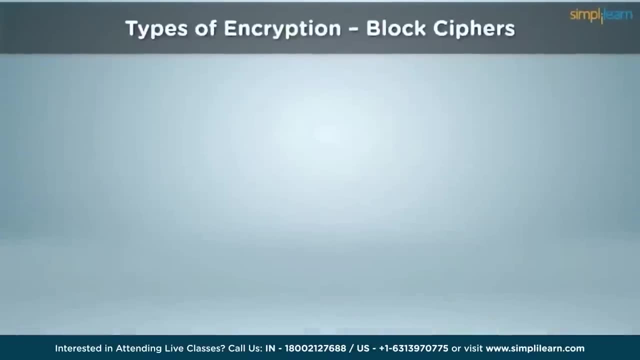 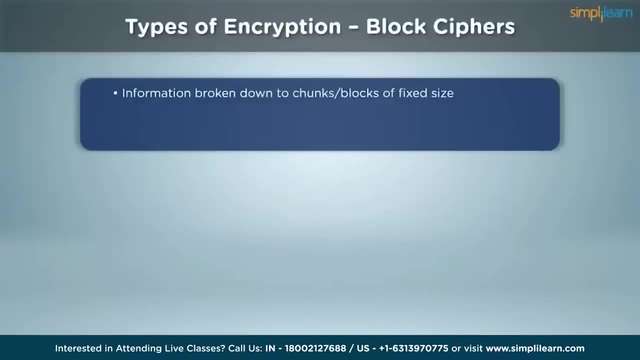 a supplement in the algorithmic function. The output is in binary form, which is then converted into the decimal or hexadecimal format to give our final ciphertext. On the other hand, block ciphers dissect the raw information into chunks of data of fixed size. The size of these blocks depend on the exact cipher being used. 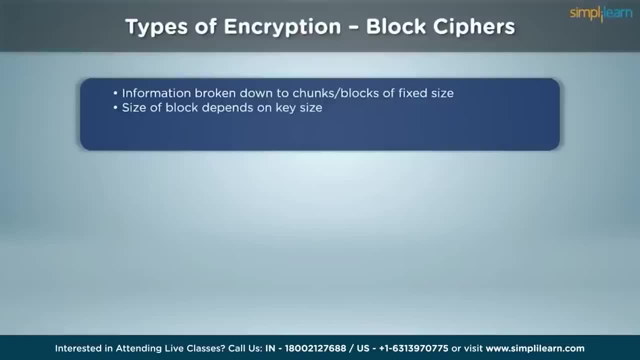 A 128-bit block cipher is a block cipher. A 128-bit block cipher will break the plain text into blocks of 128-bit each and encrypt those blocks instead of a single digit. Once these blocks are encrypted individually, they are chained together to form our final. 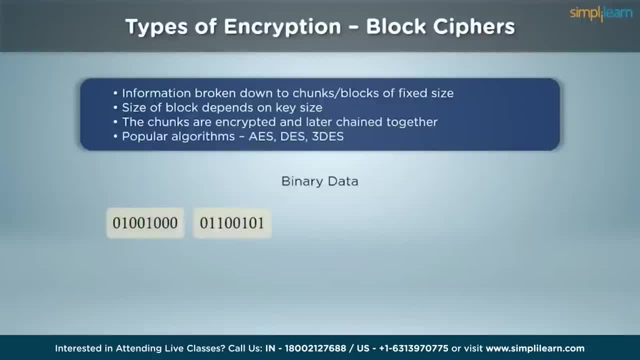 ciphertext. Block ciphers are much slower, but they are more tamper-proof and are used in some of the most widely used algorithms employed today. Just like stream ciphers, the original ciphertext is converted into binary format before beginning the process. Once the conversion is complete, the block ciphers are sent to the receiver. 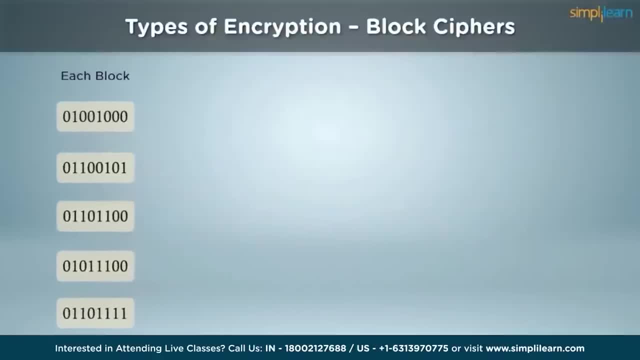 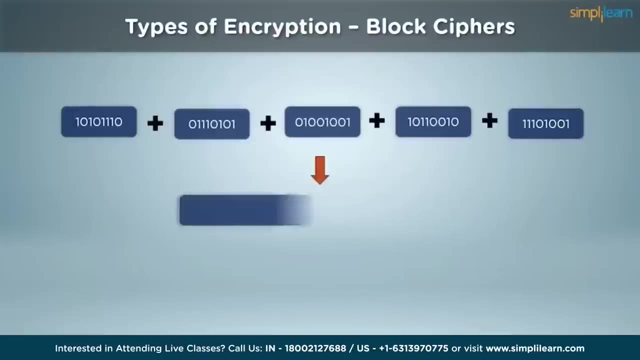 The block ciphers are sent to the receiver. The blocks are passed through the encryption algorithm along with the encryption key. This would provide us with the encrypted blocks of binary data. Once these blocks are combined, we get a final binary string. This string is then converted into hexadecimal format to get our ciphertext. 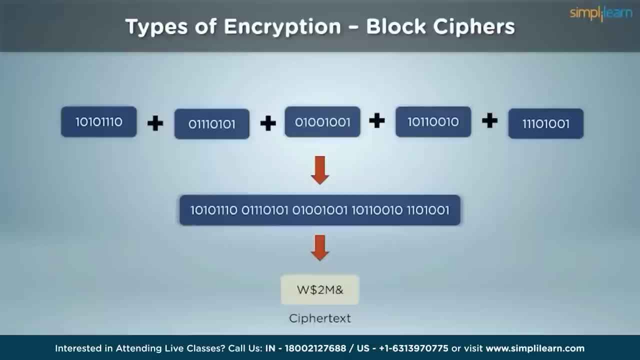 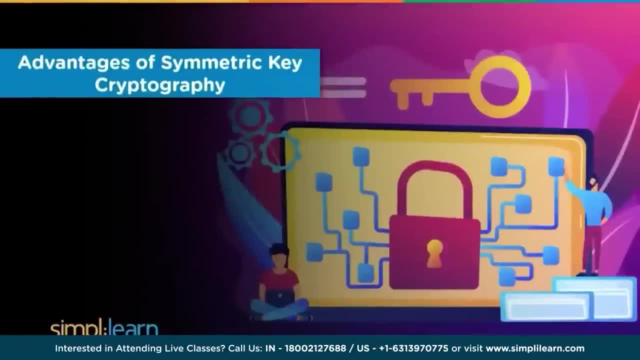 Today, the most popular symmetric key algorithms like AES, DES and 3DES are all block cipher texts and the most popular and most commonly used are the Ciphertext-in-Code and Ciphertext-in-Code sub-sets. With so many factors coming into play, there are quite a few things: symmetric key cryptography. 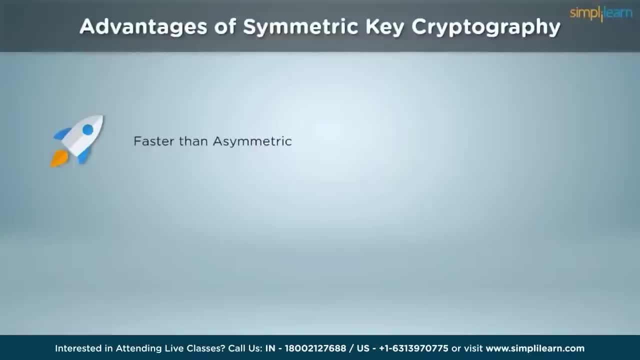 excels at, while falling short in some other. Symmetric key cryptography is a much faster variant when compared to asymmetric key cryptography. There is only one key in play, unlike asymmetric encryption, and this drastically improves calculation speed in the encryption and decryption under similar computational limitations. Fewer calculations help in better memory. 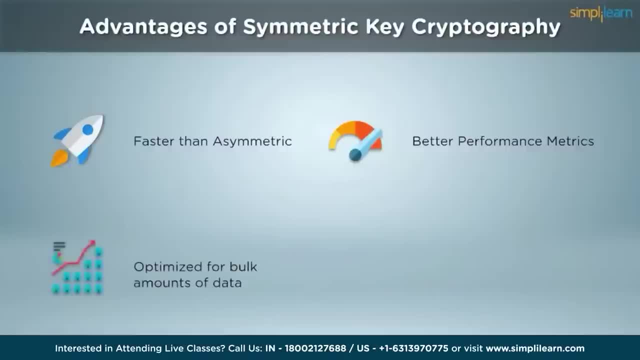 management for the whole system. Bulk amounts of data that need to be encrypted are very well suited for symmetric algorithms, Since they are much quicker. handling large amounts of data is simple and easy to use in servers and data farms. This helps in better latency during data recall and fewer mixed. 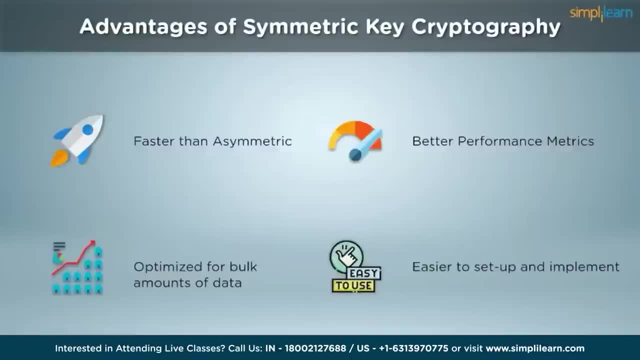 packets. Thanks to its simple single key structure, symmetric key cryptography algorithms are much easier to set up a communication channel with and offer a much more straightforward maintenance duties Once the secret key is transmitted to both the sender and receiver without any prior mishandling. 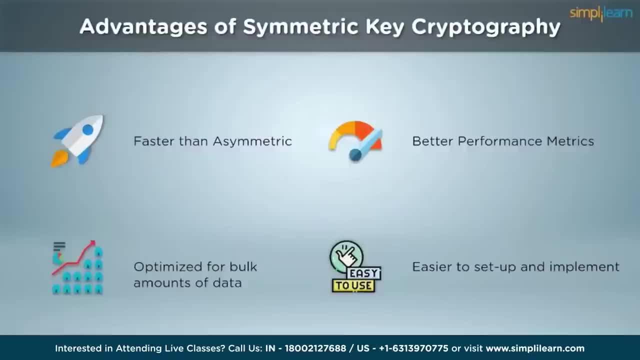 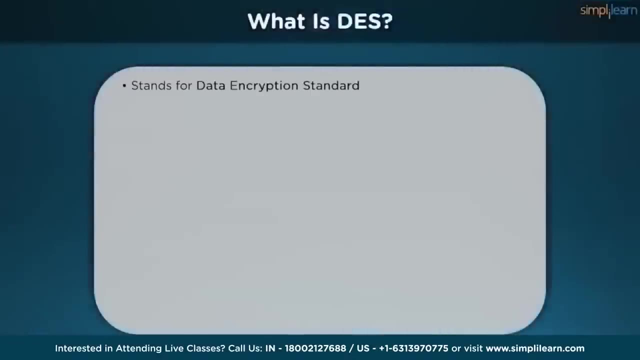 the rest of the system aligns easily and everyday communications becomes easy and secure If the algorithm is applied as per the documentation. symmetric algorithms are very robust and can encrypt vast amounts of data with very less overhead. DES algorithm stands for data encryption standard. 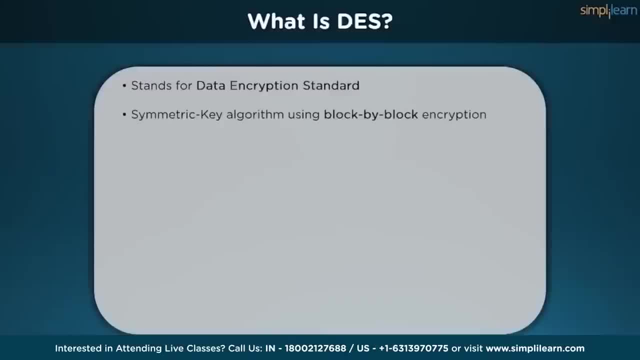 It is a symmetric key cipher that is used to encrypt and re-crypt information in a block by block manner. Each block is encrypted individually and they are later chained together to form our final cipher text, which is then sent to a receiver. DES takes the original, unaltered piece of 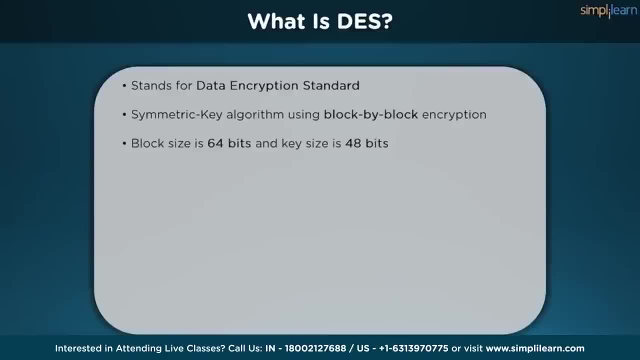 data, called the plain text, in a 64-bit block and it is converted into an encrypted text that is called the cipher text. It uses 48-bit keys during the encryption process and follows a specific structure called the Fistel cipher structure during the entire process. It is a symmetric key. 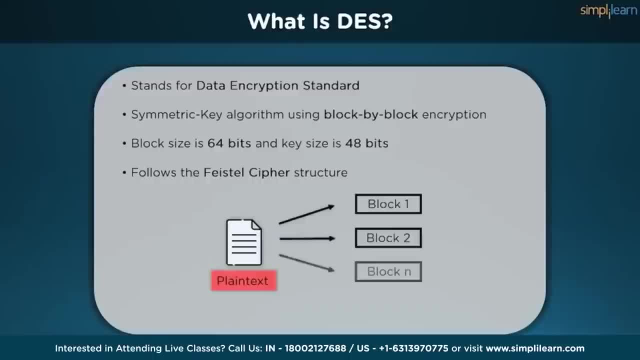 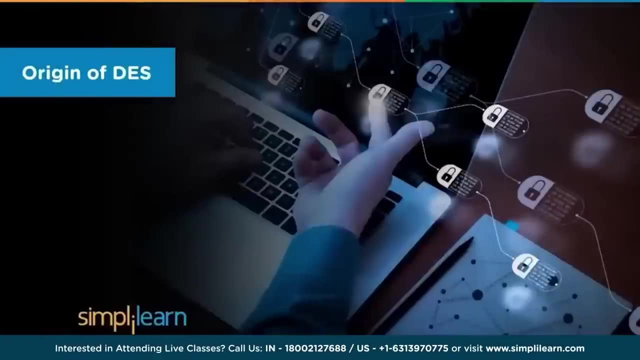 algorithm, which means DES can reuse the keys used in the encryption format to decrypt the cipher text back to the original plain text. Once the 64-bit blocks are encrypted, they can be combined together before being transmitted. Let's take a look at the origin and the reason DES was founded. 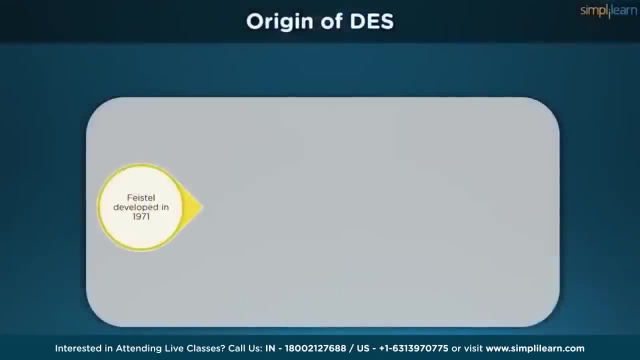 DES is based on a Fistel block cipher called Lucifer, developed in 1971 by a IBM cryptography researcher, Horst Fistel. DES uses 16 rounds of this Fistel structure, using a different key for each round. It also utilizes a random function with two inputs and provides a single output variable. DES became the 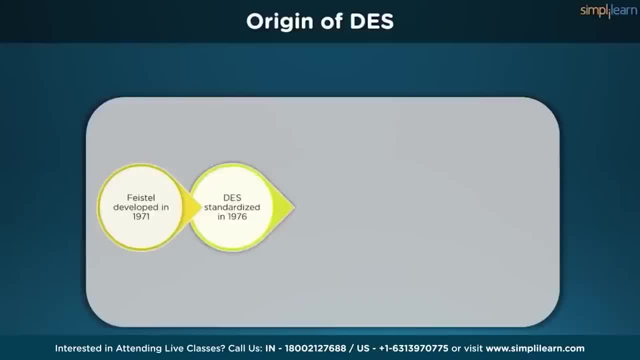 organization's approved encryption standard in November 1976 and was later reaffirmed as a standard in 1983, 1988 and finally in 1999.. But eventually DES was cracked and it was no longer considered a secure solution for all official routes of communication. Consequently, triple DES was 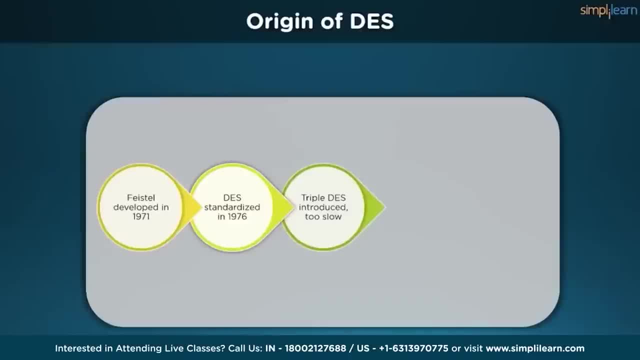 developed. Triple DES is a symmetric key block cipher that uses a double DES cipher: Encrypt with the first key, delete encryption with the second key and encrypt again with a third key. There is also a variation of the two keys where the first and second key are duplicate of each other, But triple DES was. 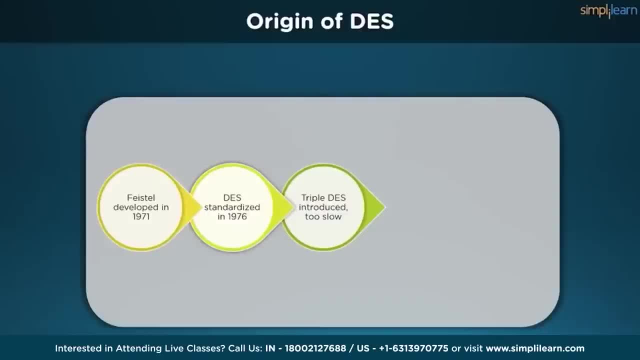 ultimately deemed too slow for the growing need for fast communication channels, and people eventually fell back to using DES for encrypting messages. In order to search for a better alternative, a public-wide competition was organized and helped cryptographers develop their own algorithm as a proposal for the next global standard. This is where the 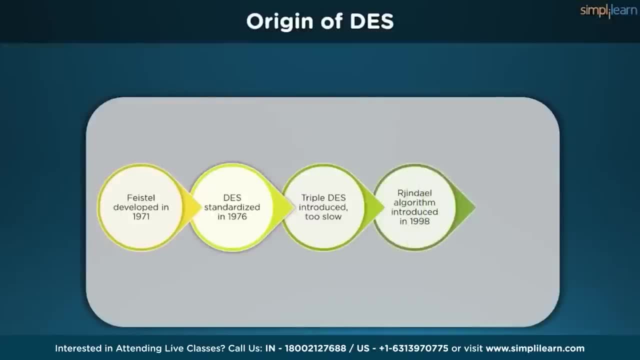 Vindal algorithm came into play and was later credited to be the next advanced encryption standard. For a long time, DES was the standard for data encryption for data security. Its rule ended in 2002 when, finally, the advanced encryption replace DES as an acceptable standard following a public competition for a place. 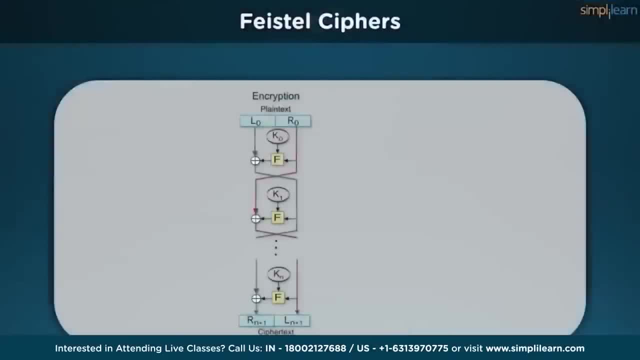 To understand the structure of a Fistel cipher, we can use the following image as a reference. The block being encrypted is divided into two parts, one of which is being passed on to the function, while the other part is XORed with the function's output. 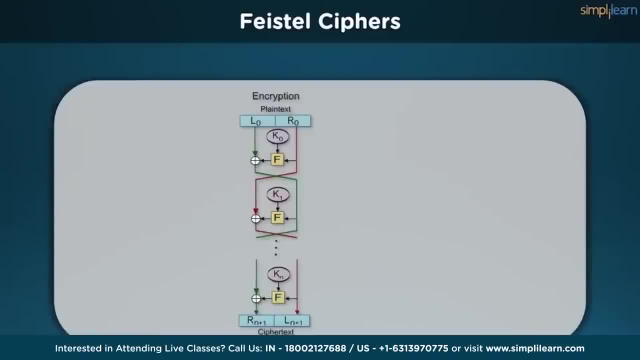 The function also uses the encryption key that differs for each individual round. This keeps going on until the last step, where the right hand side and the left hand side are being swapped. Here we receive our final ciphertext For the decryption process. the entire procedure is reversed, starting from the order of the 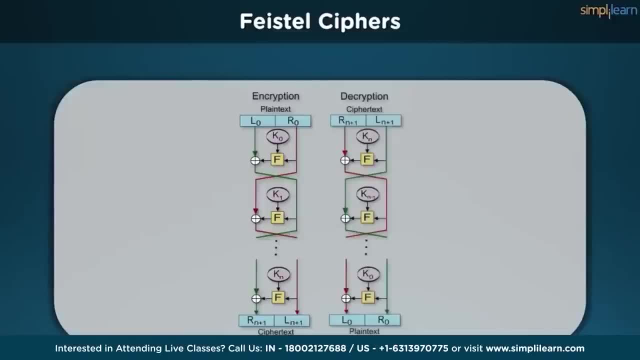 keys to the block sorting. If the entire process is repeated in a reverse order, we will eventually get back our plain text, and this simplicity helps the speed. Overall, this was later detrimental to the efficiency of the algorithm, hence the security was compromised. 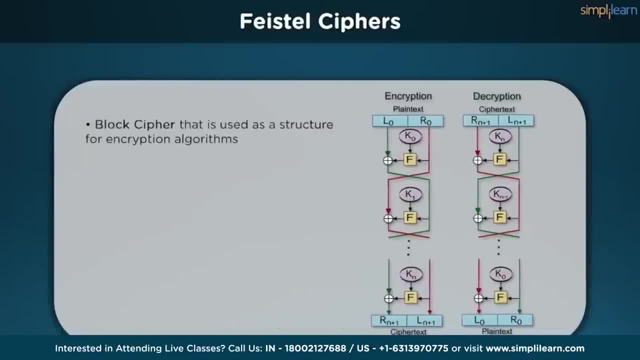 A Fistel block cipher is a structure used to derive many symmetric block ciphers, such as DES, which, as we have discussed in our previous commentary. Fistel cipher proposed a structure that implements substitution and permutation alternately, so that we can obtain ciphertext from the plaintext and vice versa. 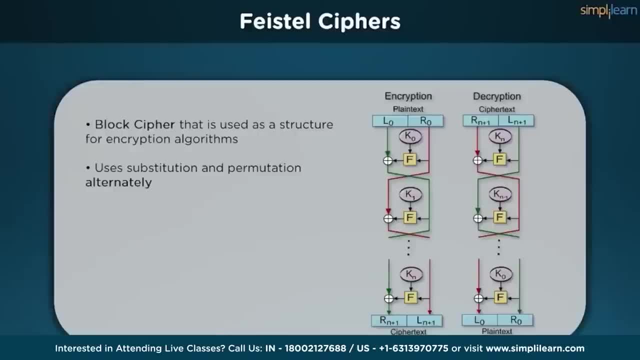 This helps in reducing the redundancy of the program and increases the complexity to combat brute force attacks. The Fistel cipher is actually based on the Shannon structure that was proposed in 1945.. The Fistel cipher is the structure suggested by Horst Feistel, which was considered to be 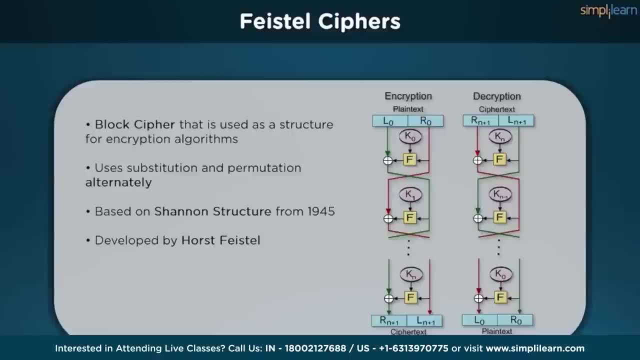 a backbone while developing many symmetric block ciphers. The Shannon structure highlights the implementation of alternate confusion and diffusion And, like we already discussed, the Fistel cipher structure can be completely reversed depending on the data. However, we must consider the fact that to decrypt the information by reversing the Feistel, 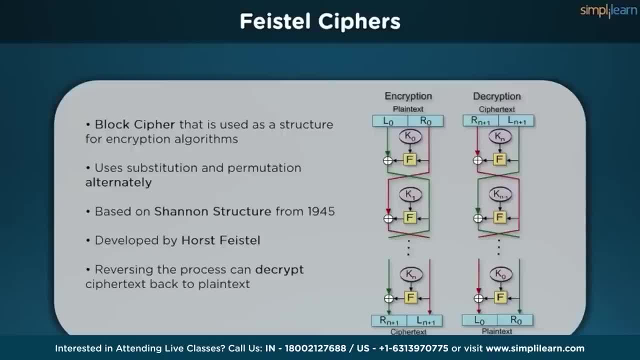 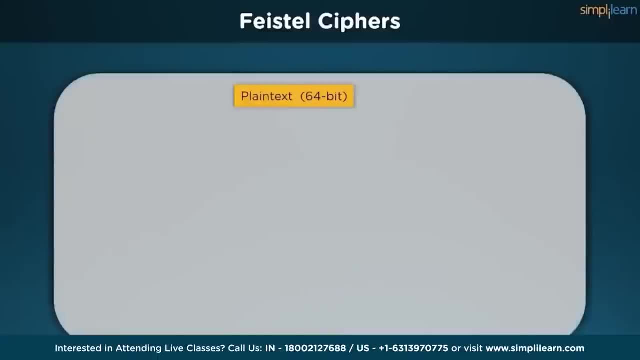 structure, we will need the exact polynomial. So let's see how it works. To understand how the blocks are being calculated, we take a plaintext which is of 64-bit, and when that is later divided into two equal halves of 32-bit each. 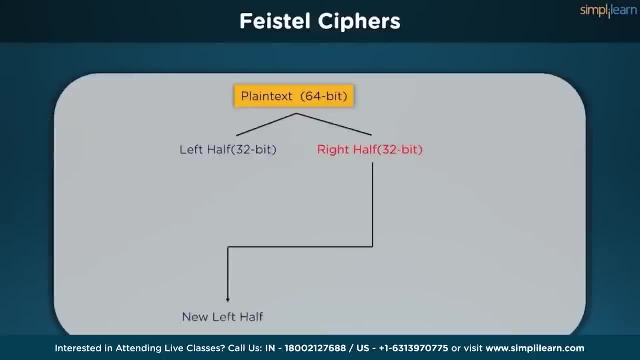 In this, the right half is immediately transferred to the next round to become the new left half of the second round. The right hand is again passed off to a function which uses an encryption key that is unique to each round in the Fistel cipher. 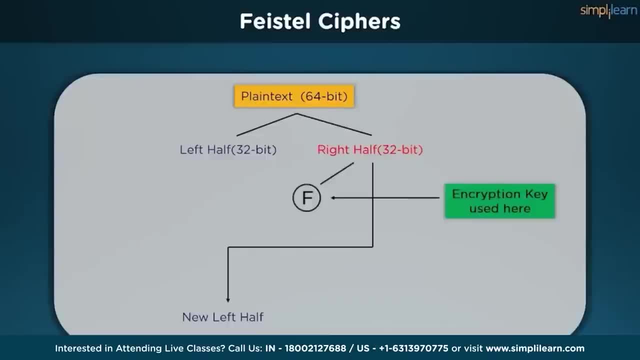 What happens? Whatever the function gives off as an output, it is passed on as an XOR input with the left half of the initial plaintext. The next output will become the right half of the second round for the plaintext. This entire process constitutes of a single round in the Fistel cipher. 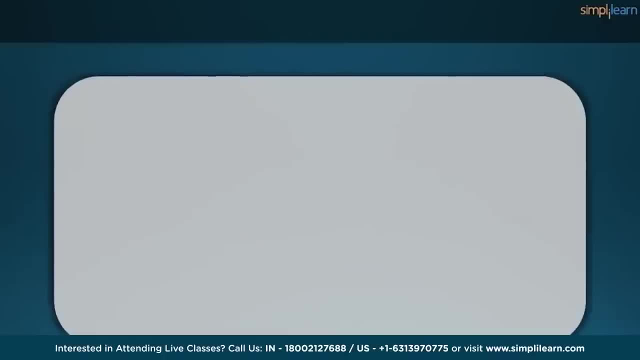 To take into account what happens in the polynomial function, we take one half of the block and pass it through an expansion box. The work of the expansion box is to increase the number of blocks. For example, we take a block for the first round and pass it through another block for. 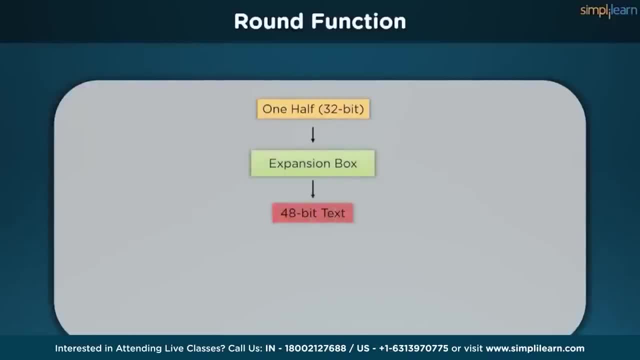 the second round the size of the half from 32-bit to 48-bit text. This is done to make the text compatible to a 48-bit keys we have generated beforehand. Once we pass it through the XOR function, we get a 48-bit text as an output. 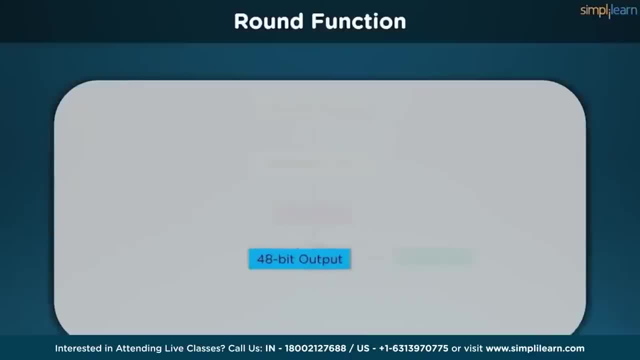 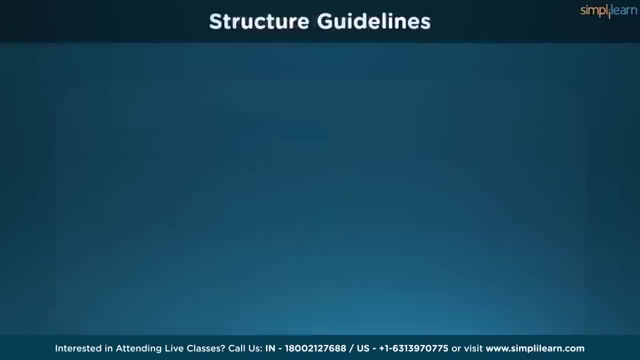 Now remember, a half should be of 32-bit. So this 48-bit output is then later passed on to a substitution box. This substitution box reduces its size from 48-bit to 32-bit output, which is then later XORed with the first half of the plaintext. 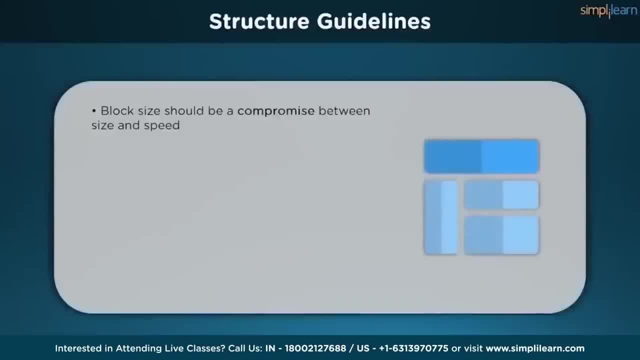 A block cipher is considered the safest if the size of the block is large, But large block sizes can also slow down encryption speed and the decryption speed. Generally, the size is 64-bit. Sometimes modern block ciphers like AES have a 128-bit block size as well. 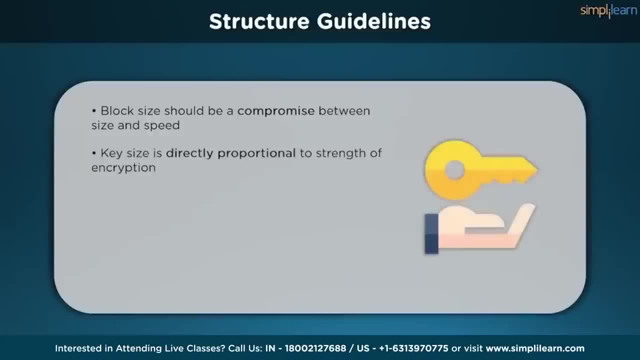 The security of the block cipher increases with increasing key size, But larger key sizes can also increase the security of the block cipher. Earlier, 64-bit keys were considered sufficient. Modern ciphers need to use 128-bit keys due to the increasing complexity of today's computational. 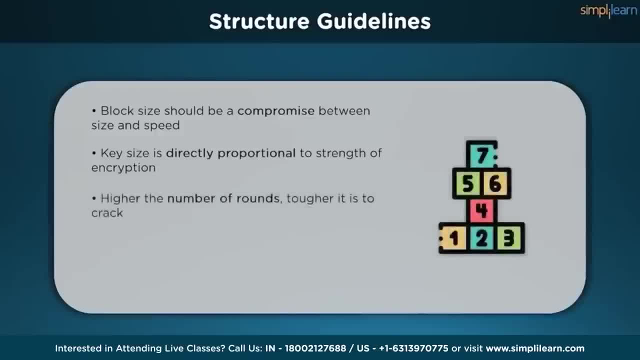 standards. The increasing number of rounds also increases the security of the block cipher. Similarly, they are inversely proportional to the speed of encryption. A highly complex round function enhances the security of the block cipher. However, we must maintain a balance, The balance between the speed and security. 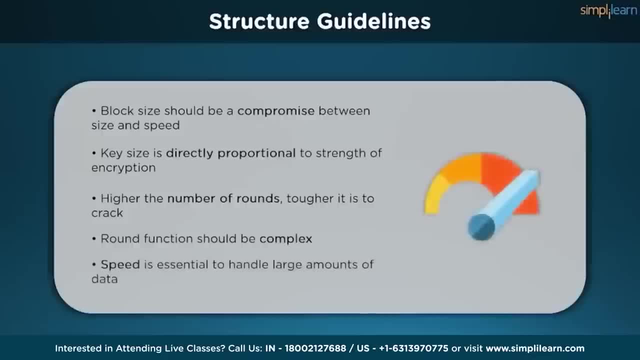 The symmetric block cipher is implemented in a software application to achieve better execution speed. There is no use of an algorithm if it cannot be implemented in a real-life framework that can help organizations to encrypt or decrypt the data in a timely manner. Now that we understand the basics of Fistel ciphers, we can take a look at how DES manages. 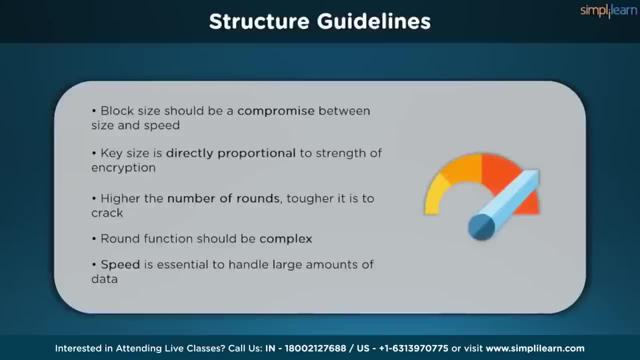 to run through 16 rounds of this structure and provide the ciphertext at the end. In the first round, the Cipher is used to decrypt data and decrypt the data. The second round is used to decrypt data. The third round is used to decrypt data. 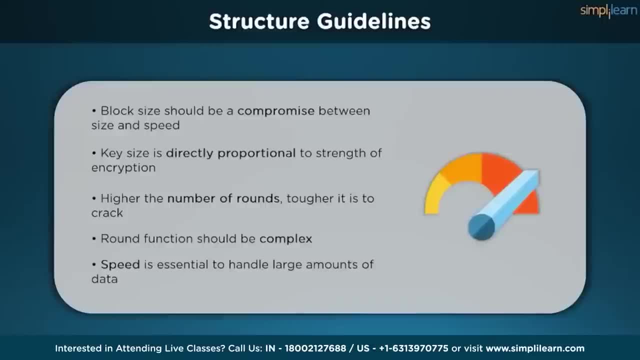 The fourth round is used to decrypt data. The fifth round is used to decrypt data. The fourth round is used to decrypt data- be implemented in a real-life framework that can help organizations to encrypt or decrypt the data in a timely manner. Now that we understand the basics of VSTL ciphers, we can take a look at how DES manages. 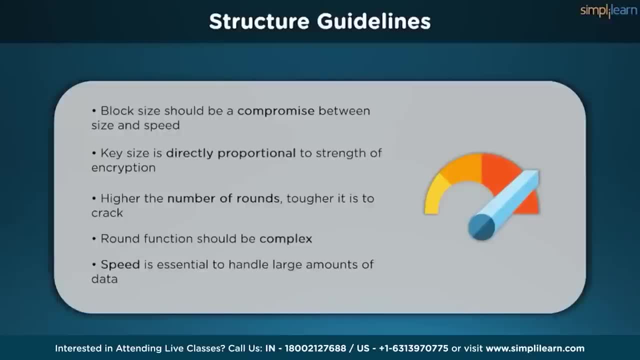 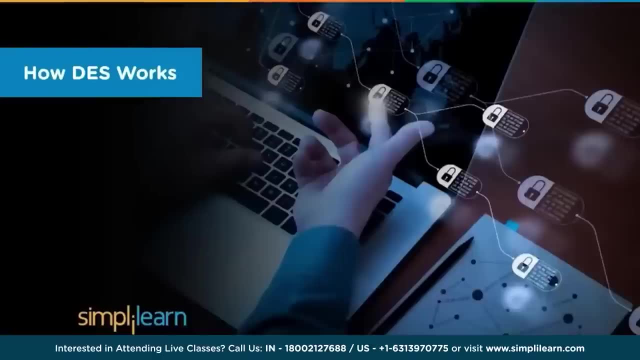 to run through 16 rounds of this structure and provide the ciphertext at the end. Now that we understand the basics of VSTL ciphers, we can take a look at how DES manages to run through 16 rounds of this structure and provide a ciphertext. 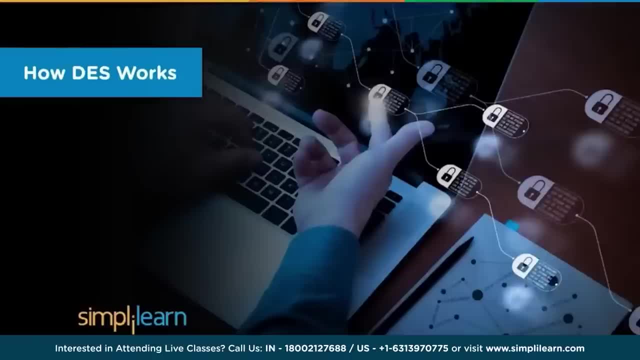 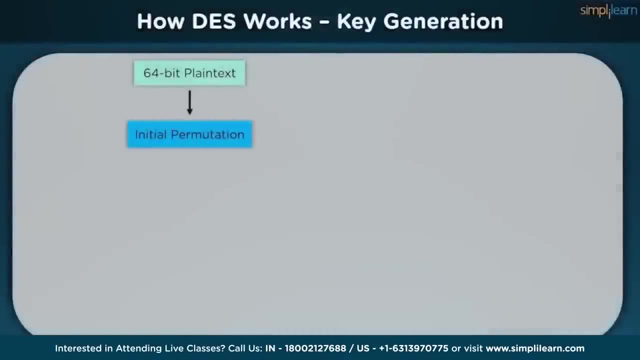 In simple terms, DES takes a 64-bit plaintext and converts it into a 64-bit ciphertext And since we are talking about asymmetric algorithms, the same key is being used when it is decrypting the data as well. We first take a 64-bit plaintext and we pass it through an initial permutation function. 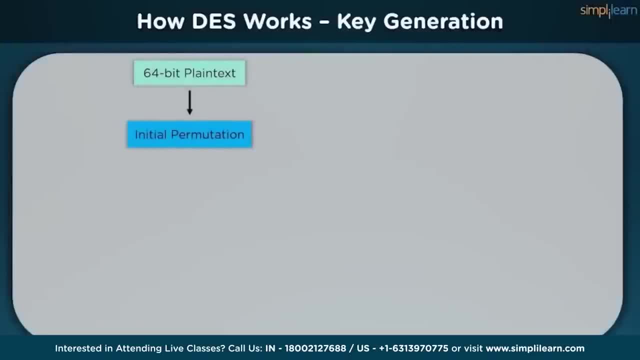 The initial permutation function has the job of dividing the block into two different parts so that we can perform VSTL cipher structures on it. There are multiple ways to do this. There are multiple ways to do this. There are multiple rounds being procured in the DES algorithm, namely 16 rounds of VSTL. 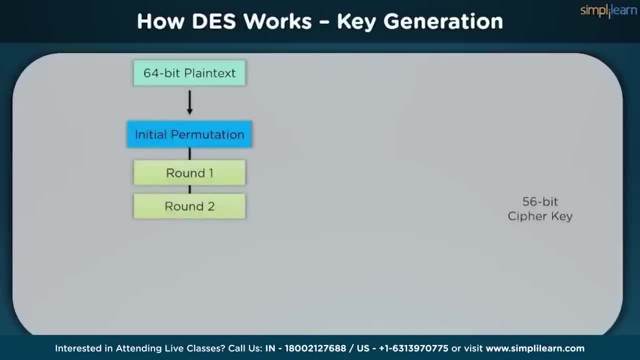 cipher structure. Each of these rounds will need keys. Initially we take a 56-bit cipher key, but it is a single key. We pass it on to a round key generator, which generates 16 different keys for each single round that the VSTL cipher is being run. 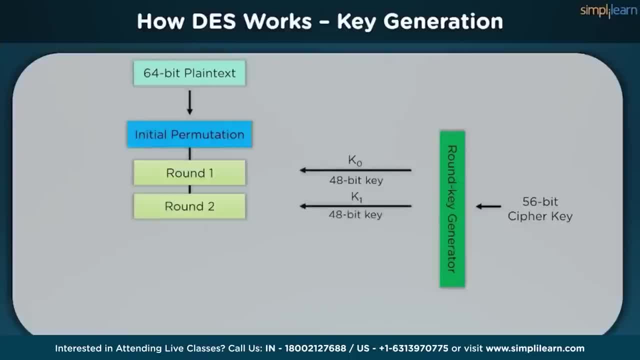 These keys are passed on to the rounds as 48 bits. The size of these 48-bit keys is the reason we use the substitution and permutation bonds in the polynomial functions of the VSTL ciphers. When passing through all these rounds, we reach round 16, where the final key is passed. 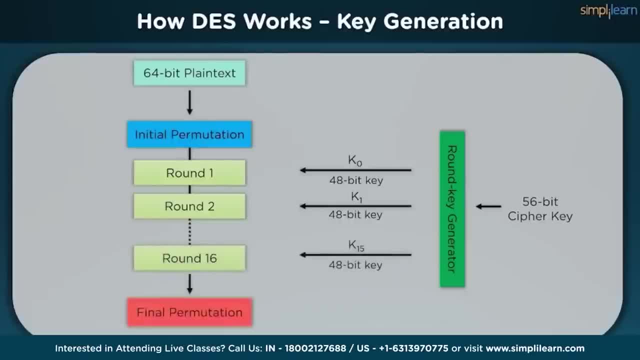 on from the round key generator and we get a final permutation. In the final permutation, the rounds are swapped and we get a final ciphertext. This is the entire process of DES, with 16 rounds of VSTL ciphers encompassed in it. 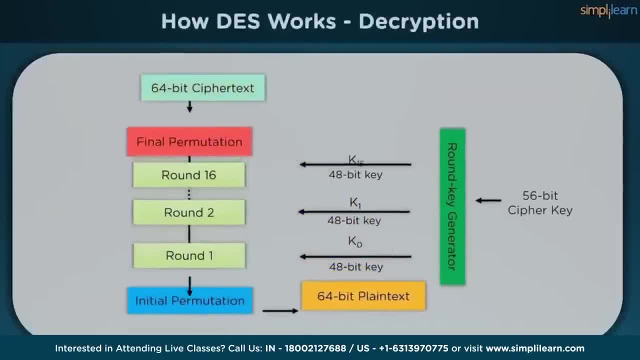 To decrypt a ciphertext back to the plaintext, we just have to reverse the process we did in the DES algorithm and reverse the process we did in the VSTL algorithm. This kind of simplicity is what gave DES the bonus when it comes to speed, but eventually. 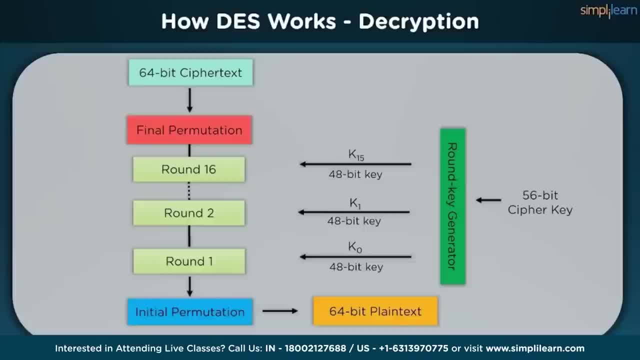 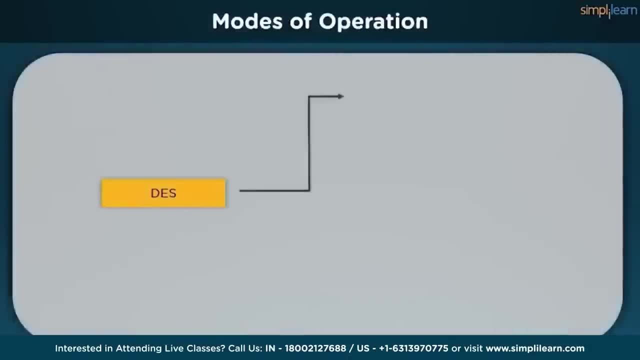 it was detrimental to the overall efficiency of the program. when it comes to security factors, DES have 5 different modes of operation to choose from. One of those is electronic codebook. Each 64-bit block is encrypted and decrypted independently in the electronic codebook format. 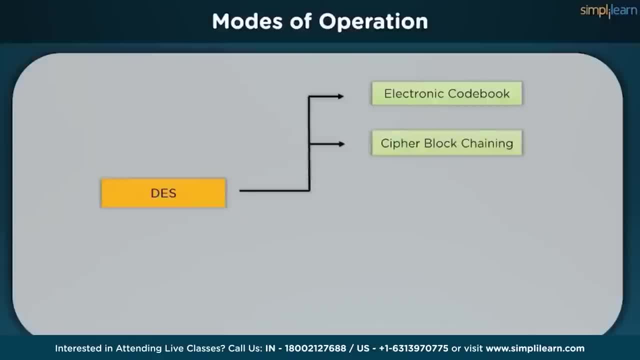 We also have cipherblockchaining or the CBC method. Here, each 64-bit block depends on the previous one, and all of them use an initialization vector. We have a cipherfeedback block mechanism where the preceding ciphertext becomes the input for the encryption algorithm. 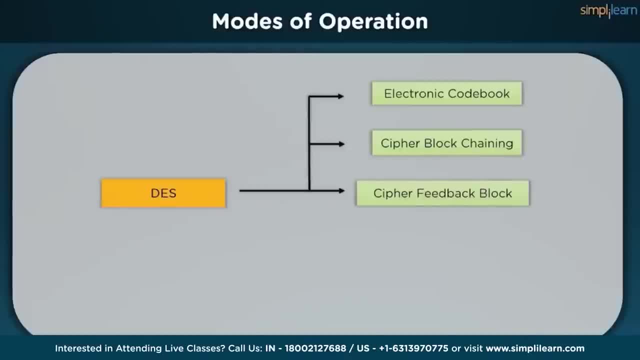 It produces a pseudo-random output which in turn, is XORed with the plaintext. There is an output-feedback method as well, which is the same as cipherfeedback, except that the encryption algorithm input is the output from the preceding DES. A counter method has a different way of approach, where each plaintext block is XORed with an. 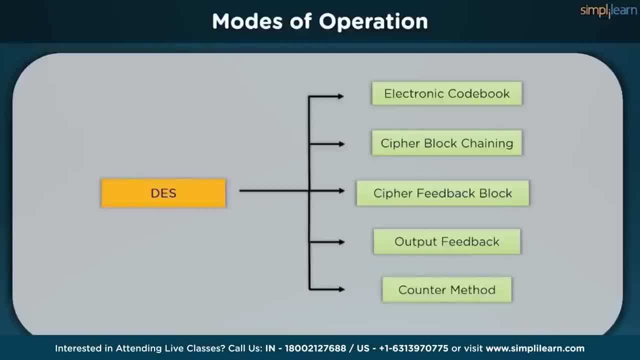 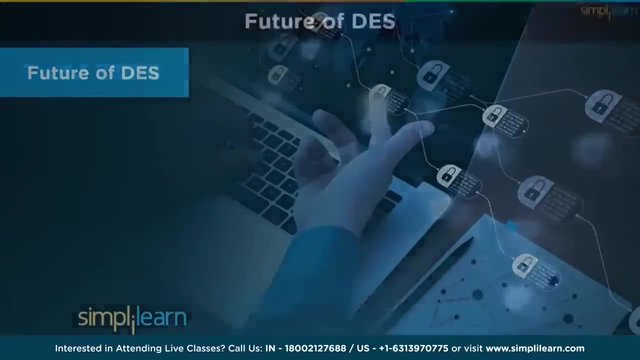 encrypted counter. The counter is then incremented for each subsequent block. There are a few other alternatives to these modes of operation, but the 5 mentioned above are the most widely used in the industry and recommended by cryptographers worldwide. Let's take a look at the future of DES. 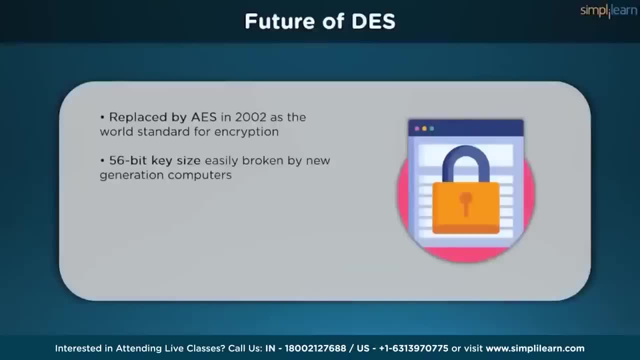 The dominants of DES ended in 2002 when their Advanced Encryption was invented. They have died more than 32,000 times and now they are just in the construction phase. standard replaced the DES encryption algorithm as the accepted standard. it was done following: 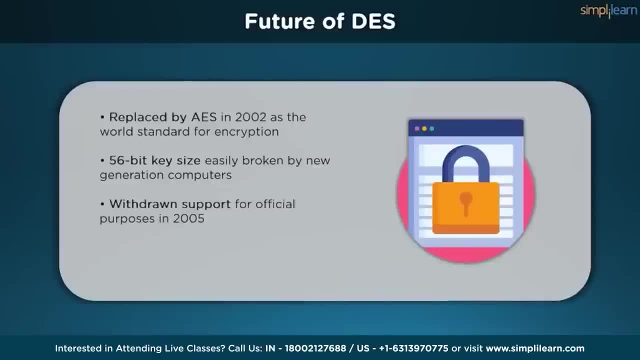 a public competition to find a replacement. NIST officially withdrew the global acceptance standard in May 2005,, although Triple DES has approved for some sensitive government information through 2030.. NIST also had to change the DES algorithm because its key length was too short, given the increased processing power of the new computers. Encryption power: 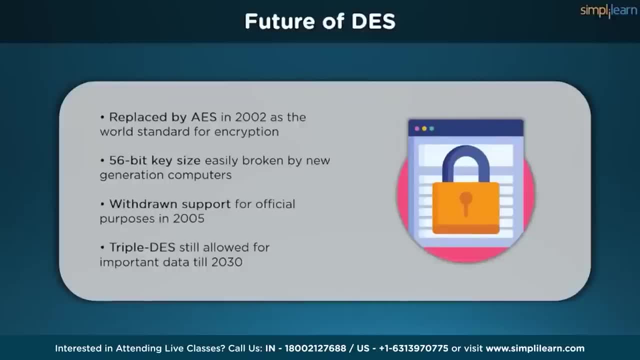 is related to the size of the key, and DES found itself a victim of ongoing technological advances in computing. We have received a point where 56-bit was no longer a challenge to the computers of cracking. Note that because DES is no longer the NIST federal standard. 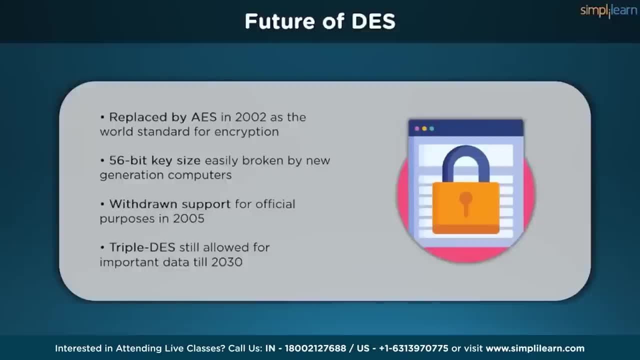 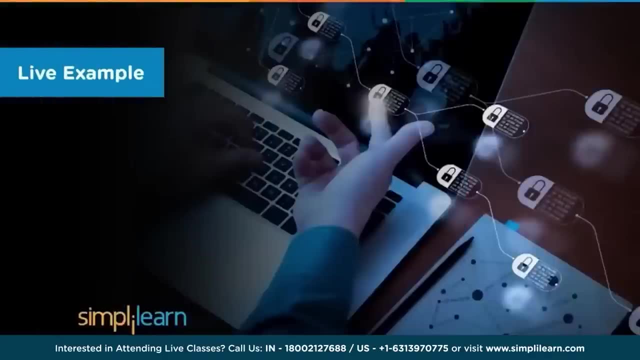 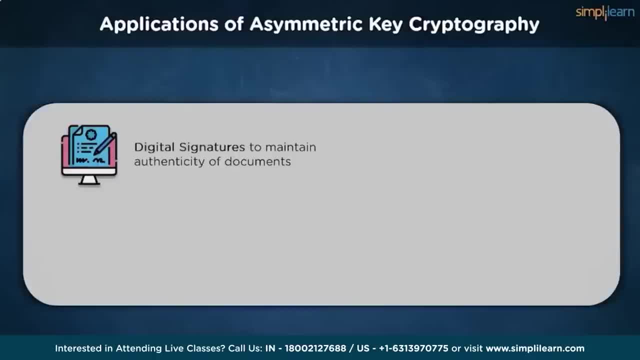 tool called CYPHERTEXT. We can use an online tool called CYPHERTEXT. We can use an online. Anyone who needs to verify the authenticity of such signatures can use the sender's public key to decrypt the signature. Since the public and the private keys are linked to each other mathematically, It's impossible to repeat this verification with duplicate keys. 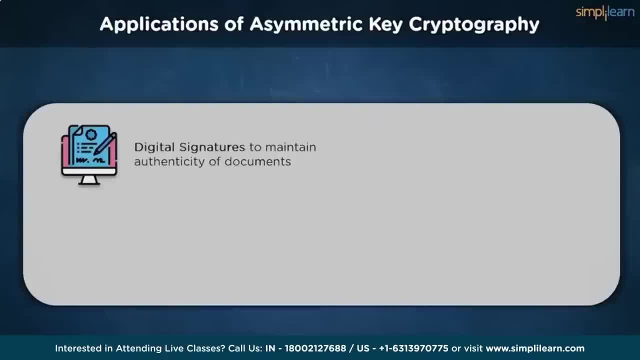 Document encryption has been made very simple by today's standards, but the background implementation follows a similar approach. In blockchain architecture, asymmetric key cryptography is used to authorize transactions and maintain the system Thanks to its two key structures. changes are reflected across the blockchains peer-to-peer network only if it is approved from both ends. 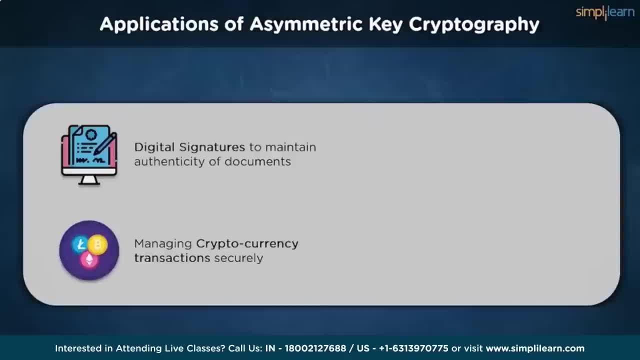 Along with asymmetric key cryptography. stamp up of architecture, its non-repudiation Characteristic, also helps in keeping the network stable. We can also use asymmetric key cryptography combined with symmetric key cryptography to monitor SSL or TLS encrypted Browsing sessions to make sure nobody can steal up personal information when accessing banking websites. 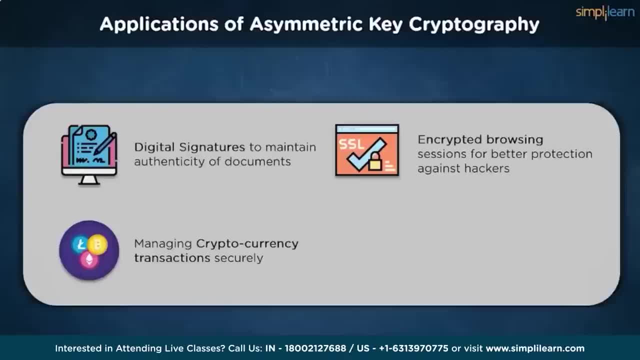 or the Internet in general. it plays a significant role in verifying websites of authenticity, Exchanging the necessary encryption keys required and generating a session using those keys to ensure maximum security, Instead of the rather insecure HTTP website format. Security parameters differ on a session by session basis, So the verification process is consistent and utterly essential to modern data security. 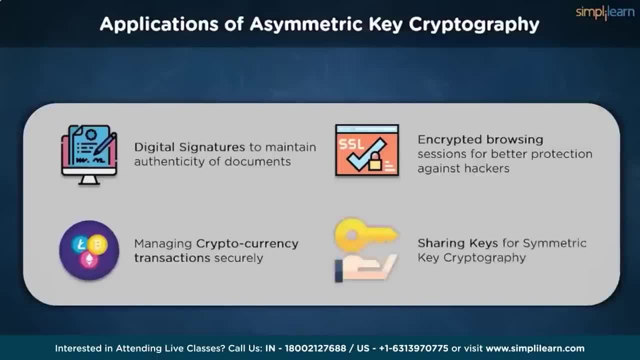 Another great use of the asymmetric key cryptography structure is transmitting keys For symmetric key cryptography, with the most significant difficulty in symmetric encryption being key exchange. asymmetric keys can help clear the shortcoming. The original message is first encrypted using a symmetric key. The key used for encrypting the data is then converted into the ciphertext using the receivers public key. 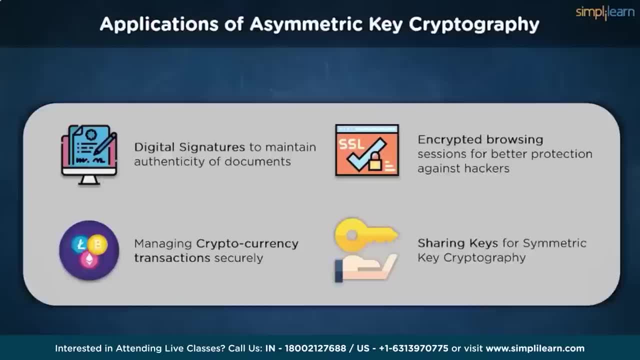 Now we have two ciphertext to transmit to the receiver. on Receiving both of them, the receiver uses his private key to decrypt the symmetric key. He can then use it to decrypt the original information on Getting the key used to encrypt the data, while this may seem more complicated than just asymmetric key cryptography alone. 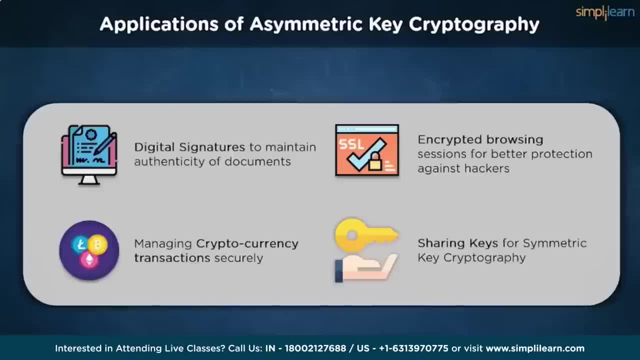 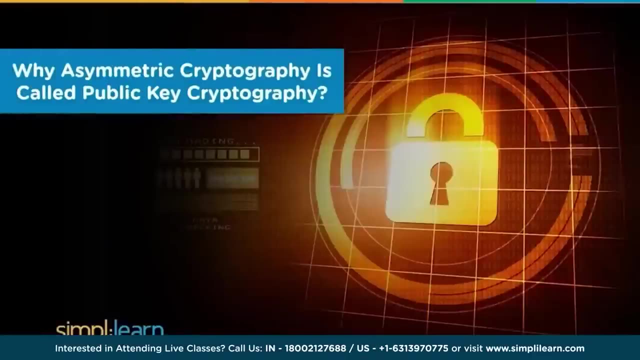 Symmetric encryption algorithms are much more optimized for vast amounts of data. on some occasions, Encrypting the key using asymmetric algorithms will definitely be more memory efficient and secure. You might remember us discussing why symmetric encryption was called private key cryptography. Let us understand why asymmetric falls under the public key cryptography. 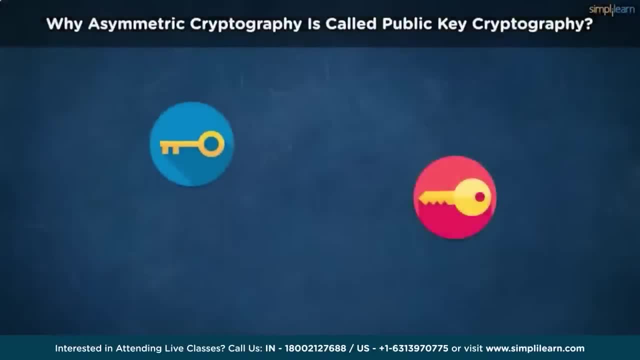 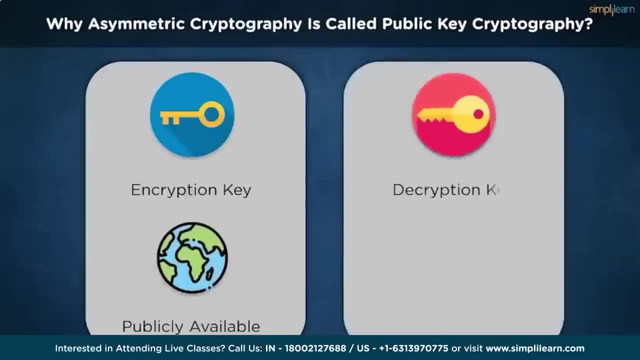 We have two keys at our disposal. The encryption key is available to everyone. The decryption key is supposed to be private. Unlike symmetric key cryptography, There is no need to share anything privately to have an encrypted messaging system. to put that into perspective, We share our email address with anyone looking to communicate with us. 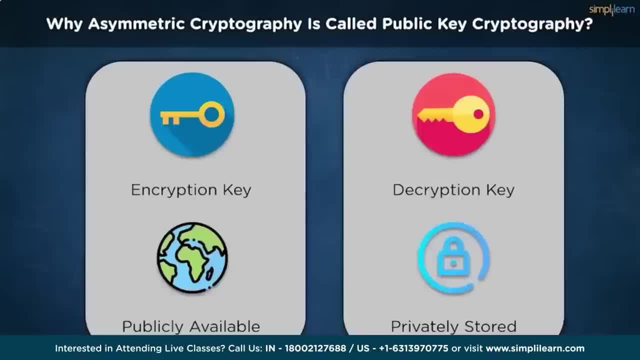 It is supposed to be public by design, so that our email login credentials are private and they help in preventing any data mishandling, Since there is nothing hidden from the world if they want to send us any encrypted information. this category is called the public key cryptography. 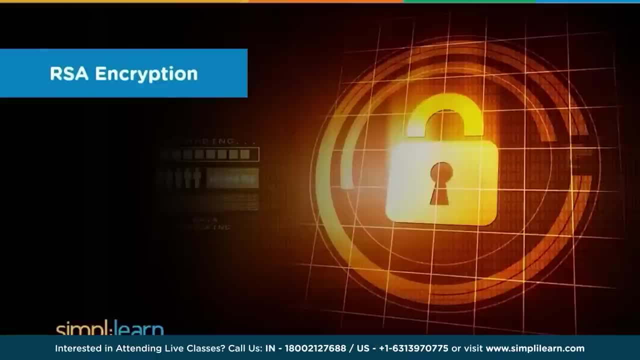 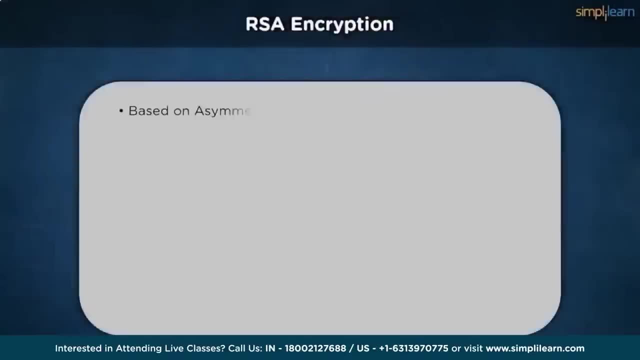 There are quite a few algorithms being used to follow the blockchain's associate with some Raspberry Optimus. I favor the RSC encryption. RSC encryption is the most widely used encryption or public key encryption standard using asymmetric key approach, Named after its founders Rivest, Shamir and Edelman. 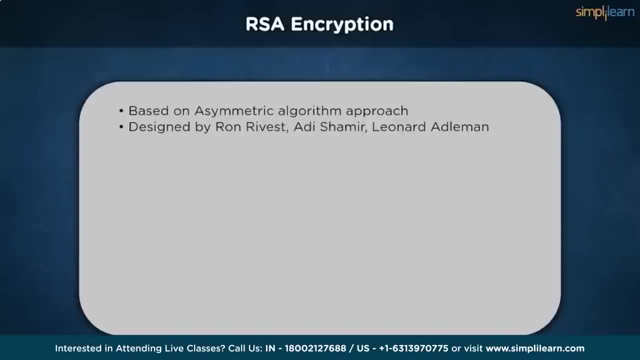 It uses blocks proportionally- block ciphers- to obscure the information. If you are unfamiliar with how block ciphers work, they are encryption algorithms that divide the original data into blocks of equal size. The block size depends on the exact cipher being used. Once they are broken down, these blocks are encrypted individually and later chained together. 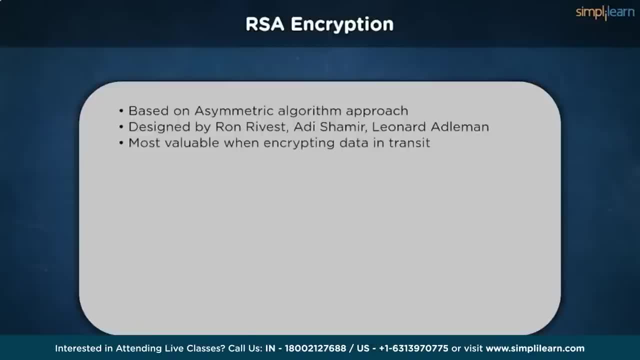 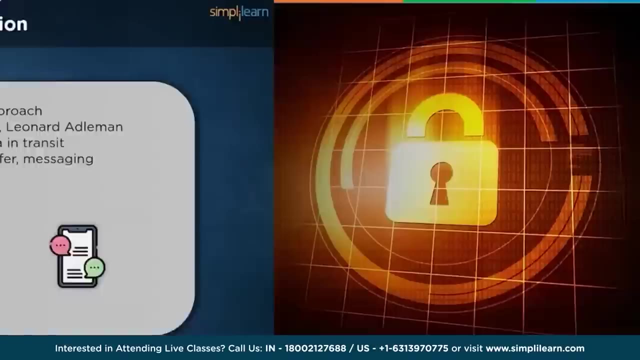 to form the final ciphertext. Widely considered to be the most secure form of encryption, albeit relatively slower than symmetric encryption algorithms. it is widely used in web browsing, secure identification, VPNs, emails and other chat applications. With so many variables in play, there must be some advantages that give asymmetric key. 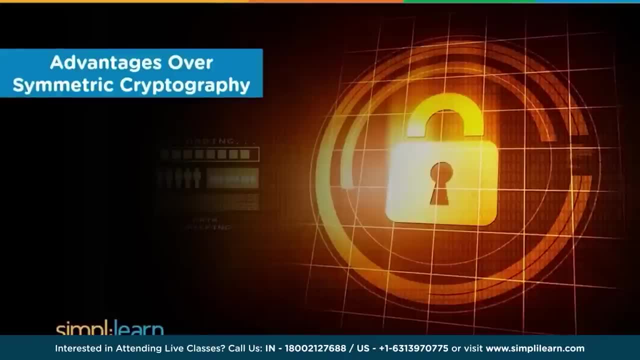 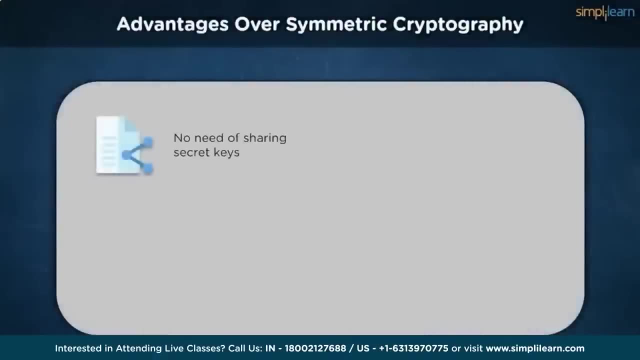 cryptography an edge over the traditional symmetric encryption methodologies. Let's go through some of them. There is no need for any reliable key-sharing channel in asymmetric encryption. It was an added risk in private key cryptography. that has been completely eliminated in public key architecture. 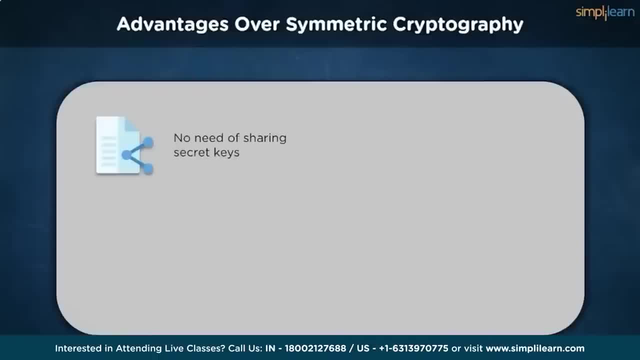 The key which is made public cannot decrypt any confidential information, and the only key that can decrypt doesn't need to be shared publicly under any circumstance. We have much more extensive key lengths in RSA encryption and other asymmetric algorithms like 2048-bit key and 4096-bit keys. 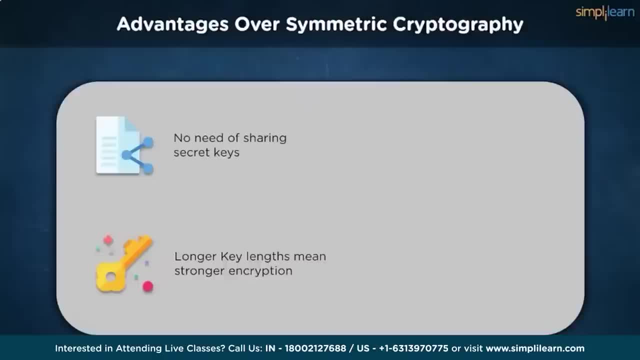 Larger keys are much harder to break into via brute force and are much more secure. Asymmetric key cryptography can be used in many ways. It can be used as a proof of authenticity, since only the rightful owner of the keys can generate the messages to be decrypted by the private key. 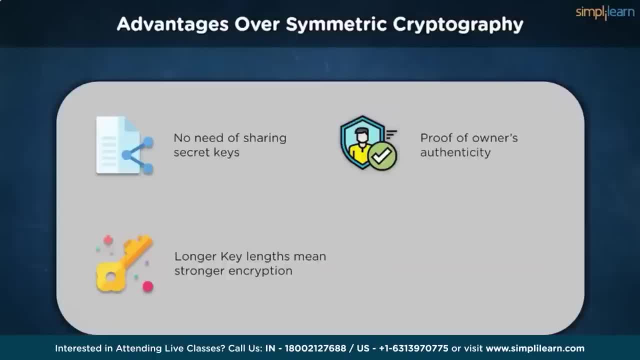 The situation can also be reversed: Encryption is done using a private key and decryption is done by the public key, which would not function if the correct private key is not used to generate the message, hence proving the authenticity of the owner. It also has a tamper protection feature where the message cannot be intercepted and changed. 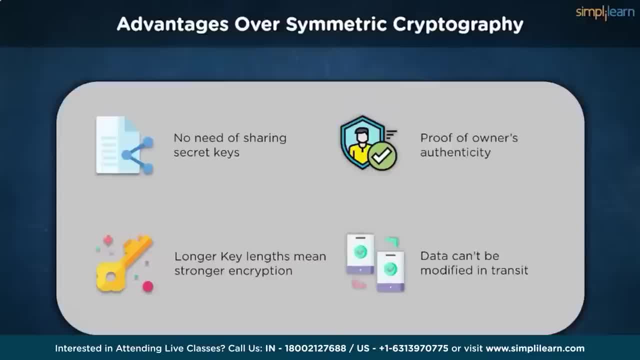 without invalidating the private key used to encrypt the data. Consequently, it can be used as a proof of authenticity, since only the rightful owner of the keys can generate the messages to be decrypted by the private key. The public key cannot decrypt the message and it is easy to realize the information. 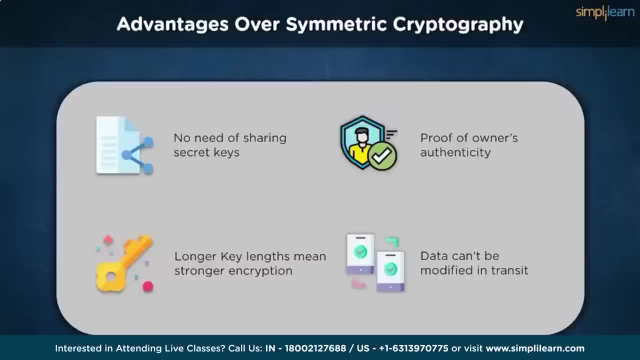 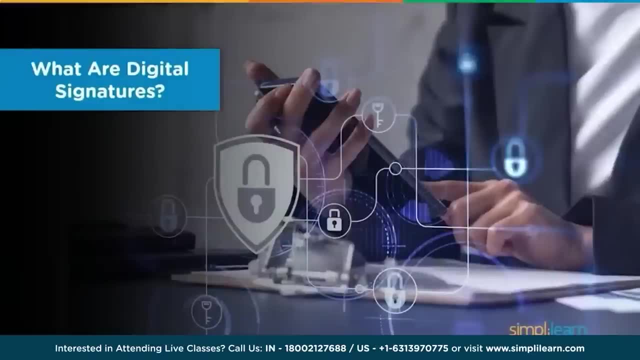 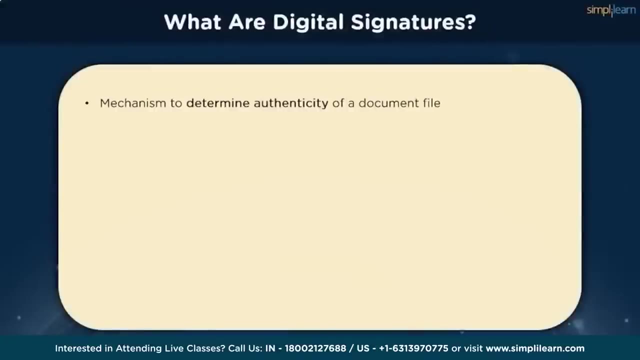 is not 100% legitimate when and where the case requires. Now that we have a proper revision, let's understand what digital signatures are before moving on to the algorithm. The objective of digital signatures is to authenticate and verify documents and data. This is necessary to avoid tampering and digital modification or forgery of any kind during 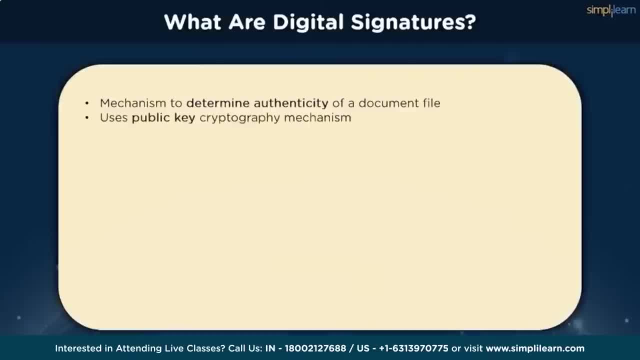 the execution of official documents. They work on the public key cryptography architecture, with one exception. Typically, an asymmetric key system encrypts using a public key and decrypts with a private key. For digital signatures, however, the reverse is true: The signature is encrypted using a private key and is decrypted with the public key. 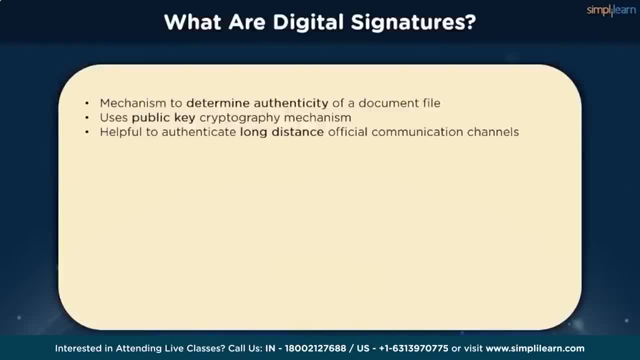 Because the keys are inked together. decoding it with the public key verifies that the proper private key was used to sign the document. Let's go through each step to understand the procedure thoroughly. In step 1, we have M, which is the original plain text message, and it is passed onto. 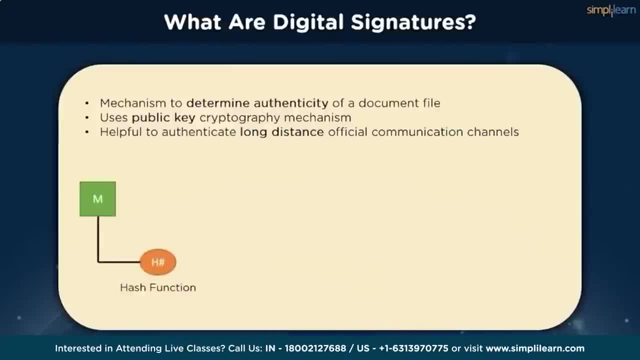 a hash function denoted by H hash to create a digest. Next, it bundles the message together with the hash digest and encrypts it using the sender's private key. Next, it sends the encrypted message to the public key. Next, it sends the encrypted message to the private key. 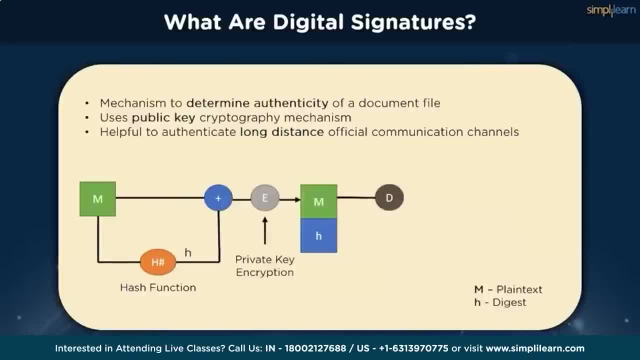 Next, it sends the encrypted message to the public key. Next, it sends the encrypted message to the private key. Next, it sends the encrypted message to the receiver, who can decrypt it using the sender's public key. Once the message is decrypted, it is passed through the same hash function: H hash to generate. 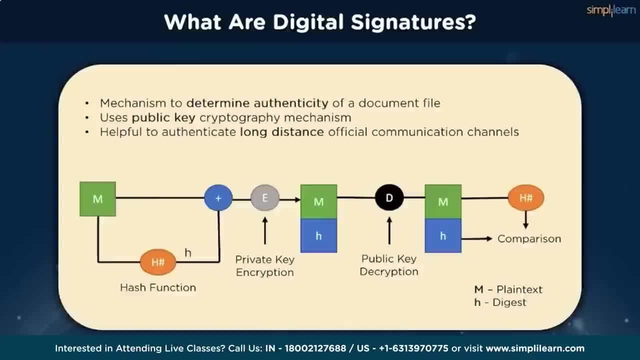 a similar digest. It compares the newly generated hash with the bundled hash value received, along with the message. If they match, it verifies data integrity. In many instances, they provide a layer of validation and security to messages through non-secured channels. Properly implemented, a digital signature gives the receiver reason to believe that. 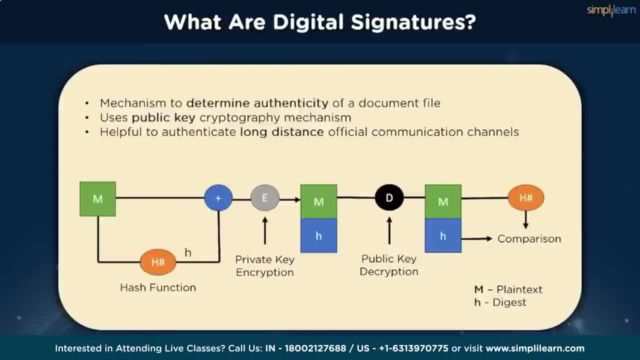 the message was sent by the claimed sender. Digital signatures are equivalent to traditional handwritten signatures in many respects, but properly implemented digital signatures are more difficult to forge than the handwritten type. Digital signature schemes, in the sense used here, are cryptographically based and must. 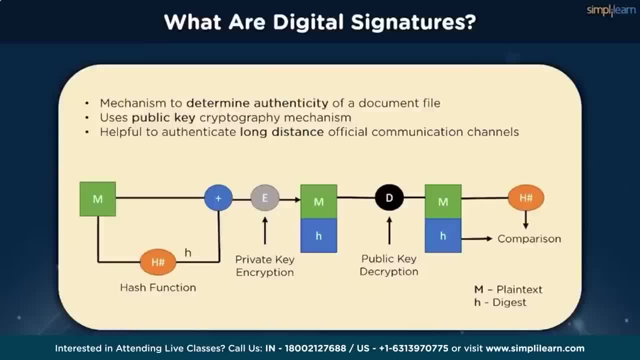 be implemented properly to be effective. They can also provide non-repudiation, meaning that the signer cannot successfully connect to the private key. In the case of a private key, the signer can easily claim that they did not sign a message while also claiming their private key remains secret. 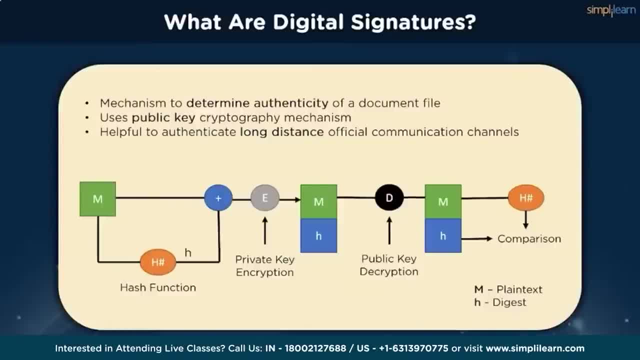 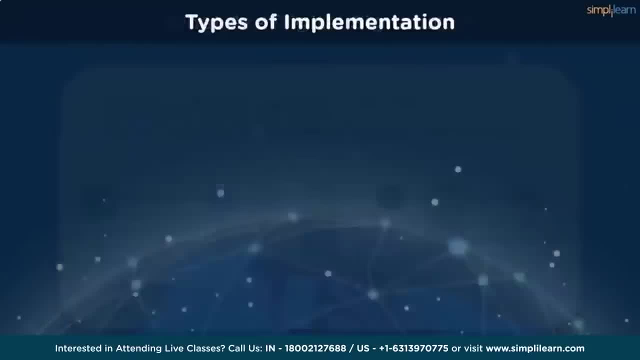 Further, some non-repudiation schemes offer a timestamp for the digital signature so that, even if the private key is exposed, the signature is valid. To implement the concept of digital signature in real world, we have two primary algorithms to follow. 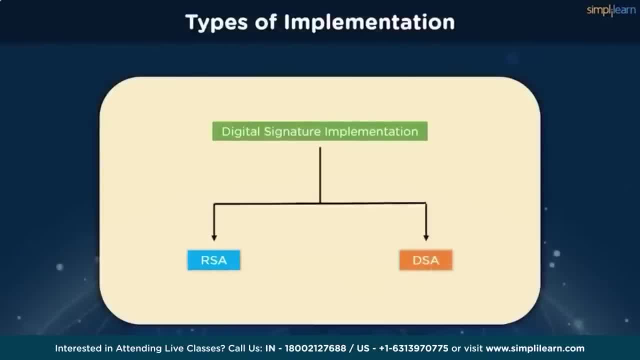 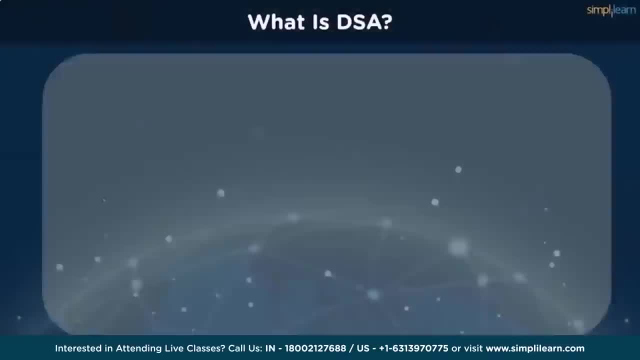 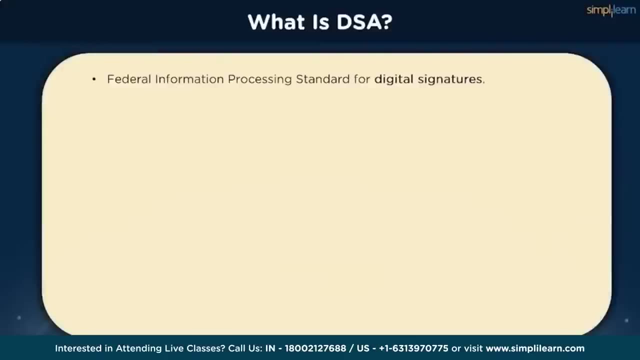 So let's go ahead and see what the DSA algorithm is. So let's go ahead and see what the DSA algorithm is. The DSA algorithm is a FIPA standard, which is a Federal Information Processing standard for digital signatures. 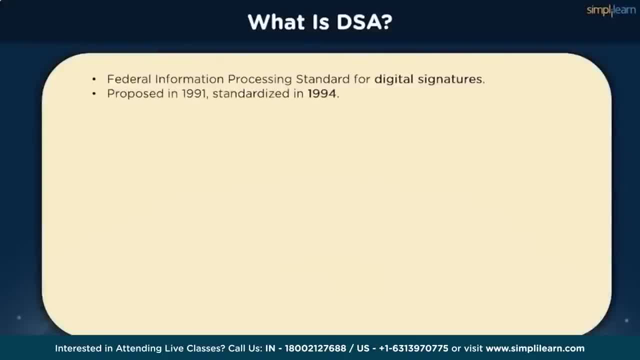 It was proposed in 1991, and globally standardized in 1994 by the National Institute of Standards and Technology. It functions on the framework of modular, exponential and discrete logarithmic problems which are difficult to compute as a force brewed system. Unlike DSA, most signature types are generated by signing message digest with the private. 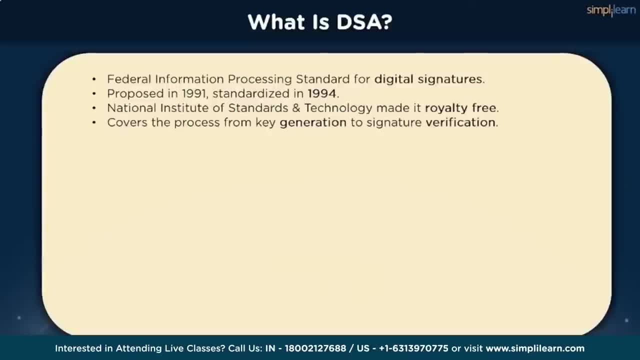 key of the originator. This creates a digital thumbprint of the data. Since just the message digest is signed, the signature is generally much smaller compared to the data that was signed. As a result, digital signatures impose less load on processors at the time of signing. 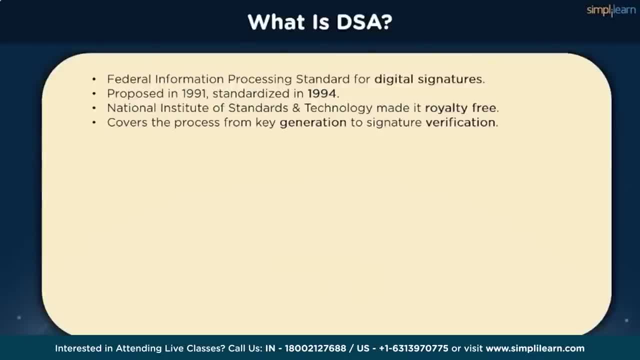 execution and they use small volumes of bandwidth. DSA, on the other hand, does not encrypt message digest using private key or decrypt message digest using public key. Instead, it uses mathematical functions to create a digital signature consisting of two 160-bit numbers, which are originated from the message digests and the private key. 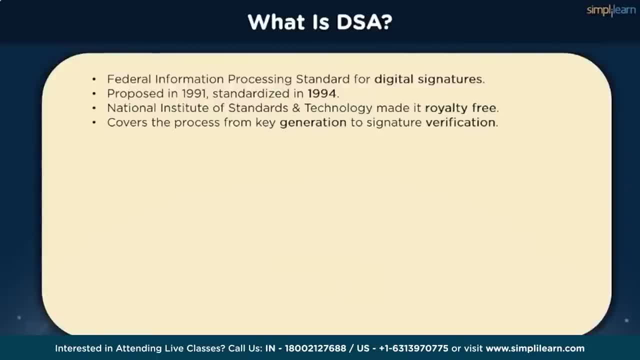 DSAs make use of the public key for authenticating the signature, but the authorization process is much more complicated when compared with RSA. DSA also provides three benefits, Which is the message: authentication, integrity, verification and non-repudiation. In the image, we can see the entire process of DSA validation. 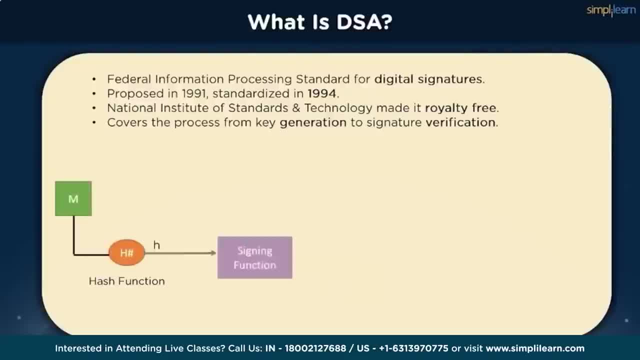 A plain text message is passed onto a hash function where the digest is generated, which is passed onto a signing function. Signing function also has other parameters, like a global variable g, a random variable k and the private key of the sender. The outputs are then bundled onto a single pack with a plain text. 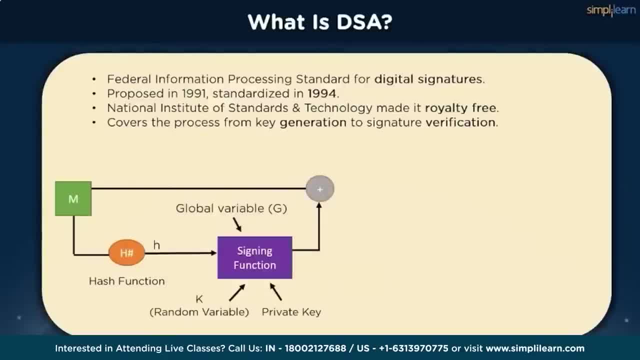 The plain text is then sent to the receiver. The two outputs we receive from the signing functions are the two 160-bit numbers denoted by S and R. On the receiver end we pass the plain text through the same hash function to regenerate the message digest. 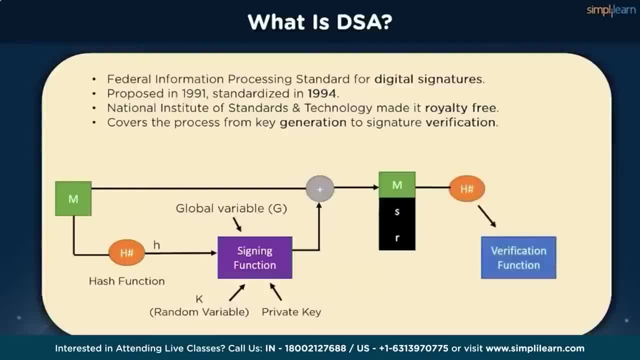 It is passed onto the verification function, which has other requirements such as the public key of the sender, global variable g and S and R received from the sender. The output we receive from the signing function is then passed onto the public key of the. 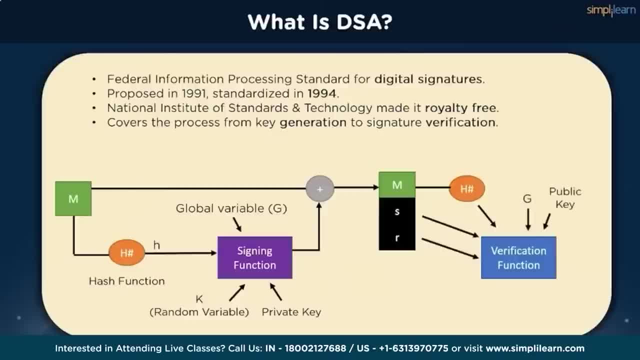 sender. The value generated by the function is then compared to R. If they match, then the verification process is complete and data integrity is verified. This was an overview of the way the DSA algorithm works. You already know it depends on logarithmic functions to calculate the outputs. 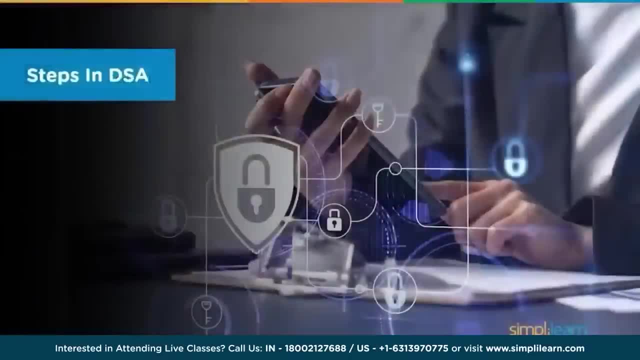 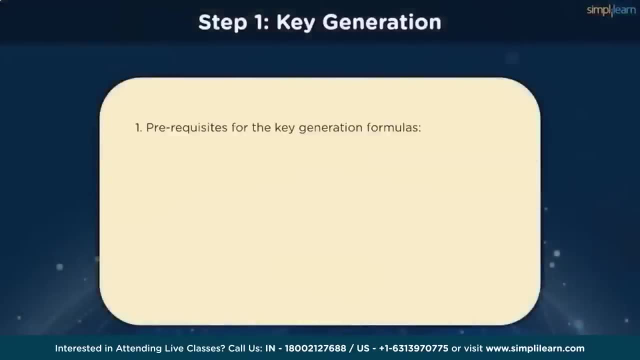 So let us see how we can do the same in our next section. We have three phases here, the first of which is key generation. To generate the keys, we need some prerequisites. We select a Q which becomes a prime divisor. We select a prime number, P, such that P minus one mod Q equal to zero. 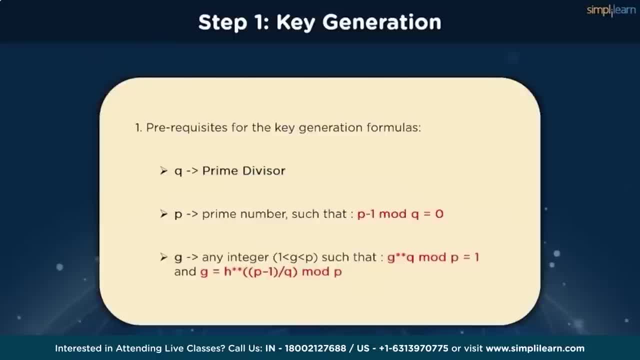 We also select a random integer G, which must satisfy the two formulas being mentioned on the screen right now. Once these values are selected, we can go ahead with generating the keys. The private key can be denoted by X and it is any random integer that falls between the. 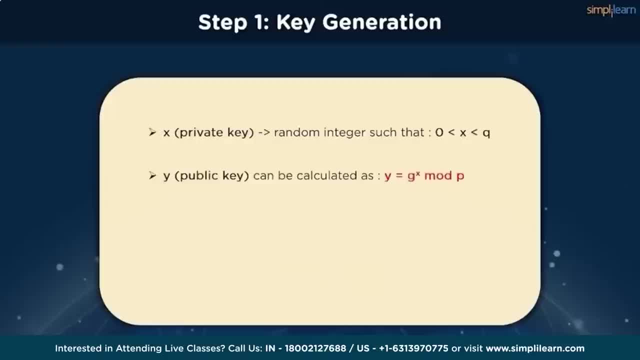 bracket of zero And the value of Q. The public key can be calculated as Y equal to G, to the power X mod P, where Y stands for the public key. The private key can then be packaged as a bundle which comprises of values of P, Q. 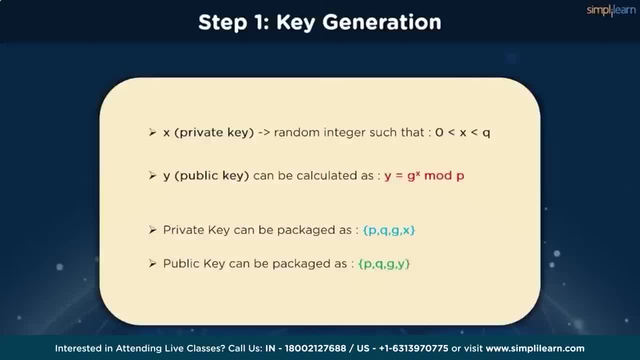 G and X. Similarly, the public key can also be packaged as a bundle having the values of P, Q, G and Y. Once we're done with key generation, we can start verifying the solution. Once the keys are generated, we can start generating the signature. 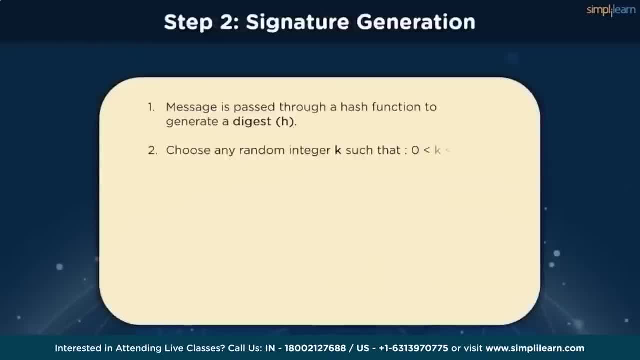 The message is passed through a hash function. to generate the digest edge first We can choose any random integer, K which falls under the bracket of zero, and Q. To calculate the first 160-bit number of a signing function of R, we use the formula: 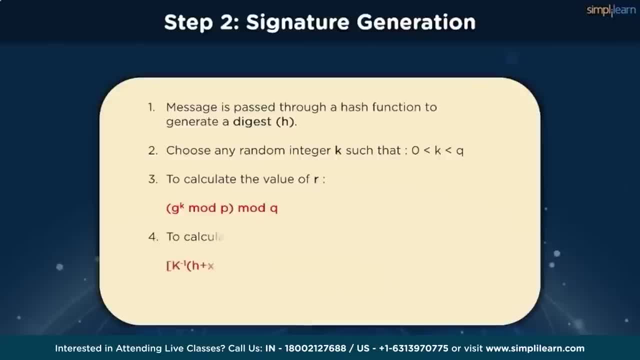 G to the power K mod P into mod Q. Similarly, to calculate the value of R, we use the formula G to the power K mod P into mod Q. To calculate the value of the second output, that is, S, we use the following formula that: 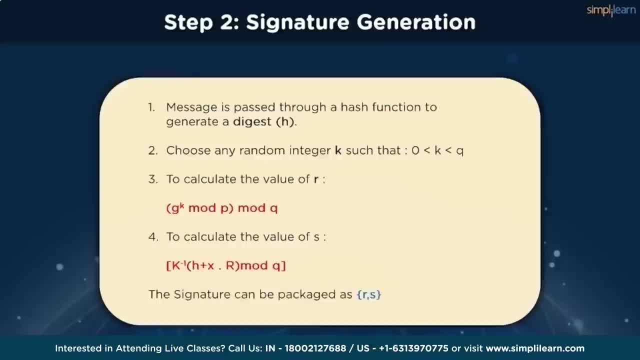 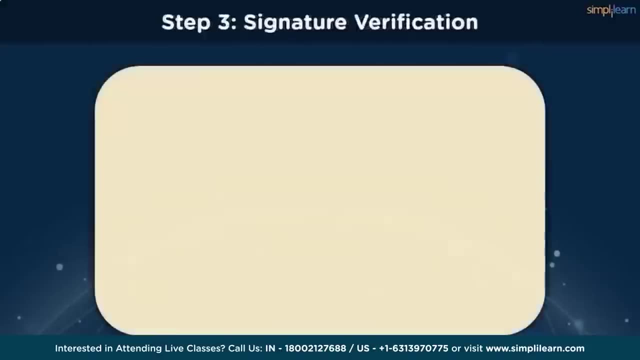 is shown on the screen. The signature can then be packaged as a bundle having R and S. This bundle, along with the plain text message, is then passed on to the receiver. Now, with the third phase, we have to verify the signature. 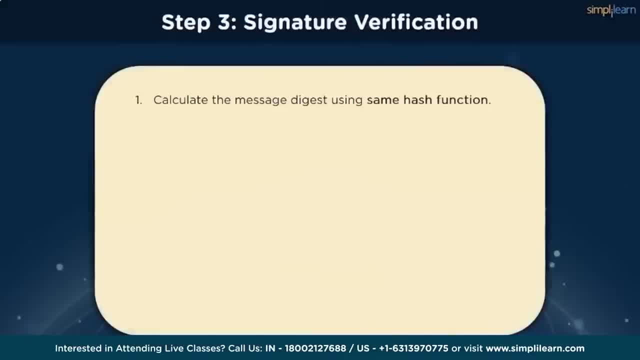 We first calculate the message digest received in the bundle by passing it through the same hash function. We calculate the value of the second output, that is, S. We use the following formula that is shown on the screen. We calculate the value of W, U1, and U2 using the formulas shown on the screen. 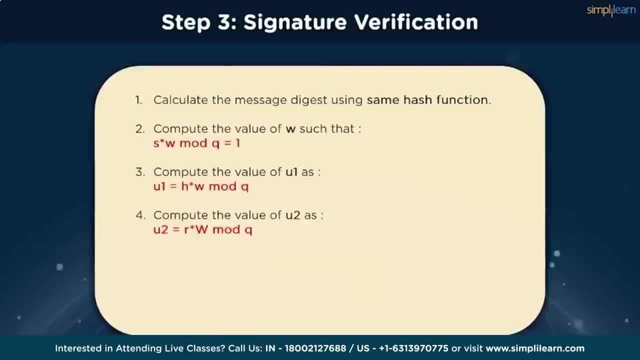 We have to calculate a verification component which is then to be compared with the value of R being sent by the sender. This verification component can be calculated using the following formula: Once calculated, this can be compared with the value of R. If the values match, then 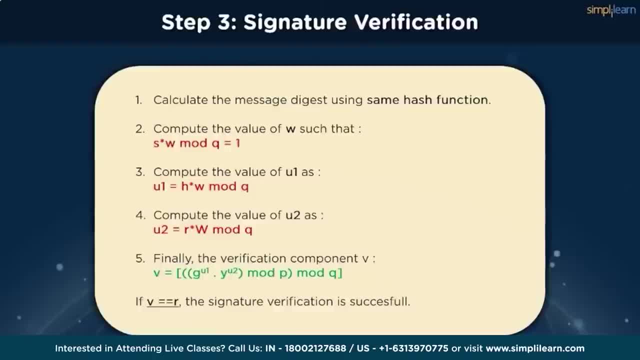 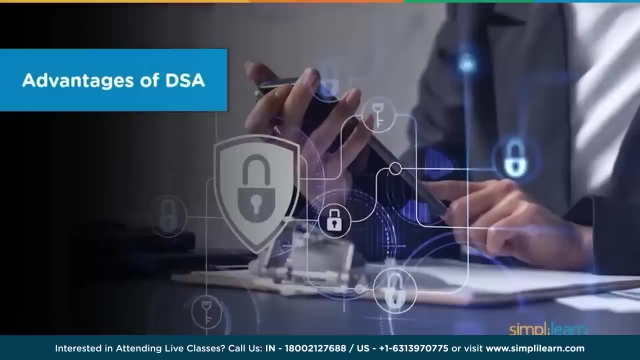 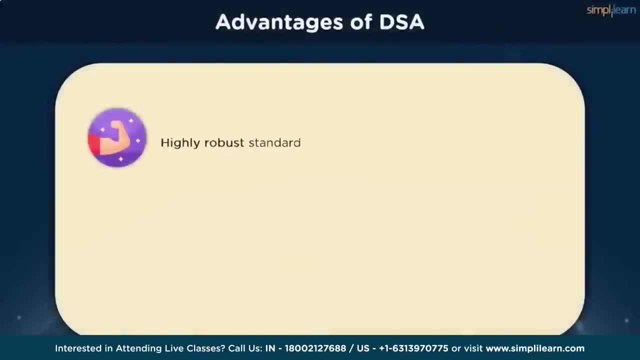 the signature verification is successful and our entire process is complete, starting from key generation to the next step. With so many steps to follow, we are bound to have a few advantages to boot. this, and we would be right to think so. DSA is highly robust in the security and stability aspect when compared to alternative signature. 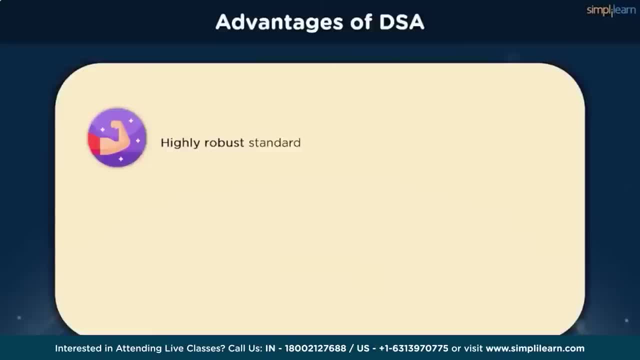 verification algorithms. We have a few other ciphers that aim to achieve the simplicity and flexibility of DSA, but it has been a tough ask for all of us. The key generation is much faster when compared to the RSA algorithm and such While the actual encryption and decryption process may falter a little in comparison. 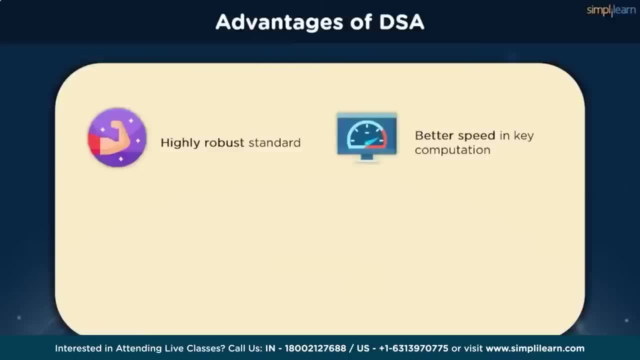 a quicker start in the beginning is well-known to optimize a lot of frameworks, DSA requires less storage space to work its entire cycle. In contrast, its direct correspondent, that is, RSA algorithm, needs a certain amount of computational and data storage space. 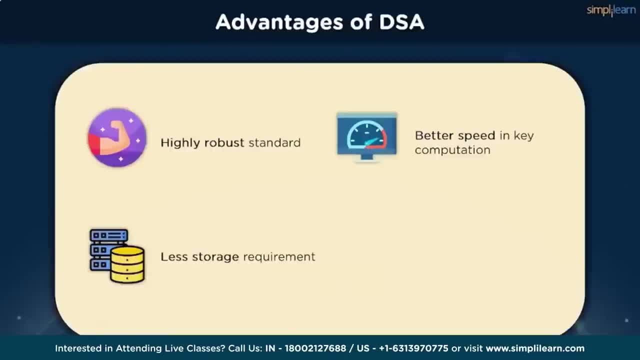 This is not the case with DSA, which has been optimized to work with weaker hardware and lesser resources. The DSA is patented, but NIST has made this patent available worldwide royalty-free. A draft version of the speculation FIPS 1865 indicates that DSA will no longer be approved. 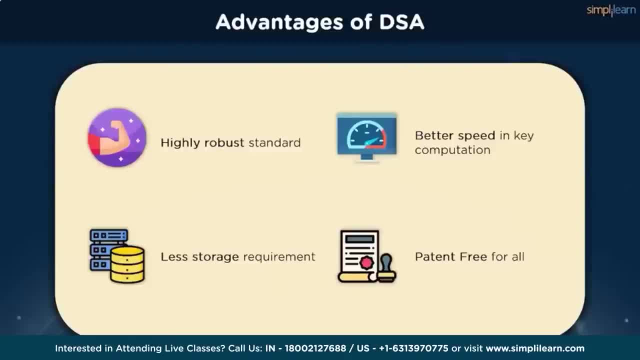 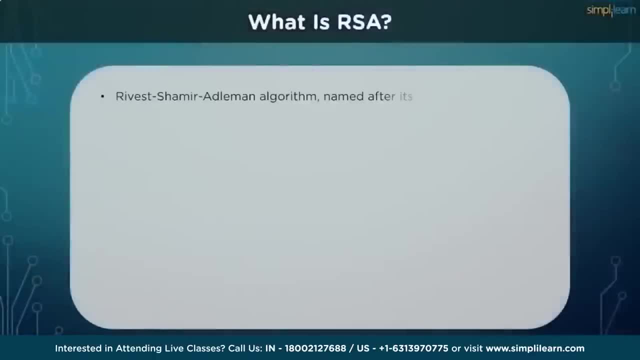 for digital signature generation, but it may be used to verify signatures generated prior to the implementation date of that standard. The RSA algorithm is a public-key signature algorithm developed by Ron Rivest, Adi Shamir and Leonard Edelman. The paper was first published in 1977 and the algorithm uses logarithmic functions to 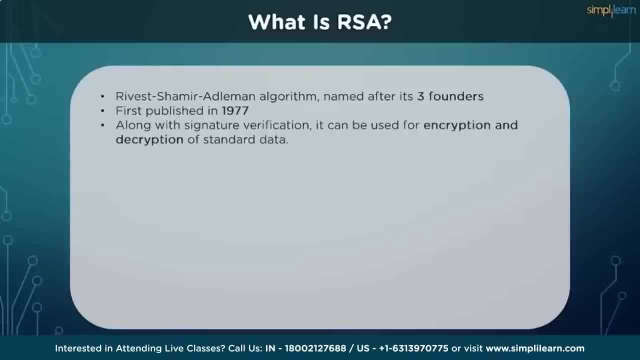 keep the working complex enough to withstand brute force and streamlined enough to be fast. post-deployment, RSA can also encrypt and decrypt general information to securely exchange data, along with handling digital signature verification. Let us understand how it achieved this. We take our plain text message M. We pass it through a hash function to generate the. 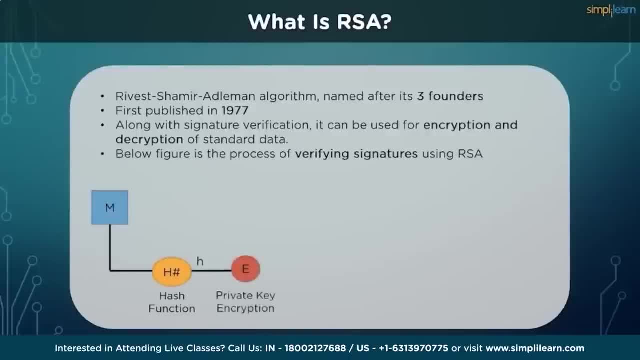 digest H, which is then encrypted using the sender's private key. This is appended to the original plain text message and sent over to the receiver. Once the receiver receives the bundle, we can pass the plain text message through the same hash function to generate a digest and the ciphertext can be decrypted using the. 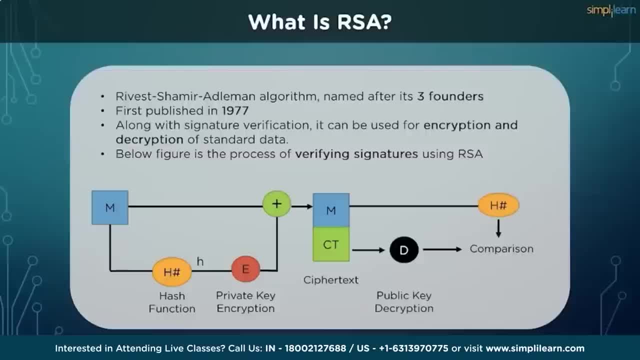 public key of the sender. The remaining hashes are compared. If the values match, then the data integrity is verified and the sender is authenticated. Apart from digital signatures, the main case of RSA is encryption and decryption of private information before being transmitted across communication channel. 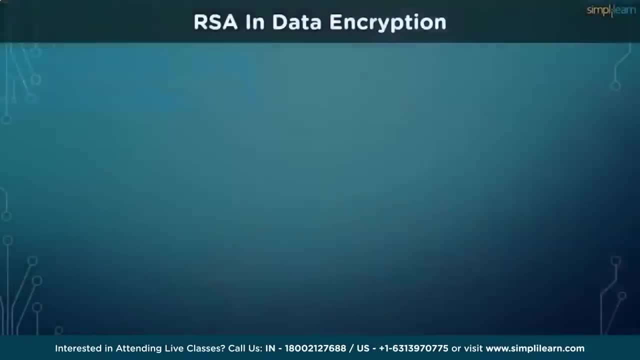 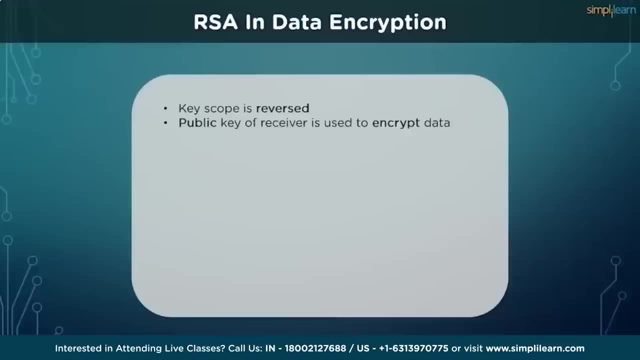 This is where the data encryption comes into play. When using RSA for encryption and decryption of general data, it reverses the key set usage. Unlike signature verification, it receives the receiver's public key to encrypt the data and uses the receiver's private key in decrypting the data. 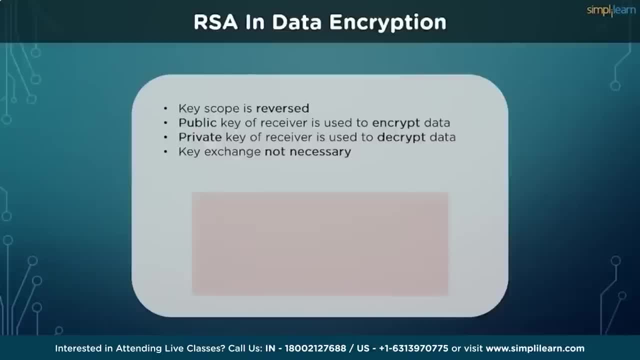 Thus, there is no need to exchange any keys in this scenario. There are two broad components when it comes to RSA cryptography. One of them is key generation. Key generation employs a step of generating the private and the public keys that are going to be used for encrypting and decrypting the data. 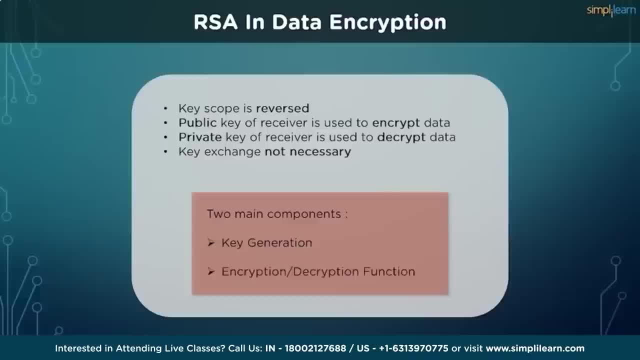 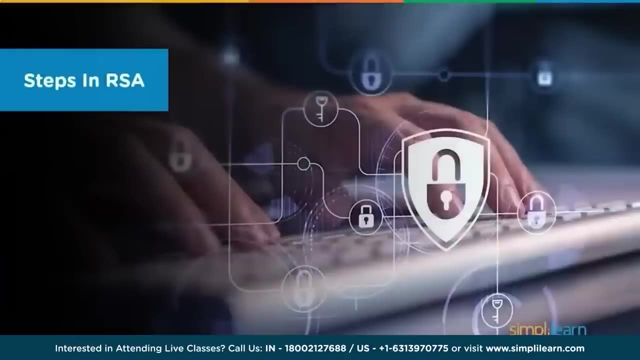 The second part is the encryption and decryption functions. These are the ciphers and steps that need to be done when scrambling the data or recovering the data from the ciphertext. You will now understand each of these steps in our next subtopic. Keeping the previous two concepts in mind, let us go ahead and see how the entire process. 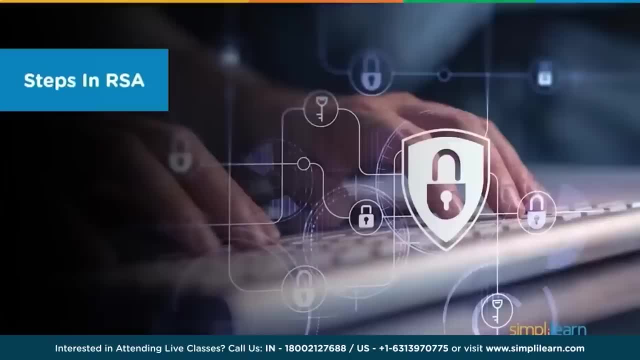 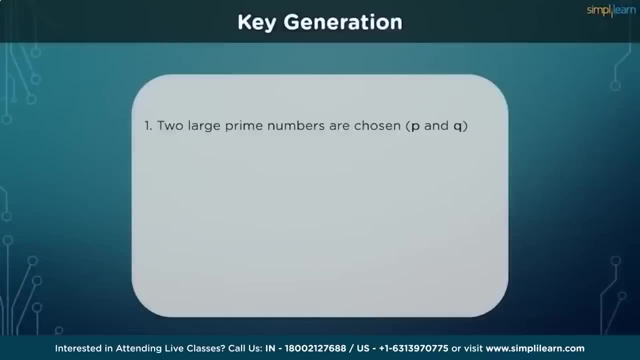 works, starting from creating the key pair to encrypting and decrypting the information. You need to generate the public and private keys before running the functions. to generate ciphertext and plaintext, They use certain variables and parameters, all of which are explained. We first use two large prime numbers. 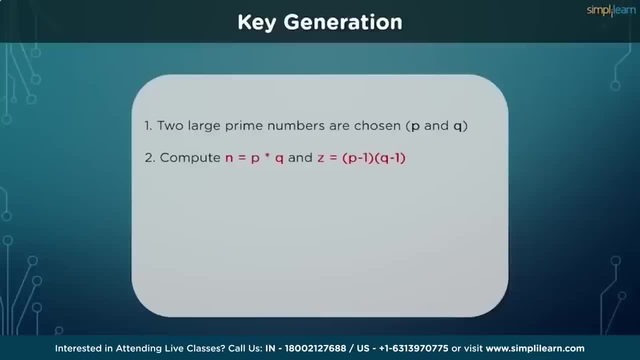 These can be denoted by p and q. We can compute the value of n as n equal to p into q and compute the value of z as p minus 1 into q minus 1.. A number e is chosen at random, satisfying the following conditions, and a number d is: 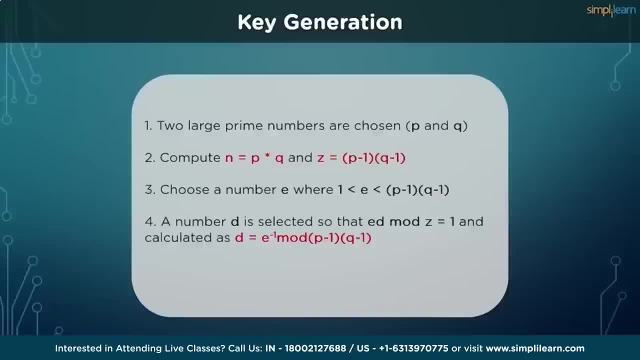 also selected at random following the formula ed mod z equal to 1, and it can be calculated with the formula given below. The public key is then packaged as a bundle with n and e. The private key is packaged as a bundle using n and d. 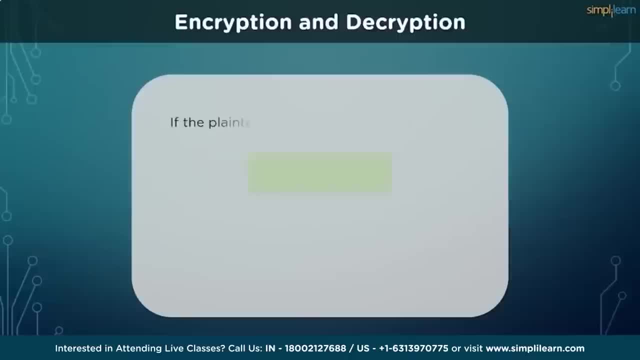 This sums up the key generation process. For the encryption and decryption function we use the formulas c and m. The ciphertext can be calculated as c equal to m to the power e mod n, and the plaintext can be calculated from the ciphertext as c power d mod n. 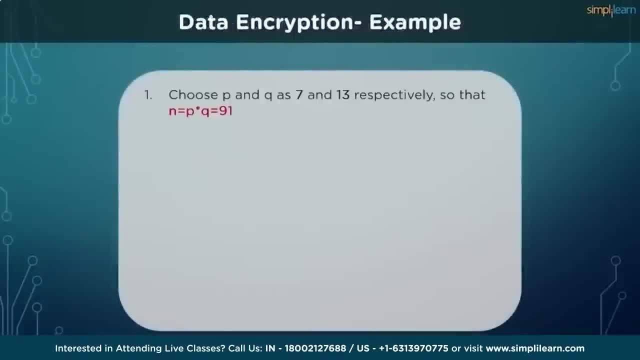 When it comes to a data encryption example, let's take p and q as 7 and 13.. The value of n can be calculated as 7 and 13.. The ciphertext can be calculated as 91.. If we select the value of e to be 5, it satisfies all the criteria that we need it to. 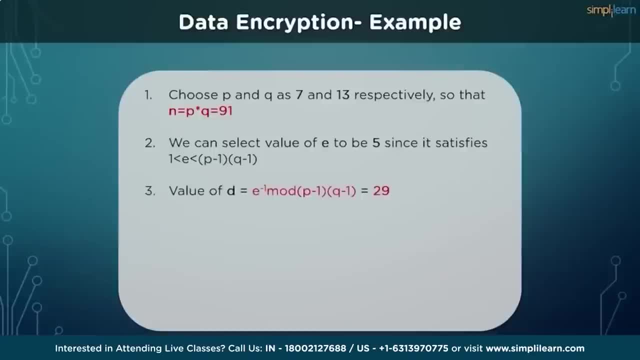 The value of d can be calculated using the following function, which gives it as 29.. The public key can then be packaged as 91 comma 5 and the private key can then be packaged as 91 comma 29.. The plaintext: if it is 10, which is denoted by m, 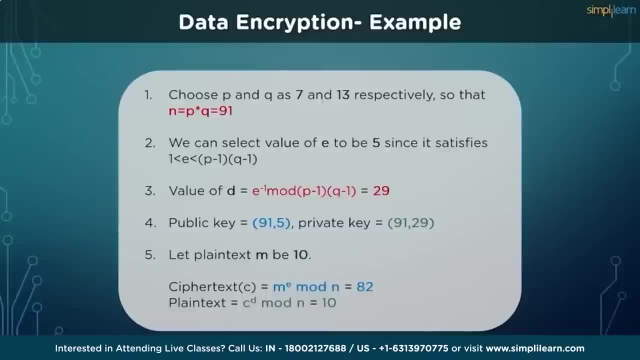 Ciphertext can be calculated to the formula c equal to m to the power e mod n. The plaintext, if it is 10, which is denoted by m, Ciphertext can be calculated to the formula c equal to m to the power e mod n which gives: 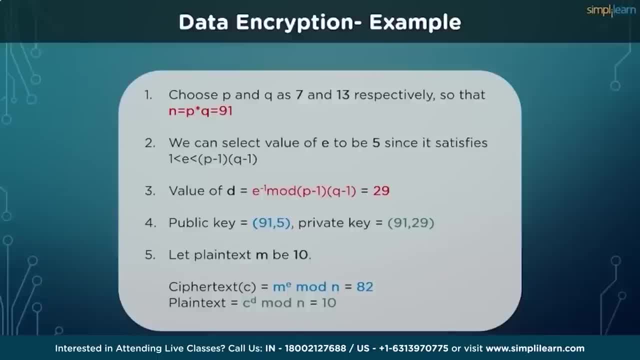 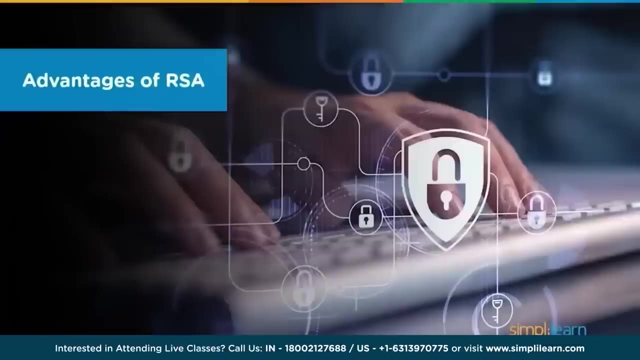 us 82.. If somebody receives this ciphertext, they can calculate the plaintext using the formula c to the power d mod n, which gives us the value of 10 as selected as our plaintext. We can now look at the factors that make the RSA algorithm stand out versus its competitors. 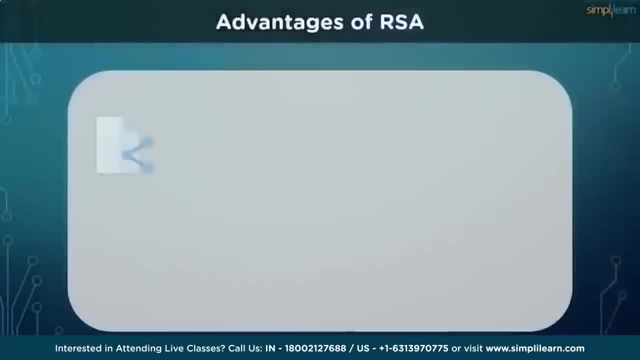 in the advantageous topics of this lesson. RSA encryption depends on using the receiver's public key, so that you don't have to share any secret key to receive the messages from others. This was the most glaring flaw faced by symmetric algorithms, which were eventually fixed by 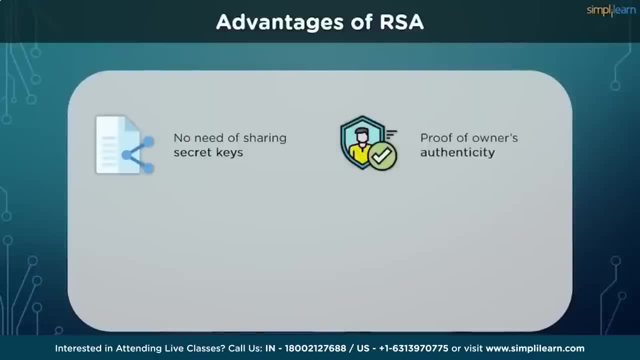 asymmetric cryptography structure. Since the key pairs are related to each other, a receiver cannot intercept the message since they didn't have the correct private keys to decrypt the information. If a public key can decrypt the information, the sender cannot refuse signing it with his. 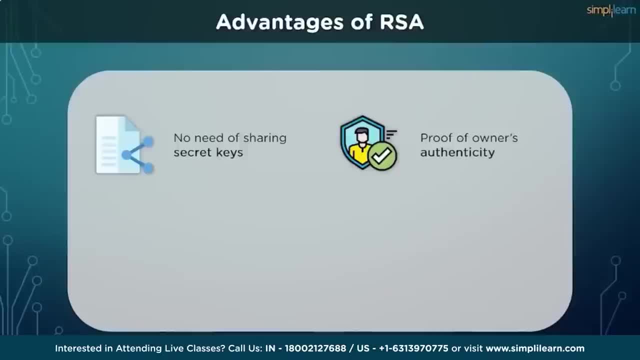 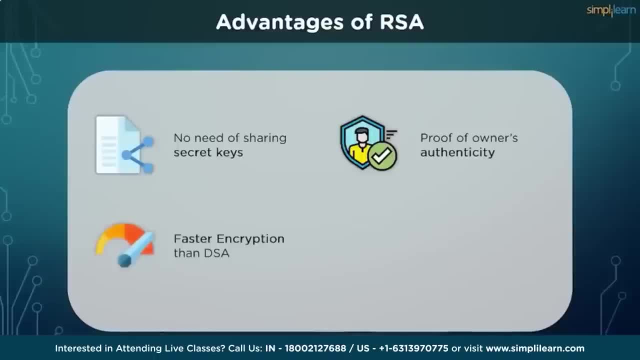 The encryption process is fast and easy. The encryption process is fast and easy. RSA encryption is faster than that of the DSA algorithm, Even if the key generation in slower in RSA. many systems across the world tend to reuse the same keys so that they can spend less time in key generation and more time on actual 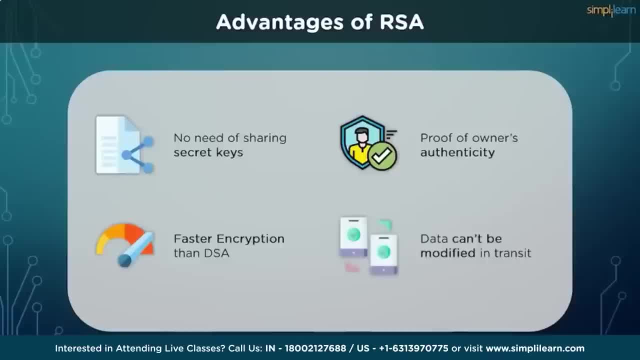 ciphertext management Data will be tamper-proof in transit, since meddling with the data will alter the usage of the keys. The private key won't be able to decrypt the information, hence alerting the receiver of any kind of manipulation in between. The receiver must be aware of any third party. 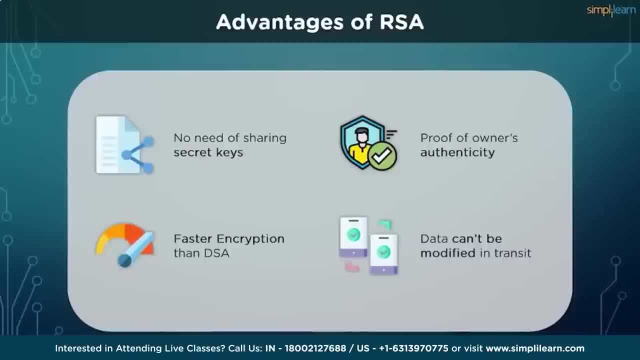 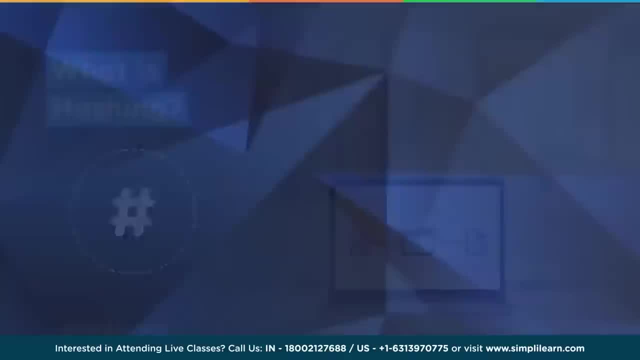 any third party who possesses the private key, since they can alter the data mid transit, the cases of which are rather low. imagine creating an account on a new website. you provide your email address and set a password that you are confident and you would not forget what about. 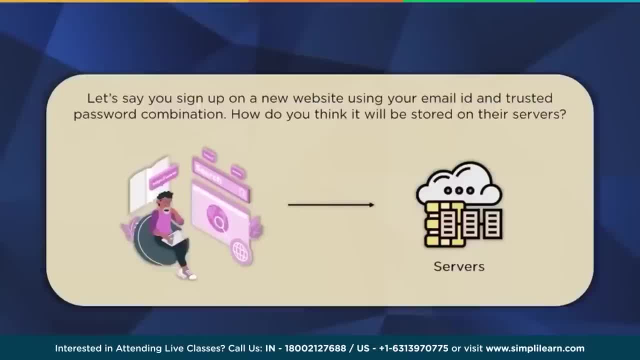 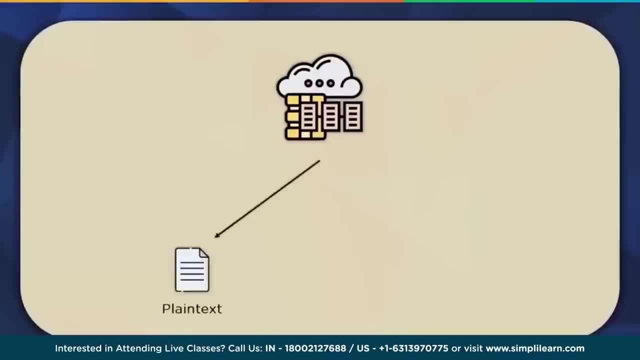 the website owner? how securely are they going to store your password? for website administrators, they have three alternatives. they can either store the passwords in a plain text format, they can encrypt the passwords using an encryption and decryption key, or they can store the passwords in a hash value. let's have a look at each of these. when a password is stored in plain text format, 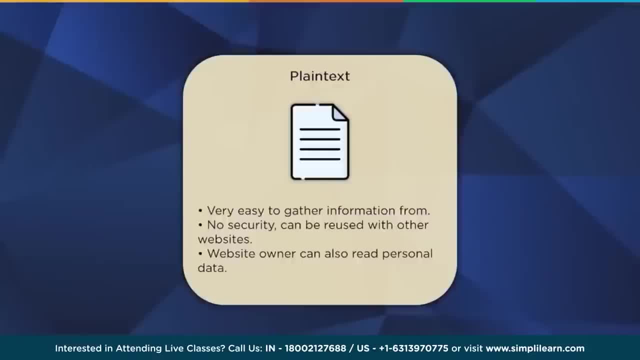 it is considered to be the most unsafe option, since anyone in the company can read your passwords. a single hack and a data server breach will expose all the accounts credentials without needing any extra effort to counter this. owners can encrypt the passwords and keep them in the server, and they can store the passwords in a hash value. let's have a look at each of these. 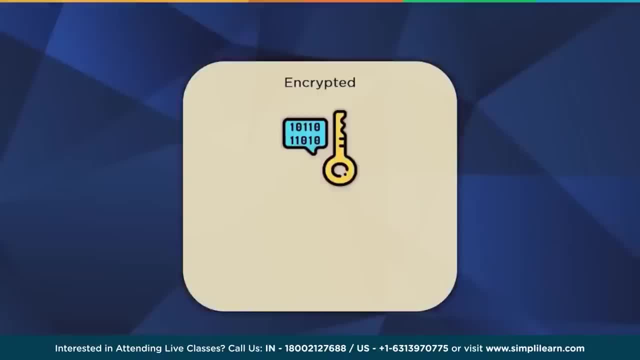 servers as a second alternative, but that would mean they also have to store the decryption key somewhere on their servers. in the event of a data breach or the server hack, both the decryption key and encrypted passwords will be leaked, thus making it a single point of failure. what if there was an? 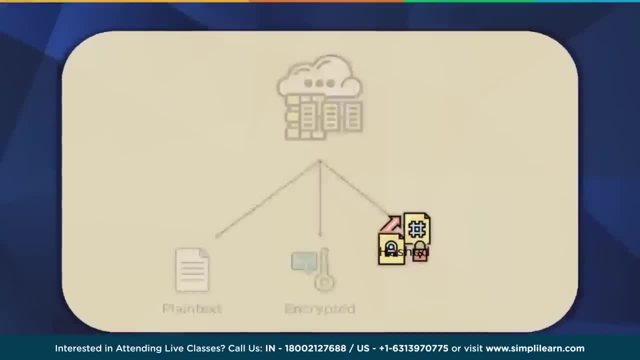 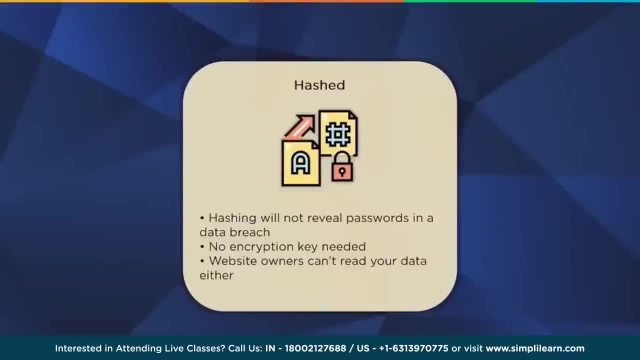 option to store the passwords after scrambling them completely, but with no way to decrypt them. this is where hashing comes to play, since only the hashed values are stored in the server, though encryption is needed, with no plain text passwords to protect. your credentials are saved from the website. 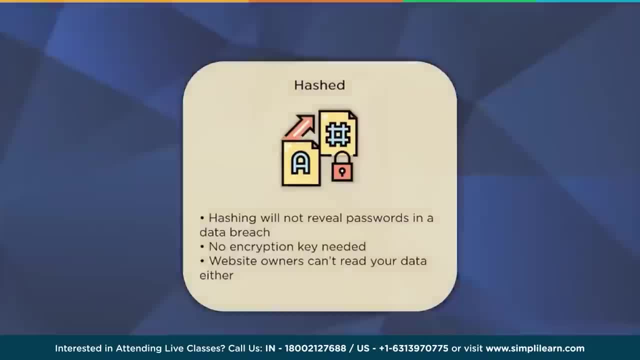 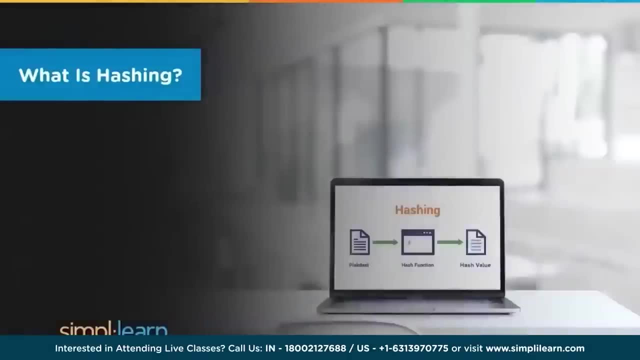 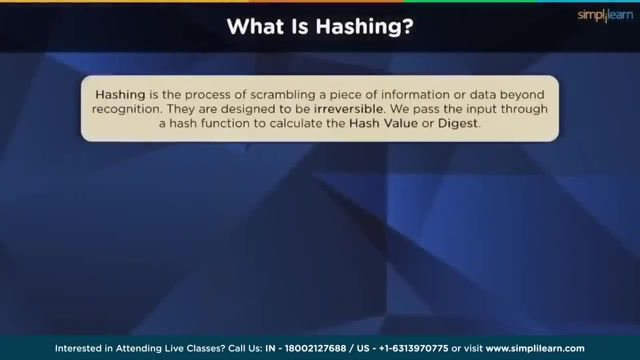 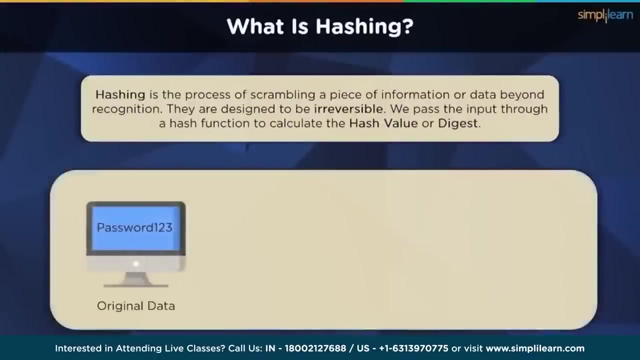 administrators. considering all the pros, hashed passwords are the industry standard when it comes to storing credentials nowadays. before getting too deep into the topic, let's get a brief overview of how hashing works. hashing is the process of scrambling a piece of information or data beyond recognition. we can achieve this by using hash functions, which are essentially 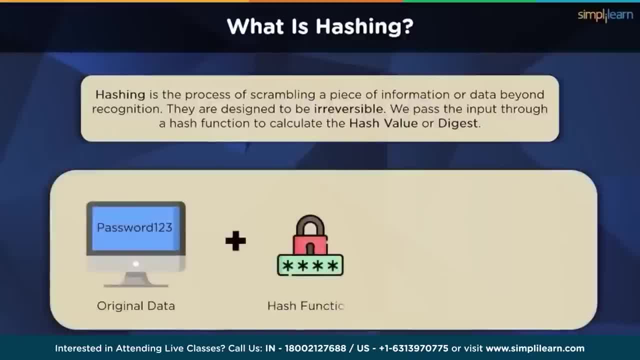 algorithms that perform mathematical operations on the main plain text. the value generated after passing the plain text information through the hash function is called the hash value digest or, in general, just the hash of the original data. while this may sound similar to encryption, the major differences- hashes are made to be irreversible. no decryption key can. 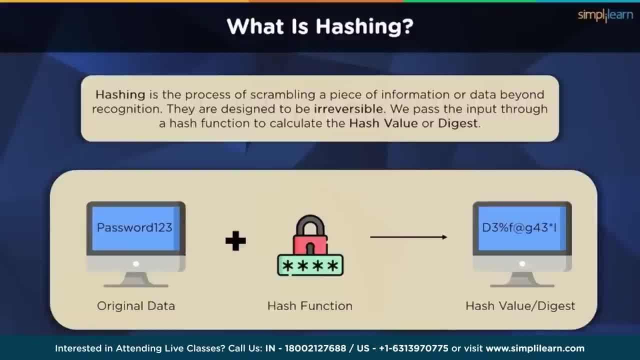 convert or digest back to its original value. however, a few hashing algorithms have been broken due to the increase in computational data, while the hash function is stored within a single hash function- complexity of today's new generation computers and processors. There are new algorithms that stand the test of time and are still in use among multiple. 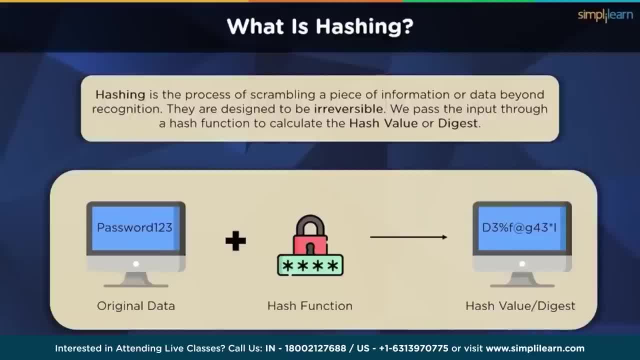 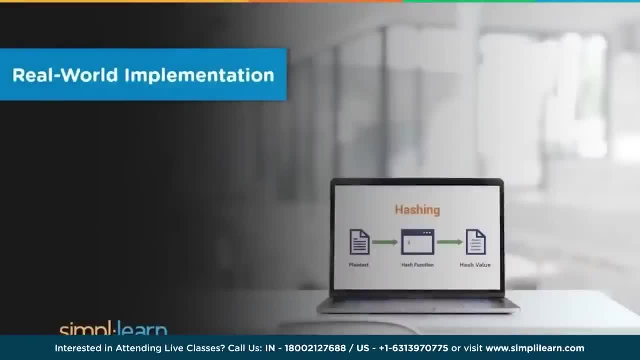 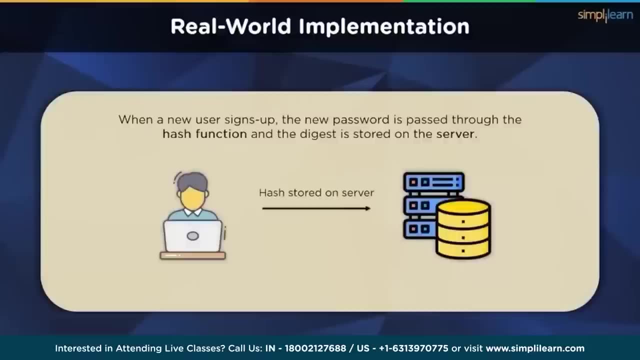 areas for password storage, identity verification, etc. Like we discussed earlier, websites use hashing to store the users passwords. So how do they make use of these hash passwords? When a user signs up to create a new account, the password is then run through the hash function and the 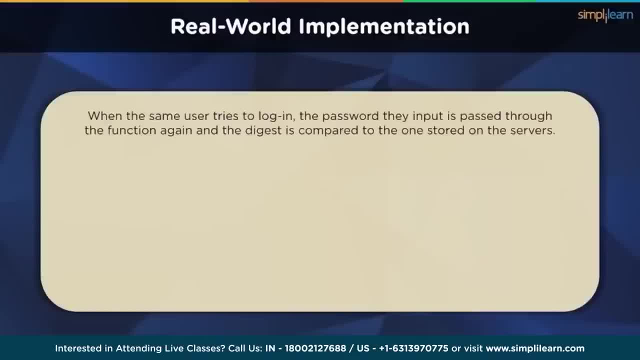 resulting hash value is stored on the servers. So the next time a user comes to log in to the account, the password he enters is passed through the same hash function and compared to the hash stored on the main server. If the newly calculated hash is the same as the one stored on the website server, the 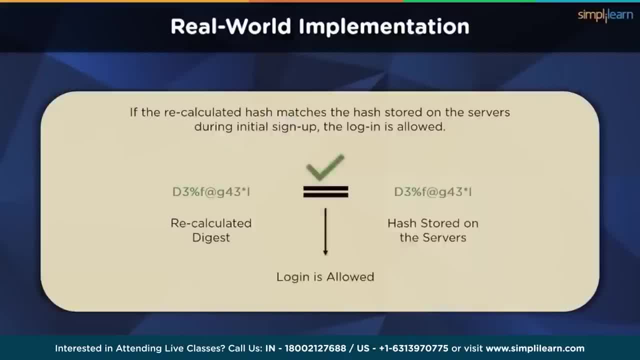 password must have been correct because, according to hash functions terminology, same inputs will always provide the same outputs. If the hashes do not match, then the password entered during login is not the same as the password entered during the signout. Hence the login will be denied This way. 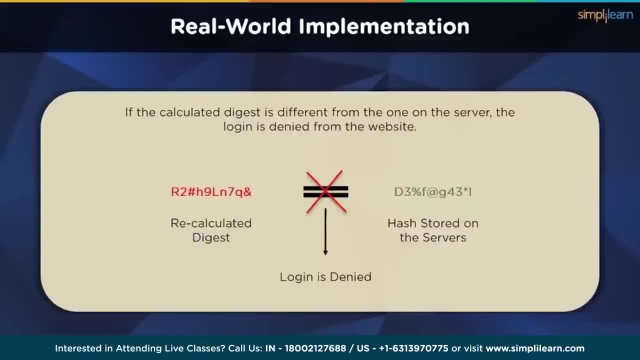 no plain text passwords get stored, preventing both the owner from snooping on user data and protecting users privacy in the unfortunate event of a data breach or a hack. Apart from password storage, hashing can also be used to perform integrity checks. When a file is uploaded on the internet, the file's hash value is generated and it is uploaded along. 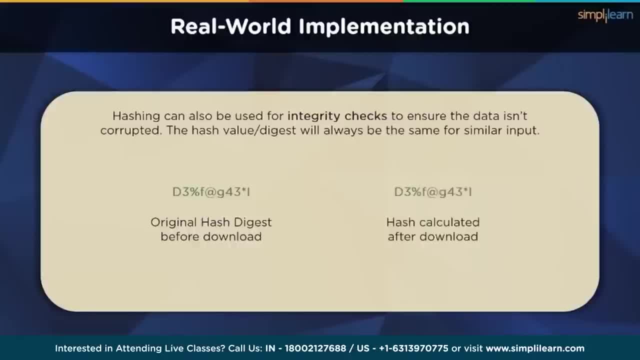 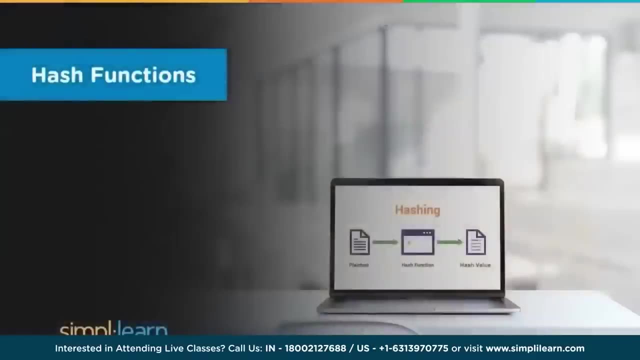 with the original information. When a new user downloads the file, he can calculate the digest of the downloaded file using the same hash function. When the hash values are compared, if they match, then file integrity has been maintained and there has been no data corruption, Since so much important information is being passed onto the hash function. 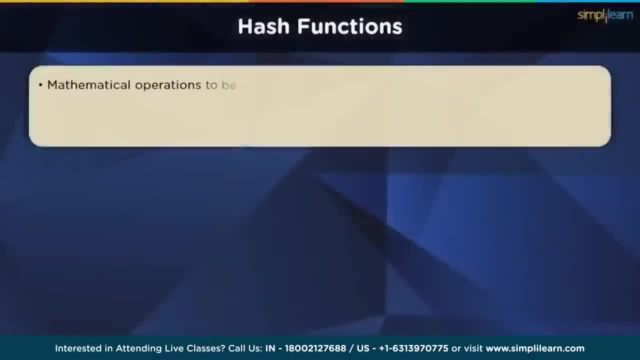 we need to understand how they work. A hash function is a set of mathematical calculations operated on two blocks, blocks of data. The main input is broken down into two blocks of similar size. The block size is dependent on the algorithm that is being used. 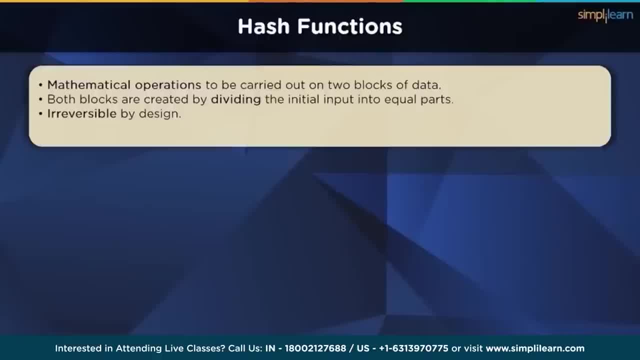 Hash functions are designed to be one way. They shouldn't be reversible, at least by design. Some algorithms, like the previously mentioned MD5, have been compromised, but more secure algorithms are being used today, like the SHA family of algorithms, The digest size. 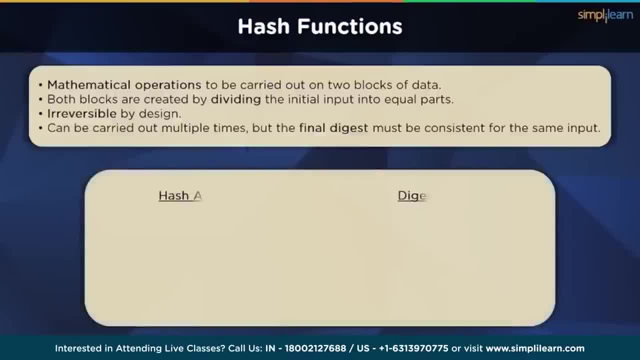 is also dependent on the respective algorithm being used. MD5 has a digest of 128 bits, while SHA-256 has a digest of 256 bits. This digest must always be the same for the same input, irrespective of how many times the calculations are carried out. This is a very 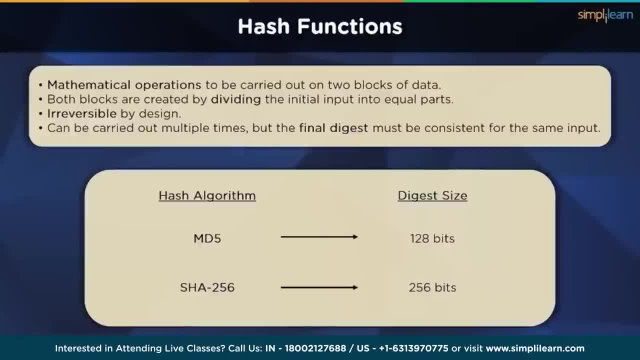 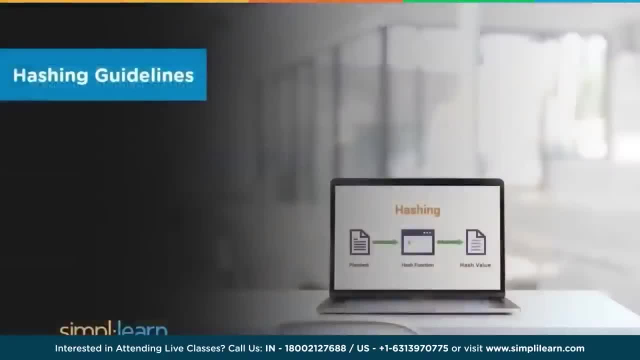 crucial feature, since comparing the hash value is the only way to check if the data is untouched. as the functions are not reversible, There are certain requirements of a hash function. There must be several hash functions that need to be met before they are accepted. While some of them are easy to guess, others are placed in order to preserve security in. 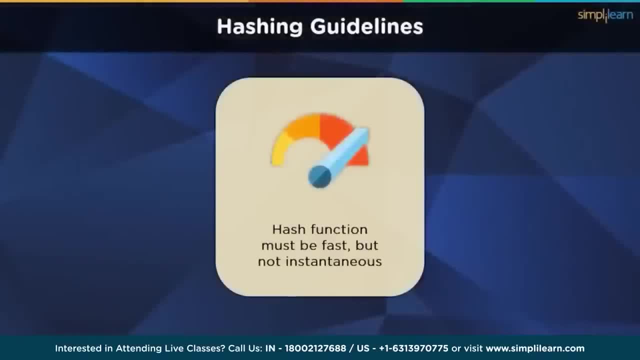 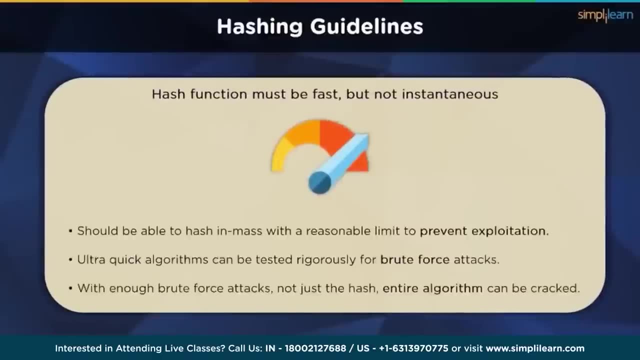 the long run. The hash function must be quick enough to encrypt large amounts of data at a relatively fast pace, but it also shouldn't be very fast. Running the algorithm on all cylinders makes the functions easy to bootforce and a security liability. There must be a balance to allow the hash function to handle large amounts of data and 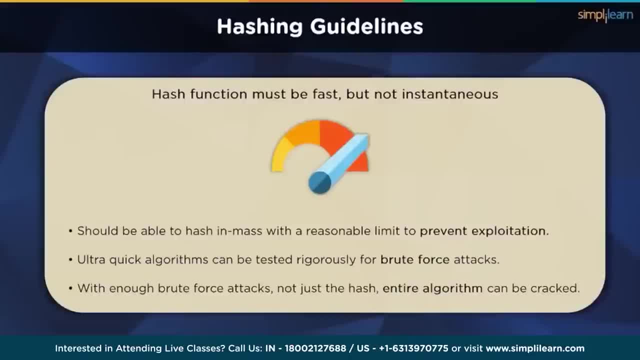 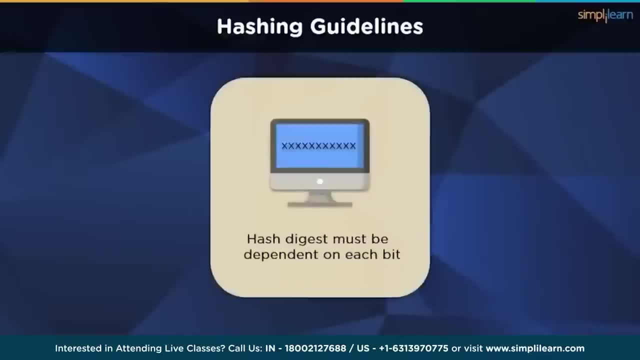 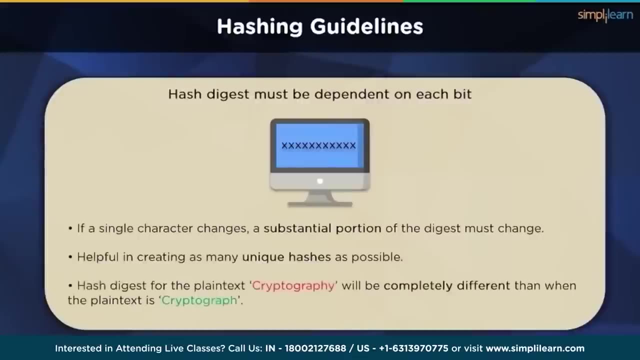 not make it ridiculous, ridiculously easy to brute force by running through all the possible combinations. The hash function must be dependent on each bit of the input. The input can be text, audio video or any other file extension If a single character is being changed. 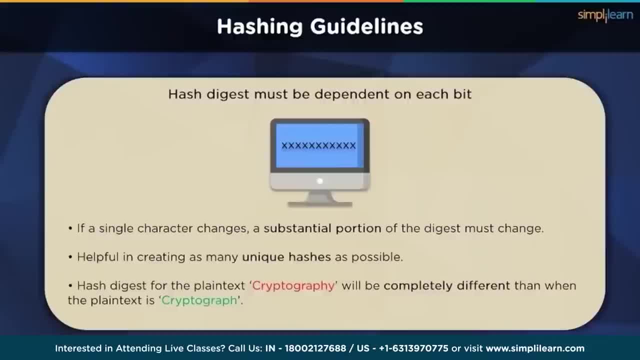 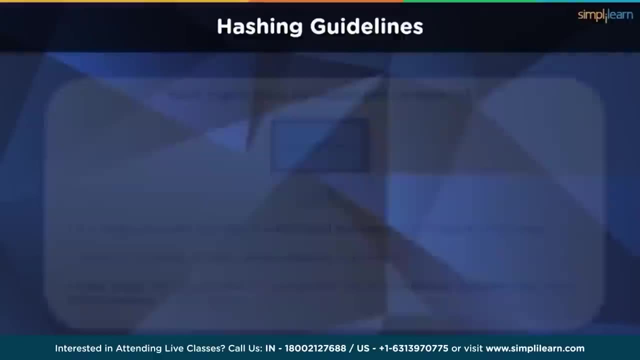 it doesn't matter how small that character may be. the entire digest must have a distinctly different hash value. This is essential to create unique digests for every password that is being stored. But what if two different users are using the same password? Since the hash function is the same for all users, both the digests will be the same. 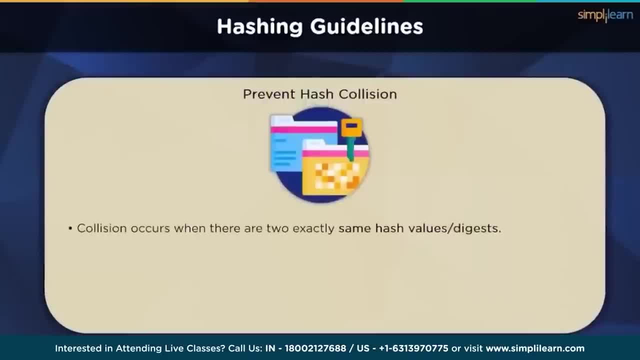 This is called a hash collision. You may think this must be a rare occasion where two users have exactly the same password, but that is not the case. We have techniques like salting that can be used to reduce these hash collisions, as we will discuss later in this video. 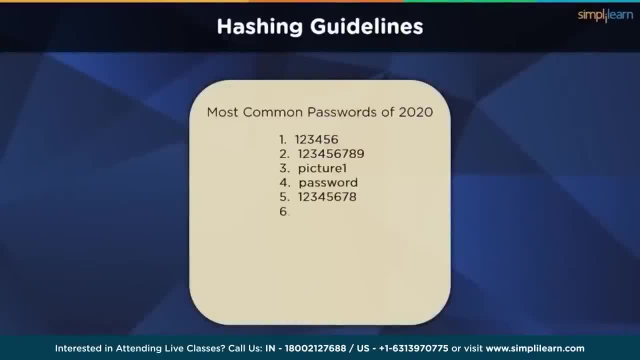 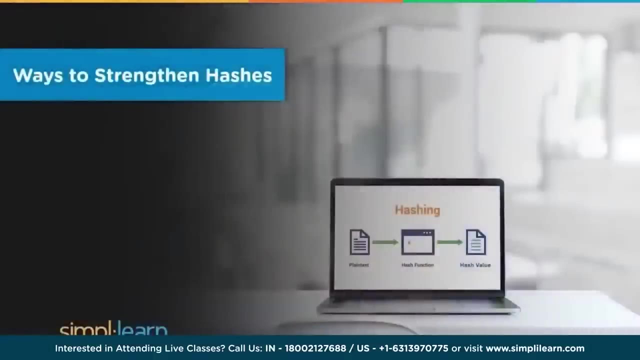 You would be shocked to see the most used passwords of all of these passwords are laughably insecure and since many people use the same passwords repeatedly on different websites, hash collisions are more common than one would expect. Let's say, the hash functions find two users having the same password. 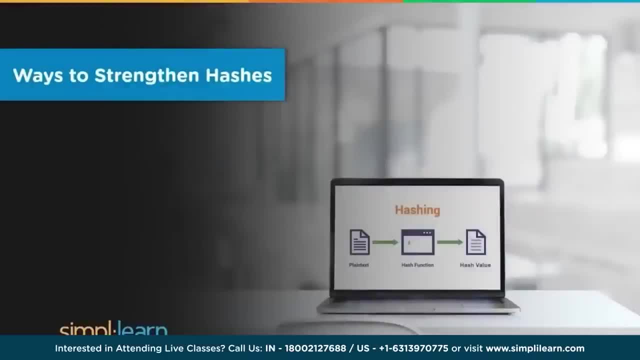 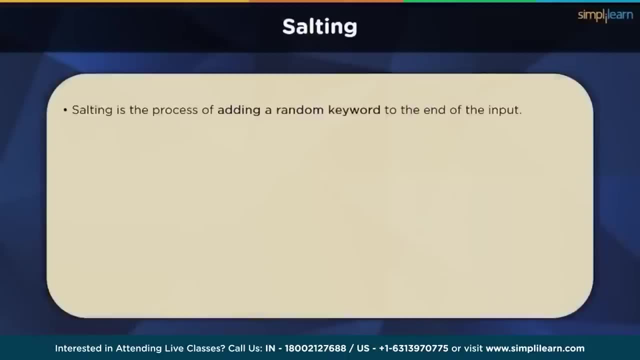 How can they store both the hashes without messing up the original data? This is where salting and peppering come to play. Salting is the process of adding a random keyword to the end of the input before it is passed on to the hash function. 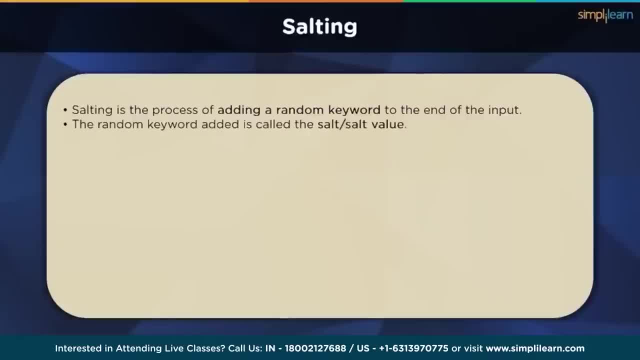 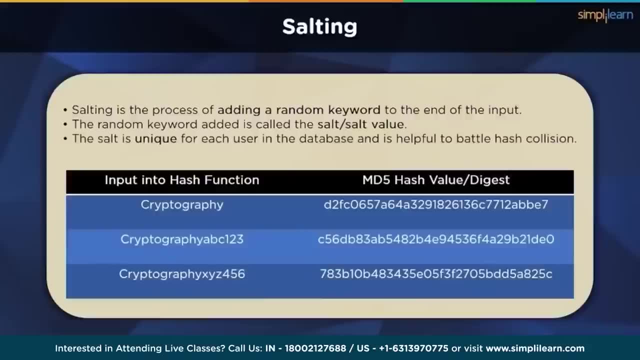 This random keyword is unique for each user on the system, and it is called the salt value or just the salt, So even if two passwords are exactly the same, the salt value will differ, and so will their digest. There is a small problem with this process, though. 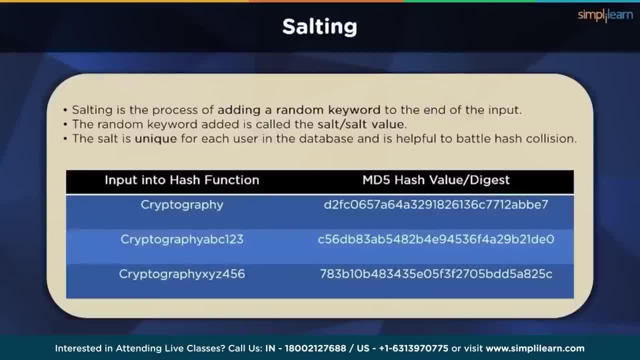 Since the salt is unique for each user, they need to be stored in the database along with the passwords and sometimes even in plain text, to speed up the process of continuous verification. If the server is hacked, then the hashes will need to be be brute-forced, which takes a lot of time. But if they receive the salts as well, the 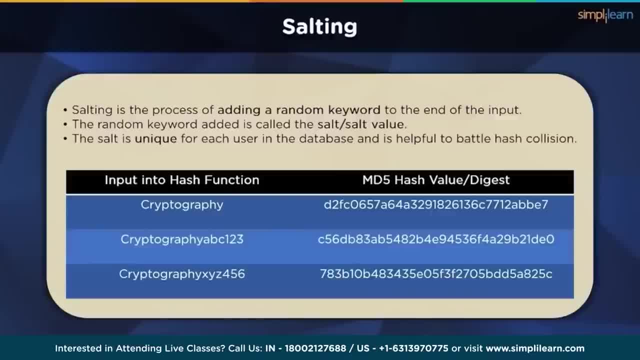 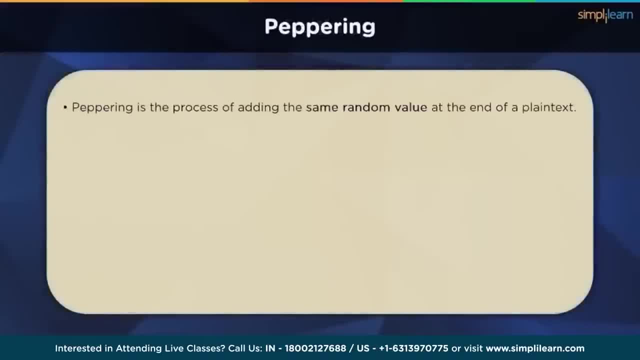 entire process becomes very fast. This is something that peppering aims to solve. Peppering is the process of adding a random string of data to the input before passing them through the hash function, But this time the random string is not unique for each user. 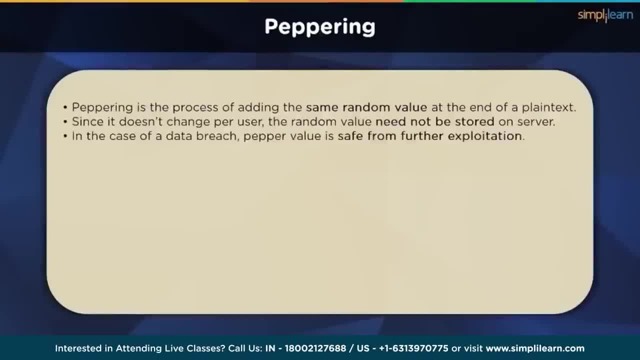 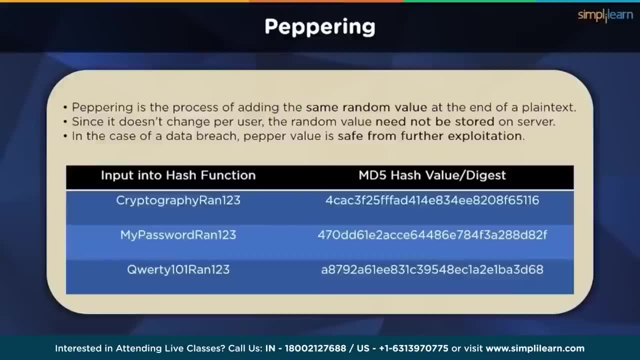 It is supposed to be common for all users in the database and the extra bit added is called the pepper. in this case, The pepper isn't stored on the servers. It is mostly hard-coded onto the website source code. since it's going to be the same for all credentials. 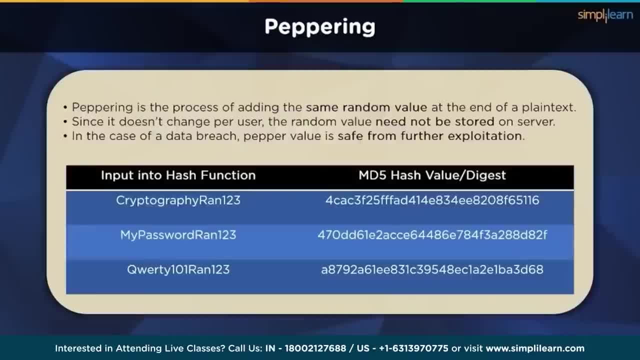 This way, even if the servers get hacked, they will not have the right pepper needed to crack into all the passwords. Many websites use a combination of salting and peppering to solve the problem of hash collision and bolster security. Since brute-force takes such a long time, many hackers avoid taking the effort. The returns of the hash-collision-boolster-security returns are just as fast as the returns of the hash-collision-boolster-security returns. The returns are just as fast as the returns of the hash-collision-boolster-security returns. The returns are just as fast as the returns. 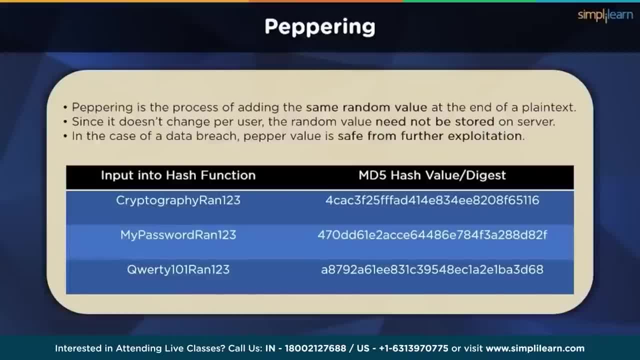 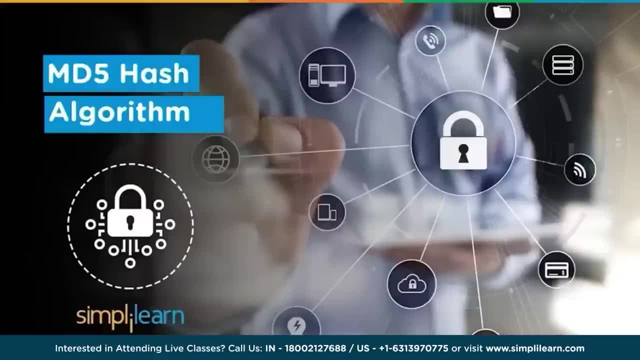 returns are mostly not worth it and the possible combinations of using both salting and peppering is humongous. With the consensus aiming towards an educated public on digital privacy, it's no surprise to see an increasing interest in encryption algorithms. We have already covered the major names like the DES and the AES algorithm. 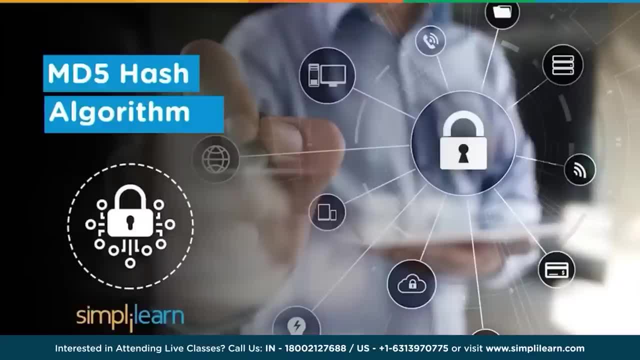 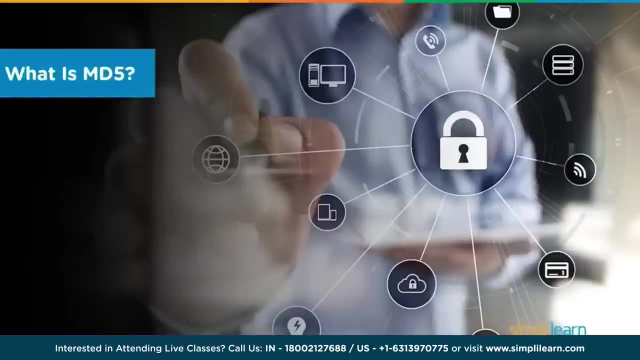 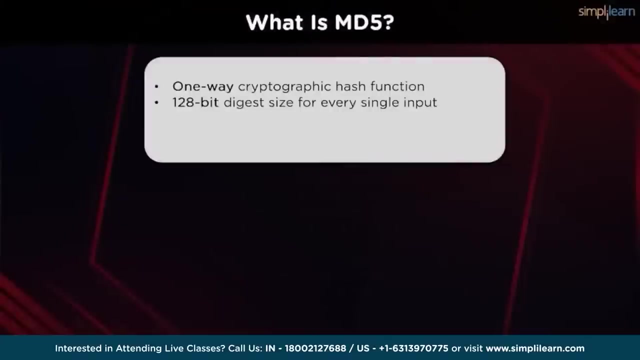 MD5 algorithm was one of the first hashing algorithms to take the global stage as a successor to the MD4.. Despite the security vulnerabilities encountered in the future, MD5 still remains a crucial part of data infrastructure in a multitude of environments. The MD5 hashing algorithm is a one-way cryptographic function that accepts a message of any length. 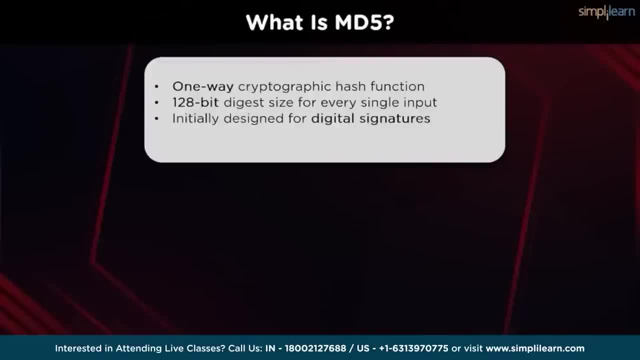 as input and it returns as output a fixed-length digest value to be used for authenticating the original messages. The digest size is always 128 bits. Irrespective of the size of the message, the digest size is always 128 bits. Irrespective of the size of the message, the digest size is always 128 bits. 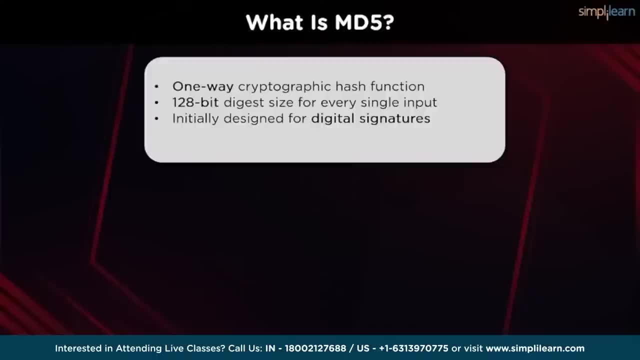 Irrespective of the size of the message, the digest size is always 128 bits. The MD5 hash function was originally designed for use as a secure cryptographic hash algorithm to authenticate digital signatures. MD5 has also been depreciated for uses other than as a non-cryptographic checksum to verify. 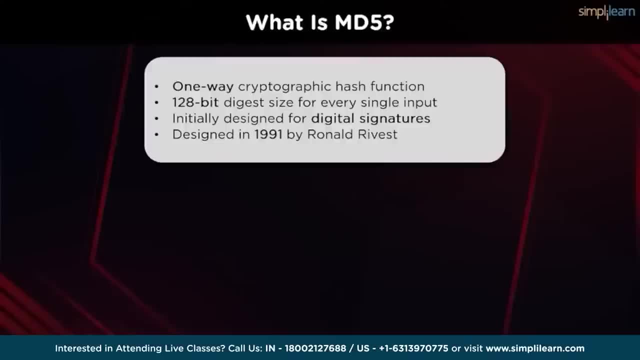 data integrity and detect unintentional data corruption. Ronald Rivest, founder of RSA Data Security Institute, professor at MIT, designed MD5 as an improvement to a prior message digest algorithm which was developed by the RSA for YouTube. He established the product and людисти pi без kiş, branded by Amazon, which was quite 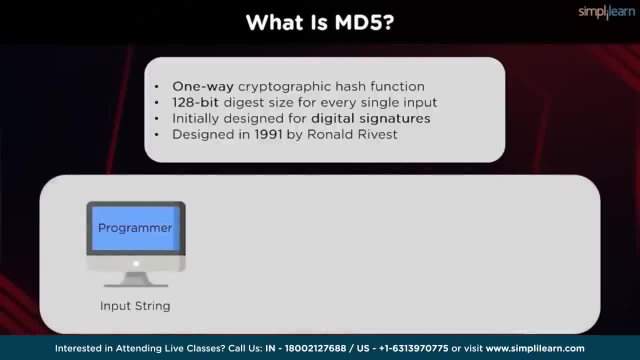 dreadful. As acze'd already iterated before, the process is straightforward. We pass a plaintext message to the MD5 hash function, which in turn performs certain mathematical operations on the cleared text to scramble the data. The 128 bit digest received from this is going to be radically different from the plaintext. 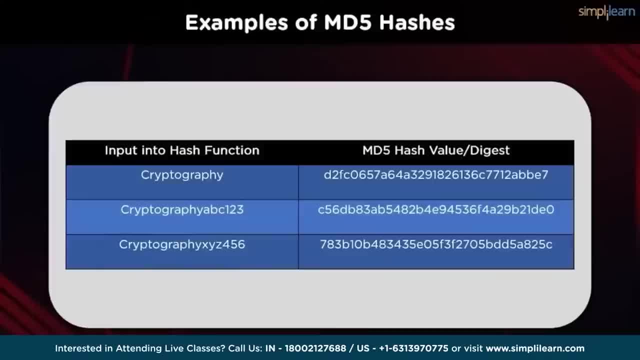 The goal of any message digest function is to produce digest that appear to be random To be considered cryptographically secure. the hash function should be shrimp Simply: I have duplicate, you had無 động, So I can suddenly come back here. and stick should meet two requirements: First, that it is impossible for an attacker to 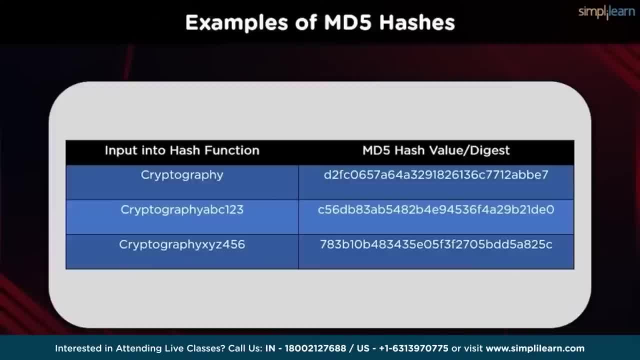 generate a message that matches a specific hash value, and second, that it is impossible for an attacker to create two messages that produce the same hash value. Even a slight change in the plaintext should trigger a drastic difference in the two digests. This goes a long way in preventing hash collisions. 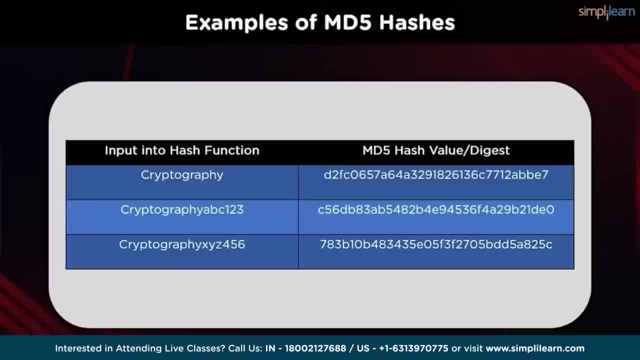 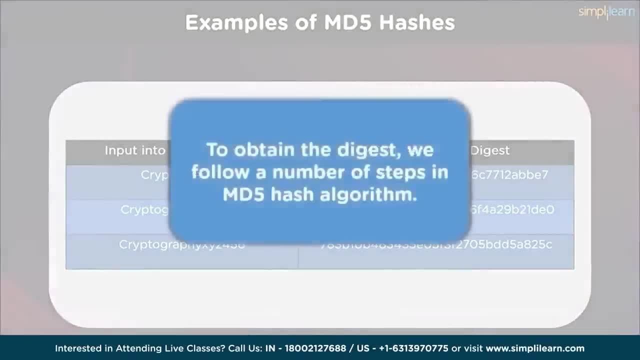 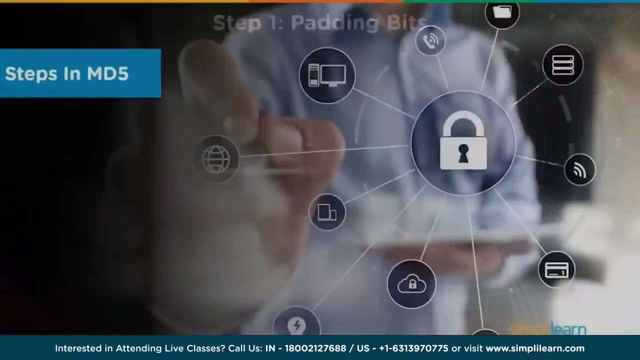 which take place when two different plaintexts have the same digest. To achieve this level of intricacy, there are a number of steps to be followed before we receive the digest. Let us take a look at the detailed procedure as to how the Md5 hash algorithm works. 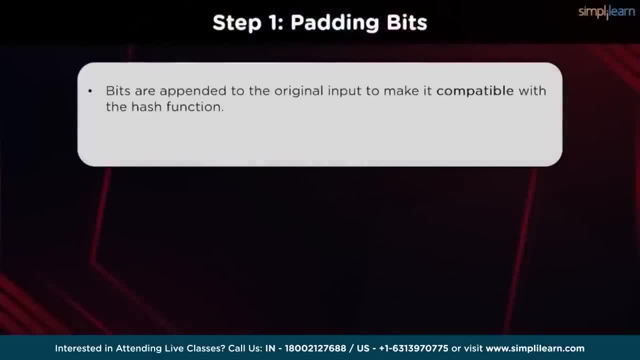 The first step is to make the plaintext compatible with the hash function. To do this, we need to pad the bits in the message. When we receive the input string, we have to make sure the size is 64 bits short of a multiple of 512.. When it 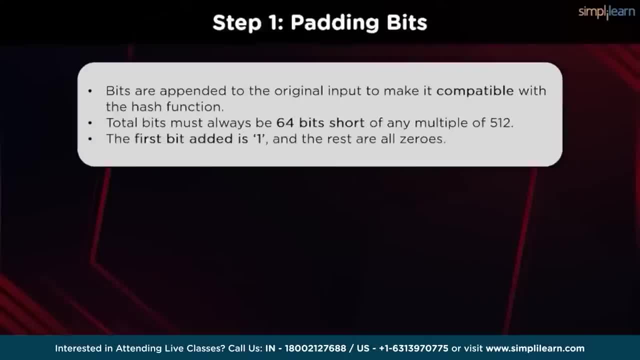 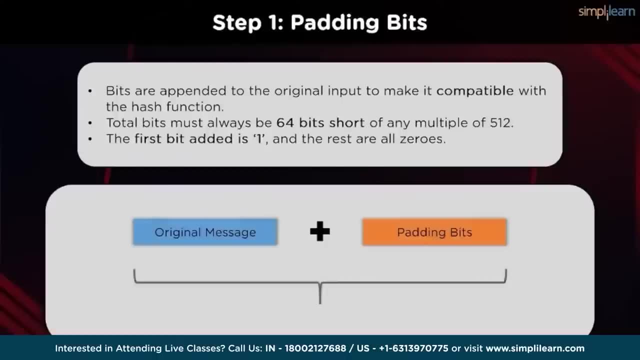 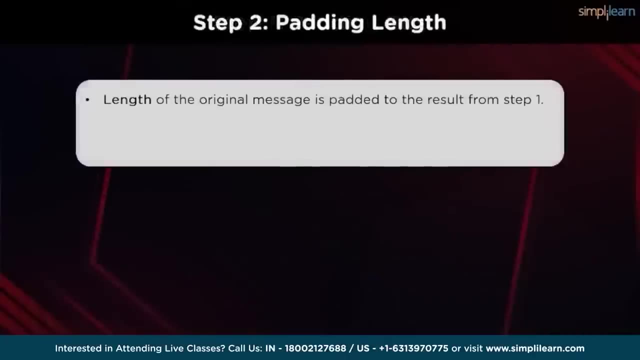 comes to padding the bits, we must add 1 first, followed by zeros to round out the extra characters. This prepares the string to have a length of just 64 bits, less than any multiple of 512.. Here on out, we can proceed on to the next step, where we have to pad the length bits. 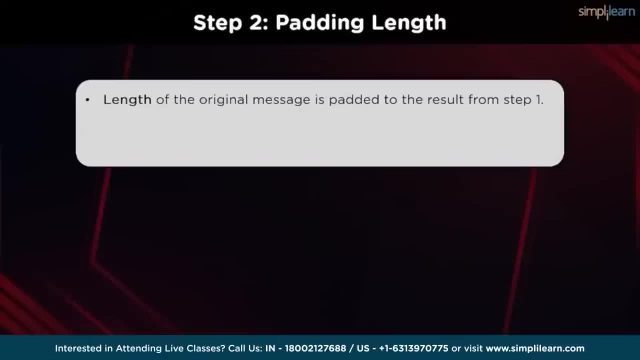 Initially, in the first step we appended the message in such a way that the total length of the bits in the message was 64 bits, short of any multiple of 512.. Now we add the length bits in such a way that the total number of bits in the message is perfectly a multiple. 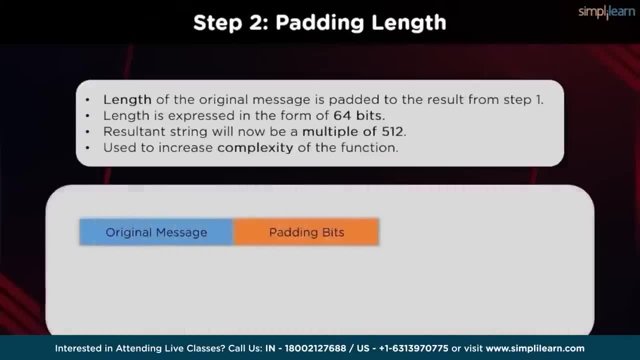 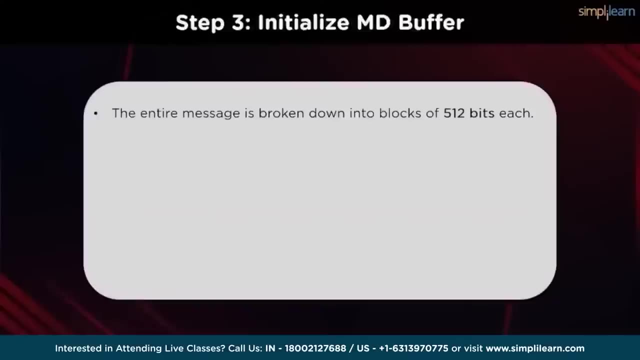 of 512.. That means 64 bits. lengths to be precise- are added to the message. Our final string to be hashed is now a definite multiple of 512.. The next step would be to initialize the message digest buffer. The entire hashing plaintext is now broken down into 512-bit blocks. There are 4 buffers. 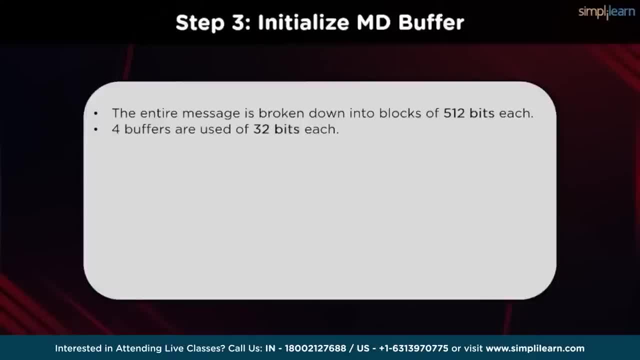 or registers that are of 32 bits each, named A, B, C and D. These are the 4 words that are going to store the values of each of these sub-blocks. The first iteration to follow these registers will have fixed hexadecimal values, as shown on the screen below. 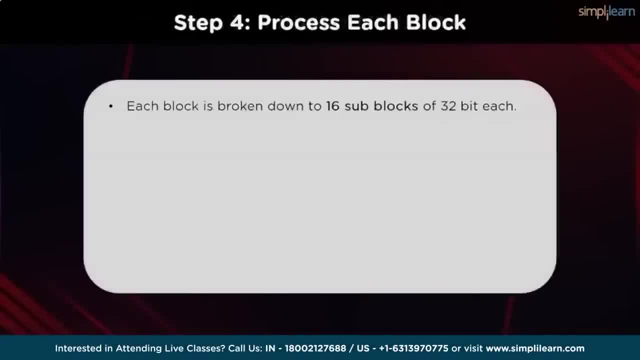 Once these values are initialized, we can start the initialization process Of these 512 blocks. we can divide each of them into 16 further sub-blocks of 32 bits each. For each of these sub-blocks, we run 4 rounds of operations having the 4 buffer. 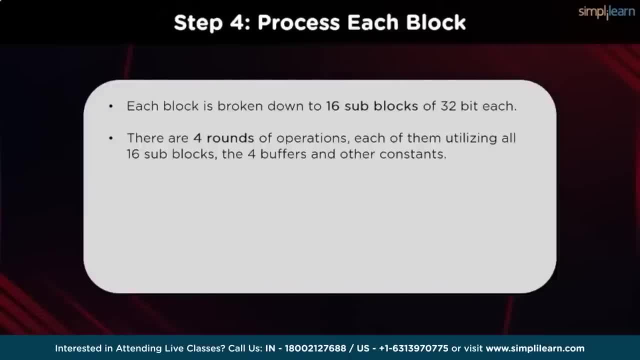 variables A, B, C and D. These rounds require the other constant variables as well, which differ with each round of operation. The constant values are stored in a random array of 64 elements, Since each 32-bit sub-block is run 4 times 16 such sub-blocks equal the total. 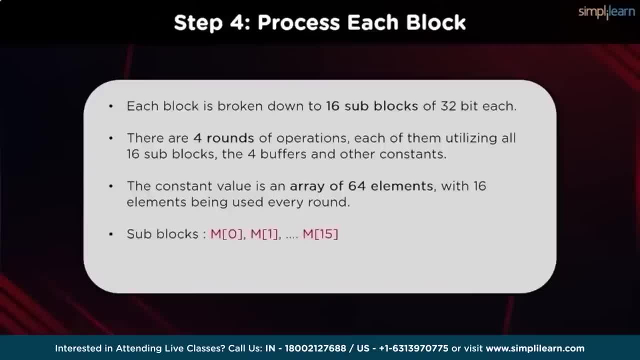 64 constant values needed for a single block iteration. The sub-blocks can be denoted by the alphabet M and the constant values are denoted by the alphabet T. Coming to the actual round of operation, we see our 4 buffers which already have pre-initialized. 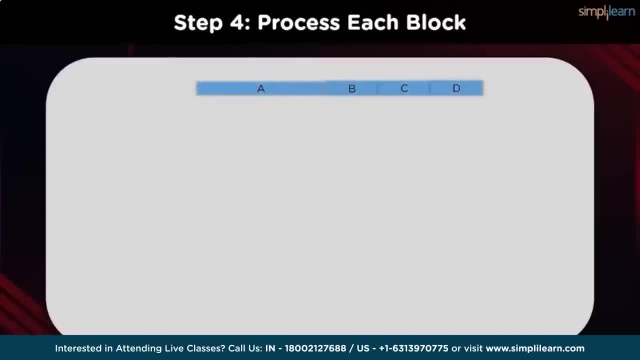 values for the first iteration. At the very beginning, the values of buffers B, C and D are passed on to a non-linear logarithmic function. The formula behind this function changes by the particular round being 1,, 2,, 3,, 4,, 5,, 6,, 7,, 8,, 9,, 10,, 11,, 12,, 12,, 13,, 13,, 13,. 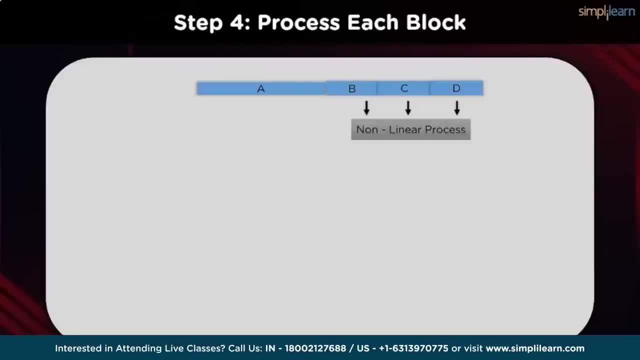 14,, 14,, 14,, 15,, 16,, 17,, 18,, 19,, 20 and 20.. The output of this function is calculated and it is added to the raw value stored in buffer A. The output of this addition is added. 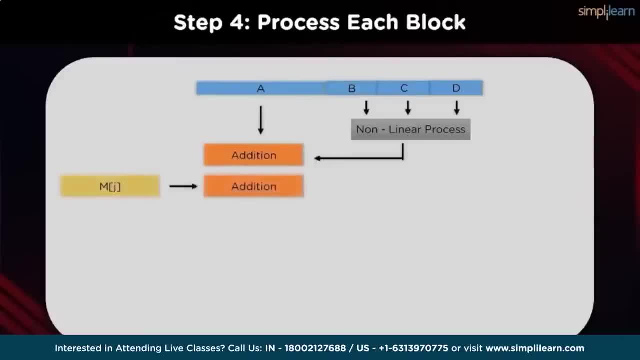 to the particular 32-bit sub-block using which we are running the 4 operations. The output of this requisite function then needs to be added to a constant value derived from the constant array K, Since we have 64 different elements in the array. since we 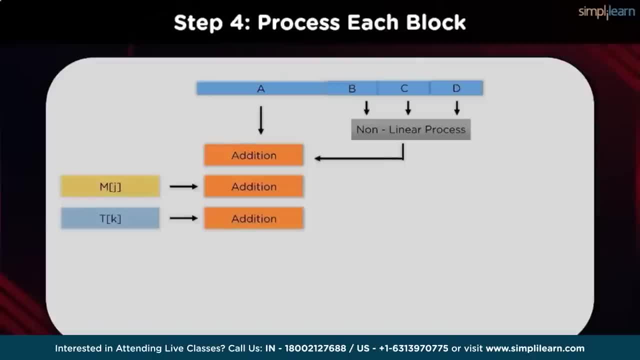 have 64 different elements in the array, we can use a distinct element for each iteration of a particular block. The next step involves a circular shift that increases the complexity of the hash algorithm and is necessary to create a unique digest for each individual input. The output generated is later added to the value stored in the buffer B, The final. 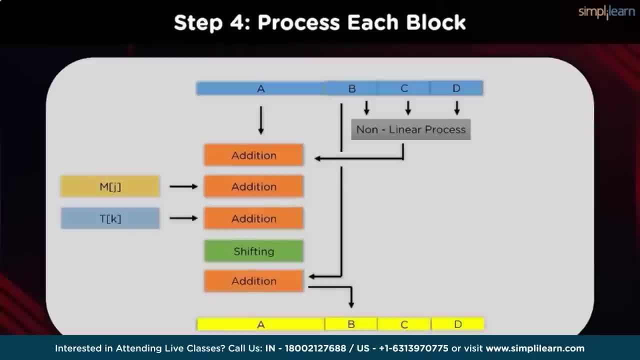 output is now stored in the second buffer of B of the output register. Individual values of C, D and A are derived from the preceding element before the iteration started, meaning the value of B gets stored in C, value of C gets stored in D and the value of D in A. 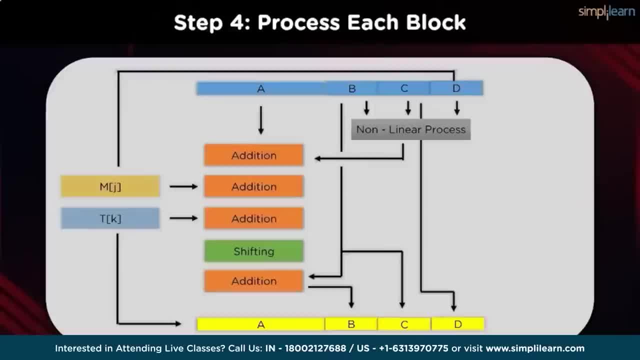 Now that we have a full register ready for this sub-block, the values of A, B, C, D are moved on as input to the next sub-block. Once all sixteen sub-blocks are completed, the final register value is saved and the next 512-bit block begins. At the end of all the 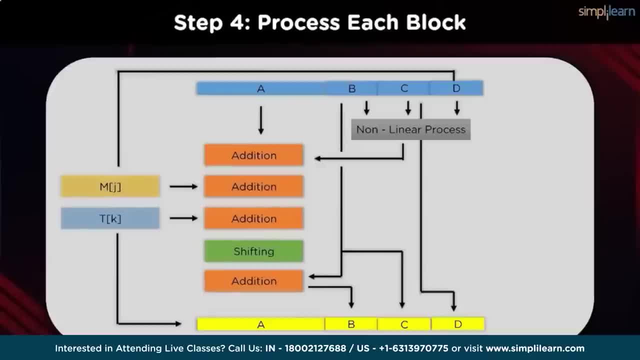 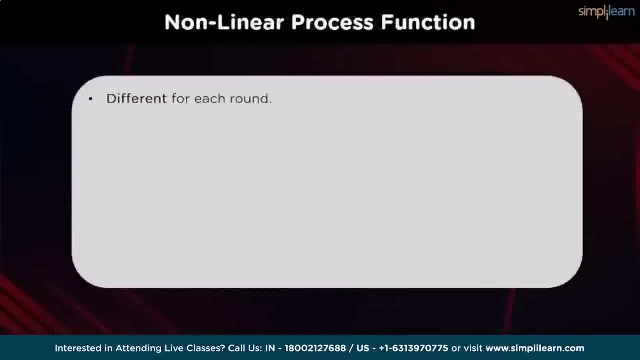 these blocks, we get a final digest of the MD5 algorithm. Regarding the nonlinear process mentioned in the first step, the formula changes for each round it's being run on. This is done to maintain the computational complexity of the algorithm and to increase randomness of the procedure. The formula for each of the four rounds uses the same parameters that. 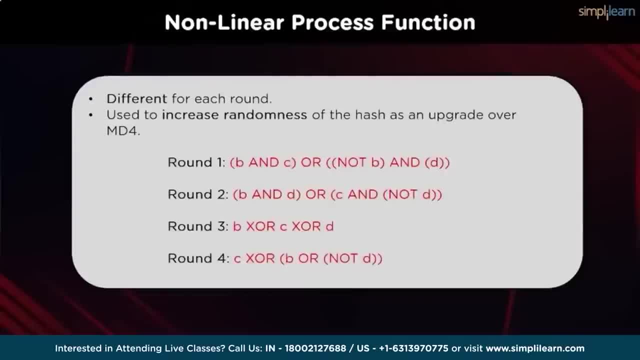 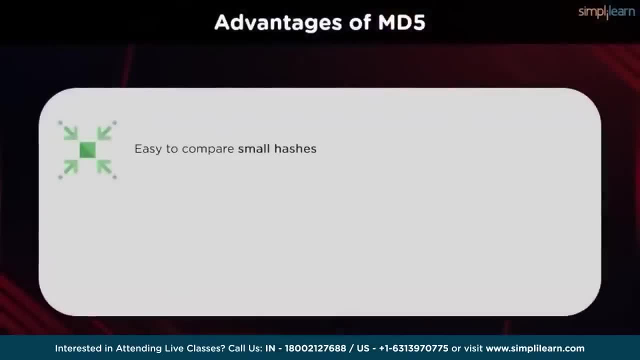 is B, C and D to generate a single output. The formulas being used are shown on the screen right now. Unlike the latest hash algorithm families, a 32-bit digest is relatively easier to compare when verifying the digests. They don't consume a noticeable amount of disk storage and are 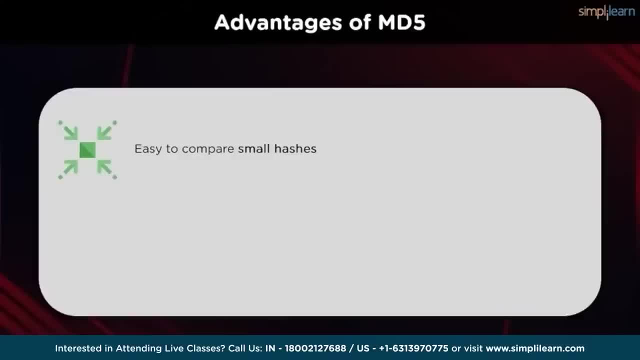 comparatively easier to remember and reiterate. Passwords need not be stored in plain text format, making them accessible for hackers and malicious actors. When using digests, the database security also gets a boost, since the sizes of all the hashed values will be the same In the event of a hack or a breach. 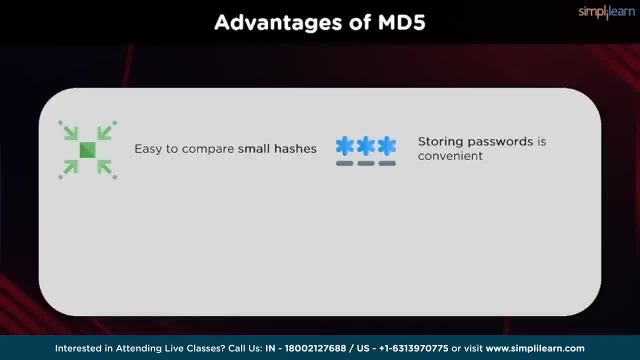 the malicious actor will only receive the hashed values, so there is no way to regenerate the plain text, which would be the user passwords in this case. Since the functions are irreversible by design, hashing has become a compulsion when storing user credentials on the server. 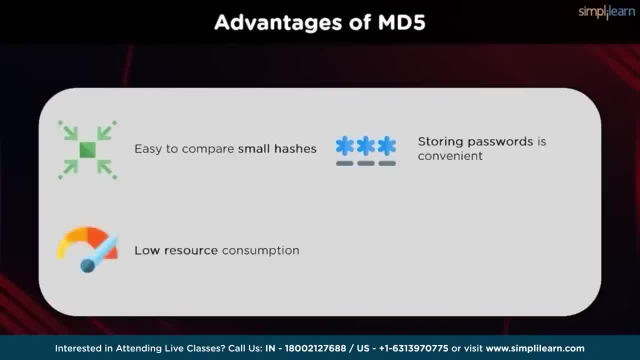 nowadays, A relatively low memory footprint is necessary when it comes to integrating multiple services in a single hash. A relatively low memory footprint is necessary when it comes to integrating multiple services in a single hash. When it comes to integrating multiple services in a single hash. 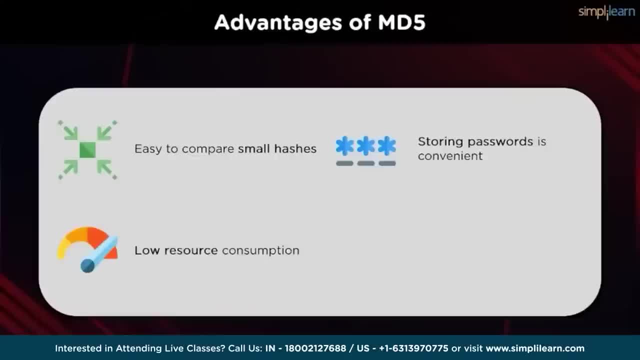 everything belongs to one hash. The address academic is easy for Git to import. I'll explain more how. but you haveroz address icon isn't a good option. You can also from the網 to others. if It doesn't show, the system portholes. 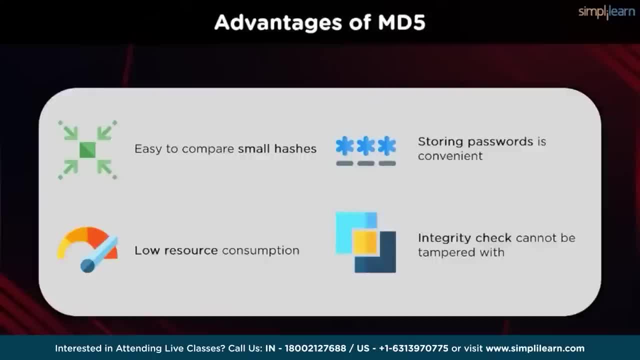 You can monitor file corruption by comparing hash values before and after. transit is match. file integrity checks are valid and we can avoid data corruption. hash functions will always give the same output for the similar input, irrespective of the iteration parameters. it also helps in ensuring that the data hasn't been tampered with on route to the receiver of. 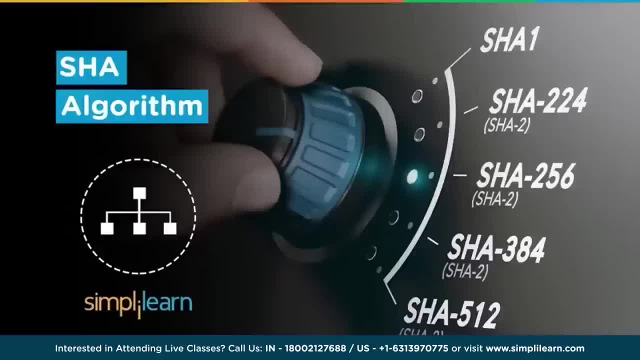 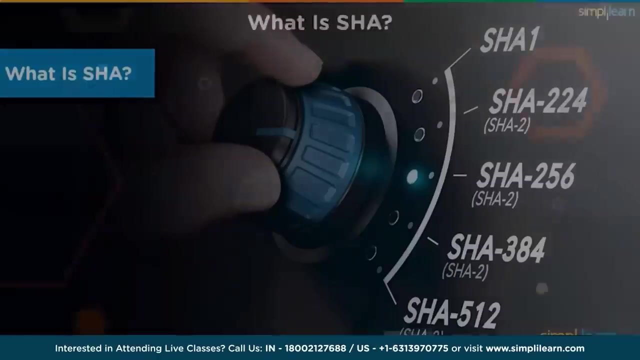 the message. we use our Wi-Fi every day for work and we use the internet for entertainment and communication. the dependency on technology is at an all-time high, thanks to the radical developments and innovation in these last two decades. a big portion of this belongs to ensuring secure channels of communication and data transmission: the secure hash algorithm. 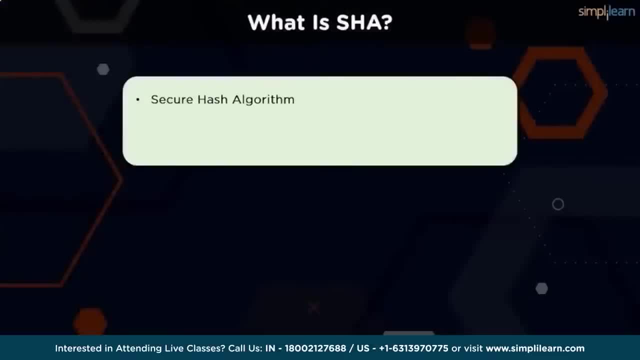 our family of cryptographic hash functions that are published by the National Institute of Standards and Technology. along with the NSA, it was passed as a federal instrument information processing standard, also known as a five PS. it has four different families of hash functions. SSJ 0 is a 160-bit hash function published in 1993 and it was closed down later. 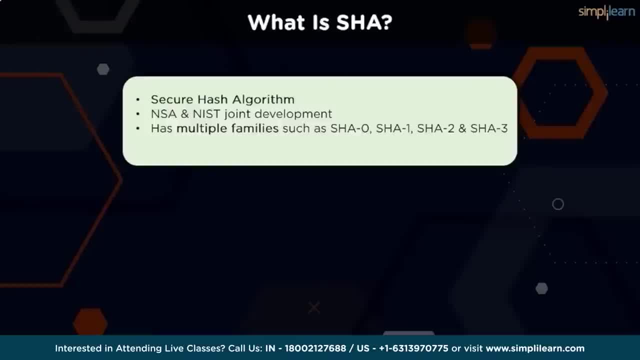 after an undisclosed significant flaw. SHC one is also a 160-bit hash function which resembles the earlier MD 5 algorithm. this was designed by the NSA to be a part of the digital signature algorithm. SHC 2 is a family of two similar hash functions which is used to control the data transfer. 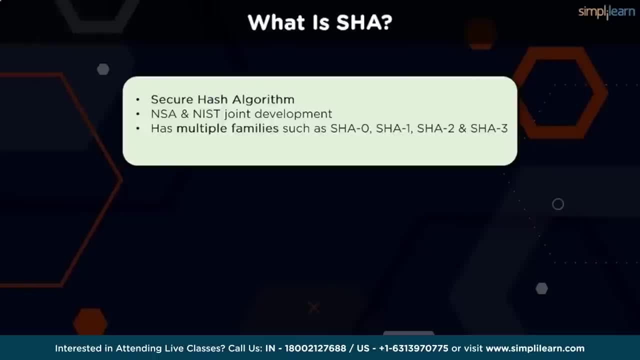 hash functions with different block sizes, known as the SHI 256 and the SHI 512. they differ in the word size: SHI 256 uses 32-bit words by SHI 512 uses 64-bit words. SHI 3 is a hash function. 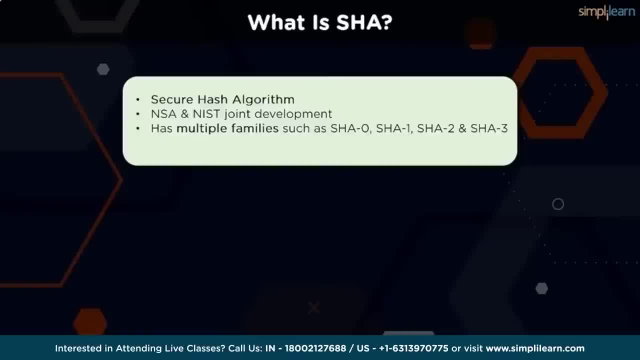 properly known as KK. it was chosen in 2012 after a public competition among non NSA desires. it supports the same hash lens as HH II and its internal structure differs significantly from the hash length of the hash function and its internal structure differs significantly from the hash length of the hash function and its internal structure differs significantly from. 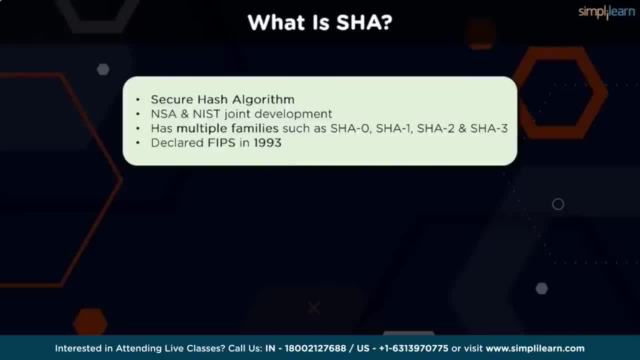 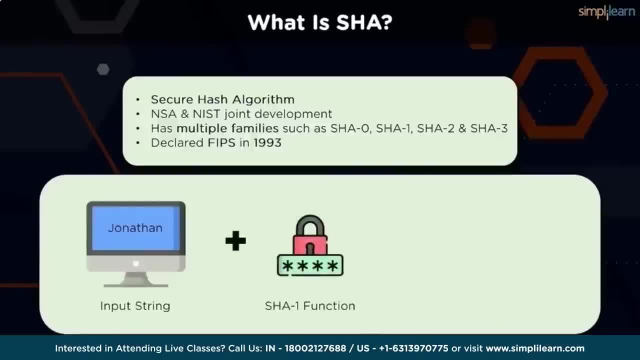 from the rest of the SHA family. As we have already iterated, the process is straightforward. We pass a plain text message to the SHA hash function, which in turn performs certain mathematical operations on the clear text to scramble the data The 160-bit digest received from this. 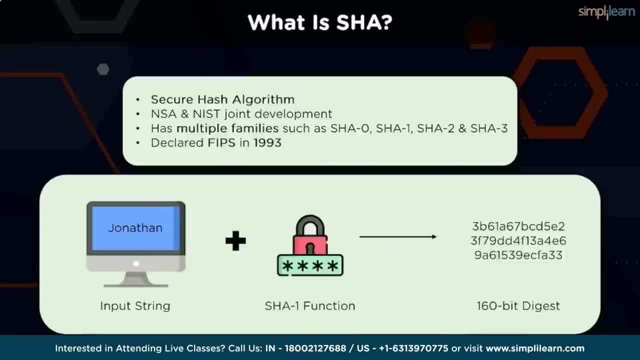 is going to be radically different from the plain text. The goal of any hash function is to produce digests that appear to be random To be considered cryptographically secure. the hash function should meet two requirements. First, that it is impossible for an attacker 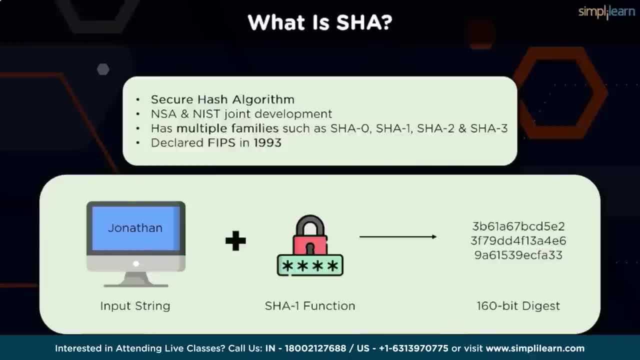 to generate a message that matches a specific hash value. And second, it should be impossible for an attacker to create two messages producing the exactly same hash value. Even a slight change in the plain text should trigger a drastic difference in the true digest. This goes a long way in preventing hash collisions. 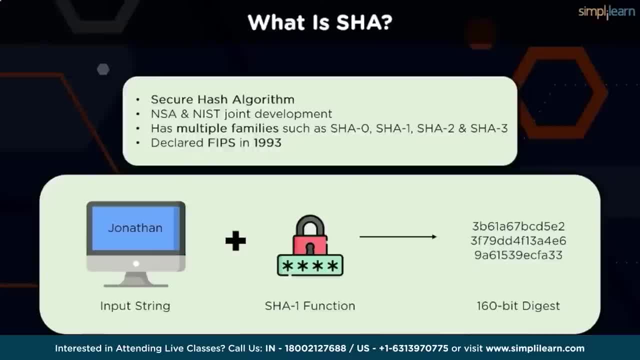 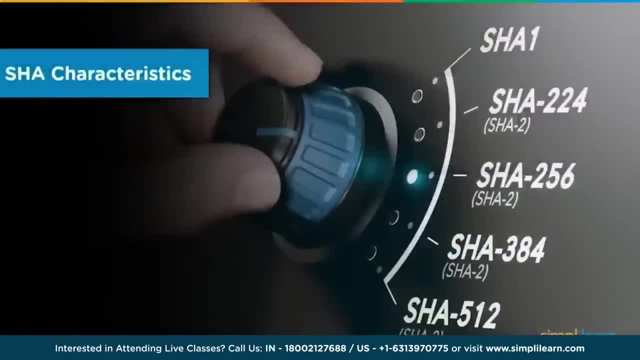 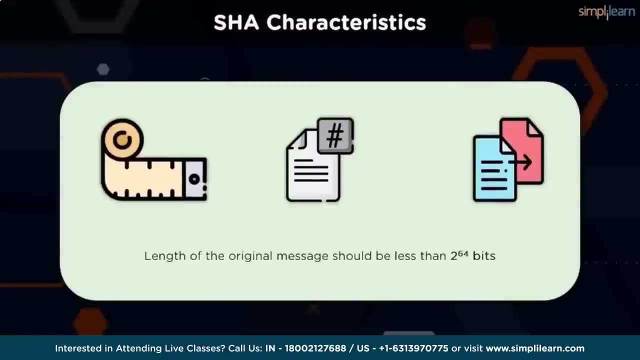 which takes place when two different plain texts have the same digest. The SHA family functions have some characteristics that they need to follow while generating the digest. Let's go through a few of them. The length of the clear text should be less than 2. 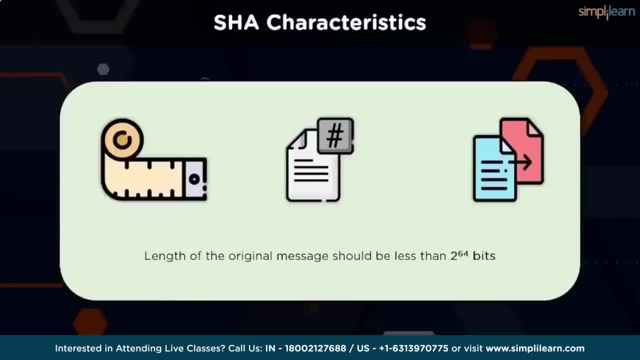 to the power, 64 bits in the case of SHA-1 and SHA-256.. This is essential to keep the plain text compatible with the hash function and the size needs to be in comparison area. to keep the digest as random as possible, The length of the hash digest should be 256 bits in the SHA-256. 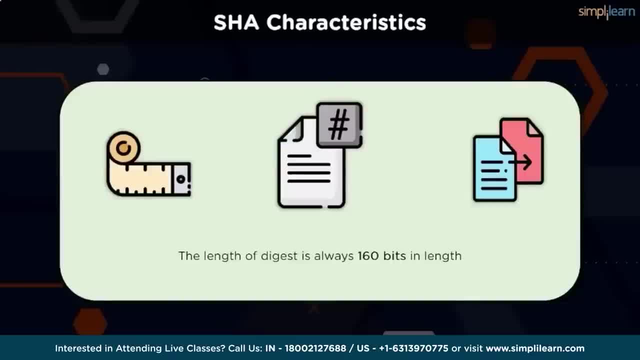 algorithm, 512 bits in the SHA-512 algorithm and so on. Bigger digest usually suggests significantly more calculations at the cost of speed and space. We typically go for the longest digest to bolster security, but there must be a definite balance between the speed. 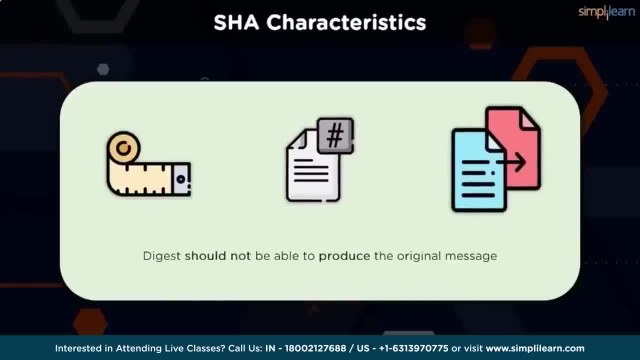 and security of a hash function. hash function of the SHA-512, SHA-256 are irreversible. You should neither get a plain text when you have the digest beforehand, nor should the digest provide the original value when you pass it through the same hash function again. Another case of protection is that 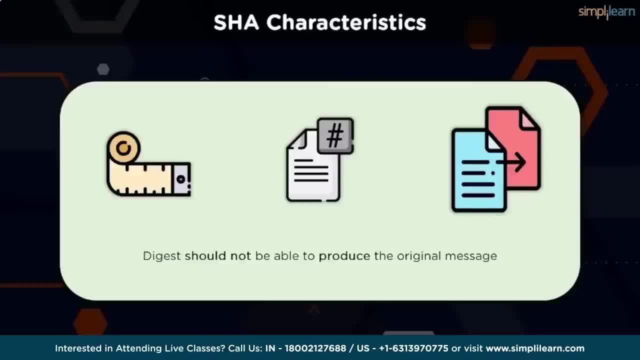 when the hash digest is passed into the SHA function for a second time, we should get a completely different digest from the first instance. This is done to reduce the chance of brute force attacks. To achieve this level of intricacy, there are a number of steps. 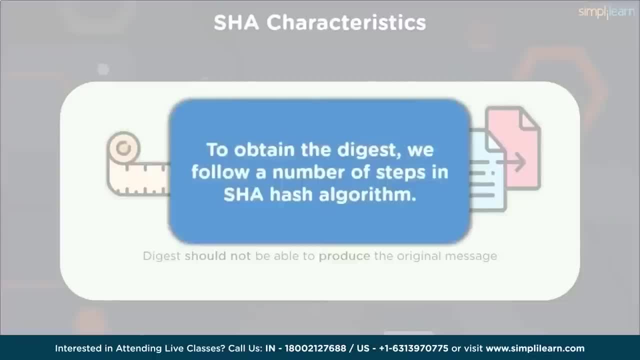 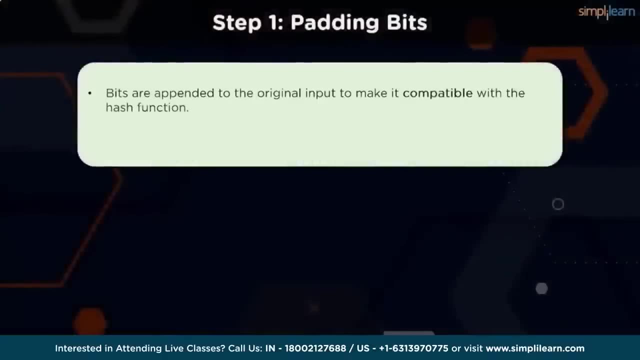 to be followed before we receive the digest. Let us take a look at the detailed procedure as to how the SHA algorithm works. The first step is to make the plain text compatible with the hash function. To do this, we need to pad the bits in the message When you receive. 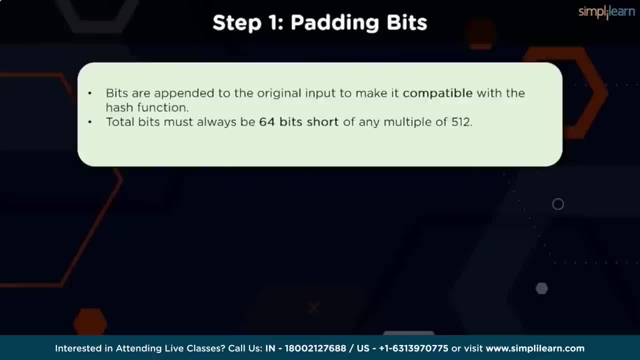 the input string, you have to make sure the size is 64-bit short of a multiple of 512.. When it comes to the input string, you have to make sure the size is 64-bit short of a multiple of 512.. When it comes to padding the bits, you must add one first followed. 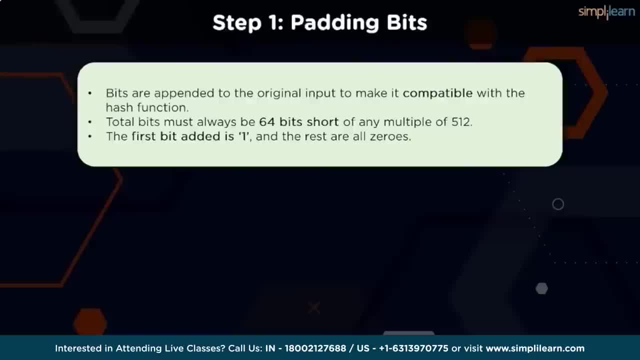 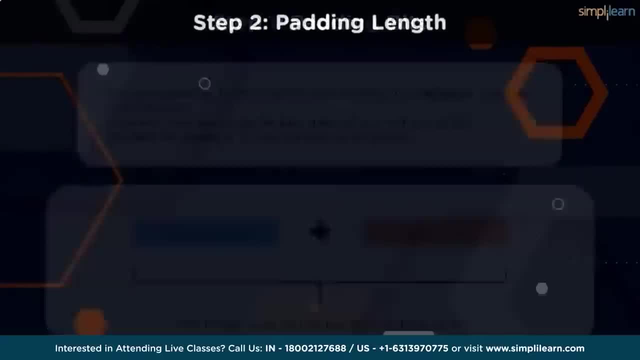 by the remaining zeros to round out the extra characters. This prepares our string to have a length just 64-bits, less than any multiple of 512.. Here on out we can proceed to the next step, where we have to pad the length bits Initially. 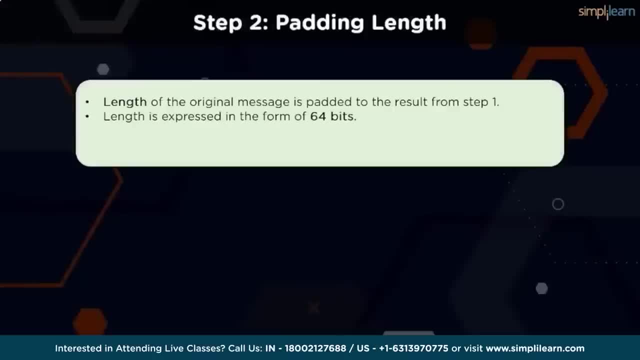 in the first step we appended the message in such a way that the total number of bits in the message was 64-bit short from becoming a multiple of 512.. Now we add the length of bits in such a way that the total number of bits in the message is a perfect multiple. 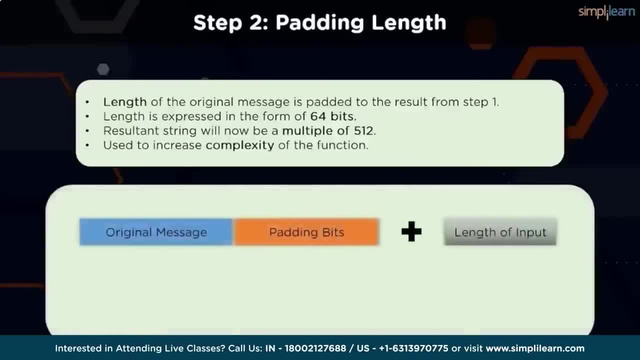 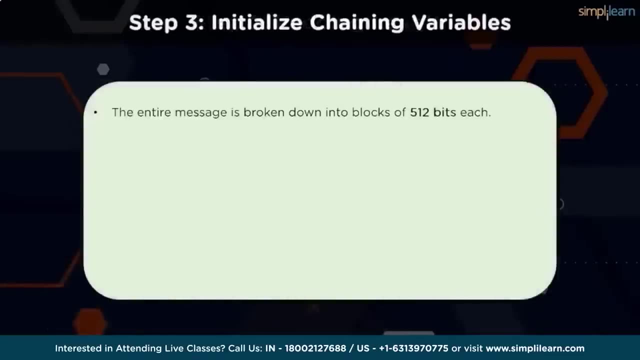 of 512.. That means 64-bits plus the length of the original message becomes a multiple of 512.. This becomes a final string that needs to be hashed. In the next step we have to initialize these chaining variables, The entire plain text. 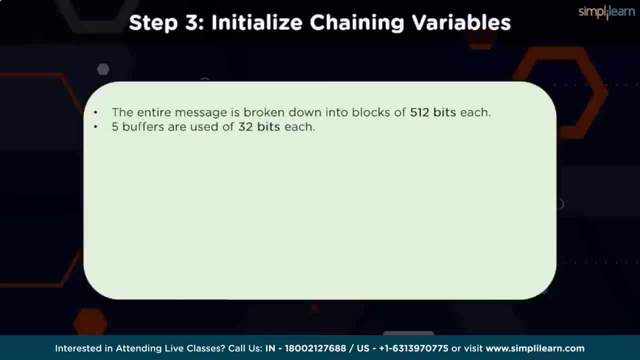 message can now be broken down into blocks of 512 bits each. Unlike other hash functions, other hash algorithms like MD5, which use 4 registers or buffers, SHA family use 5 buffers of 32 bits each. They are named A, B, C, D and E. These registers go through multiple 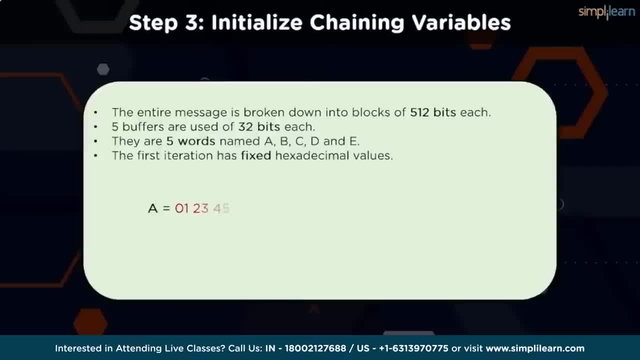 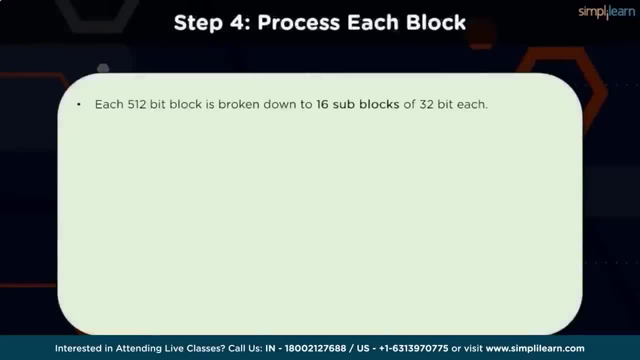 rounds of operation where the first iteration has fixed hexadecimal values, as can be seen in the screen. Moving on, we have to process each of the 512-bit blocks by breaking each of them into 16 sub-blocks of 32 bits each. This goes through 4 rounds of operation that use the entire register and have the 512-bit. 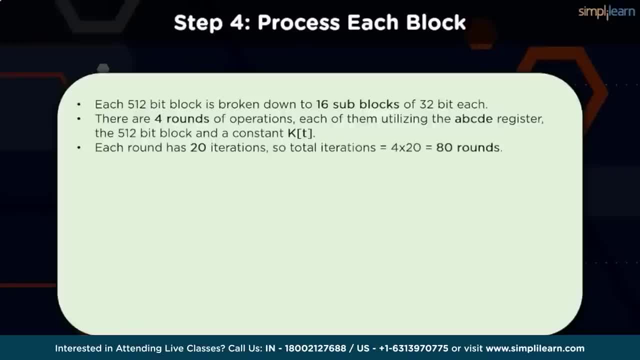 block, along with the constant array Out of those 4 rounds. each round has 20 iterations, So in general we have 80 rounds. sum total, The constant value of k is an array of 80 elements. Of those 80, 16 elements are being. 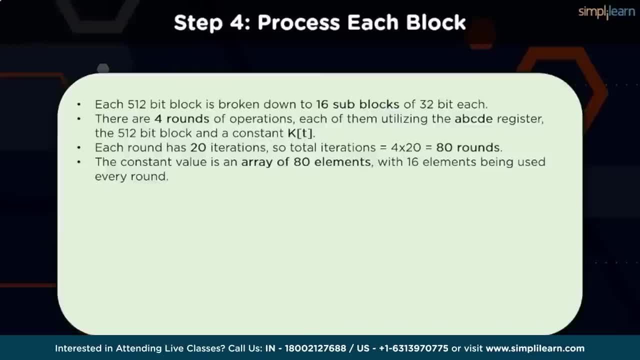 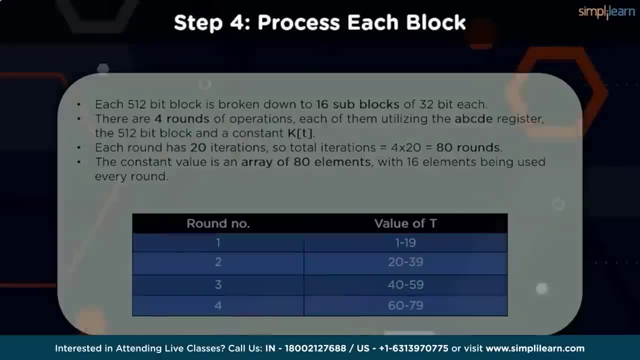 used each round, So that comes out to 80 rounds for each of those elements. The value of t differs by the number of elements. The value of t differs by the number of elements. The value of t is the number of rounds, as can be seen in the table below. 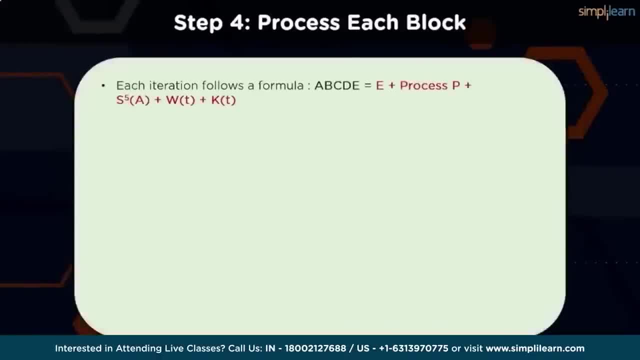 A single formula is necessary to calculate the output of each round and iteration. The formula can be A, B, C, D. E register is equal to E plus a non-linear process, P, along with a circular shift of A plus Wt plus Kt. In this formula, A, B, C, D is the register value. 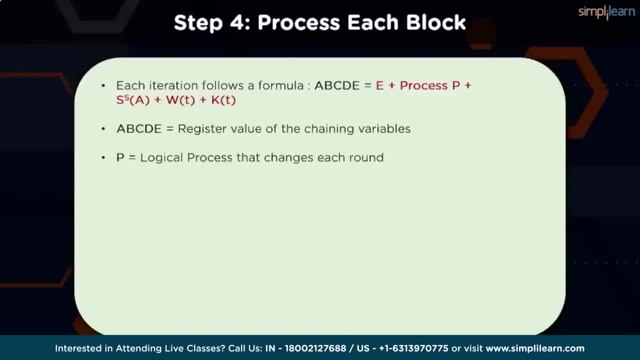 of the chaining variables, as we discussed before. P is the logical process, which has a different formula for each round. S5 is a circular shift by 5 bits. Wt is a 32-bit string derived from the existing subblock. This can be calculated depending on the iteration at hand. 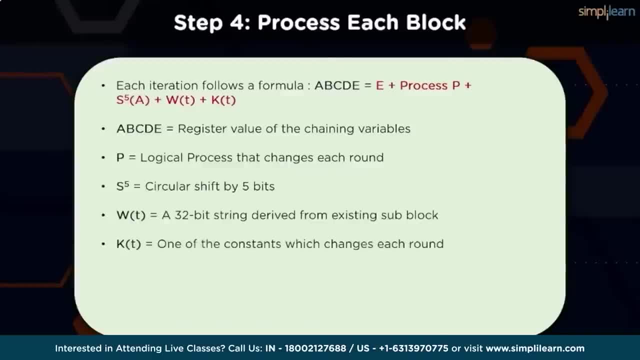 Kt signifies a single element of the 80-character element array, which changes depending on the particular round at hand. For the values of Wt, the first 16 values are the same as that of the subblocks, So there is no extra calculation needed. For the next 64 elements, the value of Wt can be calculated. 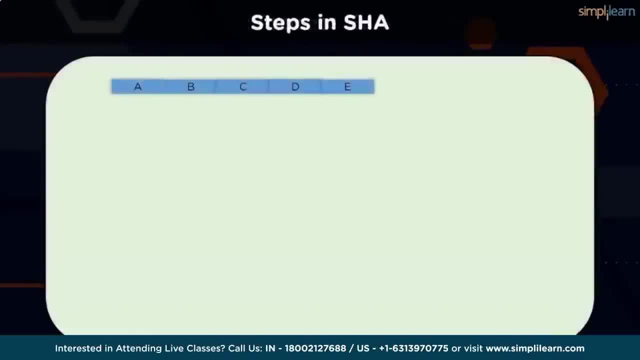 as shown in the formula here. To better understand this, let's take a look at how each of this goes in a sequential process. We have an initial register using the 5 words of 32 bits each. In the first step, we put the values of A, B, C and D to the subsequent register as 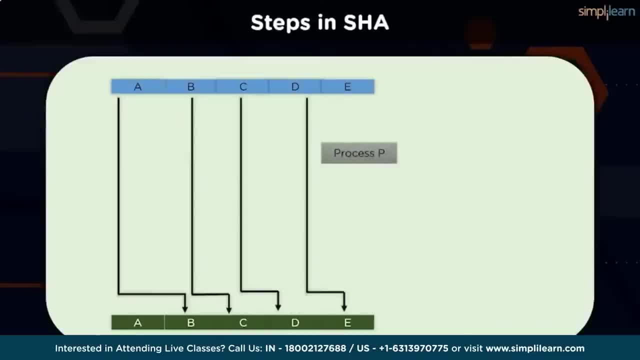 the output. Next, we use a non-linear process, P, that changes depending on the round and uses the values of B, C and D as input. Whatever output is generated from the nonlinear process, it is added with the value of the E register. Next, 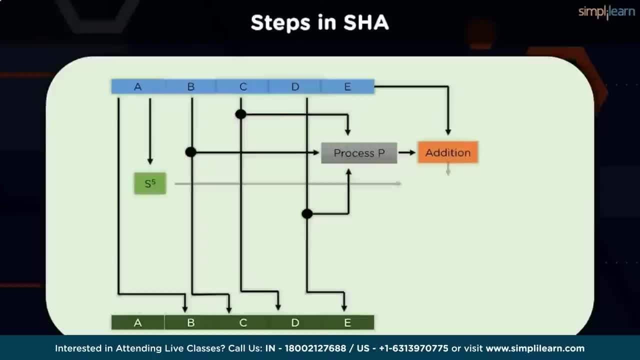 the value of A is circular, shifted by five bits and is added with the output generated in the previous step. The next step is adding the value of WT and the constant element of KT. The current output is then stored in the register A. Similarly, this iteration is repeated. 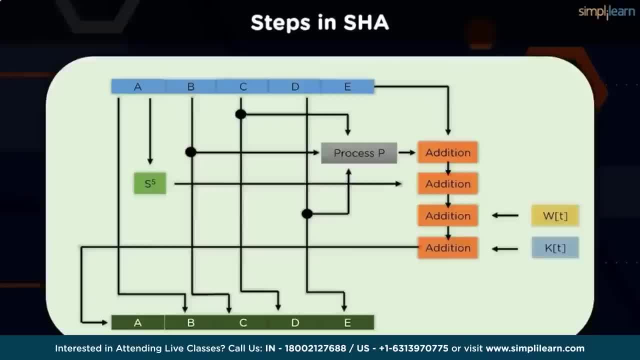 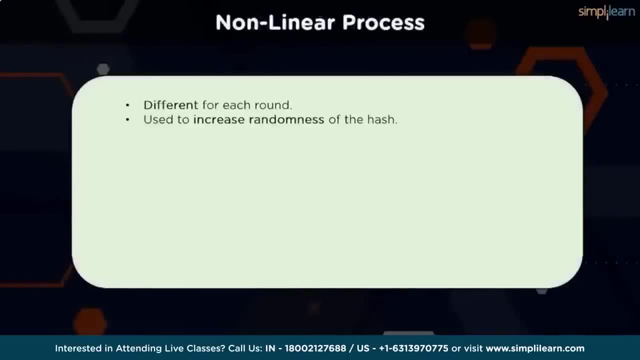 every round and for each sub block in the process. Once all the registers are complete and all the sub blocks are joined together to form the single ciphertext message, we will have our hashed output. Regarding the nonlinear process P that uses the values of B, C and D as input. the formula changes every round to maintain a complexity of the program. 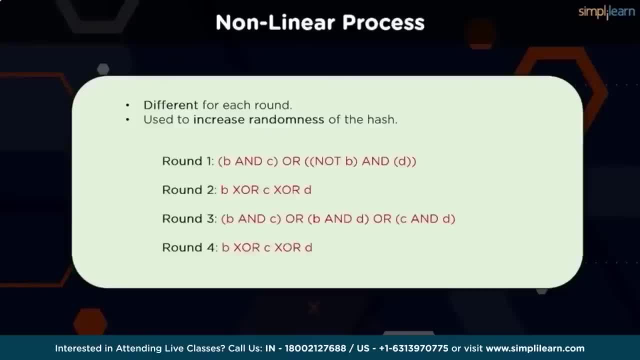 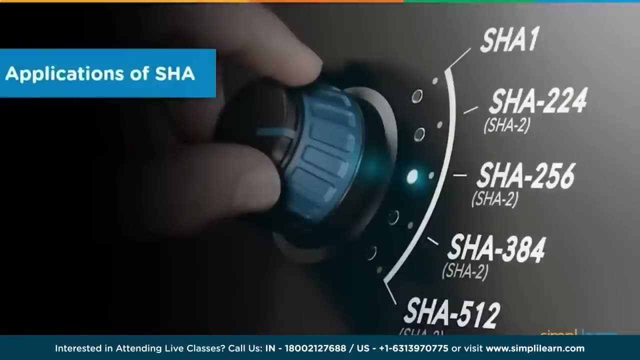 that can withstand brute force attack. Depending on the round, the values are passed through a logical operation, which is then added with the values of WT, KT and so on. Now that we understand how to get our hash digest from the plaintext, let us learn about the advantages we obtain when using the SHA. 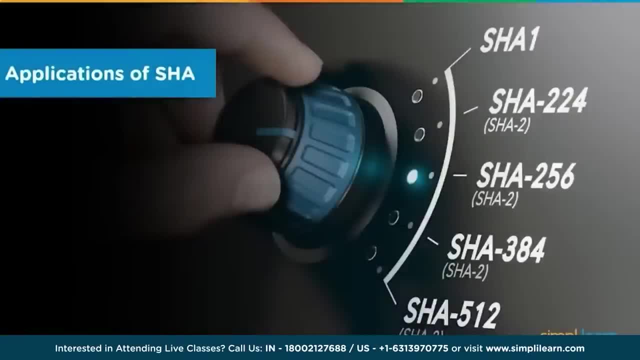 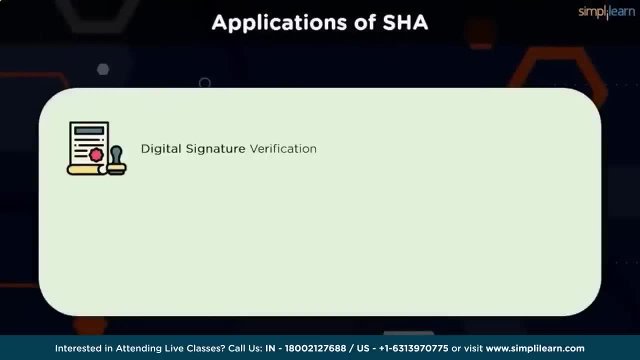 hash algorithm instead of relying on data in a plaintext format. Digital signatures follow asymmetric encryption methodology to verify the authenticity of a document or a file. Hash algorithms like SHA-256 and the industry standard SHA-512 go a long way in ensuring the verification of signatures. Passwords need not be stored in a plaintext format. 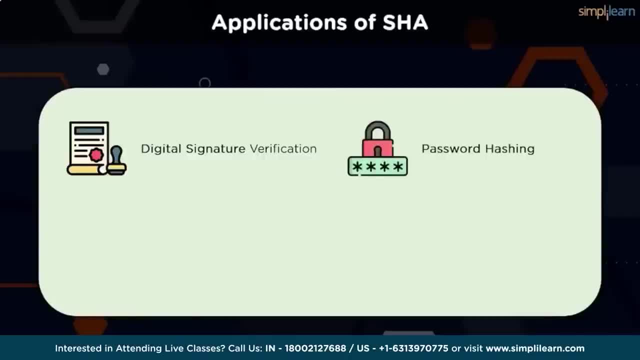 which makes them accessible to hackers and other malicious actors. When using digest, the database security also gets a boost, since the size of all hash values will be the same. In the event of a hack or a breach, the malicious actor will only receive the hash values which. 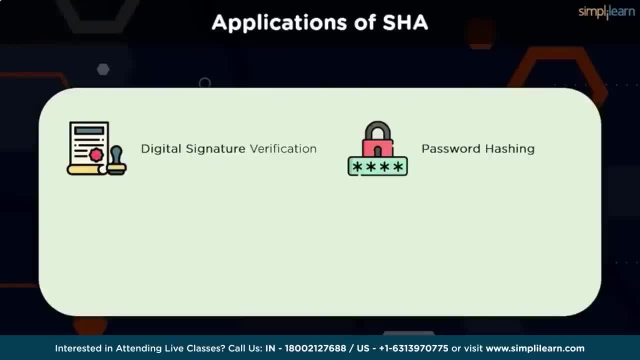 means that the hash will not be stored in the plaintext format. In this case, the plaintext would be user credentials. Since the hash functions are irreversible by design, it has become a compulsion when storing passwords on the servers. The SSL handshake is a crucial segment of the web browsing sessions and it's done using. 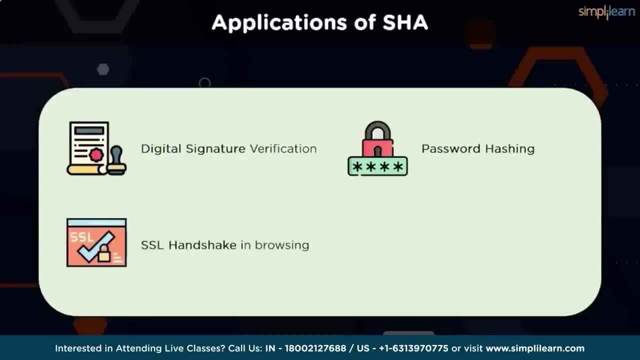 SHA functions. It consists of your web browsers and the web servers agreeing on encryption keys and hashing authentication to prepare a secure connection. It relies on a complex combination of symmetric and asymmetric algorithms which ensure the confidentiality of the data transmitted between a web server and a web client. like the browsers, 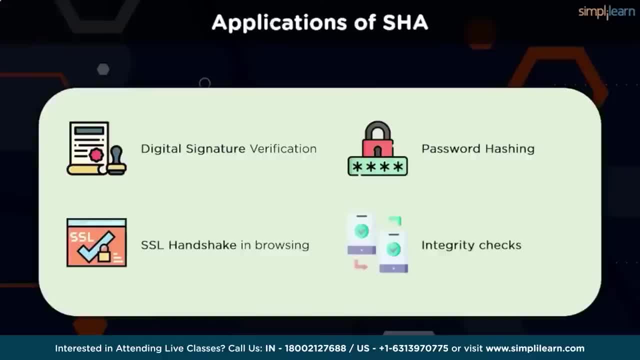 You can monitor file corruption by comparing hash values before and after transit. Once the hashes match, file integrity checks are valid and data corruption is avoided. Hash functions will always give the same output for the same input, irrespective of the iteration parameters. It also helps in 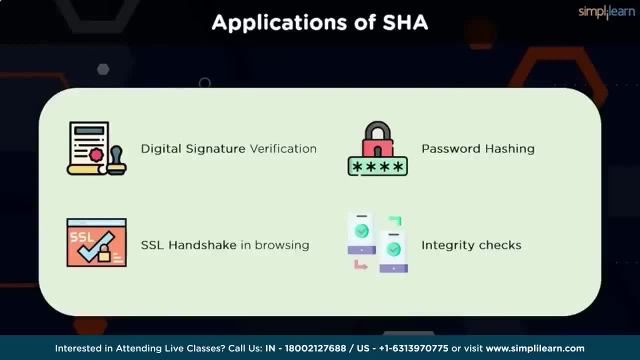 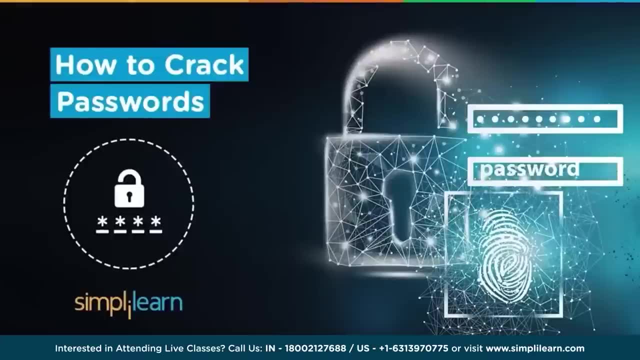 ensuring that the data hasn't been tampered with en route to the receiver of the message. Passwords are by far the most common type of user authentication. They are popular because their theory makes perfect sense to individuals and is reasonably simple to implement for developers. On the other hand, poorly constructed passwords can pose security flaws. A well-designed 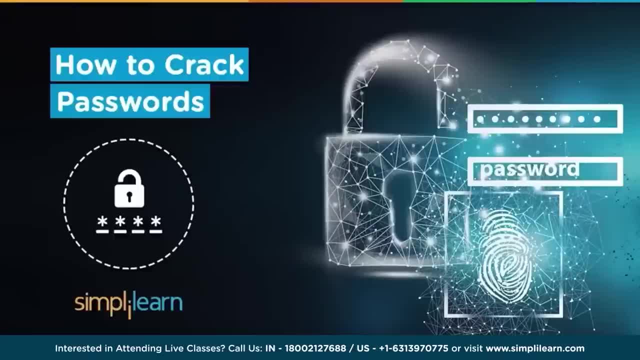 password-based authentication process does not save the user's actual password. This would make it far too simple for a hacker or a malevolent insider to access all of the passwords. In this video, you will learn how to crack passwords and simultaneously try to make your. 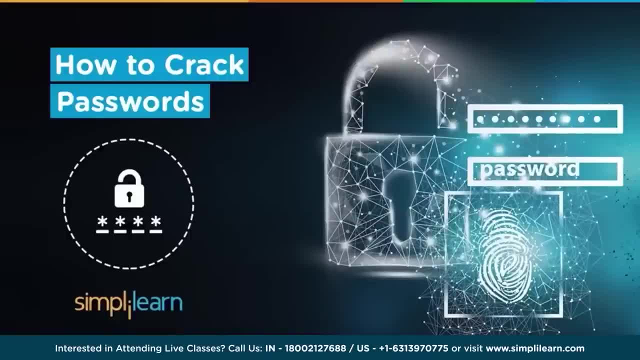 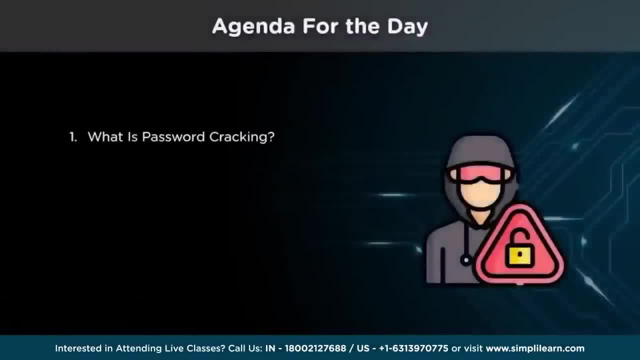 passwords as brute force resistant as possible. Let's take a look at the topics to be covered today. We start by learning about what is password cracking in general. Next, we take a look at the different techniques of password cracking that hackers use in order. 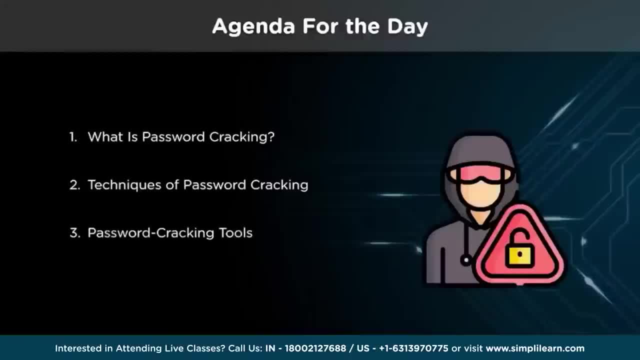 to generate user credentials for hacking. Moving on, we take a look at the multiple tools that hackers can use to generate these hashes and the passwords. Finally, we take a look at the steps and the guidelines that users can follow to prevent their passwords from being cracked. 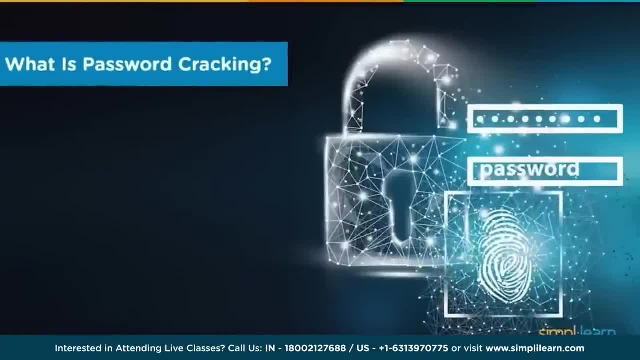 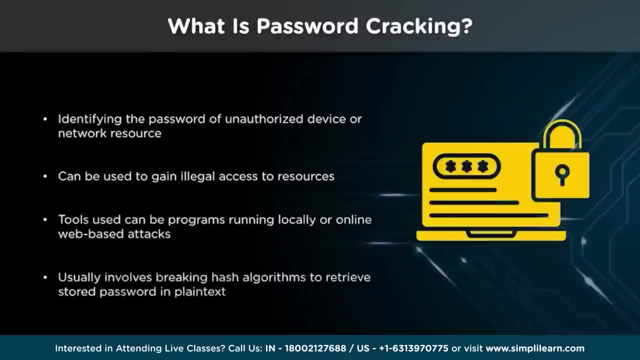 Let's start by giving a basic idea about password cracking. Password cracking is the process of identifying an unknown password to a computer or a network resource using a program code. It can also assist a threat actor in gaining illegal access to the computer. Malicious actors can engage in various criminal activities with the information obtained through. 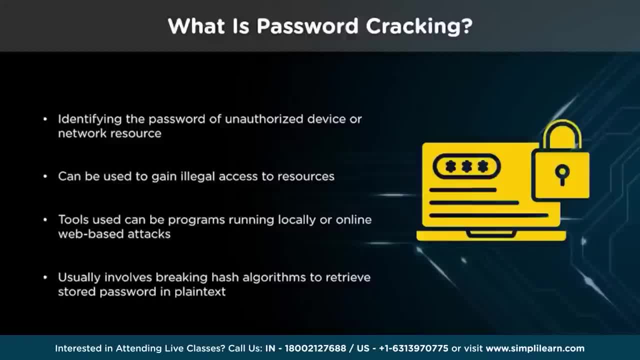 password cracking. The procedure might entail comparing a set of words to guessed credentials or using an algorithm to guess the password repeatedly. Password cracking can be done for several reasons, but the most malicious reason is in order to gain unauthorized access to a computer without the owner's awareness. This 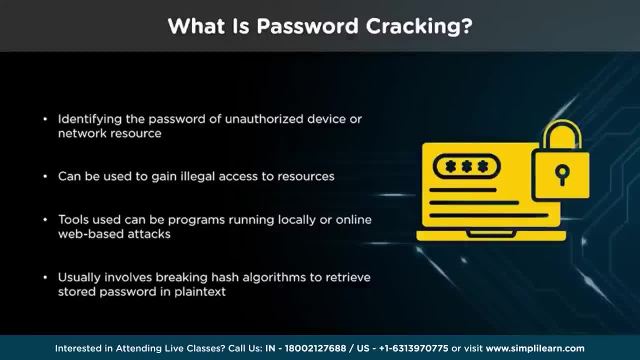 results in cybercrime, such as stealing passwords for the purpose of accessing banking information. Other non-malicious reasons for password cracking occur when someone has stolen a computer or a computer. These reasons include the possibility that the computer is being hacked. Password cracking is a process that can be done for multiple reasons. This can also: 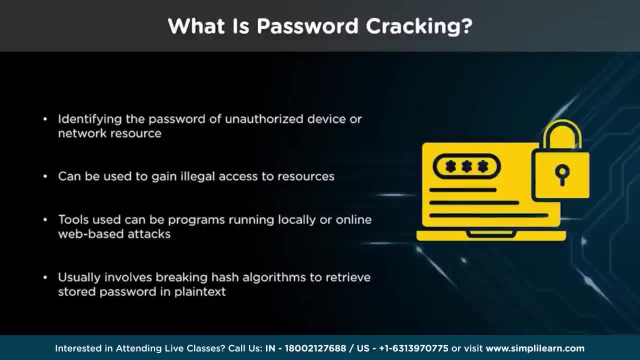 be done for multiple reasons, such as the power of a computer, The number of passwords, and the number of passwords and the number of passwords are different, For example, if the computer is someone has misplaced or forgotten a password. Another example of non-malicious password cracking may take place if a system administrator 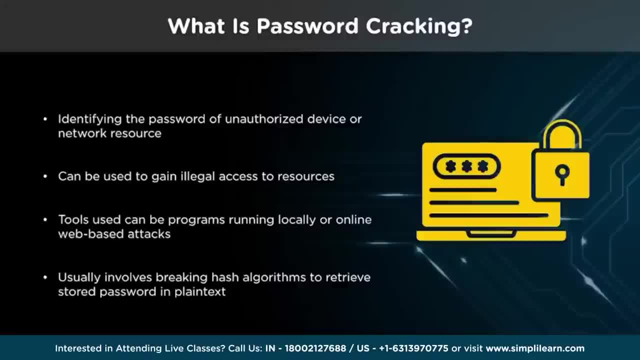 is conducting tests on password strength as a form of security test. This enables so that the hacker cannot easily access protected systems. The best way that users can protect their passwords from cracking is to ensure that they choose strong passwords. Typically, passwords must contain a combination of mixed-case random letters, digits and symbols. 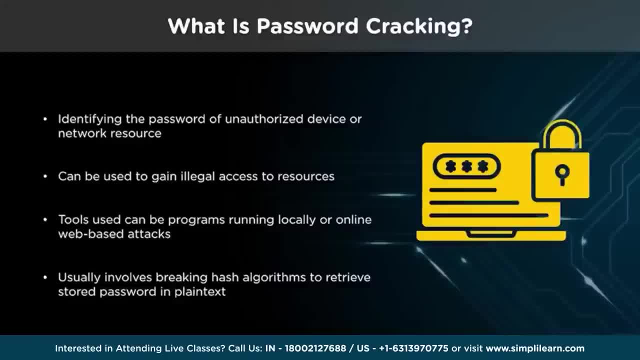 Strong passwords should never be actual words. In addition, strong passwords are at least 8 characters long. In many password-protected applications, users are notified of the strength of the password they have chosen upon entering it. The user can then modify it and strengthen the password based on the indications of its 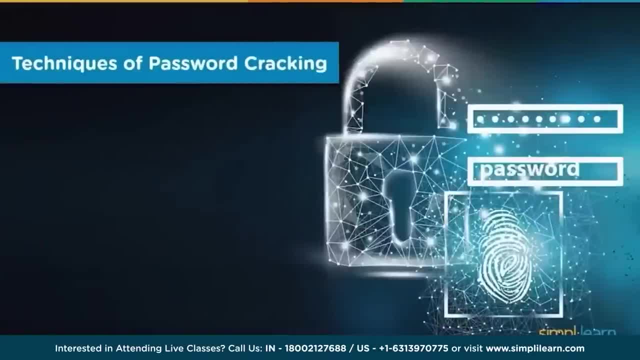 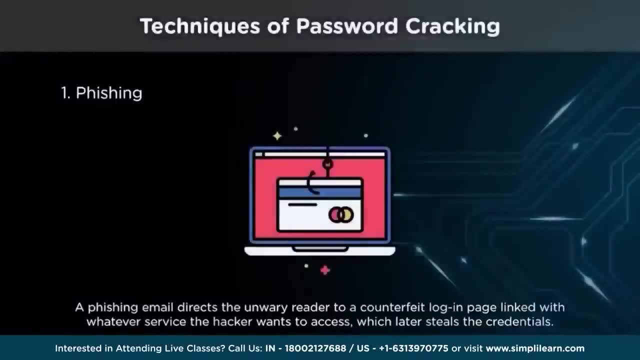 strength. Now that we understand the basics of password cracking, let's go to the basic techniques hackers use to retrieve passwords from general victims. Asking the customer for their password is a simple approach. A phishing email directs the unwary reader to a counterfeit login page, linked with whatever. 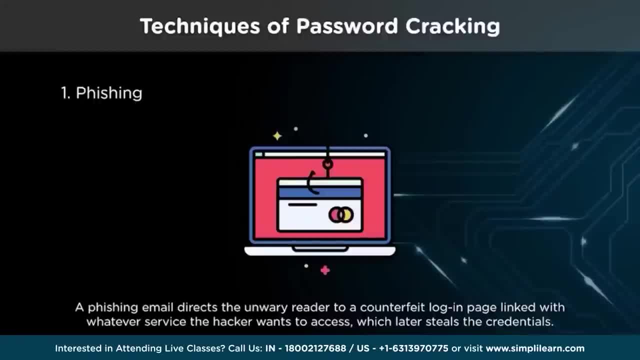 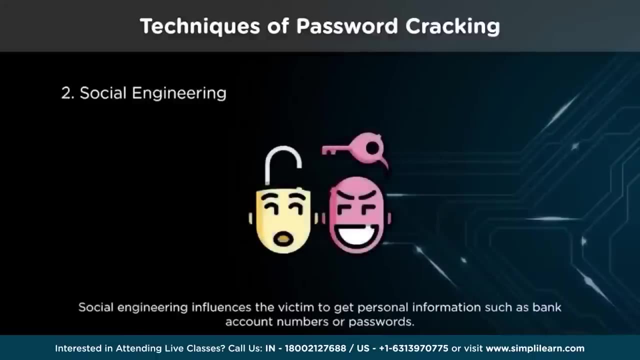 service the hacker wants to access, generally by demanding the user fix some critical security flaw or aid in a database reset. That page then captures their password, which the hacker can subsequently exploit for their own purpose. Social engineering influences the victim to get personal information such as bank account. 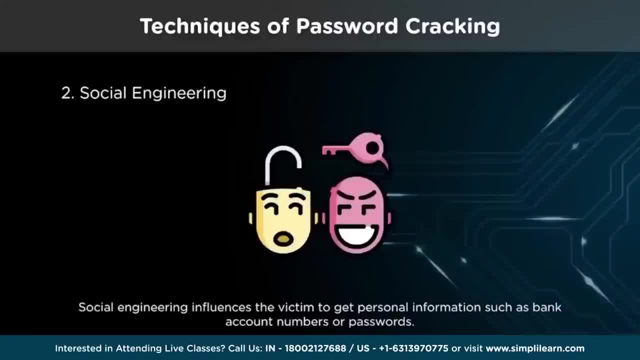 numbers or passwords. The strategy is popular among hackers because they realize that humans are the gateway to vital credentials and information. Through social engineering, the employee tried and true tactics to exploit and influence age-old human tendencies rather than devising novel means to breach secure and advanced. 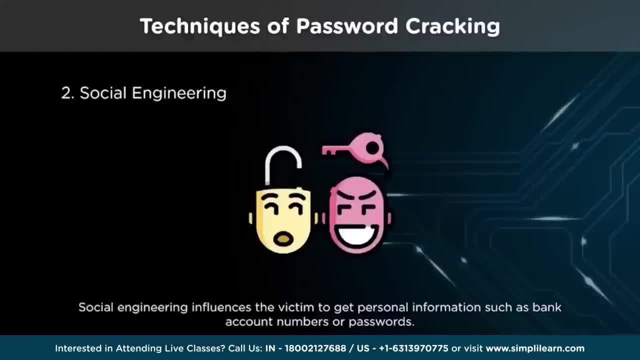 technologies. It has been demonstrated that many firms either lack adequate security or are overly friendly and trustworthy, when they should not be. They allow granting access to critical facilities based on a uniform or a software. This is the first time a hacker has done this. 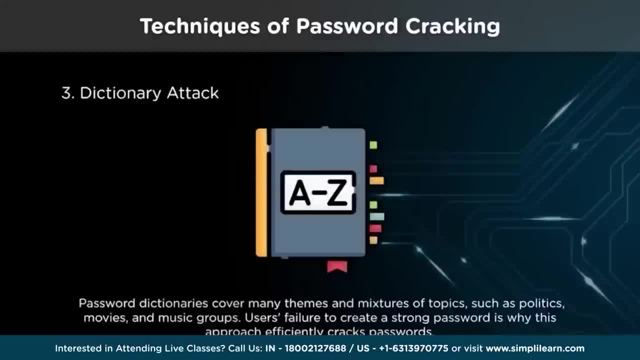 This is the first time a hacker has done this. It is a job story. A hacker searches a password dictionary for the correct password in the case of a dictionary attack. Password dictionaries cover many themes and a mixture of topics such as politics, movies. 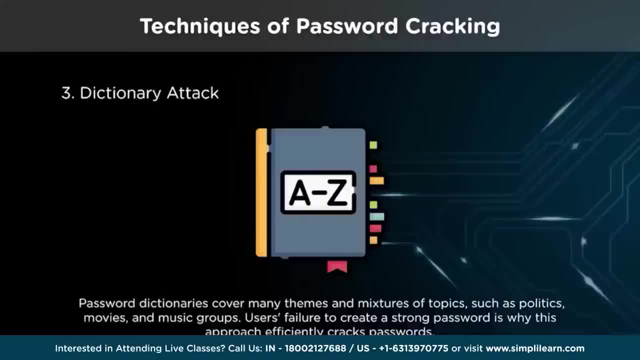 and music groups Users'. failure to create a strong password is why this approach efficiently cracks passwords day-to-day. Simply said, this assault employs the same terms that many individuals use as passwords. A hacker can compare the password hash obtained to the hashes of the password dictionaries. 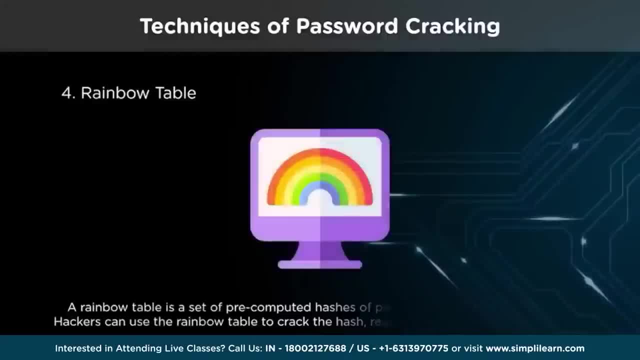 to find the correct plain text password. Now that the passwords have been hashed, the hackers attempt to achieve authentication by breaking the password hash. They accomplish this by employing a rainbow table, which is a set of pre-computed hashes of portable password combinations. 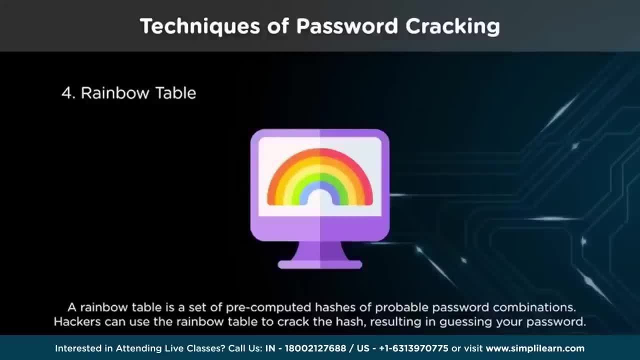 Hackers can use the rainbow table to crack the hash, resulting in guessing your password. As a result, it retrieves the password hash from the system and eliminates any need to break it. Furthermore, it does not necessitate the discovery of the password itself. 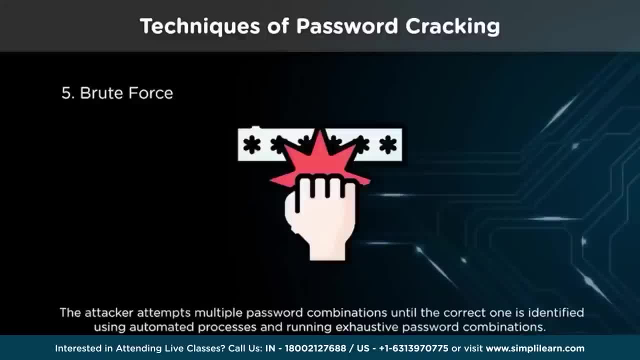 The breach is accomplished if the hash matches In a brute force assault. the attacker attempts multiple password combinations until the correct one is identified. The attacker uses software to automate this process and run exhaustive password combinations in a substantially shorter length of time. With the growth of hardware and technology in recent years, such programs have been invigorated. 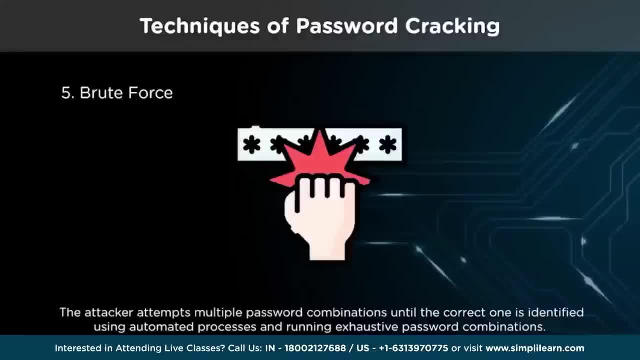 It won't be quick if your password is more than a few characters, But it will eventually reveal your password. Brute force assaults can be sped up by throwing more processing resources at them. With so many different techniques coming together to crack passwords, none of them are useful without the right tools. 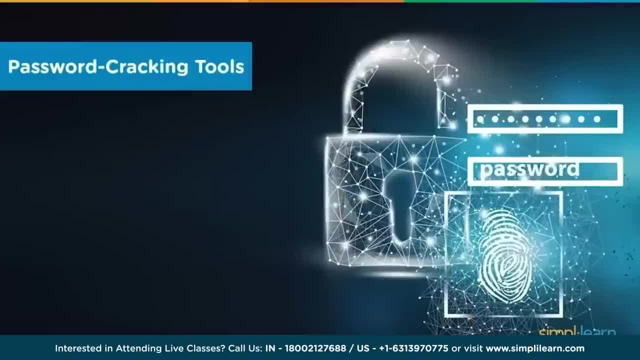 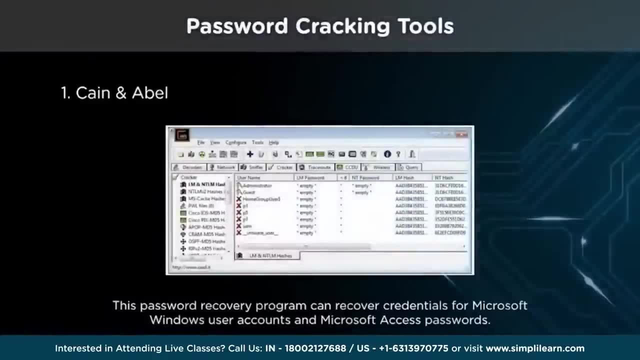 There are a plethora of scripts and snippets of code that can retrieve passwords from either encrypted storage or from the hash digest. Let's go through some of these tools. Cain and Able is a password recovery tool for Microsoft operating systems. It allows easy recovery of various kinds of passwords by sniffing the network. 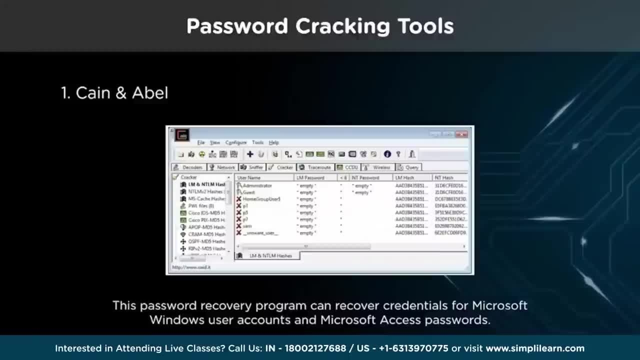 cracking encrypted passwords using dictionary brute force and cryptanalysis attacks, Recording VoIP conversations, decoding scrambled passwords, recovering wireless network keys, etc. are some of the other features of Cain and Able. The latest version is faster and contains a lot of new features like ARP, Poison Routing. 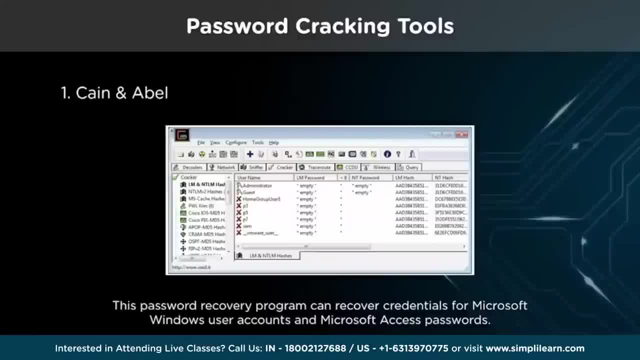 which enables sniffing on switched LANs and man-in-the-middle attacks. The sniffer in this version can also analyze passwords and can also analyze encrypted protocols such as SSH1 and HTTPS, while containing filters to capture credentials from a wide range of authentication mechanisms. 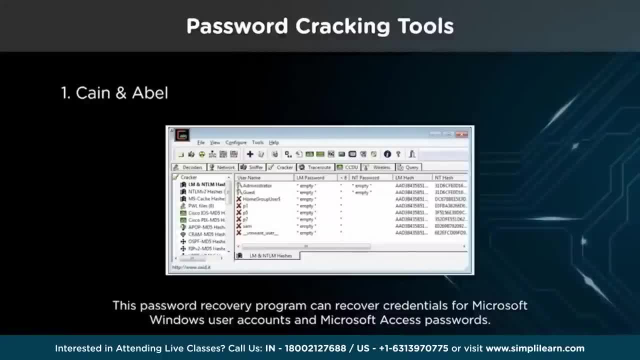 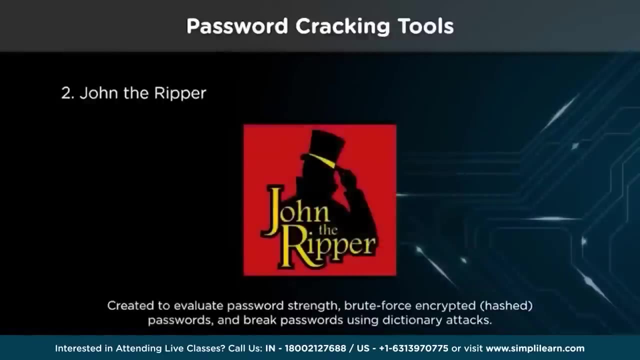 It also ships routing protocol, authentication monitors and route extractors. Dictionary and brute force crackers are also present, along with common hashing algorithms and several specific authentications, password hash calculators and other features. John the Ripper is a password cracking app that was first released in 1996 for Unix-based computers. 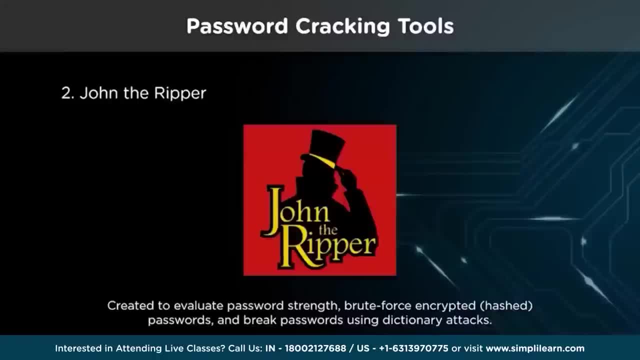 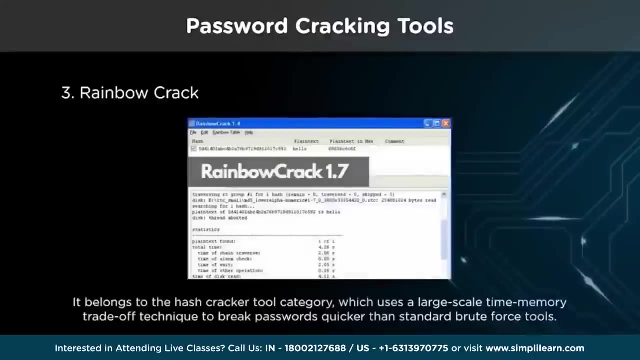 It was created to evaluate password strength, brute force, encrypted hash passwords and break passwords using dictionary attacks. It can use dictionary attacks, rainbow tables and other attacks, depending on the target type. Rainbow Crack is a password tracking application that uses time-memory trade-off algorithm. 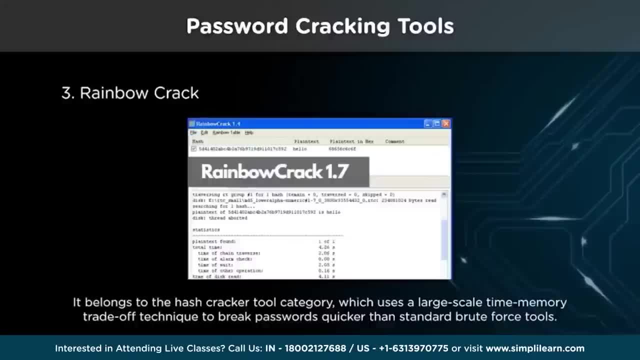 to crack password hashes with rainbow tables. Rainbow tables make password cracking more easier and faster than traditional brute force attacks. It is like a dictionary containing nearly every possible password and the pre-calculated hashes. Creating this kind of dictionary takes much more time than cracking a single hash. 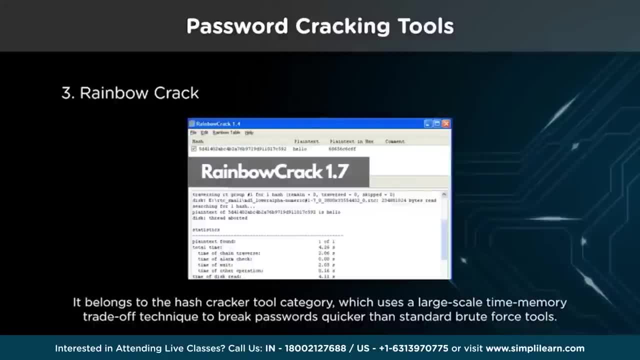 but after that you can use the same dictionary over and over again. This procedure might take a long time. However, once the table is ready, it can break passwords far quicker than brute force methods, With so many tools ready to nab our passwords. 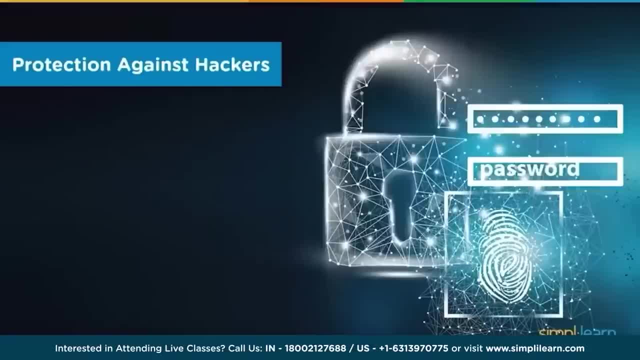 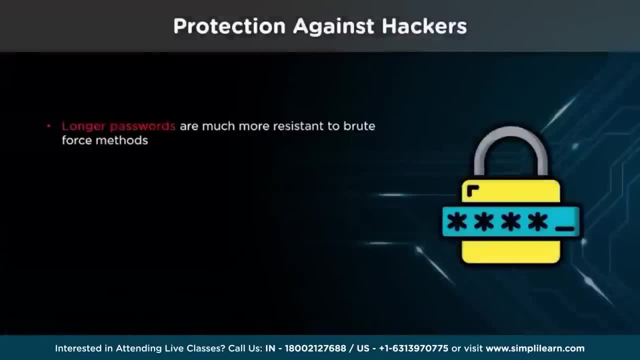 there are a certain set of rules users can follow to protect their credentials from being compromised. Let's cover some of these guidelines. Longer passwords are required, making the brute force mechanism tougher to implement. Longer passwords and passphrases have been demonstrated to boost security significantly. 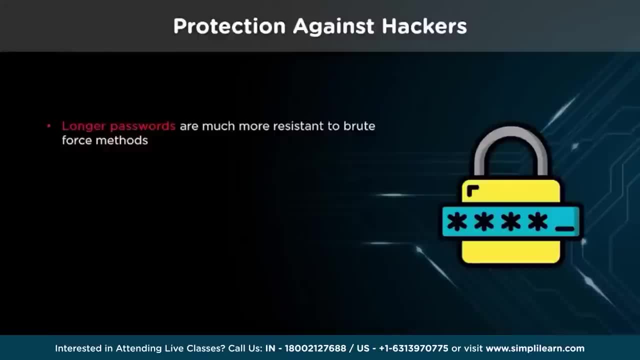 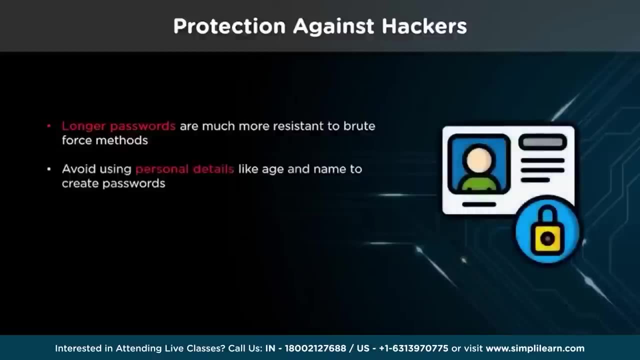 However, it is still critical to avoid lengthier passwords that have previously been hacked or that feature often in cracking dictionaries. This password policy encourages users to be more careful to establish passwords that do not contain personal information. As previously said, most users create passwords utilizing personal information. 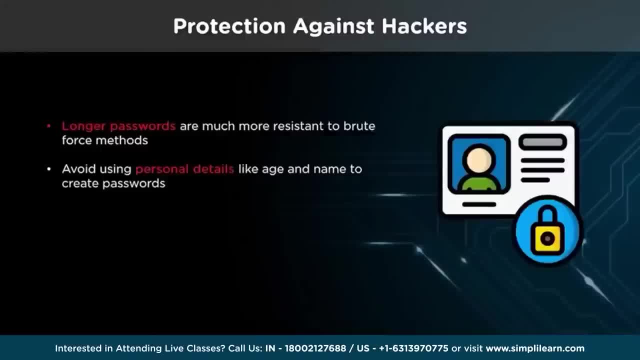 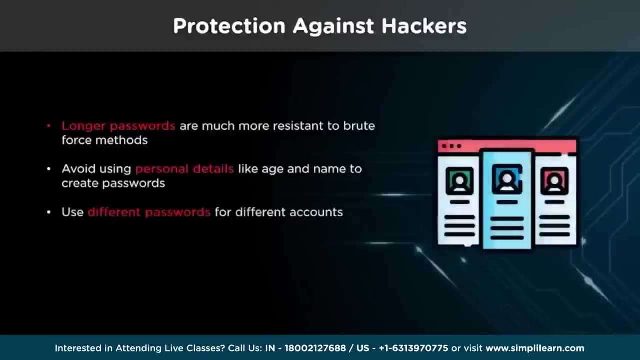 such as hobbies, nicknames, pet or family member names, etc. If a hacker has access to personal information about a specific user, for example via social media, they will test password combinations based on that knowledge. Password regulations should compel users to distinguish between security and convenience. 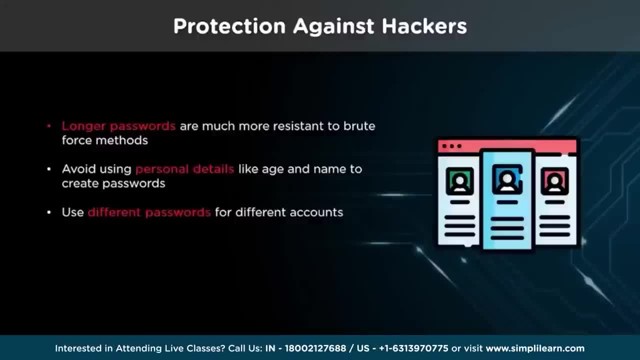 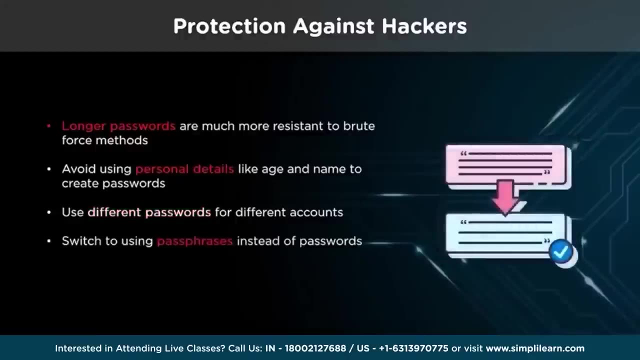 Users should be prohibited from using the same password for all services. Password sharing between users, including those who work in the same department or use the same equipment, should be avoided. A single breached password doesn't affect your other accounts. with this policy, Some password regulations necessitate the creation of a passphrase rather than a password. 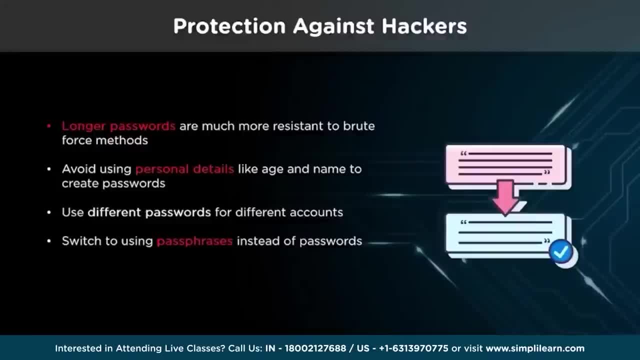 While passphrases serve the same objective, their length makes them more difficult to break. In addition to letters, a good pass should include numbers and symbols. Passwords may be easier for users to remember than passphrases. However, the latter is much more breach-resistant. 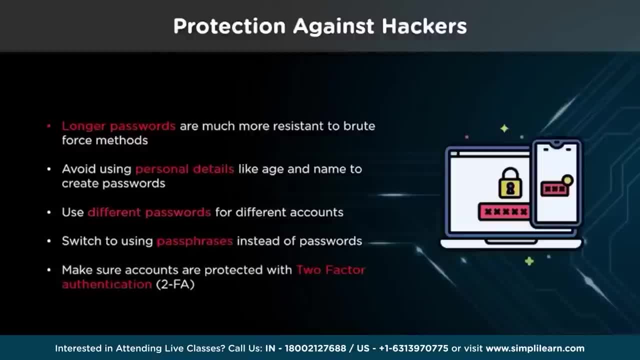 Two-factor authentication, or 2FA, can help secure an online account or even a smartphone. 2FA does this by asking the user to provide two forms of information: a password or a personal identification PIN, and a code texted to the user's smartphone or a fingerprint, before accessing whatever is secured. 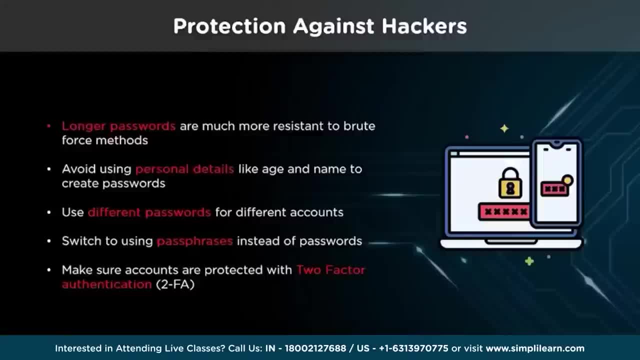 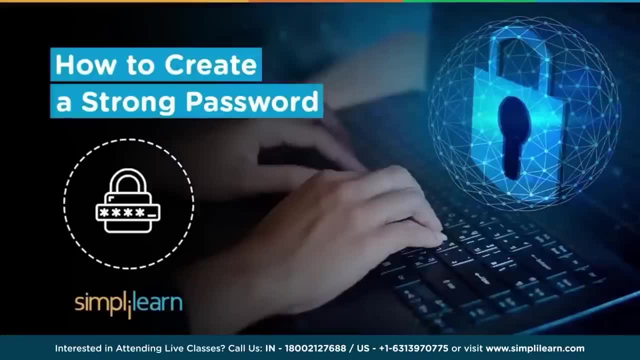 This helps discourage unauthorized entries to an account without the original owner's permission. At this point, you may wonder why you need a strong password in the first place. Even if most websites are safe, there is still a danger that someone will try to access or exploit your information. 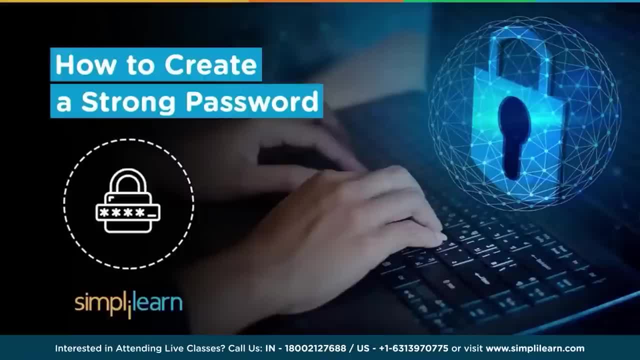 A strong password is among the most effective ways to protect your accounts and personal information from hackers. You should follow certain rules and guidelines while creating a strong password. Password managers are also recommended to help remember the created passwords for convenience of usage. With that being said, let's take a look at the topics we are covering today. 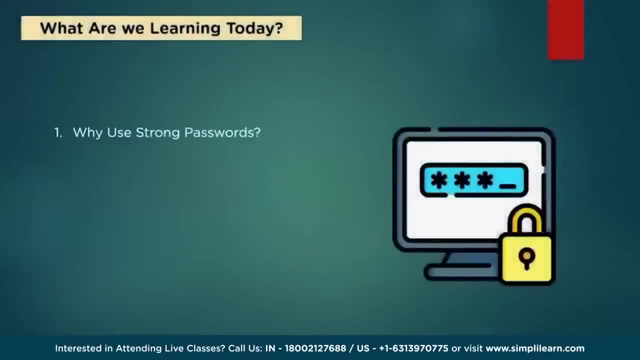 We start by learning about the state of password cracking in today's world and why creating strong passwords is an absolute must for every account. Next, we will look at some guidelines and rules that help strengthen passwords and make password cracking a daunting task for hackers. 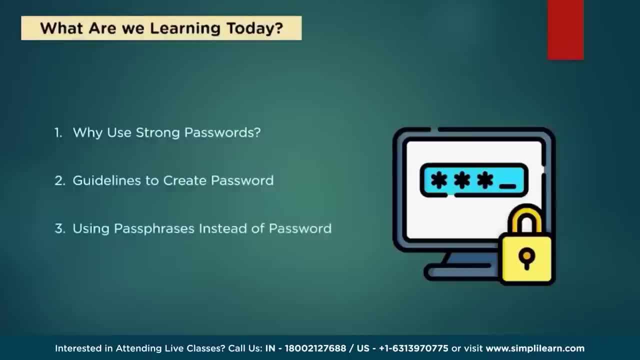 Moving on, we understand why passphrases have gone in popularity and are being recommended for credentialing. And finally, we take a look at how password managers help alleviate the problem of creating and remembering complex passwords along with other critical personal information. Let's start by learning about why strong passwords have become an absolute necessity. 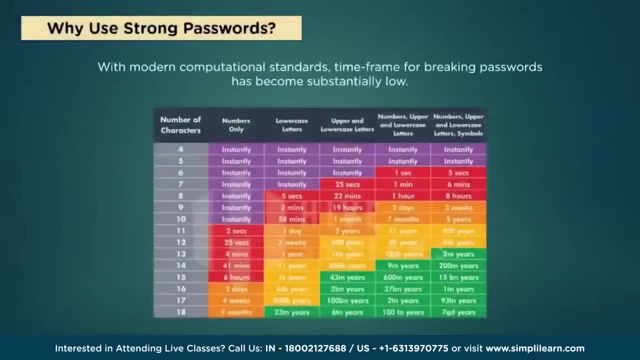 One of the most common ways that hackers break into computers is by guessing passwords. Simple and commonly used passwords enable intruders to easily gain access and control a computing device. Conversely, a password that is difficult to guess makes it prohibitively difficult for common hackers to break into a machine and will force them to look for another target. 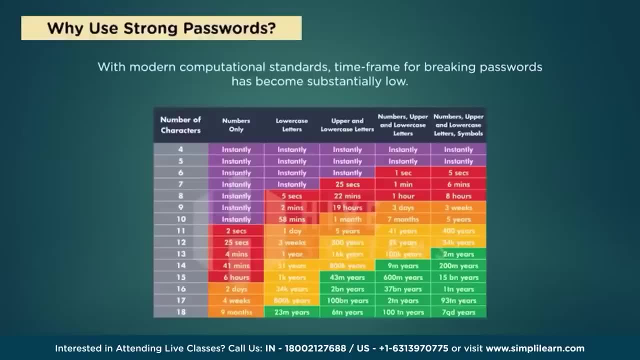 The more difficult the password, the lower the likelihood that one's computer will fall victim to an unwanted intrusion. Many individuals opt to tie their websites to something they can readily recall, to generally easy, memorable combos. However, this does not make the password unique. 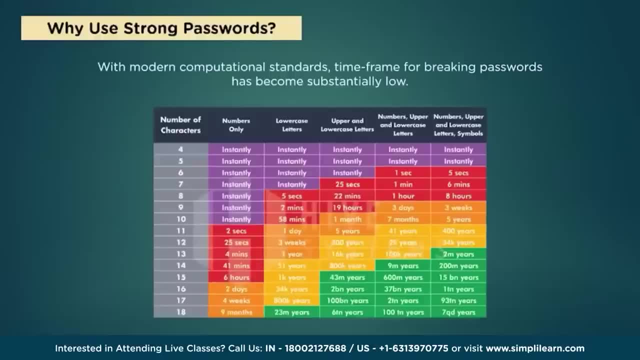 In fact, it's the reverse. Passwords are handled by 53% of individuals using their recollections and memory. With modern computational standards, simple passwords take seconds and a couple of minutes at worst to be completely brute-forced. According to global surveys, more than 60% of people use the same passwords. 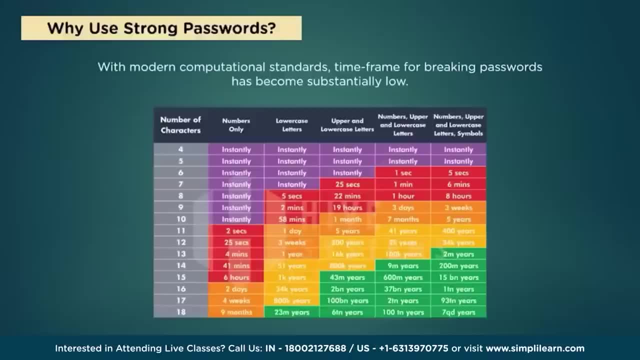 for their personal and job applications. While this may allow the user never to forget the password, it makes a single point of failure: the only pin to drop. If one of the accounts gets breached. all subsequent accounts are as good as hacked. To further elaborate on how you can create strong passwords, 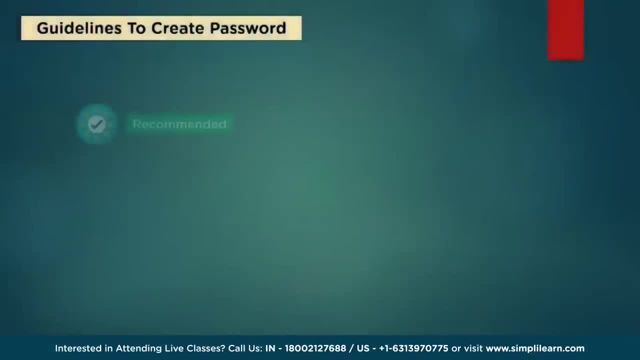 let's go through some of the guidelines. Let's go through some do's and don'ts to understand how to create new passwords for our accounts. It is recommended to keep the password length at least 12 characters to ensure brute forcing to be difficult. 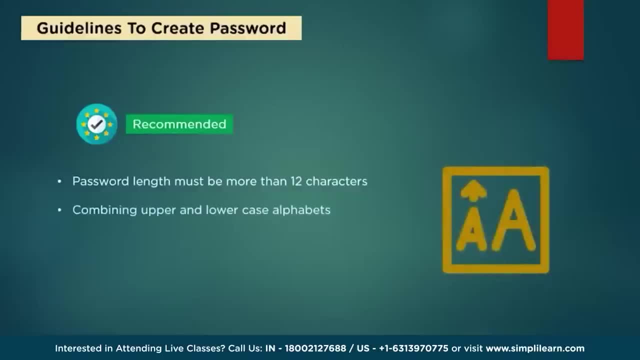 A combination of upper and lowercase alphabets is an absolute necessity when creating strong passwords. It is also recommended to use numerics along with those alphabets to create a complicated password. Finally, special characters help in making a password much more brute force resistant. 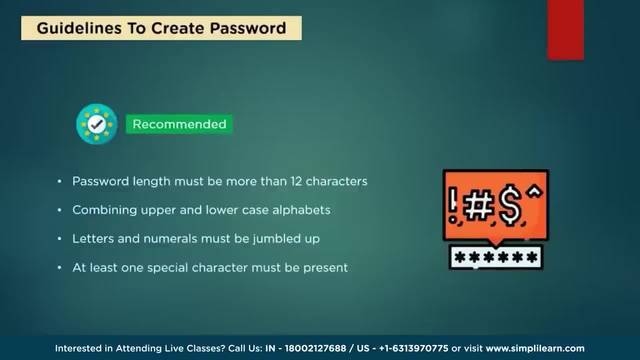 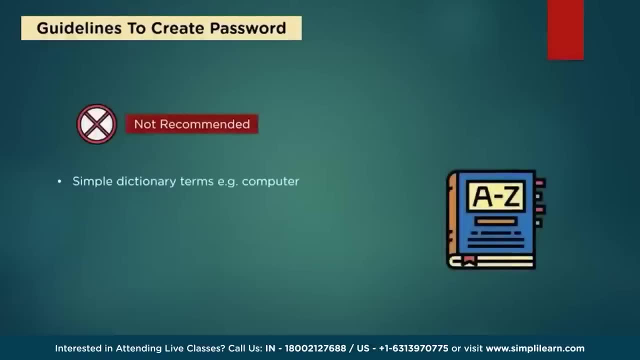 than any number of alphabets or letters can make. Moving over to the don'ts section, it is absolutely not recommended to keep simple dictionary terms such as computer or even the word password as your credential, because those are very easy to be brute forced. 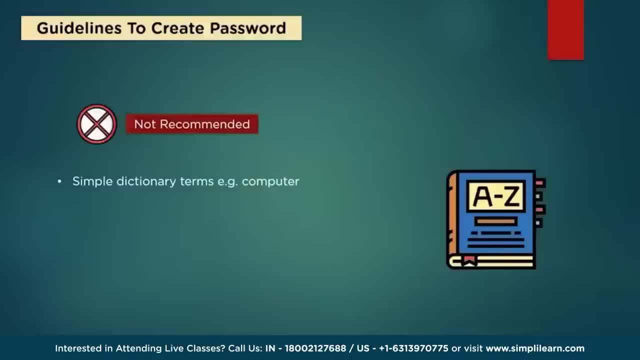 and are usually present in majority of the dictionary attack word list. Similarly, changing a single alphabet or a single character in a dictionary word does not make it brute force resistant, considering there are already algorithms present that can counter this tactic, Using the same character multiple times in a password. 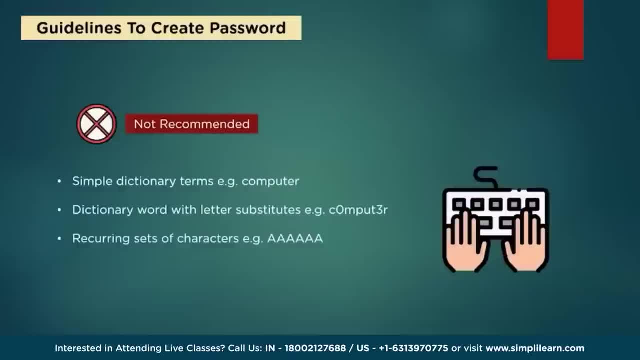 also reduces the strength and makes it easier to crack for hackers. Apart from using single characters multiple times, following patterns that are present on the traditional English keyboard, such as E-W-E-R-T-Y, or the line below the main alphabet, such as the Z-X-C-V-B-N-M, etc. 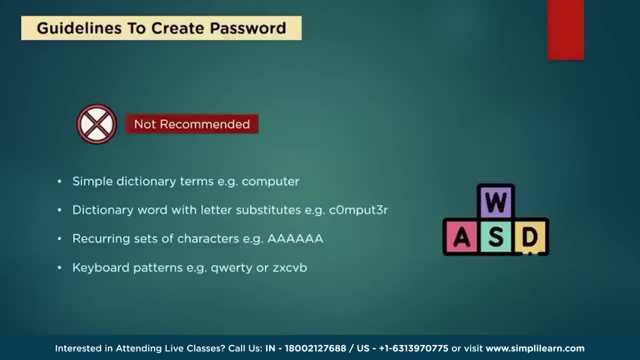 make it easier to guess, since these are, once again, common combinations that are present in word list already. Finally, the most important part being not using personal information, such as birthdays, addresses and other important information, in the passwords. More often than not, if a hacker is trying to break into your account, 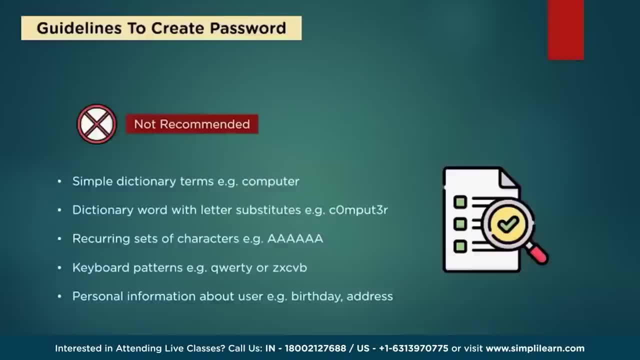 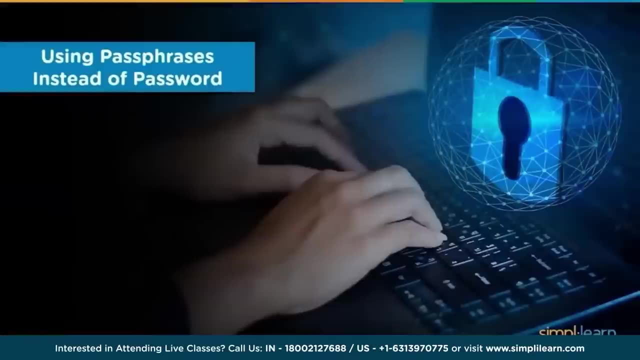 there has been some amount of research done, be it via social media or any other medium. If they have already this information present with them, breaking into your account becomes all the more easier Now that you understand how to create strong password. look at how passphrases have become prevalent. 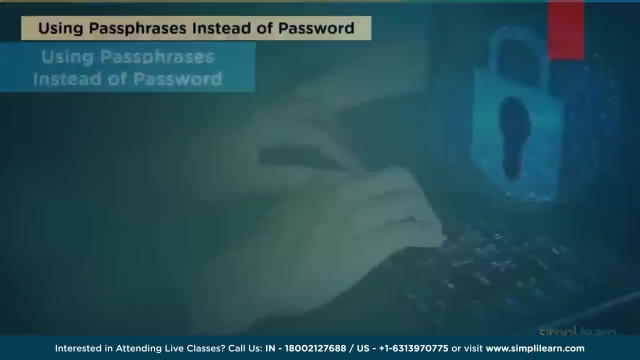 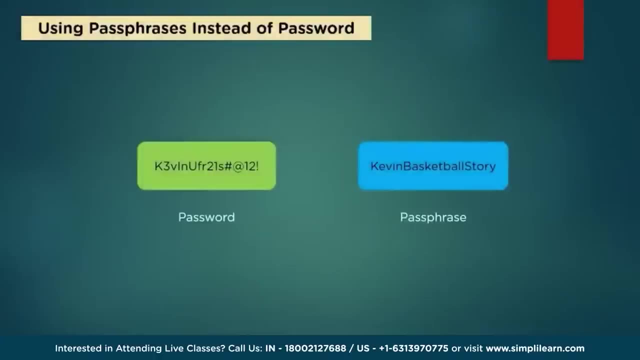 as a replacement for plain text passwords. A passphrase is a sentence-like string of words used for authentication that is longer than a traditional password, easy to remember and difficult to crack. Typical passwords range, on an average, from 8 to 16 characters, while passphrases can reach up to 100 characters or more. 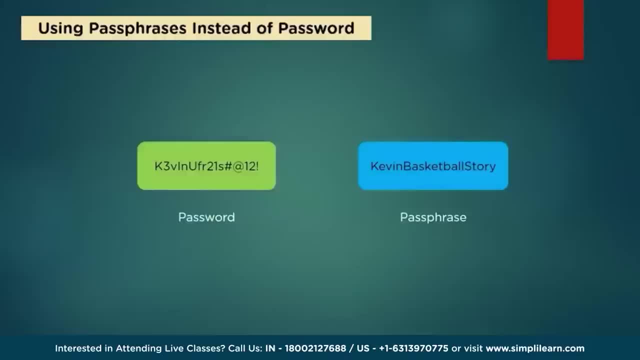 Using a long passphrase instead of a short password to create a digital signature is one of the many ways that users can strengthen the security of their data, devices and accounts. The longer a passphrase is, the more likely a user is to incorporate bits of entropy or factors. 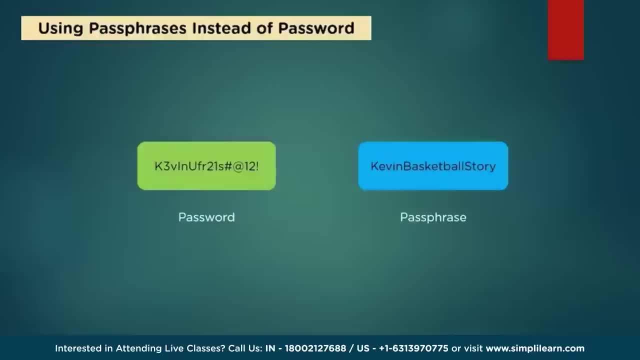 that make it less predictable to potential attackers. As more websites, applications and services increase the user security requirements, a passphrase is a fast and easy way to meet these criteria. Let's take a look at some of the advantages that passphrases have over common passwords. 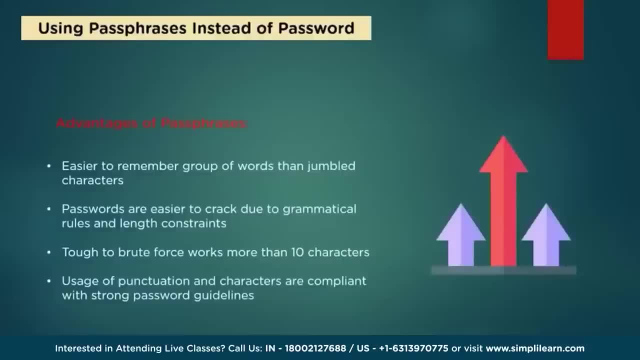 Passphrases are simpler to remember than just a random assortment of symbols and characters. It's easier to comprehend a line from your favorite song or a quotation than a short but difficult password. Passwords are reasonably easy for humans and robots to guess or crack. 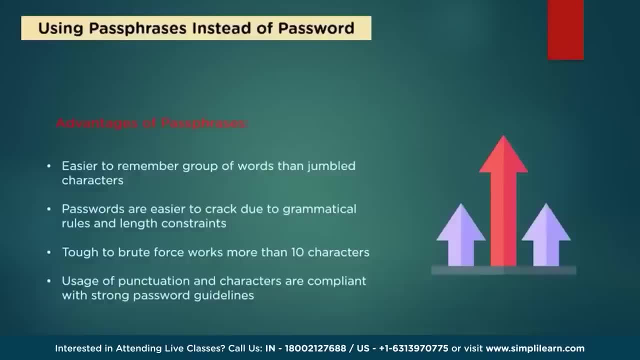 Online thieves have also advanced and created cutting-edge hacking tools to crack even the most complex passwords. Passphrases are nearly hard to crack, since most efficient password-cracking programs fail at approximately 10 characters. As a result, even the most sophisticated cracking tool will be unable to guess. 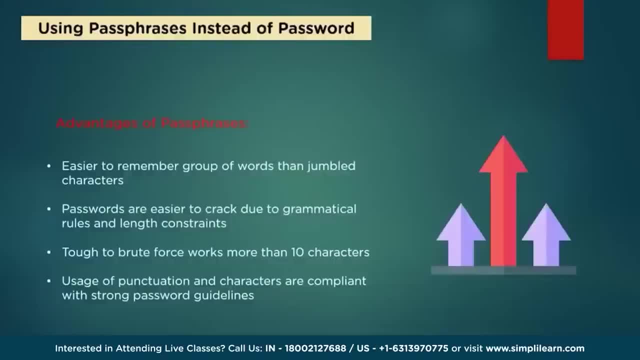 brute force or pre-compute these passwords. Compliance with password-setting rules with ease are passphrases. The usage of punctuation and upper and lower-case passwords satisfy the password complexity criteria. Most operating systems and apps support passphrases. Phrases of up to 127 characters are permitted on all major operating systems. 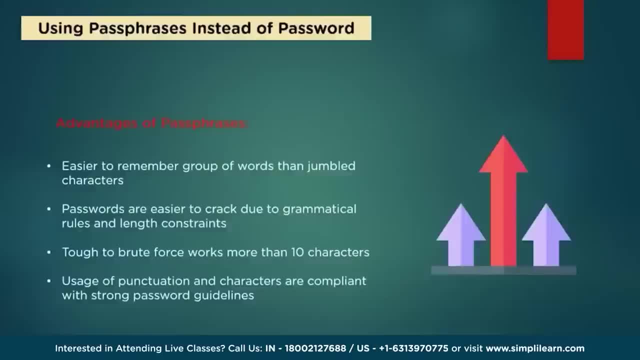 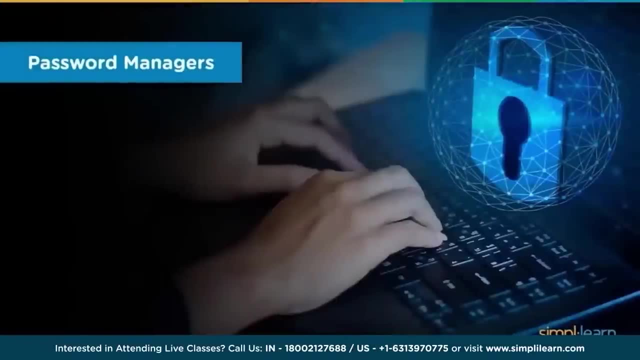 including Windows, Linux and Mac. As a result, for optimal protection, you can use lengthier passphrases, But when creating a strong password, the major problem people come across is remembering these passwords or the passphrases. This is where you can find a use for a password manager. 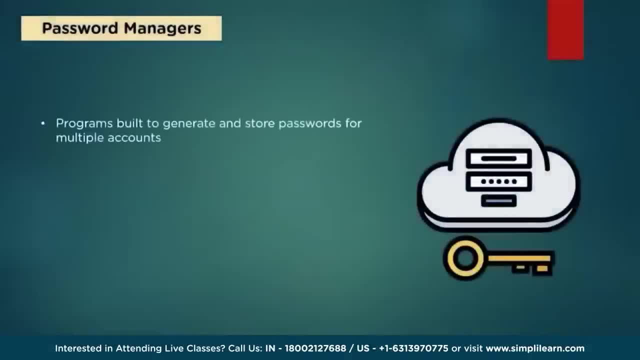 When you establish accounts or change passwords, password managers generate new strong passwords and they keep all of them in one place, protected by a single strong master password. If you maintain your master password, the manager will retain everything else, including your username and passphrases, and fill them in for you whenever you sign on to a website. 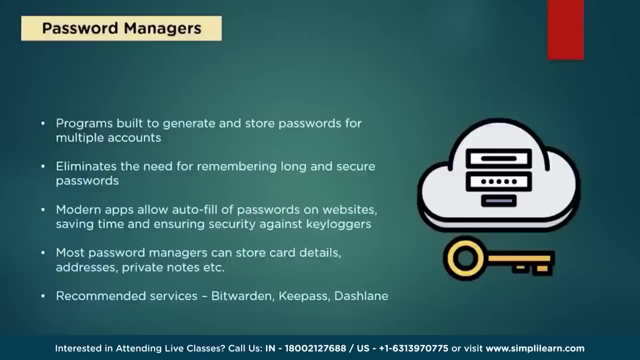 or app on your computer or phone. There is no good memory needed for this. This implies that everyone may use the most recent suggestions for strong passwords, such as extended phrases, symbols, grammar and capitalization. Password managers enable consumers to write a single master password. 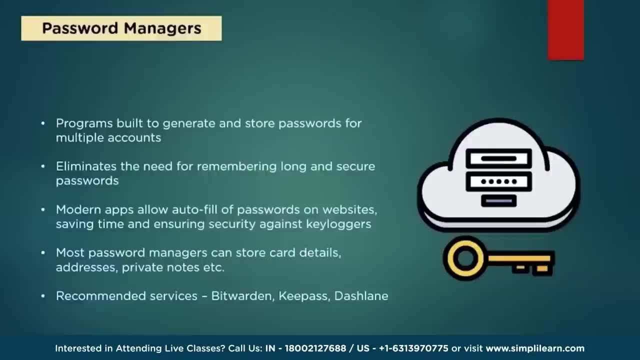 and automatically fill each website with their own unique set of credentials And not just passwords. Credit card information may be stored securely with several password managers. Some others make multi-factor authentication or use a second test, such as answering a question once the correct password is input. 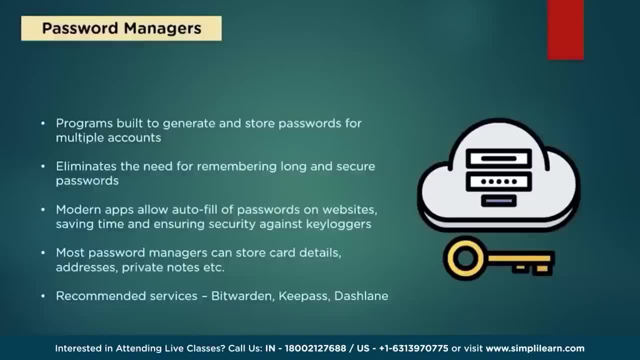 which is a simple and effective solution to verify legitimate login inputs. Among the global players in password managers, services like Bitwarden, KeePass and Dashlane have been running for years now and are very worthy recommendations if you want to get started with password management. 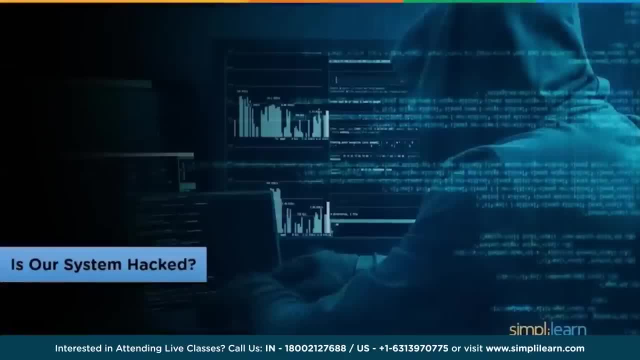 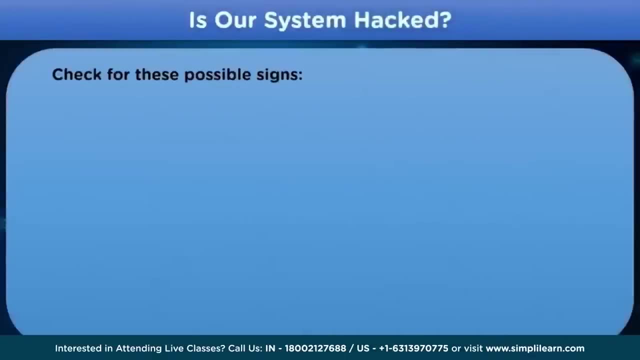 Now that we understand what is hacking, let's take a look at some points to know whether a system is already hacked or not. The first point regarding how to check whether a system is hacked or not can be cases where the system security is switched off by unknown means. 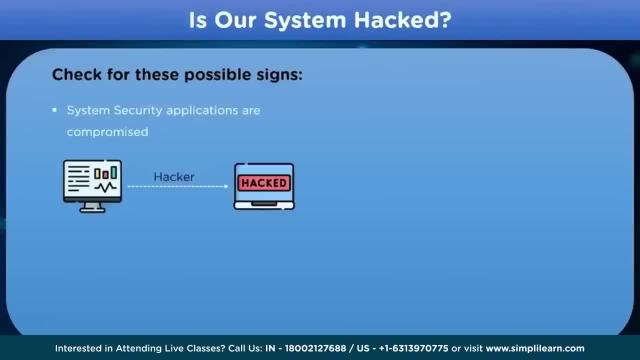 and it is not visible to the user. This is one of the most primary checkpoints to know if a system is hacked or not. Next point to check whether a system is hacked or not would be frequent antivirus software failures which are due to the interference from hacking attempts. 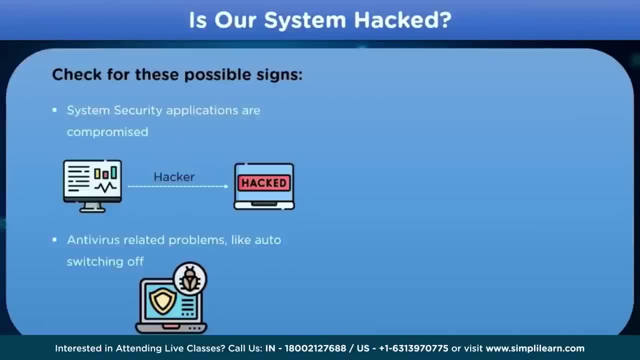 performed by a professional hacker or a cybercriminal. Then we also face problems regarding system's reaction speed, which is affected due to the execution of unknown applications in the background of the system, Which also affects the hardware resources in the device. Next, we also face problems regarding passwords. 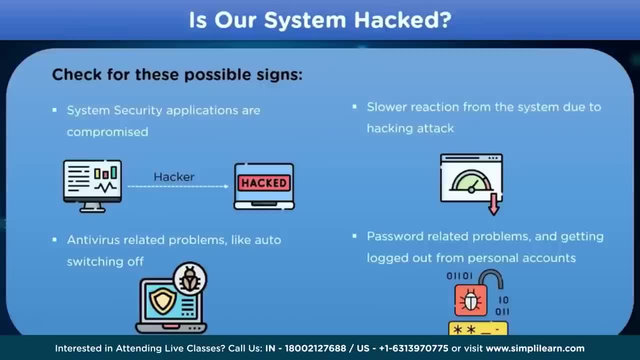 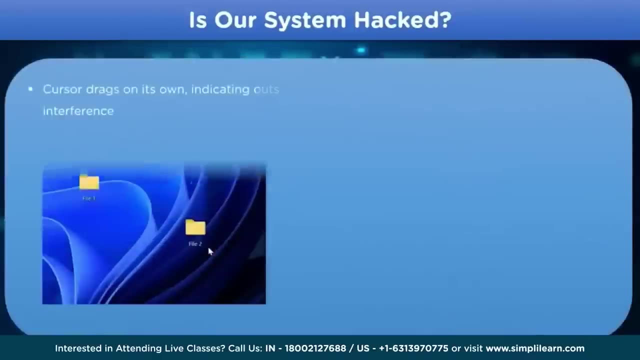 which are no longer working or are changed without a user's intervention, which might indicate that there was some unknown hacking activity that took place in our account. Let's take a look at some more points regarding the topic. There are often cases when the system's cursor move on its own. 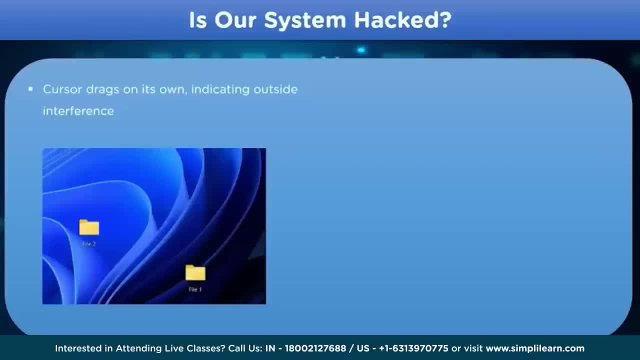 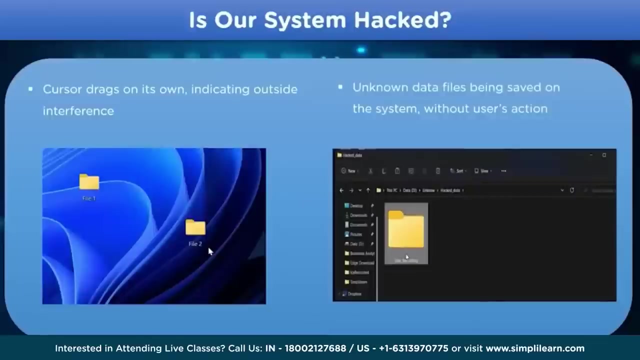 and perform tasks indicating that the system is being used by someone else using an illegal hacking method. There are also cases when we often see files and folders being created in the storage disk on the system which is unknown to us. To better understand the points regarding how to identify, 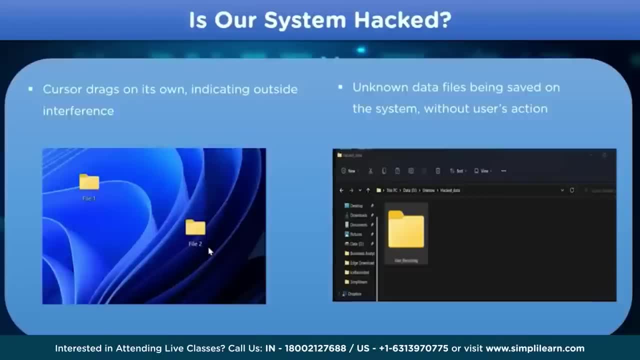 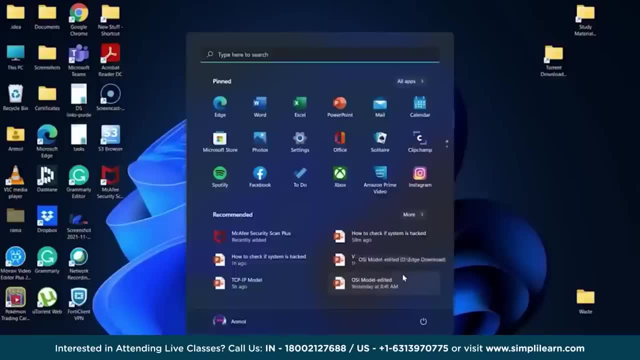 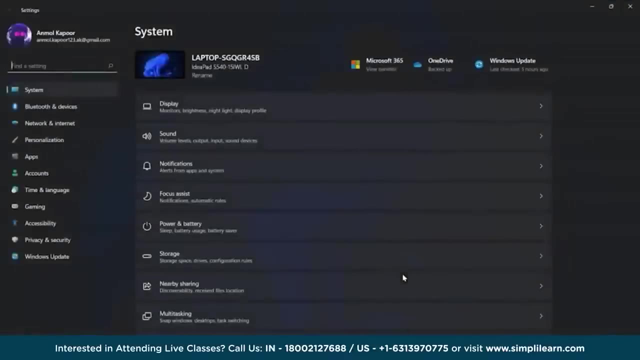 whether our system is hacked or not. let's take a look. Then let's start with the first point. If we want to check whether our system is hacked or not, the first point would be to choose the settings option and using privacy and security and moving on to the Windows security. 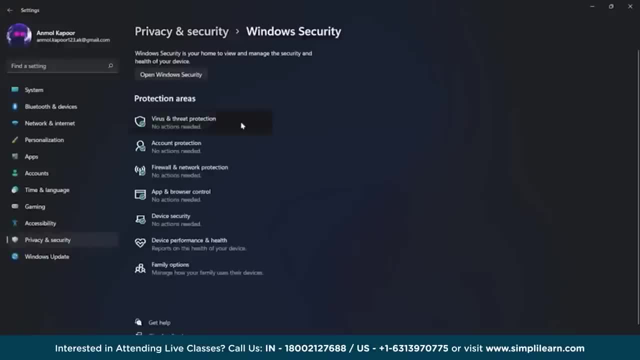 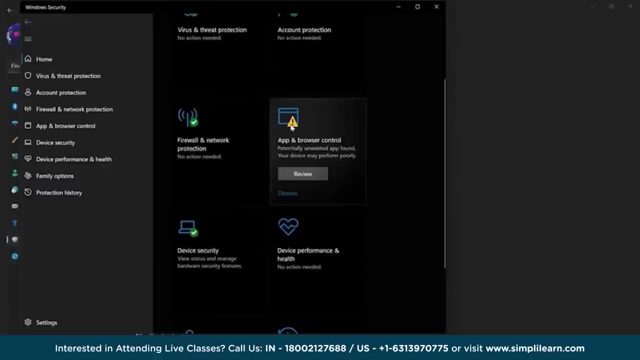 This option that is available on our system allows us to see various protection applications that are available on the system. If we see any problem regarding any one of them, for example, apps and browser control, in my system it says there is a problem with it, which might be due to hacking attempts that was done on my system. 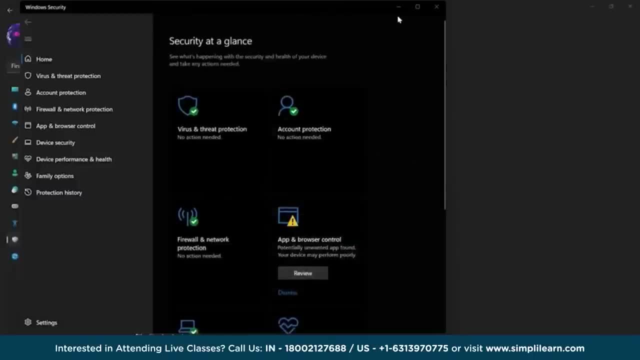 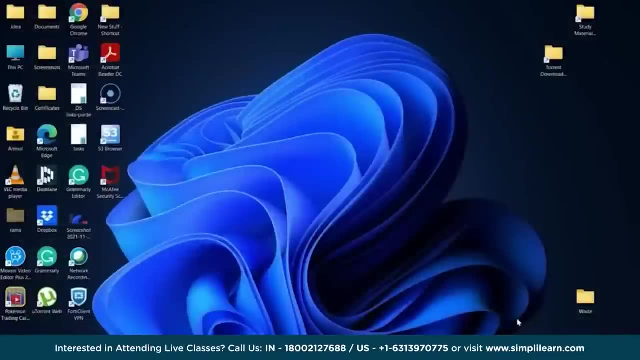 Now let's take a look at the other option: how we can check whether our system is hacked or not. That would be checking the antivirus software that is installed in our system. If you face problems regarding that, this might be the issue. According to my antivirus software, it says my computer is at risk. 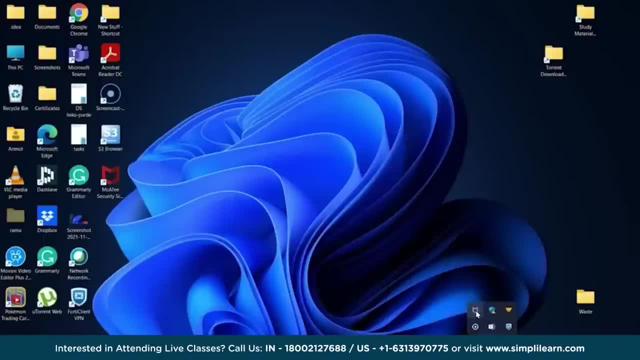 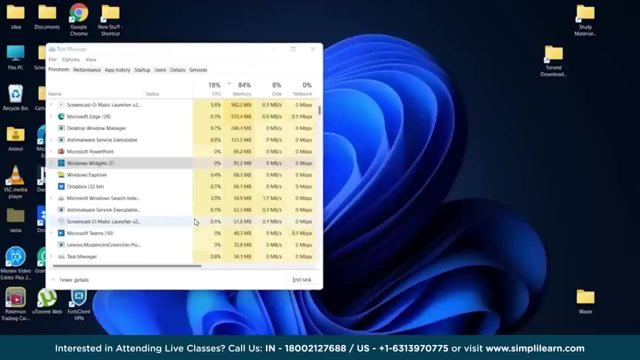 This might be due to the interference from a cybercriminal or a hacker while using different illegal software during its hacking attempt. Then there are also cases where we see there are unknown programs being executed in the background of our system, which we can take a look using the Task Manager software. 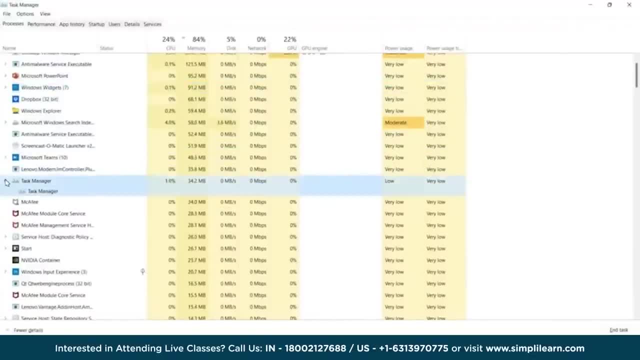 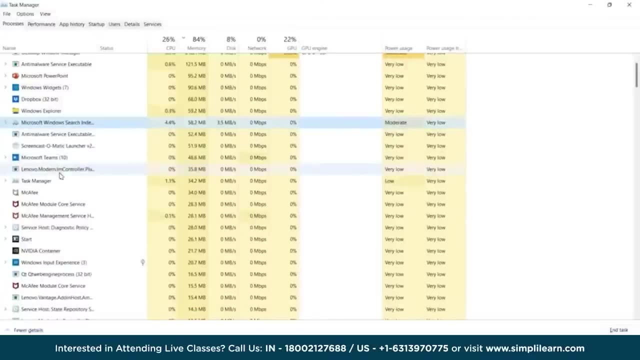 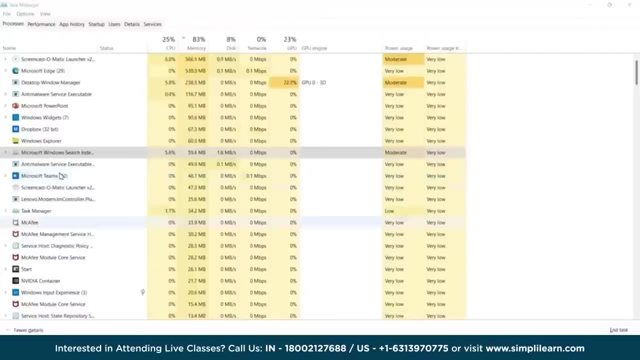 Using the Task Manager, we can take a look at each and every application that is being executed in the system and see the origin. If we find any unknown program or application, we can assume that it might be due to a hacking attempt. Moving on, if we want to check further, 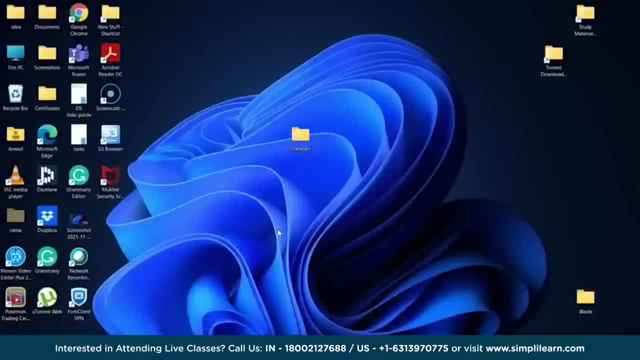 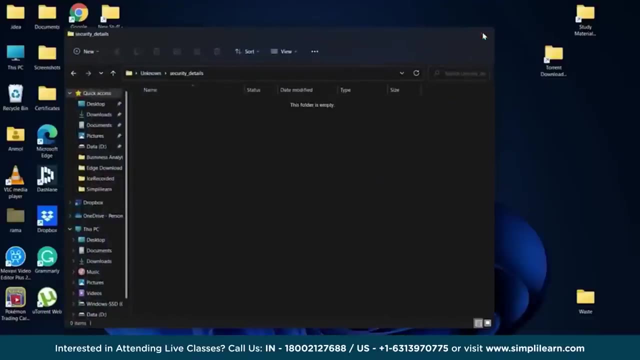 whether our system is hacked or not, we can check for files or folders that are being created unknown to us, For example, this unknown folder which contains some security details that are unknown to me. This might be also due to a hacking attempt by a hacker or a cybercriminal. 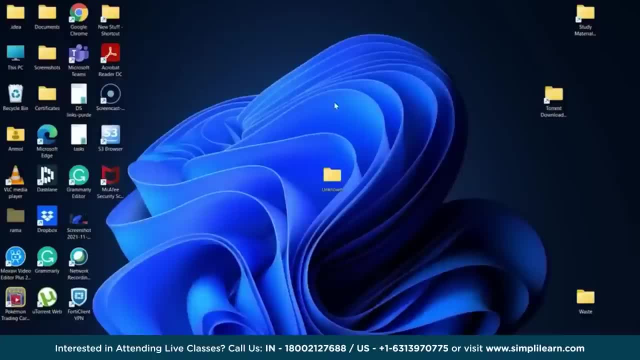 Then there are also cases when the system's cursor move on its own and perform tasks that are not initiated by us and performs copying of different folders or data from one file to other. This is due to a hacking attempt that was done on a system and the hacker has taken control of a system. 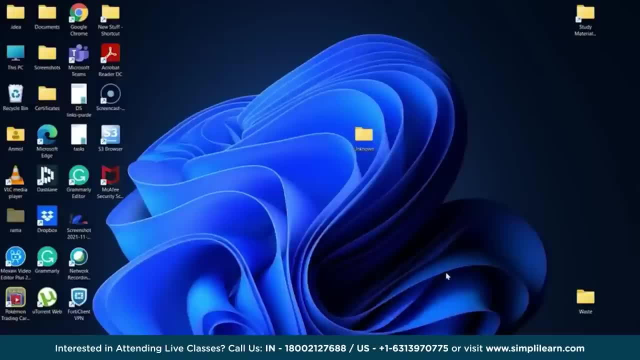 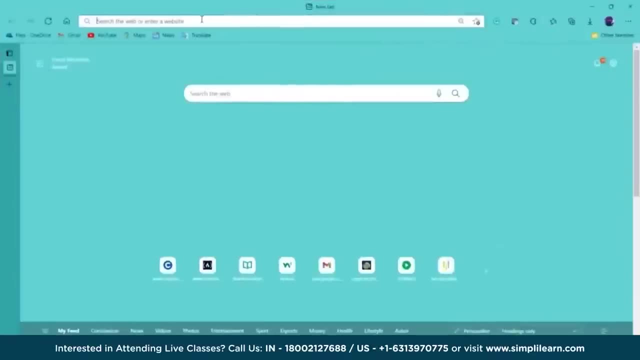 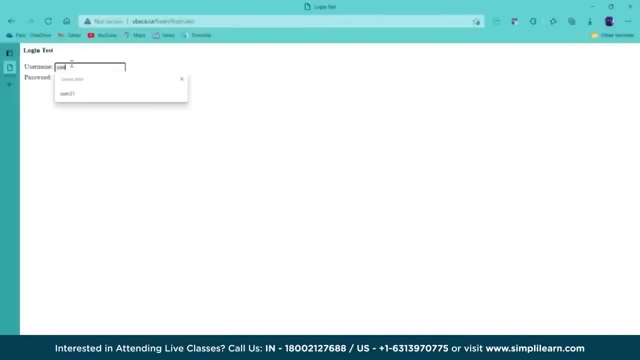 Then there are also cases regarding login issues or password problems. For example, if I want to access into my account and there is a problem with the password, it might be due to the attempt of hacking into my account by a professional hacker. Seems like there is a problem with the username. 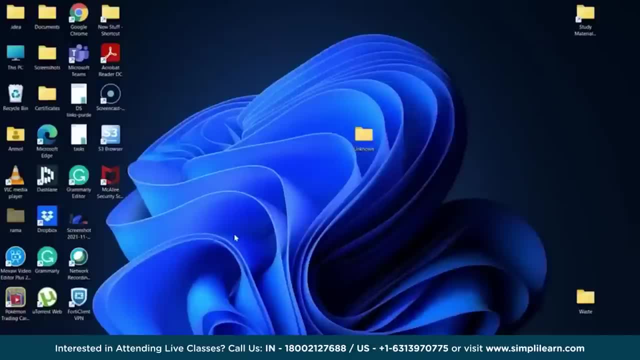 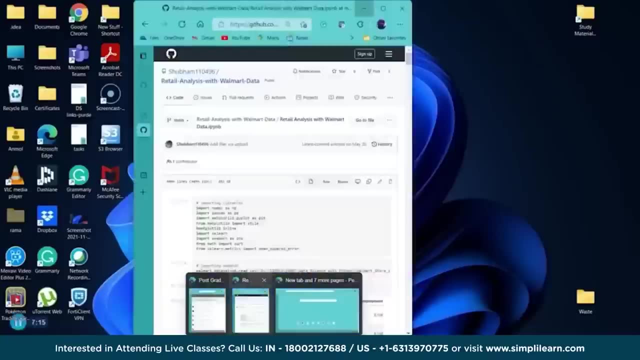 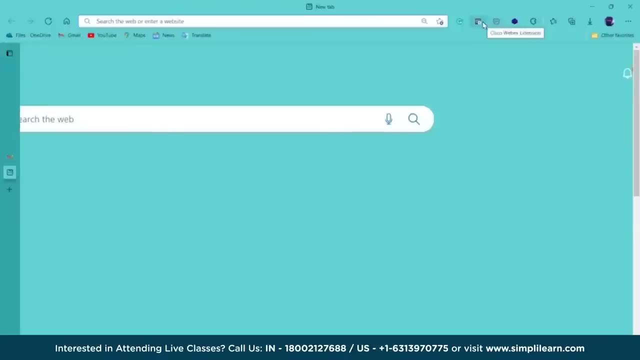 which means there was a hacking attempt by a professional hacker. We can further check hacking attempts by accessing our web browser and checking whether there is some extra add-ons or unknown add-ons that wasn't installed by us. This might also indicate a hacking attempt on the system. 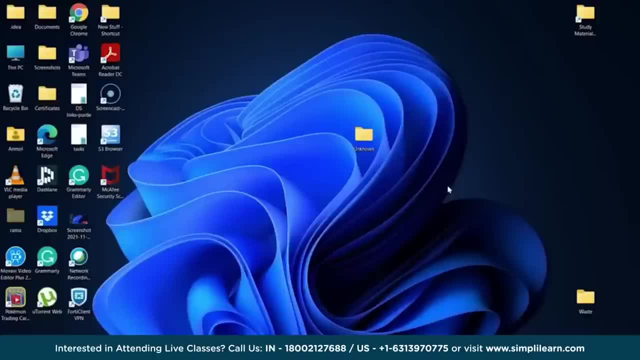 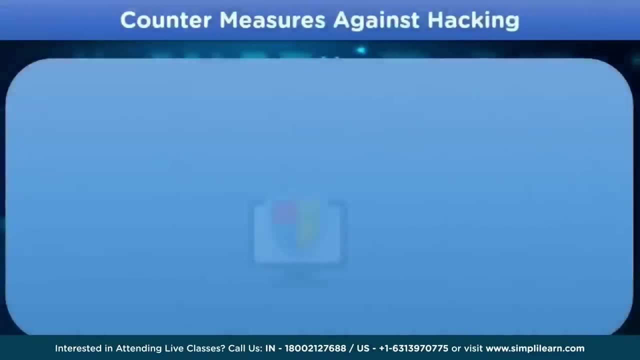 Now that we are clear about how to check whether a system is hacked or not, let's take a look at some of the countermeasures against hacking. Let's begin. The first point regarding how to avoid hacking is: do regular manual security checks and keep the system security updated. 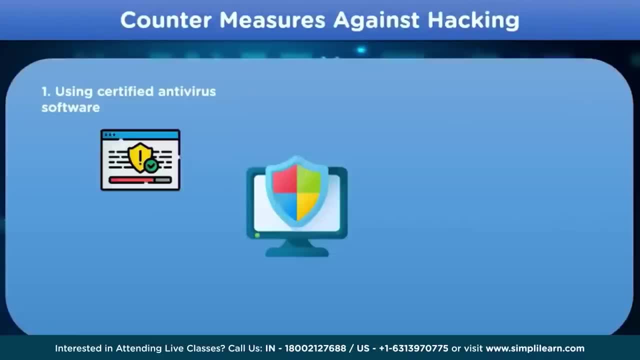 Using certified antivirus software is a basic countermeasure against hacking attempts And, if possible, visit only secure websites for surfing on the internet, or use VPN or other internet security applications to mask your system's network to avoid any hacking attempts for the device. Then we have 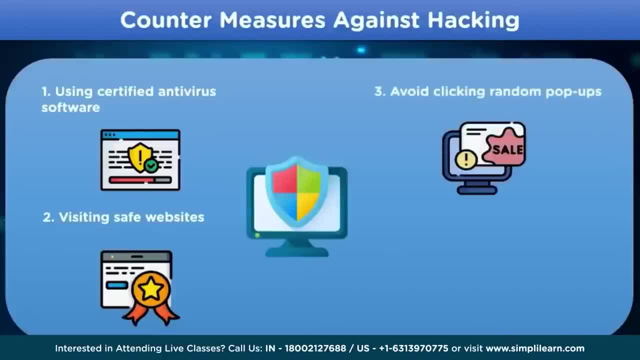 avoid clicking on random web pop-ups and ads to avoid hackers from getting into a system and accessing a device data. And, lastly, use strong passwords or complex passwords for your login details. Applying these countermeasures, we can avoid hacking to a certain extent. 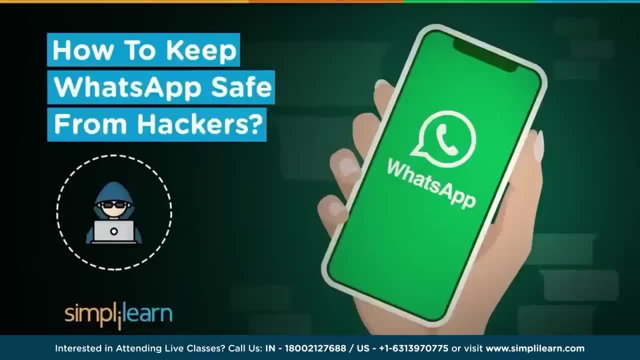 The concept of instant messaging crossed into the mainstream in the 1990s, allowing friends, acquaintances, colleagues and like-minded thinkers from all over the world to connect in real time. Since then, instant messaging has revolutionized how we communicate and today over a billion people are signed up. 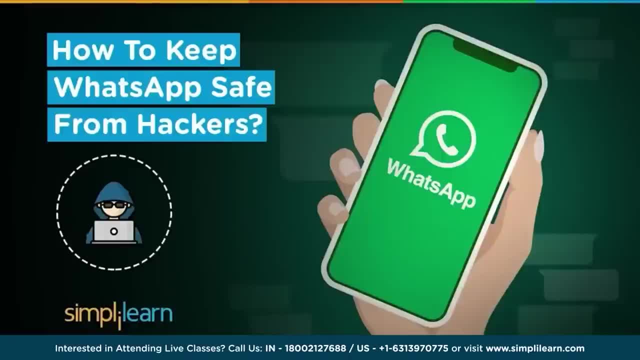 for at least one messaging app. The present instant messaging experience is seamless and it intuitively integrates features like video, photos, voice, e-commerce and gaming with plain old messaging. Among these apps, WhatsApp has comfortably found its place among the most popular messaging platforms. 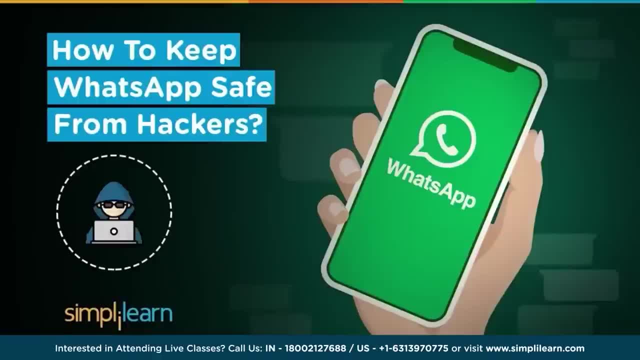 Like everyone associated with the internet, a matter of security is never far away. Considering the huge user base of this messaging app, hackers are always on the lookout for compromised accounts to grab. Today, we are going to cover some of the ways we can protect our WhatsApp account. 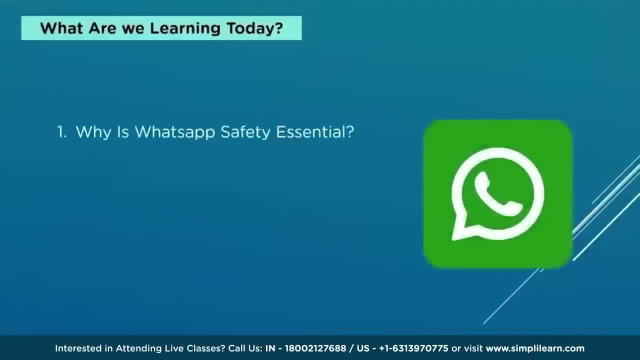 from falling into malicious hands. We start by learning about the importance of security when it comes to WhatsApp and instant messaging apps in general. Next, we cover some of the most important steps that should be followed in order to protect our WhatsApp accounts from hackers. Finally, we learn what we should do. 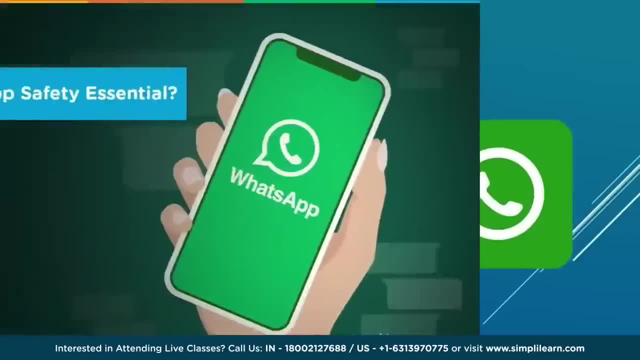 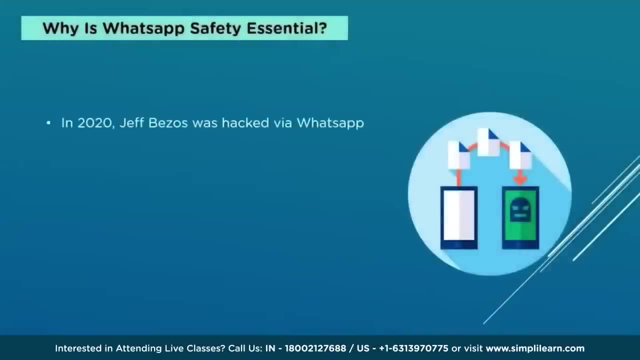 when a WhatsApp account gets compromised. Let's start by learning why we need to focus on the safety of WhatsApp. In the year of 2020. the big news was about Amazon CEO Jeff Bezos and his phone being hacked by Saudi Arabia. A report coming from the Guardian suggested. 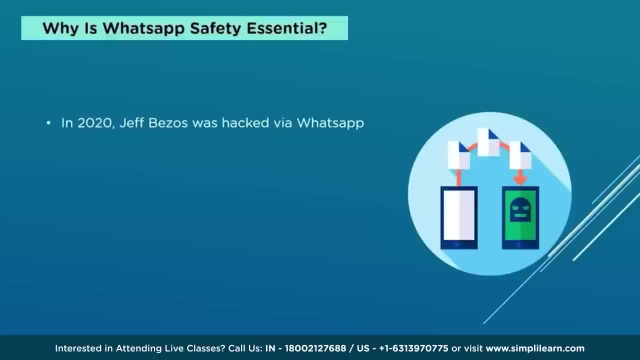 that Bezos' phone was hacked via a video file sent on WhatsApp. The report said that Bezos' mobile phone was hacked by a Saudi Arabian prince in the year 2018 and gigabytes worth of data was stolen from the device. While there are some issues being resolved, 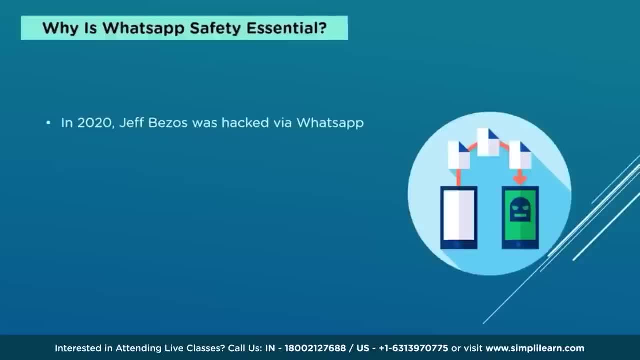 and raised about the report, which states with the medium to high confidence that Jeff Bezos' phone was hacked. it does raise a security fear for regular users. After all, if the phone of one of the world's most powerful men can be hacked, the same can happen to any one of us as well. 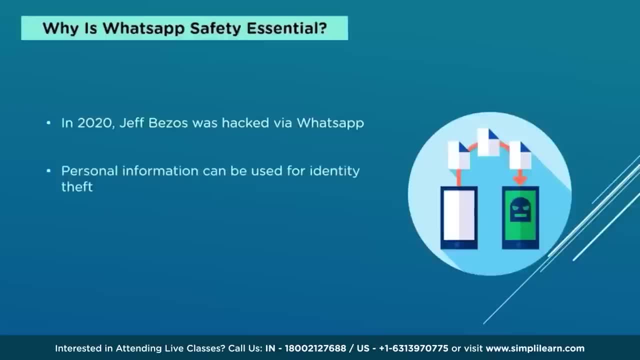 When it comes to regular users, we exchange messages with our loved ones regarding a paradigm of topics. The information which may seem trivial initially can later function as ammunition for a campaign regarding identity theft. Basic information like preferred data banks, occasional dining places, can go a long way in social engineering attacks. 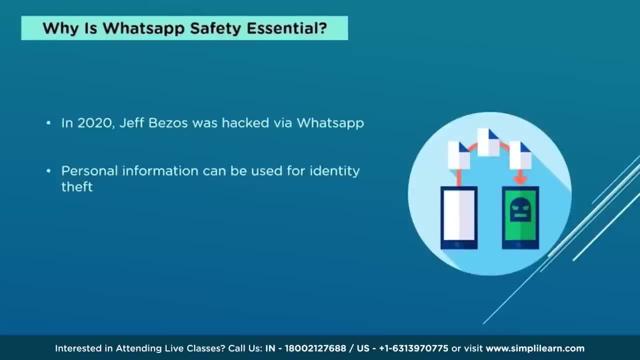 further increasing the need for secure messaging habits. WhatsApp uses end-to-end encryption to protect all communication on its platform. These encryption keys not only make it impossible to decrypt messages, but they also prevent third parties and even WhatsApp from accessing messages or calls, But not entirely. 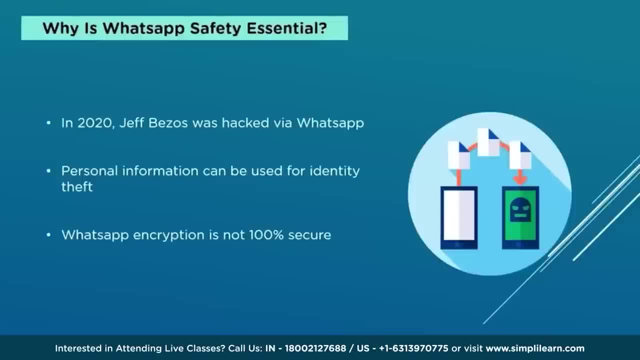 Although end-to-end encryption makes WhatsApp more secure than other communication apps, no app is 100% secure and safe to use. Like any application or digital device, WhatsApp is often targeted by bad actors. It also has access to your contacts and tracks where and how long you use it. 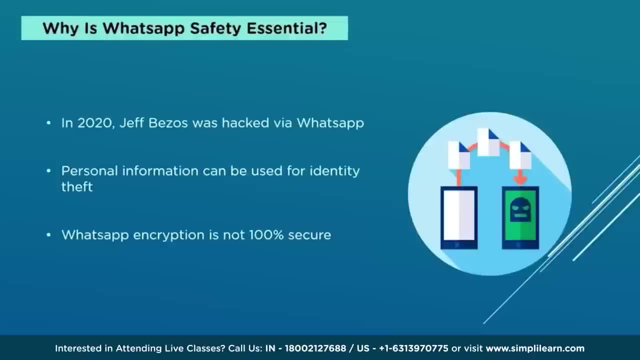 putting your privacy and personal information at risk. We all have access to our cell phones, so it's no surprise that SMS two-factor authentication is one of the most widespread types of MFA available. You don't need any apps or digital keys and it's not tied to a specific ecosystem. 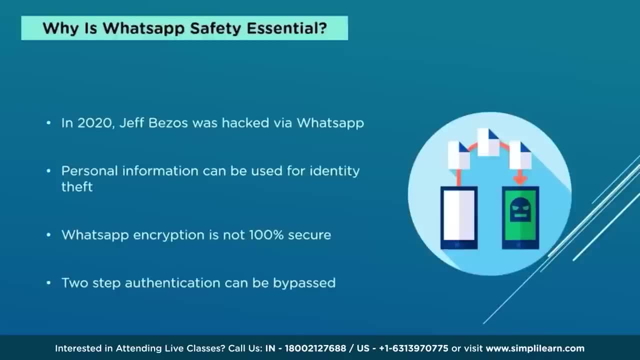 Unfortunately, it's also not a secure multi-factor authentication method. The nature of SMS itself opens up your organization to a host of risks. Hackers may have many ways to leverage SMS to find a way into your accounts and network, Be it via spoofed SIM cards or message hijacking. 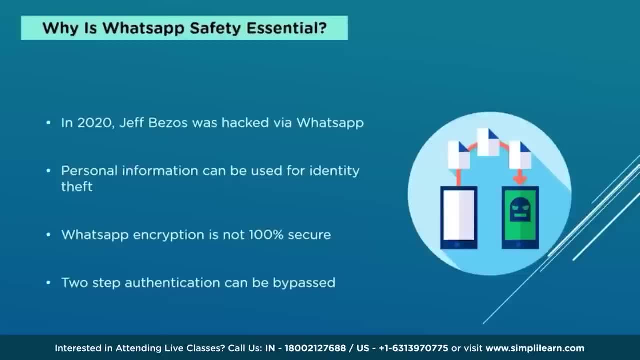 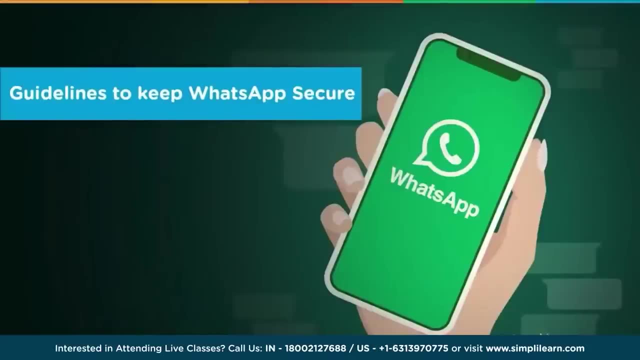 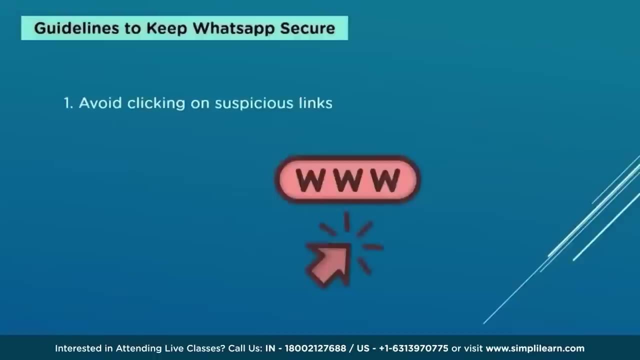 WhatsApp 2FA using SMS isn't a foolproof solution. Now that we understand the variety of reasons why WhatsApp needs extra security, let's go through some of the ways we can achieve this. It is more than probable that one fine day, you might receive a WhatsApp message. 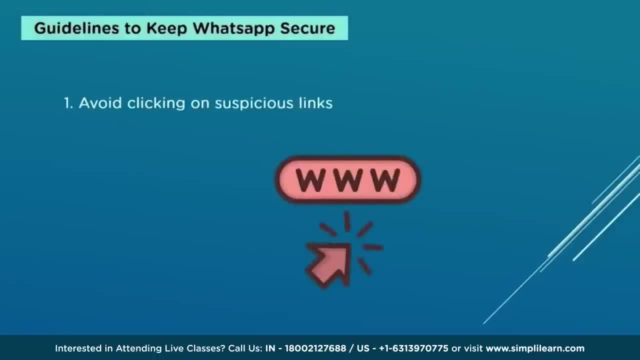 or even an SMS that reads that your order is delayed, please check its data here. or your account is locked and please unlock it here. or even some tempting messages like win free 3G and movie tickets here. Some of them may sound intimidating and some of them may be lucrative. 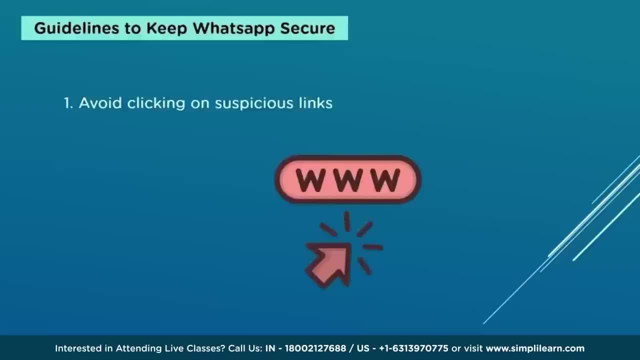 but they all have one purpose: to trick you into clicking that link, and once you do that, it's already over. It will install malware on your phone and you won't have a clue about it Only when you start noticing that your phone bills are abnormally high. 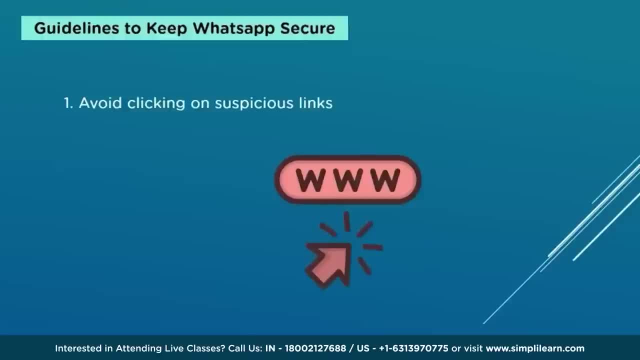 or your bank account has been used without your permission. the realization will dawn upon you that something is wrong with your phone, But by then it may be too late. WhatsApp in itself provides various privacy options to users. The messaging platform provides users with option to choose who they want to share. 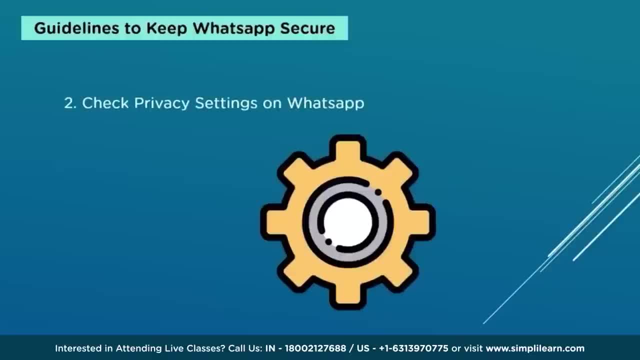 their profile, photo status and other details with. It's a good idea to change the settings to contacts only. This means only phone numbers that are saved on your smartphone will be able to see your profile, photo status, phone number and auto-delete status as well. 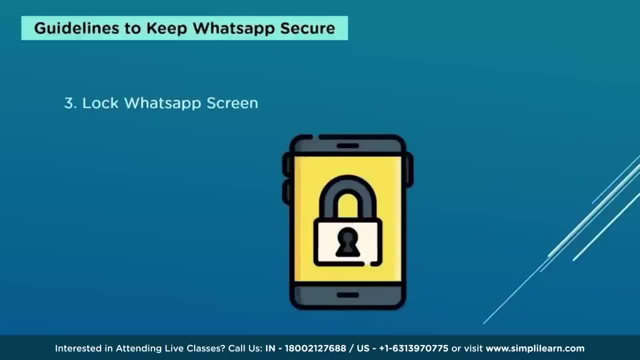 Make sure you enable the option to lock the screen every time WhatsApp is closed. This will ensure no one else but you can open your WhatsApp account. Just head to the settings menu, privacy, and select the screen lock option. You will then need to register your phone. 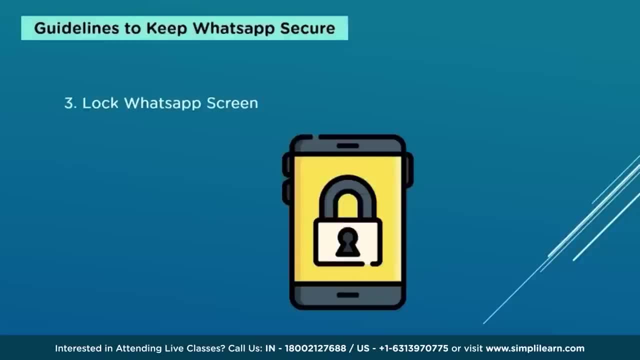 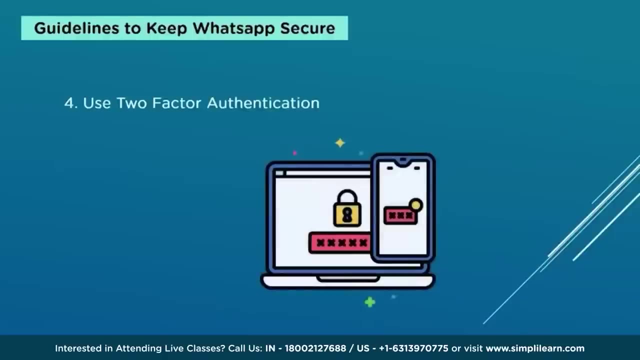 with your fingerprint. After the process is completed, you will have to scan your fingerprint every time you open the WhatsApp app. This adds an extra layer of security. The two-step verification works as an extra layer of security and helps WhatsApp users to protect their OTPs and documents. 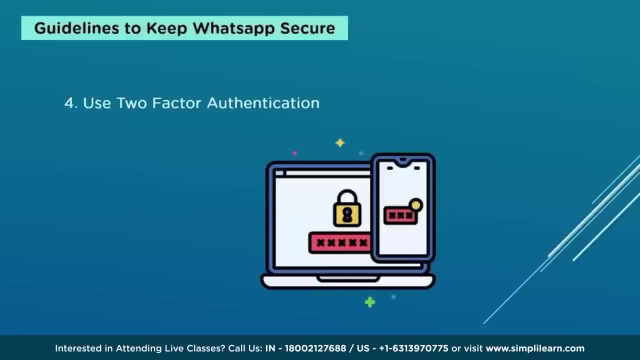 shared through WhatsApp. It's very easy to set up a PIN to activate a two-step verification. Users have to enter it periodically. once it is activated, WhatsApp will sometimes keep asking users to enter their six-digit passcode. Users cannot disable this without disabling. 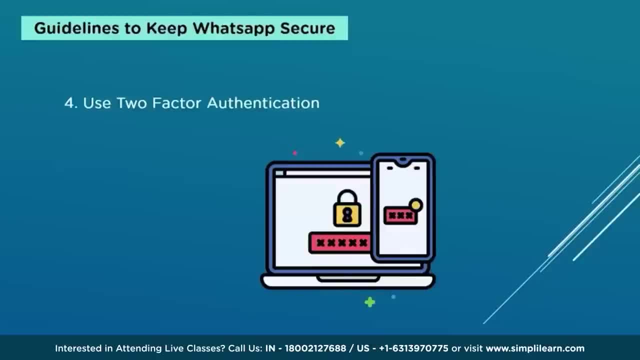 the two-step verification feature altogether. In case users do not provide WhatsApp with an email ID and want to disable two-step verification, then the number will be permitted to re-verify on WhatsApp without the passcode. after seven days, However, the users will lose all pending. 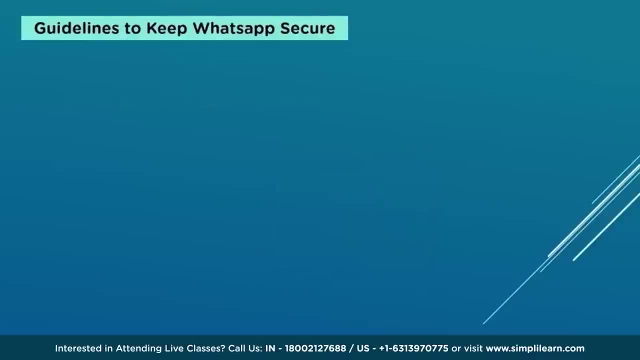 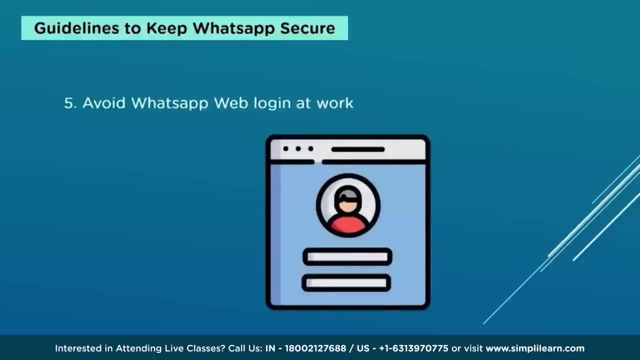 messages upon re-verifying. We often have the tendency to log into WhatsApp web at the office and then leave the account open on the desktop. This habit can actually create problems for you. Someone else sitting on the same PC can access all your chats without you even. 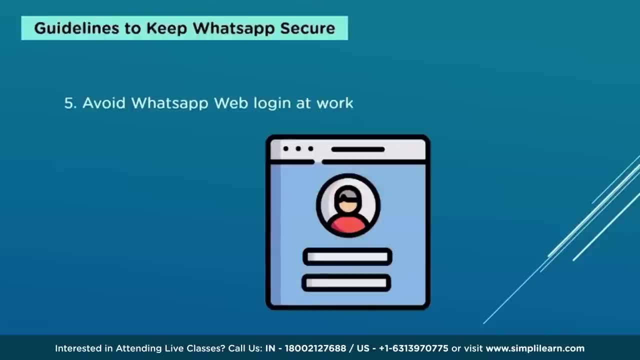 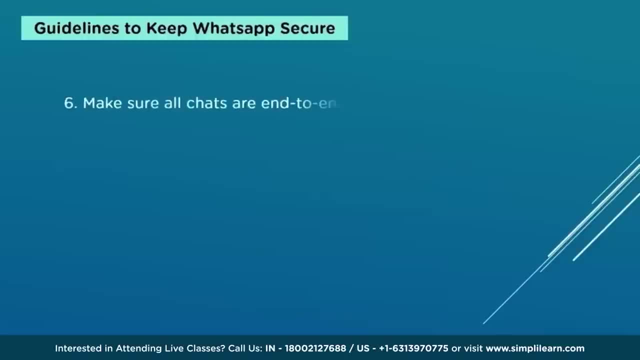 realizing it. It's a good practice to log out from WhatsApp web before leaving the office. It just takes a few seconds to log in again by just scanning the code and you're done. All WhatsApp users should ensure that the chats are end-to-end encrypted. 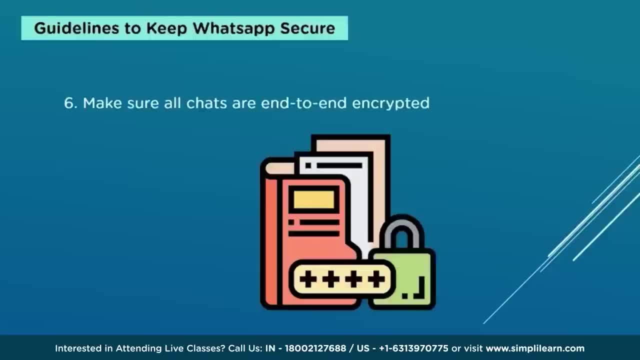 To verify that a chat is end-to-end encrypted: open the chat. tap on the name of the contact to open the contact info screen and then tap encryption to view the QR code and a 60-digit number. WhatsApp end-to-end encryption ensures that only you and your contact can read. 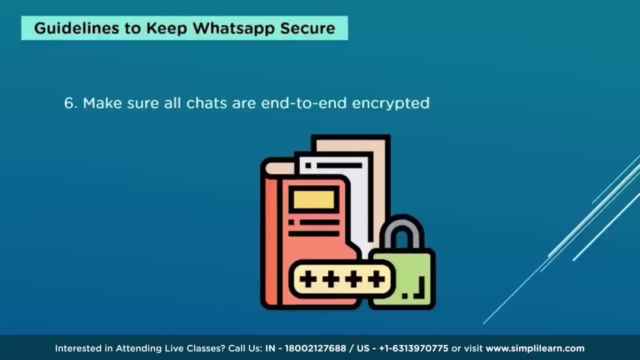 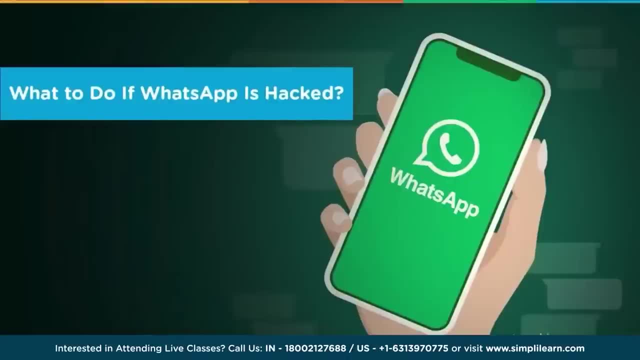 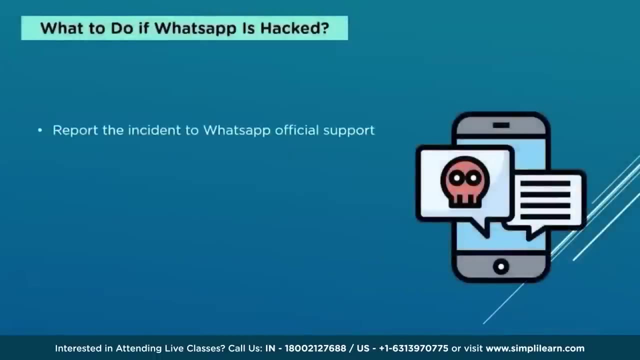 the messages that are being exchanged and nobody in between, not even WhatsApp. With the necessary guidelines out of the way, let us go through the recommended course of action. should our WhatsApp accounts be compromised, The first and most important thing that you need to do is report the issue to. 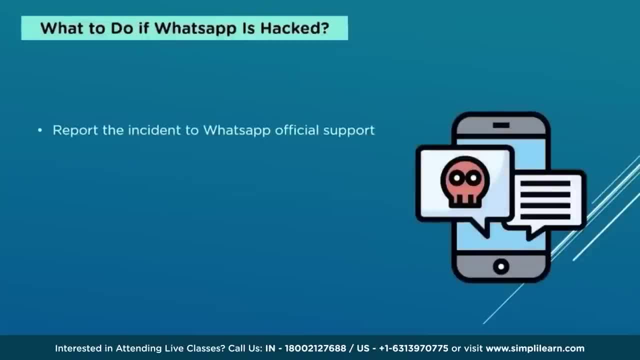 the WhatsApp support team for assistance. Make sure that you reach out to the support team through its help desk and report the hacking attempt. WhatsApp help center will take the shortest time to resolve your issue via email or within the app itself. This will help you. 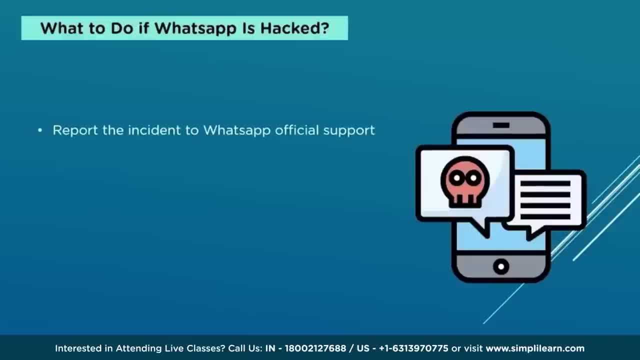 to take prompt legal action against the hackers. If you can't access your email, call the support team. In some cases, the support will deactivate your WhatsApp account and request you to reactivate it within 30 days if you don't want it to be. 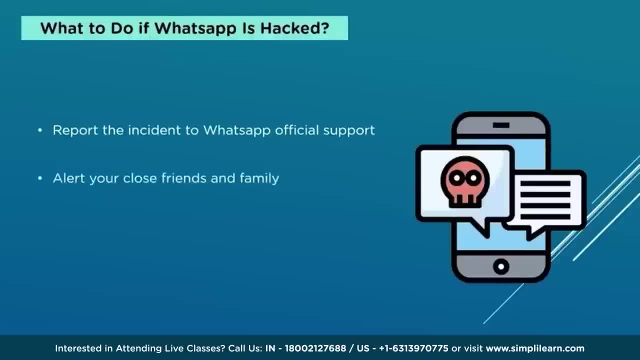 deleted completely. When someone compromises your WhatsApp account, they can now send messages to your contact stating that the company sent your verification code and gain access to their account. That's why one of the first things you'll want to do is send a message to your friends and family, letting them 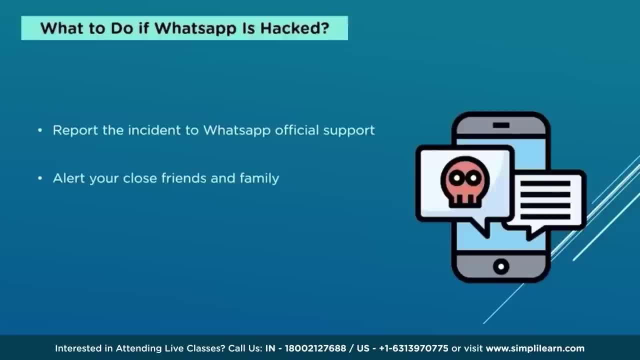 know that you've lost access to your account. This action prevents further exploitation of your account and others. Another reason you'll want to let your contacts know you have no access to your WhatsApp account is that they may phish for personal information From your. 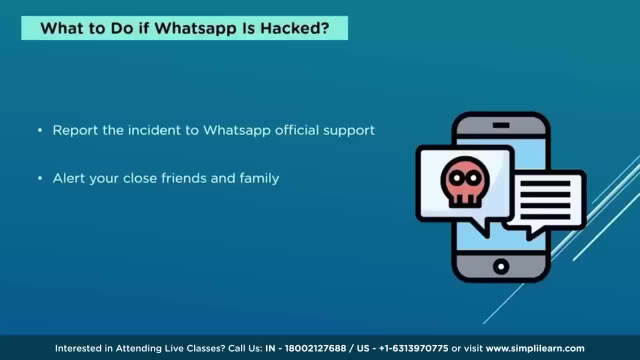 banking number to your email address. hackers will cleverly attempt to gain as much access to your personal information as possible. WhatsApp Web is an extension of WhatsApp Messenger over the web that facilitates easy synchronization of our smartphone and personal computer. This is the biggest security threat that hackers 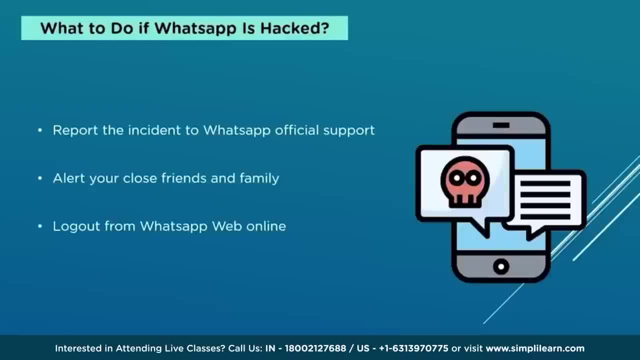 can easily exploit to get into your personal data over WhatsApp. Therefore, it is highly recommended that you use this WhatsApp feature carefully. Once you notice that your WhatsApp Messenger has been hacked, go to your WhatsApp Web and tap or click on the Logout from All. 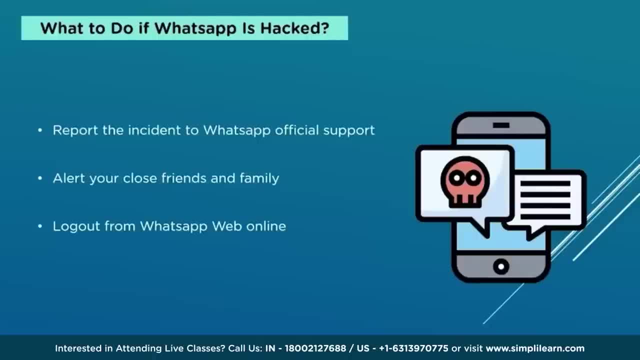 Computers option. This will allow you to activate all the web extensions of your account. Under the unfortunate circumstances where the account recovery doesn't seem likely, you can always ask WhatsApp's support to delete your account permanently. While far from the ideal solution, it can. 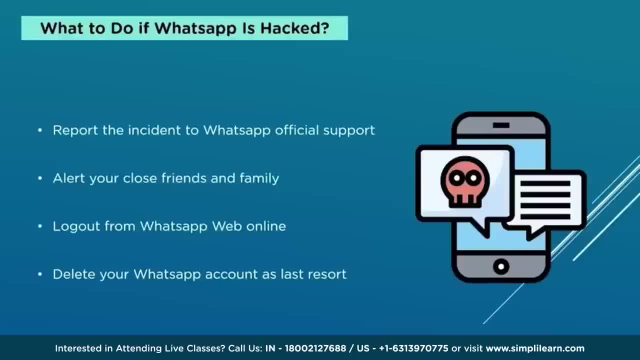 act as a fail-safe option. if you want to protect your personal data at any cost possible, You can always open a new account later, with the security issues mitigated. It's no secret that the majority of our internet usage is at the risk of being hacked, and that's why. 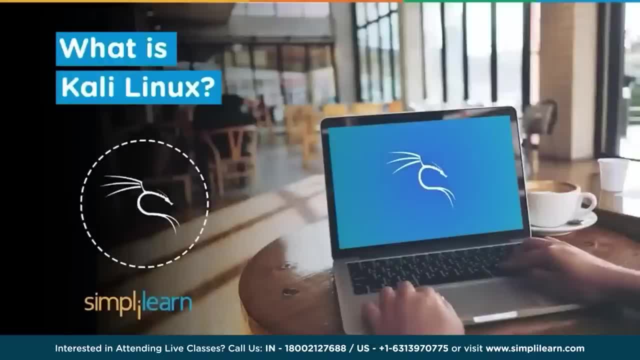 it's important to keep an eye out for this feature, be it via unsafe messaging applications or misconfigured operating systems. To counteract this void of digital security, penetration testing has become the norm when it comes to vulnerability assessment. Kali Linux is an operating system that has become a 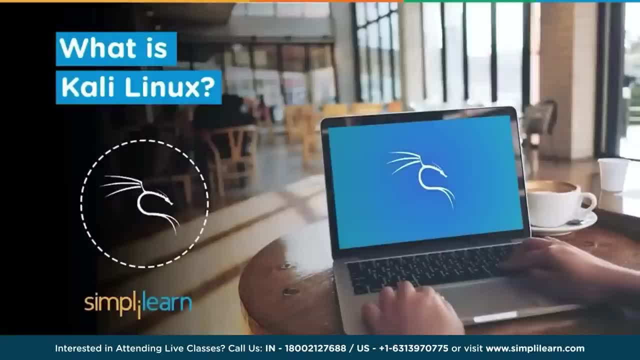 well-known weapon in this fight against hackers, A Linux distribution that is made specifically for penetration testers. Kali Linux has layers of features that we will be covering in today's lesson. Let's take a look at the topics to be covered in this video. 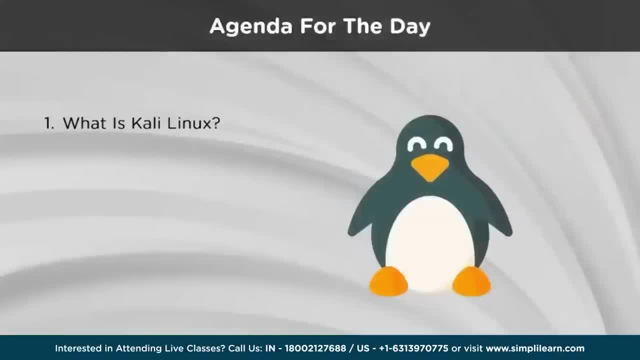 We start by learning about Kali Linux and a basic explanation of its purpose. We take a look at the history of Kali Linux, from the story of its origin to its current-day exploits. Next we learn a few distinct features of Kali that. 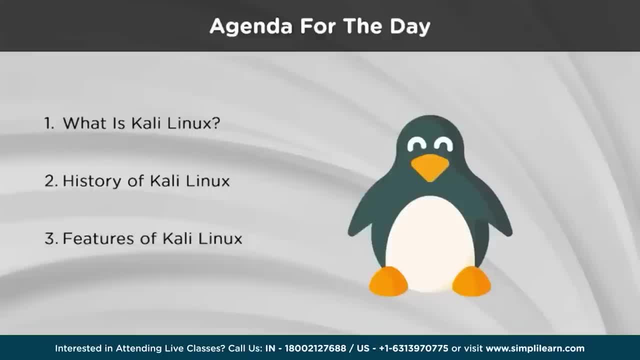 make it an attractive choice for penetration testers worldwide. Finally, we take a look at the multiple ways we can install Kali Linux to start our journey in the world of penetration testing. Let's start by learning about Kali Linux in general. Let's start by learning about Kali. 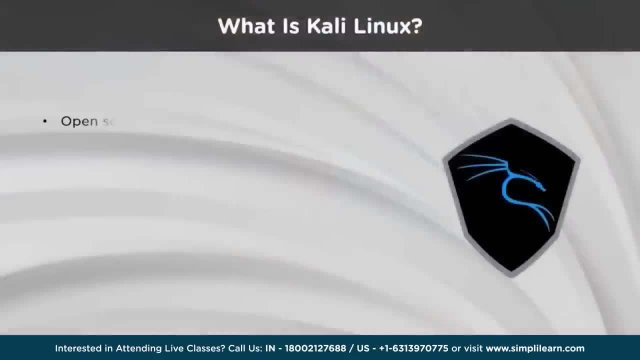 Linux in general. Let's start by learning about Kali Linux in general. Kali Linux, which is formerly known as Backtrack Linux, is an open-source Linux distribution aimed at advanced penetration testing and security auditing. It contains several hundred tools that are targeted towards various information. 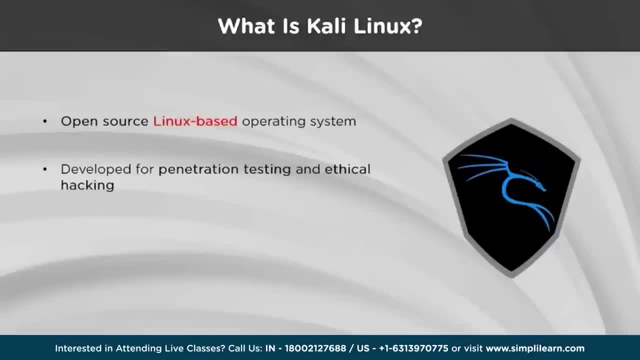 security tasks such as penetration, testing, security research, computer forensics and reverse engineering. Kali Linux is a multiple platform solution accessible and freely available to information security professionals and users worldwide. and users worldwide Among all the Linux distributions. 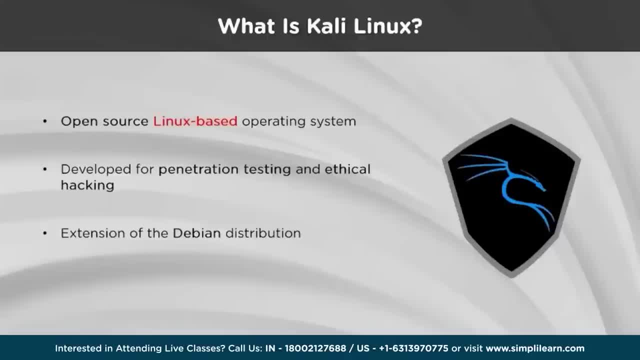 Kali Linux takes its roots from the Debian operating system. Debian has been a highly dependable and stable distribution for many years, providing a similarly strong foundation to the Kali desktop, While the operating system is capable of practically modifying every single part of our installation. 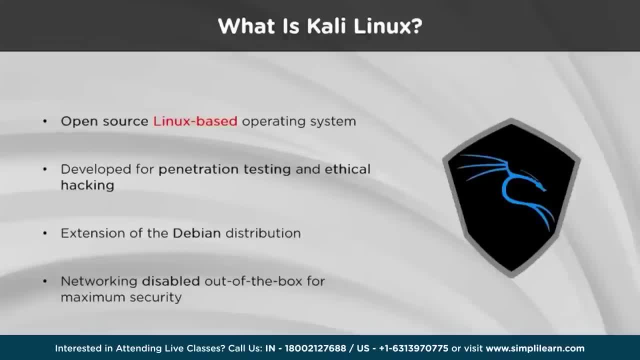 the networking components of Kali become disabled by default. This is done to prevent any external factors from affecting the installation procedure which may pose a risk in critical environments. Apart from boosting security, it allows a deeper element of control to the most enthusiastic of users. 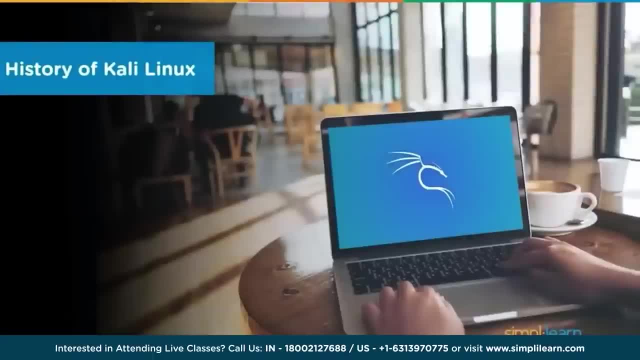 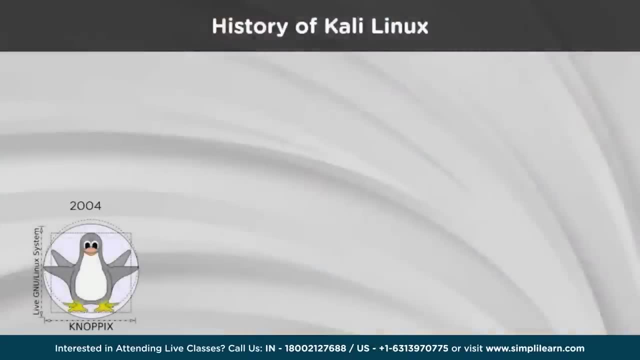 We did not get Kali Linux since the first day. How did it come into existence? Let's take a look at some of its history. Kali Linux is based on years of knowledge and experience in building, penetration, testing and operating systems During all these project lifelines. 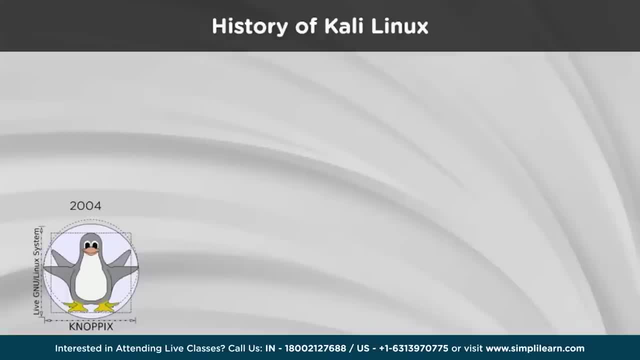 there have been only a few different developers, as the team has always been small. The first project was called Wopix, which stands for White Hat Nopix. As can be inferred from the name, it was based on the Nopix operating. 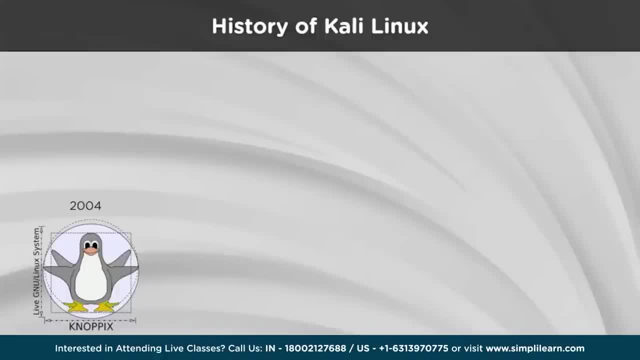 system. as its underlying OS, Wopix had releases ranging from version 2.0 to 2.7.. This made way for the next project, which was known as Wax or the long hand. being White Hat Slacks, The name change. 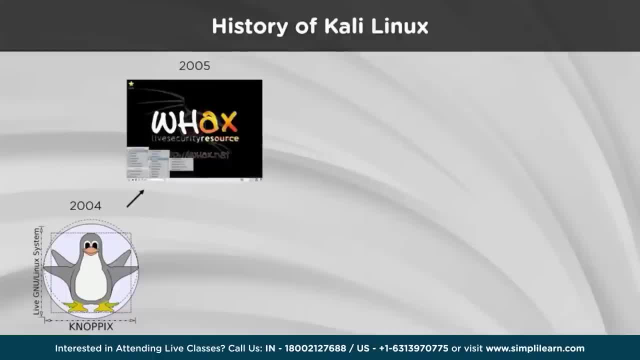 was because the base OS was changed from Nopix to Slacks Wax started at version 3 as a nod it carrying on from Wopix, There was a similar OS being produced at the same time, Auditor Security Collection, often being shorted. 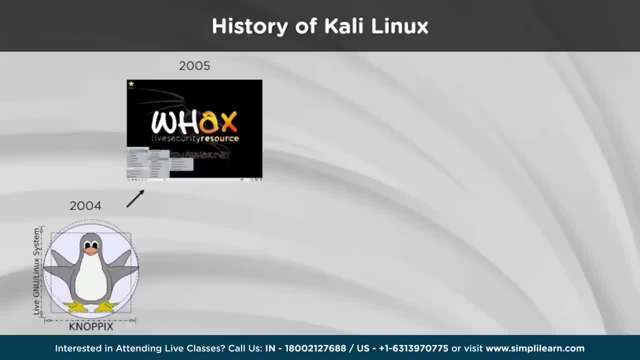 to just Auditor, which was once again using Nopix. Its efforts were combined with Wax to produce Backtrack. Backtrack was based on Slackware from version 1 to version 3, but switched to Ubuntu later on with version 4 to version 5.. 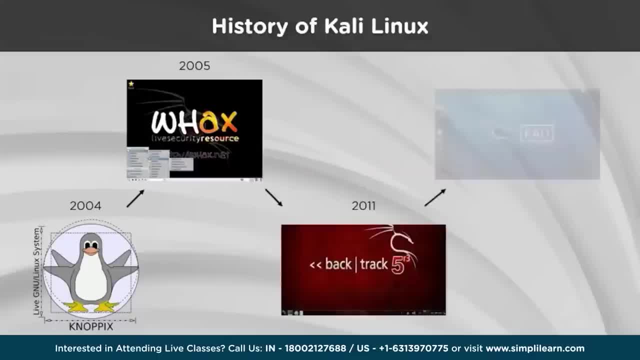 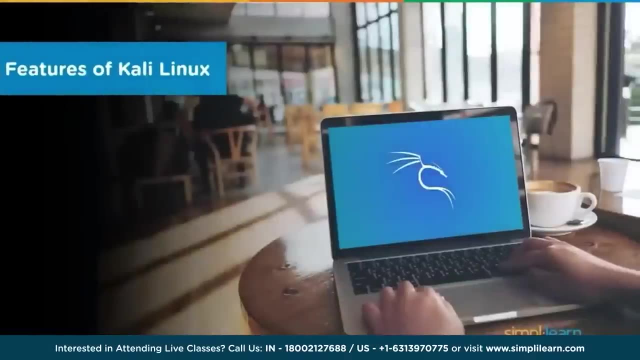 Using the experience gained from all of this, Kali Linux came after Backtrack in 2013.. Kali started off using Debian stable as the engine under the hood, before moving to Debian testing when Kali Linux became a rolling operating system. Now that we understand. 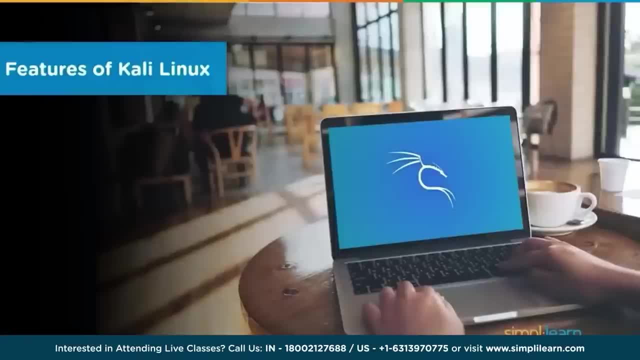 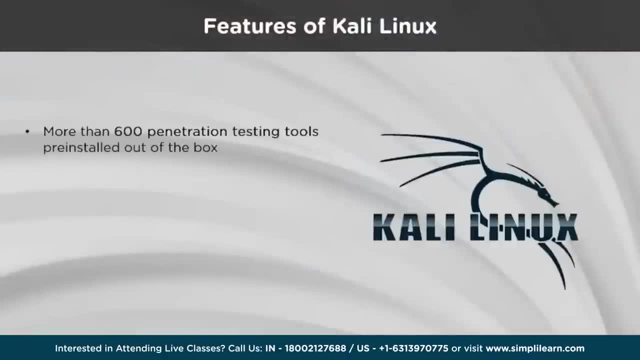 the history and the purpose of Kali Linux. let us learn a little more about its distinct features. The latest version of Kali comes with more than 600 penetration tools pre-installed. After reviewing every tool that was included in Backtrack, developers have eliminated 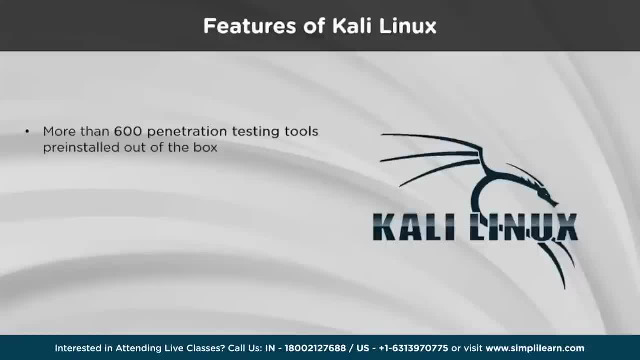 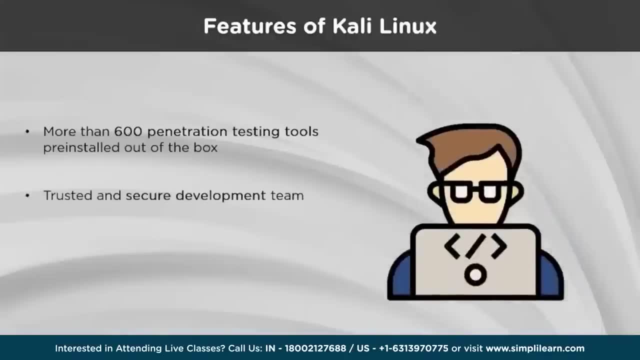 a great number of tools that either simply did not work or which duplicated other tools that provided the same or similar functionality. The Kali Linux team is made up of a small group of individuals who are the only ones trusted to commit packages and interact with the repositories. 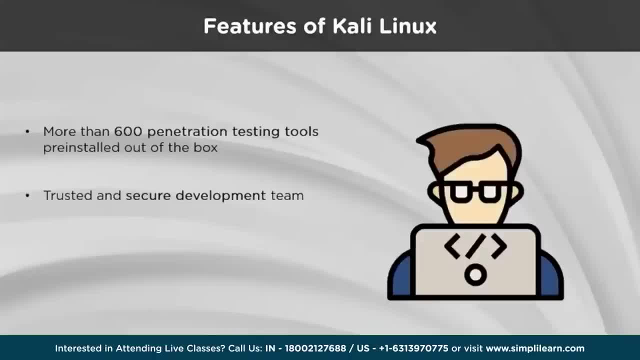 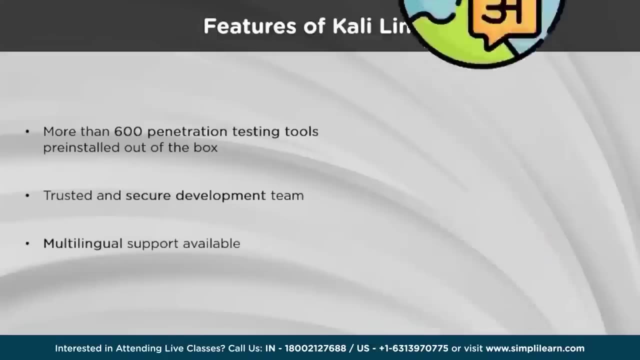 all of which is done using multiple secure protocols. Restricting access of critical code bases to external assets greatly reduces the risk of source contamination, which can cause Kali Linux users worldwide a great deal of damage as a direct victim of cybercrime. Although penetration tools tend 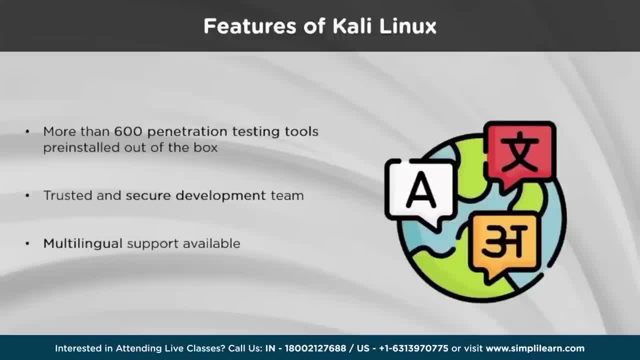 to be written in English. the developers have ensured that Kali includes true multilingual support, allowing more users to operate in their native language and locate the tools they need for the job. The more comfortable a user feels with the intricacies of their operating system, the easier it is to. 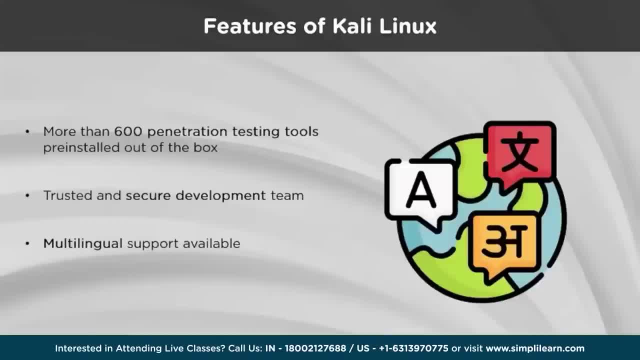 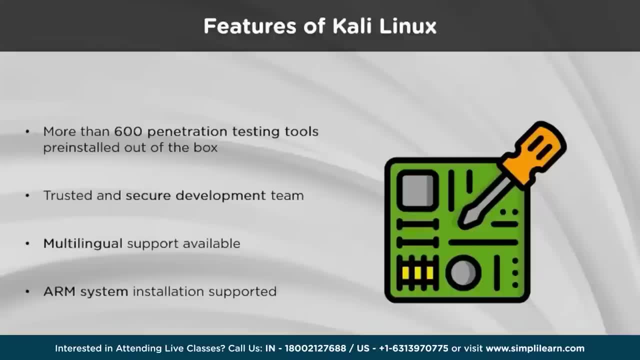 maintain a stronghold over the configuration and the device in general. Since ARM-based single board systems like the Raspberry Pi are becoming more and more prevalent and inexpensive, the development team knew that Kali's ARM support would need to be as robust as they could manage with. 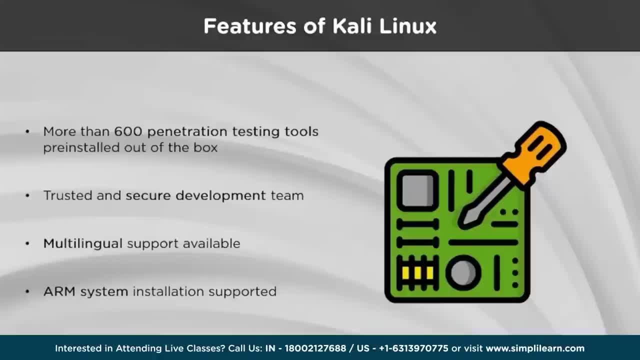 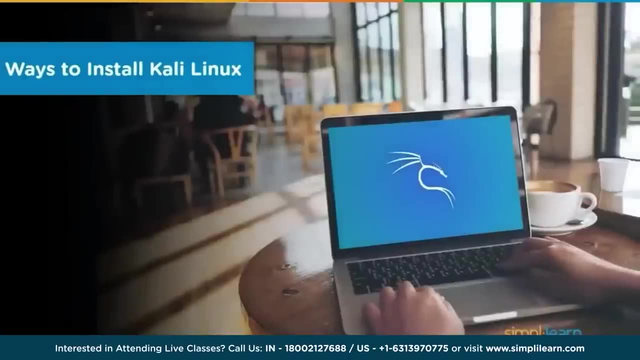 fully working installations. Kali Linux is available on a wide range of ARM devices and has ARM repositories integrated with the mainline distributions, so the tools for ARM are updated in conjunction with the rest of the distribution. All this information is necessary for users to determine if the 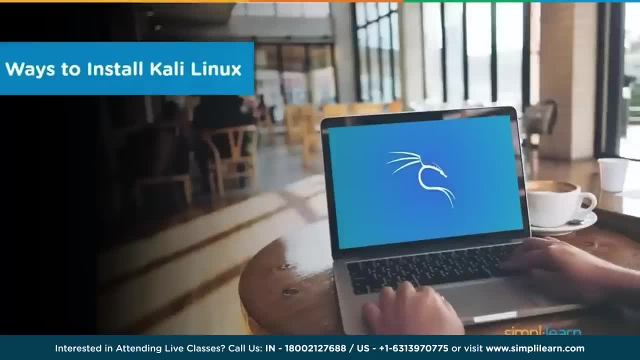 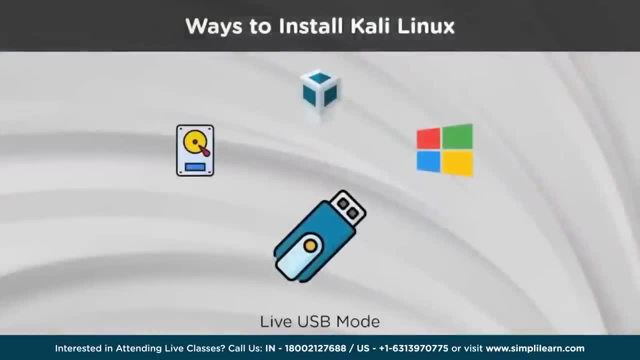 use of Kali Linux is the correct choice for them? If it is, what are the ways that they can go forward with this installation and start their penetration testing journey? The first way to use Kali Linux is by launching the distribution in a live USB mode. 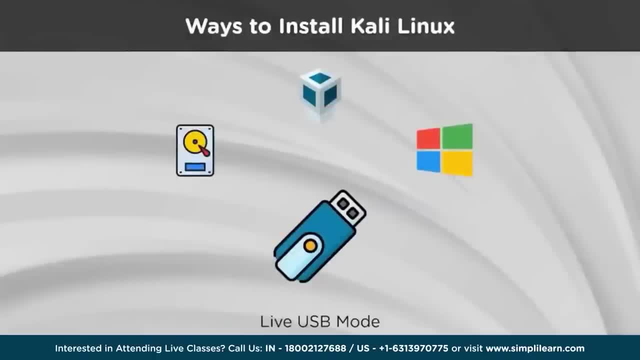 This can be achieved by downloading the installer image file or the ISO file from the Kali Linux website and flashing it to a USB drive with a capacity of at least 8GB. Some people don't need to save their data permanently, and a live USB is the perfect solution. 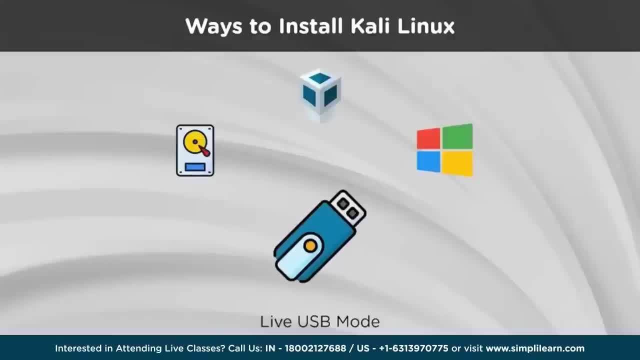 for such cases, After the ISO image is flashed, the thumb drive can be used to boot a fully working installation of the operating system, with the caveat that any changes made to the OS in this mode are not returned permanently. Some cases allow persistent usage in live USBs. 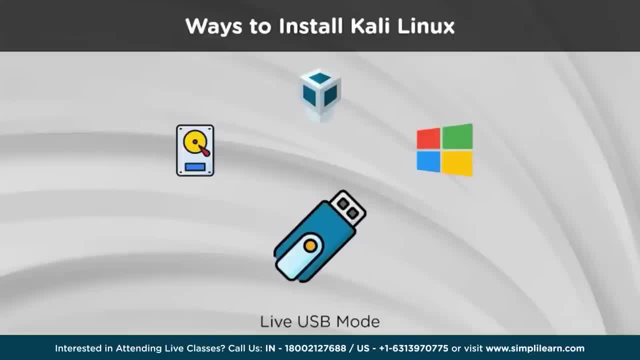 but those require further configuration than normal situations. But what if the user wants to store data permanently in the installed OS? The best and the most reliable way to ensure this is a full-fledged hard disk installation. This will ensure the complete usage of the system's hardware capabilities. 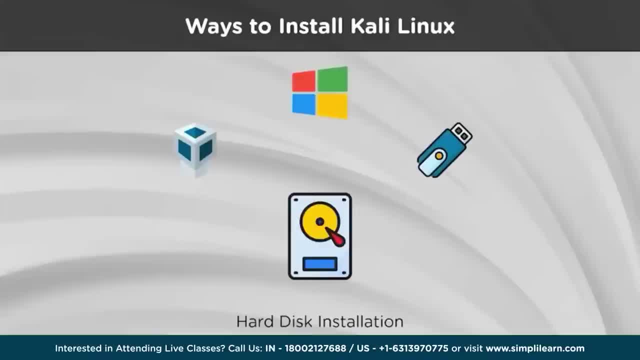 and will take into account the updates and the configurations being made to the OS. This method is supposed to override any pre-existing operating system installed on the computer, be it Windows or any other variant of Linux. The next alternative route for installing Kali Linux would be to use 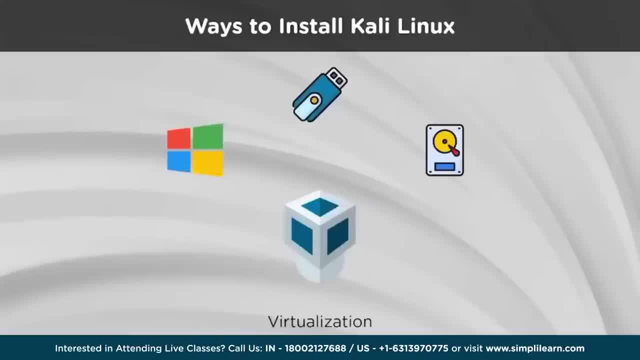 virtualization software such as VMware or VirtualBox. The software will be installed as a separate application on an already existing OS, and Kali Linux can be run as an operating system in the same computer as a window. The hardware requirements will be completely customizable, starting with the allotted RAM. 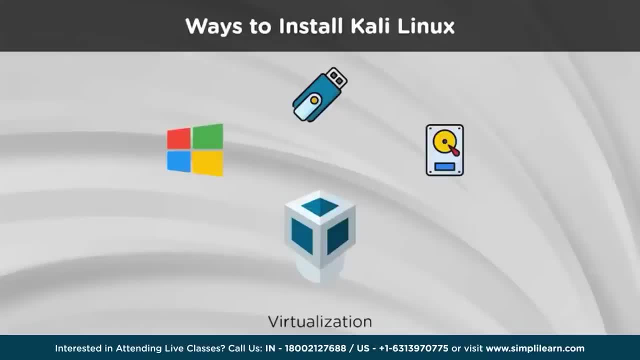 to the virtual hard disk capacity. The usage of both a host and guest operating system like Kali Linux allows users a safe environment to learn while not putting their systems at risk. If you want to learn more about how one can go forward with this method, we have a 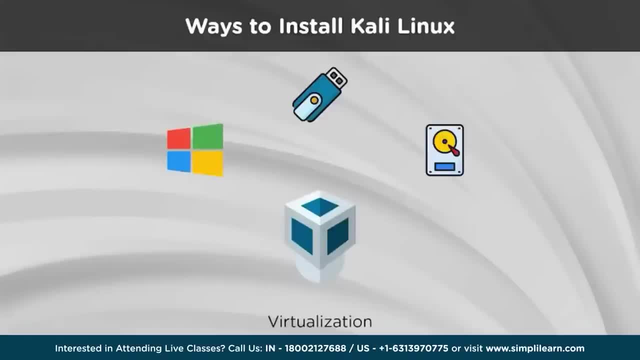 dedicated video where Kali Linux is being installed on VMware while running on a Windows 10 operating system. You can find the link in the description box to get started with your very own virtual machine. The final way to install Kali Linux is by using a dual boot system. 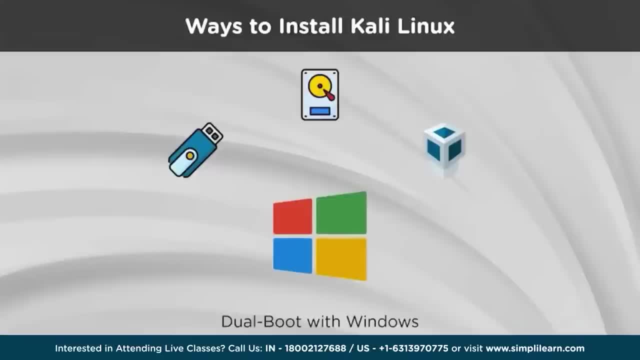 To put it in simple words, the Kali Linux OS will not be overwriting any pre-installed operating system on a machine, but will be installed alongside it. When a computer boots up, the user will get a choice to boot into either of these operating systems. 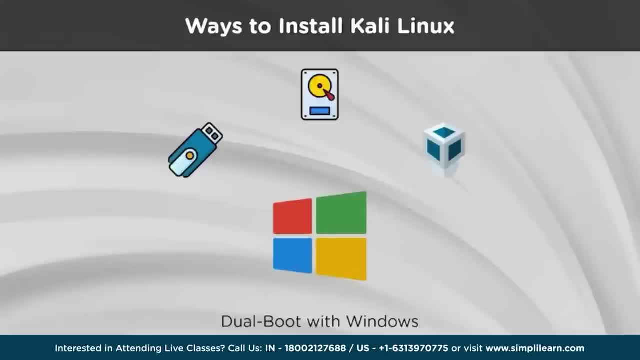 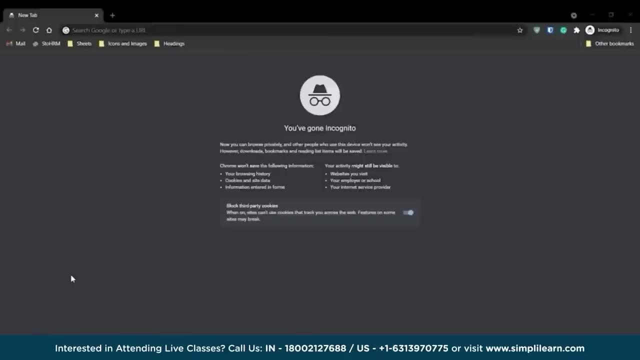 Many people prefer to keep both the Windows and Kali Linux installed, so the distribution of work and recreational activities is also allotted effectively. It gives users a safety valve should their custom Linux installation run into any bugs that cannot be fixed from within the operating system. Now for the. 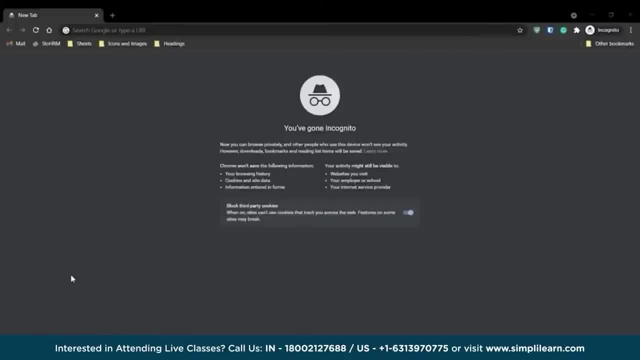 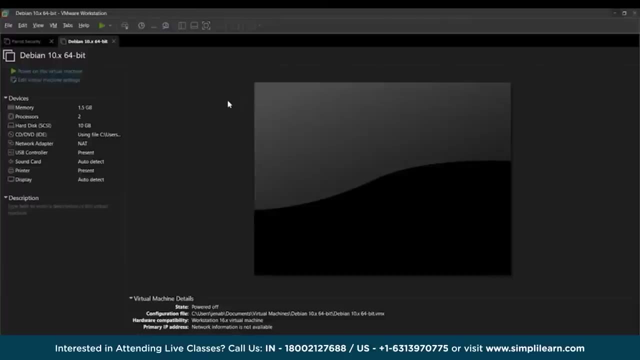 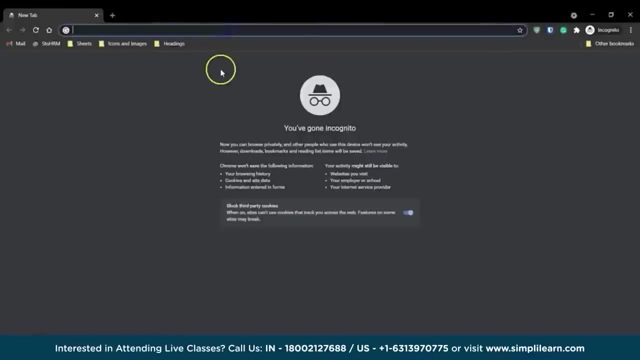 convenience of explanation, we are going to install Kali Linux today on a virtual machine software known as VMware. VMware is able to run multiple operating systems on a single host machine, which, in our case, is the Windows 10 system. To get started with Kali Linux installation, 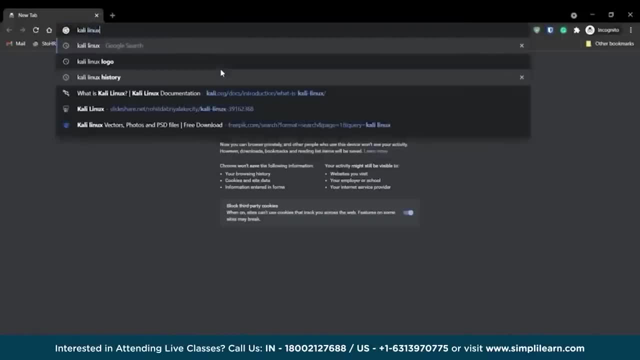 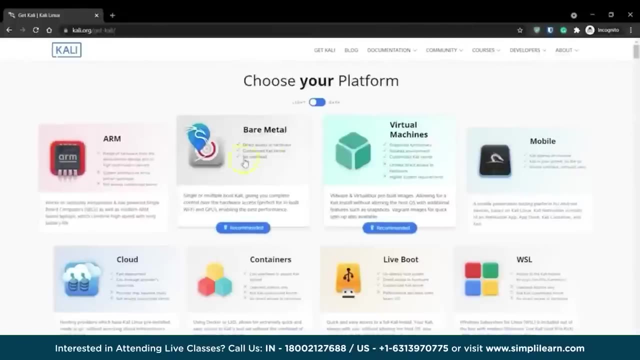 we have to go to the website to download an image file. We go to Get Kali and, as you can see, there are multiple platforms on which this operating system can be inverted As per our requirement. we are going to go with the virtual machine section. 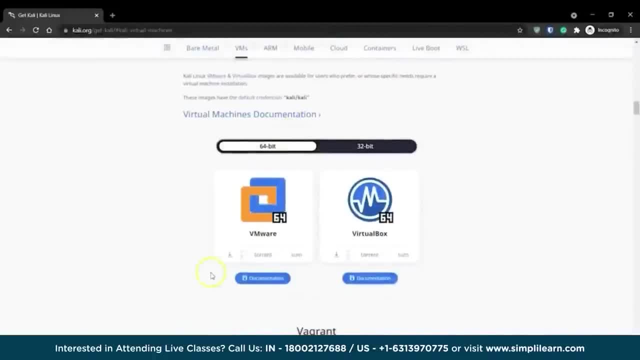 as you can see, it is already recommended by the developers. This is the download button, which will download a 64-bit ISO file. We can download 32-bit, but that is more necessary for hard metal machines or if you are going to use it for older devices, which. 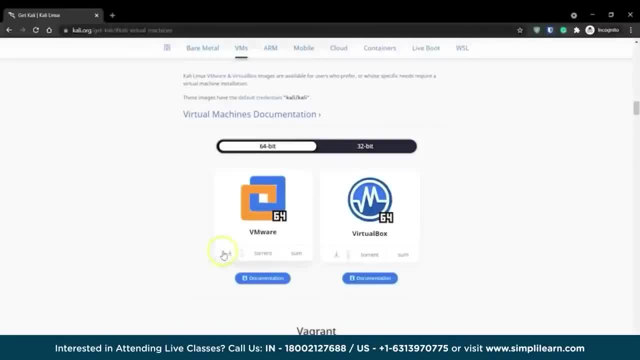 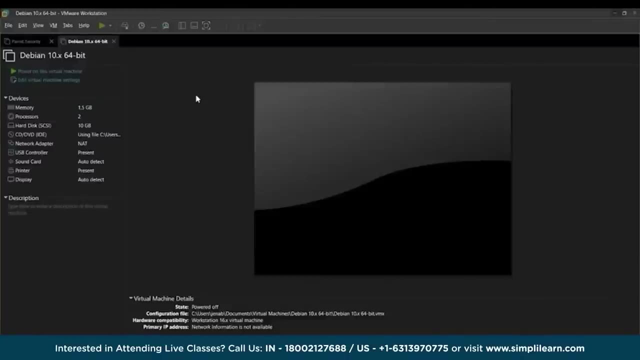 do not support 64-bit operating systems. yet After clicking on the download button, we can see we have a WinRAR archive which will have the ISO files. For now, we have downloaded the ISO file and it is already present with me, So we can start working on the VMware side. 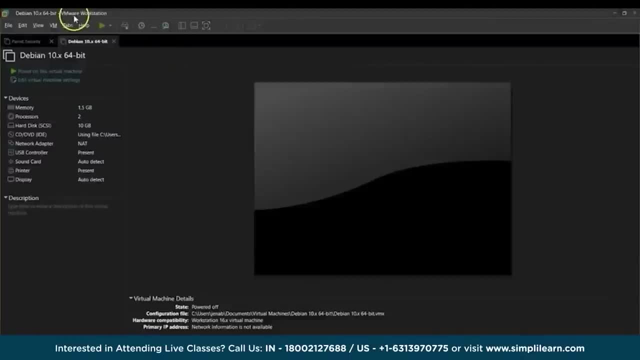 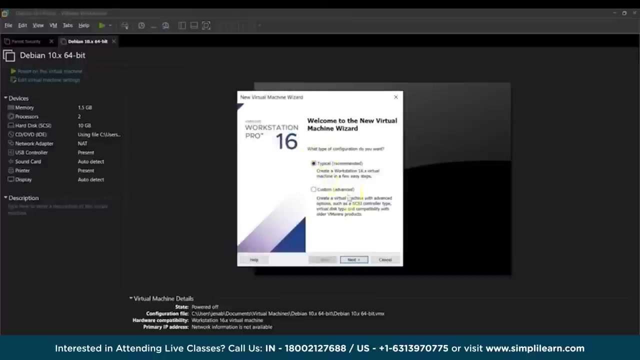 of things, Once the ISO file is downloaded, we open up VMware workstation, Go to file and we create a new virtual machine. In these two options, it is highly recommended to go with the typical setup rather than the custom one. The custom is much more advanced. 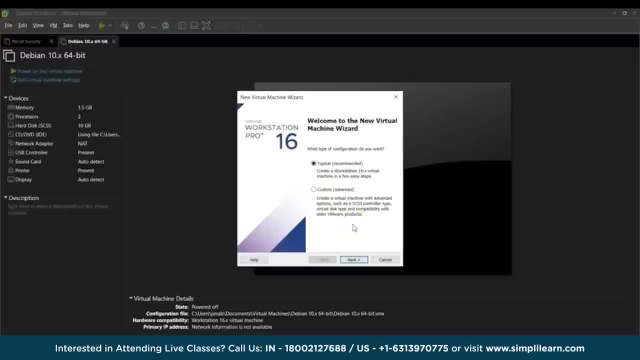 and requires much more information from the user, which is beneficial for developers and people who are well versed with virtualization software. but for 90% of the cases, typical setup will be enough. Here we can select the third option, which will be: I will install the operating system. 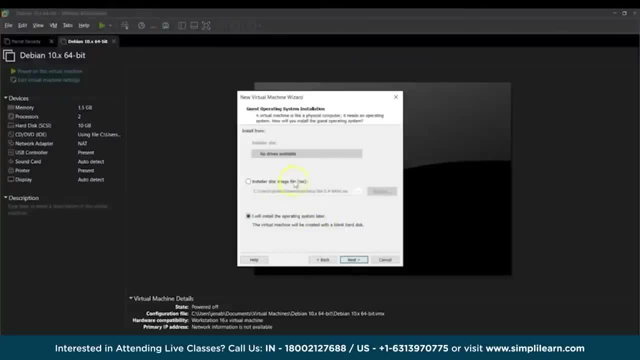 later In some operating systems we can use the ISO file here directly and VMware will install it for us. but right now, in the case of Kali Linux, the third option is always the safest. Kali Linux is a Linux distribution, so we can select Linux over here and the version. 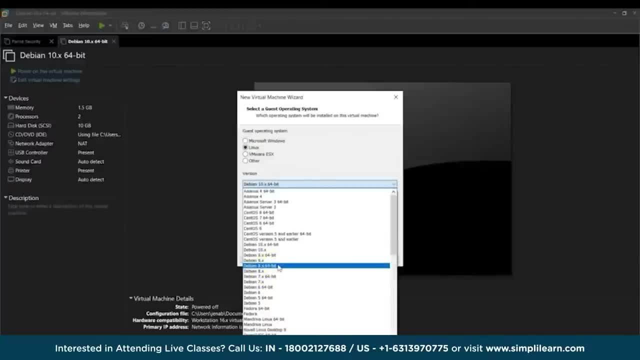 as you can see here, have multiple versions, such as the multiple kernels. Every distribution has a parent distribution. For example, Kali Linux has Debian and there are other distributions which are based or forked from some parent distribution. Kali Linux is based of Debian. 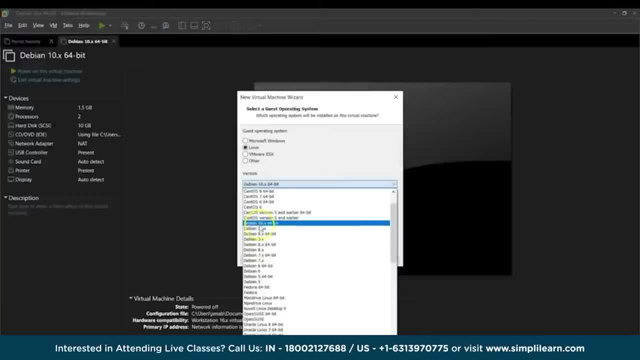 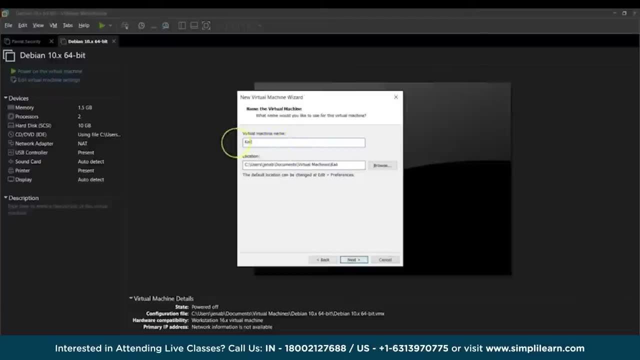 so we can go with the highest version of Debian, which is the Debian 10.x 64 bit. Go on. next, We can write any such name. We can write Kali Linux, so that it will be easier to recognize the virtual machine among this list of virtual. 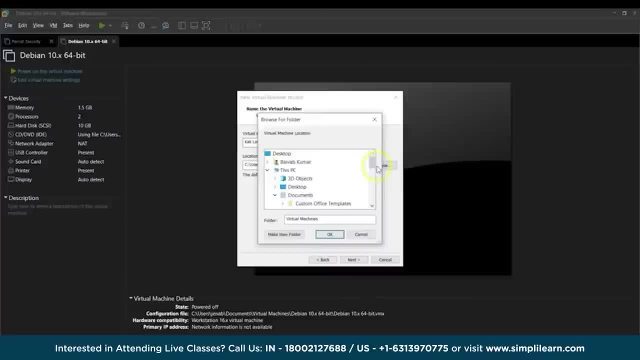 machine instances. The location can be any location You decide to put. By default it should be the documents folder. but anywhere you put, it will hold up all the information of the operating system, All the files you download, all the configurations you store. everything will be stored in this. 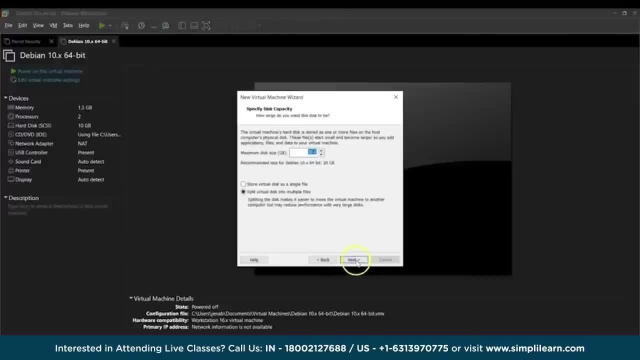 particular location that you provide. When we go next, we are asked about the disk capacity. This disk capacity will be all the storage that will be provided to your virtual machine of Kali Linux. Think of your Windows device If you have a 1 TB of hard drive. 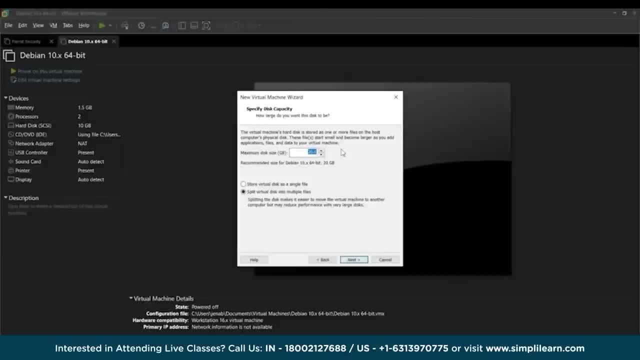 you have the entirety of the hard disk to store data on How much data you give here. you can only store up to that amount of data, Not to mention some amount of capacity will be taken up by the operating system itself to store its programs and applications. 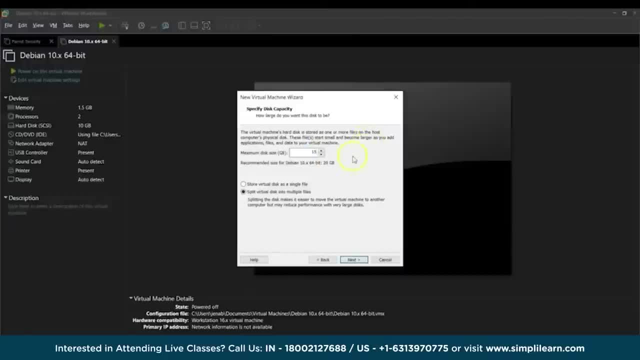 For now we can give around, let's say, 15 GB of information. or if a recommended size for Debian is 20, you can just go ahead at 20.. It depends all on the user case. if you are going to use it extensively, you can even go as high as 50 or so. 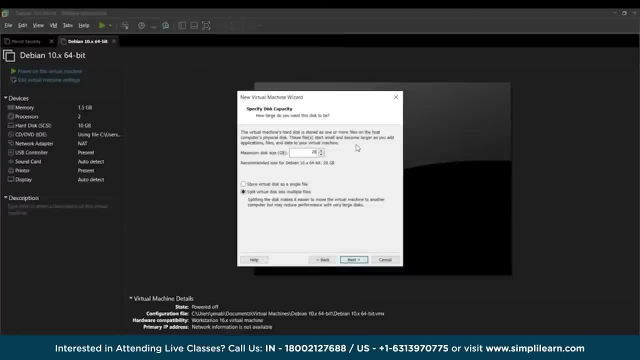 60 GB if you have plans to download many more applications and perform multiple different tests. Another option we get over here is storing virtual disks as a single file or storing them into multiple files. As we already know, this virtual machine runs entirely on VMware. 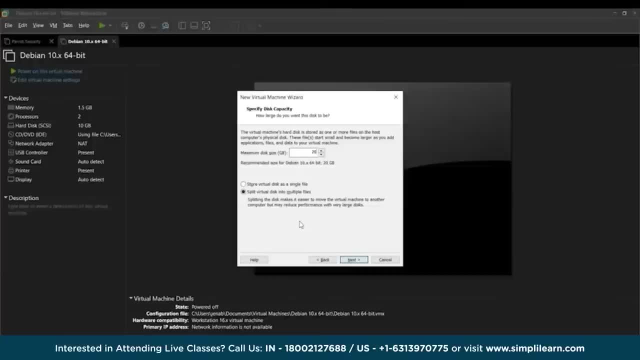 Sometimes, when transferring these virtual machine instances, let's say, from a personal computer to a work computer, you are going to need to copy up the entire folder that we had mentioned before over here. Instead, all virtual machines have a portability feature. Now, this portability feature is: 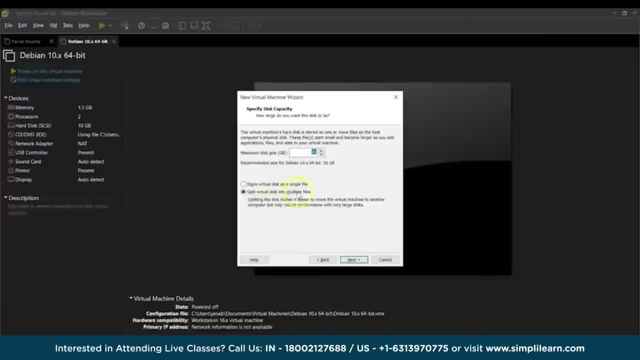 possible for all scenarios except it is much easier if you split the virtual disk into multiple files. Now, even if this makes porting virtual machines easier from either system to system or software to software, let's say, if you want to switch from VMware to VirtualBox or 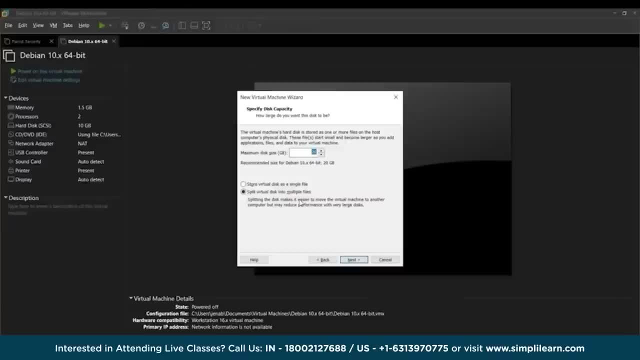 vice versa. the performance takes a small hit. It's not huge, but it's recommended to go with storing the virtual disk as a single file if you have no purposes of ever moving the virtual machine. Even if you do, it's not a complete stop that it. 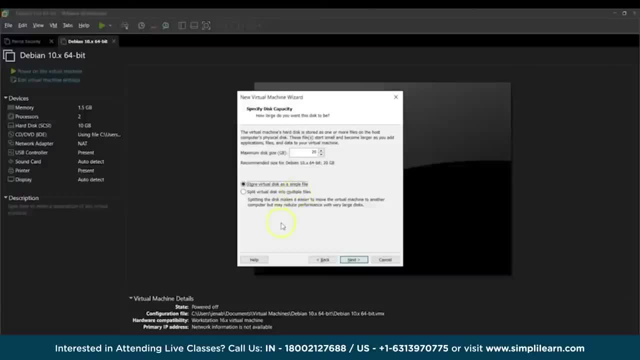 cannot be ported. It's just easier when using multiple files, But in order to get the best performance out of the virtual machine, we can store it as a single file over here. This is a summary of all the changes that we made and all the configurations that have been. 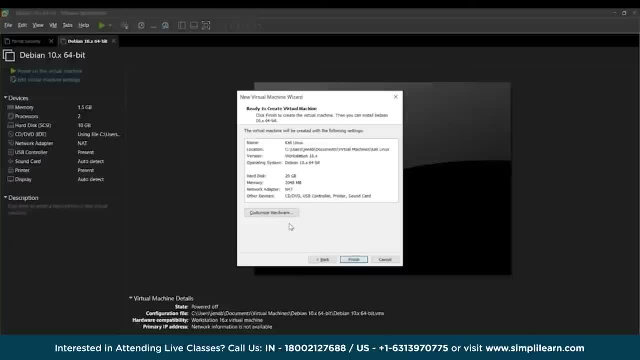 settled until now. Now, at this point of time, we have not provided the iso file yet, which is the installation file for the Kali Linux that we downloaded from this website. As of right now, we have only configured the settings of the. 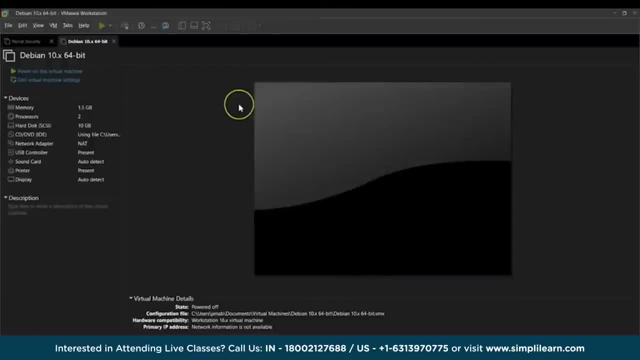 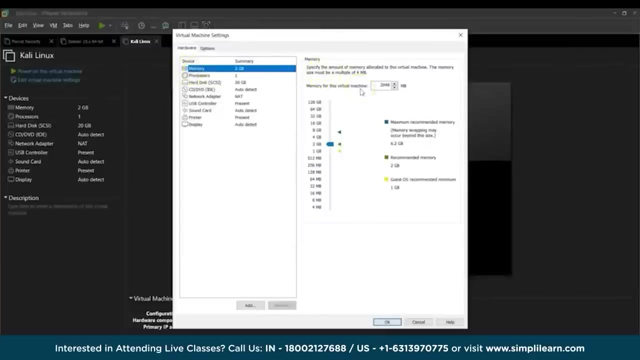 virtual machine. So we can press on Finish And we have Kali Linux in the list. Now to make the changes further, we press on Edit Virtual Machine Settings. The memory is supposed to give the RAM of the virtual machine. The devices with RAM of 8GB or. 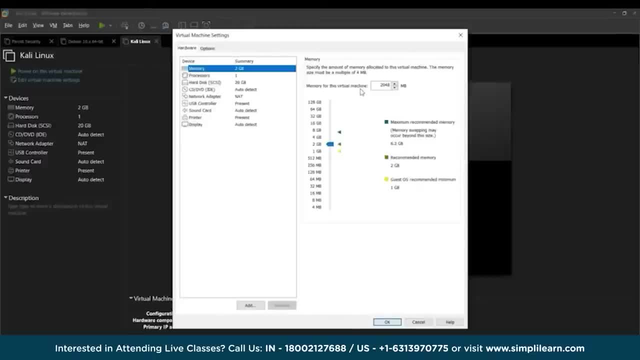 below that. giving high amount of RAM will cause performance issues and the host system If the memory has some amount of free storage left, let's say on idle storage. my Windows machine takes about 2GB, So I have 6GB of memory to provide, Although 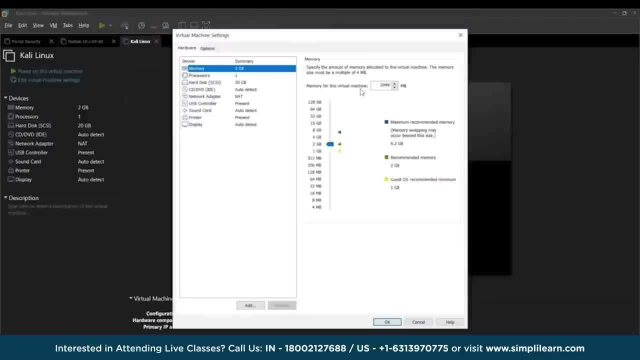 if you provide all of the 6GB, it will be much more difficult for the host system to run everything properly. So for this instance we can keep it as 2GB of memory. for the virtual machine instance, Similarly, we can use the number of processors. 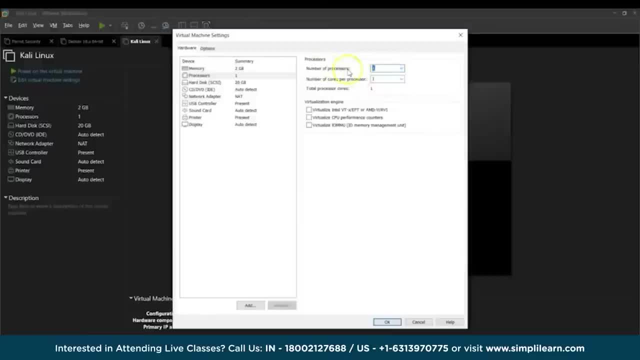 and we can customize it according to our liking. Let's say, if we want to use one processor but we want to use two different cores, we can select them as well. Hard disk is pre-set up as the SCSI hard disk and it does. 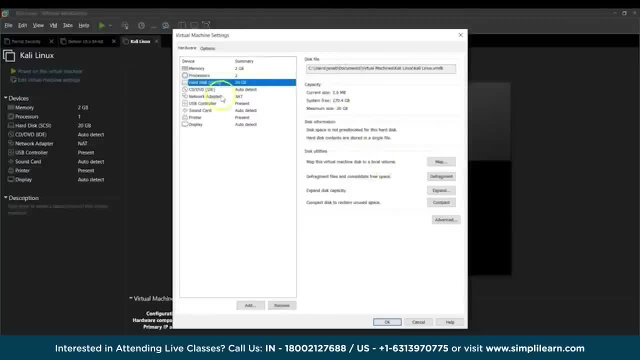 not need to be changed for the installation of this operating system at all. CD-ID DVD- This is where the installation file comes. You can think of the ISO file that we downloaded as a pen drive or a USB thumb drive which is necessary to install an operating system. 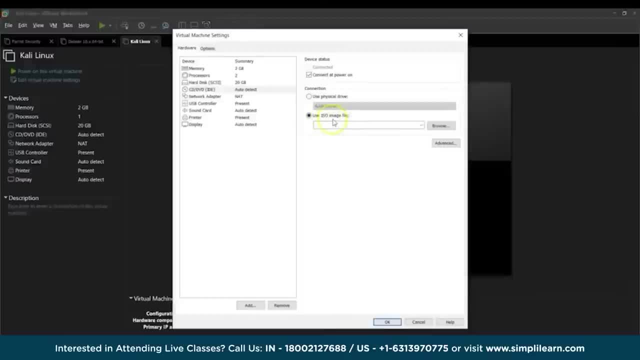 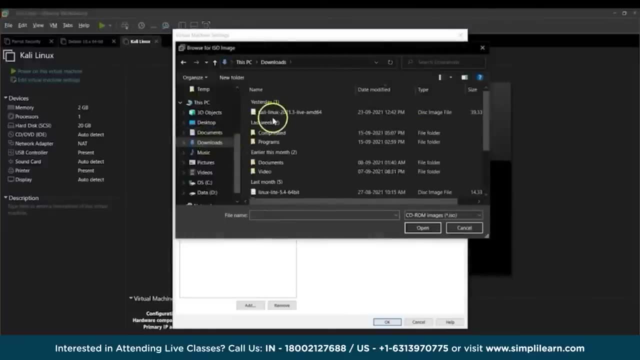 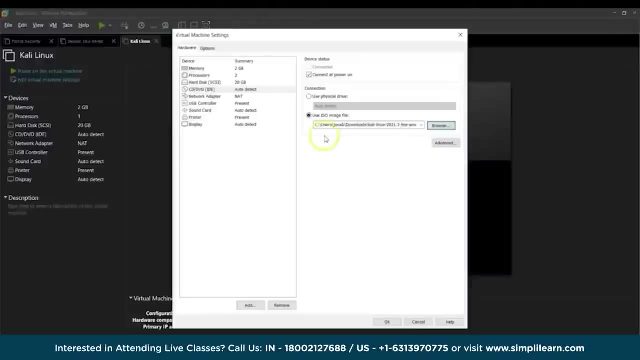 To provide this. we're going to select Use ISO image file. We're going to click on Browse, Go to Downloads and select the ISO file over here. Select Open And we can see it is already loaded up. Next, in the network adapter it is. 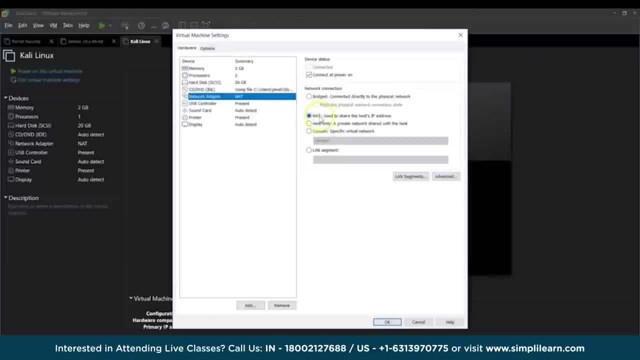 recommended to use NAT. This helps the virtual machine to draw the internet from the host machine's settings. If your host machine is connected to the internet, then the virtual machine is connected as well. There are some other options, such as host only or custom. 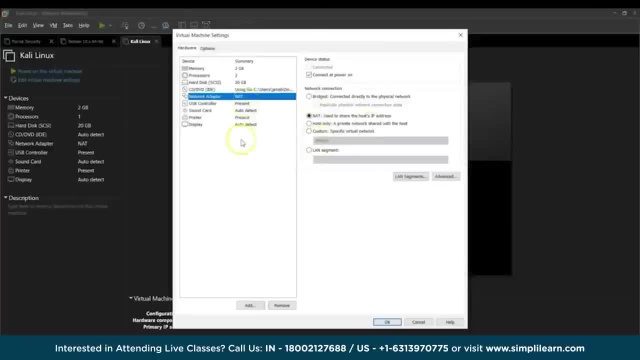 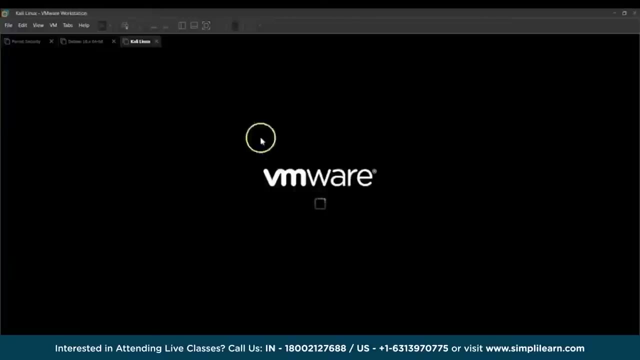 segments or LAN segments, but those are not necessary for installation. Rest of them are pretty standard, which do not need any extra configuration and can be left as it is. Press OK and now we can power on this virtual machine. In this screen we can. 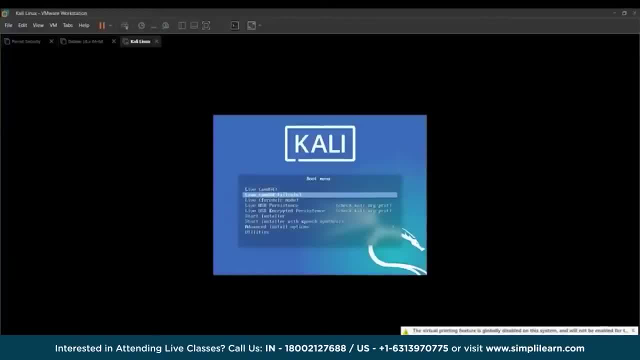 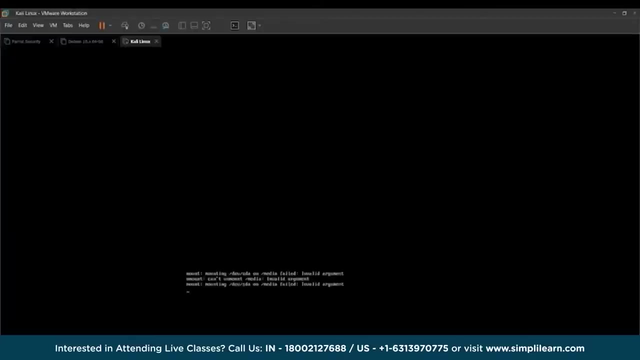 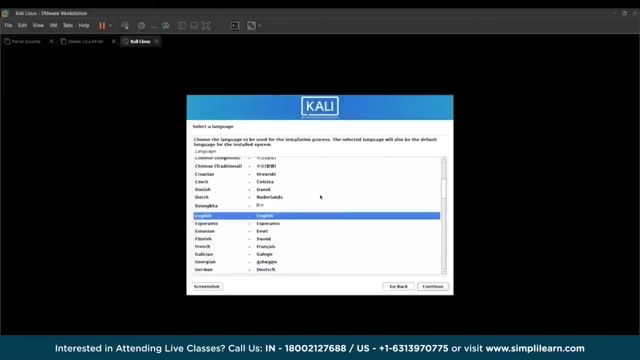 choose how we want to proceed with the installation. We have a Start Installer option over here, So we're going to press Enter on that. We're going to wait for the things to load from the ISO file. The first step in the installation is: 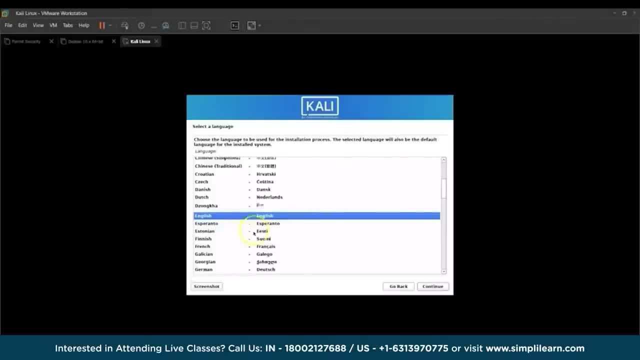 choosing the language of the operating system. For this we can go with English as standard. This is the location. This will be used for setting up the time and some of the internal settings, which depend entirely on the location of the user. So for this, 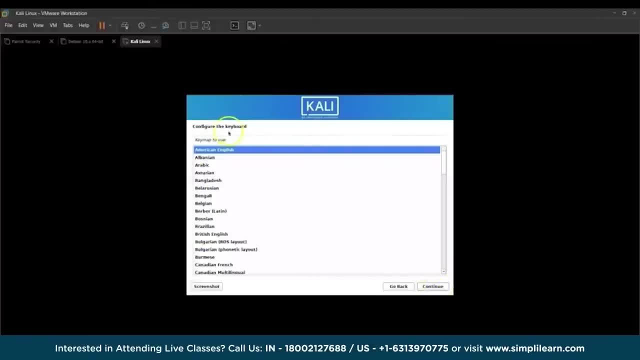 we're going to go with India Configuring the keyboard. it's always recommended to go with the American English first. Many people make a mistake of going with the Indian keyboard if it is possible, and it provides a lot of issues later on. So it's always preferred to go with the American English. 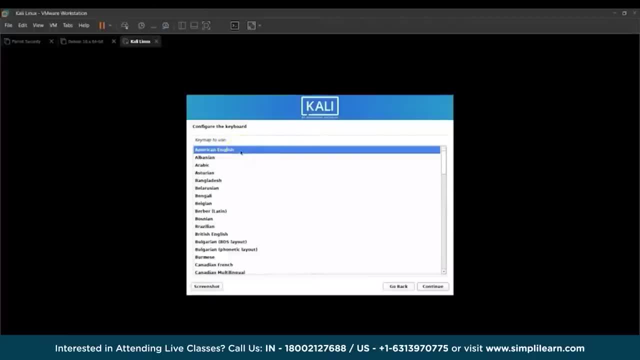 and if later we see some necessity of another keyboard that is required, we can install it later, But for now we should always stick with American English as a basic At this point. it's going to load the installation components from the iso file. 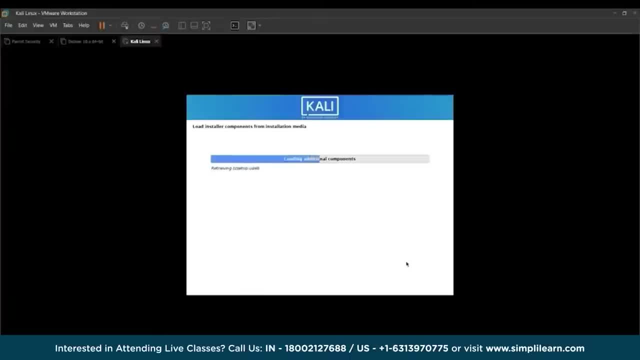 It is a big file of 3.6 GB, so it has a lot of components that need to be put into the virtual machine, which can also be used to detect hardware Once the hardware and the network configuration is done by the iso file. 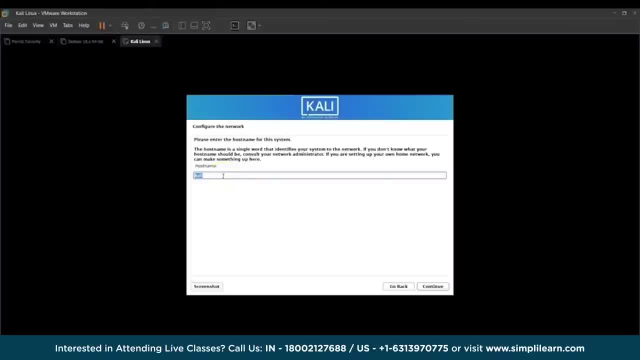 we want to write a hostname for the system. This hostname can be anything which is used to recognize this device on a local network or a LAN cable. Let's say, if we use the name Kali Domain name, we can skip it for now. 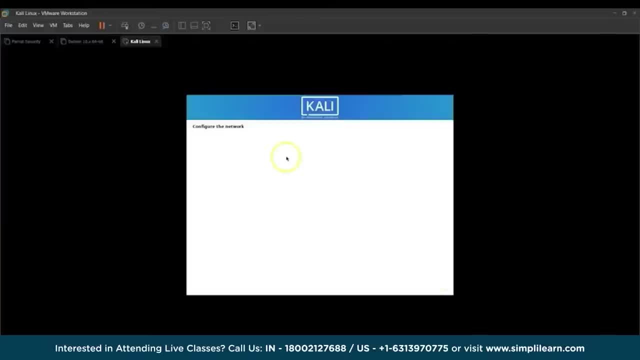 It's not necessary as such for the installation. This is the full name for the user. Let's say, we can provide the name as simply learn as a full name. Next, we're going to set up a username. This username is going to be necessary to. 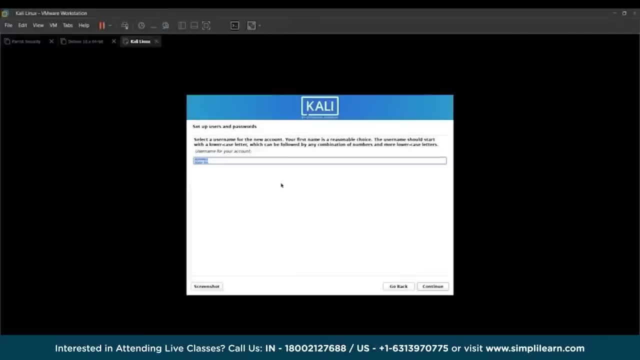 identify the user from its root accounts and the subsequent below accounts. For now, we can give it as something as simply 123.. Now we have to choose a password for the user. Now, remember, since this is the first user that is being added onto this newly installed. 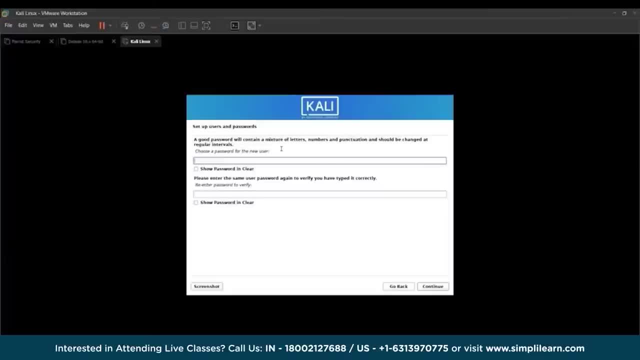 operating system. it needs to be a password for the administrator. We can use whichever password we like over here and use the same password below and press on continue. At this point it's going to detect on the components on which the operating system can be. 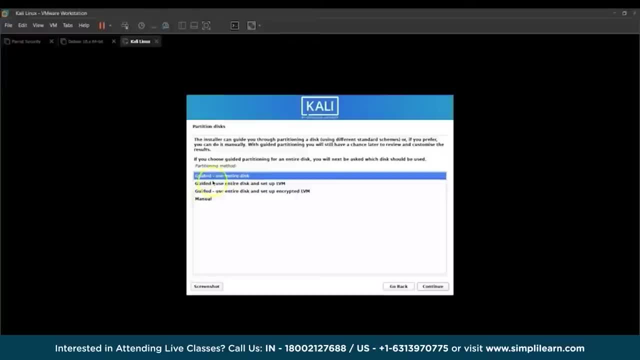 installed, like here. There are multiple options, like the use entire disk, use entire disk and setup LVM, use entire disk and setup encrypted LVM. For newcomers, it is recommended to just use the first one, since LVM encryption is something that we can learn. 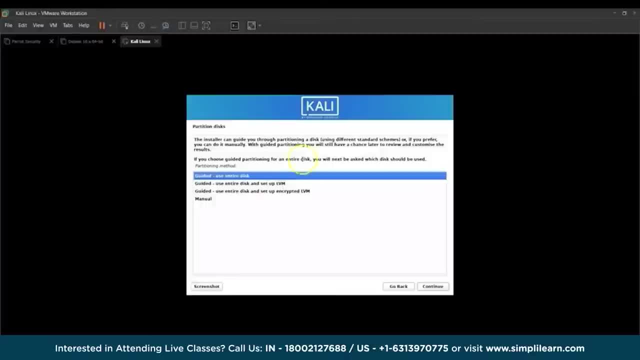 afterwards when you're much more hands-on with the Linux operating system. For now, we're going to use the use entire disk guided installation and press on continue. When we set up the virtual machine on VMware, we had set up a disk capacity that we gave. 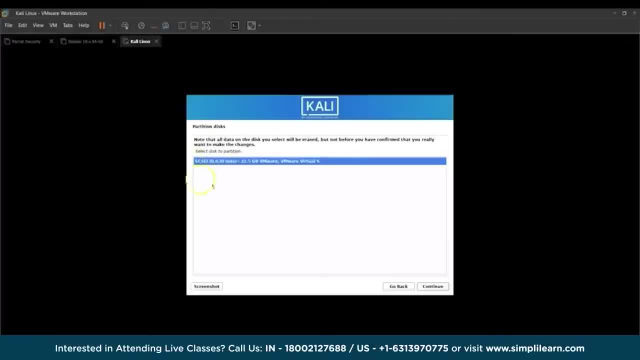 a purpose. 20 GB, That is the hard disk which is being discovered here. Even though it is a virtual disk on VMware, it acts as a normal hard disk on which an operating system can be installed. So we select this one and press on continue. 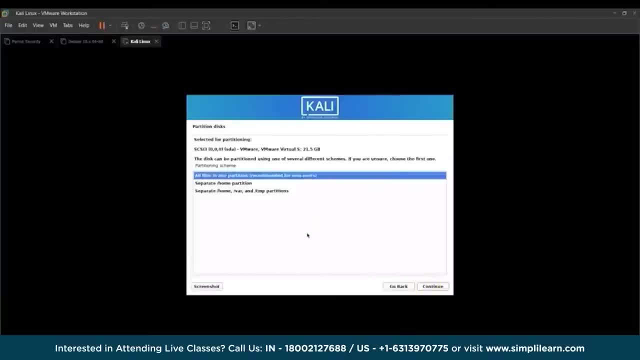 Here there is a multiple partition system. All the operating systems that are installed have different components. One is used for the keeping of the application, one for the files, other for the RAM management and other things. For newcomers, it is always recommended to keep it in one partition. 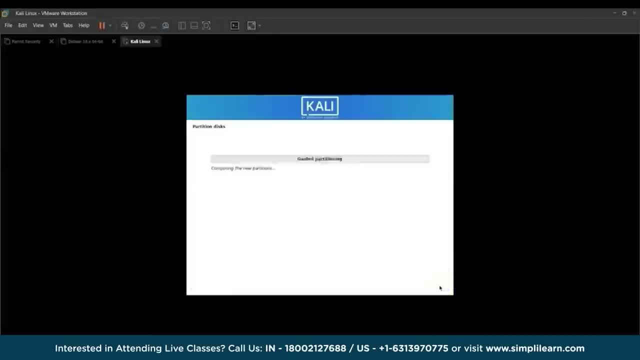 and we're going to select that and press on continue. This is just an overview of the partition it's going to make. As you can see, it has a primary partition of 20.4 GB and a logical partition of 1 GB used for swap memory. 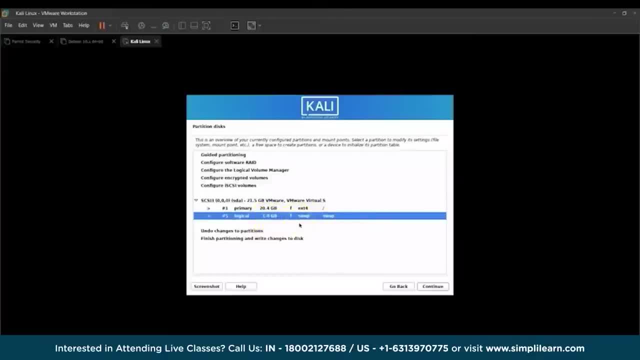 Now, these kind of naming can be confusing for people who are not well versed with Linux operating systems or, in general, virtualization. But for now, you can go ahead and press on continue. as this will be fine, We can press on finish partitioning. 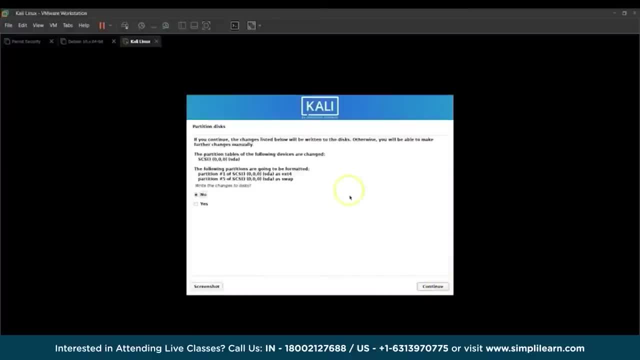 and write changes to disk and continue. It's just a confirmation page. As you can see. it shows that SCSI3 is our virtual hard disk of 20 GB disk capacity. We write the changes to the disk, We press yes and click on continue. 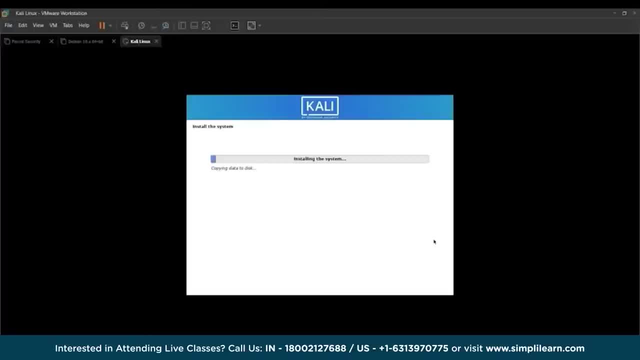 At this point the installation has started. Now. this installation will take a while, depending on the amount of RAM provided, the processors provided and how quickly the performance of the system is being hampered by the host machine. On quicker systems, this will be rather quick while. 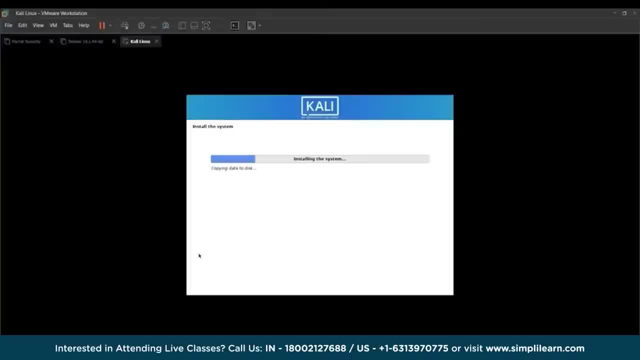 on the smaller ones. this will take a while, Since this is going to take some time to install, as it is being run on a virtual machine with only 2 GB of RAM, we're going to speed up this part of the video so we don't have to waste any more time. 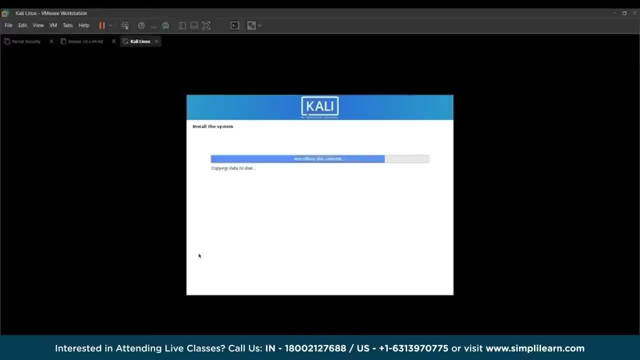 just watching the progress bar. Let's start the installation. Now that our core installation is completed, it is asking us to configure a package manager. The work of a package manager on Linux operating system is similar to the Google Play Store on Android mobile devices and the apps. 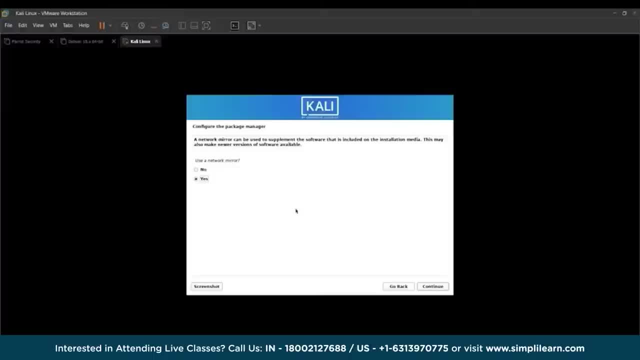 store for the Apple devices. It's an interface to install external applications which are not installed by default, Let's say for Google Chrome or any other browser which can be used to browse the internet At this point of time. it asks us to select a network mirror. We're going to select 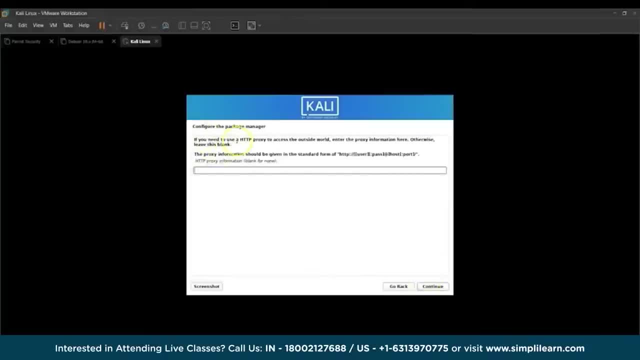 as yes and move forward with this. Next, it's going to ask us for a HTTP proxy, which we can leave it as blank and press it as continue forward. At this point of time, it's looking for updates to the Kali Linux installation. This will fetch the new builds from the Kali server. 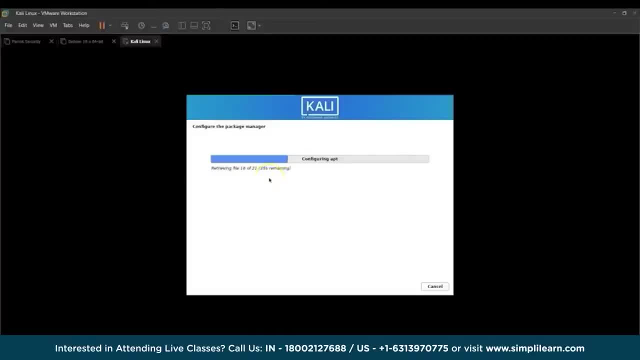 so the installation is always updated to the latest version. Now that the package manager is configured, we have the Grub bootloader. The Grub is used for selecting the operating system while booting up. Its core functionality is to allow the operating system to boot up. It's a very simple way to boot up the operating system. It's a very simple way. 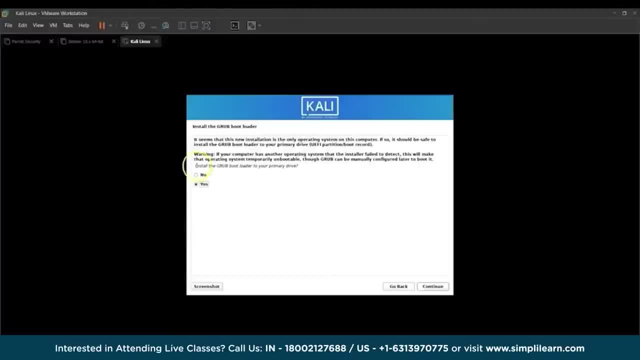 to boot up the operating system to be loaded correctly without any faults. So at this point of time, if it asks install the Grub bootloader to your primary dive, we can select it as yes and press continue. Remember the installation was conducted on dev SDA, So we're going to. 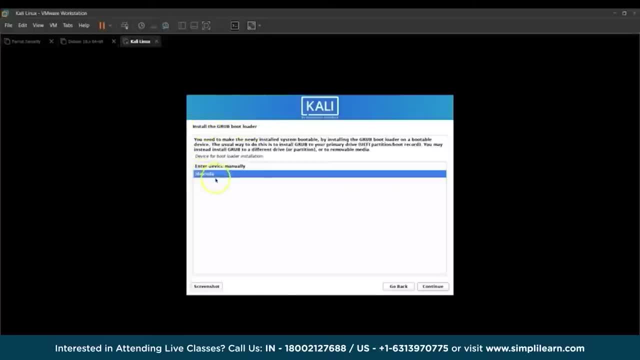 select installation of the Grub loader on the same hard disk that we have configured. Press this one and press continue. So now the Grub bootloader is being installed. The Grub is highly essential because it shows the motherboard where to start the operating system. 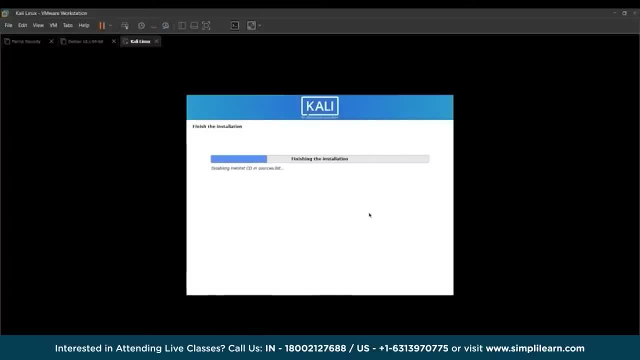 from. Even if the operating system is installed correctly and all the files are in correct order, the absence of a bootloader will not be able to launch the OS properly. As you can see, the installation is finally complete, So now we can press on continue. 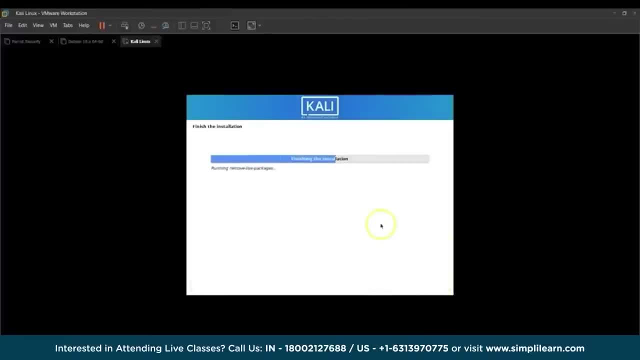 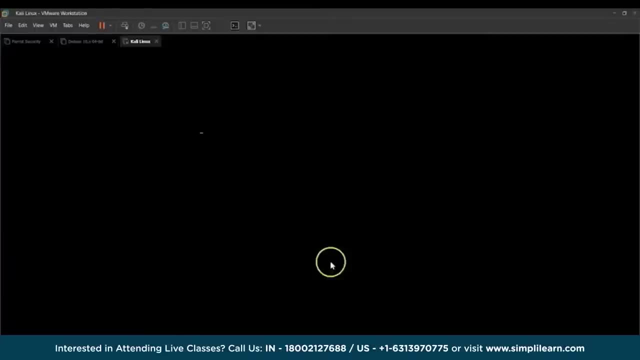 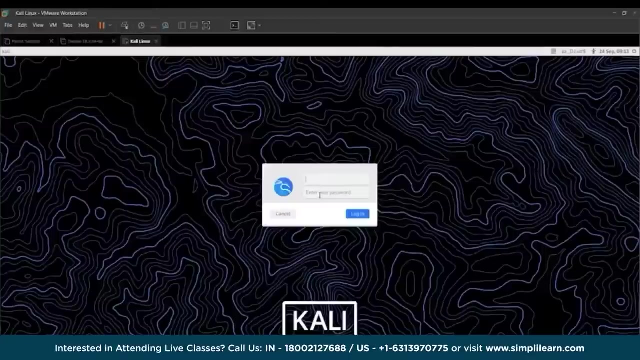 and it's going to finalize the changes. Now you can see KAL Linux being booted up straight away. It doesn't check for the ISO file anymore, since the operating system is now installed onto the virtual hard disk storage that we had configured before. Here we're going to enter our username and password that we had set up before. 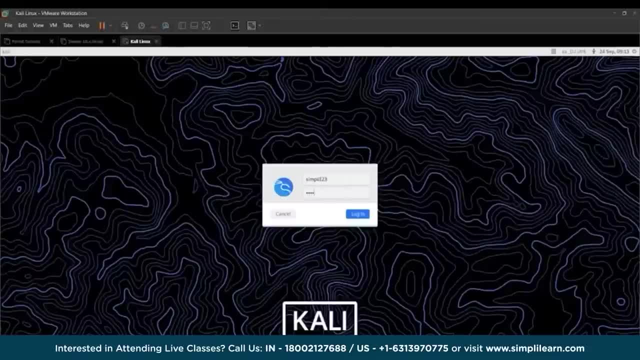 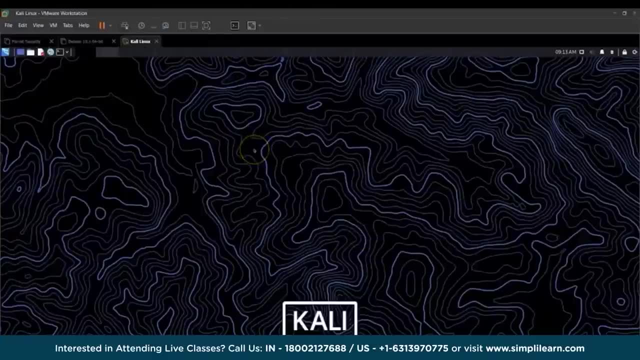 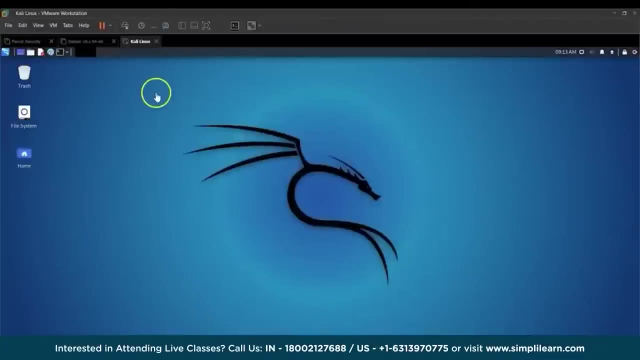 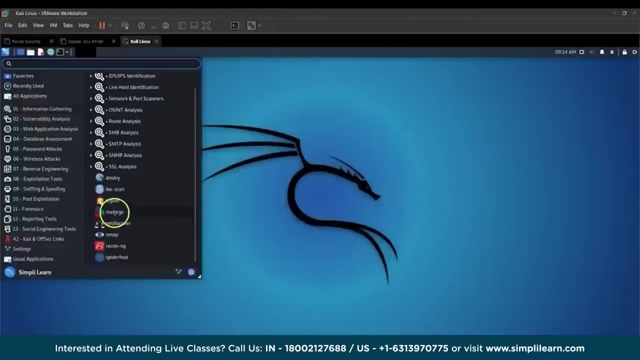 And we have the KAL Linux system booted up, and this is your homepage. We can see the installed applications over here, which are being used for penetration testing by multiple security Advisors worldwide. All of these come pre-installed with Kali Linux and others can be installed using the APT Package Manager that we had configured. 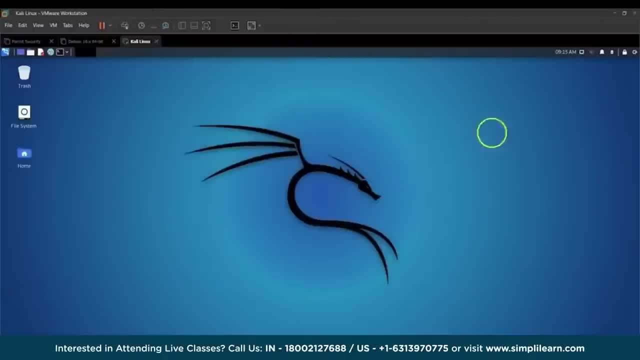 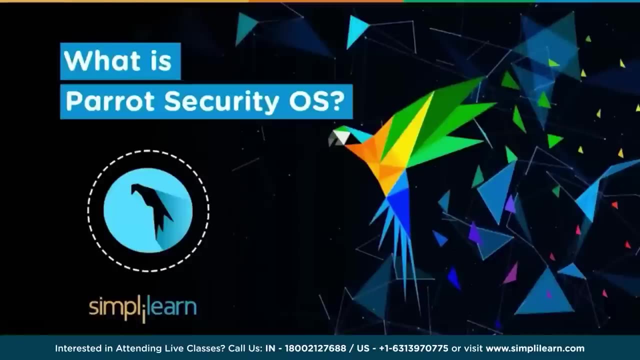 We can see a full name over here, And with this, our installation of the Kali Linux is complete. Hey everyone, it's no secret that the majority of our internet usage is at the risk of getting hacked, be it via unsafe messaging applications or misconfigured operating systems. 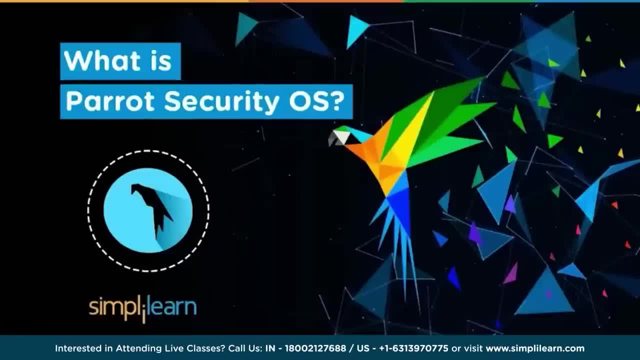 To counteract this void of digital security. penetration testing has become the norm when it comes to vulnerability assessment. Parallel Security OS is an operating system that has become a well-known weapon in this fight against hackers, While enough distribution more catered towards penetration testers specifically. 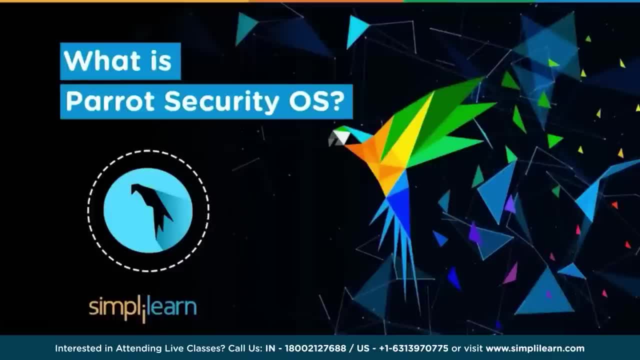 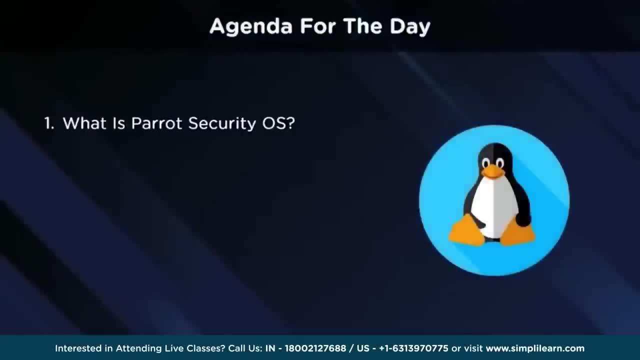 Parallel Security has layers of features that we will be covering in today's lesson. Let's take a look at the topics for this video. We start by learning about what Parallel Security is and why it should be considered as a viable alternative, next to Kali Linux, for penetration testers. 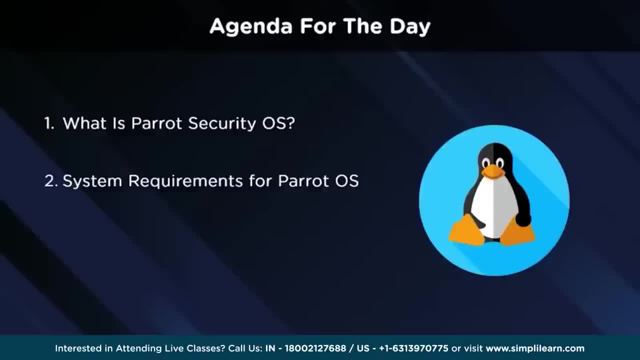 Next, we take a look at the minimum system requirements necessary to obtain optimum performance from an installation of Parallel Security. Moving on, we learn about some unique features that make Parallel Security stand out among the multiple ethical hacking operating systems available on the market. And finally, we look at the multiple ways that Parallel Security OS can be installed. 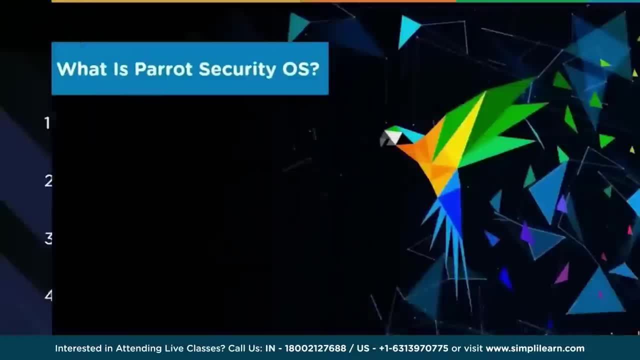 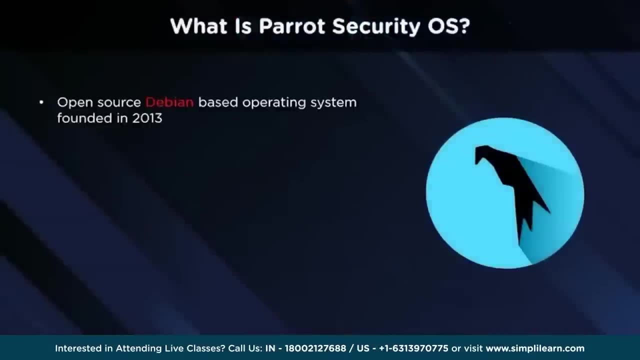 be it on a single system or for portable media. So let's start out by learning what Parallel Security is. Parallel Security OS is a Debian-based Linux distribution with an emphasis on security, privacy and development. It is built on Debian's testing branch and uses a custom hard Linux kernel, while being founded in 2013.. 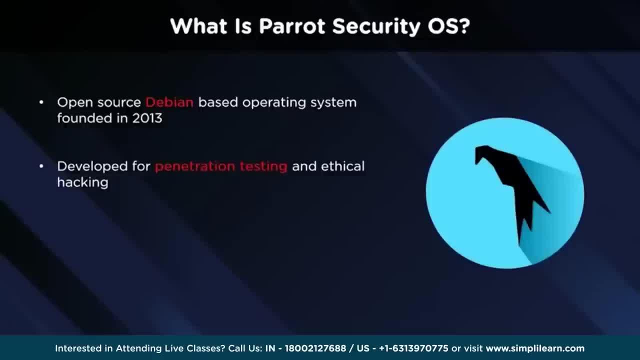 Parallel Security contains several hundred tools targeted towards various information security tasks, such as penetration, testing, security research, computer forensics and reverse engineering. It has become a multi-platform solution accessible and freely available to information security professionals and hobbyists. It features a distinct forensics mode that does not mount any of the system hard disks or partitions and has no influence on the host system. 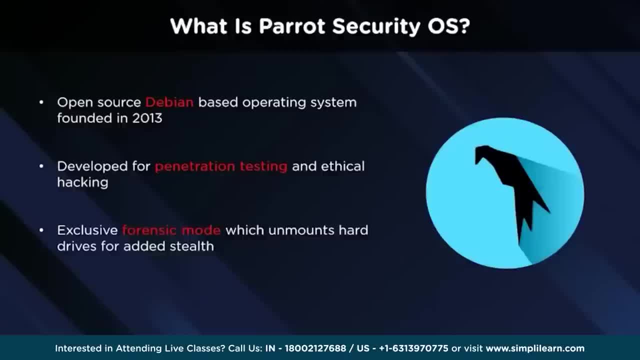 making it more stealthy than regular mode. This mode is used on the host system when there is a need for executing forensic procedures In software development. a rolling release is a paradigm in which software upgrades are rolled out constantly rather than in batches of versions. 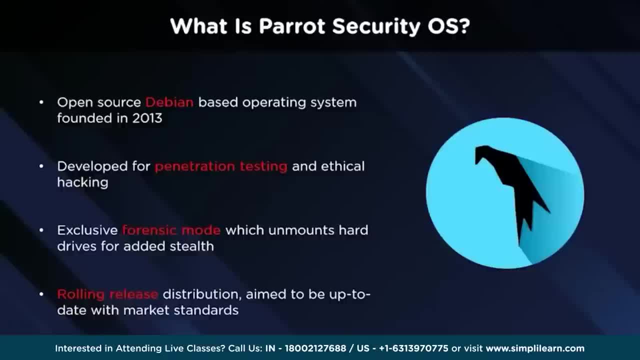 This ensures that the software is constantly up-to-date. A rolling release distribution such as Parallel Security OS follows the same concept, providing the most recent Linux kernel and software versions as they become available on the market, With a basic introduction to the operating system out of the way. 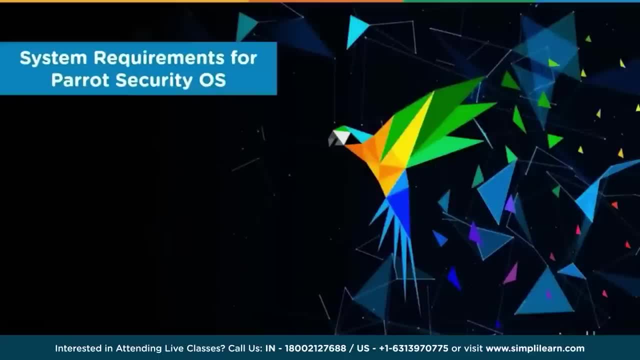 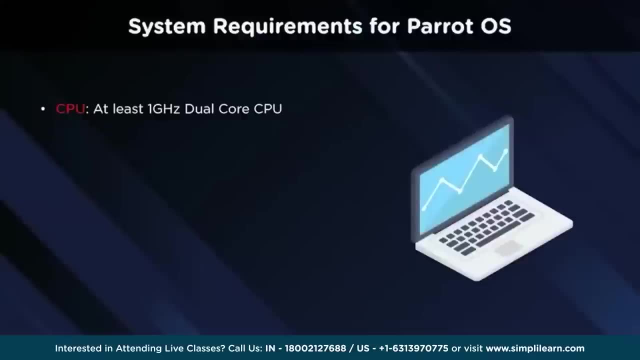 let us have a look at the bare minimum system requirements necessary to be able to run this operating system. First up, we got a CPU requirement which states that a 1 GHz dual-core CPU is the absolute minimum in order to use Barrett OS, While multiple-core systems will provide more optimum performance. a small beginner has been included. 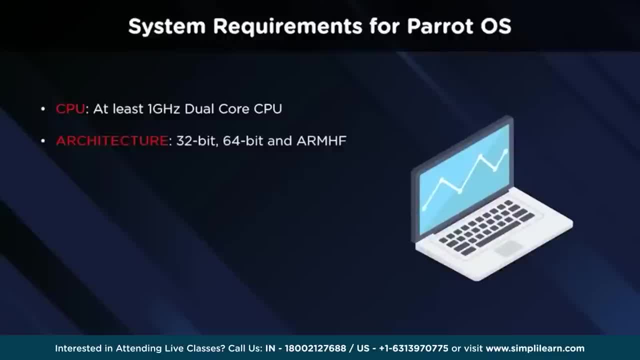 A very distinct thing to be noted is that the operating system can be installed on all variants of chipsets, be it 32-bit, 64-bit and the newly popular ARM portfolio of devices, Unlike Kali Linux, which requires some amount of graphical acceleration needed to display the operating system correctly. 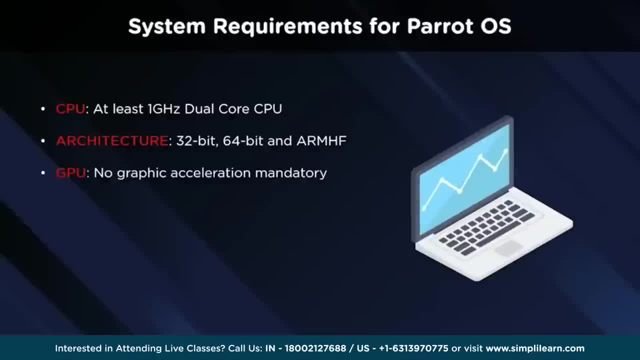 Barrett OS has no such requirements and can be used with the leanest of machines. Taking into account the RAM issue, a minimum of 256 MB to 512 MB free RAM provides the optimum usage scenarios. Even when the OS is installed on a hard drive storage media, it should theoretically occupy around 8 GB of information. 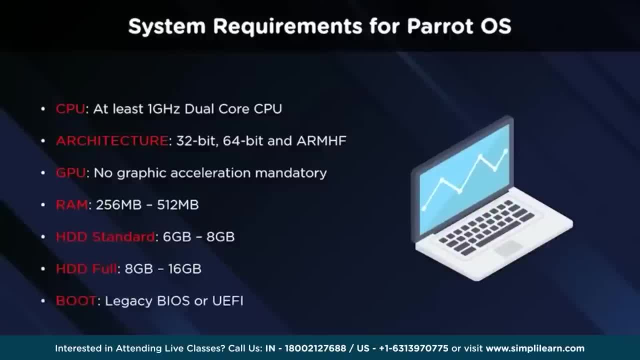 which may extend up to 16 GB, depending on the tools being installed out of the box. When it comes to booting options, we have the option of going with the legacy BIOS settings or with the more modern UEFI settings. These are just some of the requirements for the installation of Barrett Security OS. 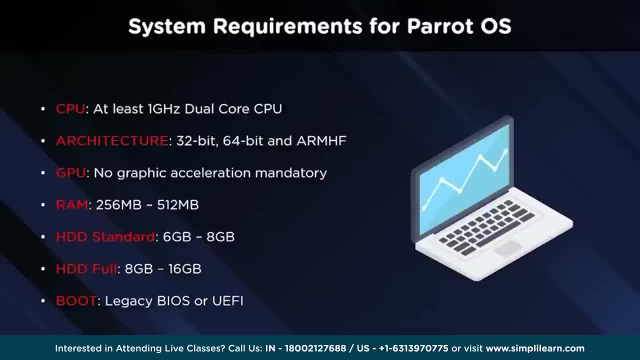 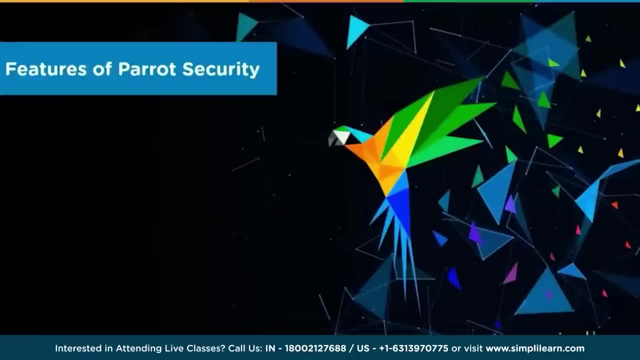 To understand this process more vividly and to learn how visualization can help install an OS in our existing computer, please follow the link to a Barrett Security installation video, linked right above. Let's understand what some of the things that make Barrett Security unique among all the other penetration testing operating systems. 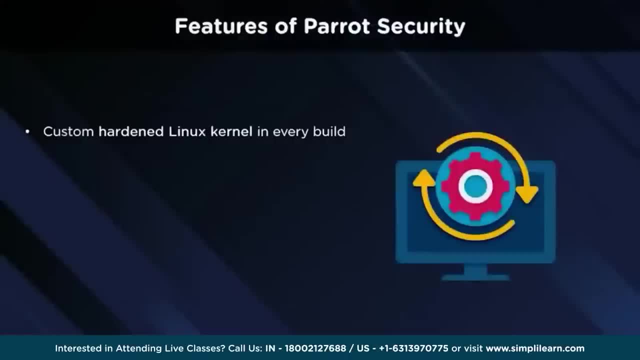 Along with all the giant catalog of scripts. Barrett Security has its own custom-hardened Linux kernel, which has been modified explicitly to provide as much security and resistance to hackers as possible. as a first line of defense, The configurations in the operating system act as a second gateway, taking care of malicious requests and dropping them off. 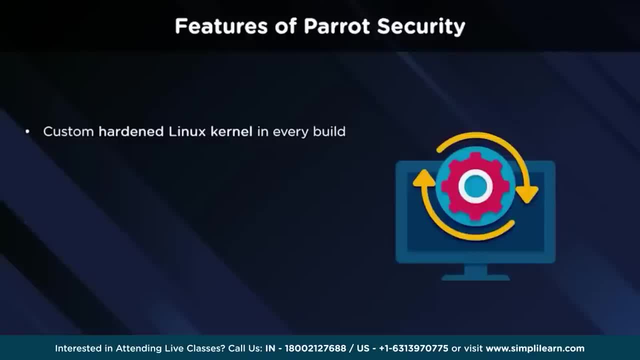 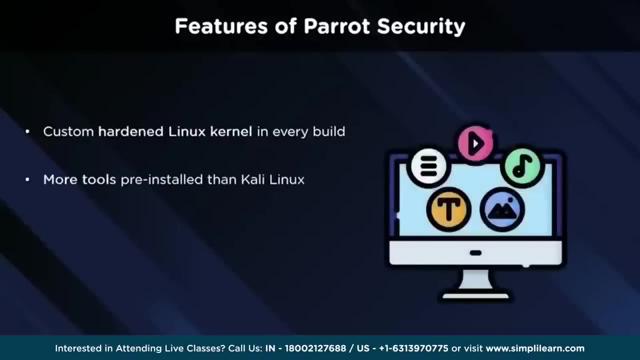 This is particularly beneficial, since, should there be a scenario where the latest Linux kernel is causing some particular issue, the Barrett OS development team will most likely iron it out first before passing it on as an update, If the custom-hardened kernel wasn't reasoning enough. 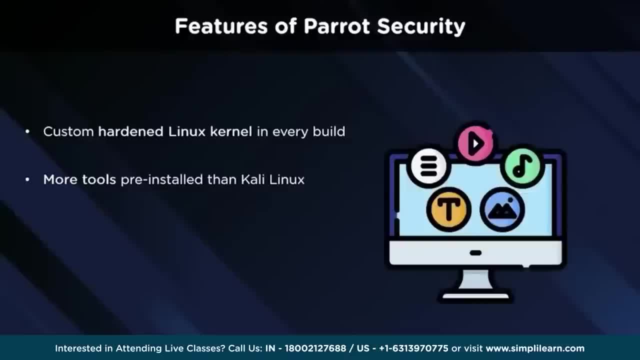 Barrett Security developers managed to install more hacking tools and scripts. to ensure a smooth transition for the Gali Linux users, All the tools you found in Gali are present in Barrett OS, and then a few extra ones for good measure. This has been achieved while keeping roughly the same size of the installation file between both operating systems. 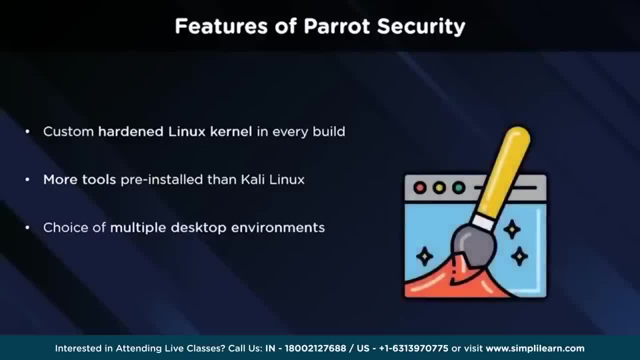 However, it's not all. productivity points for Barrett OS. They provide a choice between two different desktop environments: the Mate Desktop, which comes pre-installed by default, and KDE. For those unfamiliar with Linux terminology, you can think of desktop environments as the main UI for a Linux system. 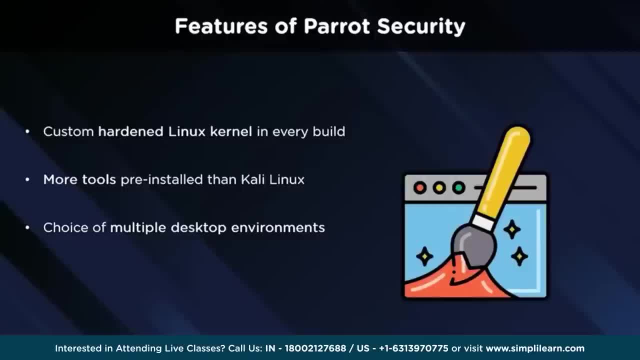 Being highly modular in nature, one can use Kali, Linux or Barrett OS while adding another desktop environment which they find appealing. While Kali has only a single option, Barrett OS has managed to provide two optimized wheels, with Mate Desktop and KDE Desktop ready-made on their website. 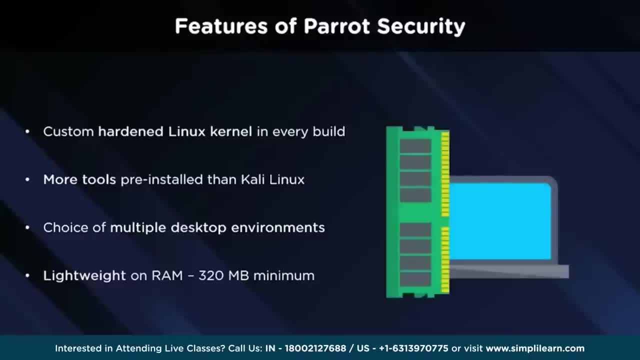 One of the primary advantages of Barrett OS over Kali is that it's relatively lightweight. This implies that it takes frequently less disk space and computing power to function properly, with as little as 320 MB of RAM required. In reality, Barrett OS is also designed to operate successfully off a USB stick. 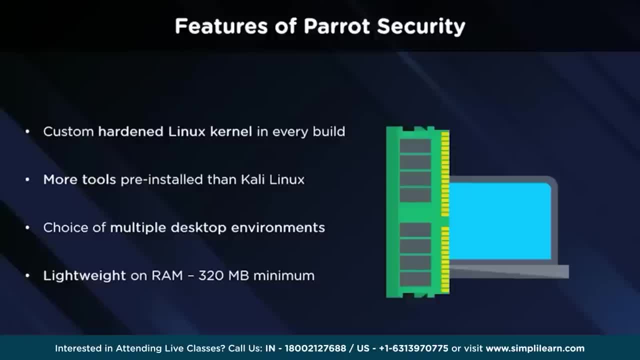 but Kali Linux does not work well from a USB stick and is generally installed in a virtual machine. Barrett OS can be seen as more of a niche distribution if you're searching for something lighter than Kali Linux. There are multiple ways to go about with this installation. 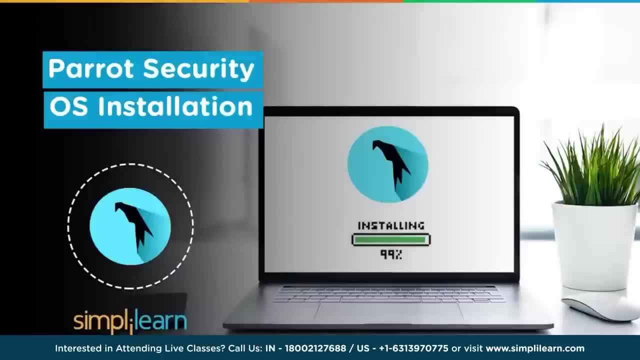 Many people prefer to install it directly onto a hard disk, where the Barrett Security OS will override whichever data the hard disk already has Now. this is beneficial if you want to preserve your data for the long term, but this might pose some trouble to people who do not have a spare hard disk. 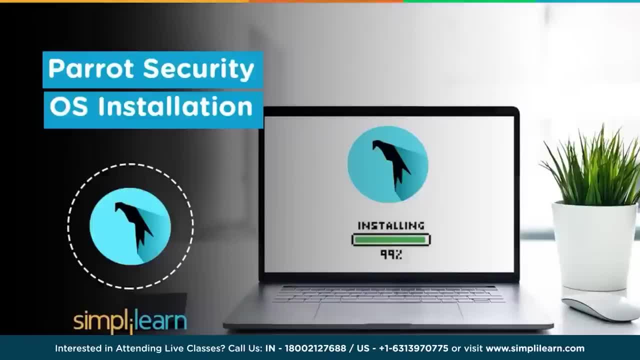 or do not want to lose their current installation of Windows operating system. Another way to use Barrett Security is by using the live boot. but whatever changes we make to the live boot operating system, those changes are removed the moment we restart or shut down the system. 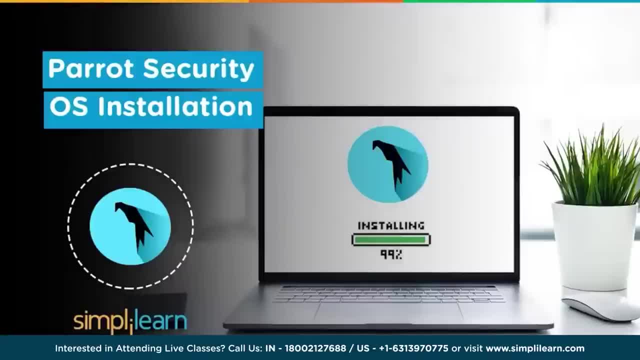 A very good common ground between both these installations is virtualization. Using virtualization software like VMware or VirtualBox, we can install Barrett Security on our systems while simultaneously saving our data and having the convenience of a host machine such as a Windows operating system. 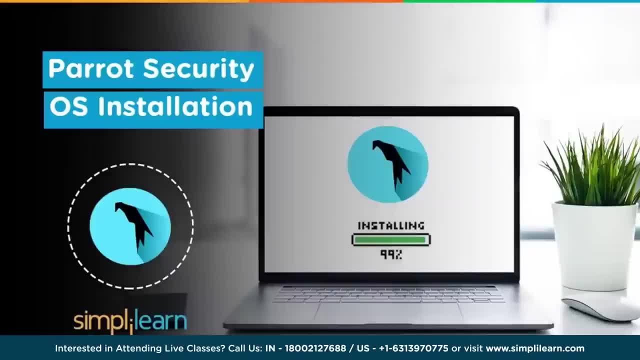 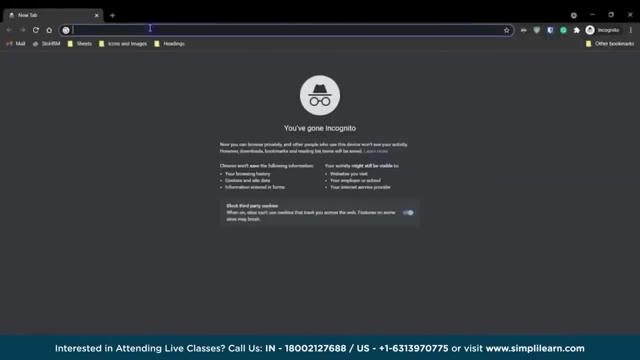 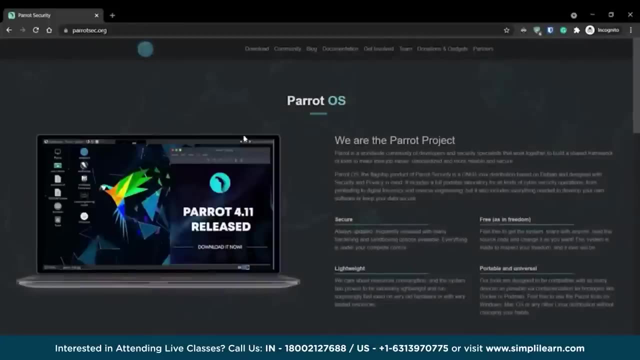 in case things go wrong. To start the installation we first need to get an ISO file for the Barrett Security operating system. This can be found on the current website, barrettsecorg. Once we enter the website, move into the download section. 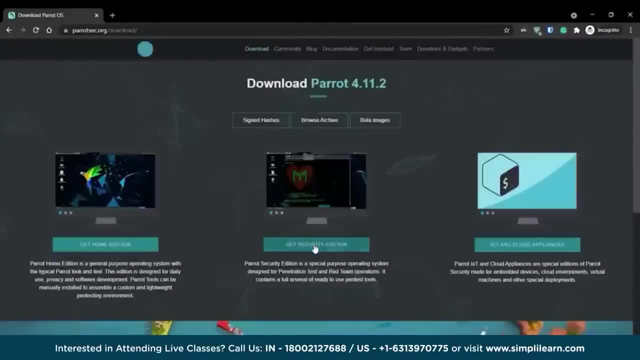 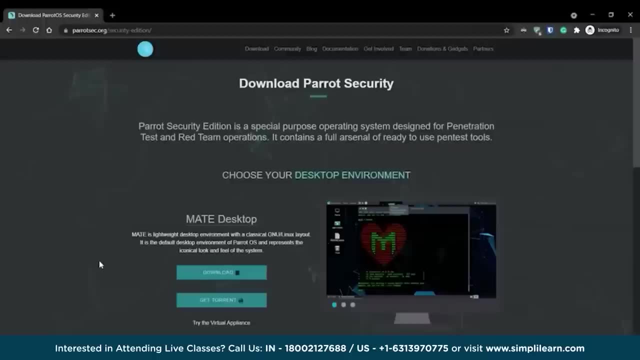 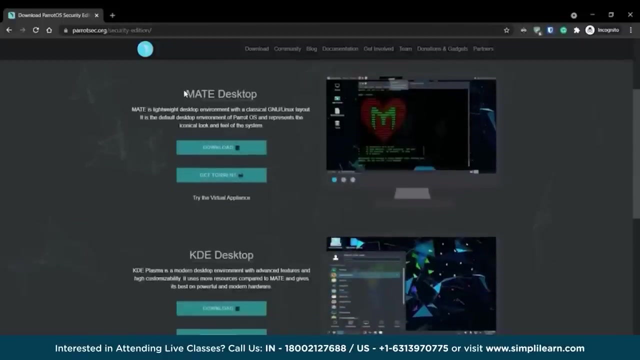 and select the Get Security edition over here. Barrett Security OS has multiple desktop environments for you to choose from. These desktop environments serve as a different user interface for the user. For example, right now we have the Mate desktop and the KDE desktop, As you can see from the screenshots. 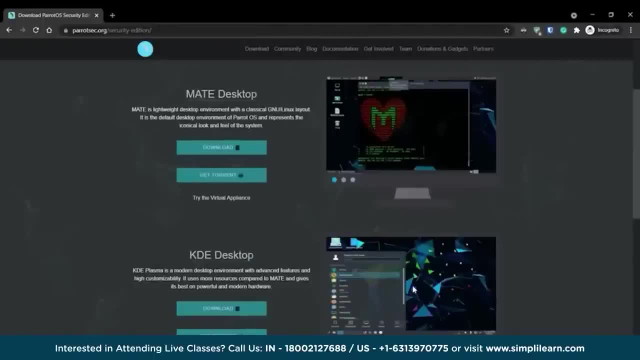 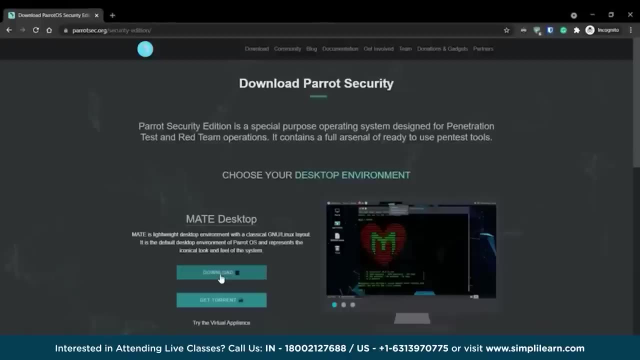 both of these look quite different while having a similar look and feel to them. For our example, let's go with the Mate desktop. We have two options: either we can go with the direct download or we can get the torrent file, For this example. 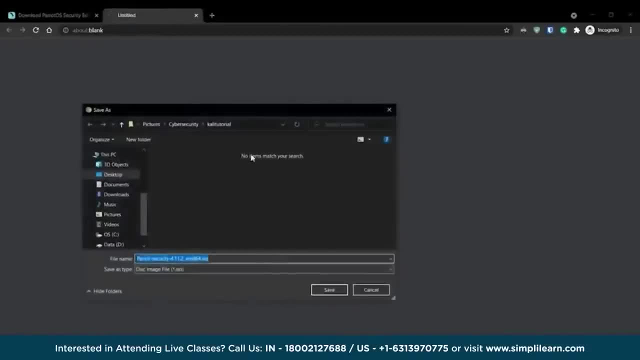 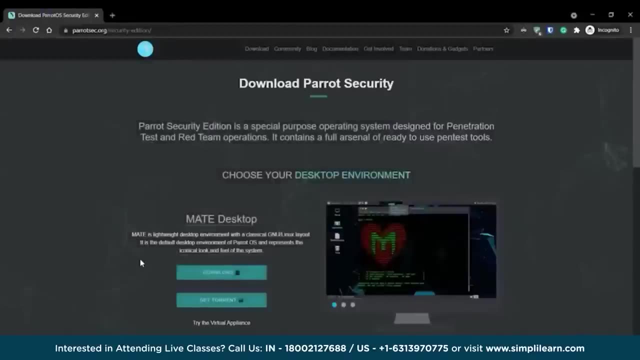 if we press on the download button and our download will start. I have already downloaded this file, but the ISO file provided over here will serve as an installation. It will have around 4.5 GB of space. It will be used to install this operating system in VMware. 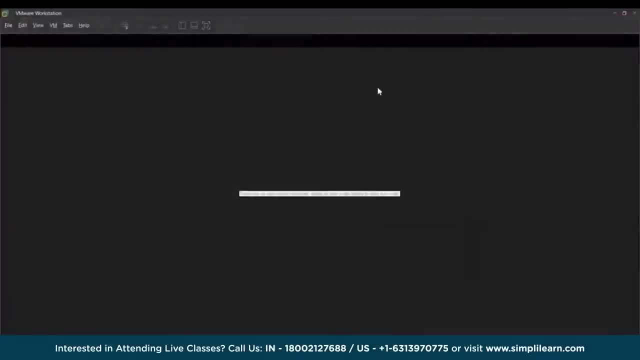 Once the file is downloaded, we can close this and open VMware Workstation. VMware can also be used as a player version or the workstation version. If you have much more familiarity with using VirtualBox for virtualization application, we can use that as well. 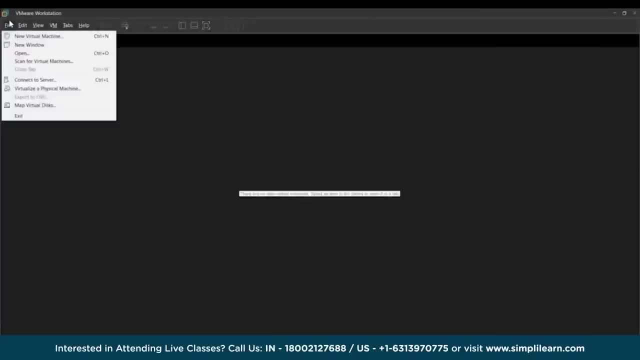 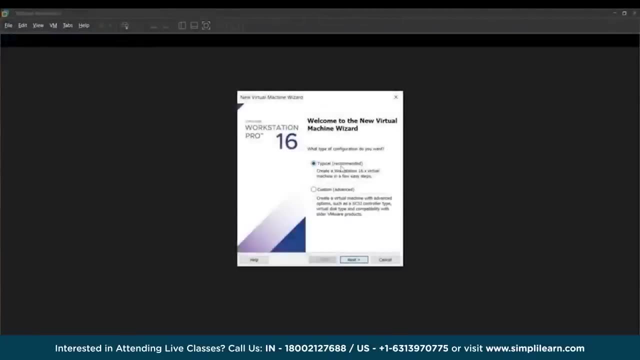 Once the VMware is opened, we click on File and select a new virtual machine For the first time installation. we're going to go with the typical and recommended installation procedure instead of an advanced one If you have already installed multiple virtual machine OSes. 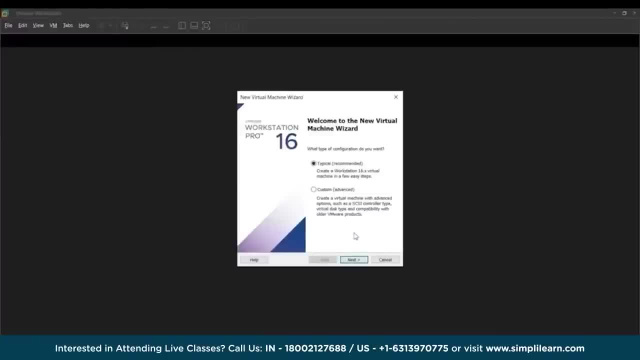 going with the advanced option will give you much more control over the hardware customization, But for now we're going to stick with the typical option. Moving on, it will ask us for a source to where to install the operating system from, Since we're going to use a live ISO first. 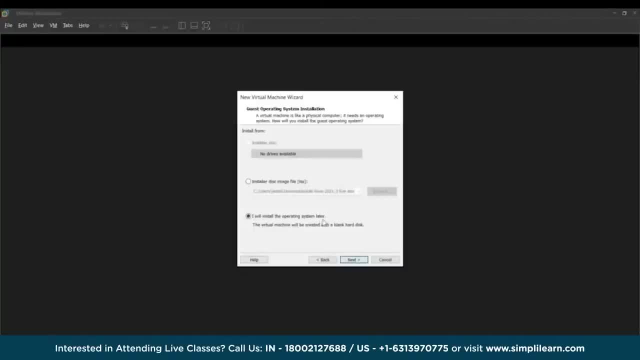 we're going to select the third option, which will be- I will install the operating system later and press Next. As we already know, Parag Security is a Debian derivative, So when selecting the guest operating system type, we're going to go with Linux. 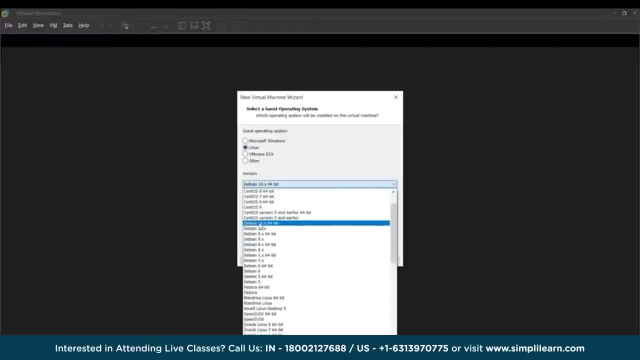 And in this selection, we're going to choose whichever the highest version of Debian is, along with a 64-bit OS We're going to click on. Next, We're going to name our virtual machine, let's say Parag Security OS. 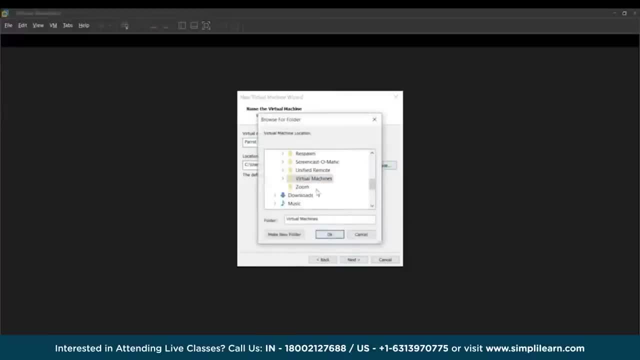 We're going to select the location where we want to save the virtual machine. This will have all the hard disks of the operating system installation. We're going to click on Next For the disk size. we're going to specify how much of the current memory are we going to allocate. 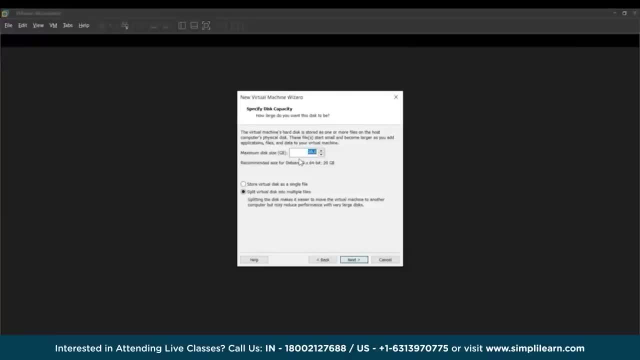 This is the hard disk memory of the operating system installation. Whatever changes we make in the operating system, whatever applications we install on the virtual instance, will all be stored in this amount of memory, While it is recommended to go with at least 15 GB of storage. 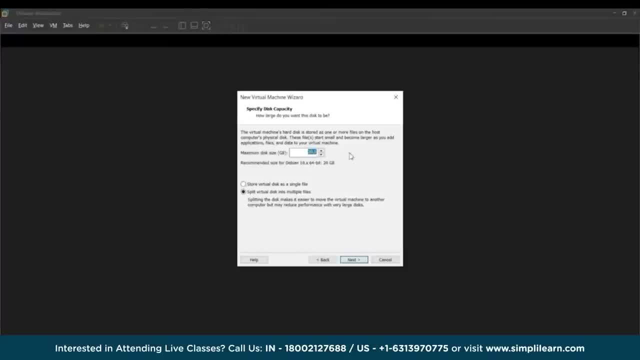 we can go as high as possible And we're going to select the recommended 20 GB. as written. When given the choice of storing the virtual disk as a single or multiple files, many people want to keep their virtual instance in a way so that it helps them stay portable. People change systems and sometimes they want to swap their instances between the work and their personal computer. If there is no portability in mind, storing the virtual disk as a single file gives the best performance and should be the recommended go-to when installing for the first time. 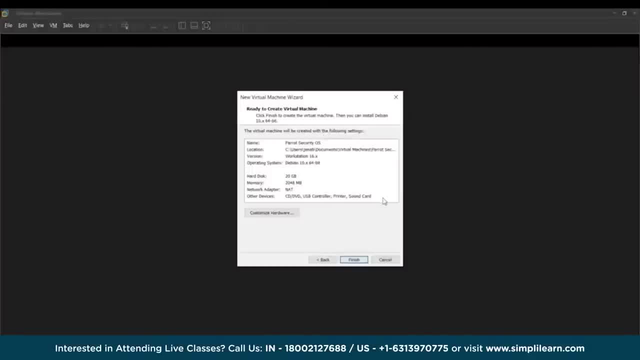 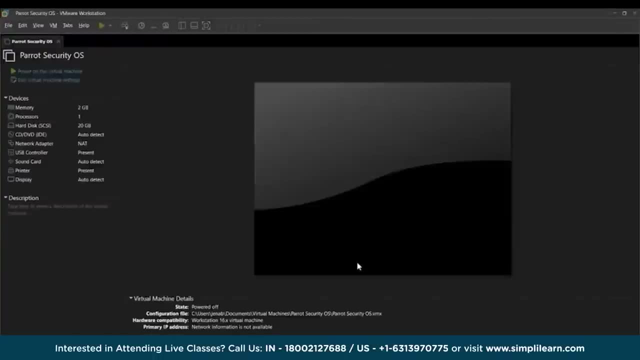 We click on Next here and it's going to give us a summary of the settings we have already settled till now. We're going to press on Finish And there we go. We have our installation first step completed Here on out. we're going to click on Edit Virtual Machine Settings. 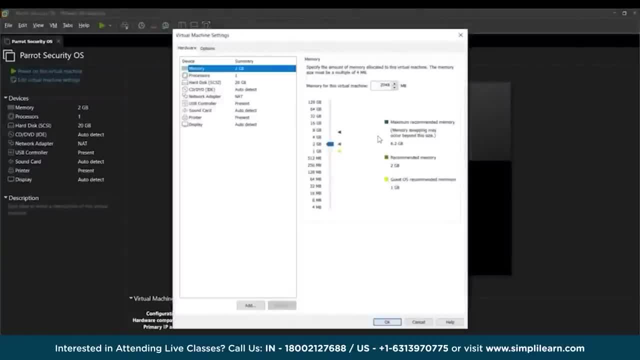 Here we're going to have a look at some of the requirements that the Parag Security OS will need. It is known to be a memory lightweight operating system, But just to have the most optimum performance we're going to provide around 2 GB of RAM. 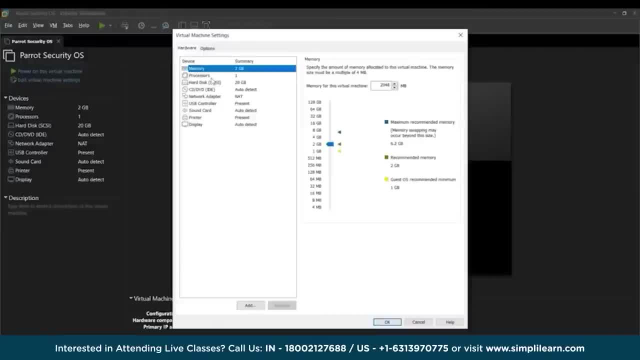 from our host system, which is a Windows 10 machine. When it comes to the processors, I'm going to increase it to 2, and the number of cores to 2 as well, So giving out a total 4 processor cores to the operating system. 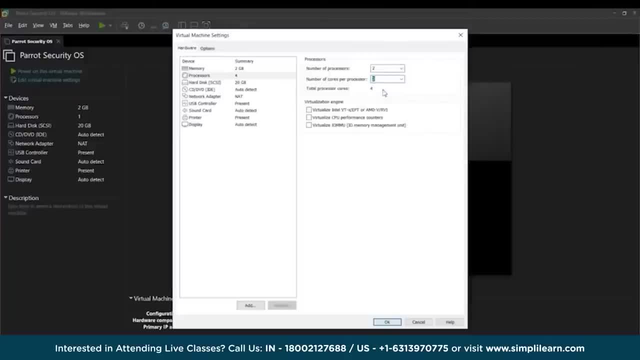 Now this depends on what are your computer rig and how much resources you can justify, So these need to be customized according to the system at hand. Hard disk size has already been set at 20 GB and the rest of them are pretty standard, and we can go on. 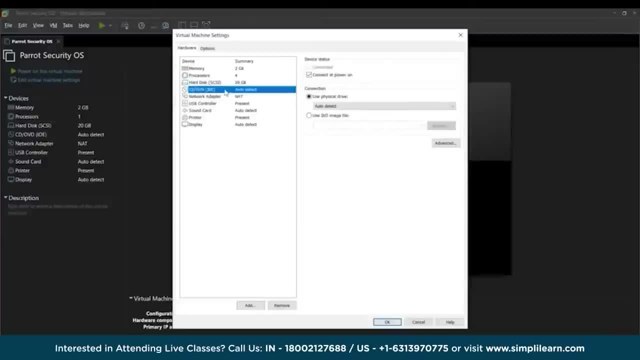 One thing that we need to make sure is selecting the CD, DVD, IDE. Here we have to use our ISO image file over here. Previously it should be used physical drive and at auto detect. We're going to use a used ISO image file over here. 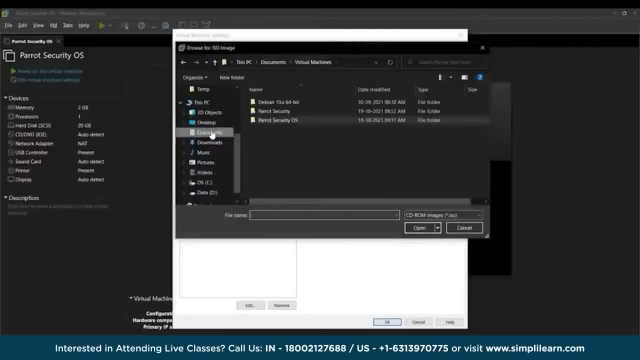 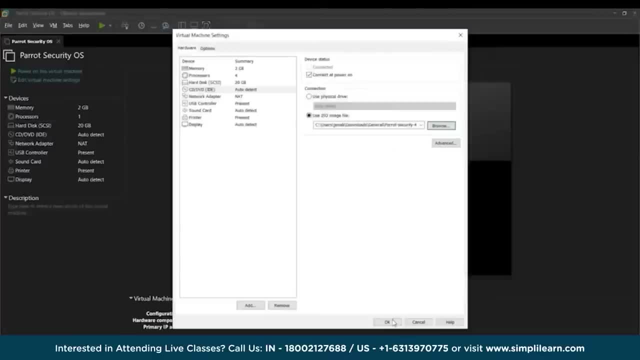 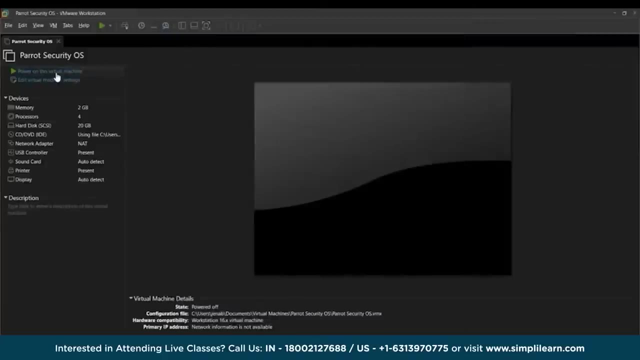 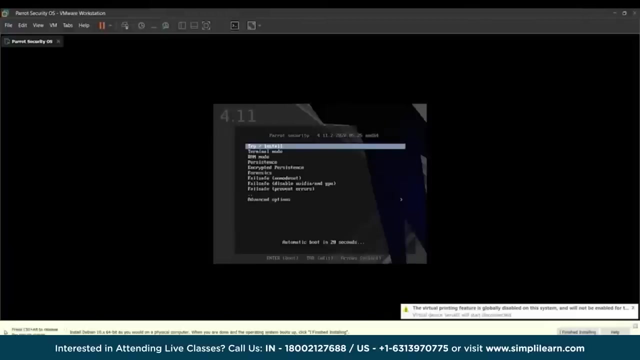 We're going to click on Browse, We're going to go to where we have downloaded the ISO file, which is over here, And select it, Press OK here And we can now power on this virtual machine. At this point of time, there are two options. 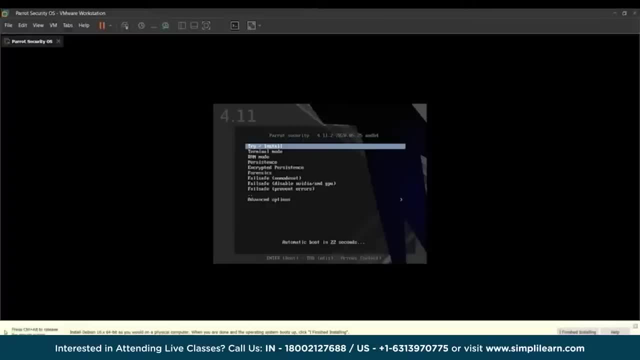 We can go with the try install option using the graphical user interface or we can go using the terminal mode To get a better user experience. we're going to go with the try install mode, specifically Press Enter And it's going to start the live boot ISO. 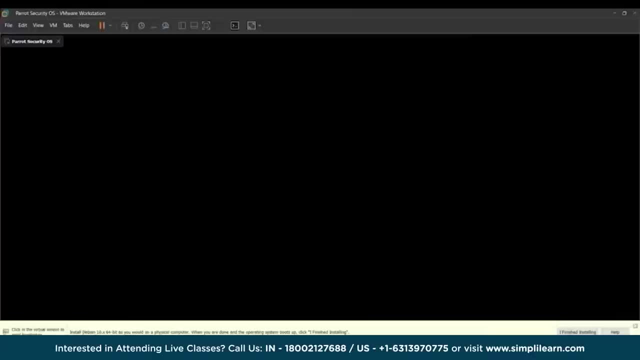 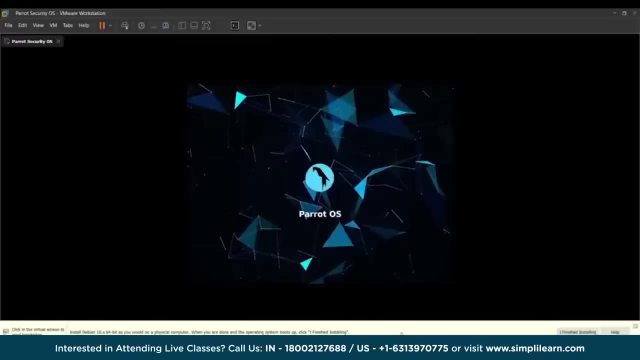 Meanwhile, VMware has a prompt over here where it will try to install some VMware tools on it. While this is not mandatory, it is much more recommended to install these tools so that we can get some additional features like drag and drop with the host system. 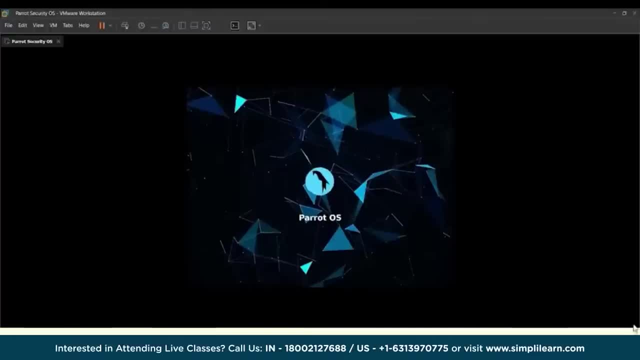 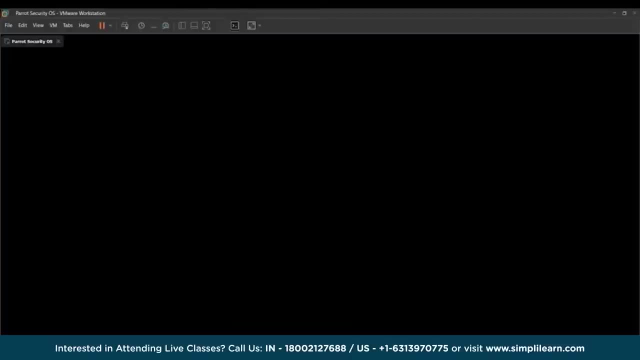 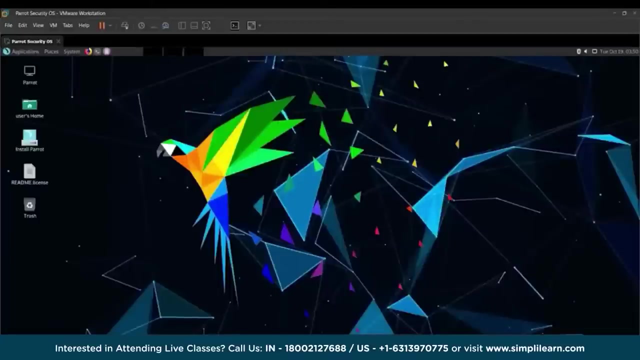 and many more things. For now we're going to close this prompt. As you can see, this is the live boot ISO of the Barrett Security Operating System. Currently it's running the Mate desktop as we have downloaded in the website. Live boot ISO is necessary. 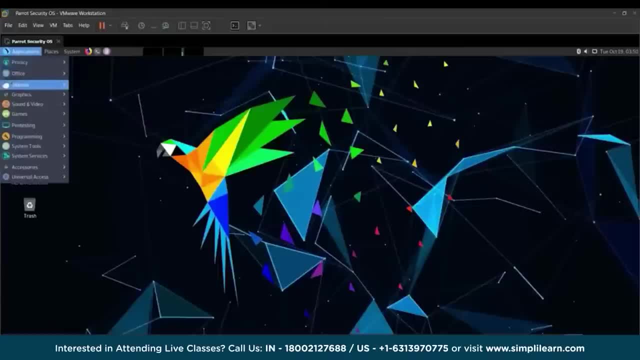 to get a good feel of the operating system. There are many good Linux distros that have this live boot option so that you can give a try of the operating system before installing it permanently. Once you're into the live boot, we can start up with the installation. 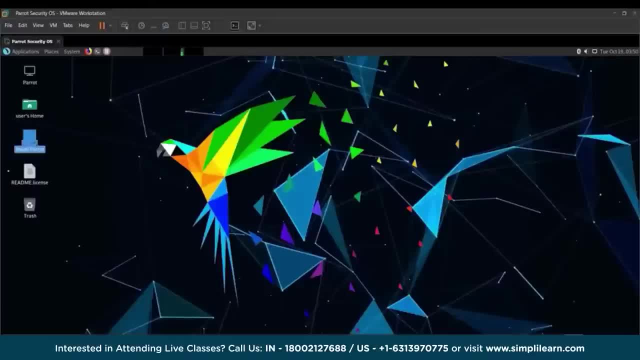 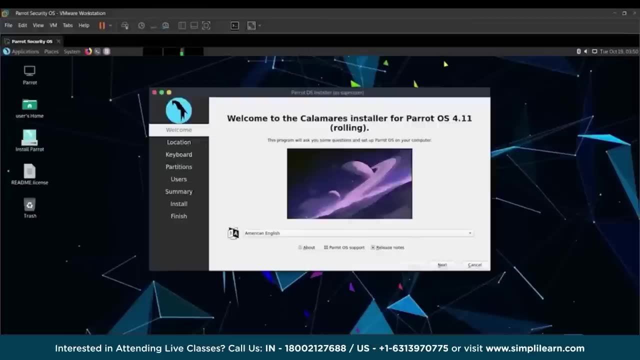 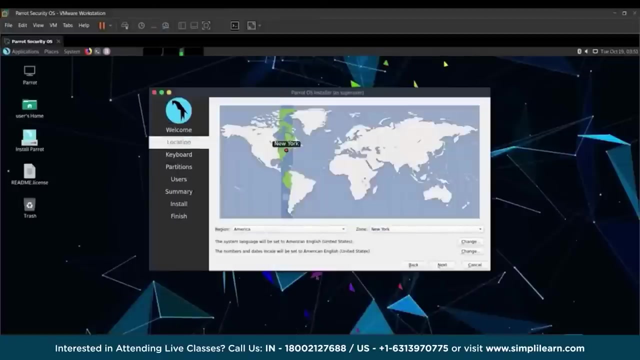 using the shortcut, as you can see. install Barrett. We're going to double click it And this is a Calamares installer. Choose your language as American English And press next. You can select your time zone according to your location. 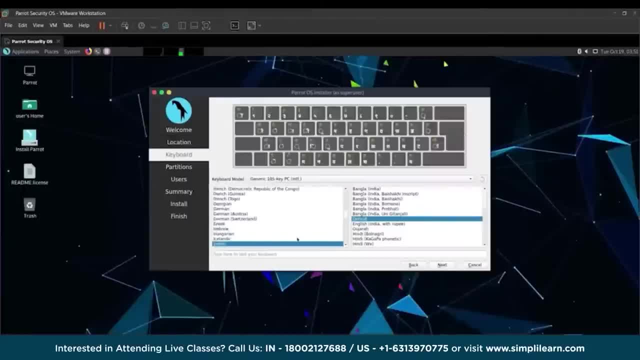 And we can go next. At this point of time, you have to choose the correct keyboard. Now, what many people get confused is choosing their own language keyboard. What people must keep in mind is what keyboard the laptop provides. Most of the systems that come pre-built. 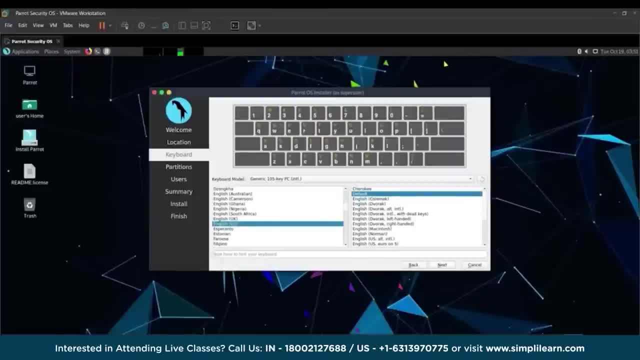 provide the English US keyboard. So, whatever keyboard you choose, make sure to type here and test that all the buttons, including the superscript and the subscript buttons, are working correctly before moving forward with this step. Once you've settled on the keyboard that you need to install, 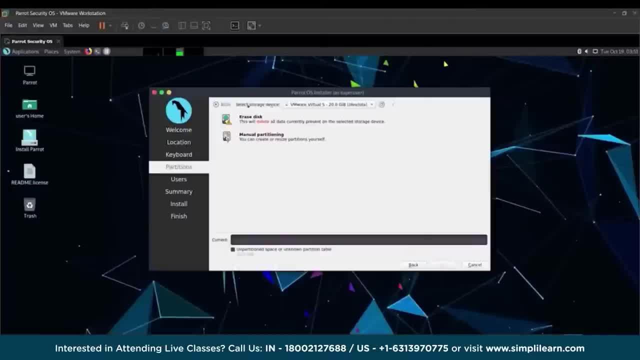 you can go ahead Here. it will ask you to select storage device And the only option you're going to get is the amount of hardware storage you have given in the virtual machine settings. We have already provided 20 GB of storage. We're going to choose that. 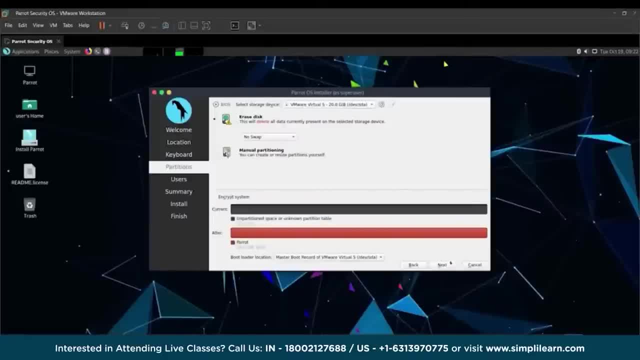 And we're going to erase this disk. Manual partitioning can be useful when you're going to install Parallel Security on an operating system or on a hard disk where it is already including a Windows OS. For now, we're going to select: erase disk. 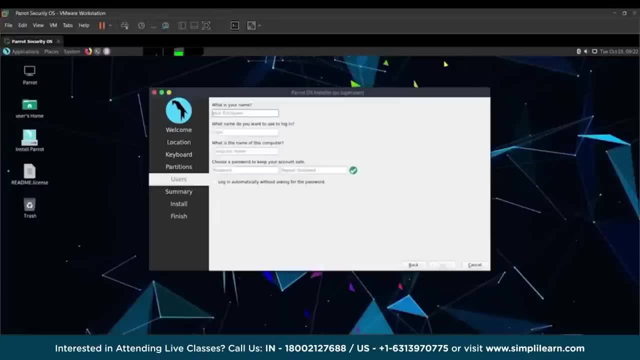 and press next. We're going to give our full name. Let it be simply learn. You can give the name of the computer and this is the username which we will use to log in. This is your root password that we're going to give over here. 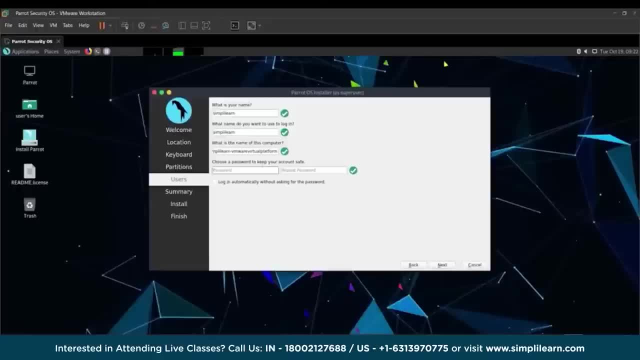 The root password of this Kali Linux will act as an administrative access and it will be necessary for making changes to the system or installing and updating software. Enter the password and repeat it over here. You have the option to log in automatically without asking for the password. 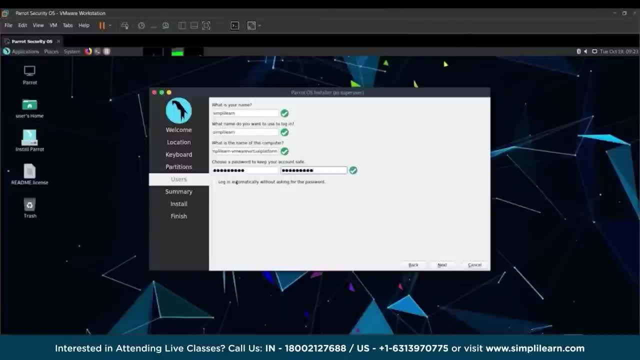 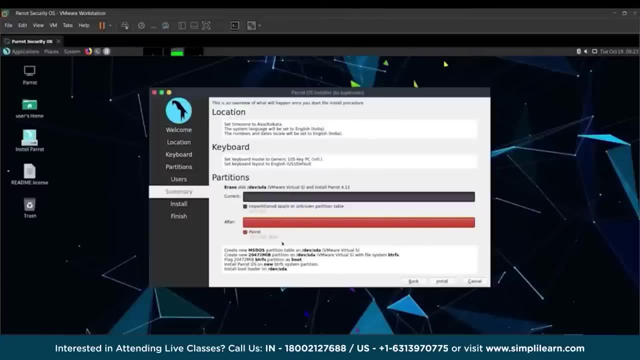 But for security purposes, it is recommended to keep this disabled. Click on next. This is another summary of the installation that we're going to move forward with. Have a look that whatever changes we have made is according to your requirements, and, once everything is checked, 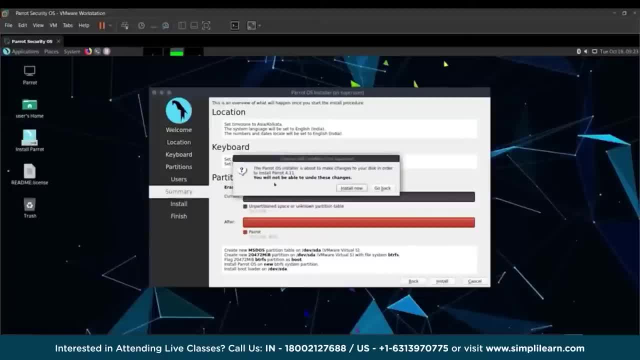 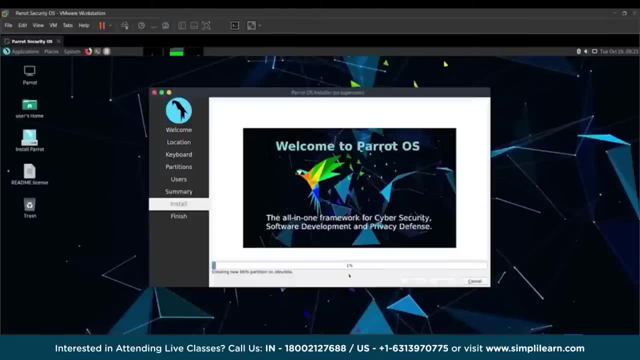 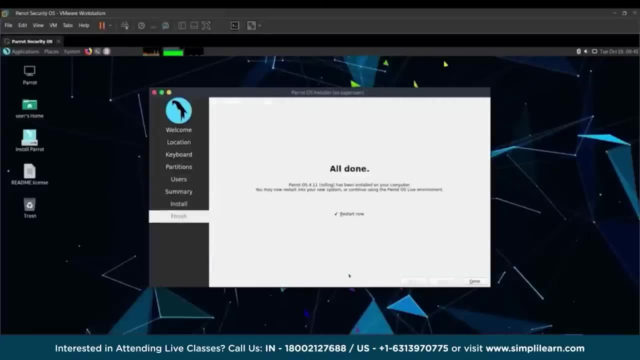 we can press on install. Click on install now And we're going to let it complete the work. As you can see, the installation of Parallel Security is now completed. We're going to make sure that we have the restart now button over here disabled. 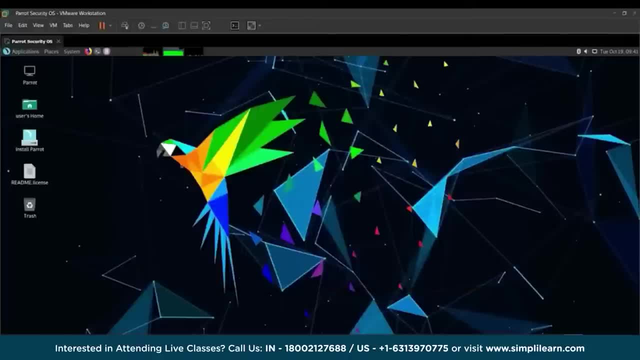 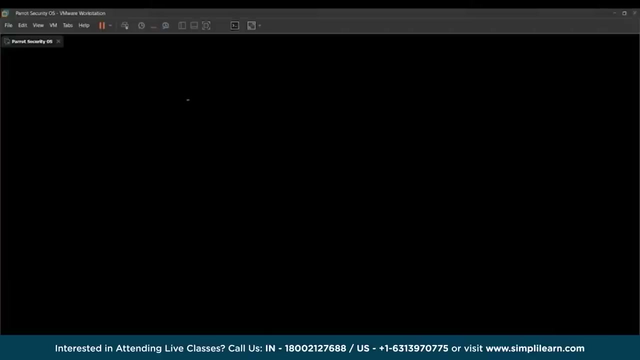 I'm going to click on done. We're going to shut down this live boot ISO. We're going to click on menu, Turn off the device And shut down. We're not restarting straight away because, if you remember correctly, in the virtual machine instance settings. 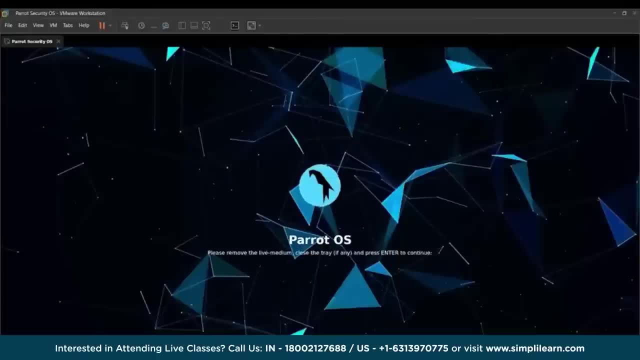 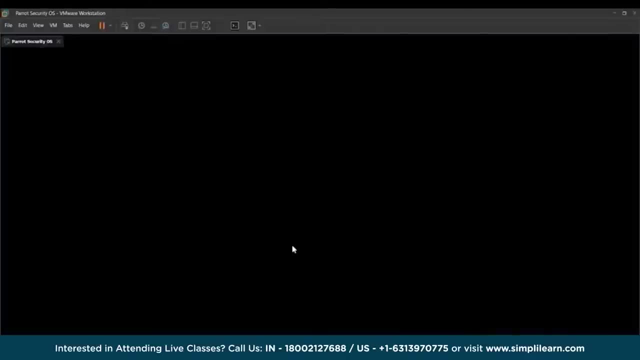 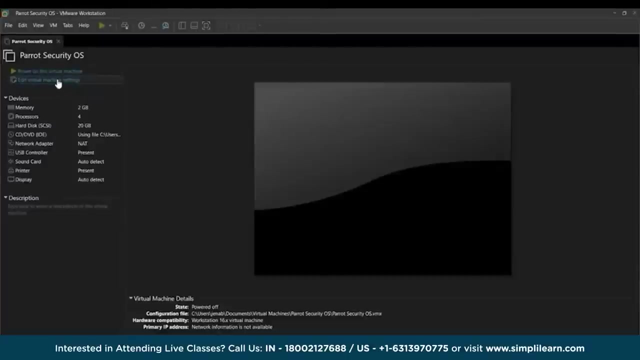 we had given it an ISO file. Please remove the live medium and press enter to continue. We can just press enter to continue And it's going to shut down. Now, to move on, we're going to click on edit virtual machine settings. 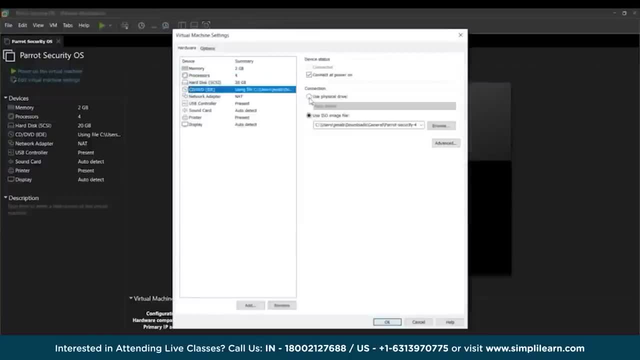 We're going to CD, DVD and we're going to use physical drive. now We're going to remove it from the ISO image file because installation has already been completed and we don't want to use the same ISO file again and again By using physical drive over here. 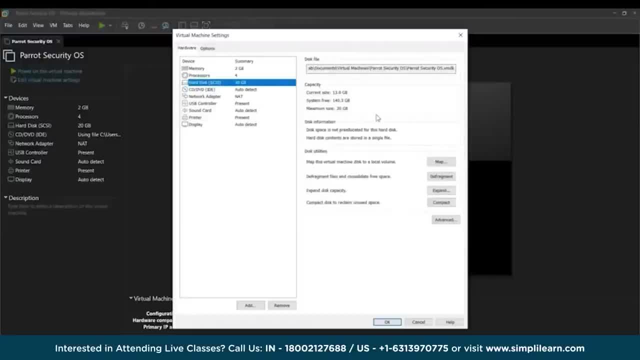 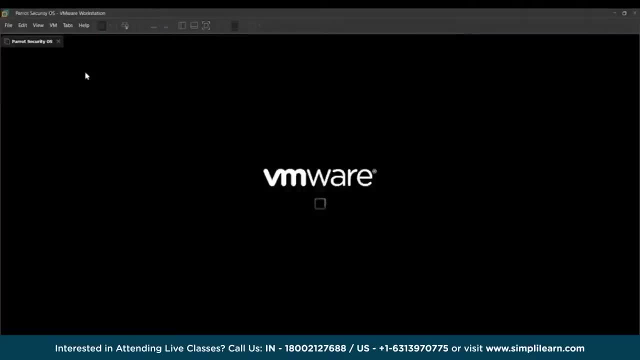 it's going to detect the 20 GB hard disk that we have already provided and installation is done on it. We're going to press OK And we're going to power on this virtual machine for testing. Make sure this: you click ES over here. 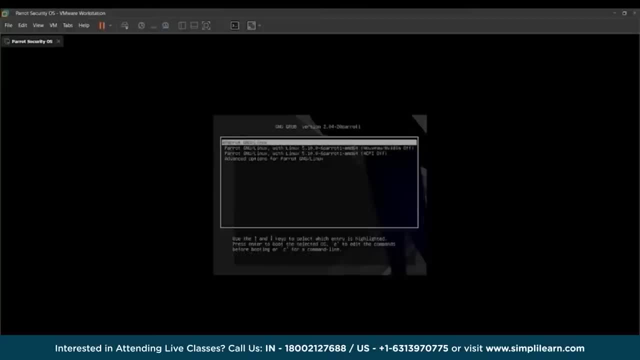 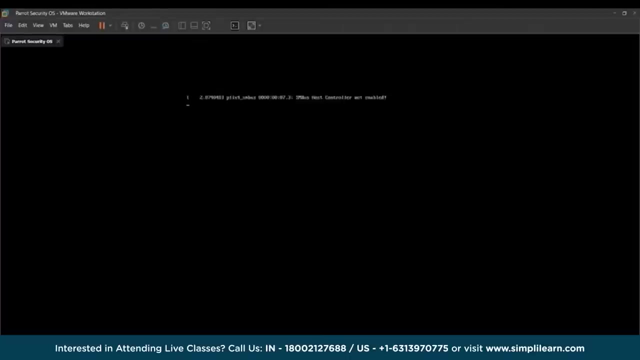 This is the grub menu. At this we get different choices, for example, which NVIDIA drivers off or with some other advanced options. More often than not, we're going to choose the first option and press enter. If you remember clearly, we did not get the option of try install. 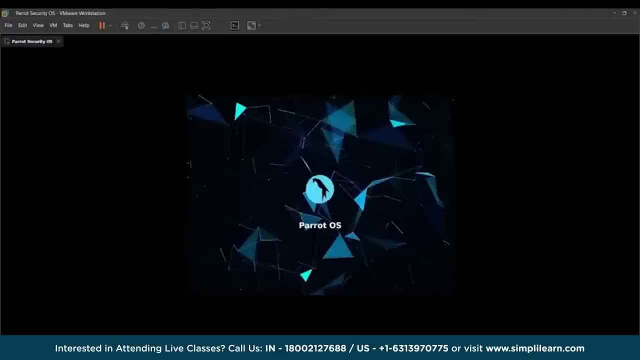 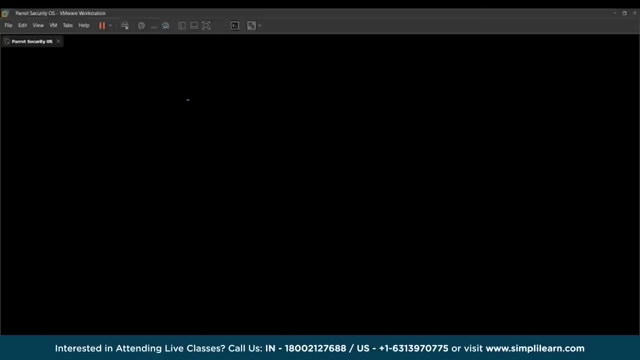 or a terminal run, just like we did in the live boot ISO. Since this is running straight from the 20 GB hard drive storage, it's going to start the OS directly. Now with the login screen, you can see our username over here. 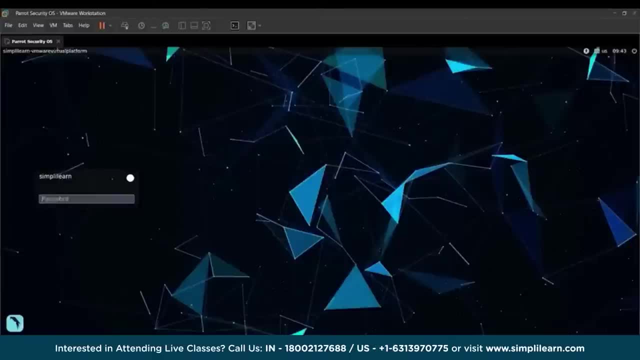 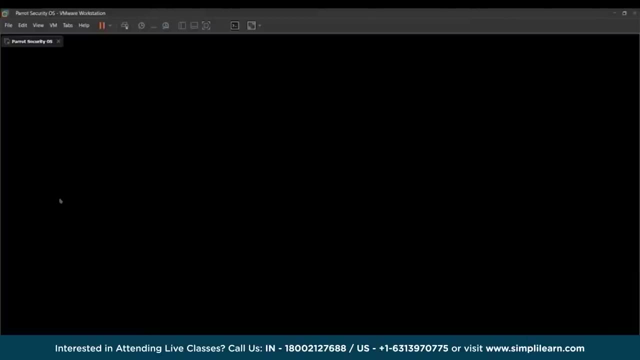 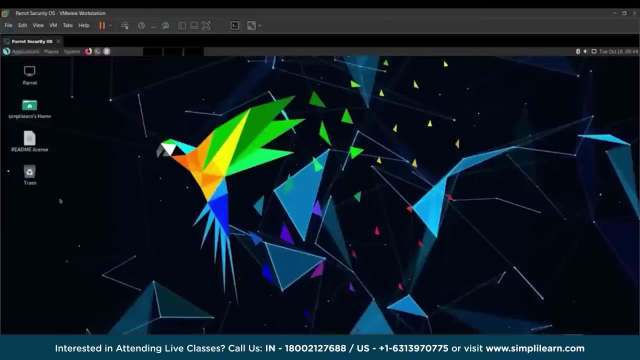 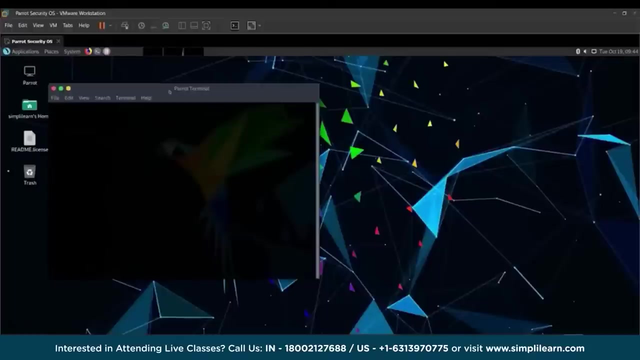 as we provided in the installation. We're going to enter our root password and press enter, And this is our currently working desktop of the Parallel Security Operating System. We can open the terminal over here And we're going to try our root password and installation. 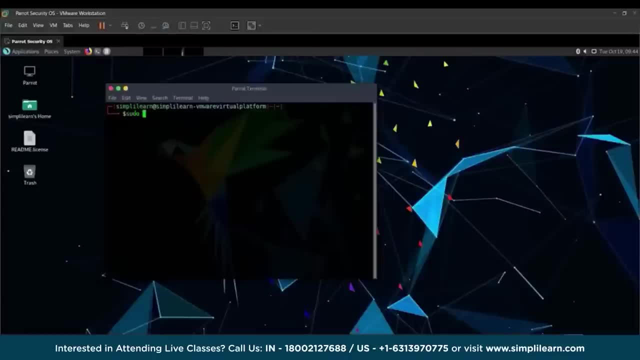 To install any software. we're going to use the keyword sudo and we're going to try the keyword sudo, apt install and neo fetch. We're going to use the root password that we used to log in. We're going to press Y for yes. 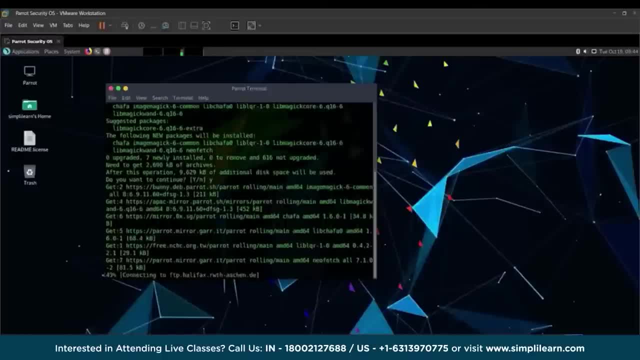 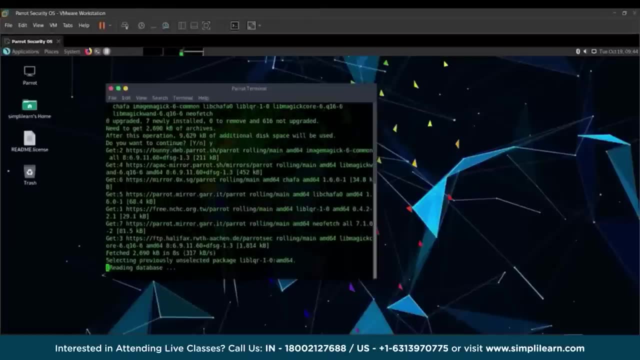 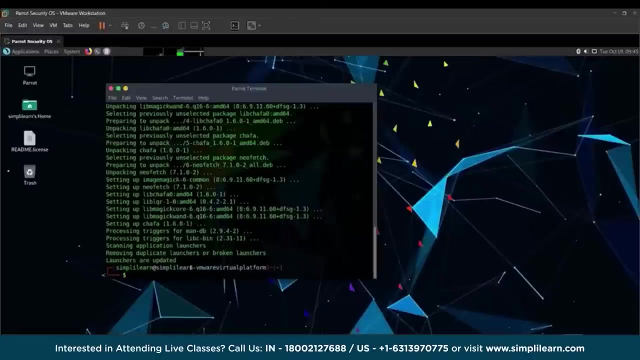 This is just an additional step that we're doing to check that the installation is done correctly with the correct amount of hardware requirements that we had provided We can try to install it. Now that we have installed neo fetch, we can write the command neo fetch. 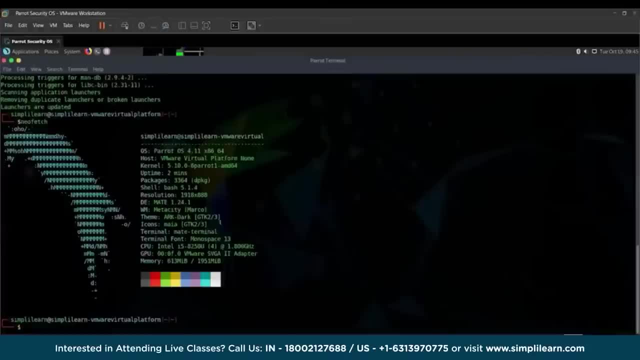 And this is going to give us some information about our installation. You can see the OS name as Parrot OS 4.11 is running on a VMware host. So the kernel versions and some of the other information, like the number of packages installed. 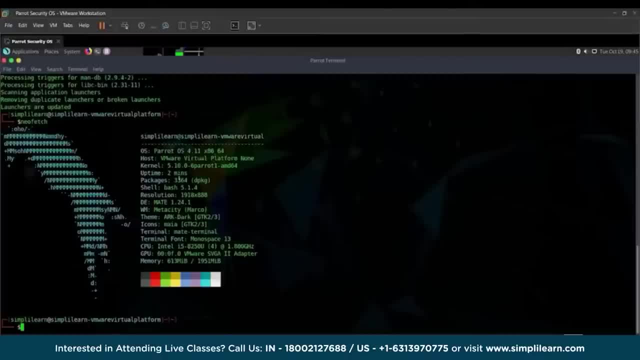 the current shell version, the number of tries. We can also see installed the current shell version, resolution of the VMware instance that we are running, the desktop environment which is made as we had downloaded once, and some other things. You can see, the memory is supposed to be 1951. 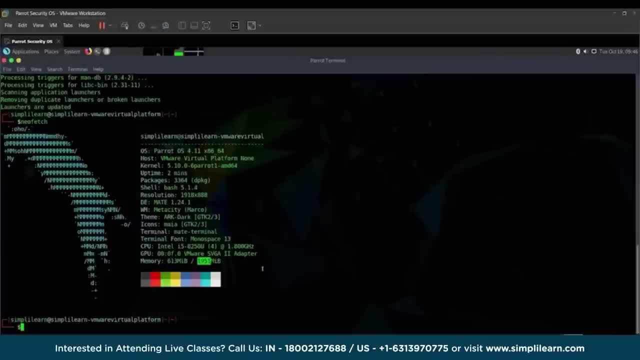 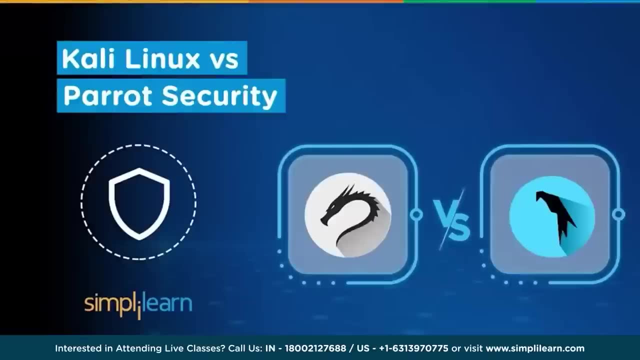 megabytes, which is supposed to equal around 2 GB of RAM usage that we had provided. Kali Linux and Parrot OS are two popular penetration testing distributions. While these operating systems each have unique offerings, the overall choice can differ between personnel thanks to their 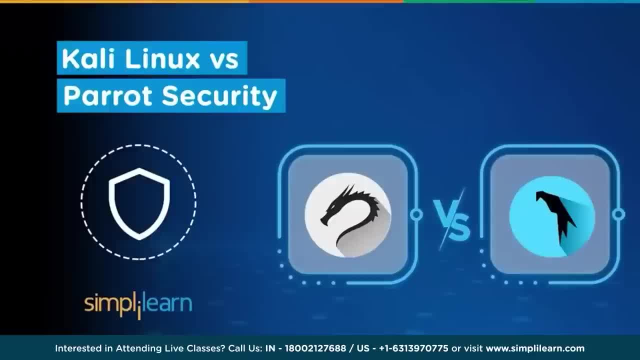 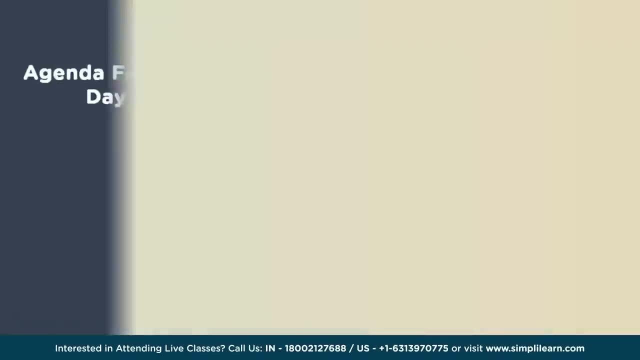 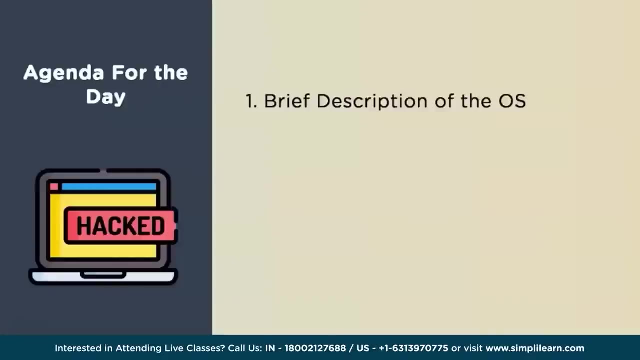 various tools and hardware specifications. Today, we will look at both these distributions and settle on the perfect choice for each type of user. Let's go through the agenda for this video. We will learn about Kali Linux and Parrot Security OS from scratch, while understanding their primary. 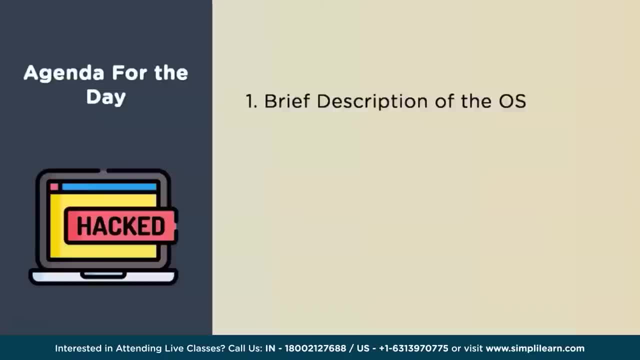 selling points as a Linux distribution catered towards penetration testers. Next, we know about some features of these operating systems that stand out of their package. Finally, we directly compare Kali Linux and Parrot Security OS, thereby making a clear-cut conclusion on which OS is. 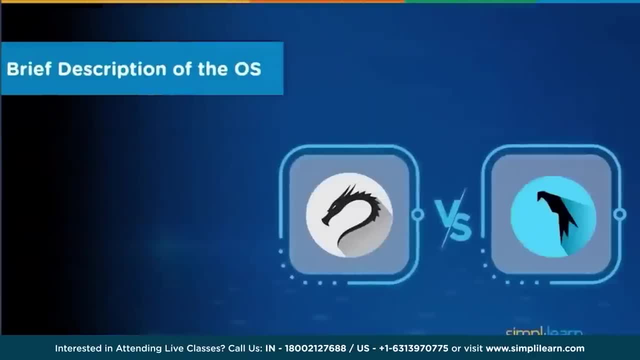 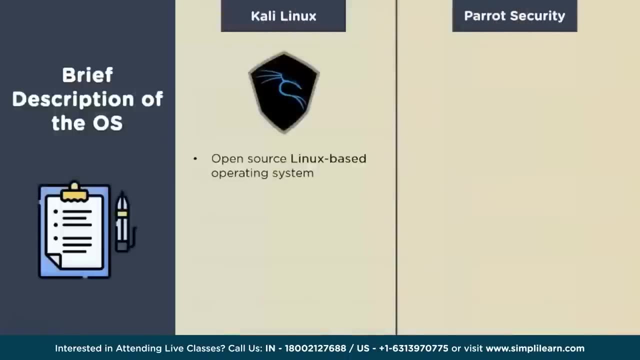 perfect on a per requirement basis. So let's start by learning about Kali Linux from a ground level. Kali Linux, which is formerly known as Backtrack Linux, is an open-source Linux distribution aimed at advanced penetration testing and security auditing. It has several hundred tools targeted towards various information. 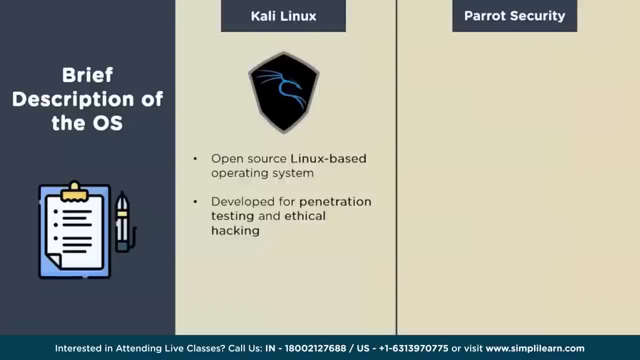 security tasks such as penetration testing, security research, computer forensics and reverse engineering. Kali Linux is a multi-platform solution accessible and freely available to information security professionals and hobbyists. Among all the Linux distributions, Kali Linux takes its roots from the Debian. 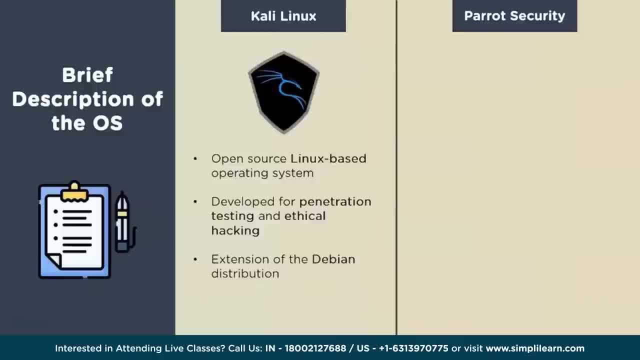 operating system. Debian has been a highly dependable and a stable distribution for many years, Providing a similarly strong foundation to the Kali Linux desktop. While the operating system can practically modify every single part of our installation, the networking components of Kali Linux come disabled by default. This is done to prevent any external 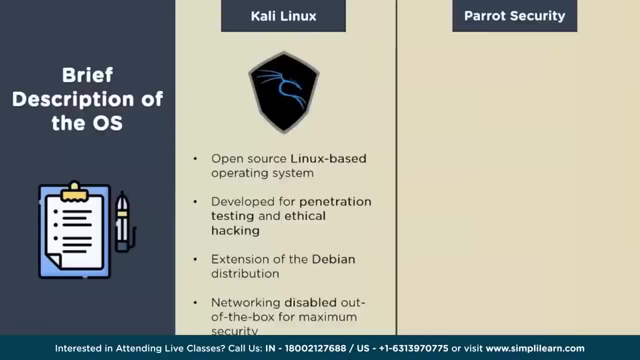 factors from affecting the installation procedure, which may pose a risk in critical environments. Apart from boosting security, it allows a more profound element of security control to the most enthusiastic of users. Now let's take a look at Parag Security operating system, Parag. 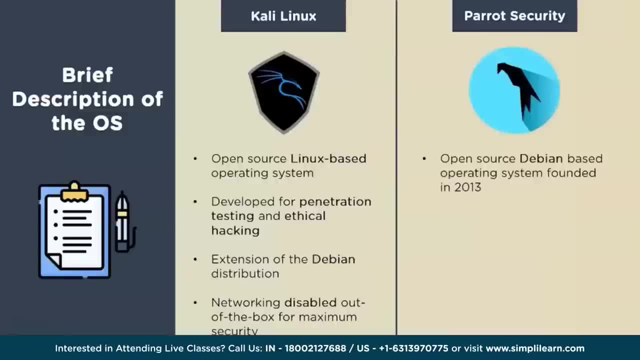 Security OS is a Debian-based Linux distribution with an emphasis on security, privacy and development. It is built on the Debian's testing branch and uses a custom-hardened Linux kernel. Parag Security contains several hundred tools targeted towards tasks such as penetration testing, computer forensics, reverse engineering and. 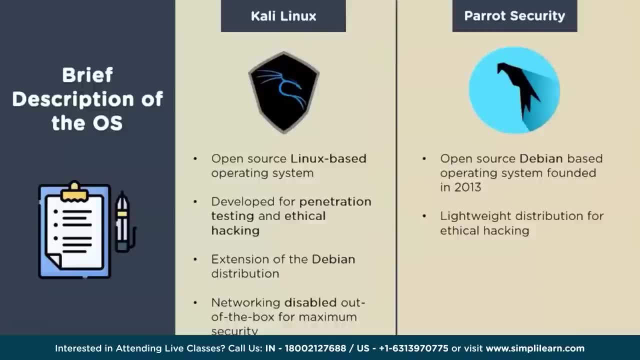 security research, It is seen as a generally lightweight distribution that can work under rigorous hardware and software specifications. It features a distinct forensics mode that does not mount any of the system's hard disks or partitions and has no influence on the host system, making it much more stealthy than its regular occurrence. 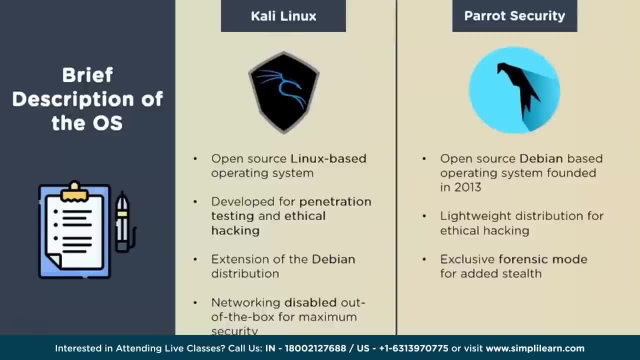 This mode is used on the host system to execute forensic procedures. A rolling release is a paradigm in which software upgrades are rolled out constantly Rather than in batches of versions. in software development, this ensures that the software is constantly up-to-date. A rolling release distribution. 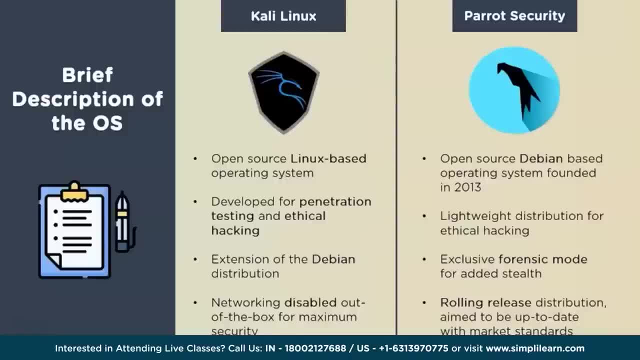 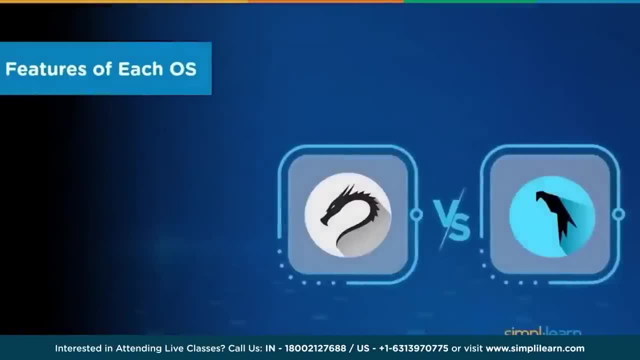 such as Parag Security OS, follows the same concept. It provides the most recent Linux kernel and software versions as soon as they become available, With a basic introduction to the operating systems. out of the way, let us take a look at the unique features of both Kali Linux. 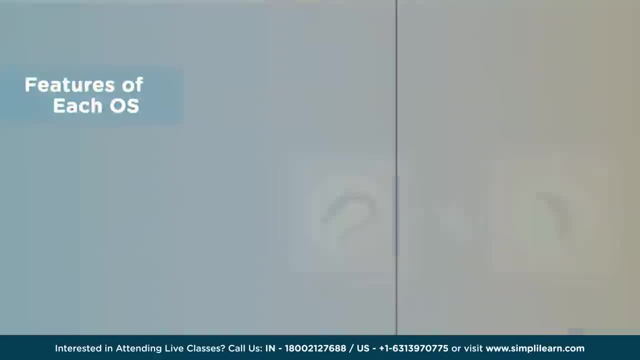 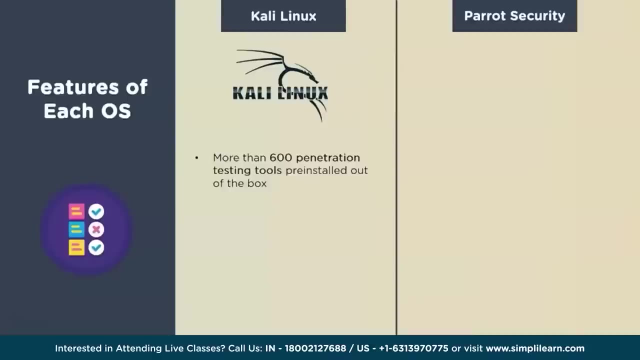 and Parag Security OS. The latest version of Kali Linux comes with more than 600 penetration tools pre-installed. After reviewing every tool included in Backtrack, developers have eliminated a significant number of tools that either simply did not work or duplicated other tools that provided the same and similar. 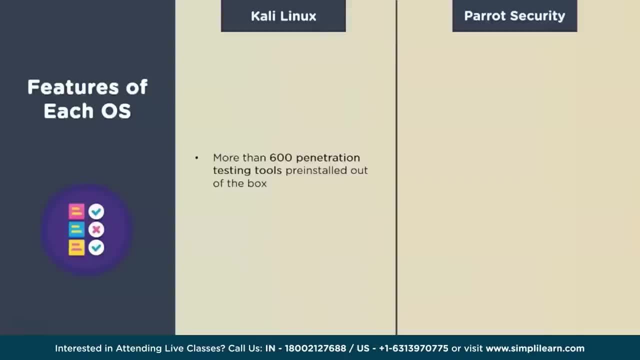 functionality. The Kali Linux team comprises a small group of individuals who are the only ones trusted to commit packages and interact with the repositories, all of which is done using multiple secure protocols. Restricting access of critical code bases to external assets dramatically reduces the risk of source contamination, which can cause Kali Linux users. 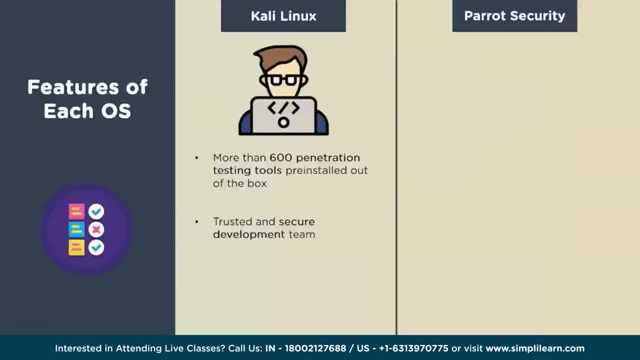 worldwide a great deal of damage as a direct victim of cybercrime. Although penetration tools tend to be written in English, the developers have ensured that Kali includes proper multilingual support, allowing more users to operate in the native language and locate the tools they need for their job. The more comfortable a user 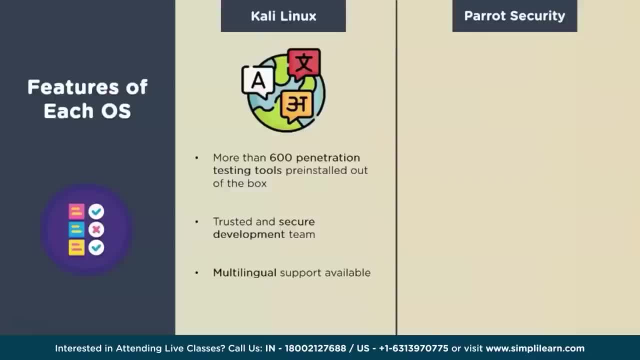 feels. with the intricacies of the operating system, the easier it is to maintain a strong hold over the configuration and the device in general. Since ARM-based single-board systems like the Raspberry Pi are becoming more prevalent and inexpensive, the development team knew that Kali's 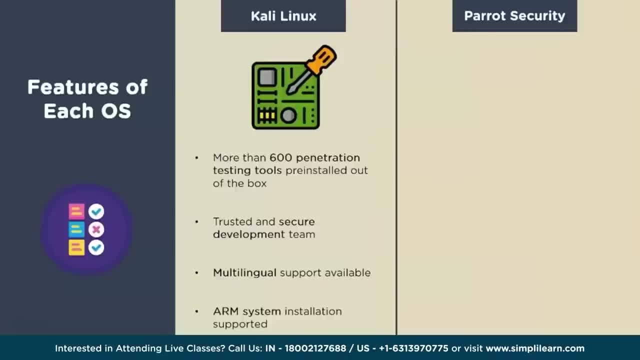 ARM support would need to be as robust as they could manage with fully working installations. Kali Linux is available on a wide range of devices and has ARM repositories integrated with the mainline distribution, so the tools for ARM are updated in conjunction with the rest of the 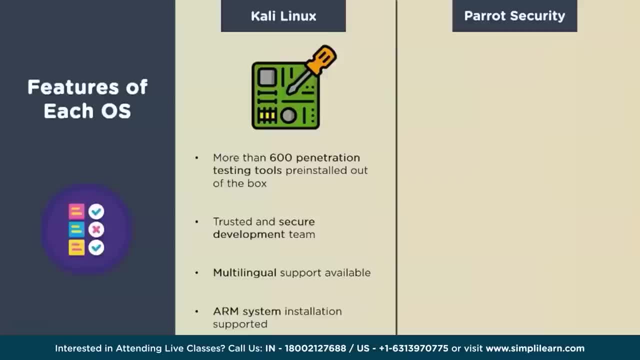 distribution. Let's take a look at some of the features of Parrot Security operating system now. Along with the giant catalog of scripts, Parrot Security OS has its own hardened Linux kernel, modified explicitly to provide as much security and resistance to hackers as possible. 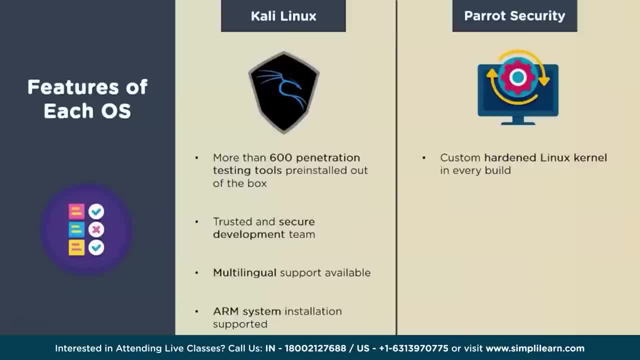 as possible in the first line of defense. The configurations in the operating system act as the second gateway, taking care of malicious requests and dropping them off. This is particularly beneficial since, should there be a scenario where the latex Linux kernel is causing some particular issue, the Parrot OS. 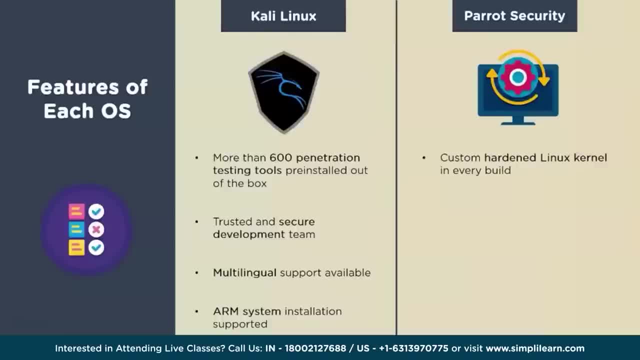 development team will most likely iron it out first before passing it on as an update. If the custom hard-nil kernel wasn't recent enough, Parrot Security OS's security developers managed to install more hacking tools and scripts to ensure a smooth transition for the Kali Linux users. 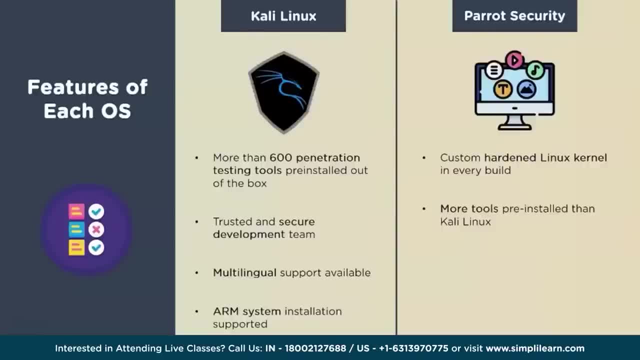 All the tools you find in Kali are present in Parrot OS, and a few extra ones for good measure, And this has been achieved while keeping roughly the same operating system size between both of them. However, it's not all. productivity points for Parrot OS. 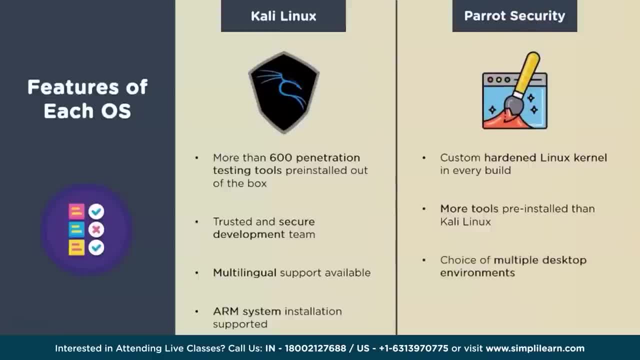 They provide a choice between two different desktop environments: MATE, which comes pre-installed by Parrot OS, and KDE. For those unfamiliar with Linux terminology, you can think of desktop environments as the main UI for a distribution, Being highly modular in nature. one can use Parrot Security OS, while 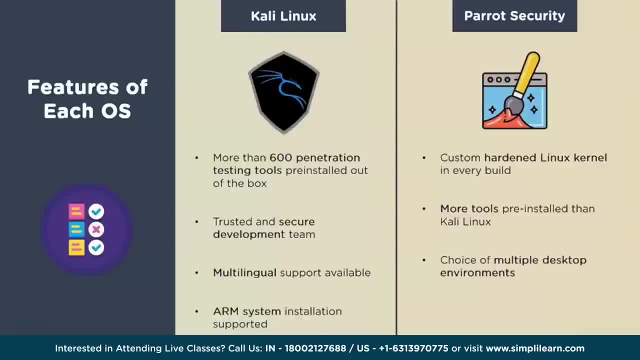 adding another desktop environment that they find appealing. While Kali Linux has only a single option, Parrot Security has provided two optimized builds with MATE desktop and KDE desktop. One of the primary advantages of Parrot OS is that it's easy to use. 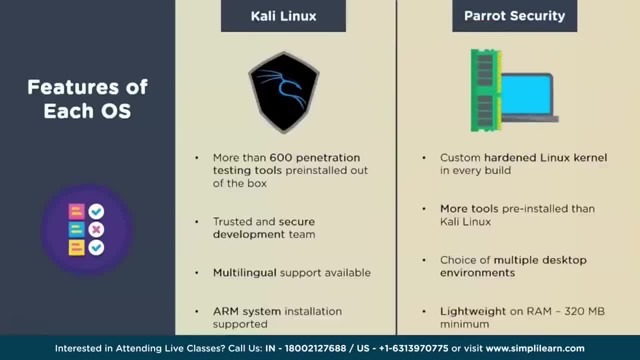 This implies that it takes significantly less disk space and computing power to function correctly, with as little as 320 MB of RAM required. In reality, Parrot OS is designed to operate successfully off a USB stick, but Kali Linux does not work well from a USB drive and is generally installed. 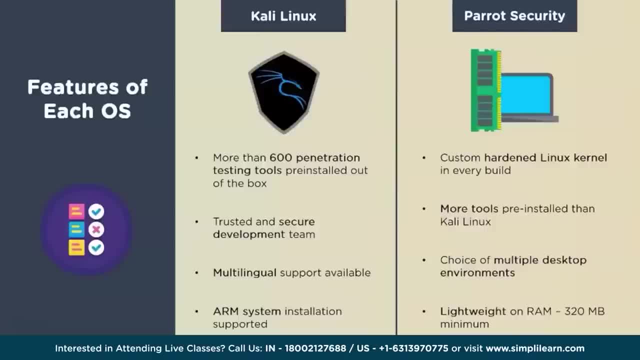 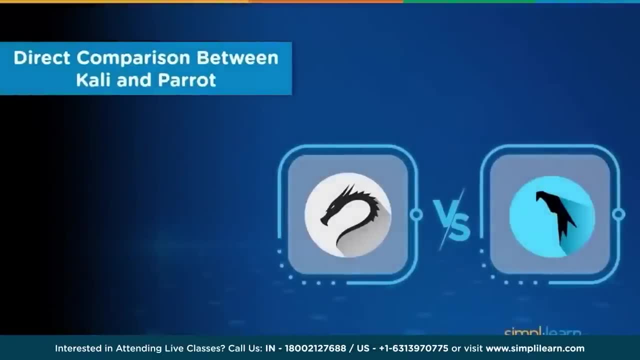 in a virtual machine. Parrot OS is more of a niche distribution if you're searching for something lighter than Kali Linux. Features are great, but what about performance? Real-world metrics? Let us compare both these operating systems directly with respect to their hardware specifications and usability. 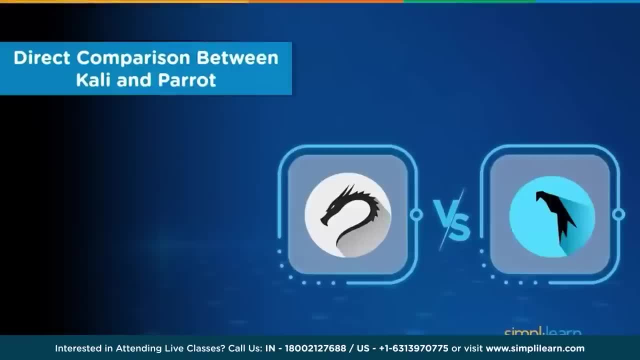 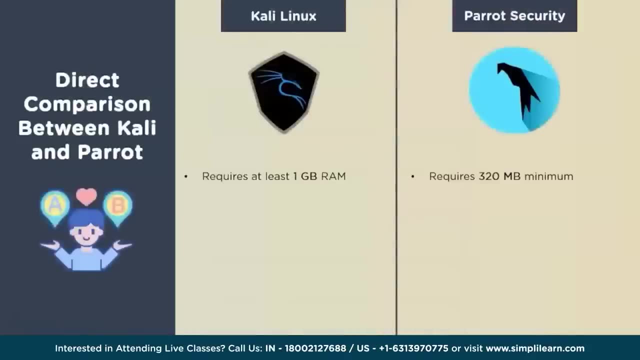 In the end, we can decide on what distribution is fit for each type of user. For the first point of comparison, let's take a look at the RAM required For optimum performance of the operating system system, which is highly essential when trying to crack hashes or something of similar nature. 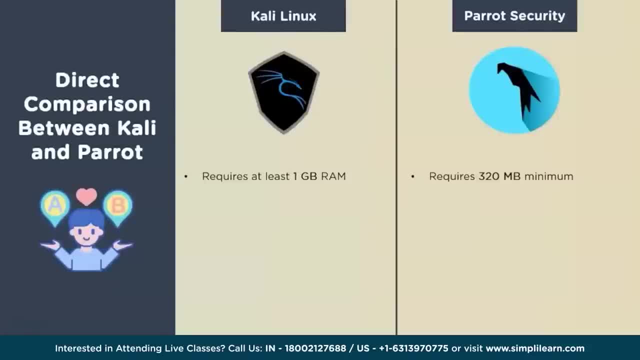 RAM usage is a very important facet. While Kali Linux demands at least 1 GB of RAM, Parallel Security can operate optimally with a minimum of 320 MB of RAM. For correctly displaying graphical elements, Kali Linux requires GPU-based acceleration. 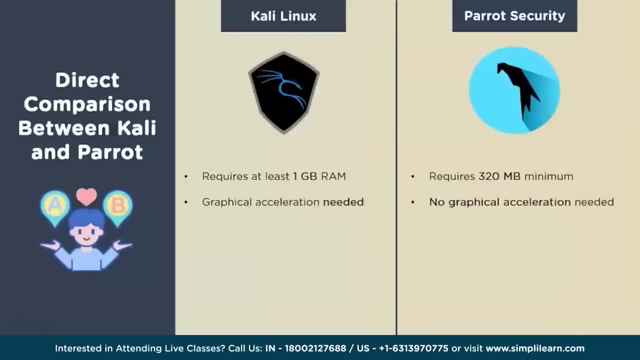 While this is not the case with Parallel Security OS, which doesn't require any graphical acceleration needed from the user side. Once these operating systems are installed on VMware using their LiveBoot ISOs, they take up a minimum amount of hard disk storage. Both of these 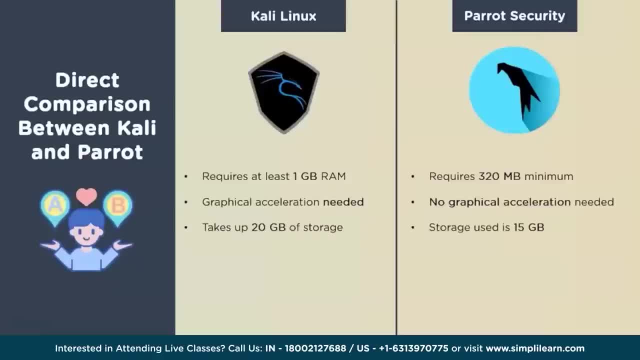 operating systems have a recommended disk storage of minimum of 20 GB in Kali Linux and a minimum of 15 GB in Parallel Security, so they can install all the tools necessary in the ISO file. When it comes to the category and the selection of tools, Kali Linux has always been the first. 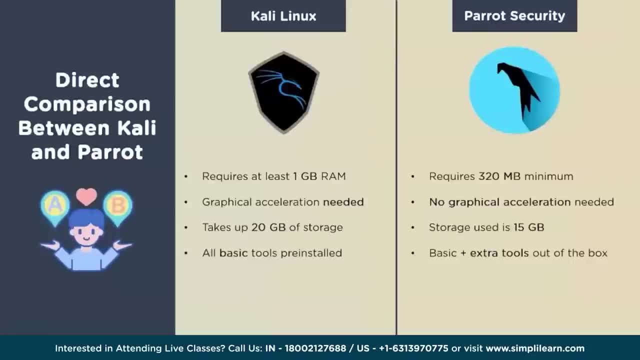 in securing every single tool available for hackers in the penetration testing industry. Parallel Security, on the other hand, has managed to take it up a notch. While specializing in wireless pen testing, Parallel Security makes it a point that all the tools that Kali Linux provides has been included in the ISO. 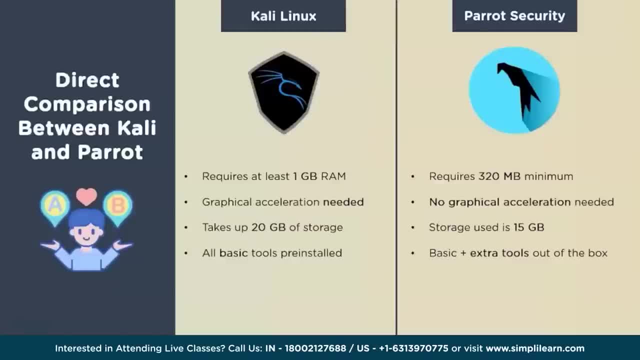 while simultaneously adding some extra tools that many users will have to install from third-party sources in Kali Linux. Being a decade-old penetration testing distribution, Kali Linux has formed up a very big community with strong support signatures. Parallel Security, on the other hand, is still growing and it is garnering much more interest among veteran 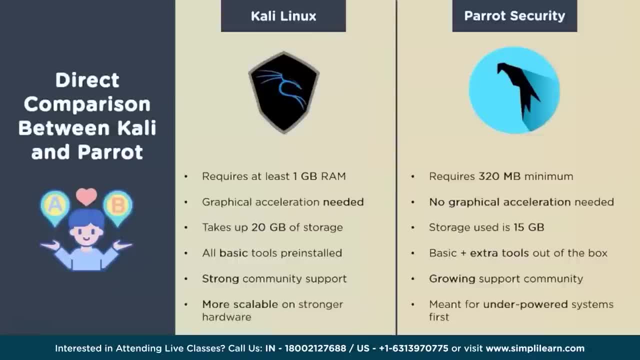 penetration testers and ethical hackers. A primary drawback of Kali Linux is the extensive hardware requirements. To perform optimally, it requires higher memory than Parallel Security. It also needs graphical acceleration, while demanding more virtual hard disk storage. Parallel Security, on the other hand, was initially designed to run off a USB drive directly, thereby requiring very minimal. 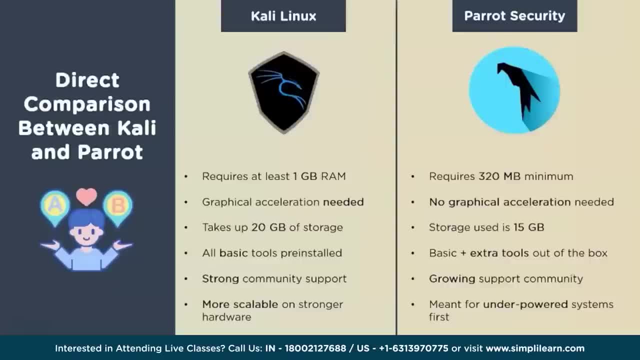 requirements from a hardware perspective, like just 320 MB of RAM and no graphical acceleration. This means Parallel Security is much more feasible for people who are not able to devote massive resources to either their virtual machine or on their laptop hard disk directly. With the comparison done between both of these operating systems, 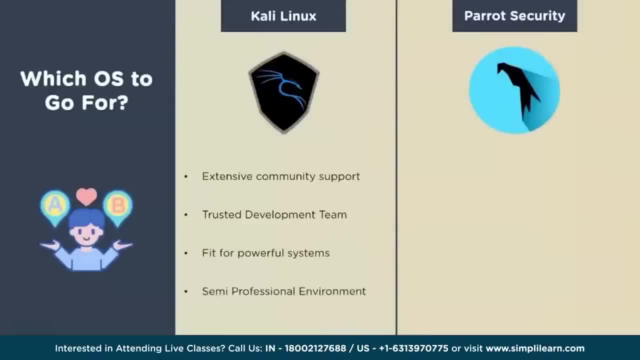 let's take a look at the type of users both of these are catered to. One can go with Kali Linux if they want the extensive community support offered by its users, if they want to go with a trusted development team that have been working on this distribution. 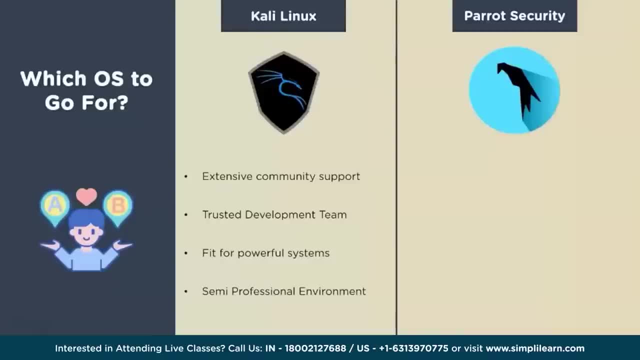 since many years. if they have a powerful system which can run Kali Linux operating optimally without having to bottleneck performance, and if they are comfortable with a semi-professional environment, which may or may not be very useful for new beginners, One can decide to go with Parallel. 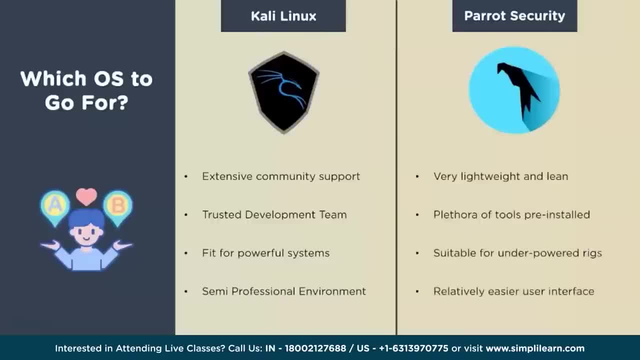 Security if they want to go with a very lightweight and lean distribution that can run pretty much on all systems. It also has a lot of tools pre-installed, and some of them are not even present on Kali Linux. It is much more suitable for underpowered rigs. 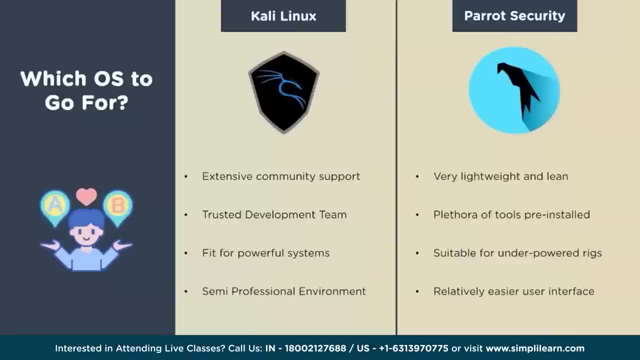 do not have a lot of hardware resources to provide to the operating system, and thereby it is much more feasible for people with underpowered laptops or no graphical acceleration. Compared to Kali Linux, Parallel Security's desktop environment is also relatively easier to use for new beginners, For people who are just getting into ethical hacking, Parallel Security does. 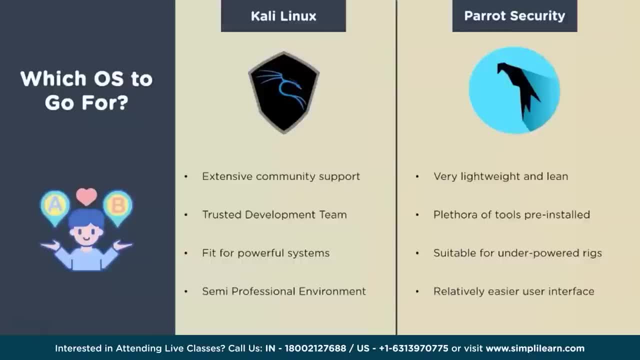 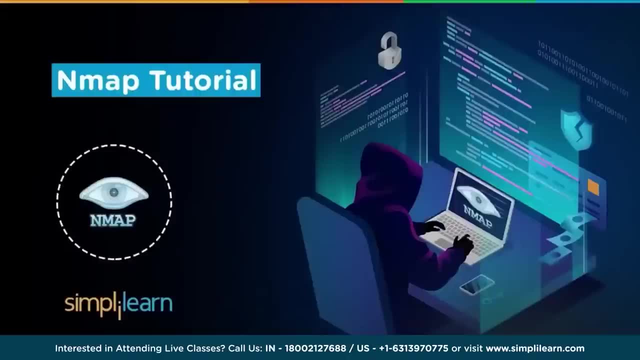 a relatively better job of introducing them to the operating system and to the various tools without having to dump them into the entire intricacies. With ethical hacking and penetration testing becoming mainstream in corporate environments, trained personnel and relevant equipment are in high demand. The right software framework can be the tipping point in a hacking. 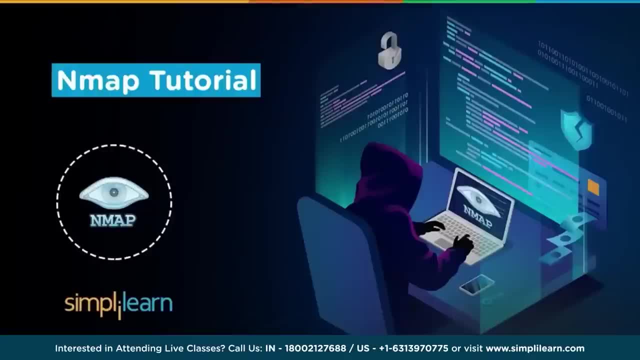 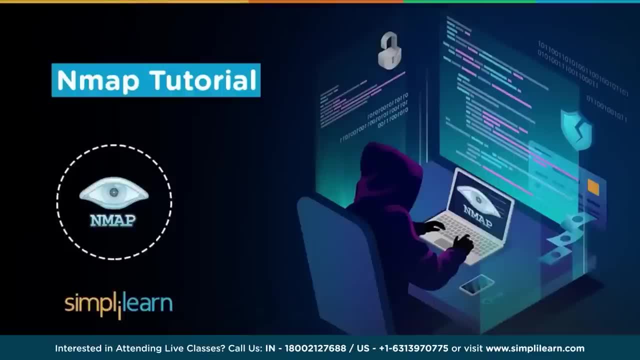 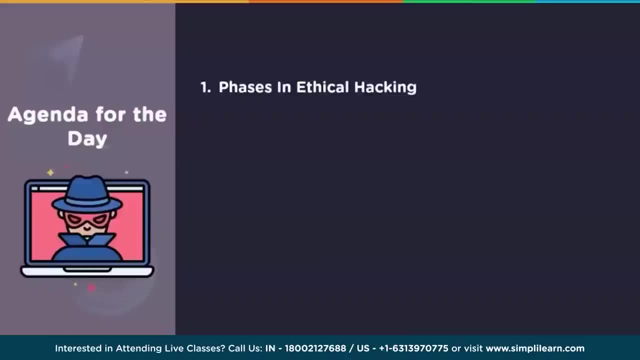 regular updates. Let's take a look at the topics to be covered today. We start by learning about the different phases in ethical hacking and where Nmap is most valuable to ethical hackers. We learn the basics of Nmap and its purpose during a penetration testing campaign. 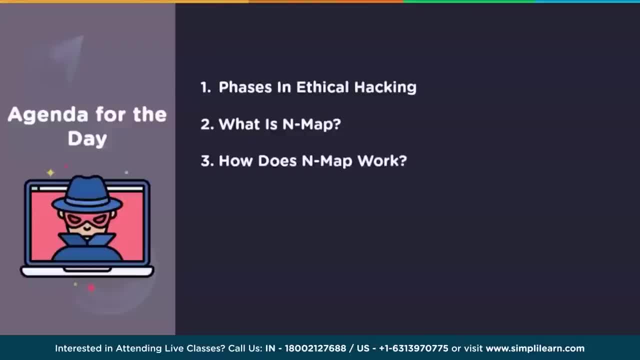 Next, we take a look at the top-level approach of Nmap as a scanning tool and how it conducts these scans on host machines. Moving on, we cover the multiple modes and types of scans that can be performed using Nmap on unsuspecting users. 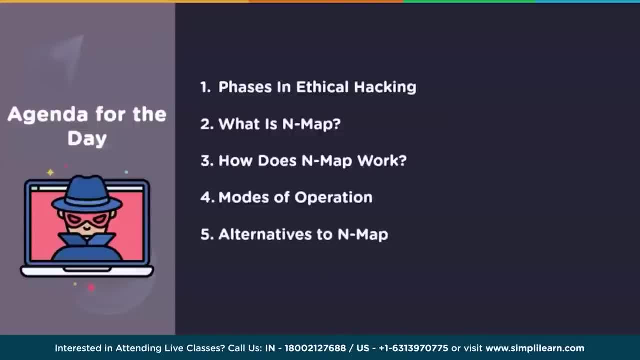 We also look at some alternatives that users can prefer if Nmap is not something they are comfortable with. while a live demonstration of the powers of Nmap will help in shedding light on the topics being taught today, Let us first understand where and why Nmap is essential. 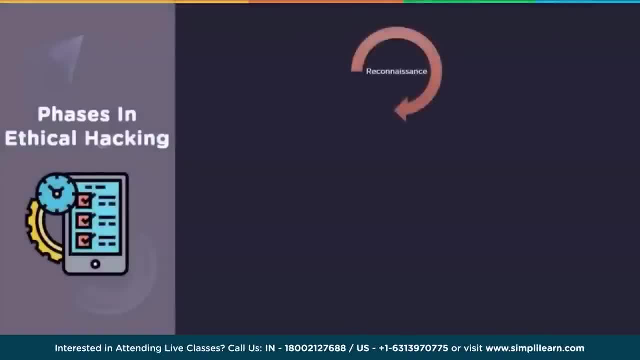 There are essentially five phases in ethical hacking. The reconnaissance phase is the first phase of the penetration test. Here the security researcher collects information about the target. It can be done actively or passively, or both. It helps security firms gather information about the target system. 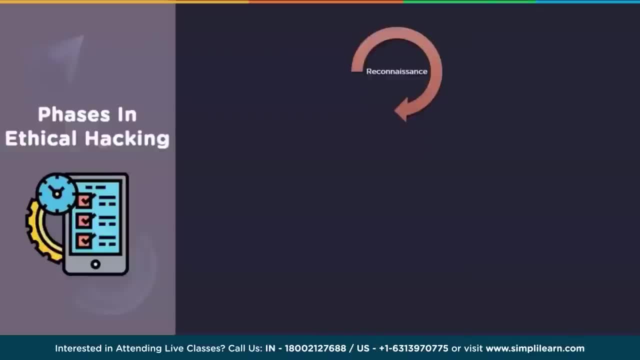 network components, active machines, etc. This activity can be performed by using the information publicly available and by using different tools. The scanning phase is more tool-oriented rather than being performed manually. The tester runs one or more scanner tools to gather more information about the target. 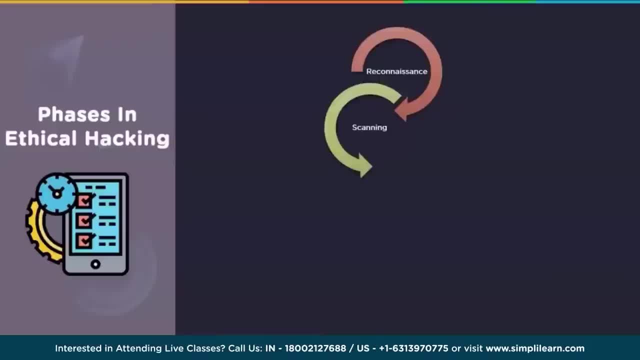 The scanner uses various scanners, such as wall dialers, port scanners, network mappers and vulnerability scanners. The penetration tester collects as many vulnerabilities which help in turn to attack a target in a more sophisticated manner. In the gaining access phase, the penetration tester tries to establish: 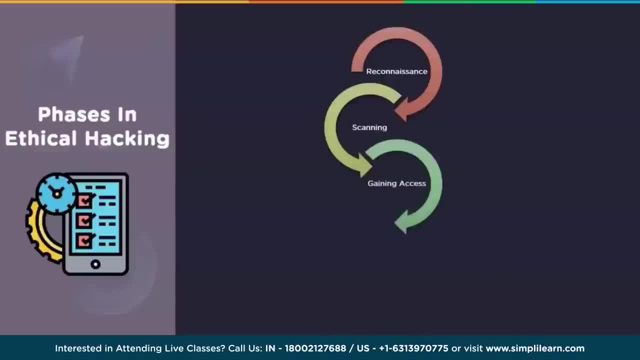 a connection with the target and exploit the vulnerabilities found in the previous phase. The exploitation may be a buffer overflow attack, denial of service attack, session hijacking and many more. Basically, the penetration tester extracts information and sensitive data from the servers by gaining access with different tools. 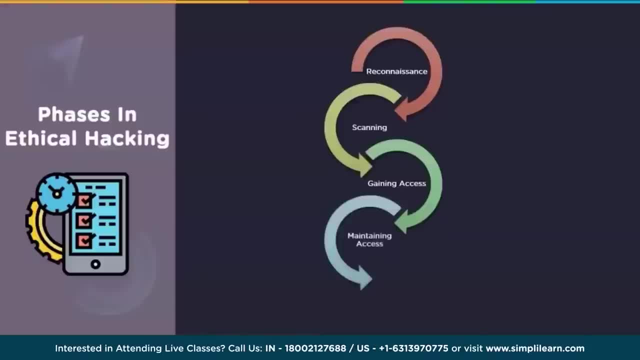 In the maintaining access phase, the penetration tester tries to create a backdoor for himself. It helps him to identify hidden vulnerabilities in the system while allowing him to come back to the system to retrieve more data further on. In the clearing tracks phase, the tester tries to remove all logs and footprints which might. 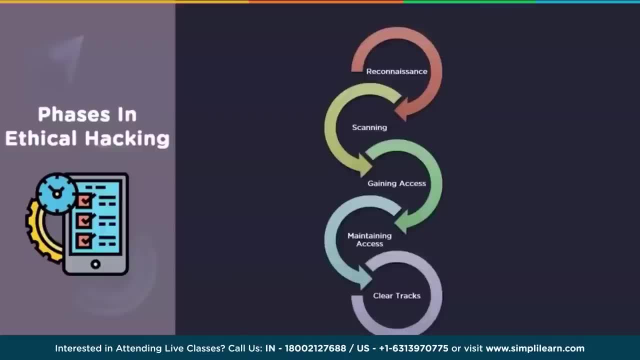 help the administrator identify his presence. This helps the tester to think like a hacker and perform corrective actions to mitigate those activities. Nmap is most beneficial in the early stages of ethical hacking, where a hacker must figure the possible entry point to a system. It is necessary to know this before running the necessary exploits, thus allowing the 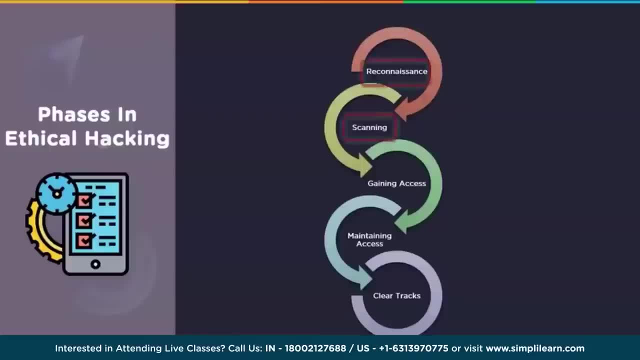 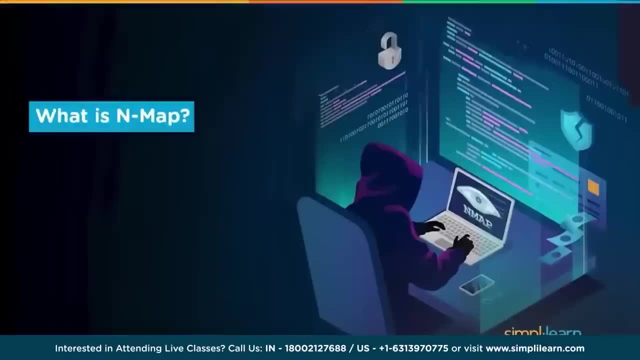 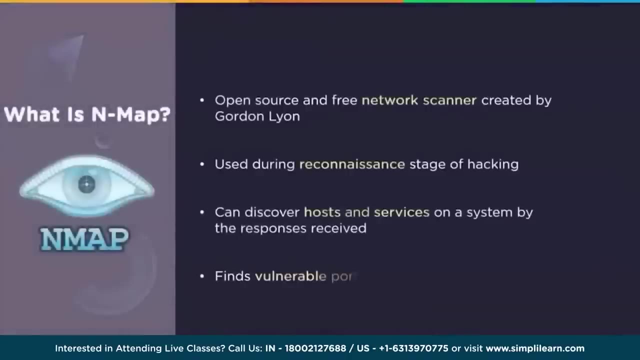 hackers to leverage any insecure openings and breach the device. So the reconnaissance and the scanning phase are the points where Nmap finds the most use. Let us now understand what Nmap is from a layman's perspective. Nmap, which stands for Network Mapper, is a free and open source utility for network discovery. 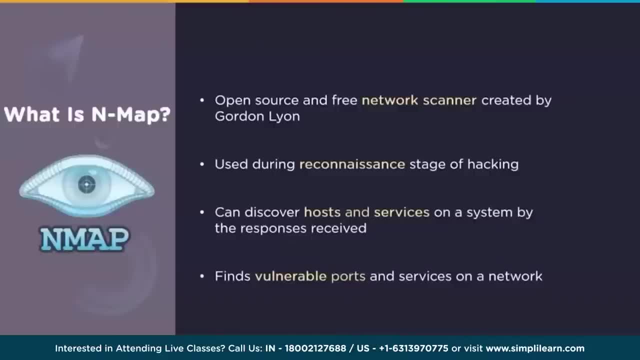 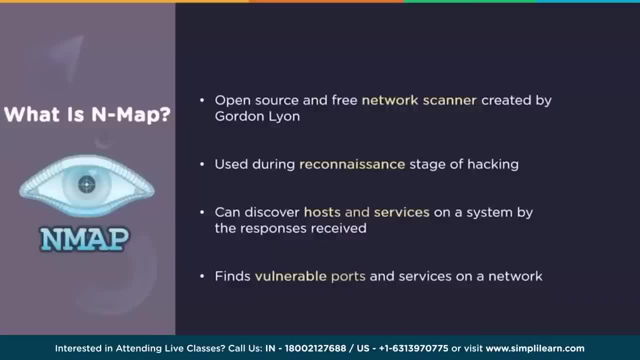 Github, Github, Github, Github, Github. It is most beneficial in the early stages of ethical hacking, where a hacker must figure the possible entry point to a system before running the necessary exploits. Nmap was developed for enterprise scale networks and can scan through thousands of connected 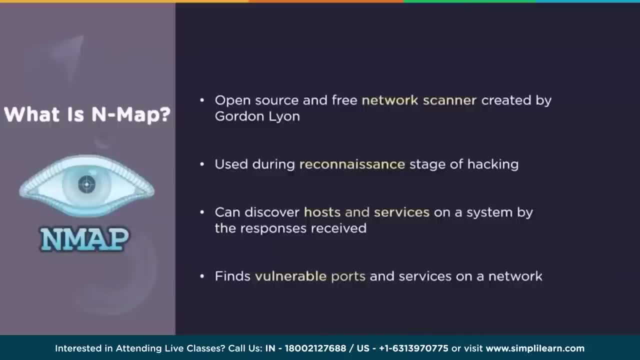 devices. However, in recent years, Nmap is being increasingly used by smaller companies as well. Nmap uses raw IP packets in novel ways to determine what hosts are available on the network, What services these hosts are offering, what operating systems they are running, what type of packet filters and firewalls are in. 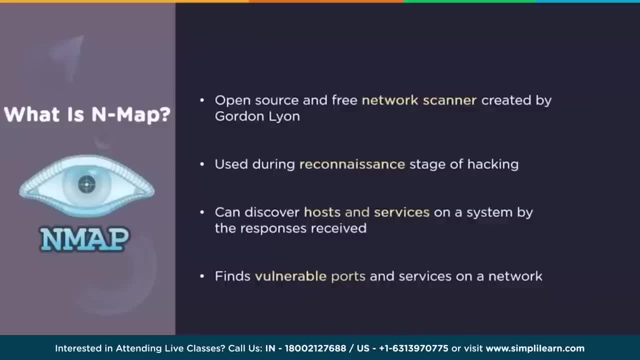 use and dozens of other characteristics. It was designed to rapidly scan large networks, but works fine against single hosts as well. The rise of the IoT in particular, now means that networks used by these companies have become more complex and therefore harder to secure, Since every application that connects to a network needs to do so via a port- the wrong. 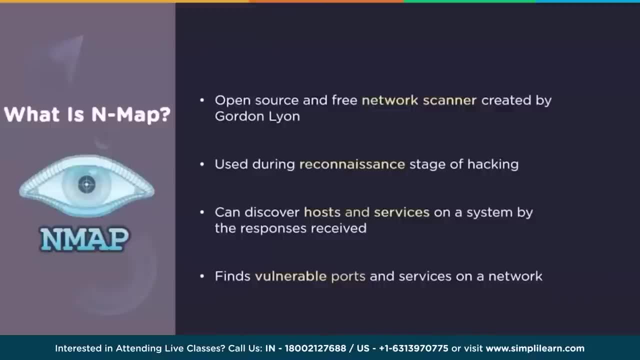 port or server configuration can open a can of worms that leads to a thorough breach of the system. The recent emergence of IoT botnets like Mirai has also simulated interest in Nmap, not least because of its ability to interrogate devices connected via the UPnP protocol, but also to 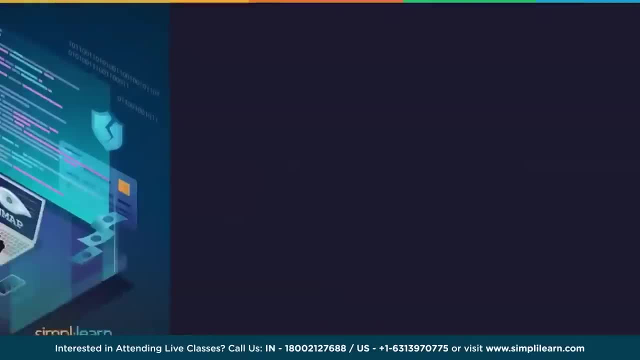 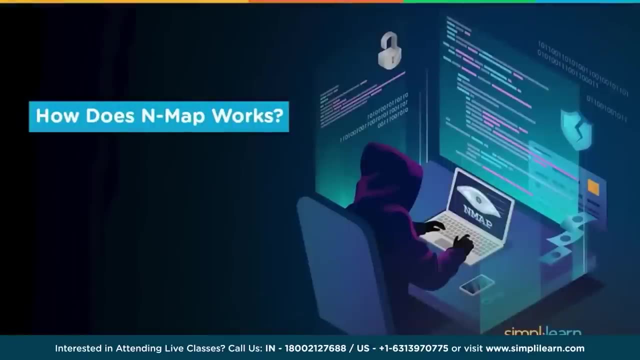 highlight any devices that may be malicious. Now that we understand what Nmap is, let us take a look at the workflow of how an ethical hacker uses this tool in penetration testing. At a practical level, Nmap is used to provide detailed, real-time information on your networks. 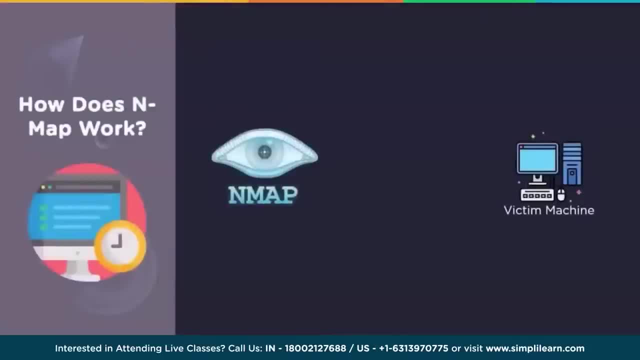 and other devices connected to them. We have the hacker running Nmap on his system, with the victim machine running a standard installation of their operating system, be it Windows, MacOS or Linux. The Nmap interface will send specially crafted packets to generate some reply from the victim. 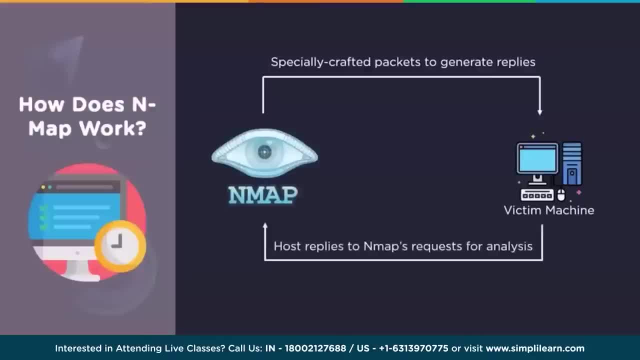 machine. The victim machine, in return will send some information back to the Nmap host, with replying some of the services and hosts that are being run on the computers. Nmap allows the network admins to find which devices are running, discover some open-source. 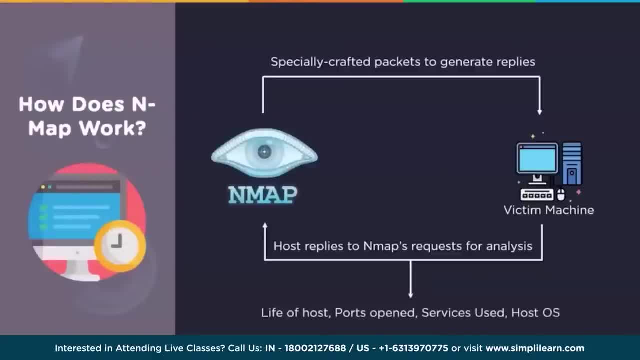 and find out which devices are running. The Nmap interface allows the network admins to find which devices are running. discover some open-source and find out which devices are running. The Nmap interface allows the network admins to find which devices are running. discover. 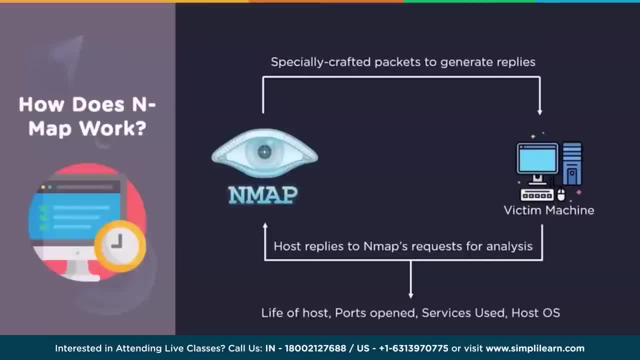 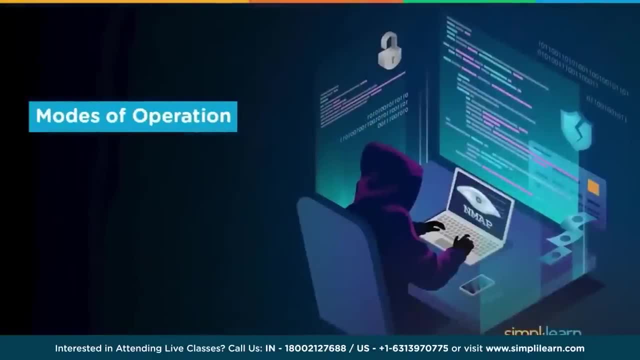 some open-source and find out which devices are running. This in turn helps discover the vulnerabilities and the possible entry points for hackers to breach into. We are now aware of how Nmap works on a basic level, but there are many varieties of scans. 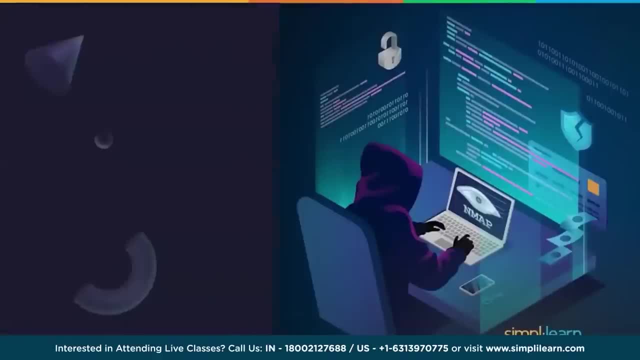 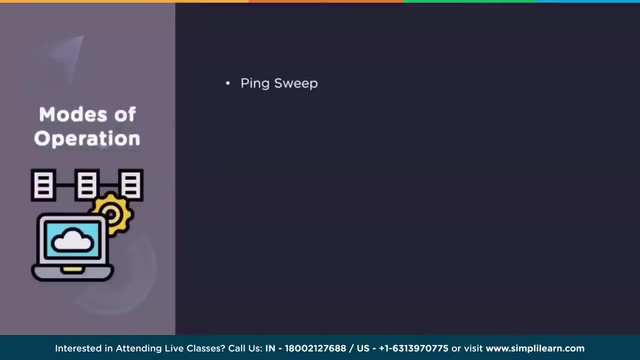 that users can run on local machines. Let us take a look at some of them. The Ping Sweep is a simple type of Nmap scan where it pings to all the available IP addresses to check which IPs respond to ICMP protocol. If the users need to know only the number of IP addresses and not many details, the 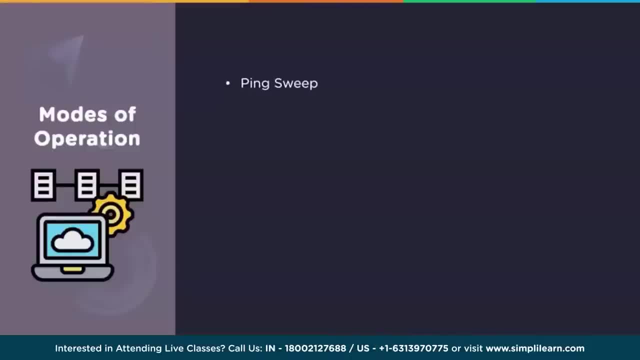 Ping Sweep is very useful. It's fast and hence the results to be known are fetched very easily. The SYN scan is the most useful type of Nmap scan which does work very quietly. It sends an SYN packet via the TCP protocol or the transfer control protocol to all the 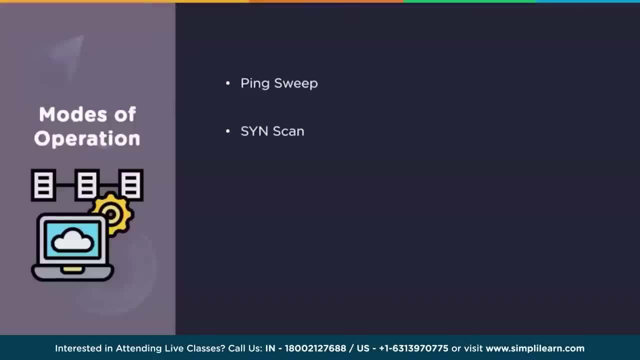 intended ports. If an acknowledgement packet is received to the system, it is sure that a port is opened there. No response means that the port is either closed or not available. Here the acknowledgement packet is not sent back to the system, assuming that the connection 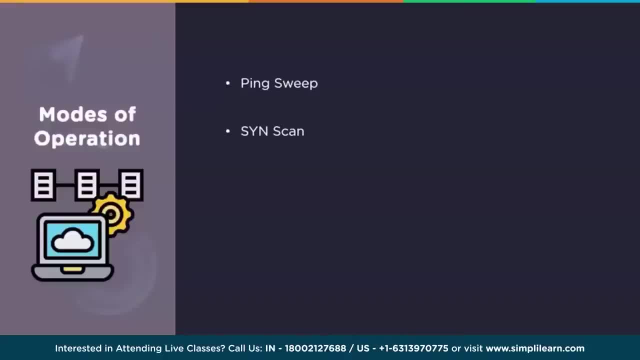 is not valid. The scan is not shown in most of the scan logs and hence it is safe to use SYN scan to identify the opened ports. The TCP connect scan is similar to SYN scan in many aspects, as it uses the TCP layer to send packets and is passed through all the ports. 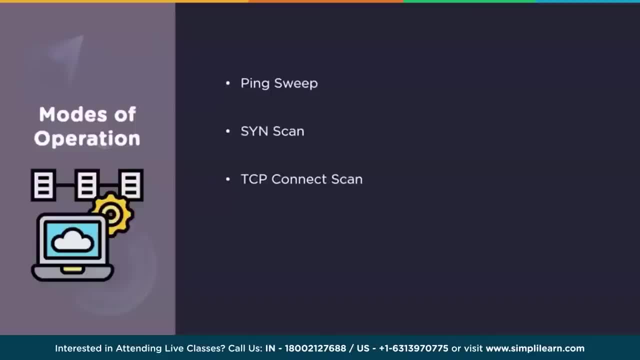 Here the difference is that the full connection is done by sending the acknowledgement packets back. The logs can easily find the TCP scan and need more power from the machines to do the work. But it is more accurate If all the accesses related to the OS are available to the user. it is better to do. 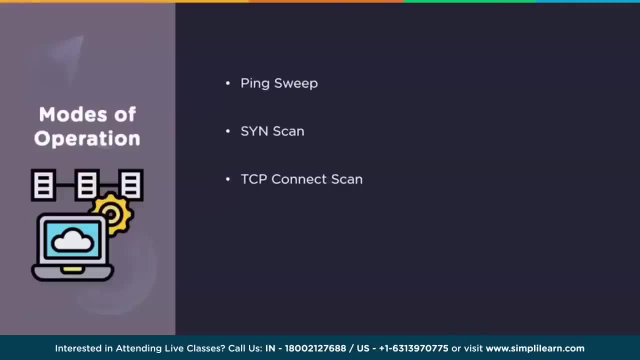 a TCP scan than an SYN scan. as all the low level and high level accesses are required for the scan, The network is also loaded more, and hence users must be careful about overloading the system and the networks. The idle scan is really used to check whether any malicious attacks are possible. 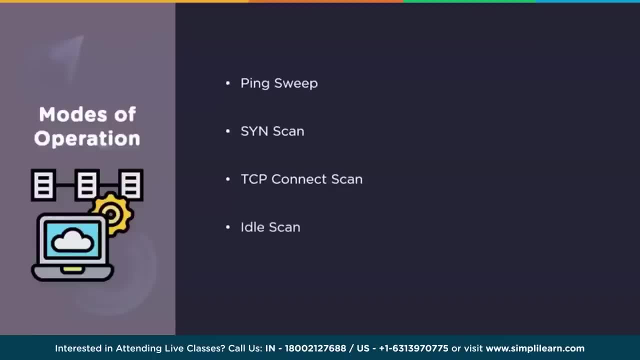 Users need not control the external host, but an IP address and a port should be given to the same. All other requirements are taken from the scanner itself. The RPC scans, or remote procedure calls, are done by hackers to make the system vulnerable to virus attacks. 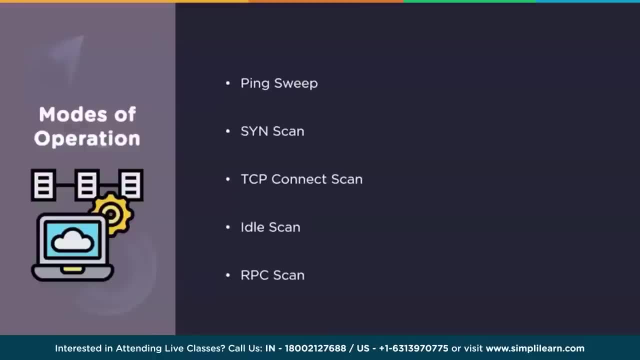 It is thus necessary to know whether our systems answer such calls and make our system open to malware. RPC scan is done to check this by finding the ports open with certain commands being run by RPC. The Windows scan is a simple scan where the application scans the acknowledgement packets. 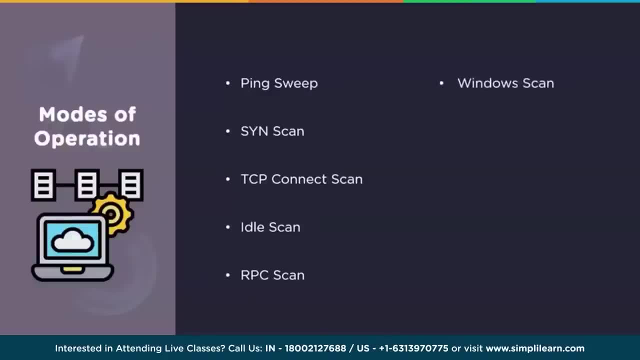 received from the ports once the SYN packets are sent. If there are any abnormalities in the ACK packets received, the scan reports the same and helps in recognizing which ports are functioning in a different manner. The bound scan is used to check the security in the file transfer protocol layer. 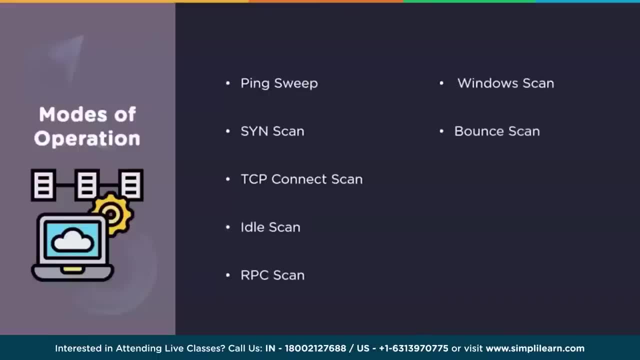 FTP layers mostly do not accept any packets and once it is rejected from the FTP layers, there are chances that it might be sent to an internal layer. The FTP layer is used to check the security in the file transfer protocol layer. FTP layers mostly do not accept any packets and once it is rejected from the FTP layers. 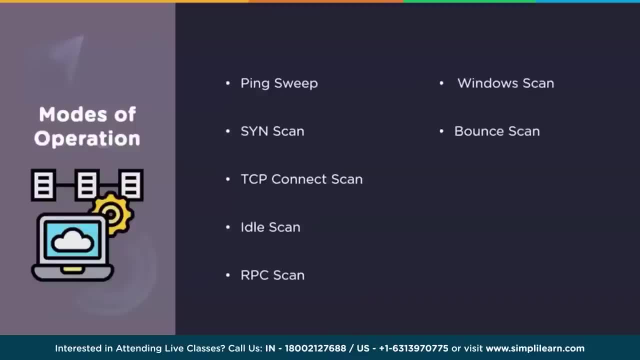 there are chances that it might be sent to an internal layer. The bound scan checks this loophole by doing exactly the same process and identifies whether a FTP layer is open to vulnerability or not. The FIN scan is similar to SYN scan, where the system that sends the packets receives. 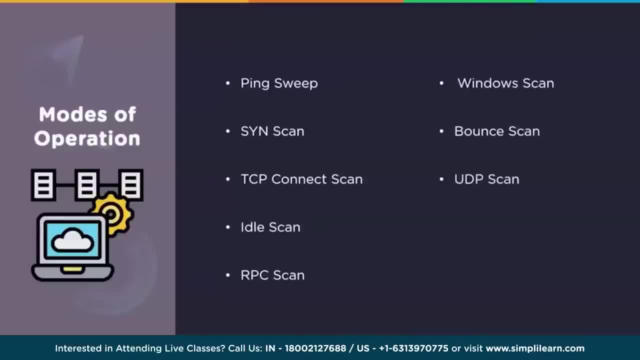 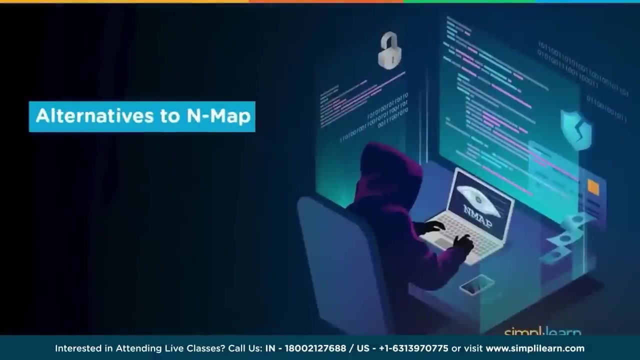 the response back, and it will mostly be a TCP FIN packet. If the system sends an RST packet, it is a false alarm and users need not be worried about the same. The Null scan is useful for other systems. When it comes to looking at alternatives, there is a wide range of free network monitoring. 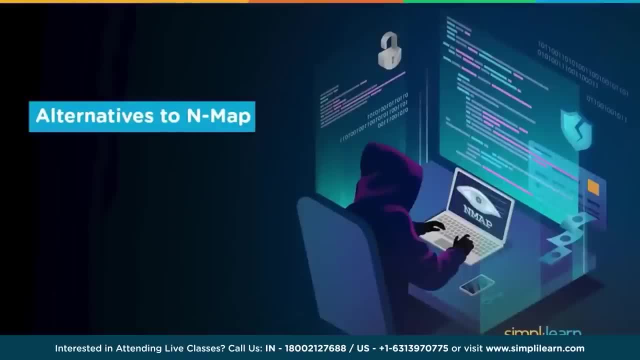 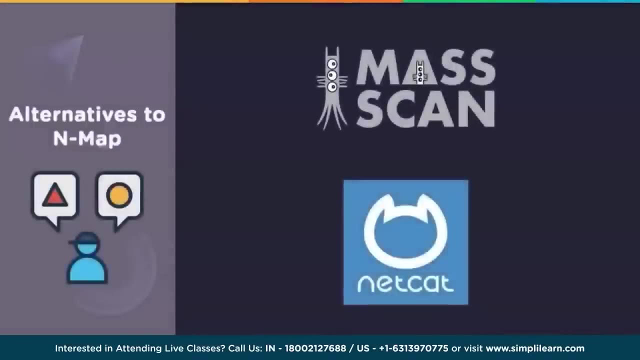 utilities, as well as free, open source vulnerability scanners available to network administrators and security auditors. What makes Nmap stand out as the tool IT and network security managers need to know? There are some alternatives to Nmap, but most of them are focused on providing specific 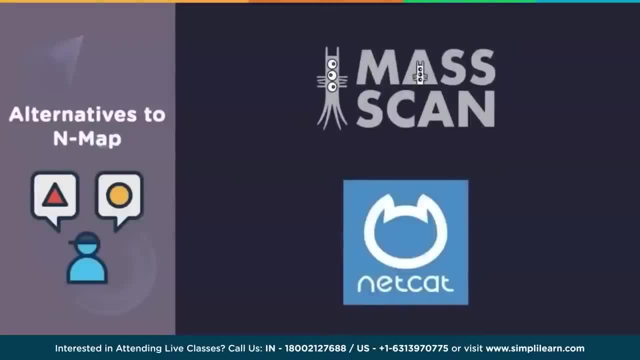 niche functionality than the average system administrator does need frequently. Mass scan, for instance, is much faster than Nmap, but provides less detail. In reality, however, Nmap provides all the functionality and speed that the average user requires, especially when used along with other similar tools like Netcap, which can be used 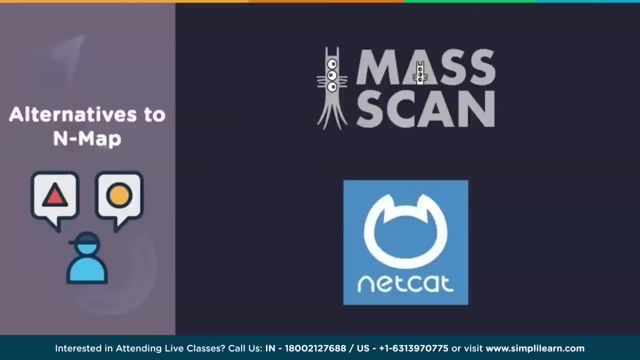 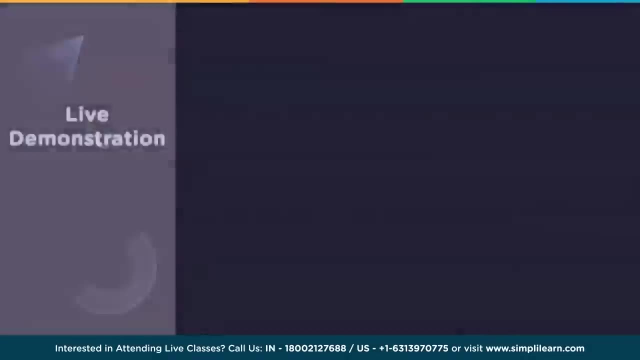 to manage and control network traffic, and Zenmap. It provides a graphical user interface for Nmap, But as an all-rounder solution to network scanning, nobody can go wrong with Nmap as their tool of choice. Let's now take a tour of Nmap based on all the things we have covered today. 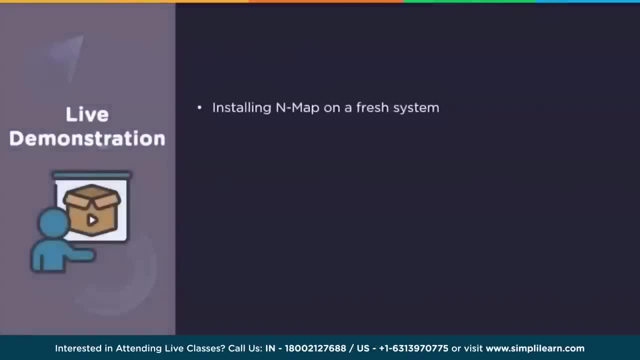 In this live demonstration, we start by learning of how to install Nmap on a fresh operating system that doesn't come pre-installed with the tool. We also cover the different types of scans that can be run on local machines, along with checking multiple inferences an ethical hacker can gather based on the data that is being 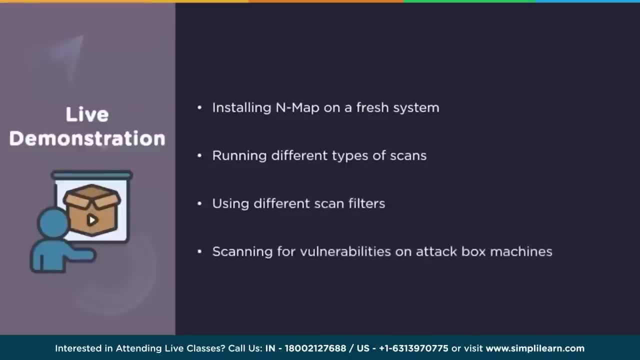 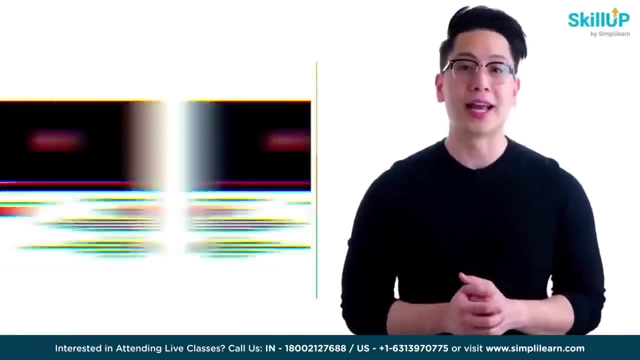 collected. Finally, we run scans on vulnerable machines to get an idea of how to proceed with the outputs we gather using this tool. If getting your learning started is half the battle, what if you could do that for free? Visit SkillUp by SimplyLearn. 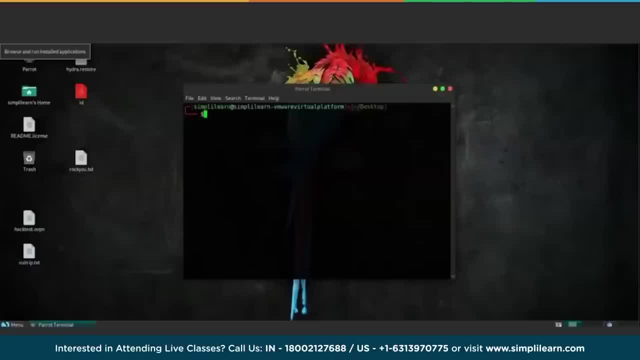 Click on the link in the description to know more. The first step in our demonstration is installing Nmap. Now it depends heavily on what Linux distribution you are going to use to perform ethical hacking. The first step in our demonstration is installing Nmap. 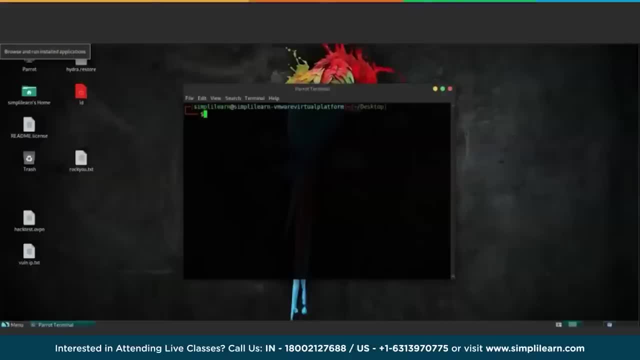 Right now I am using Parrot Security operating system. If you are not aware of what Parrot Security is, or even what Kali Linux is, we highly suggest that you check out the videos of those two operating systems on our YouTube channel so that you can get a fair idea of what they serve. 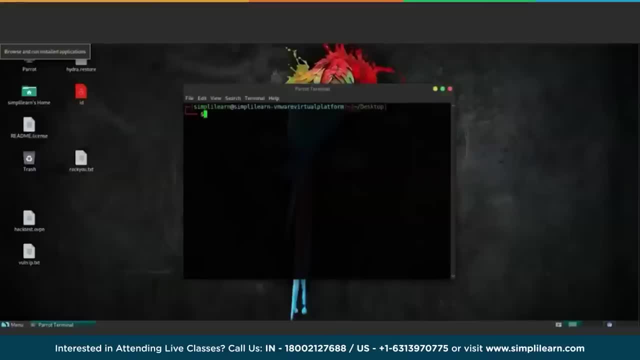 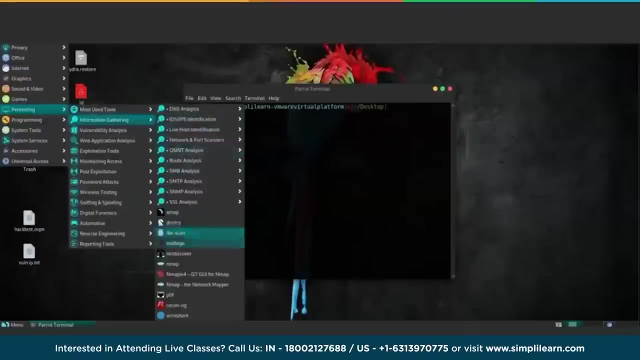 Now, if you are using any of these two operating systems, Nmap should come pre-installed by default. To check if Nmap is pre-installed or not, you can just press on Applications over here, Go to the Pentesting section, Go to this Information Gathering tab and you should be able to see Nmap right here. 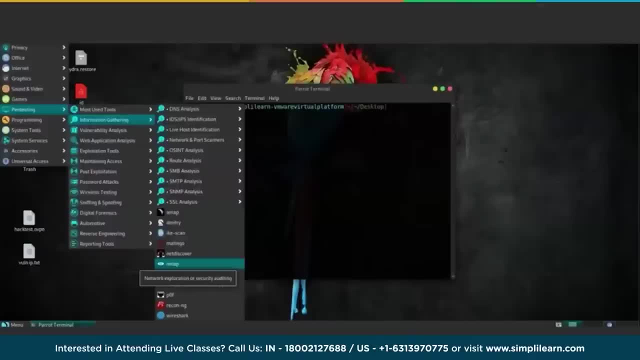 Now, let's say you do not have Nmap pre-installed. maybe you are using a Linux distribution like Ubuntu or Linux Mint or something that is based on Debian operating systems. One thing you have to make sure: that Nmap should be in the distribution repository. 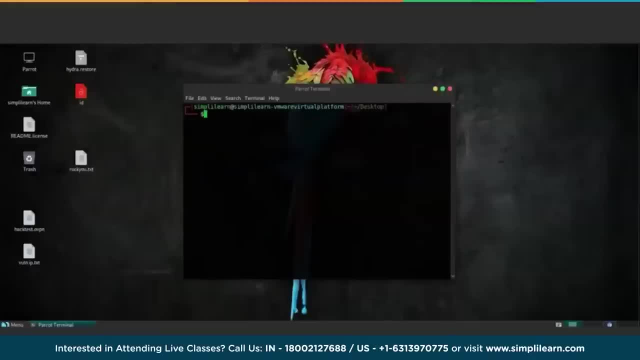 Once you check that, or even if you do not know if it is present, you can just just come on. It should be sudo apt. apt is the package manager of all Linux distributions that are based on Debian. That goes for Debian stable, Ubuntu, Linux Mint, Kali Linux, Parrot, Security and anything. 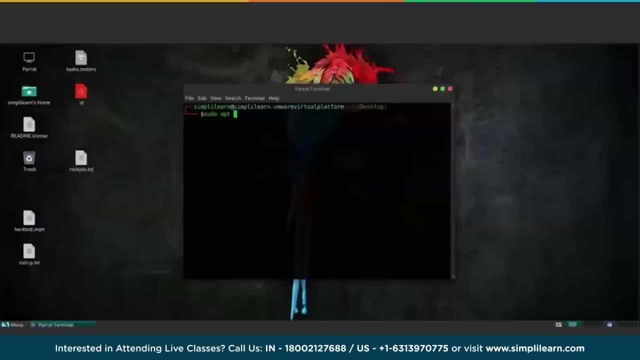 of that nature. apt is the package manager which handles the installation and removal of applications in these specific operating systems. Once you are here, just write: install apt. apt is the package manager which handles the installation and removal of applications in these specific operating systems. 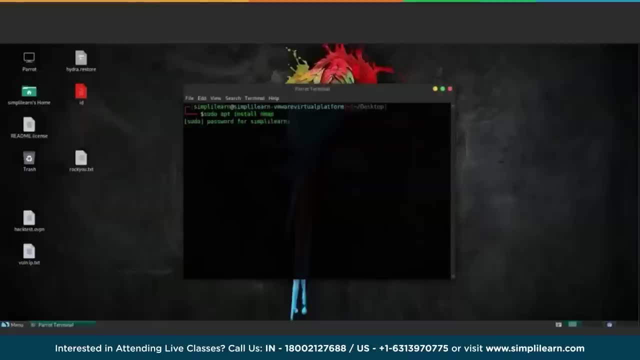 Once you have installedelaparkedpuresdmipuresdmienvpure and map, press Enter and it's going to ask you for the root password that is set when you install the operating system in the first place. 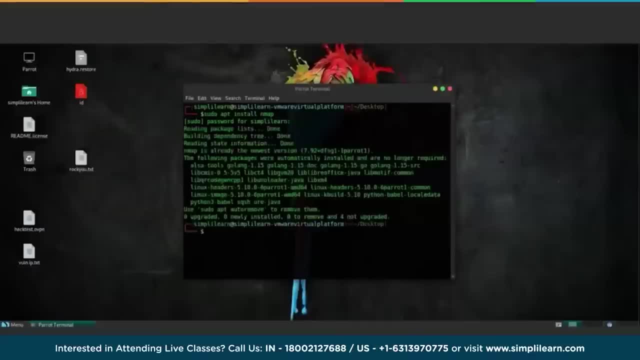 Enter your root password and press enter again. As you can see, it's saying that Nmap is already installed- the newest version, since I'm running Parrot Security operating system. Now should you be running this operating system or even Kali Linux, you should receive. 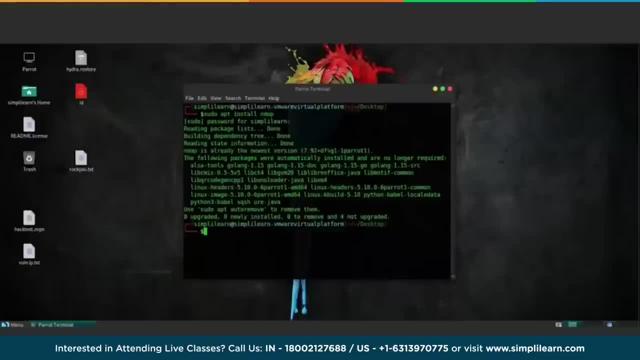 a similar message and the installation is already done. If you are using Parse Security OS system, you should receive a similar message and the installation is already done. And once you have installed that operating system, you should receive a similar message If you are using some other distribution, let's say even Blackhawks, Arch, Linux or Manjaro. 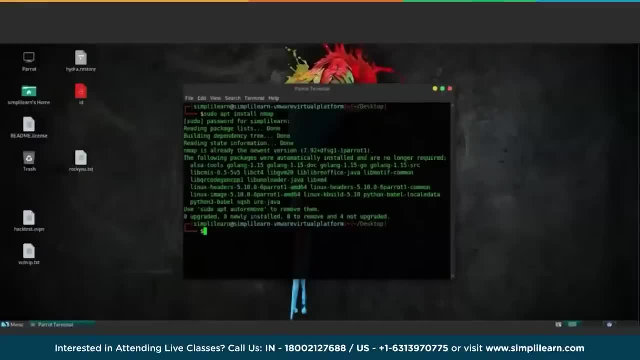 anything like that, the installation steps will be slightly different. This sudo apt install nmap command is for distributions that are derived from Debian and Ubuntu. If you want to install in Arch Linux based distributions, you have to use their package manager, which is known as PAMAC. 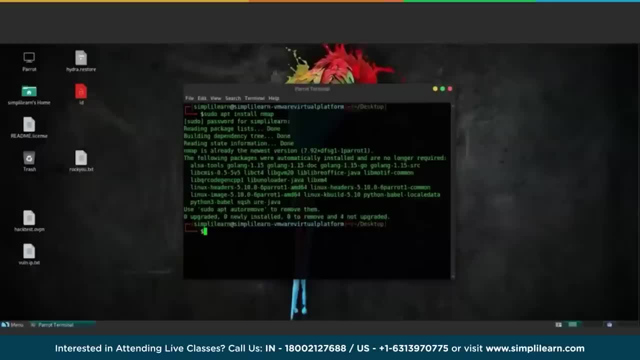 But that is for a different step, and if you want to get ethical hacking, the best way to start is by learning either Kali Linux or Parrot Security. Now that the installation is done, we're going to learn how to use nmap. 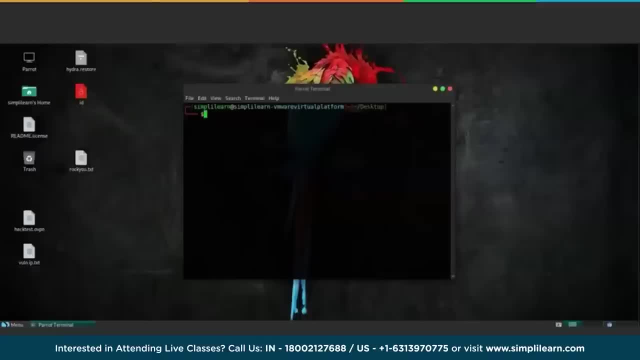 One of the most basic functions of nmap is to identify active hosts on the network. We can do this by using a ping scan. The ping scan identifies all of the IP addresses that are currently online without sending any packets to these hosts. Now to run the ping scan, we're going to write nmap. 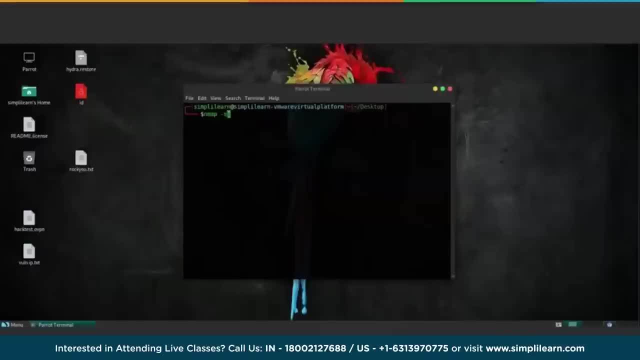 The flag we're going to mention over here is SP. Now, these flags are the different traits of the nmap scan. Depending on what flag we use, we can send different kinds of requests to the host that we are scanning. Now, before moving forward with this, let me open another terminal over here and check. 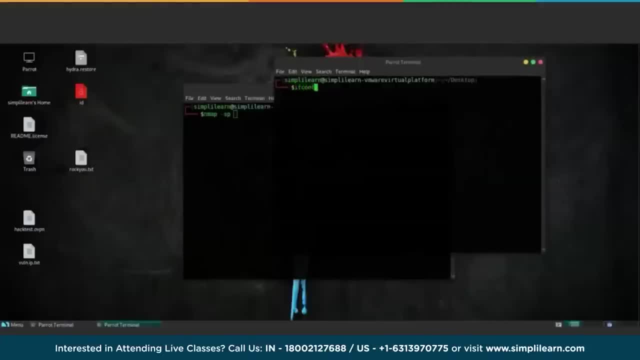 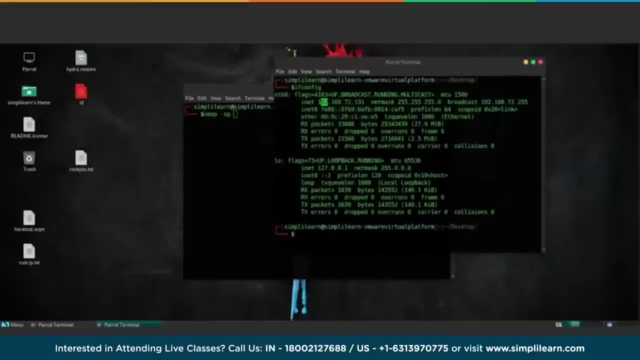 the IP address. I'm going to write the command ifconfig and find the subnet in which this system is present. As you can see, the IP address is 192.168.72.131.. Now this operating system is being run on a virtual machine software known as VMware. 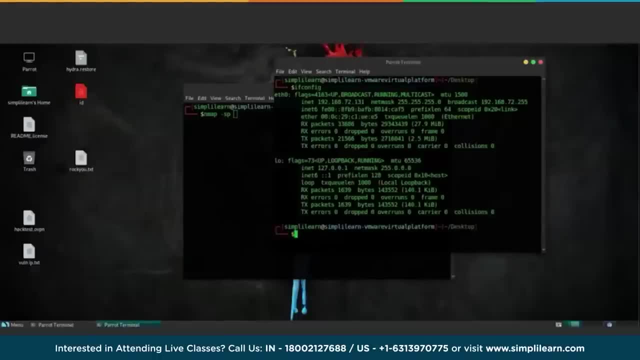 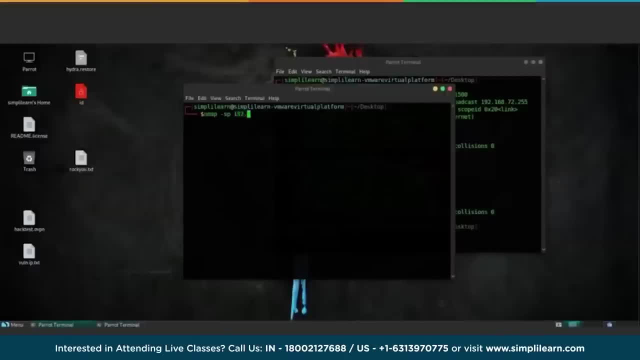 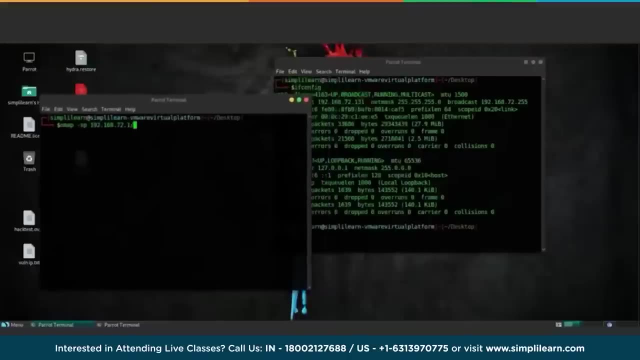 So we're going to run the ping scan. To run our scan, we're going to target 192.168 and 72.1-24.. This command then returns a list of hosts on your network and the total number of assigned IP addresses. 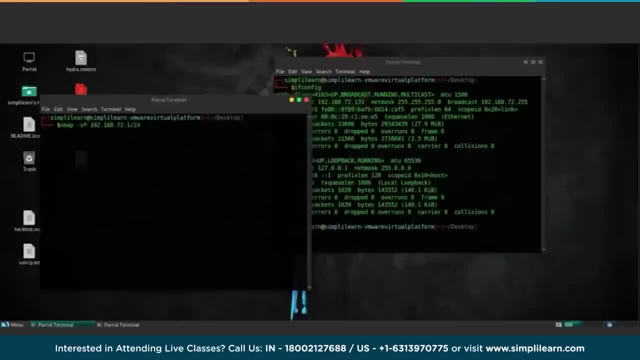 This is going to be capital P. Yeah, If you spot any hosts or IP addresses, you can run the ping scan. If you spot any hosts or IP addresses on that list that you cannot account for, you can then run further commands to investigate them further. 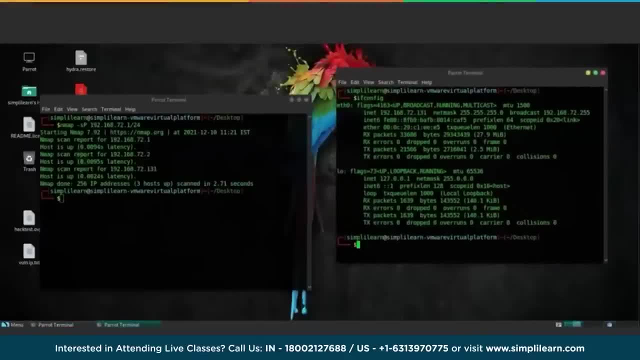 As of right now, you can see the machine. that is the Parrot Security. This IP address can be detected in the subnet. The 192.168.72.1 is my local Windows machine that is running VMware software and, ultimately, this virtual machine. 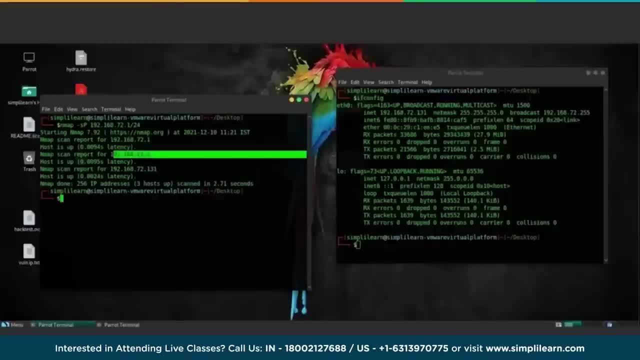 The 72.2 is the DHCP server that hosts the internet connection of the Parrot Security, So this IP address can be detected on the subnet. So this 192.168.72.1 is my local Windows machine that is running VMware software and 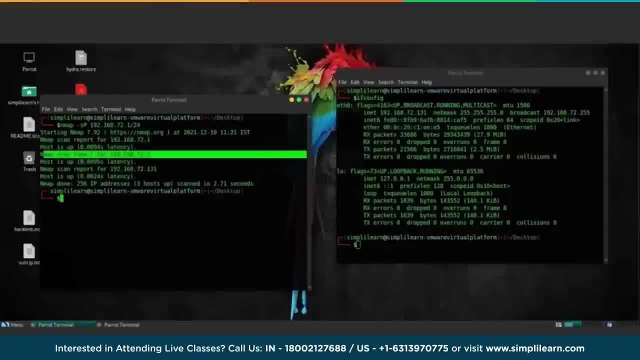 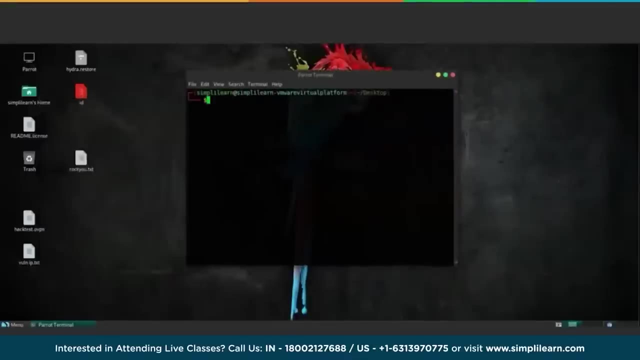 ultimately this virtual machine security. this we can ignore for now. now the Windows machine that we have over here. let's run some tests on that. we're going to clear a terminal and you can close this. actually, when scanning hosts and map commands can use server names. 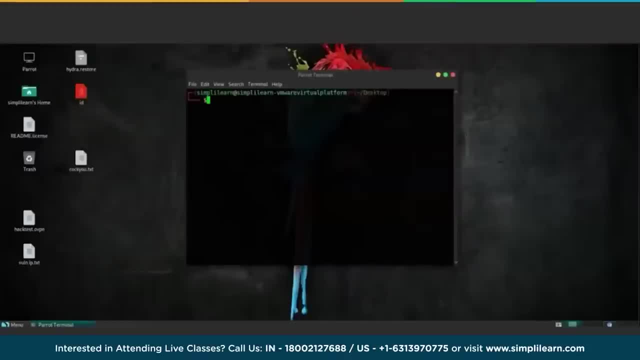 IPv4 addresses or IPv6 addresses, a basic and map command will produce information about the given host. to run a basic port scan, we can just use nmap along with the IP. now, as you remember, the IP is 192.168.72.1. this is the IP of my local Windows 10 machine. as you can see, it shows the: 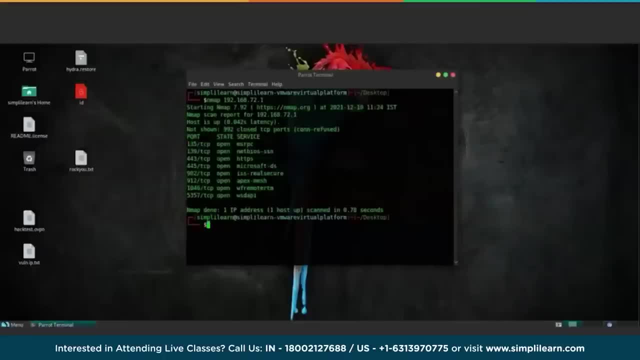 ports that are open and the particular service that these ports are running. now we can also have a detection of the operating system, the. mind you, this is not 100% correct and the reliability depends on the installation and what kind of fingerprinting measures are available now. since this does TCP IP fingerprinting, it needs some extra. 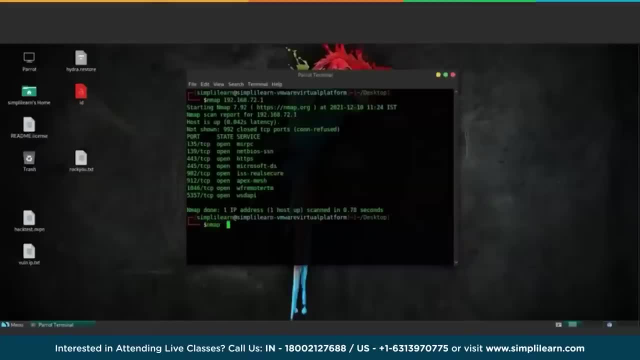 permissions. the flag that we are going to use is nmap minus o, along with the same IP address. like I said, since this is TCP ipf, ing up printing, it requires room network at this point. privileges now to provide root privileges, we're just going to add the nmap and sudo keyword. 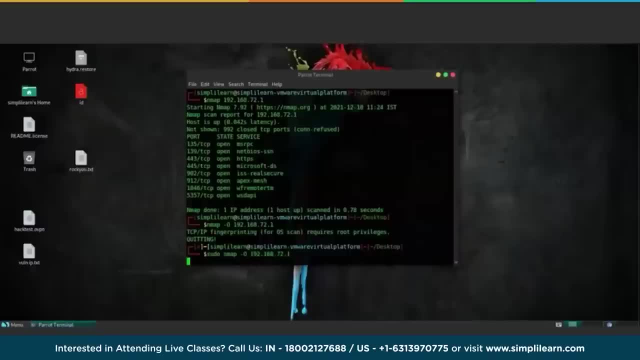 going to repeat the same command that we wrote above. as you can see, it has successfully detected that i am running microsoft windows 10 with this mac address. it has also shown the correct build number of the windows 10 system that i am using. this is useful for troubleshooting, scanning for few vulnerabilities or even locating some services. 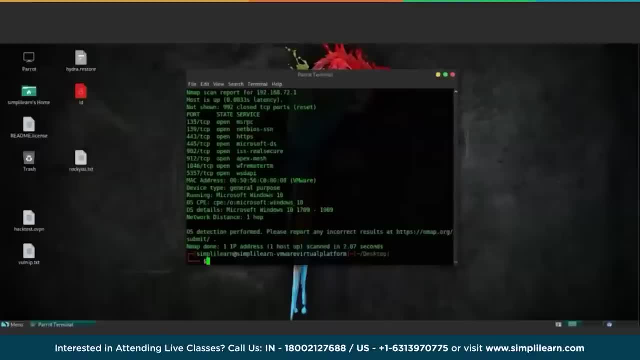 that need to be updated now to get the necessary information about these services, for example what versions they are using. we have a command known as sv, which stands for service version. we use the same ip address and press enter. now, as you can see, the scan is complete and if you can check the results of the scan above here, 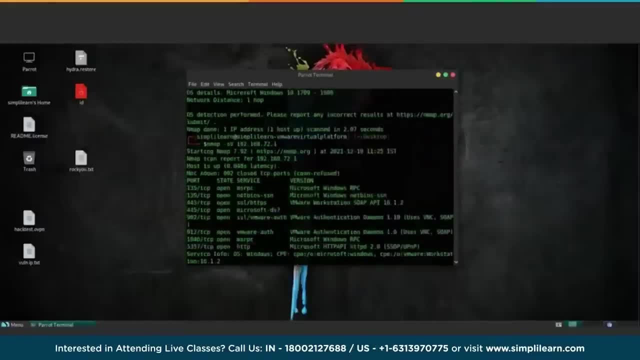 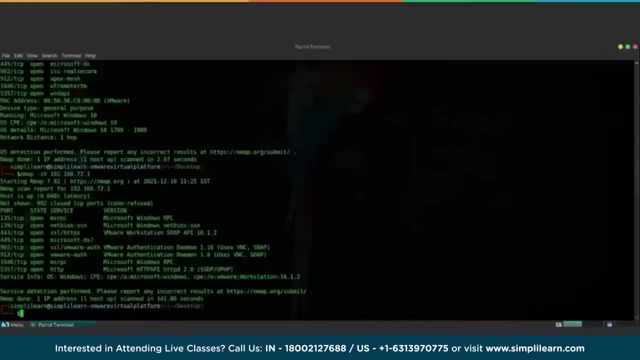 you don't see any version number for the services. here we can actually check what version they are running. now this becomes helpful when we are trying to find specific versions to fit into the WearSoft OS, because we have to know if we are able to use this version on our Mac. 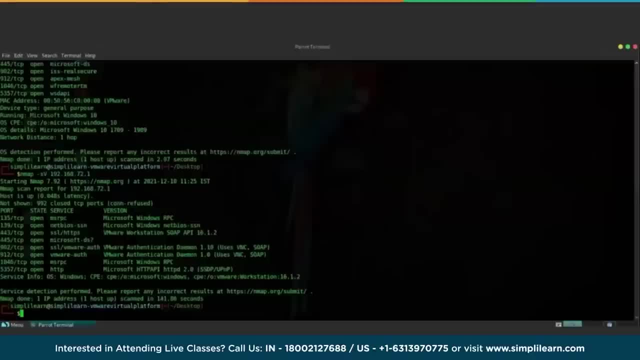 exploit. for example, if vma workstation 16.1.2 had some particular vulnerability, we can exploit it by checking this command. apart from the host scanning, port scanning is one of the most basic utilities. there are a few ways that this command can be customized as well. for example, i have already 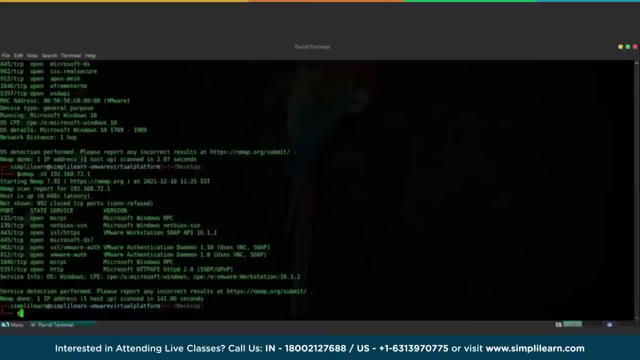 checked that the 443 command is open, but i have found out after running this lengthy scan- let's say, i only want to check if command, if the port 443 is open and map. i'm going to use the flag of minus p, which stands for port, and give 443 as an argument here, using the same ip address. 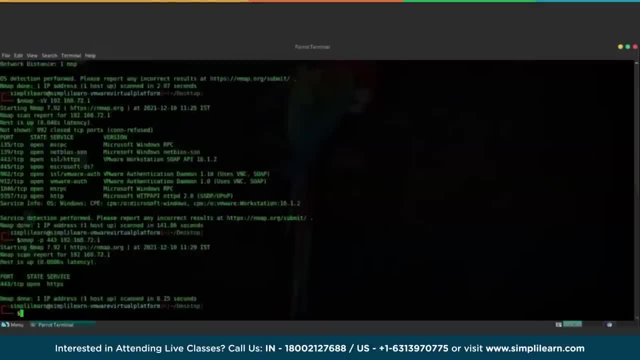 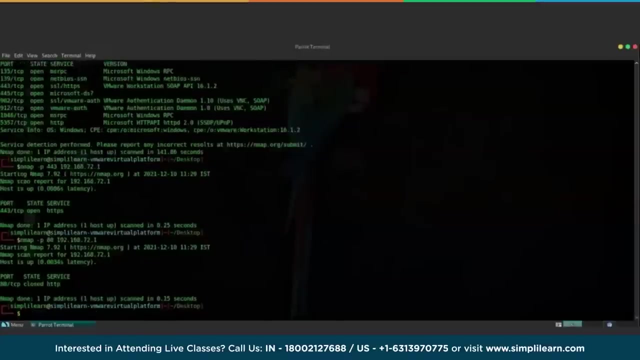 and you can see it says it's open. but we already knew it is open. let's say there was something else. uh, if let's say we're going to scan if the apache web server port is open, which usually runs on 80.. obviously, since i'm not running an apache web server, it says it's closed. 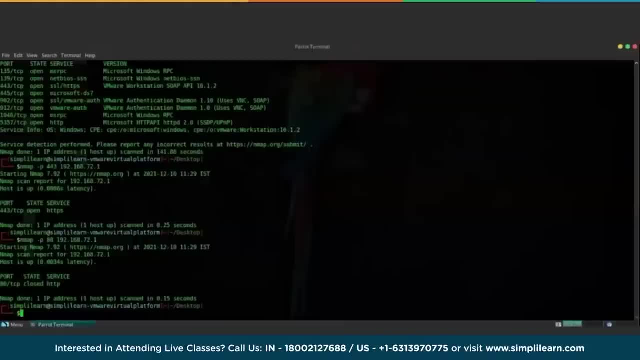 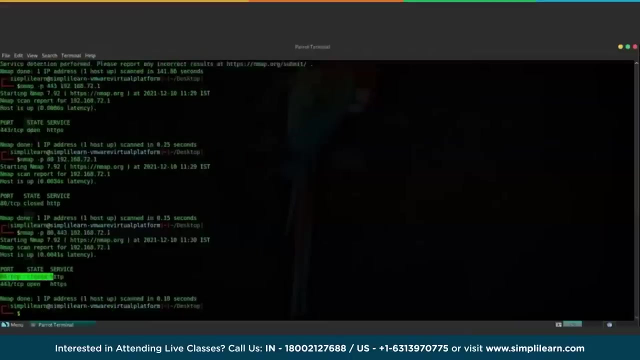 now we can combine these two commands by running both both simultaneously. to do that, we can just put a comma and complete the rest. similarly expected, 80 is closed and 443 is open. another feature of nmap for port scanning is showing off ranges. now, ranges can be beneficial when you're trying to see up to a certain limit, for example. 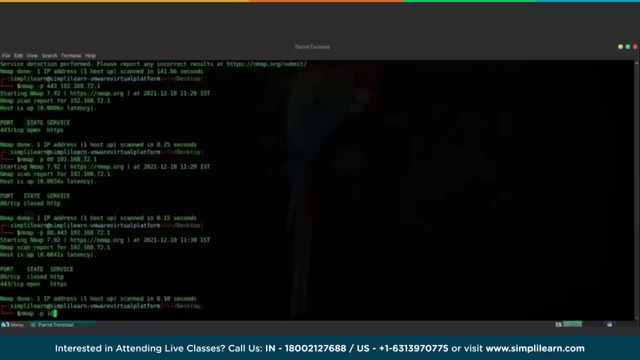 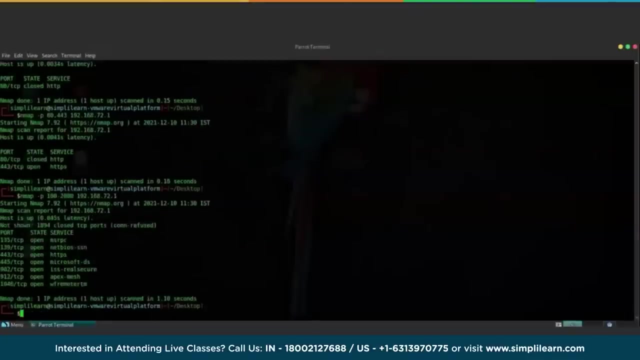 nmap minus b, we're going to check what ports are open between 100 to, let's say, 2000. this acts as a range. everything else is the same and it checks all ports in the range of 100 to 2000. whatever ports is open in between that range, it can be mentioned over here. 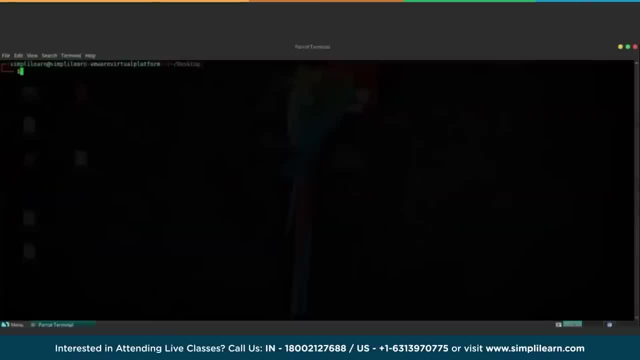 we're going to clear the screen now. another flag that can be used with nmap is the ss command. this runs a stealth scan which is a little harder to detect if you're the it admin of the system, that is being scanned and the results will more or less be the same, although this will need elevated route privileges. 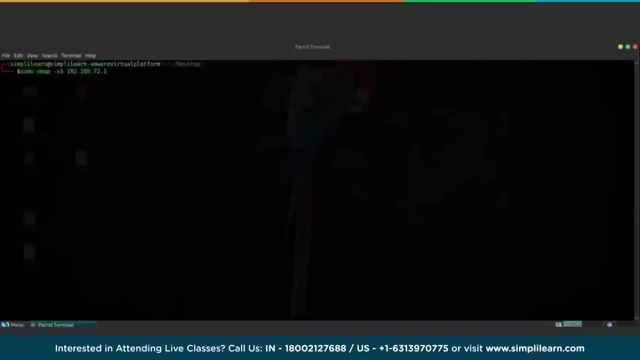 2.1. as you can see, this is more or less similar to a port scan. it just adds an extra mac address as well for good measure. but, like i said, it's more about the stealth. the normal scans usually are easier to detect when the logs are being checked. stealth scans are relatively tougher to check, so i'm 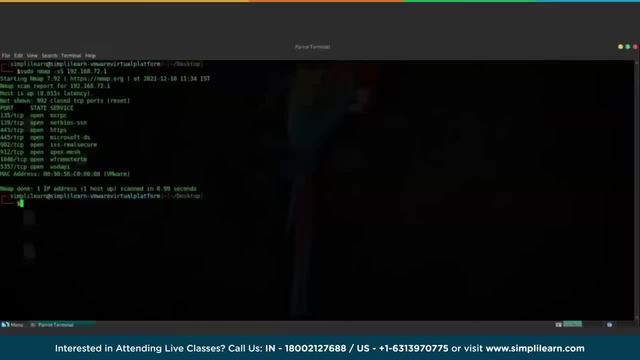 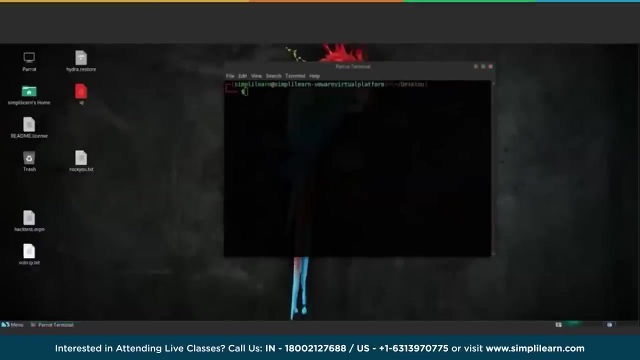 on much more intricate systems. this takes longer as well. now that we're done with both scanning, let's look at a vulnerable machine. the system that is scanning right now is this, my own personal system, with everything is pretty locked down as much as it can be. there is an attack box running in the cloud. the ip address of: 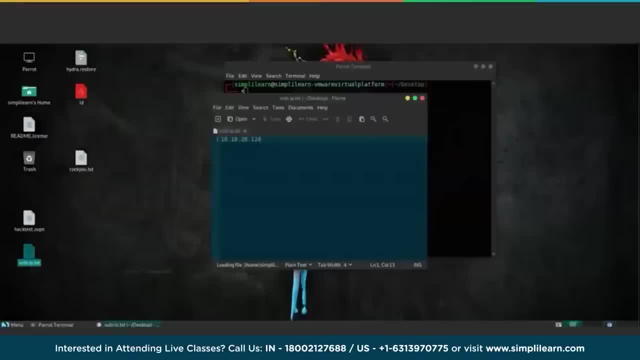 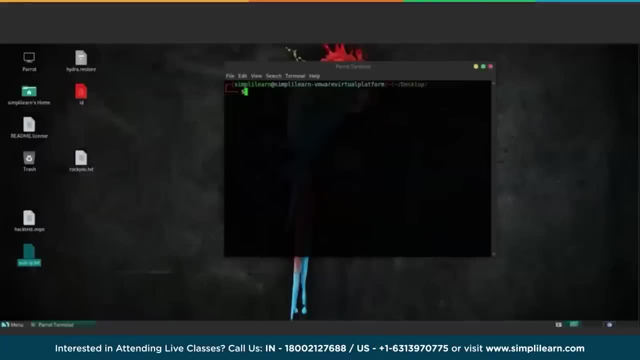 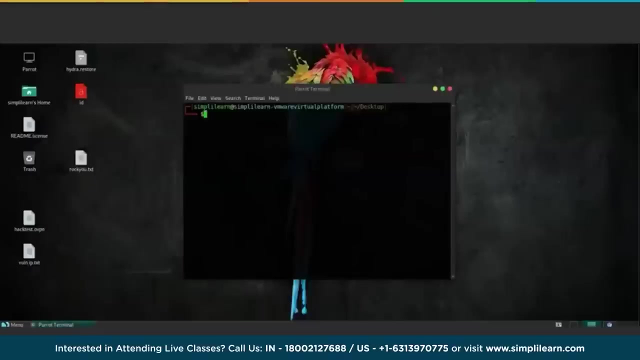 which is over here now. to be able to get into this network, we need to go to the cloud and we need to this network. we need to connect to their personal network using a vpn. so what i'm going to do is switch to a different workspace over here. i'm going to open a terminal and, if you can see over, 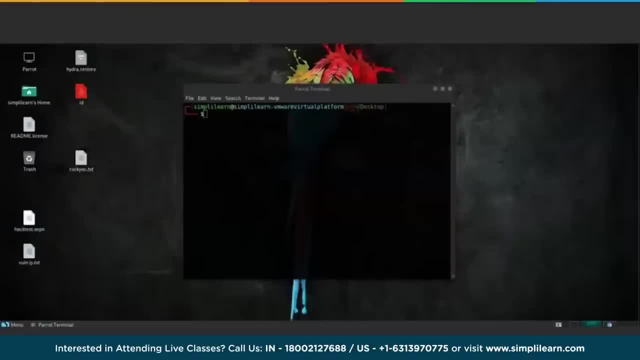 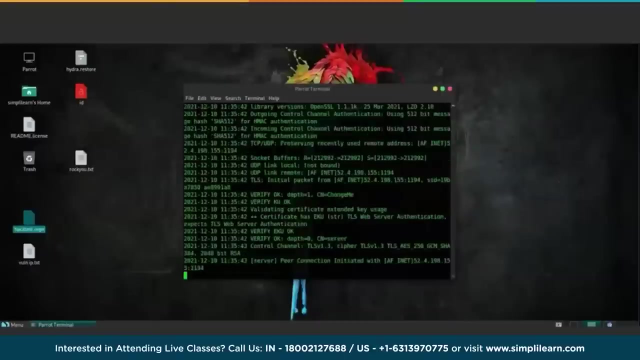 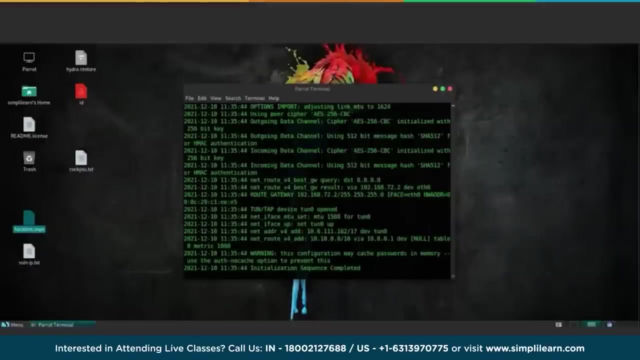 here there is a hack test dot ovpn file. i'm going to connect to their vpn network using this ovpn file and once we get the initialization sequence completed message, we know that the connection has been established. like we discussed, this is the vulnerable device ip. we're going to copy this. 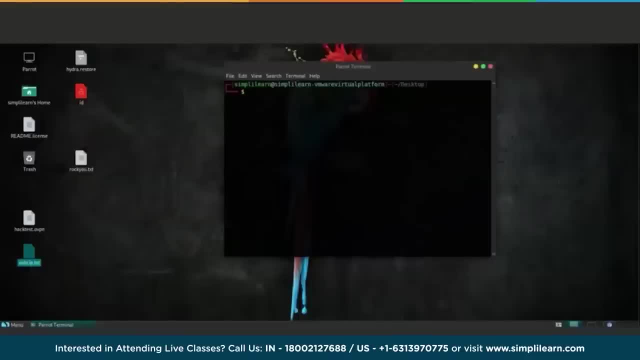 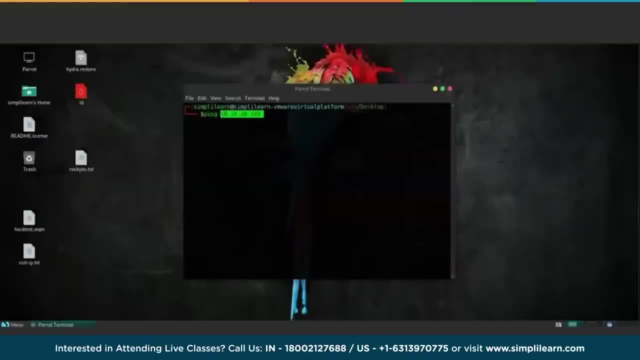 and we're going to try to ping this. let's open a new terminal. we're going to try to ping this and check if we are searching for ultimate device to ping this and check if we are able to reach this machine and, as you can see, we're getting. 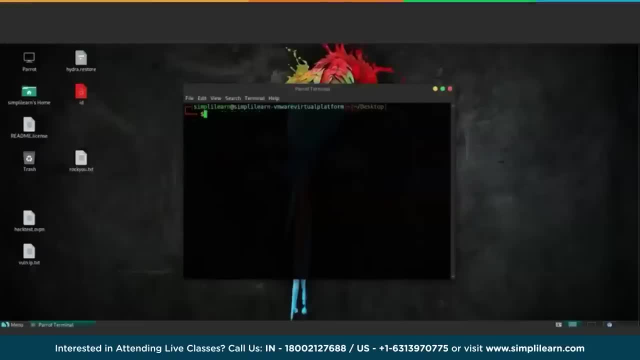 a reply back, which means we are now part of the local network where the vulnerable machine is present. let's run a service scan map with the respective versions. we ran the similar scan on my local machine. we were able to detect what version each service was running what. 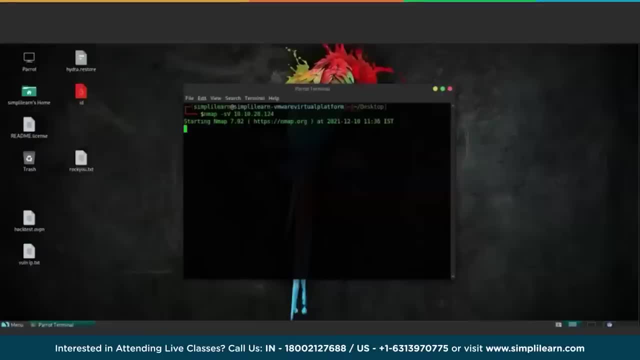 we're going to do over here, based by checking what kind of services are open on the machine running on the cloud. we're going to decide what we are going to do next and we're going to see if nmap alone can point us to a direction where we can gain access to the machine. 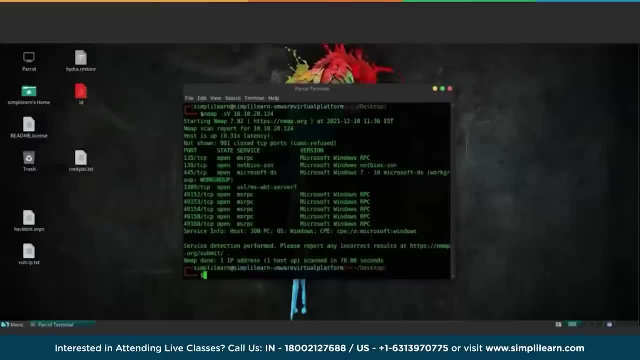 as you can see, the scan is now completed and we have some of the ports that are being opened over here and what kind of services are being opened here. they are running Now. like we discussed, this is the first stage, or sometimes even the second stage, of ethical hacking. What we can infer from here is: what are the 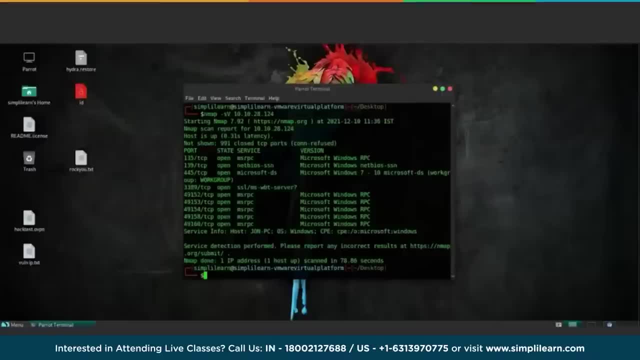 services that are being run Now. these two ports, 139 and 445, are actually Windows SMB server ports which are above the Windows Samba server. Now every service has a particular port attached to it. that will be consistent. whichever machine you may use, Apache server will always run on port 80.. SMB servers will 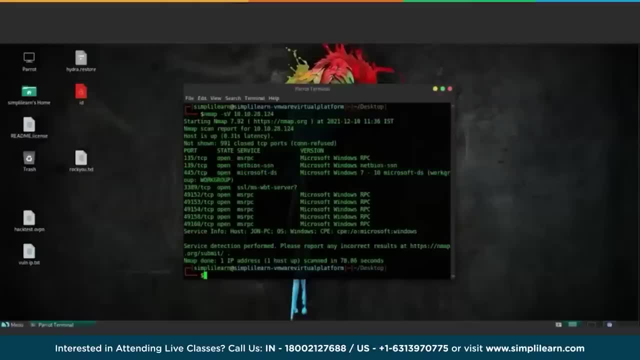 function on these two ports. Now SMB servers have had a vulnerability known as the eternal blue exploit, which was pretty well known. As of right now, from the scan results, we are not able to detect if this machine has the similar vulnerability or not, But since it has the SMB server, open it. 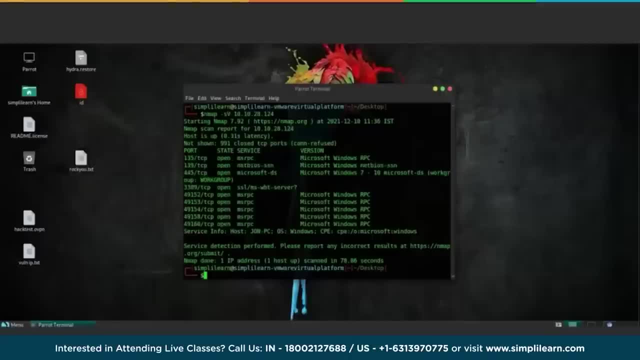 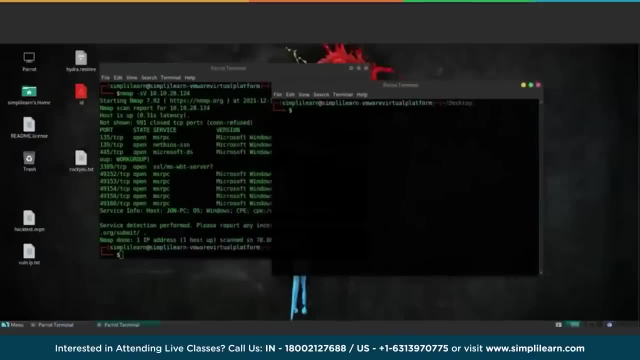 it's worth a shot that we try that exploit on this machine. now to start the exploit on this, we're going to open another terminal over here and we're going to use metasploit for trying the exploit there. we're going to write sudo msf console. msf console is the keyword. first launching the. 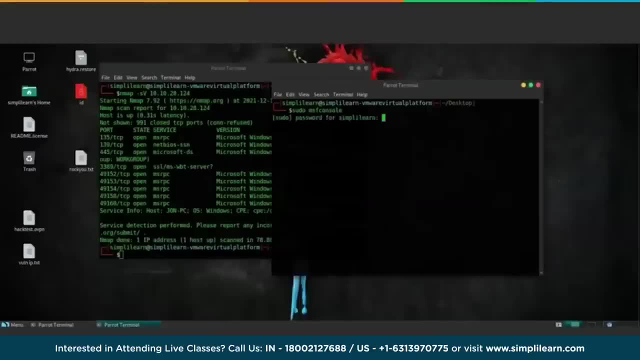 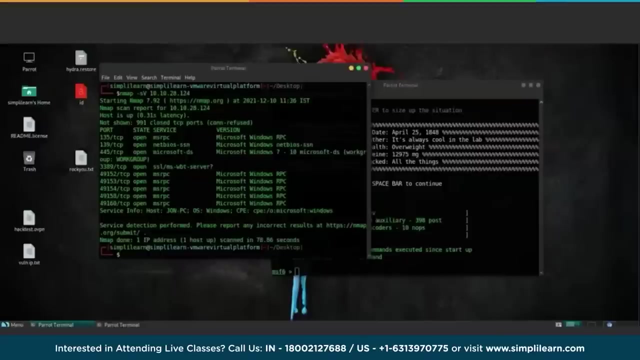 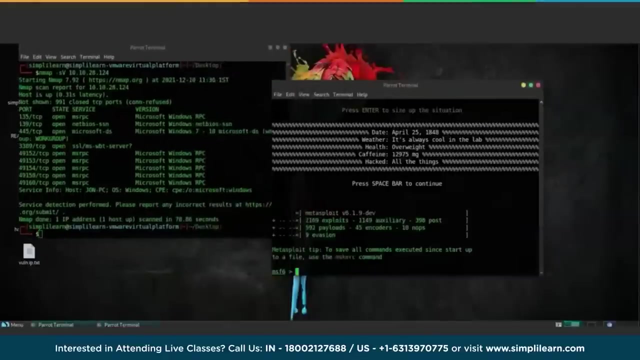 metasploit console, enter the root password and wait for metasploit to launch another than the ports. we can also see that it has checked the host name of the system and the operating system as well. now that the metasploit is open, we're going to launch the exploit now. before launching, we're going 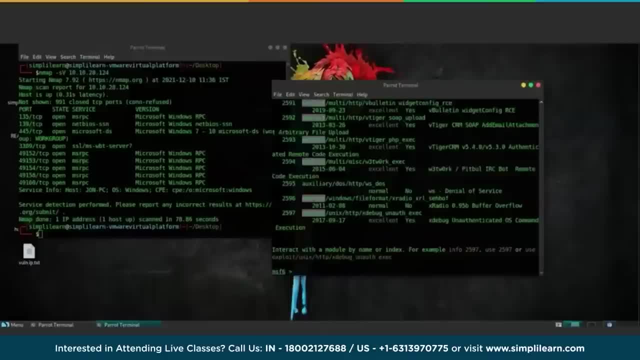 to have a crash run the exploit, you have to invite some people into the plugin, like me, to check what exploits are there for the eternal blue vulnerability. We're going to write use exploit blue and we're going to check what kind of results we are getting over here. 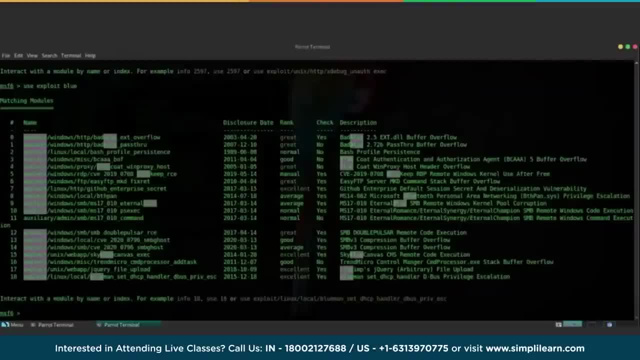 As you can see, serial number nine exploit windows smb ms-17010 eternal blue- It was first disclosed in 2017- and smb remote kernel pool corruption. Let's say we're going to use this particular exploit Now. all of this may be confusing if 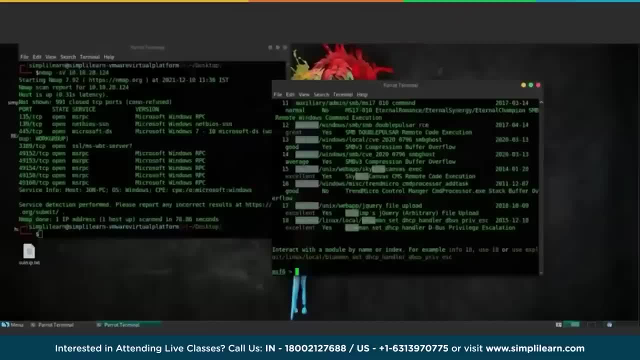 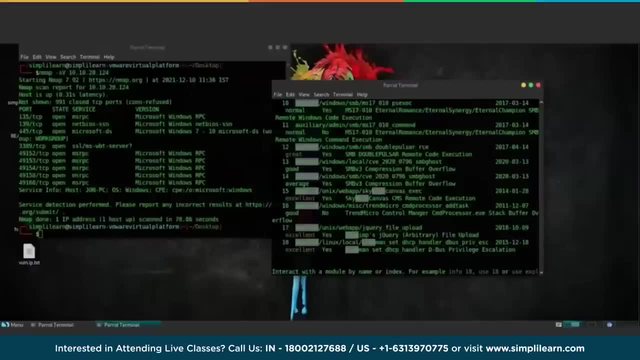 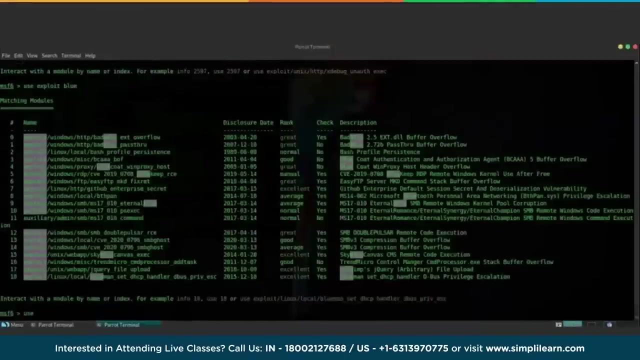 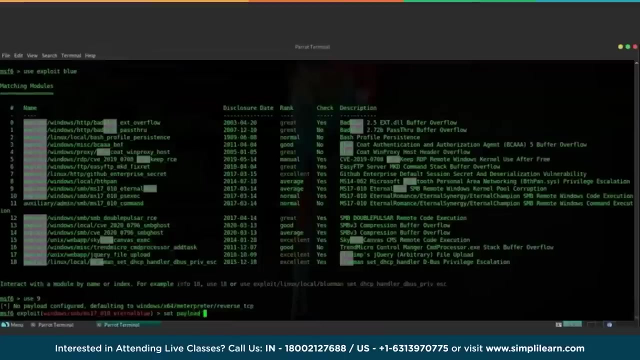 you're not aware of Metasploit, but remember this is the next stage of ethical hacking, which comes into the gaining access part. We're going to use exploit number nine, as we found above to use exploit number nine. Now we're going to set a payload, which is our malicious code that will run on the victim machine. 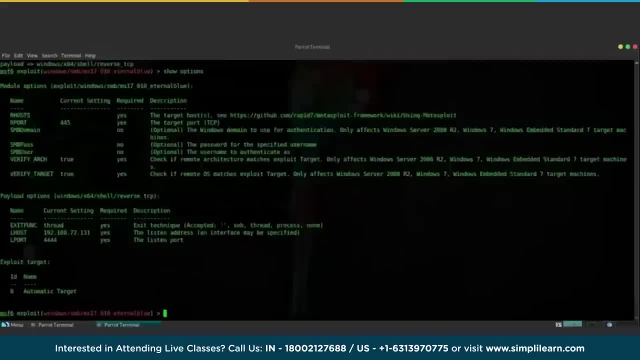 Now we're going to check some options. As you can see, it has by default pointed it to the 445 port, since that is the port where smb server can be accessed from. The parameter that's missing over here is our host, The. our host is the ip address of the vulnerable machine. 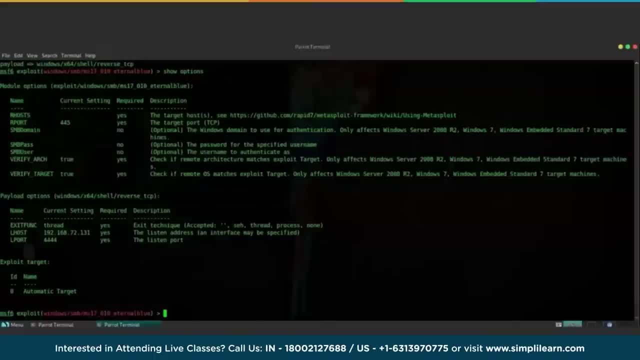 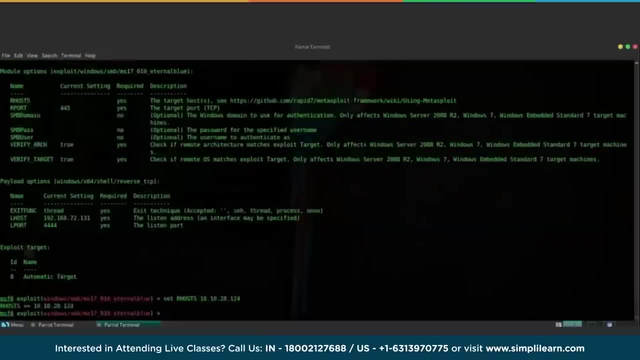 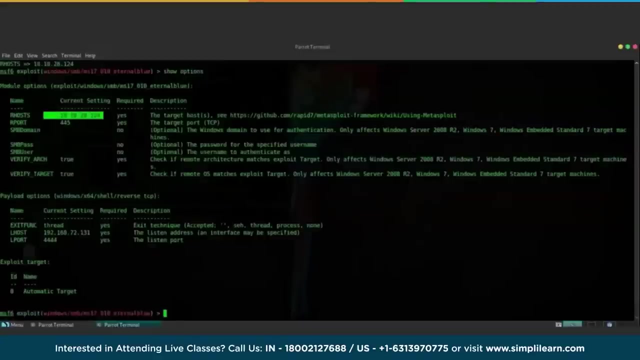 Basically the machine in which we want to attack. Now I'm going to use the set command to set the ip address. Now, if we check, we now have a victim ip address set. Another parameter that we can change is the lhost. This is: 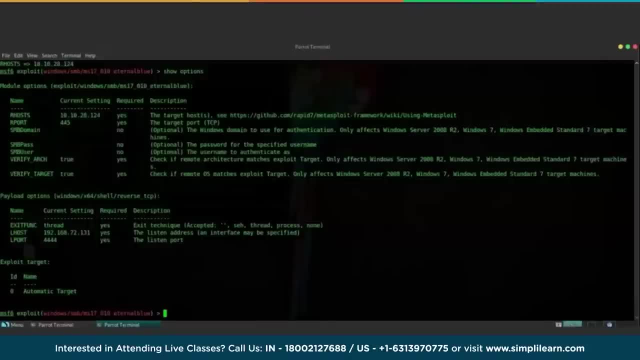 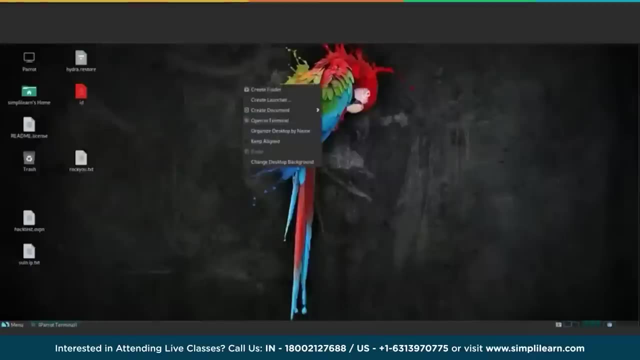 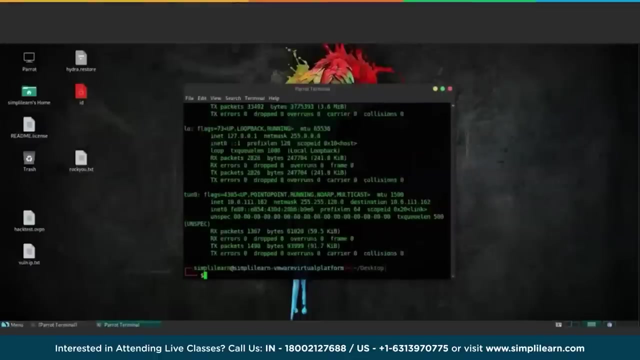 basically the ip address of our own system where we are going to gain access. Now, if you remember, we had connected using a vpn, So we're going to be assigned a new ip according to the vpn. So if we write ifconfig and check this one tun0 is the vpn adapter. This is our ip address. that 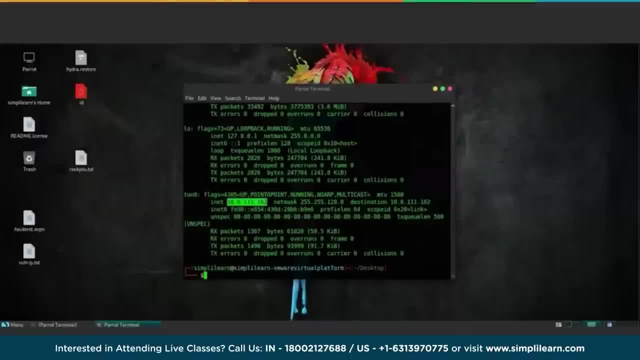 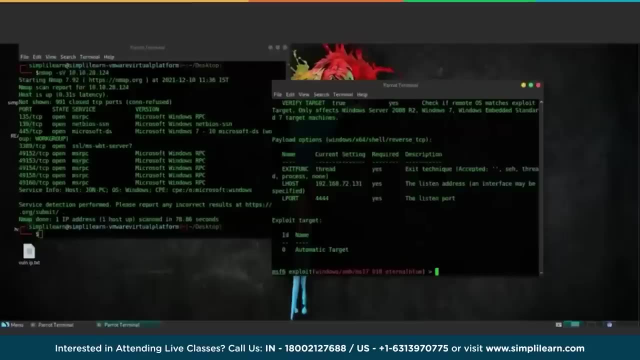 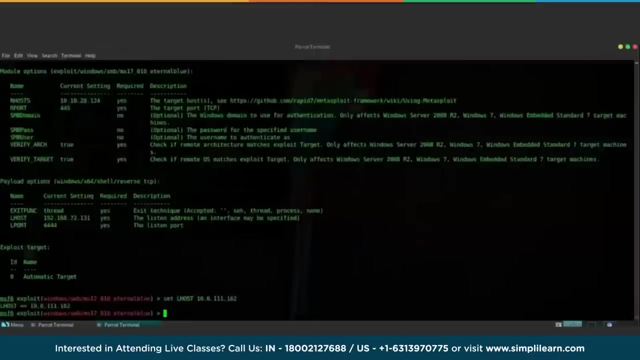 we have been assigned in the server, in the network where the vulnerable machine is present. So we're going to copy this ip address, We're going to move over to this workspace and we're going to set lhost with that ip address. With that, our options are set. Now we're going to run exploit. 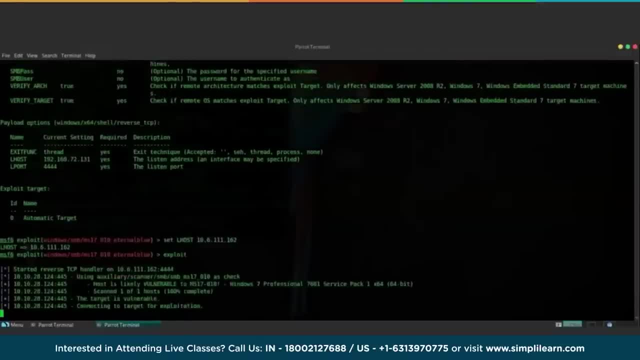 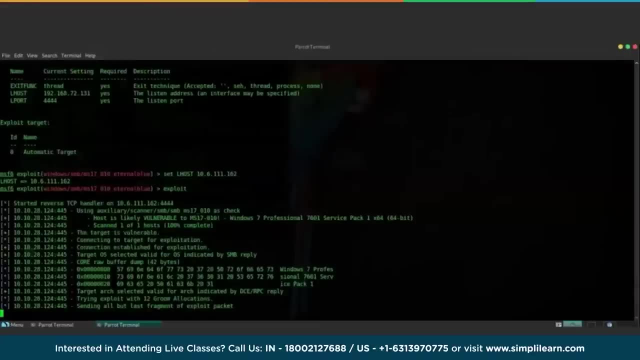 and it's going to check if samba server vulnerability is present. As you can see, it has written that the target is vulnerable to this particular exploit. It's going to say that the target is vulnerable to this particular exploit. We're going to send the malicious code and the malicious code is set in the payload that we sent above. 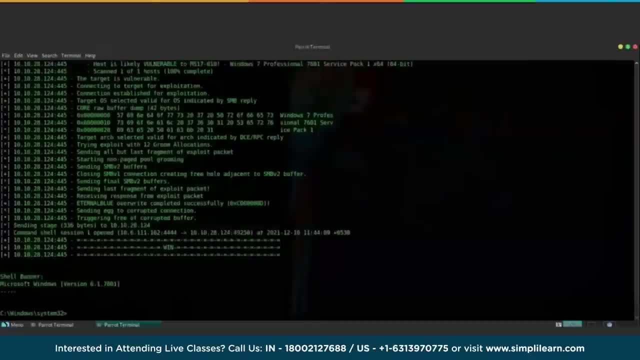 And we now have the shell command of the windows machine. As you can see, see windows system32.. To be sure that this is in fact this windows machine that is being used, we're going to write ipconfig, which is a windows system32.. This is a windows only shell command. 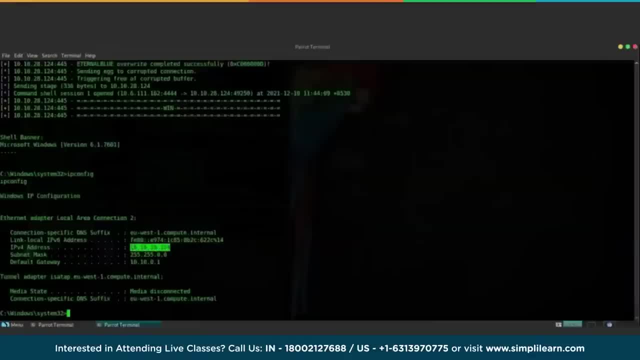 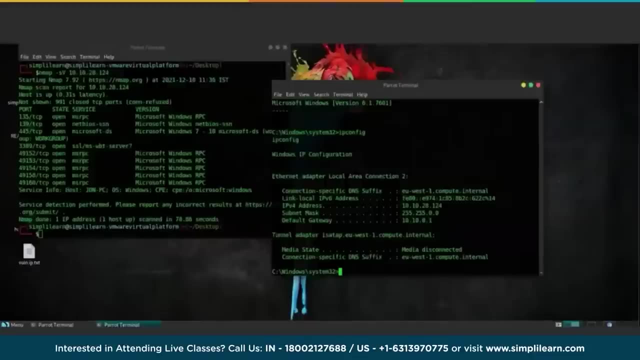 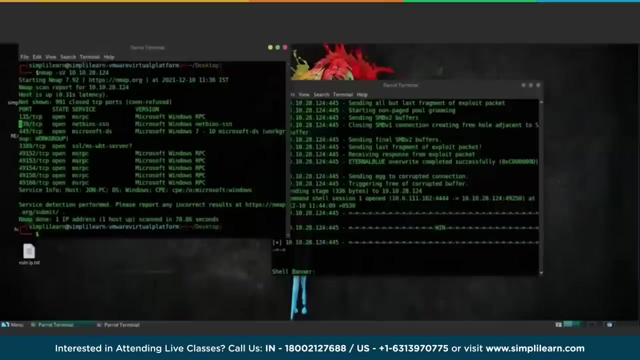 As you can see, this is the ip address that was assigned to the victim machine. Now, while a major part of this process was done on metasploit, we would not have reached this stage had we not found out that the 139 and 445 ports are open. 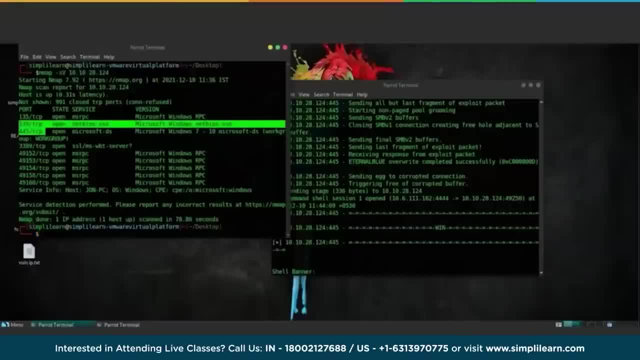 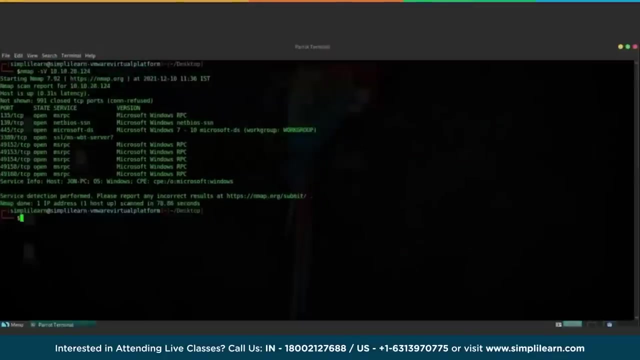 which basically pointed us that we can try the eternal blue exploit of the windows samba servers. Similarly, all the scans that we run serve as a preface to the actual stages, or the actual hacking stages, of the campaigns. This sb command was necessary because we could check what are the exact services that are being running. 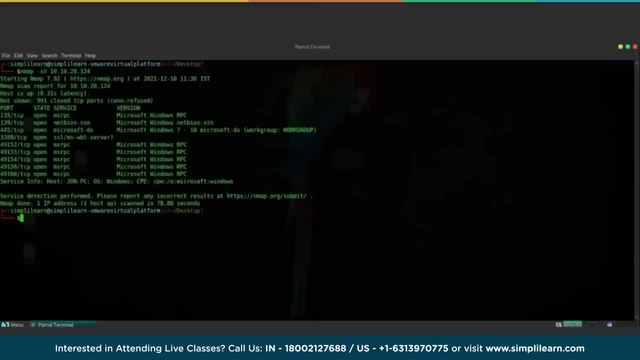 In some cases, if the apache server is being run, there are particular versions which have particular exploits. those exploits will not work on other versions, So we're going to have to check what particular version is being run and accordingly apply the exploit. That can be done in the Metasploit or you can run some other tool. 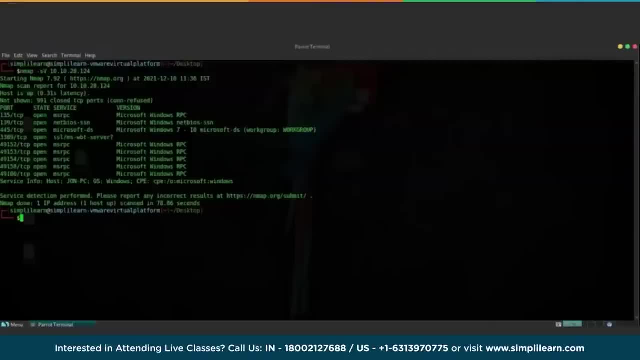 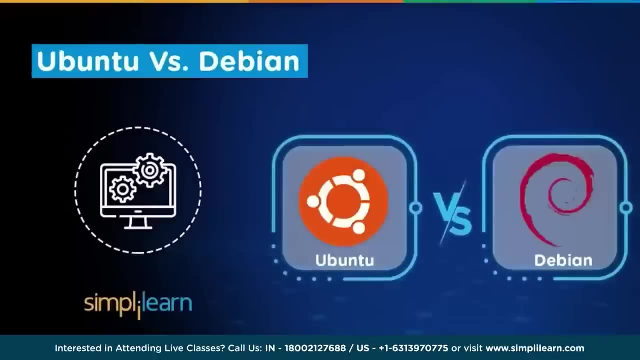 but what exact exploit we have to run and which vulnerability we have to target. that is where Nmap comes to help With the world moving towards the next generation of computer hardware. the software side of things still has a lot left to be discovered. 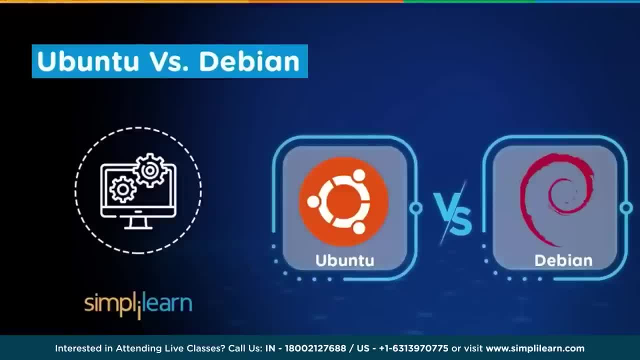 With the majority of laptops coming with Windows pre-installed, many users are devoid of the Linux operating system experience, which is more resource-friendly than the mainstream operating systems. It can be attributed to the difficulty people used to face when installing a new operating system like Linux in the old days. 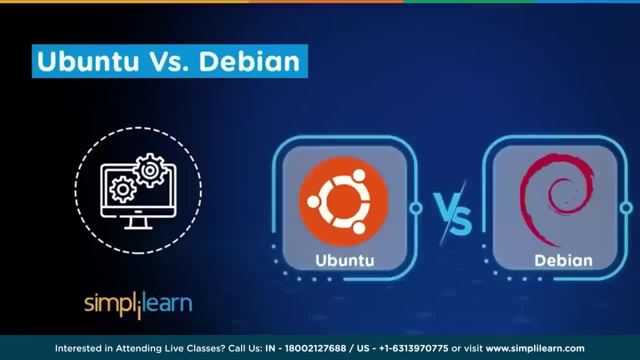 However, a lot of these issues are fixed nowadays thanks to the big names like Debian and Ubuntu, who have been instrumental in making Linux-based operating systems as user-friendly as possible. But which one of them is better for you? Let's take a look at the topics to be covered today as we answer this question for you. 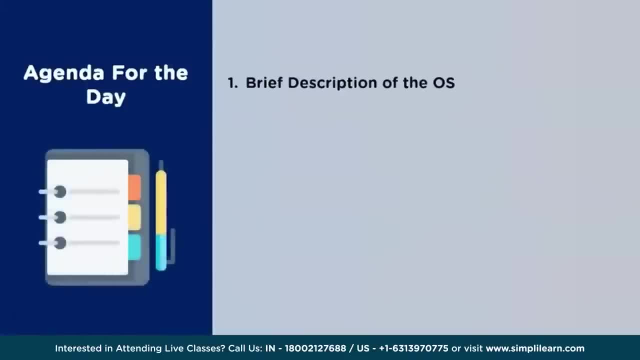 We start by learning about the operating systems from a layman's perspective and uncovering the basic offerings of both entities. Next, we cover the unique features of both Ubuntu and Debian and how they stack up against each other and other industry counterparts. 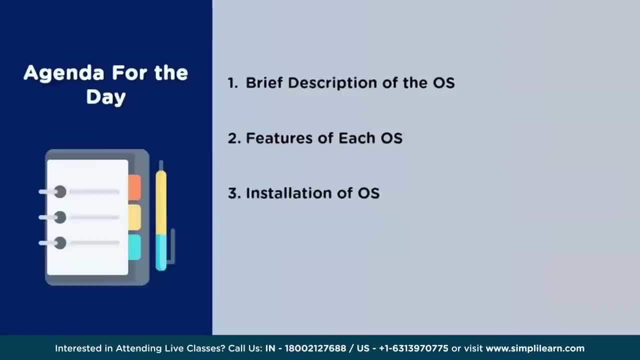 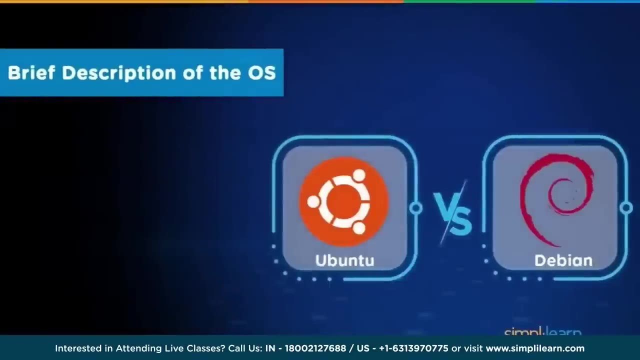 Moving on, we take a look at some pointers before installing each of these operating systems and their respective download links. Finally, we compare the contrasting features of both Ubuntu and Debian and infer the kind of users which each OS caters to. So let's start by learning about Ubuntu and Debian in general. 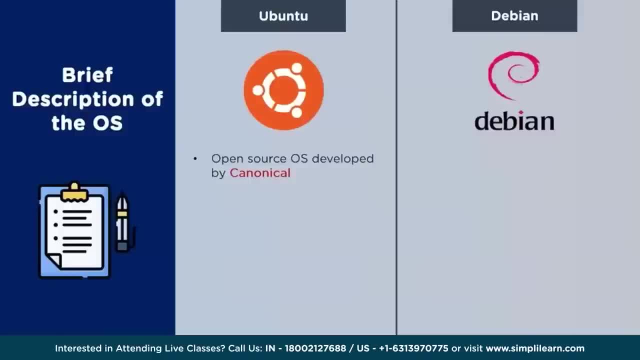 Ubuntu is an open-source, free Linux distribution. It is an operating system for cloud computing in accordance with support with OpenStack. Ubuntu is developed by the Canonical community and it is freely available. Also, Canonical Limited is responsible for the funding of Ubuntu. 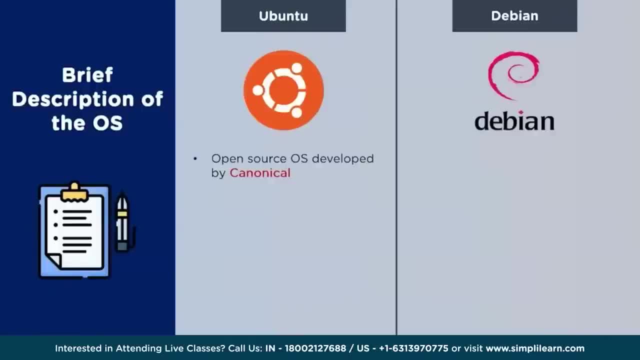 Basically, Ubuntu is released every six months. Free support is available for nine months after every release, and long-term support, which are the LTEs, is released every two years. The first release of Ubuntu was in October 2004.. You must have heard about Ubuntu, no matter what. 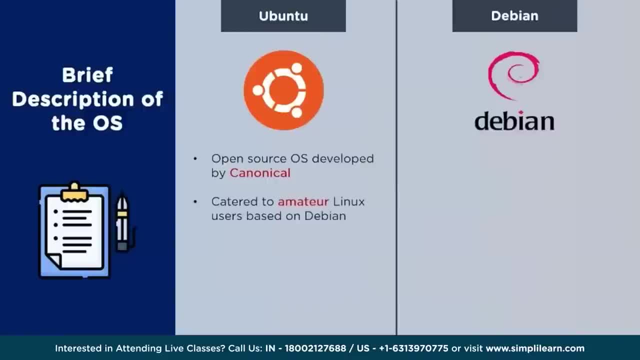 It is the most popular Linux distribution overall, not just limited to servers, but also the most popular choice for Linux desktops. It's easy to use, offers a good experience and comes pre-installed with essential tools to get a head start. 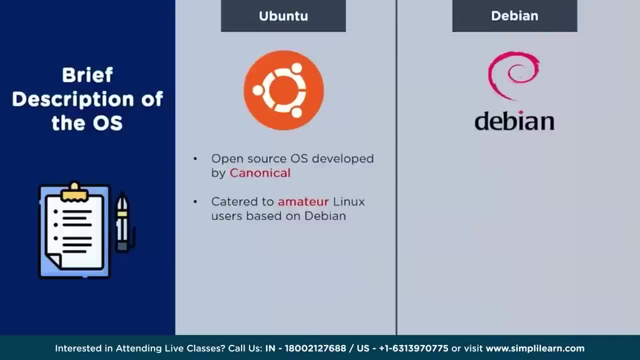 Of course, Ubuntu managed to simplify the Linux experience years back, and that is the reason why it is still so popular, even with several impressive Linux distributions available right now. Every new release is more polished and comes loaded with new features and improvements. 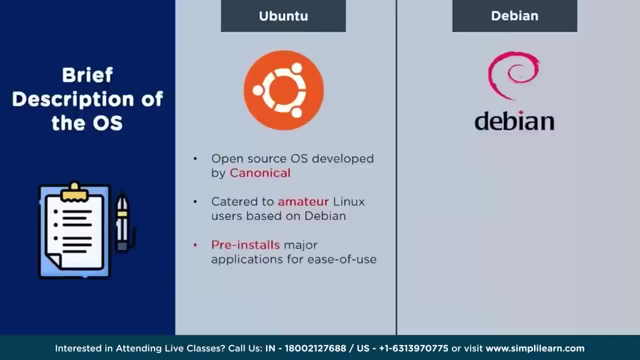 Thanks to its huge user base, a number of software vendors have made their applications compatible with Ubuntu. While the catalog may not be as extensive as Windows, the options are still well-curated. More importantly, the advantage of Linux is that most of the Linux-based operating systems 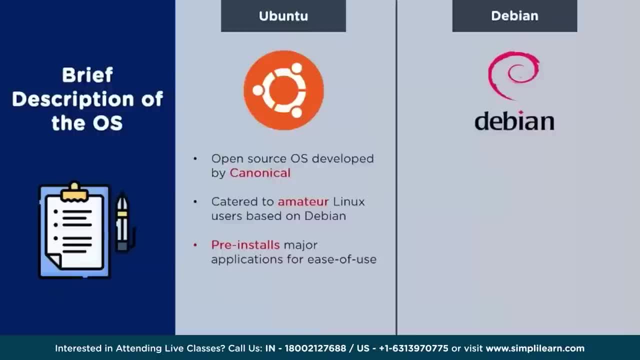 is the ability to use free and open-source alternatives to major proprietary software. While lacking some polish and overall features set, most alternatives are enough to get the job done for the majority of the users. The never-ending community support also helps in troubleshooting should things go wrong at any point in time. 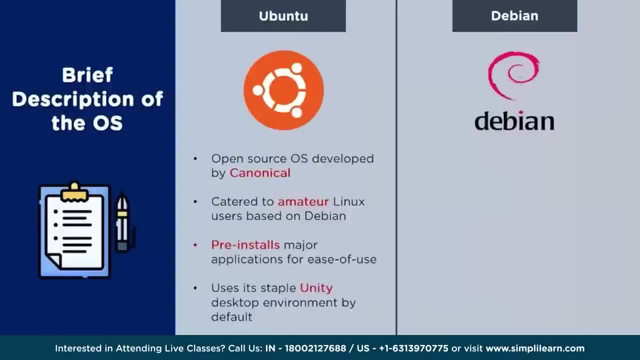 The default desktop environment in Ubuntu is GNOME or Unity. The Unity is a modern desktop environment and is a powerful search tool for finding all your applications and documents. with its base setup as GNOME, It integrates well with common applications such as audio players. 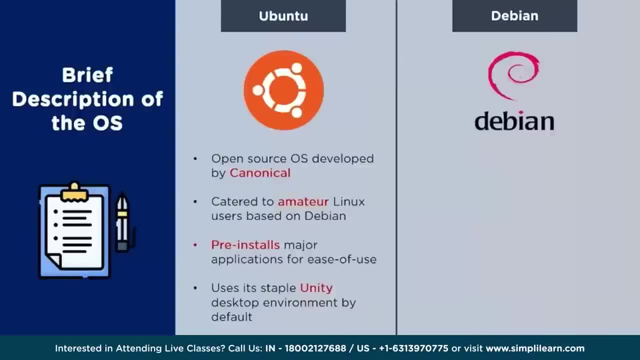 video players and social media. There are a few other desktop environments for Ubuntu as well, with Unity as its flagship environment. Debian, on the other hand, is a free operating system for your computer, which started in 1996 and is maintained by global contributors. 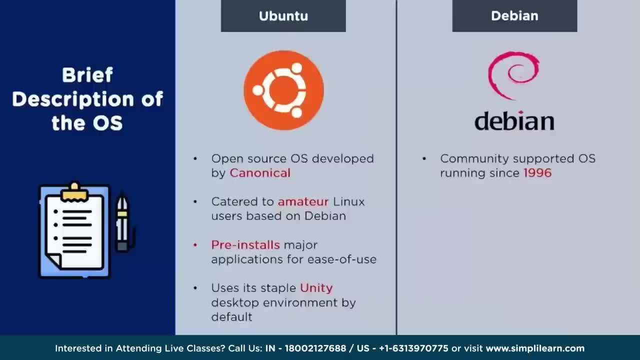 If the operating system, a set of basic programs and utilities that make your computer run, its core is the kernel. The kernel is the most fundamental program on the computer. Debian uses the Linux kernel, a completely free piece of software which was started by Linus Strohwalz. 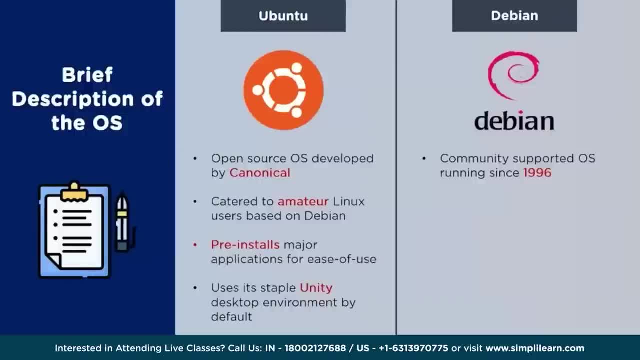 and supported by thousands of programmers worldwide. A large part of the basic tools that fill out the operating system come from the GNU project, and those tools are free as well. Debian is the mother of Linux distributions. Beginners always wonder why this not-so-good-looking 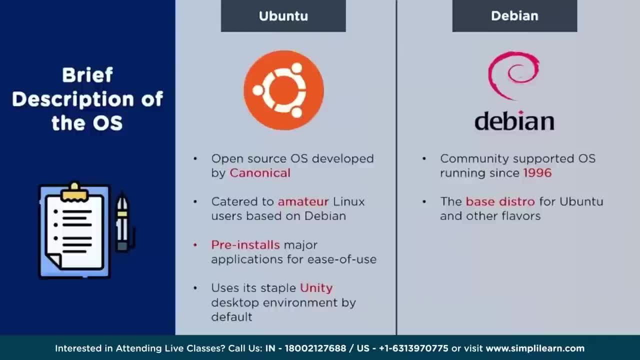 easy-to-use-distro is so popular inside the Linux developers' community, especially when there are a lot of modern distributions that are easy to use and have beautiful UI. Later on, they found out the power of Debian after using a bunch of distributions from other developers. 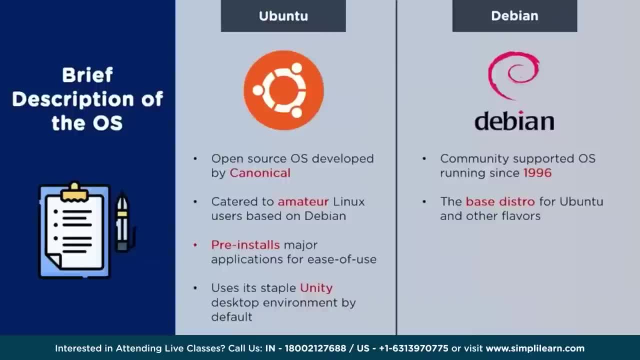 You will be surprised to know that almost all other popular consumer-level distros are based on Debian, even Ubuntu. It is so stable and feature-rich that the developers find it easy to build their distros based on Debian rather than building it from scratch. 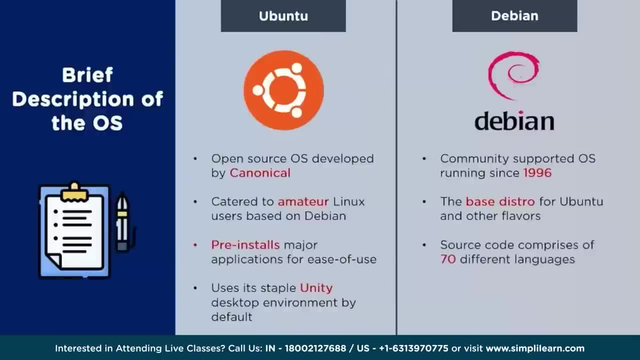 Debian is run and maintained on its GitHub repository thanks to contributions from developers worldwide. The major decisions are taken up on the Repository Issues tab, leading to community-wide feedback and a holistic approach to open-source development of the Debian operating system. Thanks to this variety of personnel, 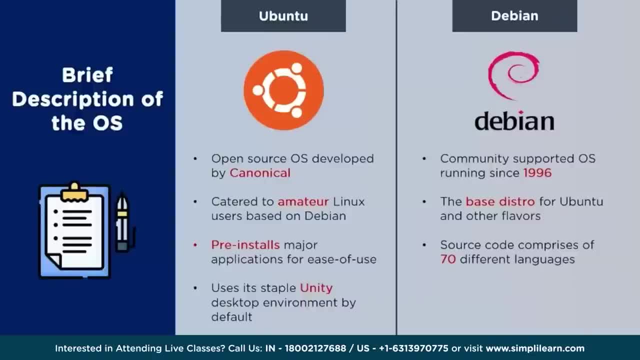 the source code of Debian comprises around 70 different programming and scripting languages. Debian supports all kinds of graphical environments, ranging from full-featured desktop environments to lighter alternatives and even minimalist window managers. Ubuntu ships with Unity desktop by default, but the package manager can install the GNOME environment if needed. 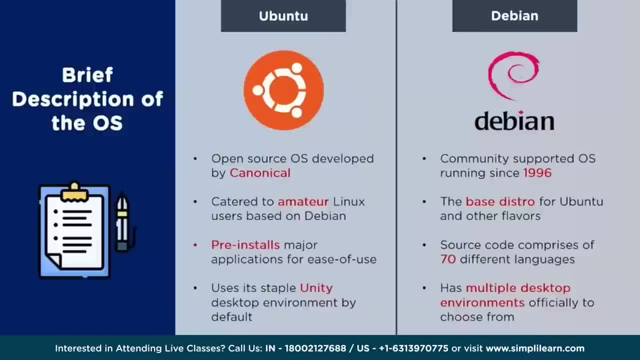 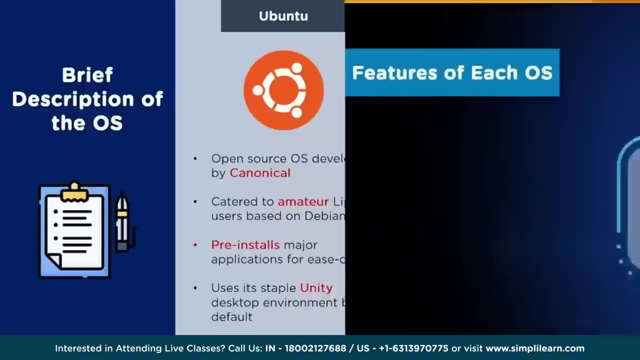 while also including Cinnamon, LDexD, Xfce, KDE and Mate. On the other hand, Debian gives you the choice of choosing which desktop environment you want from the get-go by providing ISO files for each desktop environment individually. Now that we understand. 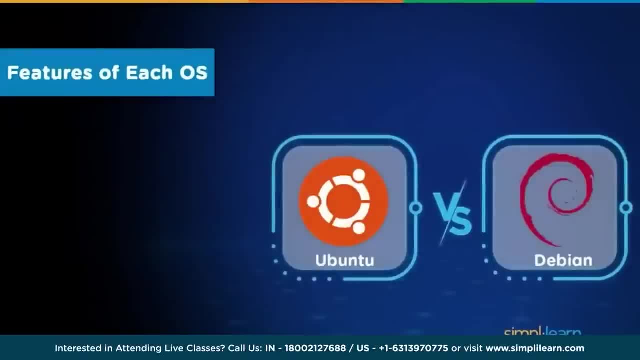 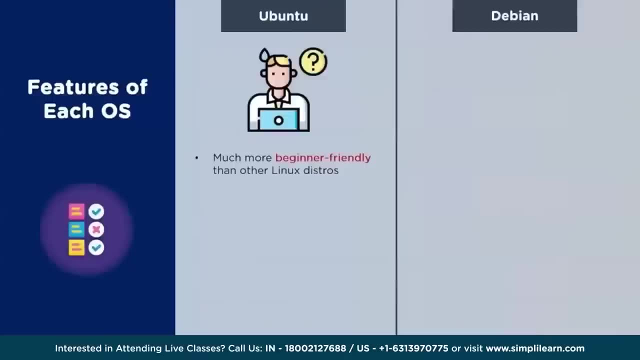 where both these operating systems stand. let us take a look at some of the best features offered by each of these distributions. Ubuntu is the closest thing to a household name among desktop Linux distributions. It is a great distribution to start with and it's even a great distribution to keep using after you're more experienced, if you're happy with it. 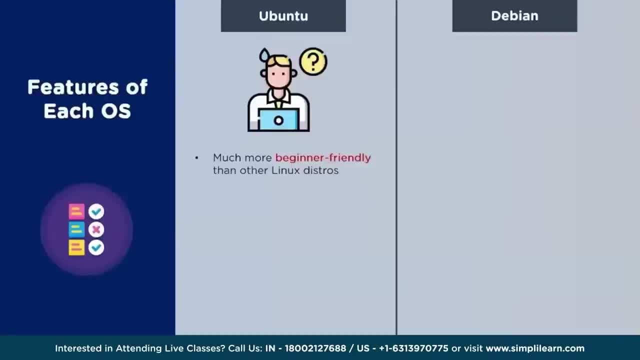 It is user-friendly in a lot of ways. It provides a simple desktop, has an easy installer and provides a checkbox during the installation process that will automatically install it. You can install Flash plugins and various codecs that you will need for multimedia support. 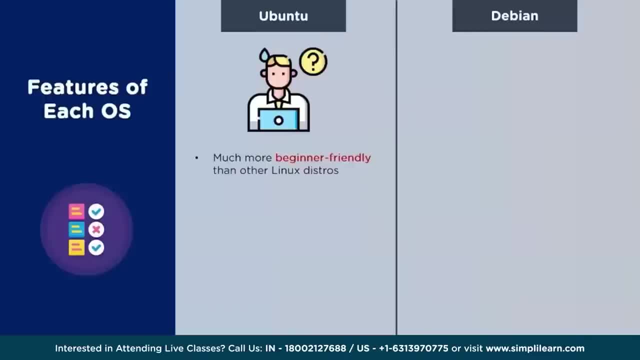 There's an additional drivers tool that will detect closed-source or proprietary drivers that might be necessary to get all your hardware working and easily install them for you. Ubuntu is produced by Canonical and their friends. It is run as an open project to enable others with diverse ideas. 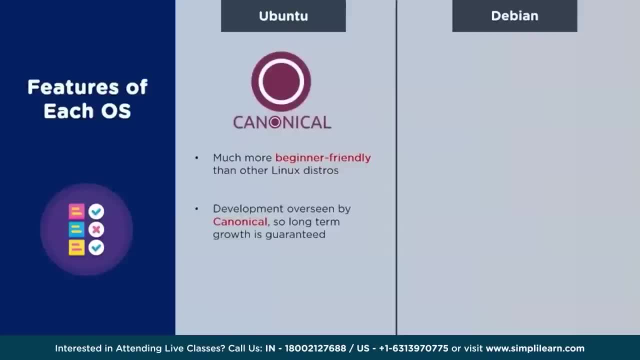 to benefit from all the work the developers do to deliver the world's best open platform. Still, Canonical is responsible for delivering six monthly milestone releases and regular LTS releases for enterprise production use. Enterprises can count on Canonical to support, secure and manage Ubuntu infrastructure and devices. 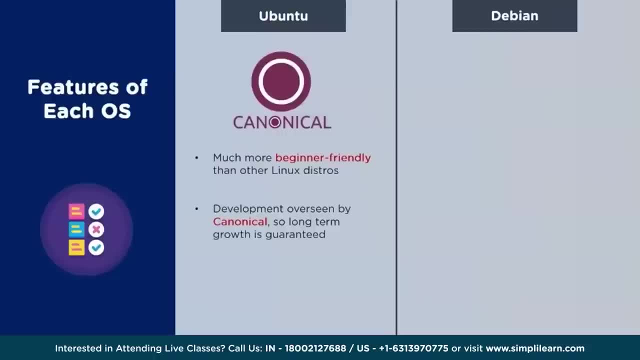 With more than 500 employees in over 39 countries, the company underpins the critical infrastructure for thousands of businesses and millions of Ubuntu users around the world. Unity Desktop was originally developed by Canonical and introduced early for netbook computers with Ubuntu 10.10.. 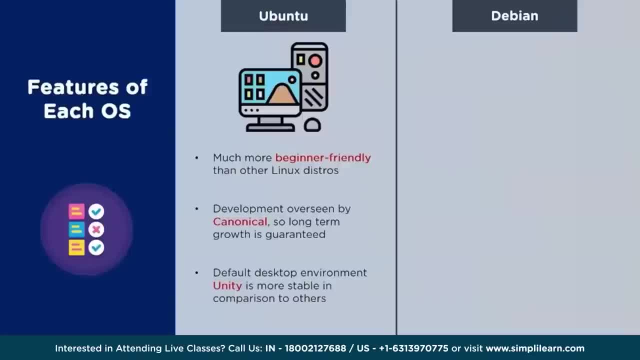 Then it went on to be the default desktop environment for Ubuntu. Eventually, it has been dropped by Canonical and replaced by GNOME. However, it has made a comeback after Ubuntu 18.04.. While being completely stable, the HUD and global menu hold up just fine with major applications. 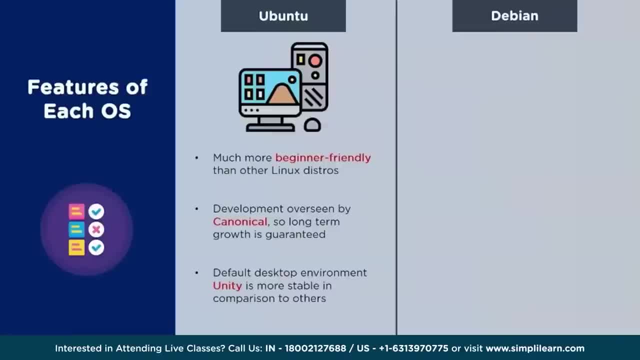 such as LibreOffice, Thunderbird and other web browsers. That means that the Unity desktop works as it is supposed to, while making you more productive. While some desktop environments have a steep learning curve, Unity is very intuitive for new users, in spite of deviating from the traditional. 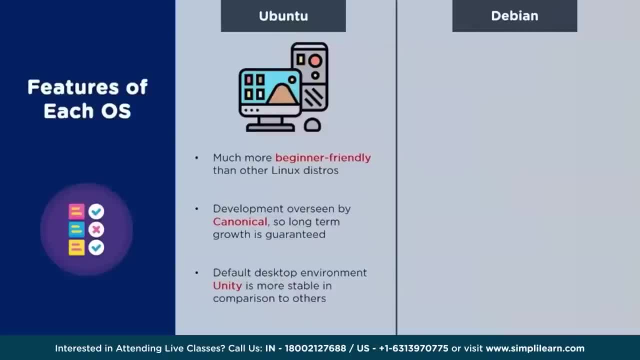 start menu format that the Windows users are generally accustomed to. The Calamares installer is a framework. By design, it is very customizable in order to satisfy a wide variety of needs and use cases. Calamares aims to be easy, usable, beautiful, pragmatic and, more importantly, distribution-agnostic. 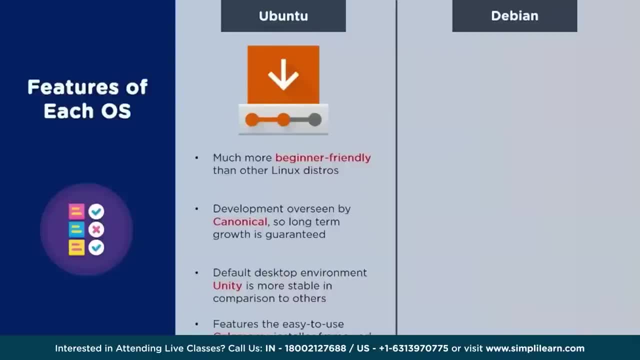 Calamares aims to be easy, usable, beautiful, pragmatic and, more importantly, distribution-agnostic. Calamares aims to be easy, usable, beautiful, pragmatic and, more importantly, distribution-agnostic. Calamares includes an advanced partitioning feature as well. 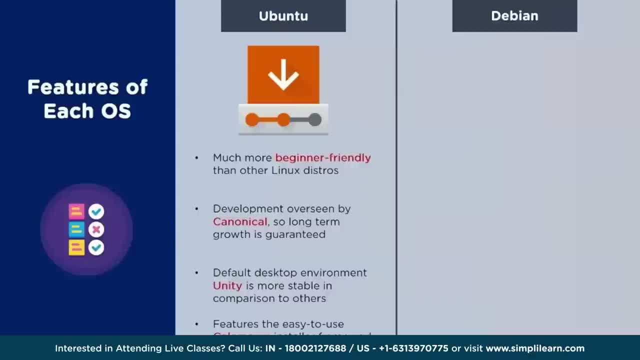 which supports for both manual and automated partitioning operations. It is the first installer with an automated replace partition option which makes it easy to reuse a partition over and over for distribution testing. Coming to Debian, it is a community distribution through and through. 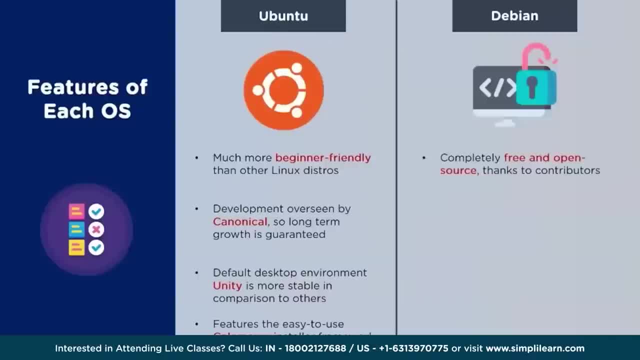 It's governed by a board of elected developers, It has its own internal structure and laws, and just about everyone working on it is a volunteer, making it completely community-driven. It is maintained and developed by programmers and developers all around the world. This form of development ensures continuity If one of the developers decides to stop working. 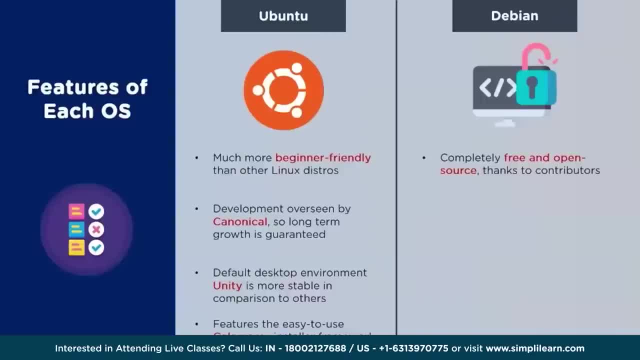 on the project. another developer might come in and take place and keep the project going on. It is completely free of centralized control and this is also one of the reasons for an undecided stable release cycle. Debian SID is the permanently unstable development version of Debian. It is where the latest versions 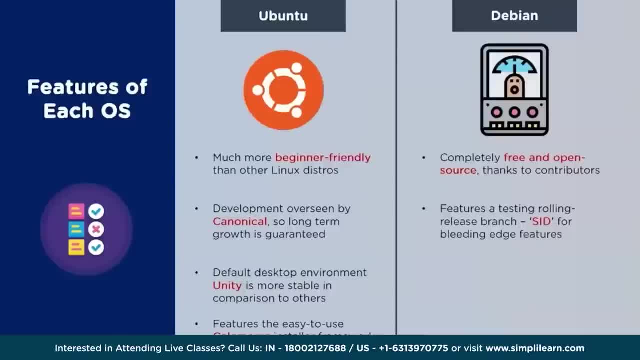 of programs are being considered for inclusion in the Debian release cycle are uploaded and tested. Because it has no official install media and the few netboot images that are built often don't work. even people who are willing to risk using a development version may have trouble installing it. 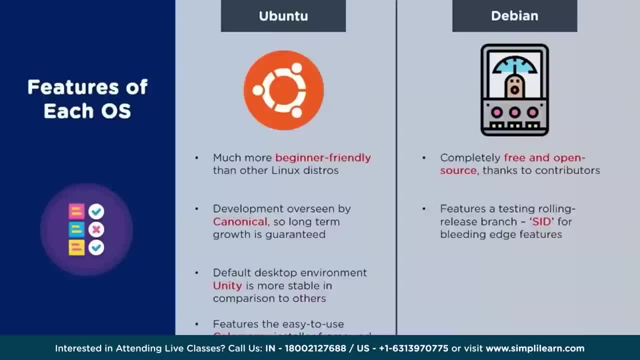 However, it still remains the best place to test new features that have not yet made their way onto the stable branch. Debian has only free and open-source software in its repositories. This is mostly ample for our users, except for users who use Debian SID. Debian has only free and open-source software in its repositories. This is mostly ample for our users, except for users who use Debian. Debian has only free and open-source software in its repositories. This is mostly ample for our users, except for users who use Debian. 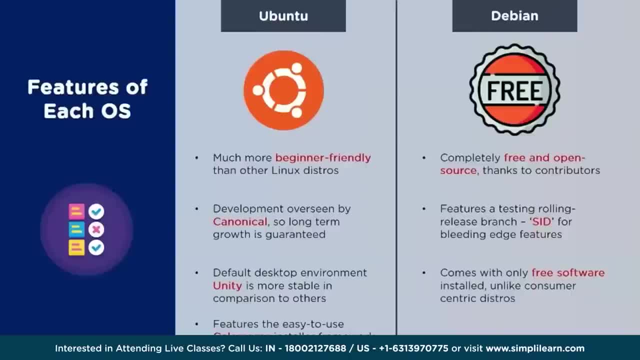 Debian has only free and open-source software in its repositories. This is mostly ample for our users, except for users who use Debian hardware that only has proprietary drivers. These repositories work well in most cases. It is possible to add other repos as well that have proprietary software, if that is the requirement. 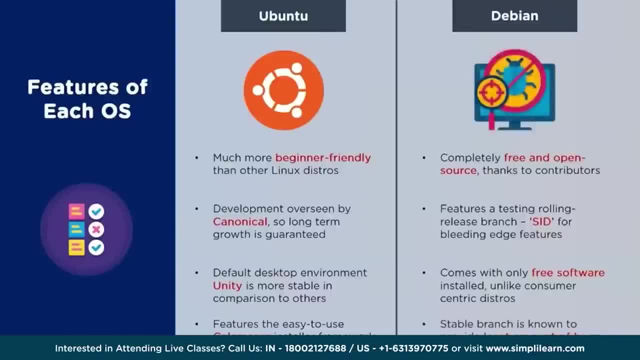 Debian's standard version is very stable, as software and libraries in it go through rigorous testing. This stability makes Debian a perfect server OS, and it's also the same reason why average users shy away from using Debian as their primary OS on desktop. This is also one of the reasons why many developers use Debian as a base for their derivatives. 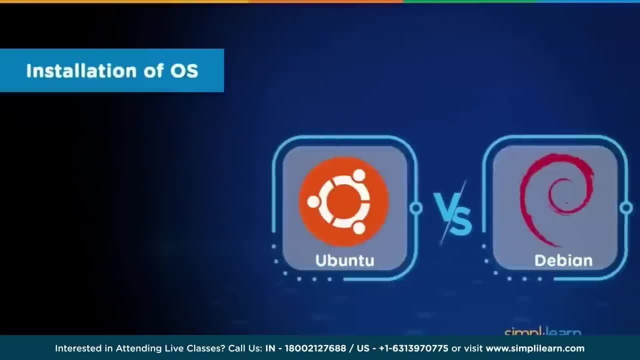 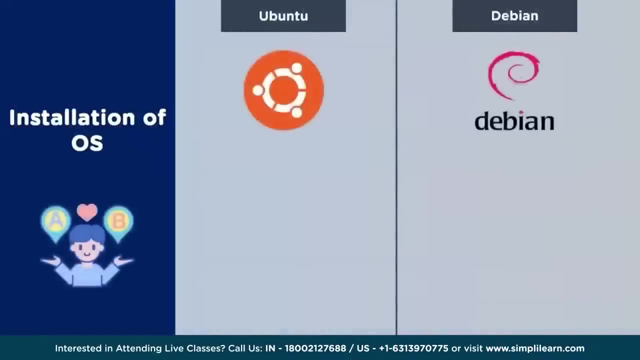 one of which is also Ubuntu. Now that we're aware of each distribution's unique features, let's take a look at how we can go ahead and install these operating systems and where we can get their downloadable images. When it comes to Ubuntu, Ubuntu has dropped the support for 32-bit systems. 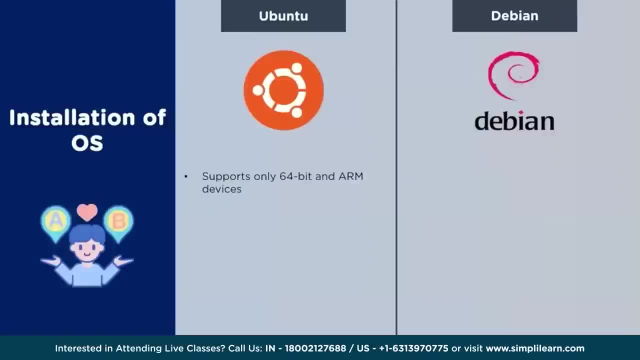 Currently, it supports only 64-bit devices and ARM devices. Installation is easy with the Calamares framework coming into ISO pre-default, and the latest ISO can be downloaded from the link being shown on the screen right now. In the case of Debian, the support for multiple range of 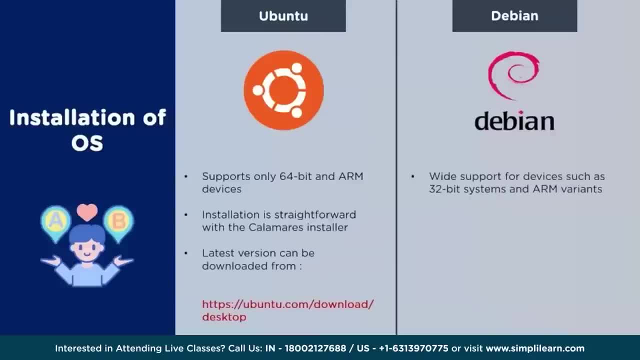 devices is still present. That can also include 32-bit systems and other smaller devices which are not modern. Even though it does not use the Calamares installer, even downloading the ISO file can be a bit hectic for newer users, Considering this is a distribution aimed at developers and intermediate users. 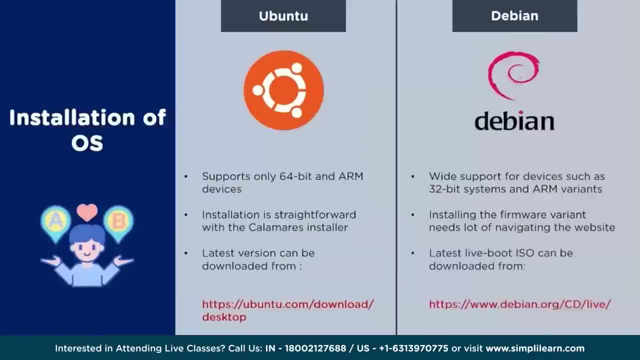 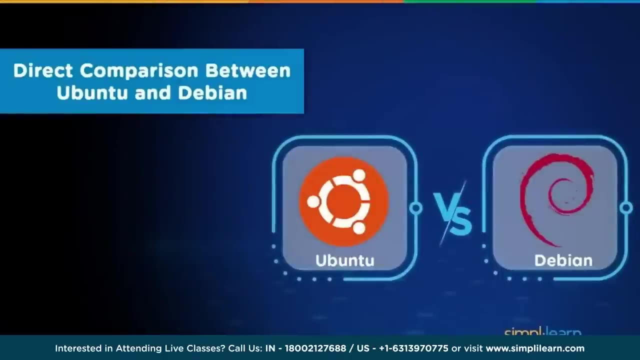 finding the right link can be difficult, because of which we have mentioned the link on the screen below where you can get the latest ISO, depending on which desktop environment you choose to go with. With the installation out of the way, let's take a direct comparison of the features between both Ubuntu and. 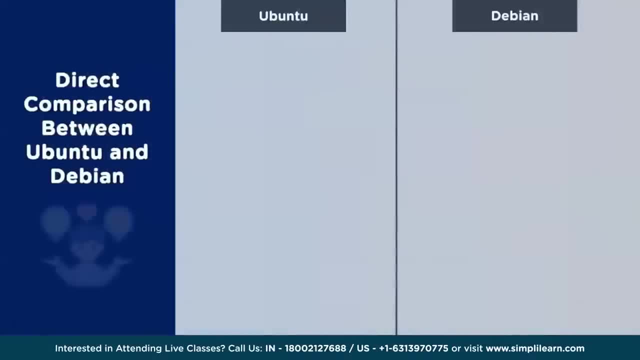 Debian. Debian is a community driven open source Linux distribution and is primarily aimed to be robust, capable and, most importantly, free. On the other hand, Ubuntu is also free on open source, like Debian, but it's backed up and developed by a canonical, which is a corporate company. Debian and Ubuntu are both 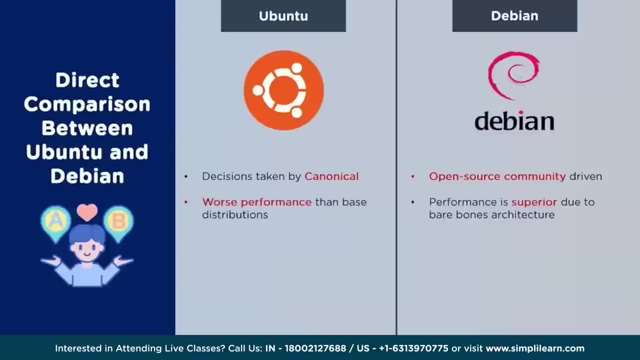 fundamentally fast. regarding performance, As Debian comes bare minimum and is not bundled or pre-packed with additional software and features, it makes it super fast and lightweight, at least when compared with Ubuntu directly. Both Ubuntu and Debian use the same APT software packaging management system. 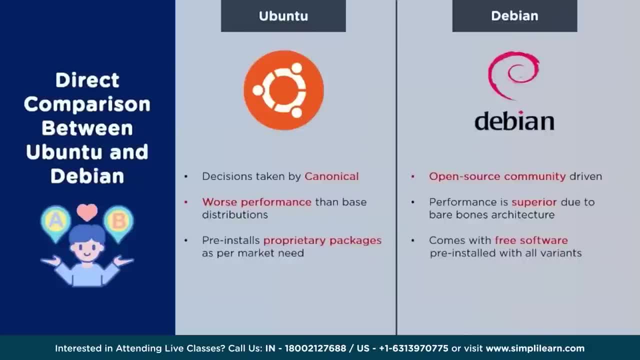 but provide a different software repository. Debian is more like promoting freedom of choosing free software. Thus, it does not include any proprietary software by default. You can always install the paid versions, but you have to enable it manually. Ubuntu focuses on usability, including all the software, including free, paid. 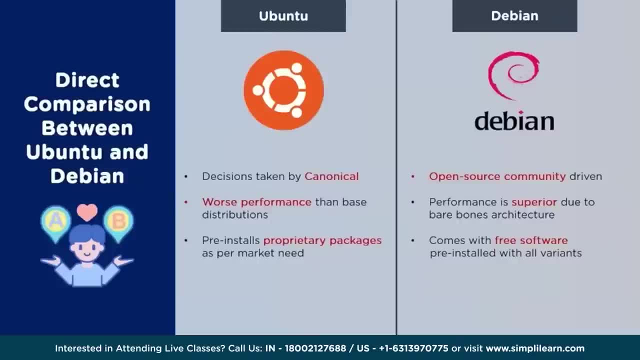 open source, closed source, etc. Ubuntu also introduced a universal package management system called Snap. It will be used across distros and thus prevent more distro-based software fragmentations. As the Debian distro does not contain any proprietary blobs, there might be some problems with drivers and firmware. 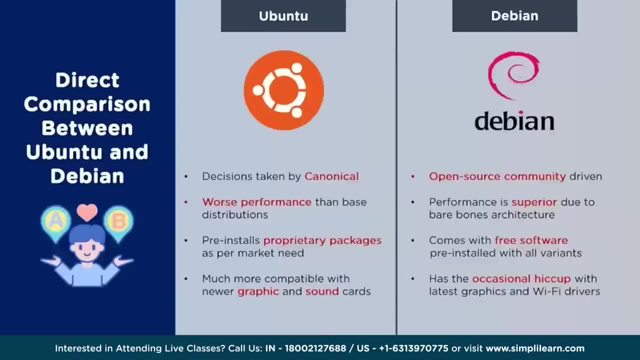 That means Debian lacks some of the essential proprietary firmware by default, but the users can enable the repository and install it manually like other paid software. On the other hand, Ubuntu Debian is more like an open source- closed source, open source, closed source, open source. 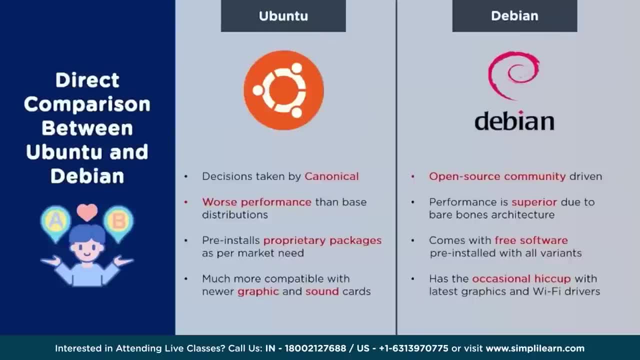 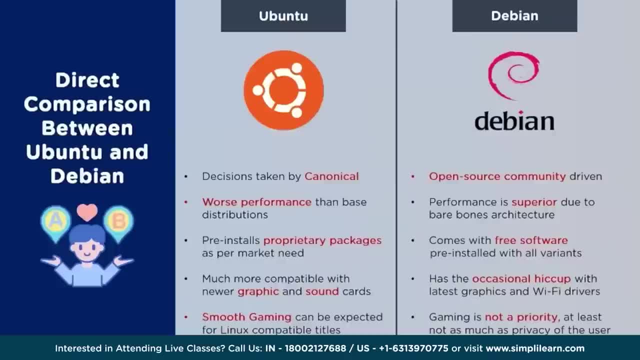 it is likely that you might end up breaking your installation. As mentioned before, Ubuntu supports certain proprietary packages as well, which often consist of graphic drivers which are essential to gaming. Debian focuses on the open source aspect of the software. Hence it can be a well-known fact that, with gamers, Ubuntu and some other distributions- 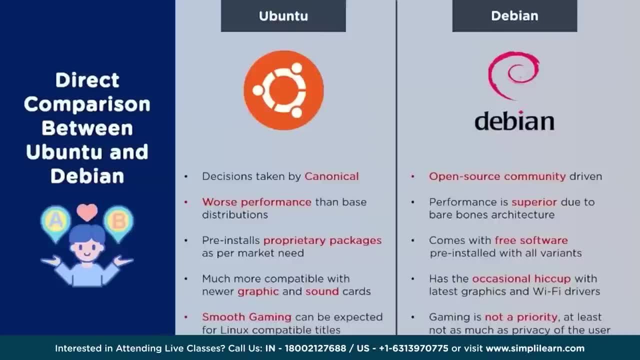 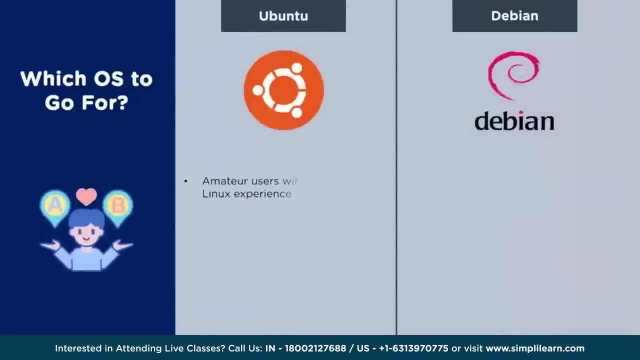 like PopOS, have been working much better regarding both software and hardware support. Regarding the audience they cater to, both Ubuntu and Debian have their pros and cons. Ubuntu is a very good distribution for amateur users with little to no experience and if they want to have the latest versions of packages and applications at all times on their systems. 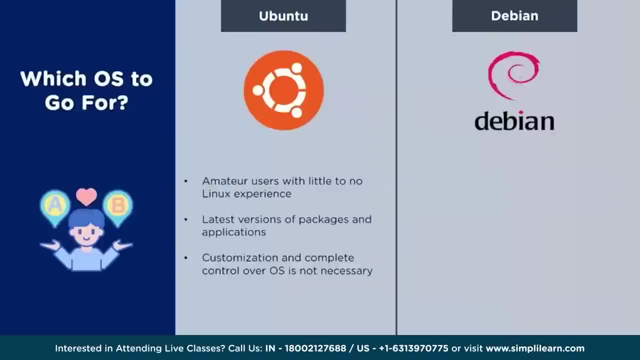 It is also for users who do not want a lot of customizability, in spite of Unity being very customized desktop environment. It is also perfect for users with newer hardware, since it comes updated with all the latest graphical devices and their respective drivers. Debian, on the other hand, is the best. 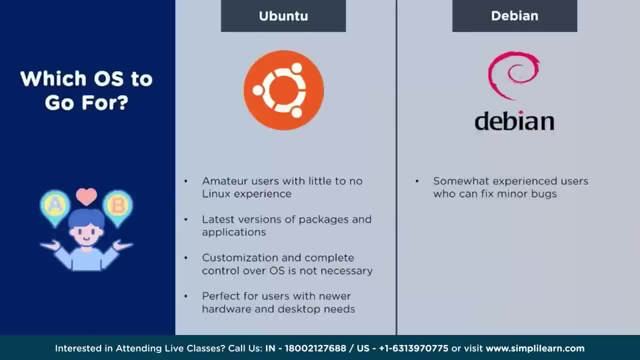 It can cater towards a little bit of experienced users who can fix some minor bugs on their own or with minimal community support. It also is for users who want to support an open source approach rather than an operating system which is devoid of any contribution from other end and is primarily 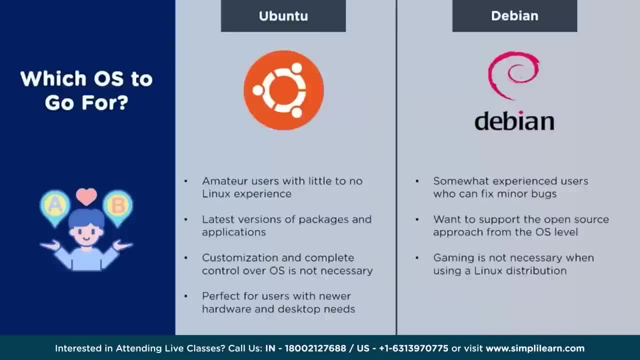 backed by a corporation. It also doesn't favor gaming, since it does not guarantee compatibility with all the newest graphic cards, or even Wi-Fi cards in some cases. However, due to the low memory overhead, Debian is the best. It is very useful for people who are looking to run home servers or even corporate environments. 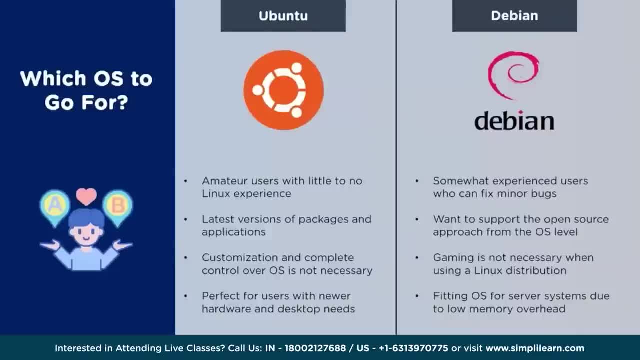 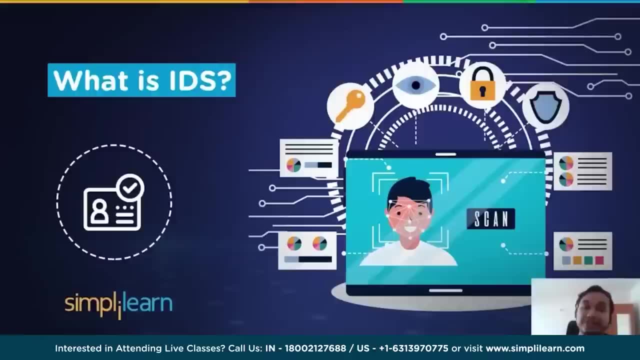 where running servers on Debian will provide much more use. Data protection is of paramount importance in today's world. The vast amount of data flow between corporations and consumer needs to be secured, considering that they are entrusted with a lot of belief. A company can spend millions of dollars on the most secure servers, but it takes a 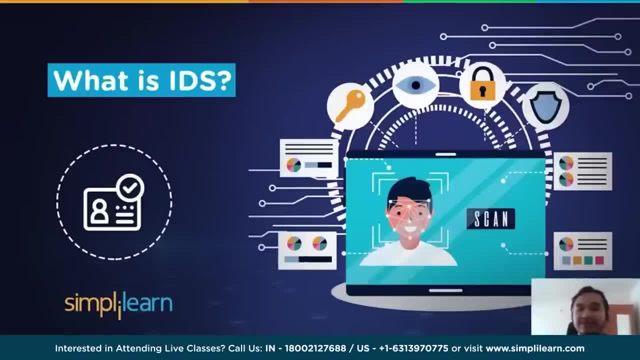 single hacker to ruin all the goodwill between the organizations. To prevent these malicious attacks. many automated security systems are used to protect their customers from the threat of data loss. Many automated security systems are used to protect their customers from the threat of data loss. 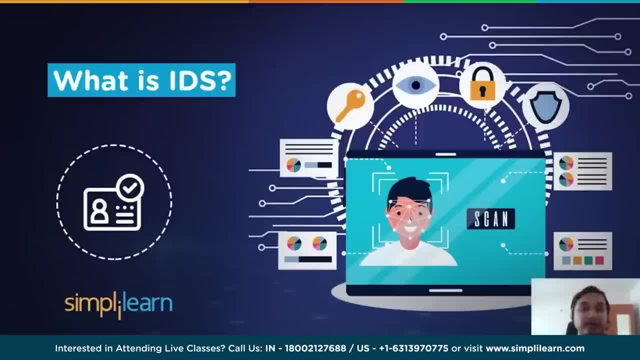 To prevent these malicious attacks. many automated security systems are used to protect their customers from the threat of data loss. humanos system have been developed, but none of them have been used entirely as IdS platforms, which also known as intrusion detection systems. Welcome to this introductory lesson on intrusion. 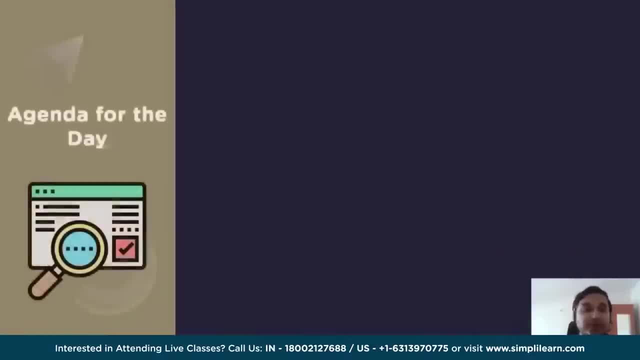 detection systems. So let's go through the topics that we are going to cover today. We started with the basic definition of ideas from a layman's perspective, So, moving on, we cover the multiple types of intruders that seek to access confidential information without any authorization. Next, we cover the basic ways to detect intrusion signatures. 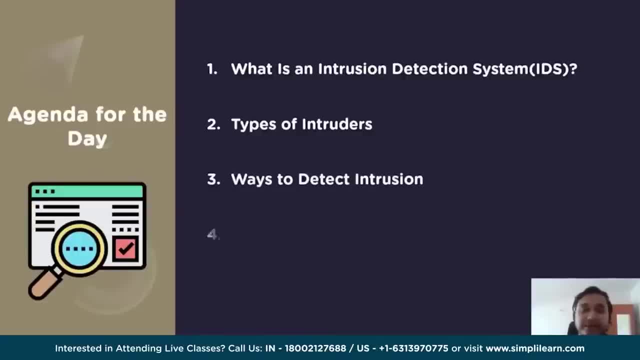 from the perspective of a network administrator. We then take a look at the different types of IDS systems that can be used in corporate environments today. A small explanation of the two types of protection is then followed by an introduction to some of the most well-known IDS tools on the market. 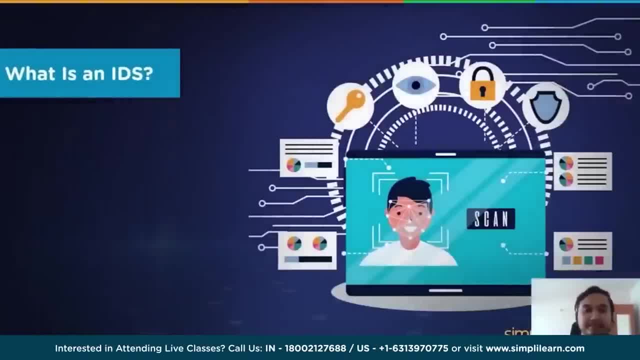 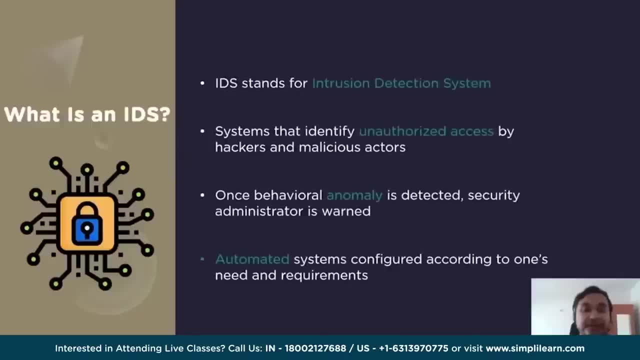 So let's get started with. what is an IDS. An intrusion detection system is an app or device that monitors inbound and outward network traffic, continuously, analyzing for activity changes and patterns, and alerts an administrator when it detects unusual behavior. An administrator then reviews alarms and take action to remove the threat. 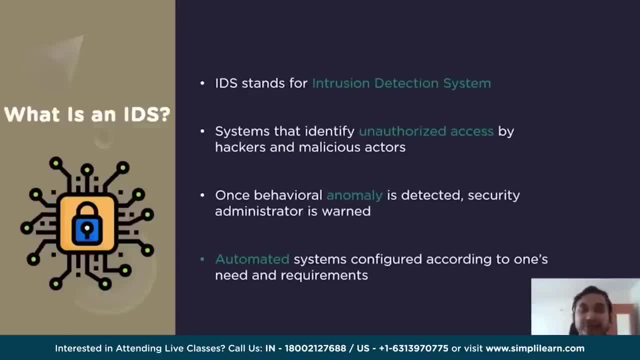 For example, an IDS might inspect the data carried by network traffic to see if it contains known malware or other malicious content. If it detects this type of threat, it sends an alert to your security team so they can investigate and remediate it Once your team receives the alert. 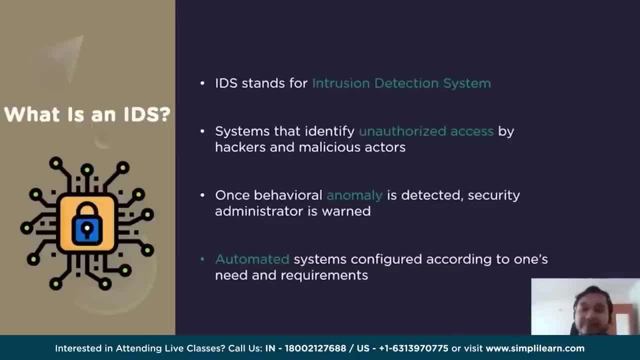 they must act quickly to prevent an attack from taking over the system. To ensure that the IDS doesn't slow down network performance, the solutions often use a switched port analyzer or a text access port to analyze a copy of the inline data traffic, so that they do not meddle with the actual traffic. 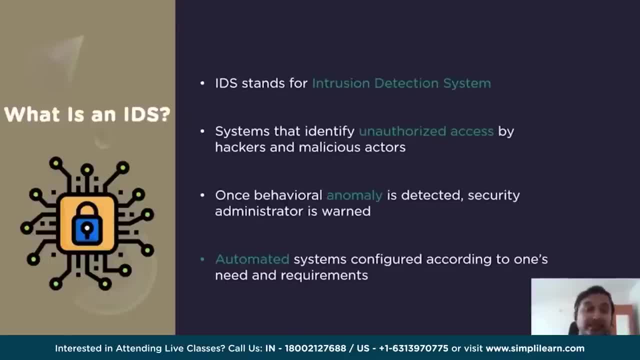 However, they do not block threat once they enter the network, as intrusion prevention systems do. Regardless of whether you set up a physical device or an IDS program, the system can recognize attack patterns with network packets, monitor user behavior, identify abnormal network activity. 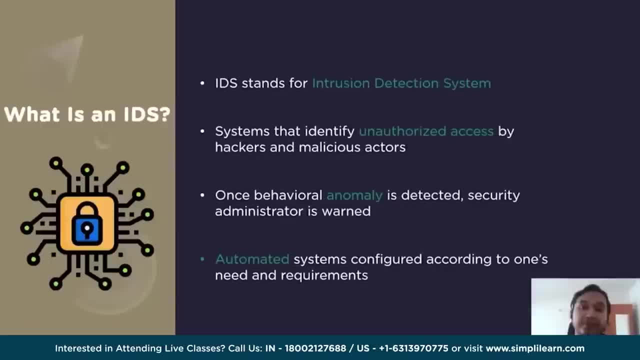 and ensure user and system activity do not go against security policies. The main goal of an IDS is to detect the anomalies before the hackers complete their objective. Once the system detects a threat, the IT team is informed and the information is passed on. Given the requirement for understanding context, 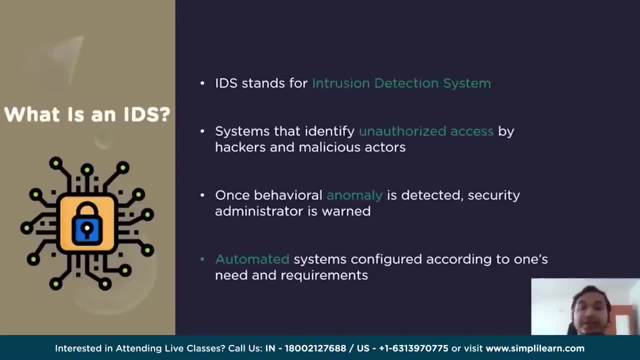 an enterprise has to be ready to make any ideas fit its own unique needs, expert advised. What this means is that an IDS cannot be a one-time. it cannot be a one-size-fits-all configuration to operate accurately and effectively, And this requires a savvy IDS analyst to tailor the ideas. 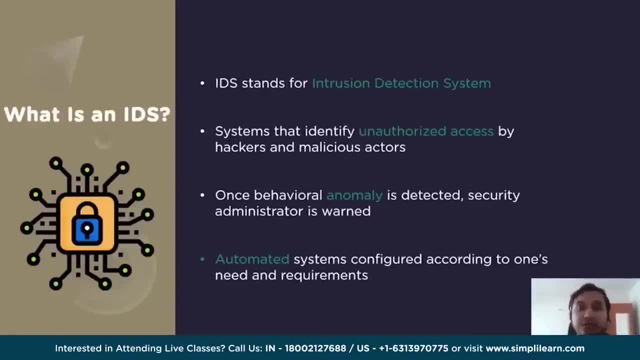 for the interests and needs of a given site, And knowledgeable trained system analysts are scarce. The trick with IDS is that you have to know what the attack is to be able to identify it. The IDS has always had the patient- zero problem. You have to have found someone who got sick and died. 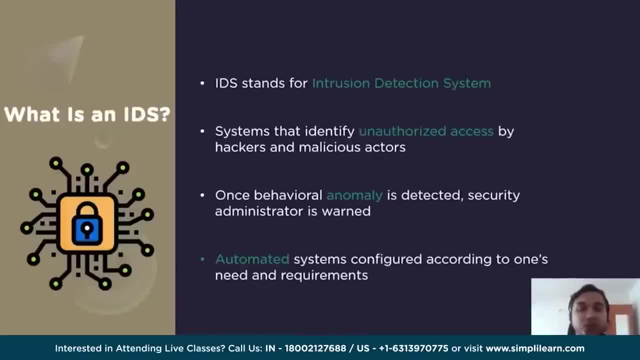 before you can identify it. It can usually go for two types of protection: active protection and passive. In a passive system, the IDS detects a potential security breach, logs the information and signals an alert. In a reactive system or an active system, 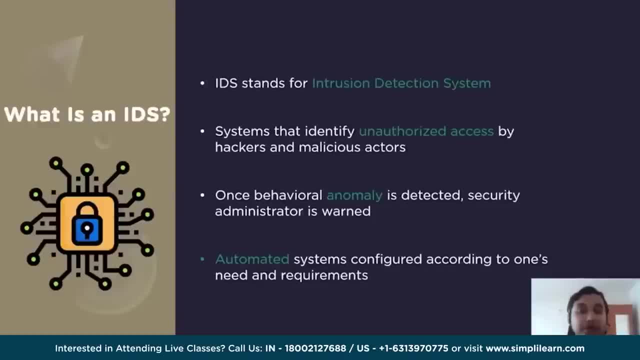 the IDS responds to the suspicious activity by logging off a user or by reprogramming the firewall to block network traffic from the suspected malicious source. Now that we understand what an IDS is, let us go through the different types of intruders IDS platforms must be aware of. 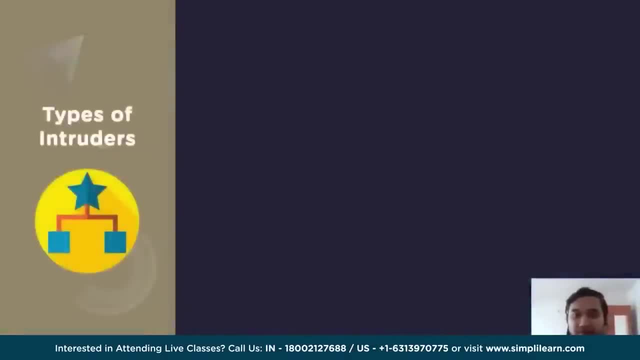 To understand this type of intruders, let us go through a scenario. We have the servers which are protected by the IDS platforms in place. So let's say a hacker tries to breach the system from outside the organization. This can be done using multiple attacks. 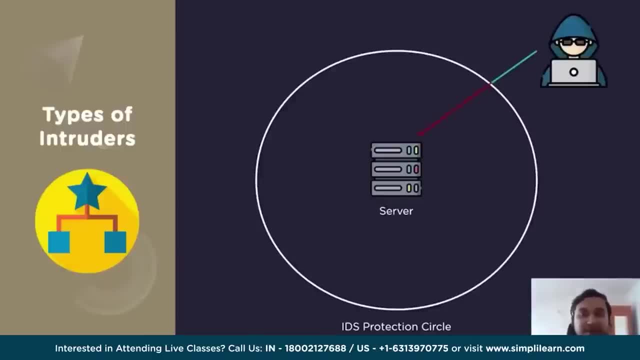 like DDoS attacks, injection attacks, etcetera. The category of individuals that are not authorized to use the system but still exploit users' privacy and confidential information using different techniques are known as masqueraders. Masquerader is an intruder that can be used as a tool to protect someone's privacy and confidential information using different techniques. are known as masqueraders. 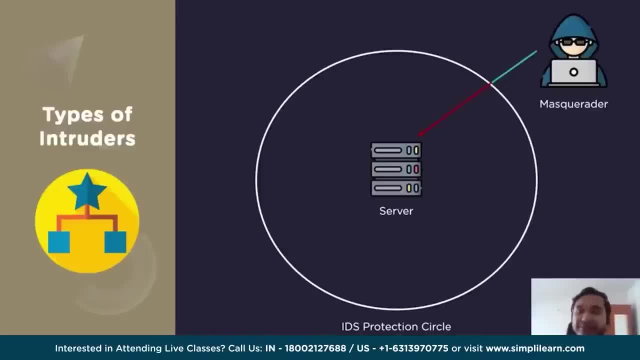 that is an outsider who does not have direct access to the system and aims to attack unethically by stealing data or information. However, there is another intruder who is theoretically harder to detect and approve than a masquerader. These are the people within the organization. 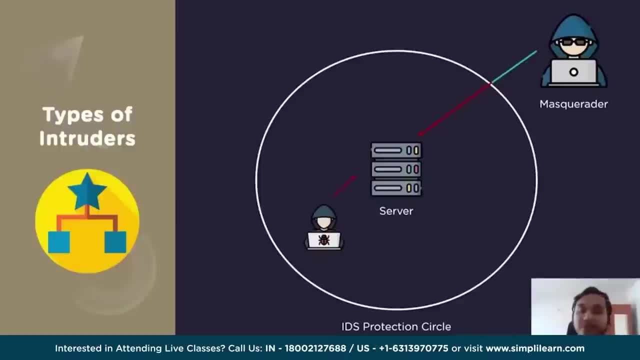 who want to weaken the security defenses, be it for corporate espionage or to aid other masqueraders- The category of individuals that are authorized to use the system but misuse the granted access and privilege. These are individuals that take undue advantage of the permissions and give access to them, and this category of intruders are known as. 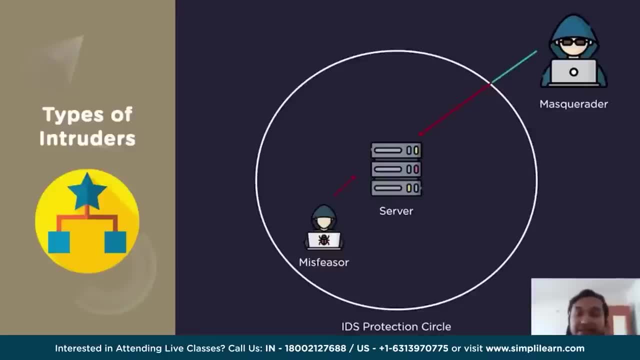 misfeasors. Misfeasors are people that are insiders and have direct access to the system which they aim to attack unethically by stealing data or information. Let us now go through some of the ways the IDeA's platforms can detect intrusion before 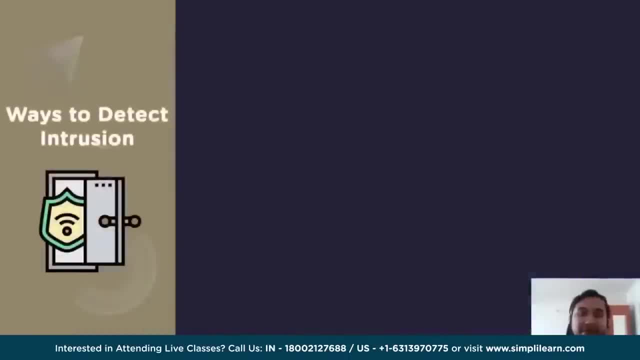 it is too late. Intrusion detection systems primarily use two key methods. One is signature based intrusion and the other is non-intrusion based intrusion. Intrusion detection systems are designed to detect possible threats by comparing the given network traffic and log data to existing attack patterns. These patterns are called sequences and could include byte. 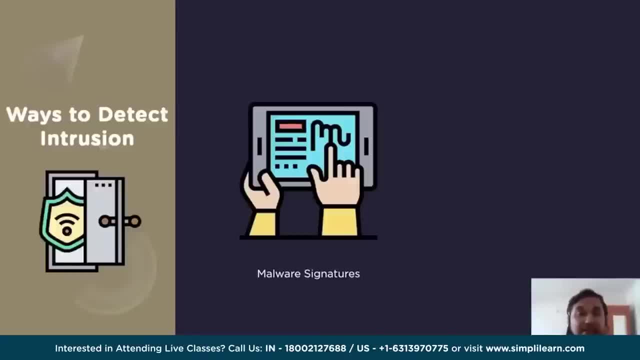 sequence, which is also known as malicious instruction sequences. Signature based detection enables you to accurately detect and identify possible known attacks. Anomaly based intrusion detection is the opposite. It is designed to pinpoint unknown attacks, such as new malware, and adapt to them on the fly using machine learning. 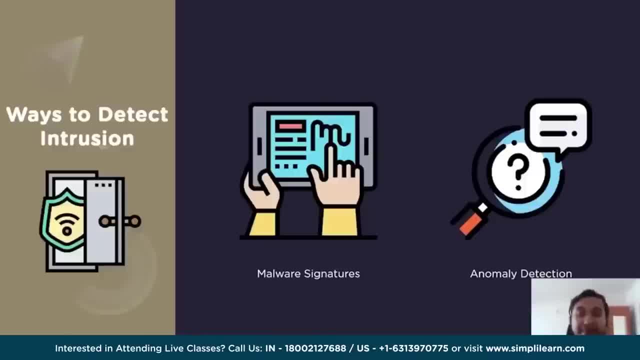 Machine learning techniques enable an intrusion detection system to create baselines of trustworthy activity, which is known as a trust model, then compare new behaviors to verified trust models. False alarms can occur when using an anomaly based IDeA, since previously unknown yet legitimate network traffic could be falsely identified as malicious activity. 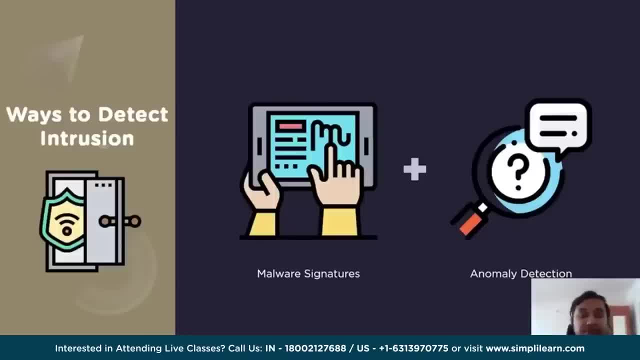 Now, if you combine both of those, you have the hybrid intrusion detection. They use signature based and anomaly based intrusion detection to increase the scope of your IDeA. This enables you to identify as many threats as possible. A comprehensive intrusion detection system can understand the evasion techniques cyber criminals use to trick. 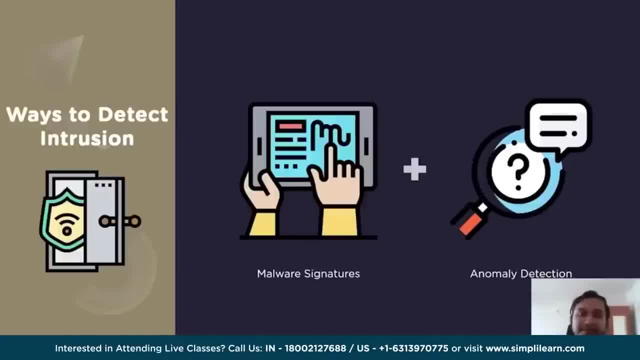 an IDeA to thinking there isn't an attack taking place. These techniques could include fragmentation, low bandwidth, attack pattern change, evasion and many more. We can now take a look at the type of protection offered by IDeA's platforms. CYBER CRIMINALS. 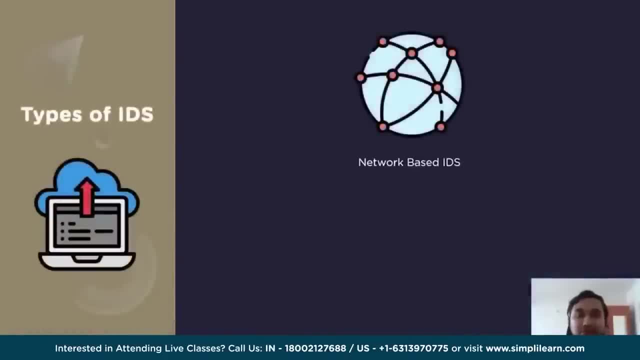 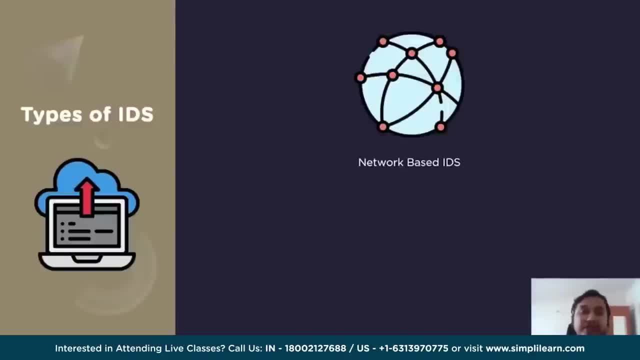 The sensors are deployed at strategic points within the network, such as within the DMZ or at the network's perimeter. The sensor can monitor individual packets of inbound and outbound traffic to and from all devices on the network. It analyzes them for malicious activity and, depending on the network architecture and 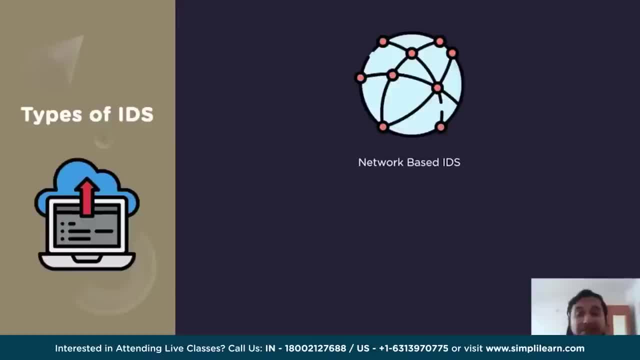 amount of traffic involved, multiple instances of network-based IDS may be necessary. The second category is host-based intrusion detection systems, or HIDs. An agent runs on all servers, endpoints and devices in the network that have access to both the internet and the internal network. 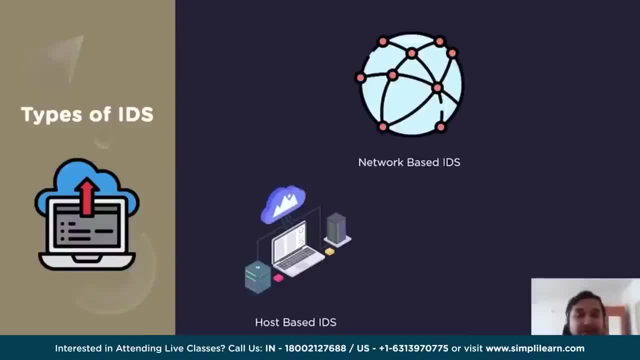 Intrusions are identified by analyzing operating specific activities, like the modification of the file system, registry or access control lists, and by monitoring system application logs as well. They augment network-based IDS systems by detecting anomalous traffic which originate within the organization or from the host that is being monitored. 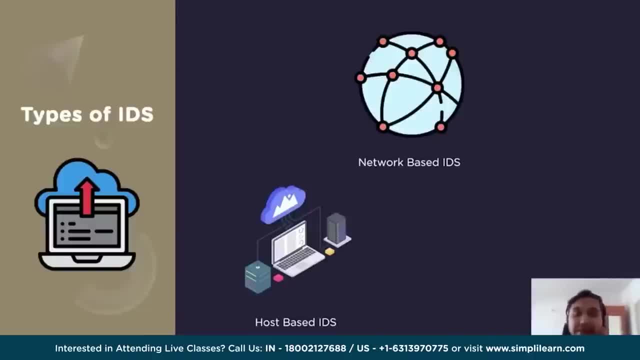 For example, a host infected with malware that is attempting to spread it to other internal hosts is an issue that a network-based IDS could potentially fail to detect. The third variant is a cloud-based intrusion detection system. Because of the internet-facing nature of the cloud, on-premises IDS solutions are not necessarily 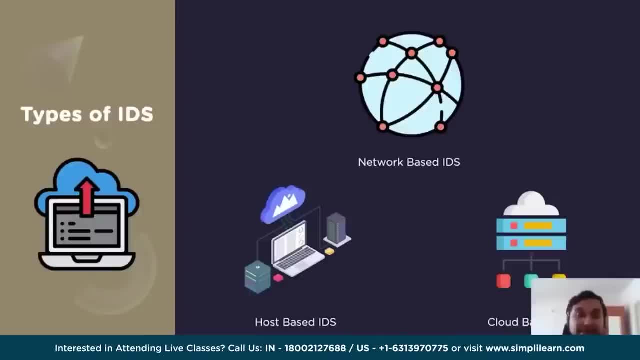 optimized for monitoring. For example, network-based sensors need to be deployed within the cloud at an advanced environment's network perimeter, and yet a cloud service provider may or may not have a way to facilitate this. Cloud-based servers use purpose-built cloud sensors that use Cloud Service Provider Application. 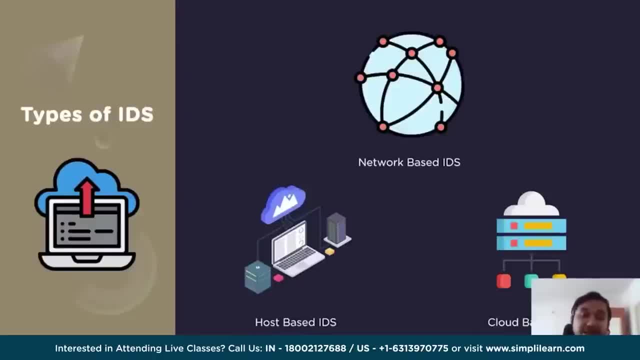 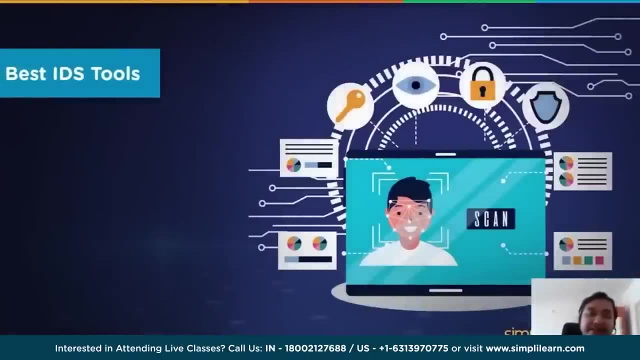 Programming Interface or Cloud Service Provider APIs, to get as much visibility as possible into your cloud environment. Now that we understand the different types of IDS deployment tactics, let us go through some tools that excel in this field, offering top-of-the-line implementations in a corporate 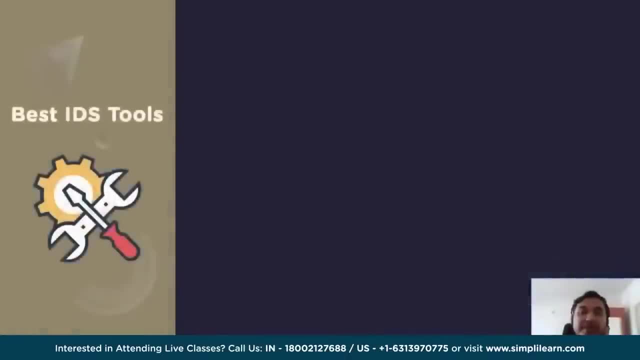 and consumer environment. The first tool being covered is the SolarWinds Security Event Manager. The SolarWinds Security Event Manager is designed to integrate real-time log data from across your infrastructure, enabling it to act both as a network-based IDS system and a host-based 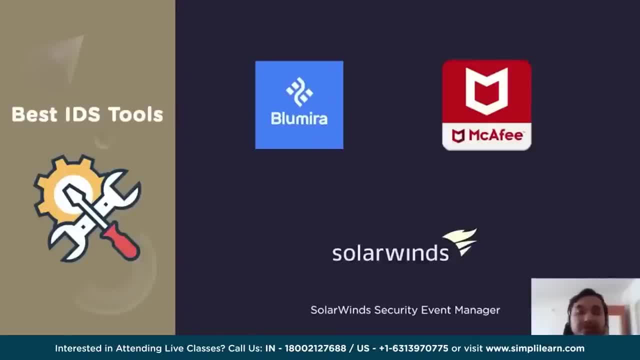 IDS system. The solution can let you discover all kinds of malicious attacks and help you protect your network from harm. It is also designed to enact both signature-based and anomaly-based intrusion detection by comparing sequences of network traffic against a set of customizable rules. Next we have the McAfee LiveSafe. 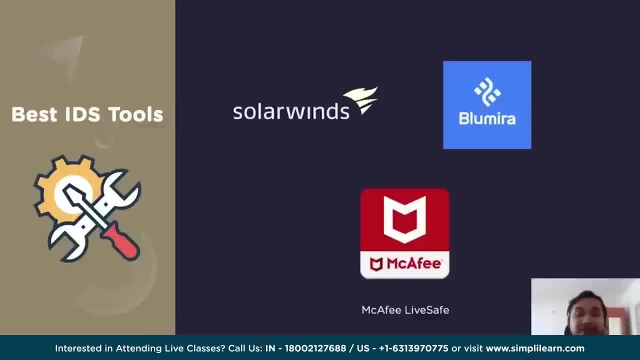 McAfee LiveSafe is an intrusion detection system designed to bring real-time threat awareness to your physical and virtual networks. It uses signature-based intrusion prevention and anomaly-based intrusion detection, along with emulation techniques, to spot and identify malicious activity. McAfee is also built to correlate threat activity with application usage, which can further prevent. 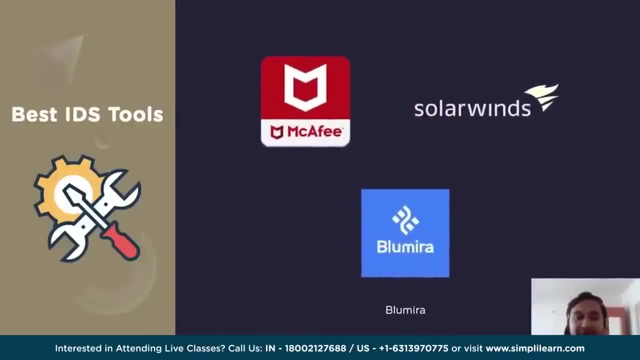 network issues stemming from network issues. Next, we have Blumera. Blumera is a security information and event management platform built to enact threat detection and responses across your cloud and on-premises environments. It is designed to continuously monitor your IT infrastructure for suspicious activity. 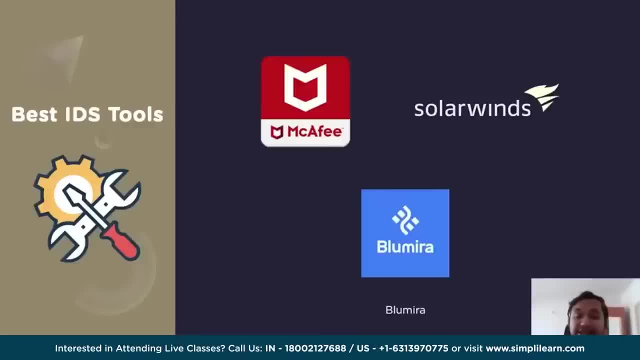 and misconfigurations, both of which could result in data leaks and compliance breaches. It enables you to respond to an attack in progress and stop malicious actors in their tracks. Blumera can be used to monitor and freeze illegal online or cyber-attacked security. 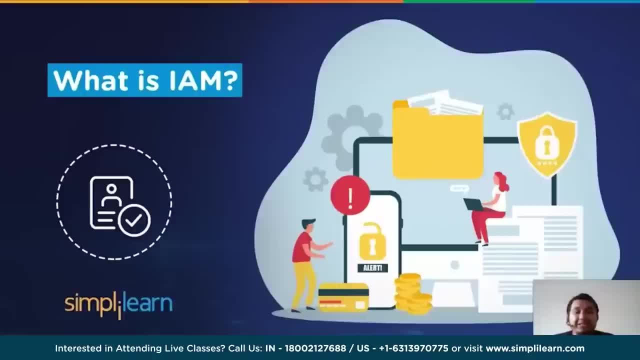 attacks and can be used as your backup security device. In other words, it can be used to control your network storage on a high frequency. by soloing the authenticatedkm drive With Blumera, you can efficiently monitor, track and control the activity of an organization. 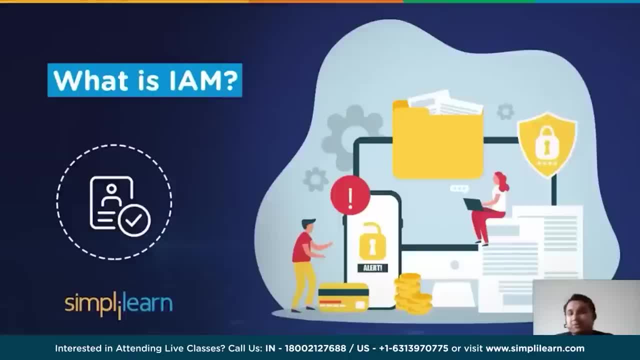 or service in the name of your security system. With Blumera, you can successfully monitor other activities in your network and control specific areas of the digital network to monitor your security and the details of your security system. This kind of work is tall and easy to do and requires quite a lot of time, time and money. 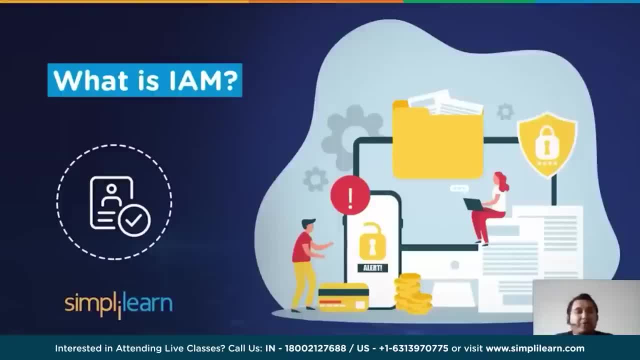 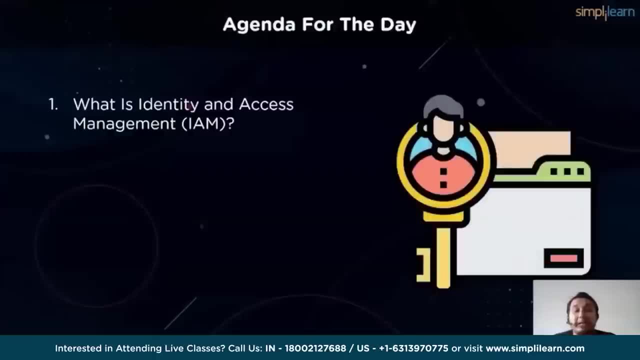 The Blumera API was originally developed with Blumera. The Blumera API is built for your personal mobile device. You can use the Blumera API to monitor your network, network protection data and other security services. We start by learning about IAM, that is, Identity and Access Management from a surface level. 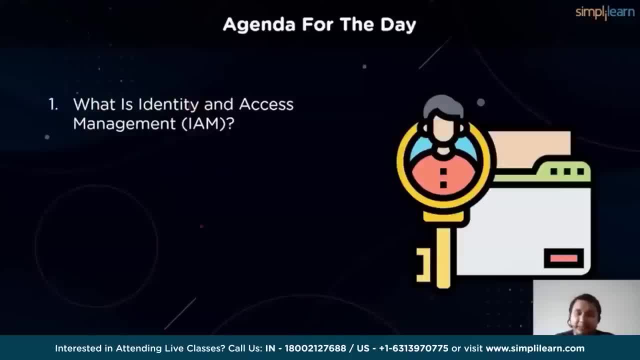 so as to put a clear idea of what it is. Next, we cover the general workflow and process of how IAM works. Moving on, we cover some of the tools that find their place in an IAM framework and are crucial components. Finally, we go through some of the advantages of the IAM, learning what makes them a lucrative. 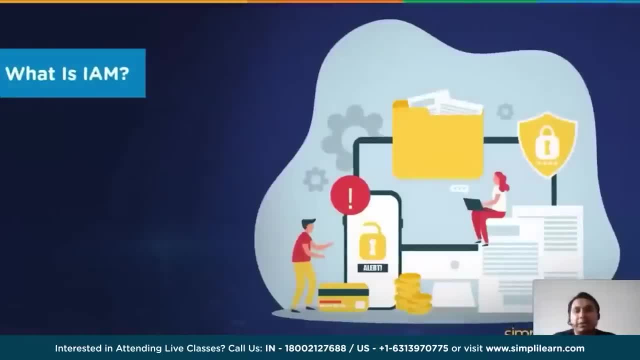 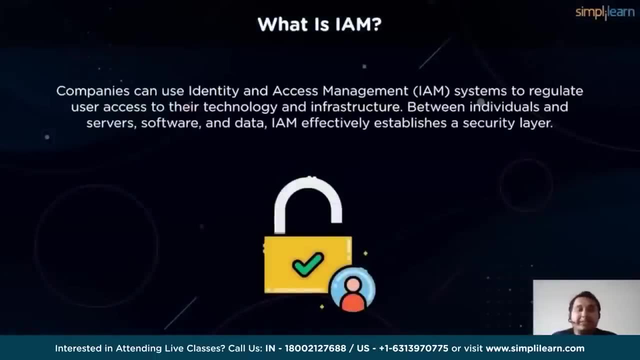 deal for organizations, So let's get started by learning about IAM from a surface level perspective. Identity and Access Management, or IAM, is a set of processes, policies and tools for defining and managing the roles and access privileges of individual network entities to a variety of cloud and on-premise applications. 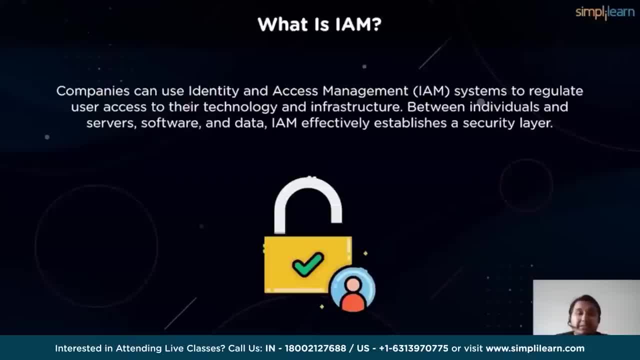 The users can include customers, partners, employees, devices like computers, smartphones, routers, etc. The core objective of IAM is to create a user-friendly network for all users. The core objective of IAM systems is one digital identity per individual or item. 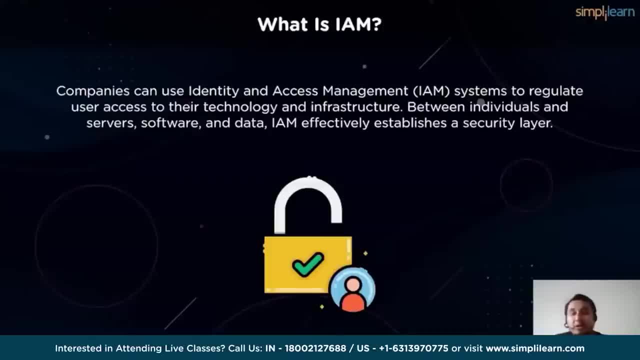 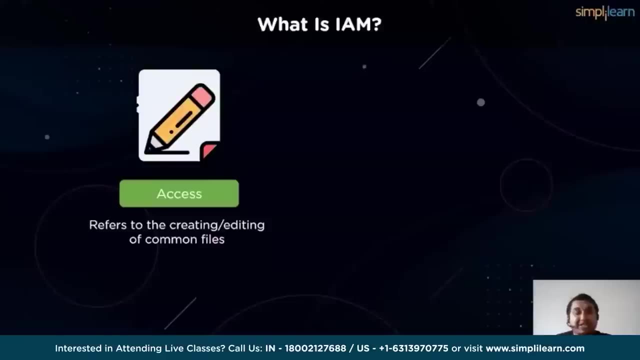 Once a digital identity has been established, it must be maintained, modified and monitored throughout each user's or device's access life cycle. Access and user are two vital IAM concepts. Access refers to the actions permitted to be done by a user, like view, create or change. 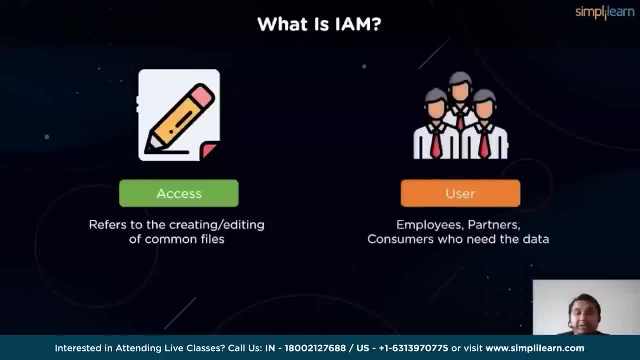 a file. Users could be employees, partners, suppliers, contractors or even customers. Furthermore, the process of setting the interface and software for the individual or item is completely related to the IAM. Furthermore, employees can be further segmented based on their roles. 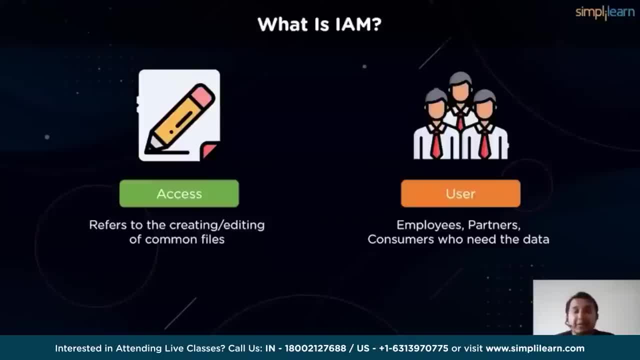 IAM systems are designed to perform three key tasks – identify, authenticate and authorize, meaning that only the right person should have access to computers, hardware, software apps, any IT resources, etc. For the entry of new users or the changing of the roles of existing users. 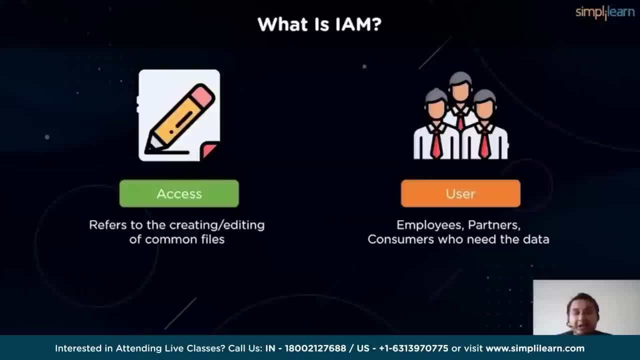 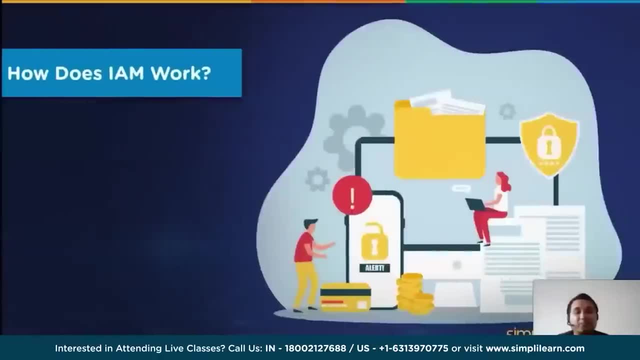 the list of access privileges must be up-to-date all the time. IAM functions usually fall under IT departments or sections that handle cybersecurity and data management. Now that we understand the importance of IAM in today's cybersecurity sphere, let us understand the process of this framework. 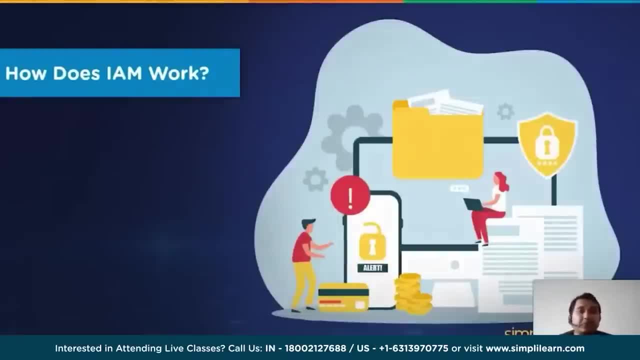 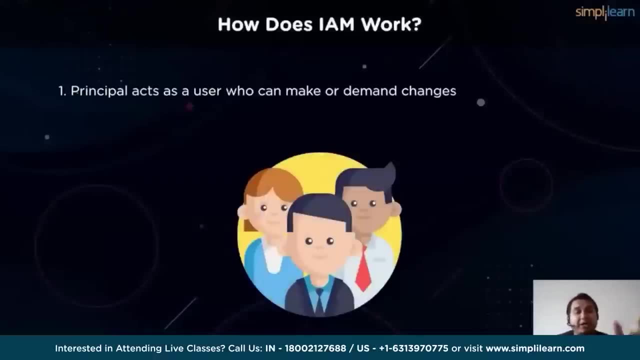 We have multiple components that aid this process. Let's start by going through each of them individually. Principal is an entity that can perform actions on an AWS resource or any cloud management system. A user, a role or an application can be a principal. 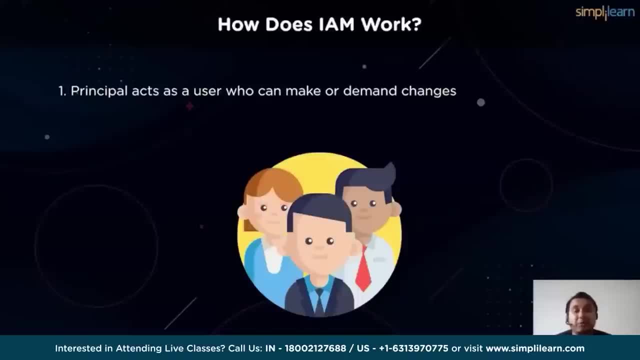 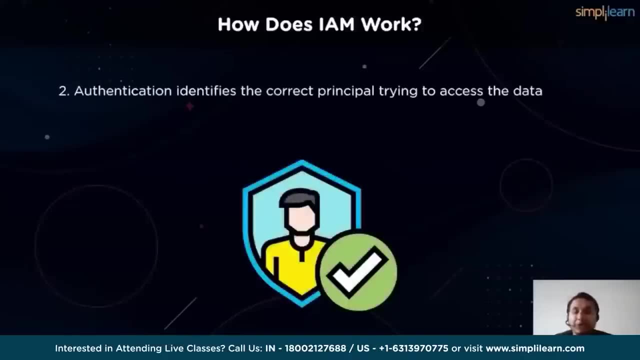 It's always the principal who raises a concern to access or modify data on servers serving as the first point of contact in the IAM workflow. Authentication is the process of confirming the identity of the principal trying to access the product. The principal must provide its credentials or required keys for authentication. 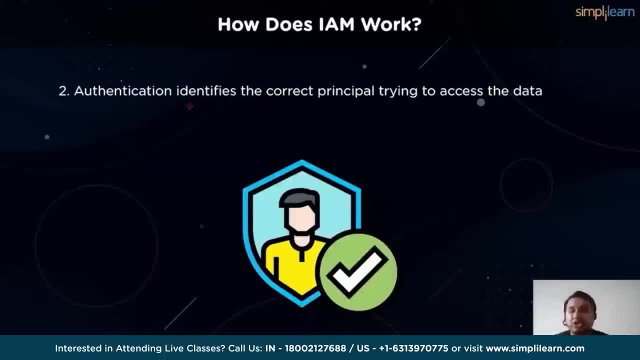 This step can be further enhanced by multiple authentication factors and geologs, among other things. Once the identity is confirmed, the principal has the ability to confirm the identity of the product. The principal has the ability to view the data behind the wall of security and take the necessary steps. 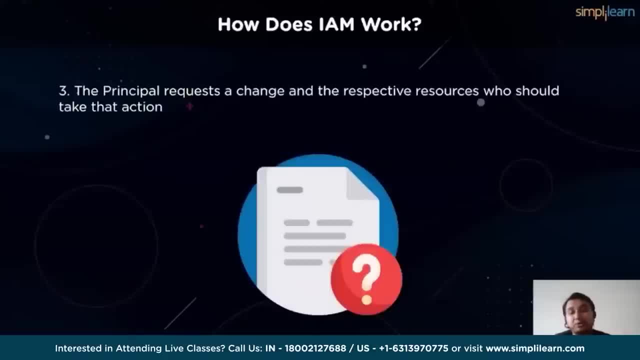 When it comes to requests, a principal then sends a request to the cloud management system specifying the action and which resource should perform it. In this step, the user can ask to modify, delete, edit or affect other users in this particular bucket of organization by changing the data or the information. 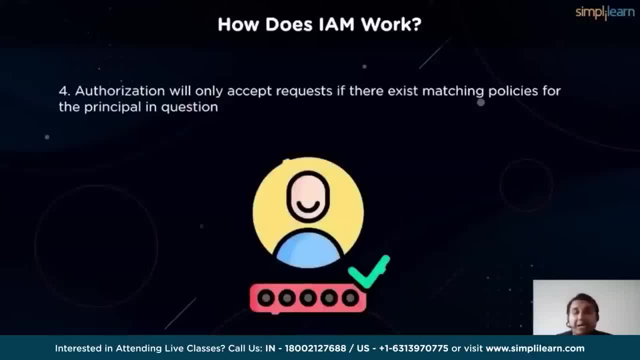 When it comes to authorization, it carries out the rest of an organization: identity and access management. The user has to verify the data and the data is being processed. once the user has been authenticated, Users are granted authorizations according to their role at an organization. 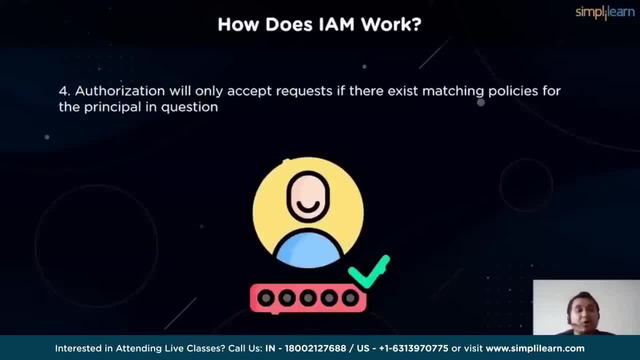 The practice is referred to as Role-Based Access Control, or RBAC. Authorizations determine a role's resources and level of access in the network. These items may include systems, applications, file shares, printers and more. For example, an accounting department employee who regularly works with payroll software must be authorized to do such. 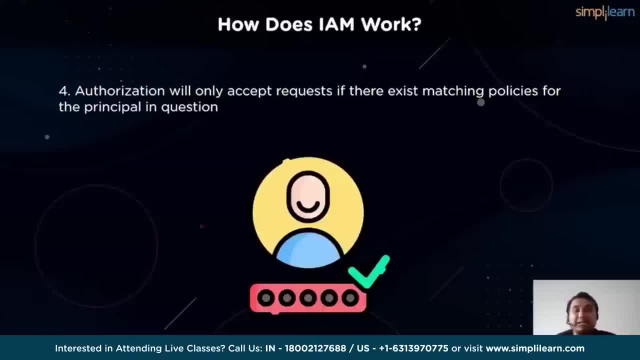 If your authentication resembles a passport, these are the things your digital identity can access with it. While authentication is fully straightforward, authorizations and their management are far more challenging. Authorizations consist of complex set of rules and policies and groups which are permitted, explicitly configured per user account. 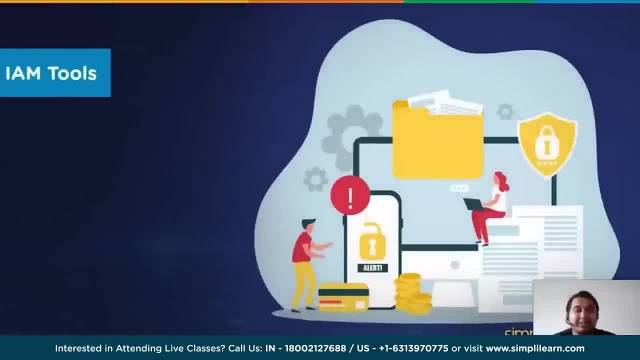 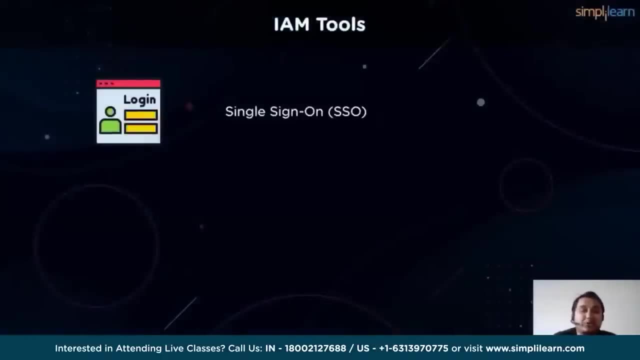 With the working of IAM frameworks out of the way, let's cover some of the tools that these systems work on. SSO is an IAM tool that enables a user to log into one of an organization's properties and automatically be logged into a design set of other properties. 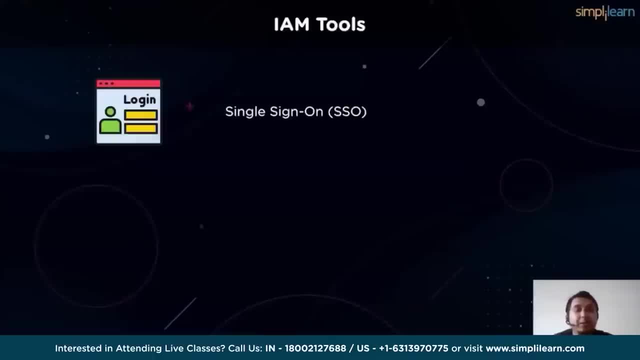 For example, when you log into Google, you're automatically logged into your Gmail and your YouTube accounts. Similarly, for users, single sign-on reduces friction, since they don't have to keep track of different credentials for every application. For organizations, SSO helps in collecting valuable insights about user behavior and preferences. 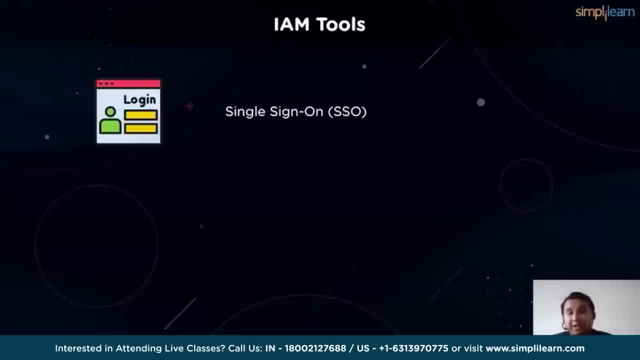 since it tracks them as they move from one application to another, Connected by one single login. Next is multi-factor authentication or MFA. Implementing multi-factor authentication is crucial to protect your organization's data from malicious intrusions, and virtually every IAM platform offers some form of MFA. 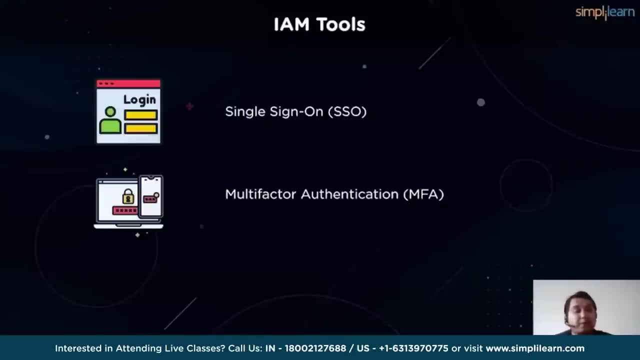 However, it's equally crucial to customize MFA with the appropriate level of security. For example, in business-to-consumer scenarios. you need to consider UX and try not to create unnecessary friction for users who don't want to be subjected to heightened scrutiny every time they log in. 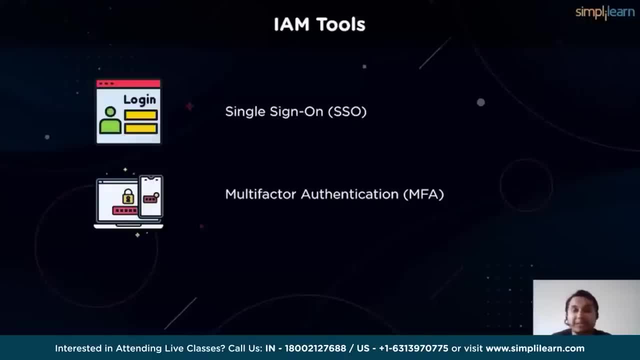 For workforce IAM. you may want a more stringent MFA, since the consequences of an unauthorized party gaining access to your private network can be so devastating. A modern IAM solution will allow you to implement MFA only when it's needed. This can be accomplished through setup authentication or adaptive authentication, in which users only trigger MFA if they're trying to access sensitive data or their behavior is flagged as risky. 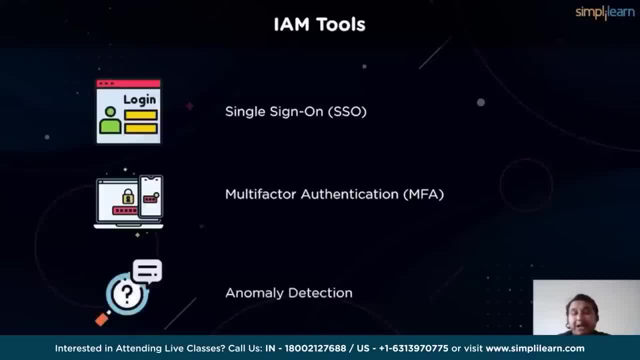 In the past few years, identity has become the preferred gateway for hackers to break into systems. Brute-force attacks, credential stuffing attacks and even highly targeted phishing campaigns are all attempts by hackers to break in through a company's front door, which is the login box. 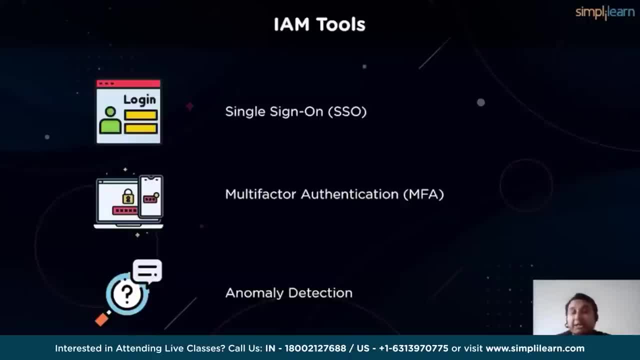 There are multiple ways IAM systems can help detect and mitigate these malicious attacks. IAM solutions detect attacks by monitoring signals such as the velocity of traffic, detection of login patterns that differ from a user's routine use of a breached password, use of a password that is not a password and the use of a password that is not a password. 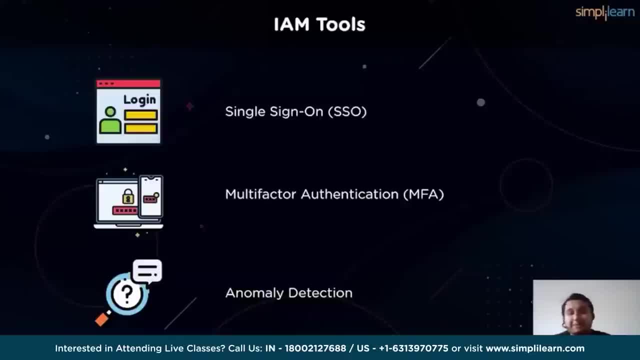 There are also ways to track the data that is being used to track devices and IP addresses with a poor reputation, among other things. These are some of the most widely used tools when it comes to IAM frameworks, But why do we go through setting up so many tools and firewalls? 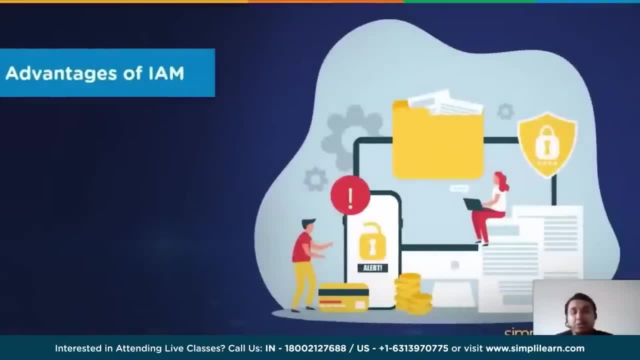 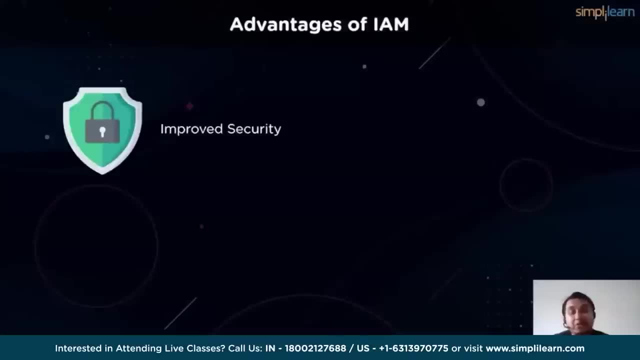 Let's go through some of the advantages of using IAM systems. in both corporate and consumer environments. IAM solution helps identify and mitigate security risks. You can use IAM to identify policy violations or remove inappropriate access privileges without having to search through multiple distributed networks. You can also leverage IAM to ensure that security measures are in place to meet regulatory and auditing requirements. 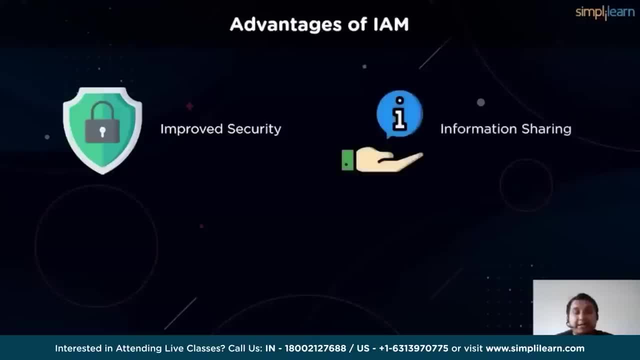 IAM provides a common platform for access and identity management information. You can apply the same security policies across all the operating systems and devices used by the organization. The IAM framework can help you enforce policies related to user authentication, privileges and validation and attend to the privilege creep problems. 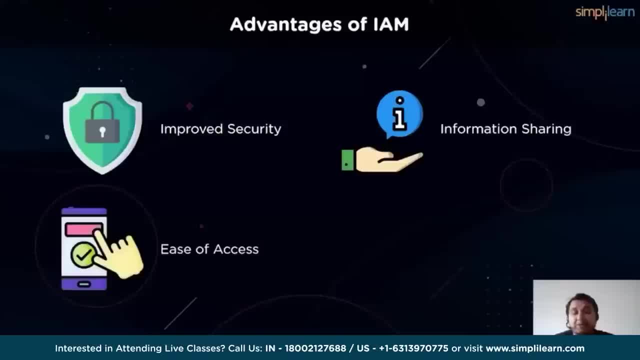 IAM systems can be used to identify and mitigate security risks. The IAM framework simplifies sign-up and user management processes for application owners, end users and system administrators. It makes it simple to provide and manage access and promotes user satisfaction. IAM services can also lower operating costs. 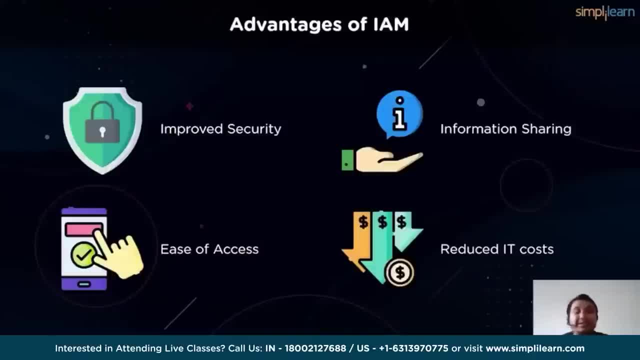 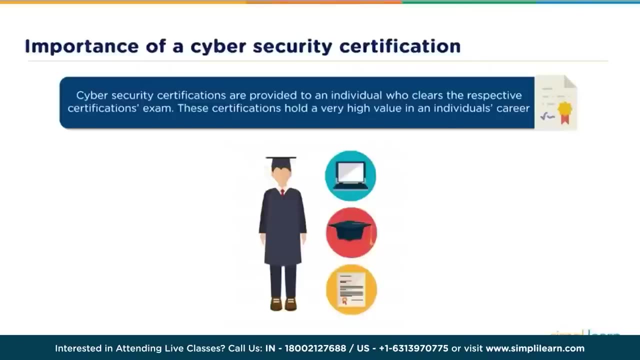 Using federated identity services means you no longer need local identities for external users. This makes application administration easier. Cloud-based IAM services can reduce the need to buy and maintain on-premise infrastructure. So importance of cybersecurity First and foremost. when I see a certification, I look at it from three different aspects. 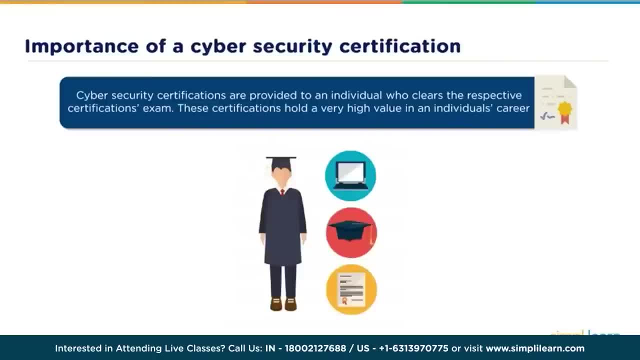 The first is the training itself, which allows me to gain the knowledge which allows me to understand the aspects of security or whatever the certification is there for. The second aspect is the exam itself. How do I need to prepare myself for the exam? 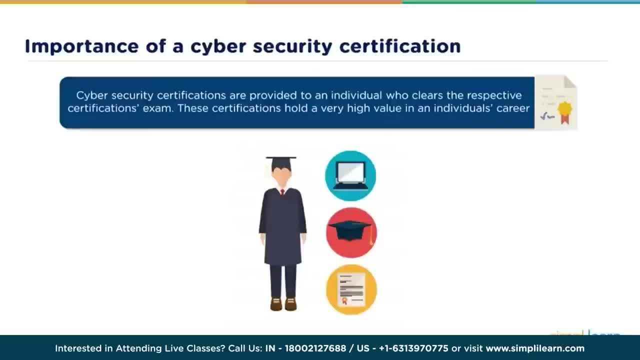 And how do I need to approach the exam? How do I need to ensure that I pass in my first attempt? And the third aspect is the certification itself which allows me to be eligible to apply for a program. And the third aspect is the certification itself which allows me to be eligible to apply for a program. 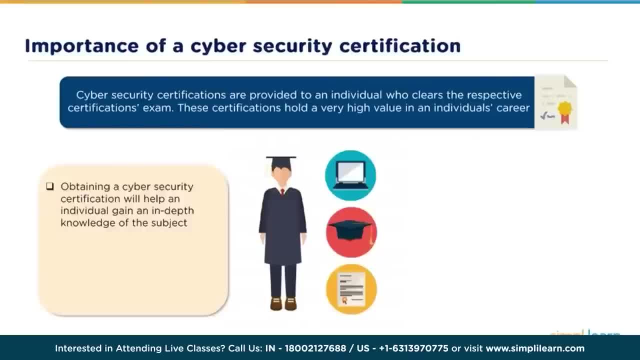 So obtaining a cybersecurity certification ensures, or shows to the organization that you're applying to, that you do have that prerequisite knowledge and you should be shortlisted for an interview. The knowledge that you have gained during the training will help you when you attend that interview and when you attempt to answer the questions asked to you. 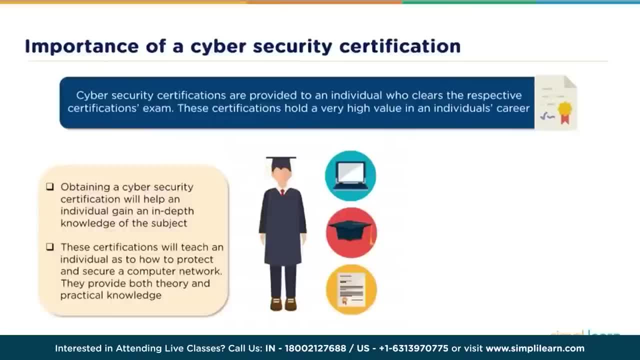 So these certifications are designed for a specific role. For example, a forensic investigation certificate will teach you how to investigate a crime, A digital crime scene. for a matter of fact, A certified ethical hacking course will teach you about penetration testing. So it is you who's going to decide which certification you require, and then attempt to get certified on it. 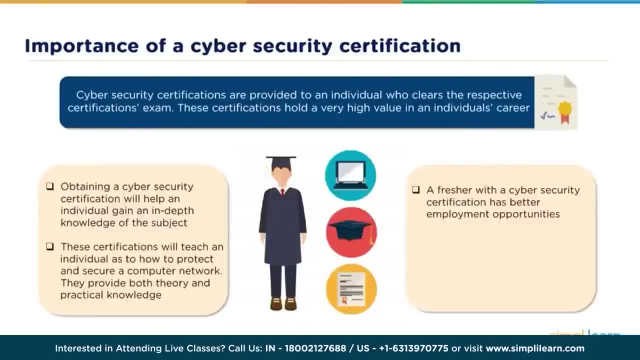 Of course, a fresher with a cybersecurity certification will have better employment opportunities because they can showcase their knowledge with the certification that they already have. Even professionals who want to enhance their careers can get into managed real or advanced certifications to improve on their knowledge and get promoted in their job profession. 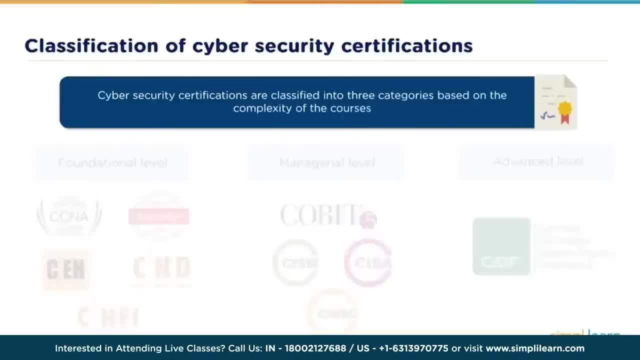 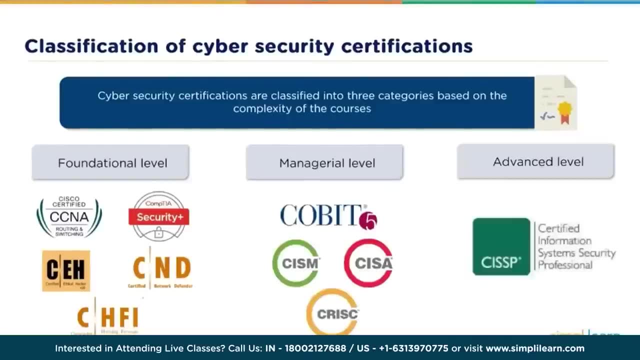 So cybersecurity certifications can be classified in three different aspects, The first one being the foundational level, then the managerial level and the advanced level. In the previous video we just had a small overview. Here we are going to discuss about what the certification covers, how the exams are conducted and the price points for each and every exam. 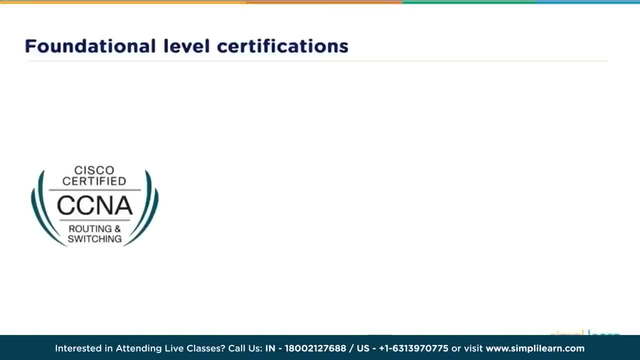 So let's start with the foundational certifications. We start off with CCNA, which is the basic certification for networking. So the CCNA routing and switching certification. So the CCNA routing and switching certification. So the CCNA routing and switching certification. 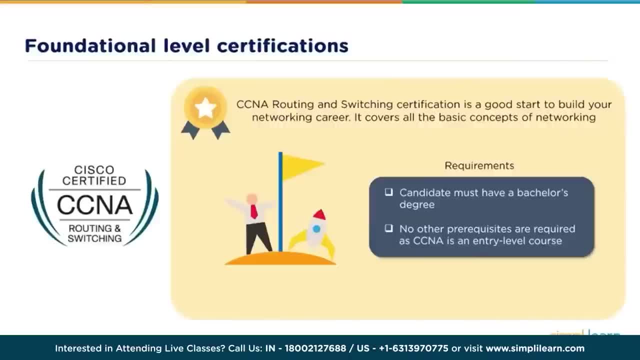 Basically, it helps you build your networking career. You will join an organization as a networking engineer where you can help the organization establish the routing, the pathing, of how data packets will travel across the network. This certification covers all the basic concepts that you require to understand networking. 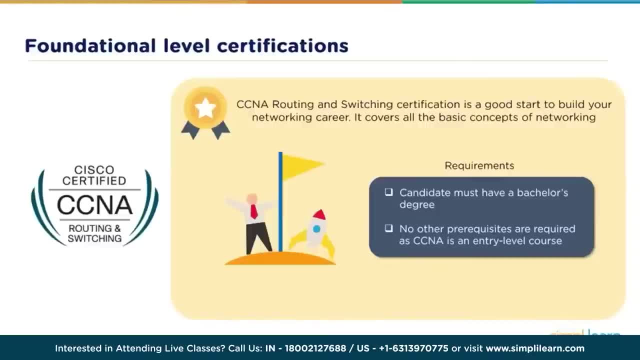 The basic requirements for this certification are that the candidate must have a bachelor's degree, But apart from that there are no other prerequisites. So it's just that you need a bachelor's degree and then you can apply. You can study for this. 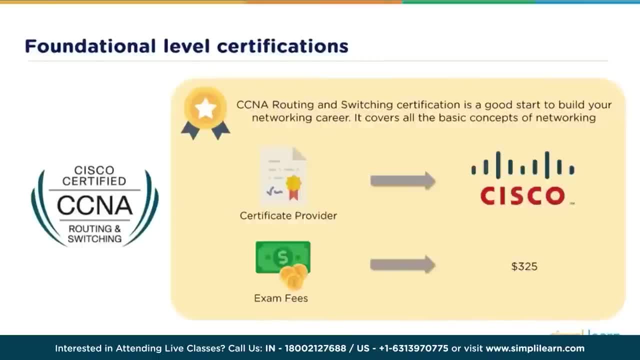 You can undergo, You can go for training and then you can attempt the exam. The certification provider obviously is Cisco, So the knowledge that is limited to this training and certification is for Cisco devices only. The exam fees for this certification is approximately $325.. 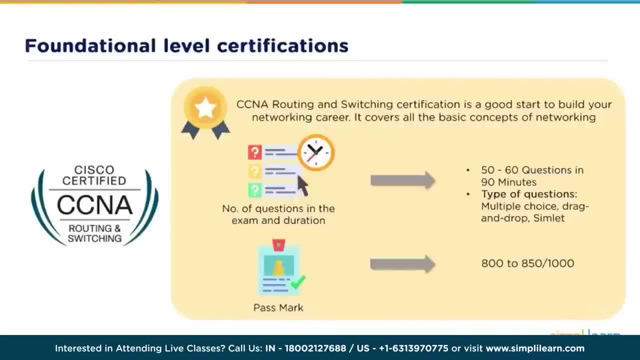 The exam. when it is conducted, it has around 50 to 60 odd questions which need to be answered in 90 minutes. The type of questions that you are going to get is multiple choice questions, where you have a question and four answers and you have to choose the correct answers among those. 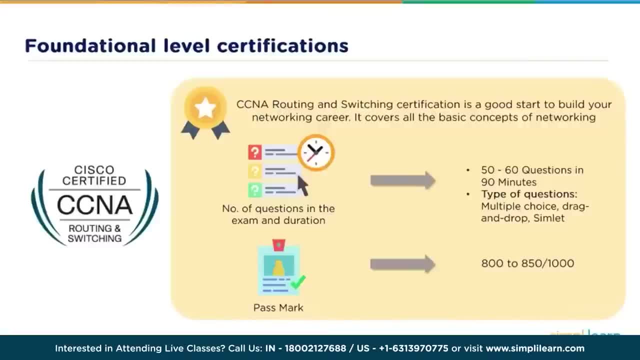 Drag and drop, where you have to click on an object and drag it to its appropriate place- probably an architectural diagram- And you have to, let's say, pick on a router and place it into a particular position. If you place it correctly, you answer the answer, the question, correctly. 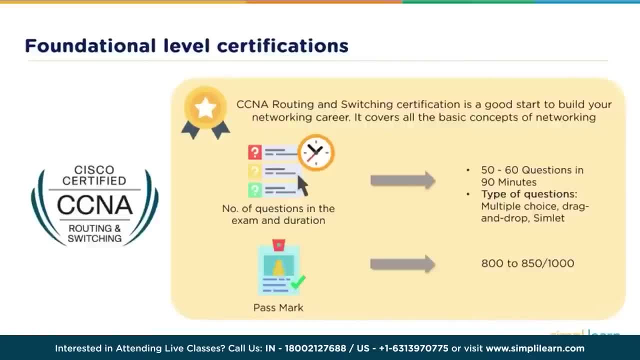 Otherwise it's wrong- And a simulator where there could be a configuration. You need to configure it in a particular manner and then check whether the configuration is correct or not. The pass mark is around 800 to 850 out of a possible thousand marks. 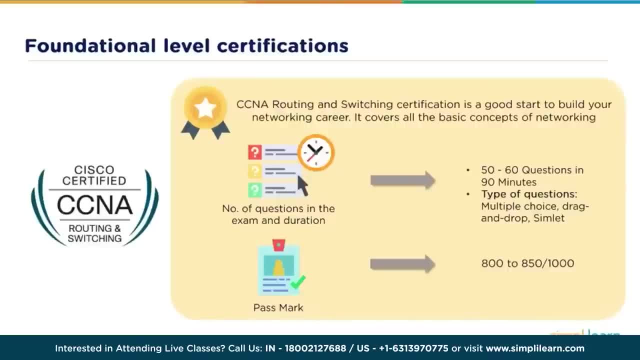 So each question will have a different weightage, depending on the depth of the question, depending on the difficult level of the question or the difficulty level of the question, which would then count towards your marks. And if you score 800 to 850, that's when you clear the exam. 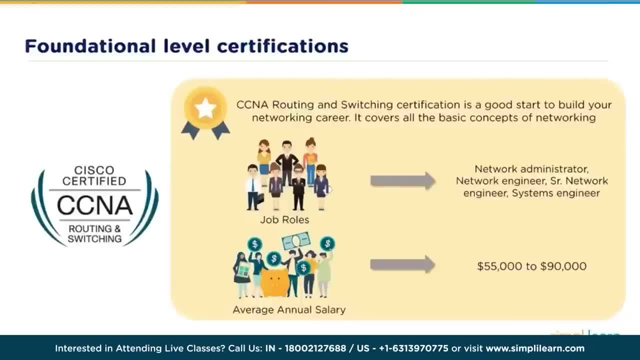 The job roles as we have discussed over here would be more on the network administrator side or a network engineer side, depending on the level of experience that you have. The salaries that are expected from these job roles in the US are around $55,000 to $90,000. 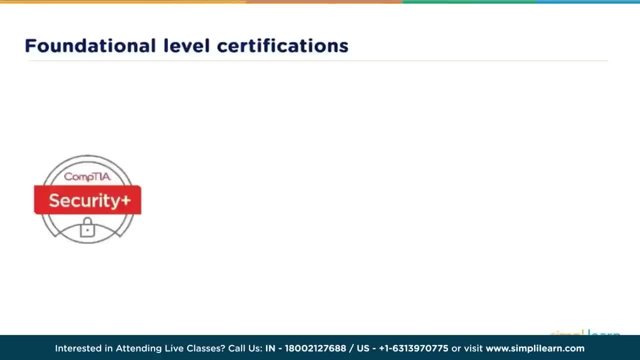 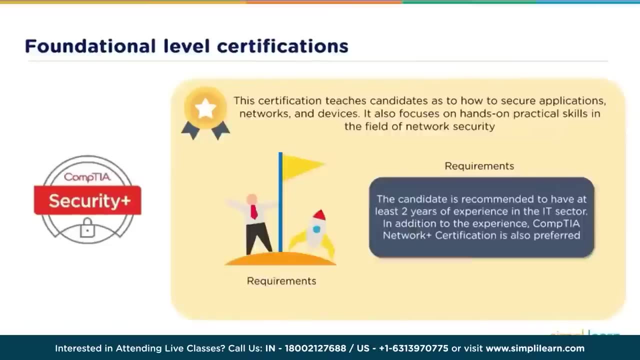 And the next one is the Comcia certification, called Security Plus. Comcia is also a global certification authority for infosec courses, So this certification teaches candidates on how to secure applications, networks and devices. It focuses on hands on practical skills in the field of network security. 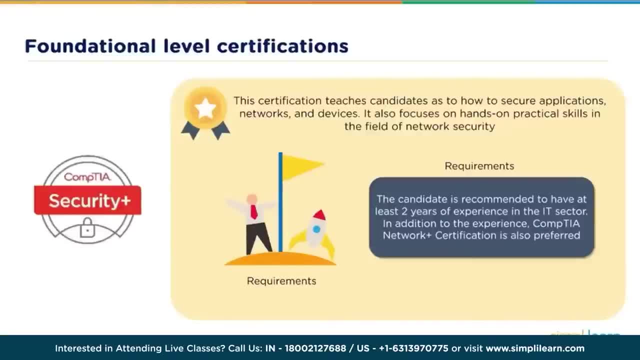 I have trained people on this certification myself so I know this certification is quite hands on. It deals with the concepts to the core. It helps you understand the concepts And then in the practical hands on demo, you need to execute the practical yourself so that you can gain that knowledge. 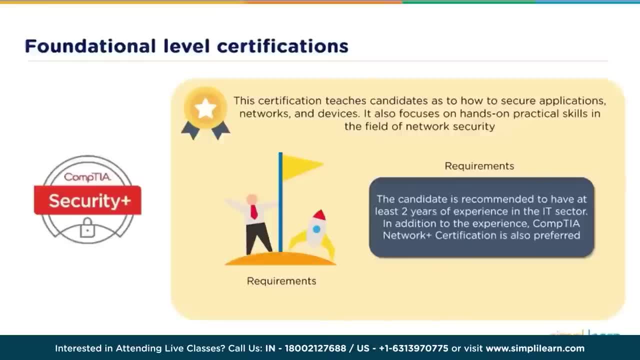 The recommended level for a candidate to attempt this training would be at least around two years of experience in the IT sector. In addition, if you have already been certified for Network Plus certification from Comcia, which is the baseline networking certification, this is also a preferred way to go for this certification. 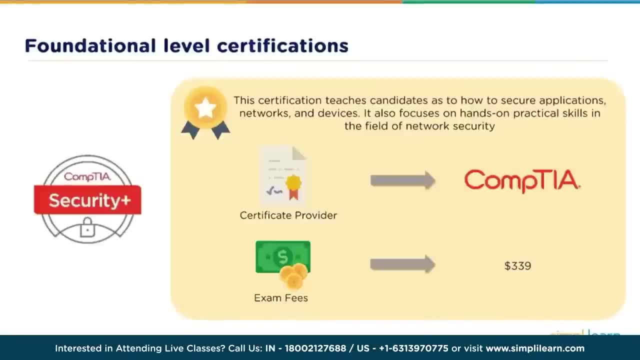 As said, Comcia is the certificate provider and the exam fees for this certification is $339.. The exam is quite simple: 90 questions in 90 minutes, That's one minute per question. It sounds like a lot of time but, believe me, the questions can be a little bit. 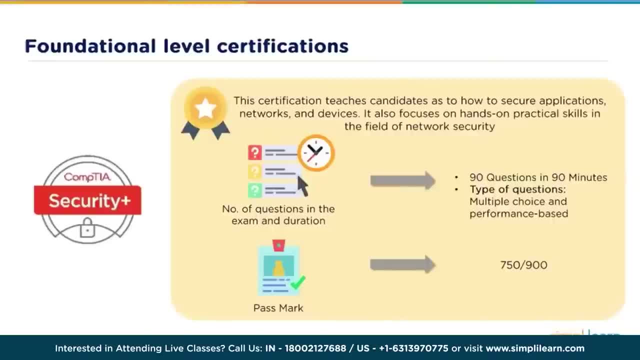 confusing, can be a little bit lengthy, so you will require all those 90 minutes to answer those questions, especially when they're tricky and they're technical in nature. The questions would be multiple choice and performance based. The pass mark for this exam is around 750 points out of a possible 900. 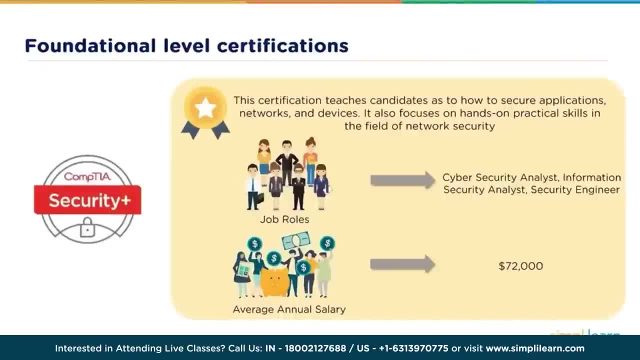 The job profiles for this kind of certification is when you want to apply for a security analyst position or a security engineer's position, where you're going to analyze some data to understand and figure out what problems are ongoing in the organization. The average annual salary of this person would be around $72,000. 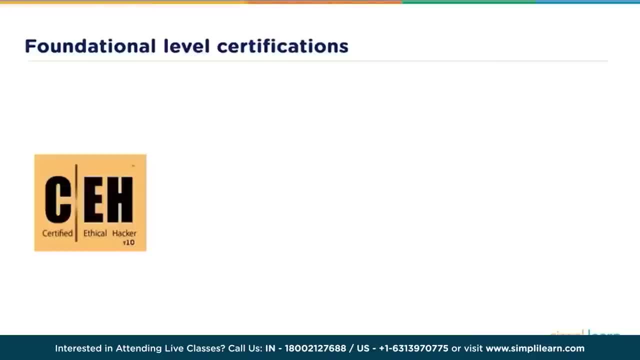 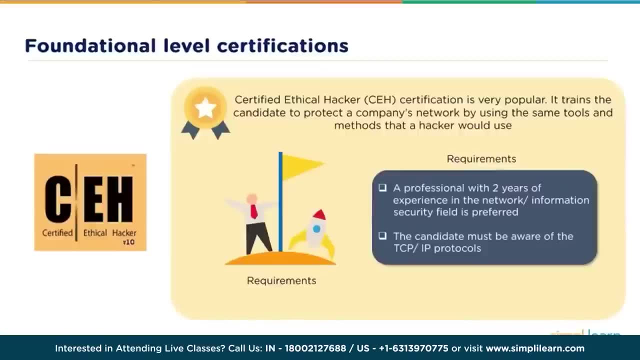 Then comes the CEH, or the Certified Ethical Hacker, training from EC Council. Now, this is a very well-known course And also EC Council is a global certifying authority very well accepted across a lot of countries. This is an offensive certification. 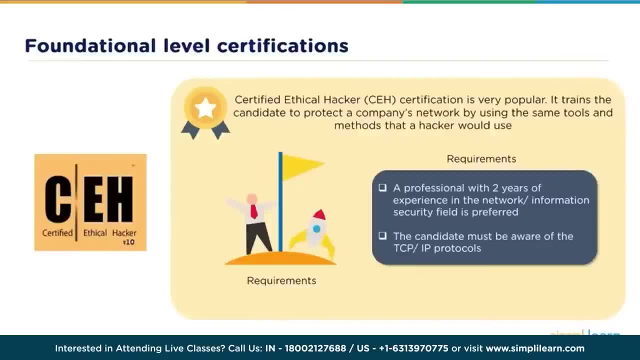 So here you're basically going to become a penetration tester. You're taught how to hack. you're taught how to attack a particular organization from an ethical hacker's perspective. So the job profiles that you'll be looking here are of a pentester where you go into. 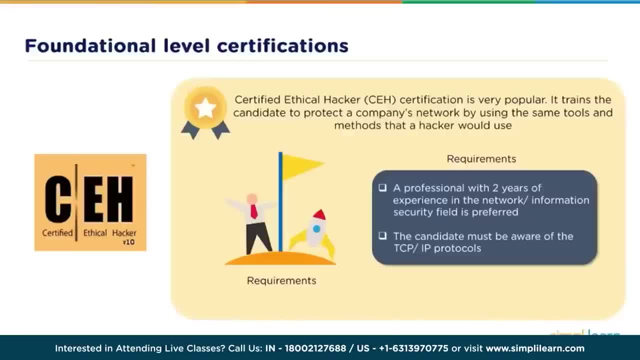 an organization, you test their security controls or you test their devices, find out flaws within them and then provide recommendations of how to plug those flaws or mitigate those flaws and improve the security of that organization. It is recommended that you have two years of experience at least in networking or 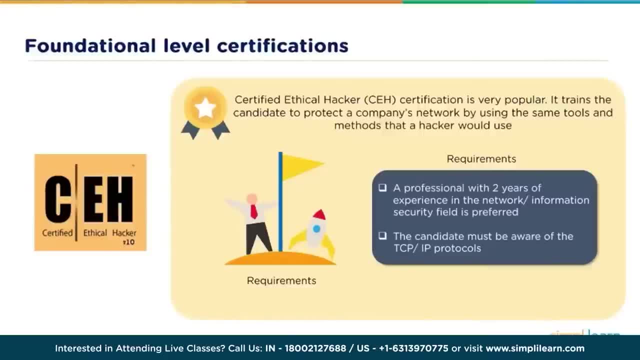 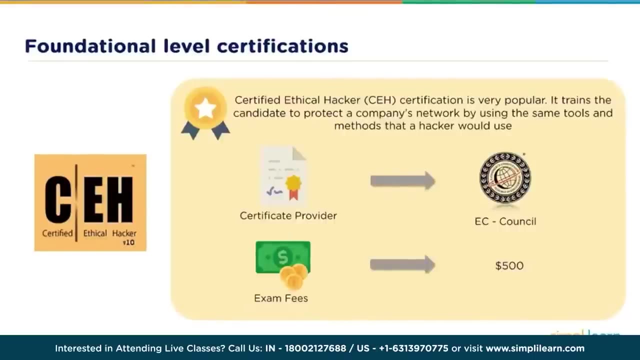 security for these. to attempt this kind of trainings and certifications, Again, a basic understanding of networking, maybe a little bit of applications, operating systems, would be necessary before attempting the certification. The certification provider is EC Council and the exam fees for this certification is $500. 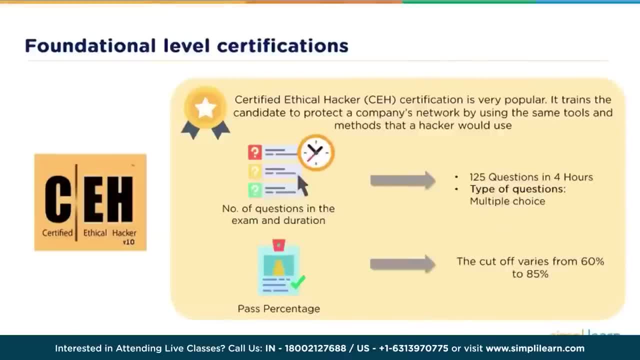 So the exam here would be 125 questions, which needs to be attempted in four hours, And you will only get multiple choice questions in here. For CEH there are two exams: One is the multiple choice questions and the second is a practical exam where you 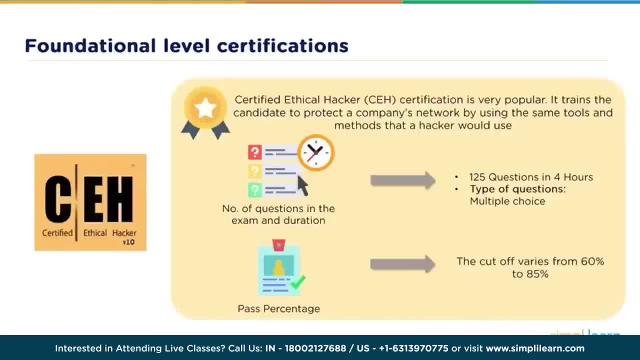 need to solve some given problems to you in an iLab scenario, And if you are able to solve them properly, you then get certified for CEH practical. The cutoff varies from 65% to 85%, depending on the questions that you have. 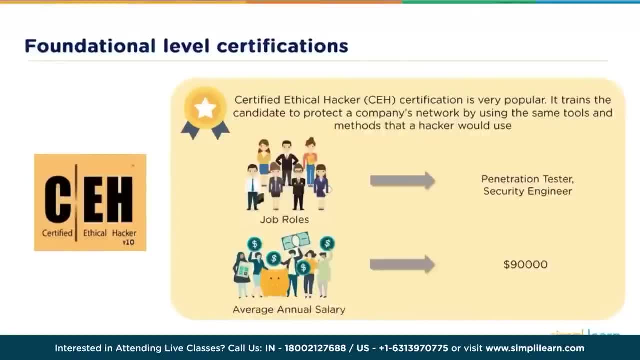 answered and the weightage associated with each and every question. As said, the job roles would be as a penetration tester, a security engineer, and your salaries would start from around $90,000 annually. Then comes the CND, or the Certified Network Defender, also from EC Council. 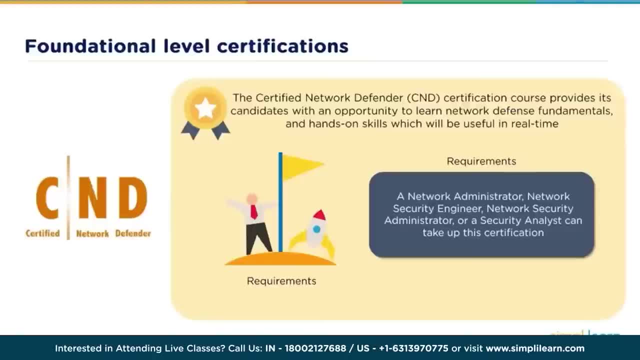 Now this is more on the network defense side. So here again the job roles would be where there's a network that you have and you're going to try to secure the network and the communications that are going to travel over the network. So you need to be a network administrator. 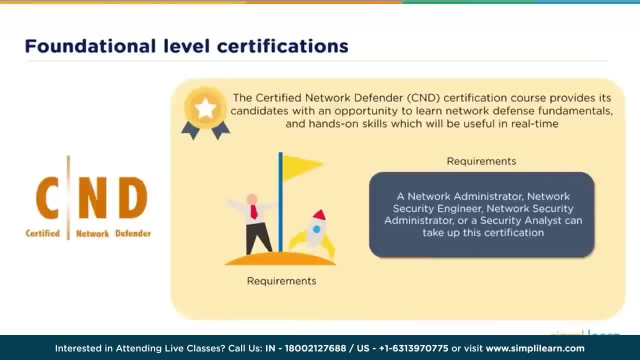 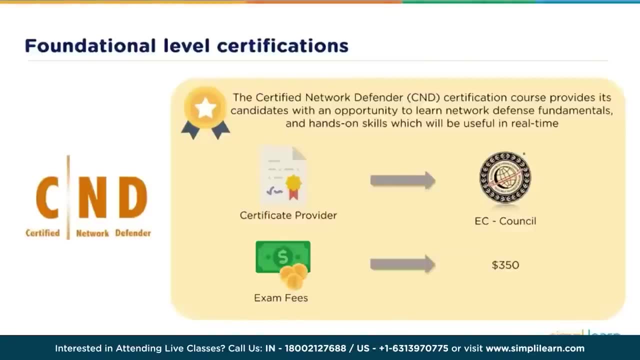 a network security engineer or in a similar profile, to understand how networks work, and then you're going to attempt to secure those networks. The certificate provider again is EC Council and the certification is placed a CEH, so it becomes network defense, then CEH, where you're going to become a penetration tester. 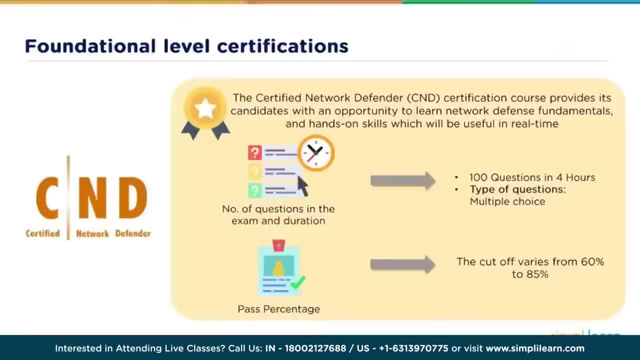 The exam fees for this certification is $350.. The exam is of 100 questions to be answered in four hours. Again, it's just a multiple choice questions, So you get a question with four options. You answer the correct one and you move on to the next question. 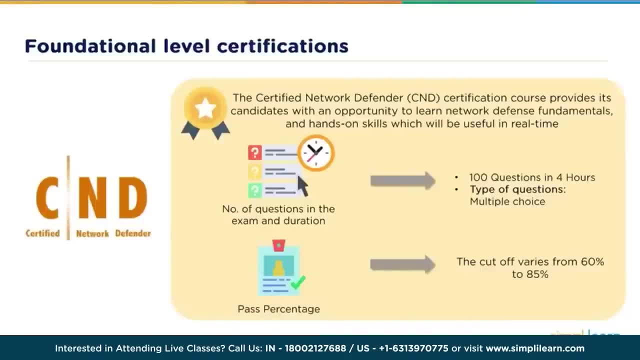 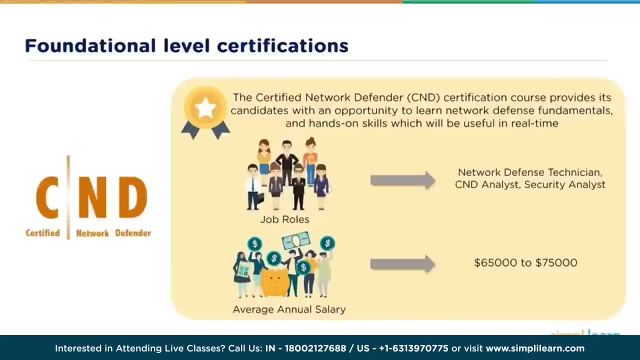 The pass percentage again varies from 60% to 85%, depending on the questions answered and the weightage of that question. Job roles to be applied: Network defense technician, CND analyst or a security analyst. from a network perspective, Salaries would range from $65,000 to $75,000 per annum. 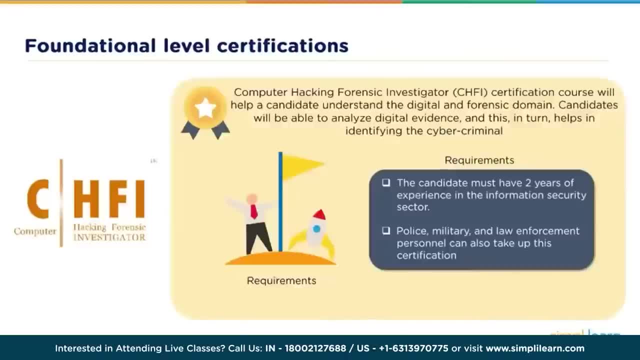 Then comes the forensic investigator course, which is exactly what it is: digital forensic investigator. This will help you understand how computers work, where data is stored and how you can retrieve that data to investigate a crime that has taken place. So the candidate must have at least two. 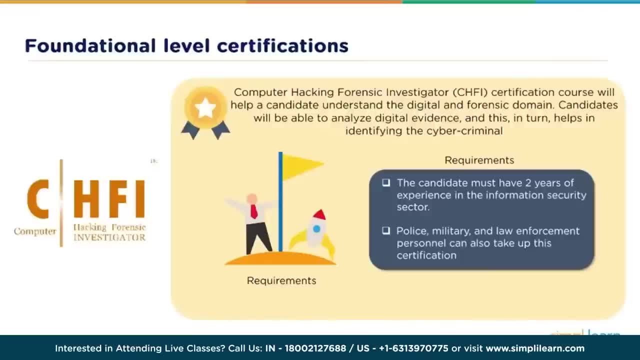 years of experience in the information security sector. They need a good understanding of how their work works work, how computers work, how operating systems work, how they store data, the location where that data is stored, how databases work, how those databases store those data, and so on and so forth. 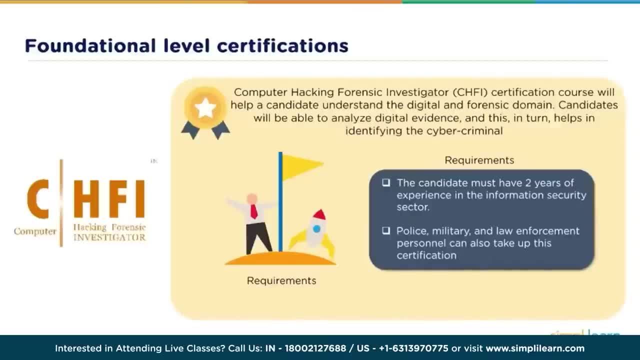 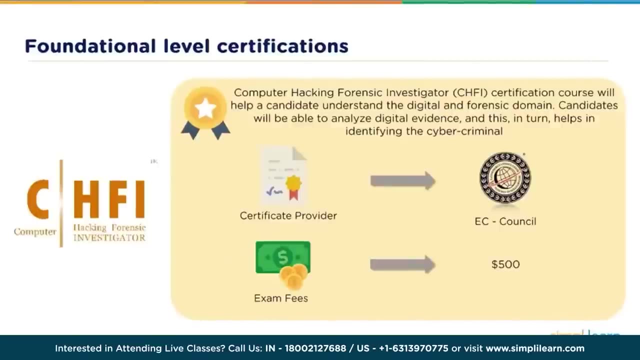 This certification is sought after mainly in the law enforcement areas, But there are a few corporates that offer forensic investigation as a service, especially when a corporate gets compromised, and they want to conduct their own investigations. The certification provider for this is also EC Council, and the exam fees are $5,000. 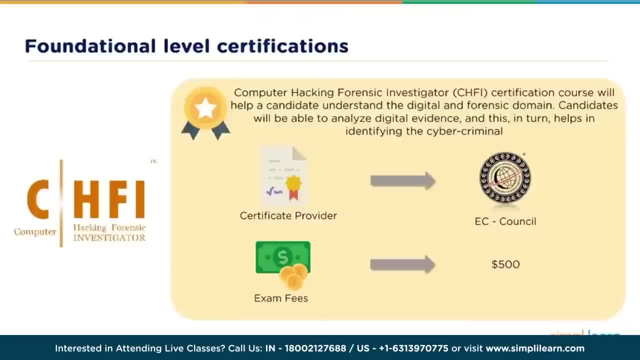 This is an advanced level certification, So understanding of applications, networks and operating systems is a must before you attend this. The exam is quite similar: One hundred and fifty questions in four hours. Again, it's just a multiple choice question exam. The cutoff again is from 60 percent to 85. 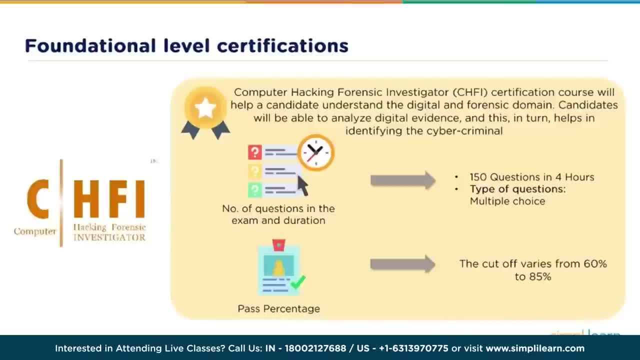 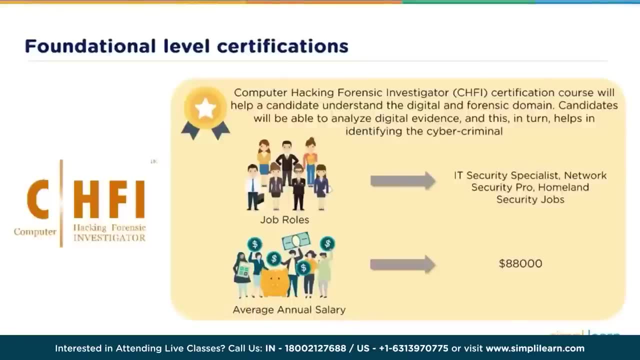 percent, depending on the questions and the weightage of each and every question. Job rules- IT security specialist, network security, pro. The job rules- forensic investigators, law enforcement agencies, security specialists, Homeland Security jobs, and your salaries would be around $88,000 and above. 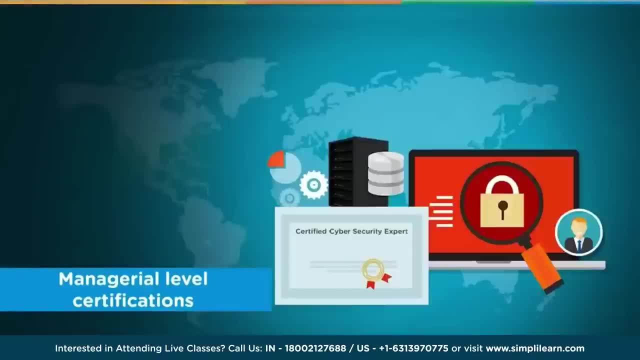 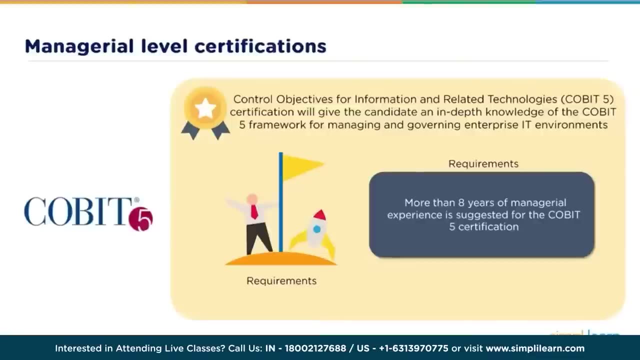 All right, Now let's talk about the managerial level certifications. COBIT stands for Control Objectives for Information and Related Technologies. It's a certification that will give a candidate an in-depth knowledge of the framework which COBIT is all about, and the framework helps you manage and govern. 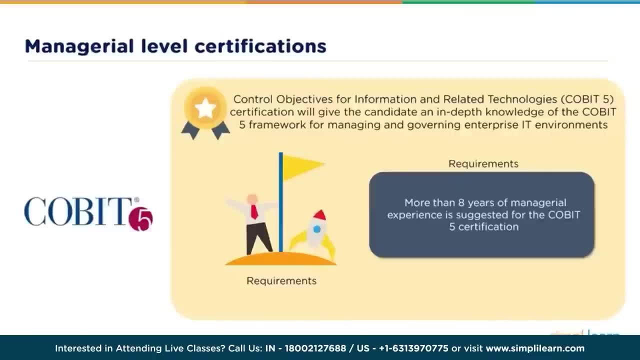 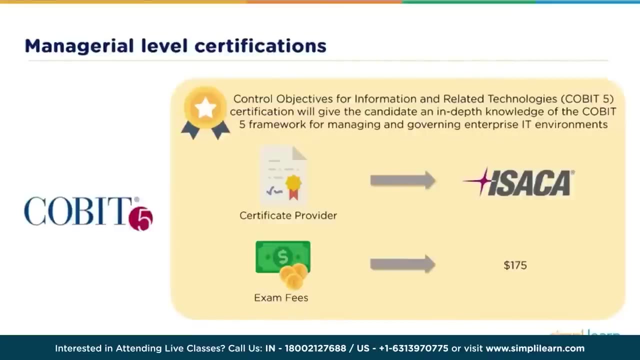 enterprise IT environments. Now, this is an advanced certification, So around eight years of managerial experience is suggested before you attempt a certification, to understand all the aspects and to help you implement the framework properly. The certification certificate provider is ISACA. The exam fees are around one hundred and seventy five dollars. 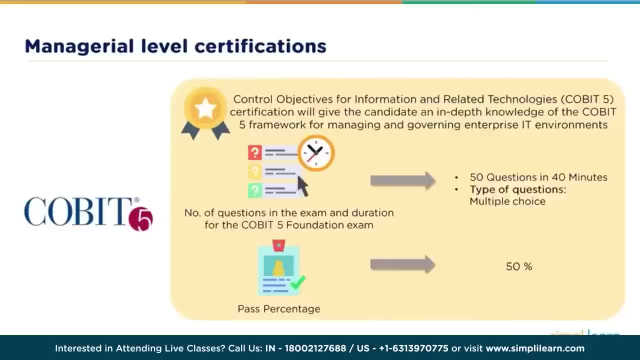 Now, this is a small exam: 50 questions, but in 40 minutes. So you really have to be on your toes. You have to know the knowledge. There's very limited time to think and you have to be fast in your answers. 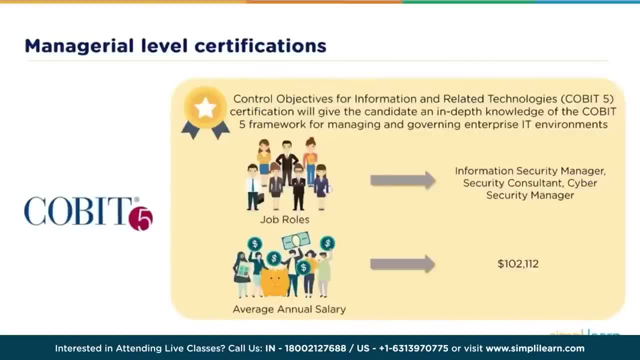 The pass percentage is 50 percent. The job rules associated with this certification would be to when you apply for information security manager or as a security consultant or a cybersecurity manager, and your roles and responsibilities would be to govern the IT space that the organization owns, So all the servers, desktops. 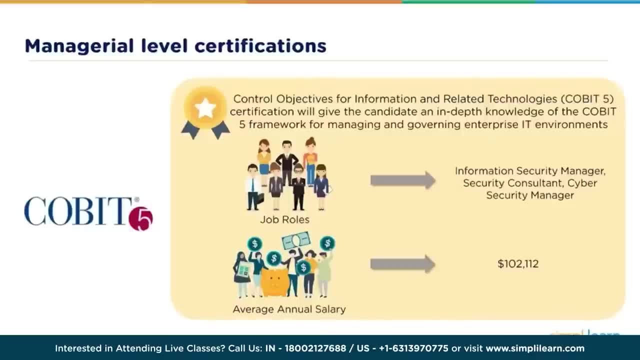 the network, the data flows, the databases, everything, and how it needs to be managed and how it needs to be governed in a secure manner. Annual salaries would be around one hundred thousand dollars plus Then the CISM, also called as. CISM it stands for Certified. 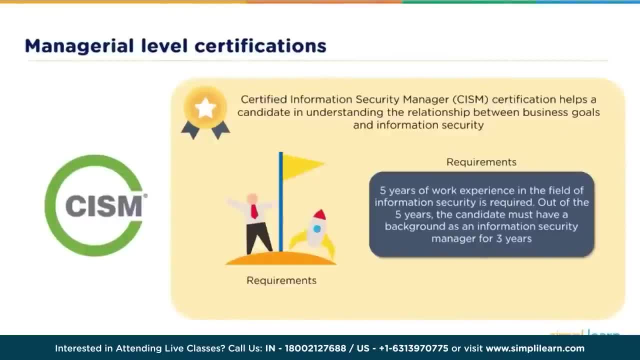 Information Security Manager and, as the name suggests, it's a security manager certification. It helps the candidate in understanding the relationship between business goals and information security. So now you're going into the space where you're not only technical in nature but you also have to understand the business needs, the goals of the business. 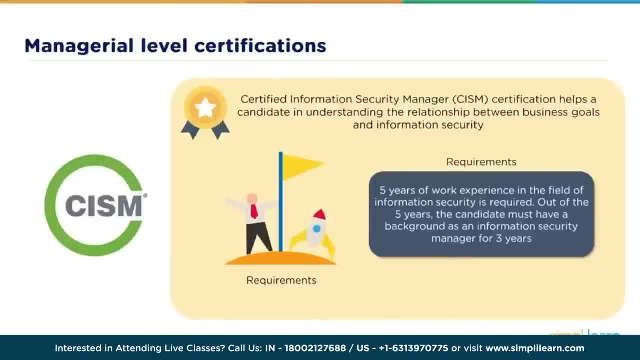 and you have to align the information security of your infrastructure along with the business needs and the business goals. So it is your inputs that are going to go to the management to see if the infrastructure is aligned with the business goals or if the infrastructure or the business goals need any fine tuning. 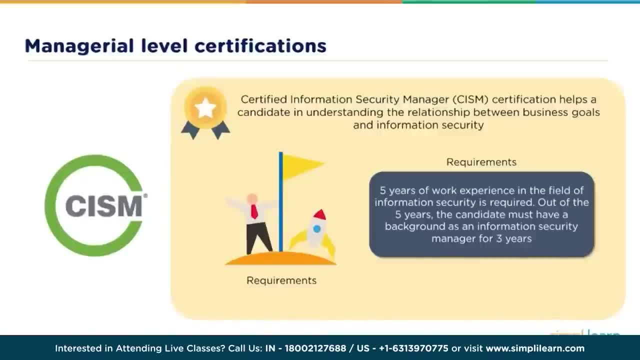 Around five years of work experience is recommended in the information security field for attempting the CISM. Out of the five years, the candidate must have a background as an information security manager for three years. So you have some experience as a manager. You have implemented those things yourselves. 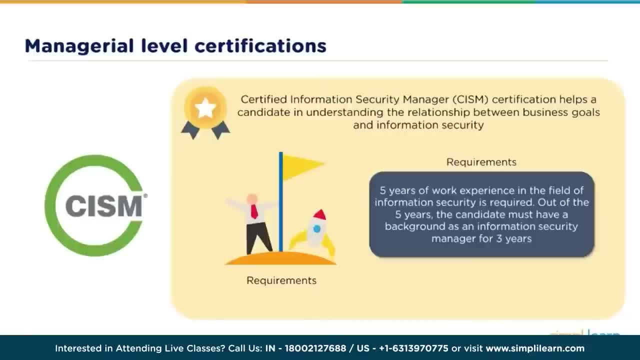 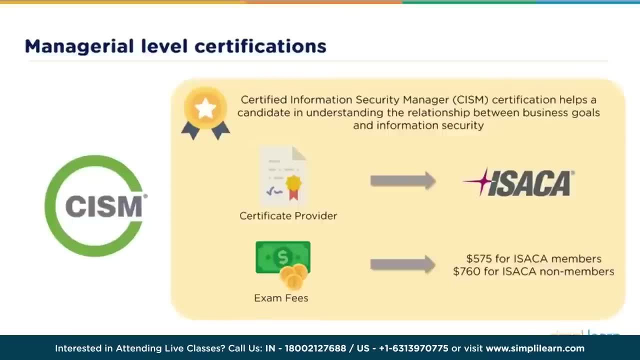 which will give you a better understanding, And then you attempt the certification Again. providing by ISACA and the exam fees for ISACA members is five hundred and seventy five dollars, for non members It is seven hundred and sixty dollars. The exam is where you have to answer one hundred and fifty questions in four hours. 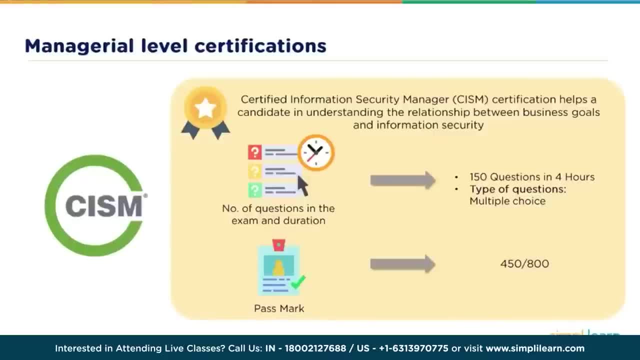 Quite a bit of time, But questions are going to be scenario based questions where they're going to give you a lot of scenarios. You have to think about it and you have to give the most probable and the correct answer for that particular scenario. The pass mark is four hundred and fifty out of eight hundred. 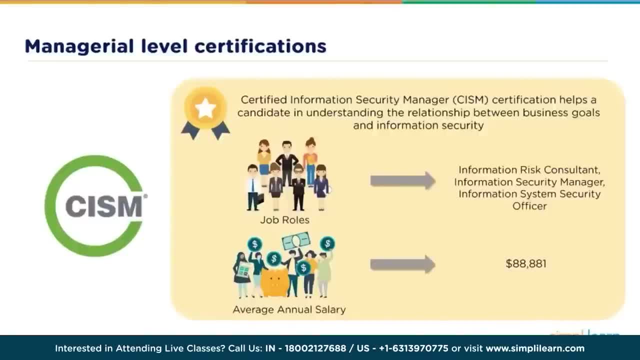 Your job profiles would be either a risk manager or a risk consultant, analyzing those requirements to the infrastructure security that that you have and to identify if there are any risks associated with the infrastructure, highlight those risks and then put in security controls and manage those controls in a way where security is mitigated. 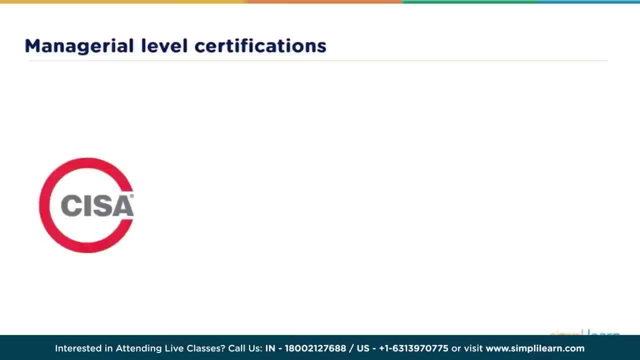 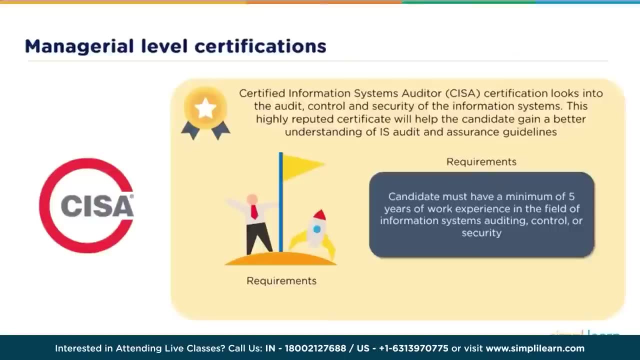 Your average salaries would be around eighty eight thousand dollars and above. Then the CISA or the CISA, the Certified Information Systems Auditor Certification. It not only looks into security, but it also looks into auditing and controls in information systems. This is a highly reputed certificate and you gain a better understanding. 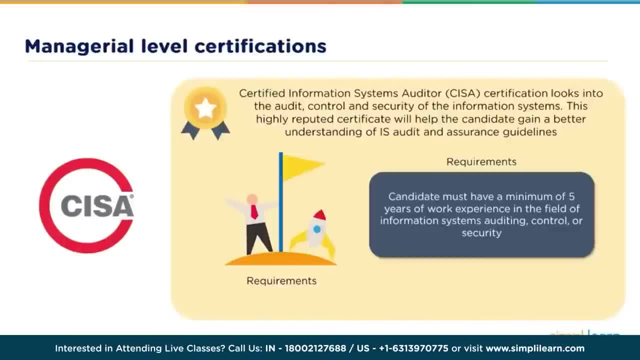 of governance regulations and auditing your information landscape. Again, a minimum of five years of work experience in the field of information systems auditing, control or security is necessary. Now here the question would be: what's the difference? Security is where you're technical in nature. 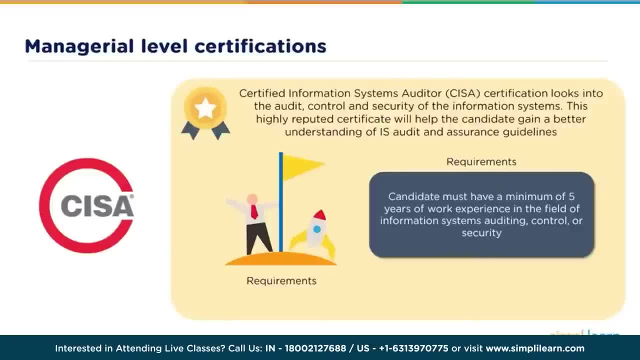 You have done, let's say, a vulnerability assessment or a penetration test. You have implemented firewalls, You have architected security Controls. are all about the security controls that you're going to implement, like firewalls, IDSS, IPSS, data loss prevention systems, maybe even UTMs and whatnot. 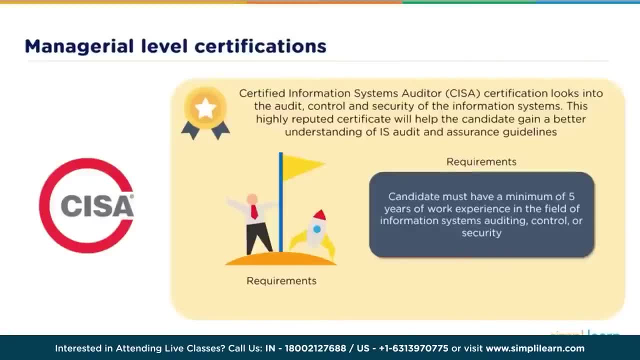 So experience in architecting or implementing those controls in an effective manner, mitigating your security or your vulnerabilities that you have identified in the organization. and auditing would basically mean about looking at compliance to ensure that everything is in place you're compliant with, let's say, ISO 27001. 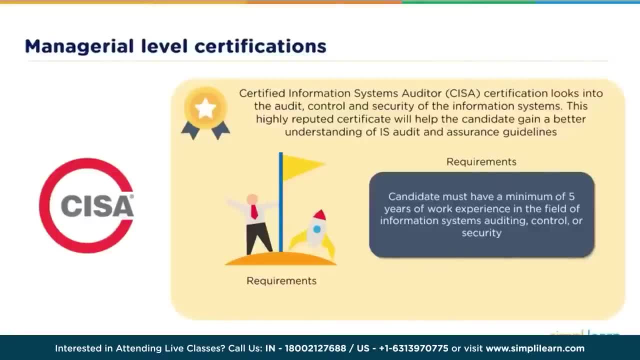 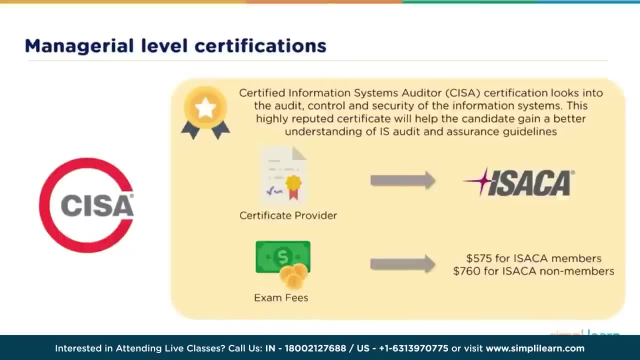 or the policies that you have created yourself, and everything is working in order. So it's more of a checklist where you're going to just check everything is in place and you're conforming to standards. This certification is also provided by ISACA and the exam fees for ISACA members. 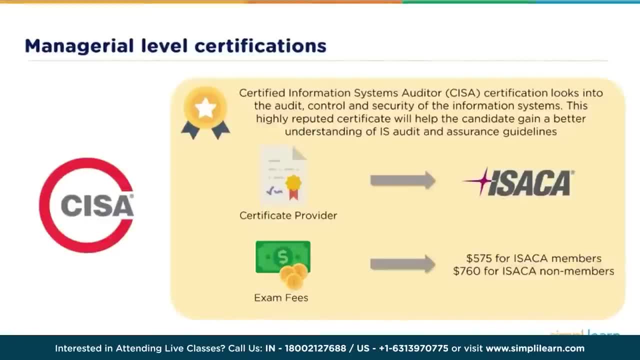 are $575,, whereas non-ISACA members will have to pay $760 for the certification: 150 questions again in four hours, multiple choice questions, scenario based. So you have to really understand the real world scenarios of where, what controls and what audit mechanism should be in place. 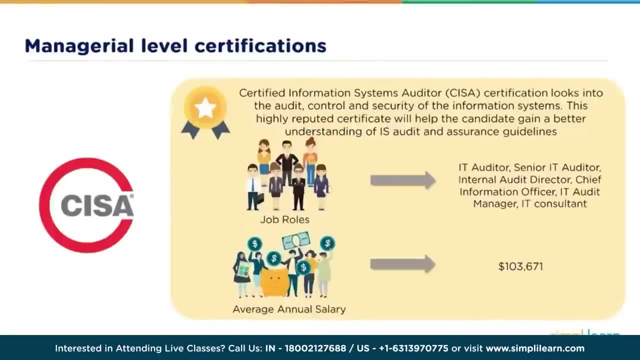 Pass mark is 450 out of 800.. Your job roles would be mainly becoming an auditor or a senior auditor, a director for information security, information audit manager or information technology consultant, where you provide intelligence on how the company should implement their infrastructure. Average salaries would be $103,000 and above. 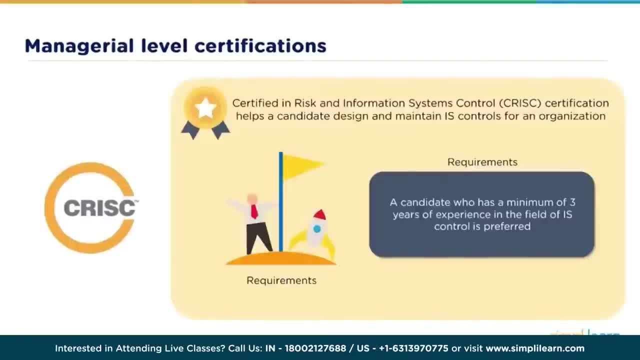 Then comes the CRISC, also known as CRISC, Qualified in risk and information systems control. certification helps the candidate design and maintain information systems controls for an organization. This is one of the most sought after certifications as far as risk management is concerned In Europe and in the US. if you have this kind of certifications, 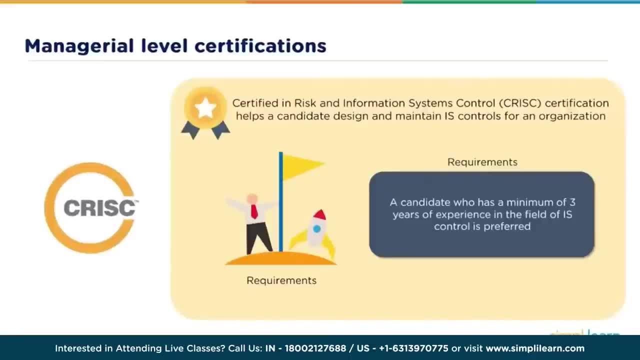 you automatically qualify for a risk manager or a security risk manager or a information security consultant kind of role. You should have a minimum of three years of experience in the field of IS controls. That means information security controls. You should have knowledge about how to mitigate risks, how to identify risks in the first place. 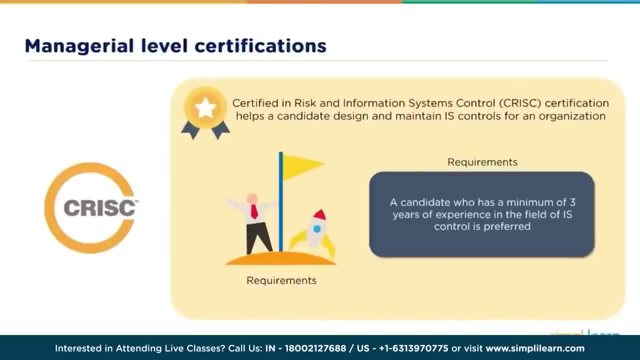 risk analysis, risk management and, after which, you're going to implement security controls to mitigate that risk or bring it to acceptable levels. At this point in time, you will also be responsible to create policies revolving those risks and how you want to calculate those risks and 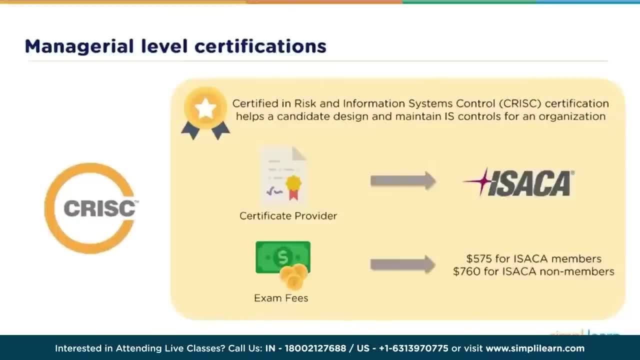 treat those risks in their lifetime? Certificate provider again is ISACA: $575 for ISACA members, $760 for non-ISACA members. That's the minimum you need to pay for the exam fees. A similar question: 150 questions to be answered in four hours. 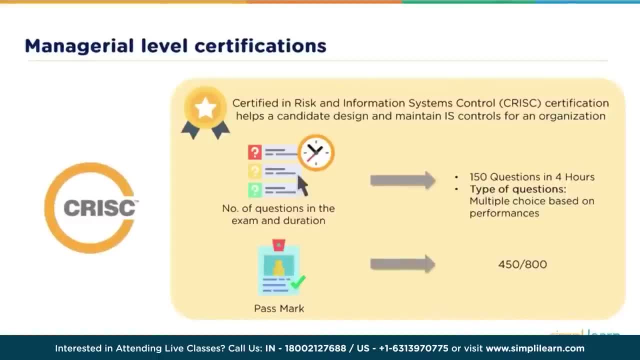 Multiple choice based on performances, So they may give you a scenario where you have to perform a risk analysis and provide a report and a solution based on your findings. Again, the pass mark is 450 out of 800.. The job profile associated, as discussed. 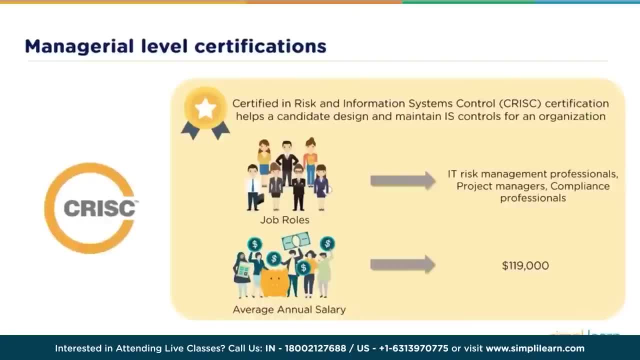 earlier are the IT risk management professionals, where they're going to identify risks, treat those risks, calculate, analyze, maybe do a business review to ascertain how the organization is going to be affected, And then you will also be looking at compliances as far as these job roles are concerned. Average annual salary would be $119,000 and above, Moving on to advanced level certification. Now this is where we come across a CISSP or the CISP certification: Certified Information Systems Security Professional. This is the gold standard of all certifications. 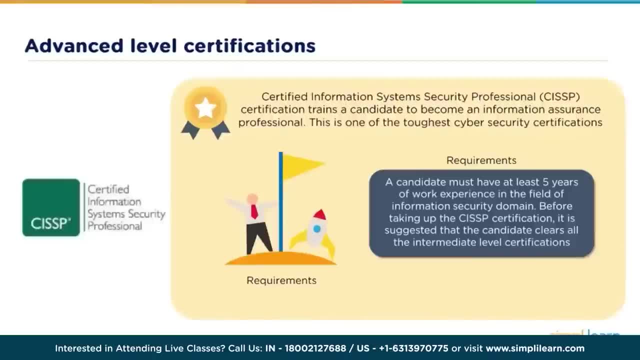 If you have this certificate, you can basically be assured of a job in the IT world. Now, just to qualify, you'll have to have five years of experience in the information security field. There are eight domains that are specified by CISSP, and you have to prove that you. 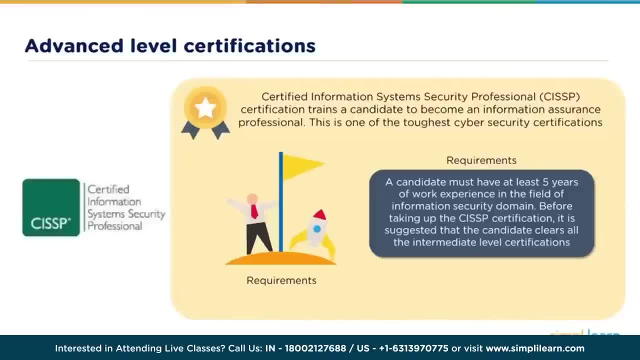 have knowledge and your work experience of around five years in at least two of those domains. If you do not have those kind of experiences, you can still attempt the exam, but you become an associate of ISE Square, which means that you get six years to accomplish the five years. 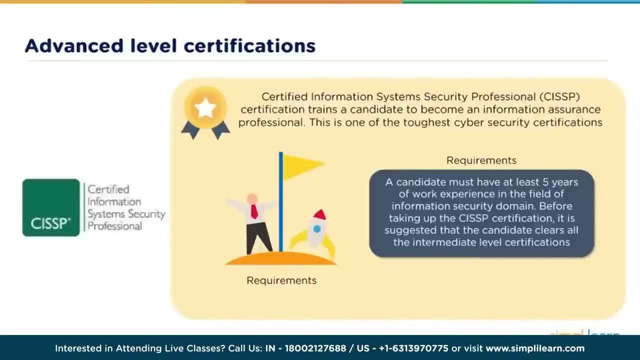 of experience requirement for the certification. Before taking up the CISP certification, it is suggested that the candidate clears all the intermediate level certifications, not all, but some of them. In fact, I have seen people do the other way around: They qualify for CISSP, they give the exam. 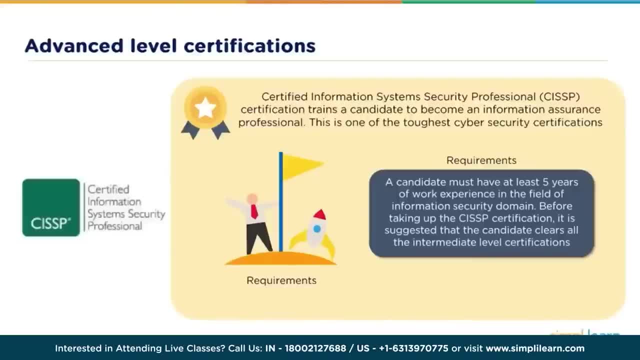 Once you're CISSP, the CISA or CISM exams are way easier to crack, But you need to have that kind of experience. I have seen people with 15 years of experience and more fail at this certification in the first attempt. The certificate provider is ISE Square. 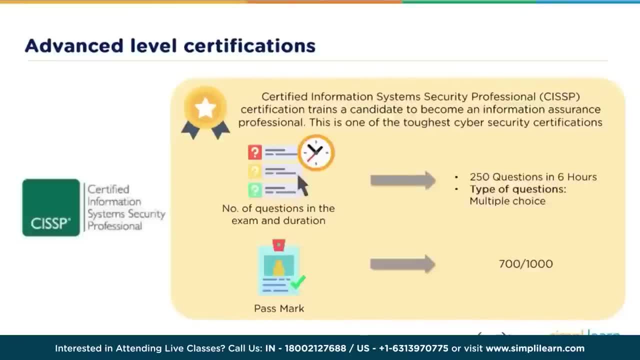 The exam fees is six hundred and ninety nine dollars. Like I said, this certification is most sought after the gold standard. In fact, there is hardly any other certifications after this that you might want to do The questions now. the exam has changed. 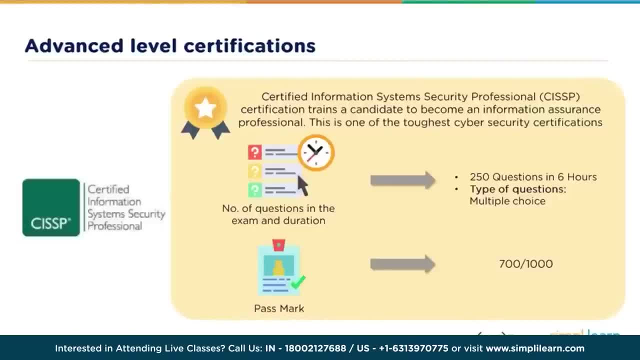 If it is the English version that you're giving, it's one hundred and fifty questions to be answered in three hours. If it is a non-English exam that you are attempting, then it is two hundred and fifty questions in six hours. It's a marathon. 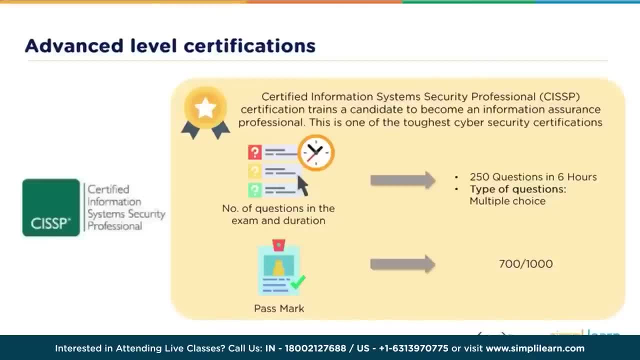 And if you're opting for the six hour exam, you need to plan it really well. It sounds It's really easy, but the questions are quite tough, The scenario based and the answers are quite confusing as well. You would get multiple choice questions. 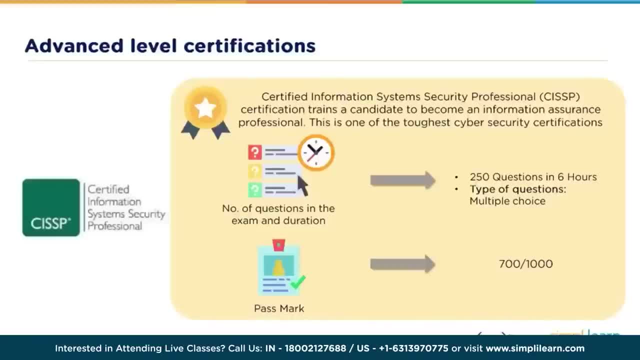 You would get drag and drop and you might get simulators as well. The pass mark is seven hundred out of one thousand, But each question has a different rate age, So it depends on which questions are asked of you and which questions you have answered correctly. 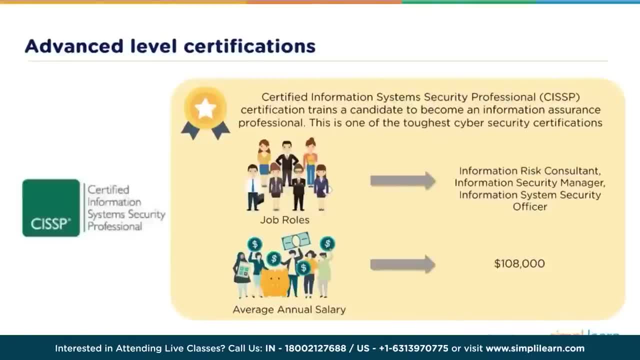 The job rules associated with this certification would be anything and everything in information security at the managerial level and above. So information security manager, risk manager, system information system security officer, the CISO role, the CISO chief information security officer- Any role that you might think of as a risk. 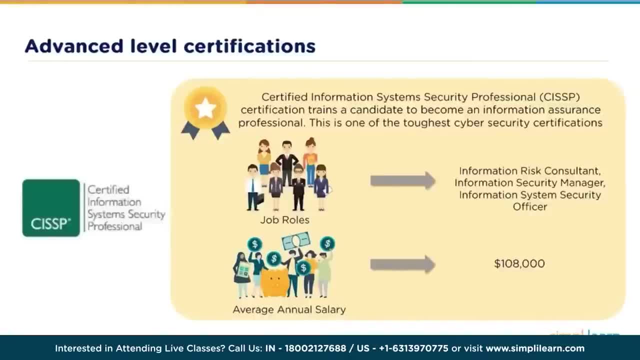 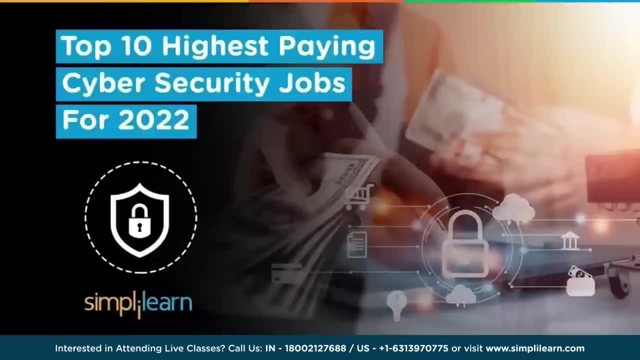 from a risk compliance strategy could be achievable after this kind of a certification. the average annual salary is one hundred and eight thousand dollars for this certification. Technology has become more intertwined with our daily lives. Hence it is no surprise that the need for skilled cybersecurity professionals is. 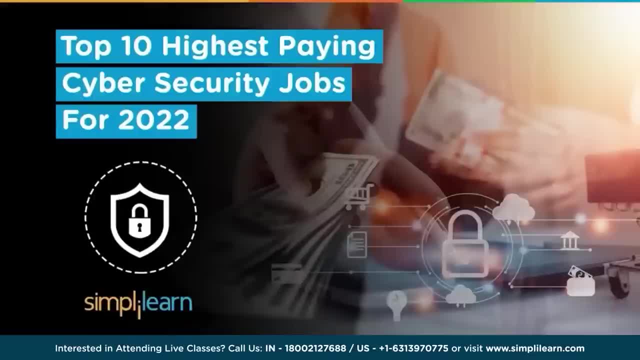 on the rise. Cybersecurity is a lucrative field and there is a dearth of skilled cybersecurity experts. Therefore, currently, a career in cybersecurity is something you should consider if you're looking for an interesting job role. On that note, Hey everyone, welcome to yet another exciting video by Simply Learn. 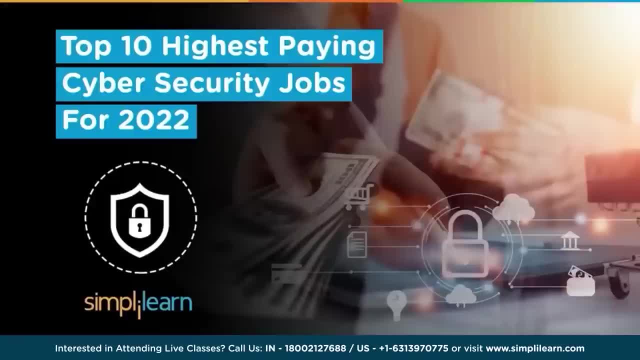 which will take you through the top ten highest paying cybersecurity jobs for 2022.. But before we begin, if you're new here and haven't subscribed already, make sure to hit the subscribe button and the bell icon for interesting tech videos every day. 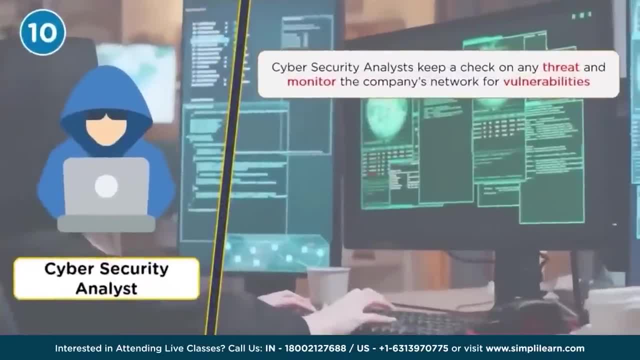 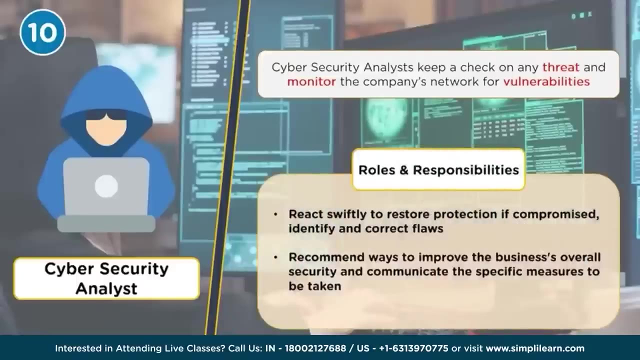 So let's get started At number 10,. we have the job role of a cybersecurity analyst. Cybersecurity analysts are professionals who keep a constant check on any threat and monitor the company's network for potential vulnerabilities. They react swiftly to restore protection if compromised. 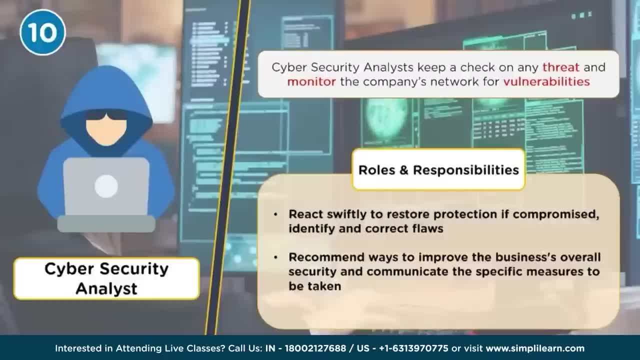 They identify and correct flaws uncovered in the company's applications, programs, security systems, computer networks and more. Cybersecurity analysts even recommend ways to improve the business's overall security and communicate the specific measures to be taken. They compile ongoing safety reports, document security issues and measures taken to resolve them. 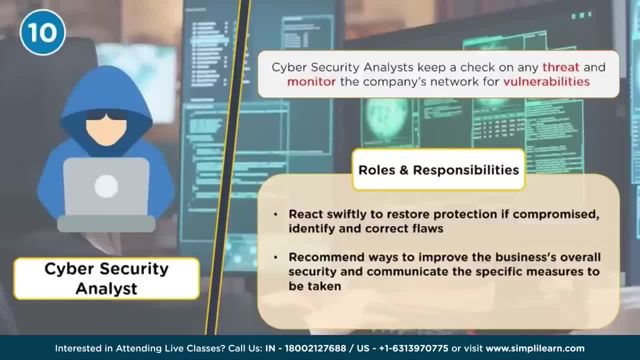 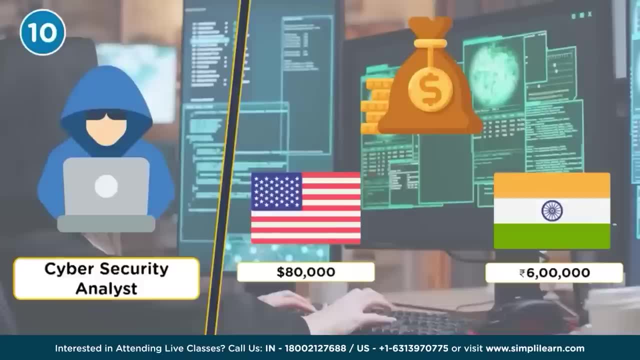 Now let's have a look at the salary of a cybersecurity analyst. According to Glassdoor, a cybersecurity analyst in the United States earns about 80,000 US dollars per annum, and in India you can earn nearly 6 lakh rupees annually. 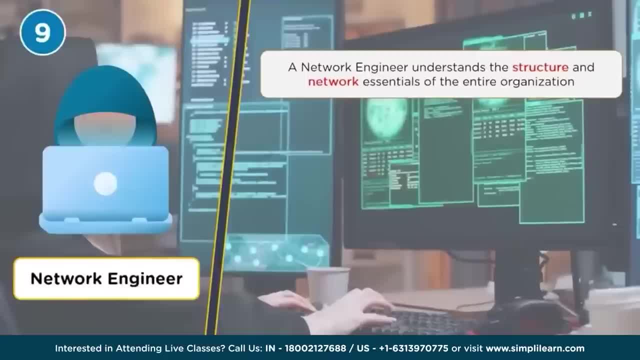 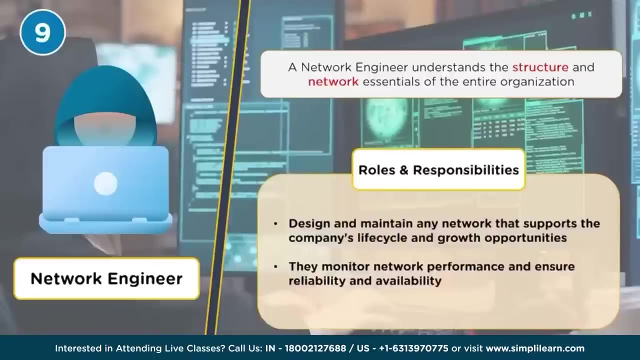 Next on our list we have the job role of a network engineer. A network engineer is a person who understands the structure and network essentials of the entire organization. at a macro level, They design and maintain any network that supports the company's lifecycle and growth opportunities. 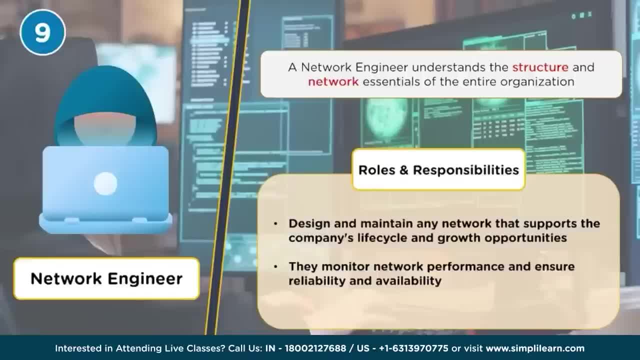 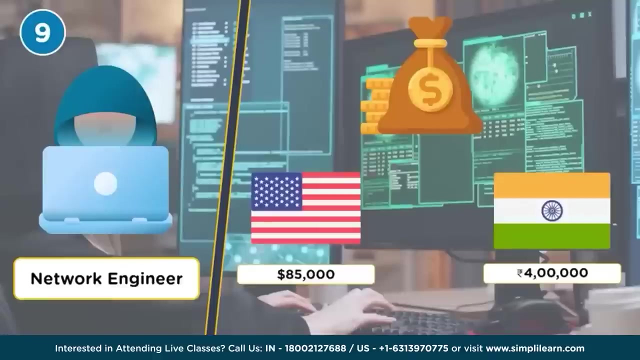 Network engineers take charge of the configuration and installation of network devices and services. They also collaborate with the security team and ensure network security through the implementation of tools and procedures in line with them. They monitor network performance and ensure reliability and availability. According to Glassdoor, a network engineer in the US earns over 85,000 US dollars. 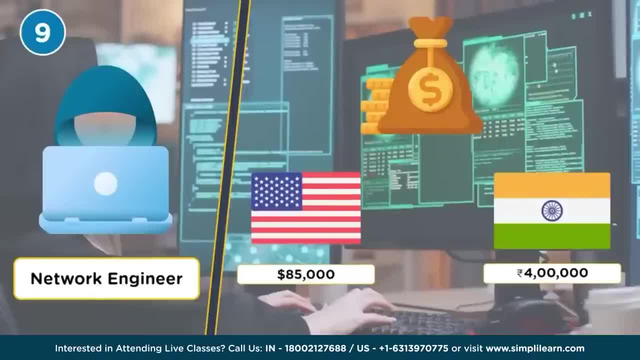 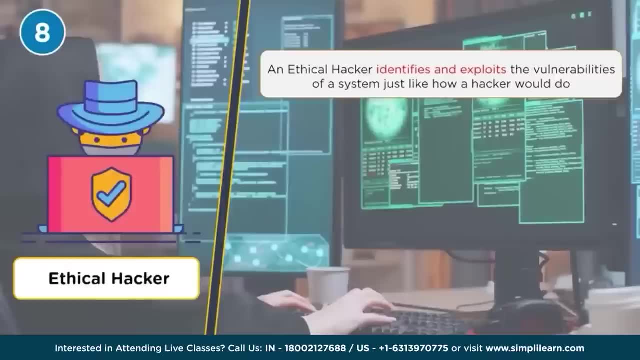 per annum, and in India, the average salary is 4 lakhs annually. Moving on, the next job role on our list is that of an ethical hacker. Ethical hackers are network security consultants who identify and exploit system vulnerabilities just like how a hacker would do. 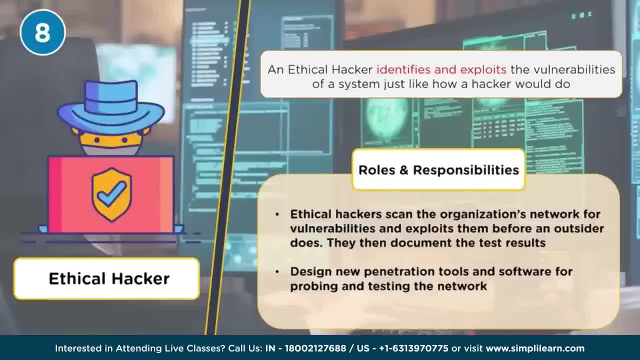 They are also known as white hat hackers. They scan the network and systems for vulnerabilities before a black hat hacker would. Ethical hackers probe and test the network using various penetration tools and software. Additionally, they also design new penetration tools and document the test results. 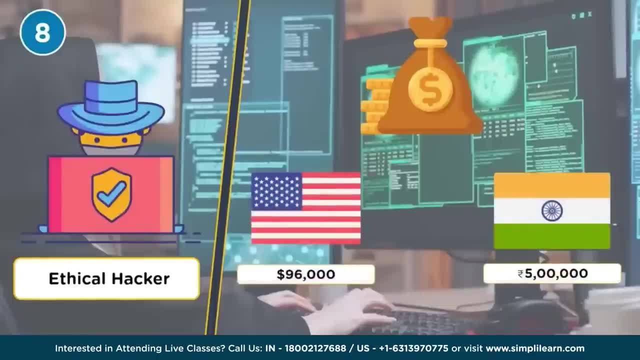 According to Payscale, in the US a certified ethical hacker earns around $96,000 on an annual average basis, and in India they make around five lakh rupees per annum. Moving to our next job role, we have malware analyst. 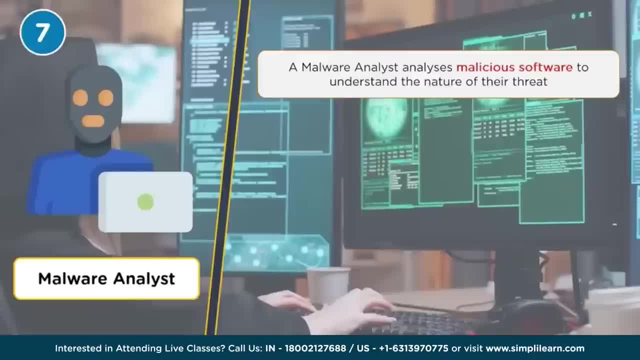 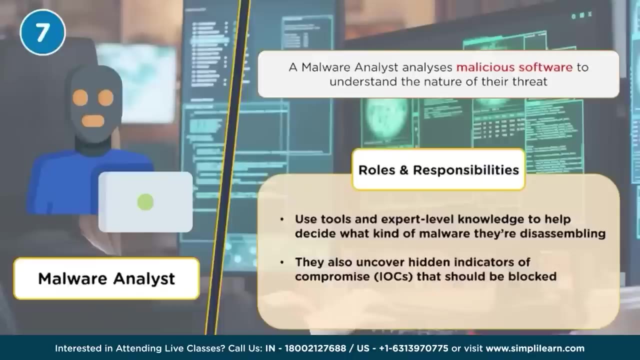 A malware analyst analyzes malicious software- that includes bots, worms and Trojans- to understand the nature of their threat. A malware analyst has a dual mentality by being both forward thinking and reverse thinking. Moving on to the responsibilities of a malware analyst, Firstly, they use tools and expert level knowledge to help decide what kind 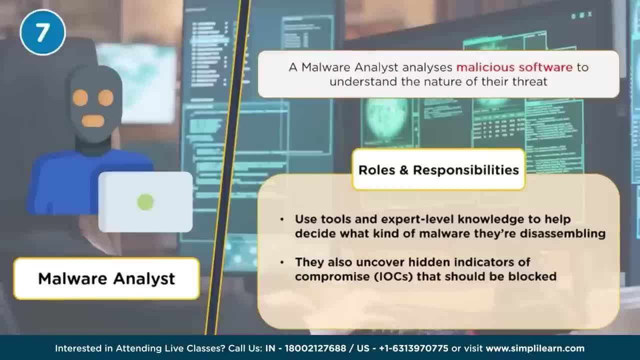 of malware they are dissembling, and if they have encountered this particular kind of malware before You will use dynamic malware analysis tools to achieve insight into software attacks. Secondly, they also uncover hidden indicators of compromise that should be blocked and keep an organization's software updated to protect against the latest malware threats. 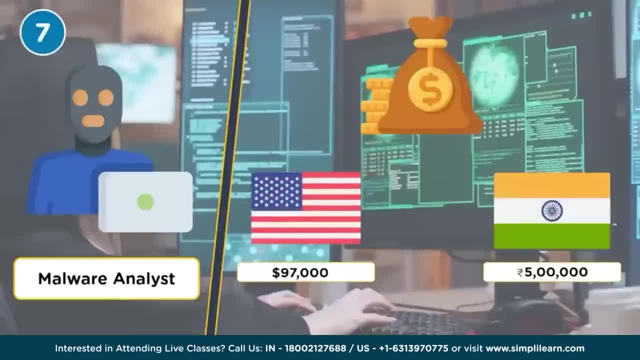 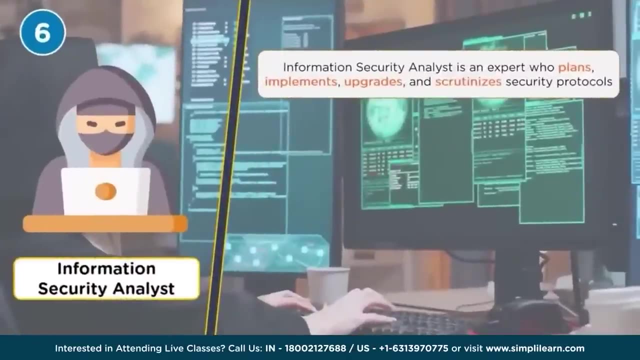 According to Glassdoor, in the US a malware analyst can earn about $97,000, and the average salary for a malware analyst is around five lakh rupees in India. Up next, we have another very interesting job role. that is, information security analyst. 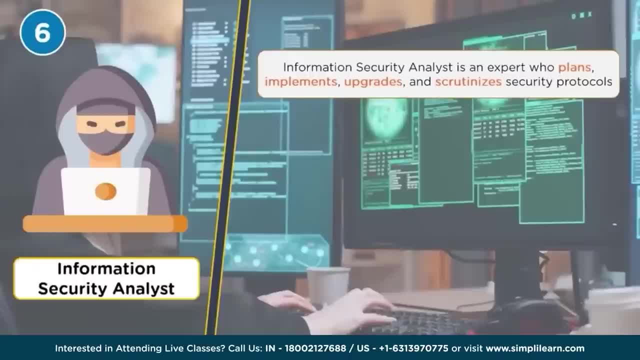 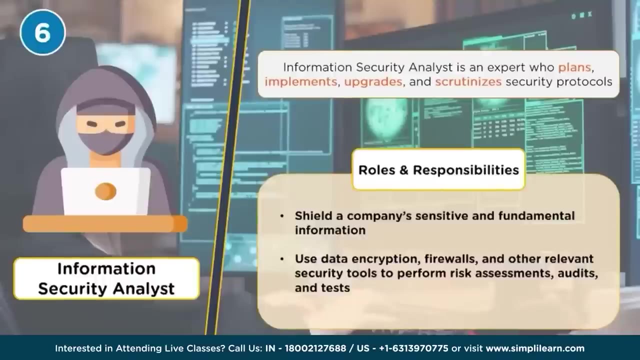 An information security analyst is an expert who plans, implements, upgrades and scrutinizes security protocols to safeguard an organization's computer networks and information. These professions play a vital role in the public, private and nonprofit business sectors, because they shield a company's sensitive and fundamental information. 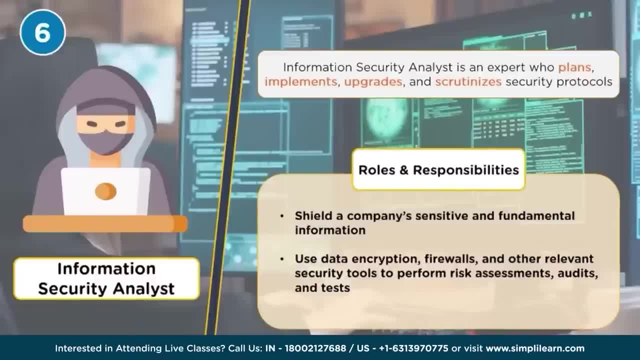 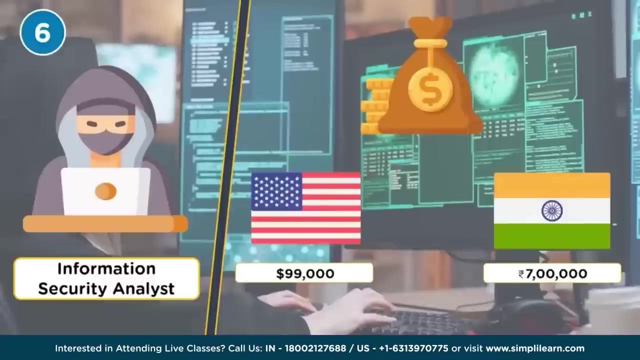 They use data encryption, firewalls and other relevant security tools and applications to cover and protect transfers of secret digital information. Information security analysts perform risk assessments, audits and tests to ensure the proper functioning of data processing activities and security measures. As per Glassdoor, the national average salary of an information security analyst: 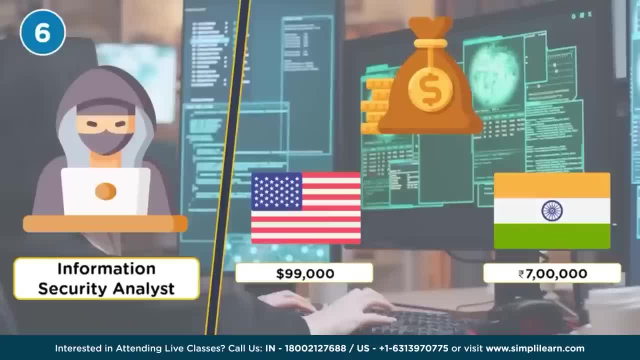 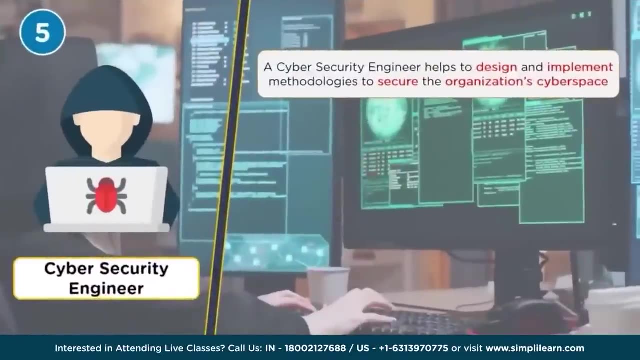 is around $99,000.. In India, the average salary of an information security analyst is around around 2.5 lakh rupees. This is a significant increase in the amount of money earned per person. To put this in one word, it means that the rate of activity is. 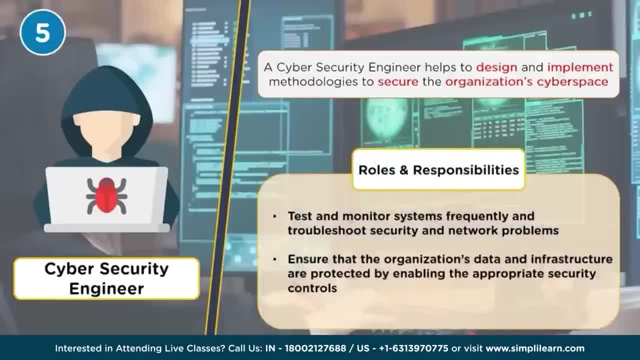 higher than the rate of activity of an artificial intelligence analyst. Let us look at the next highest paying cyber security jobs, that is, cybersecurity engineer. to defend the information, They troubleshoot security and network problems and ensure that the organization's data and infrastructure are protected. 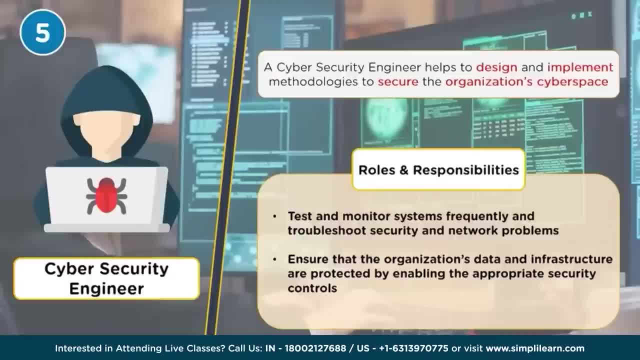 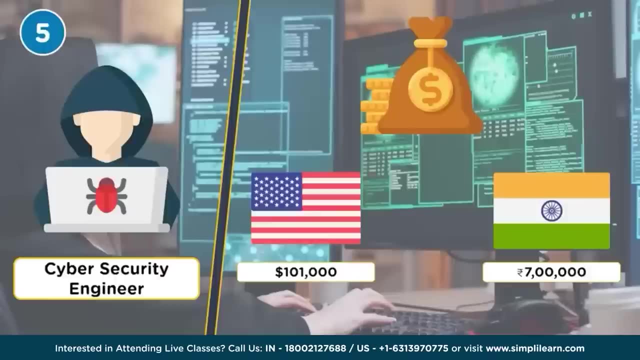 by enabling the appropriate security controls. Cybersecurity engineers also conduct tests and scans to identify any vulnerabilities in the network and system. Talking about the salary, in the United States, a cybersecurity engineer earns over $101,000 per annum As per PayScale, the average salary for a cybersecurity engineer in India. 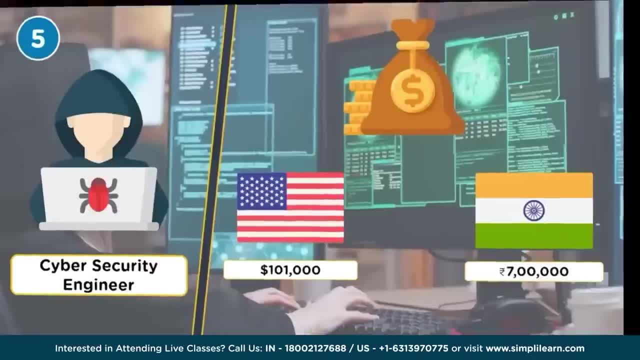 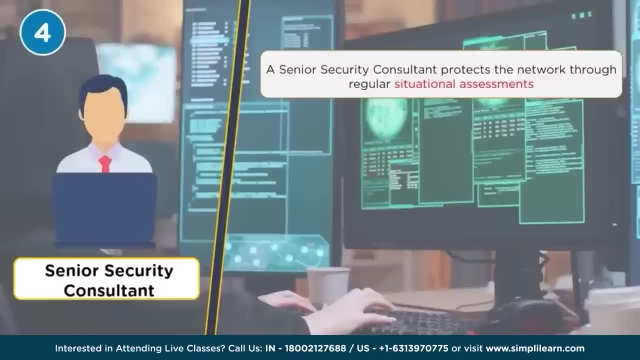 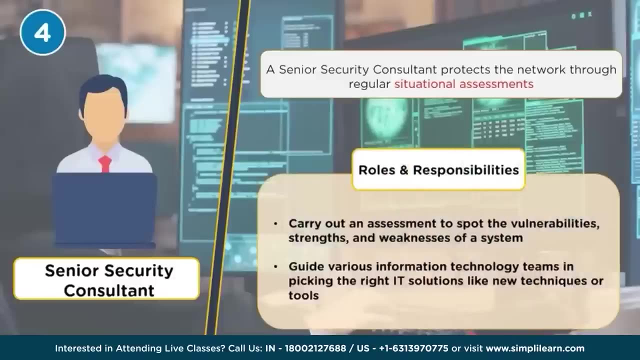 is nearly Rs 7 lakh. Moving on to the next job role, we have Senior Security Consultant. A Senior Security Consultant protects their client's network through regular situational assessments. Senior Security Consultants are required to carry out an assessment of security networks to spot a system's vulnerabilities. 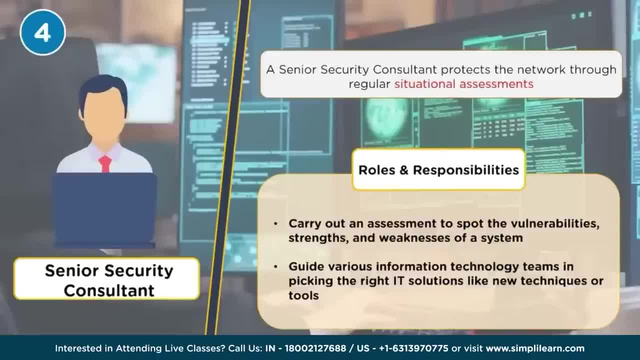 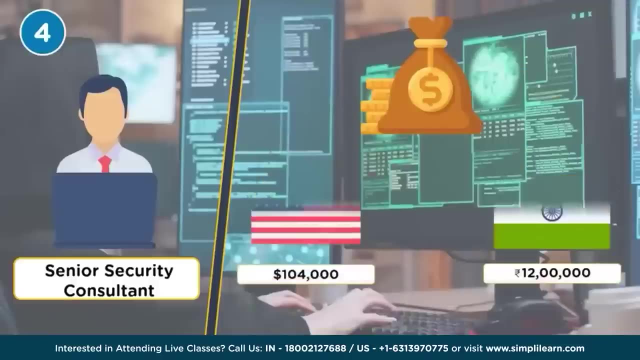 strengths and weaknesses, Following which they guide different IT teams in strengthening their security by helping them pick the right solutions like new techniques or tools. They also create preventive measures against future cyberattacks. According to Indeed, the average annual salary of a Senior Security Consultant in the States is around $104,000. 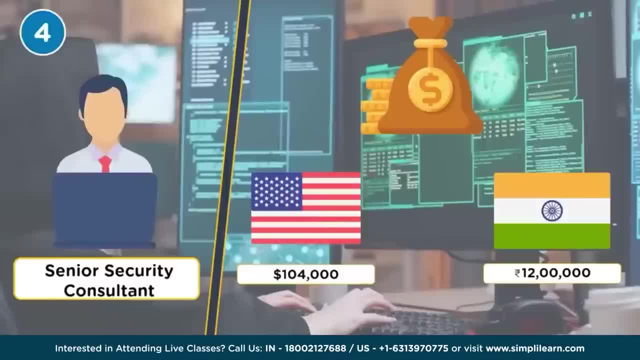 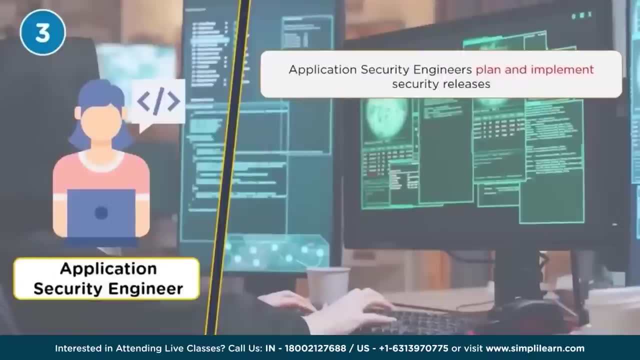 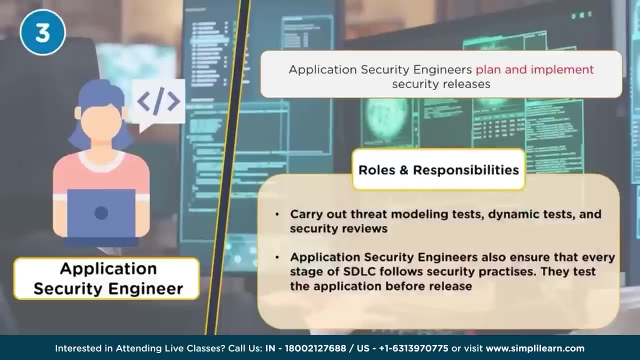 and in India it is nearly Rs 12 lakh. Next, we have the role of an Application Security Engineer. Application Security Engineers work with product managers and developers to plan and implement security releases. In order to understand any vulnerabilities within products, they carry out threat modeling tests, dynamic tests and security reviews. 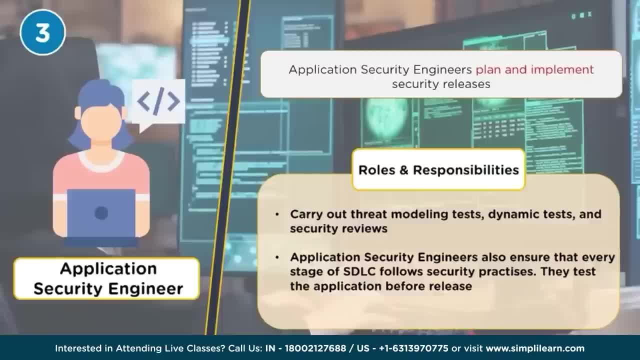 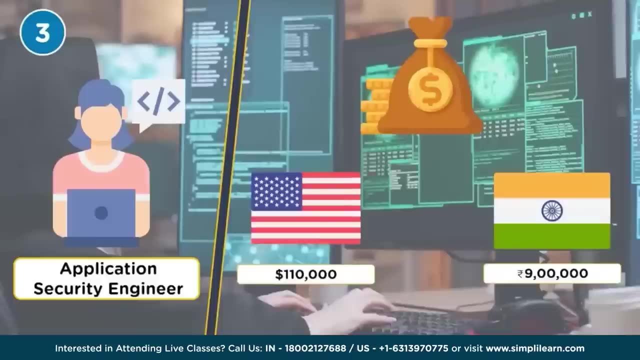 Following this, they optimize a given product's efficacy. They ensure that every step of the software development lifecycle follows best security practices. They also help in testing the application against security risks before release. According to Glassdoor in the US, an Application Security Engineer. 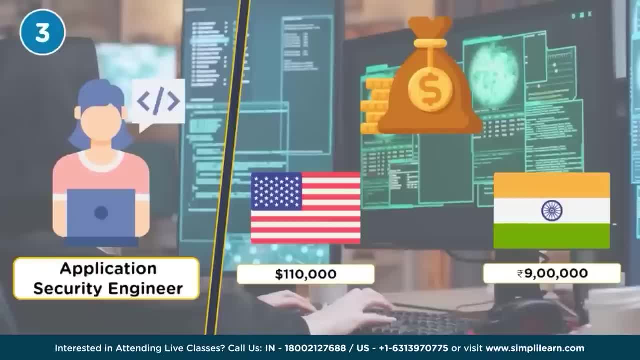 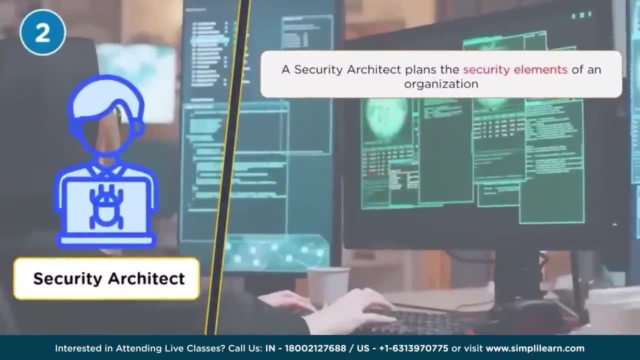 earns around $110,000 on an annual average basis and in India they make around Rs 9 lakh per annum. Moving on to our next job role, we have Security Architect. A Security Architect researches and plans the security elements for their firms. 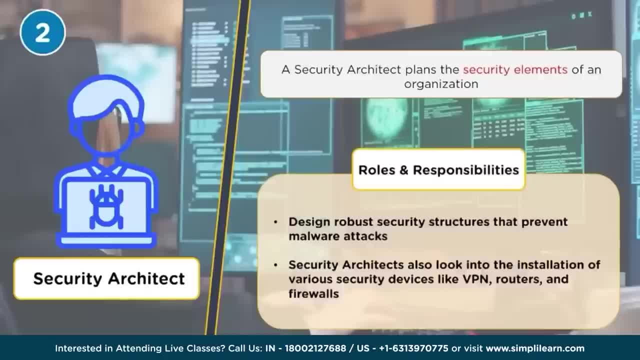 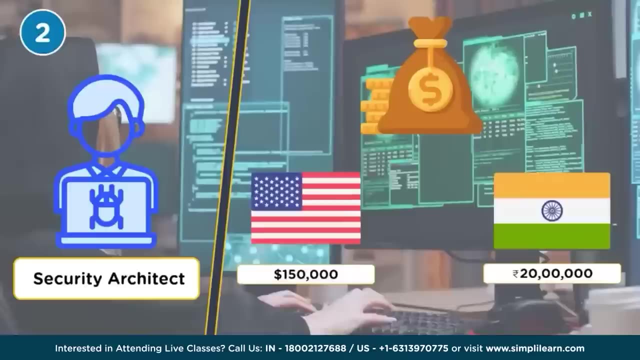 They formulate company procedures and user guides. They design robust security structures that are capable of preventing malware attacks. Additionally, they also approve the installation of VPN routers and firewalls. According to Glassdoor, a Security Architect in the US makes a handsome sum of $150,000 a year on an average. 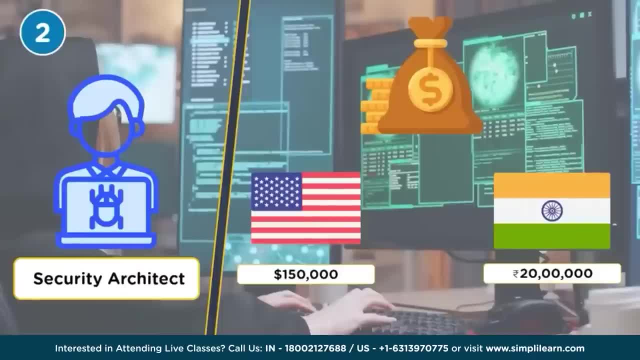 and in India they make around Rs 20 lakh per annum. And finally, at number 1, on our list, we have the role of a Chief Information Security Engineer. We have the role of a Chief Information Security Engineer. We have the role of a Chief Information Security Engineer. 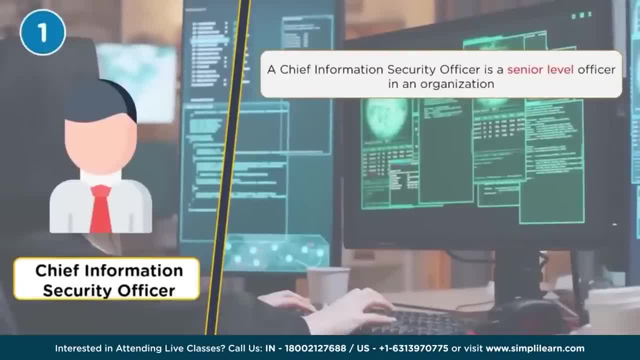 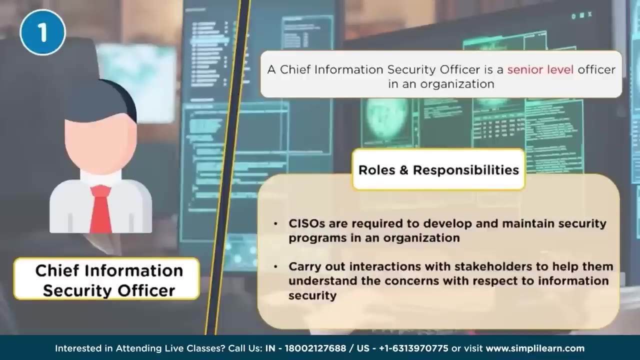 We have the role of a Chief Information Security Officer, CISO. CISOs are senior-level officers in an organization. Their duty is to ensure the safety of the information. They develop, implement and maintain information security and risk management programs. Additionally, they also interact with stakeholders. 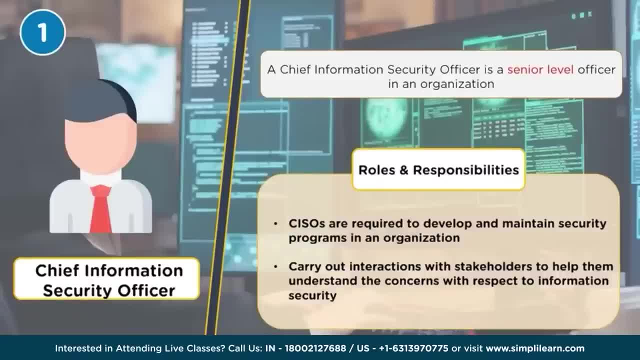 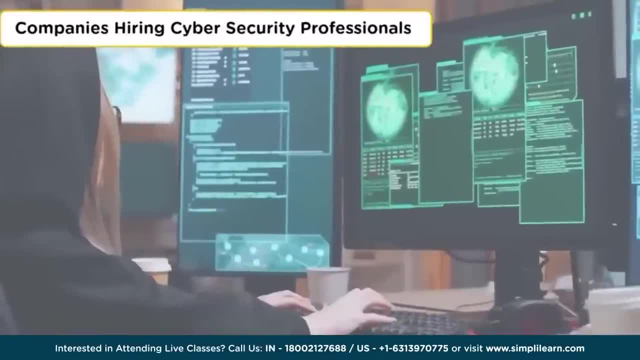 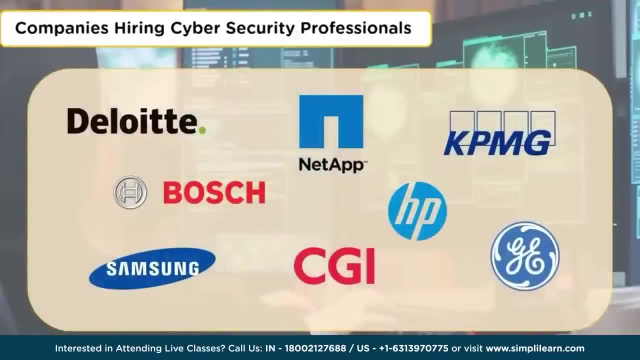 So those were the top 10 highest paying Cybersecurity jobs for 2022.. Now let's have a look at the companies hiring Cybersecurity professionals. Here we have Deloitte, NetApp, KPMG, Bosch, HP, Samsung, CGI and GE, to name a few. 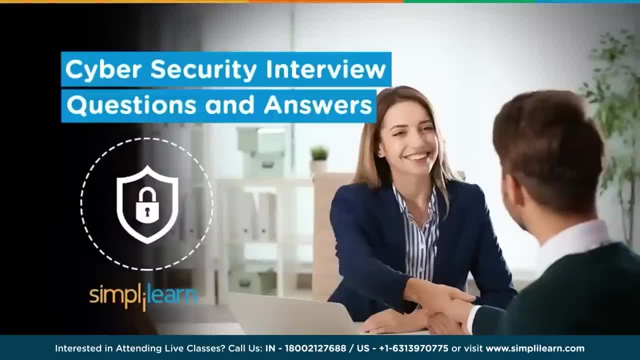 In this series we are going to discuss about the interview criteria that will be asked to candidates in the cybersecurity field. We are going to look at multiple options over here and we're going to discuss various fields in which these questions will be asked. In this video we are going to look at 10. 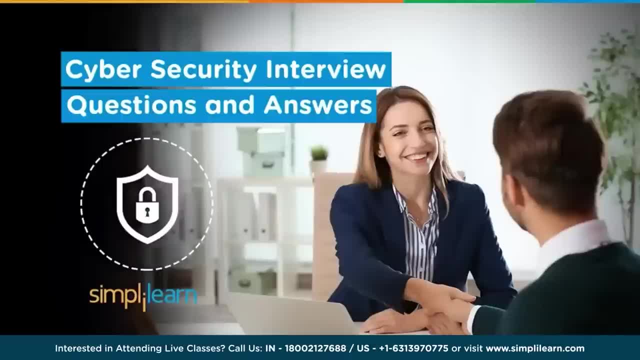 different questions on networking, then we'll have 10 more questions on software and programming, another 20 questions on operating systems and applications, 10 questions on cyber attacks and then finally, 10 questions on cryptography. So we're going to discuss over 50 odd questions each in these different fields. 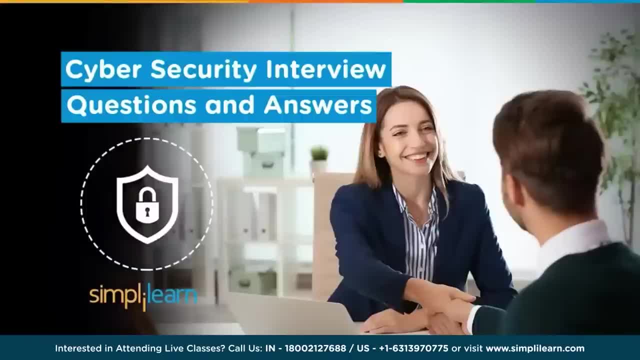 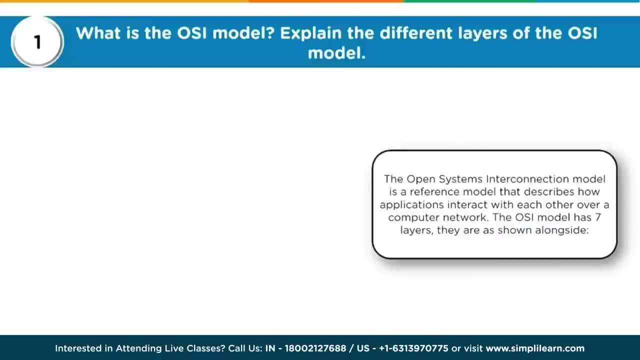 which will help you crack your interviews as far as cybersecurity is concerned. Let's start off with networking questions. Let's start off with question 1.. What is the OSI model? Explain the different layers of the OSI model. OSI, largely, is a theoretical model utilized to understand networking and 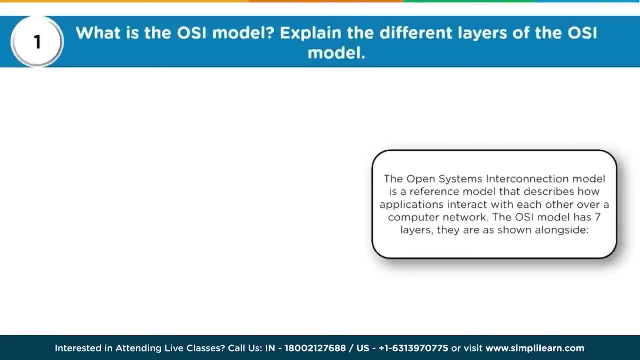 how data packets are created and how they are being processed by a computer. This is normally used by the TCP IP, the transmission control protocol over internet protocol software suite. So OSI is known as the open systems interconnection model. It is a reference model that describes how applications are going to interact via the 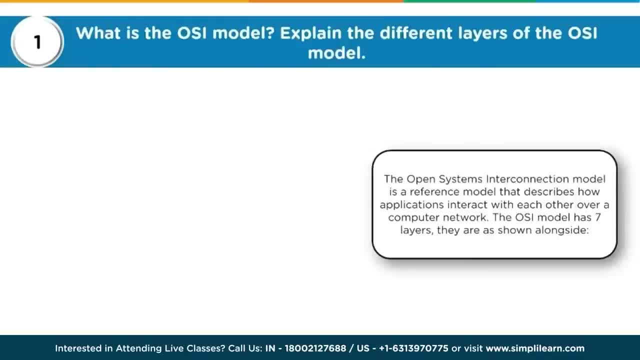 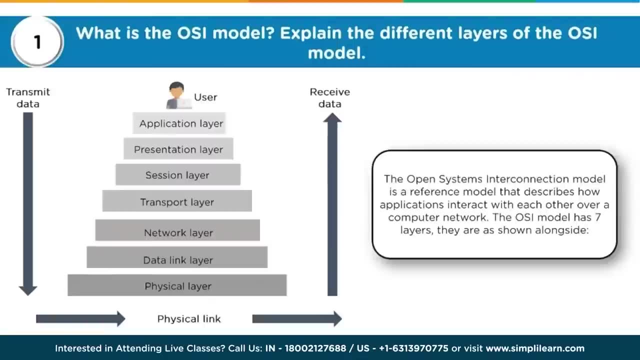 computer network. There are seven different layers that we need to understand. They are as follows. So in this diagram there are these seven different layers. We start off from the bottom. First is the physical layer, the data link layer, network layer, transport layer, session layer, presentation and application layer. 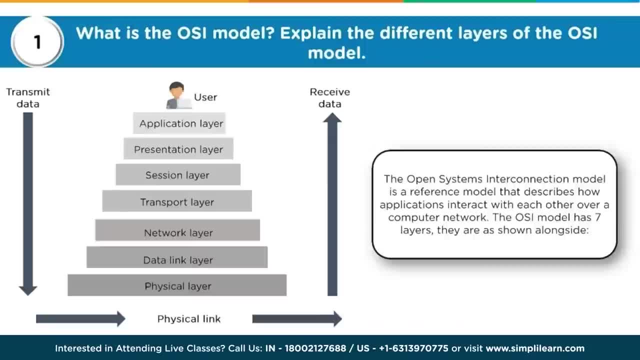 When such a question is asked in an interview, it is not only that we identify these seven layers, explaining what the OSI model is in the first place, We then try to identify these seven layers and we give a brief description about each and every layer. If there are any additional questions, they will come. 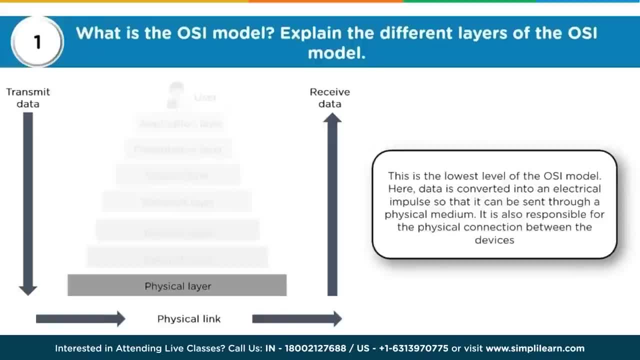 after this basic question. So let's start off with the physical layer. This is the lowest layer of the OSI model. Now, this is where any and every physicality of a computer comes into the picture. So it could be a network interface card. it. 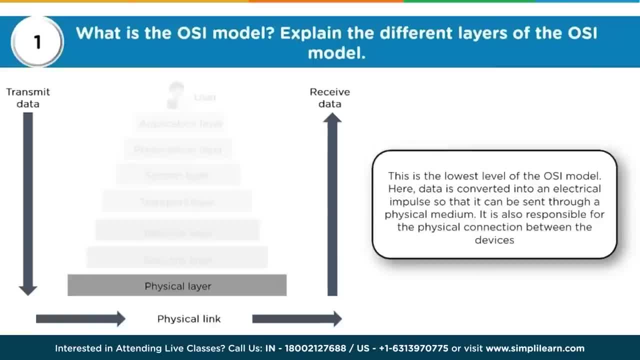 could be an RJ45 or a cat5 cable, Anything that allows data to be transmitted physically from your machine to another machine. Next comes the data link layer. So, on the data link layer, as far as networking is concerned, we just need to understand that data packet is encoded, decoded into bits, at this layer. 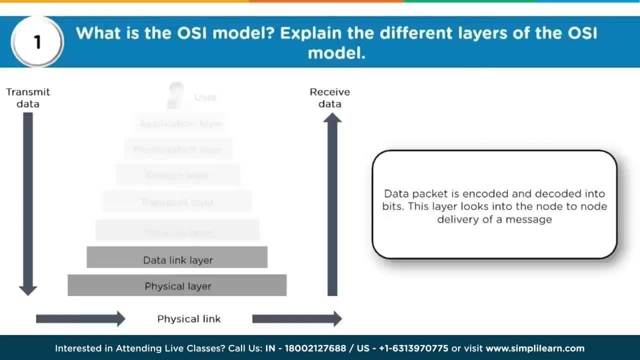 This is also the layer that deals with MAC addressing, So the physical address of every network interface card, Which is the MAC address which is utilized to route data packets over the network. This is where the MAC address resides on the data link layer. The next. 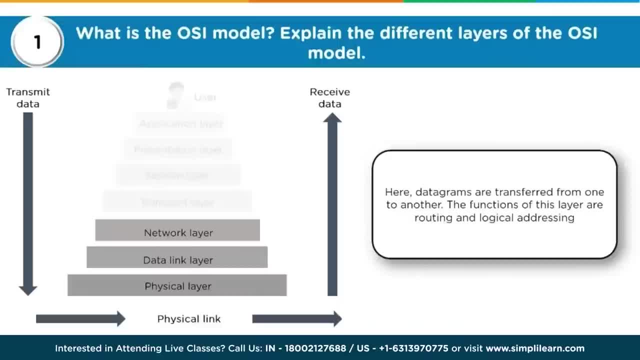 layer is the network layer. Here datagrams are transferred from one to another. The function of this layer are routing and logical addressing. The moment we talk about routing and logical addressing, IP addresses come into the picture: IP version 4, IP version 6.. So network layer will deal with IP. 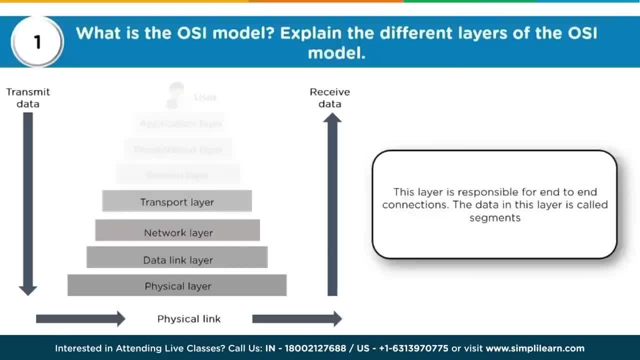 addressing and the routing of those packets. Then comes the transport layer. This is the layer responsible for end-to-end connections. That automatically signifies that this is where TCP and UDP will be working. TCP stands for transmission control protocol, UDP for user datagram protocol. TCP is a 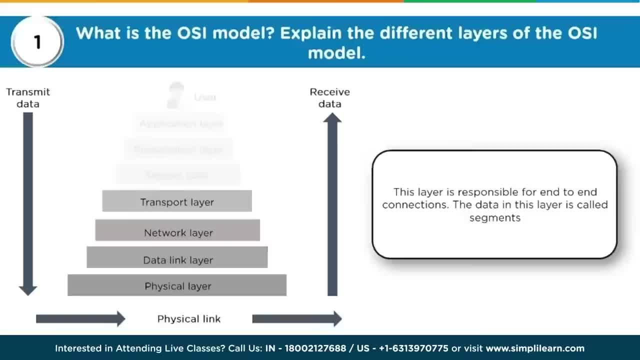 connection oriented protocol, Whereas UDP is a connection less protocol. These two protocols are utilized to establish connectivity between two machines. TCP is a more reliable method of connectivity Because there are a lot of packets that are sent across to verify that the data has been sent, Data has been received, and so on, so forth, Whereas UDP is a 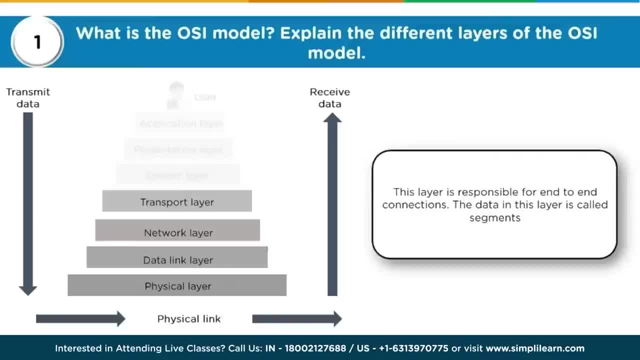 connection, less protocol where data is just dumped without verifying whether the receiver actually receives that data or not. So in a nutshell, on the transport layer, TCP and UDP make their appearance, and this is where that functionality lies. Then comes the session layer. This control signals between the computer. It 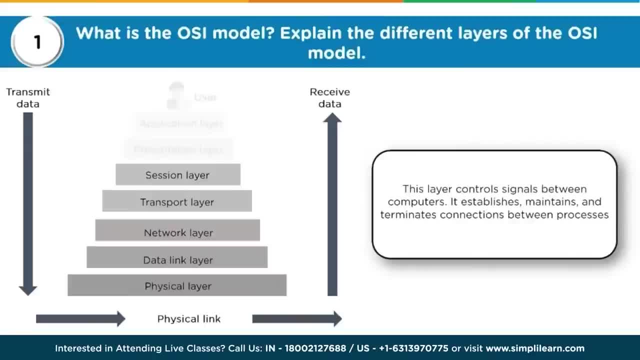 establish, maintain and terminates connections between processes. So in the transport layer, we talked about TCP and UDP. UDP being a connection less protocol where data is just transmitted without verifying whether the receiver received that data or not, Whereas TCP, we studied, is more of a reliable protocol. Thus there are different packets signals that will be. 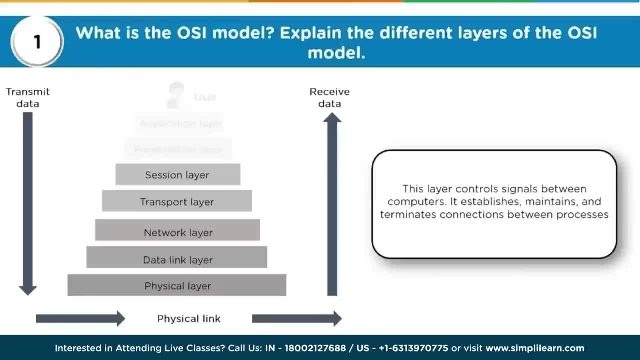 sent across to verify that data has been transmitted, It has been received properly, and then the next segment of that data is being sent. So those control signals are established using the session layer. So the three-way handshake of TCP, the acknowledgement packets and those kind of packets will be taken. 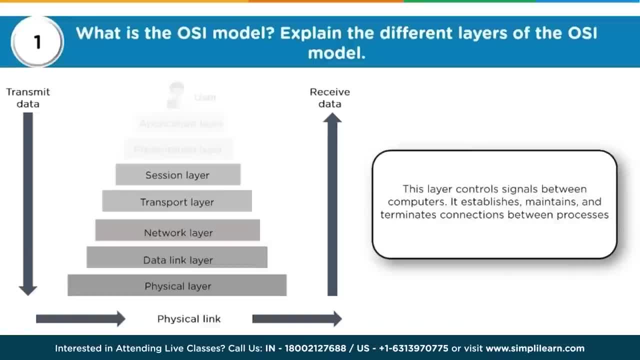 taken care of on the session layer of the OSI model. Then comes the presentation layer. The presentation layer is responsible to translate data into the application layer format. So the formatting right, MIME or encoding that is being utilized, The UTF-8 character set that we utilize for 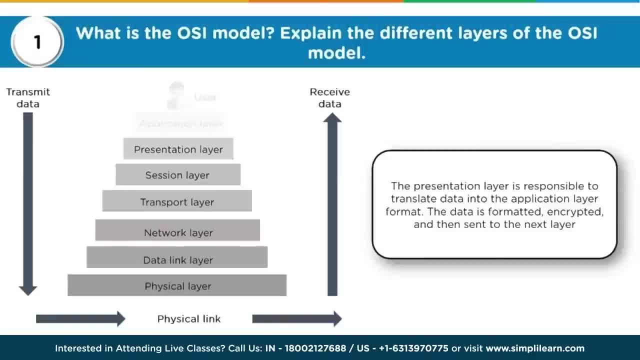 presentation Encryption mechanisms. All of these work on the presentation layer And finally comes the application layer, where the application itself uses a particular protocol so that the other machine on the receiving end, the application on that machine, will be able to understand what the communication was. 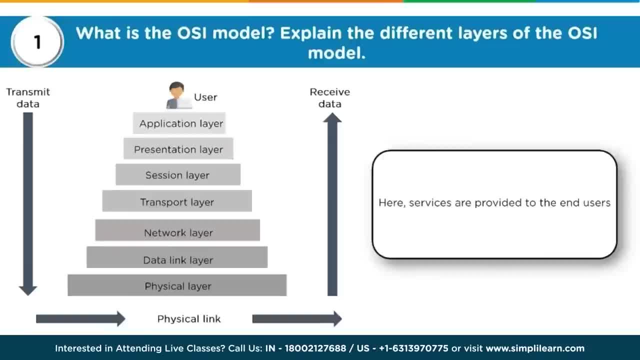 about right. So in a nutshell, if I start from up top, the application layer is generated, We will deal with any of the data that the application is generating. So maybe an user input. You're logging in, You're typing the username password. 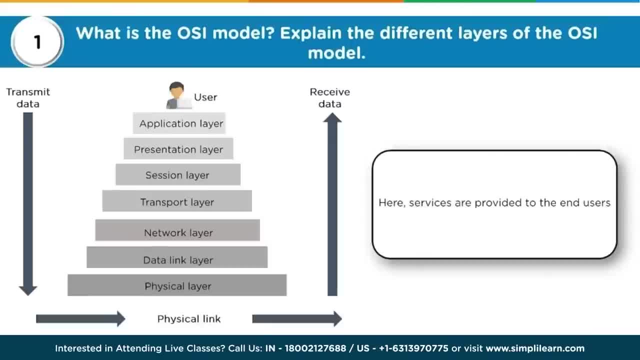 All that data will be constructed, let's say, into an HTTP or HTTPS format. That's where application layer comes into picture. Then the formatting of which into UTF-8 and the encryption of which would be done at the presentation layer. Then this transport layer and the session layer would kick in to establish a TCP session. Do the three-way handshake? Establish that connection? 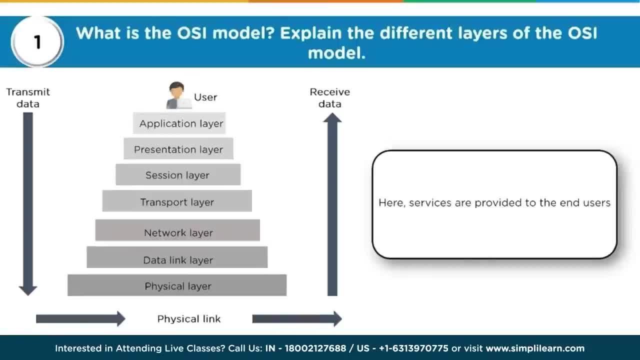 The IP addressing would be done on the network layer, MAC addressing would be done on the data link layer, And when everything is ready on the physical layer, the packet will be sent out At the receiving end. the packet will be received on the physical layer and then all these layers will be reversed And 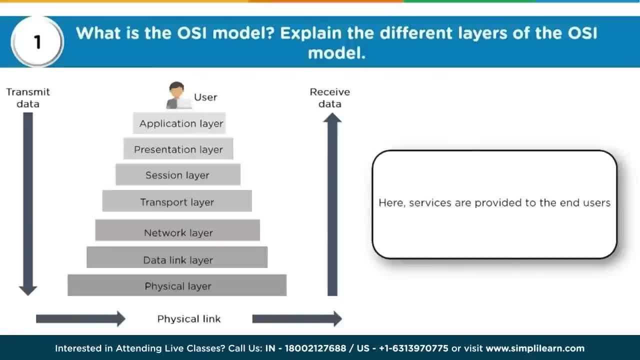 finally, at the application layer, the data will be presented to the application, who would then execute it and showcase it on the screen of the recipient. So this is the way you want to explain this question. You want to be very concise, precise About what you are explaining. You don't want to go into two hypothetical scenarios. 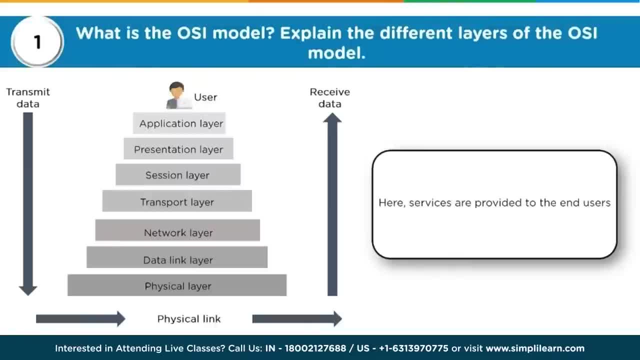 You don't want to delete a layer with the layers, You just want to give the basic functionality. You want to demonstrate that you understand what the OSI layer is, How the computer functions, and you want to move on from there. If the interviewer has any further follow-up questions, they will ask. 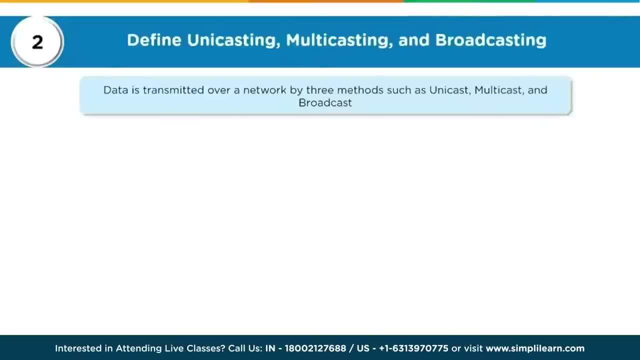 those specific questions. So that's question one. Moving on to the question two, Question two is: define unicasting, multicasting and broadcasting. This is a question which can be very lengthy but, again, most of your interview questions are designed that way. It's basically to understand how much, conceptually, you are aware about these technologies. 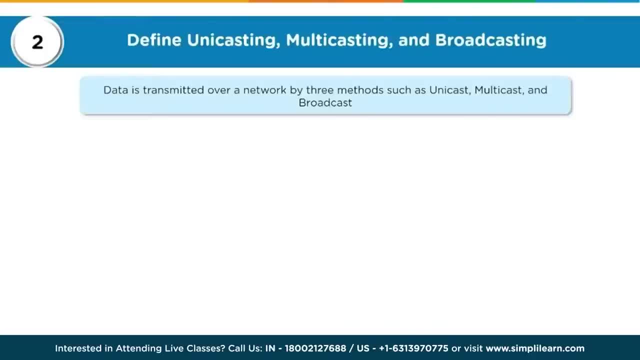 So you have to be very concise. Don't go rattling about technology too much, But in a concise manner just try to explain what these things is. So when data is being transmitted over a network, it can be transmitted either in one of these particular manners. It can either be a unicast, multicast or a. 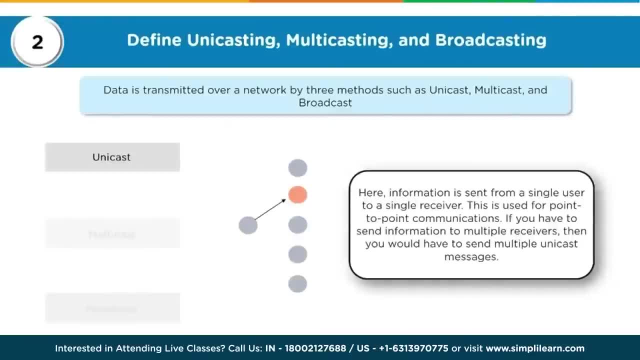 multicast. So what is unicast? Unicast is when a message is sent from a single user to a single receiver, So one to one, So one machine talking to another machine and nobody else, So also known as point-to-point communications, One point to one point If you have to send information to multiple. 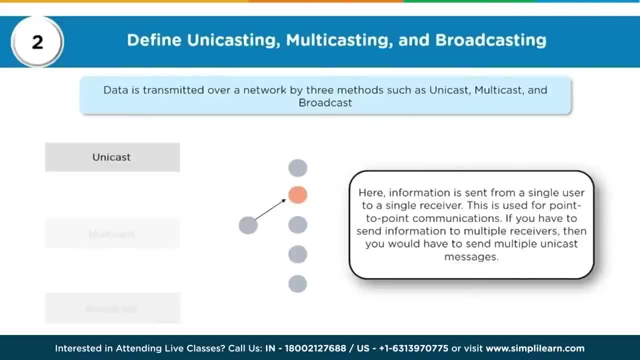 receivers, then you will have to send it using multicast. So this is where your multicast networking comes into picture. Let's assume it's a network where there are- there's a class C network- approximately 255 odd machines And within these there are two machines that want to talk to each other, If they want to talk between 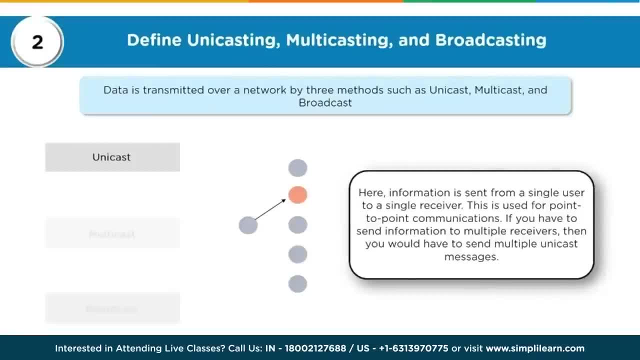 each other. it would be a point-to-point communication where they will utilize unicast, where only these two machines will have visibility of that conversation and the other machines will not even realize that this conversation is taking place If one machine wants to talk to multiple machines. 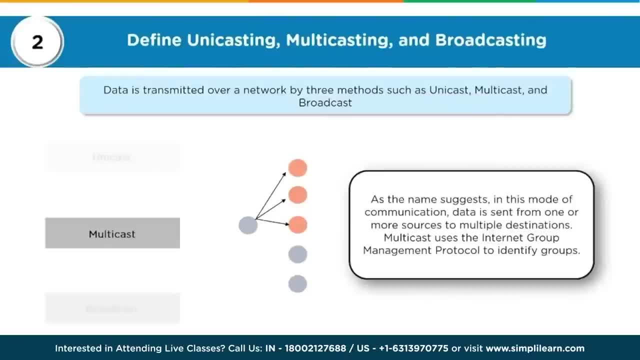 then the multicast comes into the picture, As the name suggests. in this mode of communication, data is sent from one or more or more sources to multiple destinations. Multicast uses the internet group management protocol, also known as the IGMP protocol, to identify groups. So under this IGMP protocol, 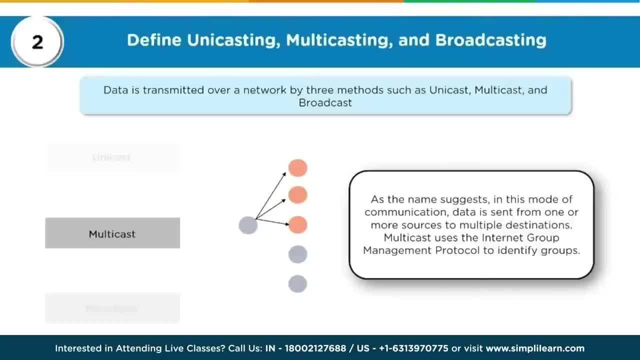 various groups are created, where machines are subscribed to those particular groups, and whenever a message needs to be sent through those groups, it will be identified by the IGMP protocol And then that particular message will be sent to those multiple machines that are members of those particular groups. And then comes the broadcast. The third method is known as the broadcast, as it 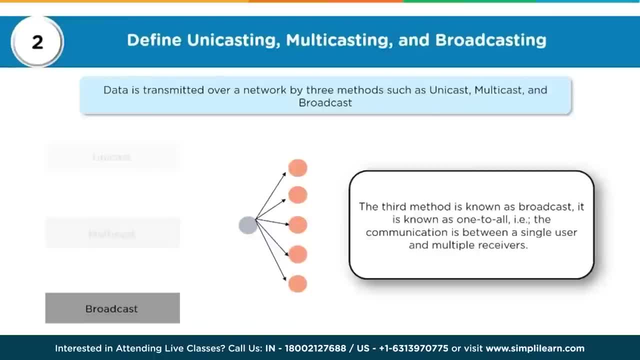 says it is going to broadcast to all. So this is one to all. that is communication between a single user and it is going to be sent to all the machines in that particular network. So the three ways, unicast is one to one, multicast is one to many. 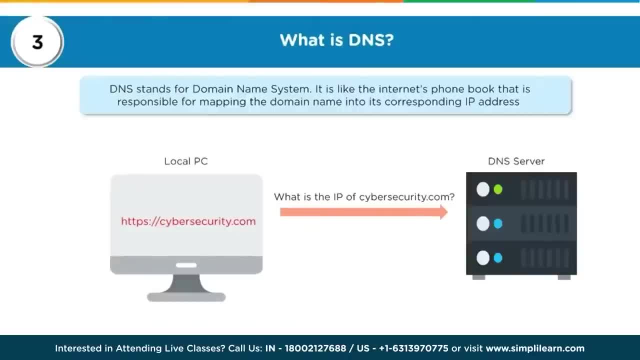 And broadcast is one to all. Then question number three: What is DNS? DNS stands for domain name system. It is like the internet's phone book that is responsible for mapping the domain name into its corresponding IP address. And let me give you an example over here. Whenever we go and open up, let's say a: 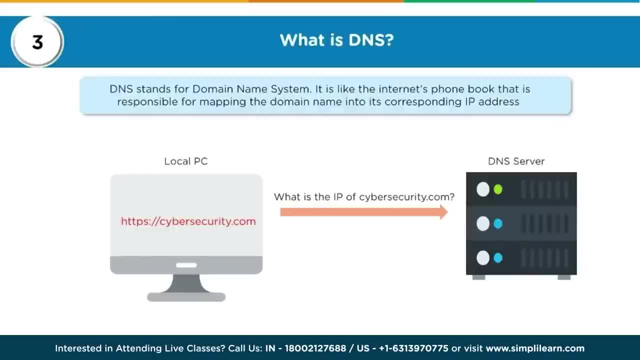 browser, a Google Chrome browser, we type in wwwgooglecom and then we press enter and magically Google comes in front of us, the website rather. Now how does the computer know who Google is? Because, as far as we are concerned, humans understand Google and words like that. Computers don't. Computers deal with binary zeros and ones. 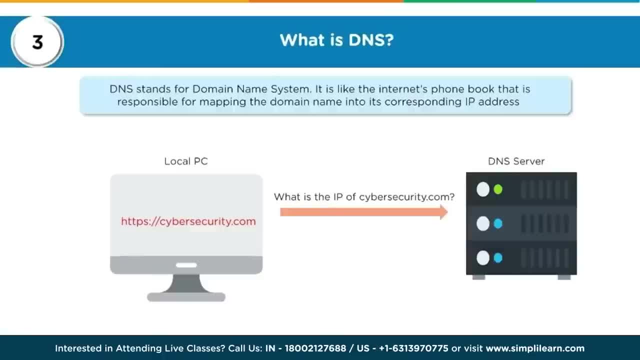 Right. and as far as internet is concerned, they will only deal with IP addresses and Mac addresses. So how does a computer know how to find googlecom and where is it located? So the moment we type in in the browser window in the address bar, googlecom and press enter, 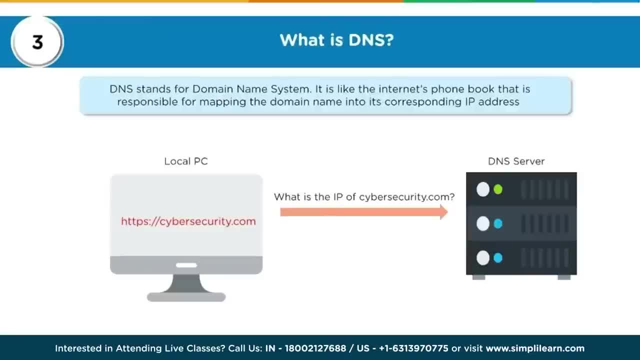 A DNS query is generated automatically by the browser where a packet is sent to our DNS servers asking what the IP address is. So, in short, DNS resolves domain names to their corresponding IP addresses. There is a DNS server which will have this index, A database of all the domains associated. 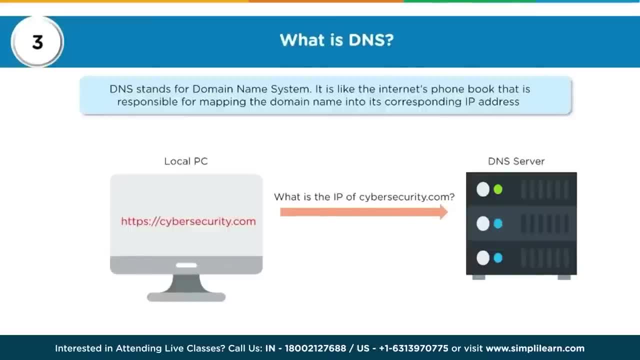 with their IP addresses. If one particular DNS server does not have that information that you're looking for, it may query another DNS server Who may have that particular response. So the first thing is when you type in domain name, it gets resolved with the DNS. It identifies the IP address corresponding to that particular domain. 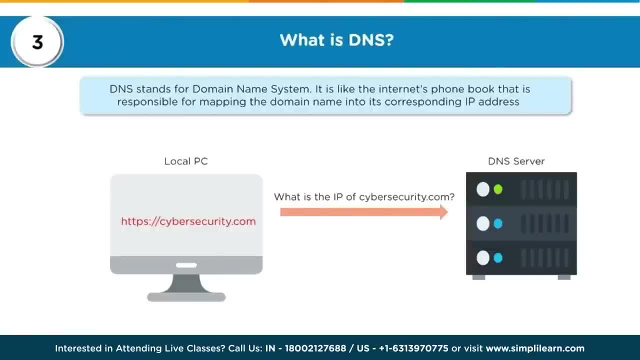 name and thus allows the computer to route that packet to the particular server where that domain name resides. So in this scenario, if you look at the screen on the local PC you have typed in cybersecuritycom, There's a DNS resolution. that a query that goes to the DNS server. What is the? 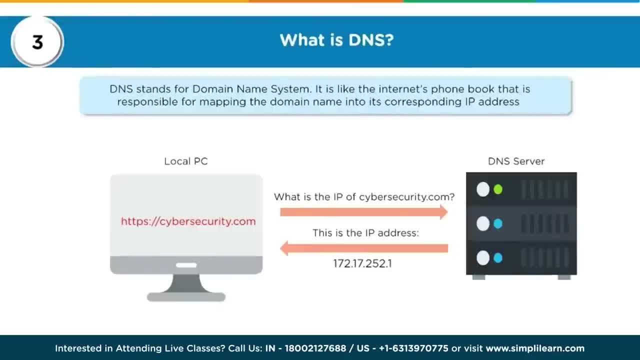 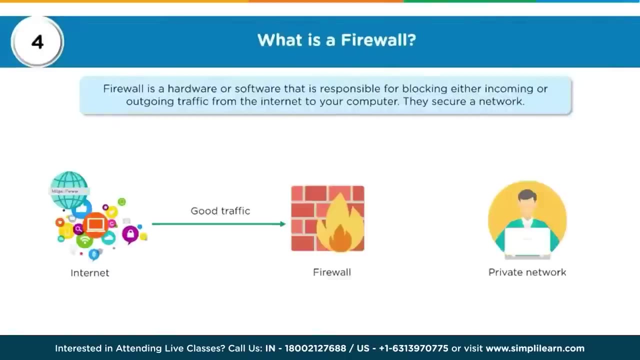 IP of cybersecuritycom, The DNS server looks it up in its particular database. If it has the corresponding IP address, it will then respond back. The IP address is 172.17.252.1, after which the packet is sent off to cybersecuritycom. Moving on to the question number four, What is a firewall? 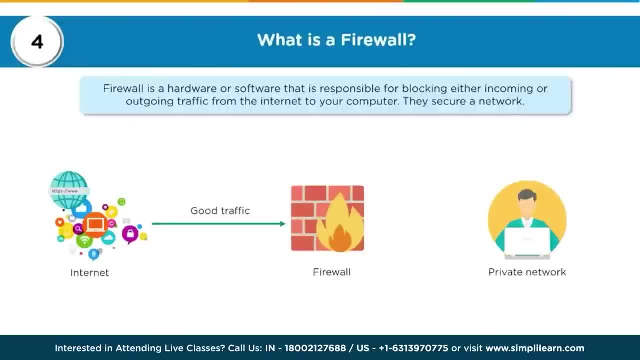 Now, this is a very good question and normally a very basic answer that I've ever heard is that a firewall is a hardware and a software firewall. But that's the functionality of a firewall. That is what- how you can install a firewall, But there are different types of. 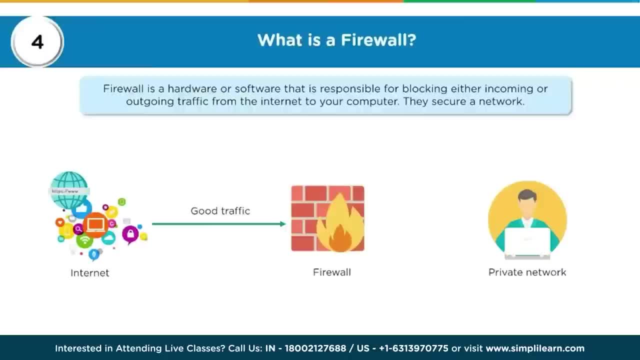 firewalls and there is a specific functionality that a firewall is created for right. So a firewall is either a hardware or software, but its responsibility is for blocking either incoming or outgoing traffic from the internet to your computer. They secure a network. So essentially the 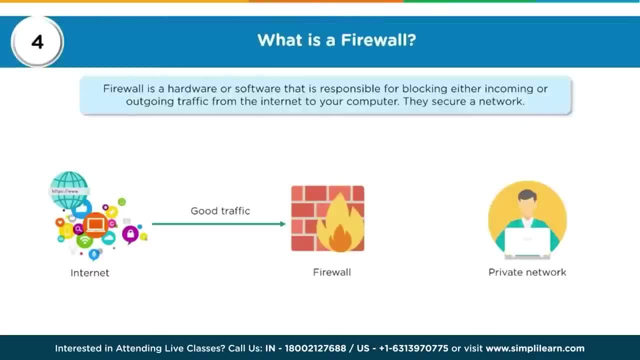 firewall will allow a connection to happen or disallow a connection to happen. It won't go beyond that. That's the basic functionality. Okay, so based on the configurations that you have done, based on the rules that you have created on the firewall, it will then, based on those rules, identify whether some traffic is allowed in that. 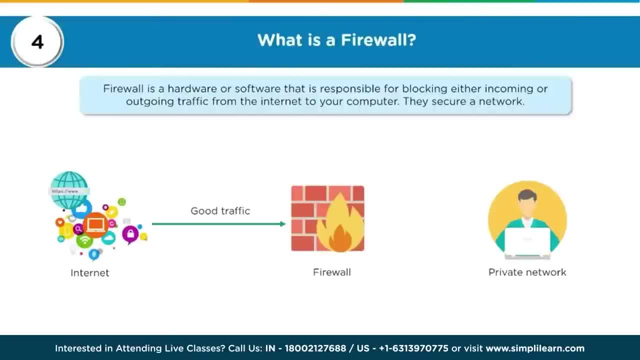 network or some traffic is to be blocked from entering that network. So, as the screen shows, the firewall rules will analyze whether the traffic is good. If yes, it will allow. If the traffic is bad, it will block the traffic and not allow that connection from happening in the first. 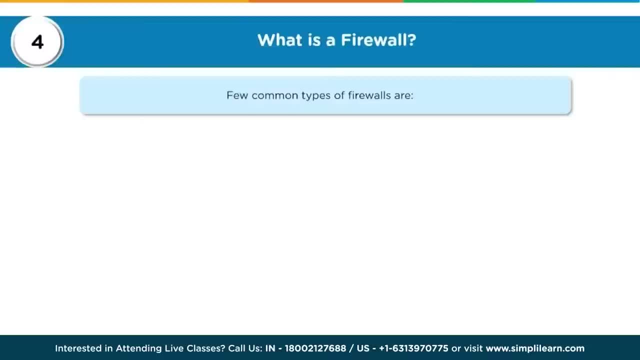 place Now, there are few common types of firewalls that also need to be included in the answer to this question, and the first one is a packet filtering firewall. These are the most common types that you will come across, which analyze packets and let them pass through only if they. 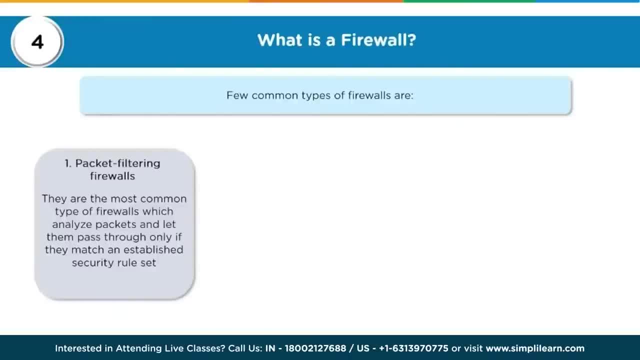 match an established security rule set Now here. people do get confused. when we say that we analyze packets, People think that these firewalls will analyze the contents of that packet, which is not correct. When the definition for a packet filtering firewall says that these firewalls analyze packets, it means that they are only analyzing the source and destination IP. 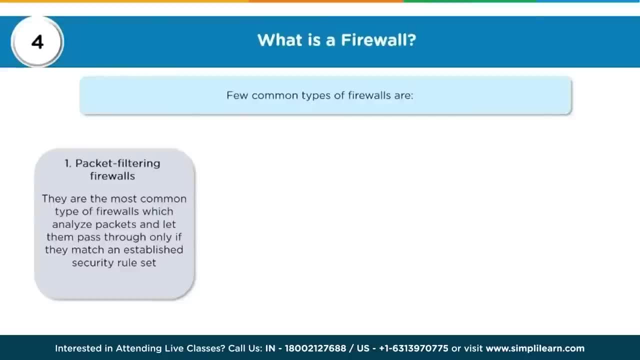 addresses, port numbers and the protocols that are mentioned in those packets. These firewalls do not have the capability of deep packet inspection, or DPI as it is known. If that capability comes into the picture, you are basically looking at an intrusion detection system or intrusion prevention. 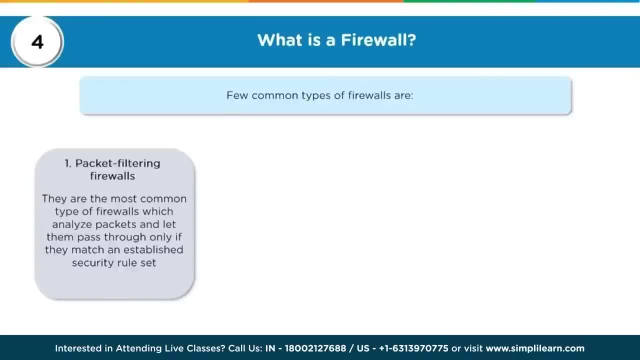 system in today's world called as a next-gen firewall, So a packet filtering firewall essentially will only analyze data packets for its source and destination, IP addresses, port numbers and the protocol that is being utilized. It will then map that information to the rules that are. 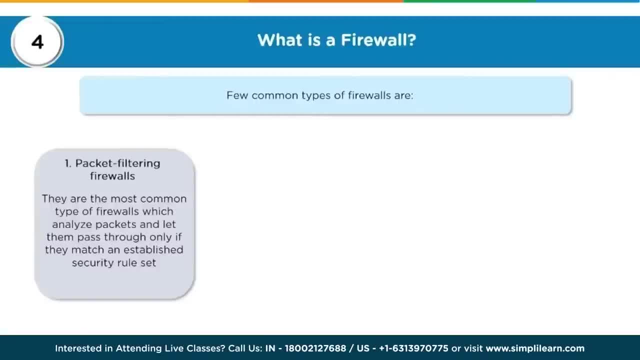 there on the firewall and based on those rules, it will either allow that connection to happen or disallow that connection from happening. The second type is a proxy firewall. These firewalls filter network traffic at the application level. So when you say application level they work at. 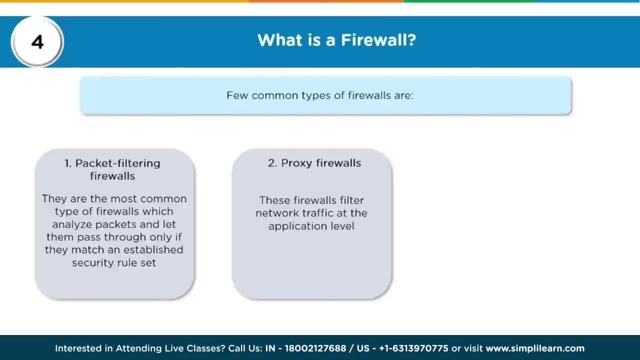 the layer 7 of the OSRF Packet. filtering firewalls- since we have mentioned that they've worked on IP addressing and port numbers- will work on the network layer of the OSI model, Also on the transport layer, because you also look at protocols. Proxy firewalls will work at layer 7, which is the application layer of. 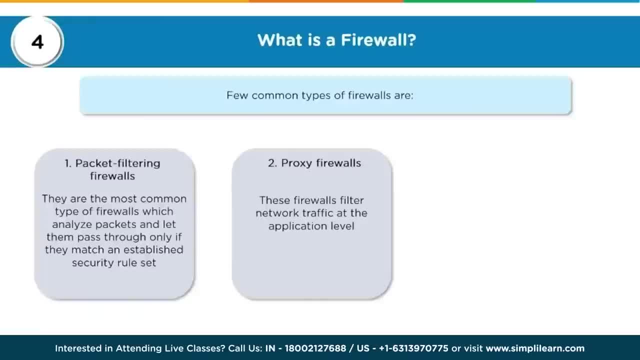 the OSI model and will deal with application level protocols such as HTTP, HTTPS, FTP, SMTP and so on, so forth. And the third one is a stateful multi-layer app inspection firewall. These filter packets at the network, transport and application layers, So they basically do the job. 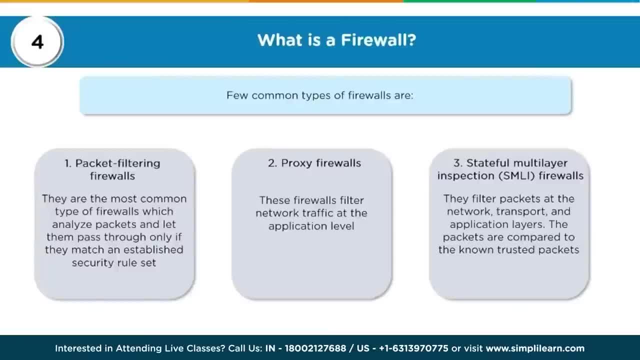 of the first and the second type of firewalls. The packets are compared to known trusted packets. but now the first question is: if there is a stateful multi-layer inspection firewall, why do we have type 1 and type 2 firewalls like packet filtering and proxy firewalls? That is because that is how. 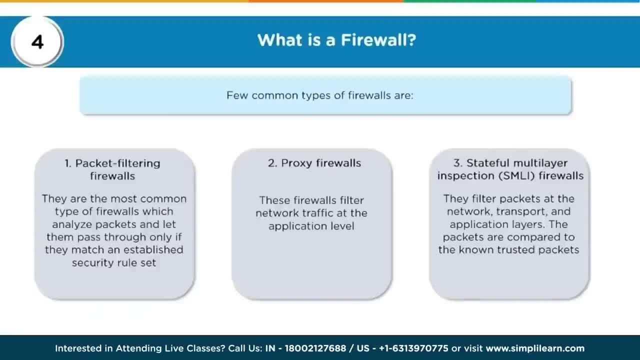 the firewalls have evolved. We started off with a packet filtering, then we added functionality to it. if a question comes, what is a firewall, you start off with the option saying it is a hardware or software. This is the responsibility. the functionality of a firewall is to allow good 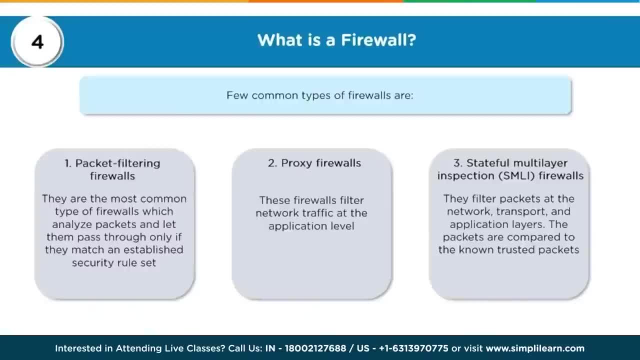 traffic and disallow bad traffic based on the rules that have been configured on the firewall. and then you've got basically three types of firewalls- packet filtering, proxy and stateful multi-layer- and just include a brief description of each of these firewalls. If getting your 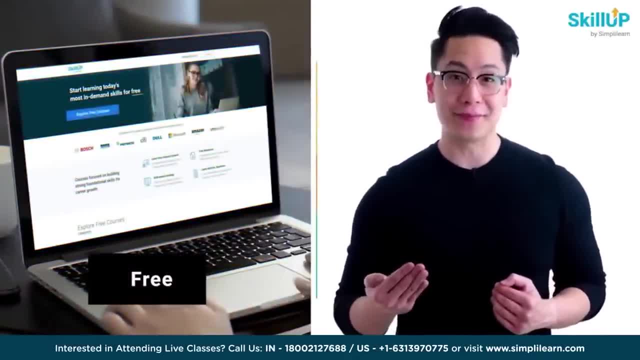 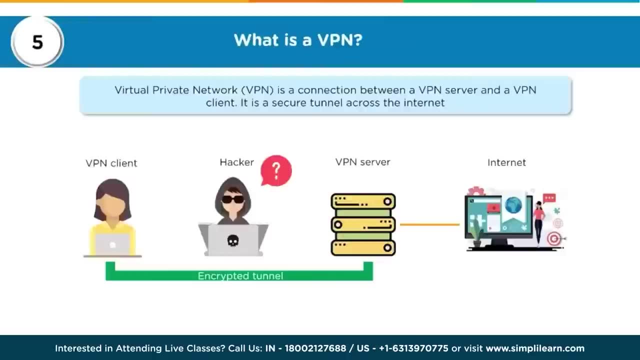 learning started is half the battle. what if you could do that for free? Then, moving on to question number five: what is a VPN? VPN is also called a virtual private network. It is a connection between a VPN server and a VPN client, So it basically creates an 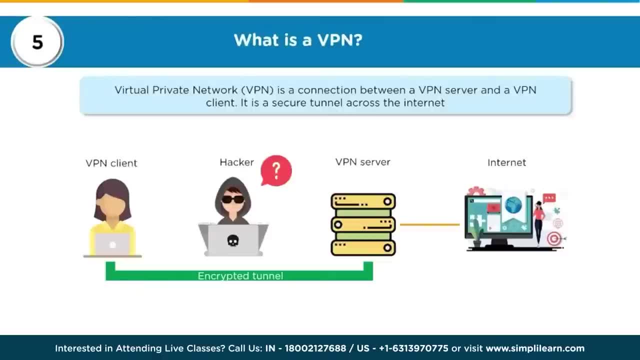 encrypted tunnel between the client and the VPN server, which is then utilized to secure the connections that you are making with the internet. So, as you can see in the diagram, the user has a VPN client installed on the machine. the VPN client then creates an encrypted tunnel to the VPN server and, through this tunnel, encrypted data is transmitted, which can then be. 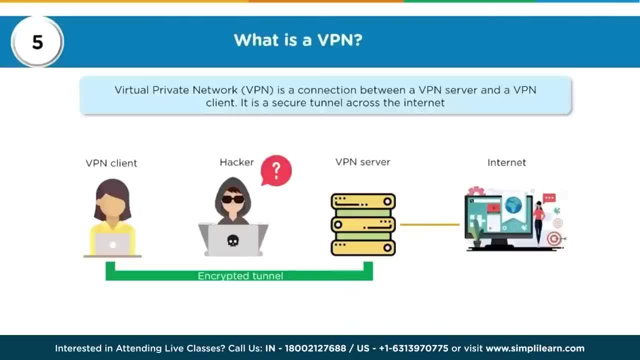 processed by the VPN server sent to the internet. information can receive can be received back by the VPN server. The VPN server will encrypt that data back and send it back to the user. So if there's a man in the middle attack that is happening or a hacker trying to eavesdrop on the 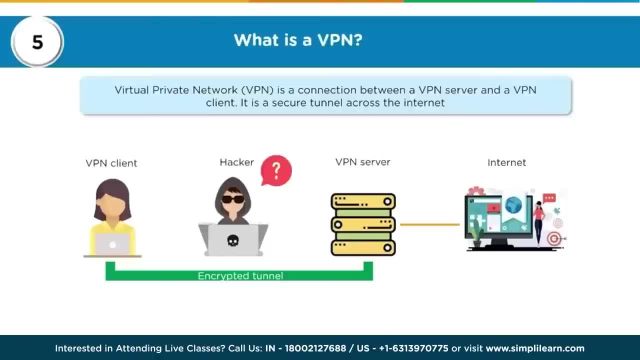 communication mechanism. It will not be able to do so because of the encrypted tunnel. It is very difficult to decrypt this or hack through this encrypted tunnel. It is possible, but it is very difficult to achieve that. Moving on to question number six, what are the advantages of distributed processing? 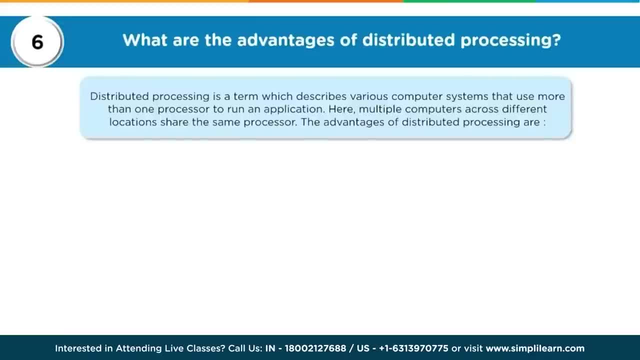 Now, before we go into advantages of distributed processing, we first have to understand what is distributed processing. So it is a term which describes various computer systems that use more than one processor to run an application. Here all the computers across different locations share the same processor. The advantages of 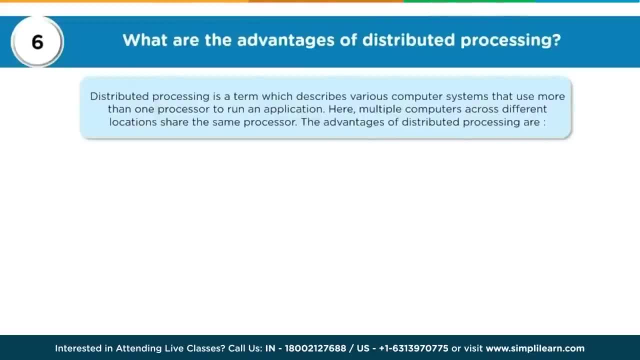 distributing processes are as follows. But before we go into the advantages, distributed computing is basically where multiple machines will pool their resources together to run a singular application, So an application that has multiple resources and can scale up and scale down as and when required. The advantages are that it can be very, very useful in data recovery, For example RAID. 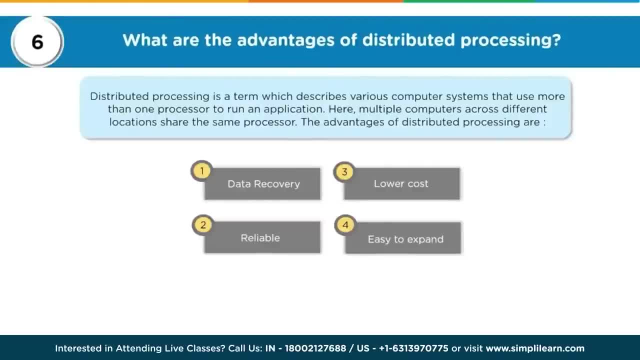 where it is very rapidly aroma your scraping data on various hard disks. It is reliable, it is cheaper, lower cost can be achieved And it is easy to expand. because of the scalability factor that we just talked about. If there is loss of data in one computer, it can then be recovered by another. 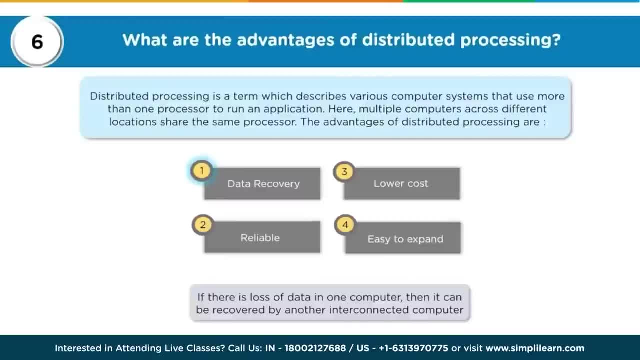 interconnected computer And one of the examples would be block chain. in today's world Right, What is backstage? This data is created live and stored on a connection of computer, So if one of the computers goes offline in that network will still have that data and the blockchain will still. 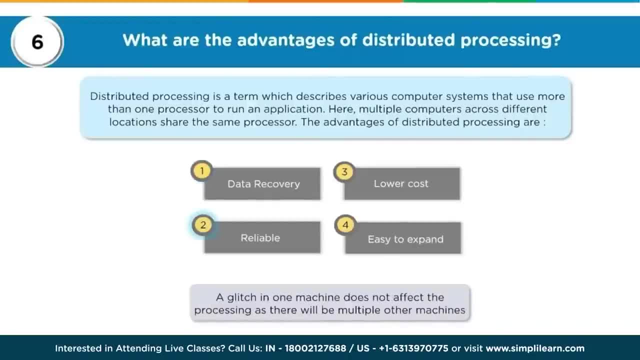 function without any issues. The second point: a glitch in one machine does not affect the processing, as there will be multiple other machines. like we discussed in the blockchain, Several cost-effective mini computers are used instead of costly or mainframe machines. So instead of having a server bank, I can. 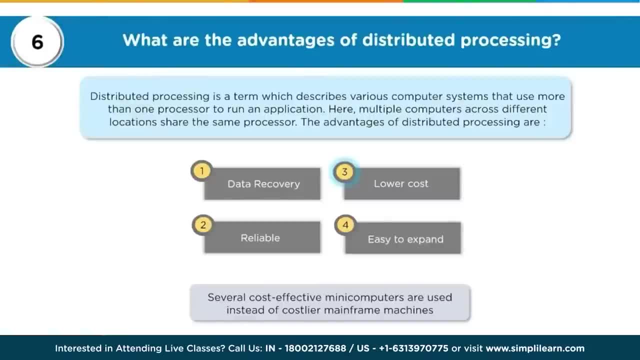 have multiple machines interconnected together and they can function in that particular blockchain or for that particular distributed processing mechanism. Depending on the amount of data processing, more computers can be attached to the network. Thus, you can increase the number of computers that can be a part of that blockchain or you can reduce them as and when. 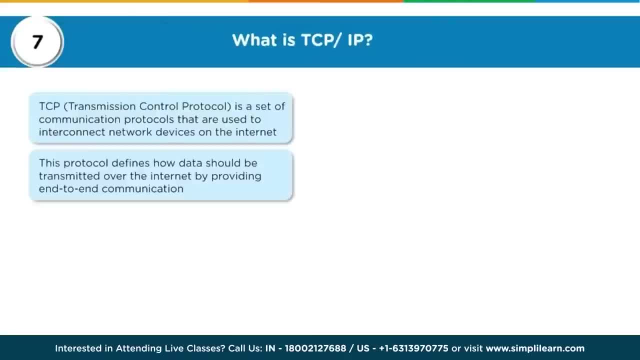 necessary. Moving on to question number seven, what is TCP IP? TCP, IP or transmission control protocol over internet protocol is a set of communication protocols that are used to interconnect networking devices on the internet. This protocol defines how data should be transmitted over the internet. This protocol defines how data should be. 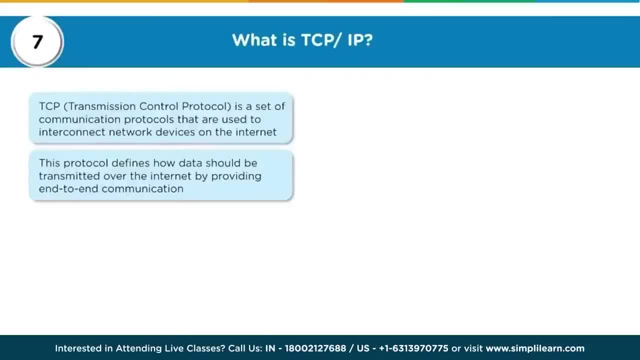 transmitted over the internet by providing end-to-end communications. So, essentially, if you want networking to be established on your machine, you will need TCP IP. Without TCP IP, there will be no work groups, there will be no domains. basically, your interconnectivity will go for a toss. TCP IP is a software. 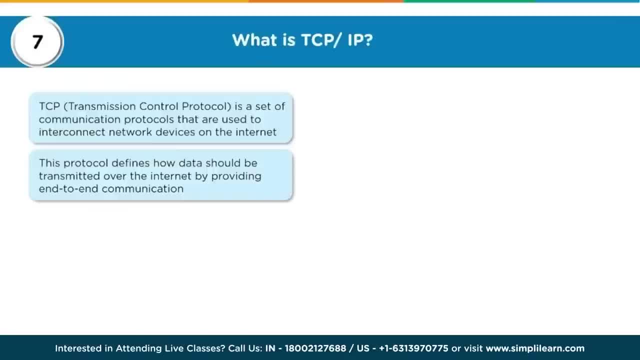 that, once installed on your machine, will then interact with the hardware, which is your network interface cards, and then your switches, wires, cables, and all those through protocols that have been already pre-configured in it. So within the TCP IP suite of software you will have all the protocols, all the 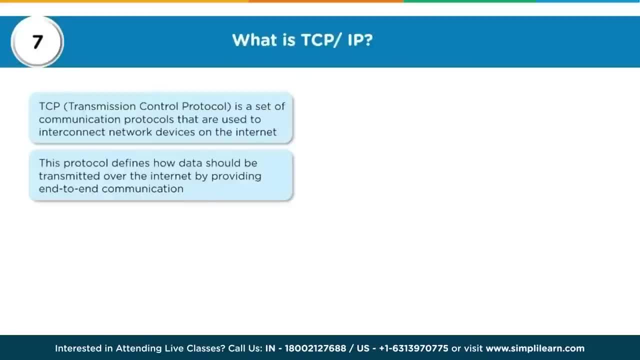 functionality of the OSI layer, and each and every protocol that works on each and every layer will be predefined and pre-configured to work in a particular manner. The Internet Protocol is all about routing each individual packet to make sure it reaches its destination. So with the TCP IP we are talking about the. 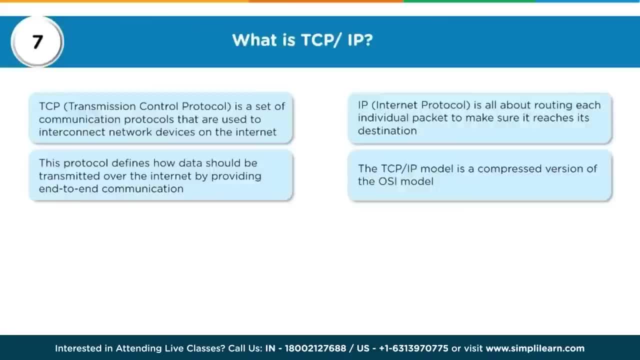 protocols that will allow you to format the data and generate it so that you can communicate it over the network. The TCP IP will then interconnect it, So the network IP. we will then convert it into a now net ip connection. IP will then deal with the routing of those packets so that the packet can be. 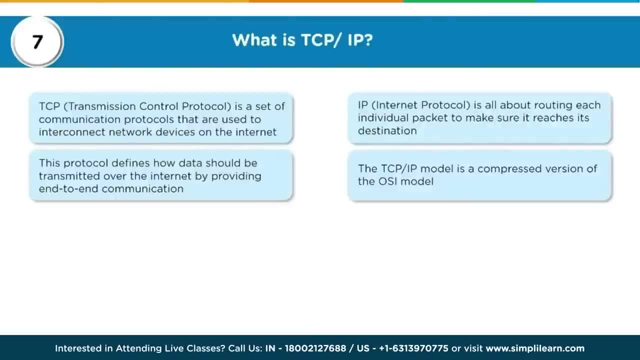 routed to the correct computer and be received by the recipient. So the TCP IP model is the compressed version of the OSI model. The seven layers will get converted into four layers: the network access layer, internet layer, transport layer and application layer. Going on to question 8, what do you mean by IP? 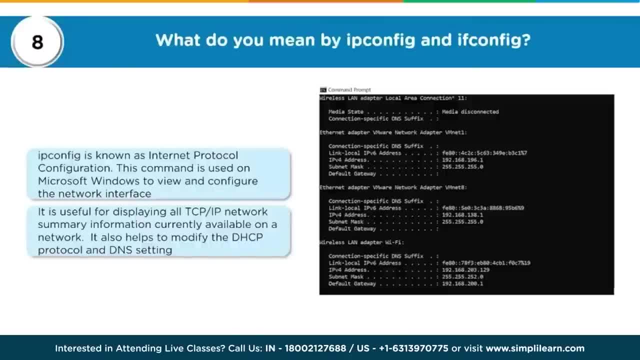 config and IF config. Both of these are commands, the first one on a Windows machine, the second one on a Linux machine. So IP config is known as the Internet Protocol Configuration. This is a command that is used on the command line interface of Microsoft Windows to view all the adapters and the 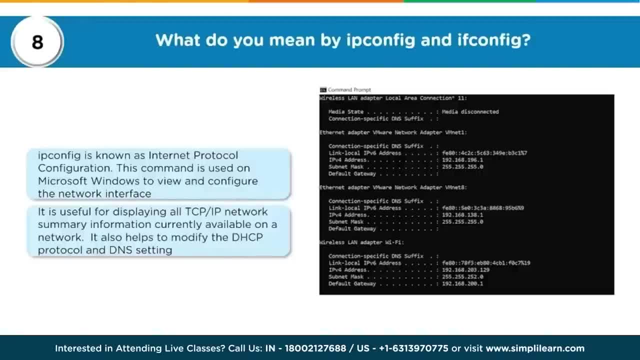 configuration of each and every adapters for their network interfaces. So, as you can see on the right hand side in the command prompt screen, if once you type in the IP config command on the C prompt and press enter, it will give you a list of all the adapters that are there, So you can see Wireless LAN adapter. 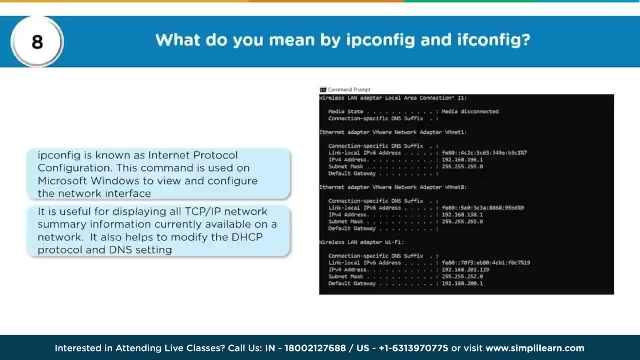 IP local area connection. the media is disconnected. it doesn't exist. at the bottom you'll see the wi-fi connection wireless LAN adapter and can give you the IP version 6 IP address, IP version 4 address, the subnet mask and the default gateway. so this is the configuration that allows the 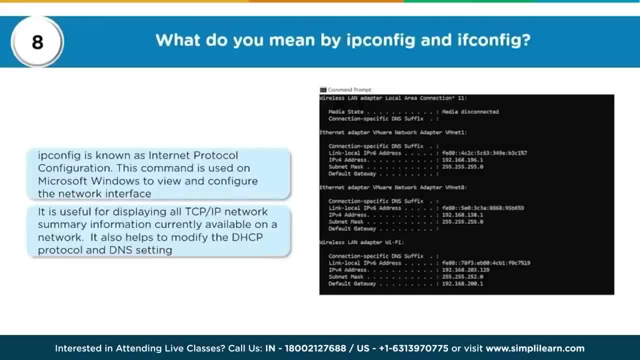 machine to know on what network it is, on, what is the default gateway for communicating to the internet, what is the subnet mask, so how many computers may exist in that particular network, and what is the IP address of that specific computer, so that it can communicate across the. 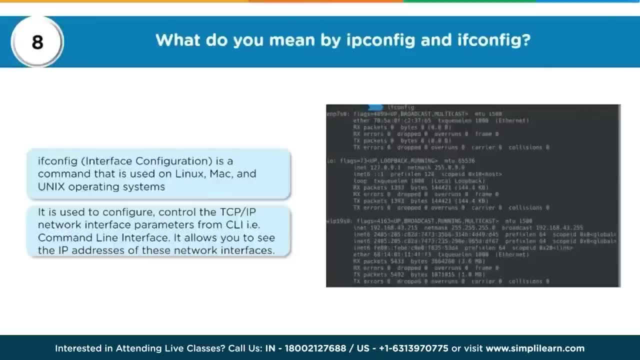 network as well. ifconfig is the same thing on the Linux, Mac or Unix operating system. so the command will also give you the list of interfaces and the configuration of each and every interface. it is used to configure, control the TCP IP network interface parameters from the command line. 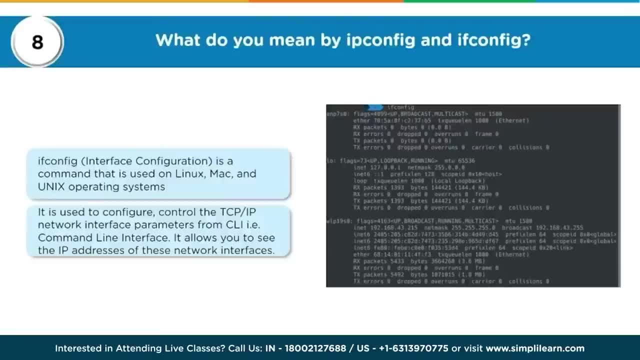 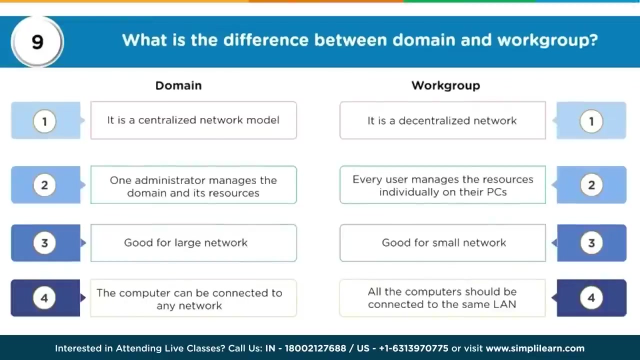 interface. it allows you to see the IP address of these network interfaces. so here you can see the WLP 19 S, the IP address being 192.168.43.215, subnet mask being 255.255.255.0, with the broadcast being 192.168.43.255. question 9: what is the difference between a domain and a? 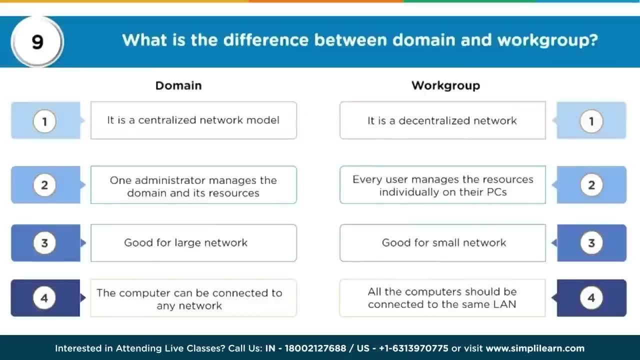 work group? this can be a very interesting question and can be a very lengthy question at the same time. a work group is nothing but a decentralized network where you have interconnected multiple machines together and each machine acts in its own individual capacity, things of itself, as a server. 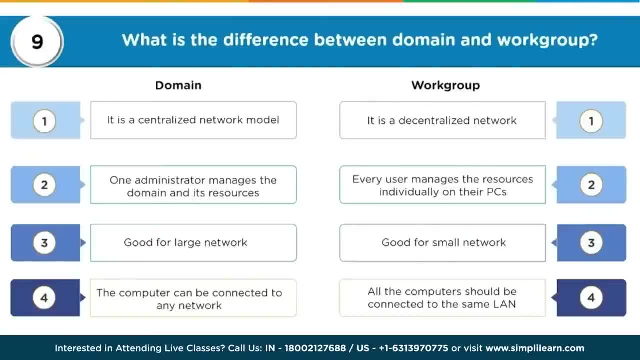 right. so a decentralized network. you, every user, manages the resources individually on their pc. so local users on their own pcs, managing the network, shares what can be shared from that particular machine, what data should be shared, should not be shared, to whom it can be shared with, and so on, so forth. it is good if you've got a small network, a few machines altogether. 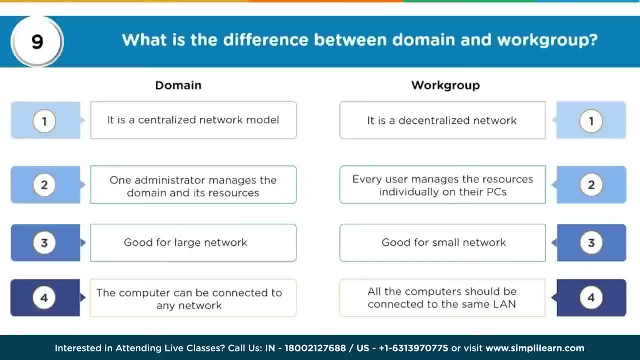 and you want them to interact with minimal management effort. right, so each computer, each user will decide what they want to allow other users to see on that particular network, and all of them would be connected over a LAN, a local area network, either a wireless or a wired one. 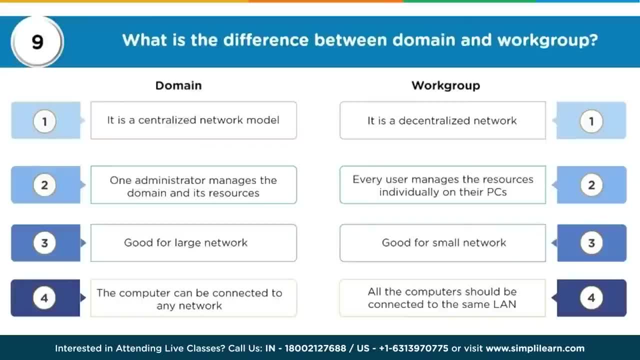 so if you look at your home wi-fi right now, that is one of the best examples of having a work group. the domain, on the other hand, is a centralized network model. so in a corporate environment, whenever you go there and you've got a domain based user. 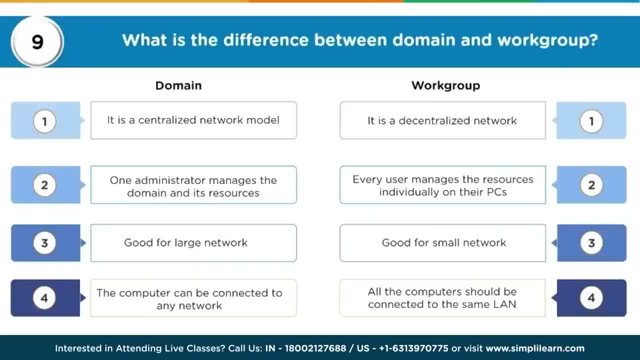 name and password which, when entered onto a particular machine, gives you access to the entire network or whatever applications and whatever resources have been allocated to you. that is where the domain comes in, so it it also uses a single sign on mechanism for all the resources that are that are to be made available to you, whereas in a work group your local user. 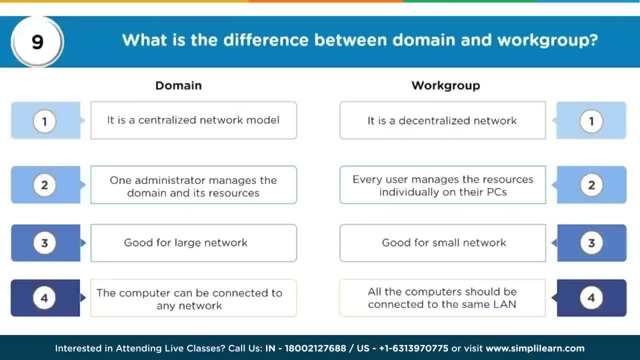 only meant for that particular computer, right? so, coming back to the domain, it is an administrator who is going to manage the entire domain and all of the resources connected to it, to the domain. the resources could be switches, routers, servers, data stores, applications, web servers, mail exchange servers and so on, so forth. so all of these are administered by an administrator. 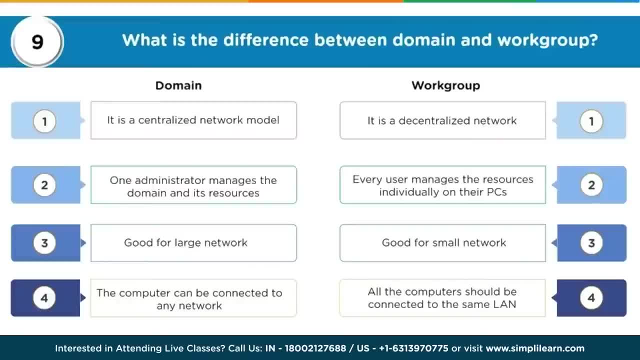 through the domain. it is the most reliable and optimum solution for a large network where multiple users are going to interconnect and share that data amongst each other. right, the computer can be connected to any network. that means you can be on the internet and through the internet using a VPN. you can be connected to any network. you can be on the internet and through. 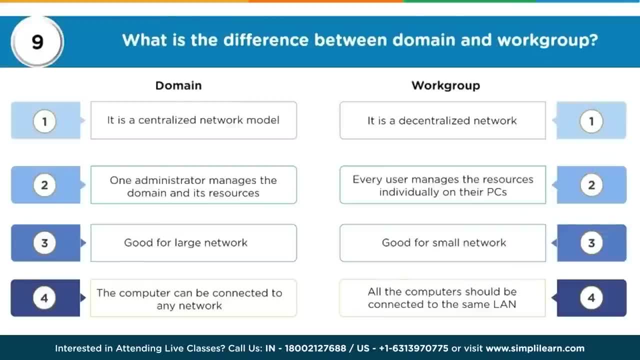 can connect to your corporate network, authenticate in and get access to whatever resources you are allowed to access, Whereas in a work group you have to be a part of that network to access that particular network. If you change your location, you go and connect to another Wi-Fi, you will lose. 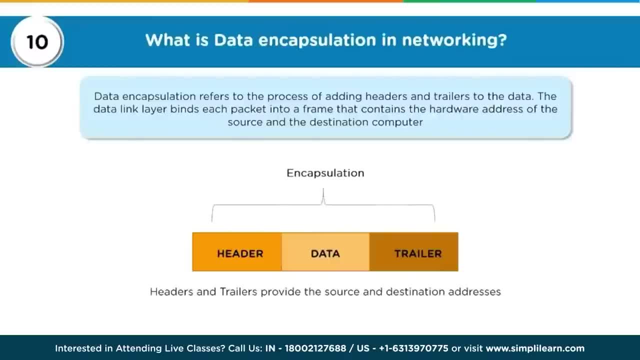 access to your previous Wi-Fi. Then the last question for the networking section: what is data encapsulation? in networking, Data encapsulation refers to the process of adding headers and trailers to the data. The data link layer binds each packet into a frame that contains the. 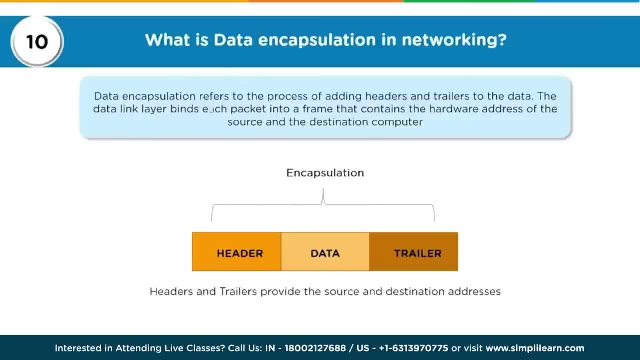 hardware address of the source and the destination computer. So in this example, when you're talking about data encapsulation, we have talked about how data that has been created by the application layer would have a header and a trailer that will give the various informations of where that data 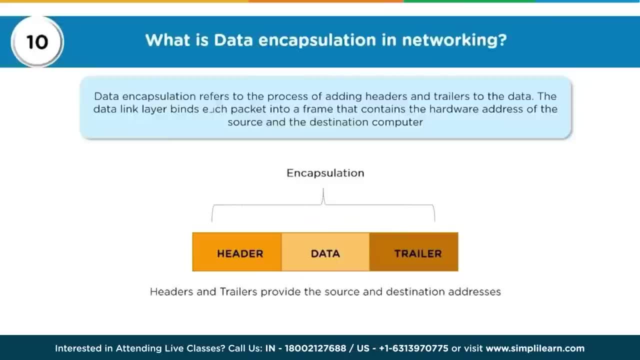 needs to be sent. So the hardware address, which is the MAC address, comes into the picture and it's added to the header. and the IP addresses, port numbers and all of those things would then be added to this trailer as well, so that the data can be then. 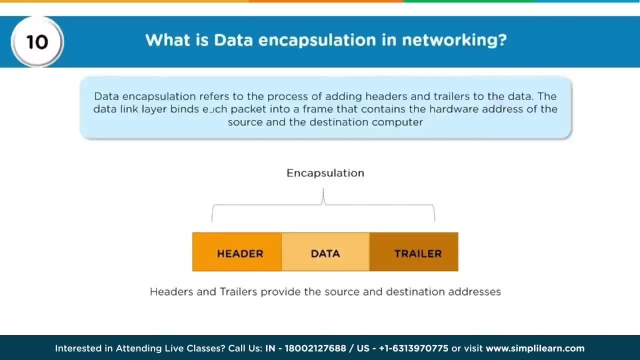 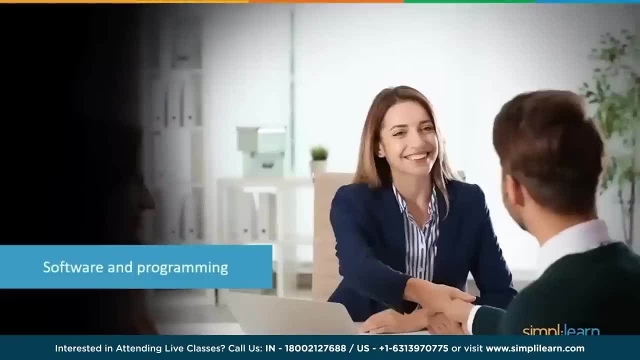 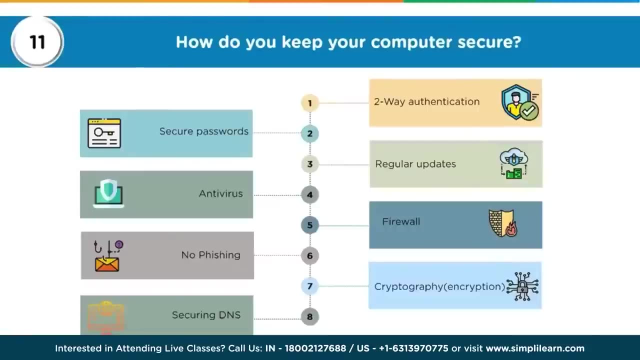 routed to the intended recipient of that particular communication. With this we end the first 10 questions in networking and in this video we are going to look at software and programming. So we're going to look at the first 10 questions, First question being: how do you keep a computer secure? 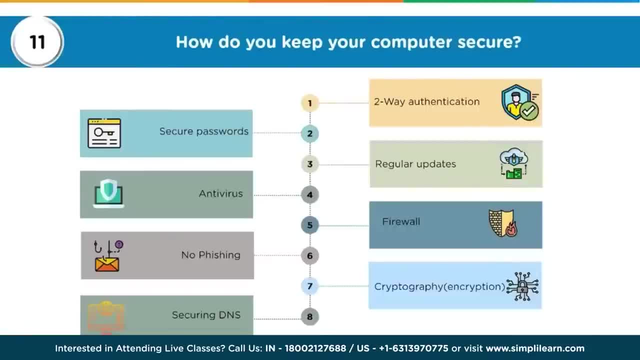 Now, this is going to be a very generic question. So you want to put your best foot forward. you want to put your best foot forward and you want to put your best foot forward, so you want to forward and you want to identify the most common methodologies on how you can keep a computer. 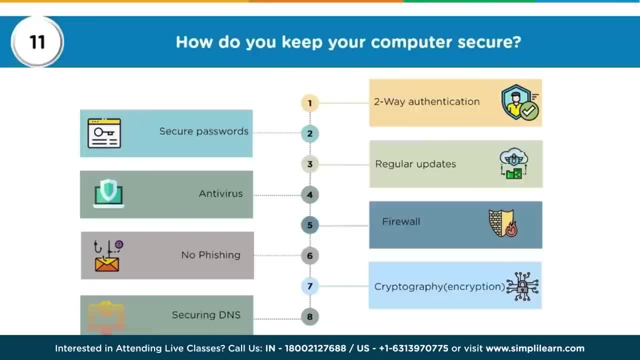 secure. So, when you talk about computers, the first thing that you want to talk about is authentication mechanisms, where you want multi-factor authentication or two-way authentication to ensure that your accounts are kept secure. Now, if you look at using passwords- depending on how, 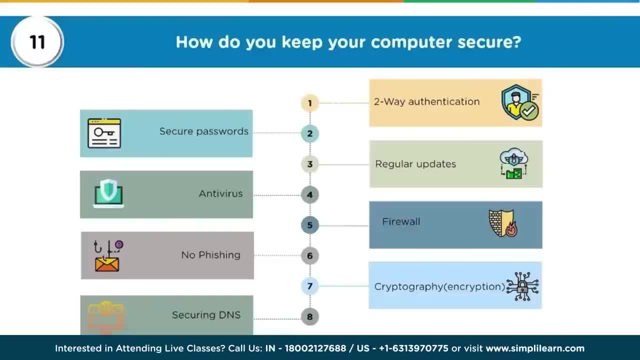 passwords are being stored by the application. password attacks can be possible: either a brute force attack or a dictionary based attack, or even password guessing attacks are possible. To mitigate those kind of attacks, we need multi-factor authentication to ensure that accounts are secure. Now, even if we are using multi-factor authentication, we also want to look at secure. 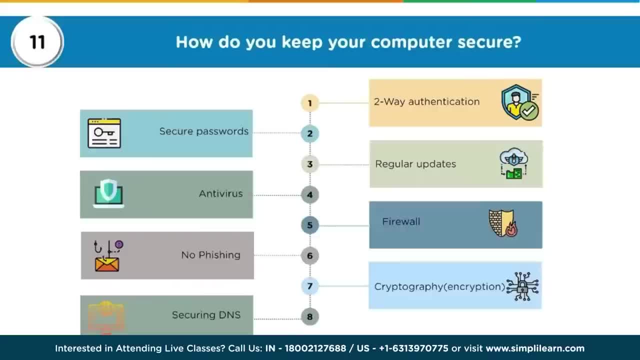 passwords, which means that the password is complex enough to withstand most of the common attacks, and a brute force attack or a dictionary attack is just not possible. So we want to randomize our passwords. We want to create a complexity where a password meets standards such as: has at least one lowercase, one uppercase character, has numerics and. 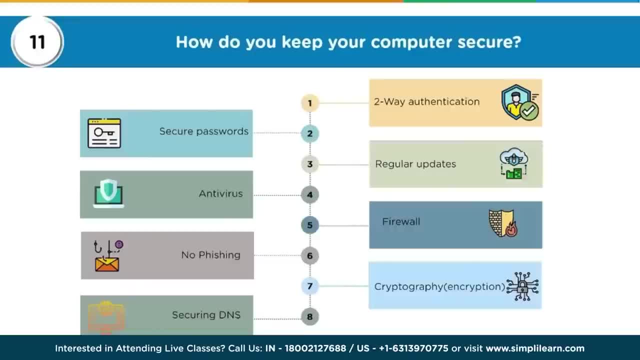 special characters and is randomized, is not based on a dictionary word, doesn't contain usernames, email addresses, phone numbers or anything that is personal to that particular user. Third, keep regular updates, which means that there will be patches that will be updated every single day. So we want to randomize our passwords. We want to create a 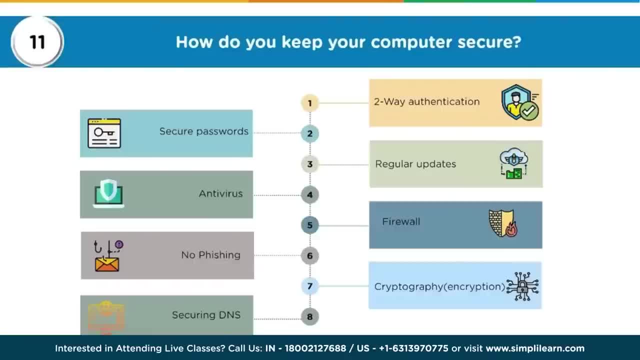 patch that will be released for the application for the software that you're utilizing. download the patches. install them on a regular basis to ensure that you are secured against the most recent attacks that have been identified. Install a good antivirus could be an internet security. 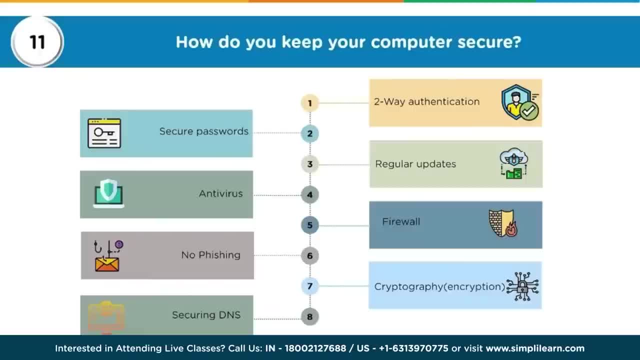 suite which will have an antivirus, an intrusion detection system, a firewall, and will help you protect yourself against ransomwares, malwares and any script-based attacks. Also have a specialized firewall on your system. could be a host-based firewall or a network-based firewall to ensure. 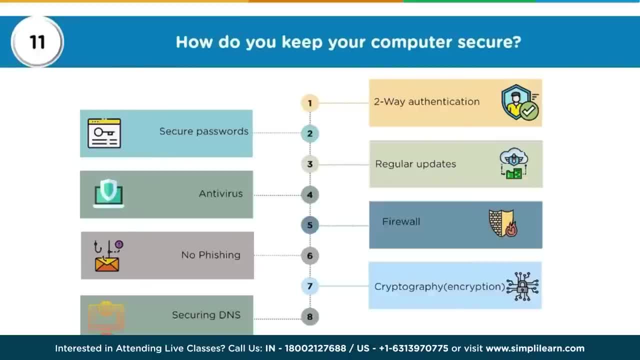 that attacks are kept at a minimum and you have your network definitions in place to allow or disallow connections from happening to your devices? Have anti-phishing softwares installed as well to ensure that you are not getting any spam mails. Even if you do, you're able to identify. 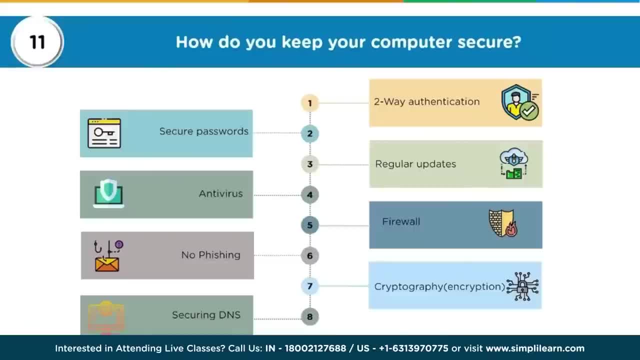 that and not fall prey or victim to those spam mails. Phishing attacks are generally like where they are directed towards individuals and they prey on the gullibility of that particular individual. So our Nigerian frauds, or the lotteries that we win on a regular basis of hundreds of 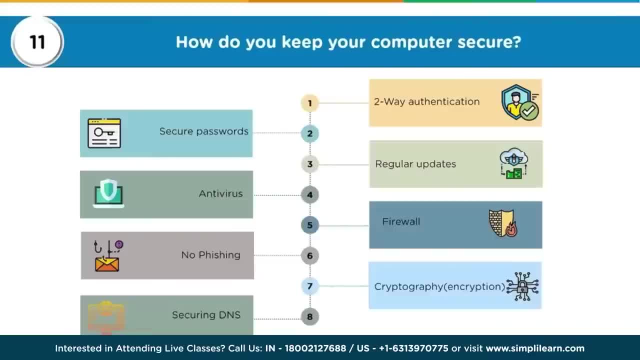 million dollars. those messages, the emails that we receive- they are all phishing emails where they're basically prone to victimize the user and then rob them of money or install some malware or do some other malicious actions. If you want to enhance encryption about data that you have stored on your devices or that is. 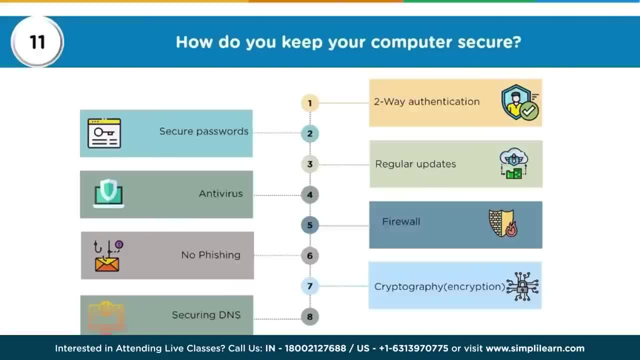 accessed by your software or being transmitted by your software. use encryption: Encrypt your data whether it is at rest, whether it is in motion or whether it is at use, thus reducing data leakage and data loss possibilities. And, finally and the foremost, secure your DNS. DNS is the domain name. 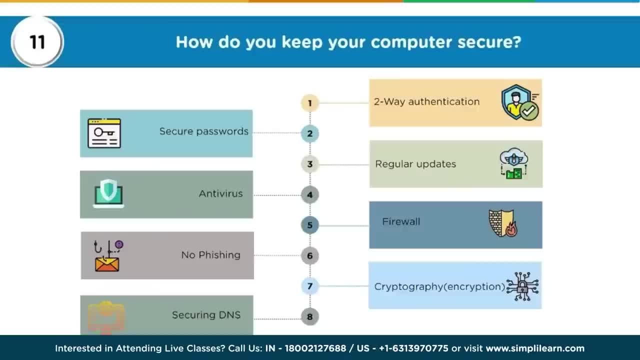 server which is utilized by computers to resolve domain names to IP addresses. If a DNS poisoning attack is possible, where your DNS settings have been modified by an attacker and you're redirected to a malicious DNS server, that server is going to redirect you to another malicious application which may have a malware or a malicious software as a payload. Also, you don't. 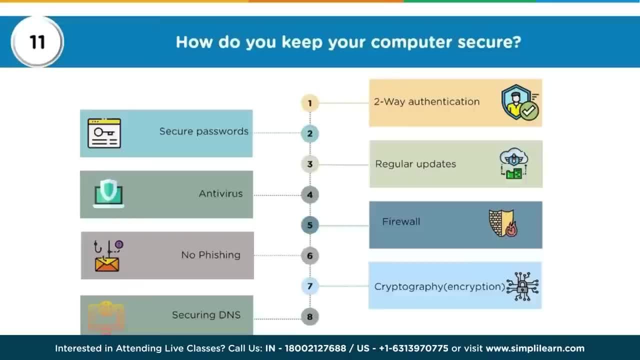 want people to know your DNS servers and the queries that you're making, so you want to use your DNS. So, in a nutshell, if you follow these eight steps, your devices, your computers, your applications are going to be as secure as possible. The next question discuss security. 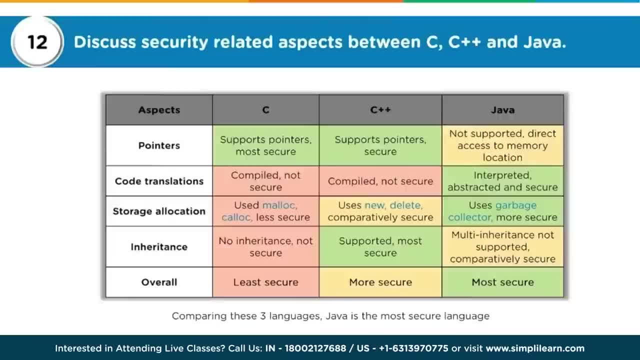 related aspects between C, C++ and Java. Now, this is an open-ended question. It depends on which level you're giving an interview on, but you're looking at it from a freshers perspective or a less experienced perspective, and thus these are some of the aspects that we want to look at, and 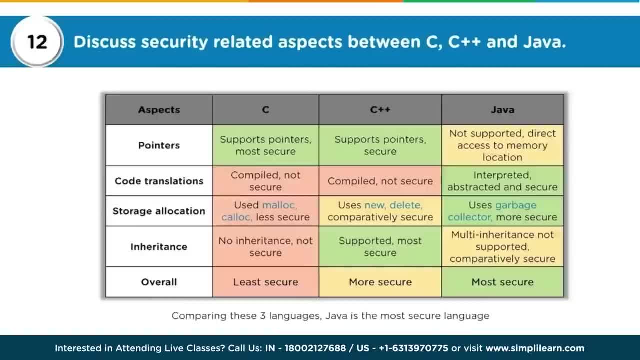 the comparisons between C, C++ and Java. Thank you. So the five aspects that we are looking at are pointers, code translations, storage, allocation, inheritance and overall security based on C, C++ and Java. So when we say pointers, we are looking at how we are going to. we are using pointers and stacks and keeps to point to. 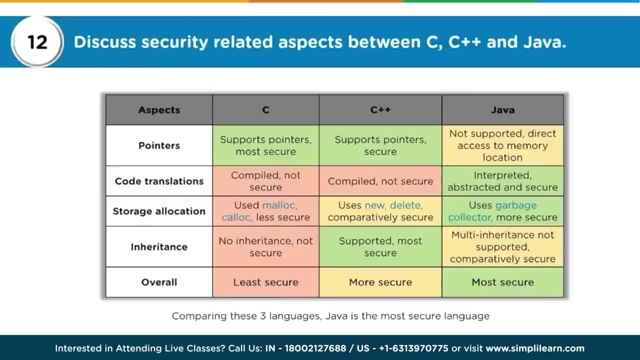 functions and how we exit those functions and how those functions are then recalled into the network. So when we say pointers, we are looking at how we are going to. we are using the next function. So C supports pointers. It is most secure. C++ also supports pointers. 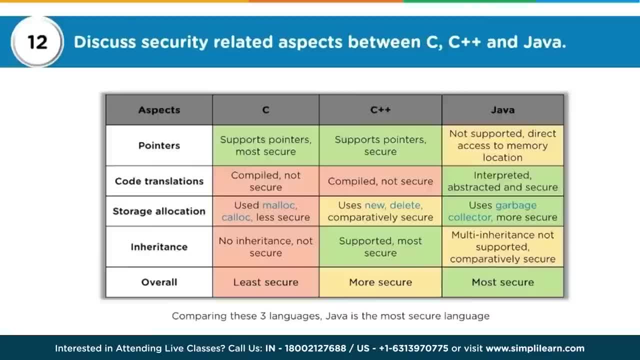 but it is a little bit less secure than C Java. it is not supported, Tarot access is given to memory allocation and thus it is the least secure as far as pointers are concerned. When we look at code translations, C is able to compile but it is not secure. Same with C. 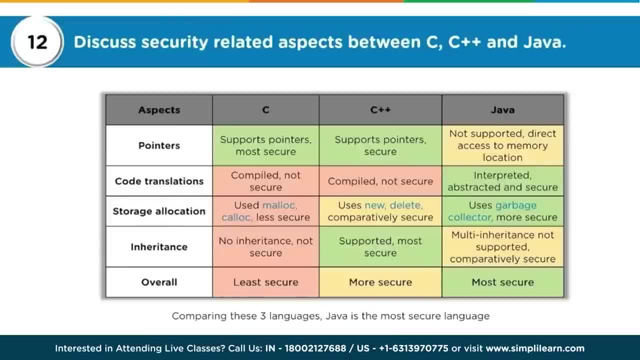 C++, but in Java it is an interpreted language and it is abstracted and secured In storage. in C we use malloc and calloc memory allocation, which is less secure because it does not have internal checks on verifying what memory is allocated and the user input that is being. 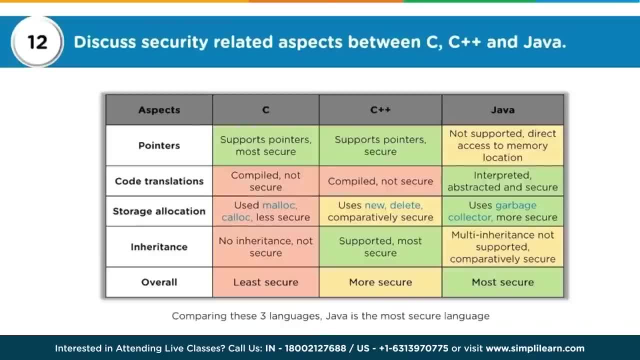 compiled or that is being input to that memory. Thus this can allow buffer overflow errors to creep in because of the non-verification of the input data. So it is the least secure. In C, C++ it uses new and delete options and is comparatively secure, but Java uses a garbage collector and 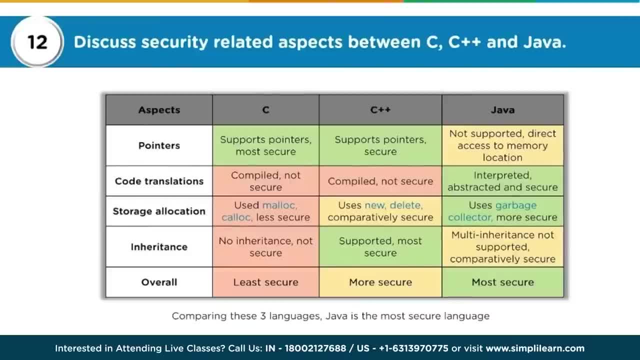 thus is the most secure. as far as storage allocation is concerned, When we talk about inheritance, the most secure is C, C++. C has no inheritance, so it is not secure. In C++ it is supported. thus it is the most secure, Whereas in Java there is multi-inheritance. 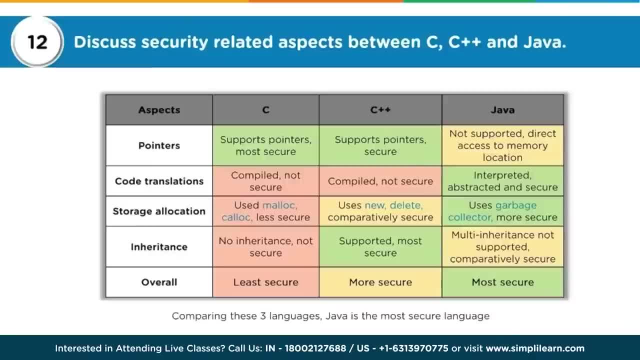 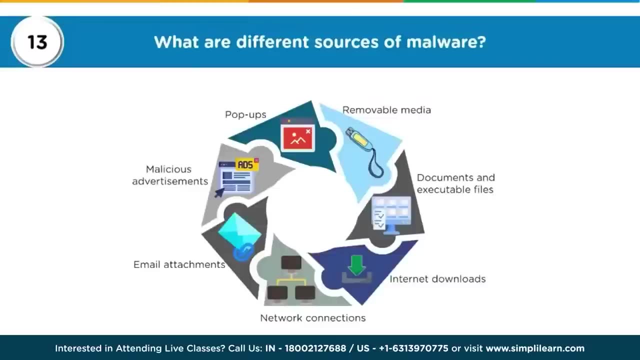 that is not supported and thus is comparatively secure. Overall, the most secure out of all these, based on these five aspects, is Java, the least secure is C and the mid-level is C++. Moving on to question 13,, what are the different sources of malware? Now, malware stands for. 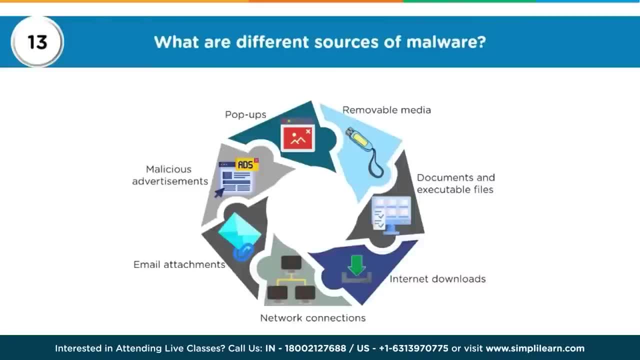 malicious software. right, Malware is basically a software that poses as a legitimate software but has a payload of a Trojan virus, PiWare, Keylogger or some malicious software that is going to have a negative impact on security. So the question here is: what are the different sources of malware We want to identify the most? 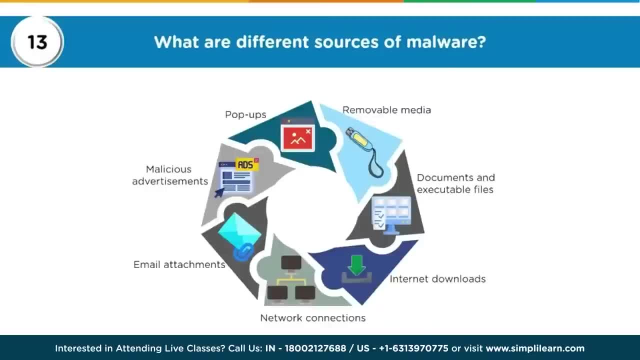 common sources through which malwares infect end-user devices in today's world And we can start with pop-up ads. So, most of the websites, if you're visiting untrusted sites, if you're being redirected to sites that you don't know about, there'll be a lot of pop-ups coming your. 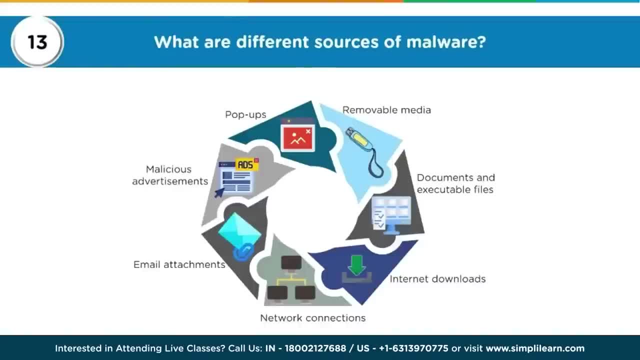 way where it says you're the one millionth visitor to this site. please click here to download your gift. Or it will say congratulations on winning a particular product for visiting this page, and so on and so forth. There are some instances where you can see a banner which is flashing at: 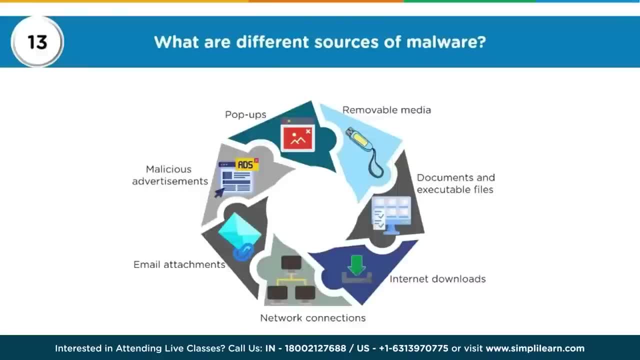 you on top of the page and says that there are eight infections that have been identified on your computer. click here to download an antivirus to clean the infections. So all of these pop-ups are there as a social engineering attack, as a phishing attack, to make gullible people click. 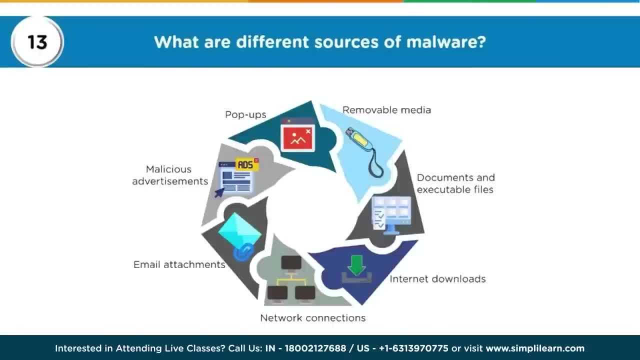 on those links and download Those malwares are the software that is posing as a security. software itself can be a malicious software which is going to install a Trojan or a virus or a bot on your machine, compromising the security of that machine. The second is removable media- USBs- and humans have a fascination. 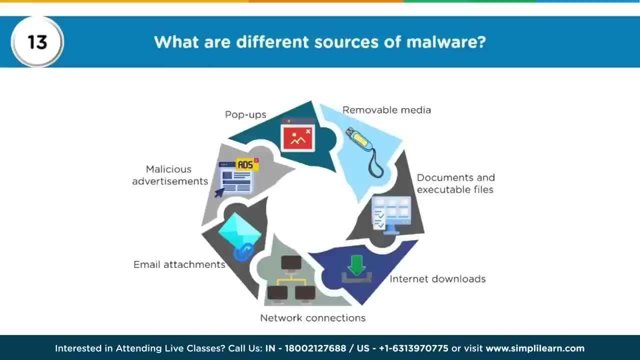 with USBs. So if you find a USB lying around, it's a free USB. you get excited about it and you want to take it home. You want to plug it into a machine and see what's on the USB. Worst case scenario. 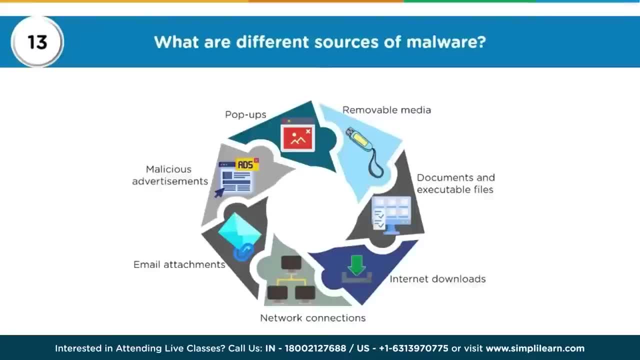 you format it and you've got a free USB to utilize. The higher the capacity, the better, But that is one of the most easiest ways people use malwares to be deployed on unsuspecting users. If there is a USB lying around, why would somebody want to forget a USB? It's most likely planted. 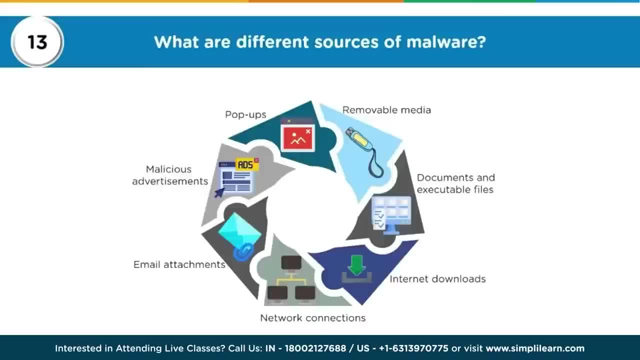 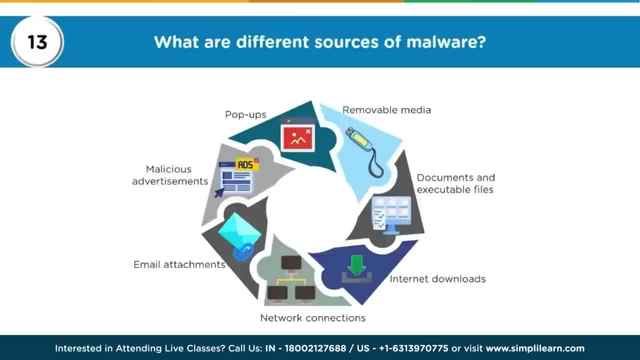 If the device is not secured enough, it is going to install the USB, Then documents and executable files. This is where your virus is and all those creeps in. So let's say you're surfing on the internet, you're looking for a software and you find the software on a particular website. 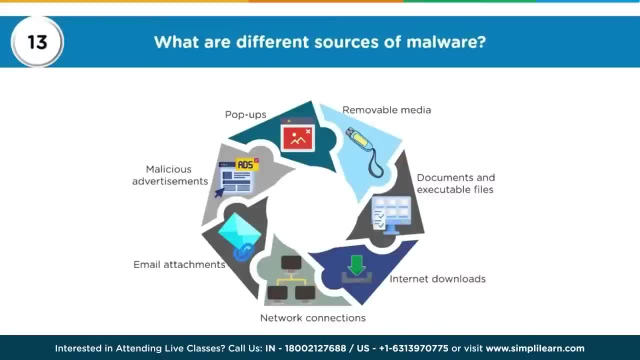 You do not verify the trustworthiness of that site and you just download and install that software. Now that software could be malware as well. Thus, if you're surfing on the internet, you're downloading files from different locations. you have to research the website, you have to research the. 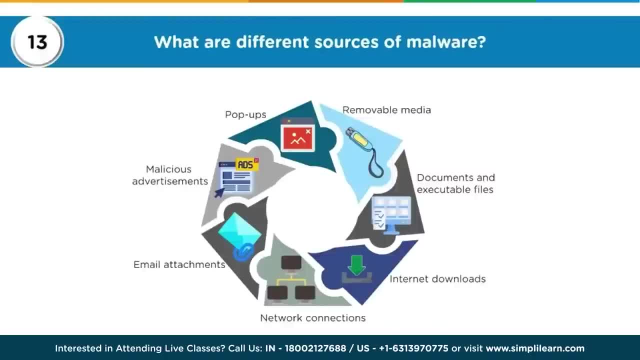 the source to ensure that it is trustworthy, and only then are you going to download and execute those files. thus internet downloads as well, and when we say internet download, it's not just untrustworthy sites. we go to torrents, we go to the dark web or the deep web and we are searching. 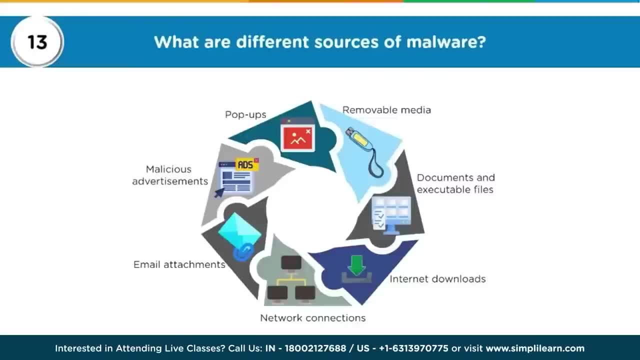 for other softwares, especially those who are researching security right, we always want, we are always on the lookout of new softwares and we are always on those forums which may not be so much trustworthy and we just download those files and start installing them. that is a very bad. 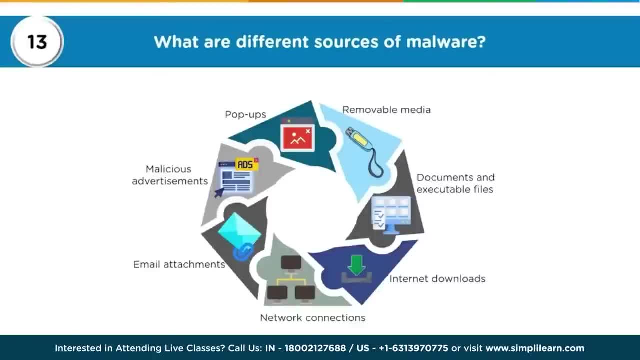 scenario right. so you have to be very careful what you're downloading from the internet. your antiviruses, your anti-phishing mechanisms, your threat intelligence mechanisms have those mechanisms installed and you want to verify where your downloads are coming from. then your network connections. if it is a p2p connection, it is a local area network connection or a metropolitan. 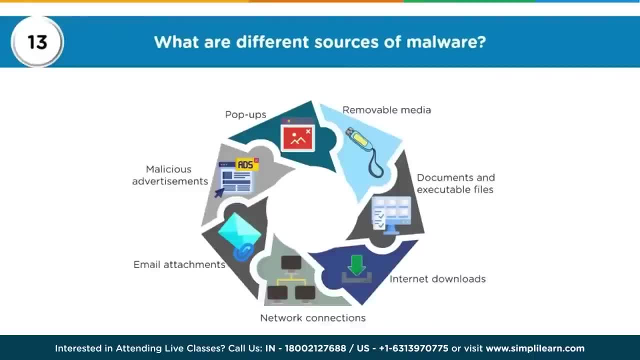 area network. you have to verify whom which devices are connected to your machines and you have to validate those connections before you want to trust those devices and before you connect to them. if you are on a public wi-fi, you probably don't want to connect to a public wi-fi in the 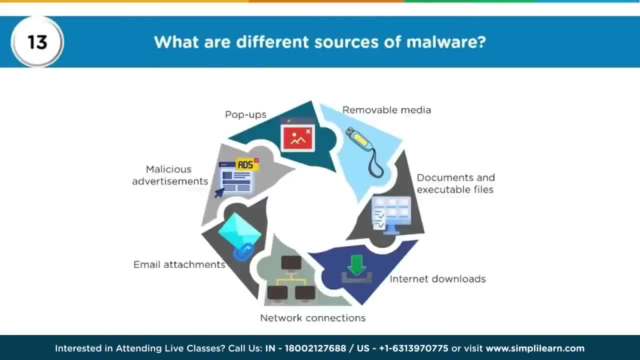 first place. then comes email attachments. there are so many attachments that come across in today's world, most of them in a zip format or a rar format. some of them come as document files, where there are macros hidden within them. macros are scripts that are recognized by Microsoft. 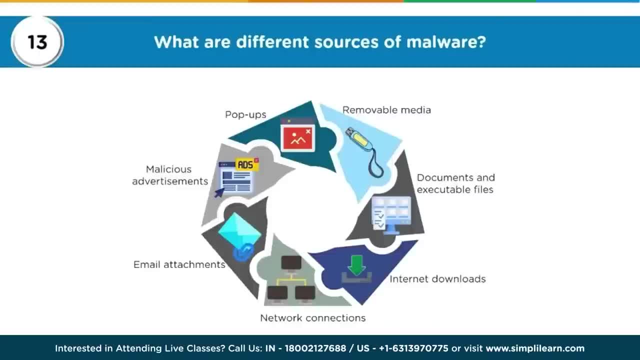 office files right. and then, finally, there are these malicious advertisements that we find online. right, let it be Facebook, let it be WhatsApp, let it be any social media platform that you go, or even your search engines. their job is to display ads. their job is not to verify whether 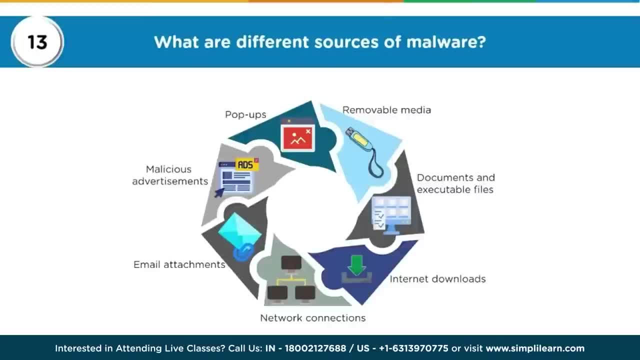 the ad is legit or not. it is for us, as consumers to be careful and valuable to our customers. It is for us, as consumers, to be careful and valuable to our customers. It is for us, as consumers, to be careful and valuable to our customers. 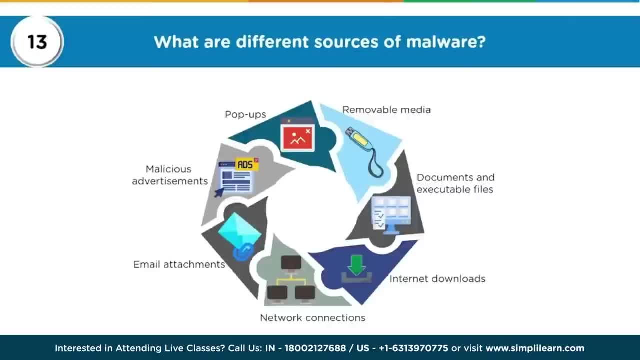 that ad and verify whether it is a genuine ad or not. so just don't start clicking on any of the ad, trusting the platform that you're on be sure that you are investigating that ad. so these are the most common sources of malware and the end user will always get infected by one of these mechanisms. 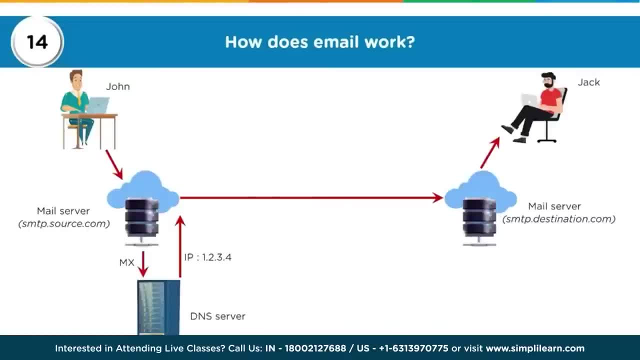 moving on to question 14, how does email work? now, this is a very can be a complex question, but we have to keep it as simple as possible and we have to identify that there are two servers where both of them either using SMTP, which is a simple message transfer protocol, where, in this scenario, John, 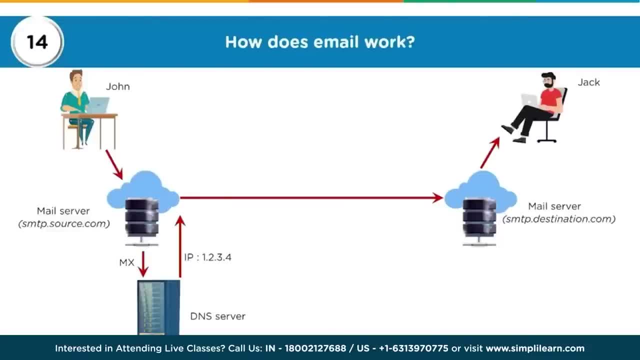 wants to send an email. thus they've got an email client installed on their machine which is connected to the mail exchange server, which has a DNS server, which maps the routing and which maps the exchange server and inboxes. so when John composes that message and clicks on send, John should be connected to a mail. 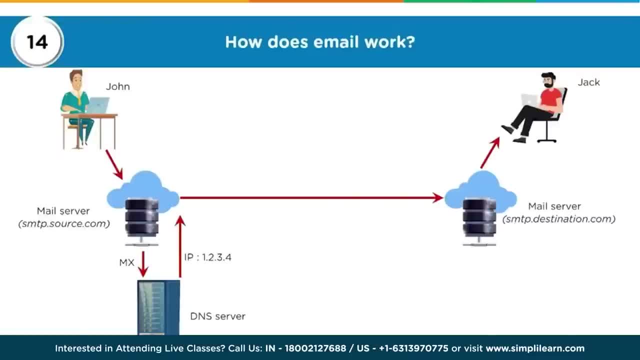 exchange server where the email is sent through that particular person's inbox. so John's inbox will then be validated and that email will then be sent through the DNS server you are through the internet and will be received by the recipient mail server. so at this point in time John also requires the recipients email address. so in this, 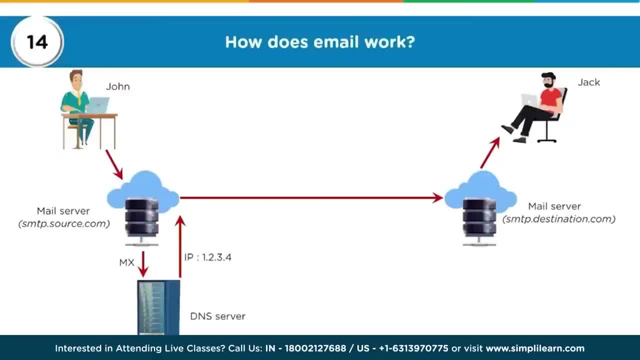 case this is Jack, so Jack, at something calm, would be the email address. so while John is composing, the to field will have Jack's email address, the from field will have John's email address. the subject field will have whatever they want to convey as a message. the message body will have the message itself and then 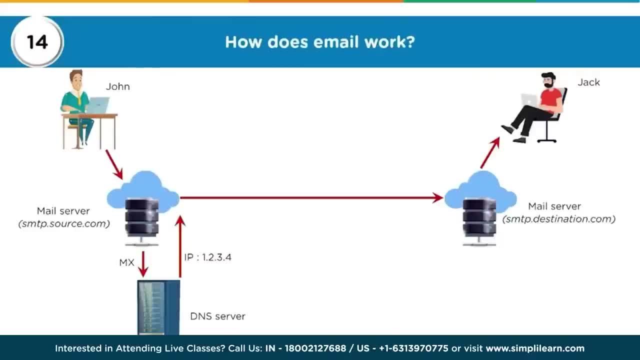 when John clicks on send, it will go to their exchange server. the exchange server will then validate the inbox and identify where that inbox is located for Jack, and then, through the internet, it will be sent to the email, to the mail server of Jack. the mail server will then identify the proper inbox that it now that that. 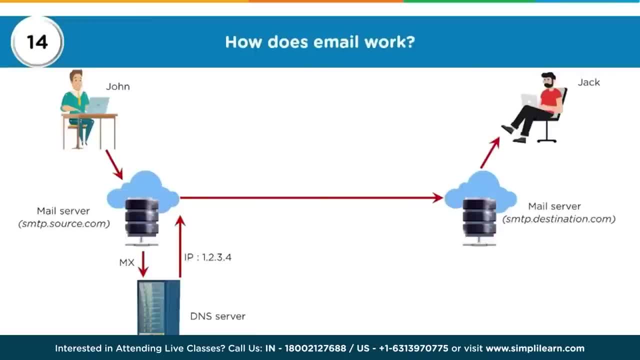 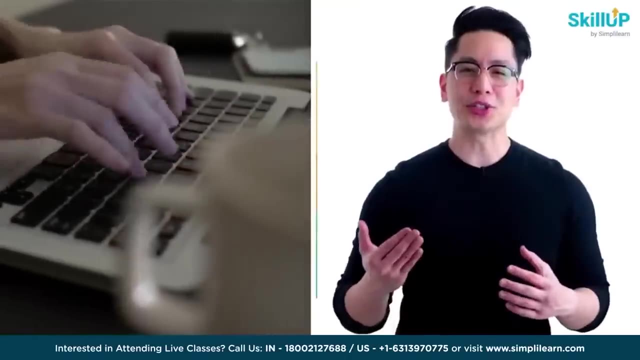 email is to be sent to and it will store that email in that particular inbox. when Jack opens their computer and accesses their inbox, this email from John will be being sent to his database. the email address will be the address of Clark's home and show theem gilt someone in the email address that the website is. 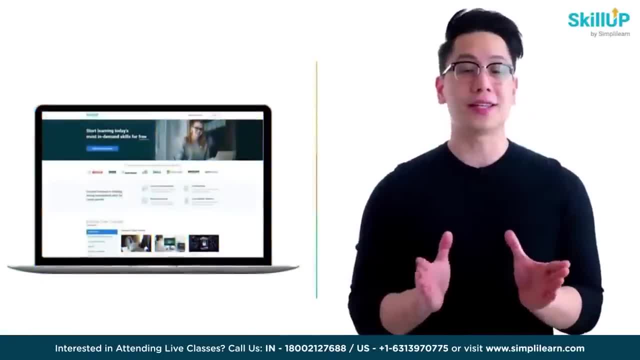 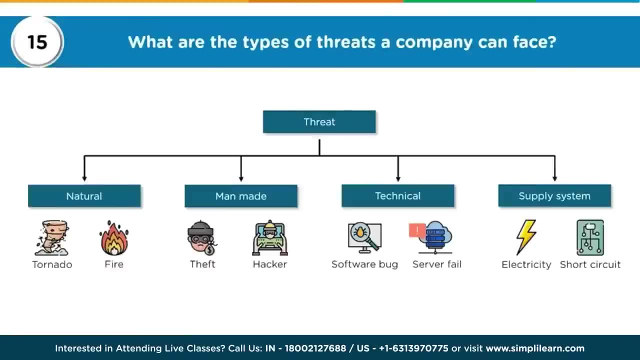 per solluġrikio's manager, that the company introduced into the knowledge system when Addison醤 Friday, with which jar washingを? what are the threats that are most likely that a company will face? so, on a broader scale, the threats that a company will always face would be classified as natural threats, man-made threats. 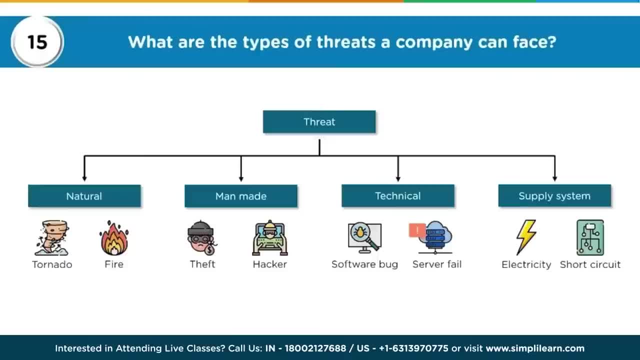 technical threats and a supply system threat. so a natural threat would be an act of god which is outside the control of human beings, could be storms or any natural occurrences like volcanoes, thunderstorms, flooding, earthquakes, fire and so on, so forth. so anything that is natural. so it 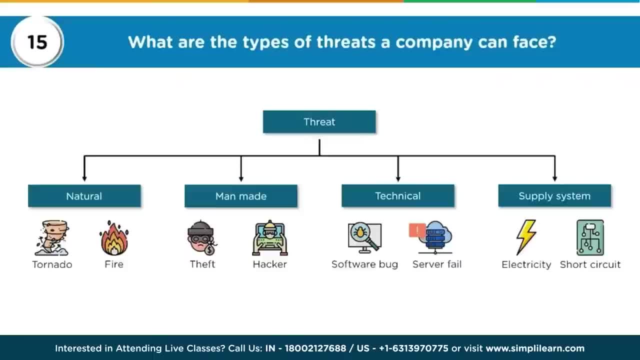 depends on the geographic location that you're in and what kind of climate that area faces, and you need to identify the immediate threats and prepare for them. so if it is flooding that you're looking at and you want to look at an office and the possibility of the office getting flooded is 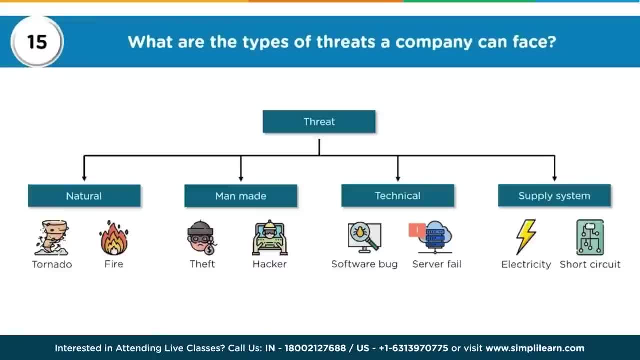 real. you probably want to have a take office at a higher floor so that the threat of flooding is minimized. for fire, we always have a fire drill where we practice our fire mechanism so that we can evacuate all humans as soon as possible and then worry about the technicalities of it. under any circumstances, under any threats, humans will always have the 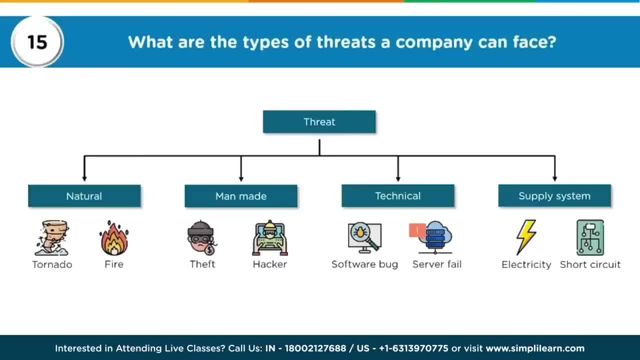 first priority and then everything else comes in. man-made threats are where man themselves are a problem. so strikes, lockouts, hackers, theft uh, war, rioting, all of those are man-made threats, uh, which we ourselves cannot be in control of. but we need to plan for them and we need to have a business continuity plan or a disaster. 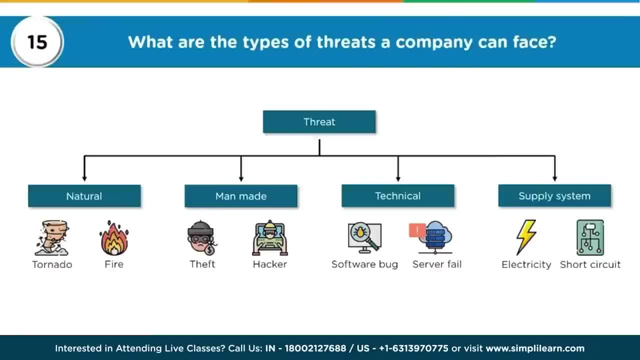 repair plan for any of these threats that have been identified. then come the technical threats. technical could be software bugs, operating system bugs, application bugs, that uh, that come with the applications that we have, or a hardware failure where a server crashes, and so on and so forth. so 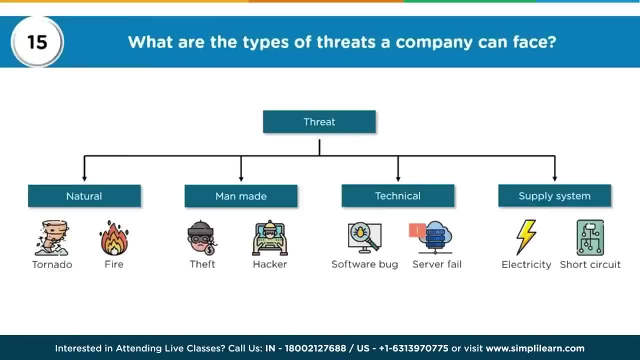 let's say a hard disk crashes, maybe, uh, the processor stops working, the motherboard stops working, ram gets corrupted, uh, any of the technical aspects stopping uh stop functioning, thus creating a break in the business, can come under technical right. so, uh, anything to do with computers, let's say a server failing or a patch that is not installed on a particular software. 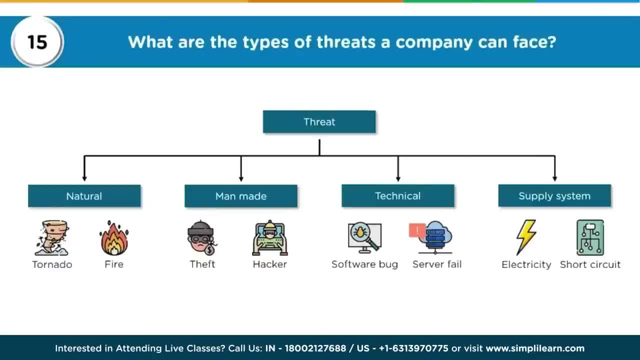 would come under technical threats. and then the supply system. the supply system are your environmental threats, which depend on your supply chain failures. what is the supply chain for the office to function? there are a lot of dependencies. that office goes through right. there are a lot of other vendors that suppose that support and provide critical infrastructure, non-critical. 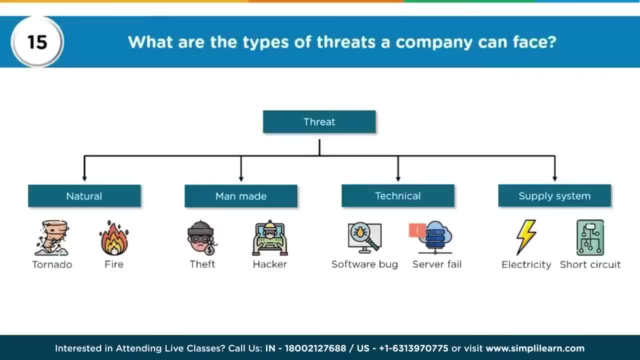 infrastructure for the office to function, for first and foremost, electricity. without electricity and you're not going to be able to function. so if there is an electricity service provider and if there's an electric outage, that's that comes under supply system. so that's a supply chain failure, where 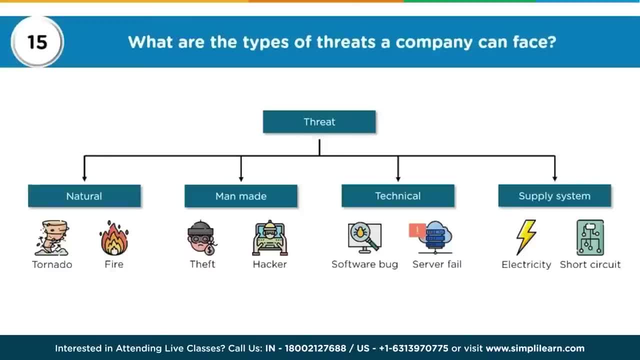 the vendor that provides electricity to you has failed in providing that particular service, and now you need a business continuity or a disaster recovery plan. so you probably have an inverter, or you all already have a power generator plant that is going to generate your own power and supply to. 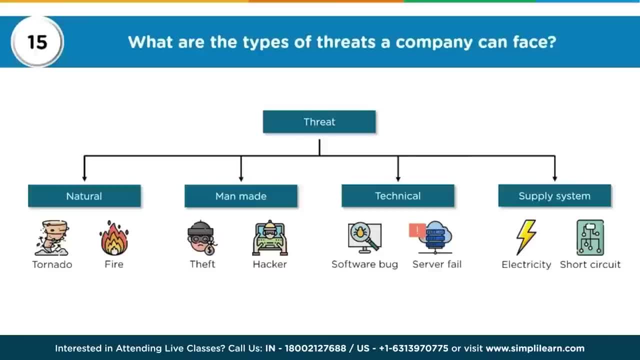 your system right. there could be short circuits because of fluctuation in the electricity. uh, maybe the internet service provider fails and your internet caches so you have a backup line for the internet from a different vendor. right, and so on, so forth. maybe your hardware vendors, who are supplying you servers, desktops, 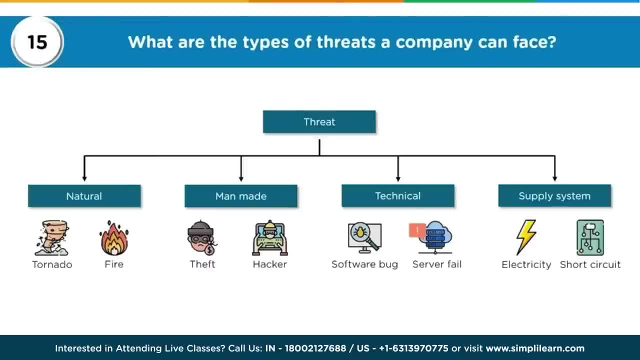 laptops and whatnot. they fail because they feel they are facing a strike or they go bankrupt and suddenly you can no longer purchase hardware from your vendor because they no longer are in business. so that's a supply chain failure. so any of these systems failing would also come under threats. 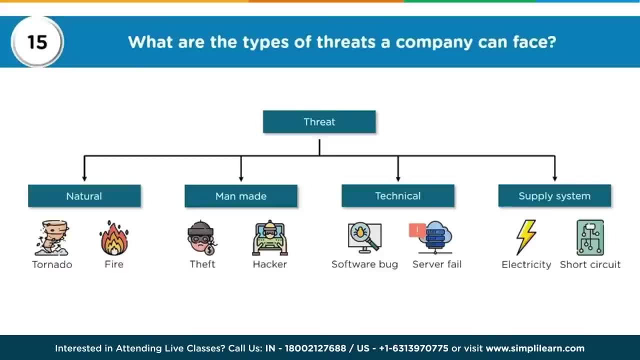 so, under a broad category, these are the first four threads that you need to identify and then you can elaborate by providing more scenarios based on the experiences that you have had towards each and every of these threats. so, natural threat, where you may have had experience, where there 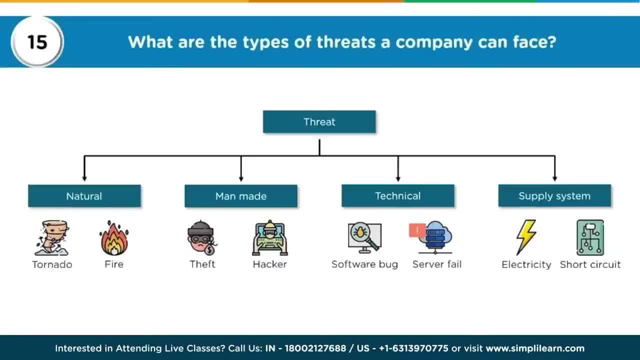 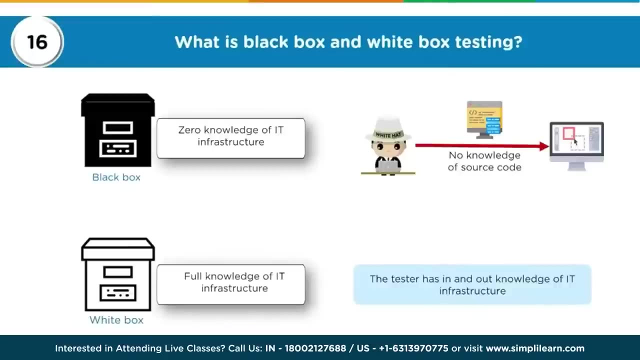 would have been, let's say, a flooding or any natural disaster which caused a problem for the continuity of your particular business. so identify each and every example for each of these threats and provide that as an example in the interview. what is black box and white box testing? 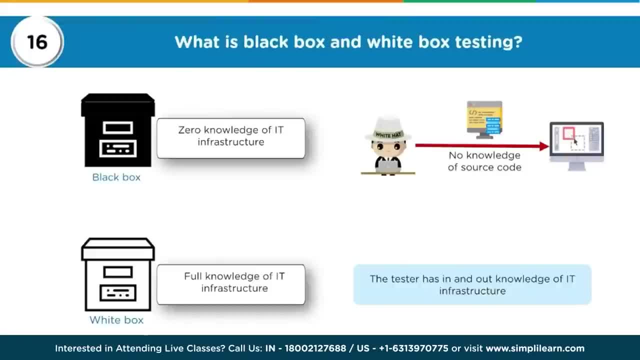 so when you are testing a software or you're testing your infrastructure, there are two different tests that you can conduct. the first one is a black box. the second one is a white box. in a black box test, there is no knowledge that is shared with the tester. so let's say you're an ethical hacker. 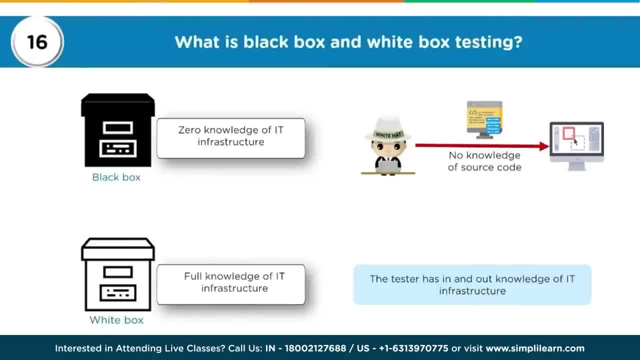 and you have been awarded a contract by an organization to test their current application, that now they are not going to give you any information. they're not going to tell you what the application is. they just probably give you an ip address and a port number where the application is hosted, and 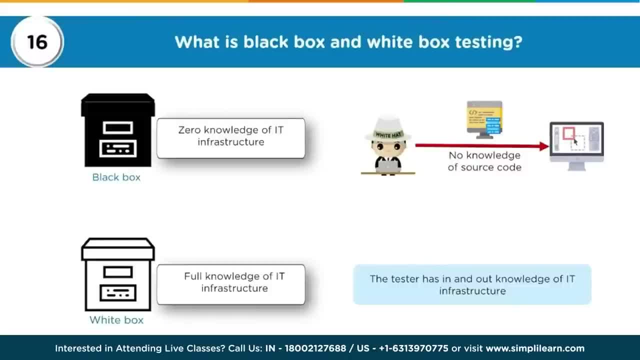 now you have to find in your own queries and try to figure out what the application is, try to gather information, see what, what information can be gathered in the first place, and based on that you're going to figure out your way, identify vulnerabilities and see if any of those 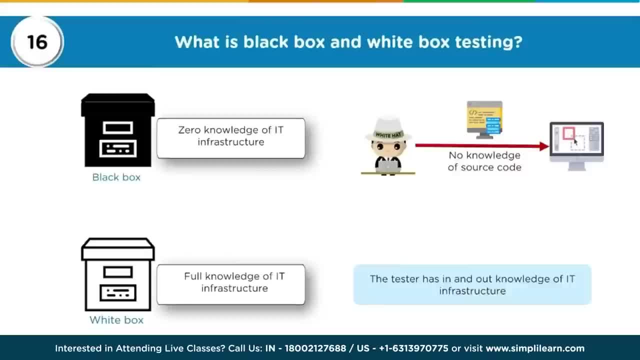 vulnerabilities can lead to an security incident. so, without any knowledge, zero of the IT infrastructure or the source code, that's a black box attack or a black box test. A white box test, on the other hand, is where full knowledge of the IT infrastructure or the source code is shared. so the ethical hacker has 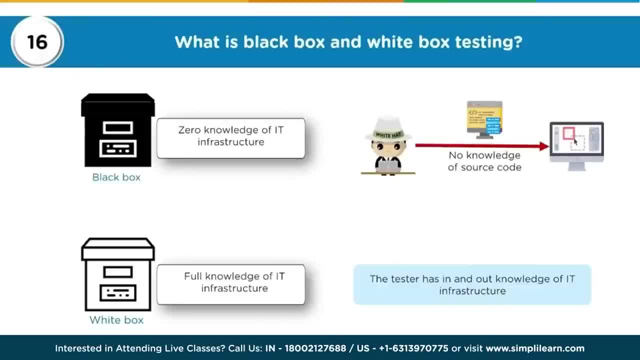 complete knowledge and, based on the knowledge, they are then going to test out the system to see if there are any flaws that they can identify right. So why would these two audits be important? because the first one, a black box audit, emulates the attack of a outsider, or external hackers, sitting outside the 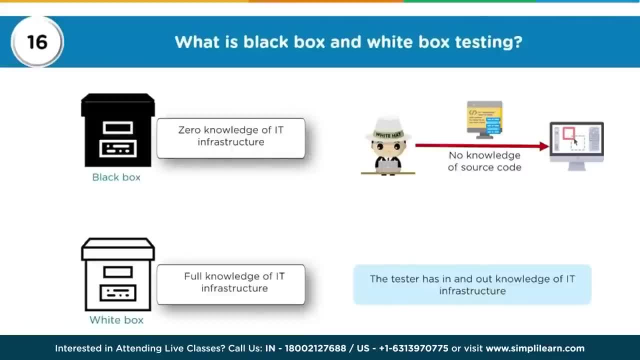 organization trying to figure their way in where, as a white box attack can emulate the attack of an insider, So a discredited employee within that organization misusing their access control or their access rights to make unvalidated profits, right. So somebody is corrupt. who has been? 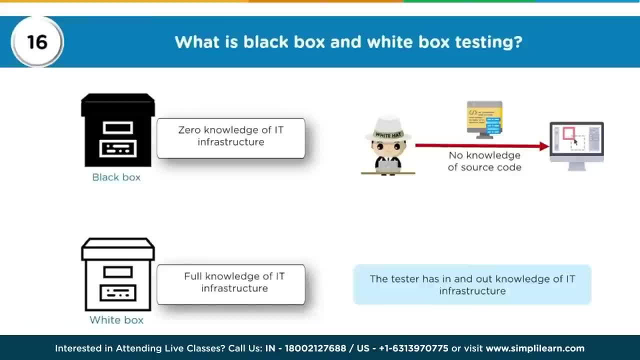 bribed who wants to sell out company secrets based. so they are going to try to find out vulnerabilities, try to stalk, steal data and try to sell it on the grey market. So a white box would emulate an internal attack, a black box would emulate an external attack. 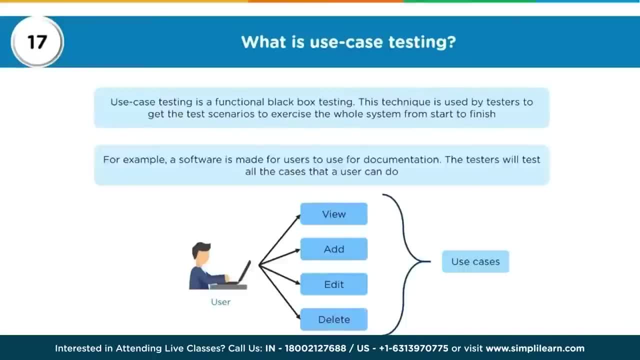 Moving on to question 17,. what is use case testing? Now, use case testing is a functional test and it is also a black box test. What is a functional test? It tests the functionality of a particular software once it has been created. Why is it a black box test? 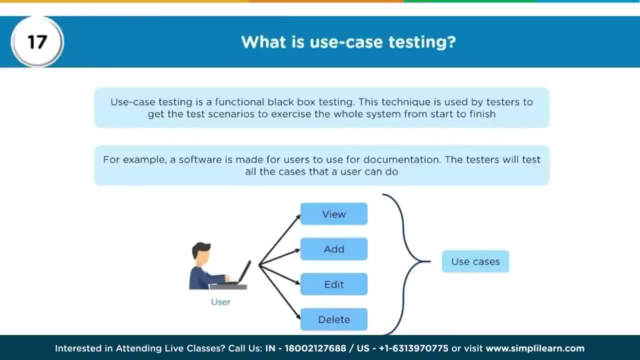 Because the user doesn't know what the functionality is. they just want to find out each and every scenario and try to see what that scenario generates as a response. They are not sure whether that is the appropriate response that should be generated or not. They're just trying to find out the response that is going to be generated after they fire. 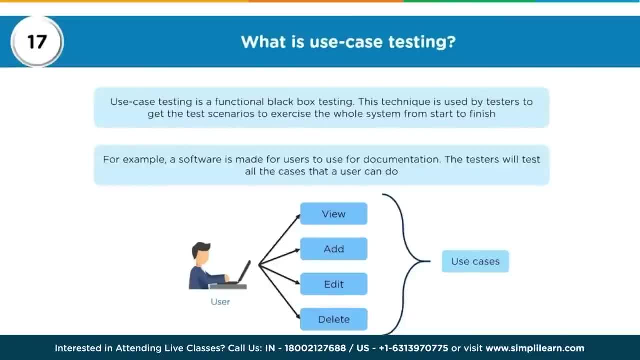 off a query. So this technique is used by testers to get the test scenarios to exercise the whole system from start to finish. So let's say it's a login mechanism for an application Right Now, a user- at this point in time the tester, since it's a black box testing- will know. 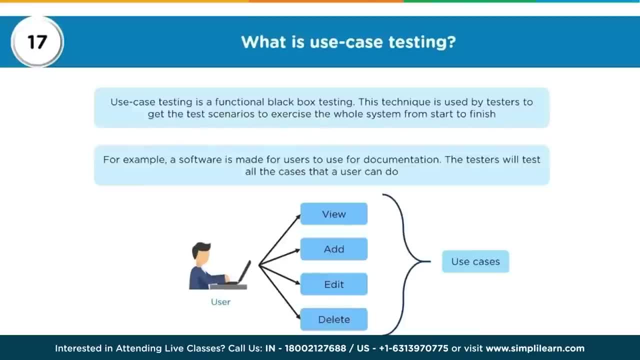 that it is a login mechanism. They will not know the details of what logging mechanisms are being utilized. So they wouldn't know whether input validation is done. They wouldn't know whether output encoding is done. They wouldn't know how the CGI calls are being made. 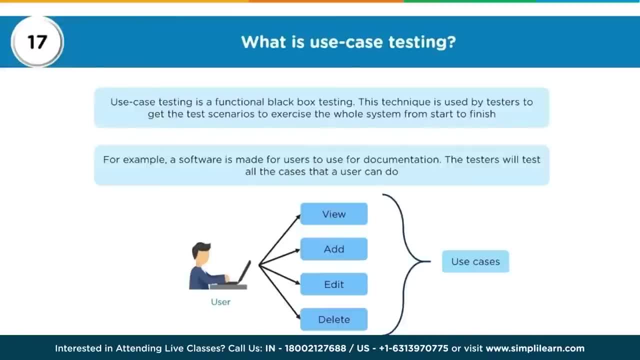 They will not know how the queries are handled at the server side and how the database is going to treat that particular query. So they have no idea whether SQL injection attacks are possible and so on. So for them, with whatever input they're going to try to insert for that login mechanism, 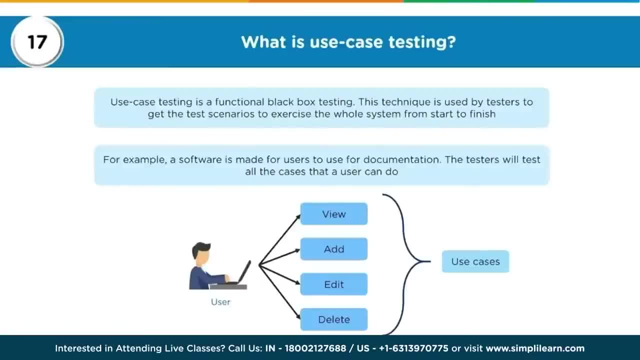 that's a functional black box test, The functionality being whether the login mechanism works and, based on the type of inputs that they're going to put in, whether it creates an unwarranted output, whether they can bypass the mechanism or they can hack into the system. because of some of the flaws that were left, 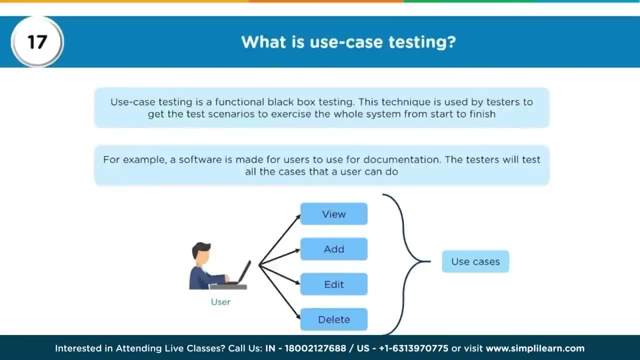 behind Right. Another example: here is a software made for users to use for documentation. The testers will test all the cases that the user can do So. can the user view a document, Can they add new documents, Can they edit documents and can they delete documents? 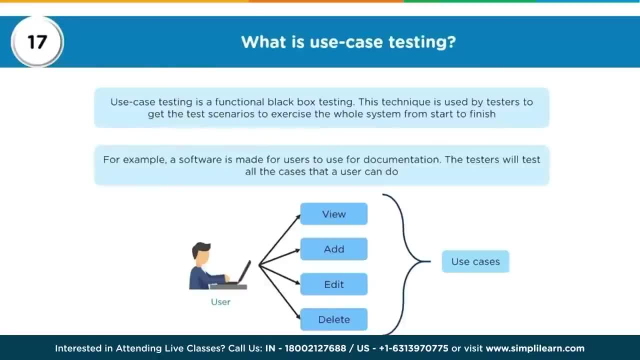 So this functionality will depend upon the access controls that have been granted to a particular user. So for this particular user, the tester, at this point in time they would not know whether they're an administrative user or they're a regular user. They'll just try to do all of these and then write the responses saying I was able to view. 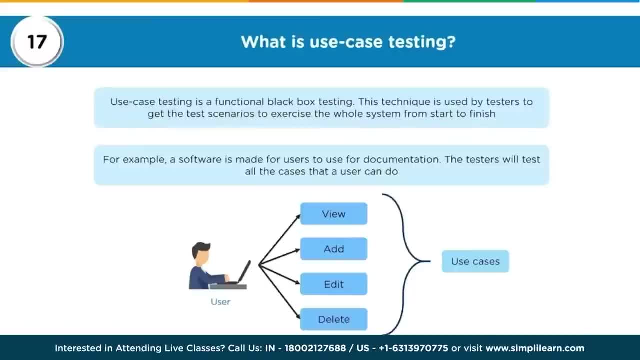 I was able to add, I was able to edit And I was able to delete. Now, the result will be then sent to a manager. The manager will look at the results and then, based on the actual access controls that were supposed to be there for this particular user, then we'll try to identify whether this is. 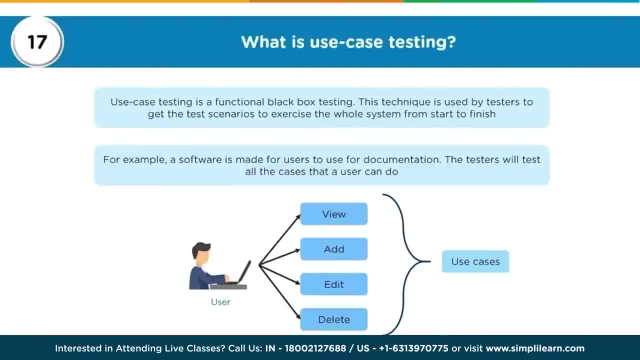 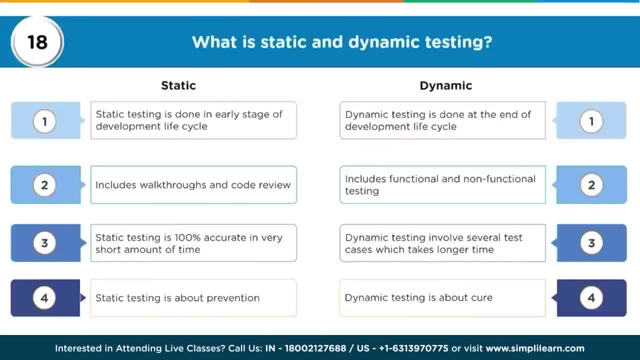 an acceptable case or whether there were any flaws within this case. Moving on to question 18,: what is static and dynamic testing? Now, this is again in application testing. Static testing is done in an early stage of development lifecycle, Software development life cycles. there are multiple of those. 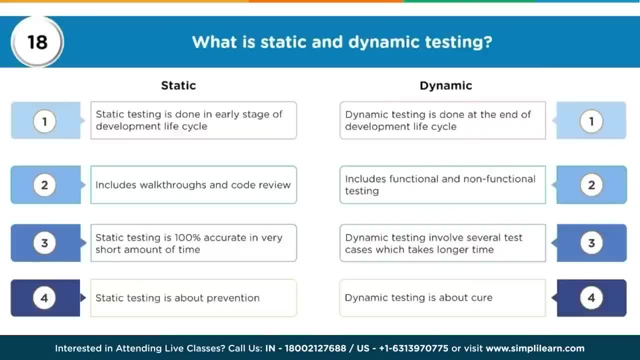 What are these life cycles? There are different stages in which the application is created and provided to the customer. So your first stage would be determining the scope of the application, determining the hardware requirements for that application, then creating a flow chart for that application. 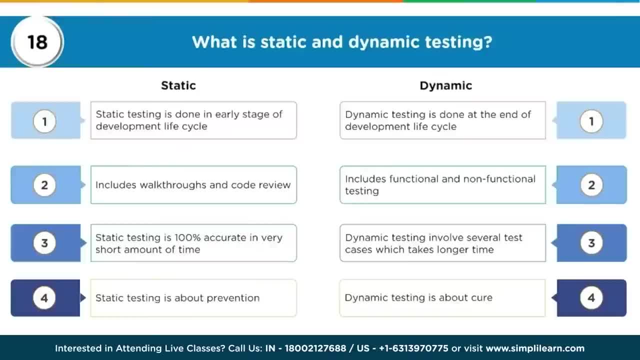 a functional chart for that application and then maybe start coding. Then an architect comes in, tests the code, verifies the code, Then the testing phase comes in, then the security testing phase comes in and then the user acceptance testing comes in. 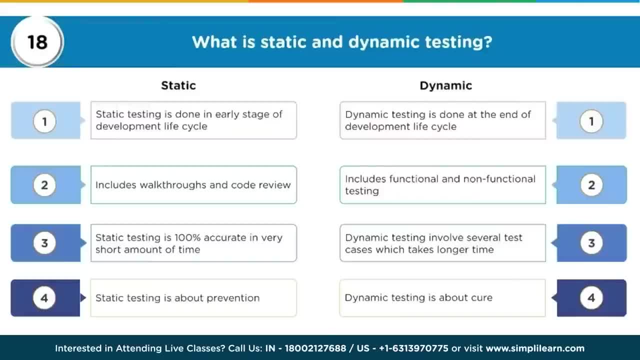 But in every stage, at the very earliest of all stages, a static test will always be started to see whatever code has been developed, whatever scope has been developed, whether that scope is going to be correct or not. This will include walkthroughs and code review. 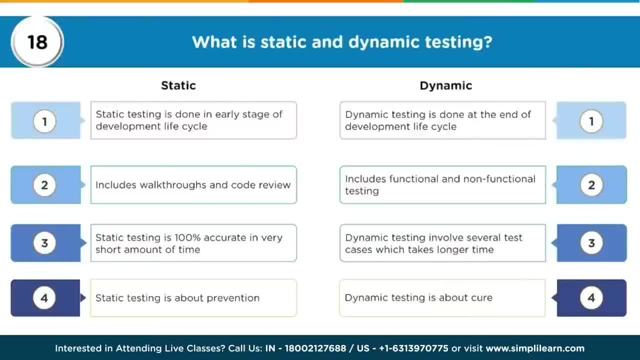 What is a walkthrough? A walkthrough is going through documents that have been generated and trying to find faults in the documented journey that has been generated. So what is a walkthrough? A walkthrough is a workflow that has been created so far. So let's say somebody has created a workflow or a flow chart for a program, how the functions. 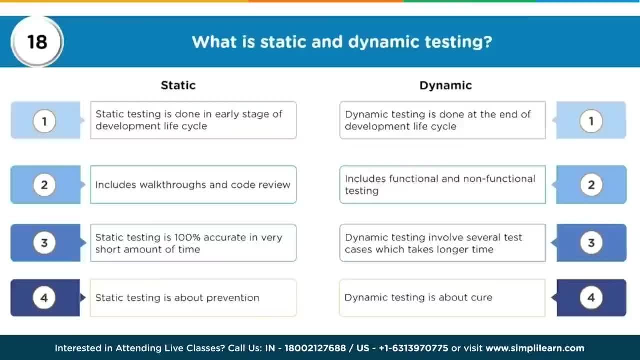 are going to be called and how they're going to be executed. So a walkthrough would be where all these responsible people will walk through that particular flow chart and find out any flaws within that and then rectify them. If there is any code that has already been written, this code will be reviewed manually. 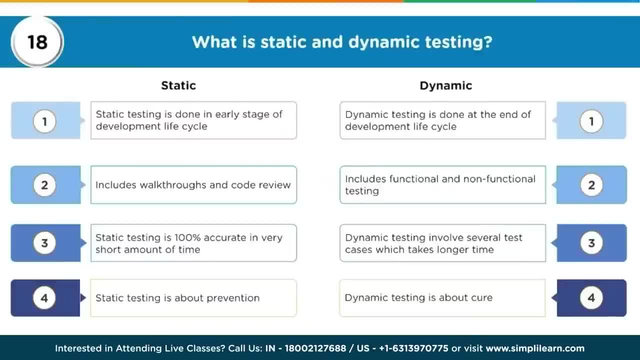 and any flaws within that code would then be identified. But a walkthrough should be 100% accurate in a very short amount of time because it is immediate. You have created it and then the export is going to test it to see whether everything is fine or not. 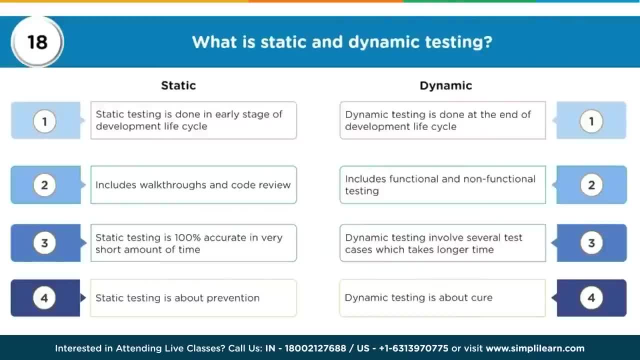 It is all about prevention mechanism. So, since you're doing it at the inception itself, if you find any flaw it gets immediately repaired. So this is about preventing vulnerabilities from creeping into that application at a later point in time, Whereas dynamic on the other side, is done at the end of the development life cycle. 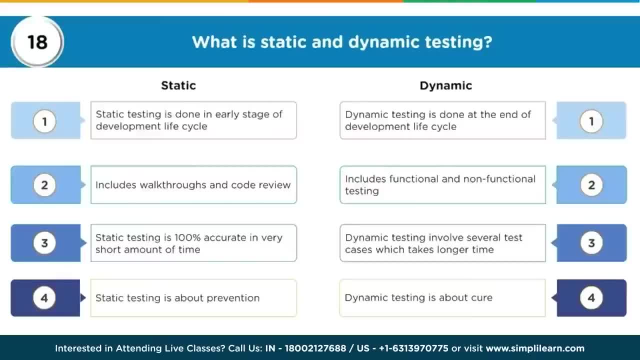 So you have generated the application, Everything is ready. Now you want to do dynamic testing includes functional and non-functional testing. Functional testing is where the application itself is being tested- the functions- to see that all the parameters that are given to the application are functioning properly. 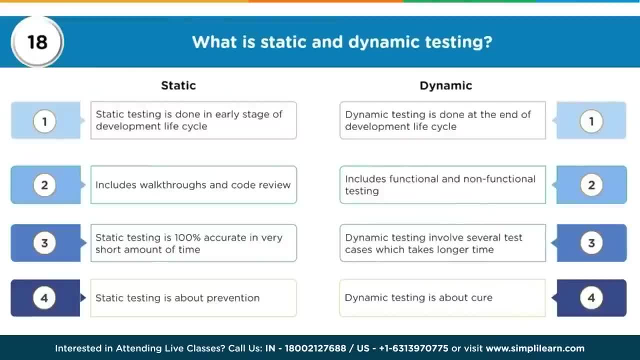 Non-functional testing would be where security parameters, administrative parameters- all of them are being verified Right. This is where your test case scenarios come in, and you're going to test each and every scenario by generating inputs and analyzing the output that the application is going to give you. 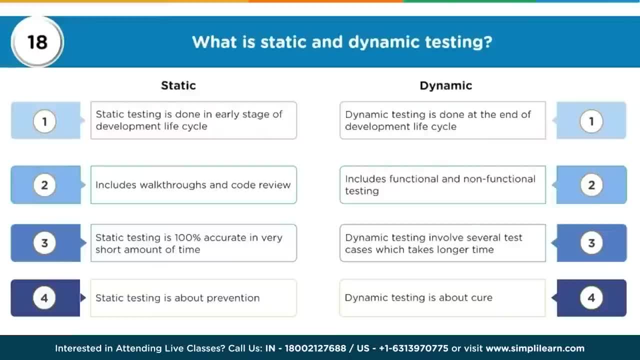 Dynamic testing is all about cure. So here you're going to identify vulnerabilities, report them to the management, and the management is then going to figure out a way of patching those vulnerabilities so that they can be mitigated. Moving on to the next question: what are the test levels in software testing? 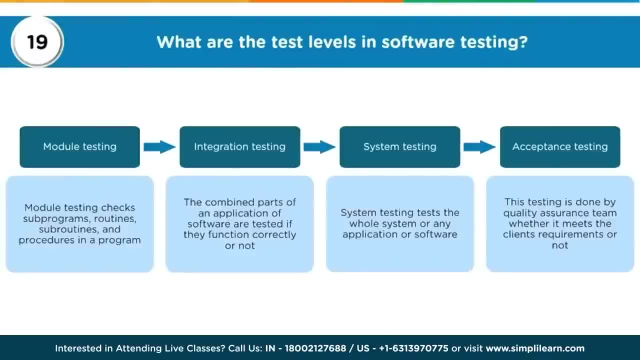 So, as far as software testing is concerned, there are four test levels: module testing, integration testing, system testing and the final one is acceptance testing. So, in the testing phase of your development lifecycle, the first thing is a module test. You're going to check your routines, your subroutines, your subprograms, procedures that are written in a program. 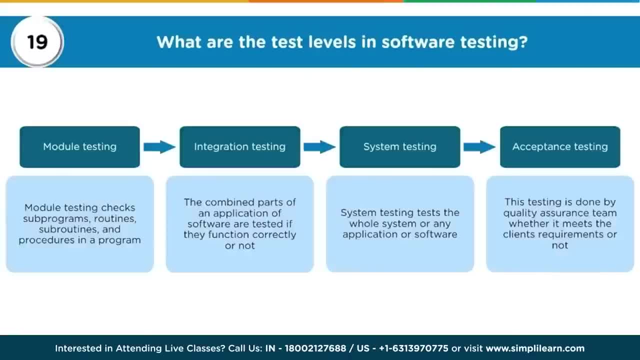 So all your functions, all your mechanisms for that application are going to be tested When you go into integration testing. the software may have been integrated With multiple softwares. there may be different API calls coming in, maybe a third party software on which you're depending upon to supply for information. 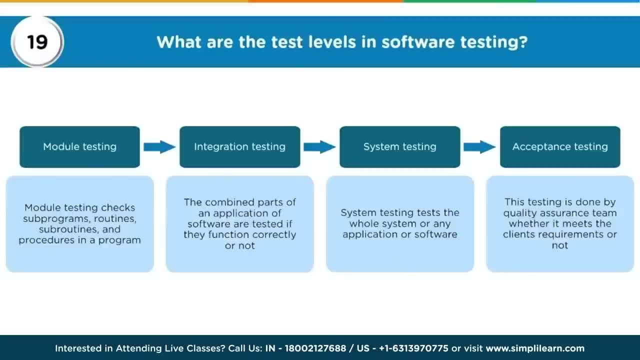 So all of these integration of various softwares, various APIs, are tested to ensure that they are functioning properly and there are no flaws, errors or mistakes left behind in the integration of all of these softwares. Then the system testing is where the entire system, so including the hardware, including the software, right 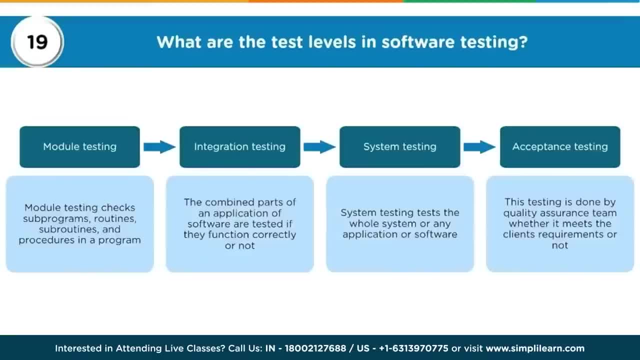 It's Starts from the installation. so now the software is complete, We know which hardware we are going to support for it. We start by installing the software and see where the installation is going to be completed properly. If there are any errors in the installation process itself, then, once it is installed, the performance of that particular application, the write speeds, the read speeds on the hard disk, the transaction speeds that the application is capable of, the network dependencies that the application may have. 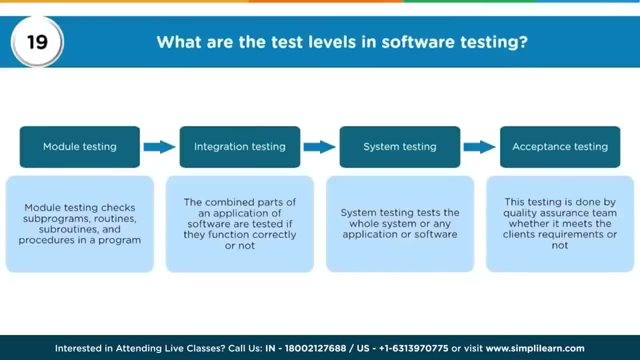 All of those Would come under system testing and then the acceptance testing, which is basically a quality assurance exercise that the application meets the client's requirements. So the client in the first stage would have given the scope of what needs to be achieved in the acceptance testing. 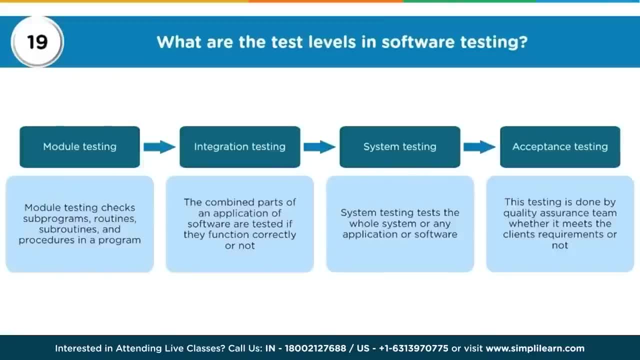 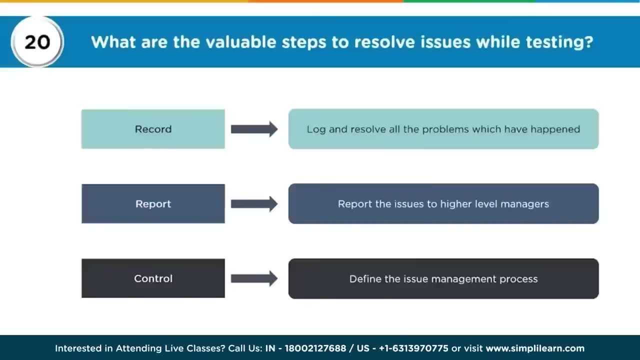 You're verifying that that scope has been met and the client requirements have been met and you can assure the client about the functionality and the performance of that particular application. coming to the last question in this software Program, What are the valuable steps to resolve issues while testing? 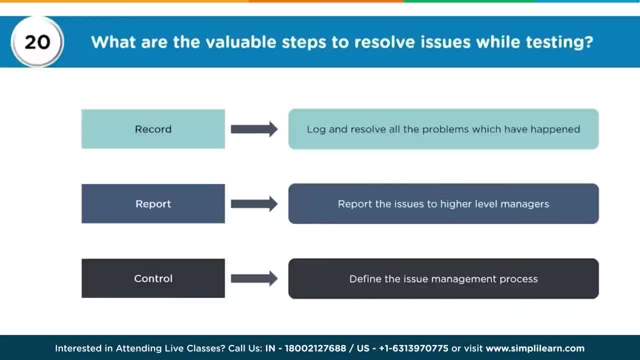 So in the previous scenarios, when we have started testing now, if you find out, when you execute a particular use case, And then you find out of law, what would be the steps that you would utilize to address those particular flaws in those tests? The first step will always be record and you're going to report it and then you're going to introduce a control process for it. 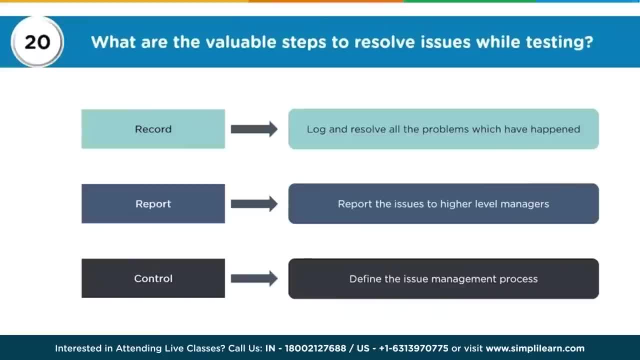 So when you say record, you're going to create Logs and you're going to try to resolve all the problems that have happened. Now, when you say resolve, you're not going to record the application, but you're going to test the system again and again to ensure that whatever is being recorded is accurate. 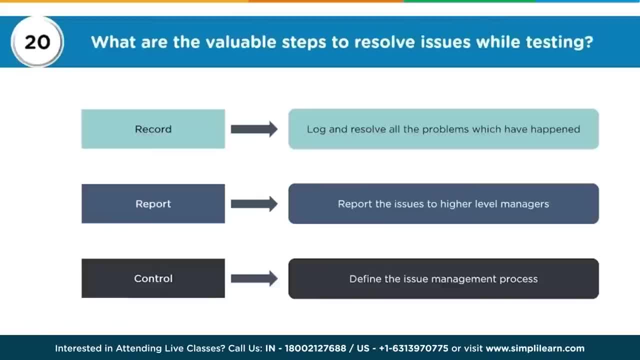 And all the logs, all the error mechanisms, all the dumps, all of those that have been generated due to this particular log of this particular error, are being captured so that they can be reported to the Higher, Higher Level managers. So the next step is, once you have recalibrated all these logs and records, you're going to report them to the higher level managers, who are then going to investigate it and go back to the developers trying to figure out the best way to mitigate those particular flaws. 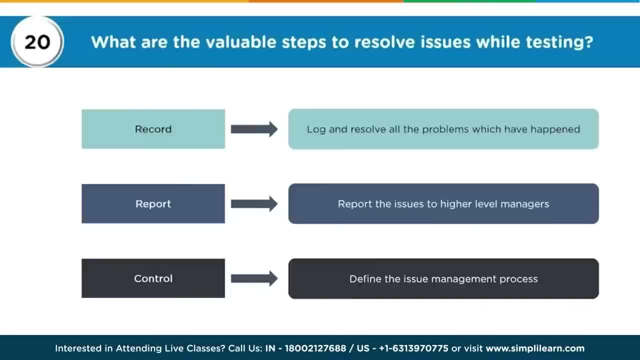 So the report writing needs also also needs to be accurate. It needs to be to the point, It needs to detail what the problem was. It will document all the steps that they were, that you took, all the inputs that you put in, and it will also 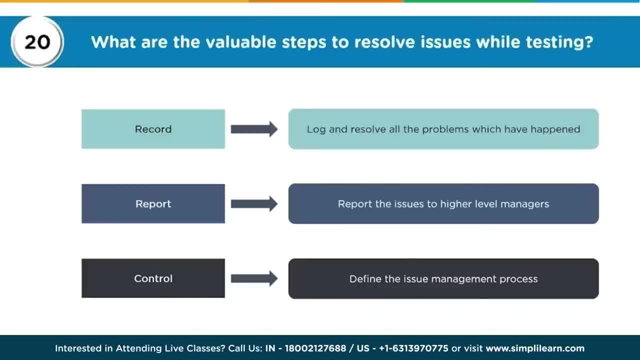 Record all the errors and it will also record all the mechanisms that were utilized and the errors that were generated. and that report will be given to the higher level managers, who can then forward it to the developers who, based on those reports, can draw, start their troubleshooting. and then the control mechanism comes in. you're going to define the issue management process. 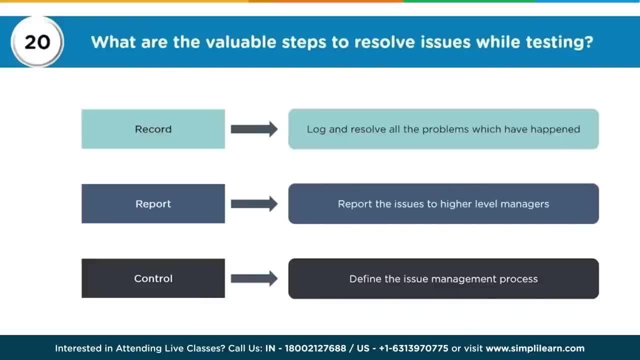 So this process needs to work in a particular manner: where you're doing a test, your recording whatever is happening, you're creating a report, The report out of it, you're sending it to the management. The management will then take those reports, study them, take it to the developers. 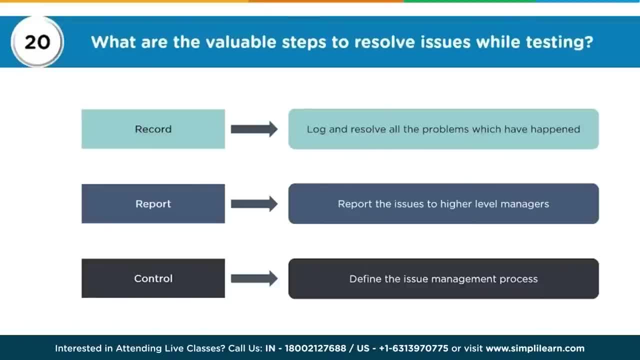 The developers will test based on their criterias. They might interact with the testers at that point in time to identify particular flaws, And then they might want to record that application on a developer patch which, once installed, will mitigate that particular flaw. And then it can come back to the testing phase again, where you can repeat those tests and validate that the flaw is no longer existed. 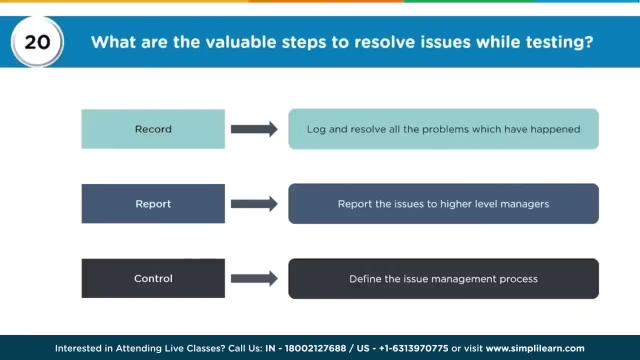 So these are the three steps that would be utilized for testing purposes. And that brings us to the first 10 questions on the software platform. In the next video we'll be looking at operating systems and applications. The first question is on virtual memory. 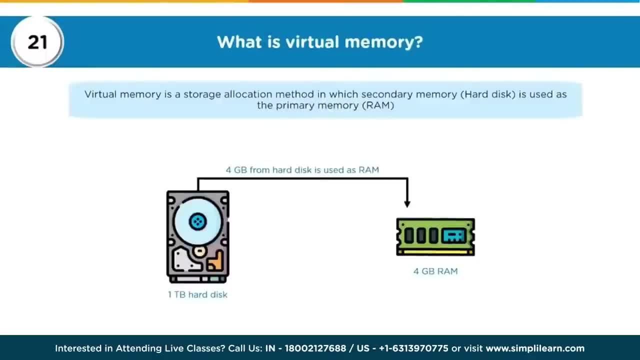 What exactly is virtual memory For a computer? we have two types of memory. First is the primary memory, which is your random access memory, which is also known as a volatile memory, And the secondary memory is your hard disk, Where your data is stored. 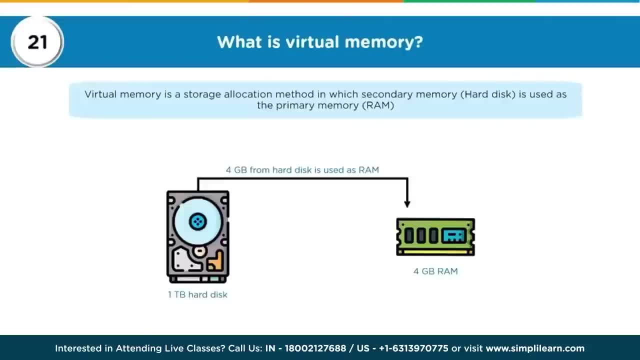 That is stored permanently. But for a computer when it has, let's say, a 4 GB memory or RAM, as in this scenario on your screen, it is going to replicate that and is going to create another 4 GB of virtual memory on the hard disk. 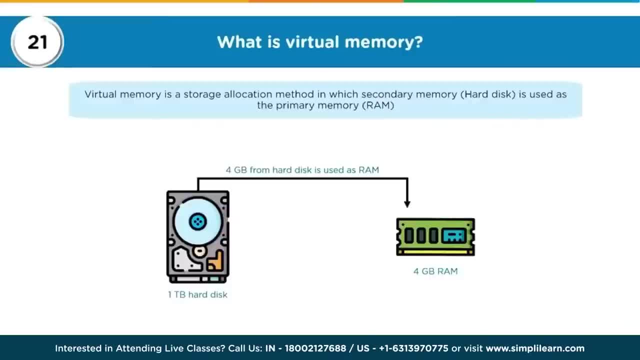 And it is going to use it in tandem along with the RAM. So if the RAM is insufficient, the processor is going to utilize the 4 GB of the virtual memory that is created on the hard disk And it is going to swap data from the RAM to the hard disk. 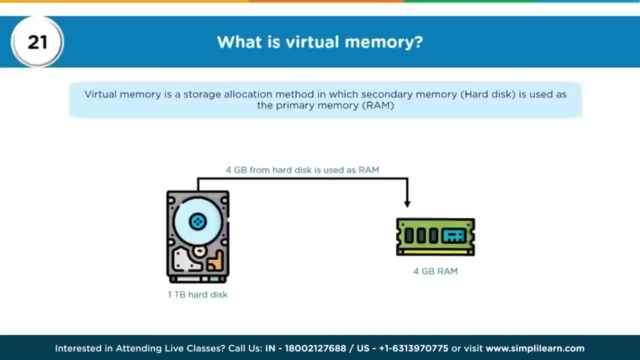 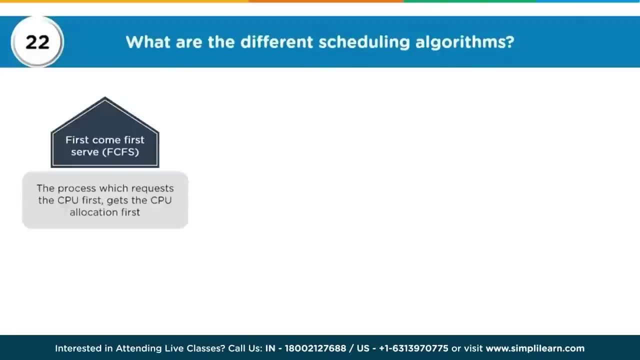 This can also be known as a page file or a swap file. The next question is: what are different scheduling algorithms? Now, the context for this question is: you're talking about a processor and you're talking about how processes are going to be fed to the processor and how the processor is going to treat these processes. 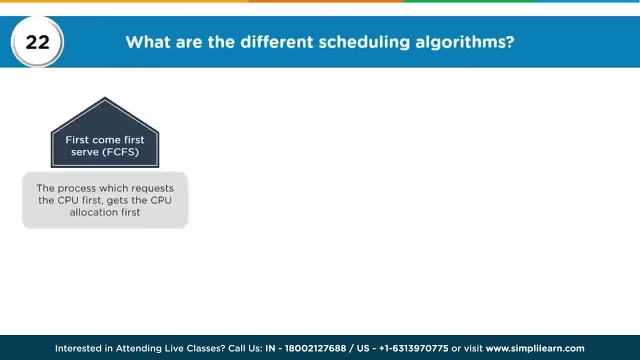 So the first is first come, first serve. So the process which requests the CPU first gets the CPU allocation first. Now, whenever there are processes that are being run by different applications, they make requests for something, Some CPU time. Now, in first come, first serve, the first service or the first process that is going to request some processing time will get that much allocated to them. 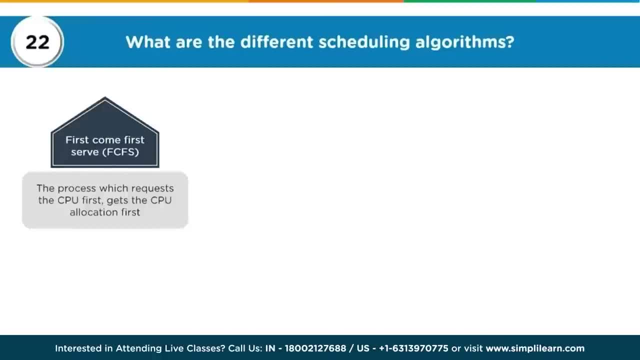 They will run through the process first and then the next, and the next, and so on, so forth. The second one is the shortest job first. This is the process where the shortest execution time for that process is calculated and that process is selected first for the CPU. 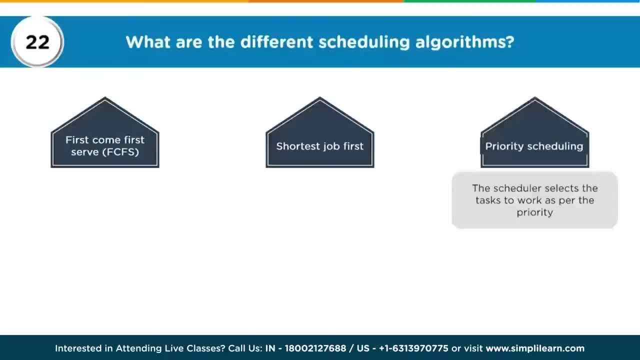 Then there is parity scheduling. This scheduler selects the tasks to work as per priority. So there would be some tasks that are marked with high priority, some would be normal and some would be low. So, based on this high, normal or low priority, all the processes will be classified. 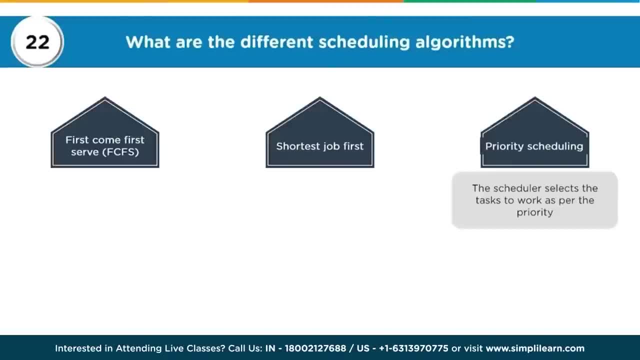 High priority will be dealt with first, then the normal and then the least priority. The fourth option is multiple level queues, where processes are assigned to a queue based on the specific property, like process priority, the size of memory, etc. So it will be classified based on the attributes given to that particular process and multiple queues will be created. 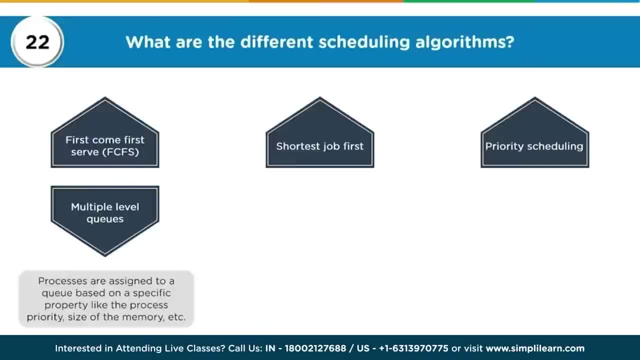 And then, based on the attributes, the processes will be processed by the CPU. Then, shortest remaining time, The process will be allocated to the task which is closest to its completion. So you look at it this way: The process that will take the least time to complete its processing. 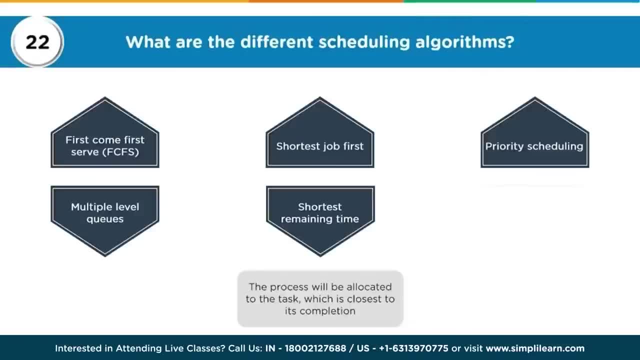 Processing will be chosen first, And then the round-robin method, where each process comes in turn gets an equal share of time. So, if there are 10 processes, each process will be allocated a certain amount of time, after which the next process will be processed, and so on, so forth. 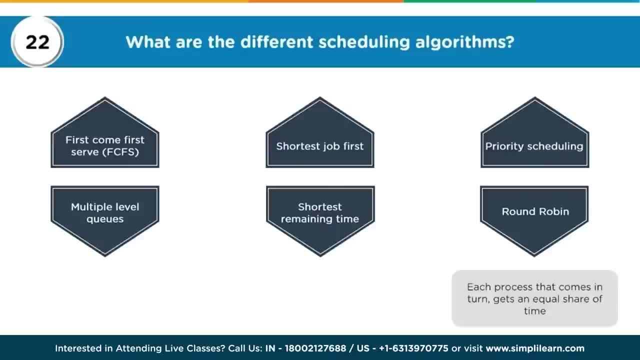 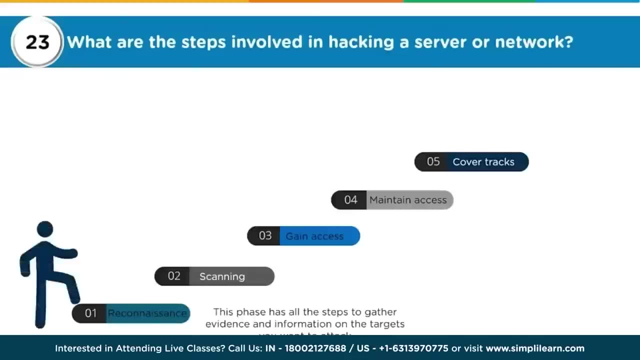 And it will continue in a round-robin fashion till all the processes get executed. So, in short, six different scheduling algorithms, depending on how the operating system deals with it. The next question is: what are the steps involved in hacking a server or a network? 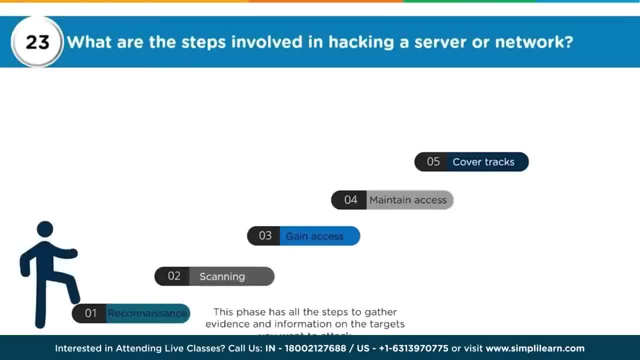 So this is more of an ethical hacking question. You're looking at devices and the interviewer asks you what kind of steps are involved. What are the activities that you would do in hacking a server or a network? Now there are no specific steps that you would define, because every hack is going to be unique. 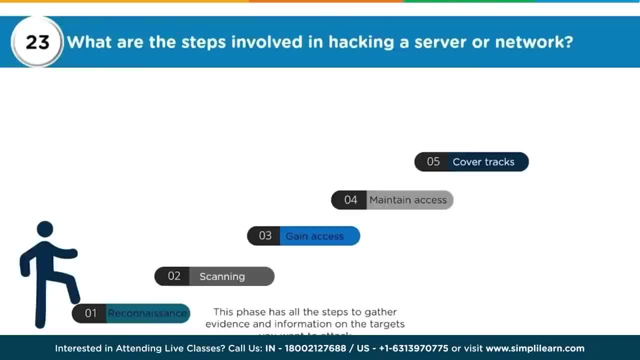 But a hack can be classified in five different steps, which are quite generic, right. So the first step will always be the recognizance step, also known as information gathering phase, also known as footprinting or fingerprinting, depending on what exactly you're doing. 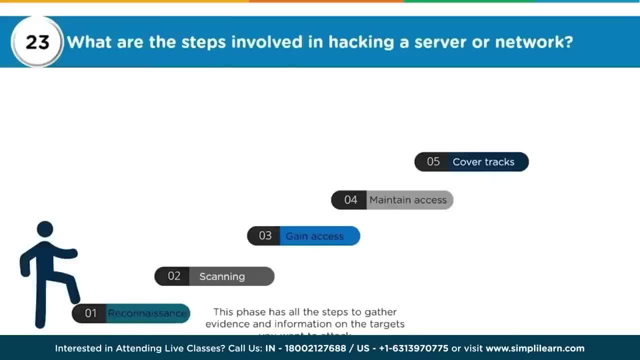 But in this phase the attacker gathers all the evidence, all the information that is possible about the targets that they want to attack. So here you're trying to get to know the victim So you can launch specific attacks towards them. You want to identify what operating system they are utilizing. 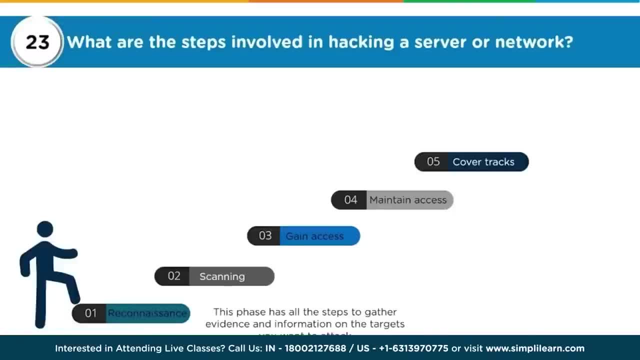 what IP addresses, MAC addresses, the versions of the operating systems and applications, the patch levels. find out vulnerabilities. find out whatever information is possible. find out the information about the person who's using those computers so you can launch social engineering attacks, and so on, so forth. 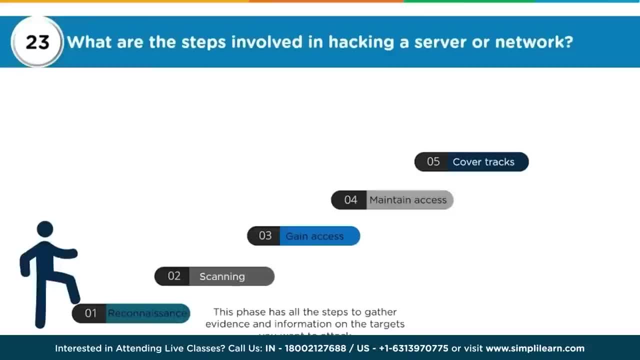 So the first step is all about gathering enough information based on which you can launch further attacks. Once you have that information comes the second phase, which is known as the scanning phase. This is more of a technical phase. So in the first step you've got your IP addresses, domain names. 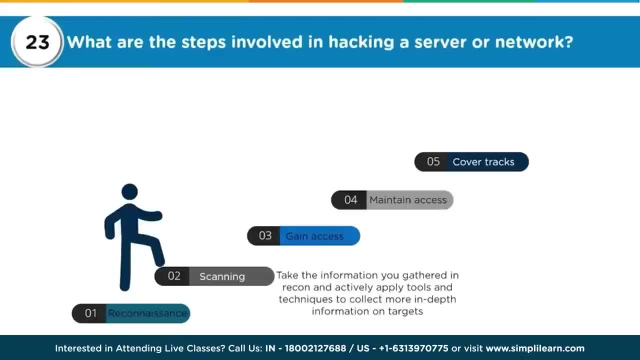 maybe even network maps, and you have identified which devices are available. Now, in the scanning phase, you're going to identify live devices And then you're going to scan them for open ports, processes, protocols, services. You're going to identify vulnerabilities. 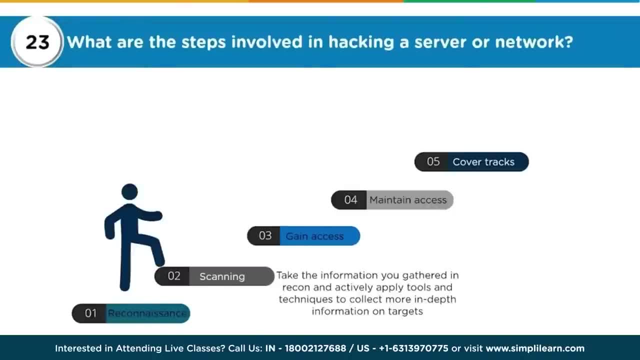 You're going to enumerate them to identify more information, and then you're going to scan them to find out which devices are available from them. Thus, at this point in time, you will have identified a certain set of vulnerabilities or a certain set of security loopholes that you can misuse. 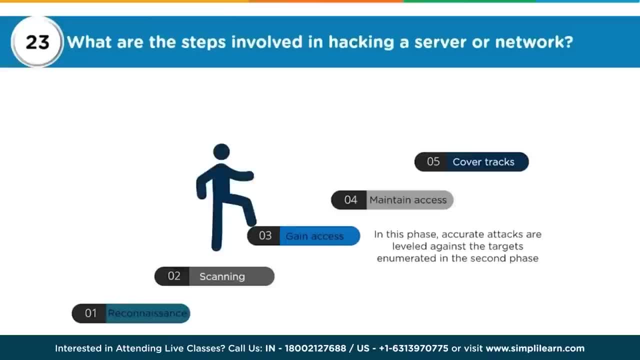 Once you have identified those, you're going to the next step, which is the gaining access step. In this, you're actually going to execute your attacks based on the vulnerabilities that you have found, and you're either going to gain access to that particular system by installing a Trojan. 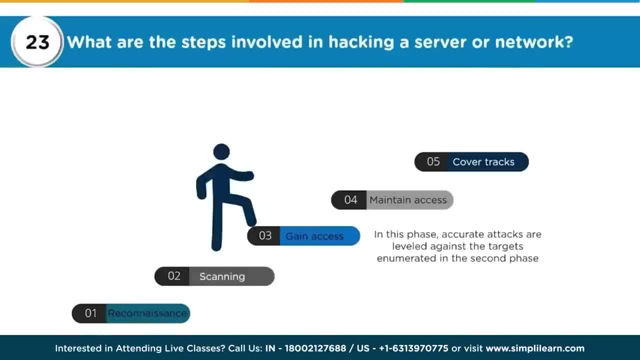 or destroy the system by installing a virus or whatever you wanted to achieve. So in the gaining access phase you would have, based on the knowledge that you have gained in the first and the second phase, you're going to launch your attacks and you're going to try to gain access to that particular device. 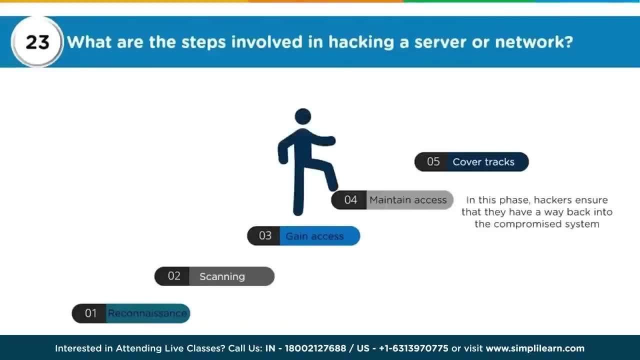 Then the next step is where you're going to maintain that access Now that you have hacked into that device. it is not necessary that you will always be able to get access to that device. Suppose you have cracked the password of that particular user. 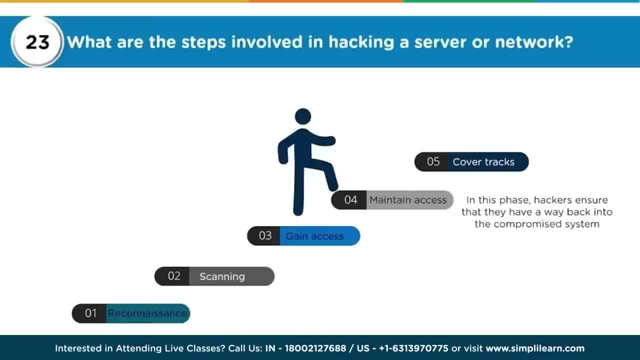 and the user changes that password after a few days, Your attack is worthless. So what you're going to do here is you're going to maintain your access. So this is where it is assumed that you want repeated access to that device, and thus you're going to install a keylogger or a Trojan or some mechanism. 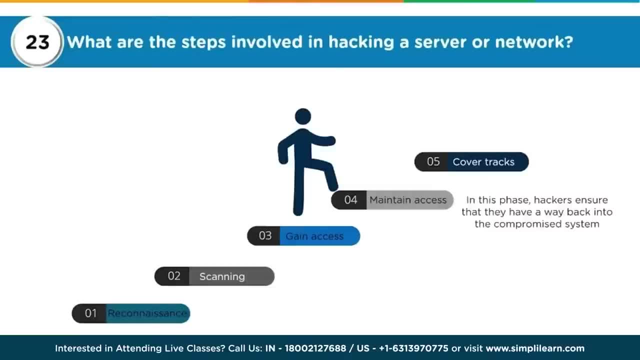 which will still allow you to get access to that device without the knowledge or the authorization of that particular user. And finally, the last step is where you're going to cover your tracks. So whatever activity that you have done so far will have created logs. 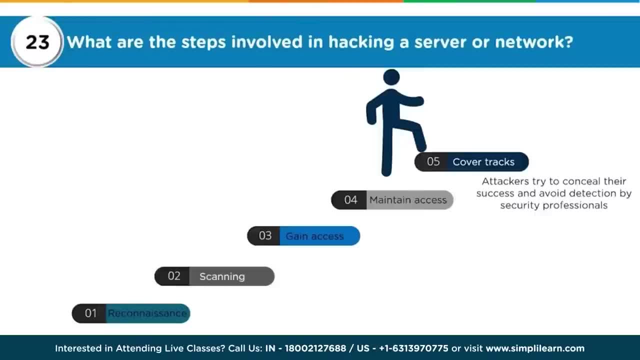 and will have created information based on which the victim will come to know that they have been compromised and may be able to trace that activity back to you. So to prevent the user or the victim from realizing that they have been hacked and to prevent them to discover who has hacked them. 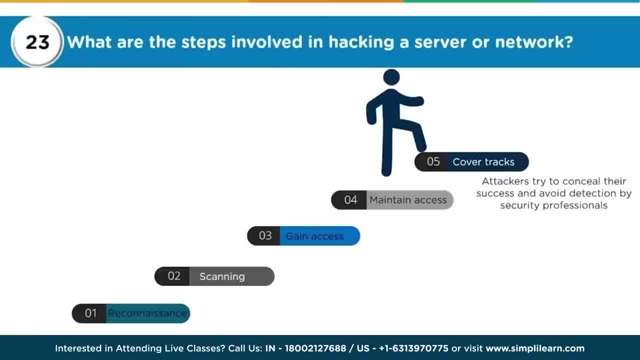 you want to cover your tracks by deleting logs and any references that point to that particular activity. You're going to hide the files that you have created. So you have installed a Trojan or a keylogger. These will create files and directories. You're going to hide them so that they are not discovered. 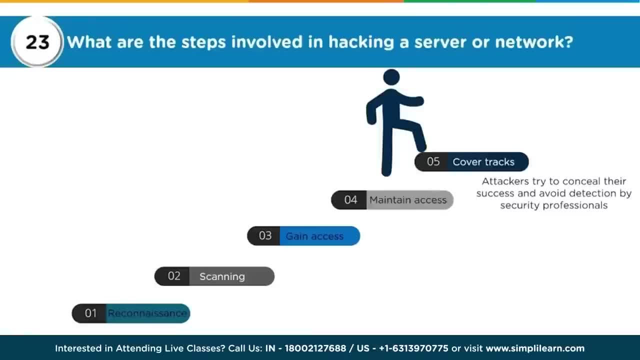 You're going to hide processes that have been created. You're going to try to hide all the activity that you have done so that to conceal the actual attack and preventing the user from realizing that they have been compromised. So these are the five steps that will be involved in hacking a server network application. 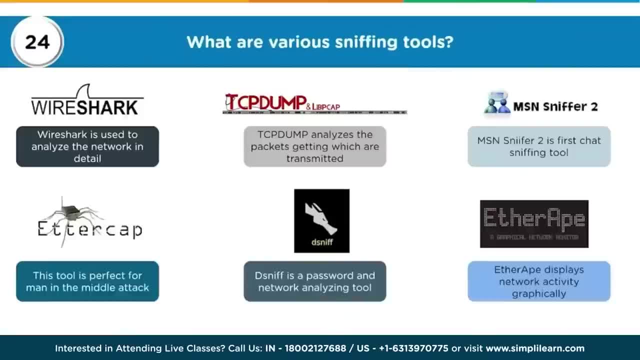 or any computing device you'll come across. The next question refers to what are the various sniffing pools. Now, this is a network-based attack where you're trying to capture data packets that have been transmitted over the network and then you're going to analyze them to see if you can capture any sensitive information. 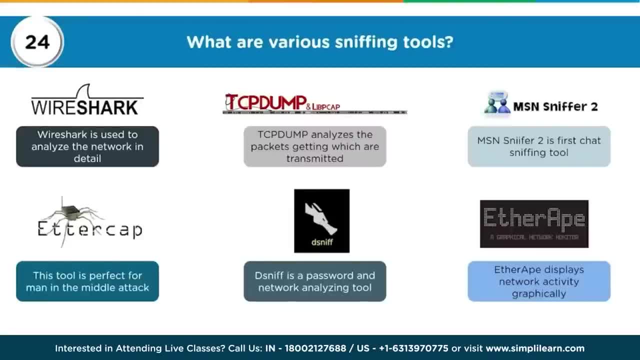 like usernames, passwords, bank details or anything of that sort. Now, these tools will also depend on which operating system you're utilizing. For example, MSN Sniffer would work on Microsoft operating systems, EtherCAT would be based on Linux, and so on and so forth. 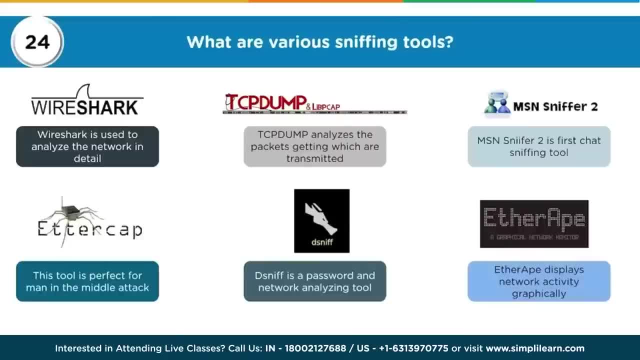 So on the screen you'll see six different sniffing pools that work on different operating systems. Wireshark is something that is common both on Windows and Linux. It is used to analyze network in detail. It is the de facto tool that you will come across in most of your ethical hacking trainings. 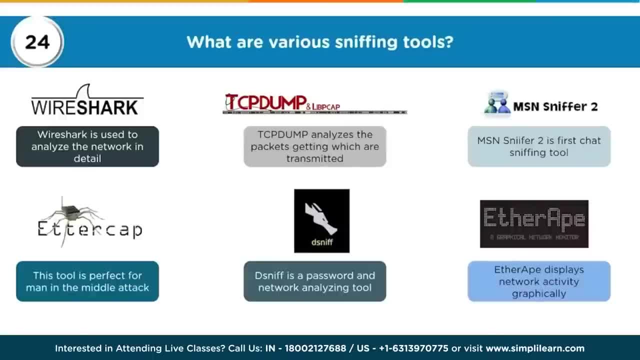 in most of your organizations when they want to do data captures. Now, data capturing, or packet capturing, is not only done by hackers to gather more information, but it is also a known troubleshooting technique used by network administrators to analyze any issues that may be going on in the network. 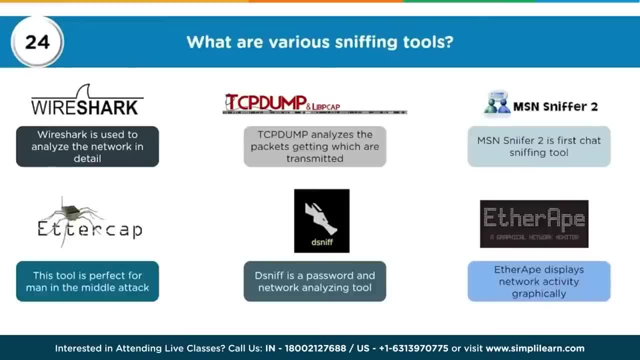 So the first tool you see on the screen is Wireshark. Like we stated, it is available for Windows Linux as well. Then there is TCP Dump, which again has the same capability of Wireshark, but is a command line version, whereas Wireshark also has a GUI. 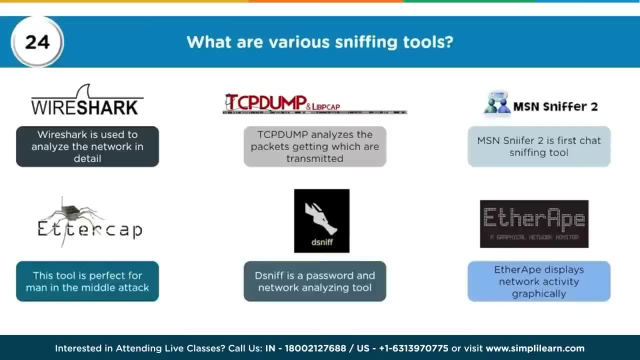 a graphical user interface. TCP Dump is available on Linux MSN Sniffer. it's a very old tool When we had MSN Messengers. MSN Messenger is no longer there, but Microsoft does or did have a Microsoft Message Analyzer tool. 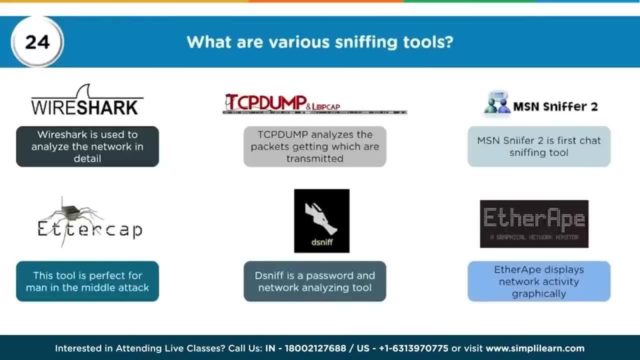 which they have stopped development since 2015.. But that's another tool that is specific for Microsoft operating systems from Microsoft that can be installed to gather more information. Then you've got EtaCAP, which is a tool to launch man-in-the-middle attacks. 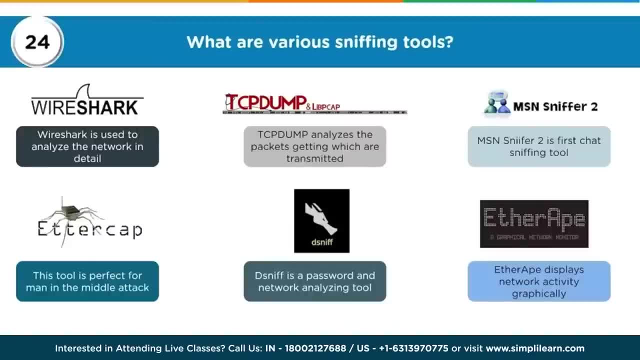 data capturing and is essentially a Linux command line based tool. Then Dsniff is another password and network capturing tool which can help you capture data packets- prominently a Linux tool, Same with EterApe. This is a graphical tool which will allow you to capture data. 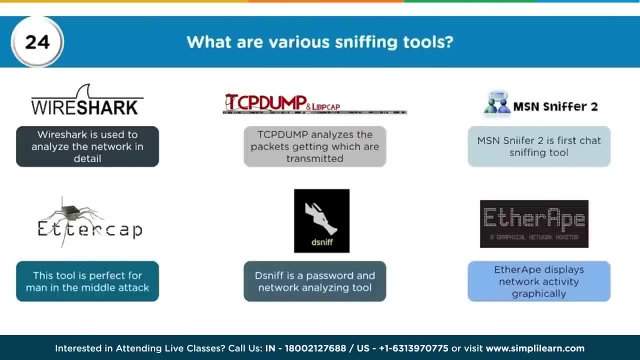 data traffics and map protocols and identify which IP addresses have been communicating with what. Essentially, all of the tools have similar functionality, except that some have additional functionality, like launching man-in-the-middle attacks or capturing, or having specific filters. that will help you identify. 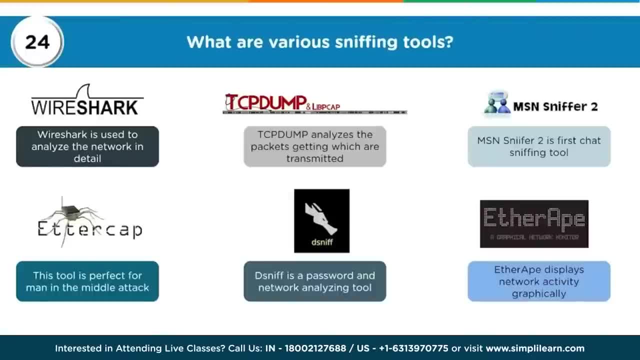 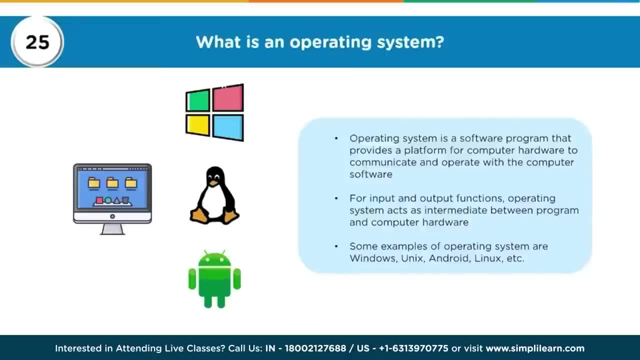 and troubleshoot some network issues that you may be facing. Moving on to the next question, what is an operating system? Now, this is a very difficult question to answer because we normally, when we want to answer this question, we start off with the functionality of an operating system. 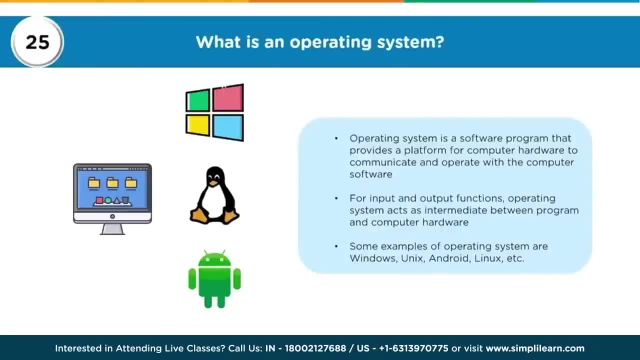 We try to describe what Windows does or what Linux does or what Mac OS does, and then we are trying to figure out what an operating system is in the first place. But an operating system essentially, as the slide says, is a software program that provides a platform for computer hardware. 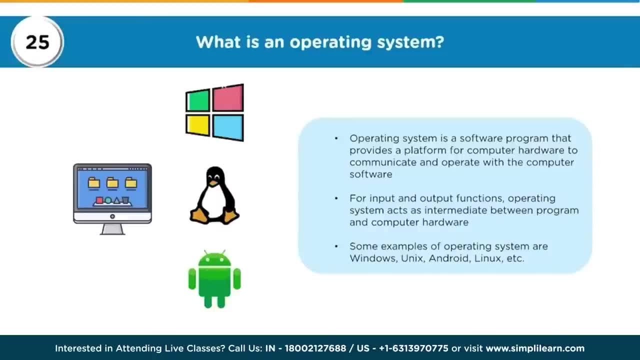 to communicate and operate with the computer software. So it is basically an enabler for human interaction with the hardware that you have. If you take the operating system out of the question, it's just some hardware which cannot interact with you. But essentially, when you have an operating system like Microsoft Windows or Linux or Mac, 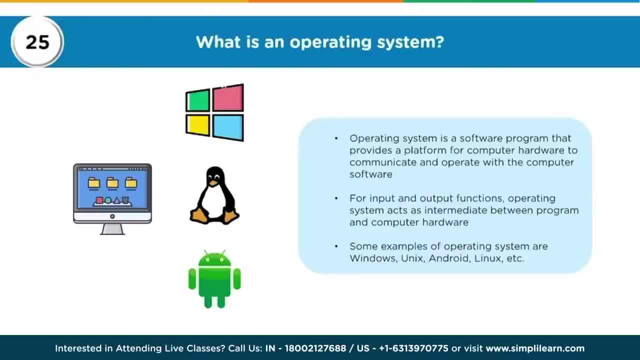 you're essentially installing an instruction system set on that particular device, which will allow you to interact and manipulate the hardware to do whatever you want that hardware to do. Essentially, when we talk about drivers for your various devices, like a driver for your LAN card or for your sound card or for your graphics card, 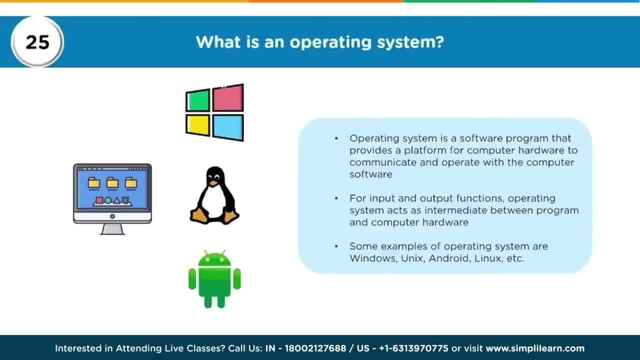 which allows you to tweak these cards for functionality. It allows us input and output functions, For example- the basic example: you open up Microsoft Office products like Microsoft Word or Excel and you get a GUI on the screen which you can interact with. 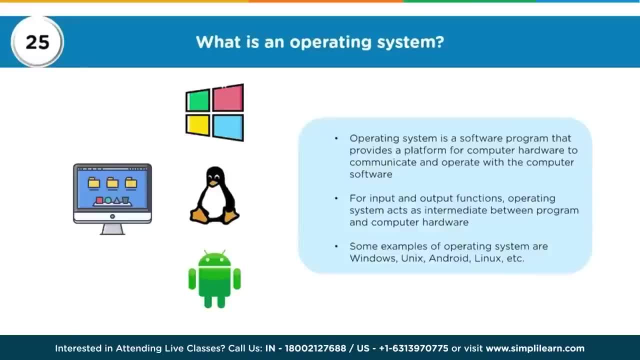 You've got a keyboard and you type on that keyboard and the computer knows what you're typing and reflects those actions on the screen by showcasing it on that particular Excel file or a Word file. So how does the computer know what to do or what you're exactly intending to do at this point in time? 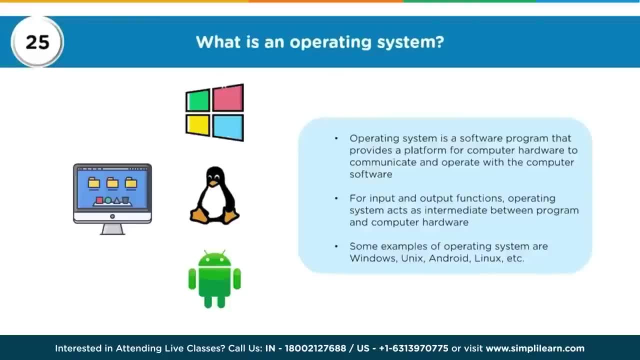 It is all the operating system that is providing you all these services: analyzing what your inputs are and then, based on the programming, it is going to execute that and show it to you on the screen. Some of the most commonly used operating systems are Microsoft Windows. 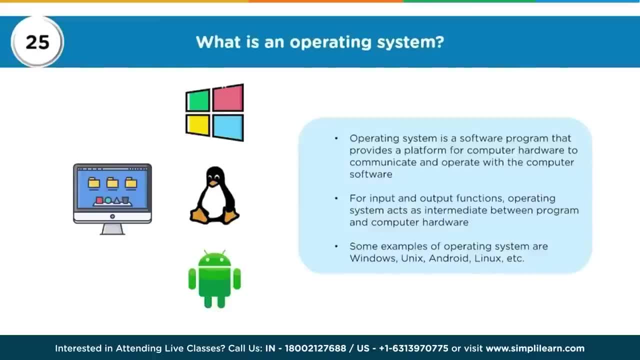 You have them in desktop as well as server variants: Unix, Linux, Again, Linux has desktop and servers. You've got Ubuntu in Linux, Red Hat and so on and so forth, And then you've got Mac OS for Apple related components. 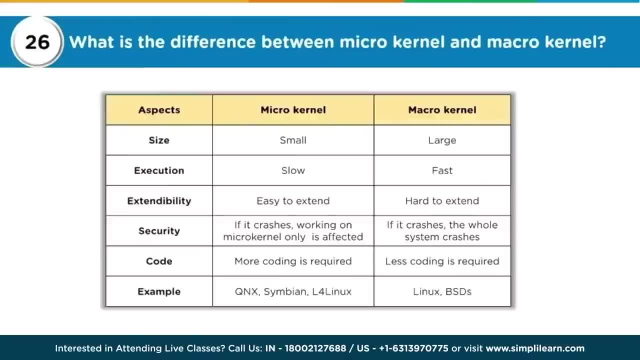 The next thing I want to talk about is the difference between microkernel and macrokernel. The first thing we need to know is: what is a kernel? Kernel is the heart of the operating system that allows that input and output to happen. It allows those drivers to be set up. 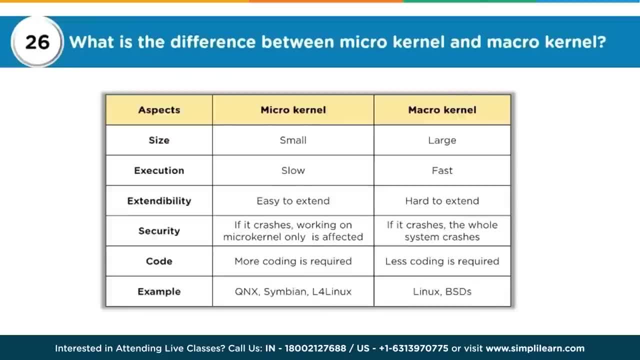 so that the hardware can interact with the software and we can then instruct the software and the hardware both to function in a particular manner. So there are two types of kernels: microkernels and a macrokernel. Macrokernel is something that we know, is something that we normally use. 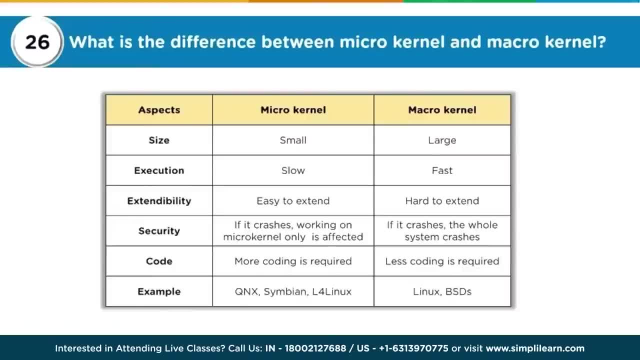 Microkernels are for operating systems that use processes directly handled by the processor. The microkernel is very small in size. Macrokernel is large because it basically is the entire image of the operating system. The execution for a microkernel is slow. The macrokernel is going to be faster. 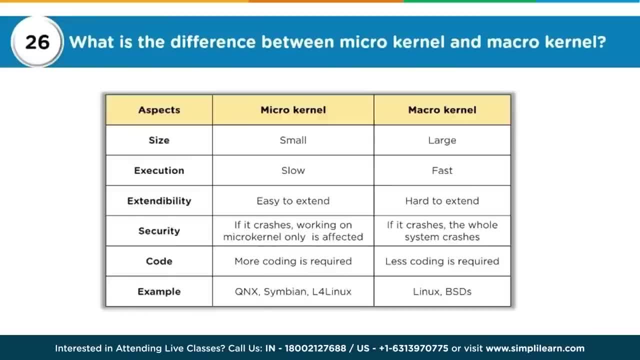 because it is more evolved. There's a lot of programming involved. Extendability: Microkernels are easy to extend. Macrokernels are hard to extend. As far as security is concerned, if a macrokernel crashes, it takes everything down with it. 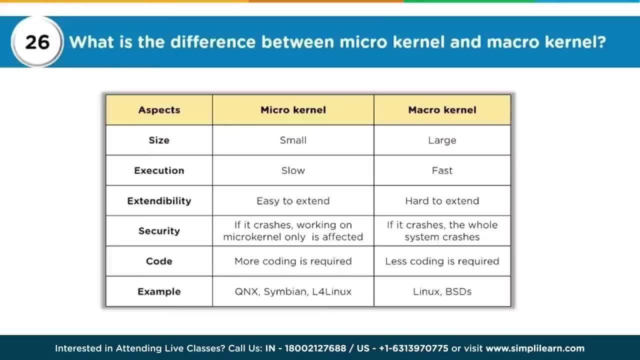 The entire operating system is going to crash. But in case of a microkernel, it is only that particular process that is going to get affected. Microkernel: there is a lot of coding involved. Macrokernel: less coding is involved. Examples of microkernels would be Symbian OSS. 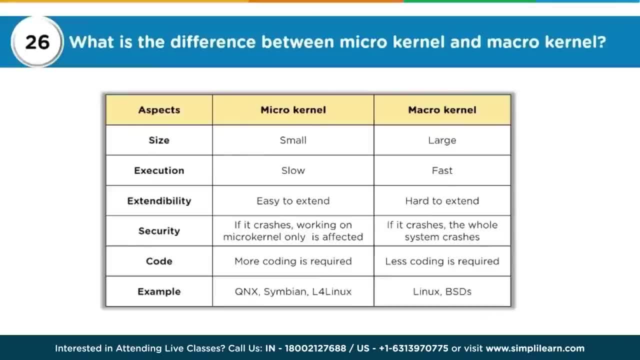 most popularly used on yesteryear phones- Nokias, if you remember those QNX, and so on and so forth. Macrokernels: your Linux or VSD operating systems essentially use macrokernels. Next question: what are the different types of operating systems? 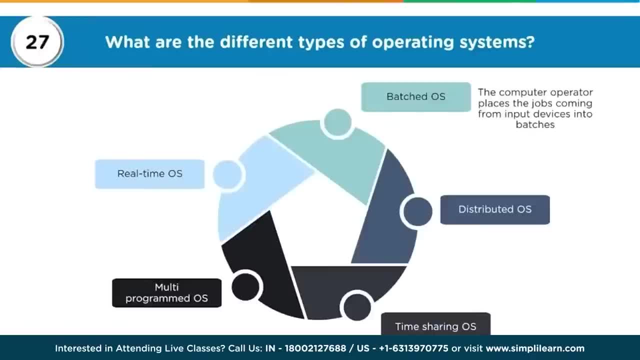 So, as you can see on the screen, five types of operating systems: batched OS, distributed operating systems, time-sharing, multi-program and real-time. What are batched operating systems? The computer operator places the jobs coming from input devices into batches. 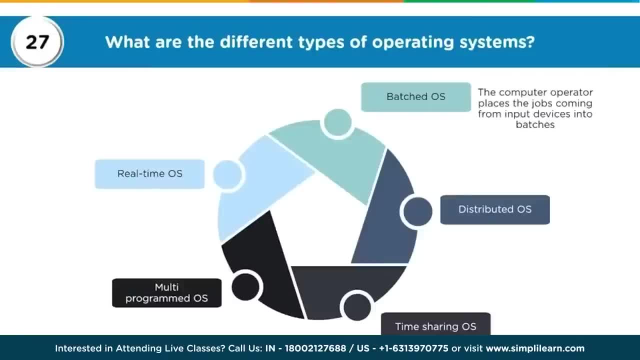 So consider this not from a desktop perspective, but from a server perspective, Where these devices are used by organizations to compute and to crunch some processes. that is going to make some business sense out of it. So when there are multiple processes coming in, multiple jobs that are going to be scheduled, 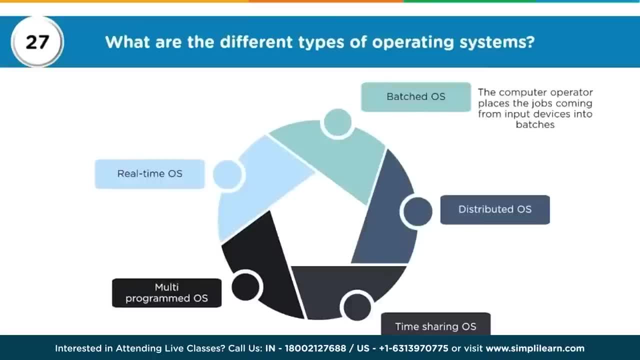 a batched OS is going to place these jobs in batches and they're going to crunch those based on the inputs that have been given by these operators. Distributed OSS, where there are multiple computers which are interconnected and are communicating through networks, So in a corporate environment. 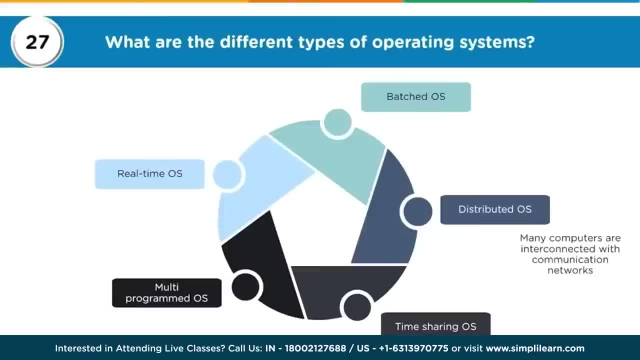 you don't use one single computer to do everything. You've got a data center, and the data center would have a cluster of servers where they're going to share some resources to crunch one particular task right. So that's where your distributed OSS come into the picture. 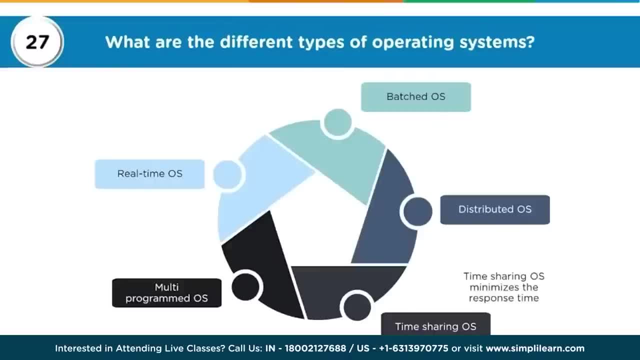 Then you have time-sharing OSS, where you are renting some time. So time-sharing OSS minimizes the response time. Example in today's world: cloud. right, You go onto the cloud, you have a virtual server server, you schedule something. 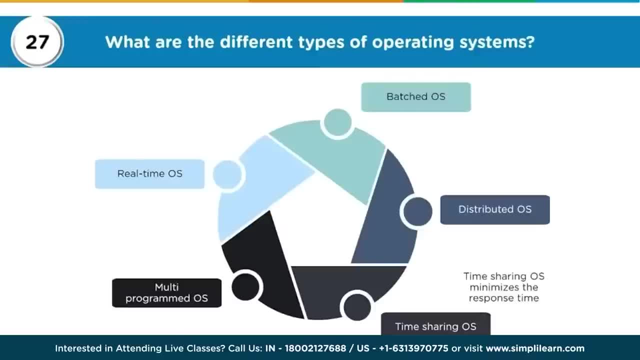 you schedule a job over there, it is executed And, for that time being, that operating system services your particular request and provides you that particular job. Any application that you see online that is executed, for example, Facebook- from a consumer's perspective, 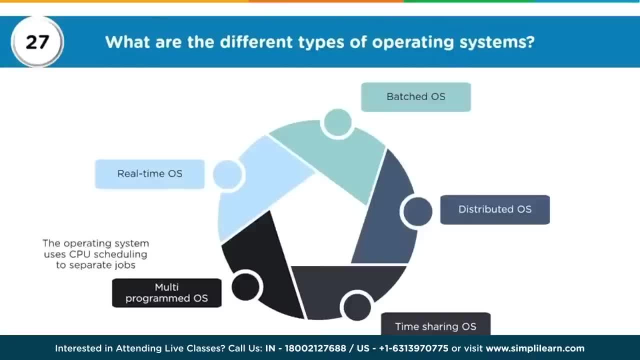 could be a time-shared experience, Then multi-programmed OSS. the operating system uses CPU scheduling to separate jobs. So you're scheduling the CPU to complete certain jobs in this particular manner And in real-time OSS, the operating system gives maximum time to critical operations. 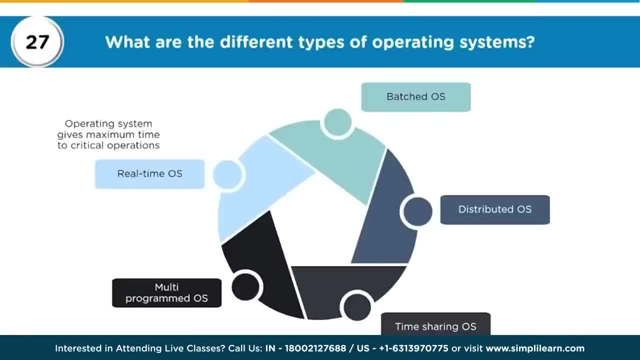 So it identifies the priority of these operations, it knows the high-priority items, the medium low-priority items and, based on that, it is going to execute these critical operations and get the job done. Moving on to the next question, 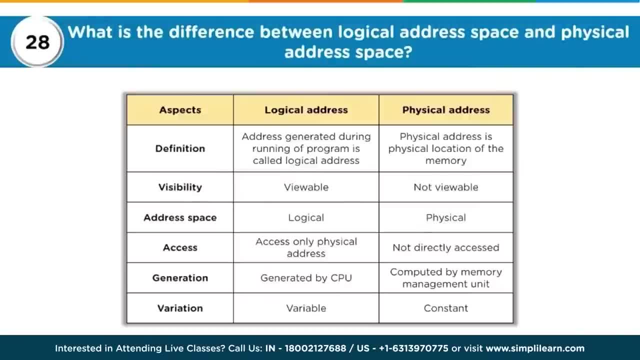 what is the difference between logical address space and physical address space? Now, when you're looking at address spaces, this is where applications come into the picture, And when you execute an application, it is going to create a particular address in the memory, where it is going to create a buffer. 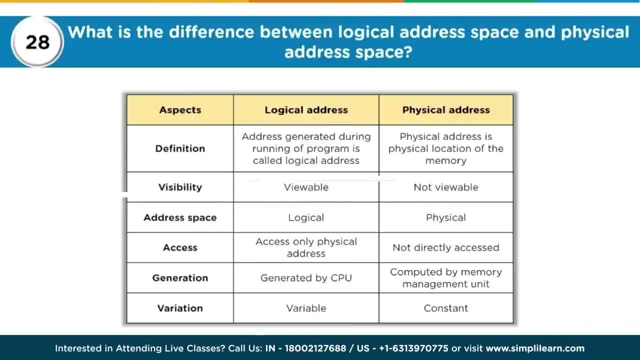 to store its own information so that it can be provided to the processor, processed and then can be returned back to the application as an output. So, as far as definitions are concerned, a logical address is generated during running of an application For a program. 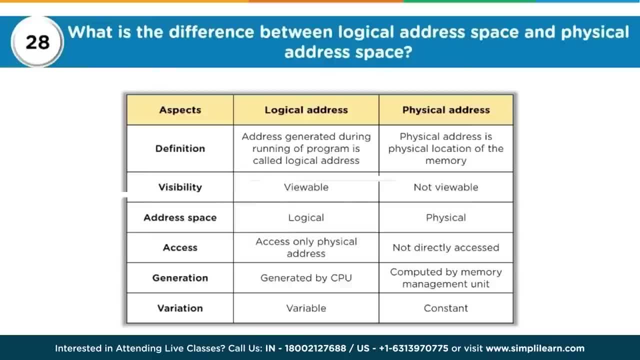 a physical address is a physical address or a physical location on the memory module itself- Right Visibility- you can view a logical address because it is programmed into a computer. So if I'm looking at C, C++ and I'm using malloc or memory allocation, 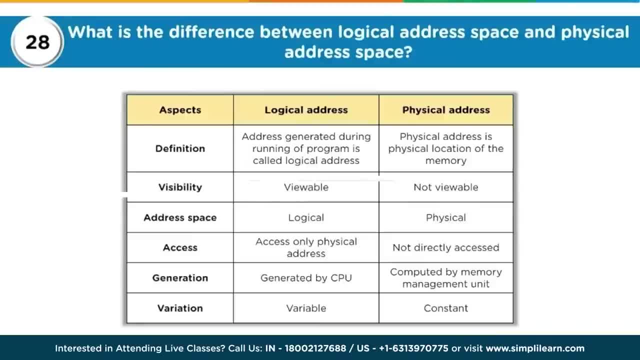 that's where the logical address is going to be created, where a buffer is going to be created for that program and whatever the user input is going to be, it's going to be stored in that buffer. But whereas physical address is concerned, 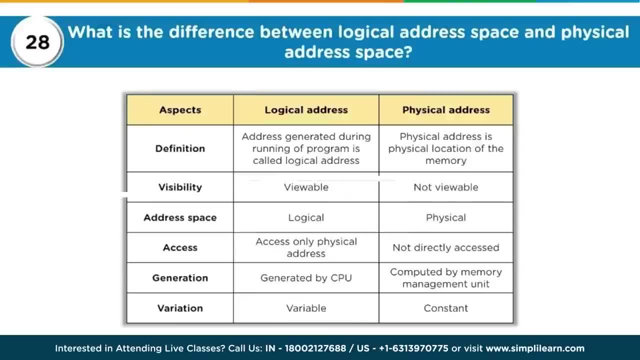 this logical address will be created on a physical store or a physical memory module, which will have its own addressing mechanism. Thus you can see the memory module but you cannot see the specific address on that particular memory module. But as far as a logical address is concerned, 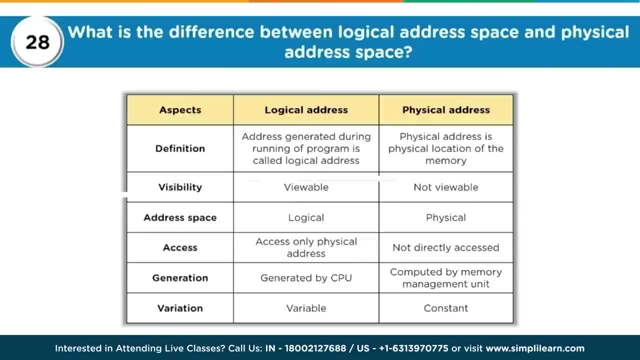 while you're programming or you're debugging the application, it will show you the logical address that has been created- the start point and the end point of the logical address that has been created for that particular program. It can be shown in a debugging environment. 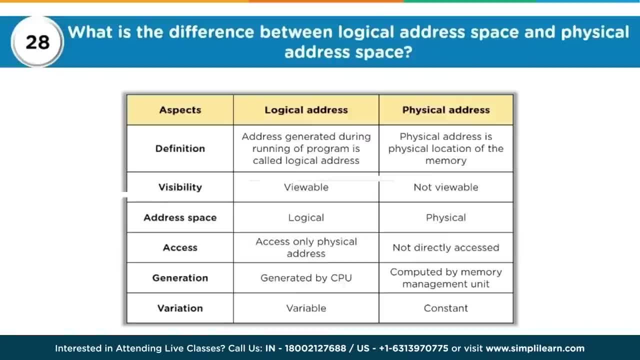 Right Address space logical and physical address is physical. like I discussed, it's the memory module itself. You can access only the physical address on that particular memory because logical addresses can be viewed but you cannot access them physically. Generation: the logical addresses are generated. 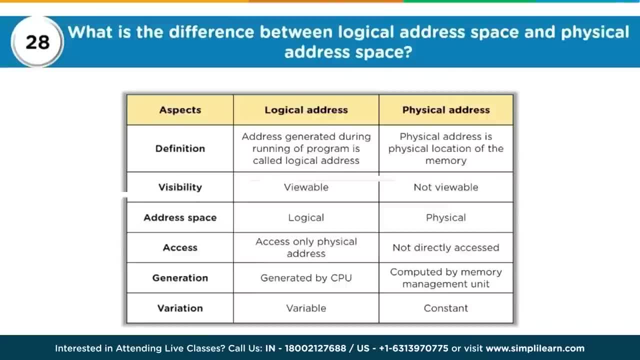 by the CPU during the processing time, whereas physical addresses are generated or computed by the memory management unit or the MMU that you have on your computers. And as far as logical addresses, they are variable, whereas the physical address is always going to be constant. 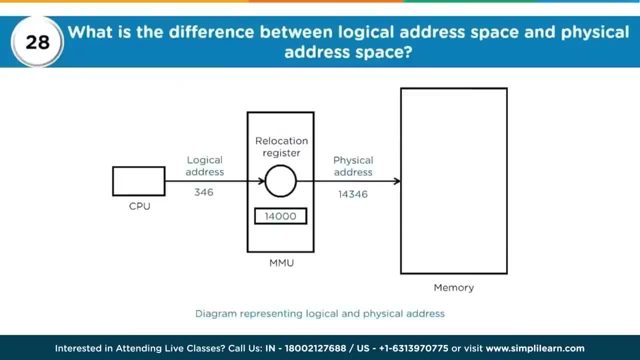 Looking at the next question, what is the difference between logical address space and physical address space? So, moving on from the previous question to this, the logical address is an address created by the CPU for the processes that need to be addressed and that need to be stored as a memory module. 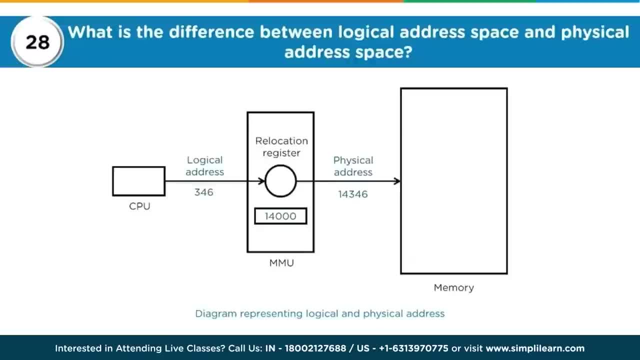 So it's a buffer in the physical memory, whereas the physical memory itself is going to be an address that is going to be there on the physical part of that memory which is going to be assigned to it by the MMU. Then the next question discusses shells. 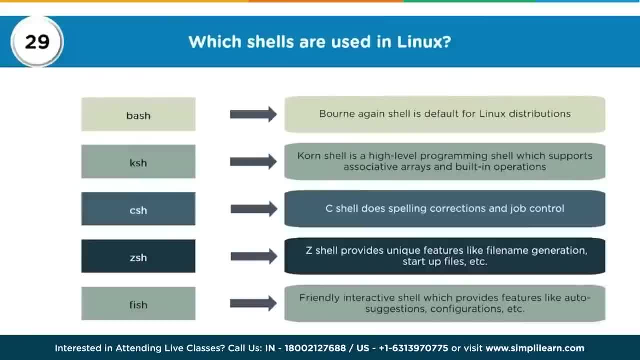 So what shells are used in Linux? Now, what is a shell? Shell is the command line interface that we utilize on a Linux machine, So the terminal window, as we call it, is a shell, And there are different variations of a shell. 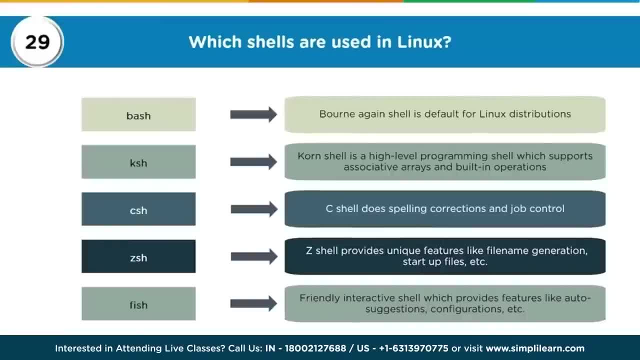 Based on what Linux operating systems you're using- The desktop operating systems that you use or the server operating systems in today's world that you're going to use normally- will always have a bash shell, which is the first shell that you see on the screen. 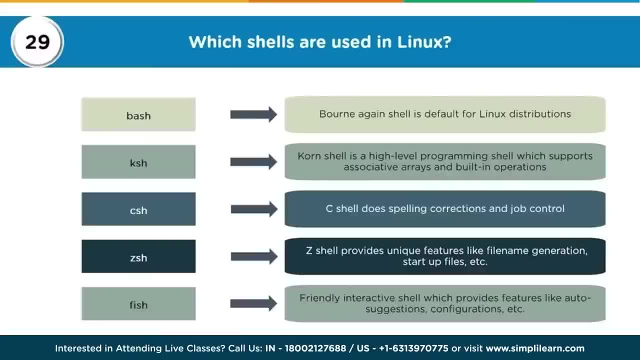 Known as a born-again shell. it is a default for Linux distribution. So as far as end consumers- regular consumers- are concerned, it is always going to be a bash shell, a born-again shell, that you're going to utilize for scripting and to execute regular commands. 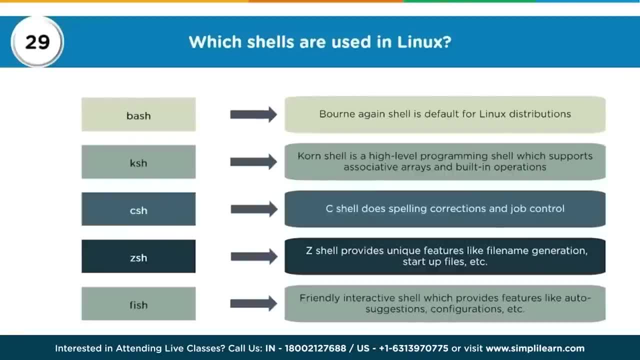 But when it comes to high-level programming or it comes to specialization tasks, then you've got the rest of these shells that you can utilize. For example, the KSH, known as a con shell, is used for high-level programming which supports associative arrays. 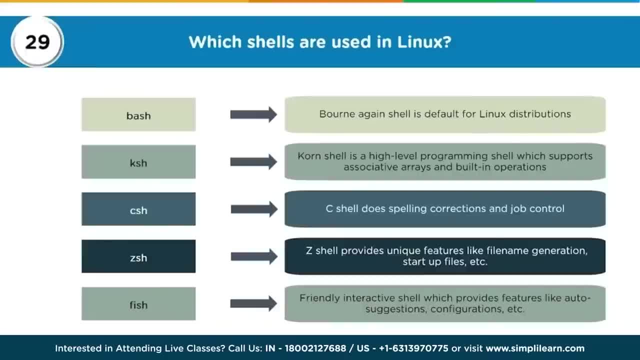 and built-in operations. The CSH or the C shell has different functionality, like spelling corrections and job controls. The ZSH or the Z shell provides unique features like file generation, startup files and FISH. friendly interactive shell, which provides features like autosuggestion. 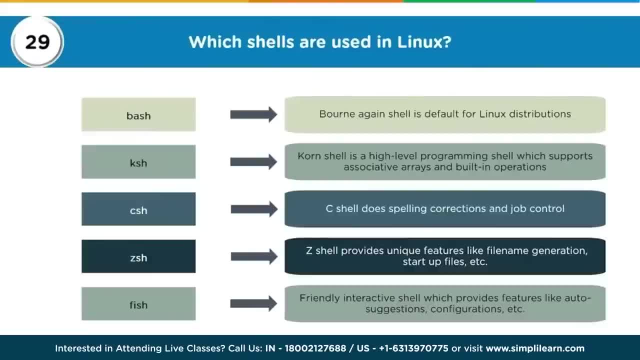 and configuration. So all of these have different functionalities depending on what usage that you have for that particular shell. The most common shell, like I stated, is the bash shell that you'll always come across in your desktop Linux operating systems. Then, looking at the next question, 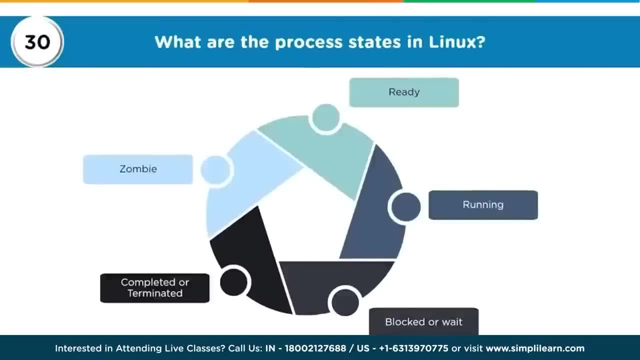 what are the process states in Linux? Now, what is a process? Process is basically a service that is running for a particular application. for that application to function, This process is going to direct user input to the processor process. it get that output back to the application. 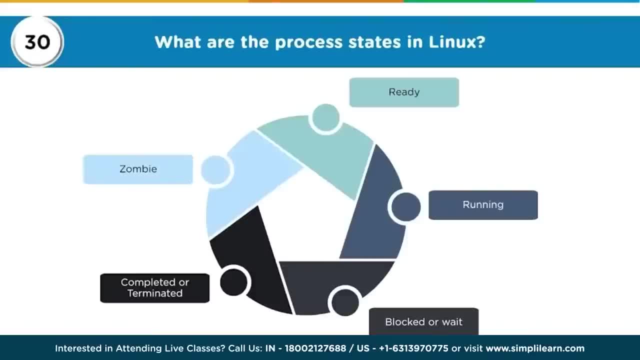 execute it and then show it onto the graphical user interface for the user. So in Linux there are five states for a process. First is the ready space, Now in ready. in this state the process is created and it is ready to run. 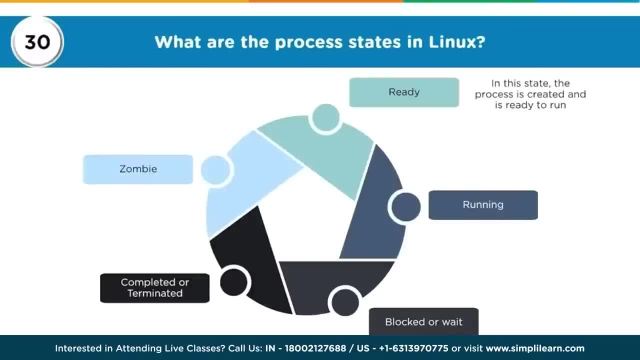 So it is waiting for input. It's ready, the application is executed. The running is when the process has been executed itself, Blocked, or wait is when user input is being looked upon. So it's waiting for user input so that it can do the processing. 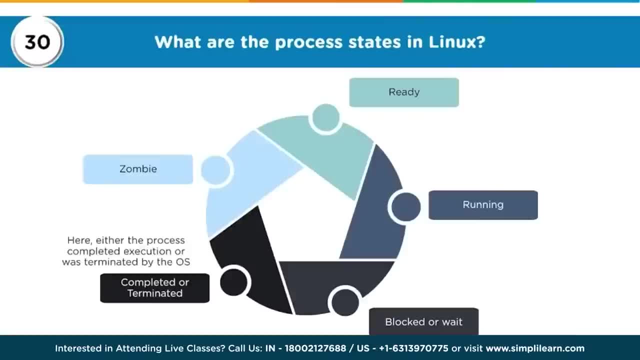 Completed or terminated. it has completed its execution or was terminated by the operating system for some reason or the other. So this is where the processing has been completed And the last state is zombie, where the process is terminated but the process table still holds. 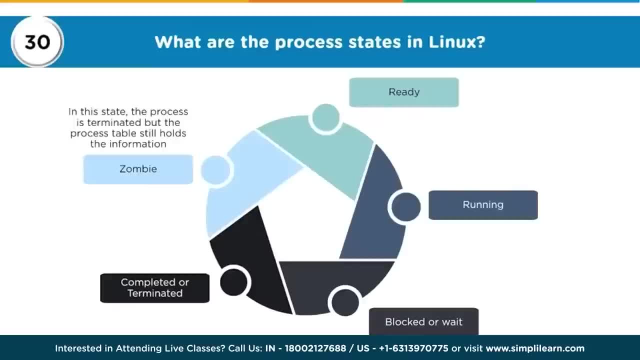 the information. Maybe it is waiting for the kill request before it gets terminated. So these are the five states for a Linux process to be in, And that brings us to the 10 questions in the operating system and application space In the next video. 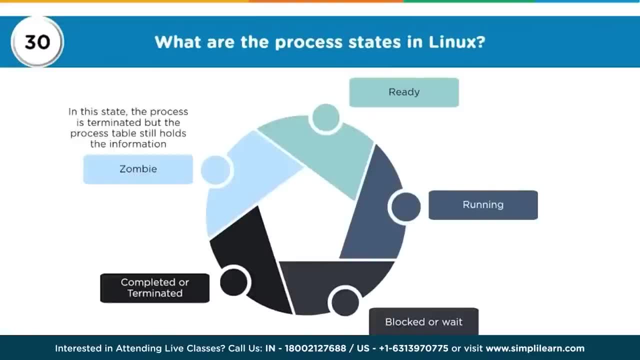 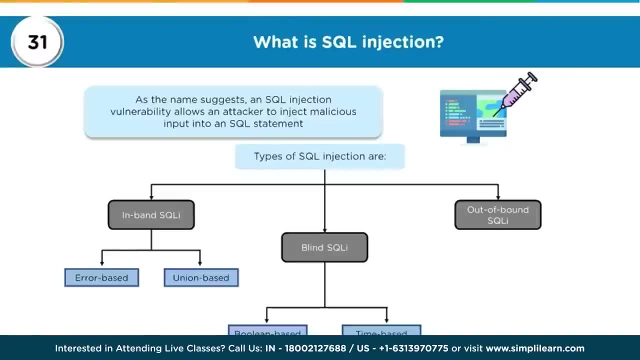 we'll be looking at 10 more questions on cyber attacks. Interview questions based on cyber attacks. Let's start off with the first one. The first question is: what is SQL injection? SQL stands for structured query language, which is a language that is used. 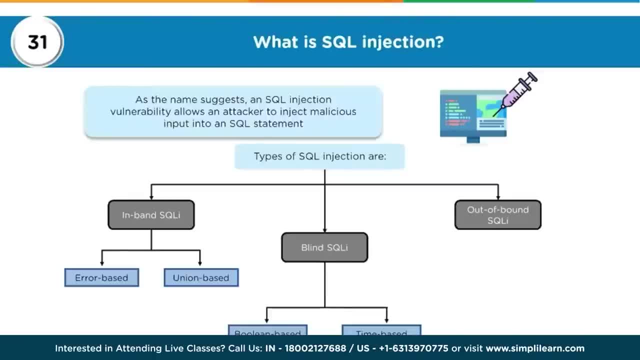 by most of your databases or your relational databases. The variations of your database would be MySQL, Microsoft SQL, Oracle, SQL. You'll have IBM databases. All of these databases utilize the structured query languages to interact with the applications. Now, all of these databases. 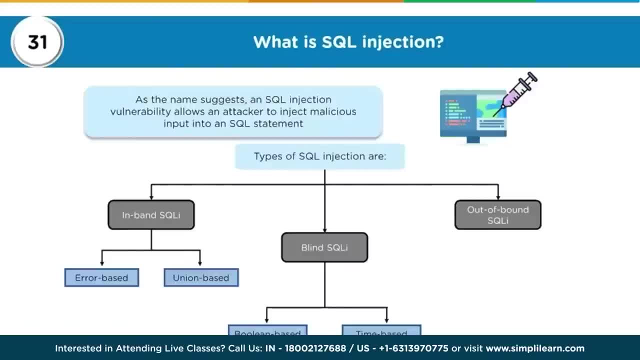 have their own syntax. So we'll have to study most of these databases based on which applications and which databases you want to provide security for. But, as the name suggests, SQL injection vulnerability or structured query language injection vulnerability is where a user can maliciously 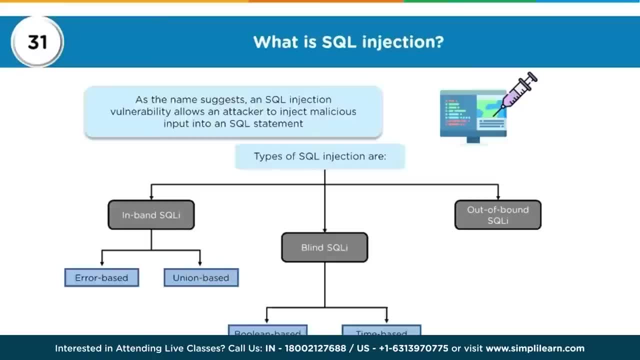 inject a SQL input or a SQL statement in a query and send it to the database and evoke a response out of it. So this vulnerability is not specifically to the database. The vulnerability lies more in the application and the coding of that application. So when the application receives a query, 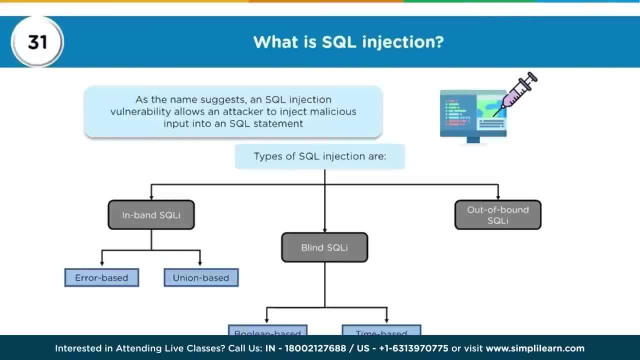 which it needs to be forwarded to the SQL database. we need to configure at the application level of what queries are allowed and what queries are not allowed. So there are different, various aspects of how to manage a SQL injection vulnerability, But the basic flaw lies. 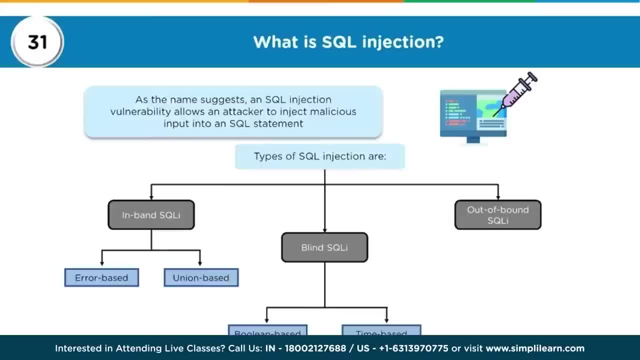 in the application where an invalidated input is accepted and sent forward to the database, where the database might confuse it into an executable statement and thus create a response that was not warranted. There are various types of SQL injections, as shown on the screen: In-band SQL injection. 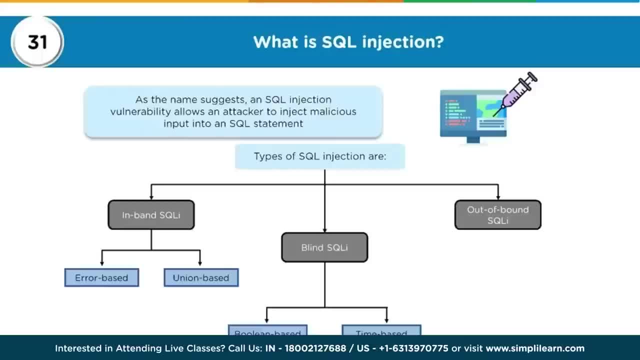 where you can look at an error-based or a union-based injection, A blind SQL injection where it is either Boolean-based or a time-based attack, And then an out-of-bound SQL injection. Essentially, you're looking at databases and you're looking at application security. 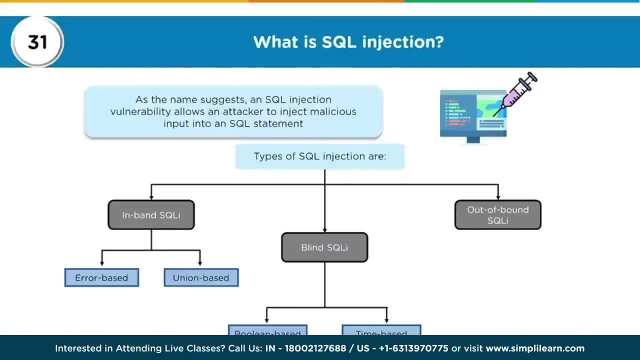 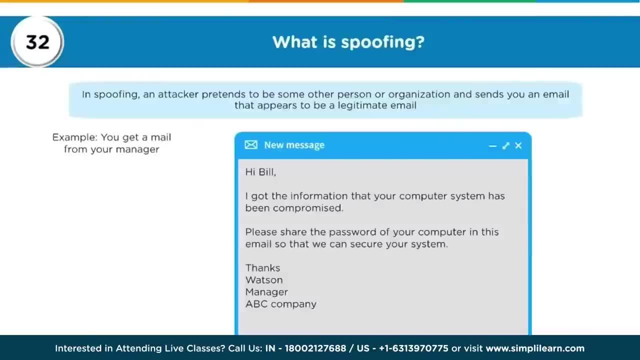 where you want to encourage you to make your coding practices so an invalidated input is mitigated. The next question is: what is spoofing? In spoofing, you're basically assuming the identity of another person. So here the attacker pretends to be some other person. 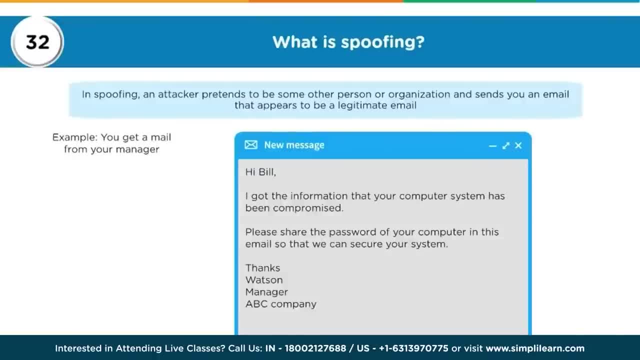 or an organization and sends you an email that appears to be a legitimate email. It looks almost genuine, It has been constructed to replicate what a genuine email would have been, And it is very difficult to spot a fake one. There are different ways to identify whether an email 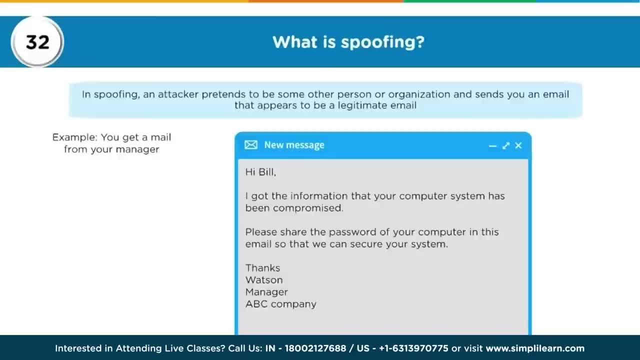 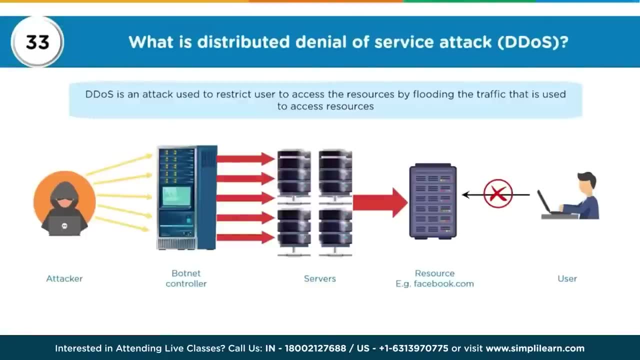 is genuine or not, But that's for a different video. Moving on to the next question: What is a distributed denial-of-service attack or a DDoS attack? Now, generally, a denial-of-service attack is an attack where legitimate users are prevented. 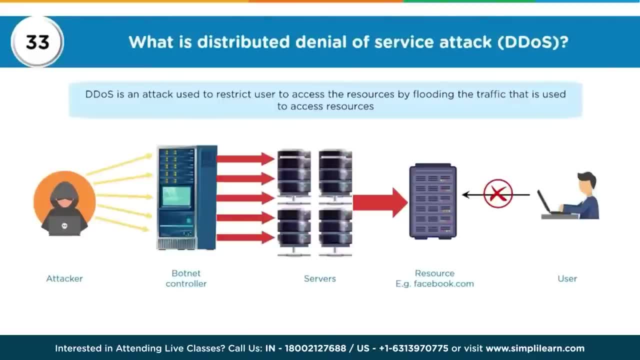 access to the resources that they legitimately can access. So, for example, if it is a bandwidth-based attack, the attacker consumes the bandwidth of the network and the user in such a way that there is no more bandwidth left for legitimate users to access the network. 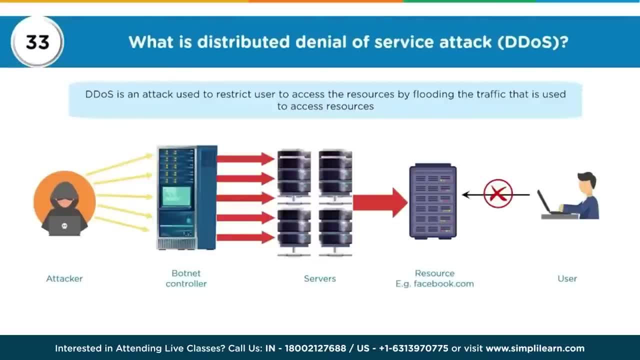 Now, a single device may not be able to generate that much amount of traffic to consume the bandwidth of a huge server. Thus the attacker will construct a botnet and through that botnet they will launch a distributed denial-of-service attack to the target victim. 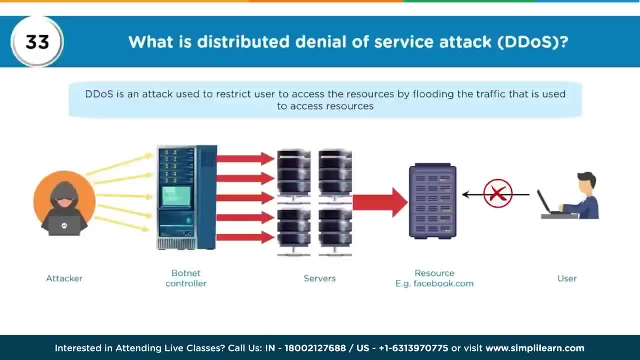 So a botnet. there are two terms that we want to look at over here. The first term is a bot and the second one being the botnet itself. Bot is a software that, once installed on a victim's machine, allows the hacker to send remote commands. 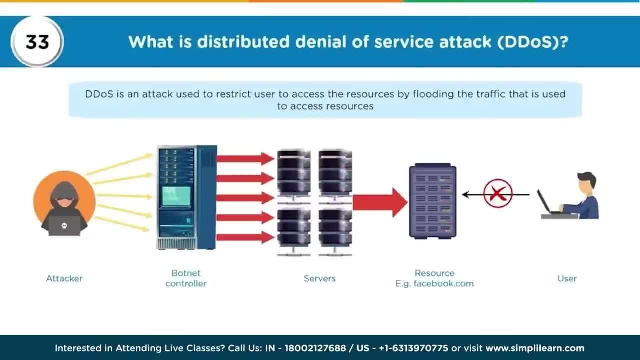 to that machine. that will make it to generate some activity. Once we have enough machines on which such bots have been implemented, the collection of these machines would be known as a botnet, So an attacker will then instruct this entire botnet to start generating data traffic. 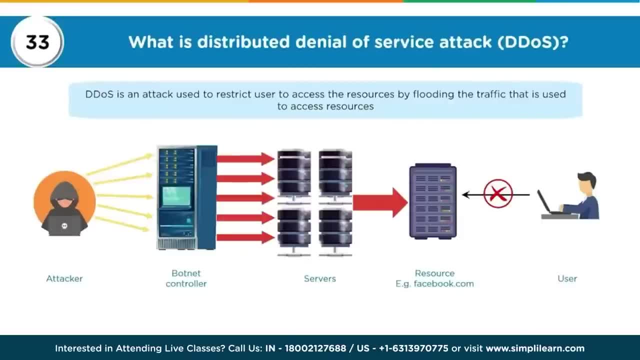 to be sent to the targeted network or to the targeted server, which will then bog down the server, thus crashing it and preventing users from accessing that particular resource. The next question is how to avoid ARP poisoning, or ARP. Now, first let's understand. 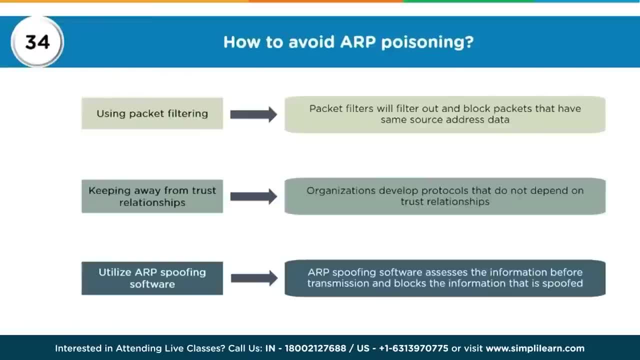 what ARP is? ARP stands for Address Resolution Protocol, which is a protocol used by computers to communicate over the network. Once you communicate with a computer and the computer boots up, it starts a discovery process of identifying its neighbors. So if I'm in a particular subnet, 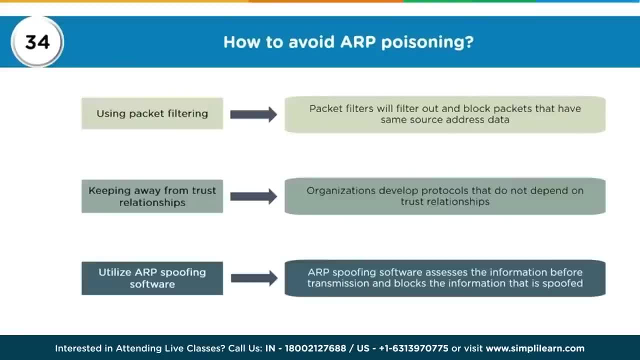 my machine will proactively send out ARP requests and address resolution protocol to find out which other machines are within the same network and which are live. Once it sends out a query, a live machine will respond to that query along with its MAC address. This information is then stored. 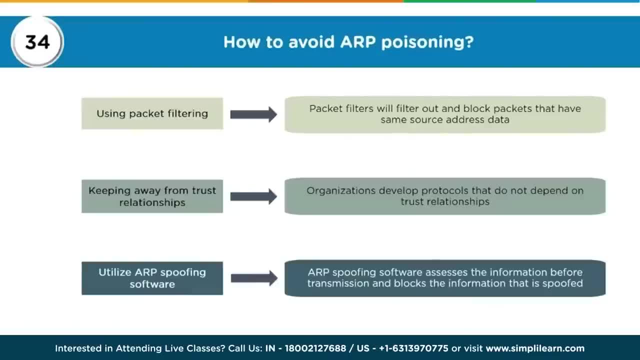 in what is known as an ARP table, or an ARP table on the machine's cache. So whenever my machine now wants to send out a packet to this particular machine, it will go to the ARP table. It will identify the IP address and the associated MAC address. 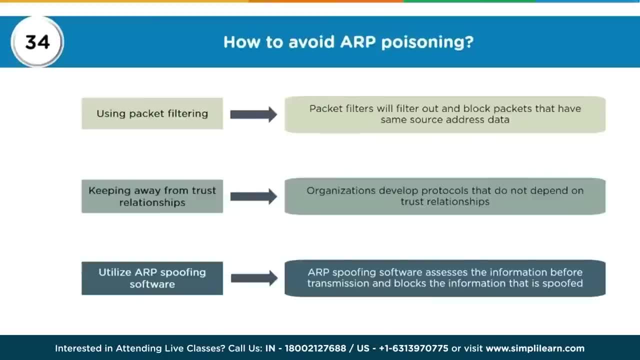 It will print that onto the data packet as a destination IP and destination MAC and send that packet across to the switch. The switch will then identify the MAC address and send the packet to the relevant machine that is connected to that particular switch. Now to confuse this switch. 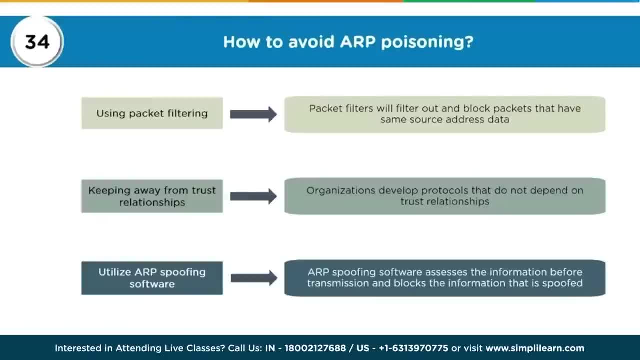 into sending it to a different machine, an ARP poisoning attack is created. This attack is generally launched to create a man-in-the-middle attack. Now, to prevent this ARP poisoning from happening in the first place, there are three different aspects that we can utilize. 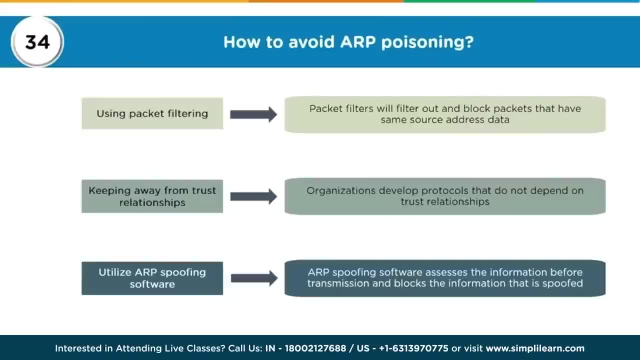 First, we can use packet filtering, which will filter out and block packets that are the same source address data. So you have identity filters and you have identified some malicious IP addresses and you want to block out some IP addresses, So you're using a packet filter firewall. 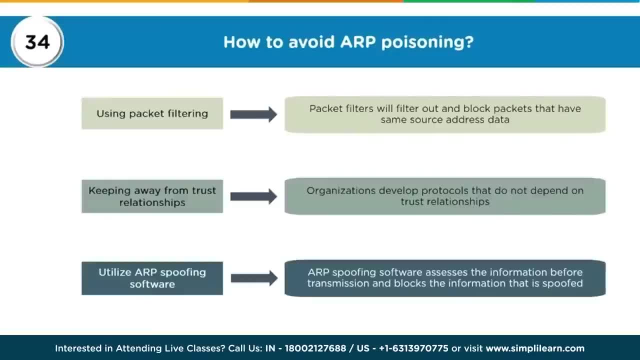 where you have instructed the firewall to filter out certain packets originating from a particular range of IP addresses. This firewall and this technique will then block those kinds of packets coming in. Second, keeping away from trust relationships, Organizations will develop protocols that do not depend. 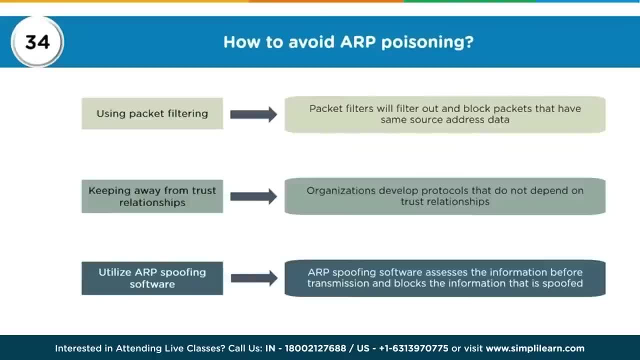 on trust relationships and thus you want to keep this protocol away from you, So you can use ARP spoofing to keep this protocol away from that. Once you have created a trust relationship, these machines should not be sending out ARP requests to other machines. 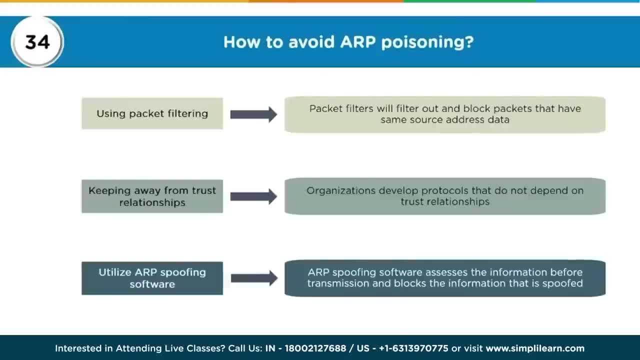 in the first place, Since the trust relationship has been defined and these machines know whom to communicate with. such kind of protocols should then be disabled, Or you can use ARP spoofing software. So there are some. there are softwares out there. 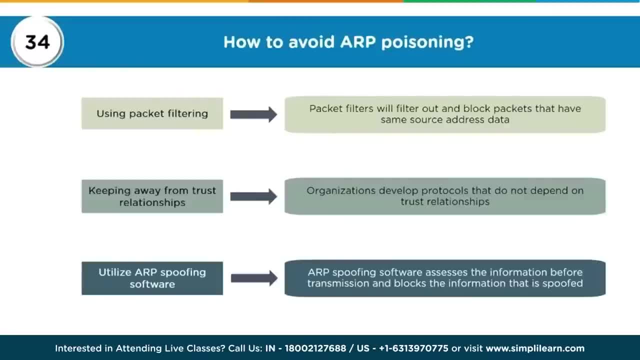 that will look for ARP spoofing and prevent that from happening in the first place. If you send out a spoofed ARP packet, that packet will be picked up by this software and it will be mitigated. Network visualizers like GlassWire, antiviruses. 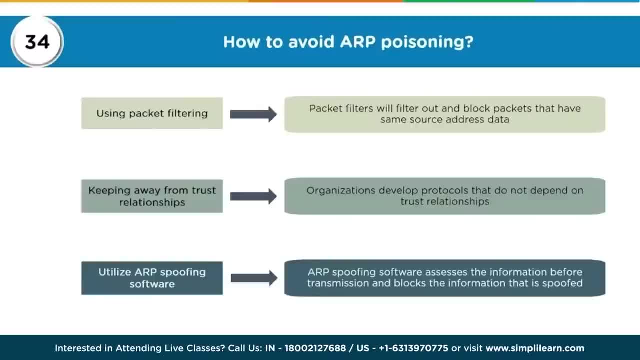 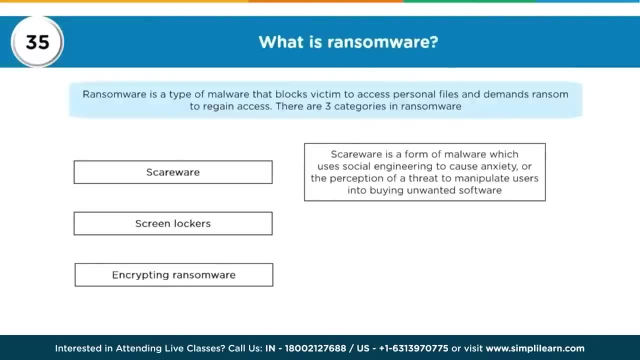 like Sophos, they have inbuilt capabilities of identifying ARP spoofing attacks and mitigate them in the first place. In the next question, we are going to discuss what is ransomware Now. ransomware is a type of malware that blocks victims to access personal files. 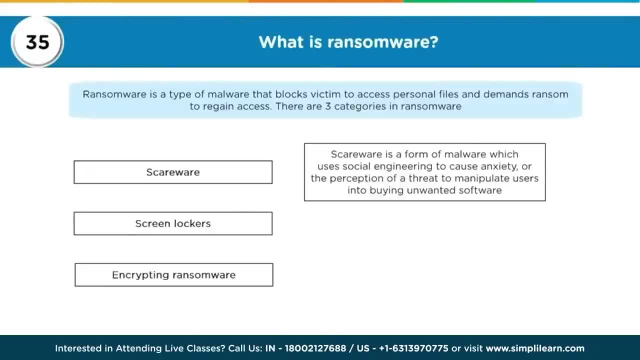 and demands ransom to regain access. There are three categories. Before we go into the categories, let's just revisit what ransomware is. Let's start with the word malware. Malware is a malicious software that poses as a legitimate software but has a payload. 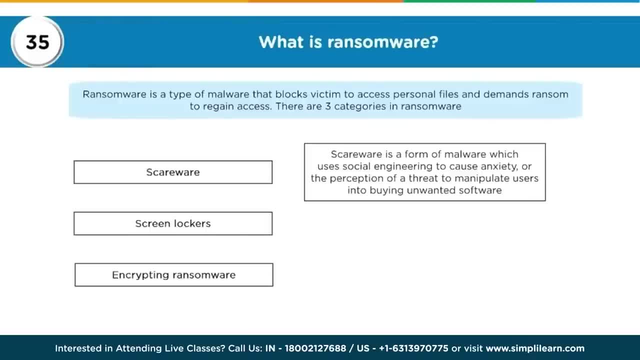 that will have a security impact on your machine. So in this instance, viruses, Trojans- all of these can be classified under malwares. So can ransomwares. A Trojan is a software that will give you a backdoor access to a particular device. 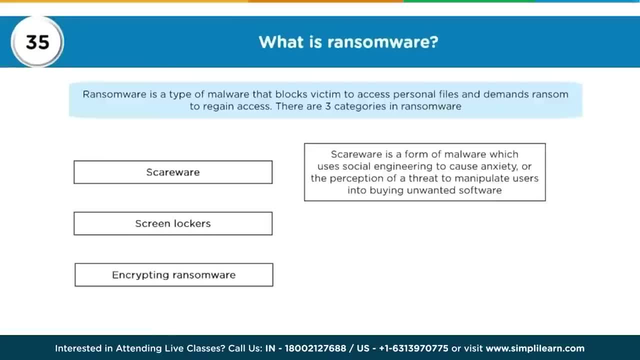 A virus will do some destructive activity on that device. A ransomware will basically encrypt the data of that particular user on that particular machine, thus rendering that data inaccessible to the users themselves, And in turn will demand a ransom to provide access to that particular. 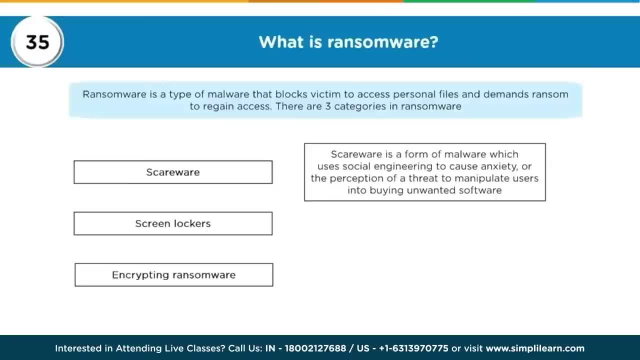 data. So the three types of ransomwares: the first one is scareware, which uses social engineering to cause anxiety or the perception of a threat to manipulate users into buying unwanted software. So this preys on the gullibility of humans. 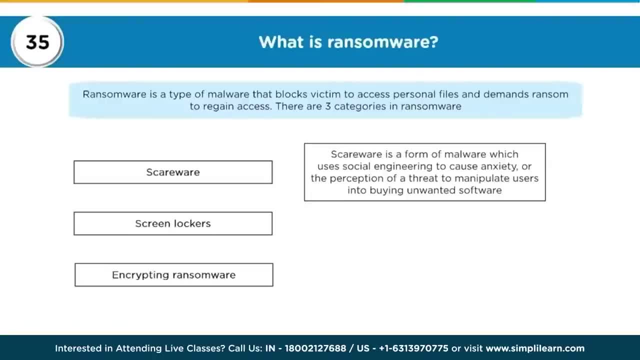 where you can see a pop-up appearing on your screen which can scare you into believing that you may have been attacked or there is a virus on your machine and then instructs you to download a particular software to mitigate that particular virus. Now the malware. 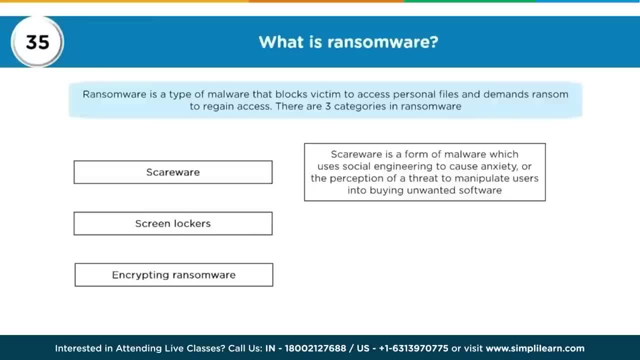 will be in this software that you will be downloading and then ransomware will be installed on your computer where locking users' computers by preventing them from logging in and displaying an official looking message. You will see a screen saver once you boot up, which prevents you. 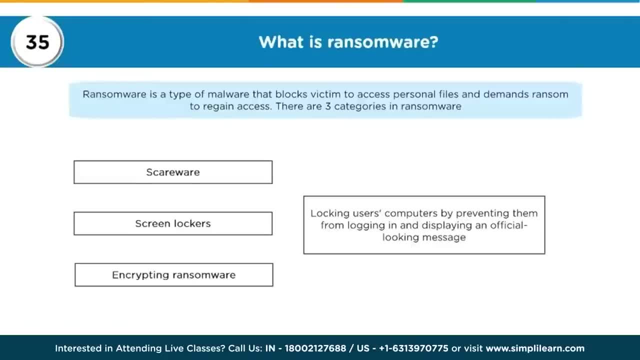 from accessing the login page, so it will not allow you to log into your own machine, but it will give you a warning that your data has been encrypted and you need to connect to a particular email address and send bitcoins over there to get a decryption key to access. 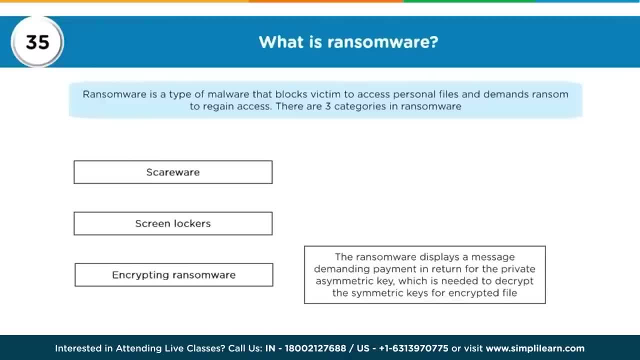 your data. This displays a message demanding payment in return for the private asymmetric key which is needed to decrypt the symmetric keys for encrypted file. So once your files have been encrypted, you might just have a blank screen in front of you where you will receive a warning message. 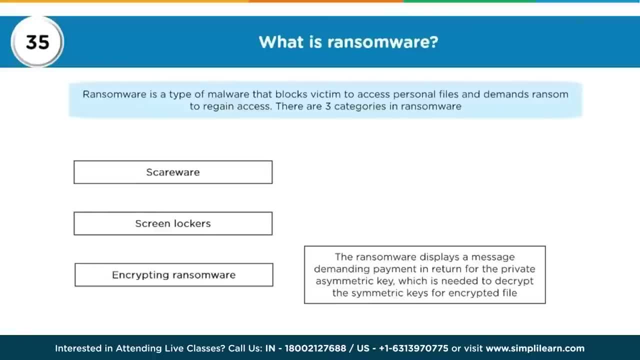 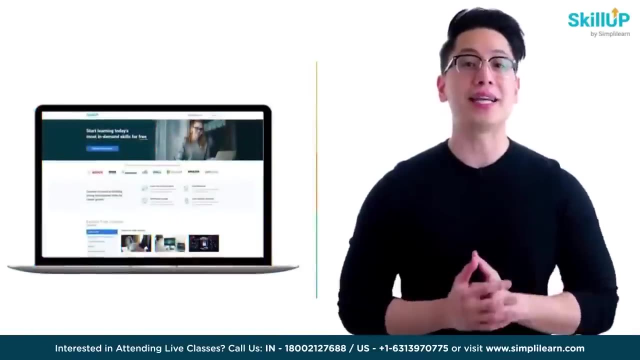 where it instructs you to pay up a ransom in bitcoins or in some cryptocurrency to some particular digital e-wallet which is not traceable and once you make that payment, they will send you a warning message telling you that your data has been decrypted and you need. 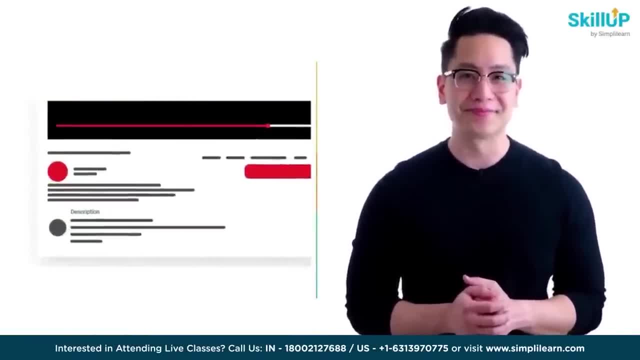 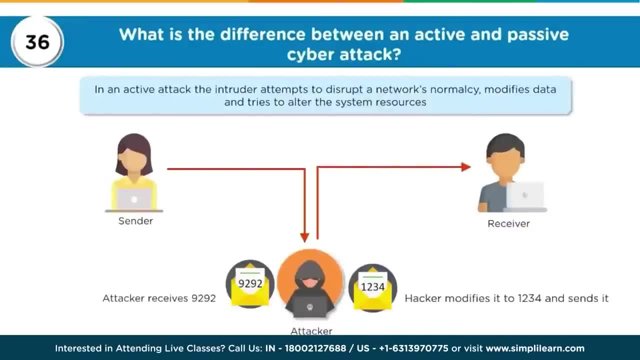 to pay up a ransom in return for that payment. If getting your learning started is half the battle, what if you could do that for free? Visit SkillUp by SimplyLearn. click on the link in the description to know more. So let's get started. 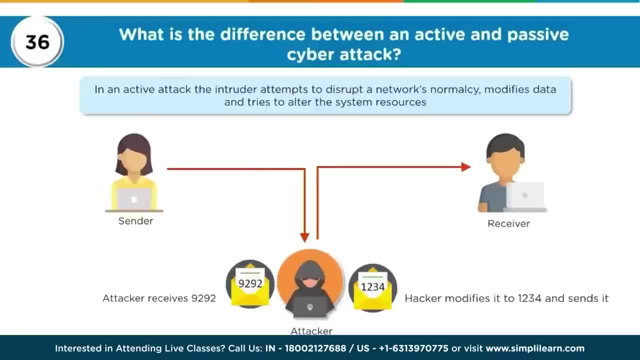 So in this video we are going to talk about how to decrypt a ransom in a way that can happen. it's either in an active manner or a passive manner. In an active manner, the intruder attempts to disrupt a network's normalcy, modifies data and tries to alter. 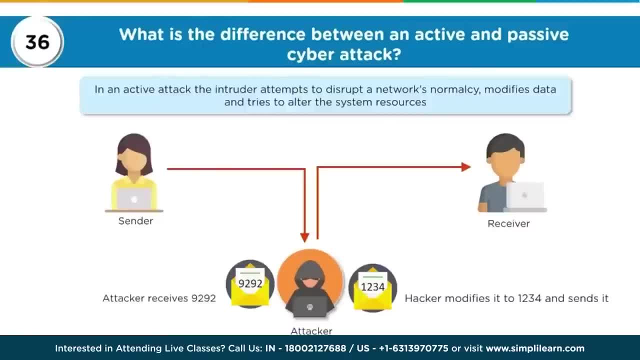 the system's resources. So this is more active, where the attacker will proactively try to destroy the network so that communications might even alter the data so that it is no longer trustworthy, Whereas in a passive attack the intruder intercepts data traveling to a network. 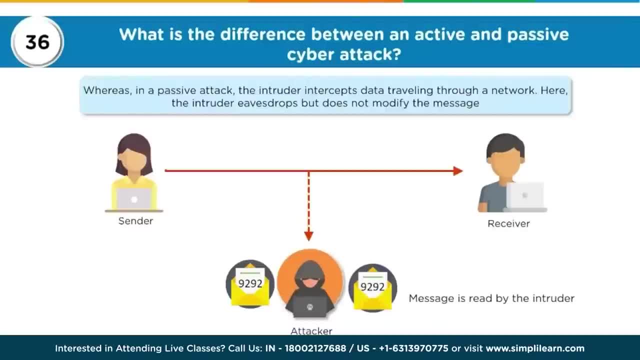 here, the intruder eavesdrops but does not modify the message. So they're just listening in. they're just observing what is going on. they're not manipulating the data, they're not stealing anything. it's just that they are monitoring the activity that's going on. 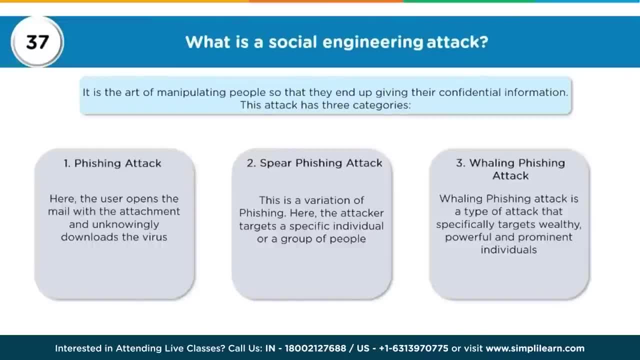 Then the next question: what is a social engineering attack? So social engineering is a very complex process that involves the human by itself. The vulnerability also lies in the human. It may be executed through a computer, but end up that is the gullibility of the human. 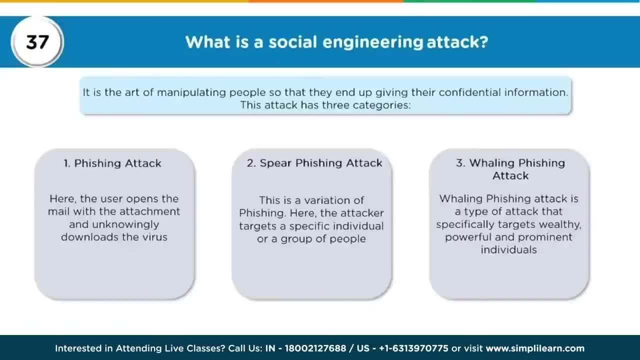 So it is the art of manipulating people so that they end up giving up confidential information. Now, there are three categories in this attack. while the first one is a phishing attack, second is a spear phishing attack and a third is a railing attack. Now, phishing attack is: 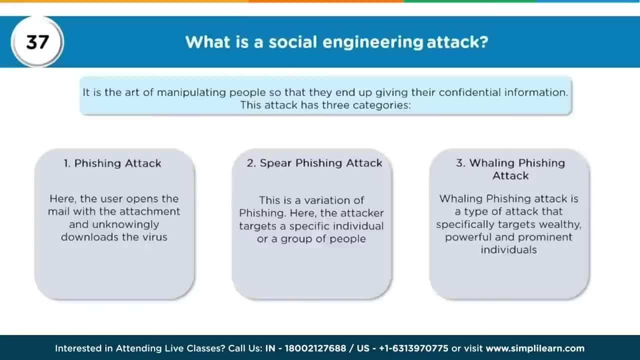 basically a generic attack. It is targeted to the world at large, whoever follows the rules of the system. So the phishing attack is basically to charge. whoever falls prey to that attack will be a victim, Whereas a spear phishing attack is a targeted attack towards a specific. 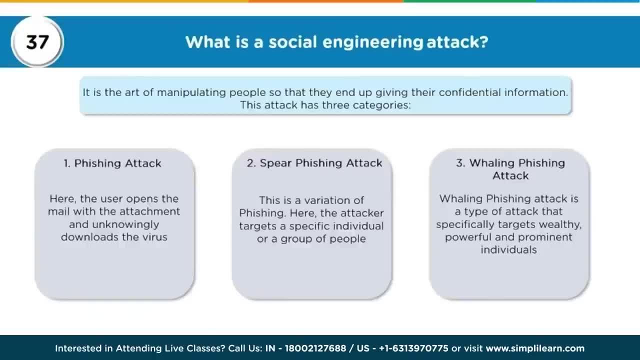 individual or a group of individuals or towards an organization. So there is a lot more research that goes into spear phishing, where you analyze the victim, you try to figure out what their vulnerabilities are and you tailor make or you try to figure out what their vulnerabilities are. 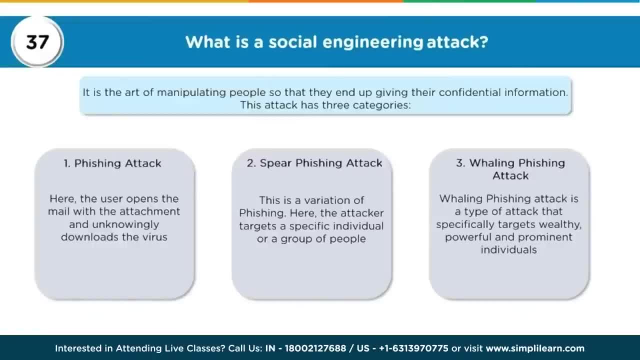 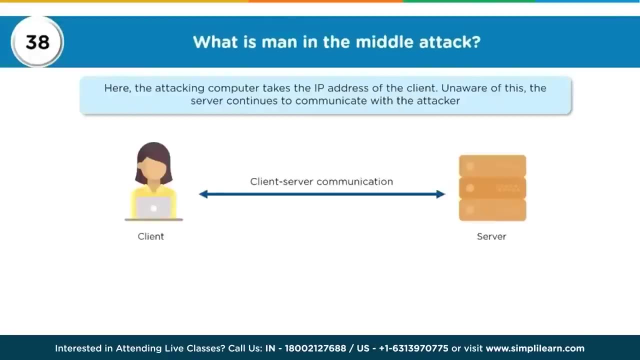 So the spear phishing attack is basically a railing attack where you are attacking top level executives, So the C level executives of an organization, politicians, movie stars, wealthy and powerful people, So any of these people, when they are attacked, it will be to leverage a man in. 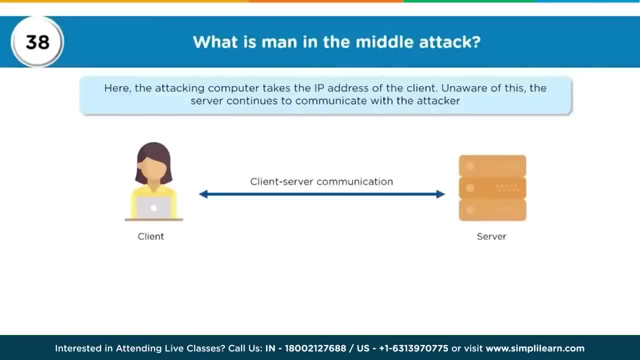 the middle attack. Now, in the man in the middle attack, the attacker attacking computer takes the IP address of the client. unaware of this, the server continues to communicate with the attacker. Now, if you remember, in a previous question we have also talked about spoofing. 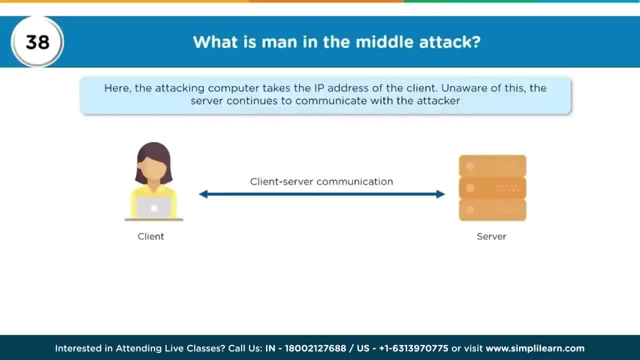 So in this scenario, attacker has spoofed their IP address to become a man in the middle. that means that they are now eavesdropping on the conversation between the actual client and the server by posing themselves as a server. In this scenario, the attacker is. 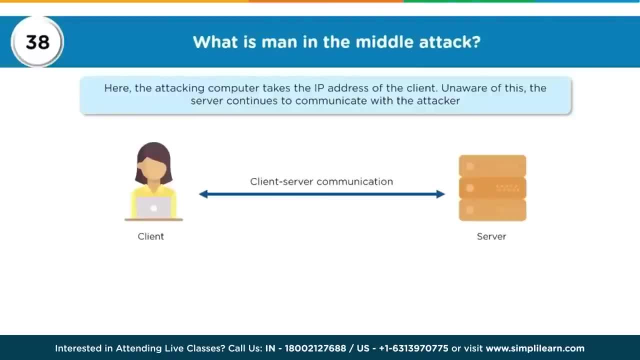 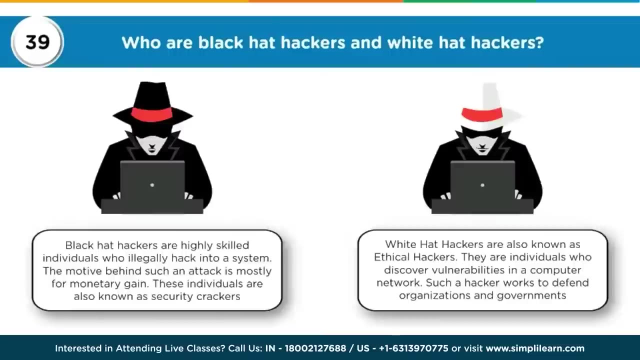 now a go between between the client and the server and can eavesdrop and can copy the information to the server. The attacker becomes a man in the middle, which means that they are now eavesdropping on the conversation that is happening between the client and. 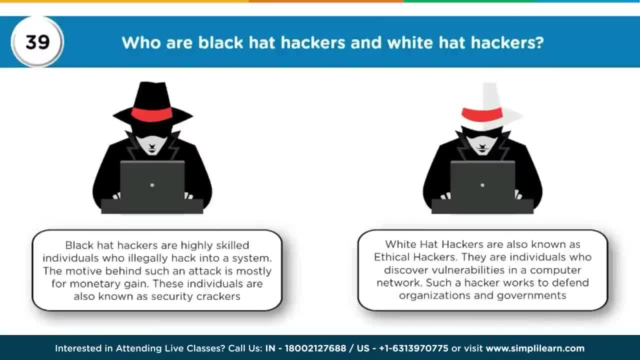 the server. The next question: who are black hat hackers and white hat hackers? The main thing is the differentiation between a black hat hackers, those who have malicious intent, those who do hacking for the intent of personal gain or for the matter of disruption. The main 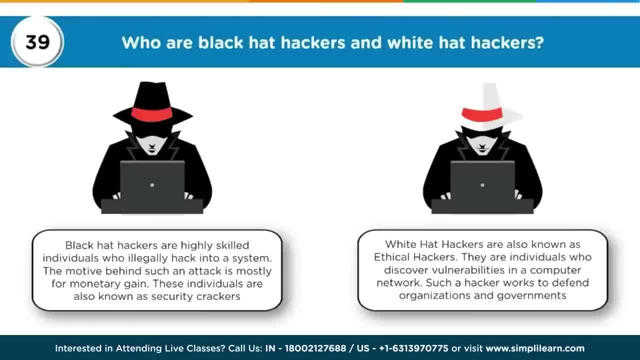 thing that black hat hackers lack is authorization. they are not authorized to do the activity that they are about to do and they are going to get unauthorized access to devices or to data which is not available to them. So the main difference between these two types of hackers. 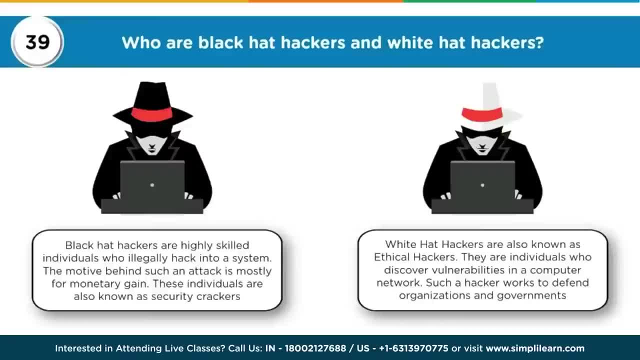 a black hat and a white hat is the intent and the authorization. So black hat hackers are not authorized to conduct whatever activity they are doing, whereas on the other side, white hat hackers will be hired by organizations. they will be provided authorization for certain activity that the white hat 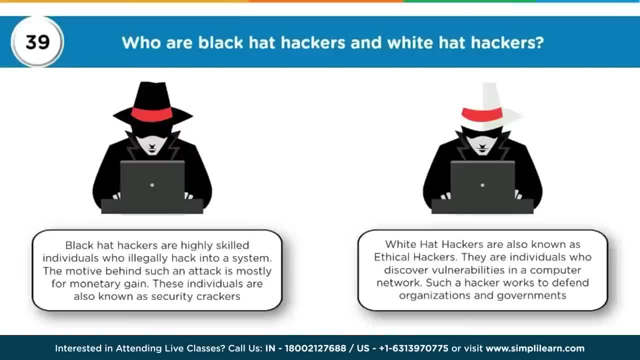 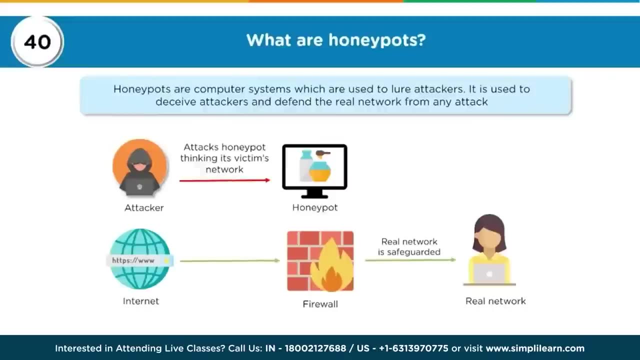 hacker can do to find out those vulnerabilities. once those vulnerabilities have been found out by the white hat hacker, they will report it to the management and guide them in implementing security controls to mitigate those vulnerabilities. What are honeypots Now? honeypots are a. 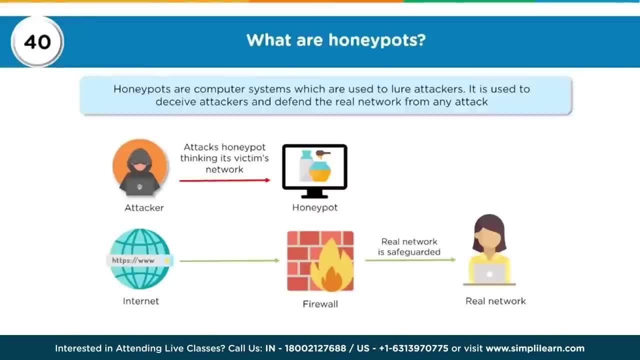 very interesting device that can be introduced in a network. These, basically, are decoy servers that are implemented in a network to attract the attention of an attacker. It is there to lure an attacker into attacking that particular device, thus creating a security blanket. for the rest, 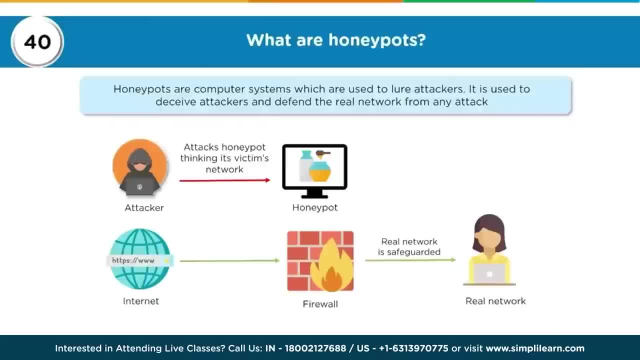 of the devices. So if an attacker has been able to bypass a file and is now trying to scan a particular network, when they scan they will come across various devices that are there in the network. They will then proceed to do a vulnerability scan on these. 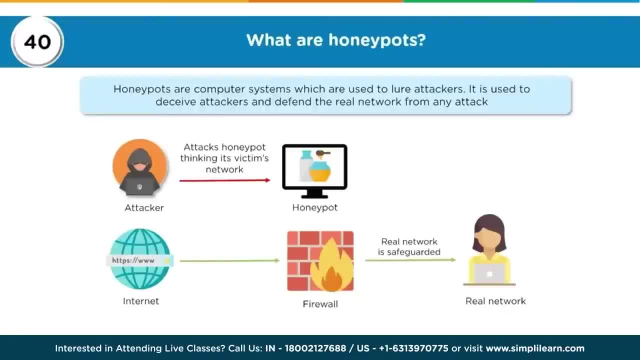 devices. The honeypot at that point in time will prove as an attraction to these attackers because it will demonstrate some vulnerabilities to the hacker which will divert their attention. So these vulnerabilities are simulated on these devices The moment the attacker then starts interacting with. 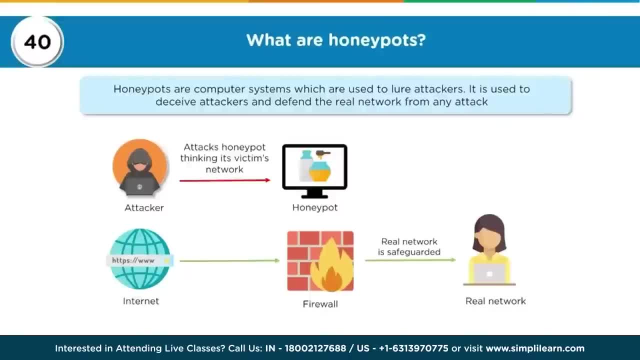 the honeypot. the honeypot will identify that as a malicious traffic and will warn the administrator about a possible attack that is going on. The administrator will then investigate through the honeypot of what activity is going on and then reconfigure their security. 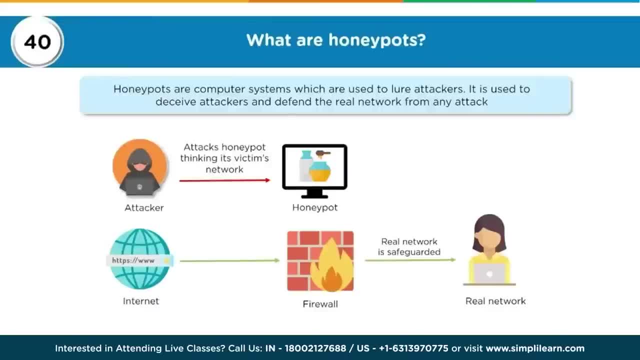 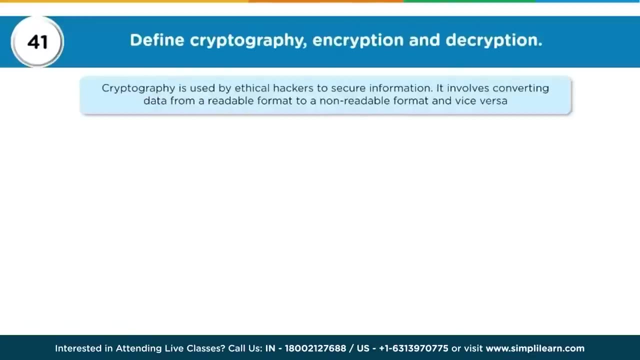 controls to block the attacker or mitigate the attack itself. So it is more of a decoy server that will showcase or simulate some vulnerabilities to protect them and safeguard the rest of the network. These are the 10 questions for cybersecurity In the next video. 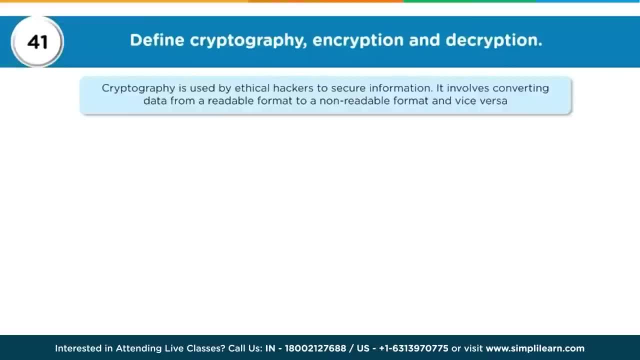 we'll be talking about cryptography. The first question: define cryptography, encryption and decryption? Now, cryptography is used by security professionals to scramble data into non-readable format, which is used in securing that information. So it involves converting data from a readable format into a 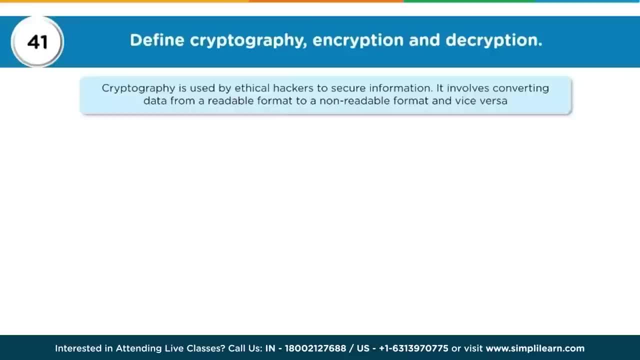 non-readable format and then reversing it back to a non-readable format again. For example, the word computer is now scrambled into looking like an unreadable format. Now, if you look at this word that it has been scrambled into, it would be very difficult. 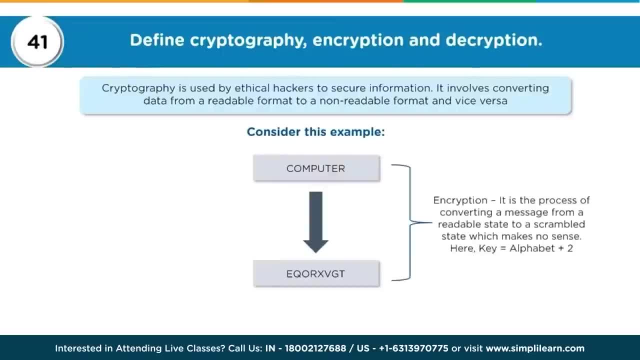 for a human to figure out what the actual word was. Now, in this scenario, we have taken an algorithm where we have made a shift of the alphabet, where we have added two alphabets to the alphabet. O plus two becomes Q, M plus two. 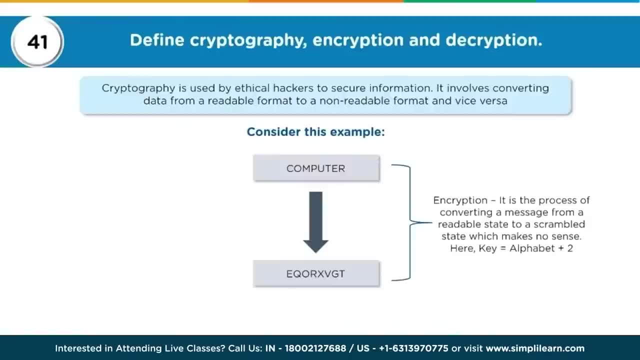 becomes O. So we have done a shift of two and thus the key over here for this algorithm is the alphabet plus two. So any person who figures that out will be able to unscramble this and convert this back into readable text. 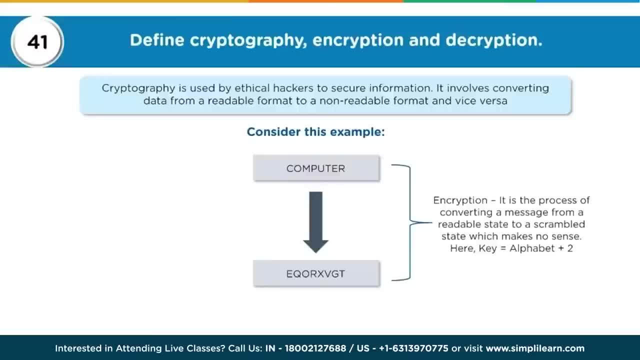 The fact of scrambling a readable text data into something that is unreadable by using a particular key is that the alphabet will be decrypted by two characters. Now, as we discussed, the decryption again is replacing the alphabet and taking it further back by two characters. 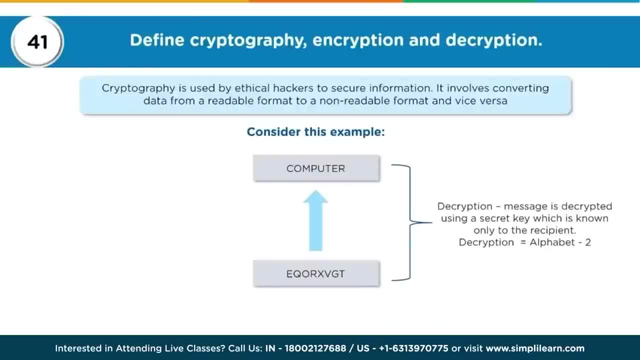 So E minus two becomes C, Q minus two becomes O, O minus two becomes M, and so on, so forth. So anybody who knows this key, the shift key, the shifting of that character, will be the fifth character from that particular character, and so on. 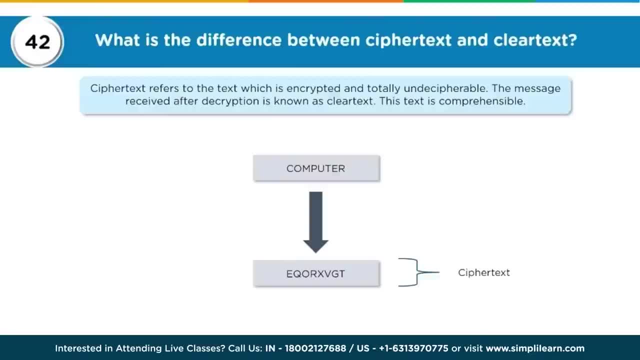 so forth. The next question: what is the difference between ciphertext and cleartext? Ciphertext refers to the text which is encrypted and totally undesirable. The message received of the text is intended to be. However, if the moment we encrypt it, 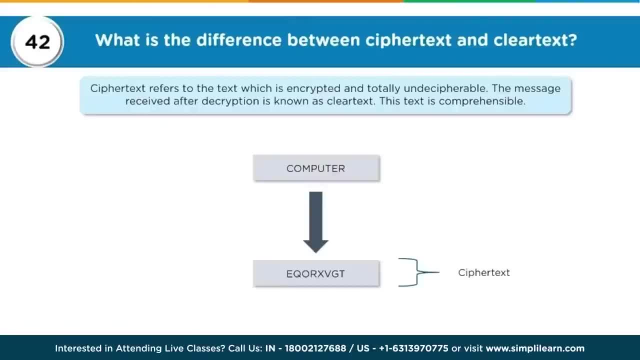 that means we scramble it into unreadable text by using any of the algorithms that we'll be looking at. that text is known as a ciphertext, and without the key, this becomes unreadable. The cleartext, as discussed, is the same as the ciphertext. 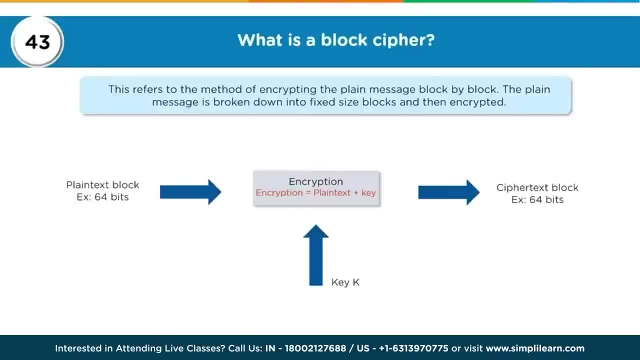 and we get the ciphertext to it. Moving on to the next question, what is a block cipher? This refers to the method of encrypting the plain message block by block. The plain message is broken down into fixed sized blocks and then encrypted. Now a block. 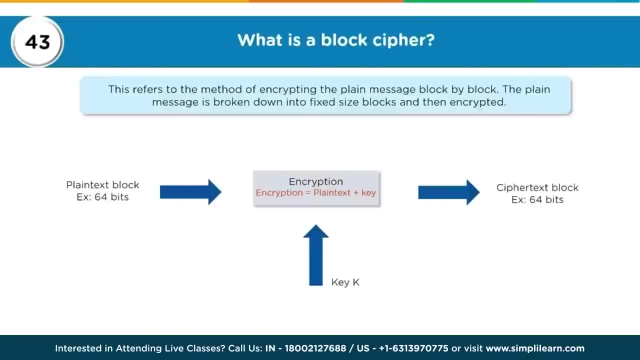 cipher is normally used for data that is stored on a hard disk. In this example, we've got plain text, which is 64 bits in size, and we've added a layer of encryption to it, So plain text plus the key that we've studied in. 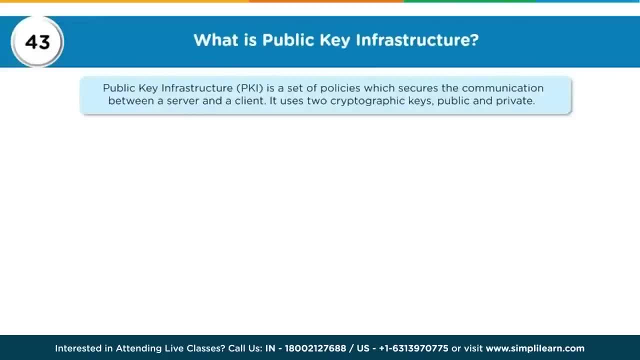 the previous questions, and then the scrambled data out of it, which is unreadable and thus encrypted. So the block cipher is a block cipher that is encrypted and it uses two cryptographic keys, public and private. So the infrastructure itself is a set of policies. 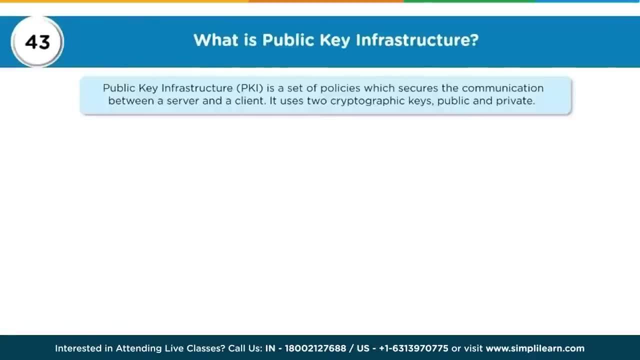 people, procedures and techniques which are standardized in nature and are globally accepted, which allow us to decrypt the private key. The other part of encryption is a symmetric encryption, where the same key is used to encrypt and the same key is used to decrypt. Now, in 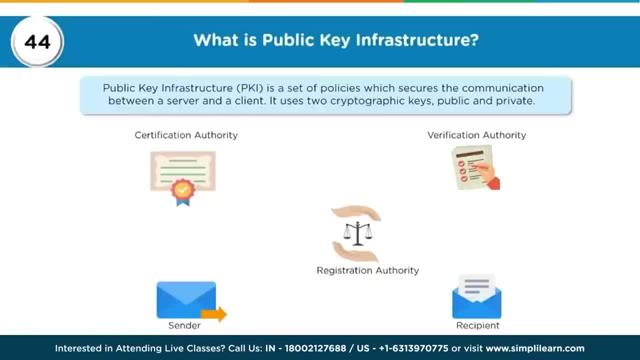 a public key infrastructure. like I said, we have standardized that. so in the standardizing part of encryption there is a key that is used to decrypt a particular transaction or a communication, a registration authority with whom they are going to register for that particular. 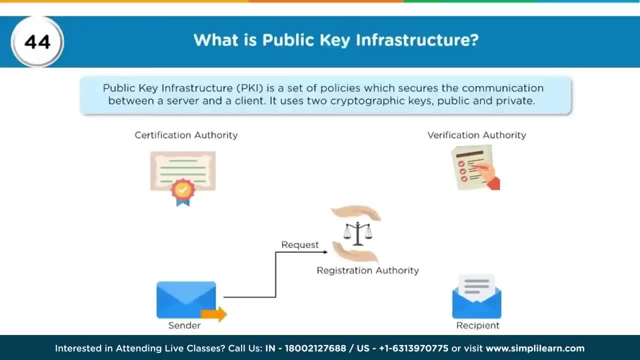 key, the certification authority, who issues that key? the registration authority would validate the genuinity of the user, so they might do some identity verification or proof of residence or something like that. Once they have identified the person and they have validated the information, they will. 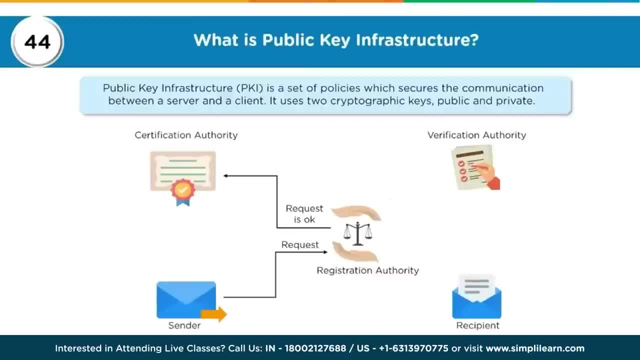 then send the request to the certification authority stating that the person will send the public key to the sender, which will be utilized by the sender for further transactions. So when the sender is going to sign some data and wants to send it across to the recipient, 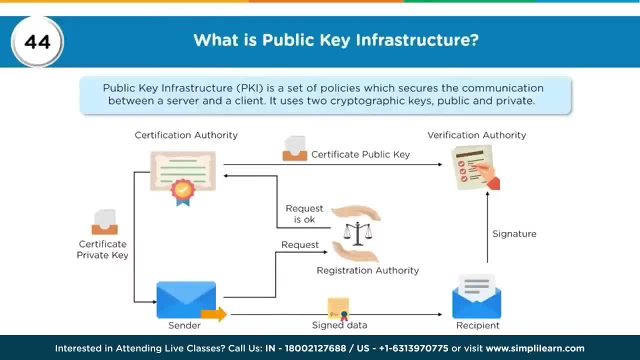 they will use the certification authority to update the private key with the verification authority. So whatever is signed by the sender, received by the recipient and they want to validate it, they will send it back to the verification authority. The verification authority will validate using: 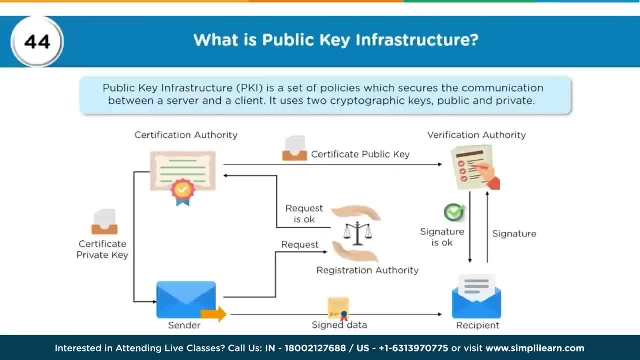 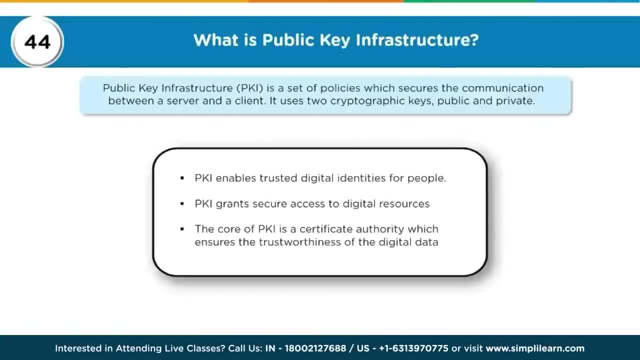 the signature and send a denial message to the recipient, and the transaction will not go through. So the PKI enables trusted digital identities for people. So the PKI grants secure access to digital resources based on the infrastructure that has been created and the 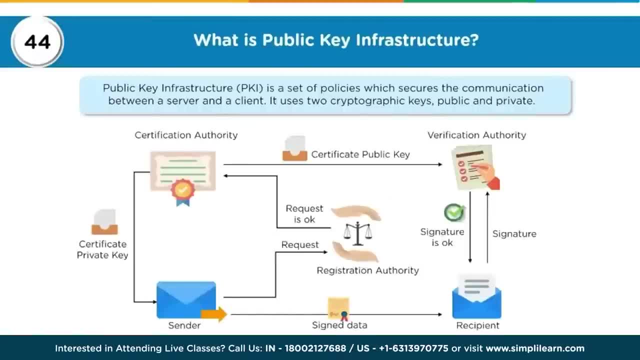 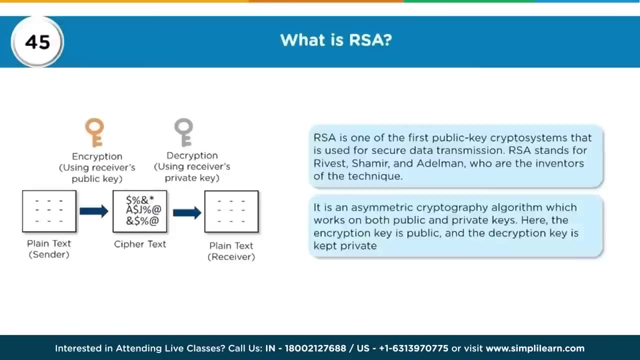 core of the PKI. These are the key players that have been standardized in the public key infrastructure. The certification authority is the authority that issues the digital certificates. The validation authority is the one who validates that digital certificate. Moving on what is RSA, 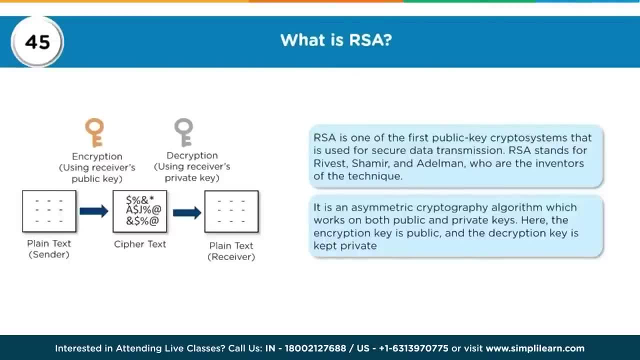 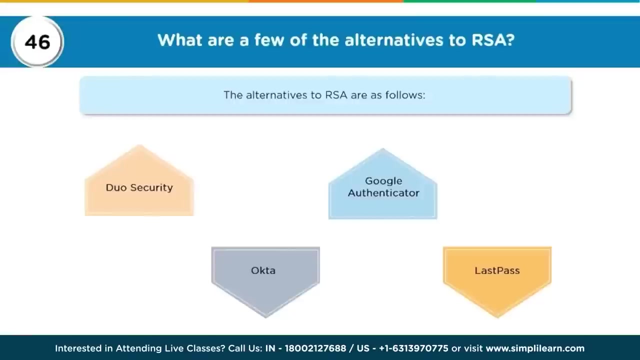 RSA is one of the first public key encryption algorithms. RSA is a multi- network of cryptographic cryptography algorithms. RSA is the first public key encryption algorithm to encrypt and decrypt the cryptographic cryptography. RSA is the first cryptographic cryptography algorithm to encrypt and decrypt cryptographic cryptography. 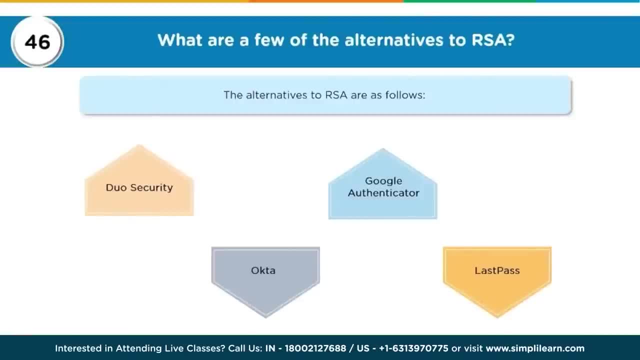 RSA is an algorithm that is used for encryption. There are a lot of other algorithms that can be utilized to alter or to scramble data, depending on your requirements. In the previous question, we have studied what RSA is and what cryptography is. RSA is a 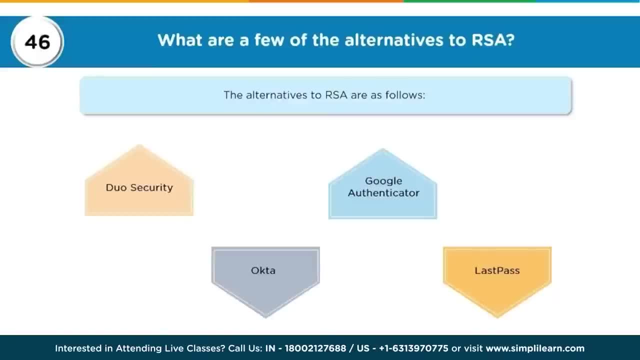 cryptographic cryptography algorithm that can be used for encryption and decrypt. cryptography. RSA is the second most important code in cryptography. RSA is the us access to those particular portals. Okta is an identity manager where you have created different digital identities and you have assigned them certain permissions and, based on your authentication. 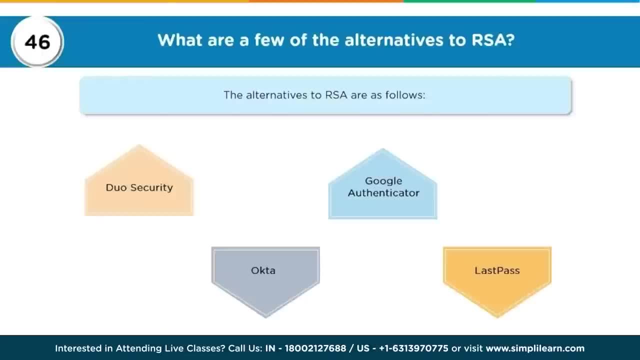 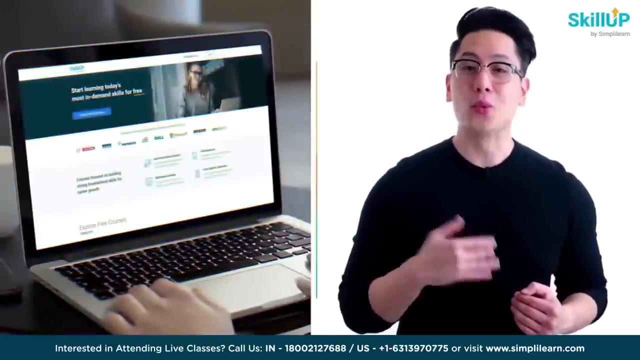 mechanisms. Okta will allow or disallow access to those different applications or different portals as you have configured it. So all four are authorization and authentication mechanisms which can be used as alternatives to RSA. If getting your learning started is half the battle, what if you could do that for free? Visit ScaleUp by SimplyLearn. Click on the link in the. 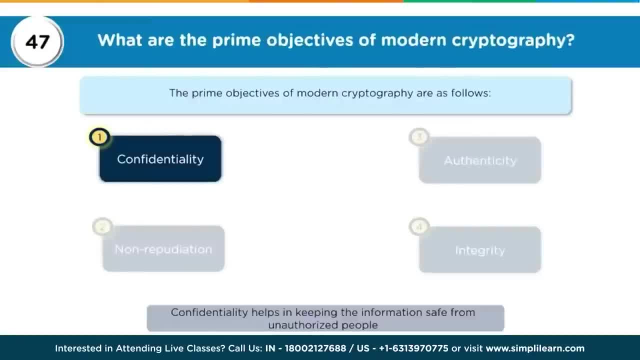 description to know more. Next question: what are the prime objectives of modern cryptography? And this is a very important question, because we've so far looked at what cryptography is and what public infrastructure is, but what is the achievement out of it? Why are we utilizing it? 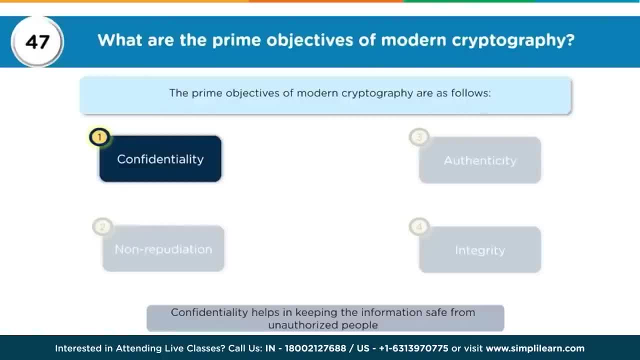 and what do we want to gain out of it? So the main and the prime objectives of modern cryptography are as follows, mentioned on your screen: The first one is confidentiality, the second one is non-repudiation, third one is authenticity and the 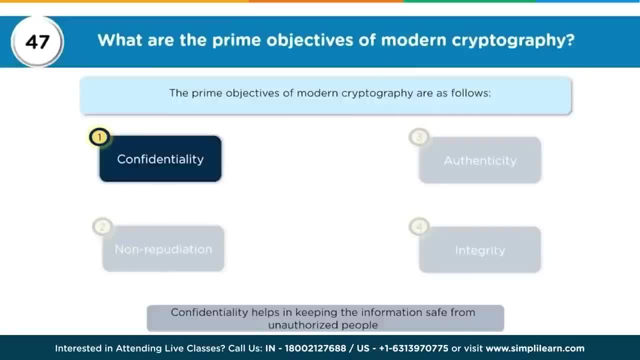 fourth one is integrity. Now, if I go back to the first one, confidentiality- that is where I want to keep data confidential. that means it will only be visible to the authorized users, right? So here I have created a list of people who have deemed as authorized users and I've created a digital 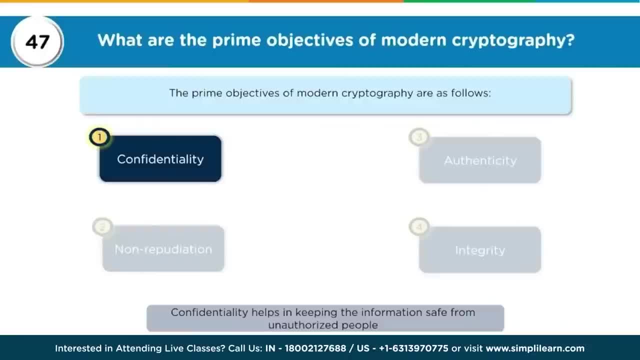 identity to them and I've given access controls to those people. Now, that is how confidentiality is ensured. So, when we want to keep data confidential, we create a list of users who we are going to allow access to certain resources and we are going to define what 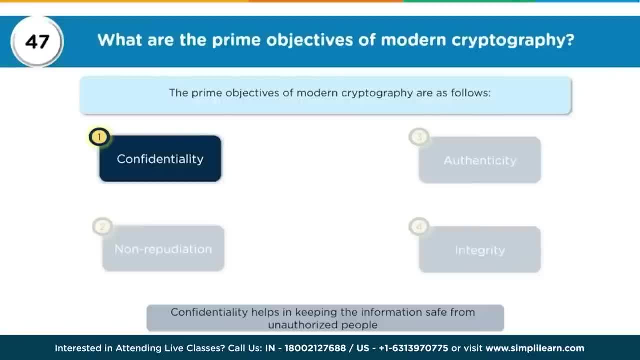 access controls are to be utilized. what access are allowed- whether they've got administrative access or user level access- and only those authorized users are going to be able to access these resources. That is how we maintain confidentiality. The next one is non-repudiation. 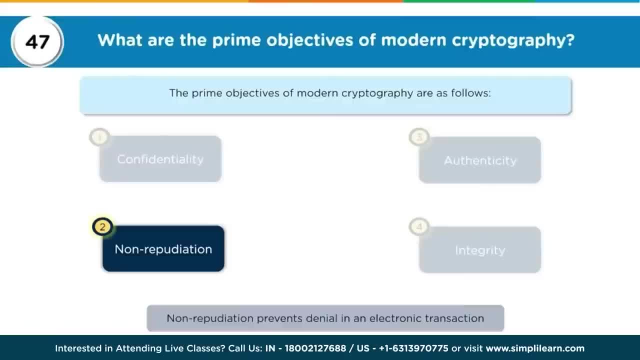 Non-repudiation is the prevention of denial of having been a part of a particular transaction. So in the public key infrastructure that we discussed, where a digital signature was utilized to sign a particular transaction and then sent to the recipient, the sender would not be able to deny. 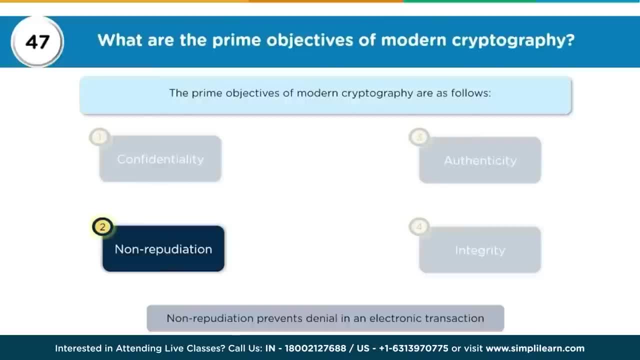 of having originated that transaction because it was using their digital certificate. Thus non-repudiation comes in the picture. One more example that we can have here is on our mobile phones when we use SMS short messaging service and we send a message to, to another person- the person- when they receive a message, the number is validated by the service. 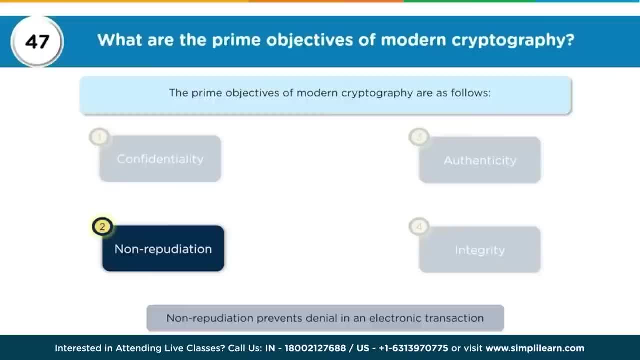 operator and thus the sender cannot deny having sent that message. The sender, at the same time, can have a delivery report sent to them that the message was delivered to the inbox of the recipient and thus, if the recipient denies having received that message, the delivery report becomes proof of. 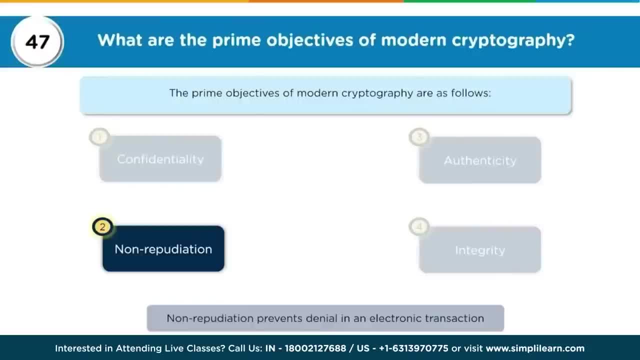 that message being delivered to their inbox. Thus, both the parties cannot deny of being a part of that particular transaction. Then comes the part of authenticity. Now, in confidentiality, we have created a digital identity, assigned it to a particular person and we have given them digital. 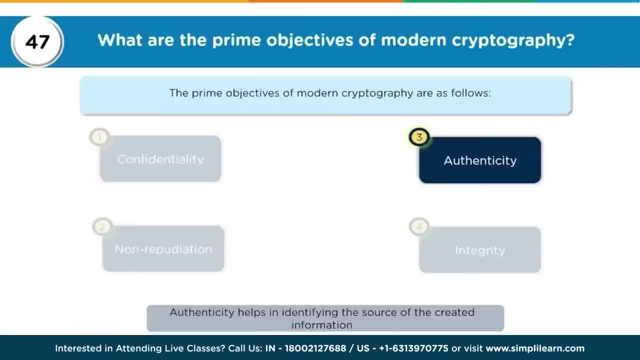 signatures, where they cannot deny having being a part of that transaction. But authenticity is the part where they try to prove that they are who they claim to be. So if I am saying that I am a claiming a digital identity, I have to prove that I am that person who I'm trying to claim to be. 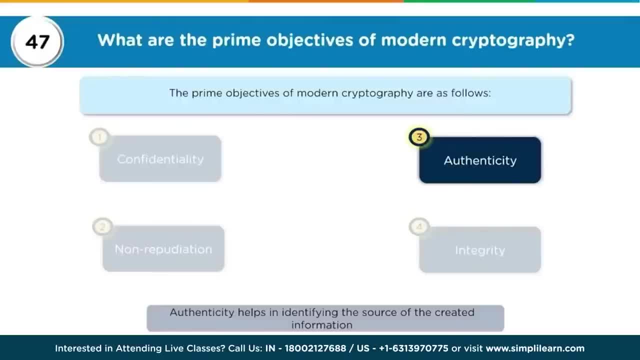 and an example to that is when we go to our gmailcom websites, it first asks us: what is our username? Our username is normally our email address, which identifies the account that we are trying to access. So this account is confidential because it is only authorized for a particular 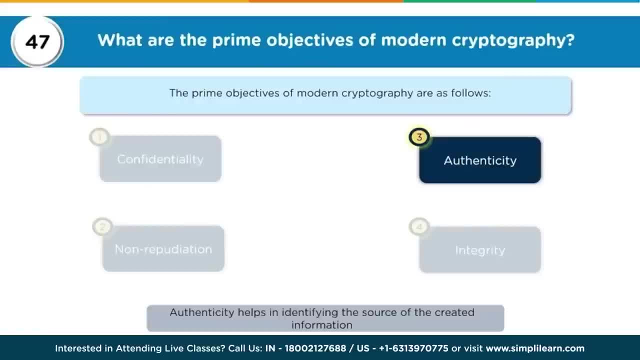 person, and once they identify themselves by identifying the email address, that's when the authentication part comes into the picture, where it asks for the password. Now, it has never, ever happened that we just go on to the gmailcom, type in a password and then it figures out which account. 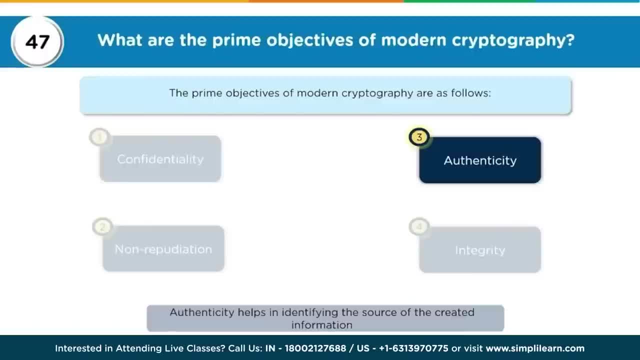 we are talking about. So the first step is always called the confidentiality part, where we identify which account we are talking about and then we try to authenticate as the owner of that particular account by providing the appropriate password to that account. If both of these match, only then do. 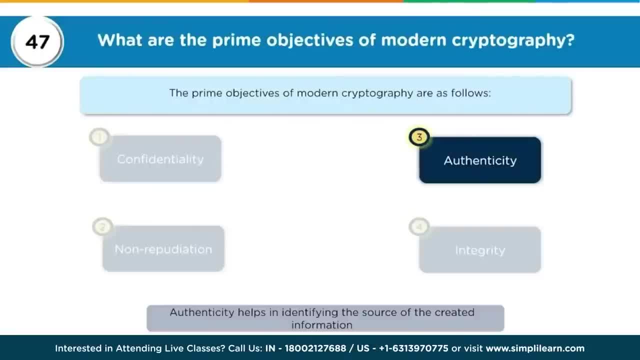 we get access to that account and we are able to make whatever transactions we want to make. Now, when we are making those transactions, non-reputation comes into the place where all our activity is also being logged. So we have identified our account, we have authenticated ourselves by providing the password, so the proof is there. 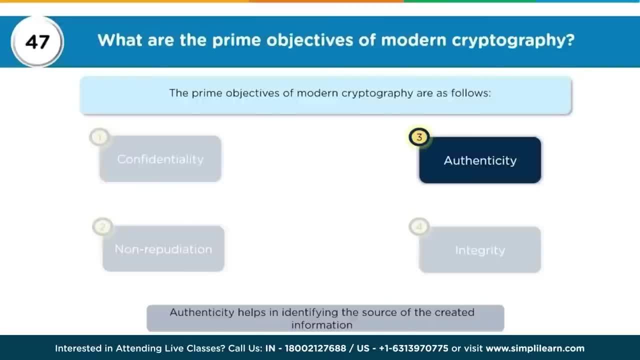 that it is us who are trying to access it. and then, whatever activity we do- send an email, receive an email, delete something, attach something- all of those activities are logged and stored as proof of what actions have been done. So tomorrow, if we deny having sent that, 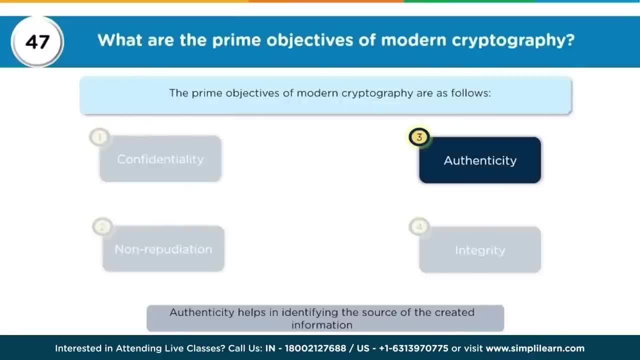 email gmail can still prove to us through those logs that that activity was done by us. And the fourth part is integrity, which ensures that the data received and sent- and sent by the sender and received by the recipient- has not been modified while in motion. So the integrity part is the trustworthiness of that data, that the 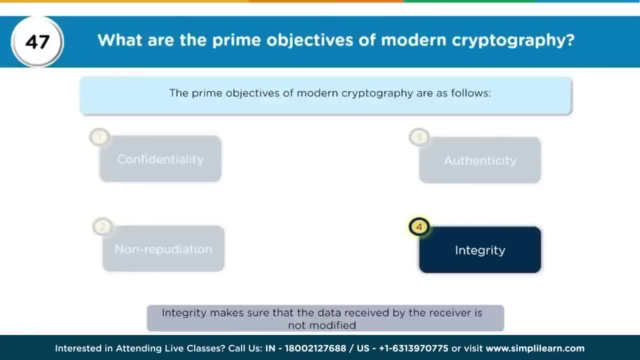 data has not been modified by any hacker or any other entity and is still trustworthy. So these are the four prime objectives of modern cryptography. Once I have scrambled that data using my public's signature, it is only my private signature that is going to decrypt it. 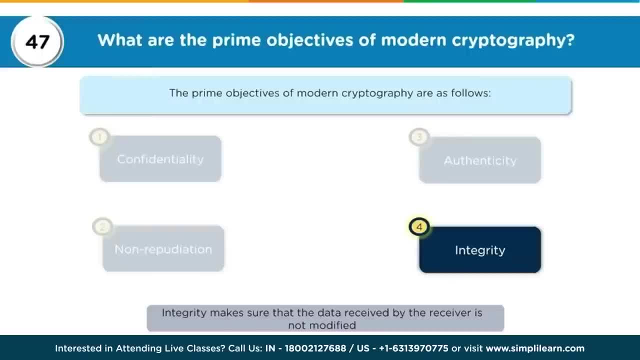 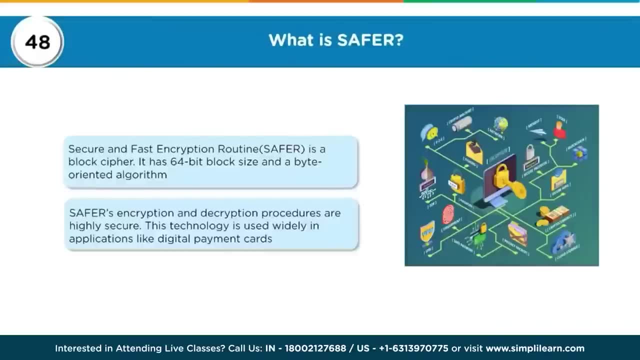 Using these mechanisms, I will be able to achieve all these four aspects of cryptography and security. Next question: what is SAFR Now? SAFR stands for secure and fast encryption routine, which is also a block cipher, As we have discussed previously. block cipher is a cipher that is used to encrypt data that is stored, So it has a 64-bit block size and 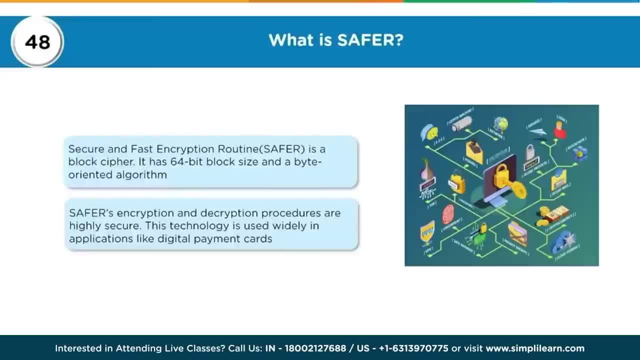 byte oriented algorithm. SAFR's encryption and decryption procedures are highly secure. This technology is widely used in applications like digital payment cards. So when you're using a digital payment gateway to make transactions, so you have. you have gone on to an online portal. you. 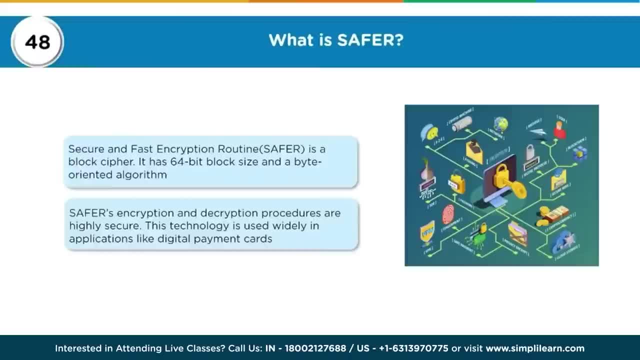 want to purchase a particular item and then it takes you to another payment gateway where you have to fill in your credit card information, sensitive information like your expiry date, CVV information and then the OTP or the password that you have created for your particular account. 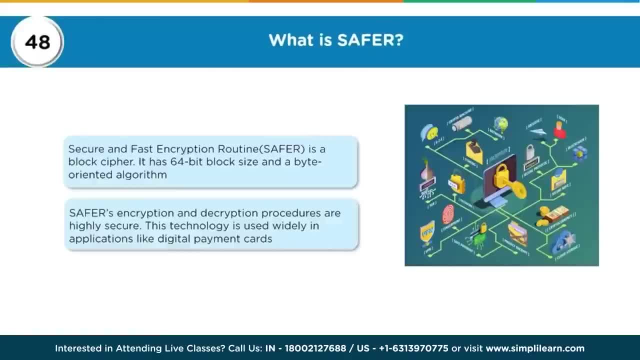 Now all of these need to be secured or highly secured, based on PCI DSS, which is the payment card industry data security standard. So these standards ensure that certain protocols are utilized to attain that level of security. SAFR is one of those block ciphers that is used under 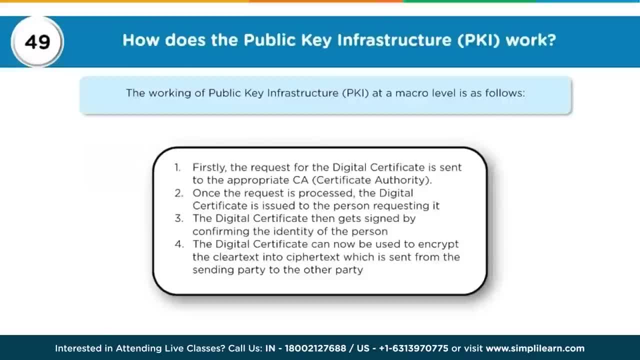 the digital payment gateway infrastructure. Next question: how does the public infrastructure, public key infrastructure- work? Now we have already discussed this in the previous diagrams. We have identified the key players: the certification authority, the registration authority. the end user who requires the digital certificate, the validation authority. who's going. 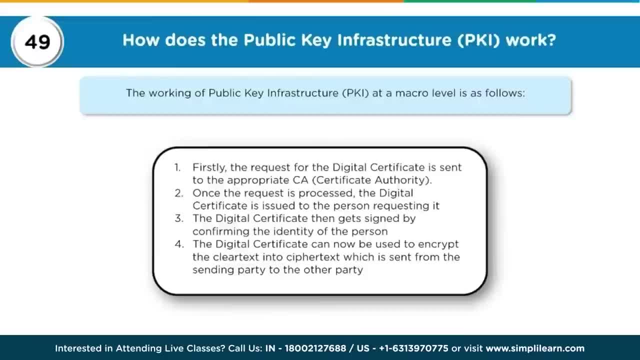 to validate it, and then the recipient, the end user with whom the transaction is going to be conducted. So the first point here is: the request for the digital certificate is sent to the registration authority, they validate it and then they okay to the certification authority, who then 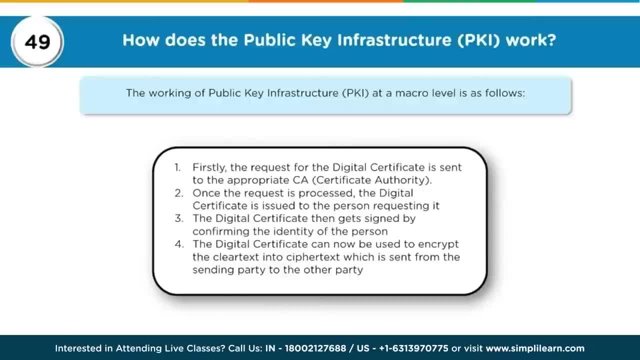 process, the request, and the digital certificate is issued to the person who has requested it. So when the person wants to conduct that transaction, they use that digital certificate to sign that transaction with the end user. The end user validates that with the validation authority and once validated, the transaction goes through. And now the last question: what is? 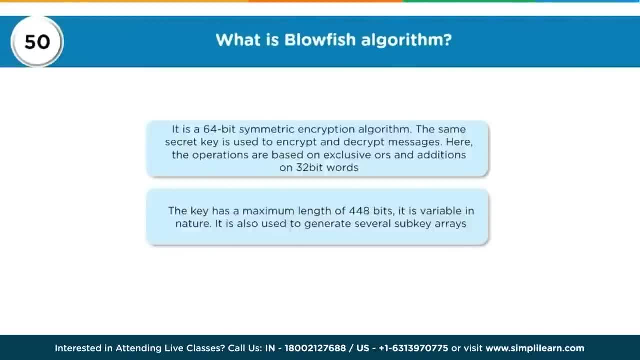 the Blowfish algorithm. It is a 64-bit symmetric encryption algorithm, So this is an algorithm that uses the same key to encrypt and the same key to decrypt- The same secret keys used to encrypt and decrypt the messages. here the operations are based on exclusive ors and additions to the 32-bit words. 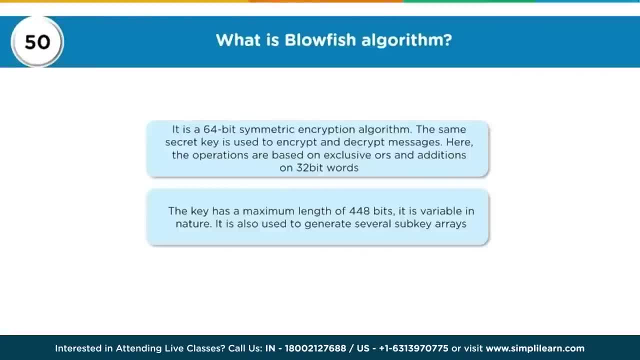 The key has a maximum length of 448 bits. Now, this is a little bit technical. you might not want to go this technical in an interview question. you just need to identify what the algorithm is used for, So whether it is a symmetric algorithm, which means it. 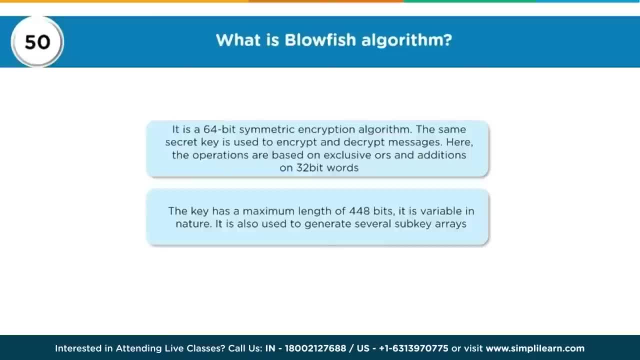 uses the same key, or asymmetric algorithm, where it uses a public key and a private key to encrypt. Thus, the Blowfish algorithm is just one more algorithm which uses symmetric encryption to encrypt and decrypt data. Algorithms that we have seen: RSA, and others that we have discussed. as far as the interview questions are concerned, what we need, 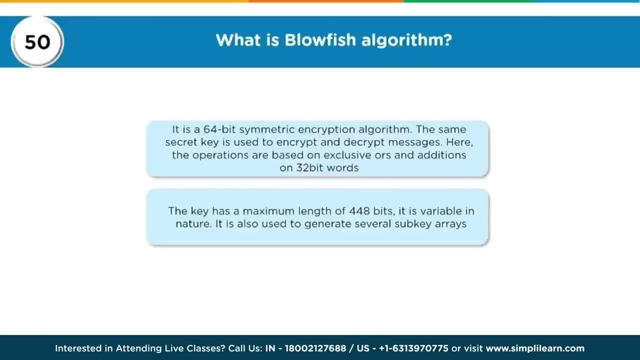 to remember is which algorithms are symmetric, which algorithms are asymmetric. what do symmetric algorithms do and what does an asymmetric algorithm do? The sub-authoritarian bid after run the test is that: what is the units key number of the algorithm which is used? don't be Money. why the 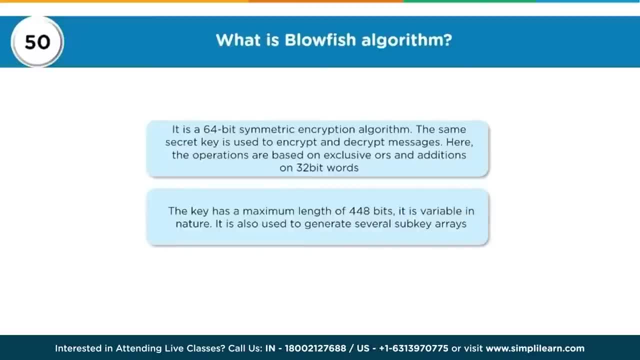 down and the bets. Calvin Green, what就是 the full wisdom of your algorithm is which algorithm is? the asymmetric algorithms too, and we also look at block ciphers and stream ciphers. block ciphers are utilized to encrypt data that is stored, stationary data, data at rest, and stream ciphers. 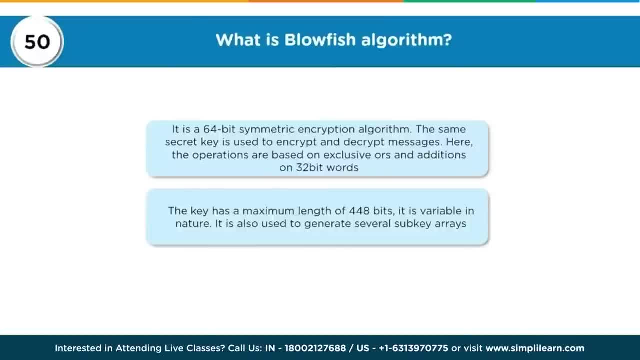 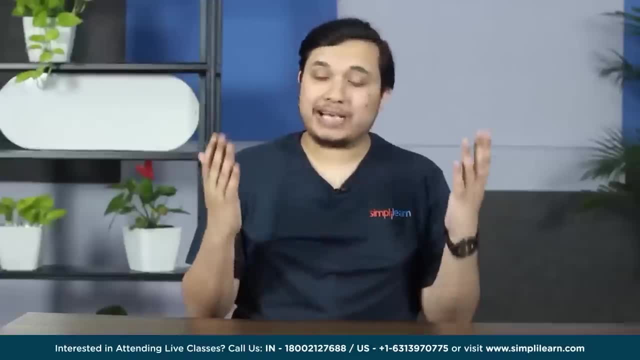 are utilized for data in motion while they're being streamed, so ssl and tls is another algorithm that comes into the picture when you're looking at streaming data. so that wraps up our full course on cyber security for 2023. we hope you had a lot to learn and will be on the lookout for any 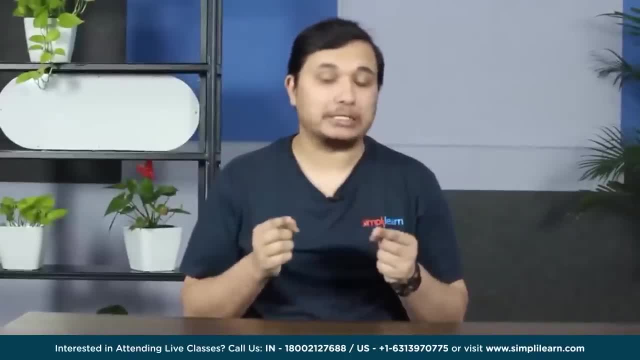 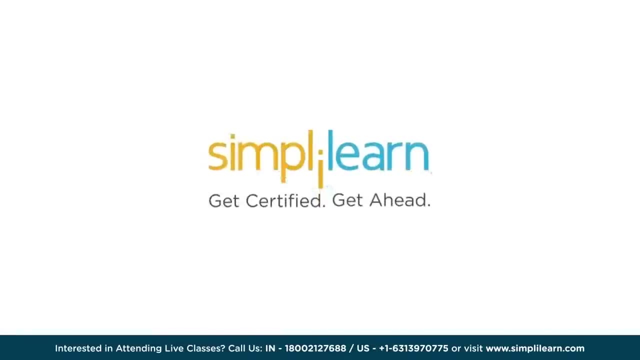 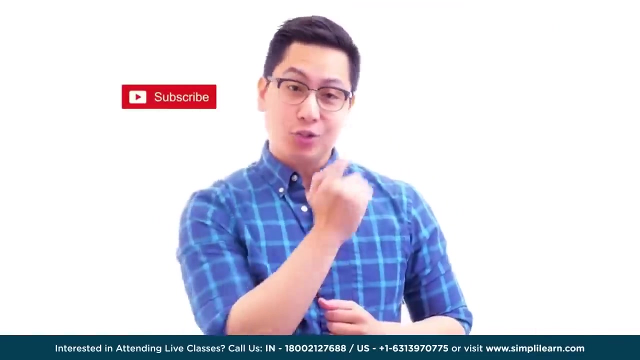 suggestions or doubts in the comment section below. so if you have any queries, you know what to do. thank you so much for tuning in today and happy learning hi there. if you like this video, subscribe to the simply learn youtube channel and click here to watch similar videos to nerd.